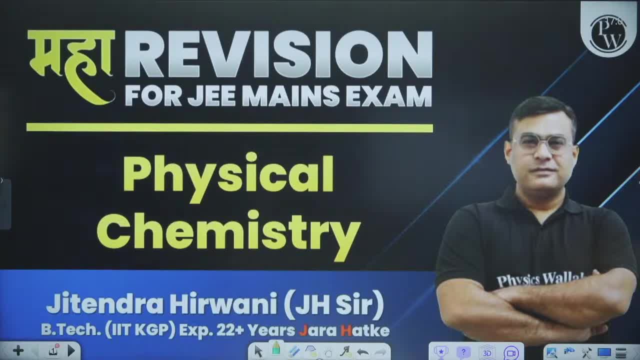 am i visible and audible? good afternoon nahi, bhai, good evening ho chukka hai not visible. not visible, kyunki abhi mai screen ke saamne nahi aya hu. screen ke saamne aane me jara kuch shan ka intijar hai. 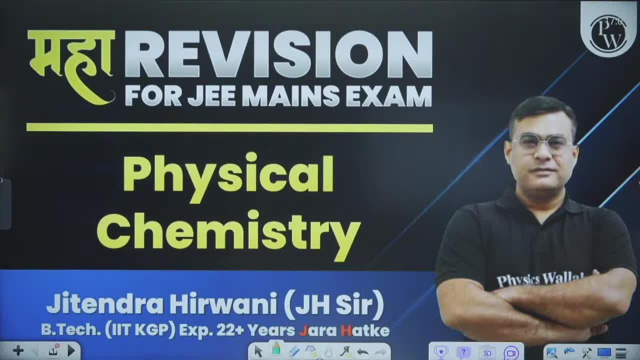 jaruri kaam chal raha hai. arey diwanu, mujhe pehchano kahan se aaya, kahan se aaya k해야 shana jate kech believed mai hun kaun pechchaan liya sabi Nice. 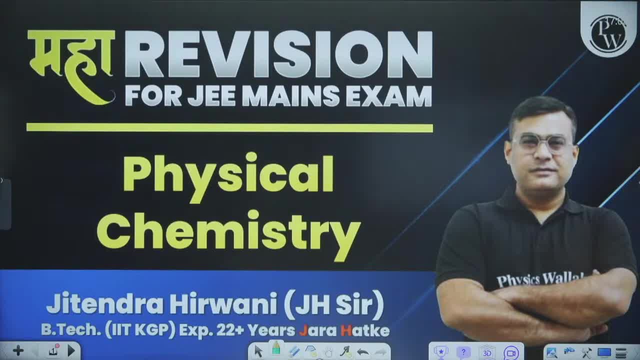 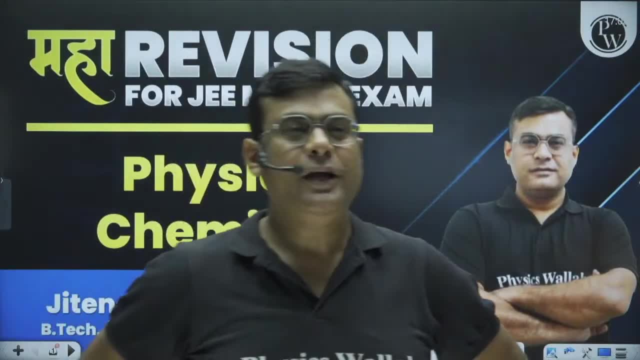 pechaan liya sabine chalo ji tob ubi uski sabi badaane ki sabi net ha chuka hai. hello bacho, kyahal chaal, kyahal chaal, kyahal chaal. how are you? how are you? 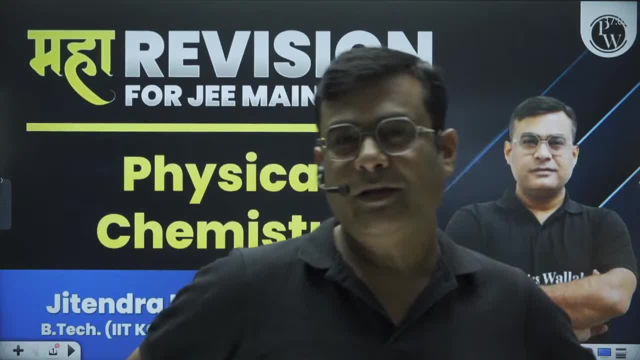 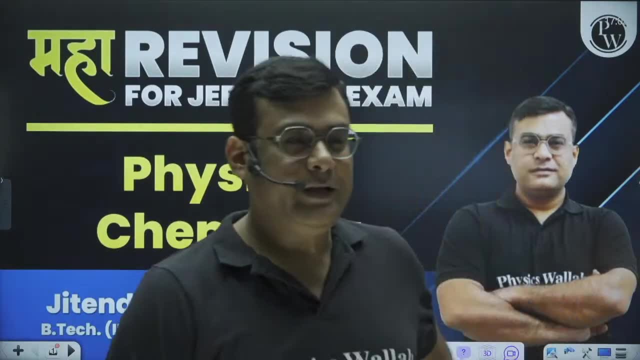 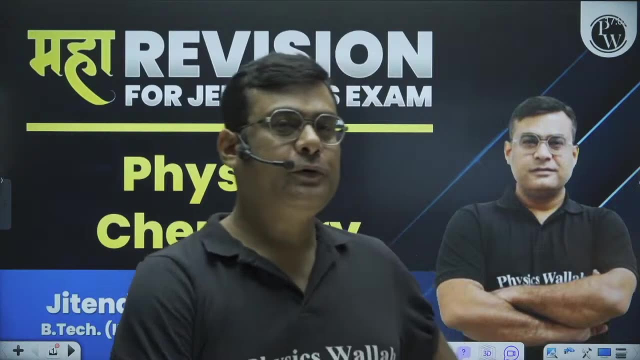 how are you? i hope aap sabi ki preparation jama jham chama chatsam chal rahi aungi thegna, aur ap api manjil, aap api lakehshai ko prapt kar nko lehi. And we, the entire team of PW, who can do small, small support for you, we are fully. 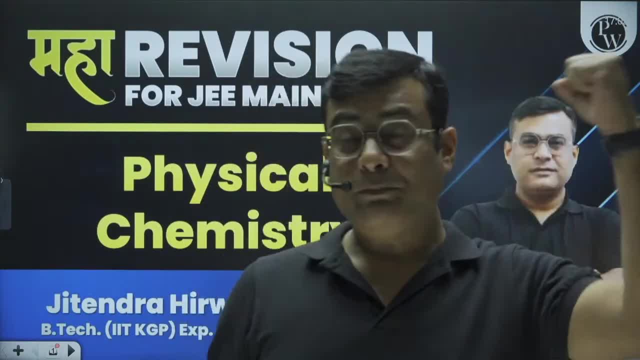 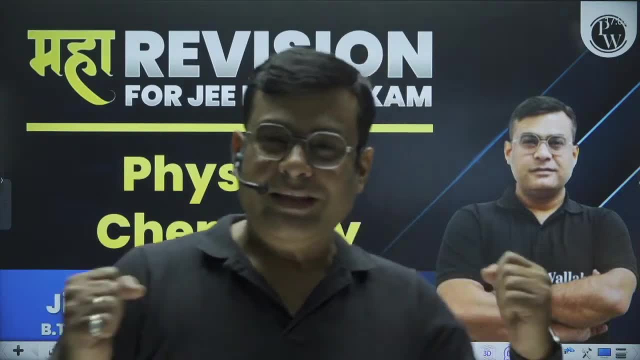 attached to you. We are trying to give you a little bit of mental, physical, emotional support to fulfill your goal, your goal, your dream, Because we know that the clap does not come from one hand, the clap comes from two hands. 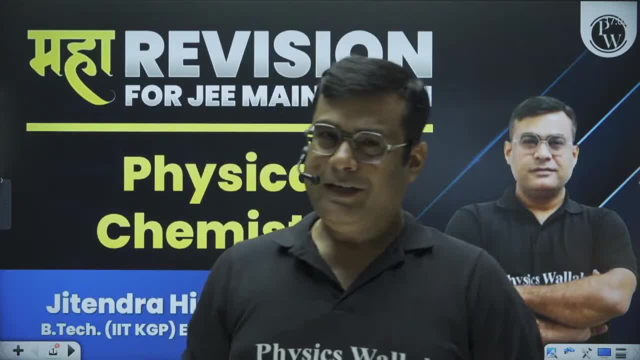 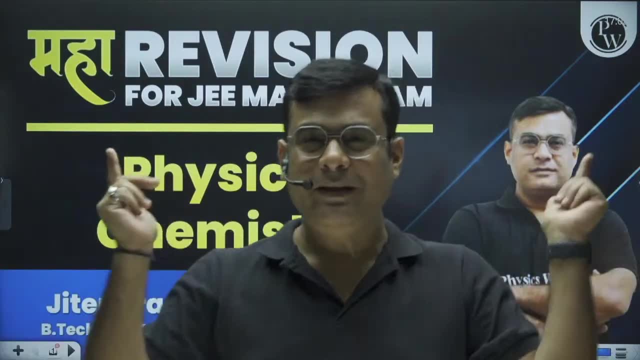 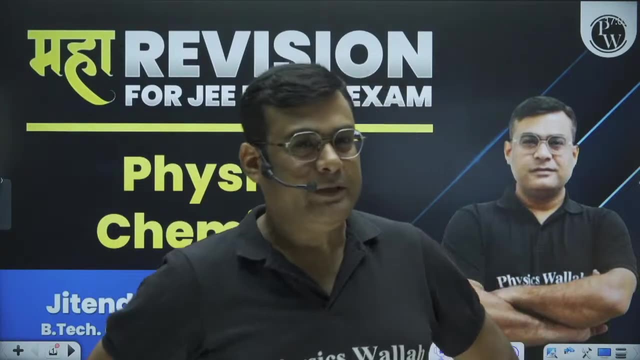 Brother, try with one hand, nothing will happen. so you try on your own and we will try on our own. But when both hands meet, the sound of the clap that is heard becomes jama, jama. Okay, so I hope many of you are children of Prayas 3.0, brother, our army 3.0, Jh army. 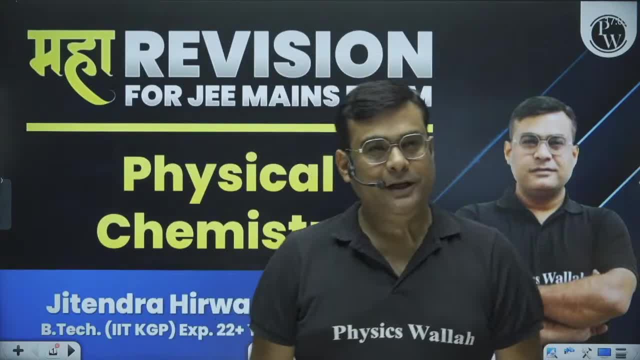 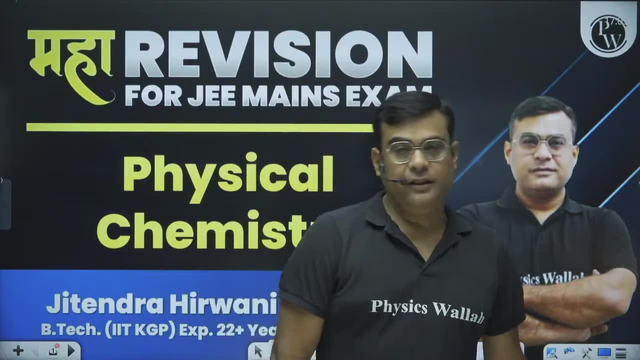 whatever it was, there will be many new children of Bharat Vash, some Prayas 2.0, 1.0, Lakshya 1.0, 2.0, 3.0, all the dear children of Bharat Vash whose dream is to become an engineer. 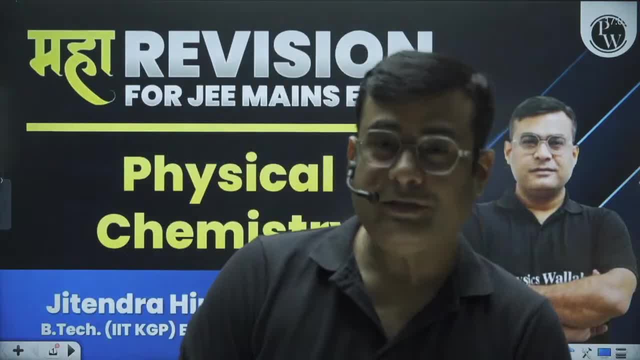 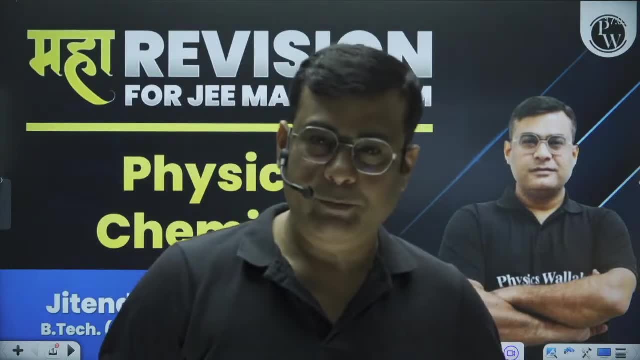 okay- and whose dream, in fact, is to become an engineer. In fact, most importantly, I have to do engineering from IIT itself. I am very happy to welcome all of them in today's jama jama session. Your dear Jitendra Nirwani JS. 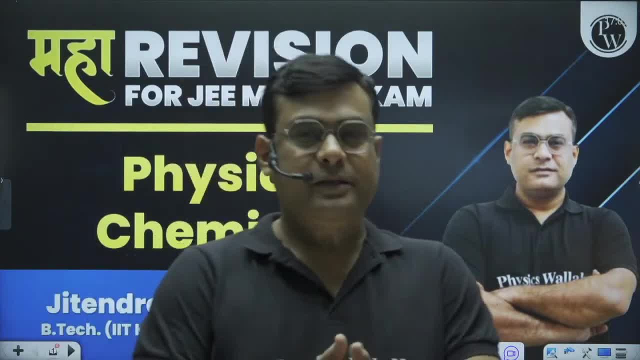 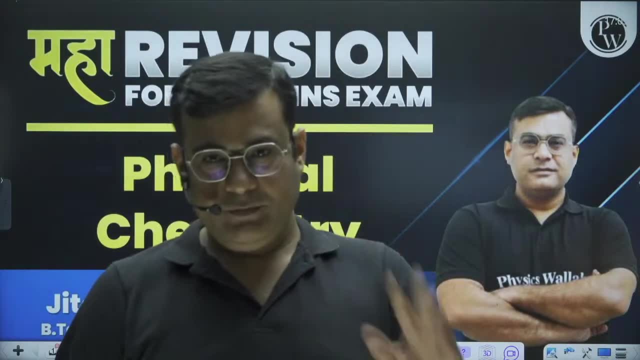 Sir of Kota, greetings to all And your already children. you also know that two sessions have been done. Today is the last day of chemistry. The first session was of organic chemistry. The second session was of inorganic chemistry. Yes, crash course also happened. 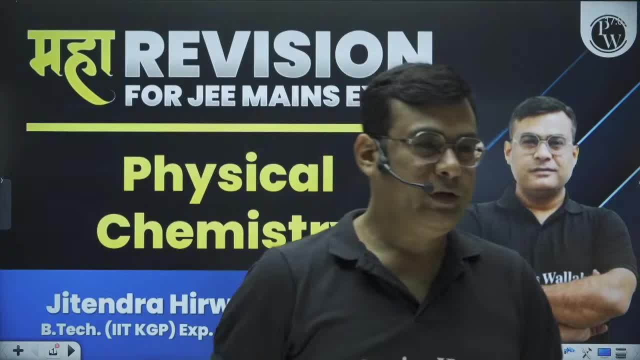 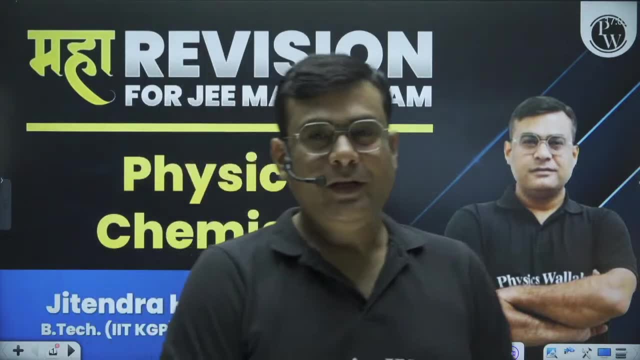 Yes, crash course also happened. There will be many children of the ultimate crash course, because I took UCC 1.0 and UCC 2.0 too, Okay, okay, so I took both of them. so there will be many children of the crash course. 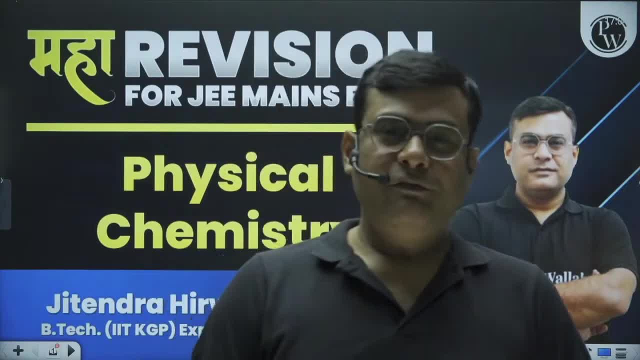 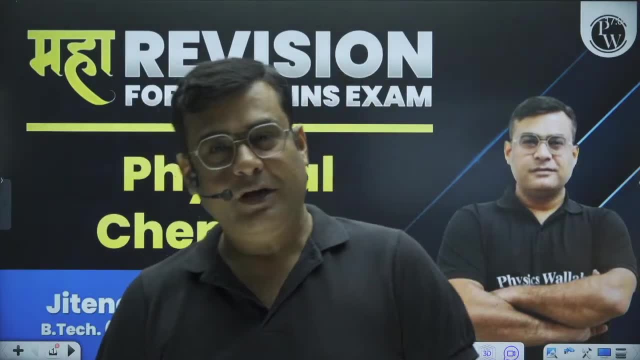 too. In fact, the first attempt of JEE was of January. I was fortunate to take this marathon there too. I got the session of 26 January and I got a lot of love from you there too. I hope and hope that today that love will remain the same to you. 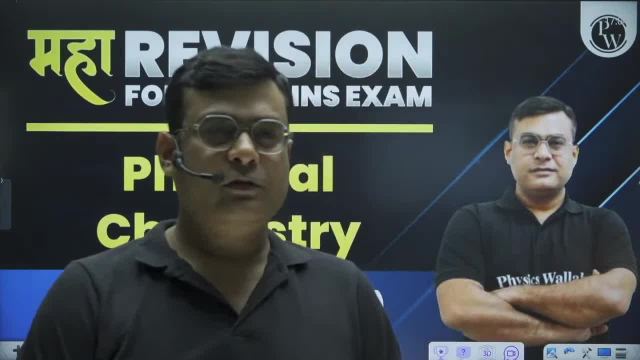 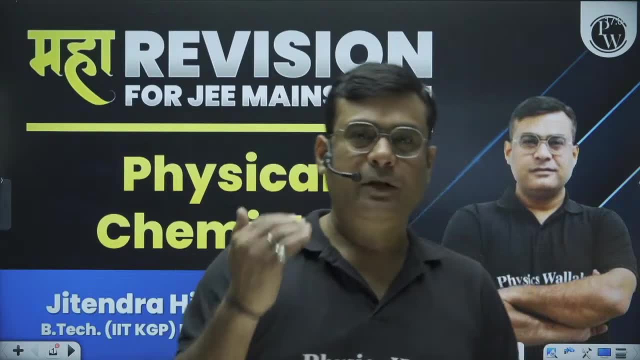 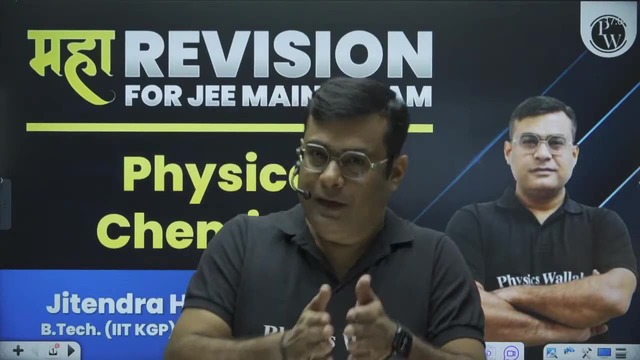 You will be happy, Thank you. Thank you so much. Even today we will try to understand every concept and every thing fully. Okay, fine then brother. organic finished, inorganic, finished, without physical chemistry. now does not complete The aim of keeping this on. the third number should be now: brother, relatively. 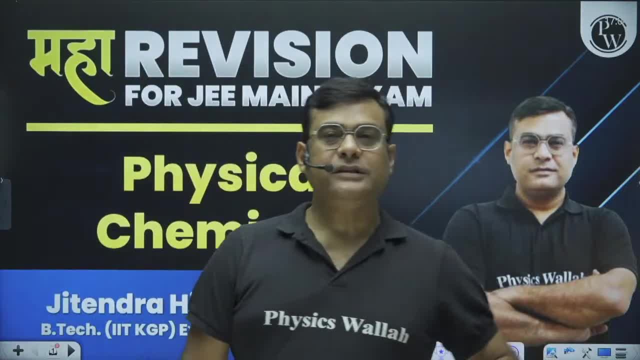 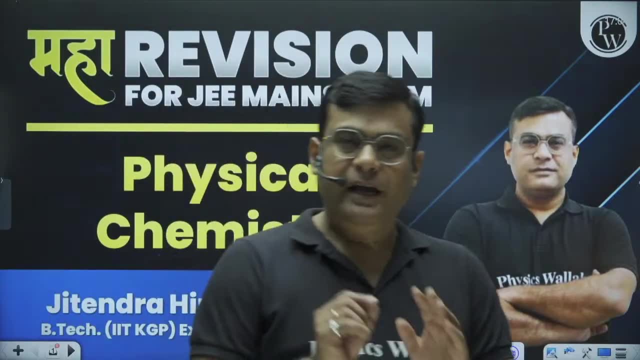 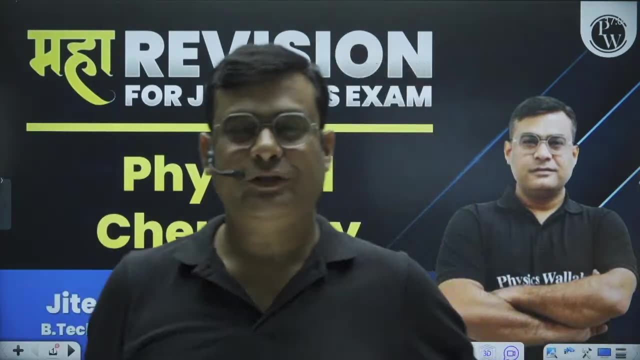 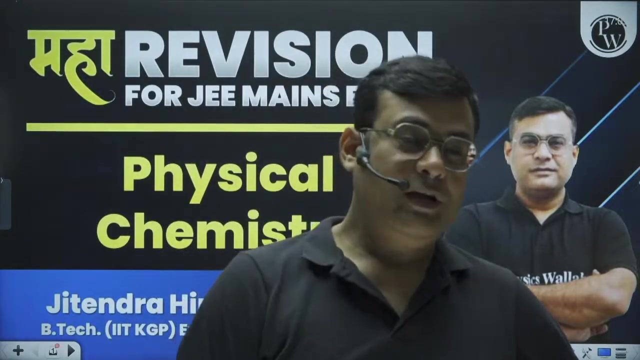 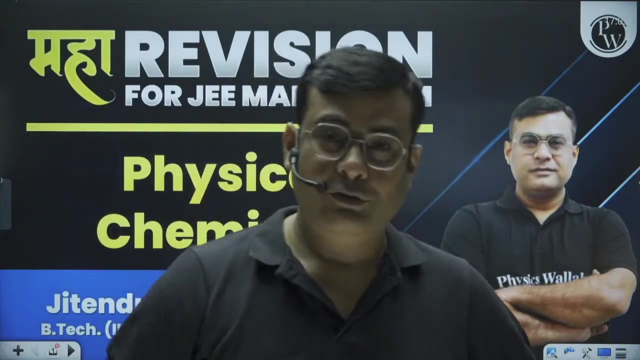 we do not have to deal with any numerical questions for organic and inorganic. there are essentially all asking Jee's question. In many cases you tend to waste the information. You add objects or if you have to solve something, then there are no numericals in the mechanism etc. but now your numericals portion is starting. today is the session of physical chemistry. tomorrow your Manish Sharma sir will take the physics of 11th. physics is complete. you had numericals. physics of 12th will be your next day and after that 2 turns of your 11th maths and 12th maths. 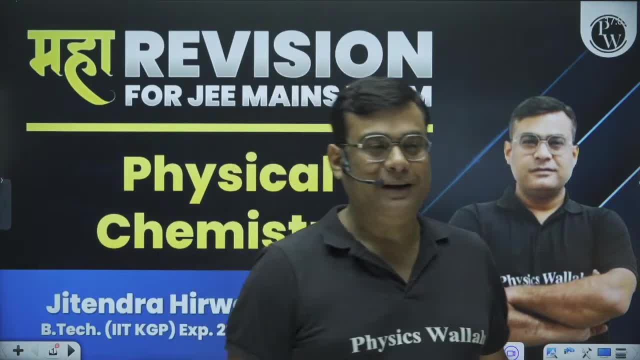 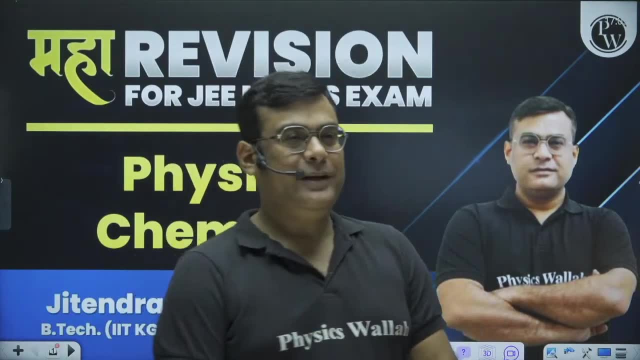 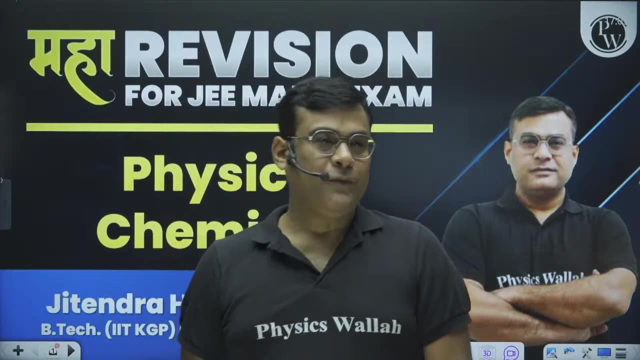 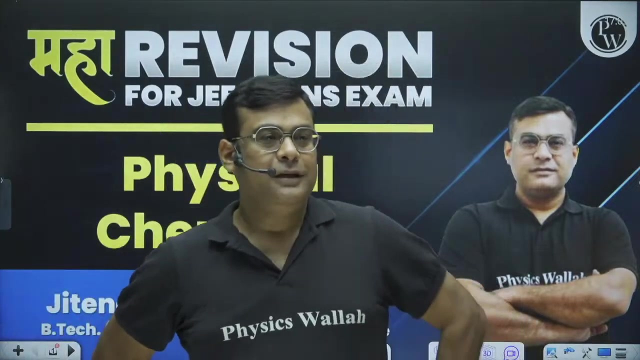 now. the points of calculation of numeral consigliere are about to start and we put ourselves in this situation now because we are giving ıyor a hand to our social students. don't forget, you know the name: HDFC. everybody had forgotten. 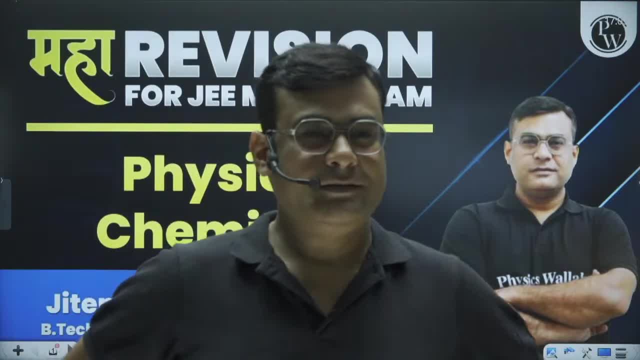 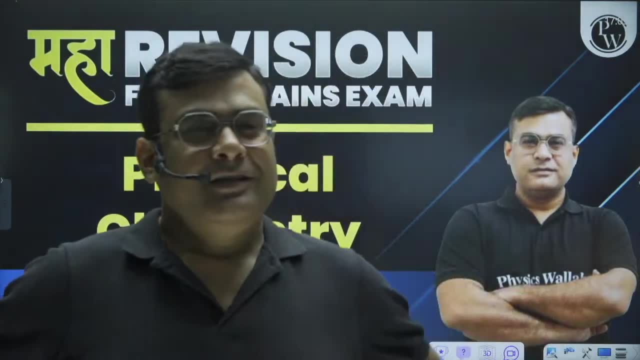 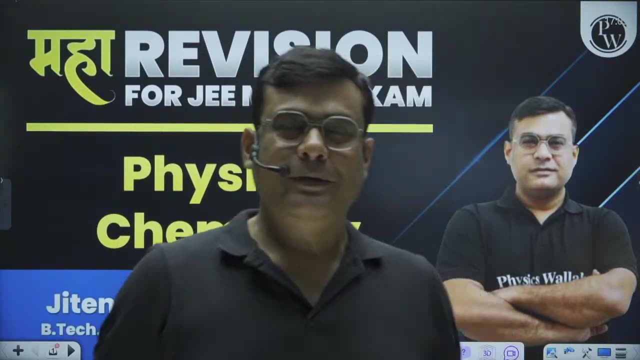 Tell me what are the grades of elementary and secondary school. kids like us. HDFC, do you remember it? list of study. HDFC is not the name of the bank. it will open your account in the bank if you do a good. 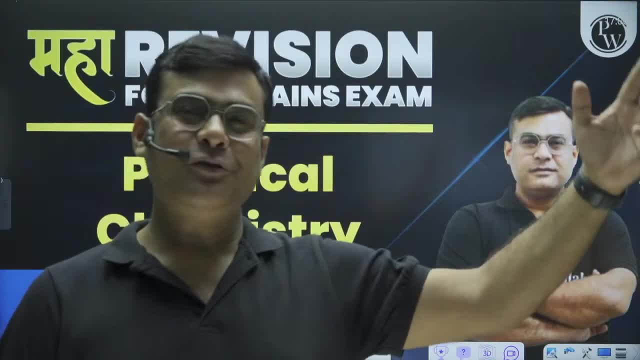 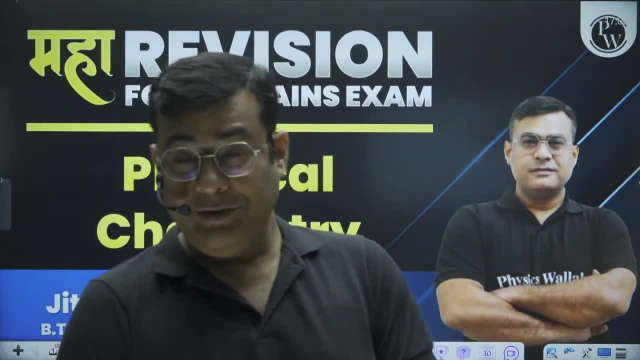 job here, then your account will open in the bank- and I want your account to open in every bank in the world, and your crores and billions of rupees are there in every account. so you must also pay attention to that as well, because one thing has also been said to the person. 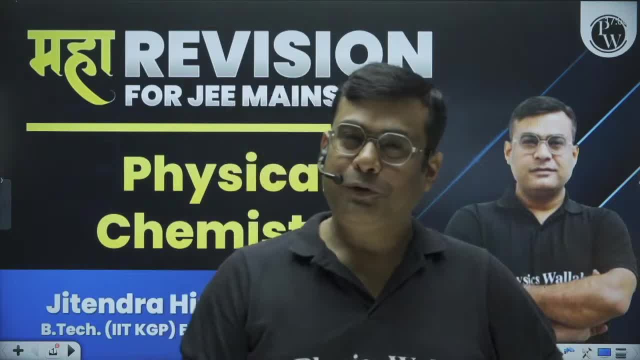 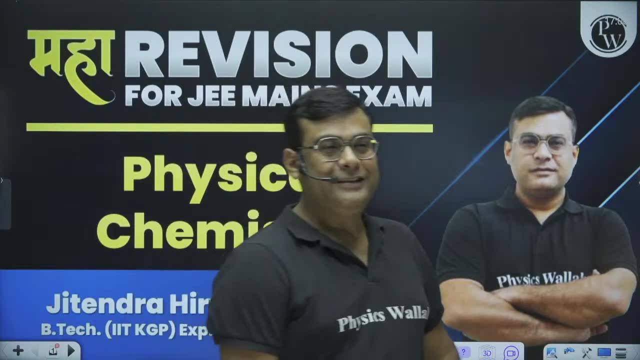 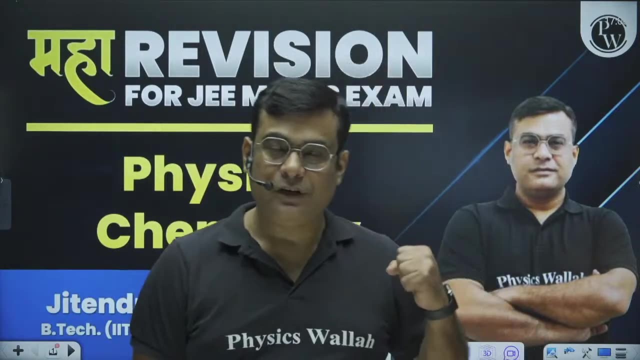 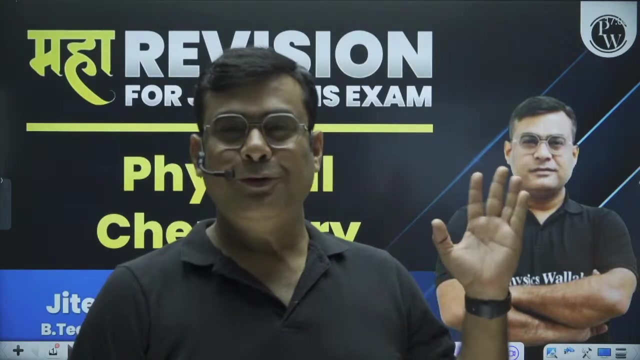 who has spent itself, the world has searched him on Google. the person who has spent himself, the world has searched him on Google. so you will spend as much time as you will spend with yourself. devote time to your studies with honesty. the same will come to you in the 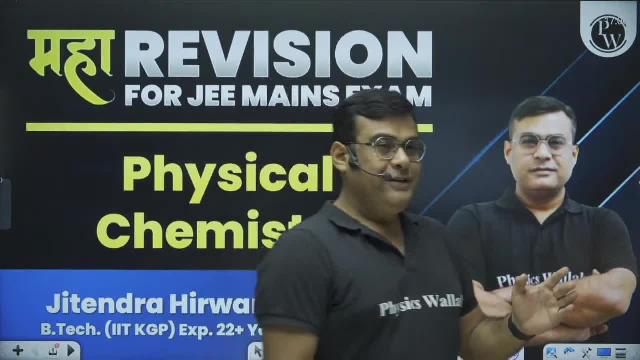 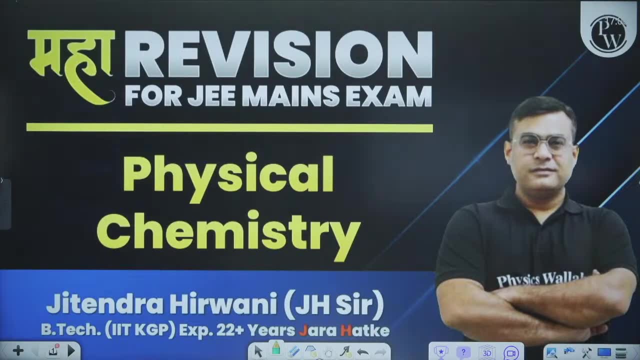 position to search on Google. And that's why there is one more good proverb, brother: that you join your own journey, right? A good proverb is a small one: either you get involved in your journey or you get involved in your journey. 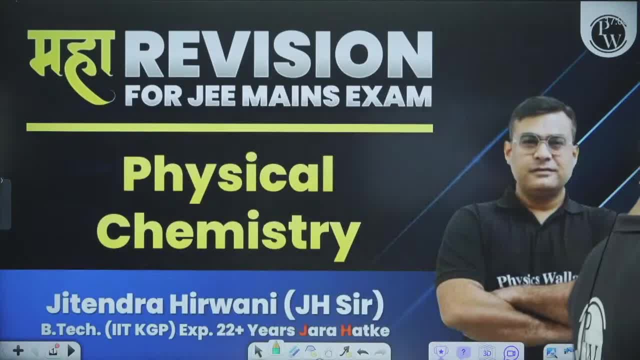 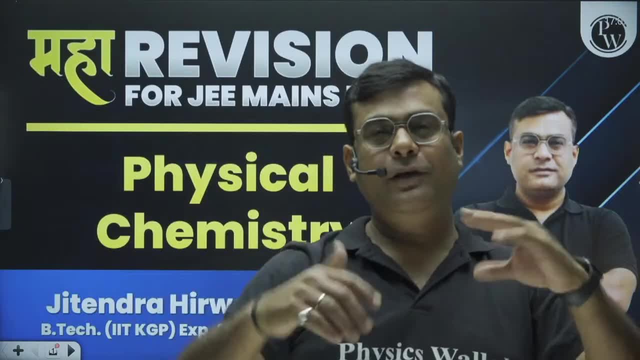 Otherwise, what will people do to you? They will include you in their journey. They will include you in their journey. That means they will do a good job and they will tell you to come and work with me. So I hope you have got a lot of all these lessons. 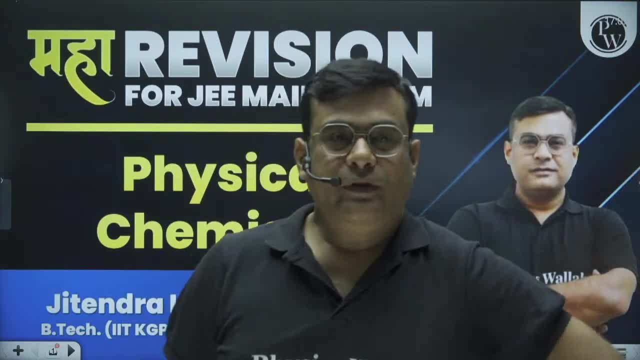 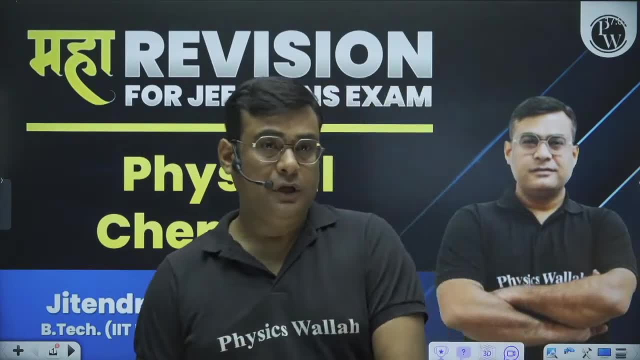 But today's session is going to be a lot of fun because most of the students may have a lot of children. Some will have the 4th, some will have the 5th, some will have the 6th, some will have the 8th, some will have the 9th. 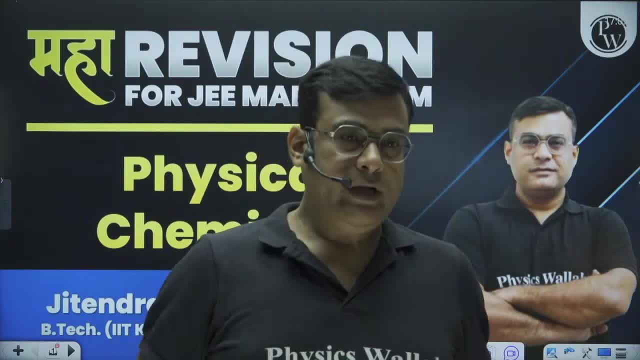 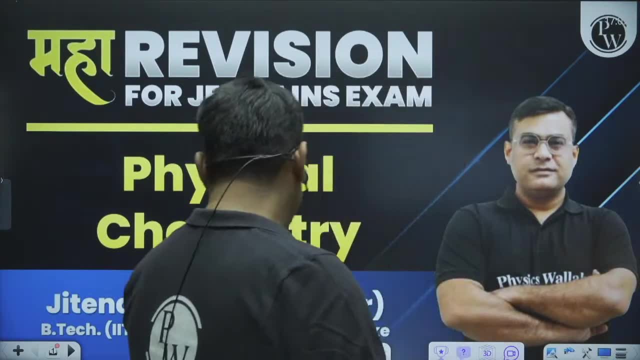 I have brought a lot of questions for you here. We might not be able to solve the whole thing because I have made 341 slides. What have I kept in this? I will tell you that The sequence of the chapter Main concept. 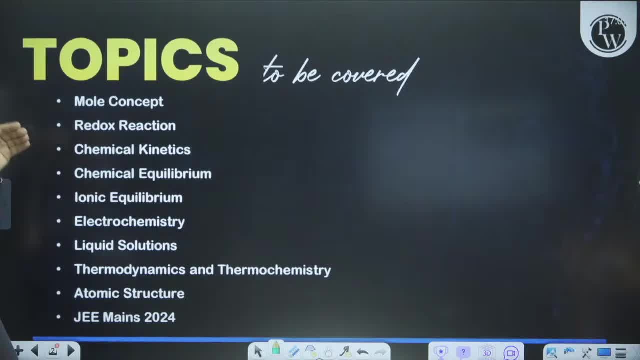 Then Redox Reaction, Then Chemical Kinetics, Chemical Equilibrium, Ionic Electrochemistry, Liquid Solution, Thermodynamics and Thermochemistry, Atomic Structure And along with that JEE Mains 2024.. All the questions that have come so far. 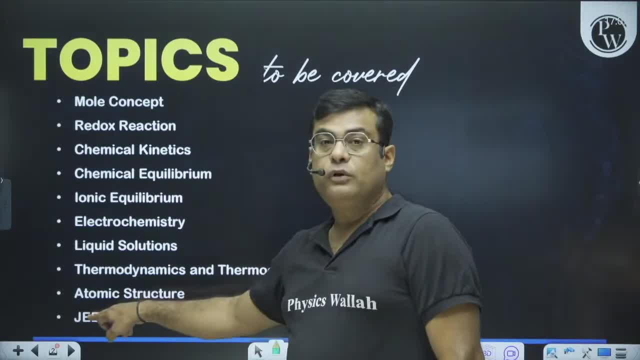 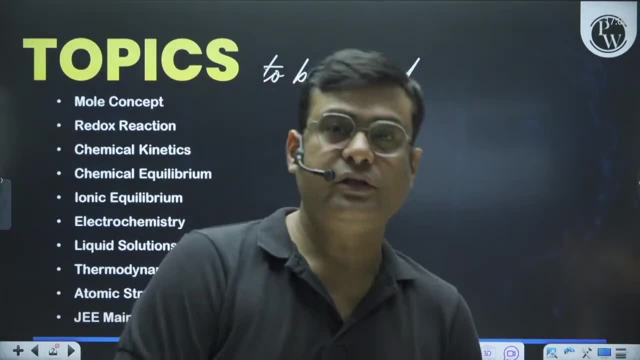 The 2024 attempt. I am going to give it to you at the end at the same time. I am going to give it to you at the end at the same time So that you know that these will be the questions that will start to appear again from the 4th of April session. 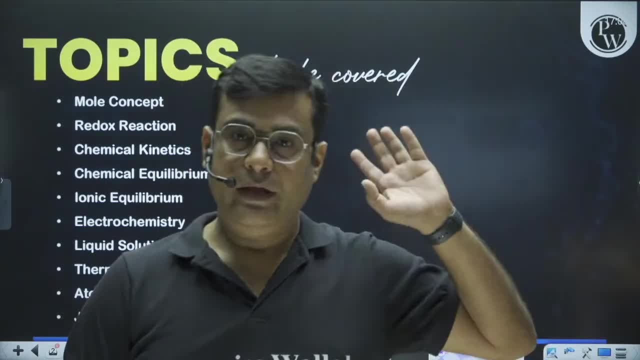 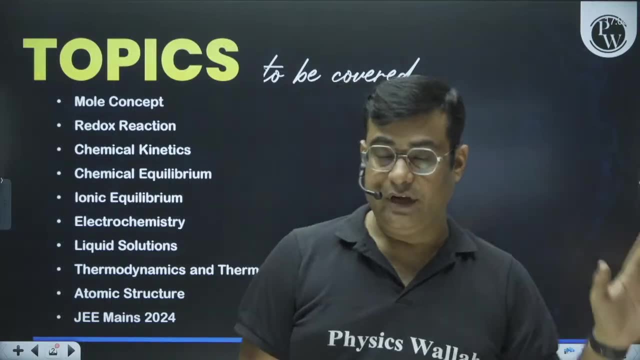 So that you know that these will be the questions that will start to appear again from the 4th of April session. I am going to give you a liquid guarantee of this: that we might solve all the questions here and we will leave something. You should definitely solve it, because still you are having sufficient time. 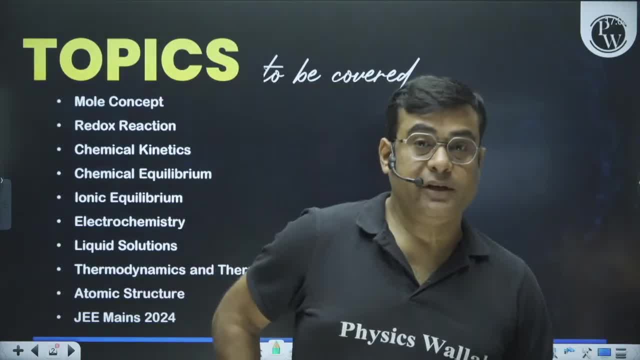 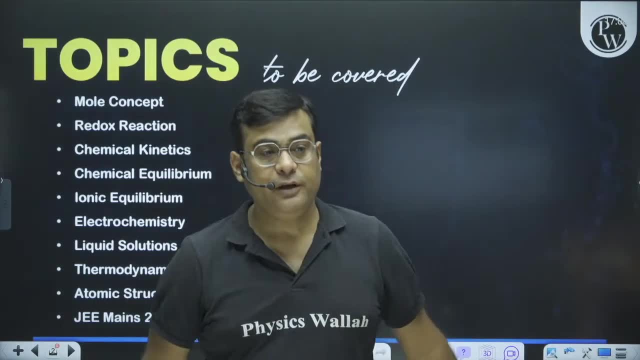 This is a live session in the evening that you have to definitely attend because you will definitely benefit from it. Every teacher who has a crispy content, who thinks that these are the most important topics, there is a full probability of getting questions on this topic. 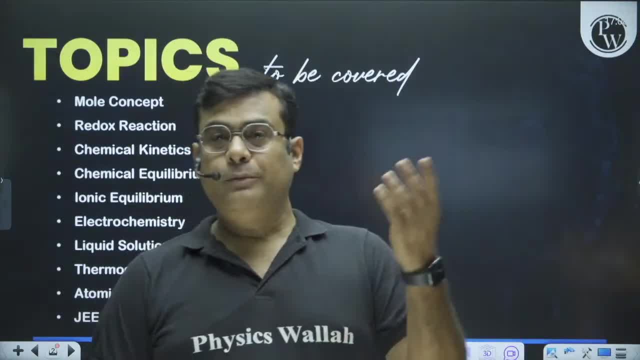 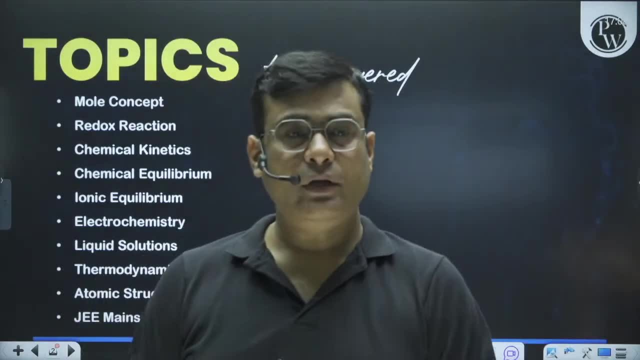 So you should attend the evening session. Apart from that, there is 31st, 1st, 2nd, 3rd, 4th day of which is 4 days, So now we can definitely do this work, because now I hope that your theory must have been completely finished. 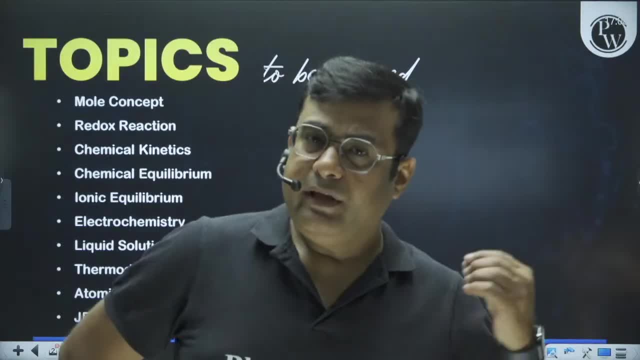 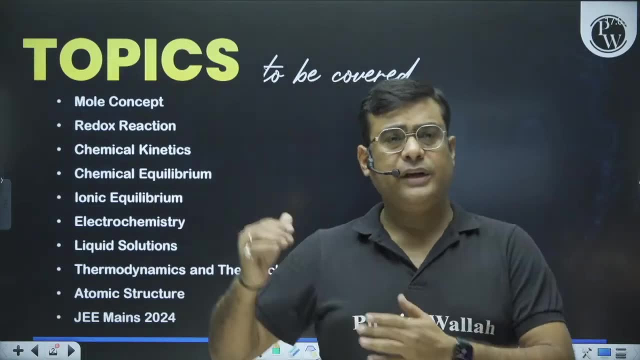 You must have finished it well Now in the revision, only the crispy formula that you have made, the short notes, etc. The formula is only 2-3 page And apart from that, you should definitely see the questions. Okay, children, so let's go to our next thing. 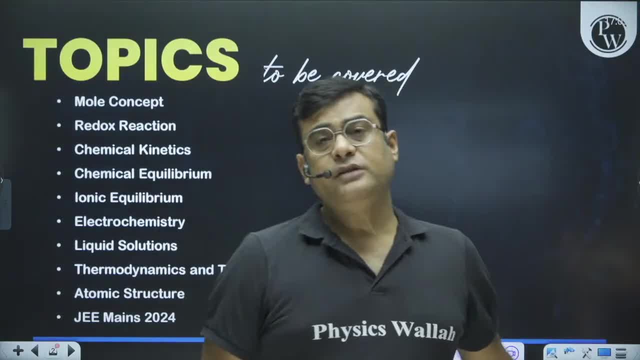 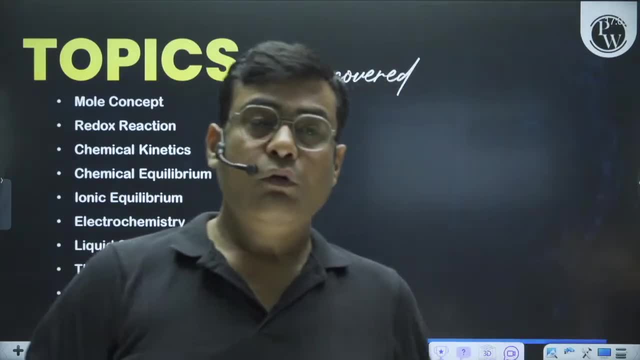 Okay, children, so let's go to our next thing. Let me tell you that JEE Mains is a repetitive exam. It is a repetitive exam, So you will start seeing a lot of questions from these questions again from the first session of 4th of April. 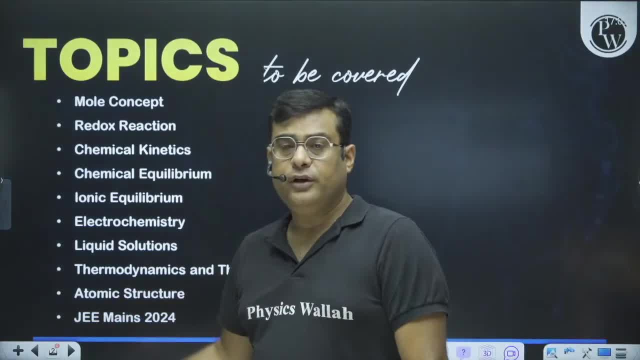 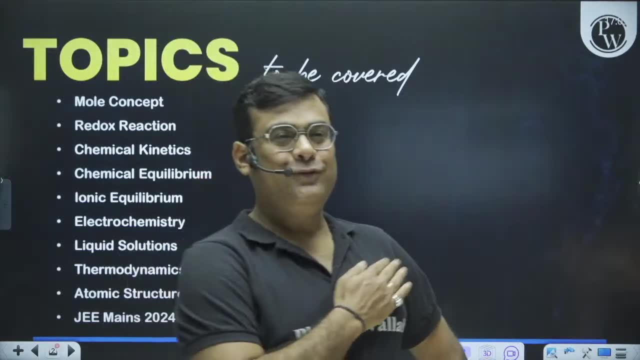 In fact you will do all the questions of JEE Mains 2024.. So I am ready to give a written guarantee I will hit the chest. I will not hit the chest. My heart is in pain, Then the chest hurts. 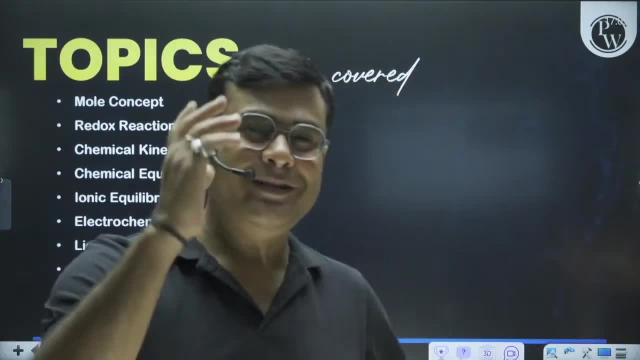 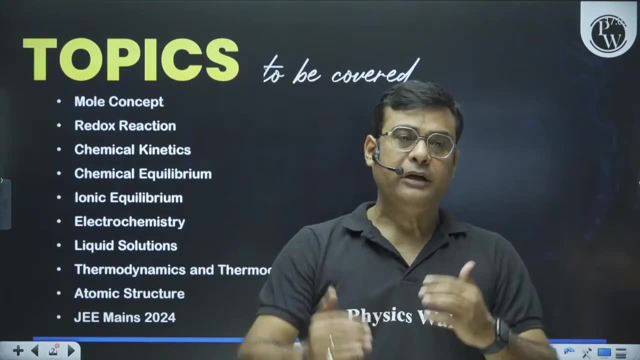 Okay, So we will not hit it, But we will definitely say this much: The last 90 questions that you have- I will not say as it is, But on the same concept you will get the same questions. You will get to see at least 20-30% again. 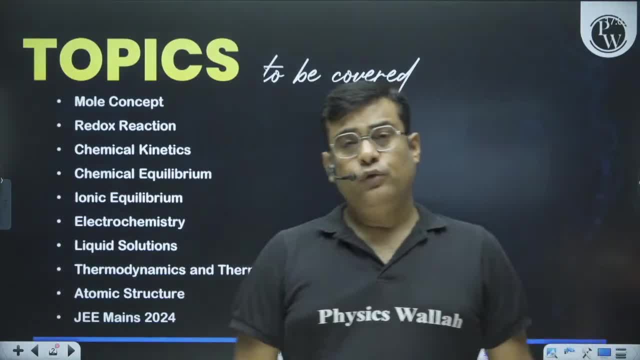 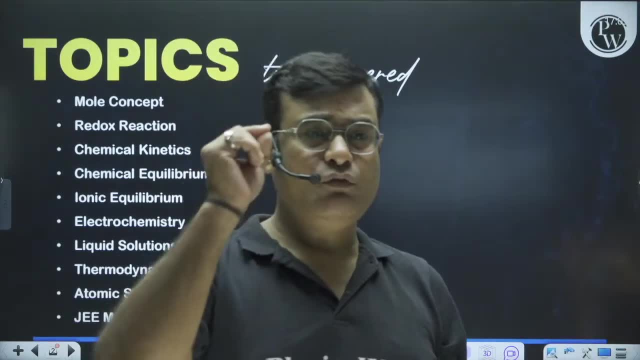 JEE Mains is a repetitive exam Which he has asked in 19,, 20,, 21,, 22,, 23 and even in January 2024.. He will ask you the same questions again and, again and again. Duration: there is no such plan. 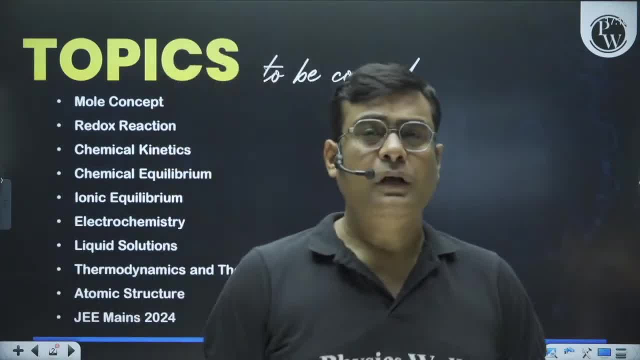 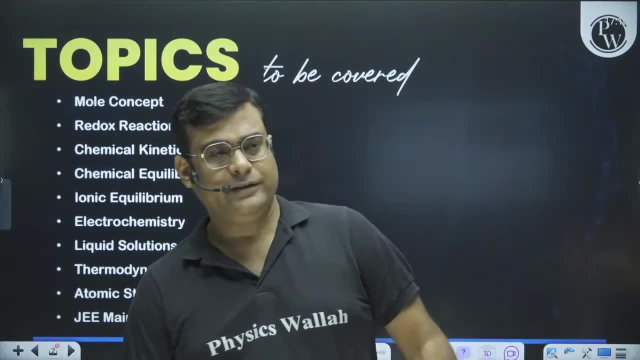 But at least for 5-6 hours you will tie your waist belt. We will take a break in the meantime. obviously, Then I will also have a little tea. You will also take a little break. But that break is fine. 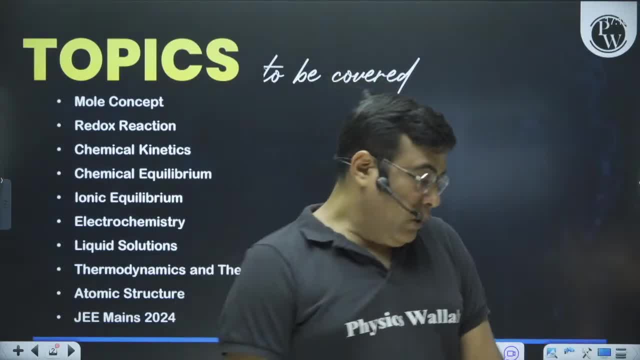 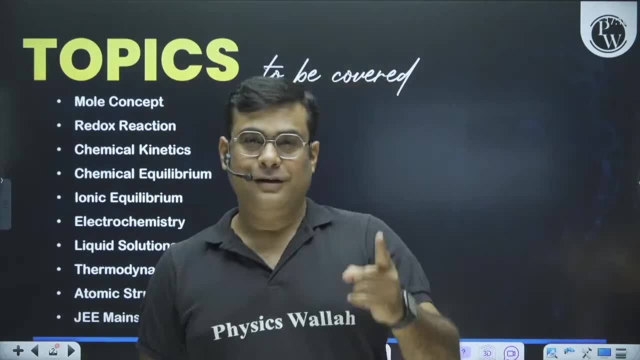 We will try to take it on half a step. So tomorrow, your 11th physics session is going to happen. Manish Sharma sir, who will take you? So our army is 3.0.. Prayas is 3.0.. 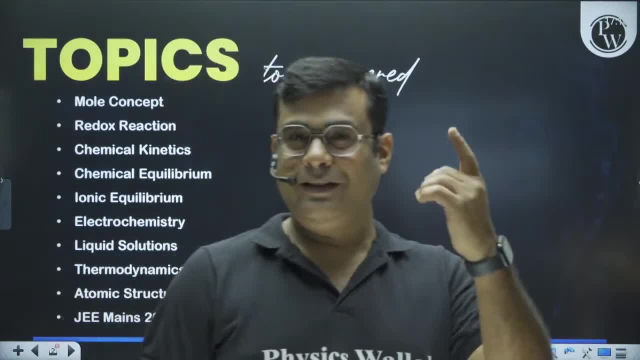 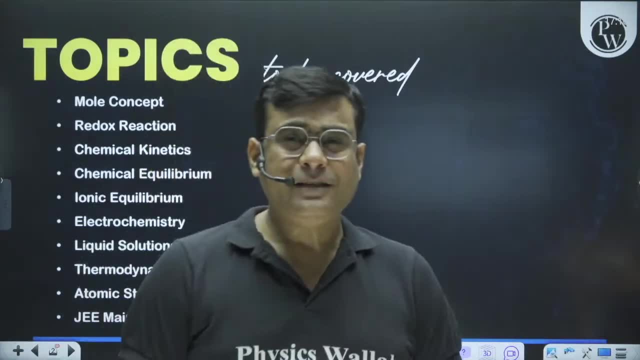 In that we have a national competition. In that we have a national competition, We will sing that anthem and start our story. What is that national anthem? Come, come, let's squeeze our hearts, Let's break the pot of Pandavas. 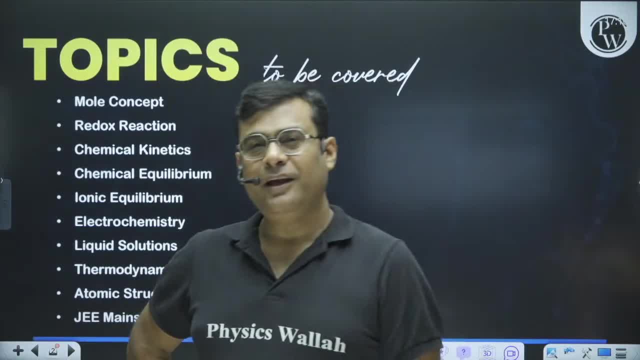 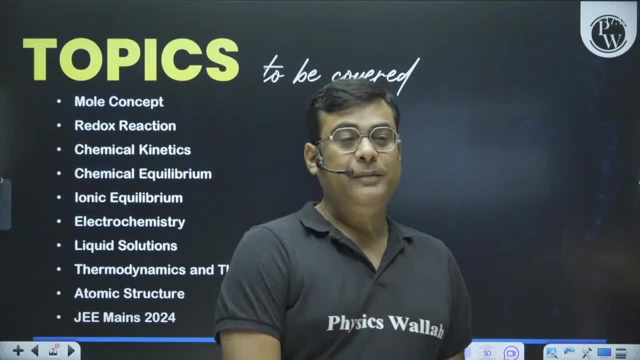 Let's take out some jaggery And break it. Day and night. play the game of hard work. Day and night, play the game of hard work. Luck is the day of hard work. Come on, Let's go Where to go. 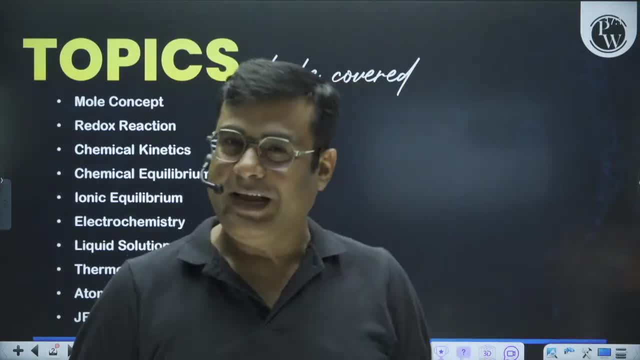 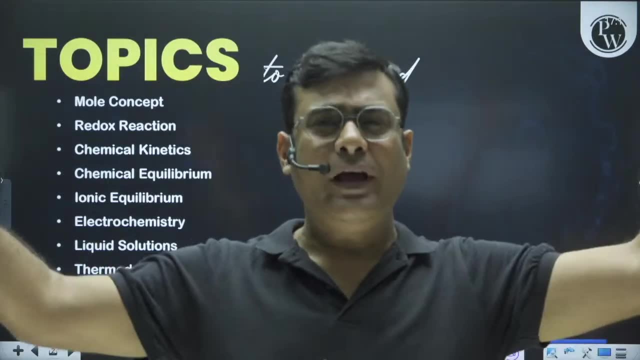 Come on, Come on, There will be a Dhen Dhen in IIT. Dhen Dhen, nennnnnn. Okay. so, whatever happened in the past, kids Before today's January, attempt, no matter what percentage is yours. 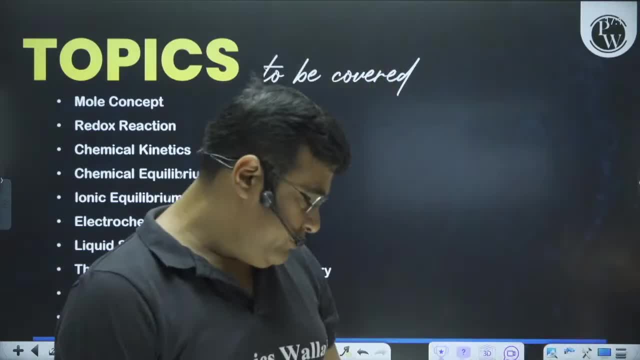 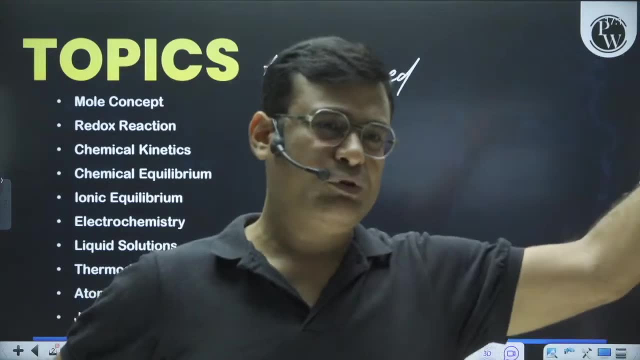 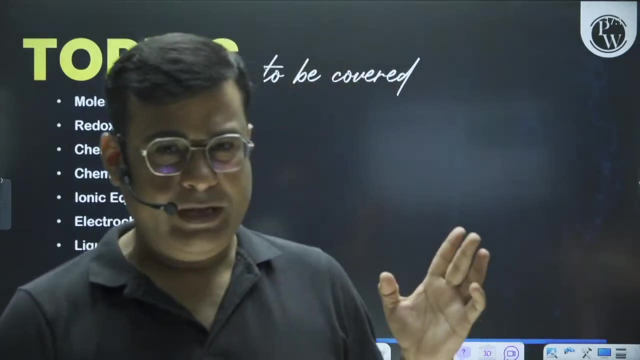 Forget about everyone, Because Chanakya said a very good thing: children, The man is not as sad by his mistake as he is sad by remembering that mistake again and again. Then those are all old things. What is our work today? that you must keep red chili, green chili with you, let us tell. 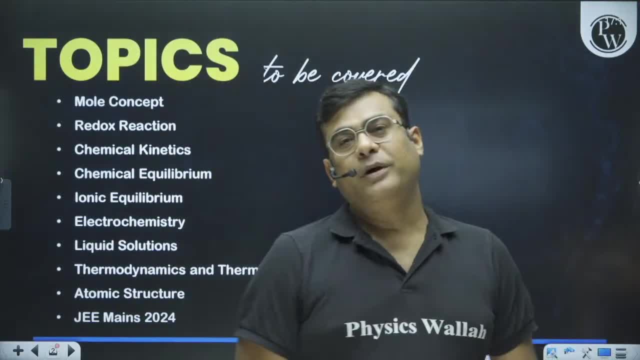 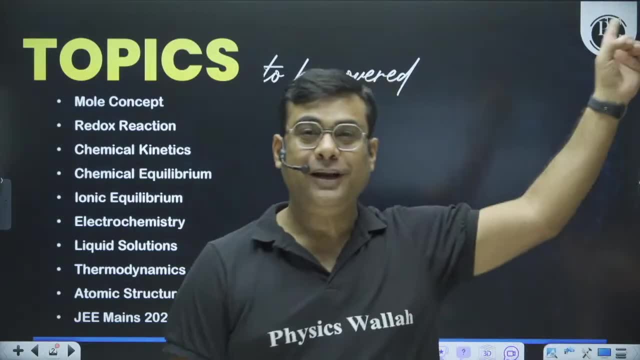 every child with three points. because it is natural to fall asleep. it is a song that I do not sleep, I do not rest. but when I do not rest, that is the second reason. but I do not know why the children fall asleep in this good work. then the reason for not. 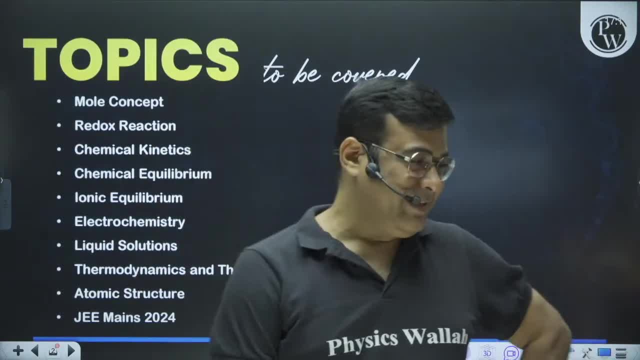 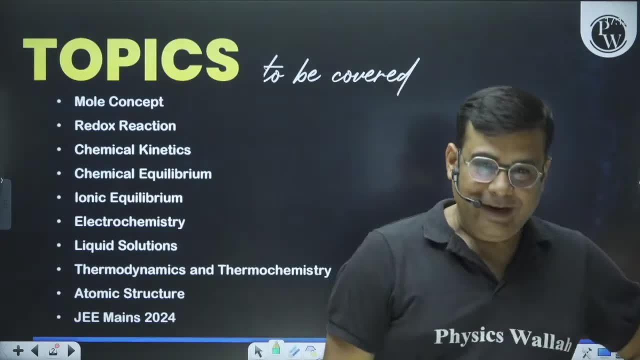 falling asleep is different. you are wise. I know everyone must have understood that. when does sleep go away? but now sleep will definitely come. then keep red chili, green chili, okay. take a cup of tea and coffee, okay. and remembering the Lord, okay, remembering. 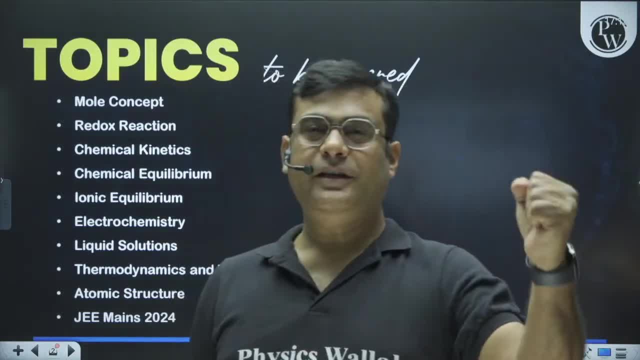 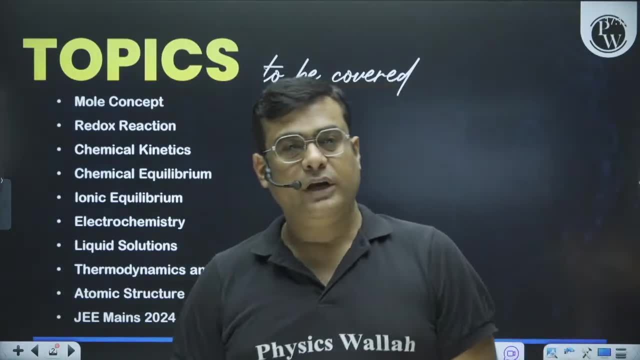 the Lord, that brother, give us the power to understand today's session. okay, we are going to start our session with full positivity, full energy, full smile. okay, so let's listen to one more line. the children are saying: give us so much power. 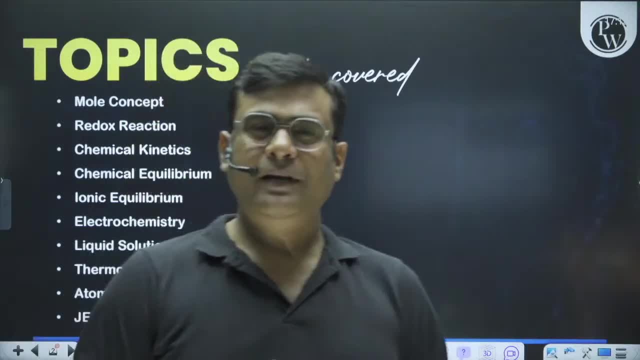 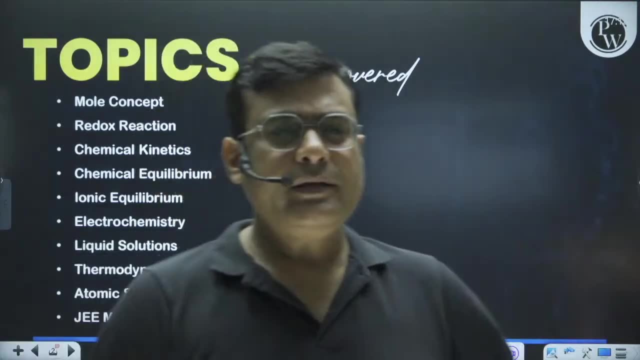 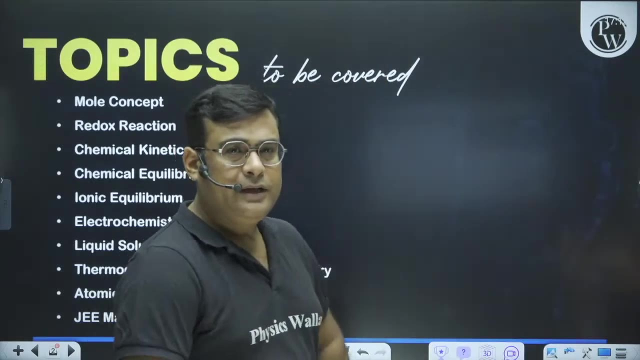 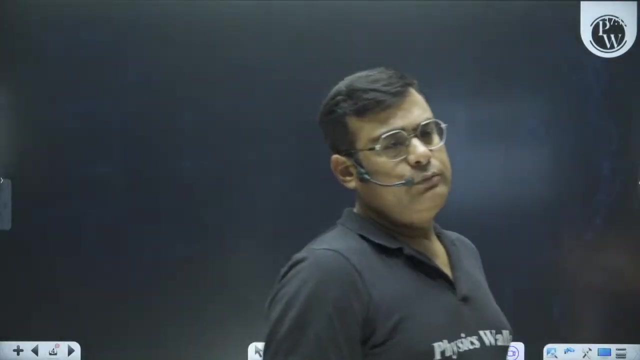 Give us so much power, the faith of the mind will not weaken. we will walk a good road. no one will forget us. okay, now, no wasting of time. first chapter: we are studying what is the concept in one crispy, two or three formulas, which are most important. 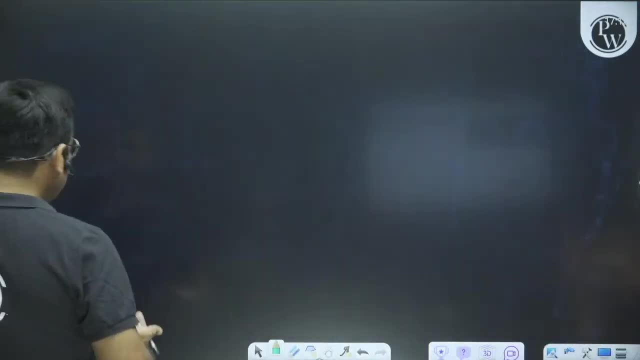 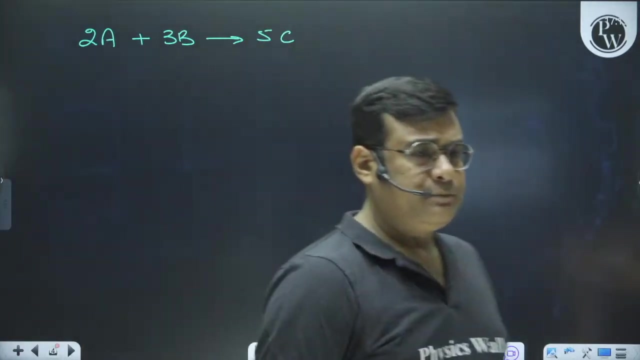 by telling those children we start our stories straight, or two or three. most important important formula to the most important concept that he more concept which is up to the door look to know. but Choco, what for us? a make questions, get through it from jungle manly jigger Amari. reaction a to a plus 3b gives Kappa 5c. 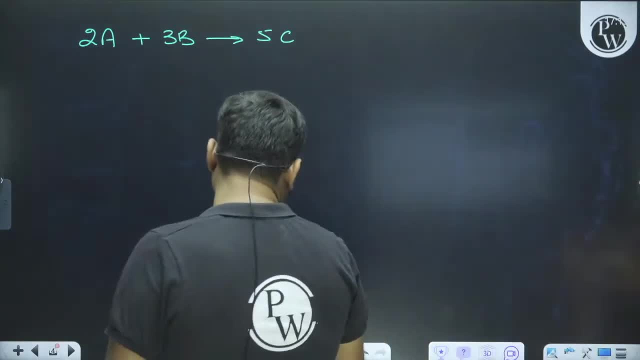 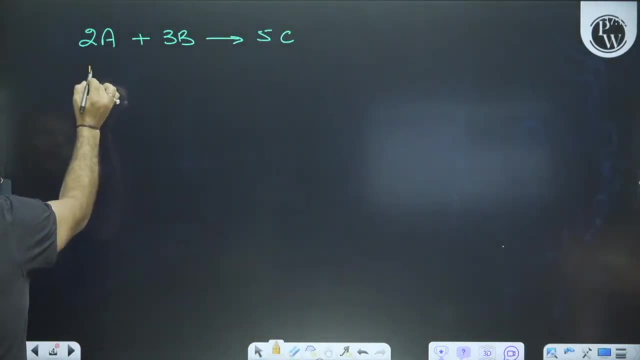 for a reaction given: a up gonna or a garish maybe, but show up with single reactant Kaim on the given single reactant malady. I'm so bold, like if I'm having one point, two moles of a. so battaglia. but to battaglia seek a. 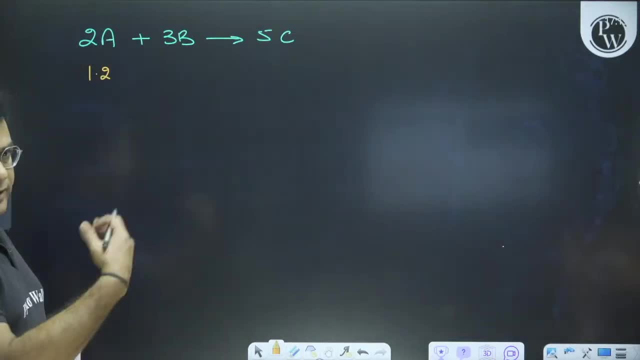 kitten a most required only seek a get remorse, but mother required only key jacket. a bolega produce only a bover. ding my question. but I'm not a kid, a guy up to wallet, but a better abhi who were ring while a question to me, right. 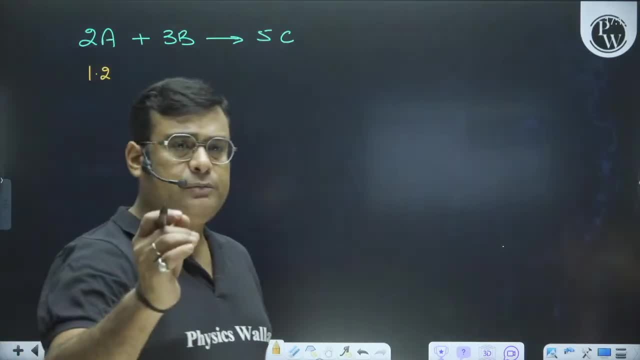 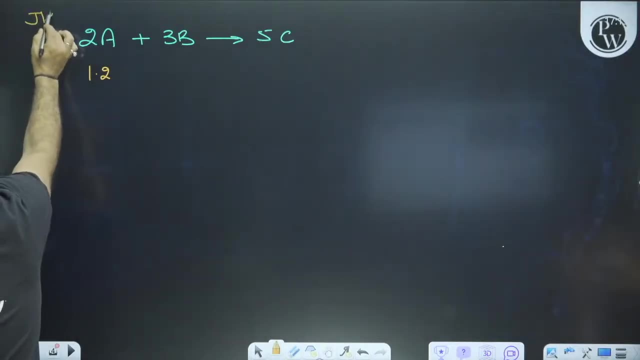 so agar is my kissy be Taraki, apple chotis a be do vida ho, but show the bus may just the second lecker. a quick trick, but I didn't, a charo, you know. but she'll say: JSC can answer the root. janta Amara. 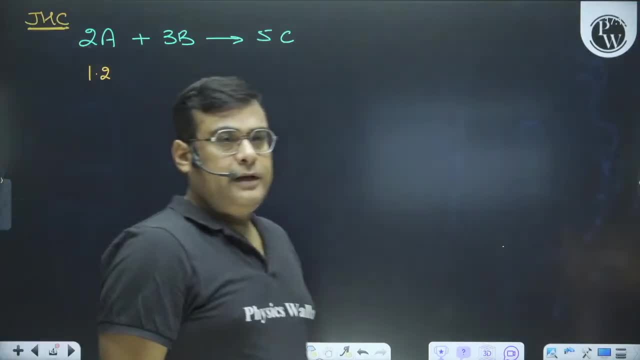 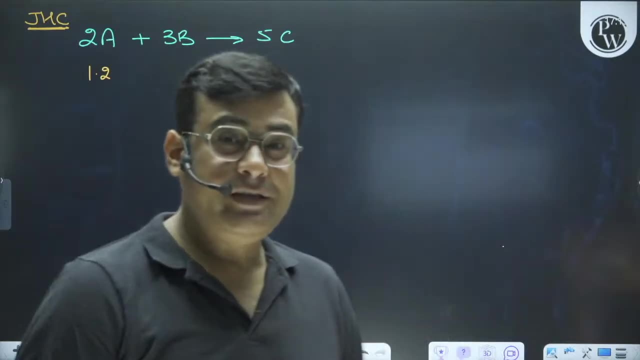 you know a bar, JSC can amper and a bill. they did a giant deal memory a dada disco. you keep kind of getting a bunch of okay, but the bottom which has JSC care, JSC Jara had a concept in a ticket, it so a. 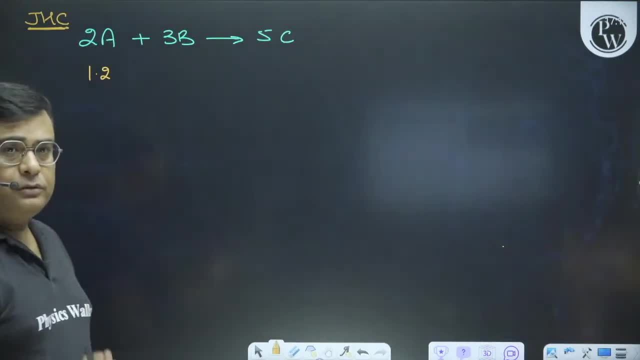 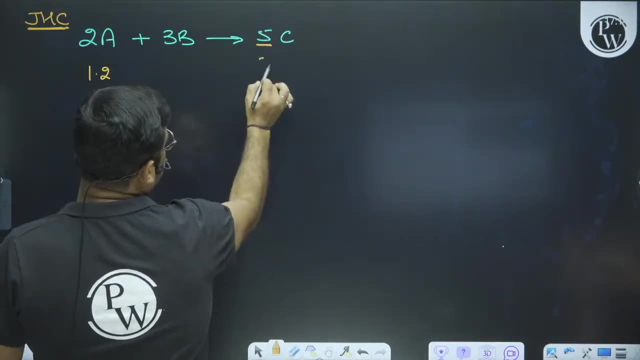 total to take on seven. but you got. but what? Allah hotel, a mirror pair, pair of a show. ask about up to nine yoga to kick simple, see up concept. laga de jayaka just gave me most nickel new on a seek an economy to seek a coefficient. 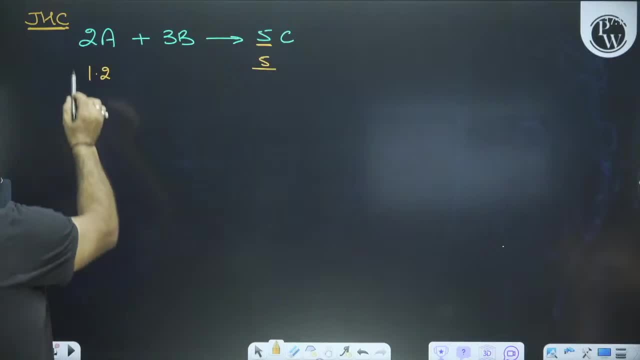 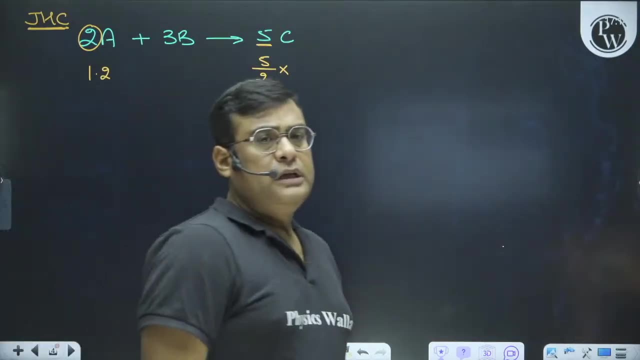 five kiss a nickel name but chose our a camels in economy at a chi statue material. How much is the stoichiometric coefficient 2 and from where do we know the stoichiometric coefficient? We know the stoichiometric coefficient from balanced chemical reactions. 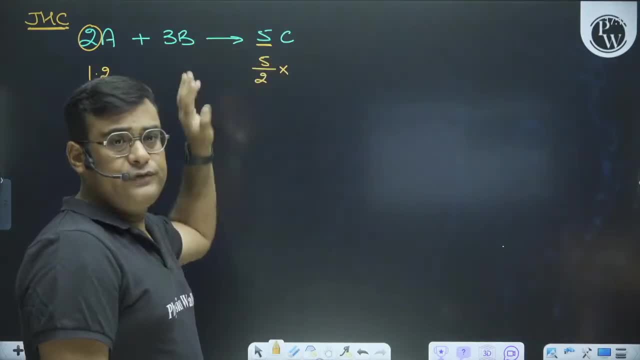 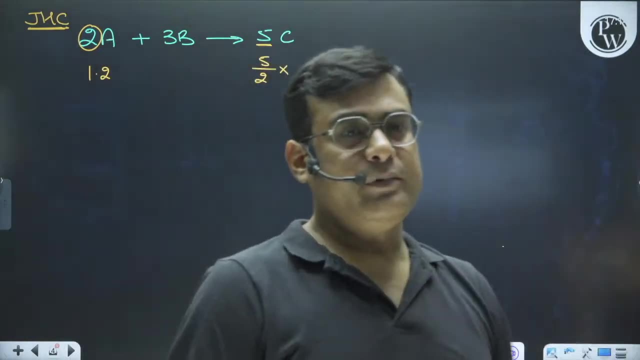 So right now I am assuming that this reaction is balanced, because the coefficient is mentioned. If it is unbalanced, then the coefficients are not mentioned here. Then the vocabulary would have written that A plus B gives you C, And if you want to take it out from A, then A's moles are 1.2.. 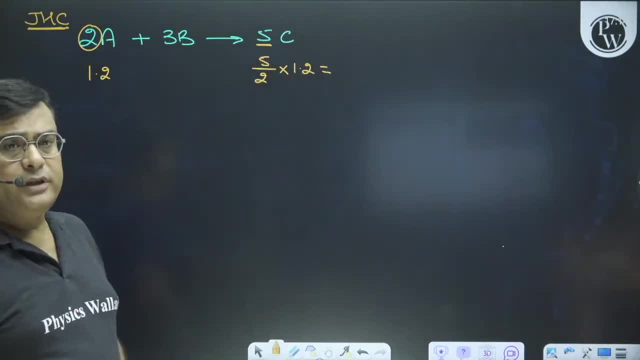 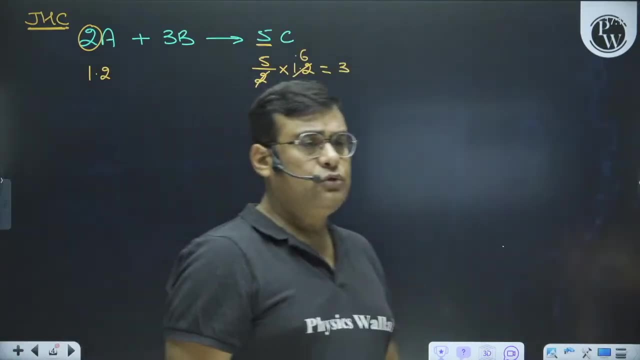 So you will definitely see a lot of questions on this. children, If any child has any kind of this kind of because in the mole, many times the child makes the most mistake in taking out the moles from one of the moles. 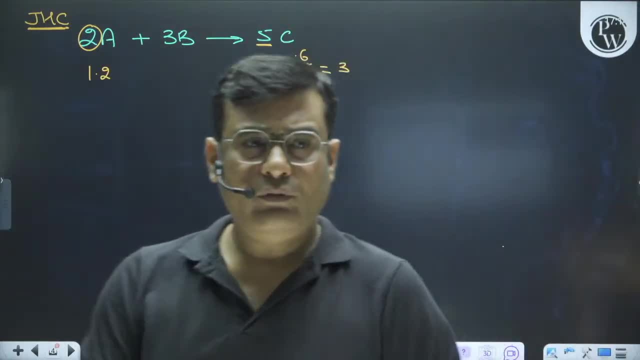 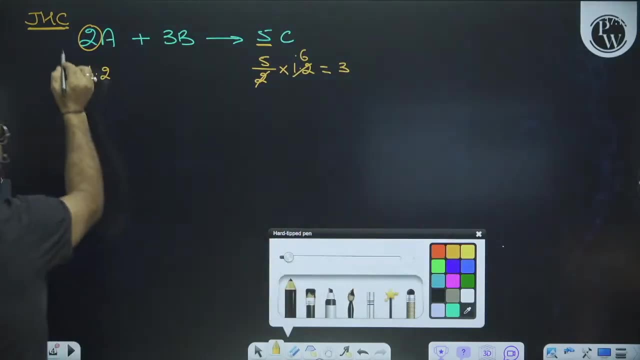 If anyone has a doubt, then after today. I think now this doubt will be solved by you. The story is over Now in this, one more smart person can do it: Jaiwala, who will also do it. This is a single given to you. 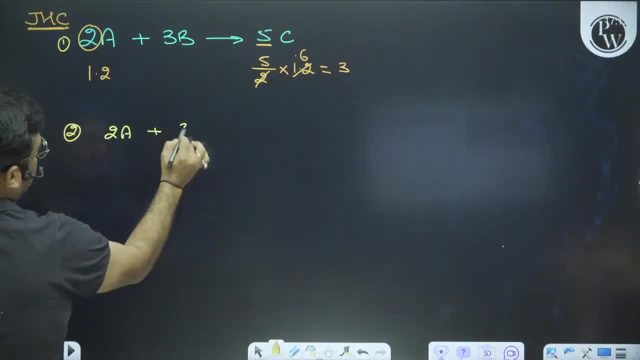 Suppose this is the reaction: 2A plus 3B gives 5C. This is the reaction: 2A plus 3B gives 5C, And the question would be that A has 1.2 moles and B has 1.5 moles. 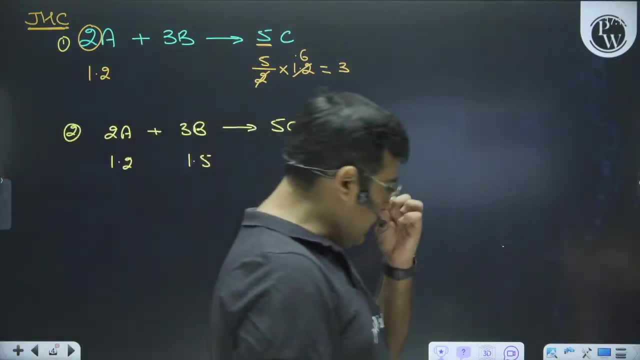 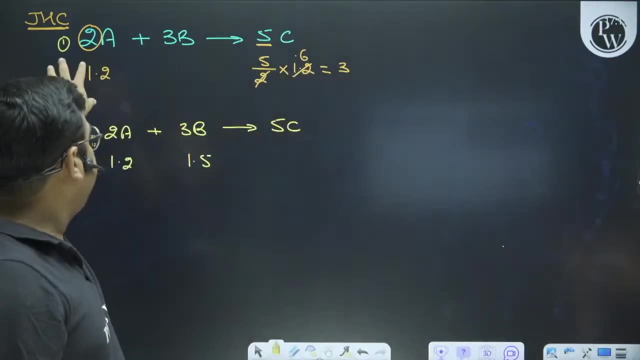 Now the question is: how many moles will be made of C? Now tell me how many moles will be made of C? So you have to take care of both the situations, children. If there is a single reactant, then you just have to do this little work. 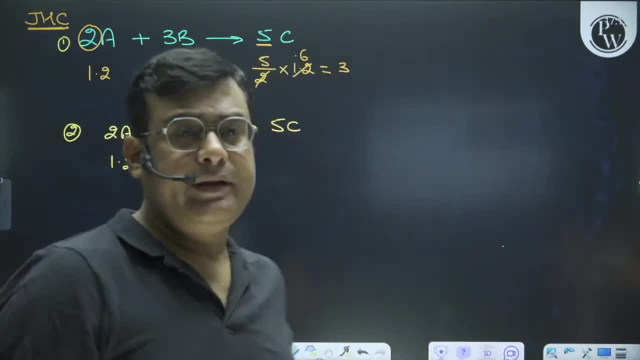 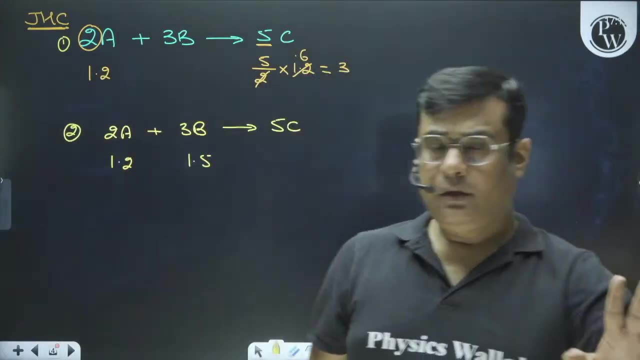 But if, if, if, if you get a double reactant, that means you have given two reactants at least. And I have told you all, children, that there have been a lot of questions on this in JEE. I don't know how to lie. 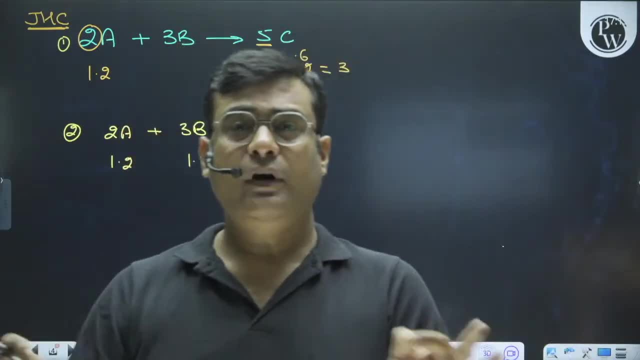 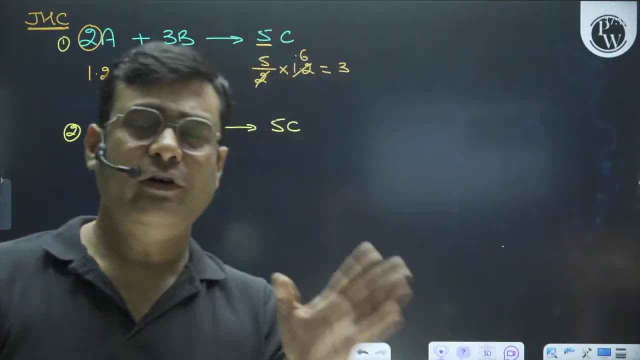 I am a true, simple, good, wise, rich, strong person, So I can't do this kind of nonsense, that I will lie to you, Okay. So, brother, this is confirmed, that the question is coming. JEE has also come in the 2024 January attempt. 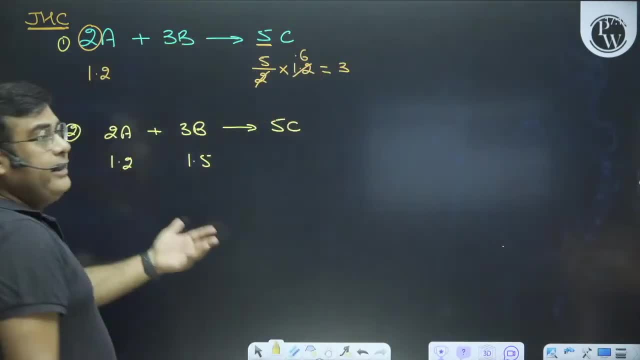 In this question. you first of all have to take care of the limiting reagent As soon as two reactants come, then you have to take care of the limiting reagent. And how do you take care of the limiting reagent, sir? 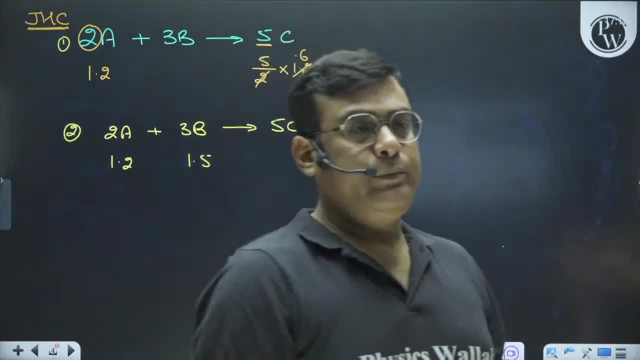 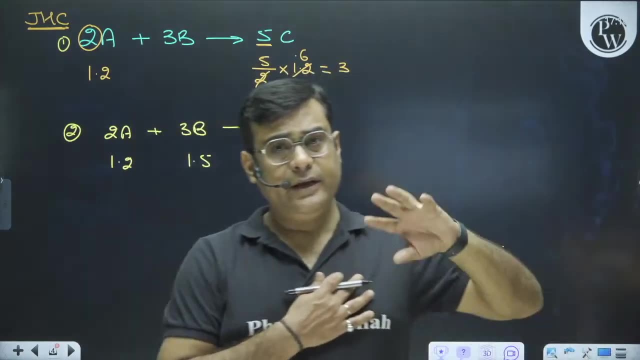 Each of the given moles has to be divided by their respective stoichiometric coefficients. Okay, Every good concept. whatever you feel, children, whatever you feel from your heart that I didn't know this thing now, because here the welcome of all the children of Bharatvarsh is there. 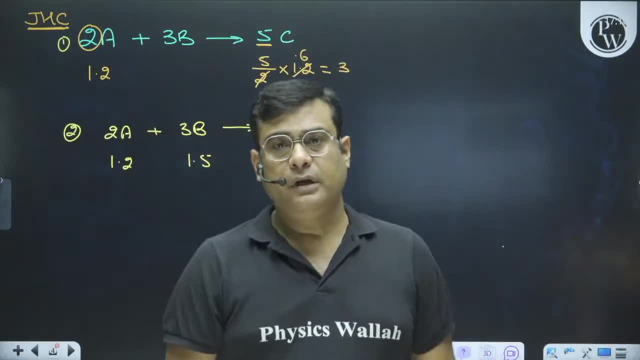 Our PWK will have children of every batch who are going to write JEE Mains on 4th, 5th, 6th, 8th to 9th April in the next five days. But there may be some children from outside. 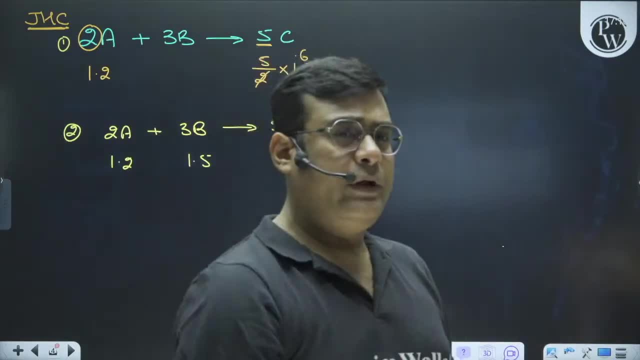 So, whatever thing you don't think about it, definitely write on it, Okay, So that we also get to know that you are understanding things. you are feeling something different, Okay, So in this, children, you will divide 1.2 by 2.. 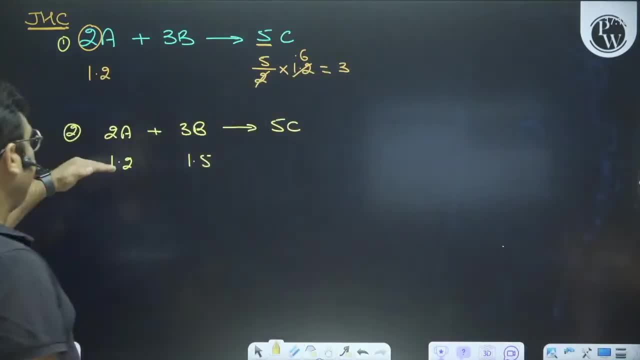 Now, dividing does not mean that you have to swear and wait. If I swear I will divide, then I will do it. Money: You have to take a rough idea. Okay, Divide 1.2 by 2.. Sir, 0.6 came. 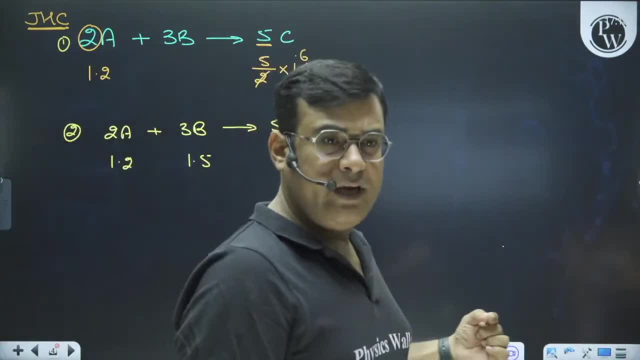 Divide 1.5 by 3. Sir 0.5 came, For which the ratio becomes small Children. it is a limiting reagent, So you have to divide 1.2 by 2. Sir 0.6 came. 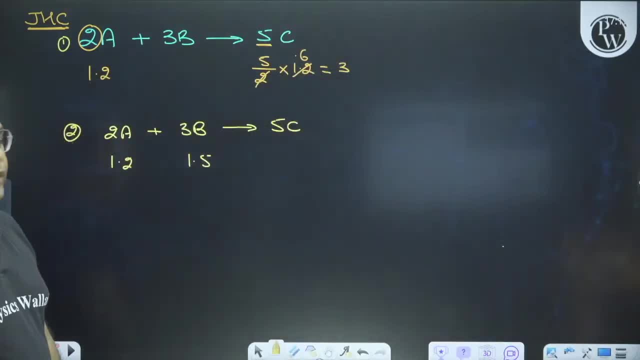 Divide 1.5 by 3.. Sir 0.5 came. Divide 1.5 by 3.. Sir 0.5 came. Divide 1.5 by 3.. Sir 0.5 came. 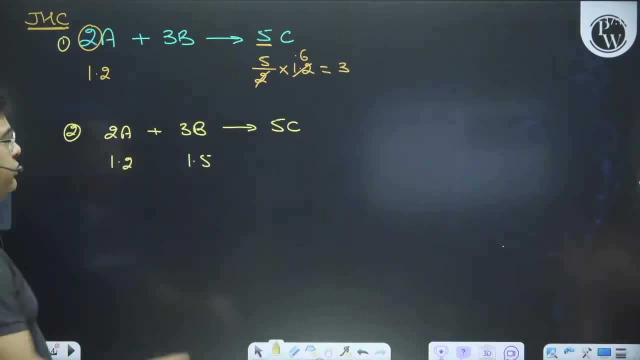 For which the ratio becomes small: Children. it is a limiting reagent. So, right now, your limiting reagent is B. Right now, your limiting reagent is B. Okay Now, if you have only been asked about the value of C, 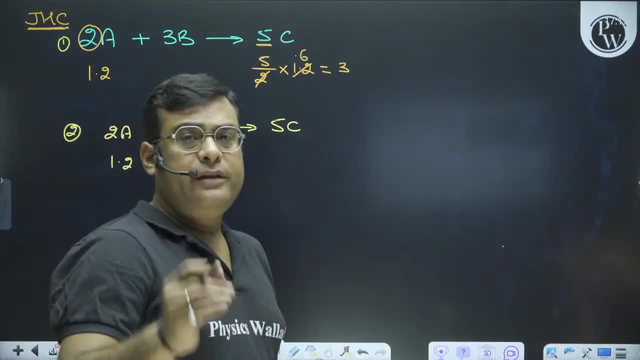 So now, after recognizing the limiting reagent, this question has also become like your single reactant. You just have to do this much. What to do, Sir? 5 by 3.. C's coefficient is 5.. B's coefficient is 3.. 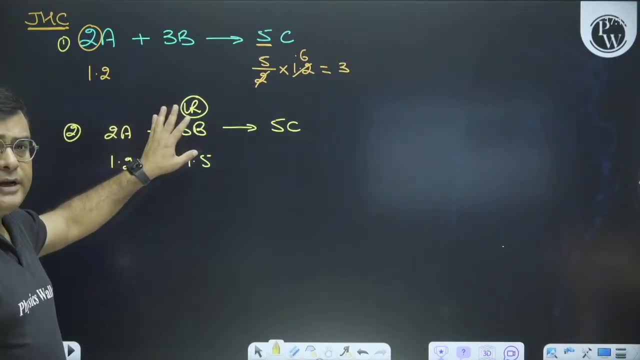 Because it is a limiting reagent. So this is also a limiting reagent. Sir 0.5 by 2.. Sir 0.5 came. Divide 1.2 by 2.. Sir 0.5 came. 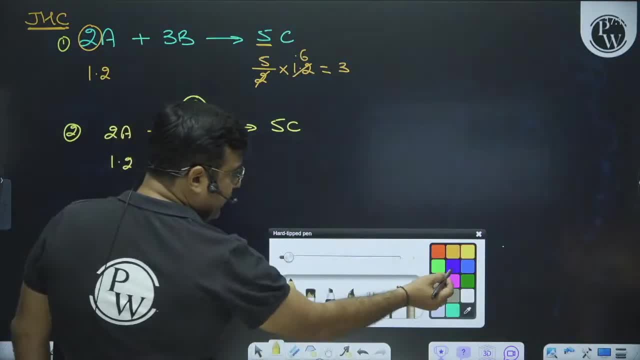 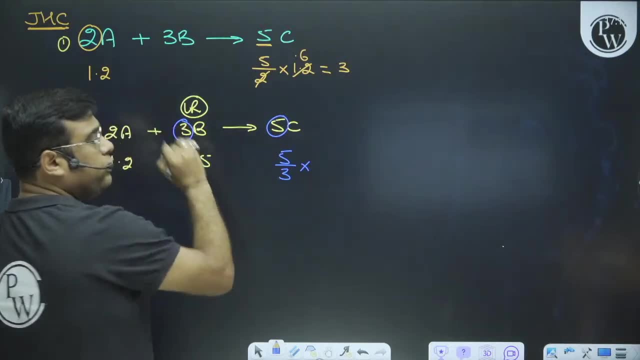 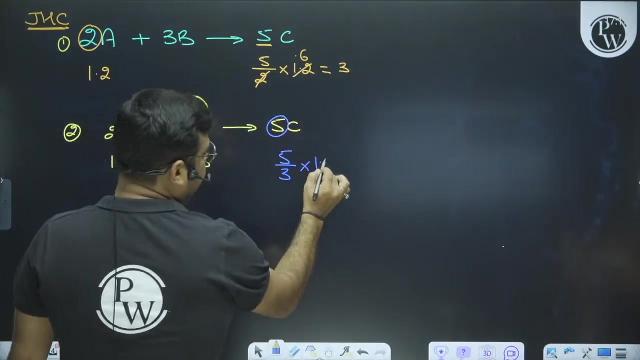 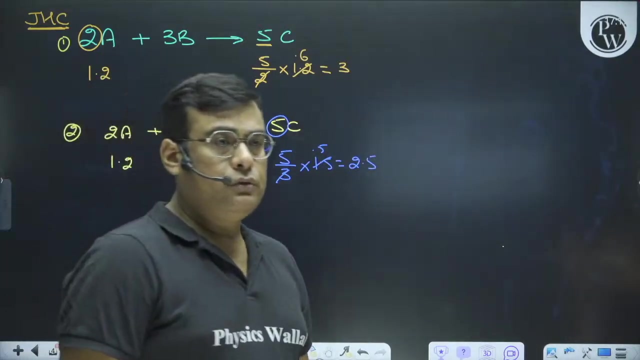 Divide 1.5 by 3.. Sir, 0.5 came Because the limiting reagent only decides how many molar products will be made into 1.5. So your answer will be 2.5.. Right, Obviously, children, if B is a limiting reagent. and ask about the product you have to pay. 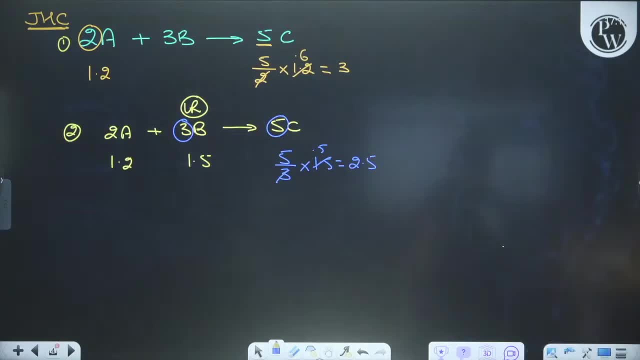 attention to 3 situations And, as I saw, the students made a mistake in this work. Yes, No, No. Then only you can get rid of the problem. I am doing this to save that problem. I have given tea to you as soon as it came, so I am doing cheers with you all. 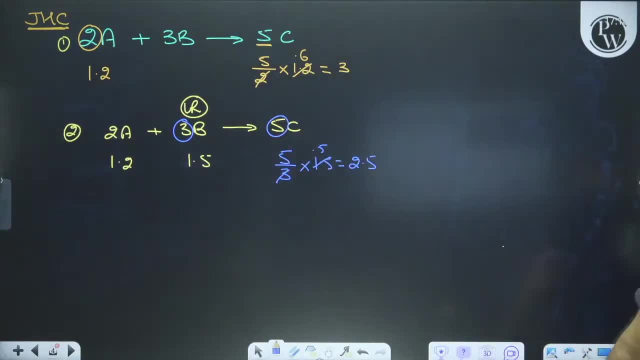 I had just told you that you also take a little bit of your tea, coffee juice. Keep applying the name of red chilli, green chilli. So what I am saying is that, if only the product. what are the three situations to take care of? 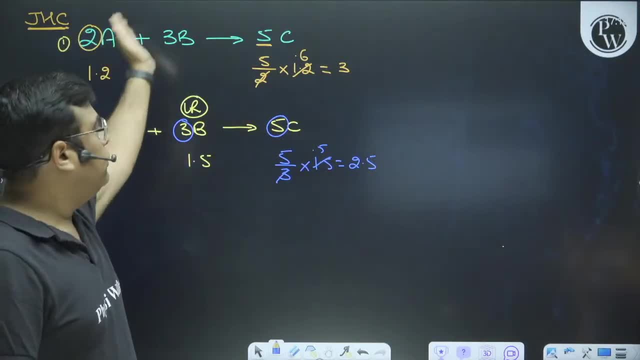 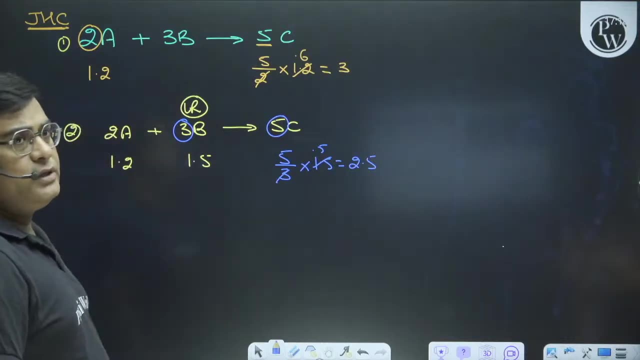 First, only one substance is given, ask the second substance from it. Next, the amount of two substances is given, ask only the product. Now, what can be the third situation, Brother? obviously, if B is a limiting resident, then A will be an excess resident. 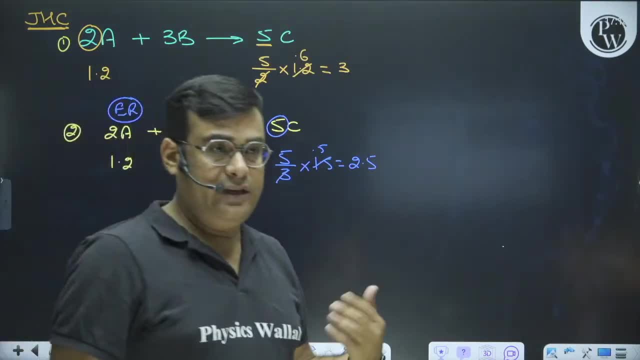 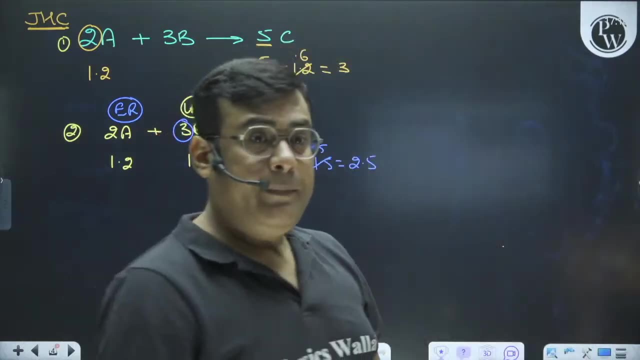 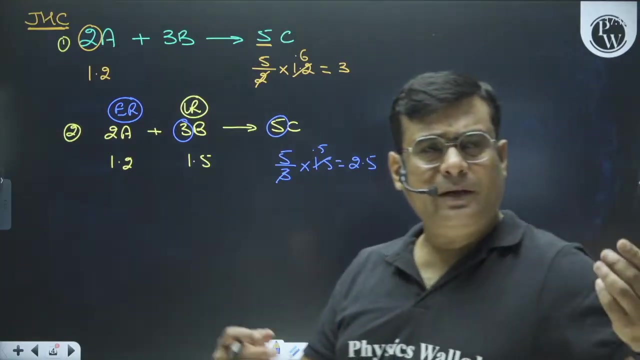 What will be A, My dear children, excess resident. And if now the question would have been that: tell us how much excess resident is left. Tell us how much excess resident is left, Then you will be able to speed up. Sachin will be on his own. 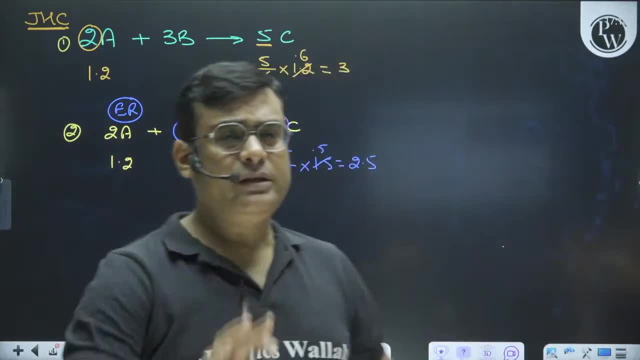 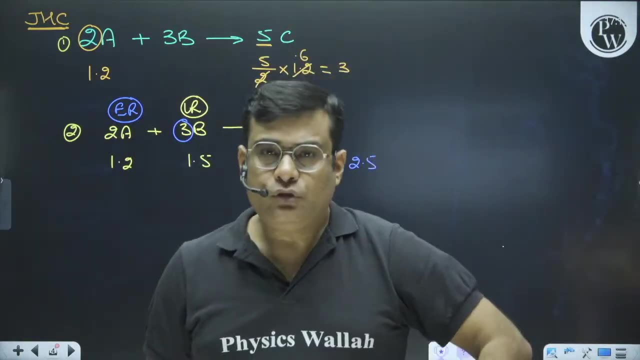 You can see that the chat is running. he will be on his own, Don't worry, Because in the beginning if I have to come to Delhi from Kota to attend some function, then when I will drive the car in the beginning it will run slowly for 10-15 minutes. 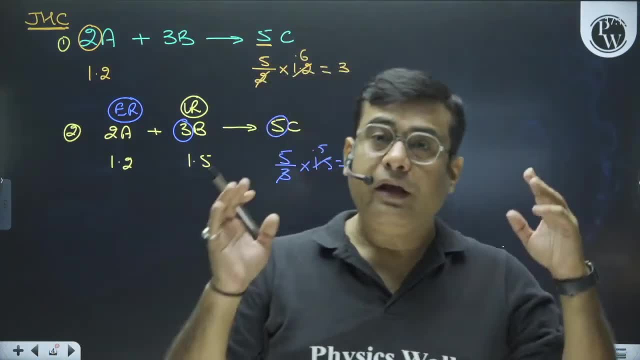 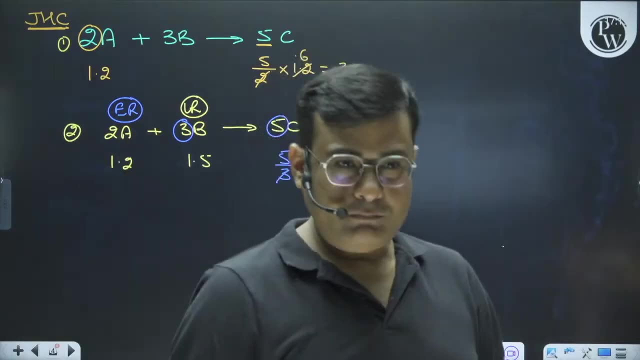 By default, the car runs on its own. I don't know why. This is a real-life fact. No one can escape this world. After that, it automatically becomes a rocket. It automatically becomes a rocket, So don't worry about it at all. 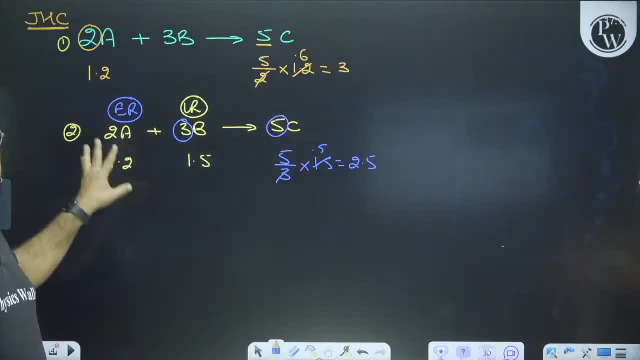 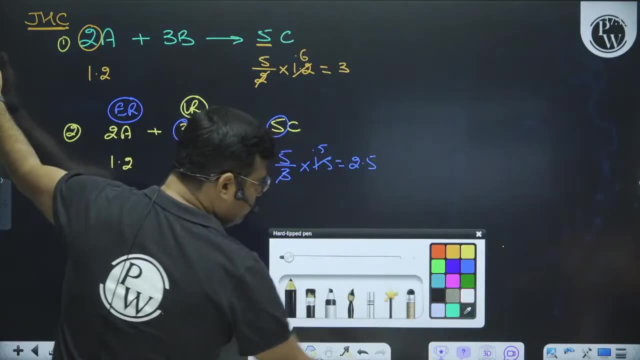 So what am I saying to you? If you ask me about excess resident, If you ask me how much excess resident is left, Then what will be your approach? Then your approach will be: my dear children. I am going to write two steps. 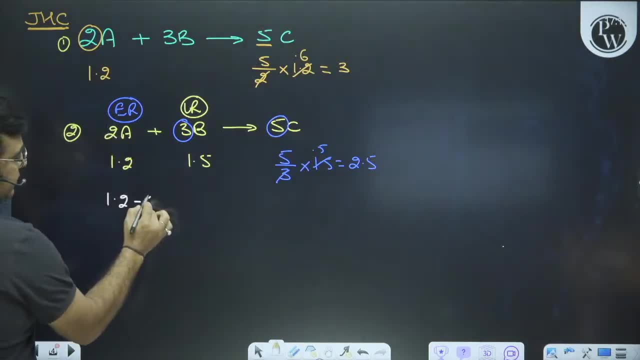 That is 1.2, which is given moles. If the coefficient of minus A is 2, then 2x, Then 1.5 minus 3x, which is the coefficient of B, And here your 5x. So keep these three concepts in mind. 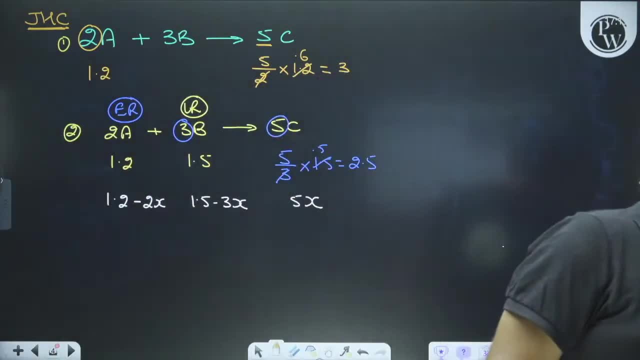 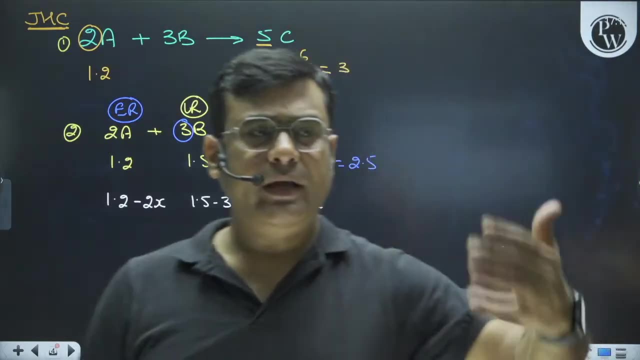 Because definitely each of you, children, Even if you don't see the direct question of the mole concept, But in chemical equilibrium, in chemical kinetics, You will have to use it somewhere. anyhow, You will have to Be sure to keep this in mind. 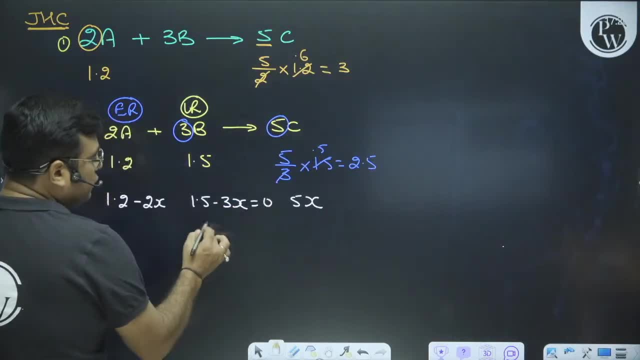 Now, because there is an imitating resident. So make it zero. If you do zero, then the value of x is 0.5.. Here you see if you do 5x.5.. So if you ask you, the moles of C. 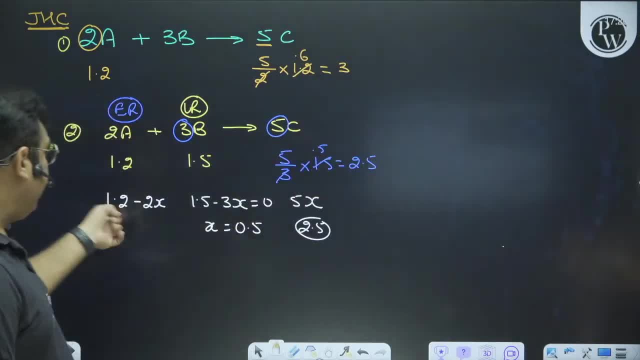 If you ask only the moles of C, Then the answer had come directly. But now he has also said how much excess resident is left. So what is minus 1.2 children 2x.5.. Now we will do all the calculations. 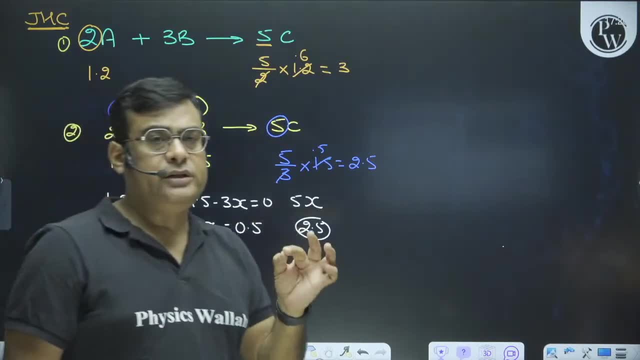 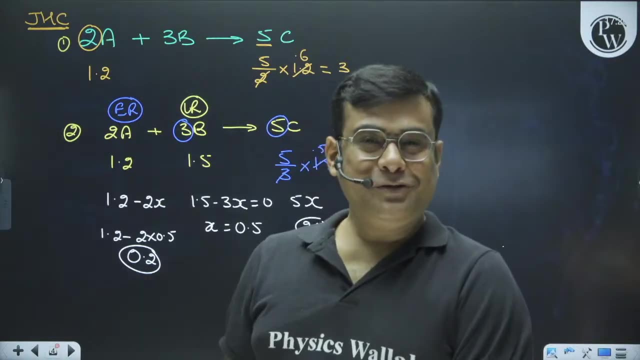 The answer has been 0.2.. So, please, these three small things. The king of my beauty is the love of my wife, The love of my dear children, like you, The love you keep doing, The pain you keep doing in my heart. 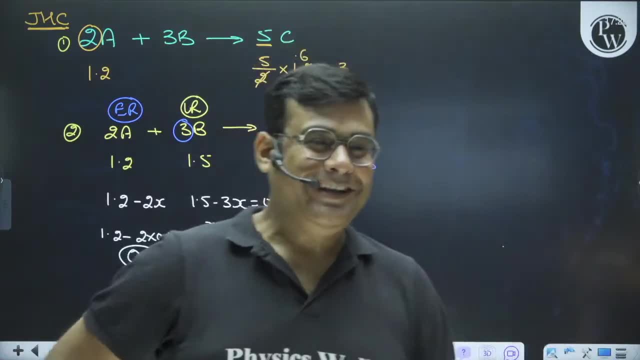 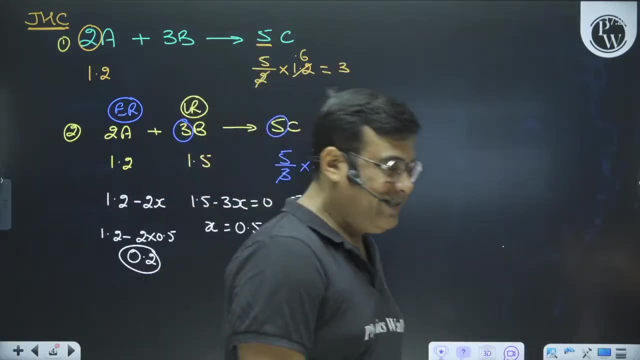 That is love. Because of this, the beauty of the face is increasing, Although the face is getting old. That is a separate thing, But the beauty of the face is increasing. So tell me, tell me, tell me: Do you understand these three concepts now? 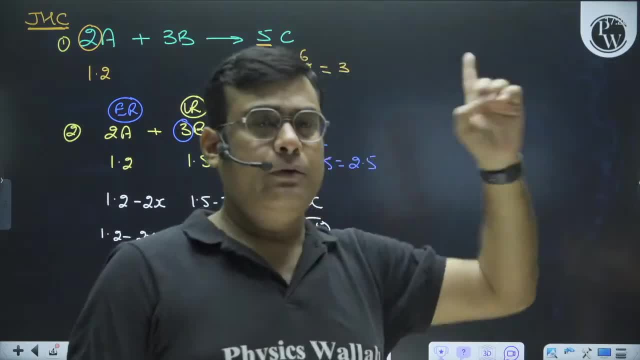 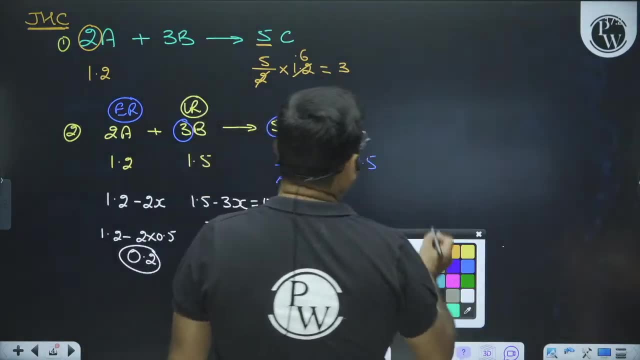 And it felt a little different. No one knows, I'm sure I'm saying that the heart will keep looking. We are in between. Let's go Now. what else do you do apart from this, children? Let me tell you one or two more formulas. 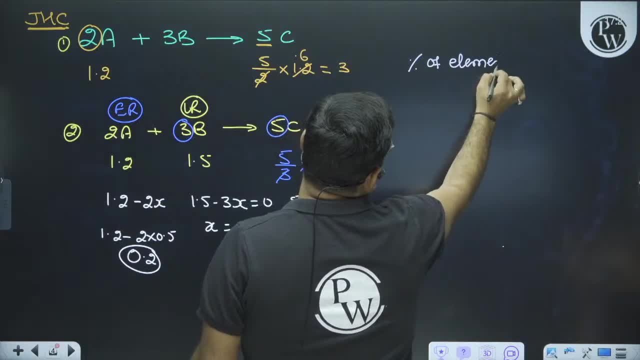 If a percent of any element is asked, And then we are coming to the questions. So the formula of percent of element is straight: Weight of element above, Weight of compound below, Or its molar mass Into 100.. Into what, my dear children? 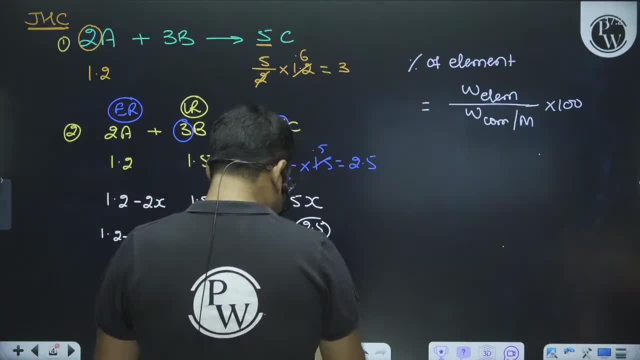 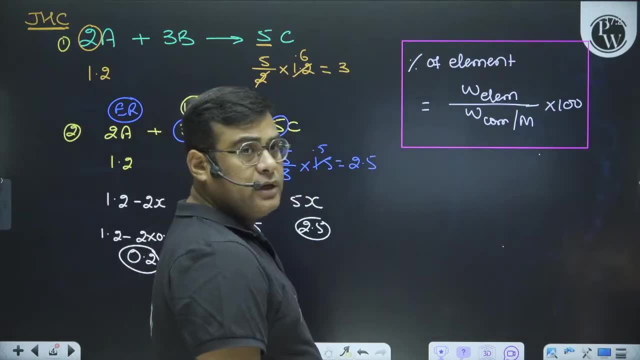 100.. One thing you also have to keep in mind. It is compulsory, Right At this time, just at this point, These small, small formulas, Be sure to keep in mind. Apart from this, sir, What other formula? 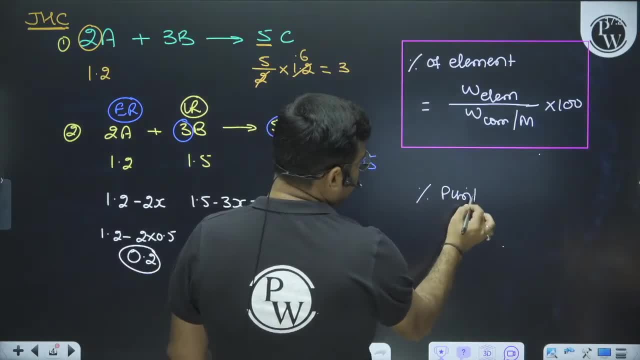 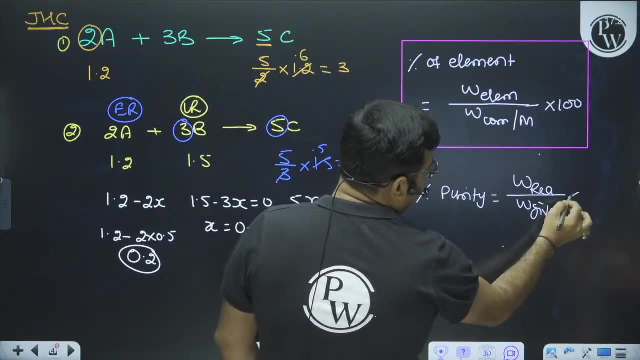 Suppose. sometimes he talks about percent purity In some question. So the formula of percent purity is Weight reacted Upon Weight given Into 100.. Sometimes, children, he talks to you about percent purity, So percent purity Is. 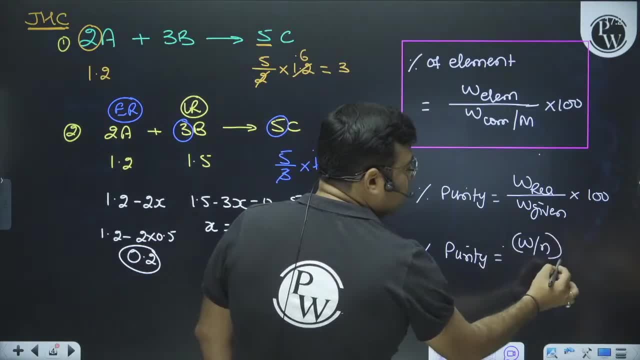 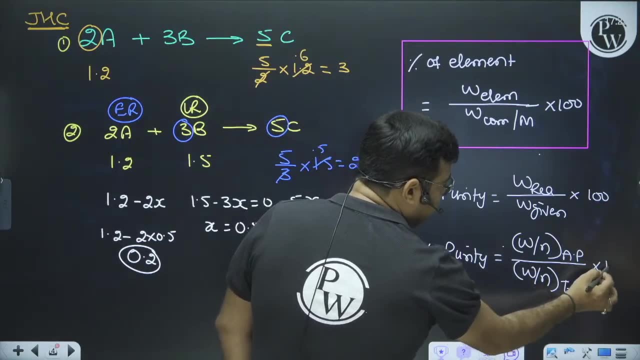 Weight Oblique Moles, Which are actually produced, Divided by Weight Oblique Moles Which are theoretically produced, Into 100.. Sir, now what is the meaning of actually produced and theoretically produced? Right, Actually? 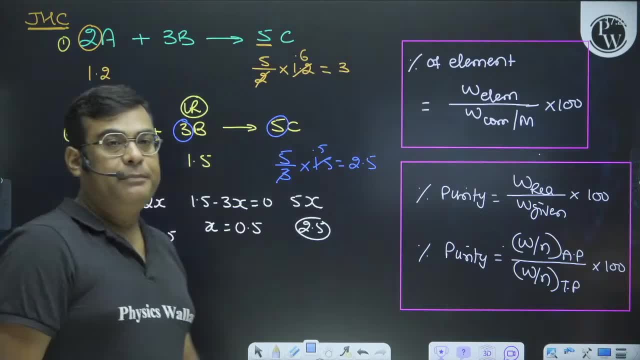 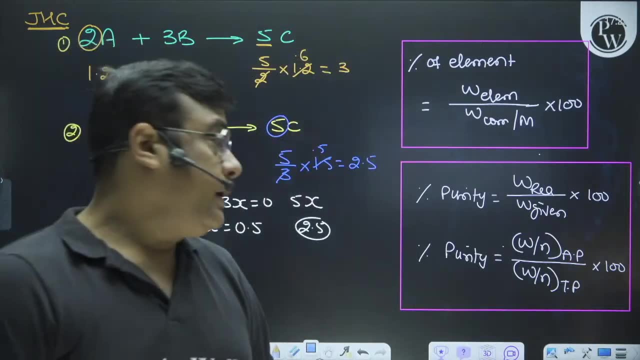 Theoretically produced Means, what you have taken out, Because here you consider the yield to be 100%, My dear children, Here you consider the yield to be 100%. Okay, But if the yield is 100%, Like these 2.5 moles, 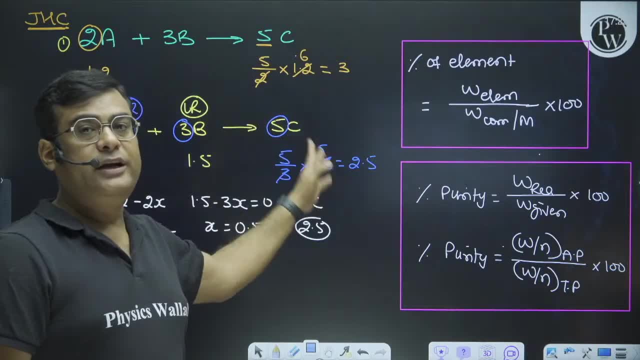 They will be when the yield is 100%. If I had said in the same question that the yield of this reaction is 80%, Then tell me how many moles of C will be made. So it is not that our concept of the mole will change at that time. 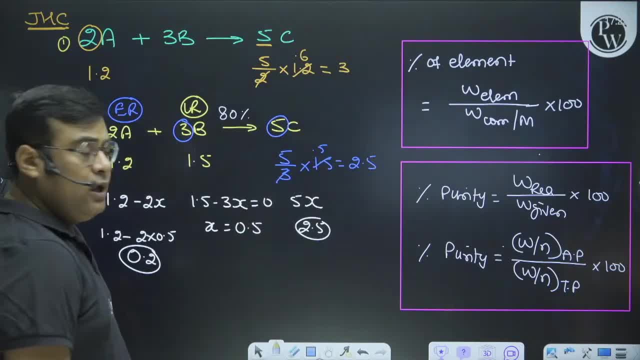 You just get 80% of 2.5 at the end, And I hope every child. Any number of 80% to be taken out: Multiply by 80.. Divide by 100.. Right, My daughter is also 70.. 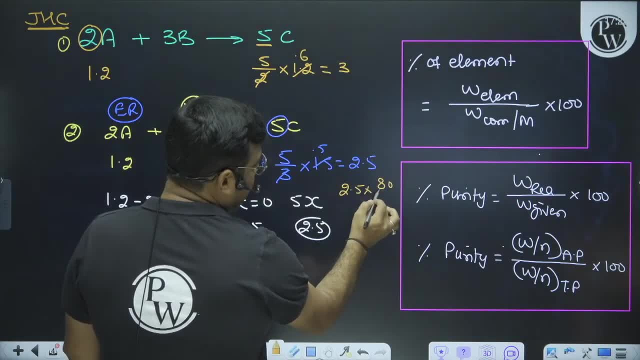 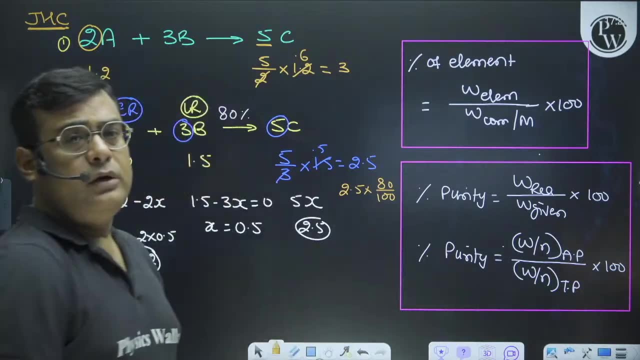 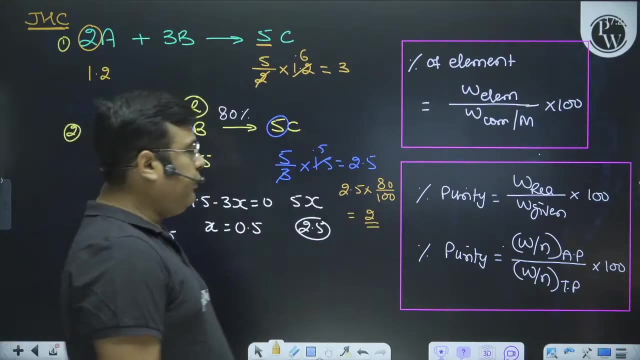 She does such a small thing, Then the answer will be 2.. Okay, People are defined by percentage purity with respect to reactants And percent. Sorry, Why have I written purity again Here too? This was percent yield And the percentage yield is. 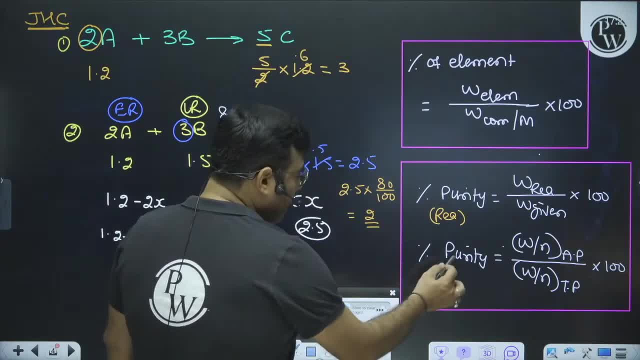 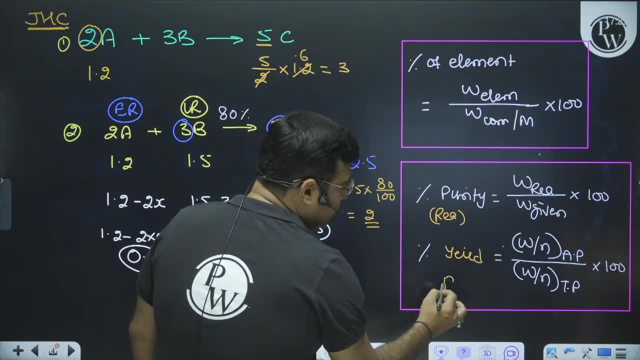 If there is any reaction at the second time Will see in the next video. Please stay tuned Your Standby. See you later. Bye, Hi percent yield, which is defined with respect to whose product. ok, and from now on, I am giving. 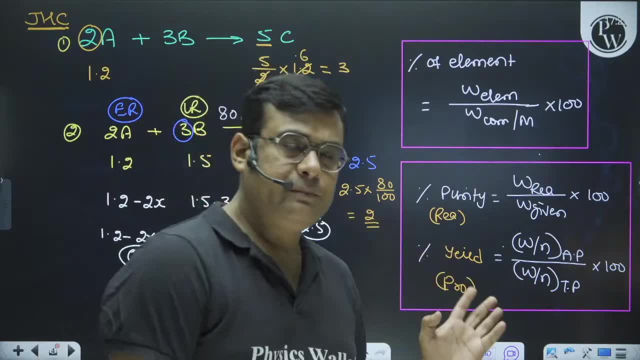 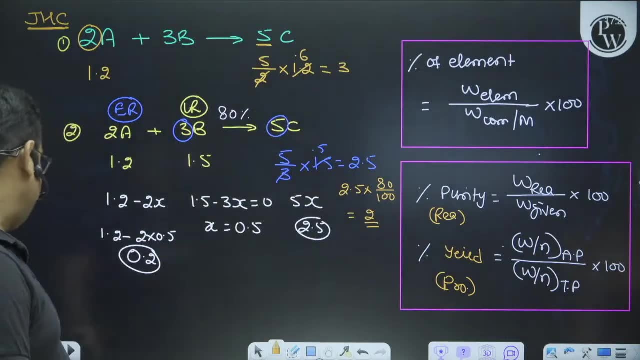 you a liquid guarantee, son. you also know that the things we are doing, definitely you will get questions on them. so guaranteed you will get questions on these things on it. apart from this, I will also tell you one more of my blessings: son jayi means in 2024 also. 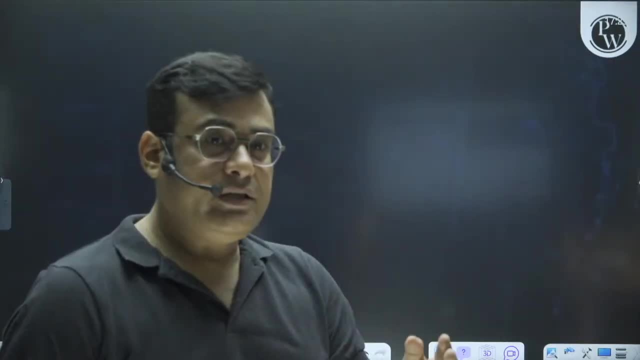 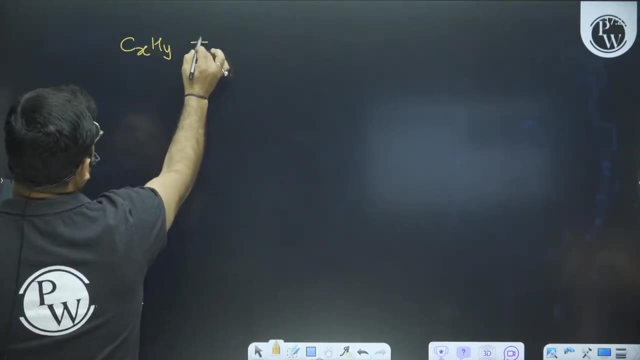 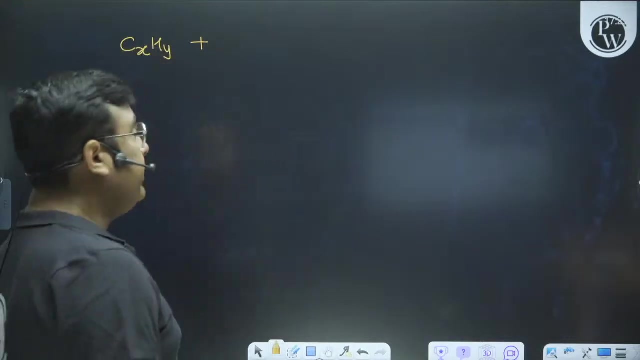 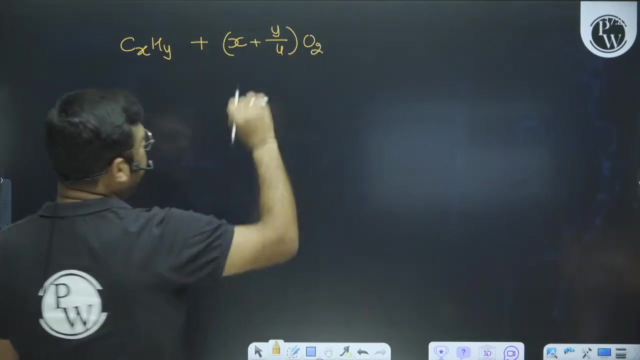 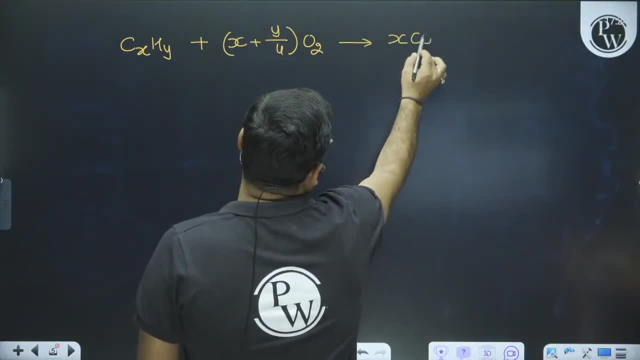 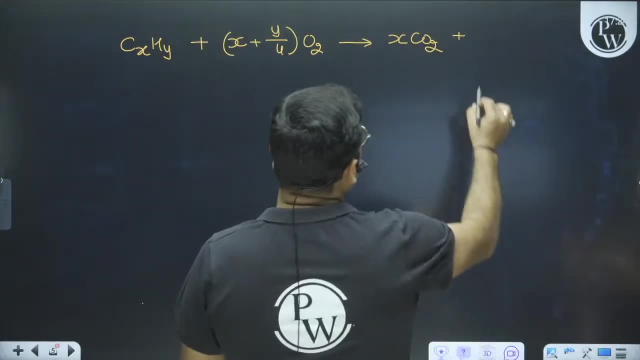 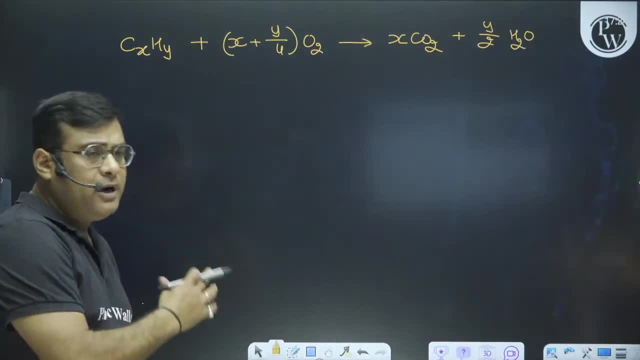 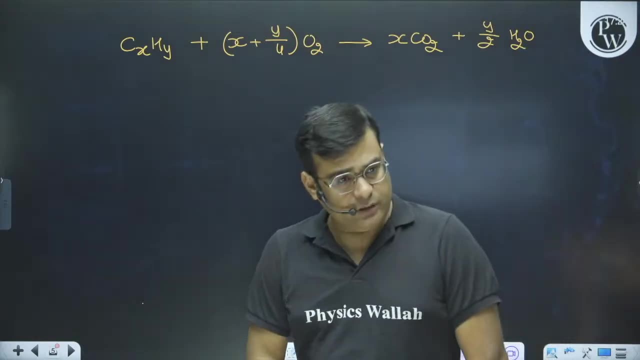 is the equation of Ramban children again and again, question management. for the first attempt of the marathon I had taken even then, I shouted and shouted and told the children: ok, I had taken the session on the 26th of January. the question came on it in the paper on the 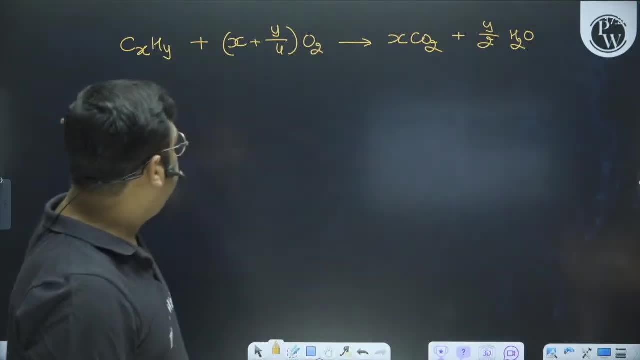 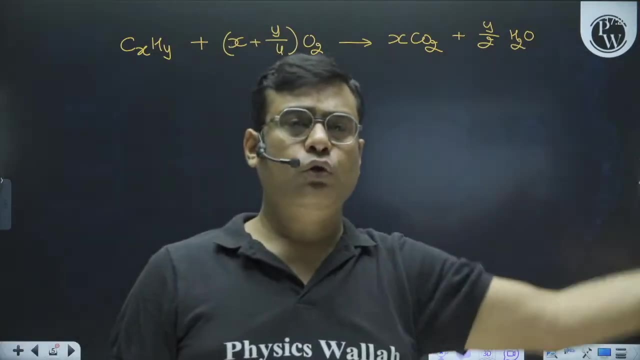 27th of January. So this is a small thing. keep in mind that we have written with respect to one mole. right, we have written this with respect to one mole. now there are two moles, there are three moles. sometimes, what does the smart one do to us? he will tell us that you have. 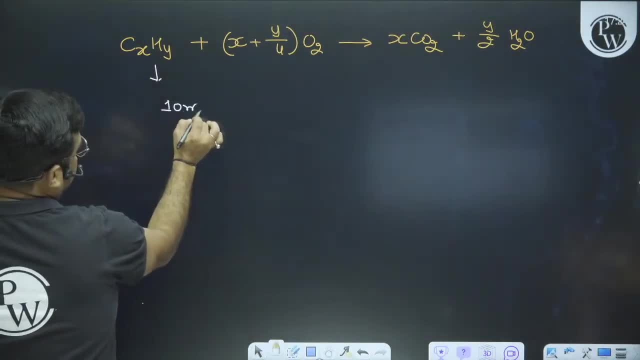 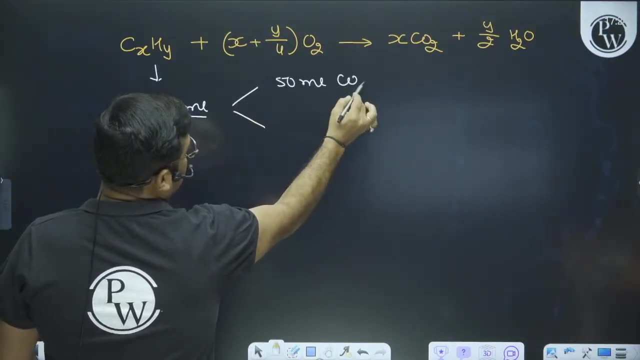 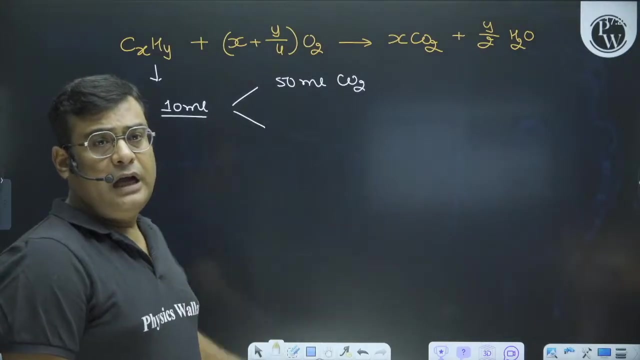 some hydrocarbon. it has 10 ml. its 10 ml on complete combustion is giving you 50 ml of co2,. ok, tell me how much carbon will be in hydrocarbon. so, brother, we have written it with respect to 1, now there are 50 for 10, so obviously there will be 5 for 1, then. 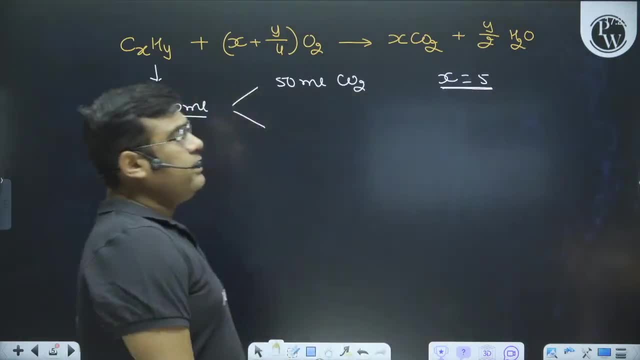 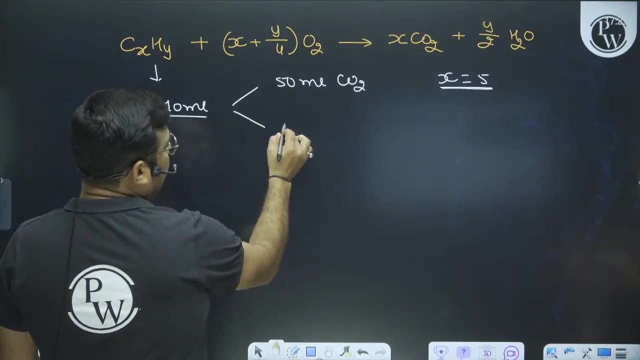 the value of x for you will be 5, there will be 50 for 10, then the value of x for you will be 5, and he is telling you that. he is telling you that he is giving you 40 ml of co2, now. 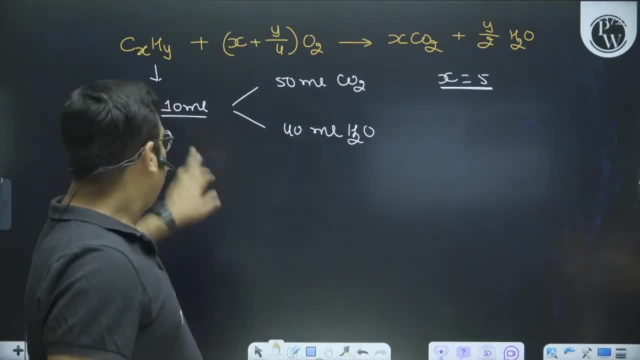 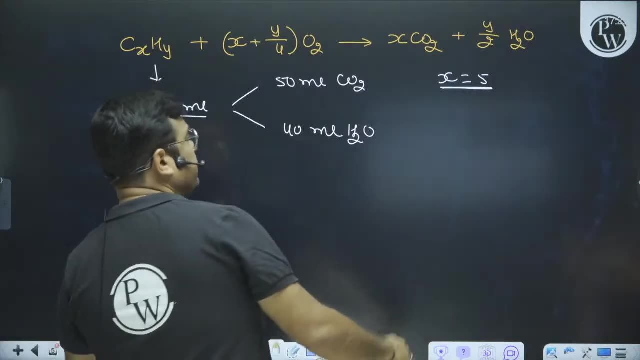 he is telling you the whole formula of hydrocarbon. so brother is giving 10 ml. 40 ml means how much will you give 1 ml? how much will you give 1 ml children? how much will you give 1 ml? we will give you. 4 means the value of y by 2.. 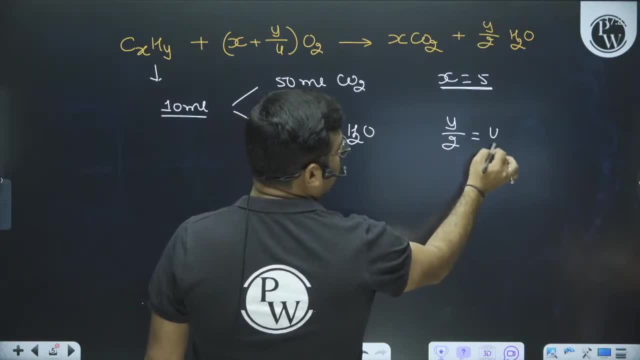 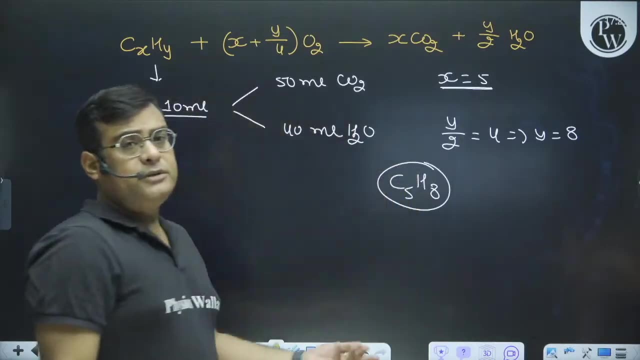 Ok, The value of y by 2 is 4, that means the value of y is 8, then the formula of your hydrocarbon is C5H8,. or ask us so much, brother that, how many ml of oxygen will you take for complete? 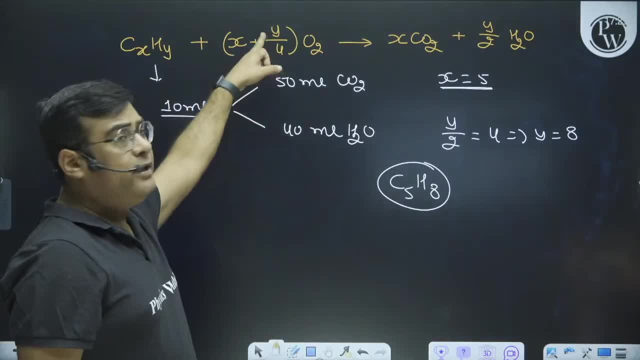 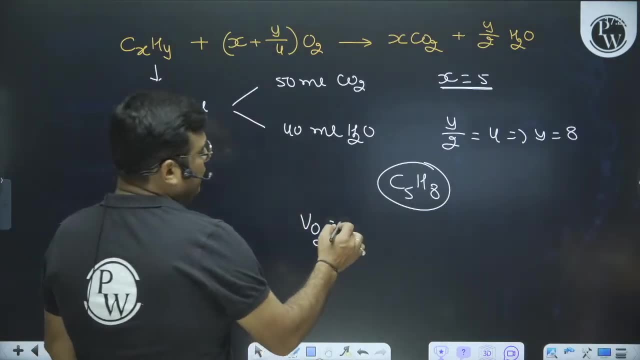 combustion. then you know, x is 5, y is 8,, 8 by 4 is 2, then 5 plus 2 we will say the volume of oxygen required which will be for complete combustion. how much will it be for 1 ml? 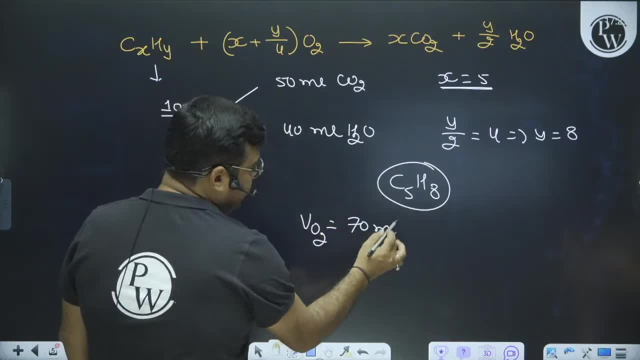 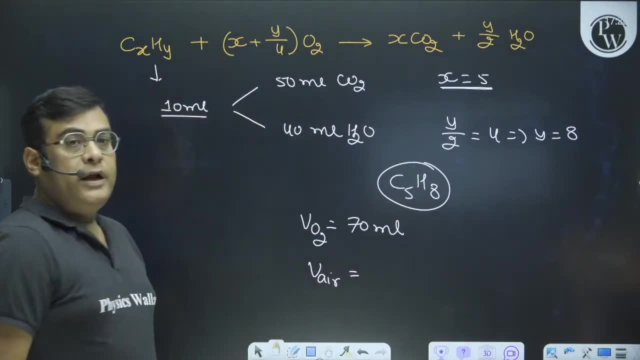 for 1 ml 7, then for total 10 ml 78.. Ok, Or do something more clever. do something more clever. tell you to tell the volume of air. right, we know that there is 20% oxygen in the air. remaining 80% nitrogen is there. 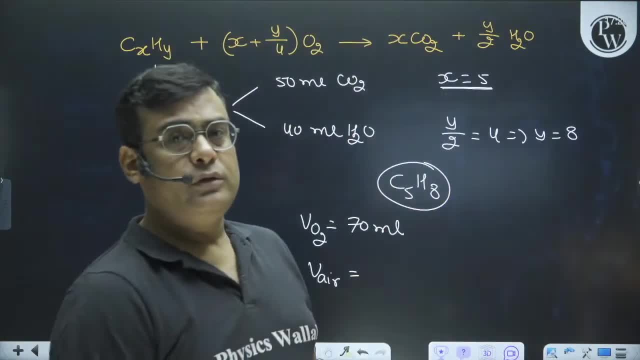 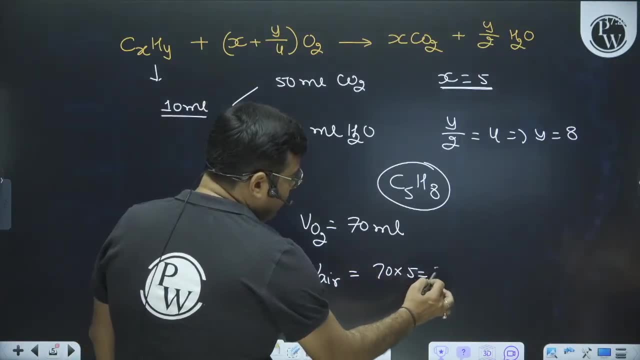 so if you look at the volume of oxygen and ask the volume of air, then its 5 times 70 into 5 means the air will take 350 ml. So this type of question is the packed question of JEE children. this 7 was written, I know. 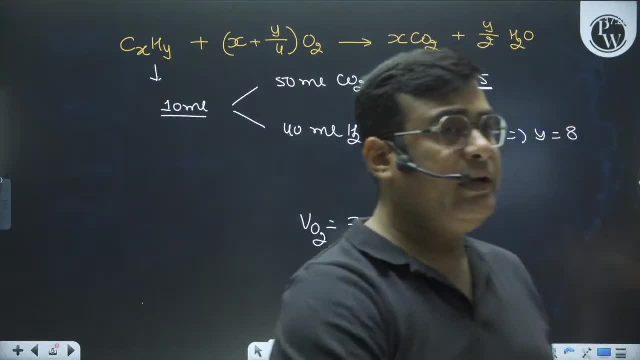 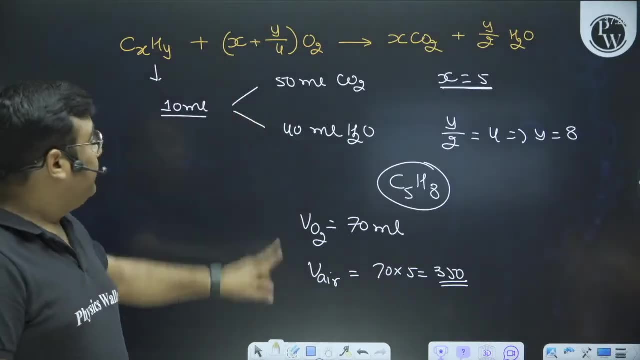 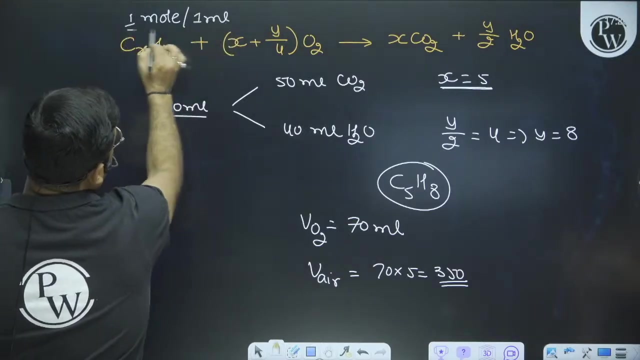 that you will make a mistake in the hurry. son, how many ml of oxygen will you take? many children have written 7,. 7 is for children. 1 ml has happened because this reaction has been written with respect to 1 mole or 1 ml. this reaction has been written with respect. 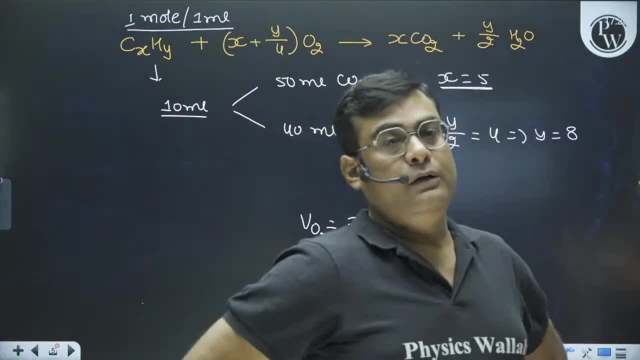 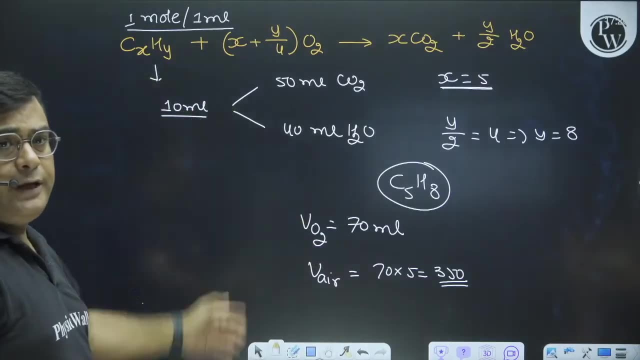 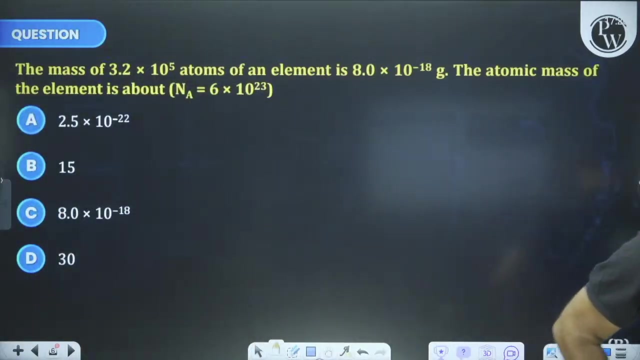 to 1 mole or 1 ml. so here a little bit of problem can happen. you have to save yourself from this. ok, then the mold concept, crispy concept. ok, I have told you. come, now we Let's move on to the next chapter, so that you get a rough idea of what can be asked of us in the main concept. 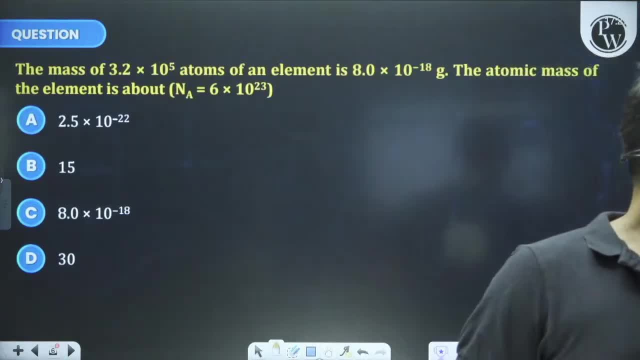 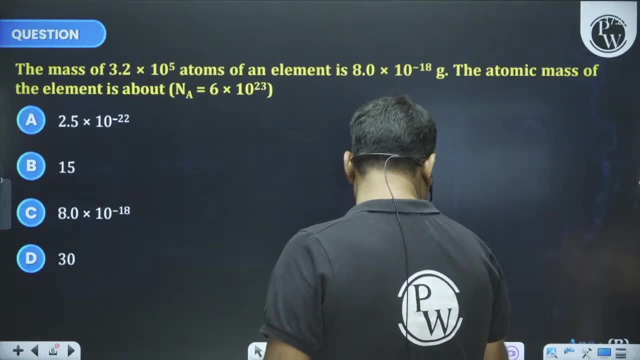 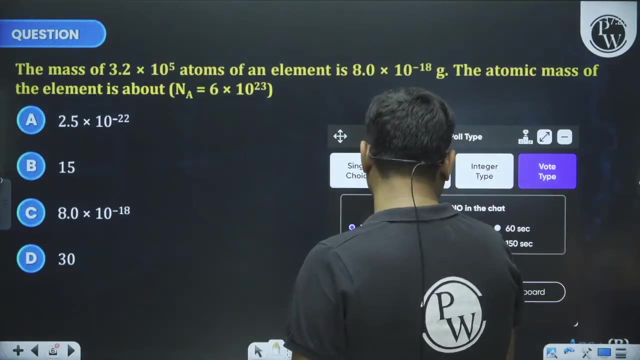 First of all, let's solve a small question: Where does this pole wall come from? Has everything changed? What type of pole? 30 seconds, Tell me quickly. Did you understand all these things? Did you get rid of any confusion? 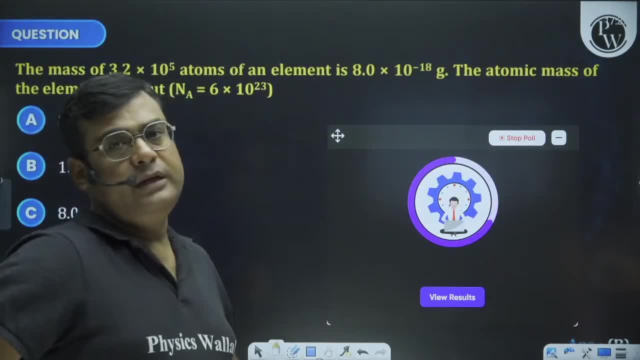 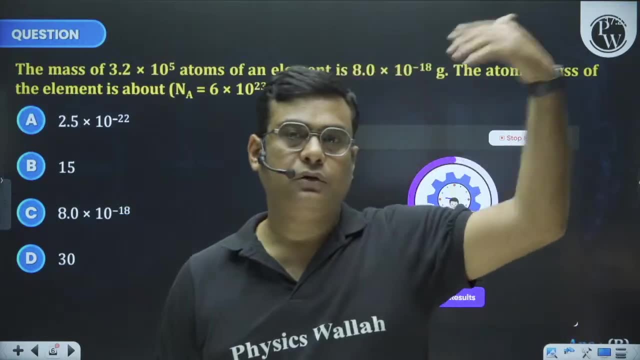 How did 350 happen? 350 happened in such a way that the oxygen was 70.. He has asked about the air. The oxygen in the air is 20%. If the air was 100, then the oxygen would be 20.. 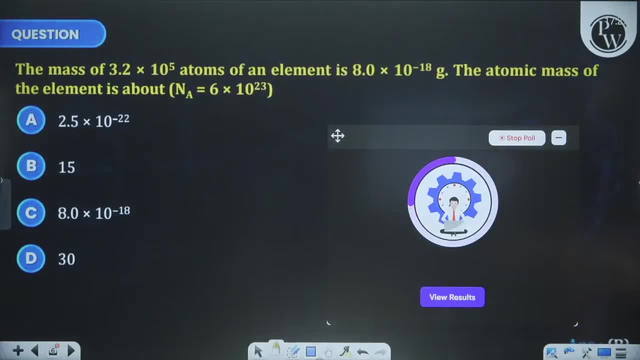 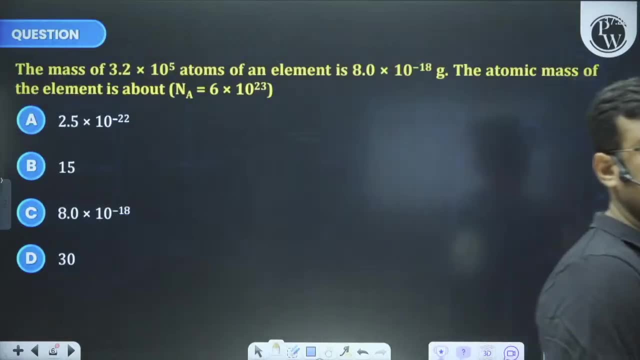 Isn't it? If the air was 100, then the oxygen would be 20.. So if the oxygen is 70, then the air should be 350.. A small poll is my information For all the questions. the poll is not possible because it will take a lot of time. 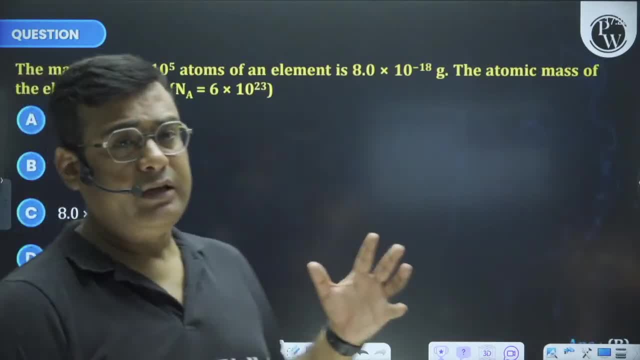 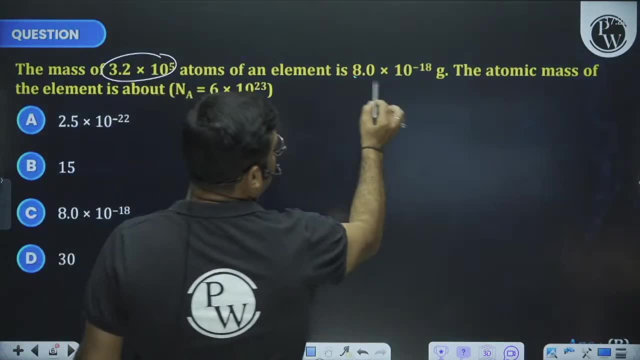 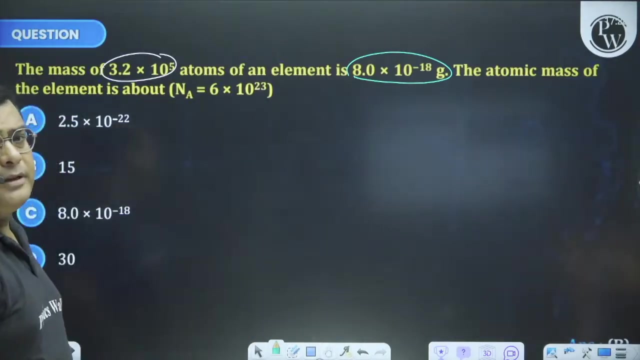 And your time is very valuable. So what is there in this? So much weight of atoms has been given to you. So tell me: how much is the atomic mass of the element? There is no problem When the atomic mass has to be taken out. how much has to be taken out? 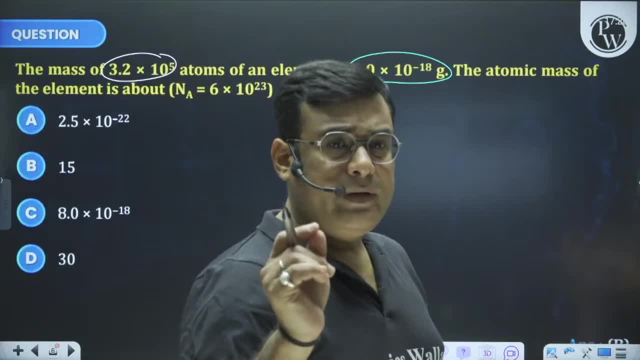 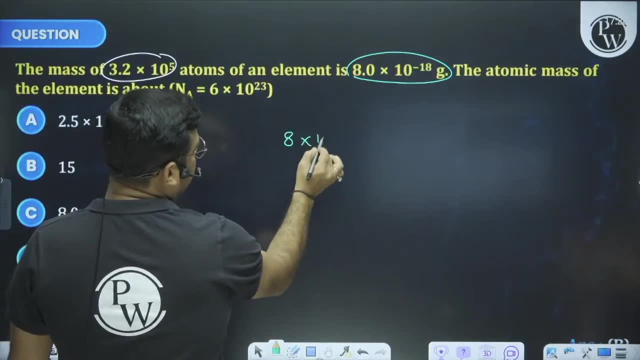 6 into 10, to the power 23.. So now I told you, HDFC Irwani has developed fast calculation. Try to do the calculation a little faster. If this much of an atom is this much, then how much of an atom? 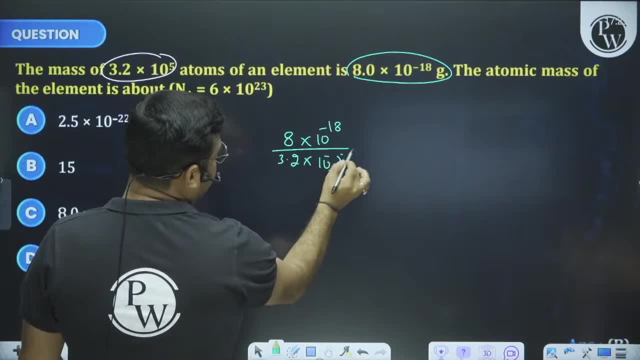 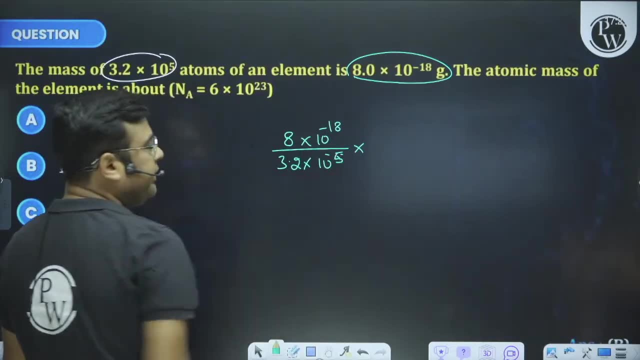 Sir, divide it. I will just request you to do this step a little faster: 3.2 into 10, to the power of minus 5.. Sir, this is of one atom, And how much do you have to take out? 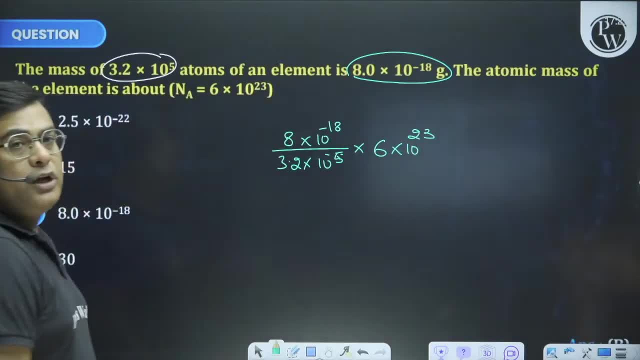 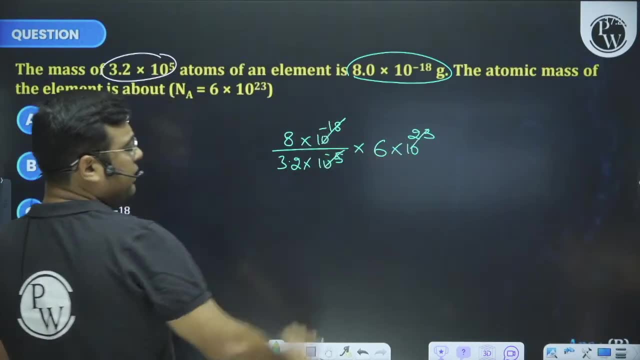 3.2 into 10, to the power of minus 5.. Sir, this is of one atom. Sir, the mass of one atom is called the atomic mass. You will have to save the calculation. See, this is the power of 10.. 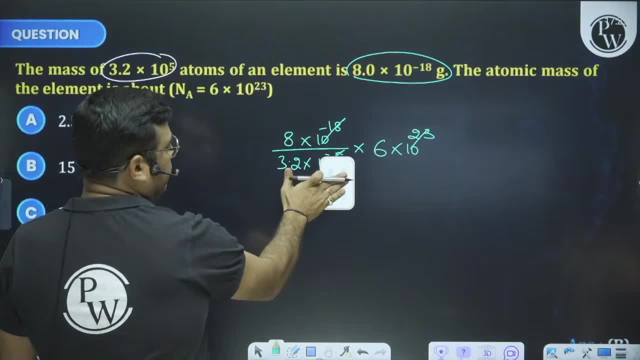 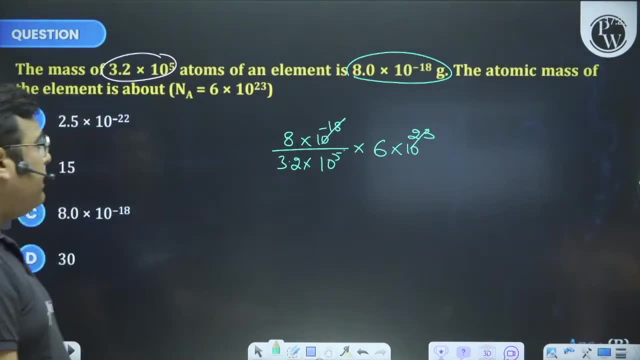 What happened? Minus 5.. What is the power of 10? Minus 18.. Sorry, there was 5 below, So I have put a minus here. So all three of these things are cancelled. Now, if you do not want to do the full calculation, HDFC means children. 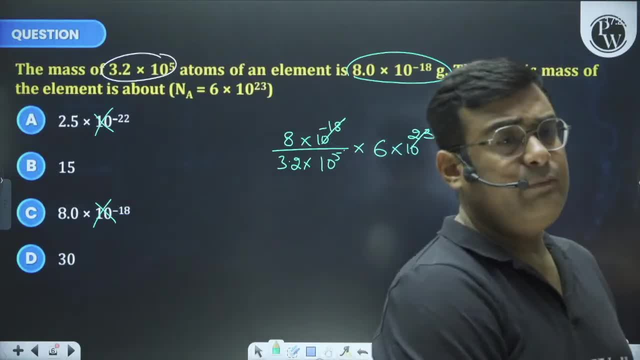 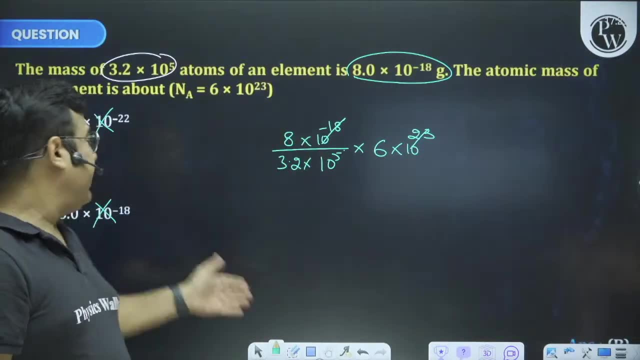 you have to keep saving the calculation. I do not solve all the questions. when I have A, B, C, D options available, this is cut. these two options are not saved. now I am seeing 6 by 3, if the children were 2, then 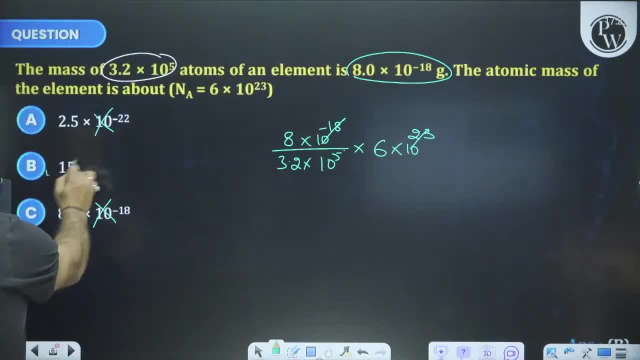 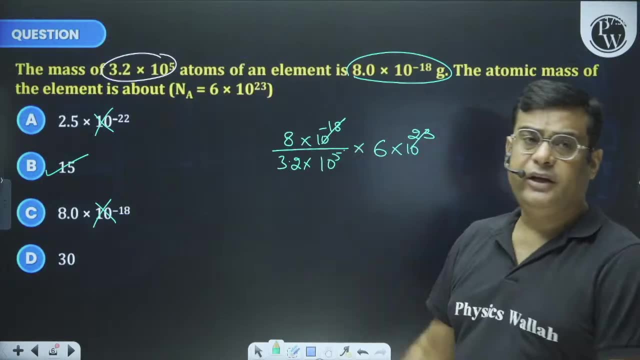 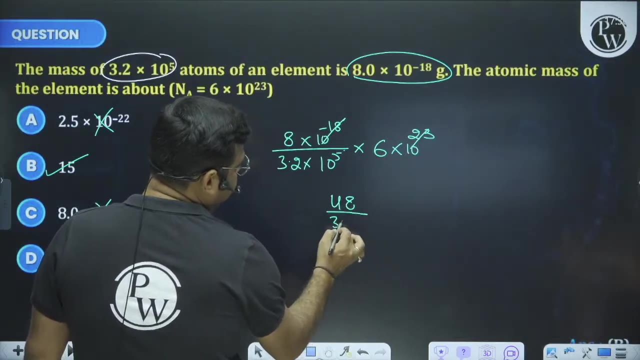 8,, 2 or 16 means my answer can only be 15,. now tell me honestly, what will the maximum children have done? this will also be solved: 8,, 6 or 48, although the calculation is not correct. I am also saying 8,, 6 or 48, and then 3.2,. then I removed the decimal I put. 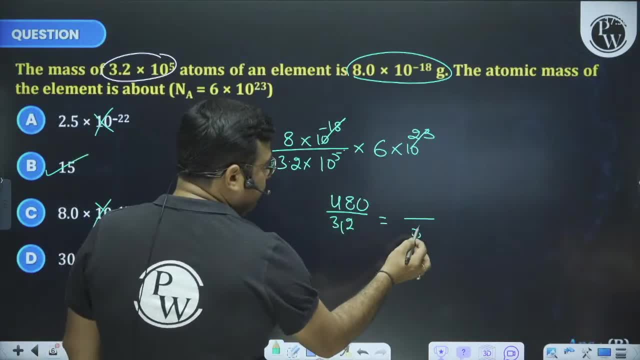 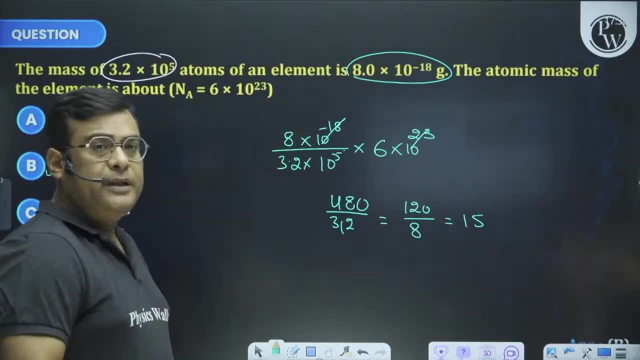 0,, sir, we divided it from 4,, 4,, 8 or 32, there, sir, 120,. then, sir, we divided it from 8, then it came to 15,. now tell me honestly, how many children did all this? tell me honestly, quickly. 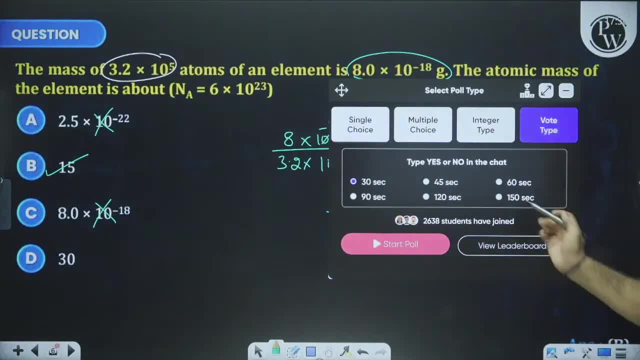 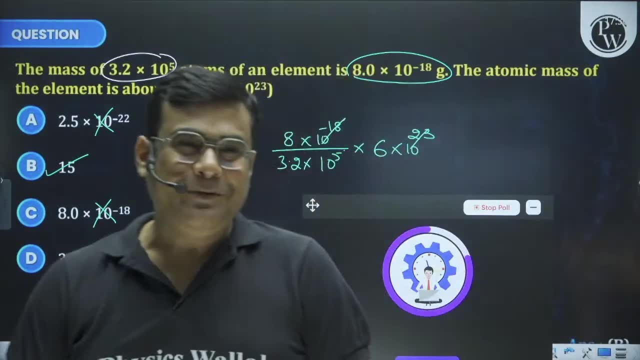 how many children come on. you will not tell me, honestly. how will you know the heart is with you? those are different things. you have given me the heart. now write it down. write it down, but I can't take it out and see it, okay. so I want to ask a small, small. 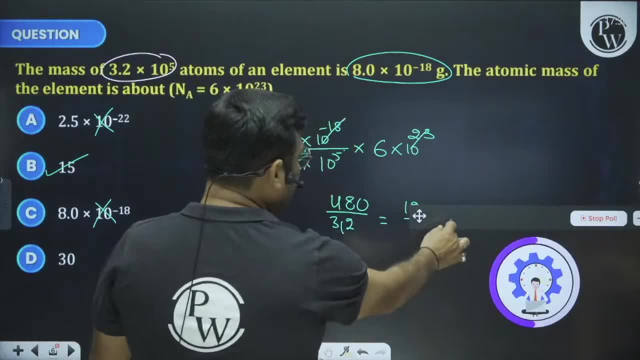 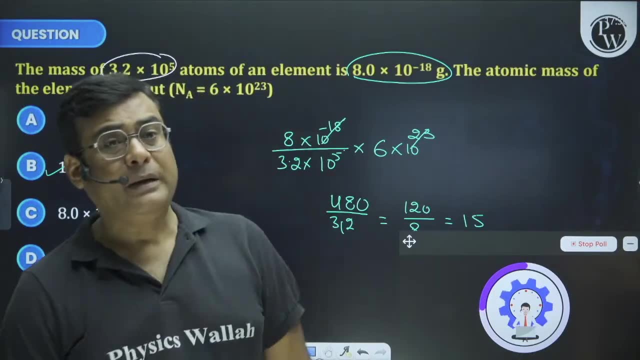 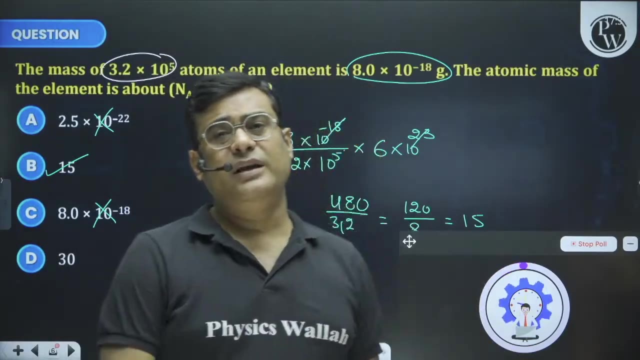 poll how many children have written it in the end, the whole one must have written like children. this speed should now increase in your questions. that is my whole purpose and I have given you the logic that now the next four turns your eleventh. physics twelfth. 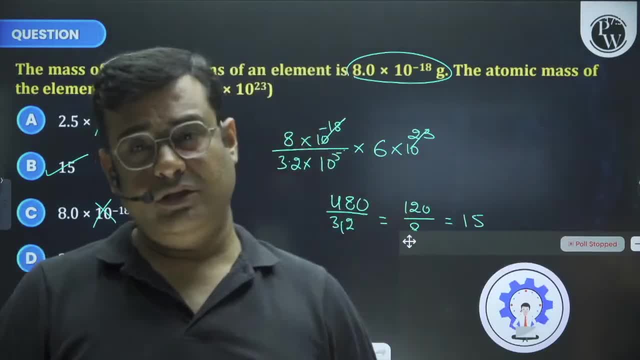 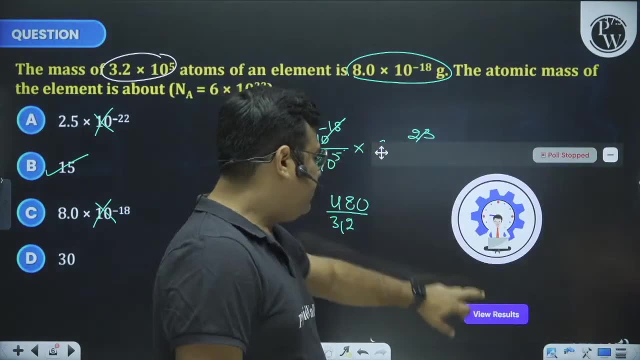 physics: okay. eleventh maths. twelfth maths. now there is a numerical question in them. right, There are less questions. there is a style to solve it in a different way. so please, little by little, children, you are in calculation from this session, so tell me, okay many. 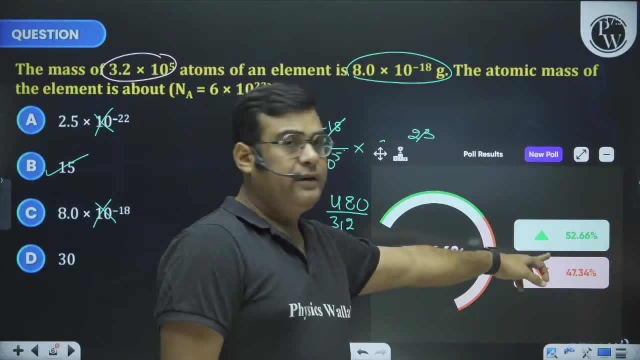 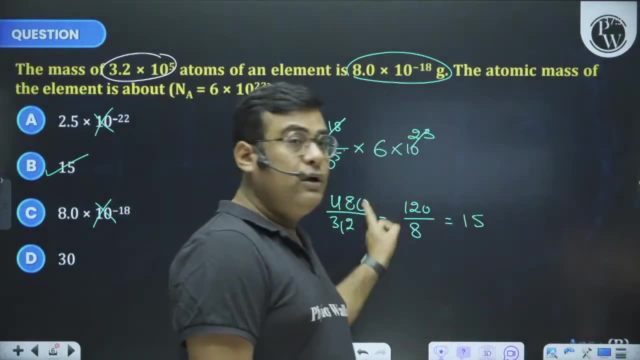 children have not done it. this is a matter of joy, but still more than fifty percent have done it in this way. so now those who are about fifty-three percent, they understand these things. and this is not my first trick, son. I will show you in every question, okay. 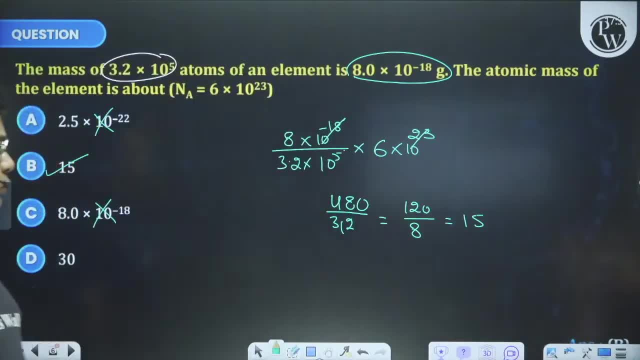 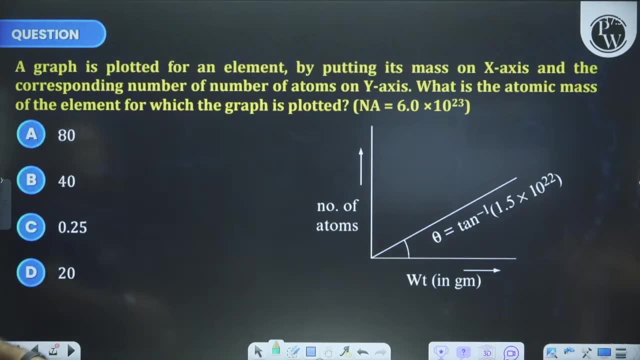 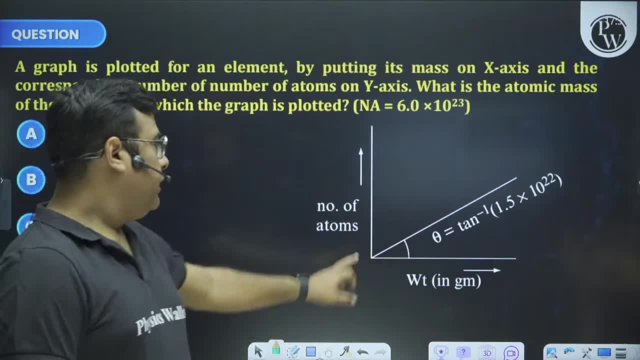 The graph is plotted for an element by putting its mass on X axis and the corresponding number of atoms on Y axis. Number of atoms: You have given the graph of weight. Okay, There is a slope given to you and the question is: what is the atomic mass, the element for? 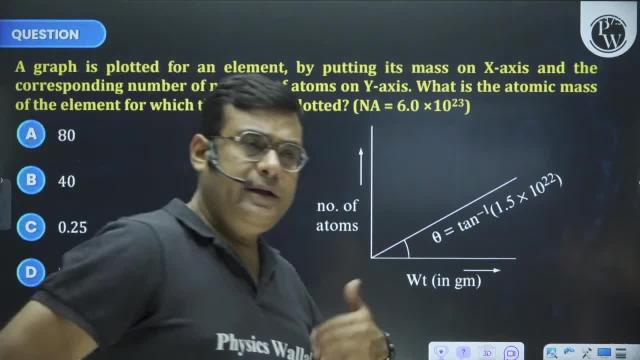 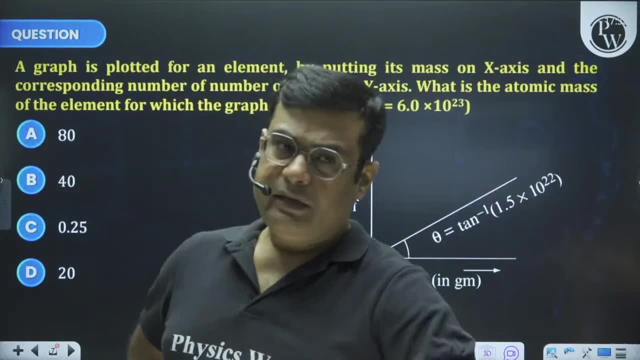 which the given graph is plotted Right. I have tried to take all kinds of questions, whether it is on the atomic mass or on the molecular mass. small, small, small questions are given on the single reactant, double reactant, percent purity. 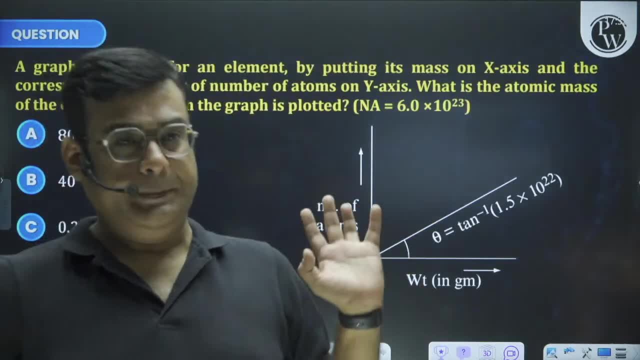 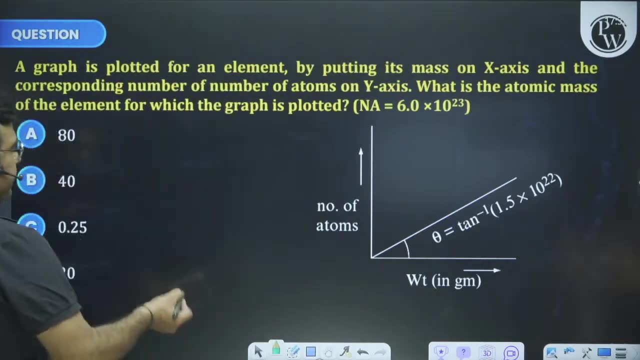 once you get a proper revision in the last time, then what do we have to do in this too? our chat is running, it's fun. what is the formula of the number of atoms if I denote it from n first? the given mass is not this number of atoms. the given mass will be divided by the atomic mass. 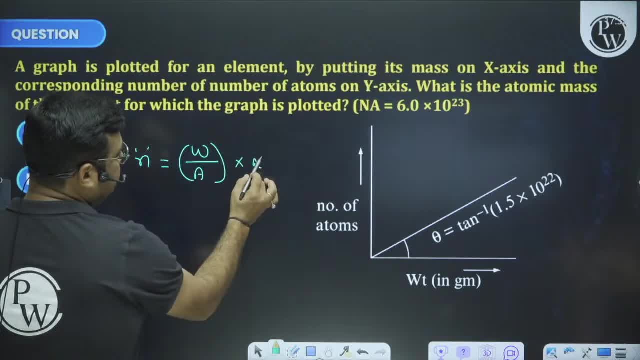 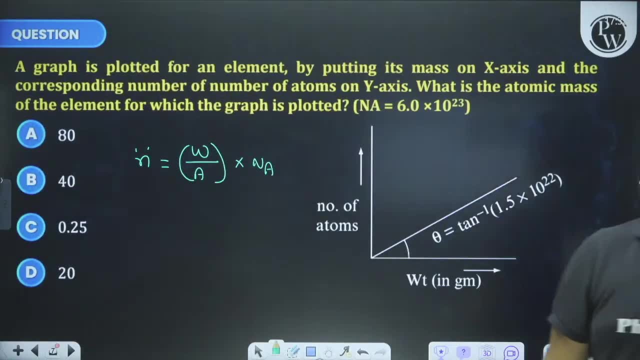 then these are the moles. and if I multiply it with n, sir, if I multiply it with n sir, then it will be the number of atoms. and now I have been given a graph between the number of atoms and weight in grams. 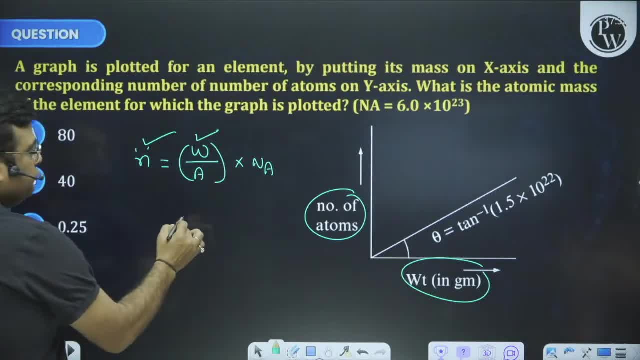 the number of atoms and weight in grams means whatever is left with me is its slope. then n a, that is 6 into 10 to the power of 23, divided by a equals to that slope given is 1.5 into 10 to the power of 22,. 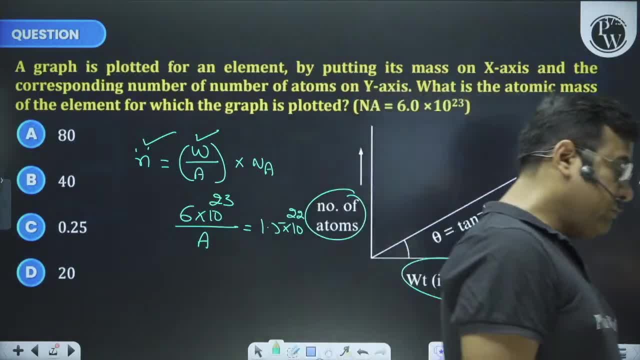 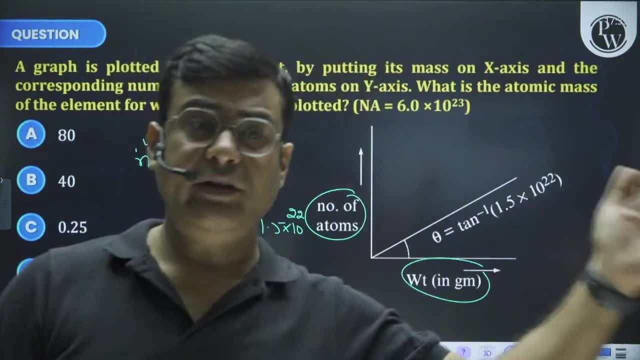 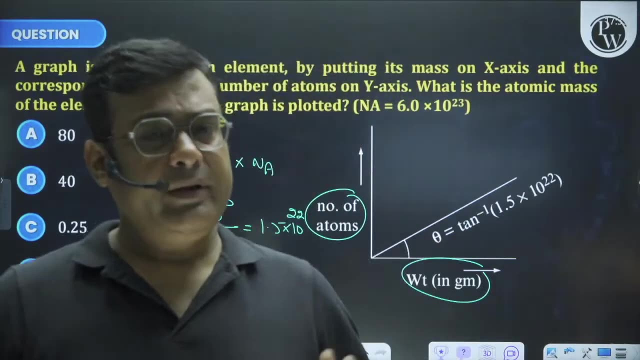 right, I hope from all of you. all of you have given the January attempt and you must have seen that very, very simple questions came from it. then the level of our questions is relatively up right, which is going to come ahead now. there are only two questions left. so, please, we will do these questions properly. it will be fun. 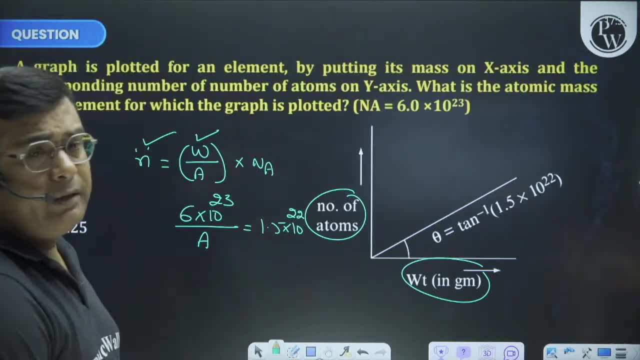 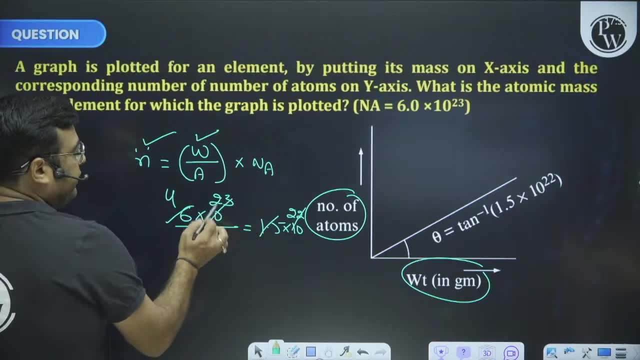 now I give advice to the children again and again: always focus on the power first. this is the power of 10,. my dear children, this is 4, and if you make it 22,, then 10 is left. the answer is 40, the story is over. 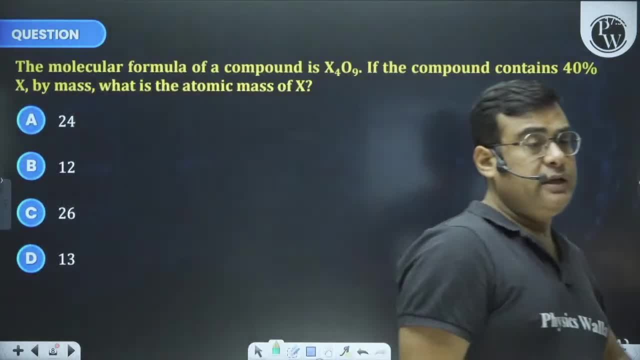 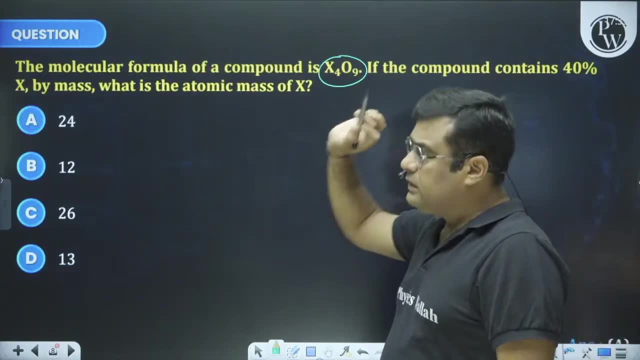 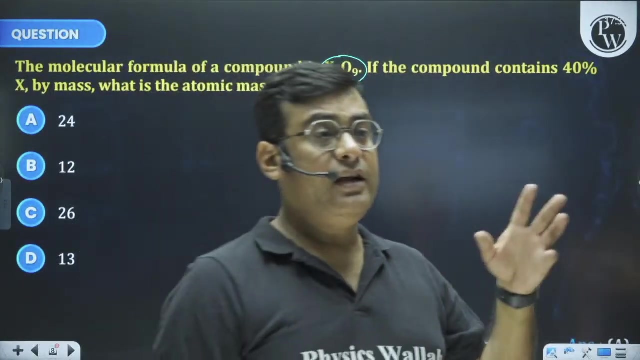 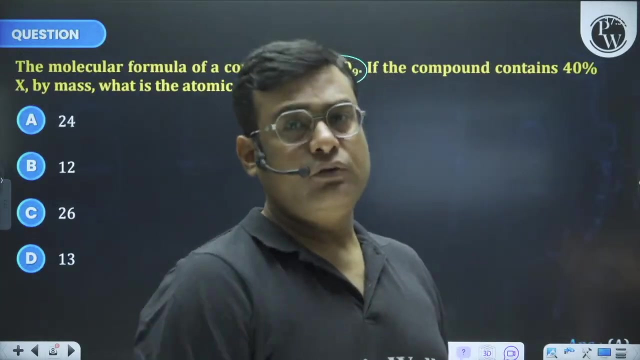 come on, let's go ahead, let's move on. what is the next question saying to us? right, the molecular formula of a compound is X409,. now, in the end of this session, you are at least right. you must have found a different way to solve 50 questions which maybe you have not yet paid attention to. you will have to solve them with the typical application. Okay, so for this question you are saying poll. please come, we will give you a poll. then let's start with the first. then if there are more questions, then I have to to leave the main part of the video until we come to the last. then I will give you two questions before moving on to the next. 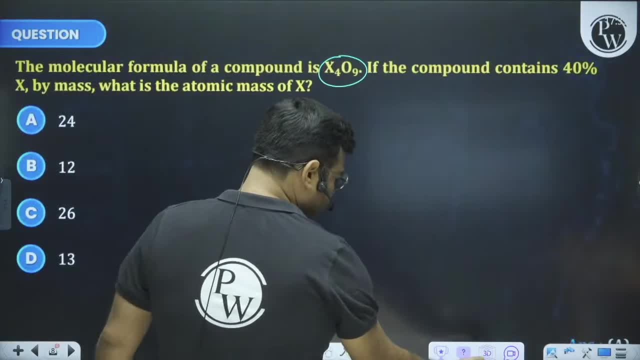 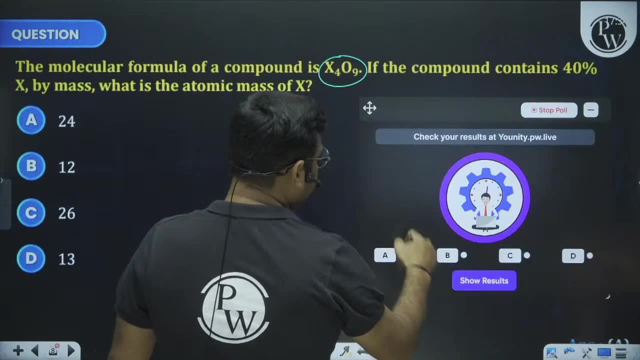 So for this question you are asking for a poll. Come, let's do a poll. Let's do a poll, Let's see the positions. Come for this question. I am giving you one minute. For this question. I am giving you one minute. 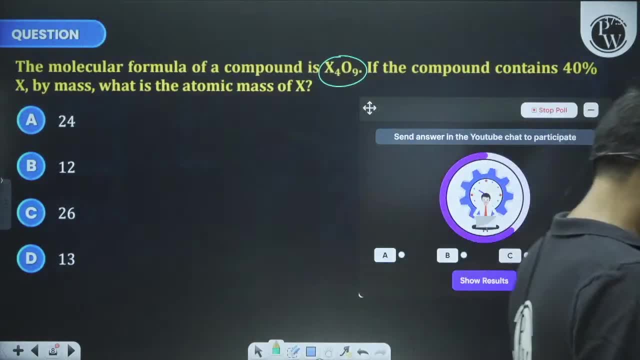 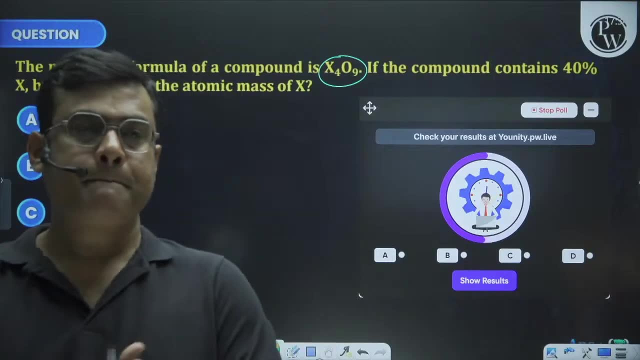 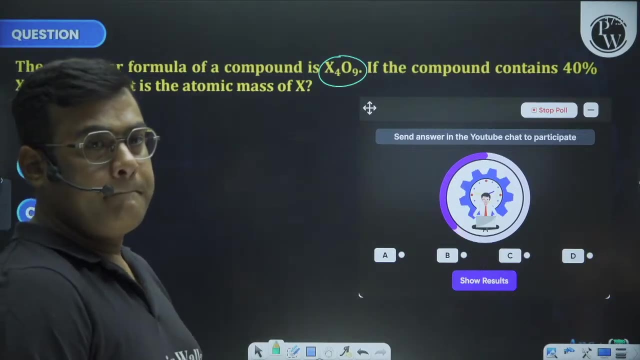 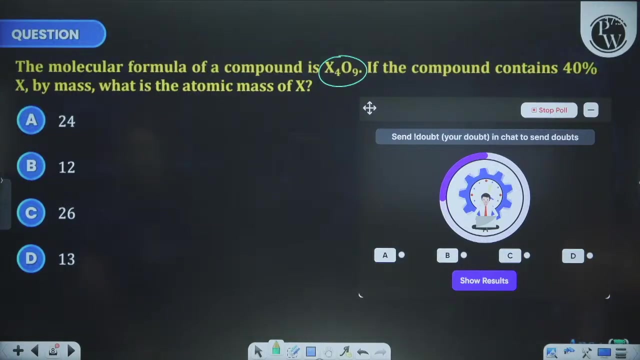 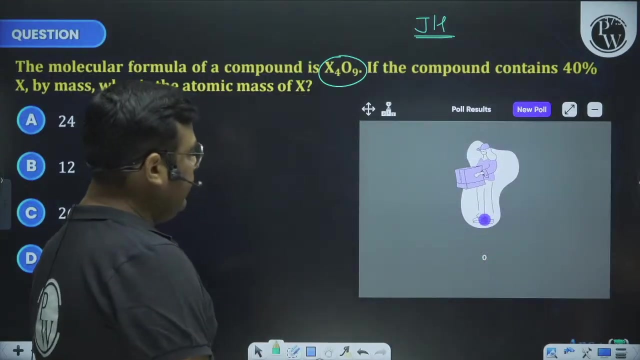 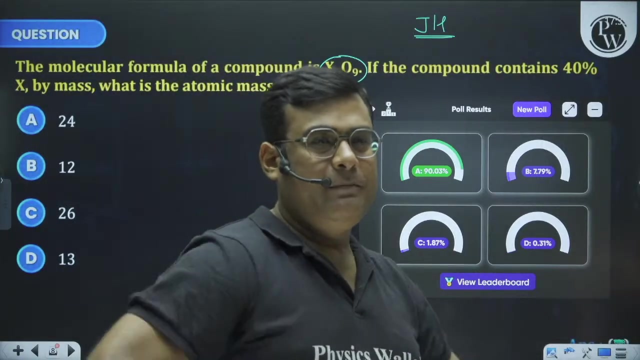 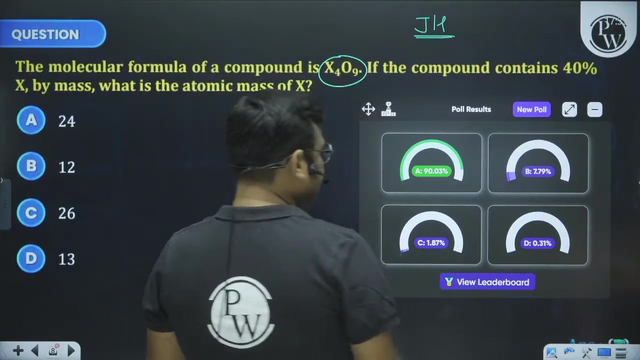 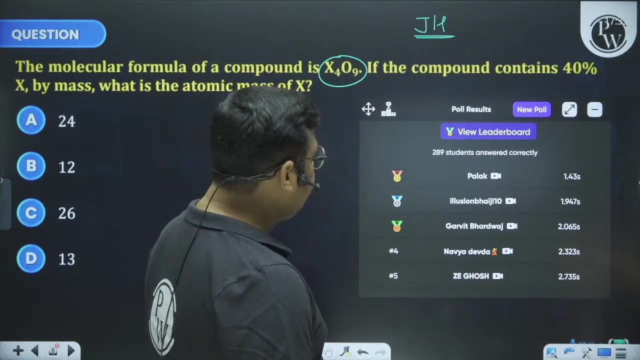 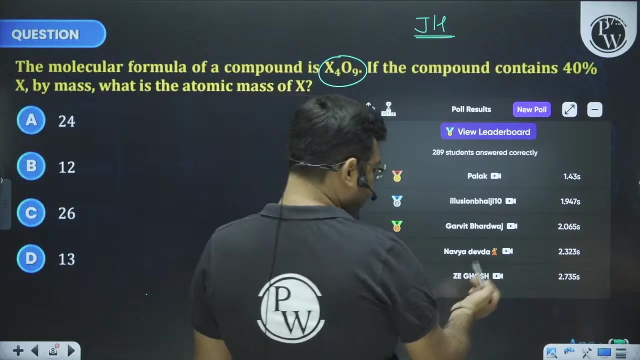 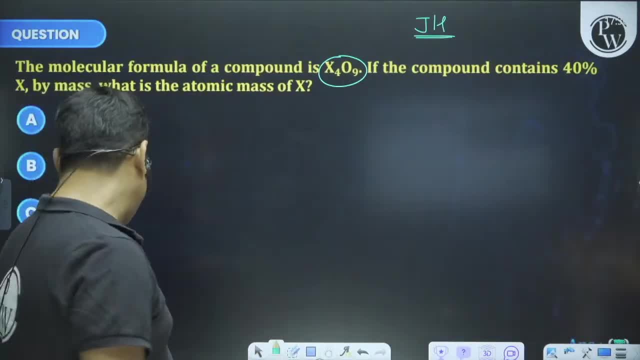 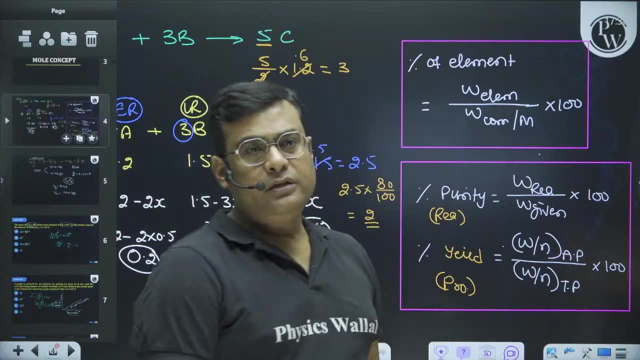 Now see, I just told you one formula. If you notice any percentage of element in any question in the world, there is no other formula other than this formula. There is no other formula other than this formula. Okay, There is no other formula other than this formula. 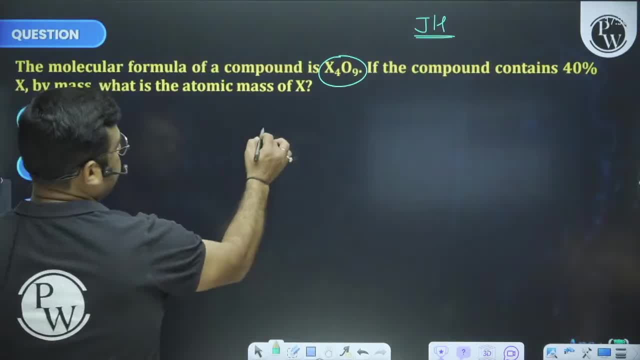 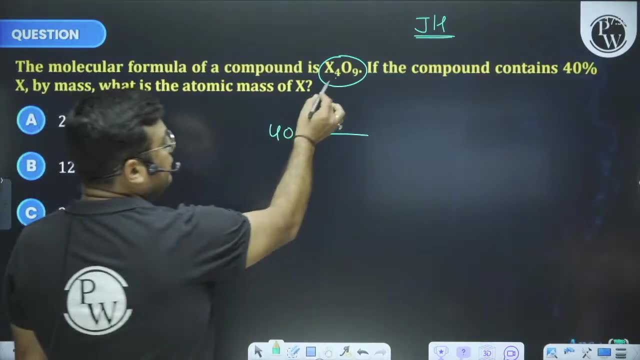 So how much percentage is seen? 40%, Sir. whose is x? So suppose I took the mass of x. Let's say I took the atomic mass of x, mass a, mana, to a case it's good- char atoms and to for a. oh yeah, it's come as: 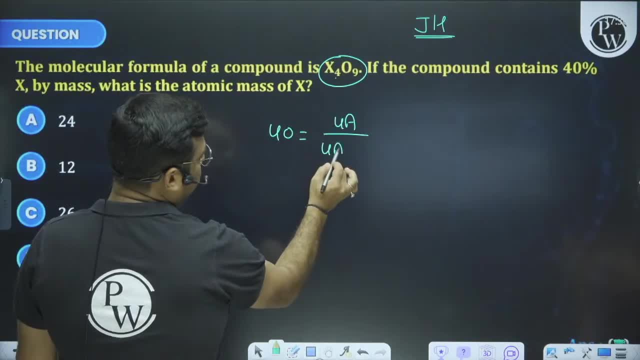 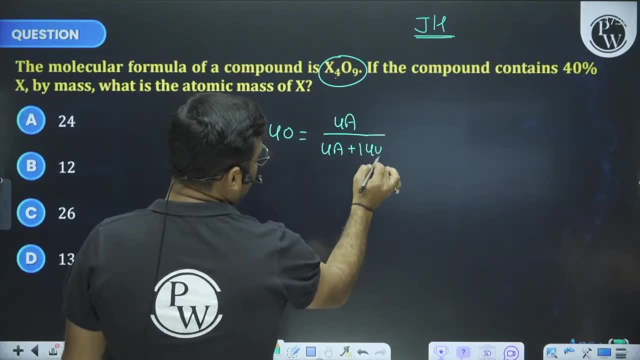 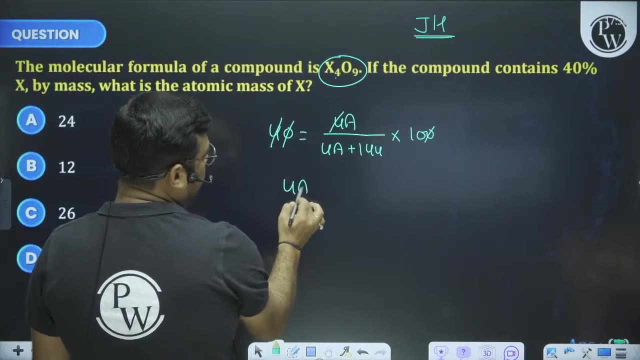 Nietzsche care, molar mass, molar mass for a plus nine oxygen, a to sixteen ninja, kitna 144, you know into kia sir, hundred TKS, a, 0 say zero, ga for, say for Gaia, sir hamara answer: oh yeah, for a plus 144 equals to: 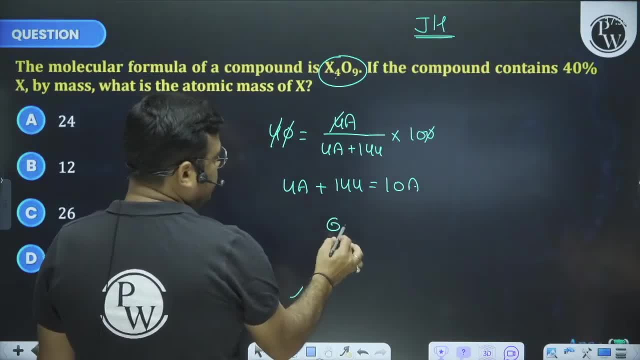 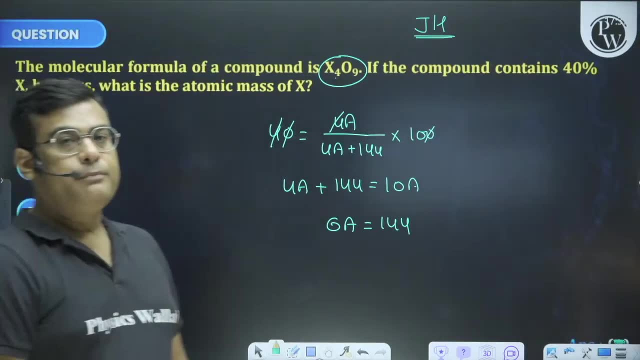 kitna ten. a matlab stick say equals to 144 matlab, a equals to up, cut 24, cut up the palli system. a up for you, but on a jar of a chunki. agar duniya ke kisi question me upko percentage digja, percentage digja a. 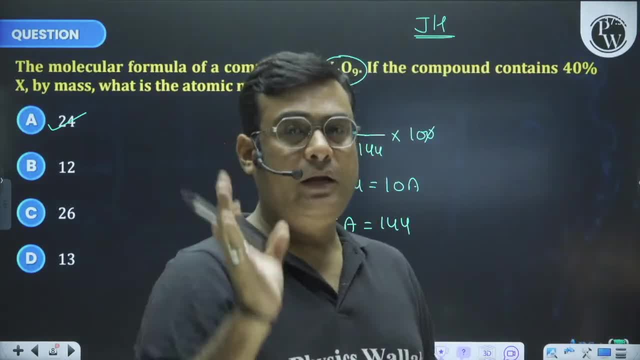 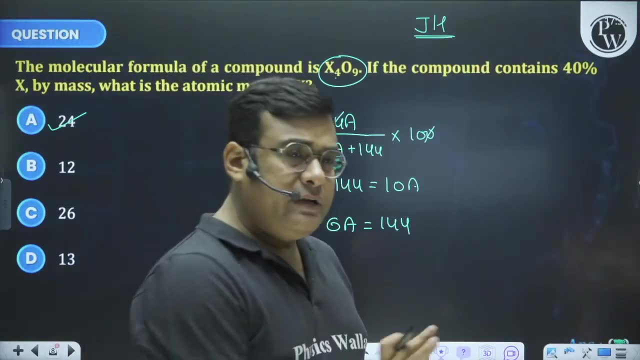 kahaani cut up is formulae kalava dosa koi formula na, but a bugger am toda sa. a bugger am toda sa apna presence of mind laga and in case efficient practice, a jinko sub kuch pata hai, but Joe. 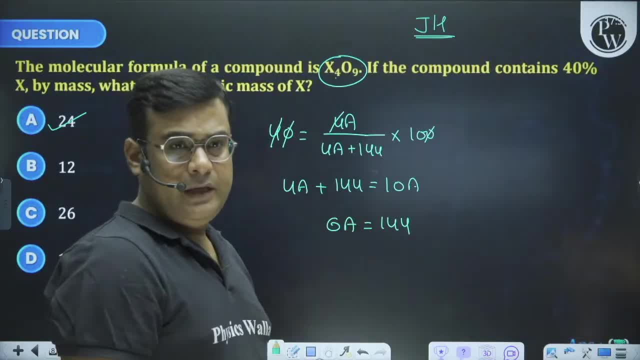 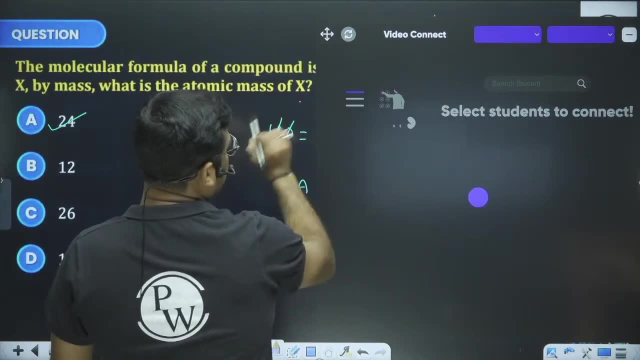 yet universal method. a her, koi si formulae se kare ga- and a ticket. but agar toda some apne dhimaak ko dhoda na cha hai to hum, maya, yeh bhi toh bol sakte hain. agar is cuff, yeh kya ho gaya, sorry. agar is ka forty percent, hey, he care to. 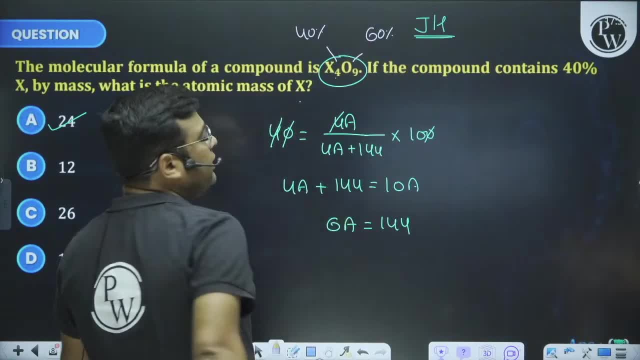 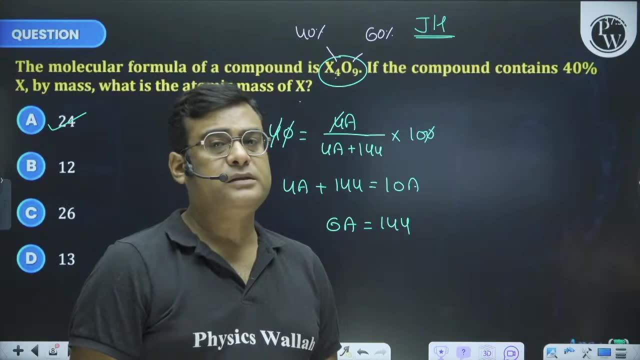 obviously oxygen ka sixty percent a a 40% dosa, 60% matlab, yeh up kiss mass ratio mehet to is to take a master show. a kiss master, show me my repair, a pair of a show to is to take a master show me. 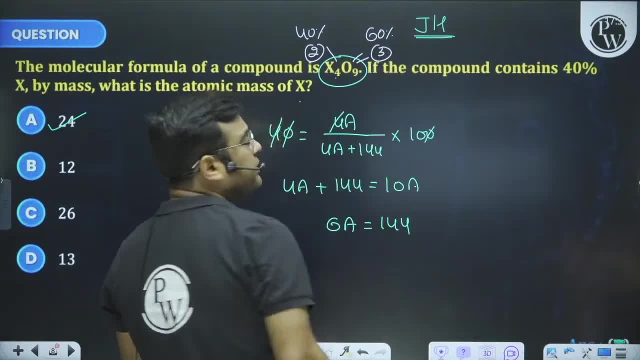 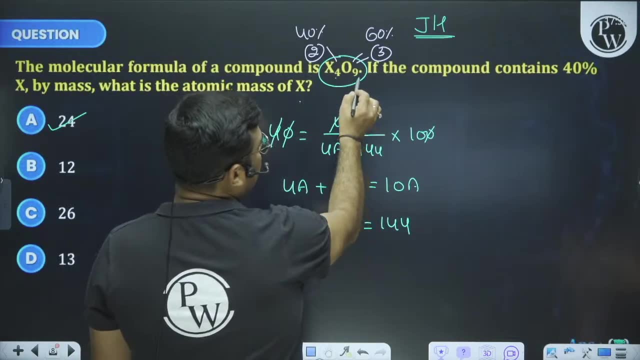 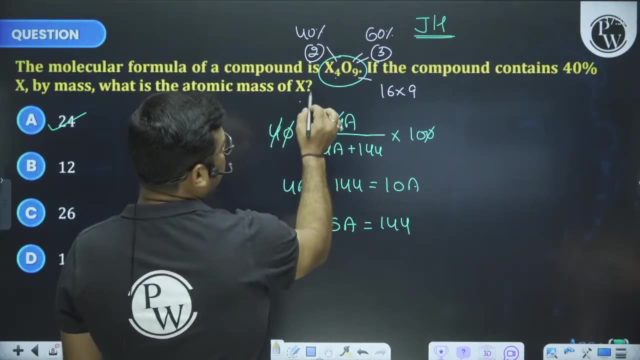 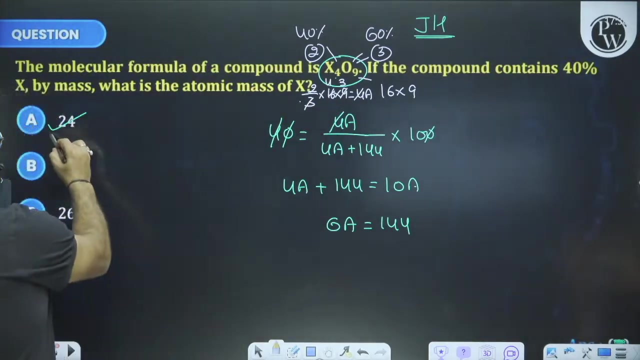 me in. this is- and I hope you get the ticket for you- he 16, 2, 4, 8, 8, 3, 0, 24,. no formula had to be applied. I am trying to explain to you. 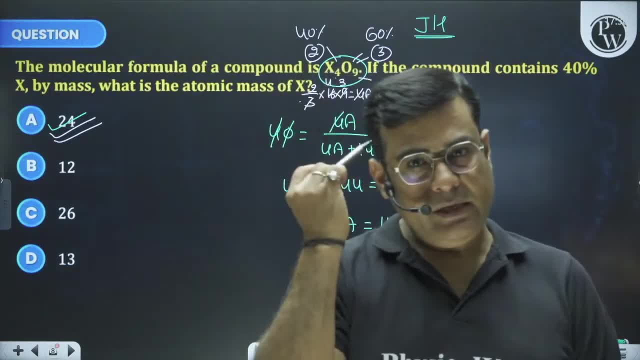 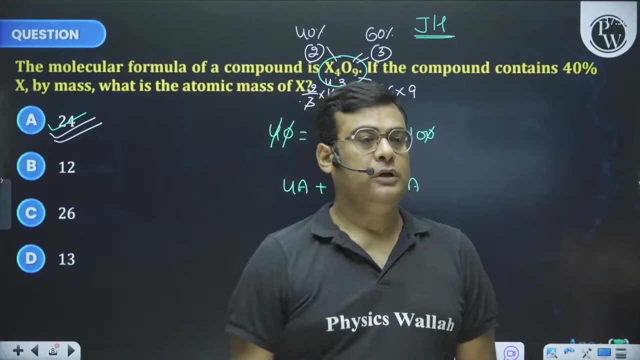 that a little bit of physical chemistry is necessary to find the right direction of the brain here, and more and more you will need it in the physical sessions that you will have tomorrow. yesterday's 11th Manish Sharma, sir, is taking you. tell me who got this trick. 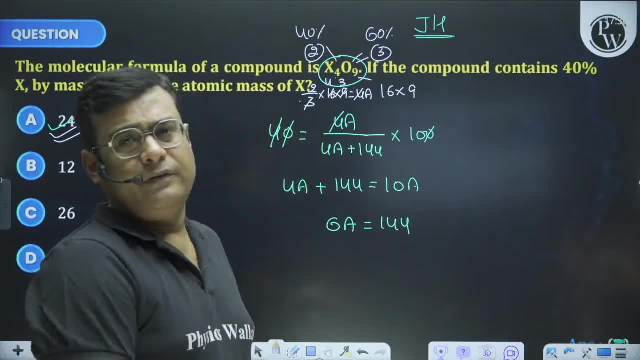 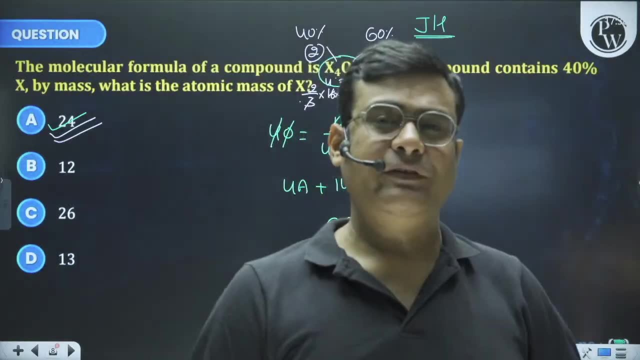 and who got the OP that there was nothing to think about. it was clearly visible. it was clearly visible. now, the single reactant we talked about. I have solved this question orally. right, HDFC is applied. it is alive. I will do a small 30 second vote: tap poll. 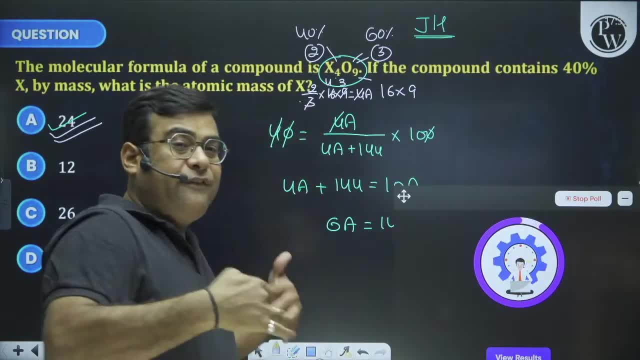 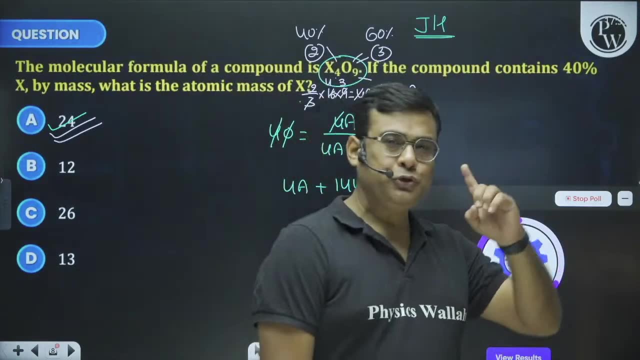 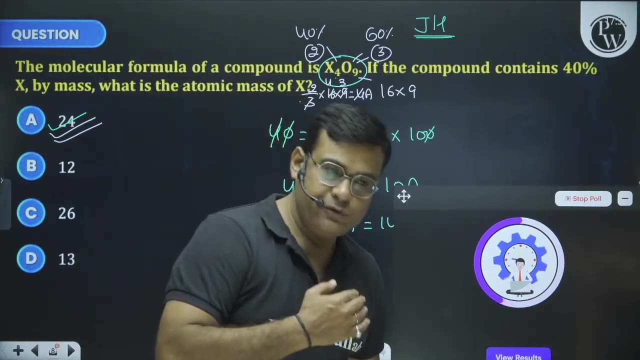 did everyone enjoy this trick? did you get to learn some different tricks? because, as much as you will think a little differently- right, think a little differently- the children have a little bit of JH. I gave the name, so now my limitation of this session is that I have to teach you. 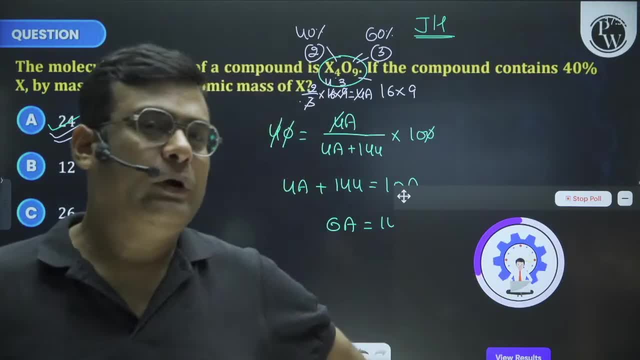 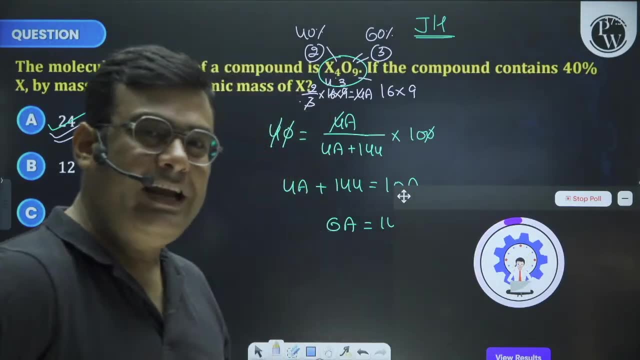 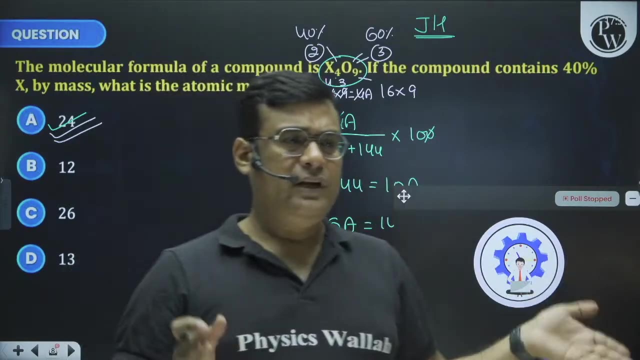 some questions day by day. but even in that, at the end of the session, I will teach you a lot of new things, new ways to solve questions. killer approaches killer. okay, did not do anything, just applied the concept, brother. 40, 60 means 2 is to 3, the story is over. 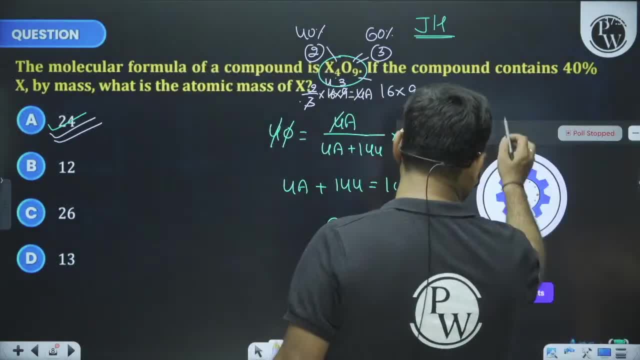 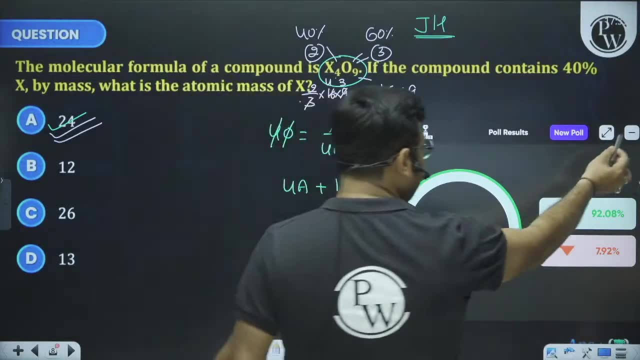 we have done it like a single reactant. okay, let's go, let's go, let's go. what does it mean? let's move on to the next question now. like this question is an orally question, the child is a small question, so I took this question as the next question. 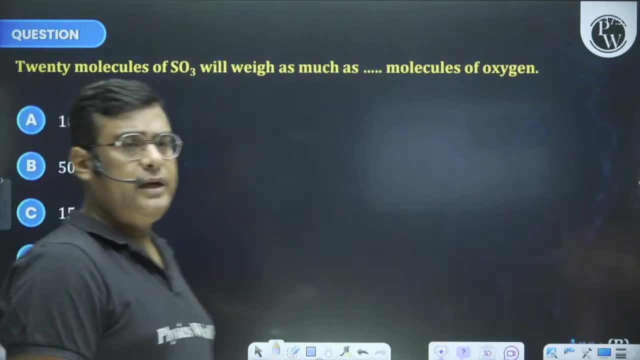 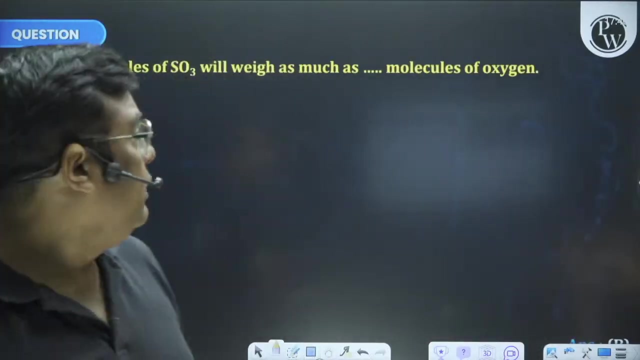 I thought you have to come to the position of doing it in an orderly manner. no, twenty molecules of SO3 will weigh as much as so many molecules of oxygen. that is going to say that if you have twenty molecules of SO3, then tell me how many molecules of oxygen. 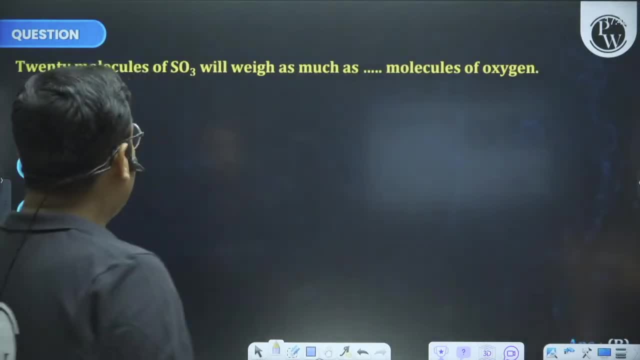 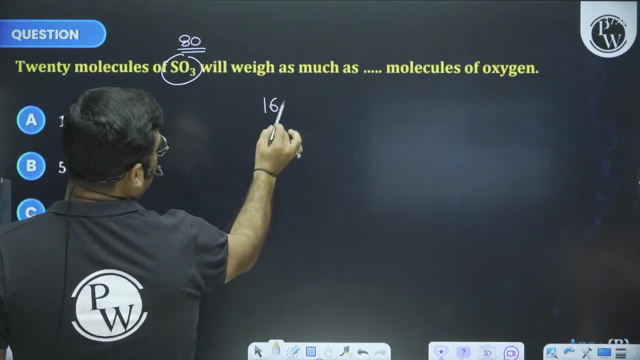 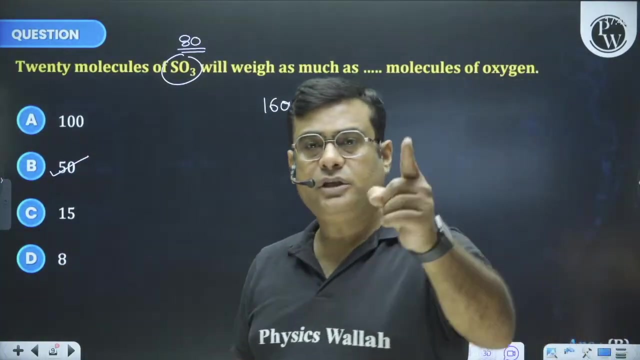 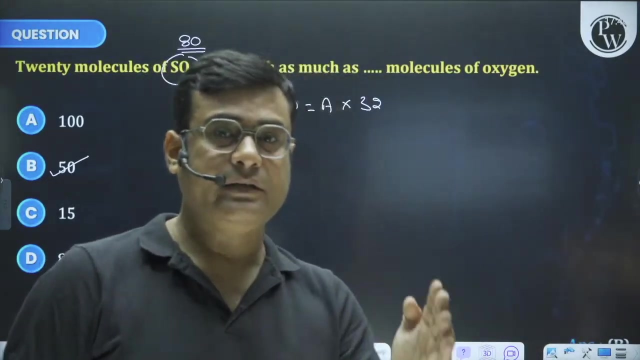 should be there now. Son of SO3. Now everyone must know the molar mass of SO3, we should also remember some molar mass, sir. it is 80, so 20 molecules means how much is its mass? 1600, now, how much is the oxygen, sir? 32, assume, we have assumed that it is A molecule. then my brother has answered directly my 50, which we know. I also know in the exam you get about 2.5 minutes to do one question, 2.5 minutes. but I want to show that we can answer the question very easily. 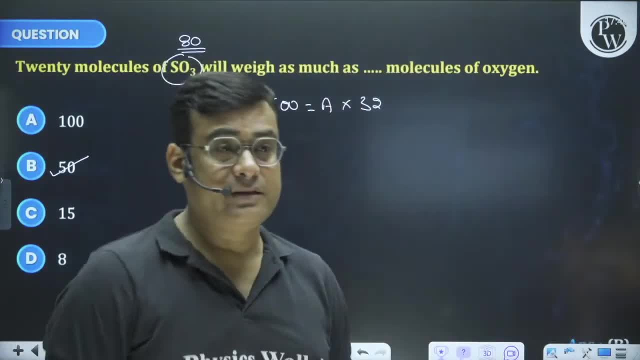 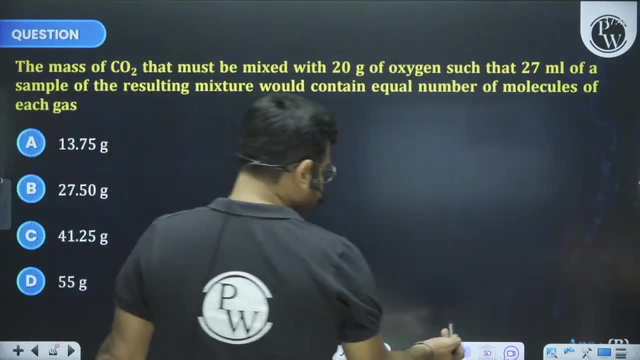 we can come to the position of doing it in 15-20 seconds. we can come, we can come. let us move to the next question. it is a little good to see. I will not do the poll again because the poll is late in every question, but I am explaining. 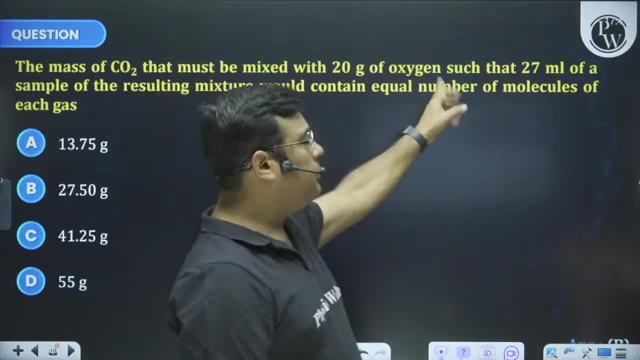 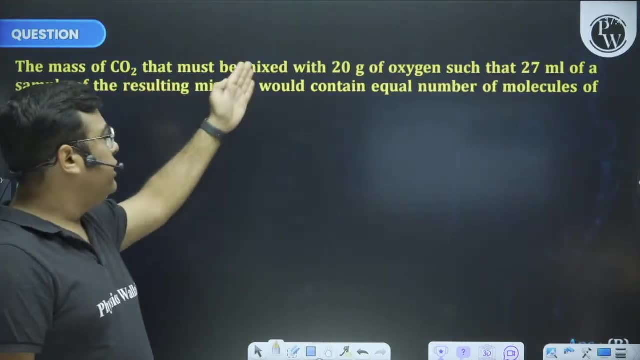 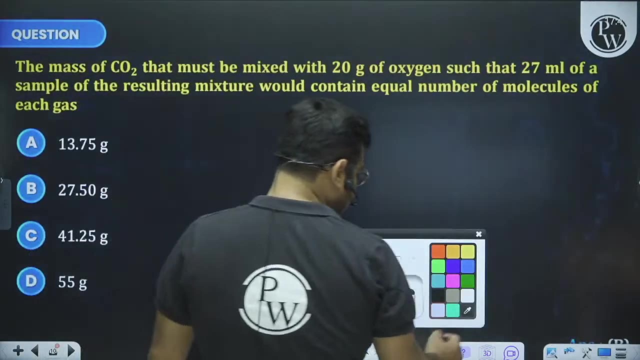 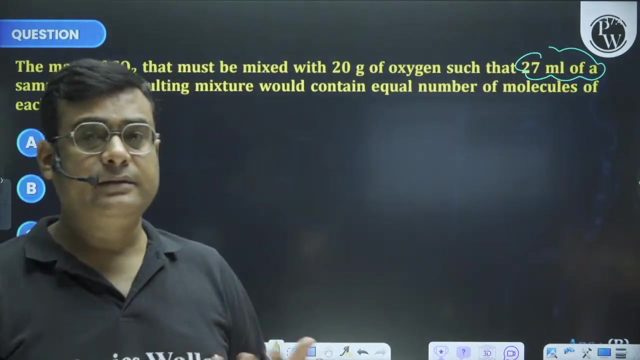 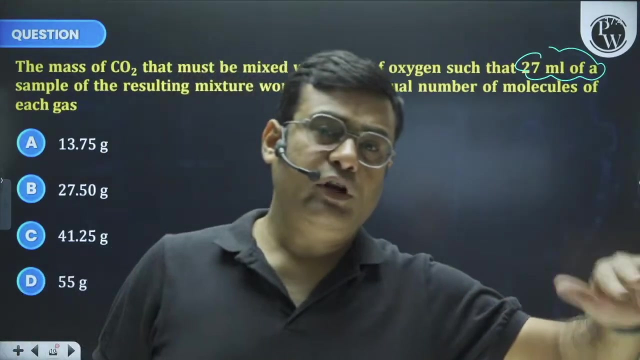 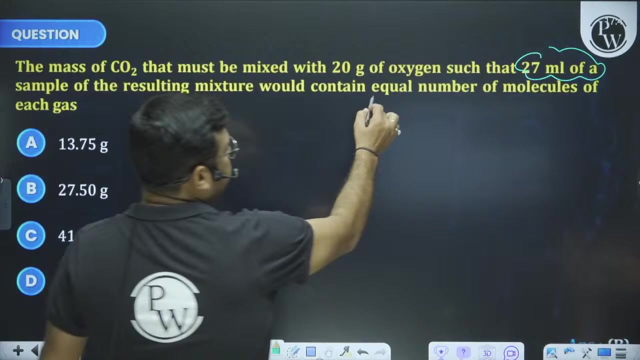 mass of CO2 that must be mixed with 20 grams of oxygen, such that 27 ml of sample of the resulting mixture would contain equal number of molecules of each gas. now, here the biggest confusion will come in the mind of the child. sir, what is the meaning of this 27 ml of sample? brother, take care of the gases, my son. if I have a container of 1 liter, if I put oxygen in it and put CO2 in it, then the volume of oxygen will also be 1 liter and the volume of CO2 will also be 1 liter. so there is no connection with this 27 ml. the main thing is that if you want an equal number of molecules, then it means that the moles of both should be equal. 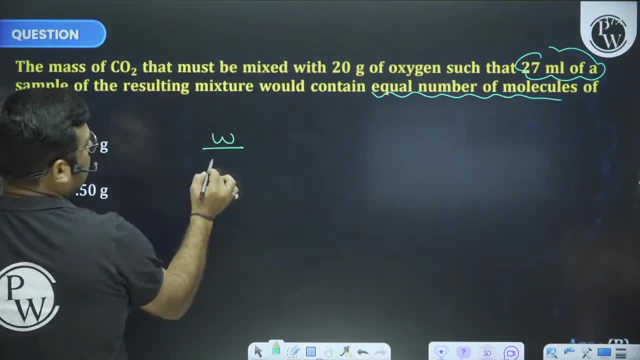 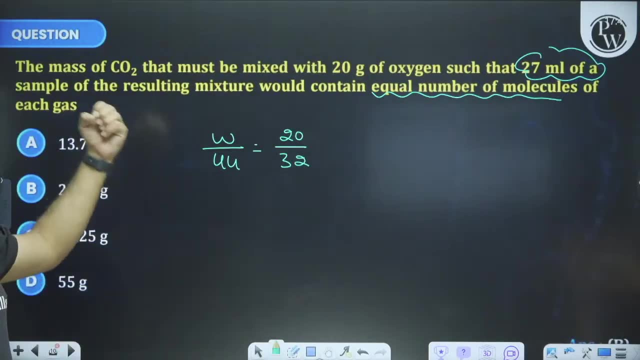 so the molar mass of W2 by CO2 will be 44 and 20, by how much? 32,. the vehicle is 22- 32. end of the story. you have directly the direct answer, And calculation has always been anxious with a little bit to make sure that the son can come from 400 anything. 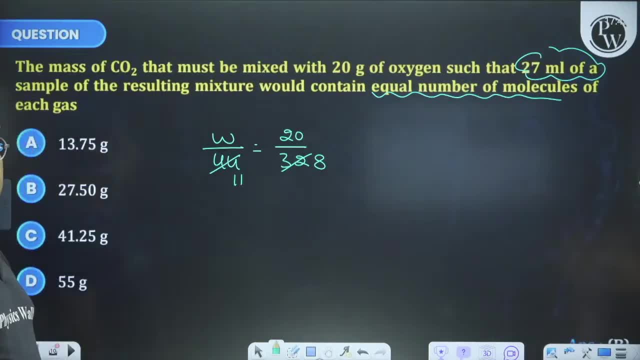 For example, four, eight go and third, two, four is right, eleven, young over and not able to see that it is here and now, can not see it when it is 20 and eight. again, to cool down only 12 not visible Nci, it will be 2 point something, otherwise it is 2.5 exactly and into 11. so 2 into 11, 22. 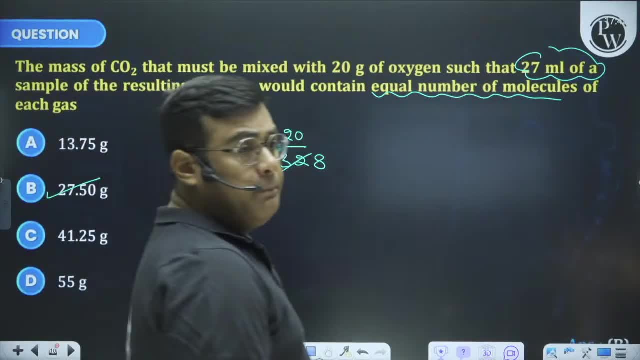 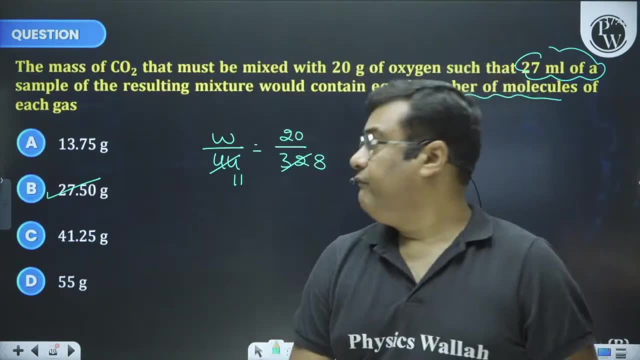 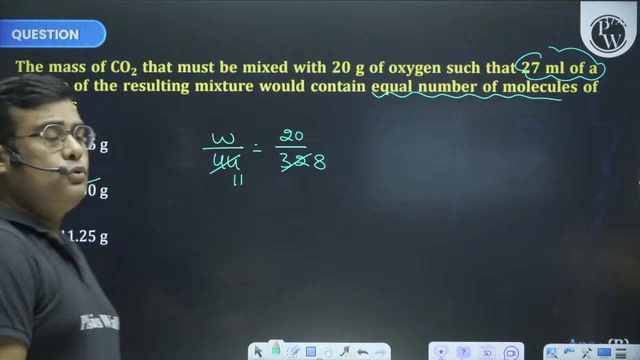 the answer around 27.5. ok, I just want to tell you that there is no compulsion to do full calculation when you are having a b, c, d type of option. when you are having a b, c, d type of option, you can save the calculation a little come. these questions are good, let's see now. 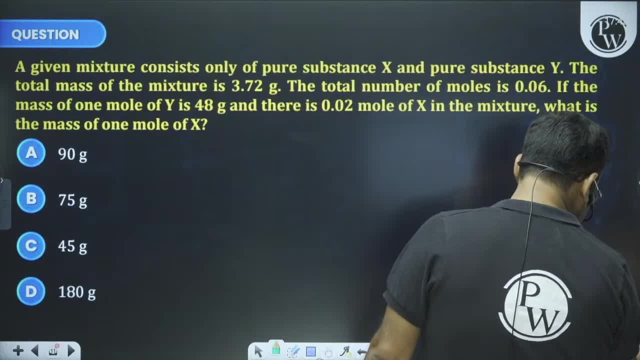 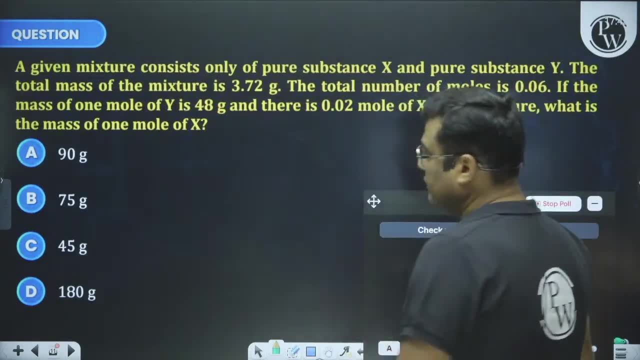 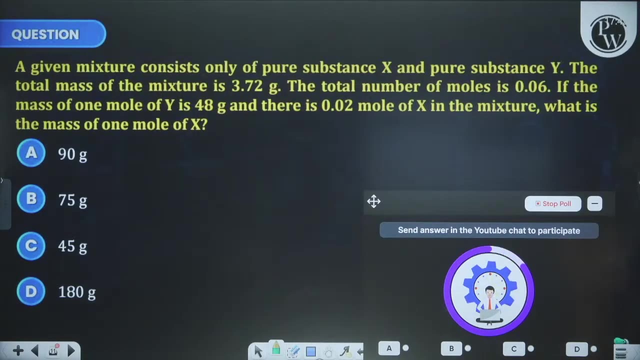 I am giving you a full minute in this. it is a good question. let's see if this type of question comes then, what will our children of 12 years answer? it integrate it. does it suit ouranden any day? that is good answer. no, works for 12 years. it is enough. he will be good for their�. 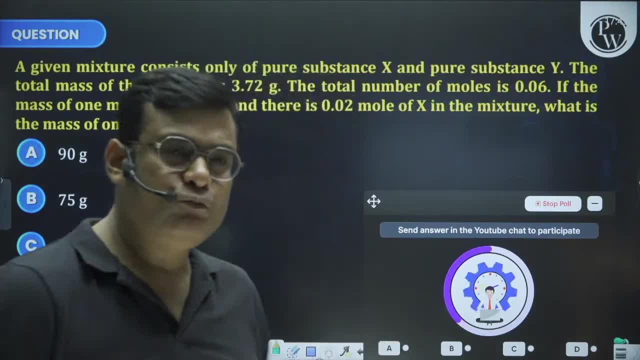 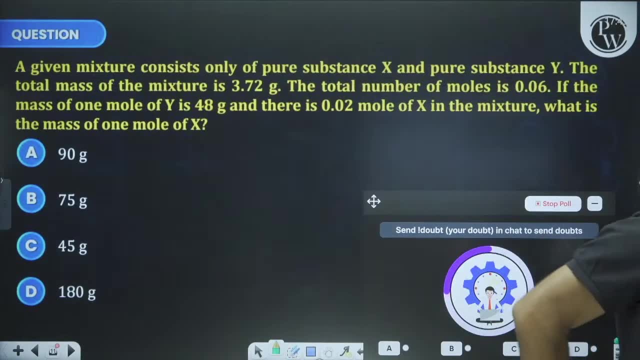 yes, hard with right. and then, yes, if he is about to go, which is he can go and understand it means next, let's say he is a man in front of the screen for 12 years. in that case he will have played very well. then what do we do to that now? then there's none. so if G is the is, it is means Karen. C is an answer to 12 years, of 13 years and ten. so I had teacher in my family, a student who has told us that our parents should take umber for three years because a post college student should take advanced or even a class. 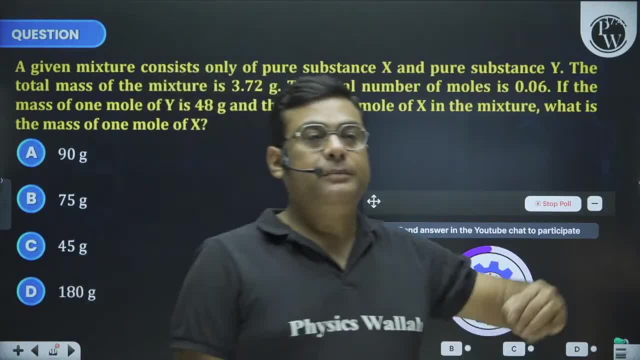 a gosh. you do still do not be an officer, and the teacher should tell us so you will know. ESC is what should be the process. you will know which is correct and I will tell you which is not correct, while else. So if the child is half of the molecule, then the air remains empty. 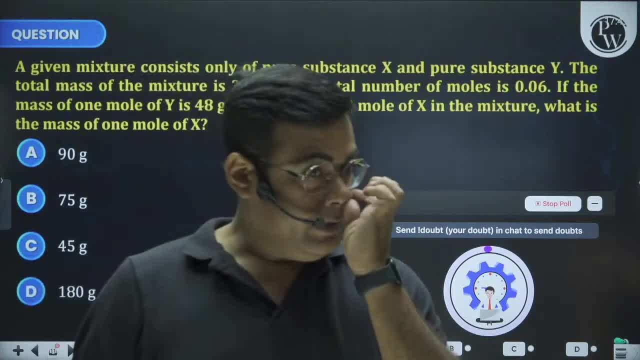 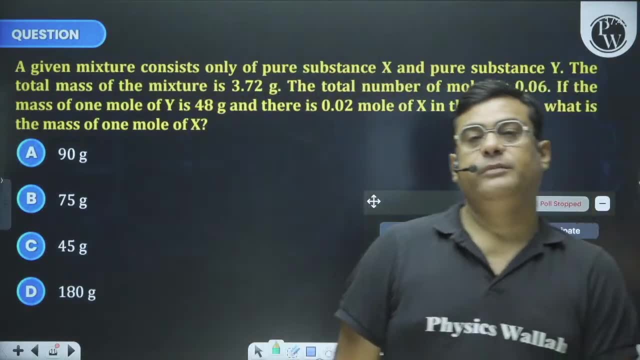 Many children are not able to remove the molecules from one molecule to the other. If it is good, then the work will be good, And if the redox is good, then it will be easy for you in inorganic chemistry. If the redox is good, then it will be easy for you in inorganic chemistry. 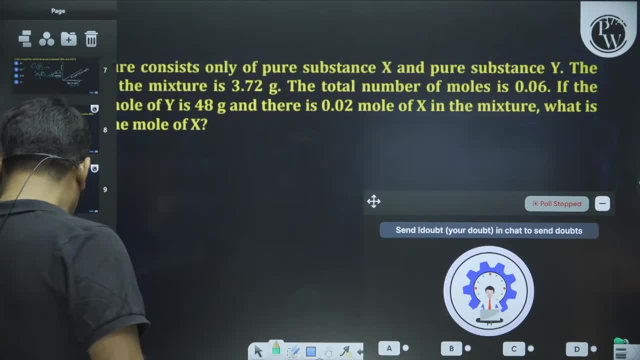 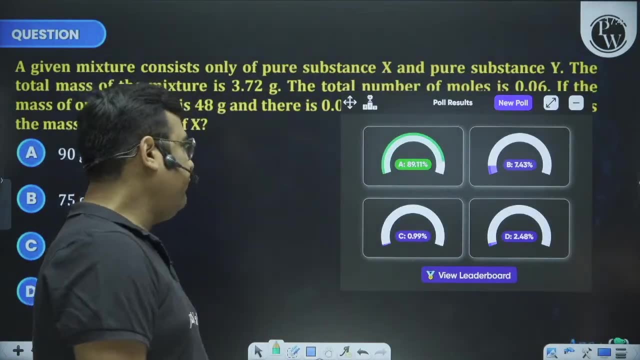 Okay, let's go. So let me see the answer first, Because I also have to solve. It was given A. I am solving it for you. Let's see the results. 89.11%. You are doing very well. 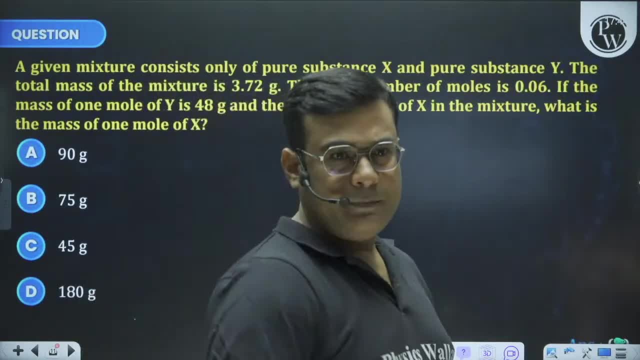 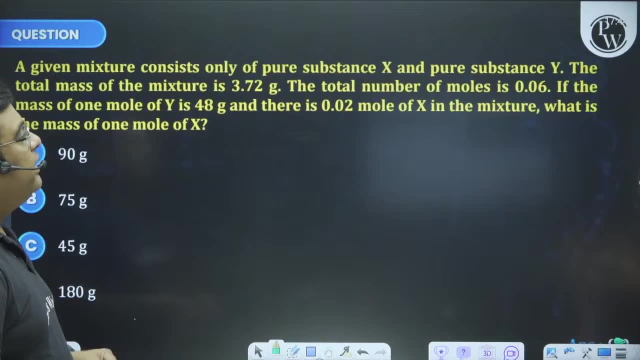 You are ready. It is a little bit of a level. It is a salute. It is a salute. It is a salute to all of you, Okay, So what is he saying? A given mixture consists only of pure substance X and pure substance Y. 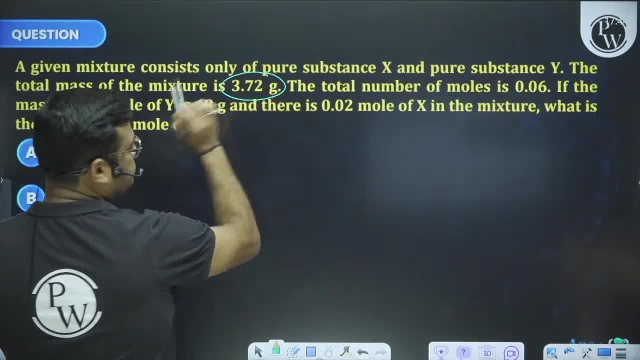 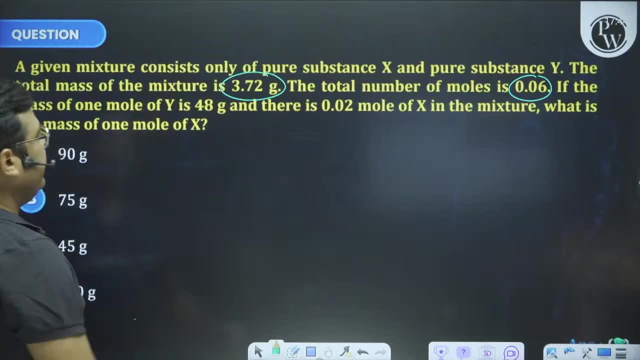 The total mass of the mixture is 3.72 gram. Okay, Total number of moles is 0.06.. Good thing If mass of 1 mole of Y means it has given its atomic mass 48. And there is 0.6.. 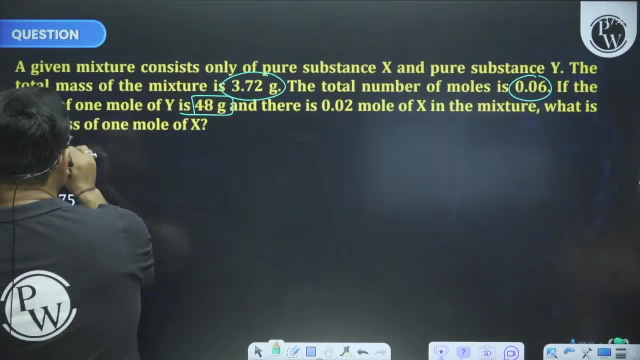 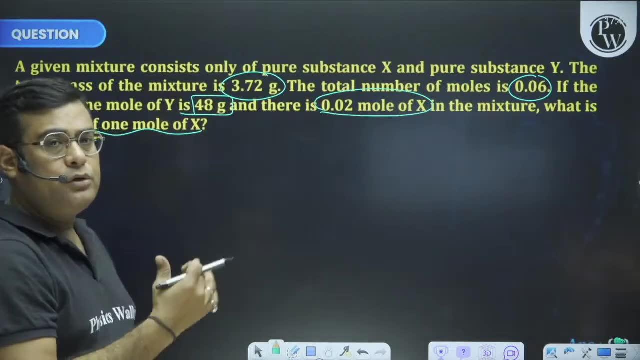 What is the mass of 0.02 moles of X in the mixture? What is the mass of 1 mole of X? Now he has said that X has 0.02 moles. What did I say, son? I have tried to ask all kinds of questions. 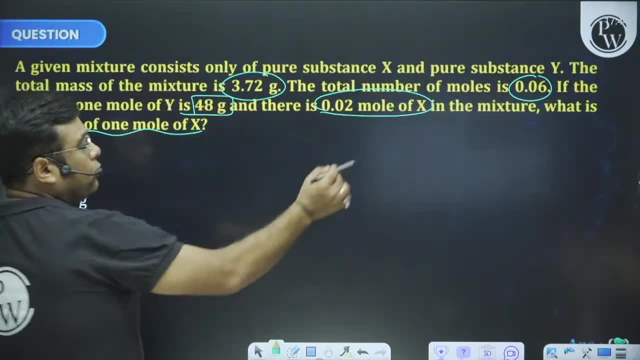 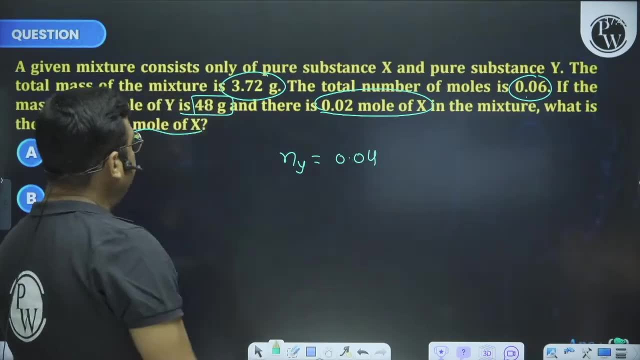 See, I have also asked the question of moles. Okay, So if the total moles are 0.06,, then that means the moles of Y have become 0.04.. Agreed, Now what is the formula of the number of moles? 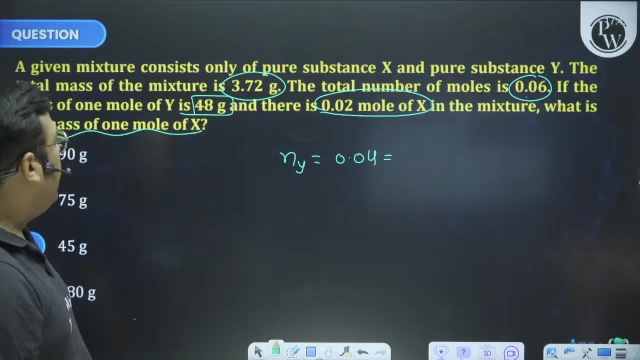 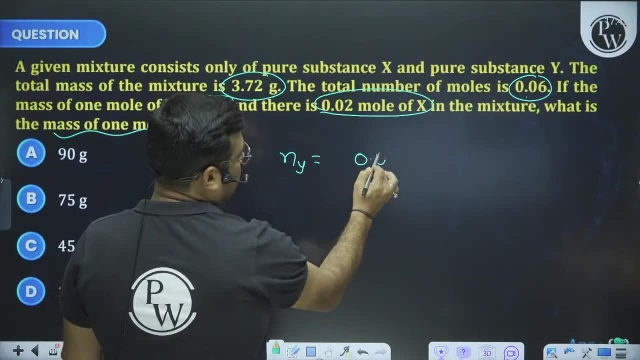 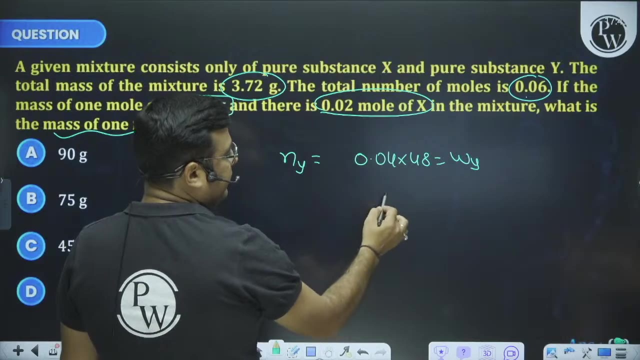 Given mass upon molar mass. Okay, Now I don't know the mass of Y, But if I multiply this 0.04 by 48, then this is the mass of Y. From the same formula: 48,, 2096,, 96,, double 192. 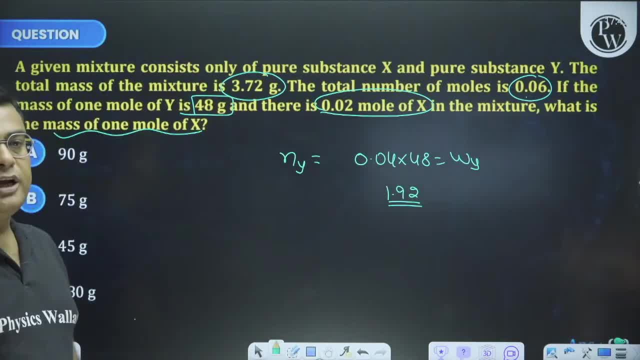 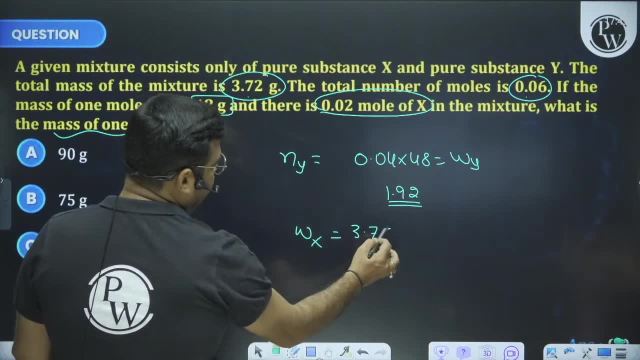 Calculation is done in this way Means you have the mass of Y: 1.92.. Okay, Total mass was 3.72.. So what is the mass of X, Sir? 1.92 out of 3.72.. 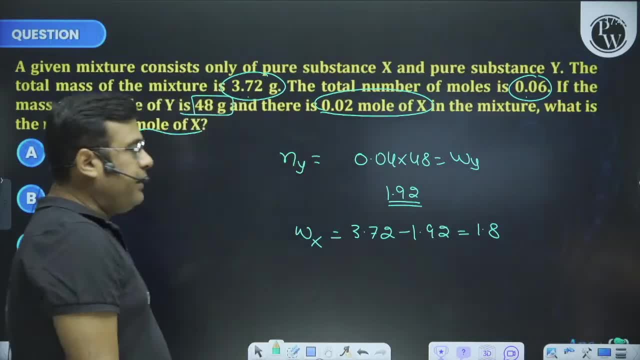 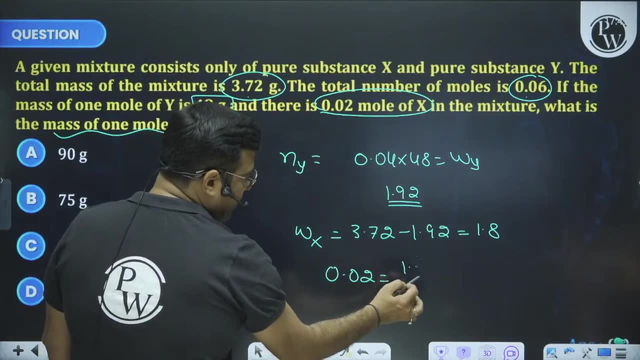 That is 1.8.. That is 1.8.. And now, what is the formula of the number of moles? We have given the moles as 0.02.. Sir, given mass upon atomic mass, Always children. 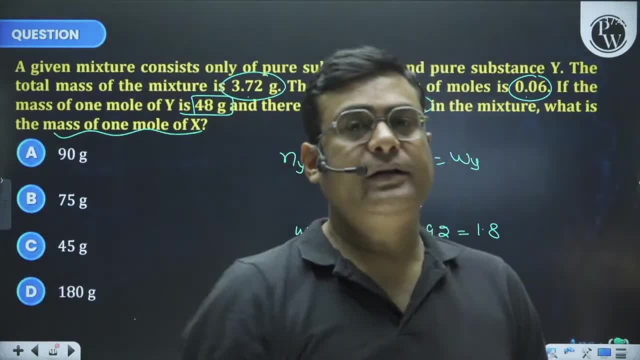 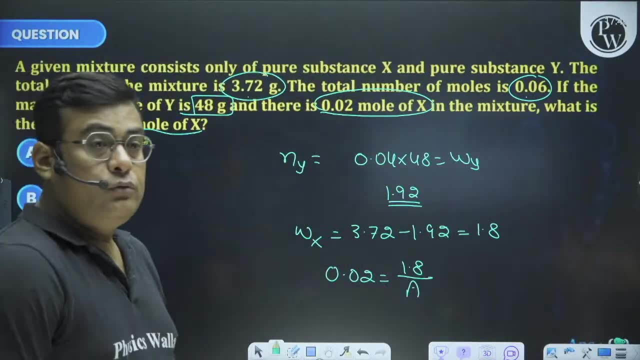 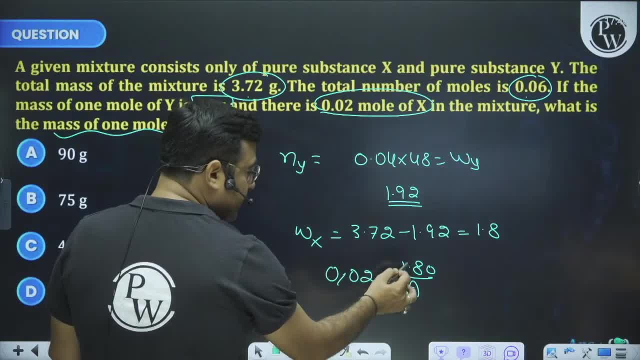 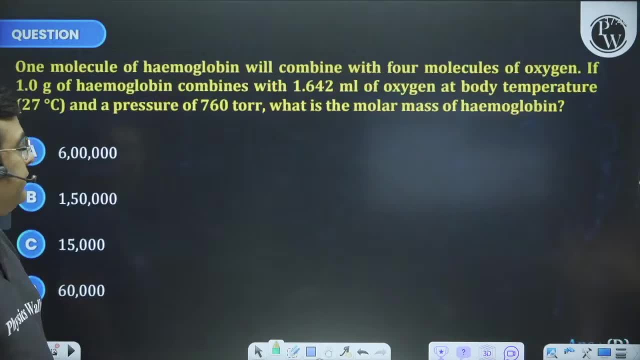 You have to do it. You have to do it slowly so that you can remove your decimals here. then 180 by 2 is the direct answer of your 90, but the maximum children have done it right then. there is nothing like this. let's go, let's go, let's go. 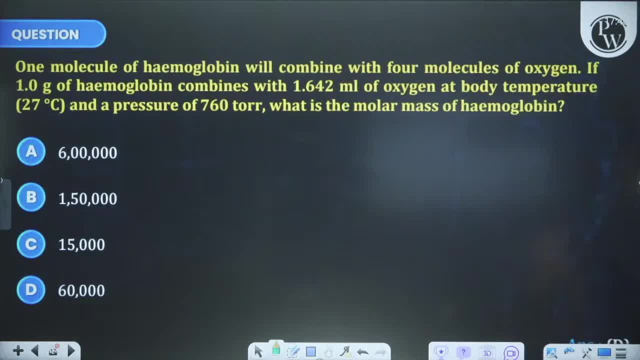 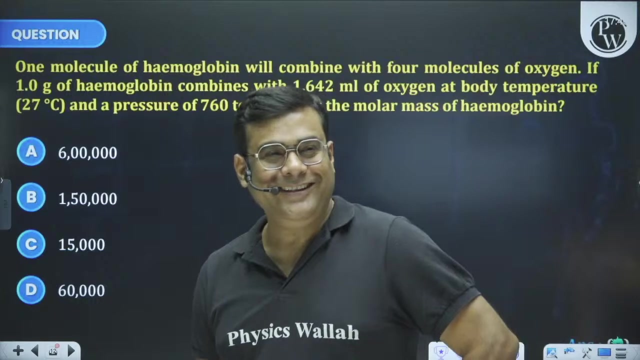 tell me. another question of a little new style. there is a question of a little new style. let's do the same thing with this cheating with you. then, son, then there is no scholar in the world. I think some people are knowing and they are ticking. don't do this, my dear. 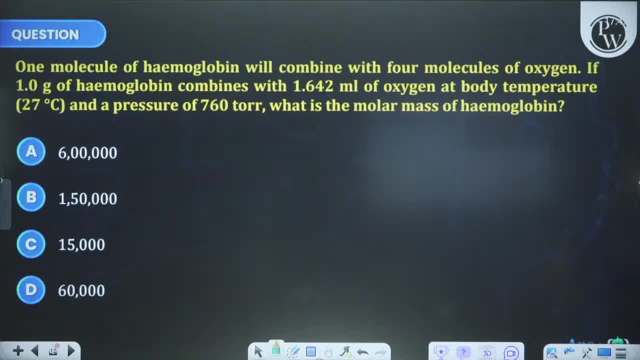 if you have difficulties in your journey, then be courageous. if you have difficulties in your journey, then be courageous. if you have difficulties in your journey, then be courageous. more increases. if there are difficulties in the journey, then the courage increases more. if 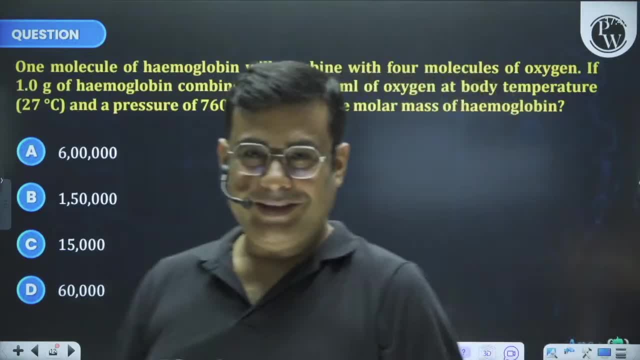 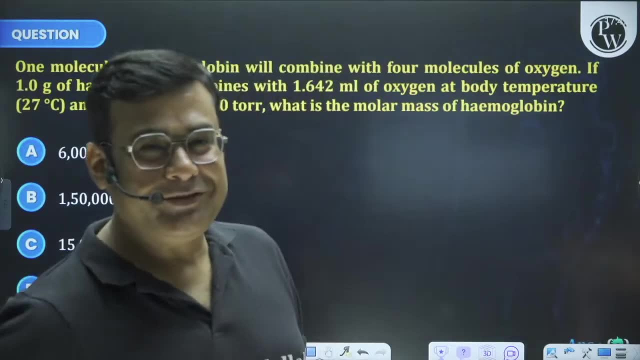 someone stops the way, then the courage increases more. when without a helmet it should not work like that. but if we go and the policeman tries to stop, then what do we do? here and there we try to run. so he is saying that if someone stops the way, then the courage. 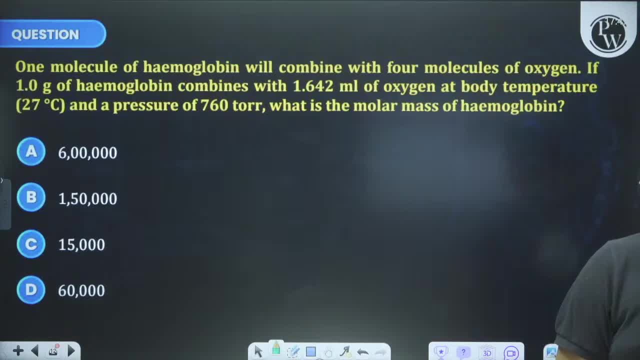 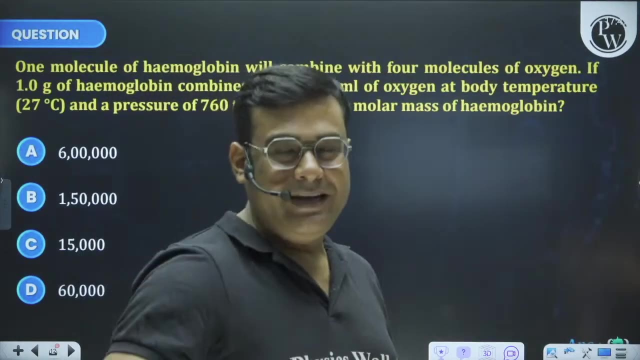 increases more means: ok, if you come on sale, then the price goes down often. if you come on sale, then the price goes down often if you don't want to sell. if you don't want to sell, then the price increases more if you don't want to sell. 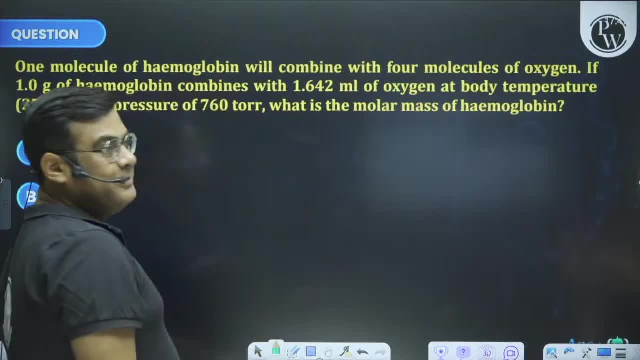 then the price increases more. come on. so I understood in this question. now what is the logic that many people are looking at the answer. now I have to take care of it a little. let's go. so what is it now, son? one molecule of hemoglobin will combine with 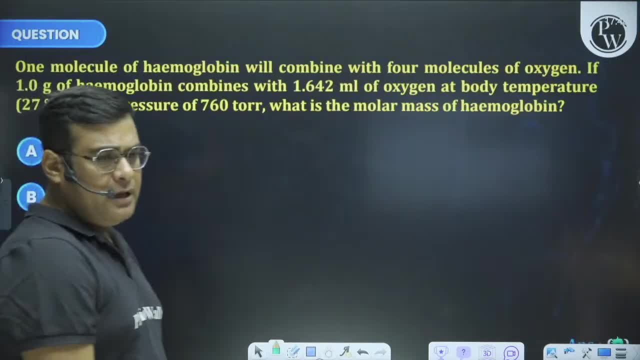 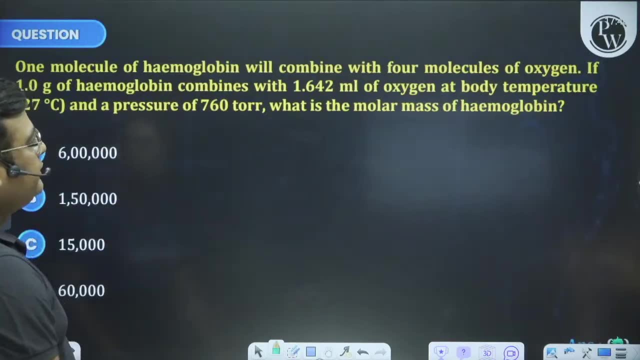 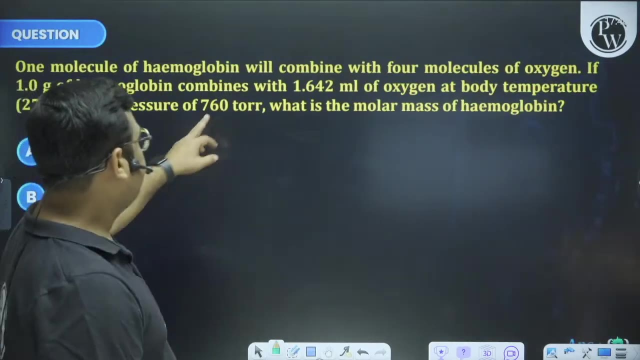 four molecules of oxygen, which we may know a lot. if one gram of hemoglobin combines one gram beta with one point six, four, two ml of oxygen at body temperature that is, 27 degrees Celsius and one press and a pressure of 760 tour, what is molar mass of hemoglobin? and our work is that we 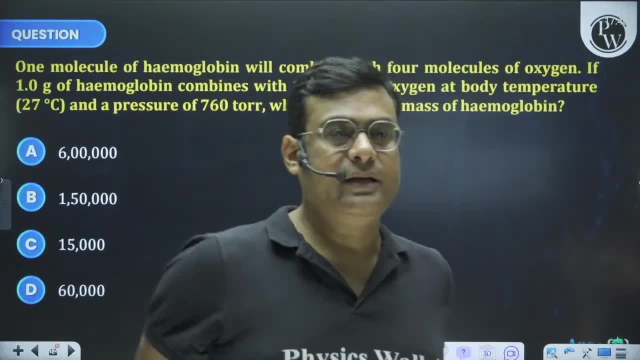 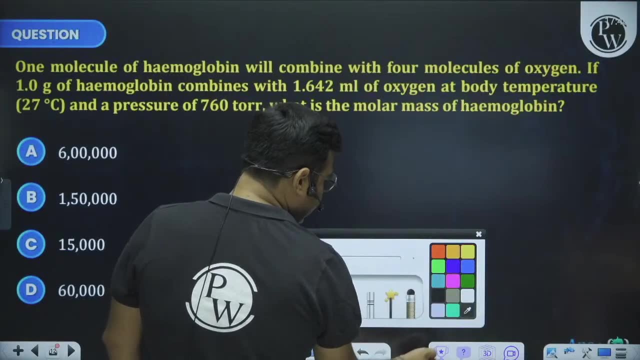 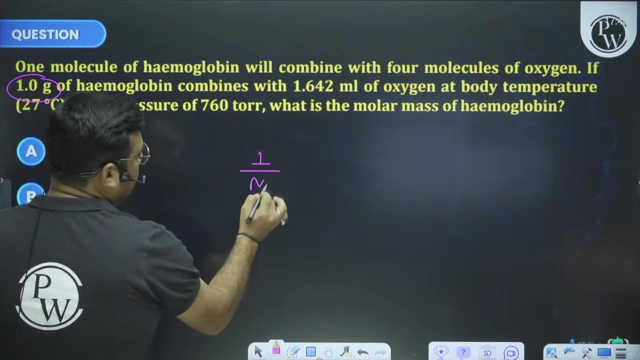 can easily set the question in our mind and work quickly. so, brother, that set will be your responsibility. now tell me. see my responsibility. I will tell you if I have one gram of organ HMO expand to bihüm. so I have band upon, I guess, its moller mother side. what happened with your Hemoglobin bachoch moles? 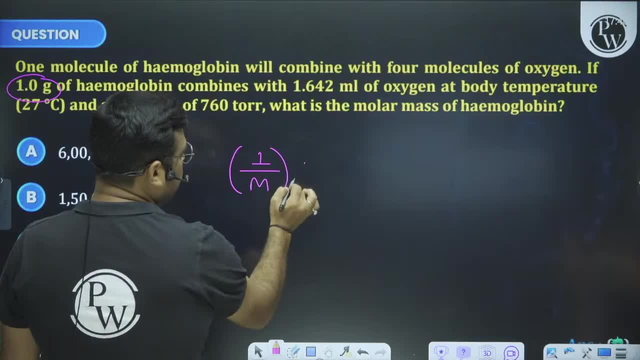 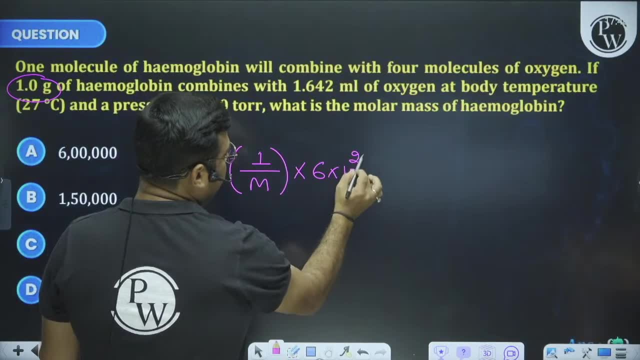 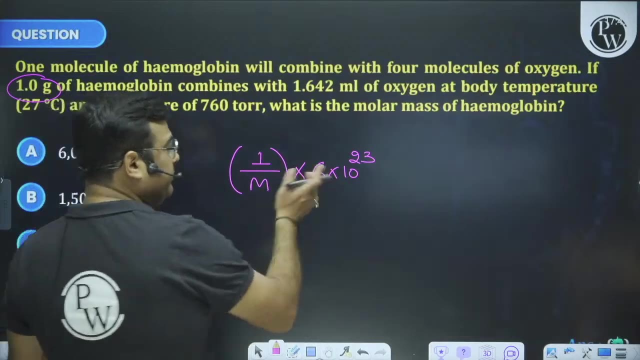 have been liked to brotherhm. that will happen to the children of haemoglobin into, into into thing if i tom same number multiply 6 into ten, k power twenty three to Ghana happened to this운� solid egg. how many of you children have taken molecules to you today? if they are, five, one hundred and forty-two? 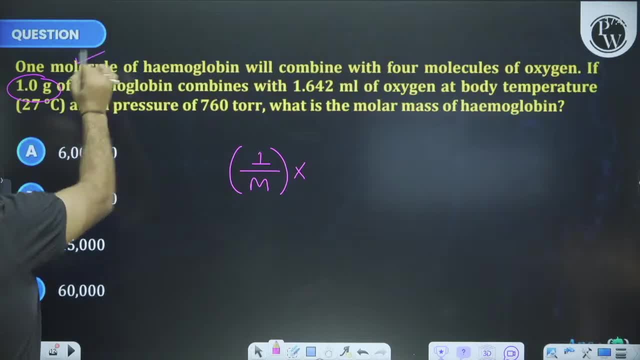 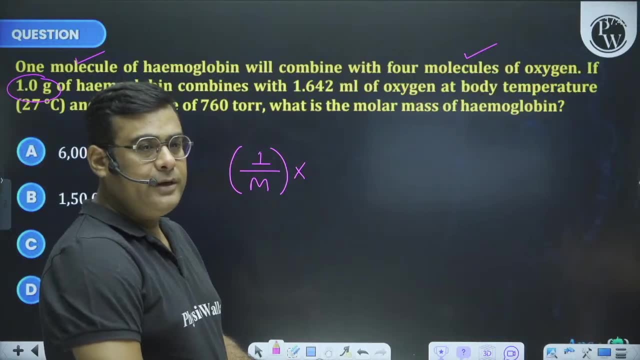 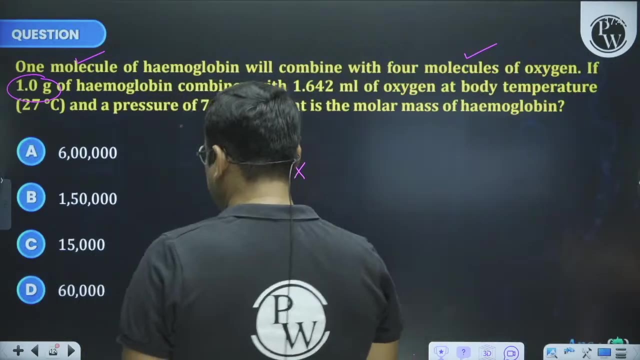 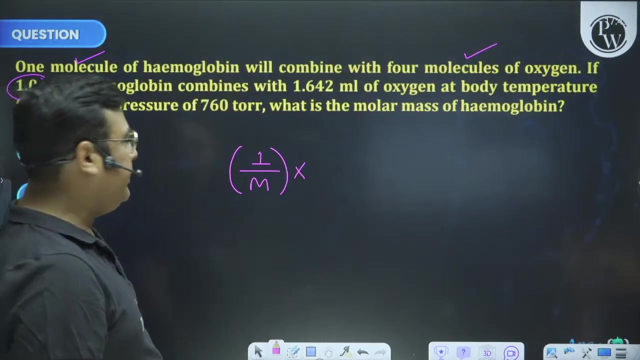 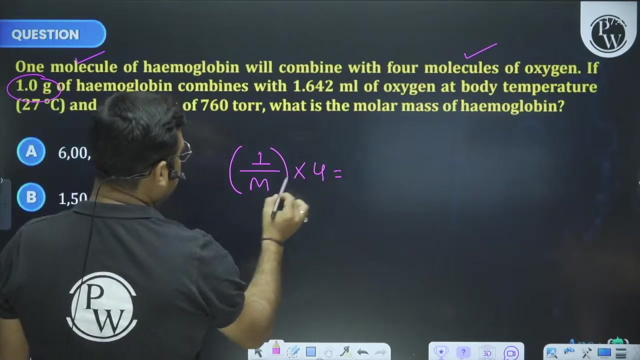 If one molecule of Hemoglobin is combining with 4 molecules of Oxygen, it means 1 mole is combining with 4 moles of Oxygen. So if I multiply it with 4 moles of Hemoglobin then that will be the moles of Oxygen. 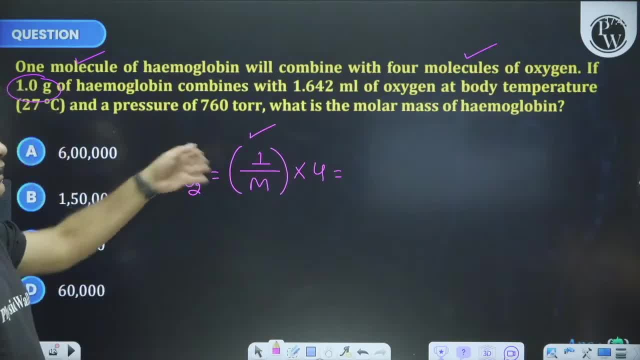 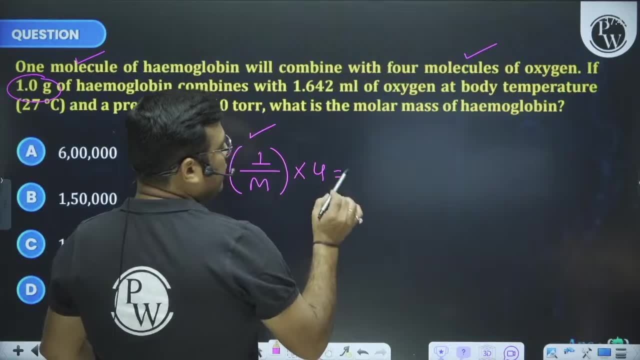 1 by m is the moles of Hemoglobin. multiply it with 4 and it will be the moles of Oxygen. And here put PV equal to nRT. Now again, try to save the calculation. In PV equal to nRT we have to subtract n. 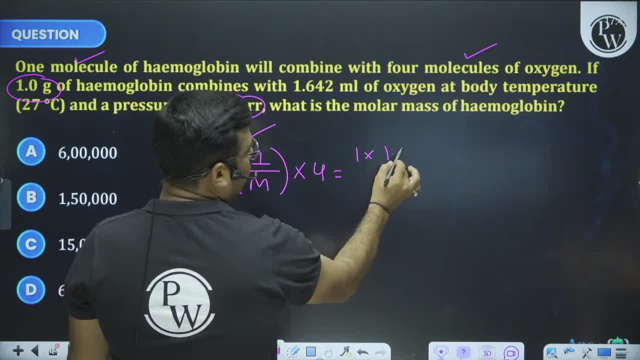 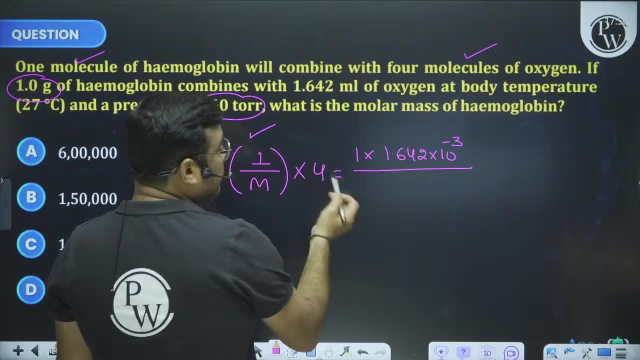 760 Torr means the pressure is 1.. The volume is 1.64 to mLA, So I multiplied it by 10 to the power of minus 3.. Now look at the value of R below. Why did you give 1.642?? 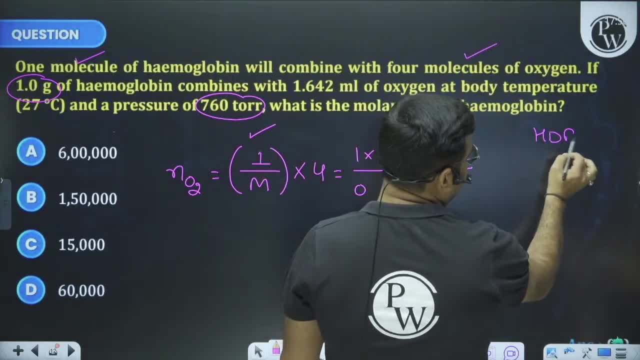 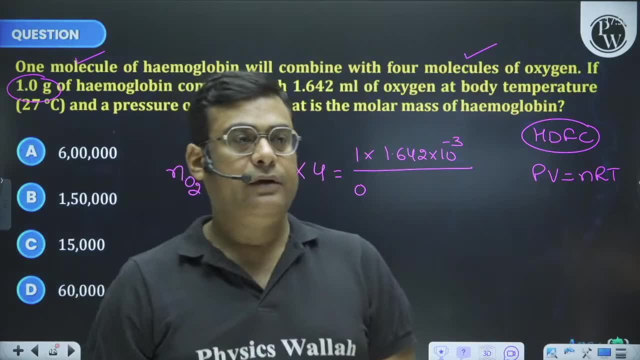 Now listen to my HDFC Hirvani's Developed Fast Calculation. PV equal to nRT. whenever you use it, whether you use it in chemistry, whether you use it in physics, you have to multiply R with T And for maximum children, 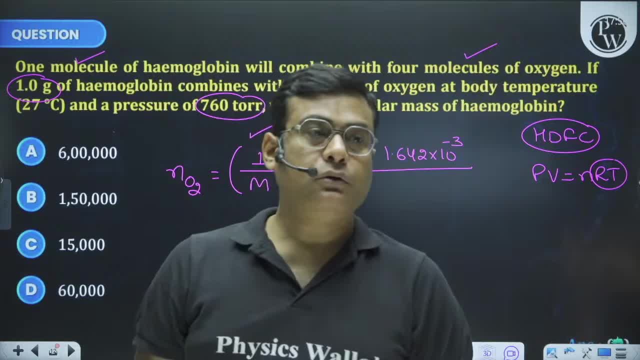 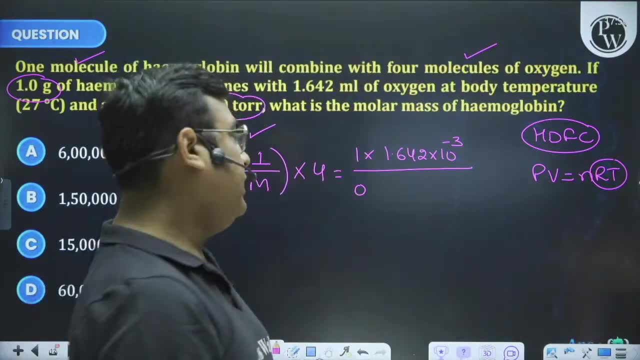 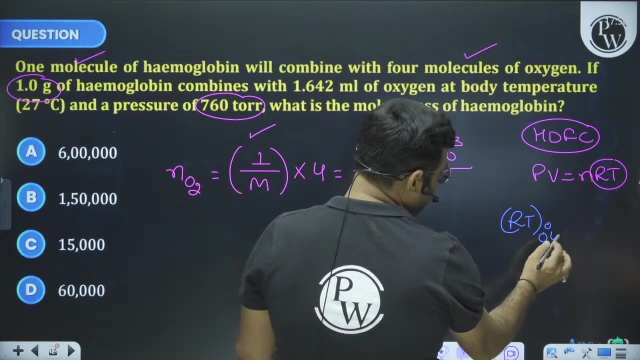 the value of R is 0.0821.. And when it has to be multiplied by 273 or 300, it has to be multiplied by 2.. Then brother gets very worried. So I am telling you two small shortcuts. The value of RT if the temperature is 0 degree Celsius. 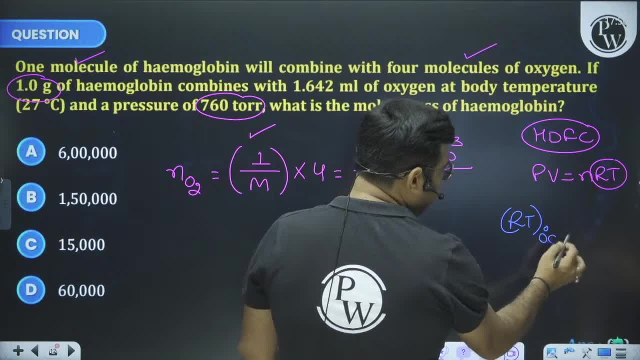 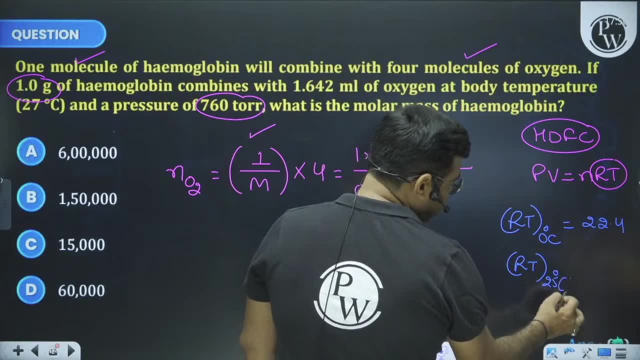 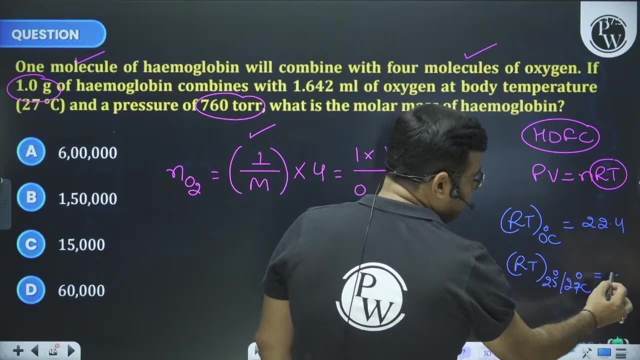 then the value of RT. if the temperature is 0 degree Celsius, then take 22.4 directly And the value of RT if your temperature is 25 or 27 degrees Celsius and take this in single ABCD options, then roughly it is 25.. 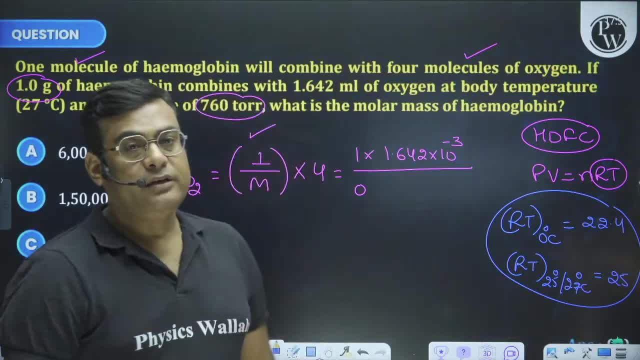 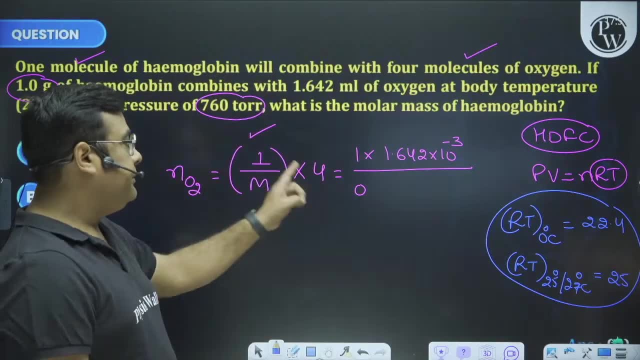 It is a little less, but in single digit ones, that is, in which there are ABCD options, you can take it. Okay. So, brother, 1 by m is the moles of hemoglobin. Let's do it into 4,. 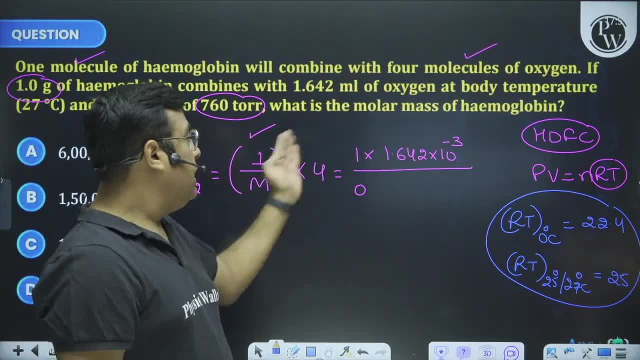 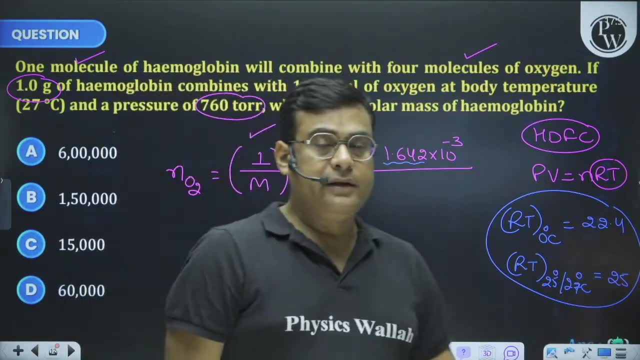 because the condition was given Moles of oxygen. Now I am removing the moles of oxygen from PV equal to nRT. Now, brother, again and again I say a song to the children a lot, Remember you hit the entry. 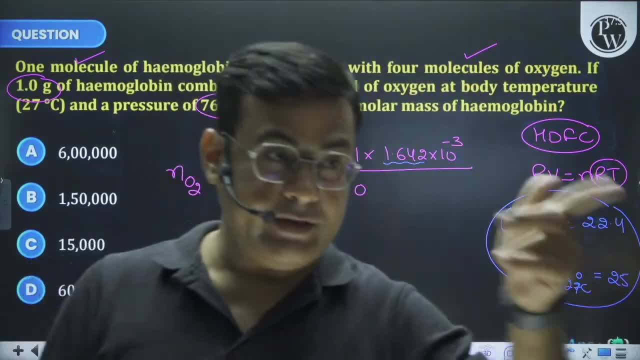 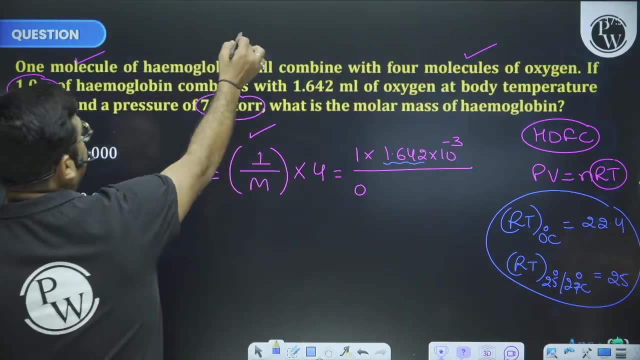 the bell rang in the heart. How did it ring? The bell rang: Turn, turn, turn. Now who hit the entry? 1.642.. Brother, the value of R is 0.0821.. So I request you that 821. 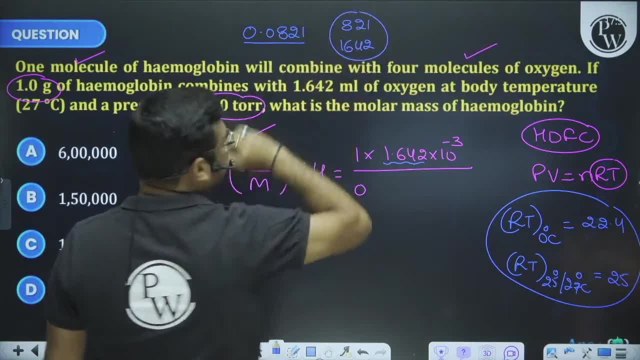 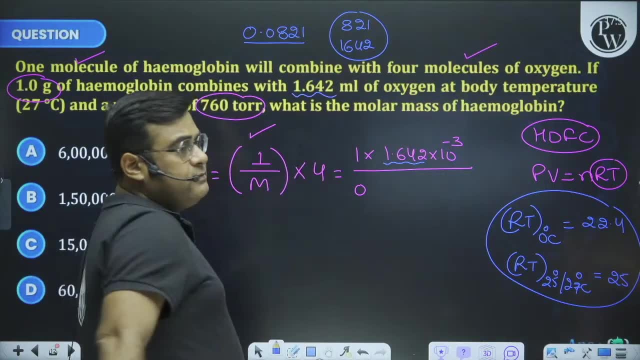 and its double, then you must have 1642 in your mind Whenever such things hit the entry. children, you will also get this in the exam. you will also get it in physics, you will also get it in chemistry. So as soon as the entry of such things comes, 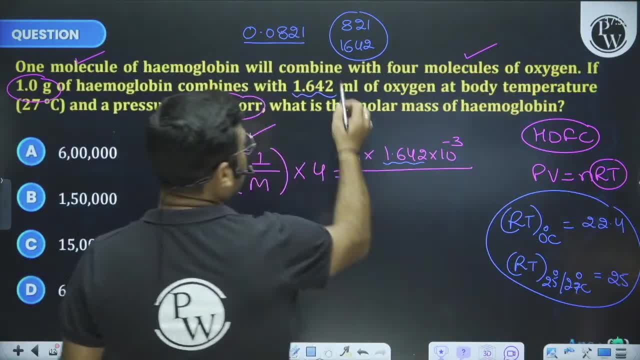 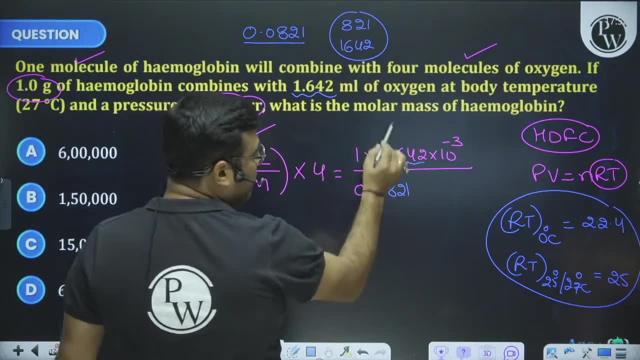 you must set it, Brother. this will be the logic in it. 1642 means I will take it 0.0821.. So that I can easily cancel it. And the temperature is 300.. The temperature is 300.. 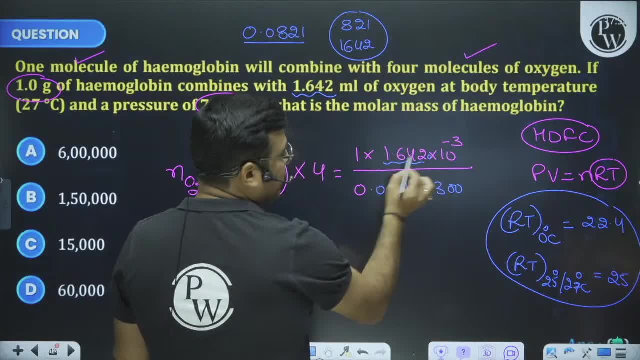 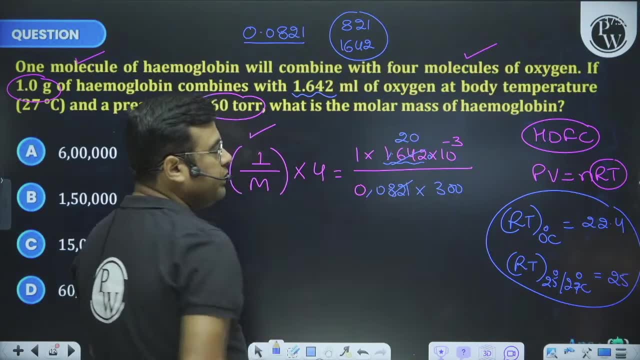 Is everyone getting my point? After decimal, I placed 4 here. Decimal removed 821 double, Sir, I just told you. so this is 20.. Are you getting my idea? 1, 0 to 1: 0 is also removed. 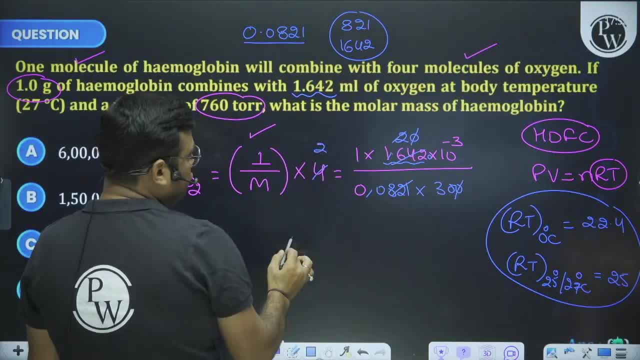 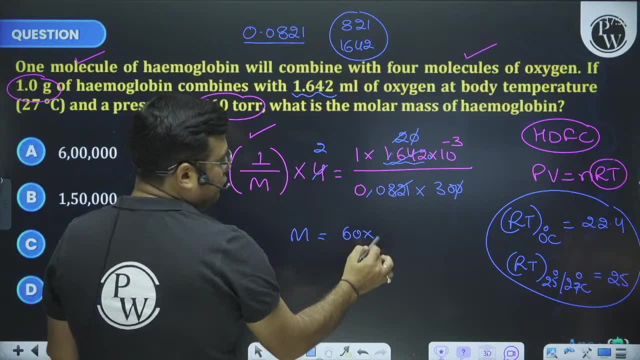 children. I did this, I did your 2.. So how much is the molar mass? now M will go there. 30 into 2 is 60. And 10 power minus 3 from there to here is plus. Your answer is 60,000.. 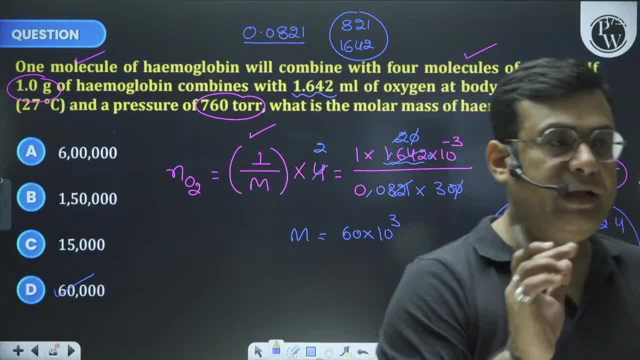 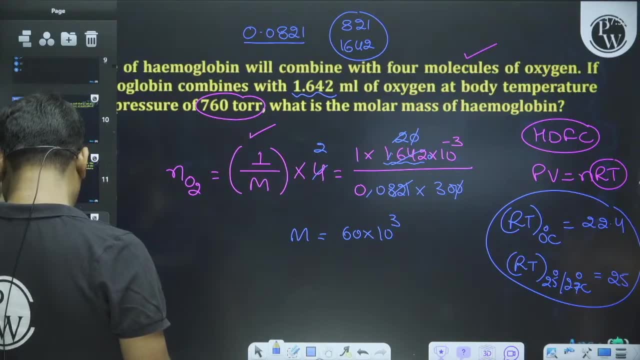 But it is a good question, children. It is a question to come. Let's assume it can come Now. you can see the answer Come. we will do genuine checking once by giving a good question, By giving a good question. 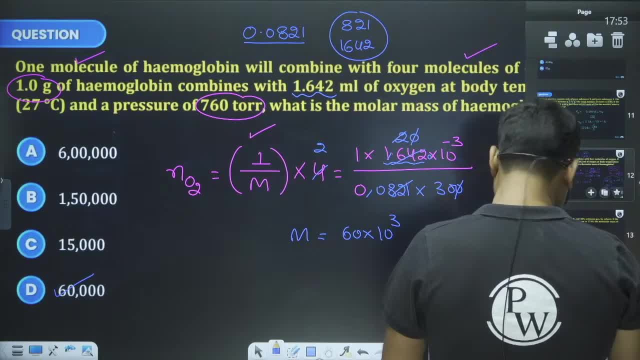 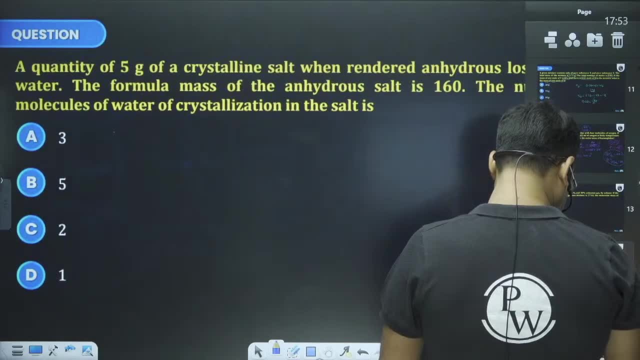 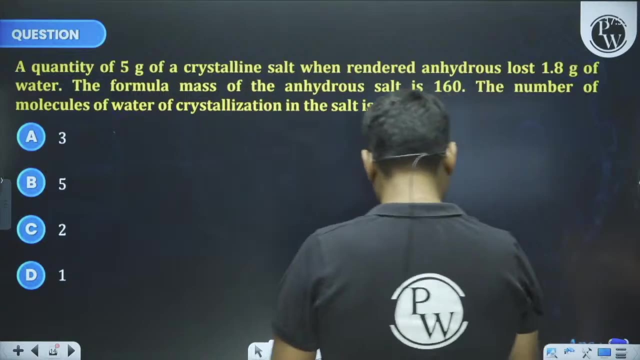 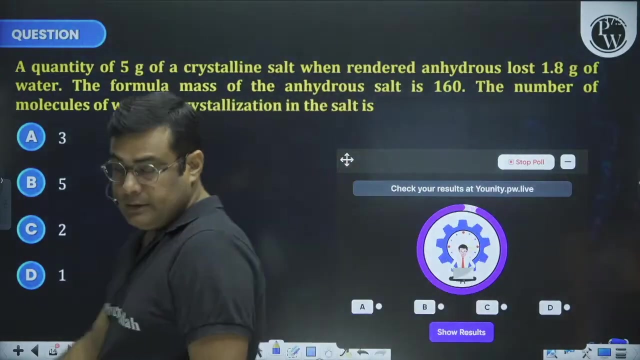 a genuine attempt will be made. Come on, tell me And come. if you are fast, let's see. I am giving time of 45 seconds. Let's do one last question, the poll one, Quickly so that we can proceed towards the next chapter. 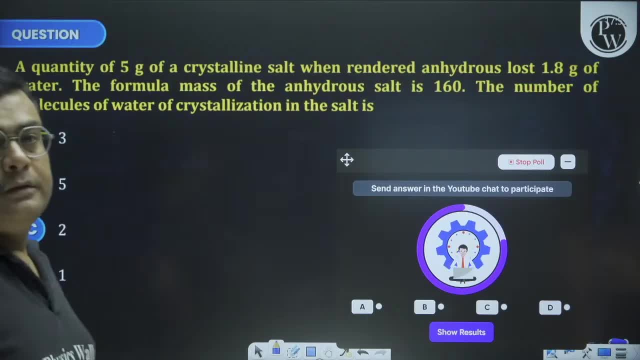 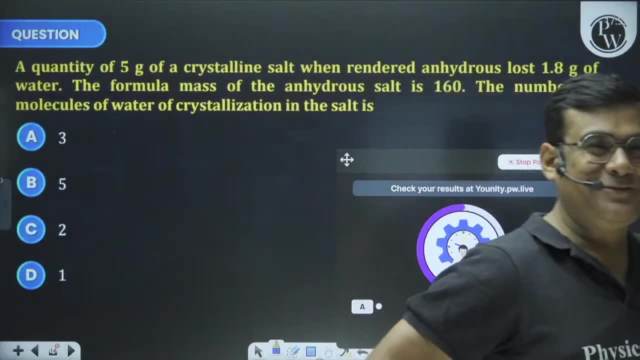 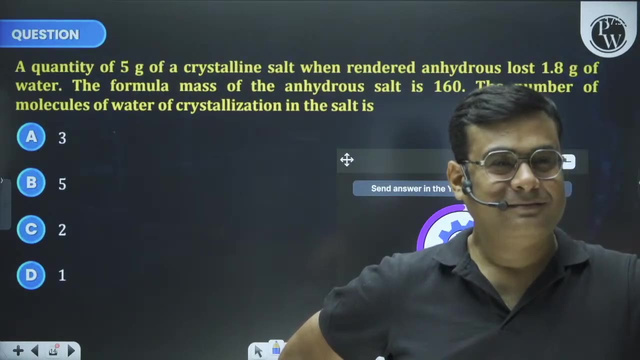 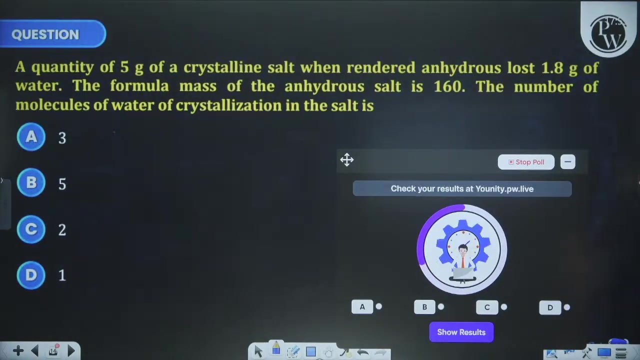 keeping in mind the time. Now all the answers are gone from here. There is a good question. He also said: Sir, we saw it. This is the answer. Yes, Sir, you have written in your text. say it again. 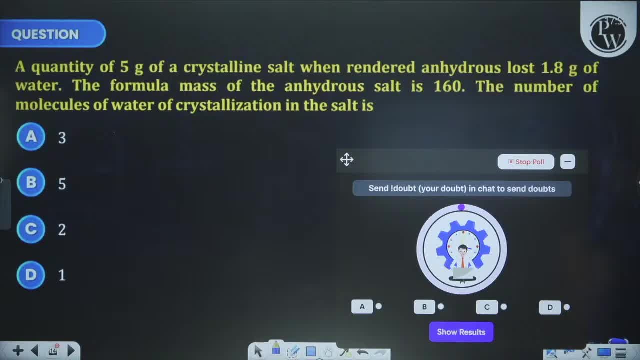 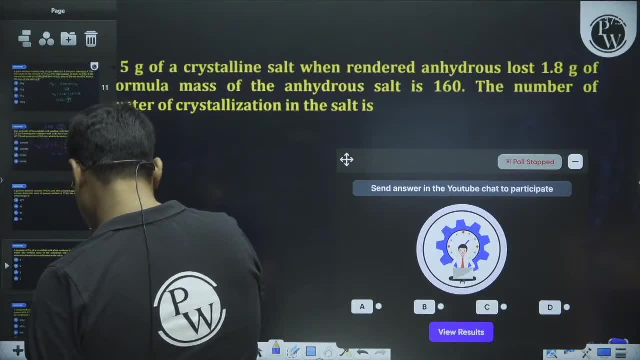 That is the answer. This is the answer. He also wrote yes, Can we think? and how? Yes, Sir, he also wrote yes. Then he wrote: I forgot what I said. I forgot what I said, But it was correct. 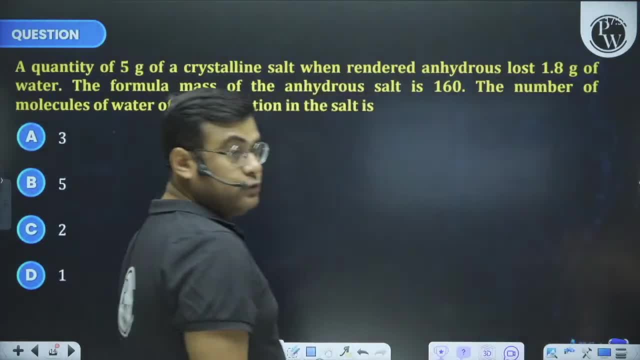 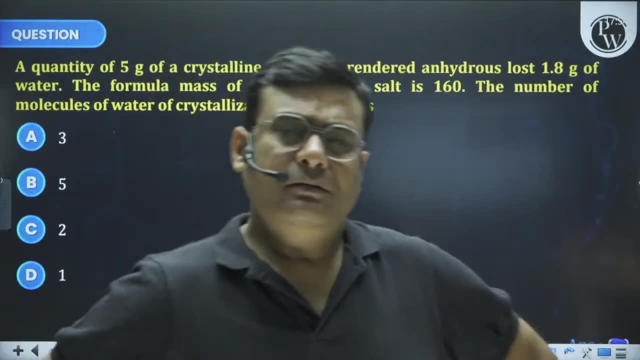 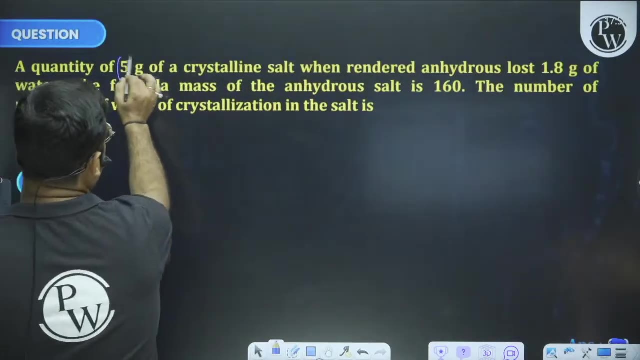 but it was correct. It was correct. I think it was correct. Now, if you want to learn how to do this orally quickly, then you will do the normal one, but if you want to think of a way to do it quickly, then you have to put a little mind. 5 grams. 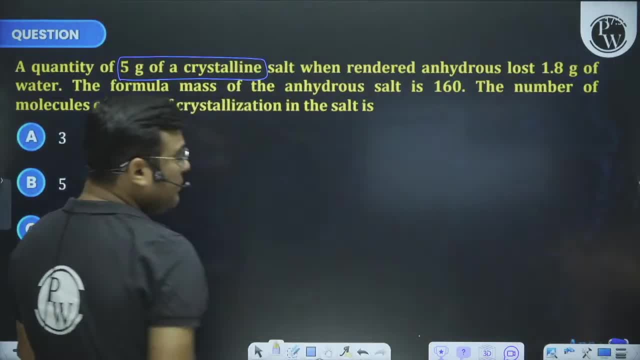 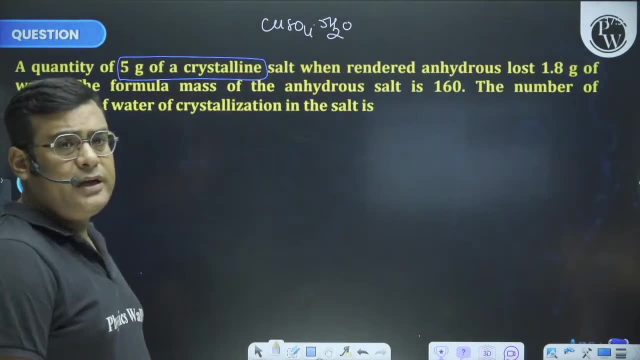 of crystalline salt. we all know that CUSO4.5H2O is blue vitriol and when it is heated it makes the water of crystallization loose. so 5 grams is, when rendered anhydrous, lost. 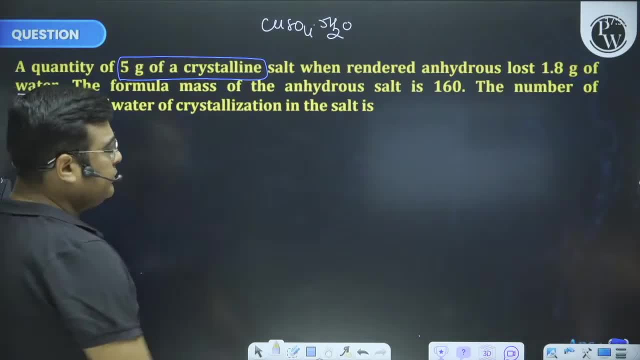 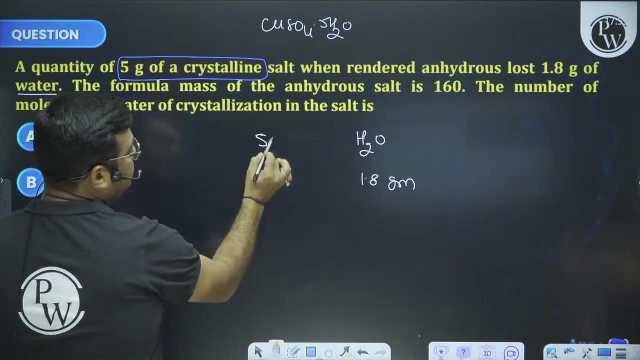 1.8 grams of water. what does this mean? what is water? water is 1.8 grams, so that means anhydrous salt. how many grams will be its weight? 3.2 grams, can I say, or not, that's. 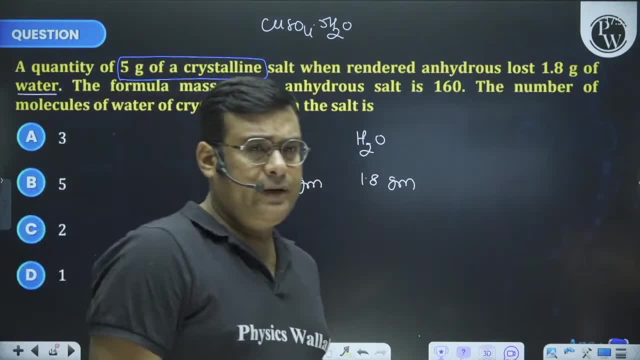 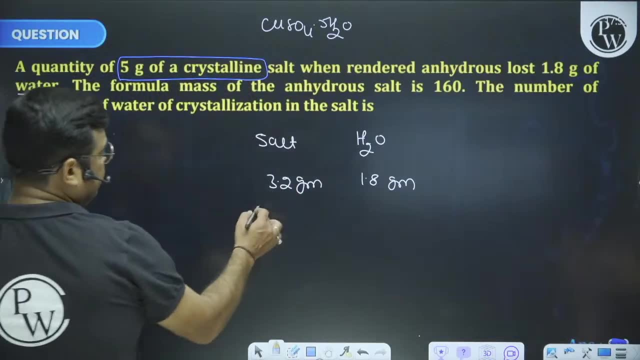 why the total of 5 grams of both was made. put logic instead of the old approach, if you learn to put logic. Now. he is saying that if the mass of anhydrous salt is 160, then if there is 1.8 grams for. 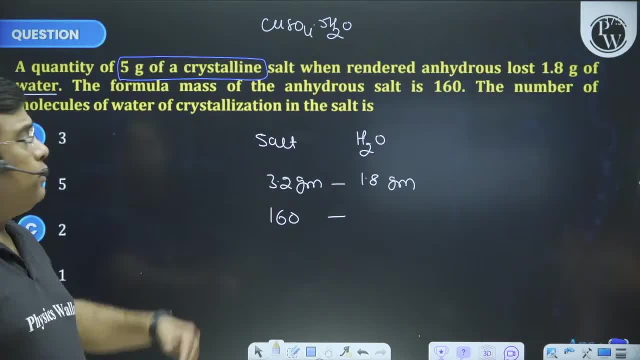 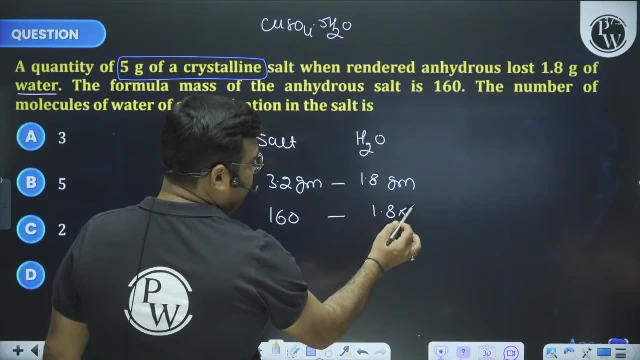 3.2 grams, then how much will it be for 1.6, that's it that will make you molecules of water, of crystallization. what do we do in such a question, sir? 1.8 unitary method into 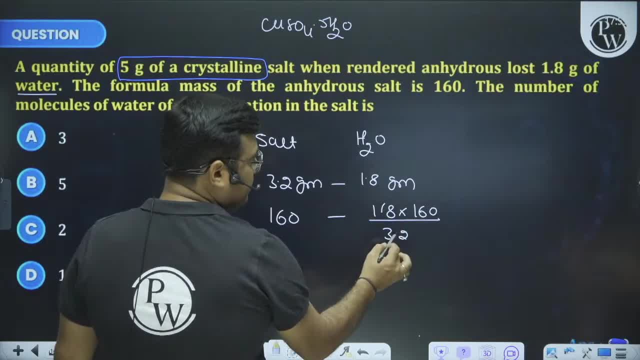 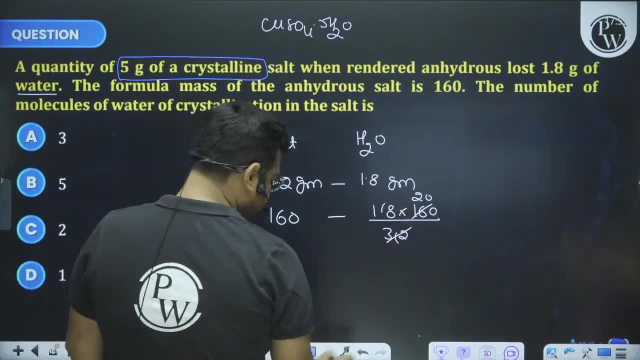 160 divided by 3.2, the decimal decimal you just said. make the same place and finish. so the total of 5.8 grams. it is done from 32, 325060, which means that if there is a water, 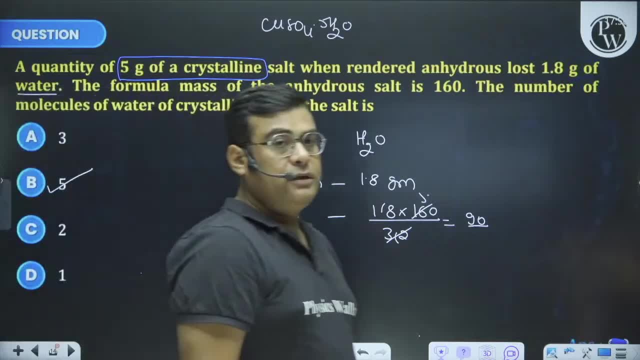 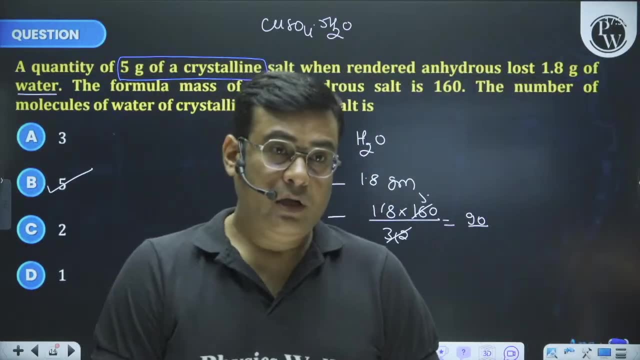 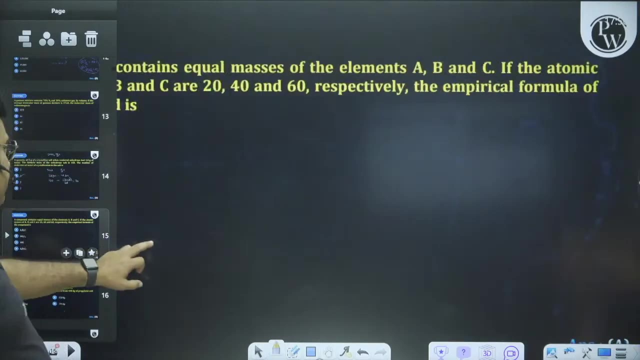 of 90 grams and the water molar mass is 18, then we are 90, sir. if divided by 5, then if you divide 18, then How many molecules are there in the water? 5 molecules like this. then in some other questions I will tell you better. now I am going to tell you that. 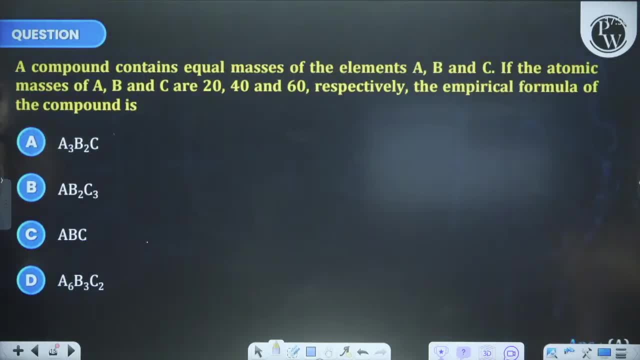 the answer is visible. you just keep watching your money. the rest, I will tell you that Rest, your honesty is with you- that you read the main question and see the answer, whether you are feeling or not. Compound contains equal masses of the elements, ABC. 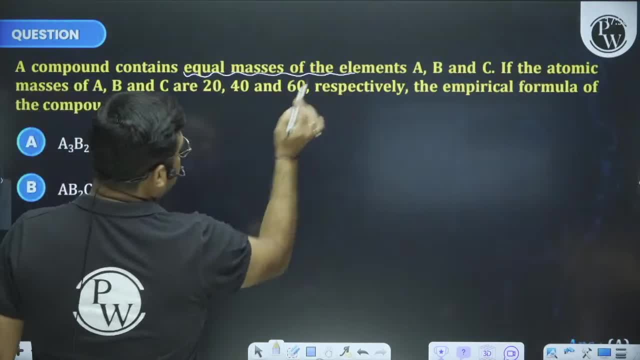 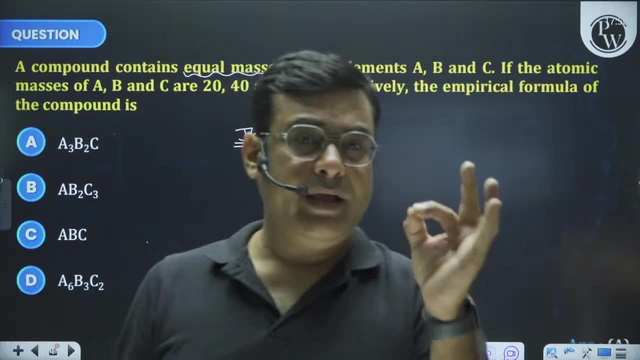 Condition given equal masses. Now I have kept this question to tell my JSC. I have seen in JEE mains that children many times questions of equal masses have come. Many times questions of equal masses have come And I am giving you a question of equal masses from today. 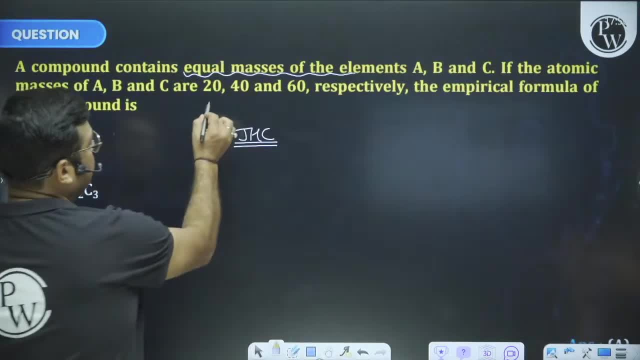 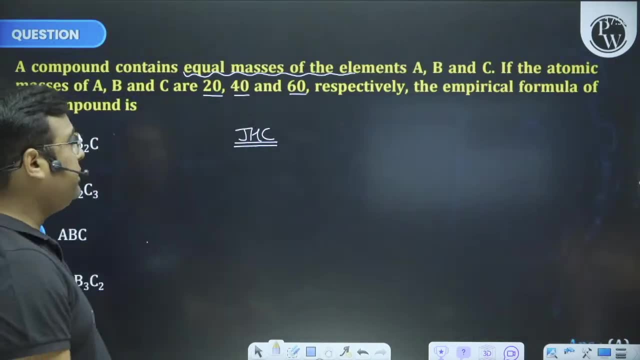 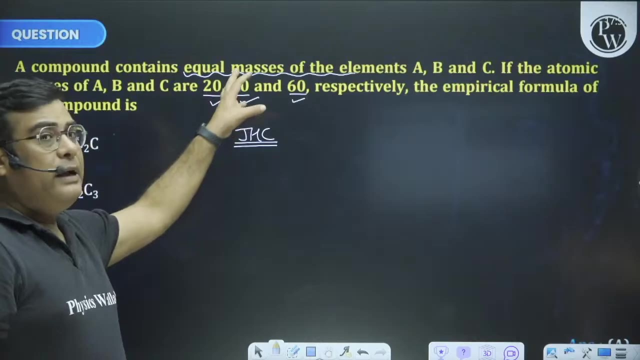 If the atomic masses of ABC are 20,, 40 or 60, what education are you going to give, sir? What education are you going to give of equal masses? I am going to give this education In equal masses. children, the atomic masses you will always see will be like this: of multiple types. 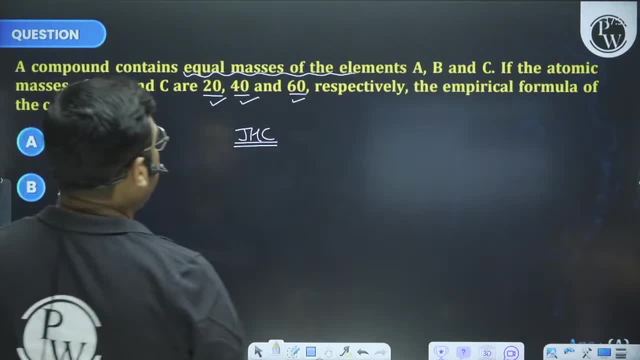 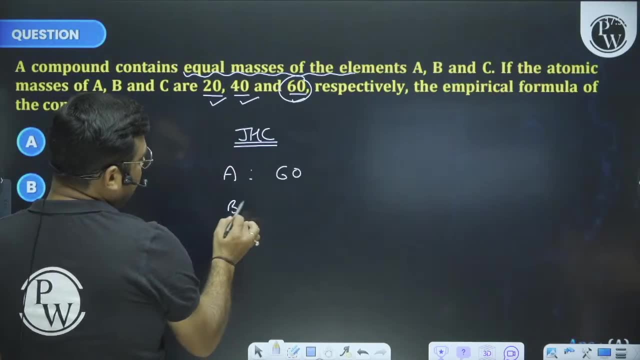 So the rule of this is that the largest atomic mass is 60. You assume that you have ABC, A also has 60 grams, B also has 60 grams And C also has 60 grams. Consider the highest molar mass. 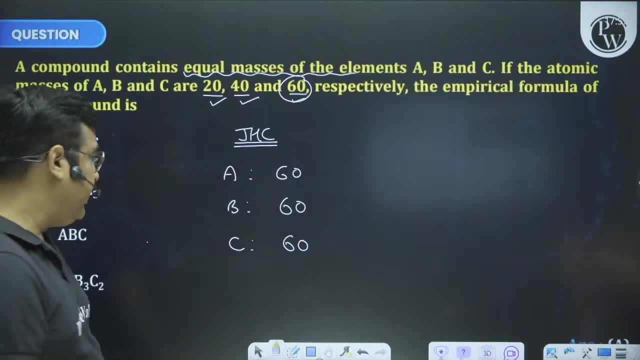 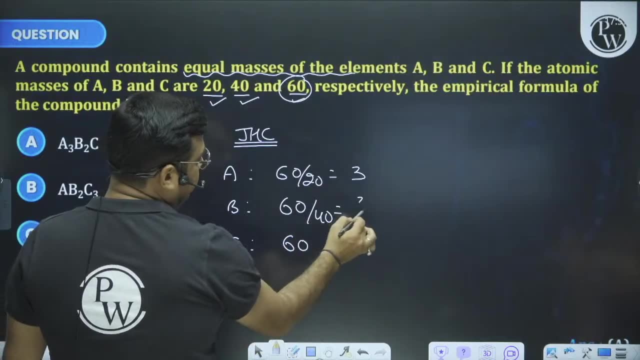 Because for the empirical formula you only need the ratio of atoms. So if A has 60 grams, then 60 by 20 means 3 atoms. 60 by 40 means 3 by 2. And 60 by 60 means 1 of C. 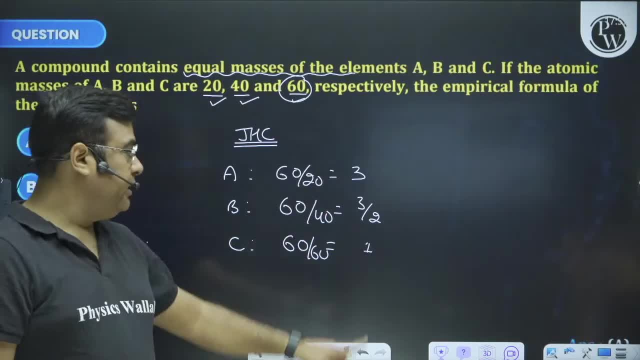 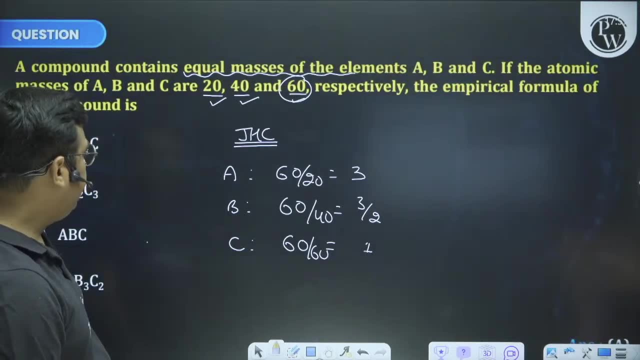 Now, brother, for the empirical formula. the atoms should always be integer. This is in the fraction Multiply by 2.. Right, So 60 by 40.. 3 by 2.. Multiply by 2.. So A is 6.. 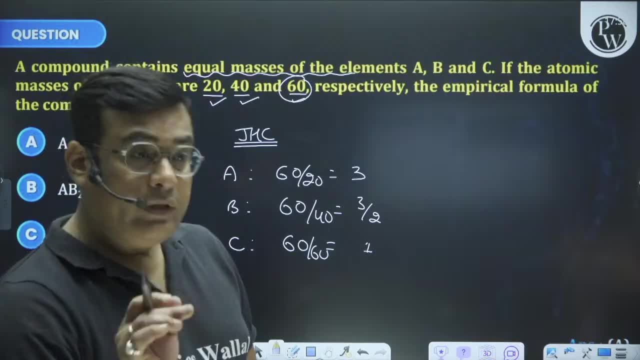 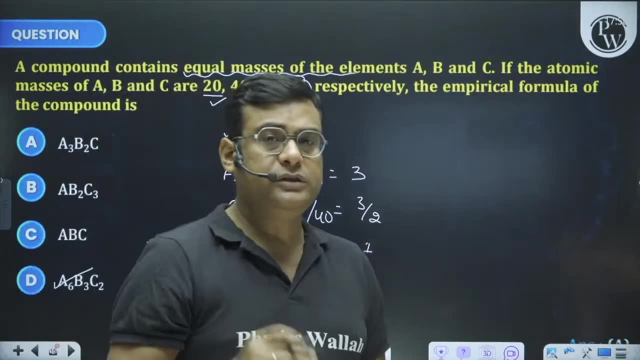 B is 3.. C is 2. Will be my answer. So this is a good JSC. Be sure to keep in mind everyone. Whatever question comes with equal masses. I have been looking at JEEK papers for 23 years. 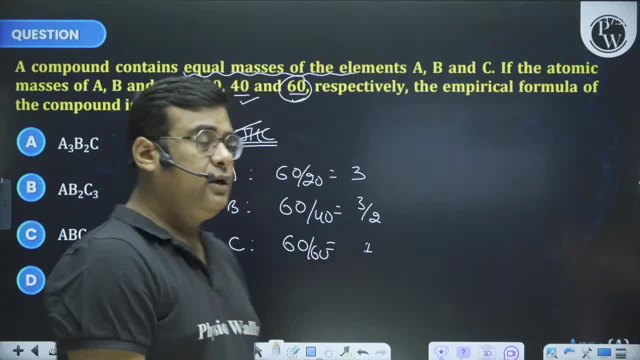 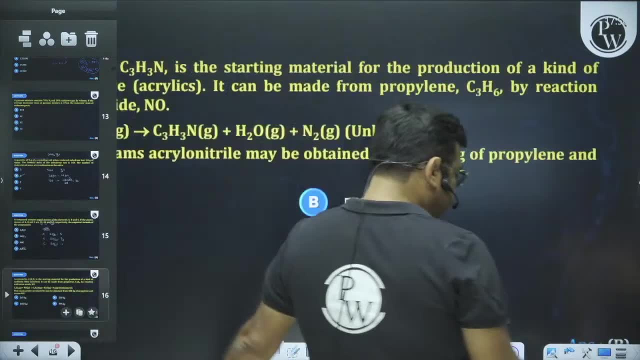 In them. he will normally give the same cases, son, whose molar masses are multiples. You can solve their trick in this way. OK, Come on, The next question is coming in front of you. This is also a good question. 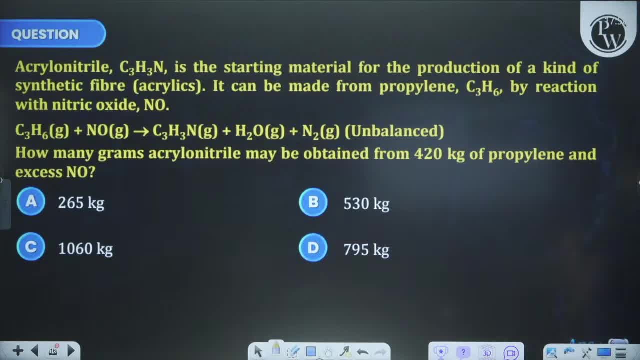 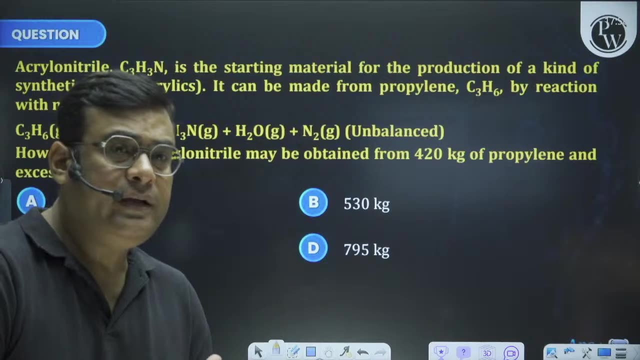 Let's see, And then we will take permission from you to move towards redox. This is also a good scary question. We can get the base, Sir. this is not equal. What is not equal, Son, I did not understand. 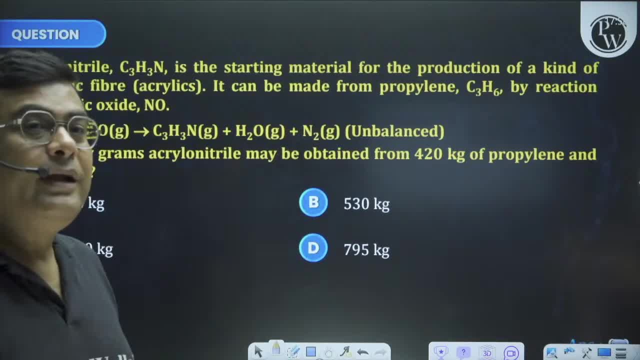 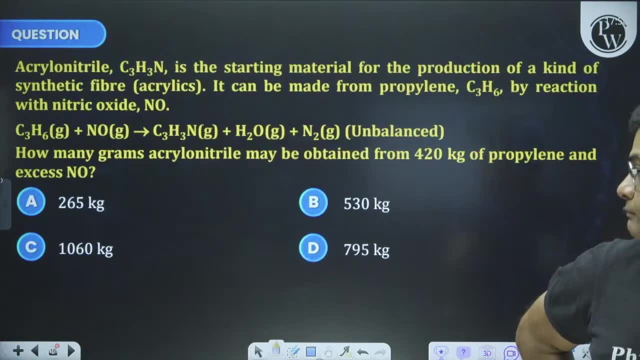 Did you see, when a person had a cramp in his anus- Son, I see this after a long time- People were saying it has turned. but when they saw it, son, What he is saying, See, the question is good. Acryl onitrile, which you hear in your organ, in which the name ki3 H3n is the static material. 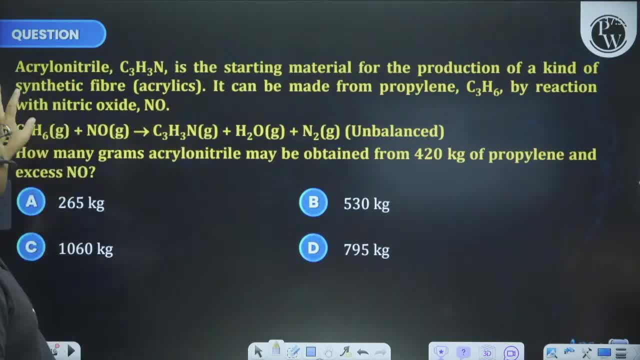 for the production of a kind of synthetic material, What of a kind of synthetic fiber acrylics? It can be made from propylene by reaction with nitric acid. NO, C3H6 plus NO gives you C3H3NH2ON2 conditions. The reaction is unbalanced. How many grams of acrylonitrile obtained from 420 grams of propylene- excess of NO? I just want to know if I need to balance the reaction in this question. What was the concept in the previous question? The concept in the previous question was that there was equal mass. 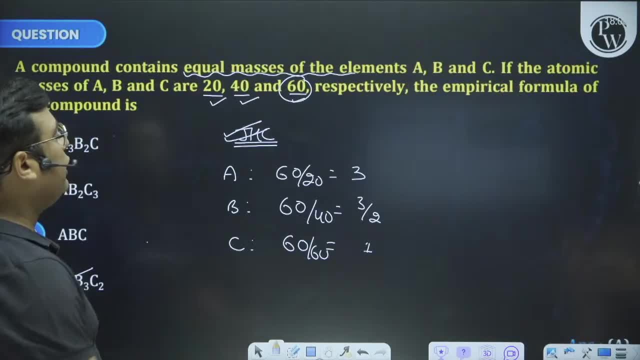 If there was equal mass, then take the larger molar mass- 60- because everyone has equal mass. I can take as much as I want. I took 60 grams of all three. If I divide the given mass by its atomic mass, then I know the number of atoms. 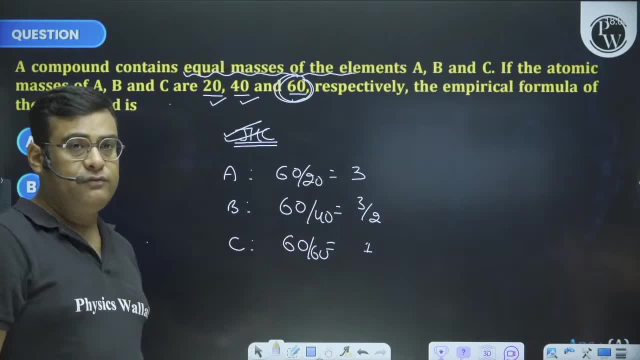 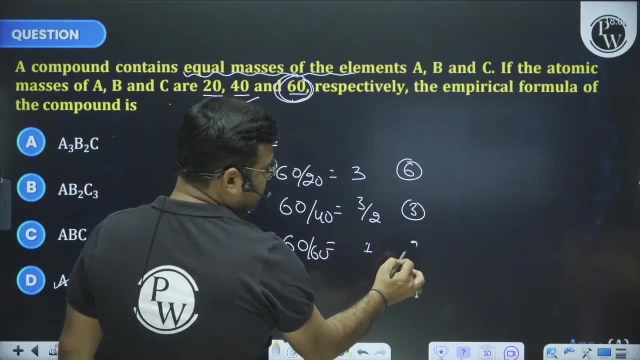 60 by 23,, 60 by 43 by 2,, 60 by 61.. Atoms should always be integers. To make an integer, I multiplied it by 2.. This is 6,, this is 3 and this is 2.. 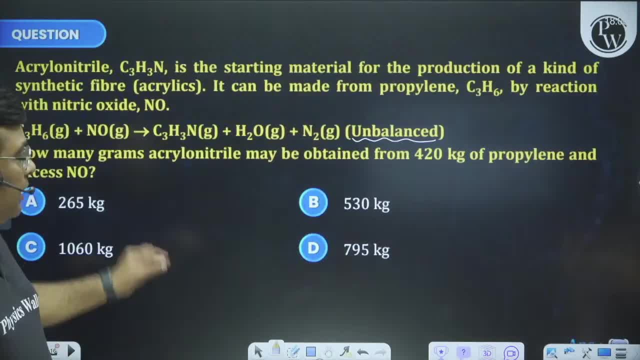 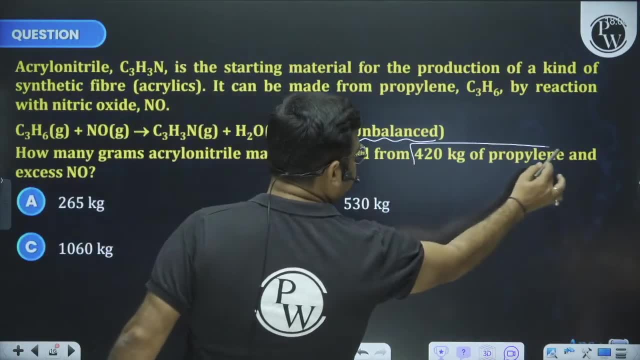 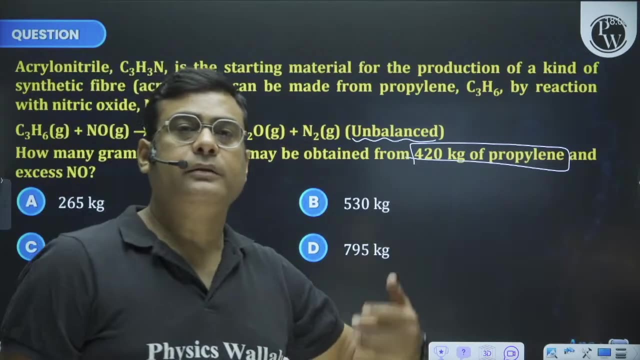 That was the concept. Now, in this question, I want to explain to the children that the first thing is that there is no talk of limiting reagent, because it has given you the amount of a single reactant. The second thing is that some children may have put it in reaction balancing for a minute. 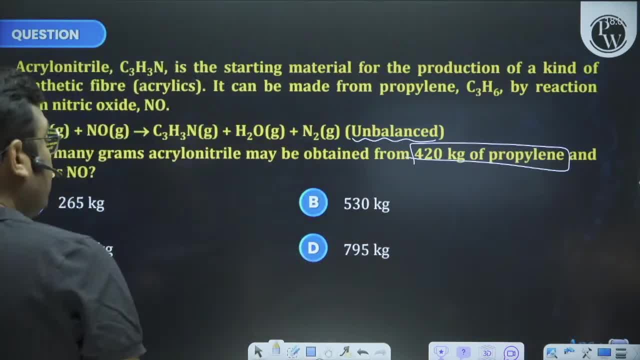 There was no need to balance the reaction. Why not? Because propylene means C3H6.. And who was asked by the children, C3H3N? I hope so. I hope you must have heard the name POAC. I hope you must have heard the name POAC. 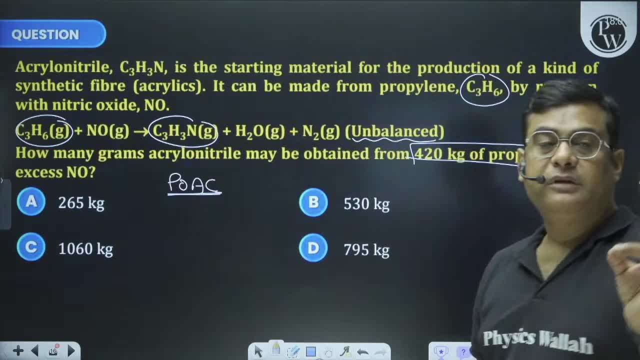 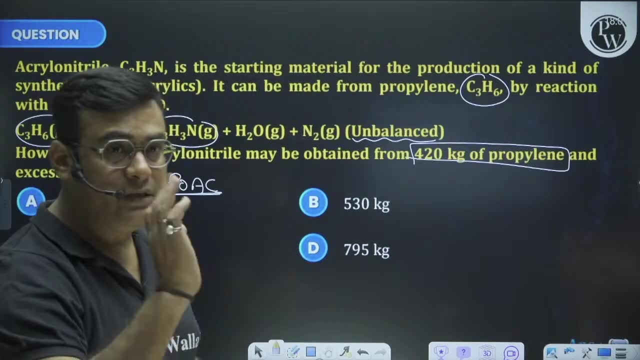 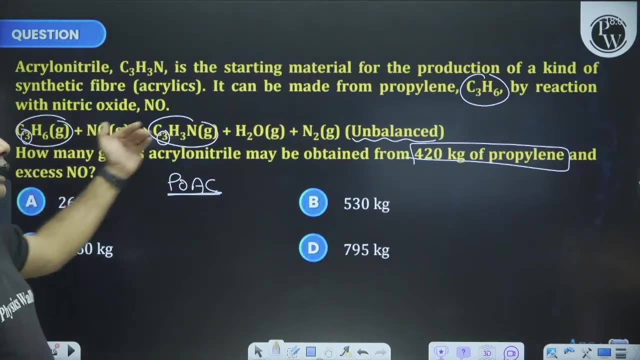 POAC means Principle of Atom Conservation, Principle of Atom Conservation. POAC means Principle of Atom Conservation If there are three atoms of carbon here, even if nitrogen is not balanced, There are three atoms of carbon here as well. Carbon has not gone anywhere else. 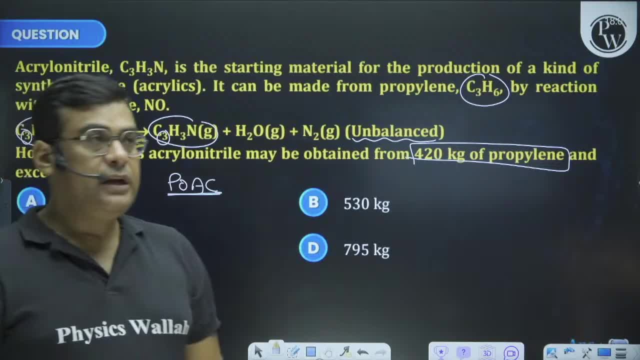 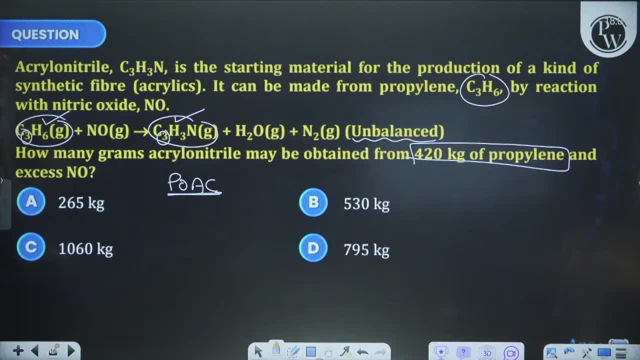 So this means, This means. This means The amounts, Because the atoms are equal on both sides. The amounts of this substance will be the same as the amounts of this substance. The amounts of this substance will be the same as the amounts of this substance. 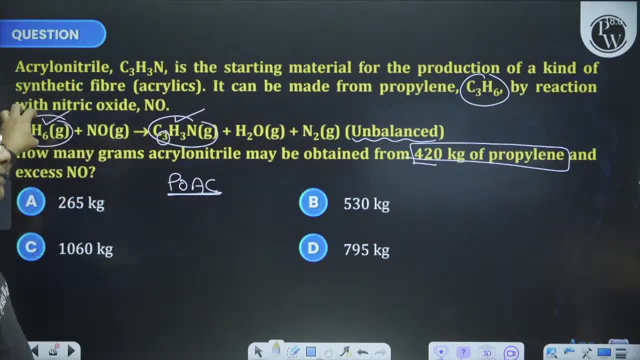 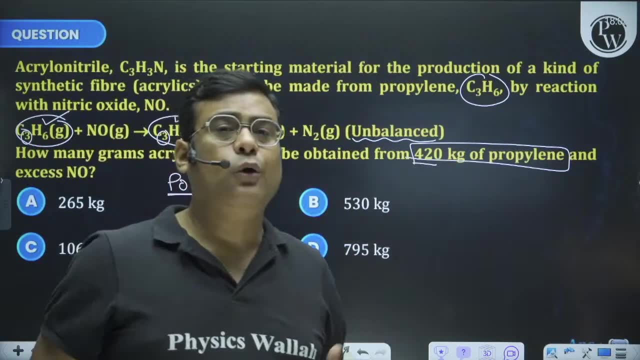 So if it had 420 kilograms, It had 420 kilograms children, So its amounts will come out of its amounts. Now, if we try to run our mind a little further, Isn't it Because JEE wants to check your mind? 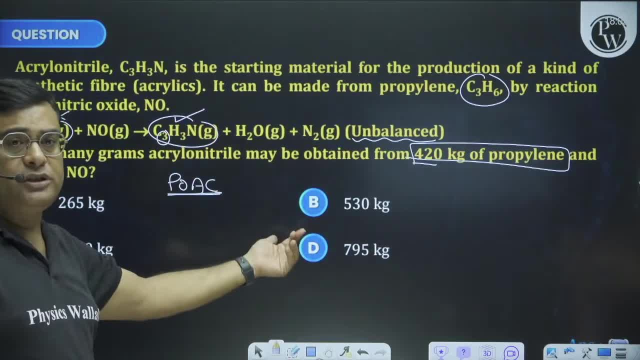 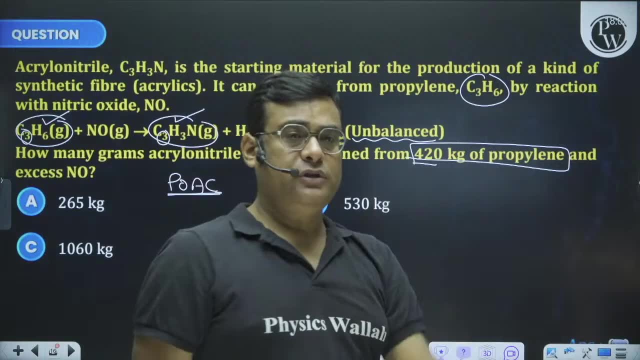 Okay, So I will do it too. I will do the balance too. Everything is there. You may be understanding that GCPT approach throughout the year from the beginning. I am trying to learn the approaches a little bit. So, brother, Brother, 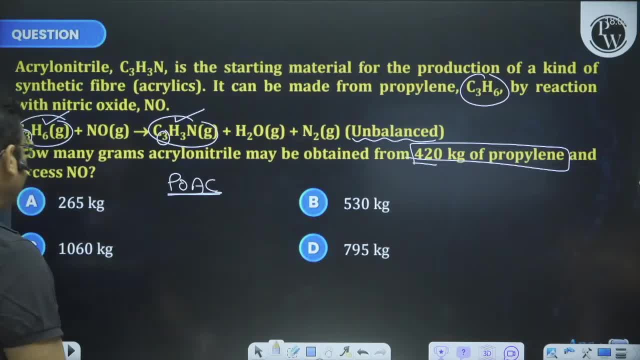 Brother, Brother, Brother. I want to say that I have to get the amounts from this, Obviously. Now, what was six in this? What was six, Sir, hydrogen. In that, hydrogen became three, Nitrogen became one, Means its 420 grams. 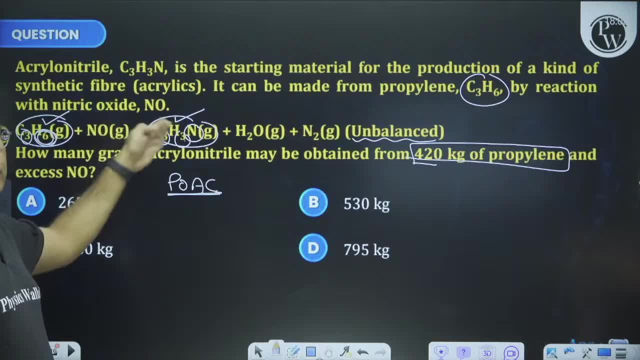 Brother, its molar mass is slightly larger than that. So what will happen to the mass Brother? its molar mass is slightly larger than that. So what will happen to the mass Brother? Listen, what will happen to the mass. 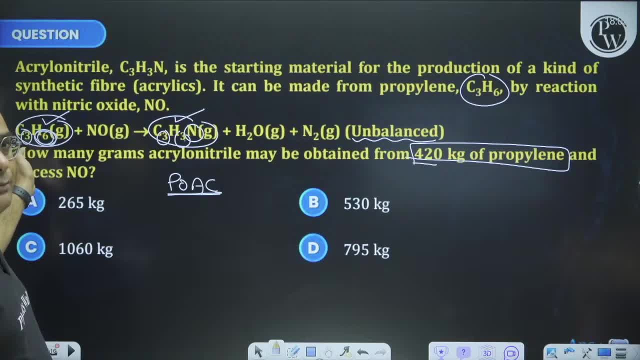 Children. it will increase a little, Isn't it? It is not doubling Its molar mass. There was a decrement of 3 here 14.. 3 has gone from it. An 11 jump has happened, Isn't it? 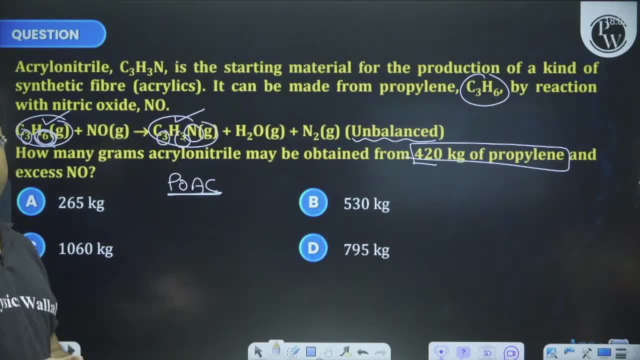 So there is an 11 jump in the total molar mass. There is an 11 jump, Doesn't it? Isn't it doubling? Then, brother, it was 420. So there is a slight jump in the molar mass. So even in its mass, a slight jump will come. 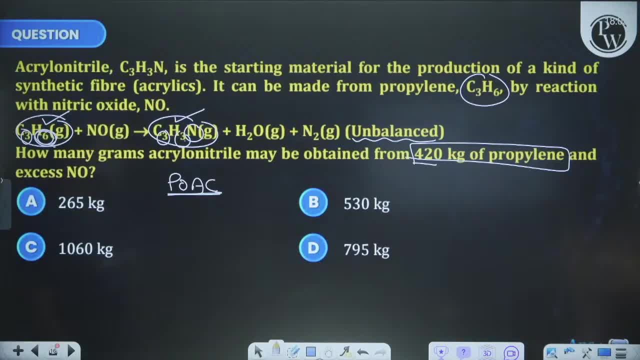 Which will be straight: 530.. There is no chance of doubling, There is no chance of more than double. Now take this. Have you done any of these? See, this has happened. See, this has happened. This has happened. See, this has happened. 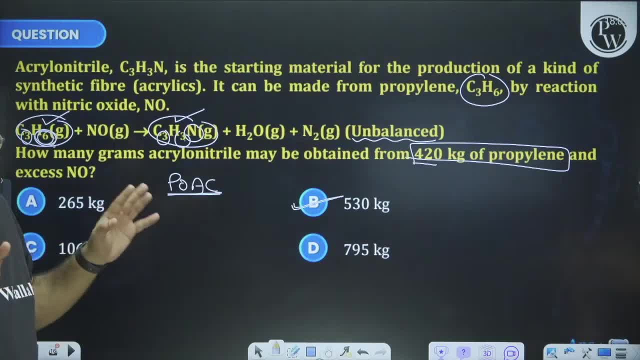 double to jada hone ka koi chance nahi hai. ab jinko, ye logic is tere. se nahi samajh me aata wo kar sakte apna bilkul, sir ki 420 by 42, or into sir molar mass se 53. 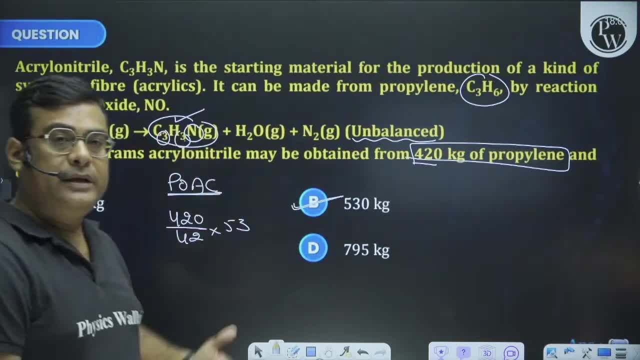 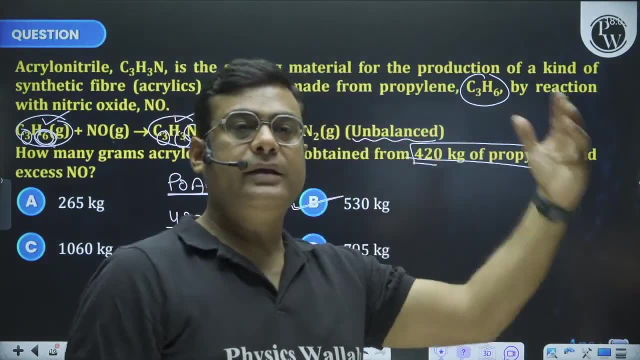 kar do, maine bhi wohi kara hai, but maine aapko bhaiya, maine aapko sikhana bhi chaaro ki thoda bot, thoda bot. aap agar apni tarike se bhi sochogay. 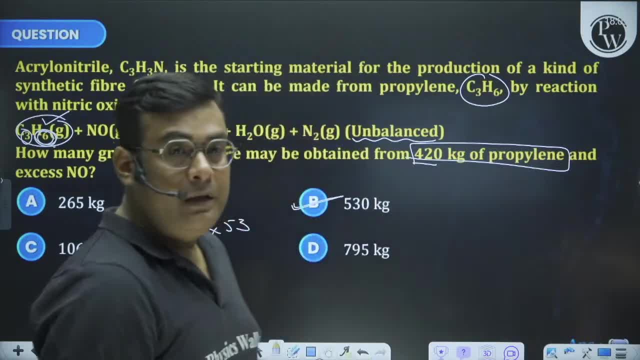 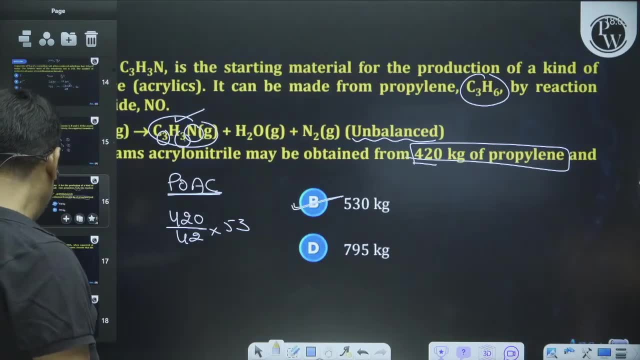 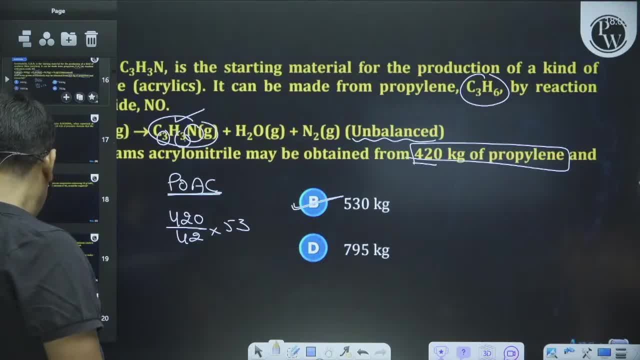 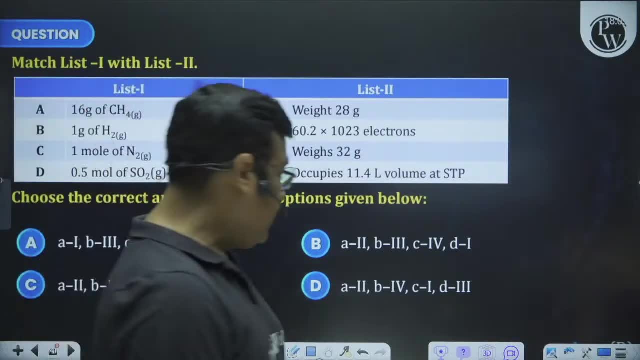 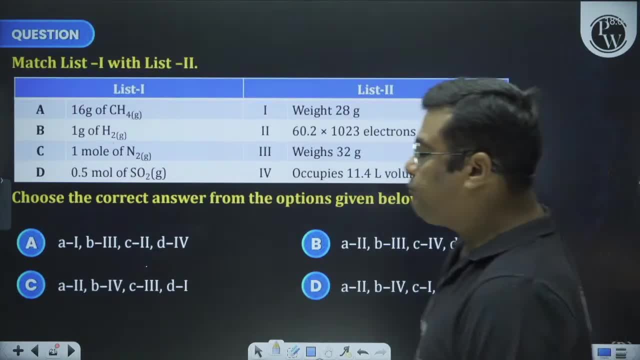 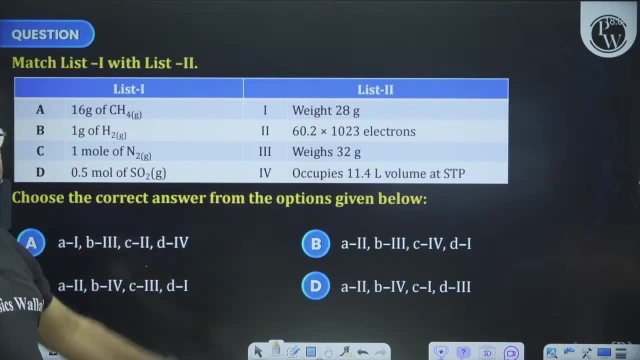 ab yeh aapka jayi ka hi purana question hai. ab isme kya hai, ki ham log ek ek option ko nikal kar apna samay khoti karte, aur mai chahata ho ki bhaiya aap apne brain ko apne. 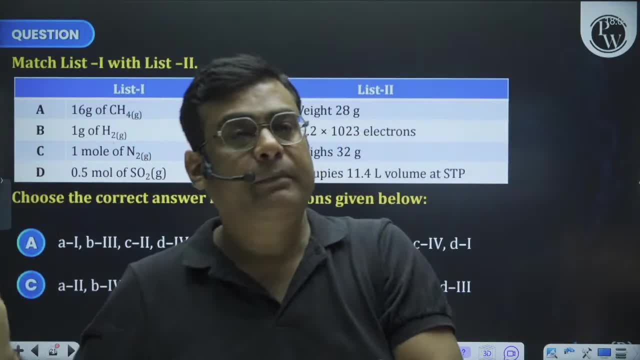 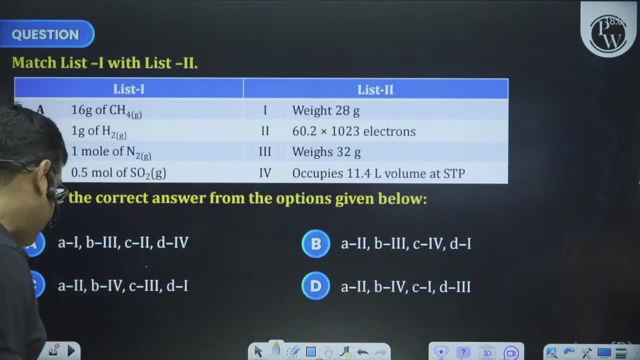 jab exam dene ja rahe hain, to usse please, ghar ke kamre ke locker me band karke na jaye usse apne saath lekar. jaye usse aap, please, apne saath lekar. jaye kyunki, agar aap usse saath leke gaye. 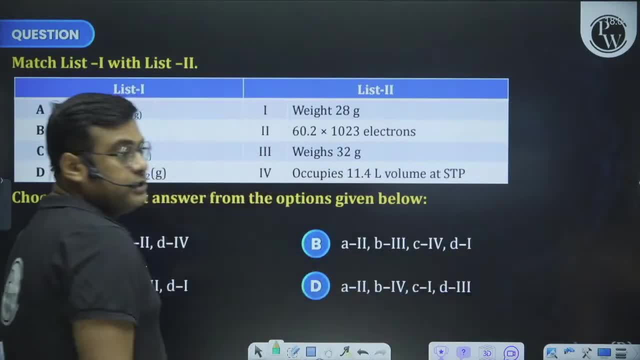 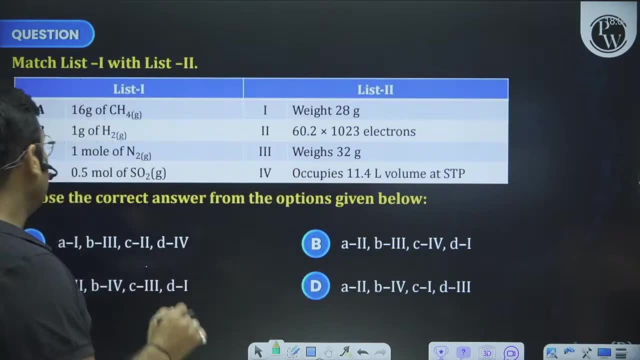 to ho sakta. aapke jo total 90 question, aare 13 is subject lagbagh 5-6. question to shayad brain: se hi solve ho jayeng kaise, sir? kya kena chaaro isme mass hai bachchon. 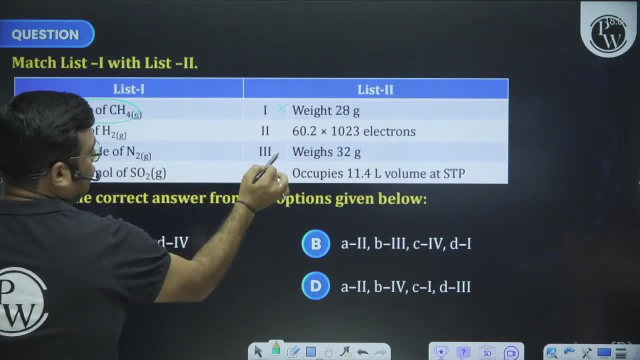 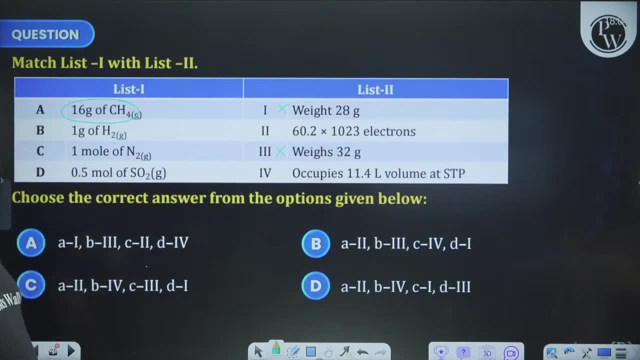 16 gram to. obviously mass ka answer mass wala to ho nahi sakta hai. mass ka answer mass wala to ho hi nahi sakta hai. ha, ya na mass ka answer 2 ya 4, me se hi koi hoga 16 gram CH4. 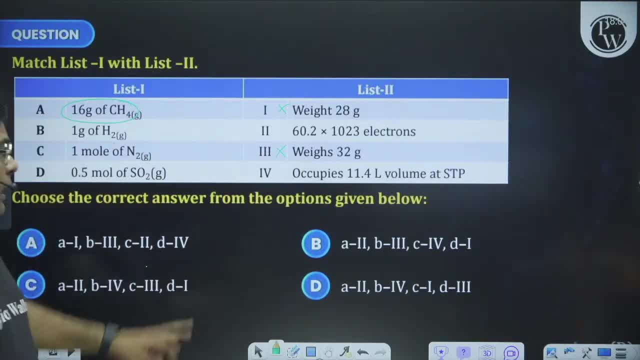 mujhe dikhi raha: saap saap, sir, ek mol hai. ab ek mol ka volume to bhaiya STP par kitna hota hai, sir, 22.7 ke aas paas hota hai. to ye to nahi ho sakta. 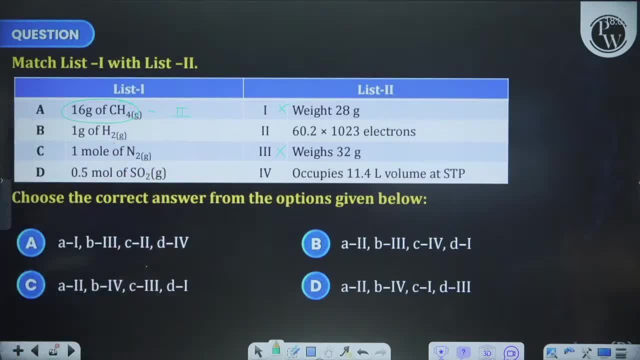 matla a ka pakka answer ho gaya. 2 a ka answer pakka ho gaya. 2 sir, ye to 3 jagay match ho gaya. koi baat nahi hai? na, koi baat nahi, beta. ab dekho 1 gram of H2. 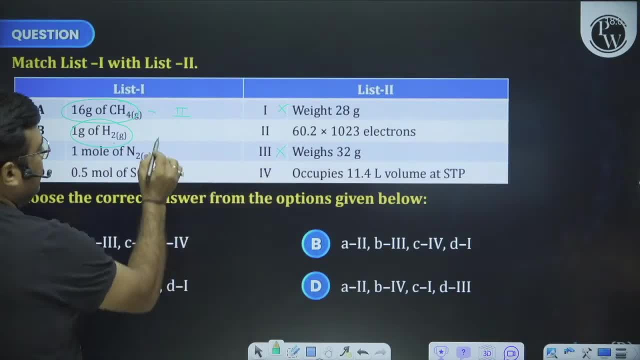 wapas in ka ye dono nahi ho sakta hai to b ka answer pakka. ab aapka 4 hi hoga b ka answer 4. sir, ye bhi 2 jagay match ho gaya 1 mol N2. ye jayi ka question hai, bachchon. 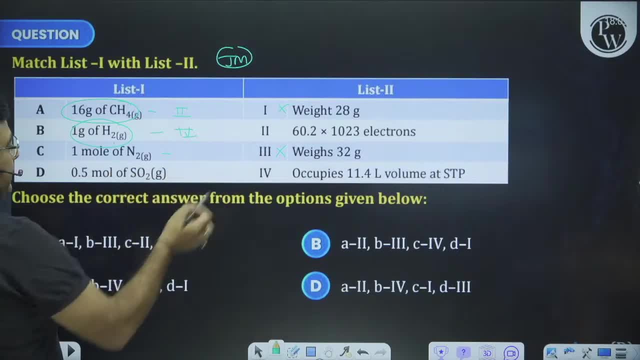 bata de raha ho 1 mol N2 in dono me mol se to mass. aega aapka answer 4: ab N2 ka mass kitna hota hai, sir, 28 to 1 ho gaya. matlab aapka answer ho gaya. 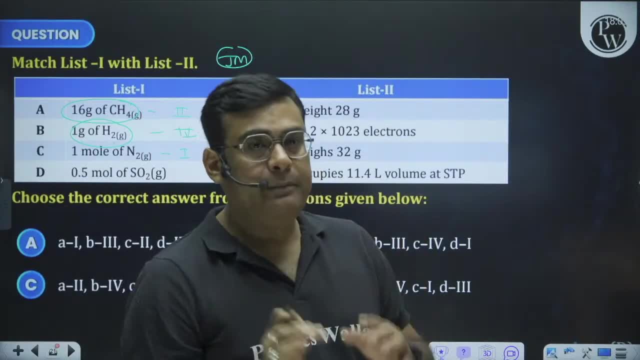 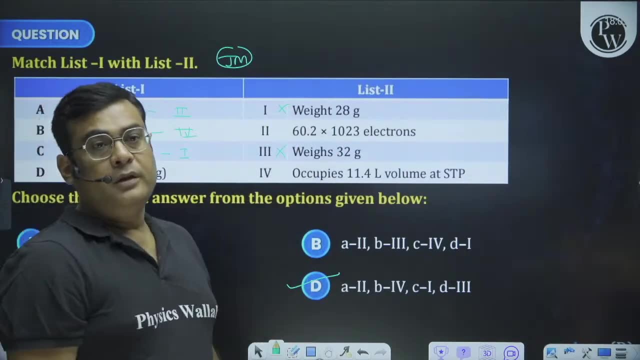 siddhe D to ab me ye samjana chaara ho bachchon ki might be. might be. hum mese kuch bachche 16 gram of CH4 me electron calculate karna chalu kar gaya hota hai na ki 16 gram CH4 me. 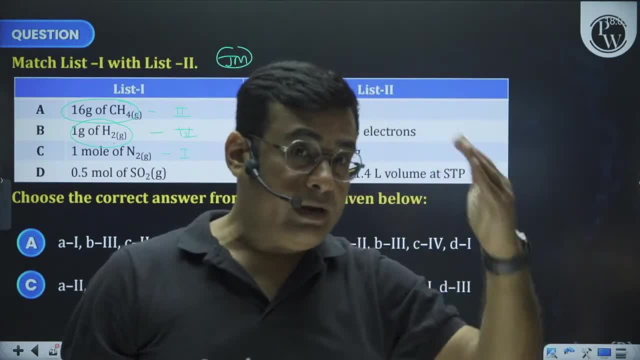 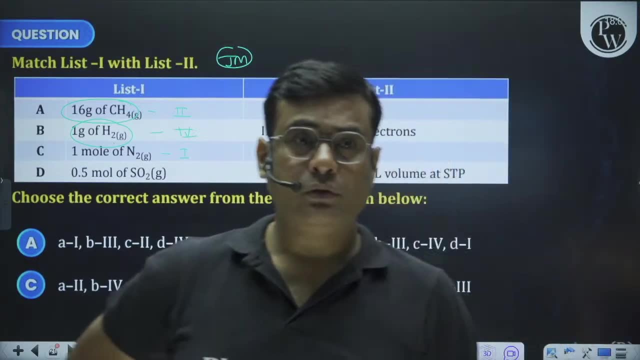 electrons kitne hai, wo solve karna, chalu kar diya hota aur kara hoga. bachchon, kuch bachchon hai. ya, abhi aap mana bhi kardo, ki nahi, sir? nahi sir, main to aap se bhi tej hoon. 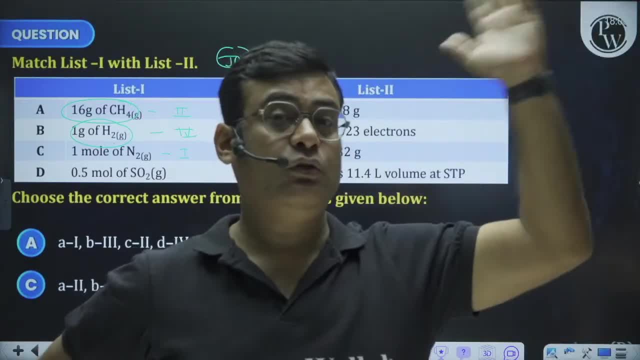 hai na main to aap se bhi tej hoon, sir, main to aesa karna makta hi nahi, sir, mujhe to us Brahma ji ne Param Pita Paramatma ne hai na us Param Pita Paramatma ne antar shakti de rakhi hai. 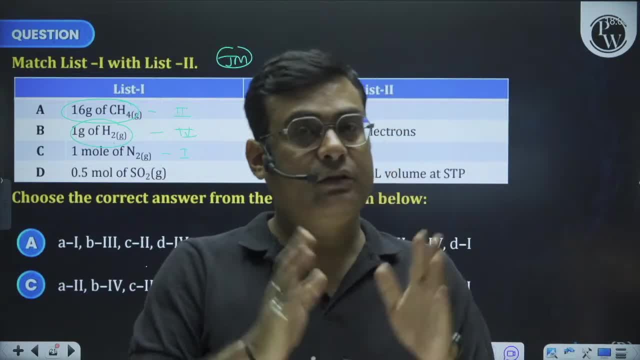 main usse se check karta hoon. theek hai na main usse se check karta hoon. to bhaiya pehli cheez me bata du, abhi aap bhale kuch bhi bol do exam ke pressure me. 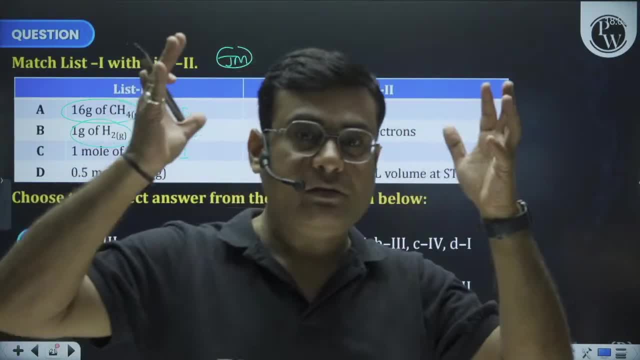 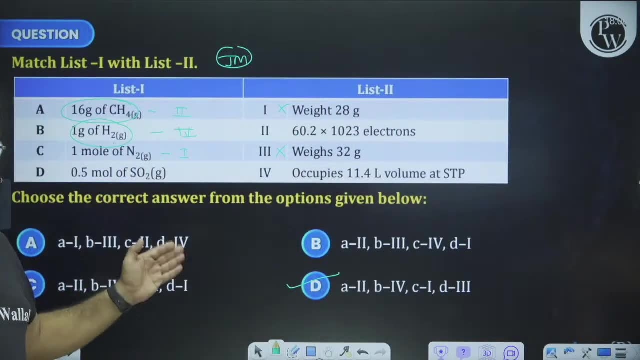 wapas aapki ye approach aahi jaati hai isle hame is mind ko mentally prepare karke jaana hota hai. then ha is mind ko mentally aapko prepare karke jaana hota hai isle, isle in cheezon ko. 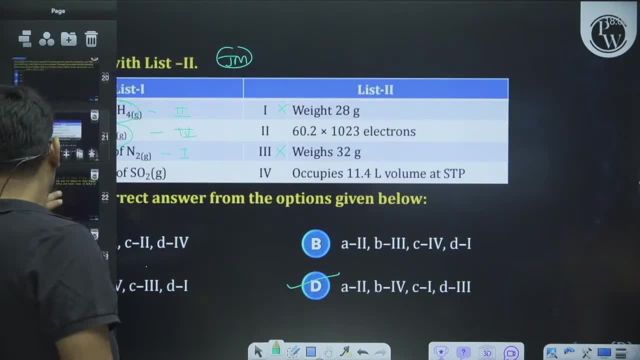 jaroor sochte samashte. chale, chale ji, bachon is asha ke saath ki mol ke ab humne kaafi question kar liye. kaafi question, ma aapko deke bhi jaara hoon, bachon aesa nahi hai. 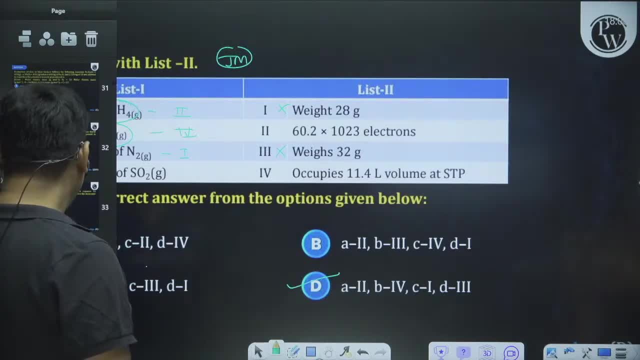 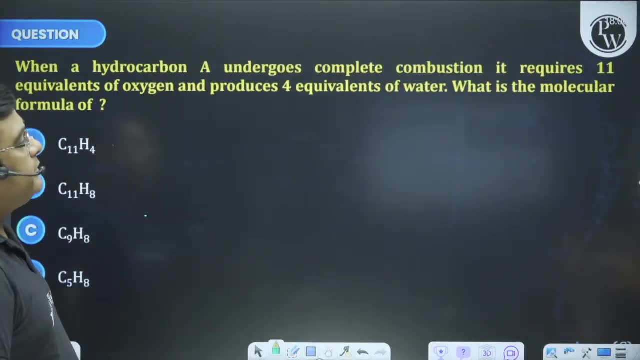 ki ma chhodke jaara hoon aapke liye kaafi saare questions theek na. ek aada question, jese combustion of hydrocarbon ka aur bata du, when a hydrocarbon a undergoes complete combustion, it requires 11 equivalents. 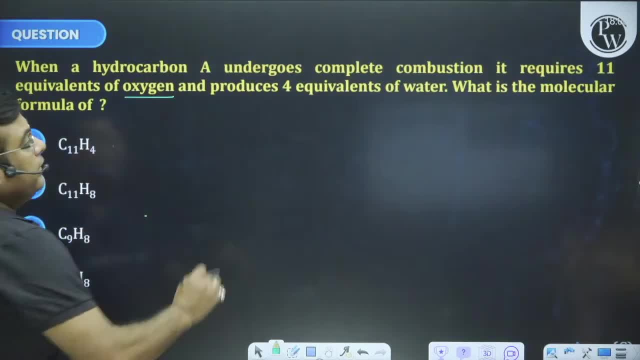 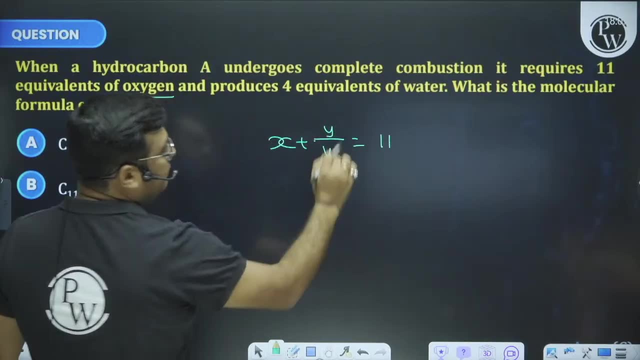 of oxygen ab hydrocarbon ke question. agar aate hai, hain na theek hai 11 equivalents to oxygen ke liye. kya rule tha amara, sir? x plus y by 4 to x plus y by 4, ki value 11 and produces? 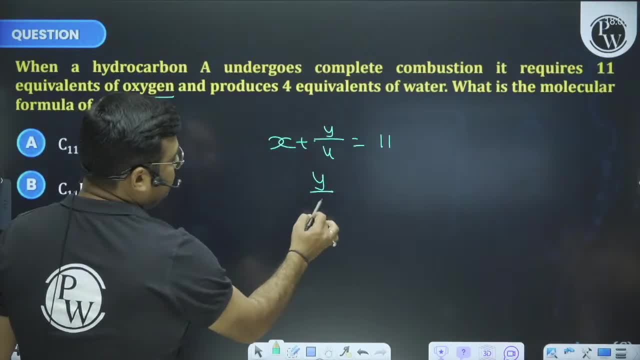 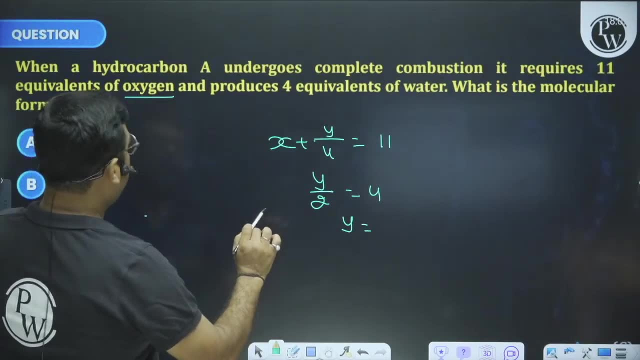 4 equivalents of water. water ke liye kya rule tha? sir y by 2 to sir y by 2 ki value hai, 4 matlab y ki value hoge. kitna kuch garbhar khutala to nahi ho raha hai. 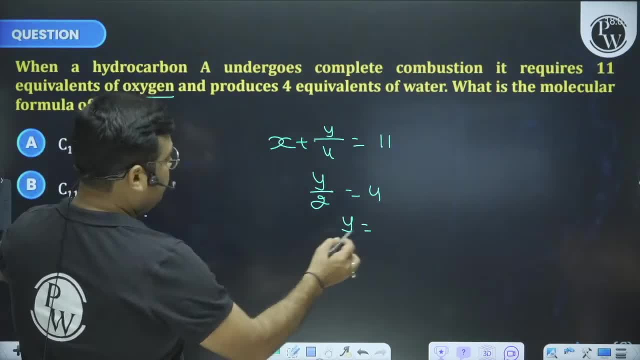 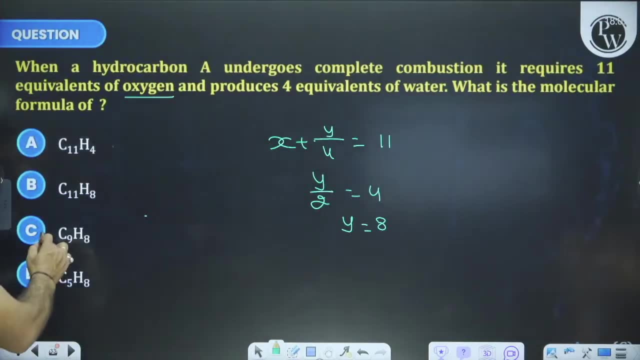 hai na. it requires 11 equivalent of oxygen. theek hai to y ki value hoge bachon 8, ab 8 by 4, kitna ho gaya 2 aur isle aapka answer ho gaya x ki value 9 c 9. 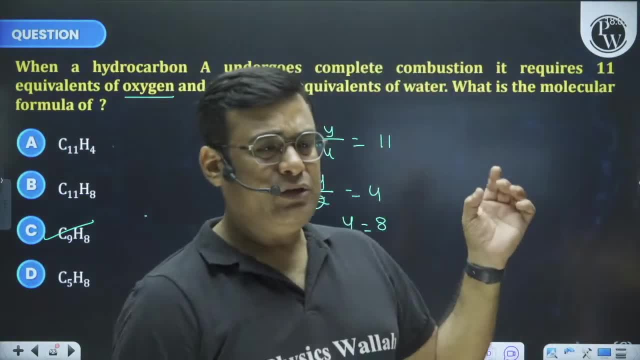 8, so ab, agar aapko hydrocarbon ka- jo abhi maine chote sa ek formula bataya- bachon agar, wo aapko yaad hai, to khat se aapko tick karna hai aur kuch dimaak aapko. 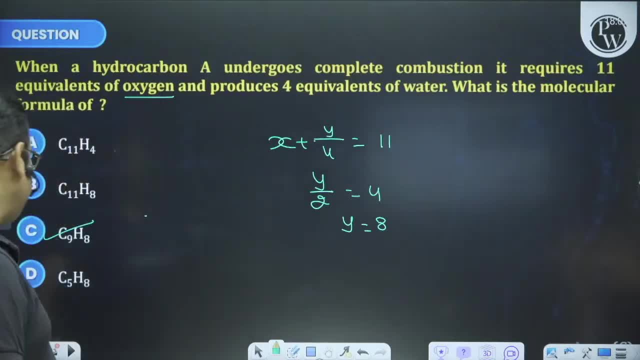 lagane ki jaruat nahi hai khe na aur isle khub bhar bhar ke question hai. bachon ab aap jaru inay ek bar attempt kariye ga ab ham barte hain amare agle, chapter ki. 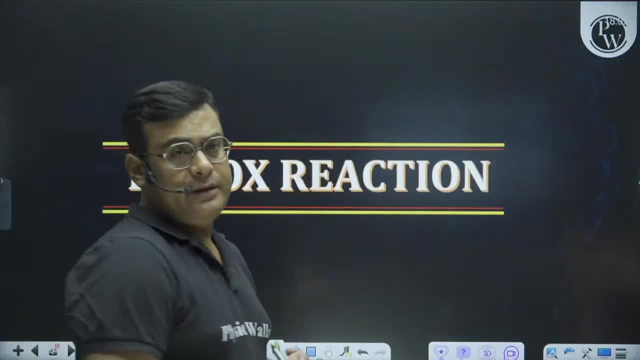 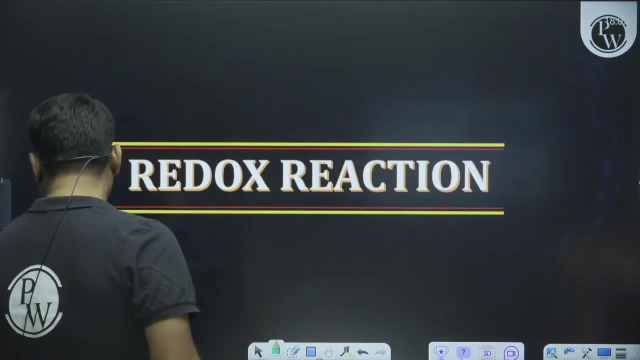 taraf, that is redox reaction, second chapter, humne lagbhag 20-25 question. hopefully maine aaram se aapko bata diye ab redox reaction ki pehle ma kuch aapko tricks bata du jo mujhe. 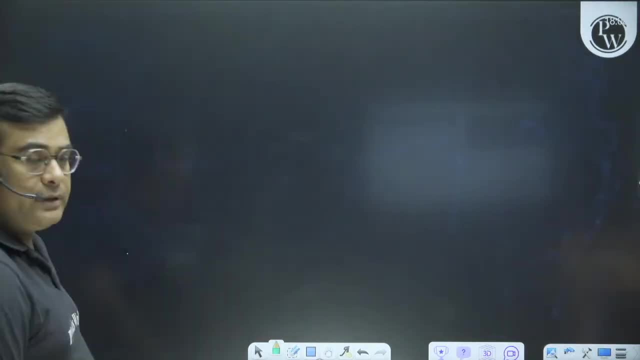 lagta hai, maire important cheeje hai. vo ma redox ki aapko bata du pehle cheez, bachon pehle cheez. which of the following reaction is redox? ya, which of the following reaction is not a redox? 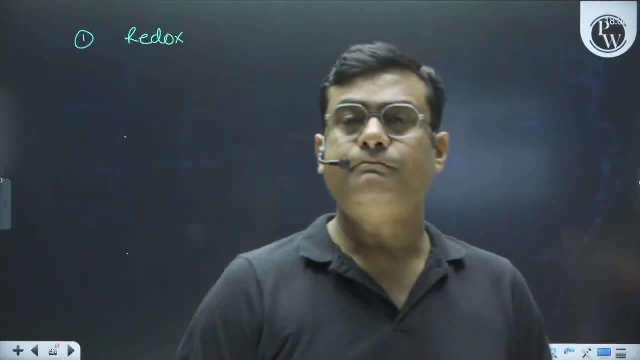 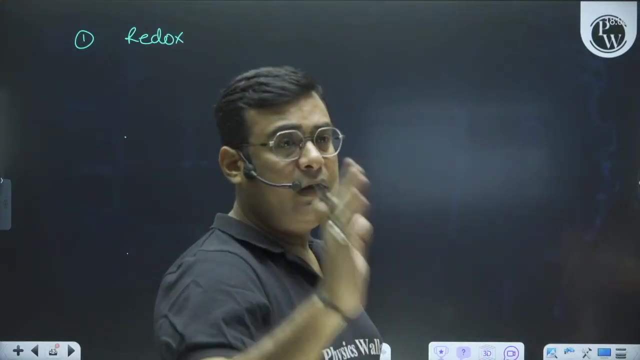 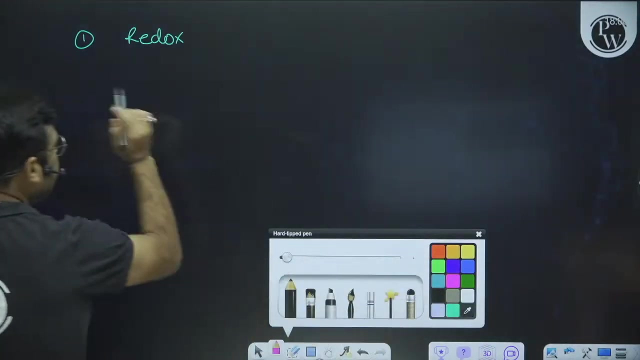 reaction is redox reaction. which is redox reaction? yeah, redox reaction, redox reaction. aapko itni mehatpun siksha dene jaa raha hu, bachon, usse aapka kaam is test dare ke question kata kata ho. 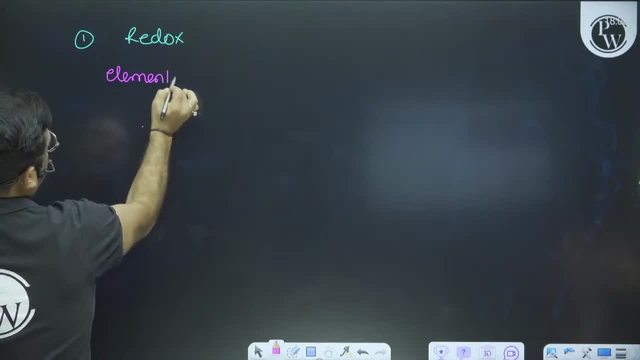 jaa agar element compound me jaa raha hai, aur main dhar dhar ke question bhi dikhau: nga bachon aapko agar element compound me jaa raha hai, bachon, or going to the compound element, the first thing, which is the following: reaction in redox and non-redox. 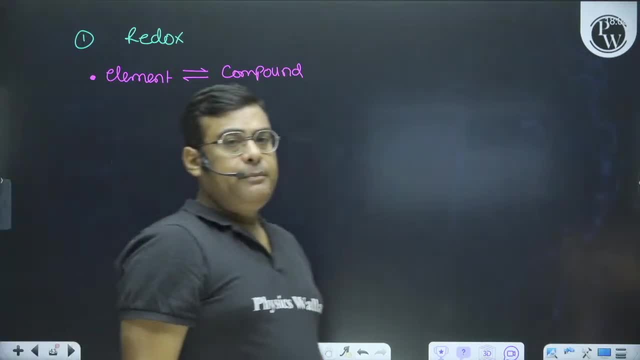 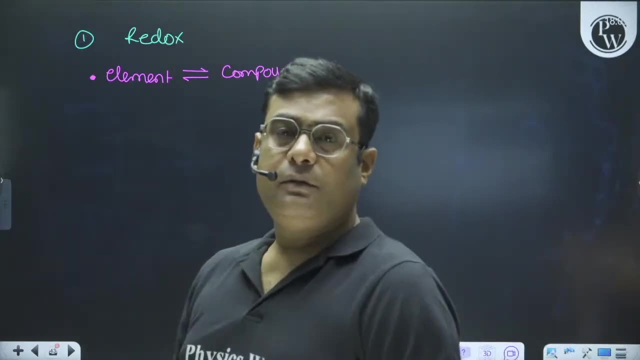 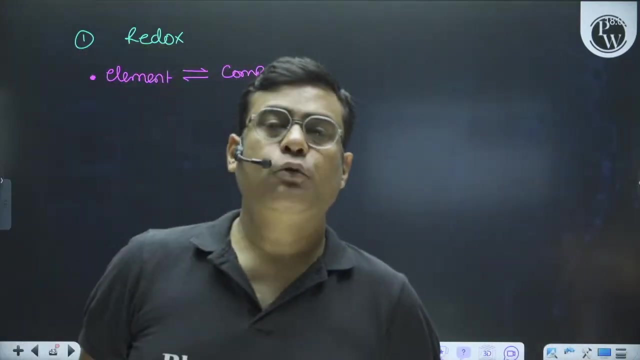 the first thing to see is this: that if the element is going to the compound or going to the compound element, then that reaction is definitely that reaction is definitely your redox reaction. if this is not happening, then you know, you know that you will have to look at the oxidation number with change. 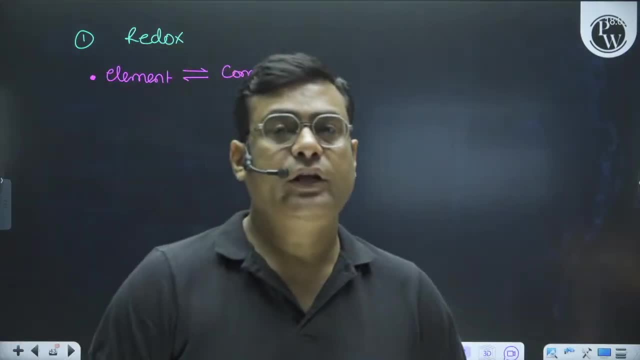 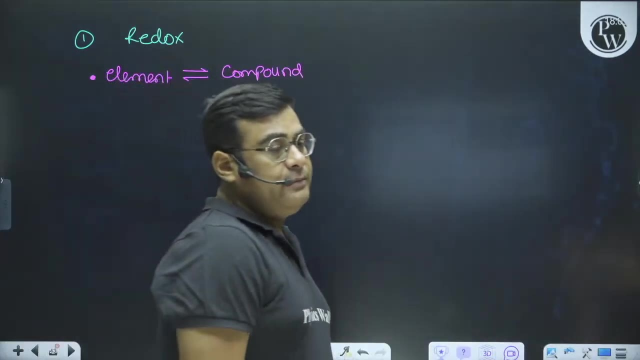 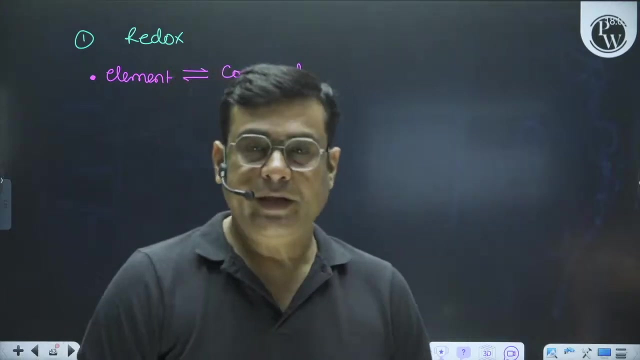 the reaction in which the oxidation number changes. that reaction is your redox. in which the oxidation number does not change. that is non-redox normally. acid based reaction is non-redox. normally, complex formation reaction is also non-redox, is it right? normally. so this is a small trick. 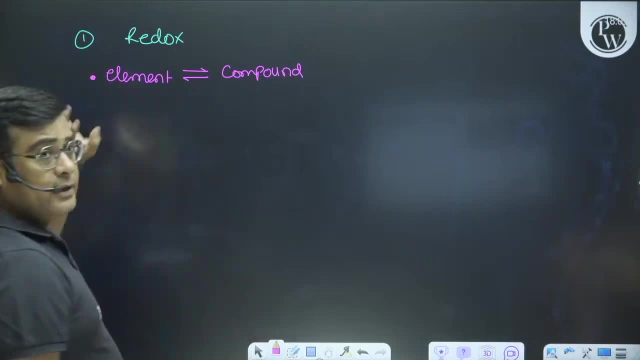 I am showing you in the questions because the JEE one uses it many times. ok, apart from this, tell me the next thing: see what H2O2. we all know that 2H2O2 gives. 2H2O plus O2 means. 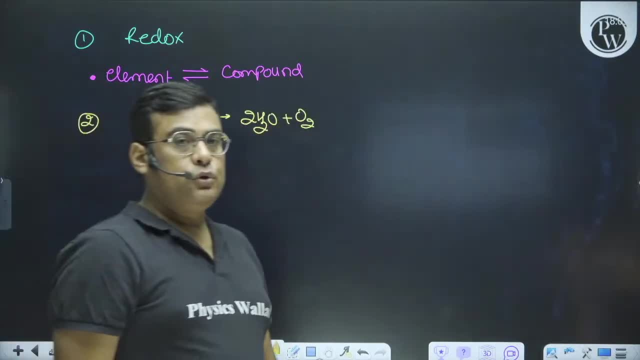 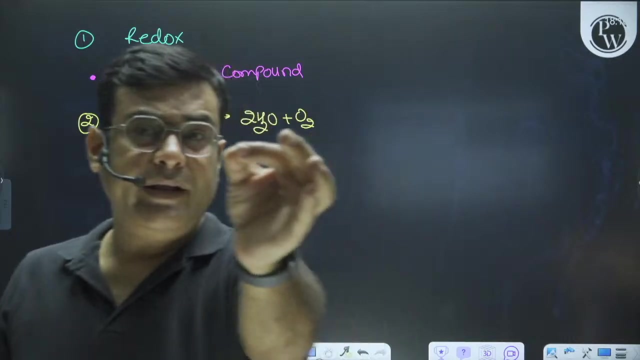 I want to say that H2O2 shows disproportionation. H2O2 shows disproportionation, my dear children, everyone knows. ok, and what is the meaning of disproportionation? it is the favorite question of JEE, above disproportionation. it is guaranteed you are also going to get. 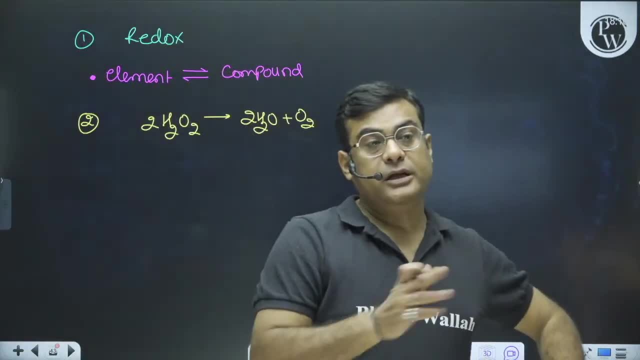 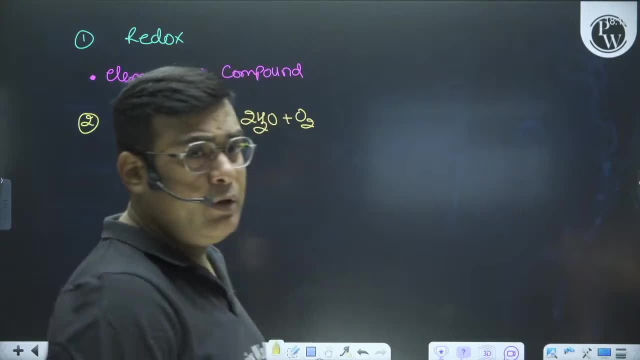 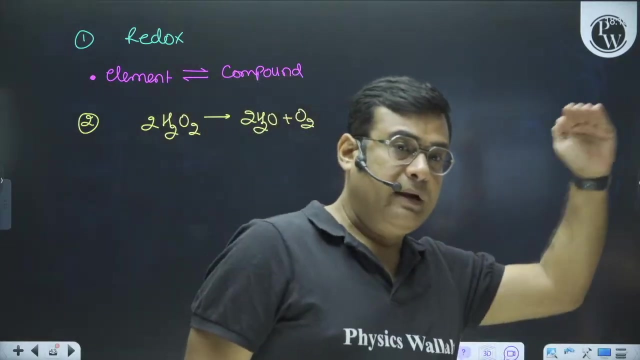 isn't it. it is guaranteed. I am saying it from now. I will not say it with my chest because it may cause you trouble, but, kids, it will happen. what does disproportionation mean? only one element changes: its oxidation number. it increases. simultaneously, oxidation number increases and decreases. 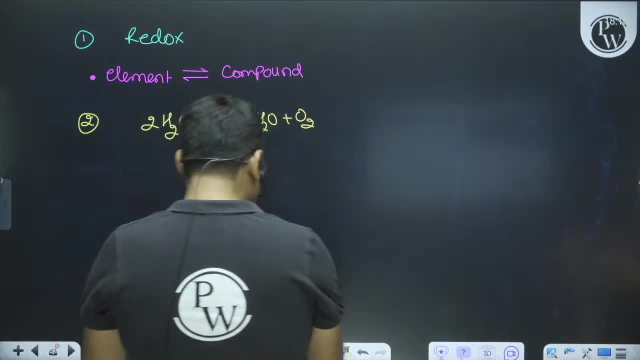 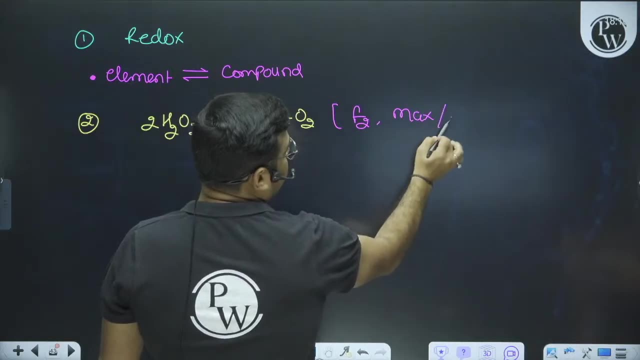 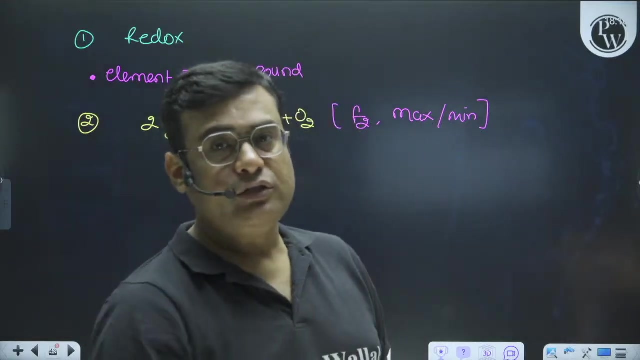 that is why it is important for you to remember that fluorine. fluorine is not disproportionate, and any compound in which any element is in its maximum or minimum oxidation number is also not going to show a disproportionate reaction. it is also not going to show a disproportionate 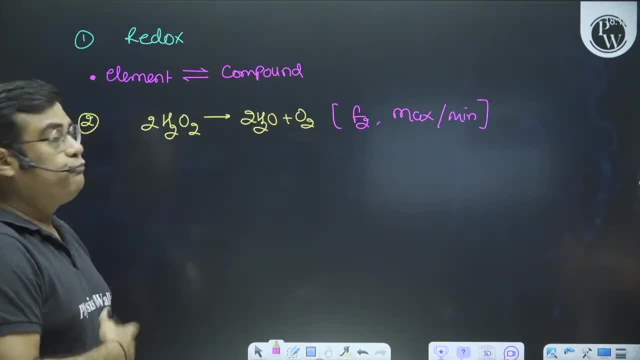 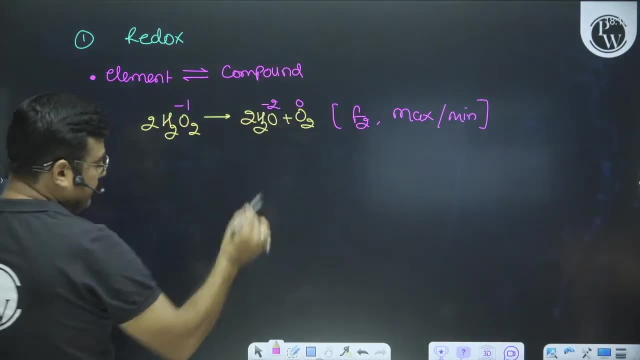 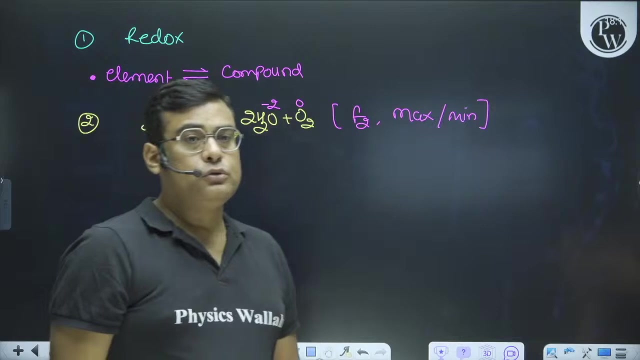 reaction. keep in mind. then, what do you want to tell, sir? you are from this: ok, oxygen is here. in minus one children, minus two zero. I want to tell you, my dear children, on H2O2,. many times the question has come: in which reaction is H2O2 working? like oxidizing? 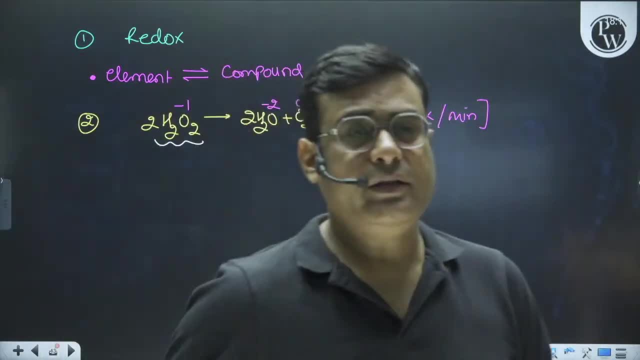 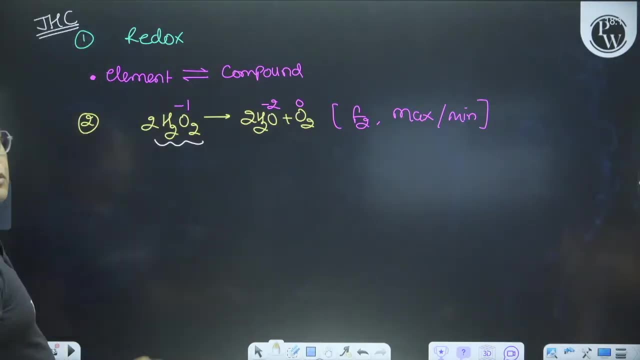 agent in which it is working like a reducing agent, then H2O2,. I am telling you all this JSC. I am telling you a little bit of the concept. there is only one logic to do these questions, that is RO. there is also a water purifier in your house, then RO is reverse. 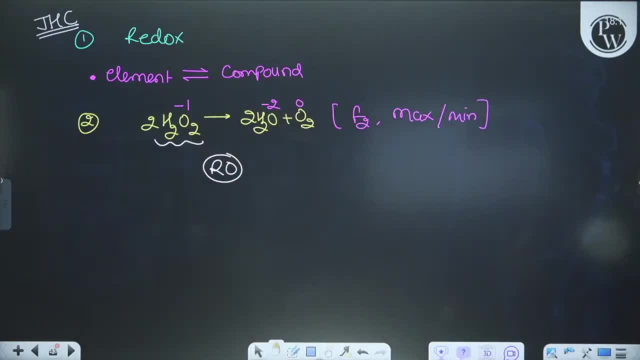 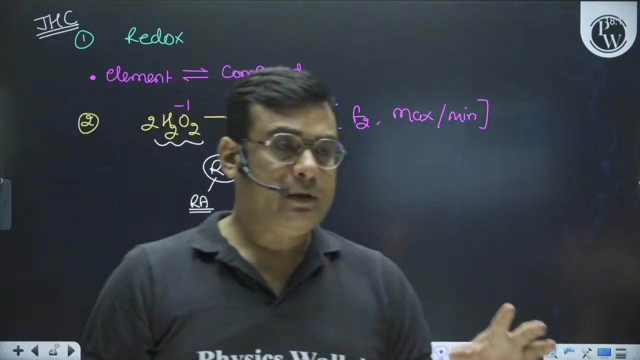 osmosis as a water purifier. RO will also be applied here. ok, but here the RO is also the same. then what is the meaning of RO here? it has the meaning of RO. remember one code, fo- H2O2- that Whenever H2O2 will work like a reducing agent, that means when it. 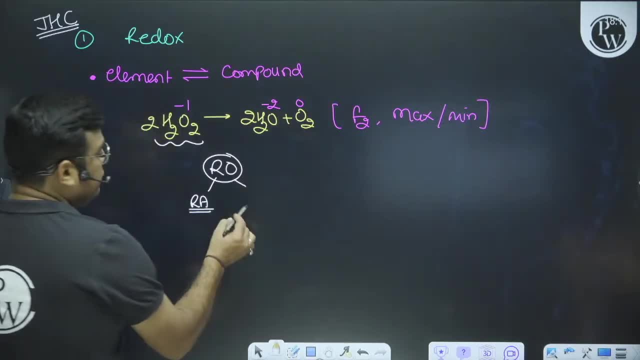 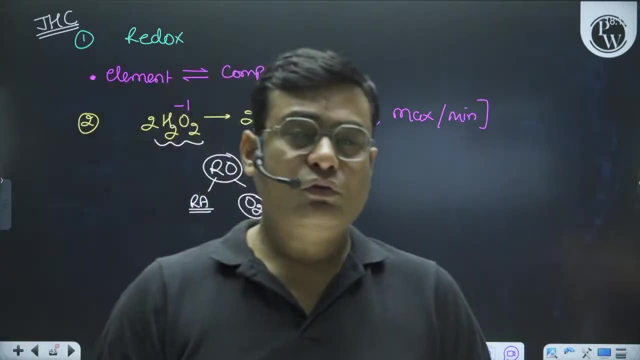 will reduce others. children. it means will also be oxidized itself, And if it itself oxidizes, it will give you oxygen. and if it itself oxidizes, it will give you oxygen. if it itself oxidizes, it will give you oxygen. 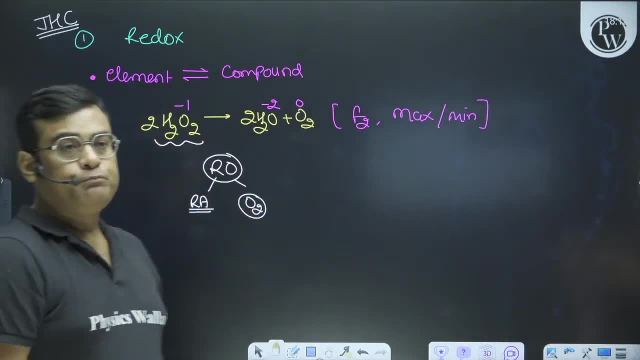 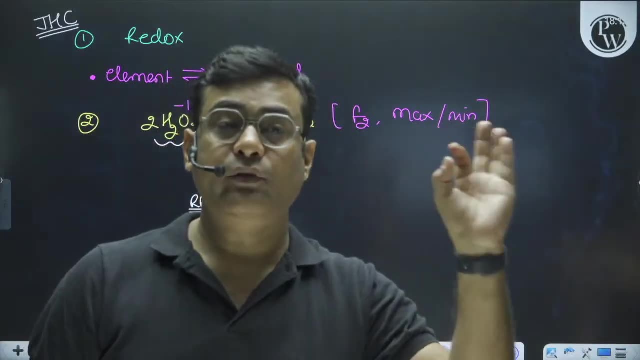 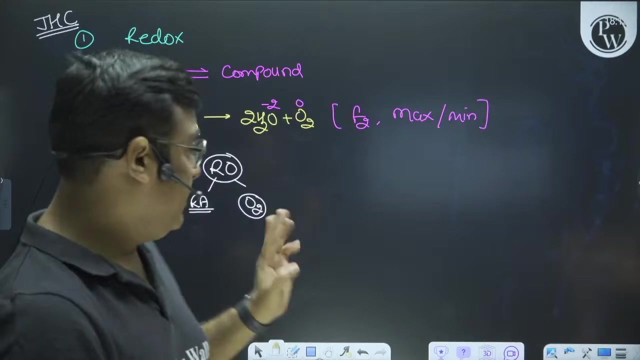 If you see any reaction in which you can see oxygen, immediately tell me that H2O2 is working as reducing agent, and if you don't see oxygen, then it is oxidizing agent. It has nothing to do with the world. just remember a small trick. 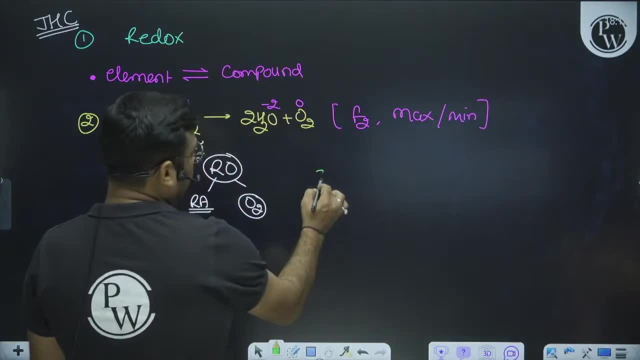 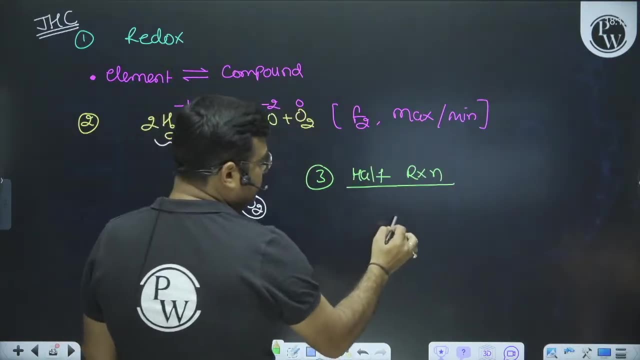 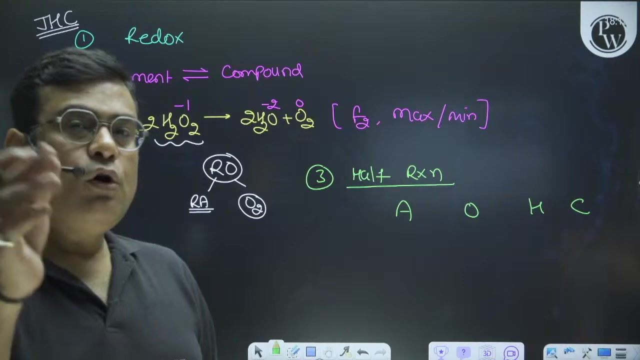 The second most important thing of this chapter is to balance the half reaction. You can do it in a few seconds. just remember my code AOHC. What is the meaning of this code? Come, let's go to Hong Kong. Where will we go? 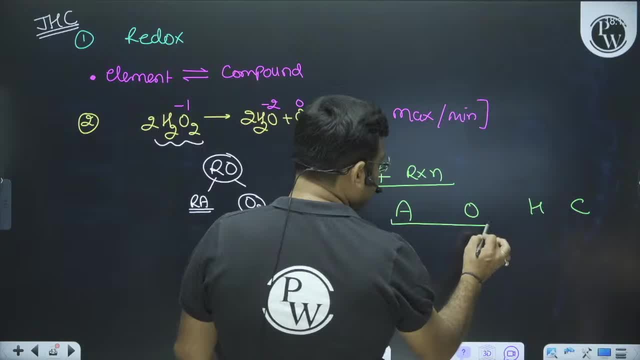 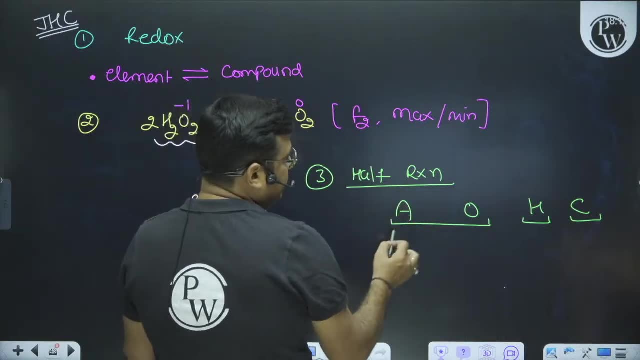 Come, let's go to Hong Kong. Come from AO, H from Hong Kong, C from Hong Kong. What are you trying to say? Malibrate it? Half reaction: First of all, you have to balance the atom, Then the oxygen. 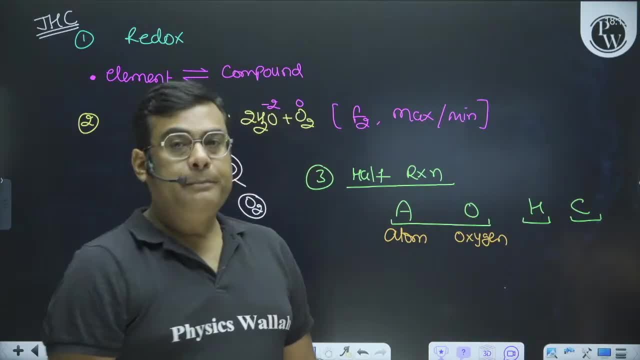 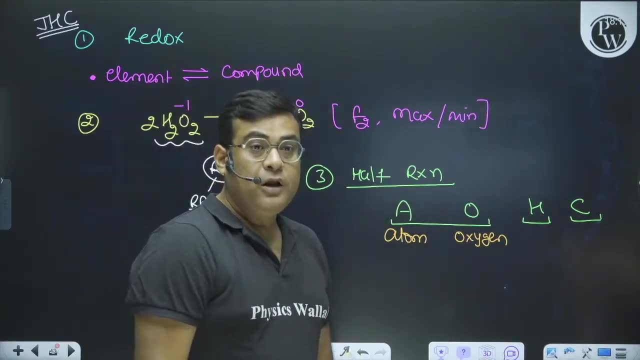 Oxygen is the desired medium. Medium means acidic. So the side where it will be less H2O is on that side. On the opposite side its double is 2H+ And the side where the oxygen is more in the basic medium H2O is on that side. 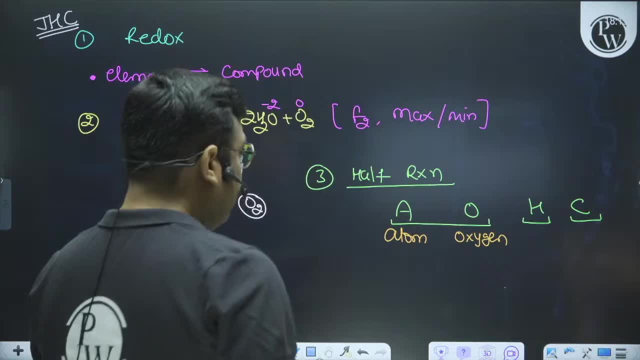 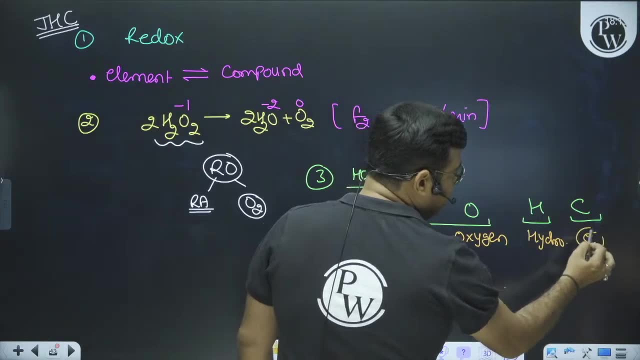 On the opposite side, its double is OH-, Then children hydrogen. Hydrogen is always balanced with H+ And then C for charge. Charge is always balanced with electrons Because it is a half reaction. Charge is always balanced with electrons Because it is a half reaction. 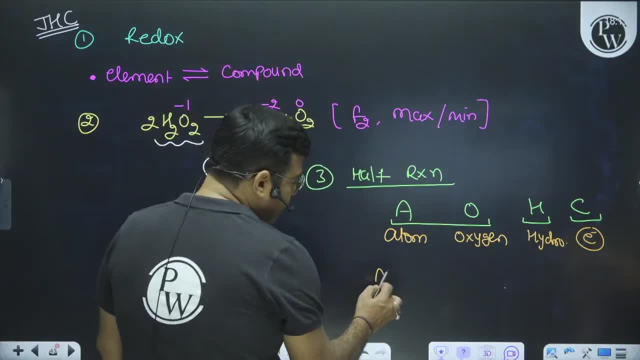 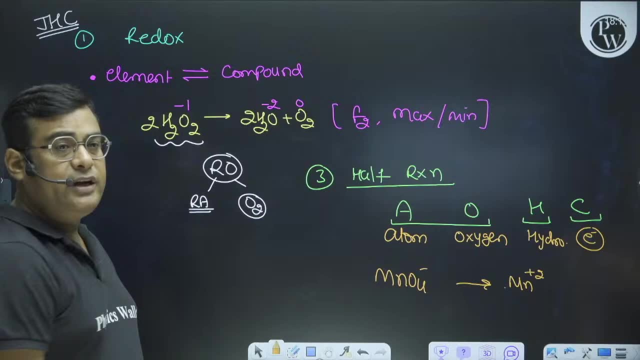 So let me give you a small example. If I am telling you that in MnO4-Mn plus 2, J-2024, there was a question in the January attempt And it happens in a pinch children, This is some Jhc. 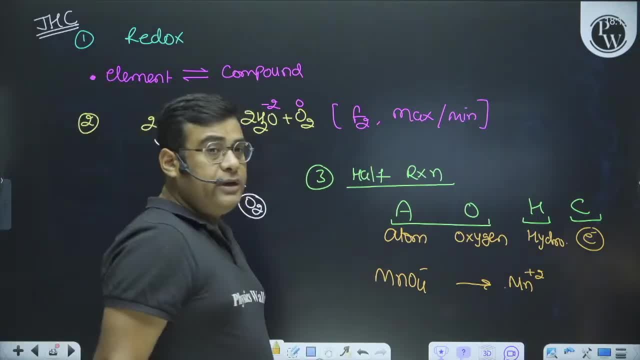 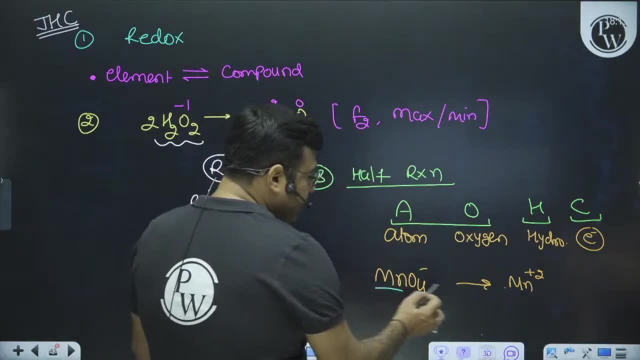 You must take care of me on this topic. I am telling you to balance this reaction in the acidic medium, So you do not have to think about anything, children. First atoms, manganese balance. Come directly to oxygen. Sir, there are 4 oxygens here. 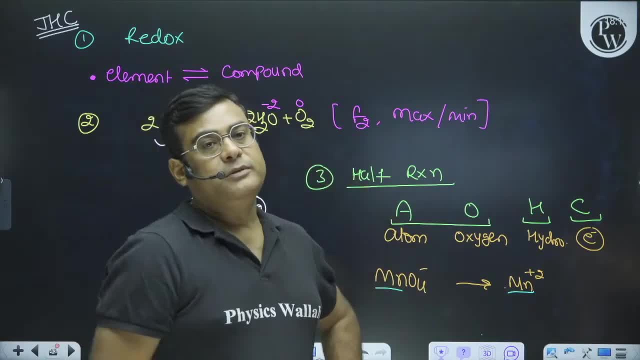 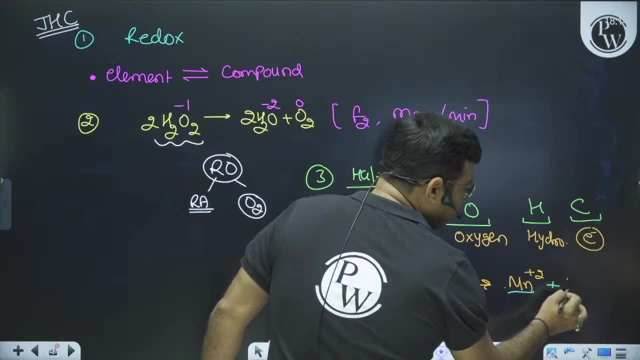 Medium acid will be mentioned And in the questions where the medium is not mentioned you have to take acid by default. So here there are 4 oxygens, children. So on this side you will put 4 water, on the opposite side 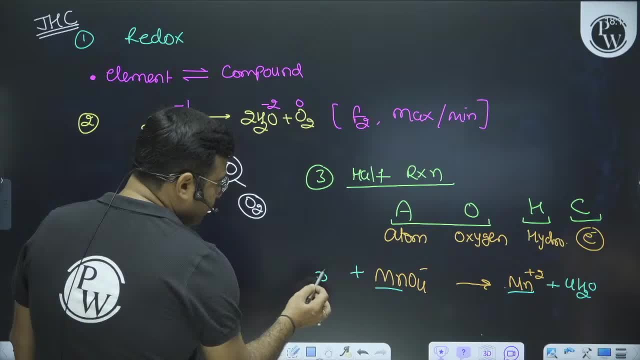 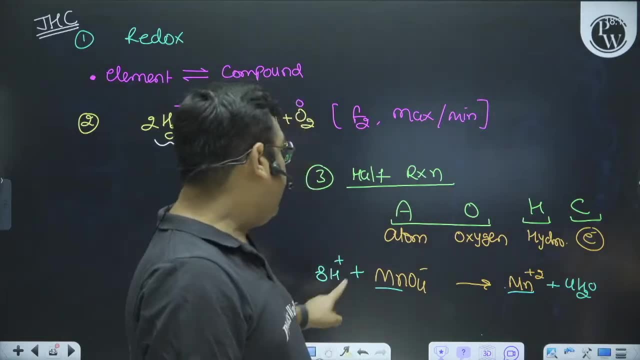 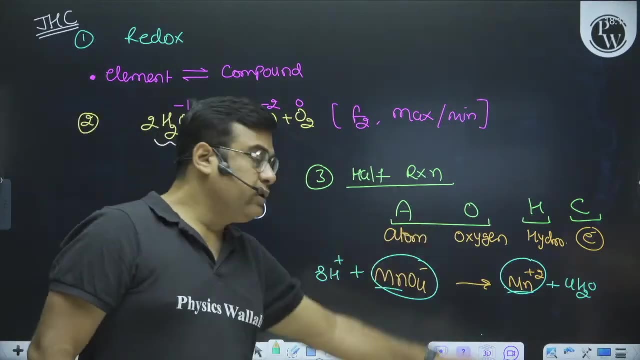 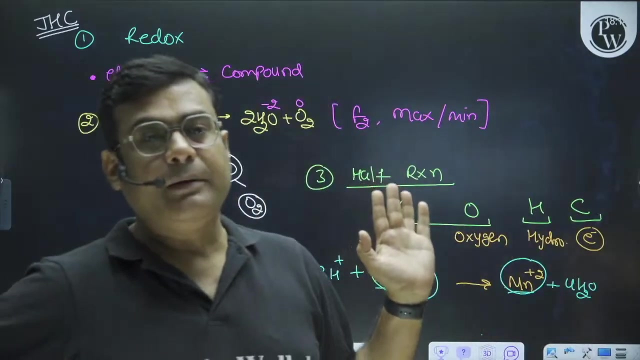 Its double, Sir. what is the double of 4? 8H+? Put it on the opposite side, Then who will you balance Hydrogen? Can I tell you a trick for hydrogen? One more good: If there is no hydrogen in the original compound that was given, then it means that the hydrogen is automatically balanced. 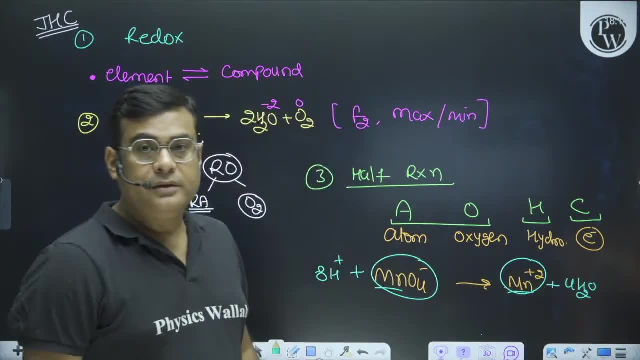 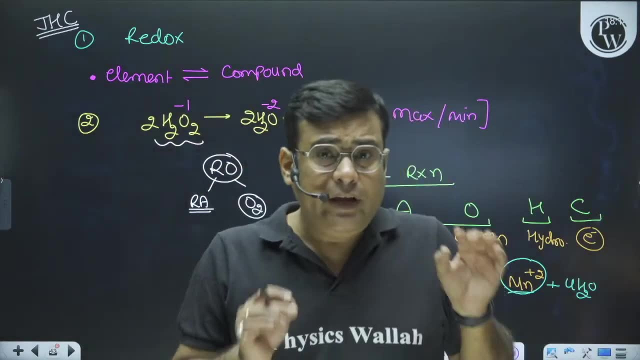 See, you put 8 hydrogen here in 4 moles of water, So automatically 8H plus has come, So you will save some time from there too. If this small time is saved children, it fills the pot from the drops. 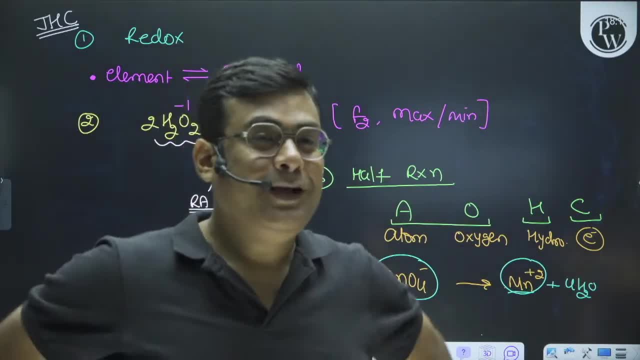 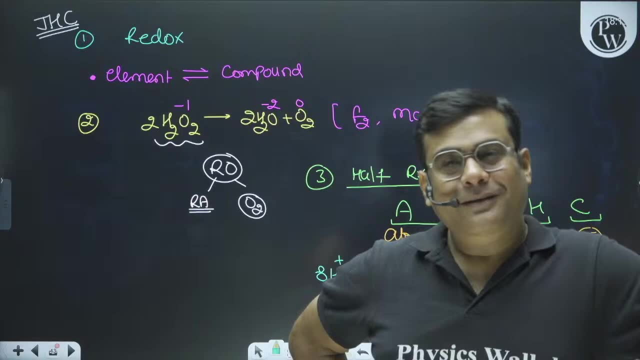 It fills the pot from the drops. It says that the ocean cannot fill it. It's mad. I'm a little bit Alright. So, seeing your love, there are some crazy talks coming out. So I am saying to you, son, it fills the pot from the drops. 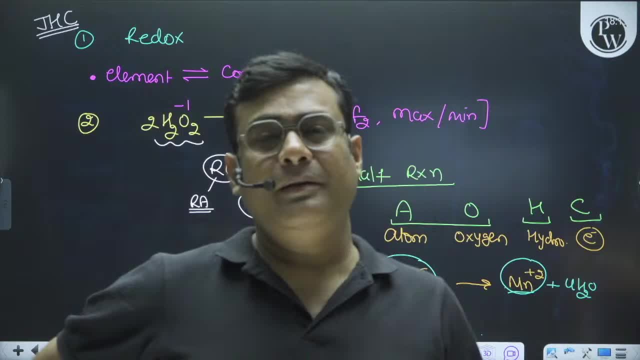 Sir, we also know saying that the tap is dropping from the tap and the water is falling. Alright, I can't stand standing for an hour and fill it, But if I let it, So, brother, he will fill it automatically, Right? 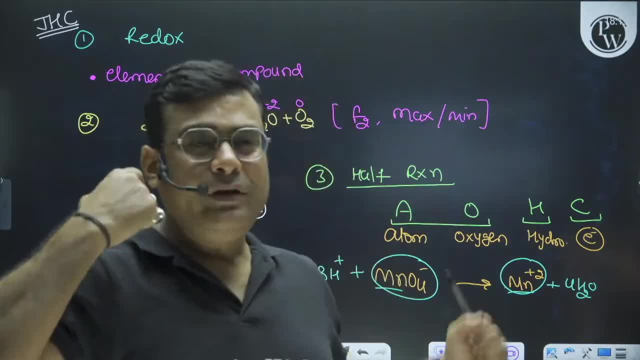 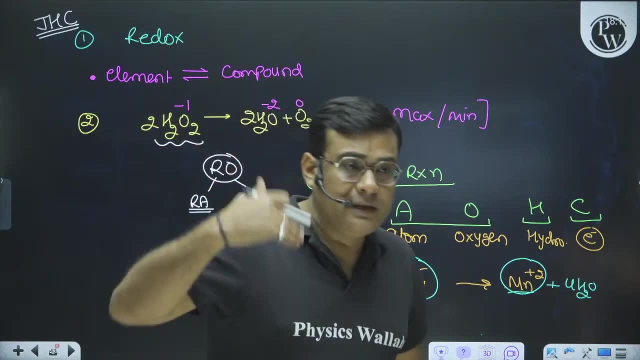 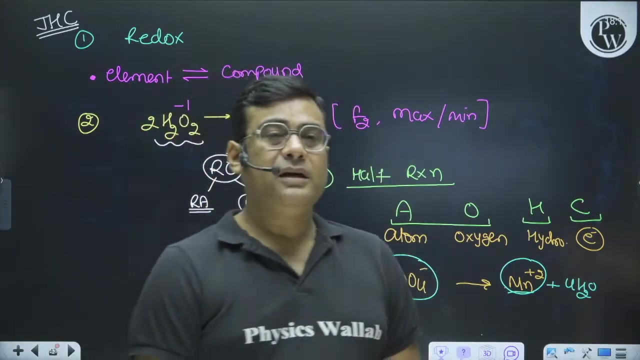 He will fill it automatically. I want to tell you that if we learn to save time in 10-15 seconds, then if we save 4-5-6 minutes and if you have extra 2 questions in the match, then normally the match is a little. 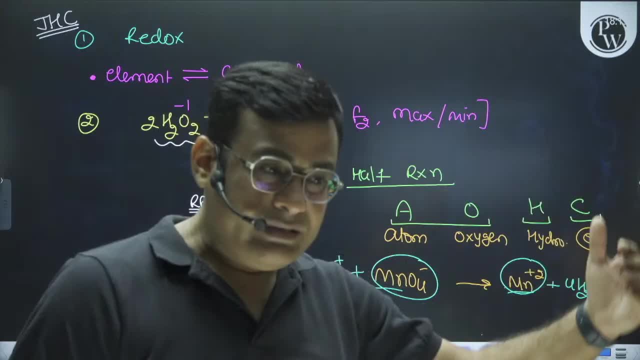 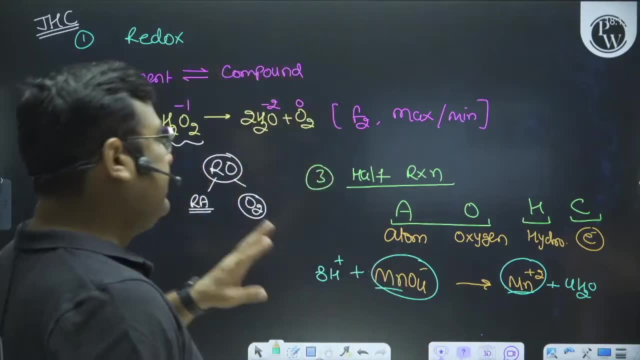 lengthy. It takes a lot of time. so if you have extra 2 questions, then you will be able to do it easily. It's just a little story. If things can be done by knowing, then why not do it? okay, what to do after this- children. 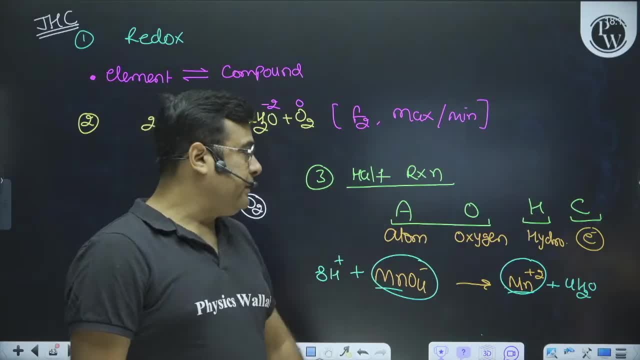 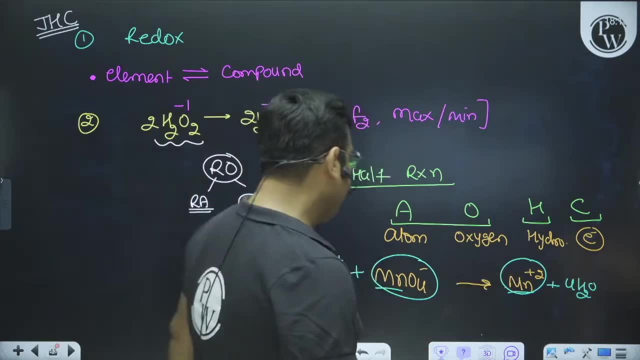 charge. here is plus 8, here is minus 1, then how much is the total charge? children plus 7, here is plus 2, then it means that your 5 electrons have come to the left hand side. Now we know, in redox children there is also a matter of equivalent weight. there is also 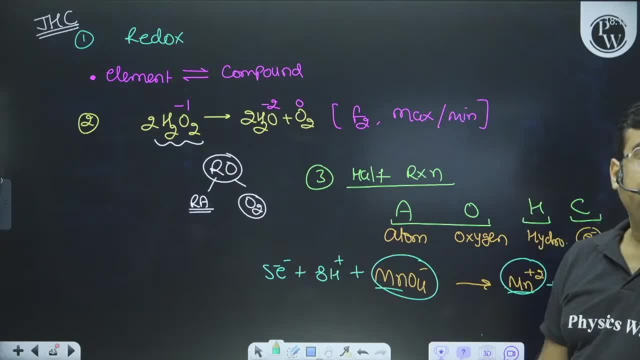 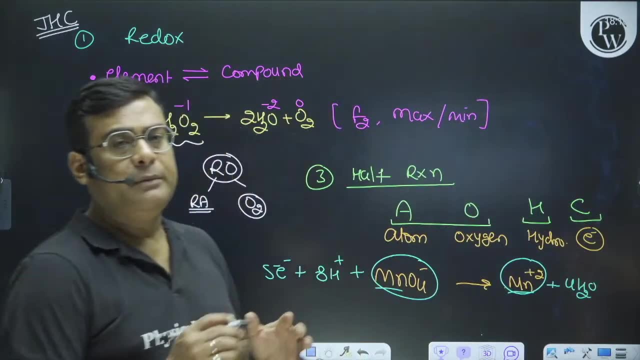 a matter of n factor. you all know about MnO4 minus Acidic medium. Acidic medium has n factor 5, this 5 is yours. okay, in this way, if you do these small, small things, in my opinion don't pass the time, son. I am not passing the time at all. 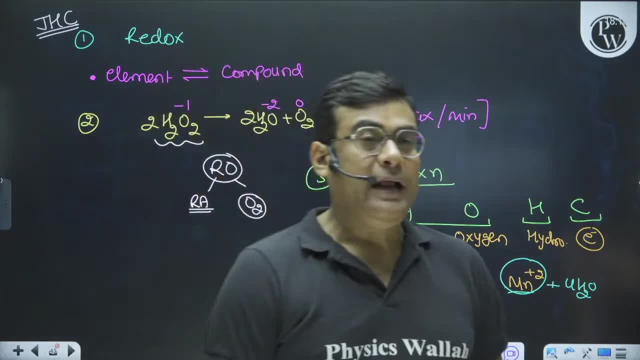 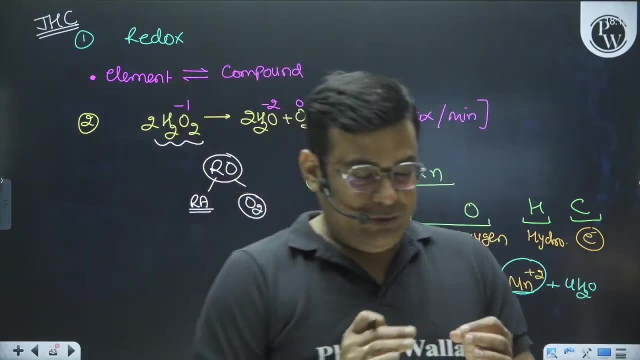 son, I don't have the right to pass the time, right. you are doing the time pass. you need so much effort to write so much time pass, right. then these are the children- children, right- who, when everything is done, then they keep saying: why am I like this? why? 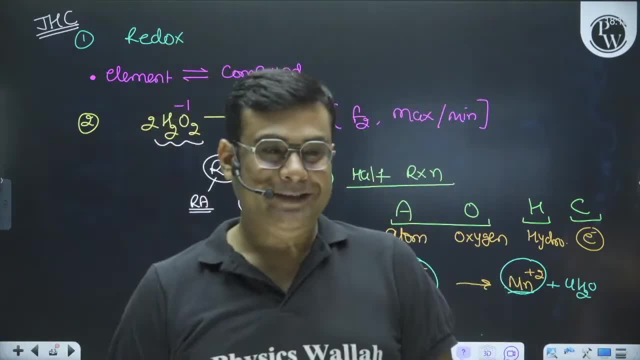 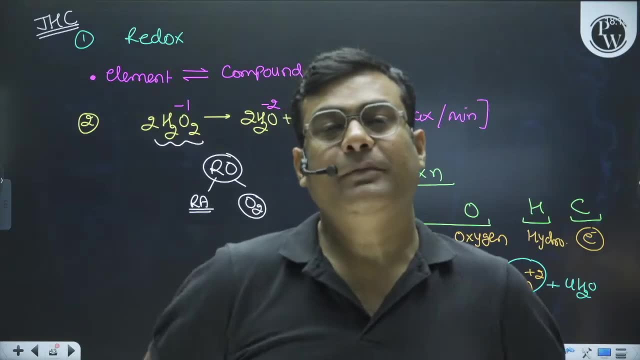 am I like this. they don't have to do anything. They don't have to do anything, right? I had a student offline. he was a good child. he kept explaining a lot to him. that read, son, read. later. there can be a problem. 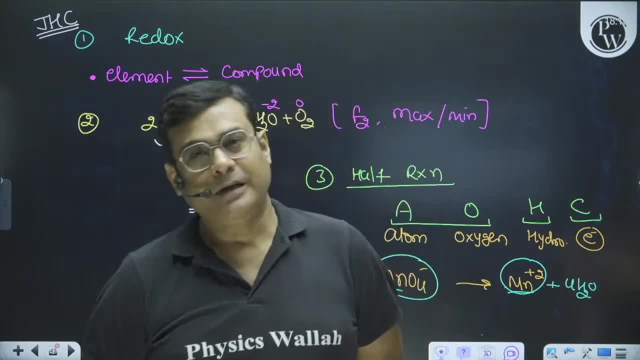 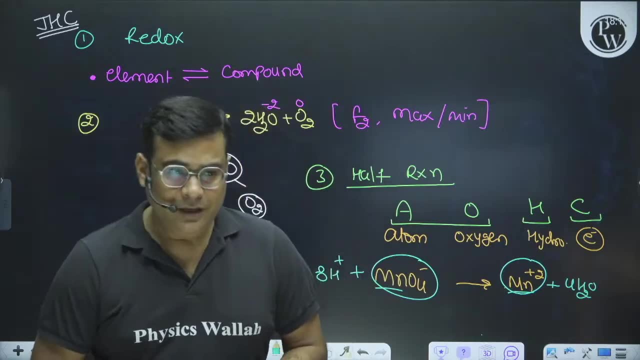 you have a good mind, then you can do good. right, you can do it. didn't listen, didn't listen, didn't listen. this is the era of online now. the children have come here for more than 4-5 years, right, by the way, let me tell you for information that from 2013, 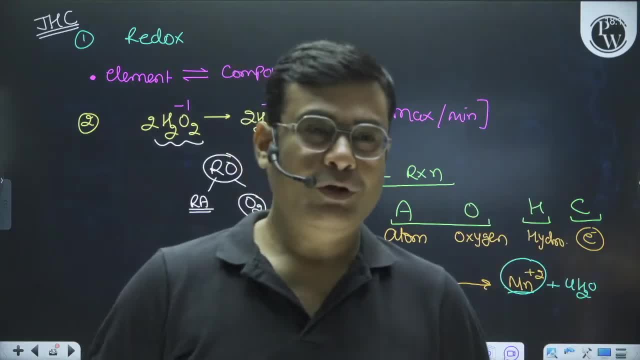 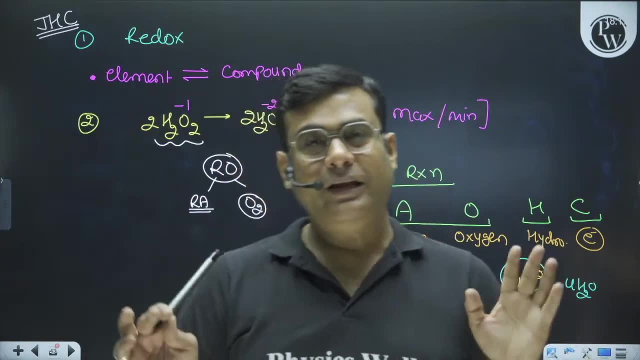 I am also in the online field. if you listen to the name of E2's education and from 2013, you will see my old videos, 11 years old from today. and in the teaching field, I have been teaching the children since 2001,. right, so I had taught pure offline for 12 years. 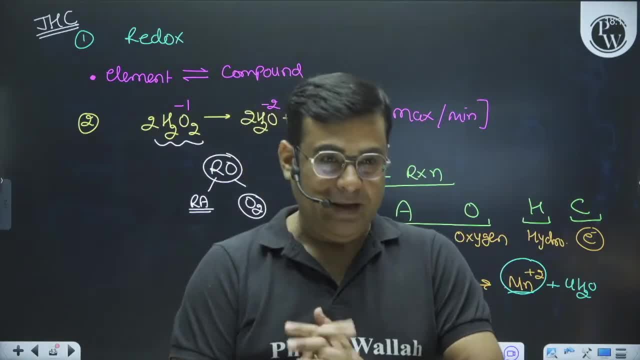 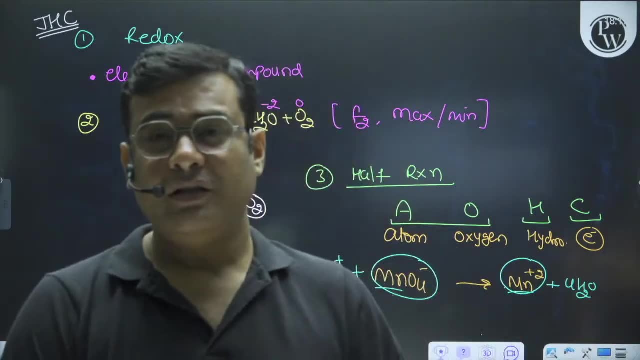 now online is in both offline. now we are online in PW, now we are online. right then, what happened? I have explained a lot to the children. we try our best in offline. the children put their heart and soul with the children. didn't listen, didn't listen. 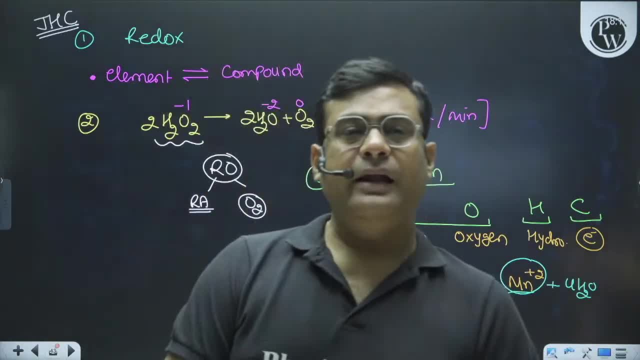 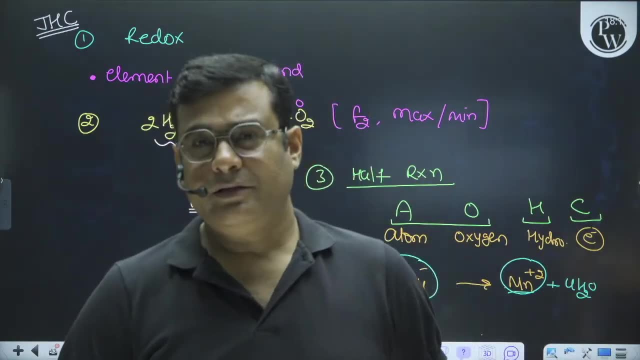 didn't listen. finally he failed. in the next attempt he did the same. then he failed. the children got upset andzn a fire came to us and once came face-to-face person. what's the old story I am telling you, son, today. I am saying before that: 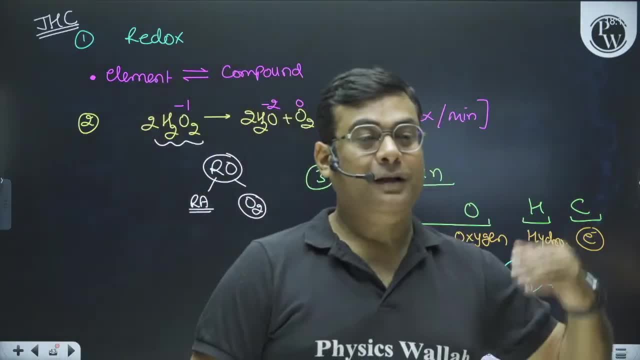 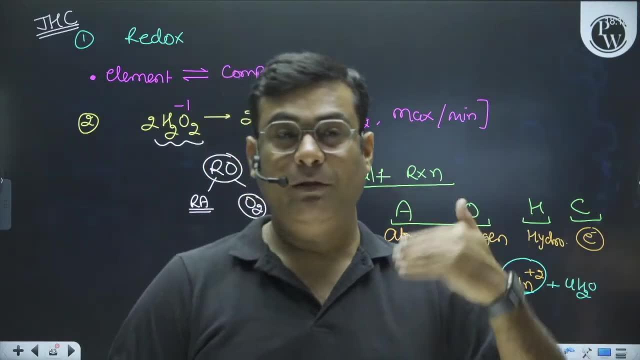 I was ruined by time, right? you kept saying that. you kept saying read, read, give attention. later you will repent. I did not listen then. time I wasted then. time has ruined me. now I am ruining the time. right now I am ruining the time. 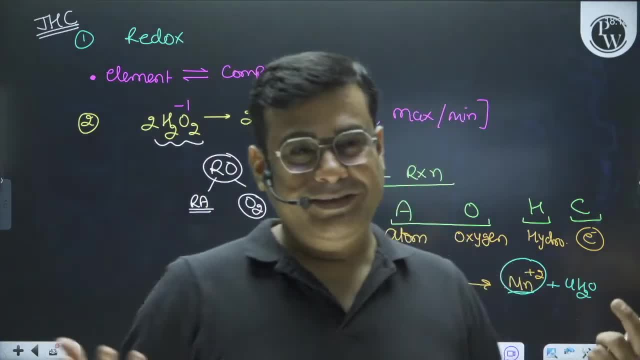 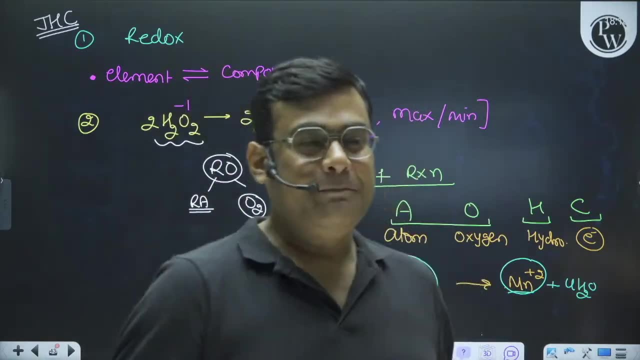 I said this is very beautiful. now first returned to the school and then my ear radiated my brain that my legs areайт. First, the time wasted him. now the time is wasting him. your time pass. writers are also doing the same thing by coming here. 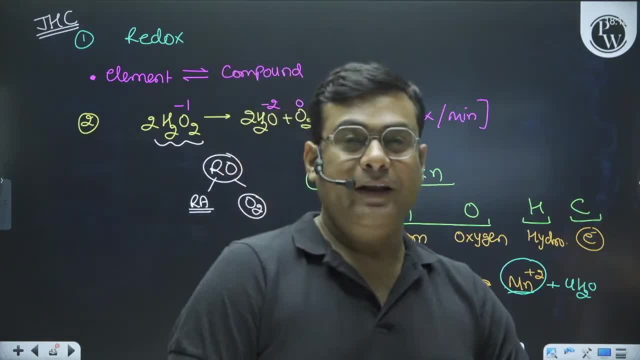 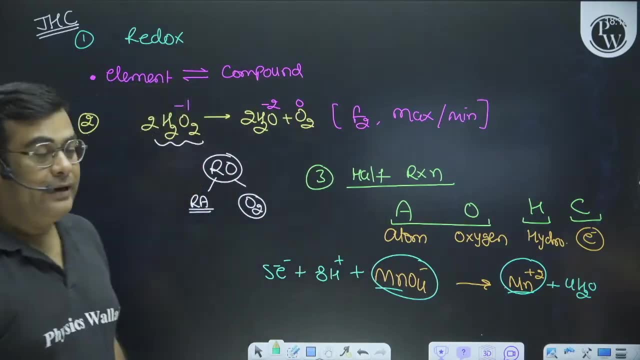 If all your concepts are so good, you are an All India Rank 1 player. then you should not have come here. my dear children, I don't want my son to come to All India Rank 1.. He will have his own exam, he will have his own room, he will have his own computer. he. 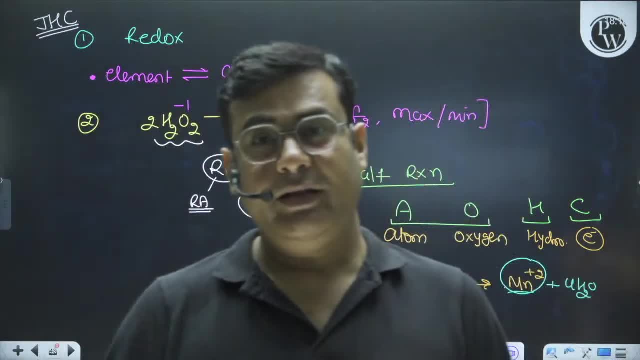 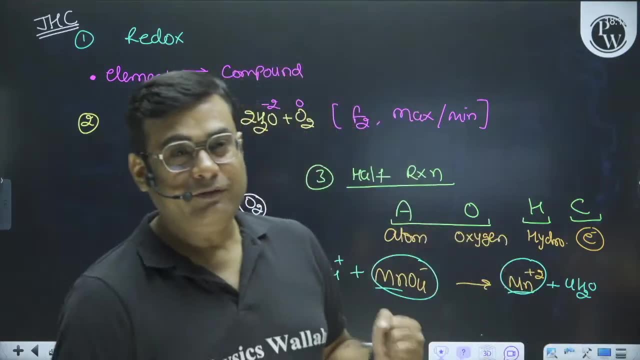 will make his own paper and in that he will come to All India Rank 1.. College can also be of those in which the single student will be the only one, and if they are the only students, then obviously All India Rank 1 will be there. 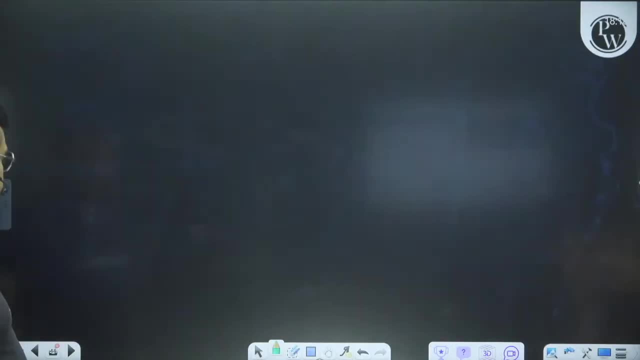 Okay, so be sure to keep this thing in mind, children. Okay, and now I will try to explain this to you in a quick way. Come on, what will be the value of XYZ in the following reaction? Now, you should know this, children. 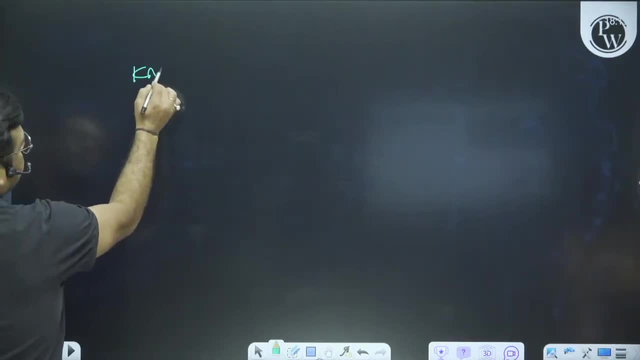 Let me tell you one more thing that you should remember: the code for KMNO4.. BAN 153.. KMNO4 has an N factor of 1 in the basic medium. It has an N factor of 5 in the acidic medium and 3 in the neutral medium. 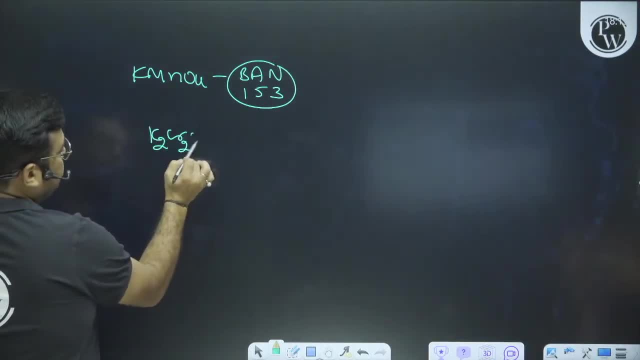 K2Cr2O7 has some well-known oxidizing agent and reducing agent N factor. You should remember that it has a 6, children. Paris salt always changes to ferric, so its N factor is 1.. Oxalate salt always changes to CO2, so its N factor is 2, because it goes from carbon plus 3 to plus 4.. 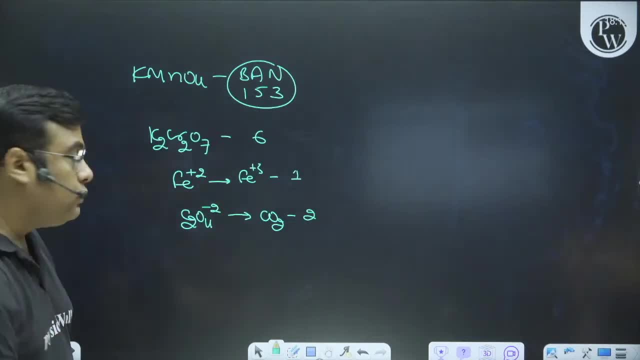 Now in oxalate salt, children, your H2C2O4 can also be there. Ki, that is goes to I minus I2, so its N factor is 1.. H2O2, oxidizing agent, reducing agent works in any way. 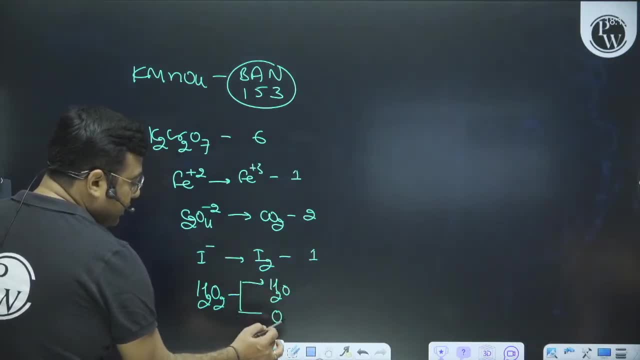 I just told you. if it works like a reducing agent, then it will go to O2.. If it works like an oxidizing agent, then it will go to H2O2.. In both cases, its N factor is 2.. 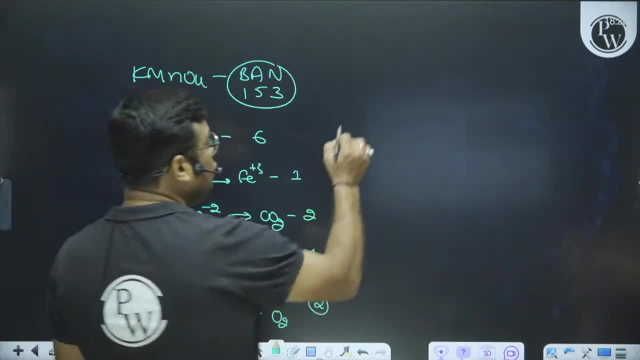 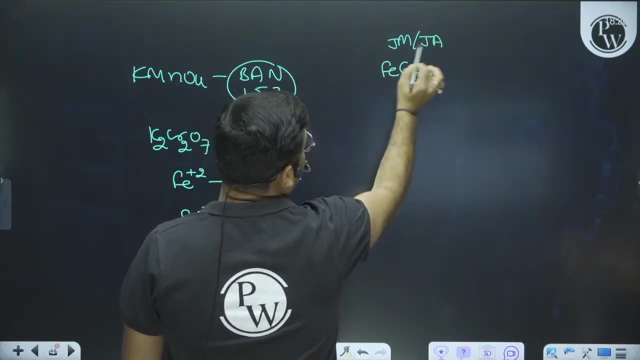 So this is well-known And the favorite of JEE is going on these days: children Ferrous oxalate, Ferrous oxalate, JEE's favorite, JEE main, so JEE advance. so This question has been asked repeatedly in both. 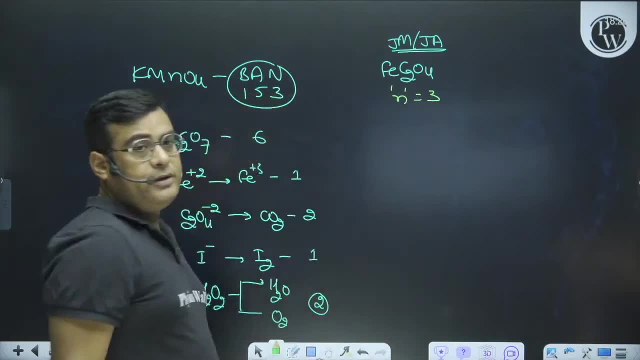 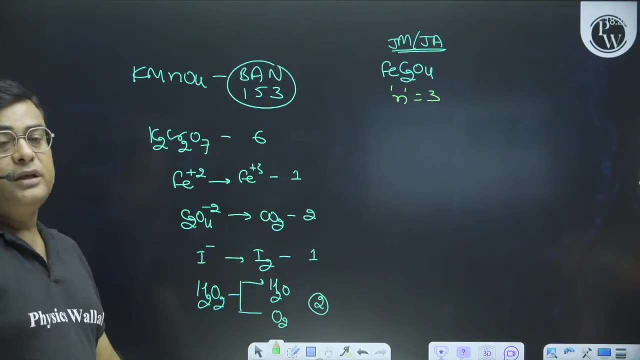 Its N factor is 3.. Because in this ferrous is also going to ferric. Change of 1. And oxalate is going to CO2.. So change of 2.. So it can also be given by mixing like this: 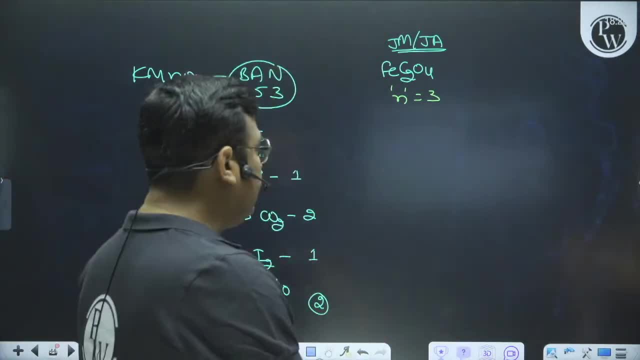 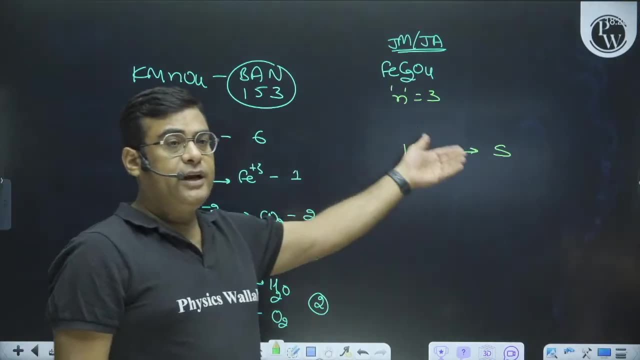 Remember these some N factors. Apart from this children N factor, If I am telling you that H2S is going to sulfur, If I am giving you a change That H2S is going to sulfur, Then there is no problem at all. 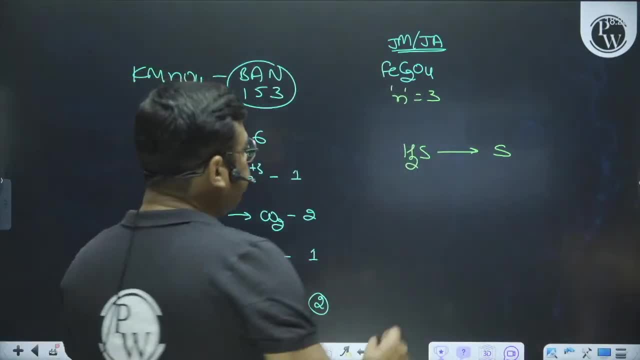 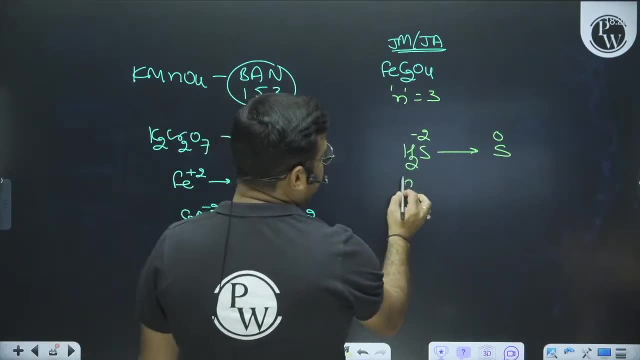 Because you have to make a change in the oxidation number. Here the oxidation number is minus 2.. Here it is 0. Change of 2 from minus 2 to 0. You will say that N factor is 2.. If I am telling you that H2S is going to SO2.. 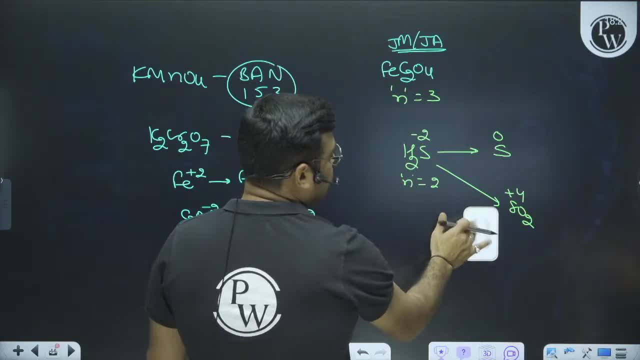 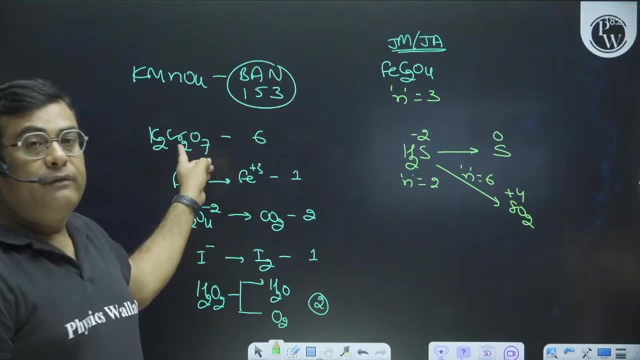 Sir, from minus 2 to plus 4.. In this reaction, the N factor of H2S. In the second one, Sir, it is 6. Like that. But if you are not given Children, then what I have written above. 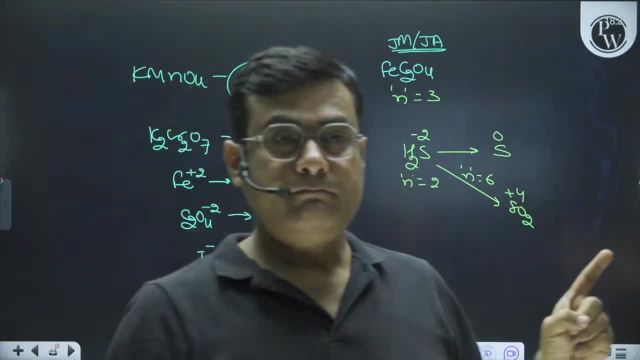 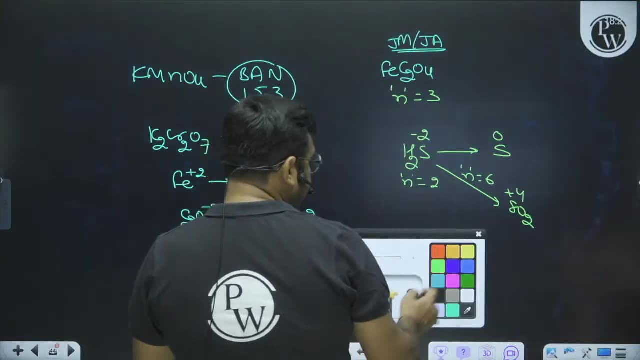 You have to keep this in mind, Isn't it? Which was the number of carbon plus the number of metal? JSC, It was the same son, It was the same. That rule is applicable only for oxalate Number of carbon plus change in metal. 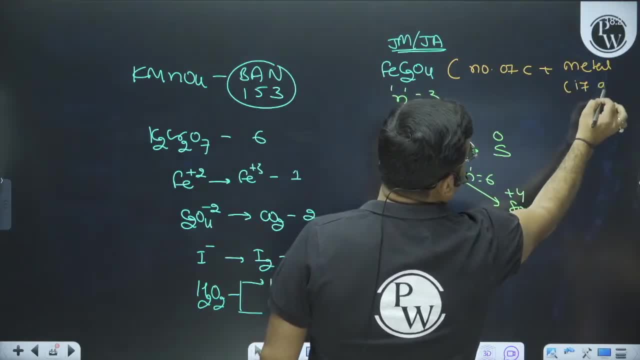 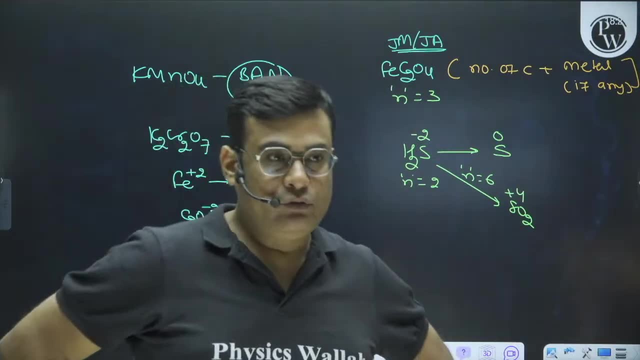 If something is happening, If any, That JSC, that you are remembering the effort. It was the same. There was 2 carbon in this Change of 2. And metal, Fe plus 2.. Ferrass, Ferrass will go to ferric. 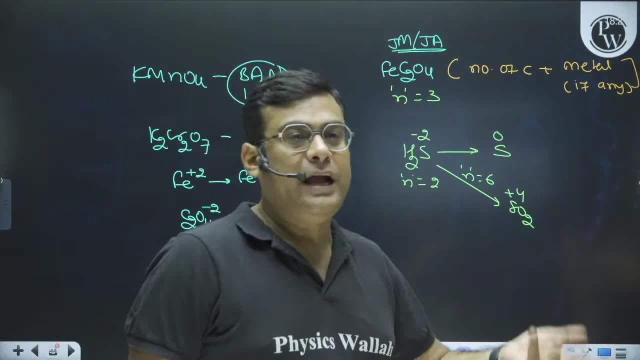 Then the change of 1. Right, No, the tea didn't come, son. The tea did not come, So now I am working with water. So now, why I told you all these things, Son, come see it quickly. 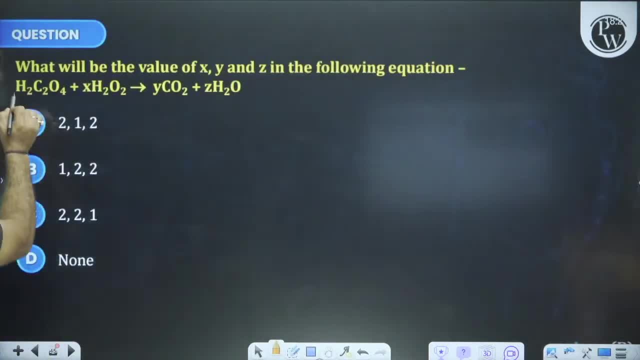 The n factor of H2C2O4 is 2.. And the n factor of H2O2 is also 2.. If you remember, then You don't have to write it. Please see Now. I don't expect you to solve the question, son. 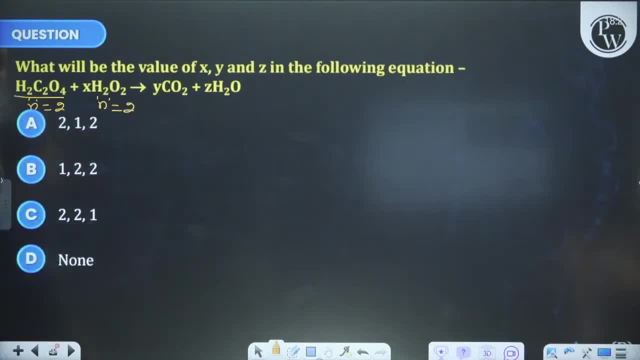 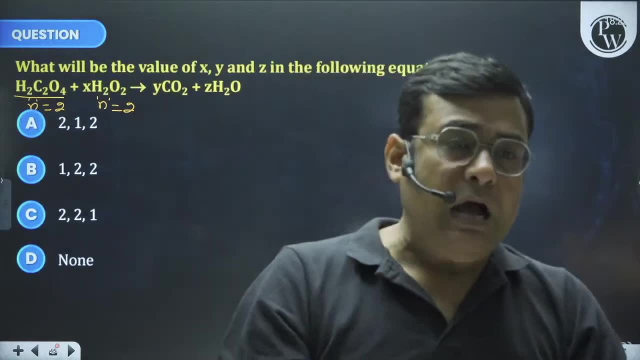 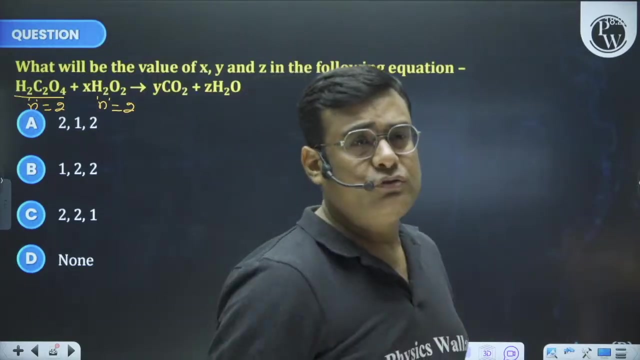 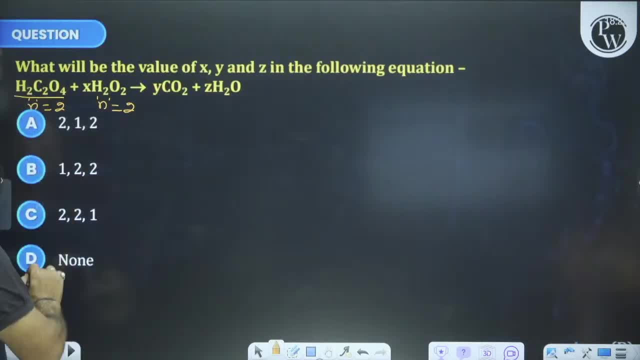 both of them are infected. 22,, that is, both of them will remain one, because here too, you will write 2,. here too, you will write 2,. you do not need to write 22, children, because after dividing, it means that the value of X is 1,. if its coefficient is 1,, then 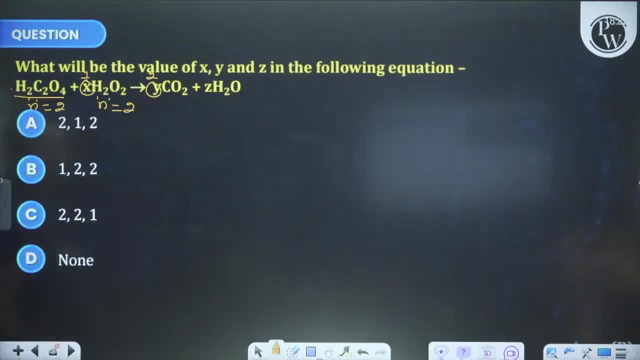 obviously the value of Y will be 2, and he has asked you X. Y has been asked. X1 has become Y2,, X1 has become Y2, look at Z more and more. if the hydrogen is 4, then Z will be your 2,. your answer will be Bombay. 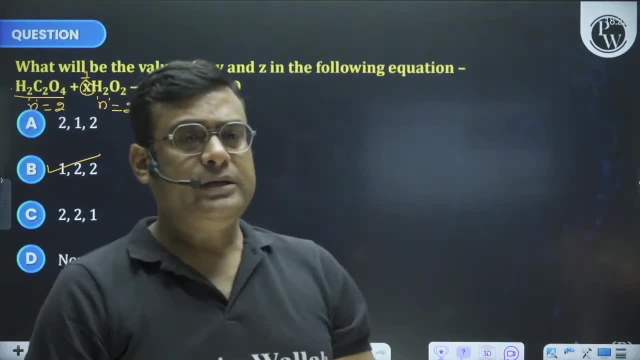 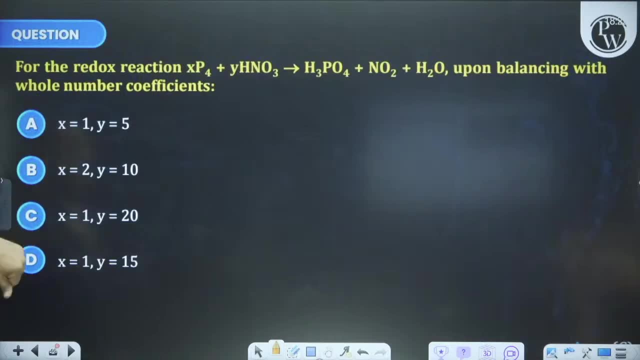 you do not have to solve anything, child, there is no problem. you just have to see, you have to tick. you just have to see, you have to tick. and now the question of redox will be solved in a pinch. see again for the reaction: XP4, Y, HNO3, this, this, this. 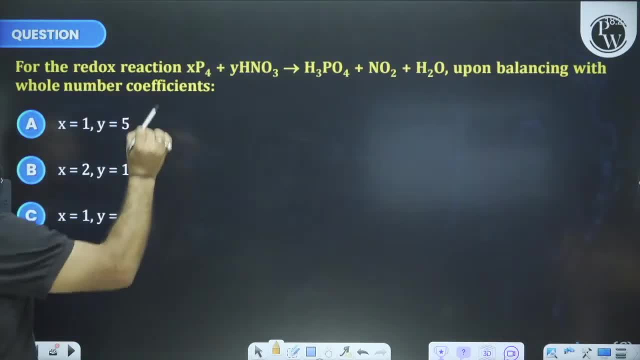 upon balancing, tell me the whole number of coefficients. now, phosphorus is going from 0 to plus 5, there is a change of 5, there are 4 atoms. the factor is 20 for the factor of Что There? 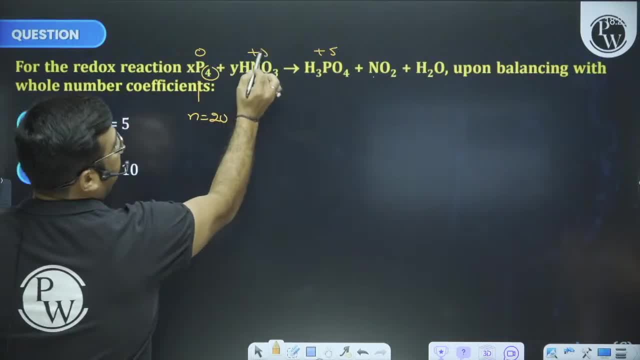 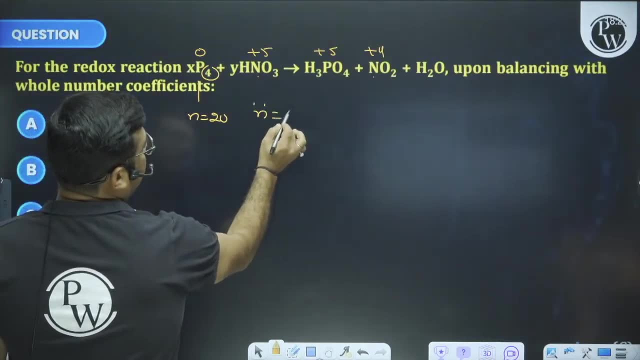 is HNO. 3 is going from plus 5 to plus 4,. ok, now it should not be necessary to write something. I am writing for you. I am adding it from plus 5 to plus 4,. the first factor is 1,. 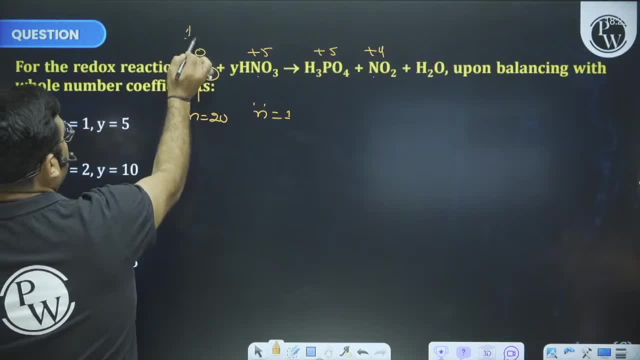 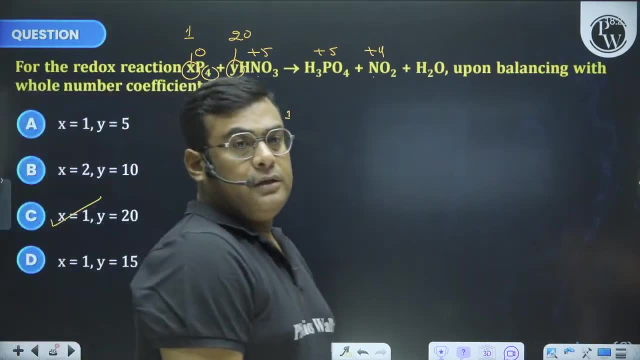 means they will be in a ratio of one is two, twenty. the value of X has become 1 and the value of Y has become 20, only this was asked done: X 1, Y2nTI, X1, Y2NTI, X1, Y2NTY. The story is over right. X 1 Y2NTI village is where the story came out. village is where the story came out. X1 Y2NTI village is where the story came out right: X1- Y2NTI. 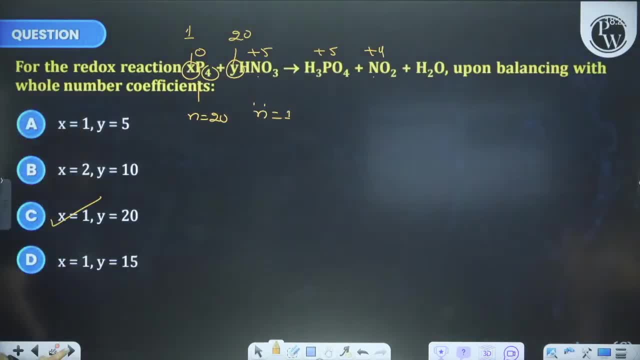 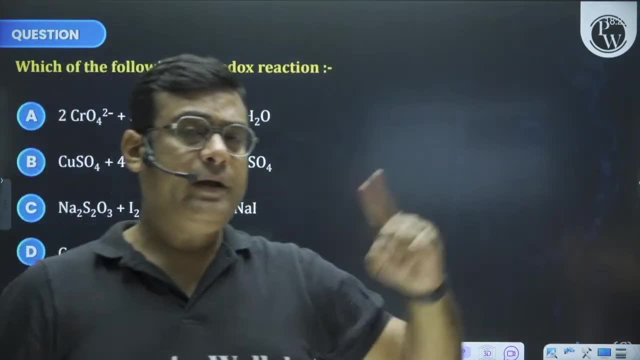 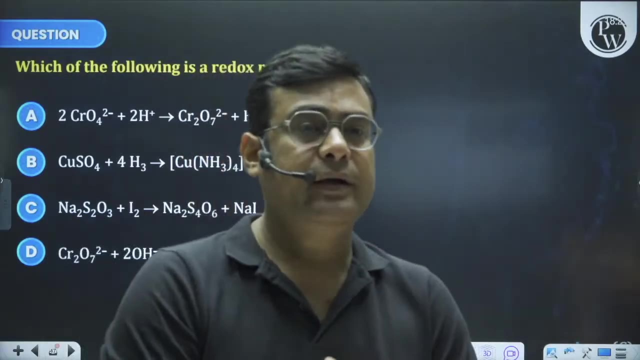 Is this correct? X1, Y2NTI: which of the following is a redox reaction? now you are told the rule that if the element is going to the compound and the compound is going to the element, then take care first of all, see this: that redox reaction will definitely happen. now see the children is. 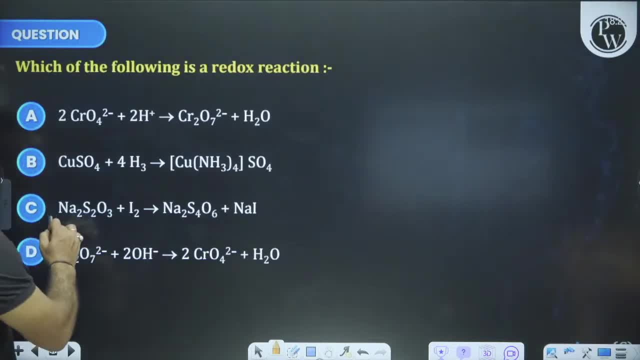 there any relation of the element compound in this? yes, sir, it is seen in option C. it was in the elemental form and it has come in the compound form. the story is over. this will be the redox. why should I waste my time thinking about the rest? I am telling you. 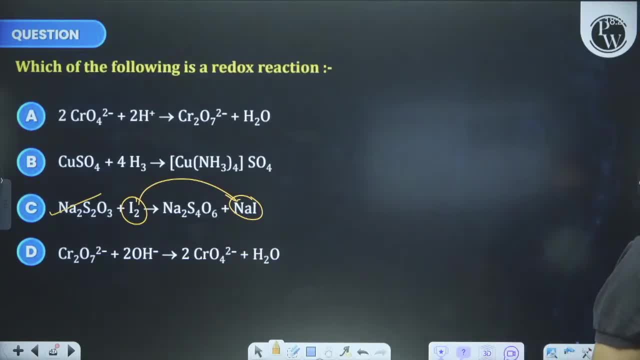 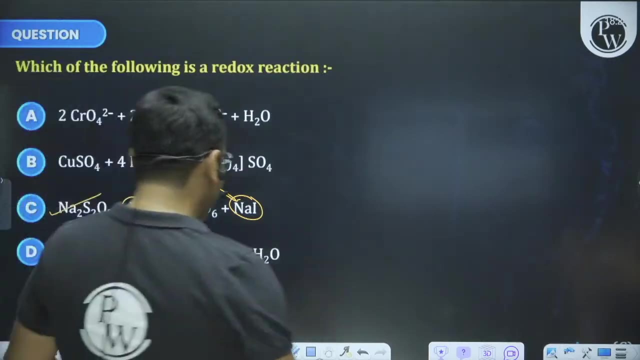 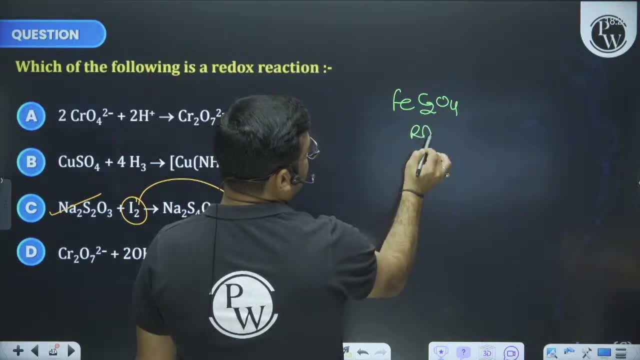 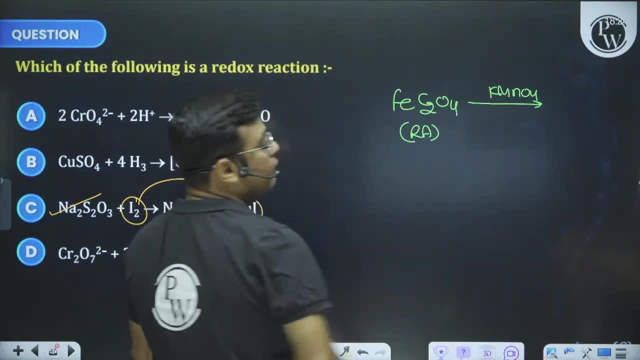 If this redox reaction works properly and if he is telling you this, that if you have to react with K-Mino4, then tell us how much will the n factor be? FeC2O4 is a compound child. There is nothing new. it is a compound. it is a ferrous oxalate performed by the combination. 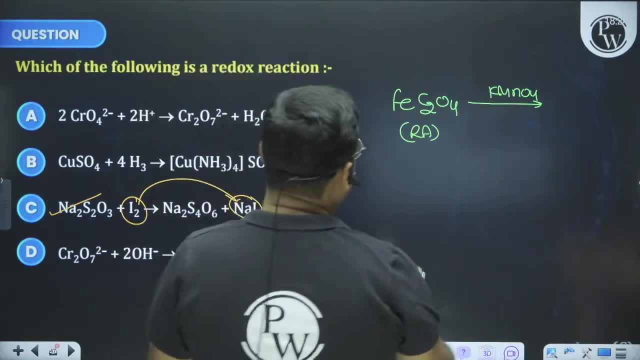 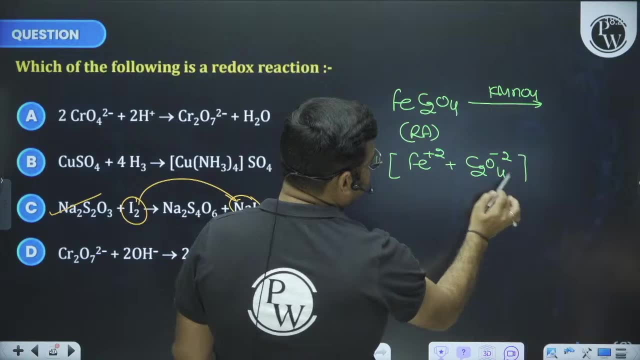 of ferrous as well as oculate. It is formed by the combination of ferrous as well as oxalate. Theuction of man is dead. what will you say? that you have met the meters are healthy, sondern pennies have spinner. 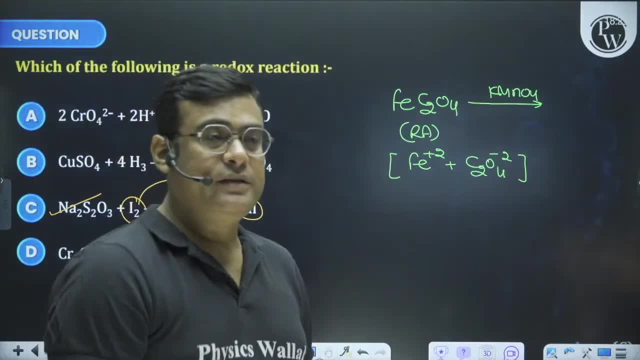 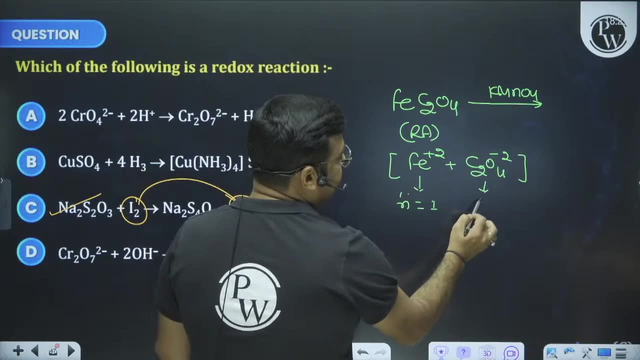 It is formed by the combination of ferrous and oxalate. that is why I said n-factor. Ferrous n-factor is 1 because it will go to ferric and oxalate n-factor is 2 because carbon is in plus 3.. 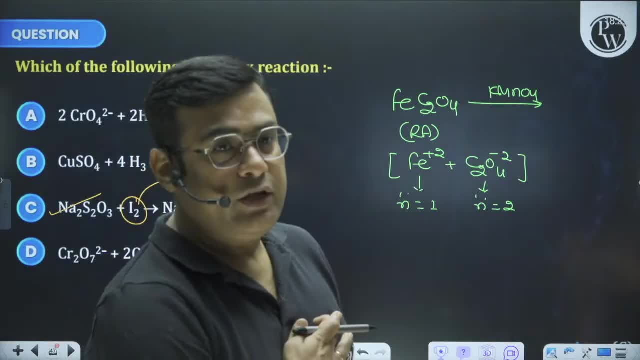 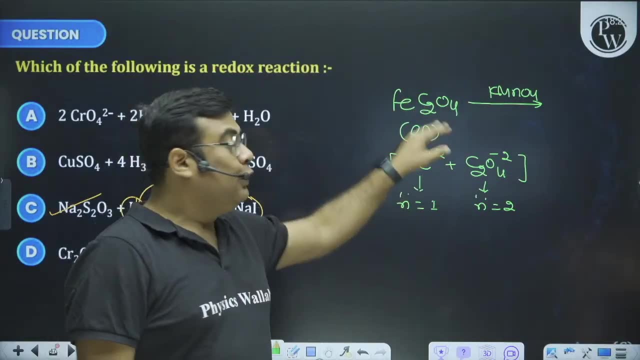 It goes from plus 3 to plus 4.. Thank you very much. if I am your favorite teacher, Everyone should have it. I teach everyone the same and I teach well. So the total n-factor of ferrous oxalate is 3.. 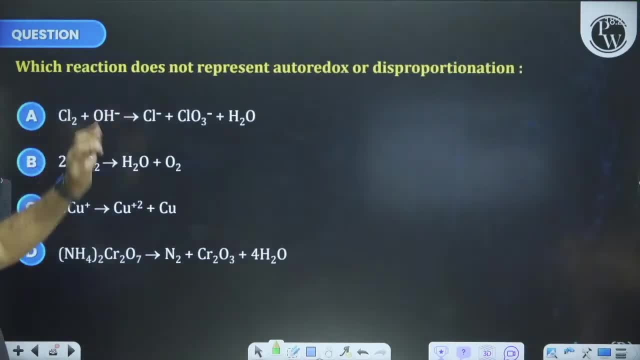 Which reaction does not represent auto redox or disproportionation. Now what was the favorite question of JEE? In auto redox, only one element will change its oxidation number. It is doing Cl2.. H2O2 is always present In Cu plus. it is seen as plus 1, plus 2, 0.. This is over. 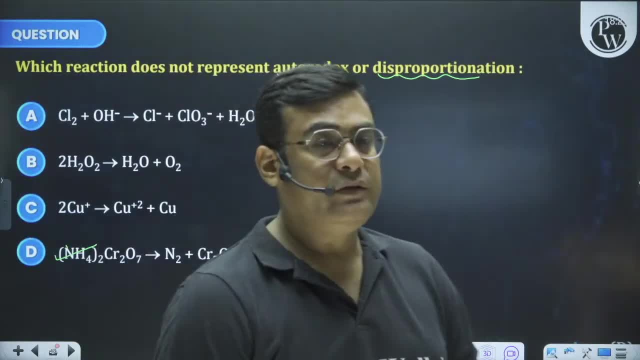 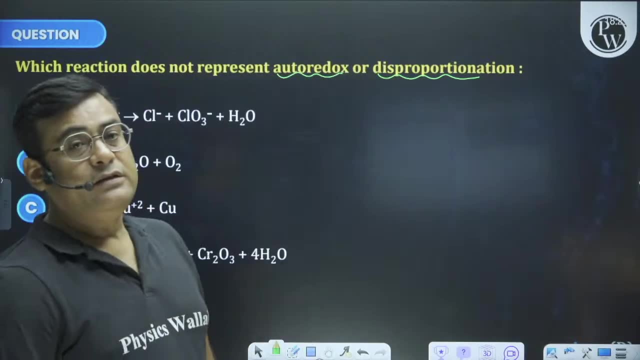 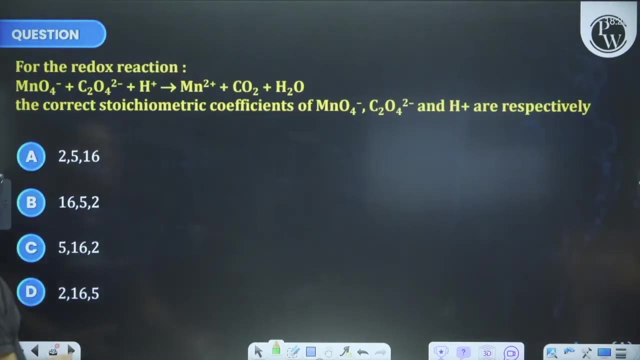 My personal observation from the question of redox is that the child is very scared. But I agree with the question of redox. relatively It is very easy. This reaction is the correct coefficient of this, this, this, This is the favorite question of JEE mains and JEE advance. 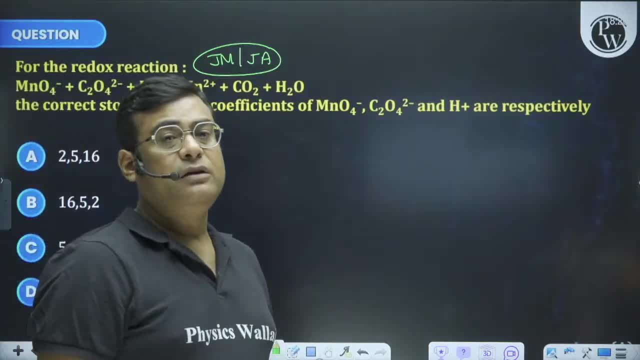 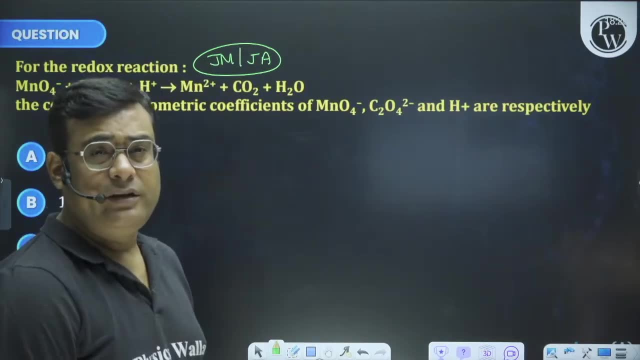 You will also see that at least 5-6 times this question has come to you. At least this question has come 5-6 times. Your teaching style is so much different, which understands me a lot, Thank you. Thank you for your hard work and determination. 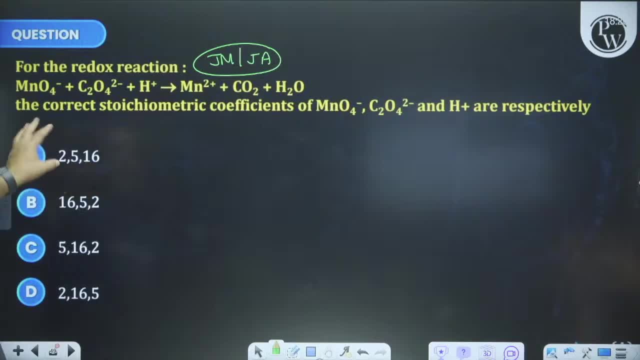 Bless to every teacher like you. Thank you, Thank you. So this is the most favorite question. Now, there is nothing to do in this too. I just said that the n-factor of MnO4 is 5.. The n-factor of oxalate is 2.. 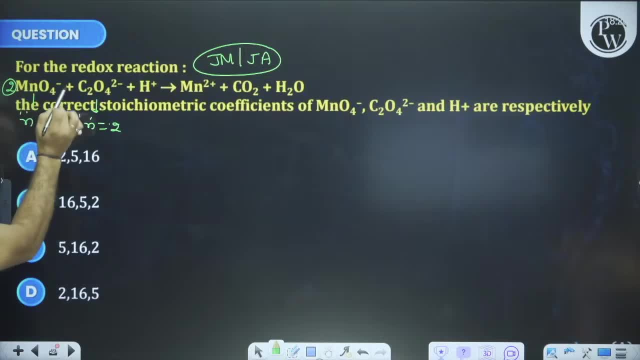 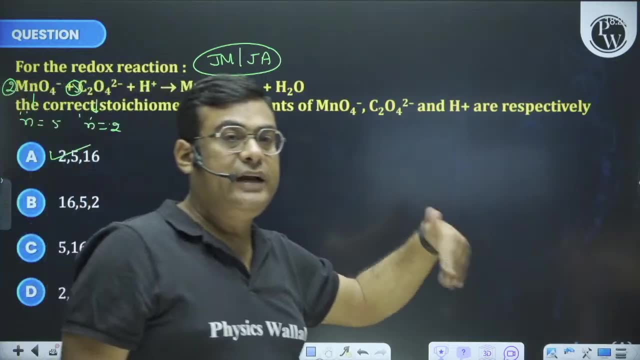 That means if you multiply cross, its coefficient will be 2.. It will be 5.. See which option is 2 and 5.. There is only option. You did not have to remove the coefficient of H plus. You did not have to remove the coefficient of H plus. 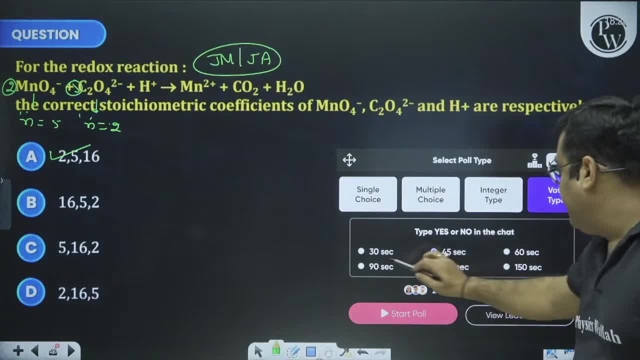 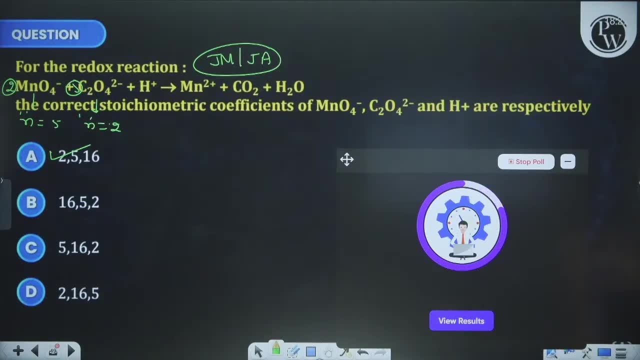 You did not have to remove the coefficient of H plus. We stopped the poll for a long time. It was a small poll of this chapter. In the poll you said: yes, sir, You understood things very well. You felt something different. Is there confidence in the redox? 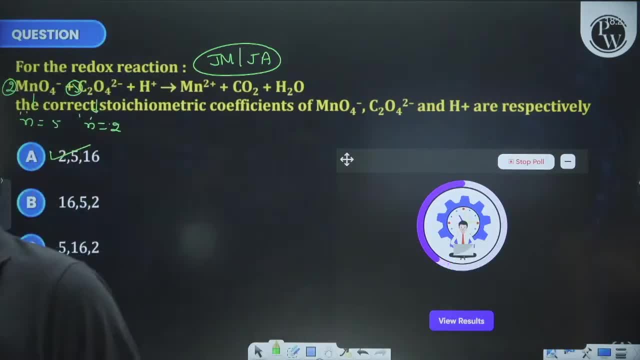 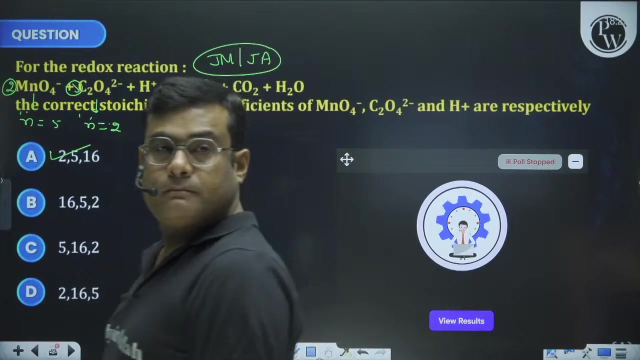 Is the speed increasing? Are things looking different? Let's talk for half a minute. Till then, through the poll, give me my motivation. Did you like something already And did you get to learn something new? The answer is yes, Tell me. 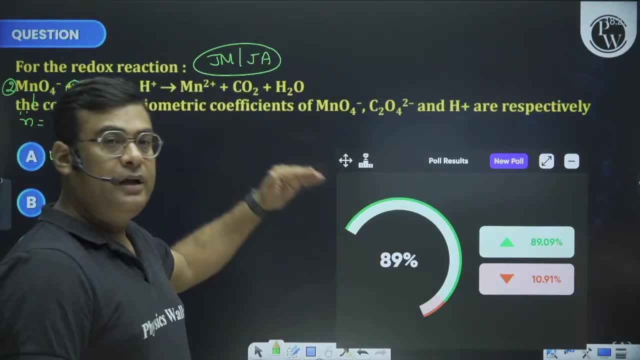 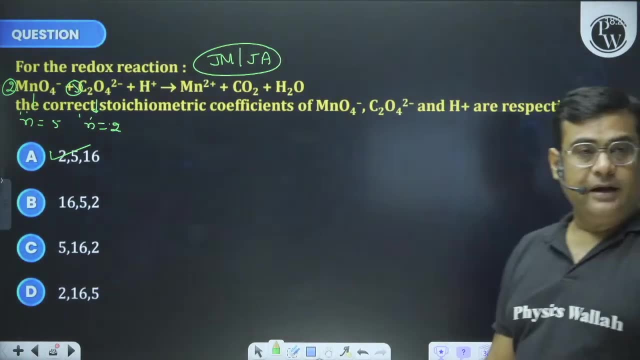 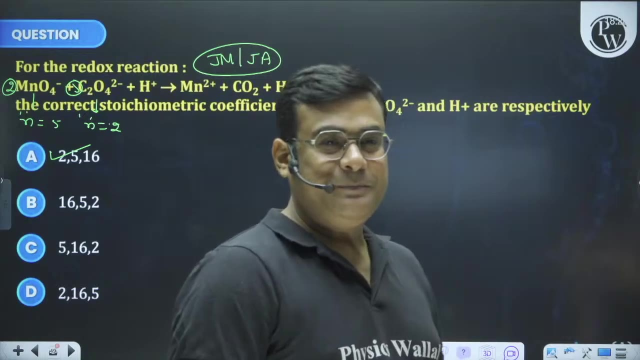 89% is not a bad figure. We are feeling something good already. We are feeling something new, so much more a chara. hey, thank you, Manisha Nirvani. sir Opie, hey, dill, hey, it's not my repair. your army 3.0 k jello, chalo, chalo. 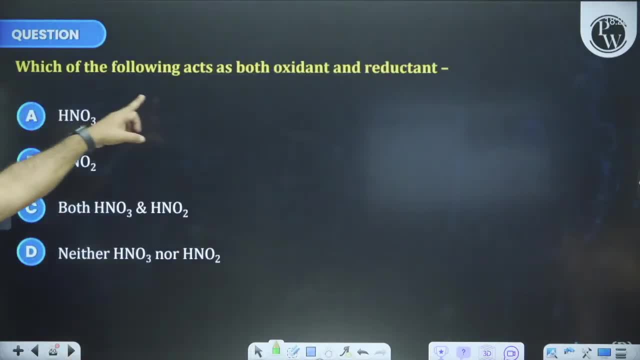 ticket or birth a much to move. a question, Barbara k Karan. a visual following act is both oxidant and deducted. you know, HNO, three men night, one up me plus five. oxidation number may have a show, Joe, maximum hey or maximum head to, but so you say over Jahi nice, Akhtar hey, so you give a local kiss. 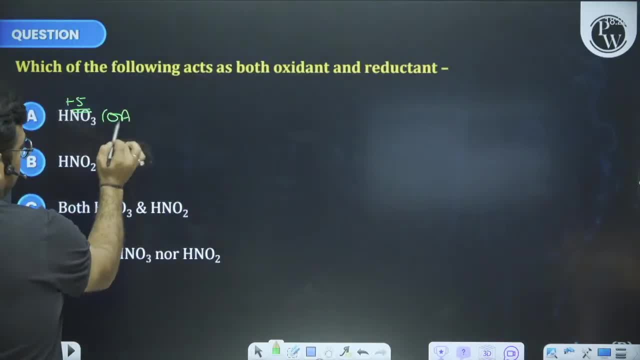 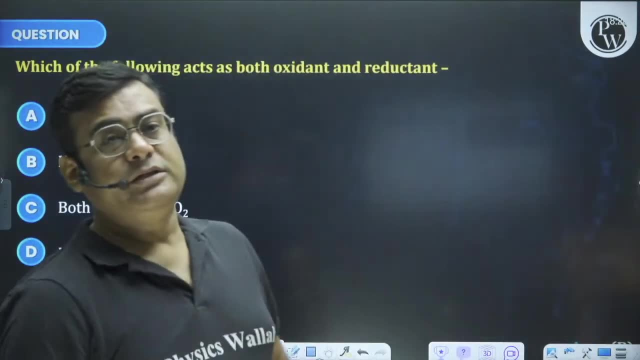 either a calm Karega oxidizing isn't I mean a be upset below beta key redox dunks a karne ka matlab, a cap key in organic be a chee ho jayaki apki in organically a joy HNO. two men at the oxidation number, which a plus three, or 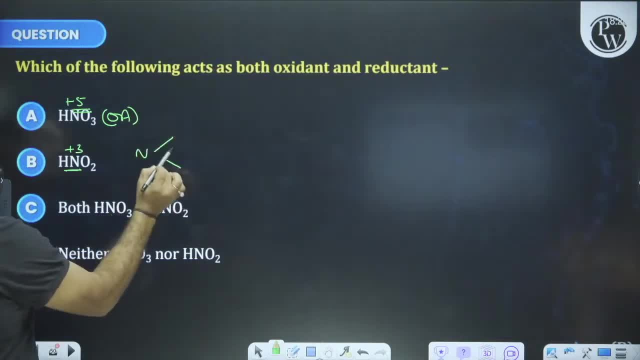 plus three may have tonight one key maximum kidney or three night one family key maximum. a surplus fight. minimum kidney minus three. you upon each a dono Jah saktah. hey, I pull a grow up. a choki ballet question could be the a but cacare with a. 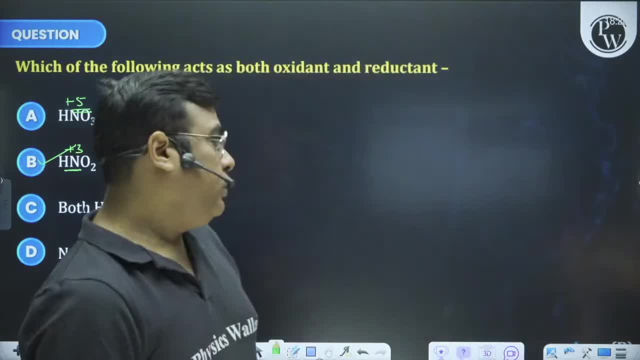 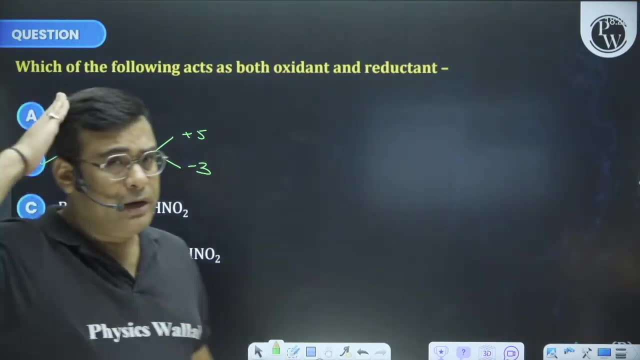 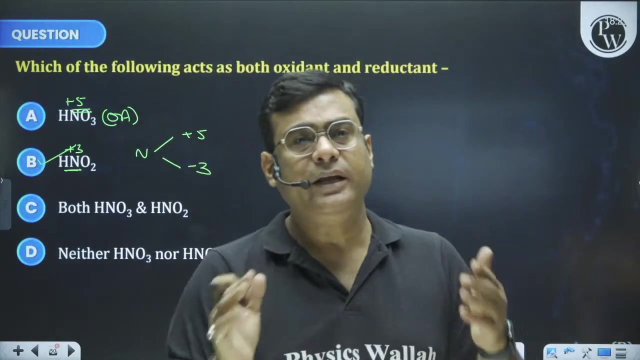 hot day in jayi man, or apne say he came a chain Joe in questions. go. excuse me, Galat karke at a beta exam. you know, pure voice, our pet upon our. a silly mistake over here. oh yeah, oh yeah, the beta. yes, I'm chalegani. no beta, yes, up chalene. 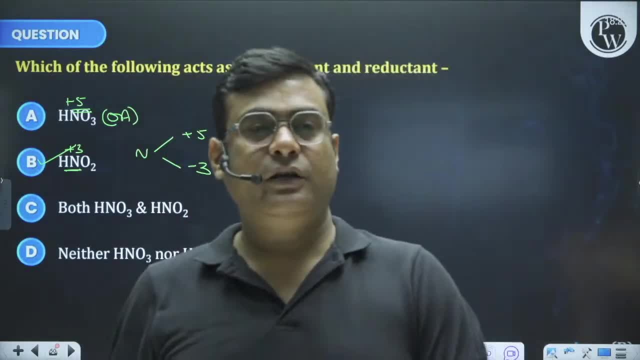 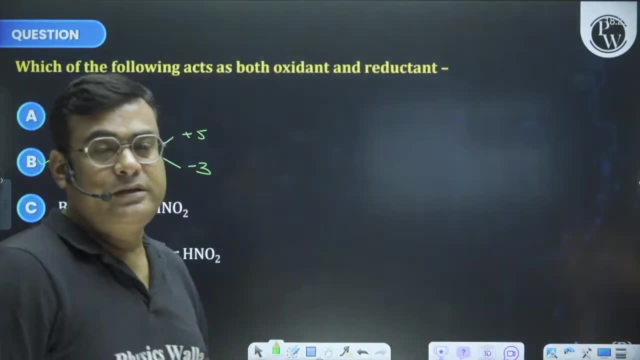 wallah nahi apkyo ki. yah, toh, apka selection. hola, yeah, apka selection nahi yoga beta up. say api koi galtian, push me on a wallah. yeah, api kiss. silly mistake, you are just a apka selection, apka person. 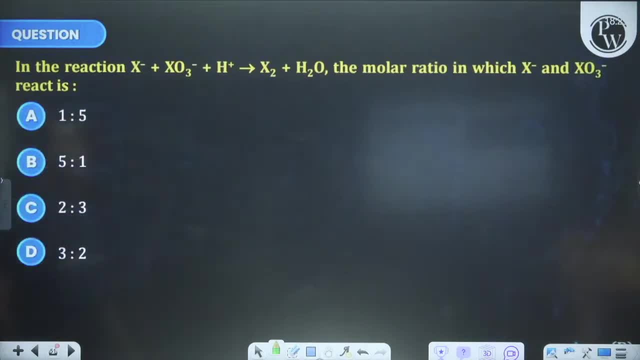 take, you are just a apka selection apka person. take, you are just a apka person. take, you are just a api kiss- silly mistake. you are just a api kiss- silly mistake. you are just a me and I in the reaction. this the molar ratio in which x minus and X minus. 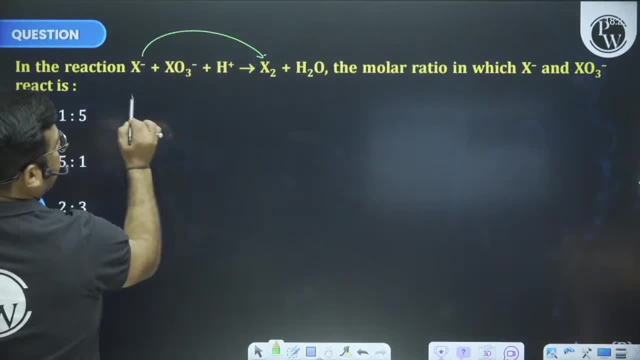 X and x- minus X, minus tracking mhajevan de kris of soft, because minus 1, minus check 0. Mgr I xo 3 minus max plus 5 May plus 5, 0 is kind factor 1 hanging and it cross multiply karajhata. h answer is 5 is to one, Connie kata. 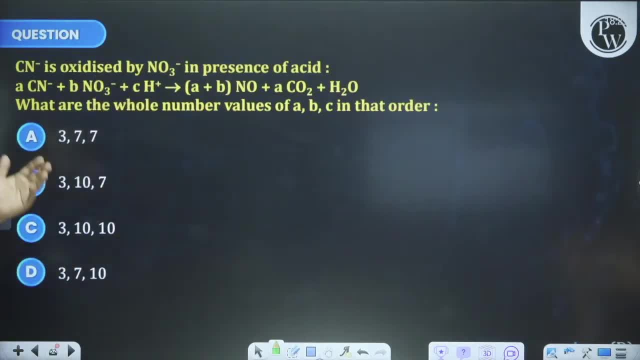 here up the key. a question for us. a mujhe lag raha hai, cha hai difficult. a dekta hai i a solar visram be hotahega. answer to a question's�a abhi sas 준 hain api kaha kiha kala. 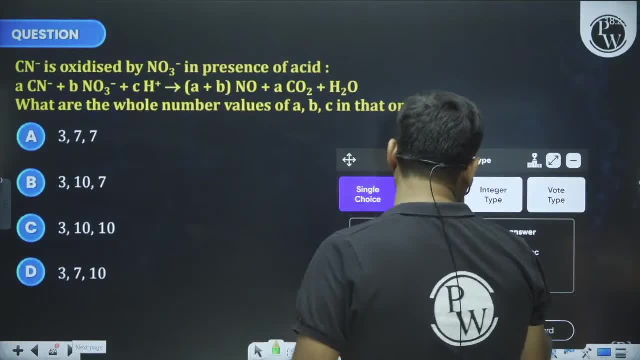 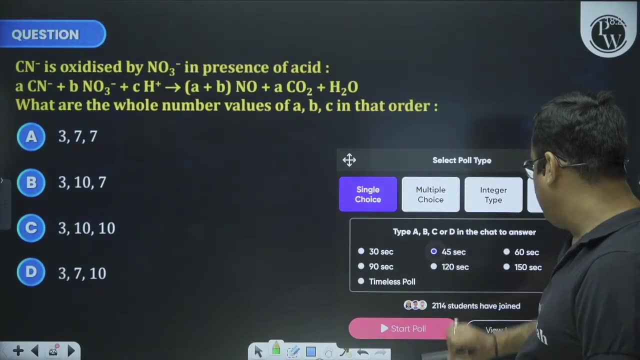 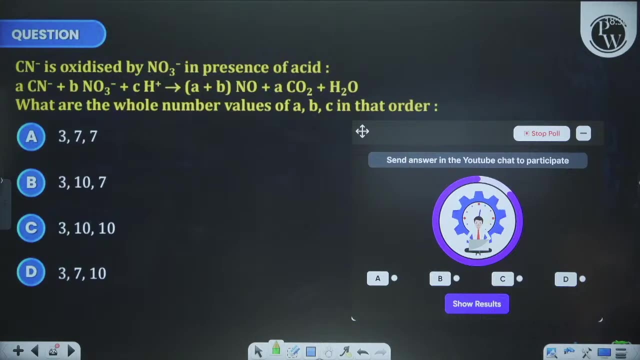 Let's see. come on, a little rest will also be done. the answer is not visible in it. so now some operator's mistake has happened. come on, let's see the time of 45 seconds. how many children do this question? to correct it. sir, my physical was weak. you have made. 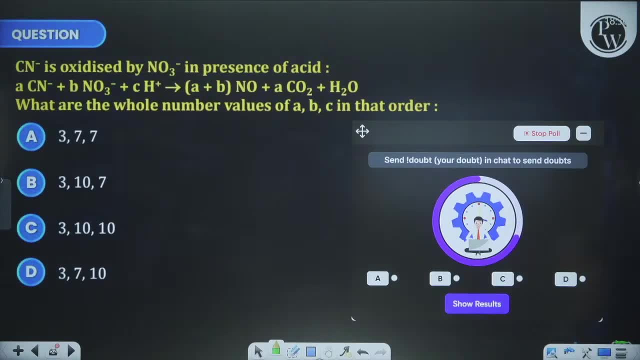 it very strong. it's a good thing, thank you. I could not read your name, so I will read it again. I'll just come to it once. I'll just stop. it's okay. it's okay. it's okay. while we're waiting, why don't they say something what's wrong? then we will. 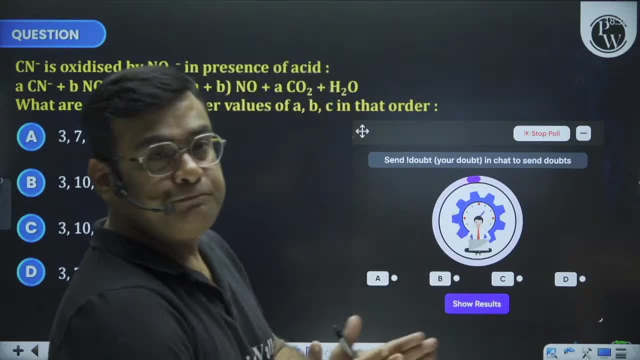 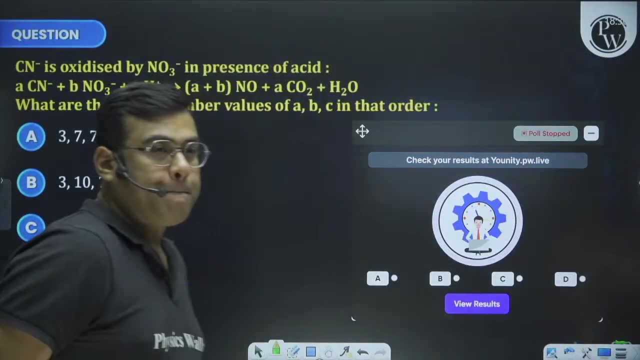 say that they have enough time. so now let's go fast. let's go fast. I'll tell you why fast. they have enough time. they have enough time, so I'll just go back. it's okay. it's See what the children are saying. the time is over. the question has not happened. the 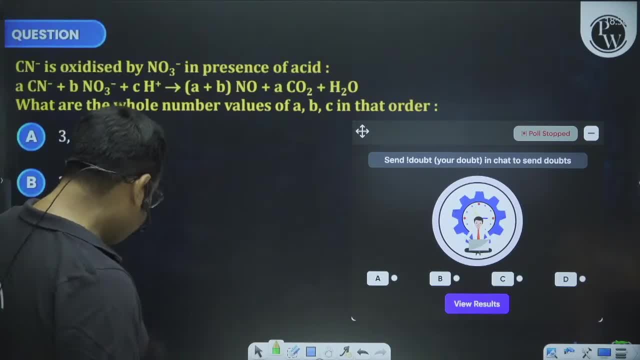 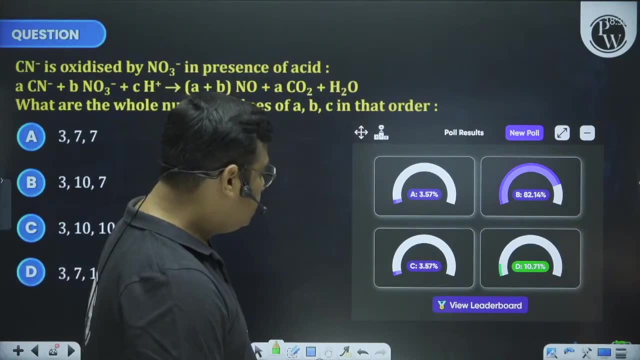 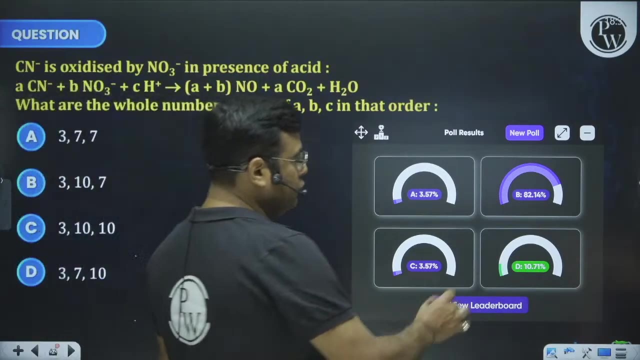 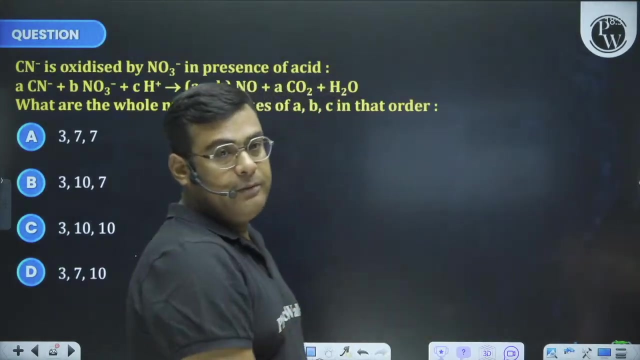 answer is D for Delhi. let's see 10%. the children are saying B. my operator did not make a mistake. 3, 10, 7, let me check it may be their mistake too. I have definitely made a mistake. it is written that it is Delhi. now let's check it once, see what. 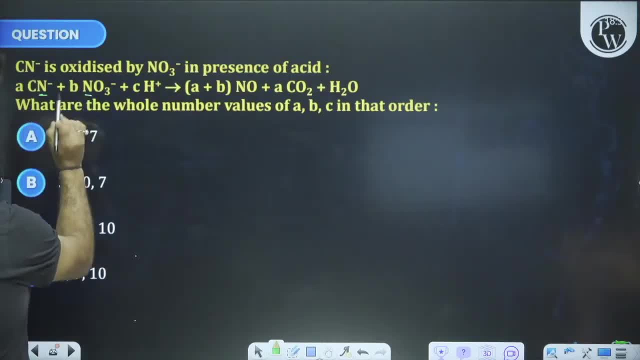 has happened in this. the nitride ion has come in two directions, that is, it has combined nitrogen and given it now there is a good role of N factor in this. see in NO3 minus in the oxidation number of nitrogen. sir, plus 5, in this plus 2, NO means, that means 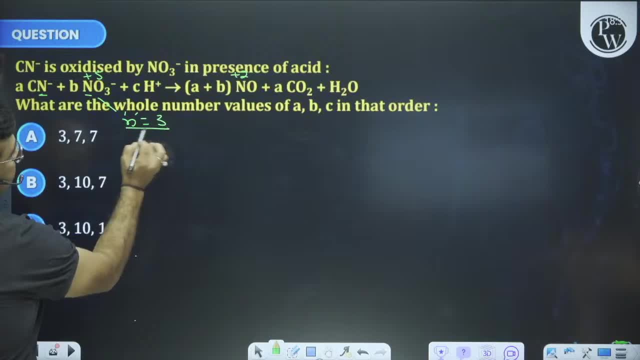 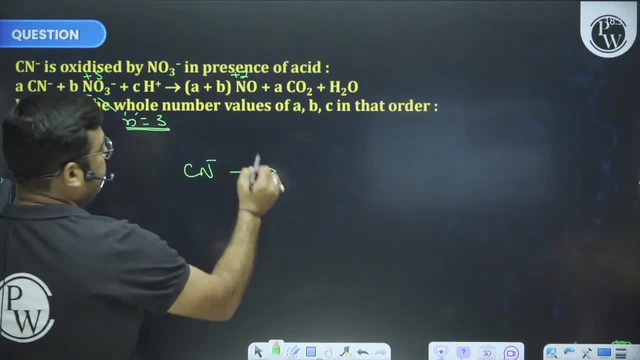 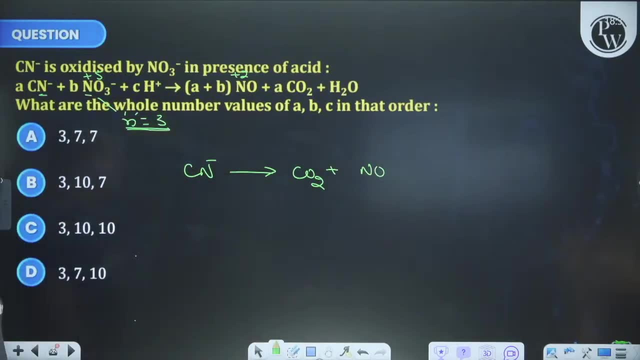 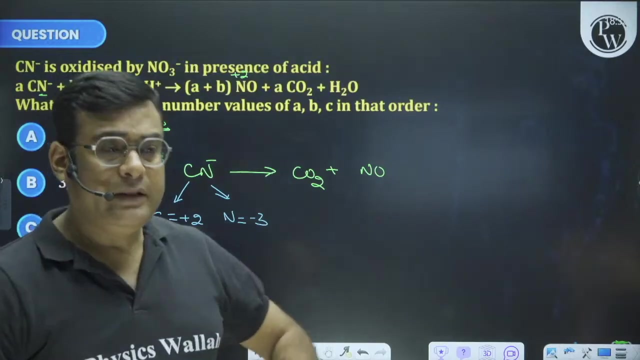 nine has been destroyed. both carbon and nitrogen are going into CO2, now you have to see this: if the carbon is in this oxidation number and in this nitrogen number, request you everyone. In cyanide, carbon is in plus 2 and nitrogen is in minus 3, it comes out of the bonding method. now there is not much time to go to the bonding method, just remember, and if you know, then it is a good thing. 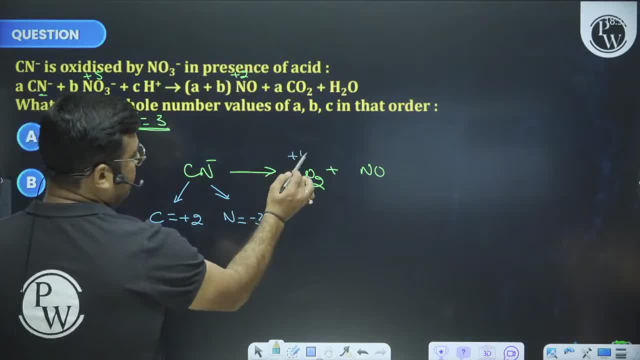 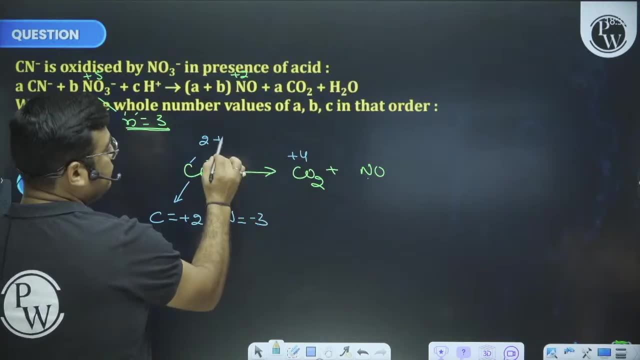 So if carbon is going from plus 2 to plus 4,, then the change for carbon is 2.. Nitrogen is going from minus 3 to plus 2, for minus 3 to plus 2, the change is 5.. 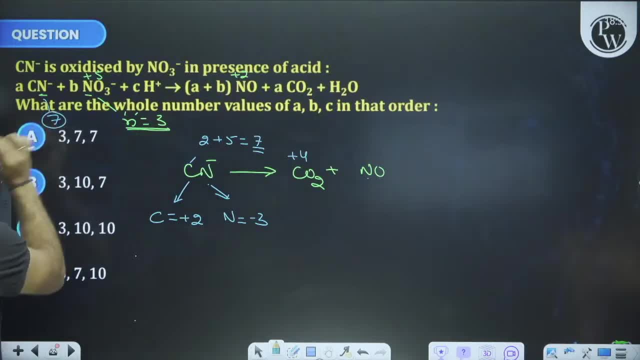 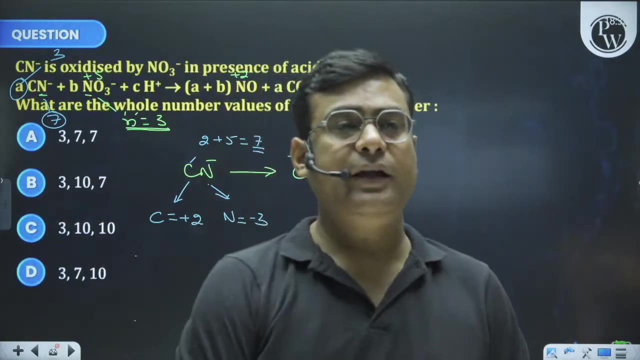 So its factor is 7 and it has to be cross multiplied. That means the value of A is 3.. Sir, why are you doing cross-multiply? One electron is loosing and the other electron is gaining. One electron will come in the left hand side and the other electron will come in the right hand side. 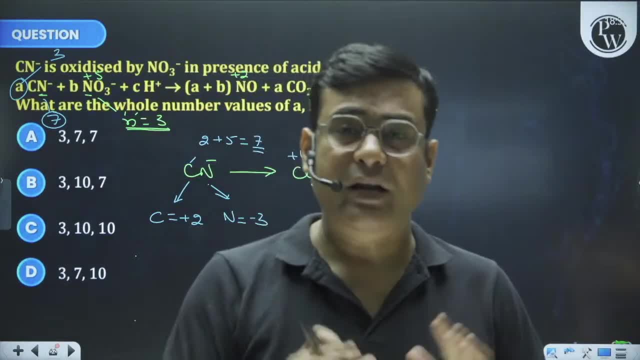 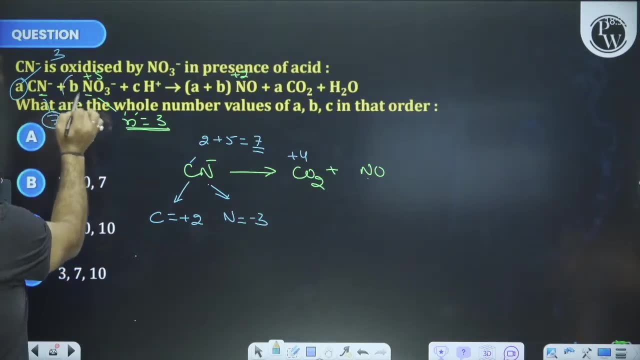 So to balance the redox reaction, cross-multiply has to be done. Everyone will know this. So that's why this is 7 and this is 7. Its coefficient is 3. And its coefficient is 7.. So it has told you A, B, C. 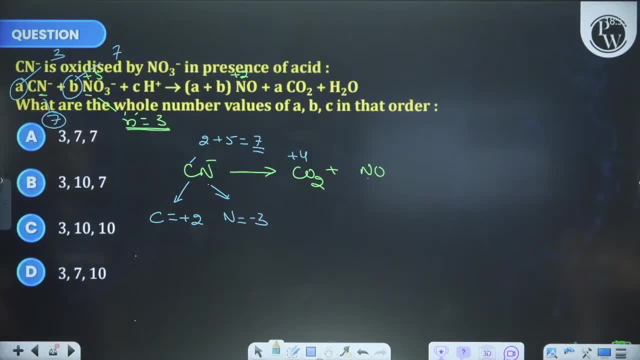 A is 3.. B is 7.. So the answer is D is correct, 3, 7, yes. Now if we are told the third value is C, So check it out. The value of A plus B is 10.. 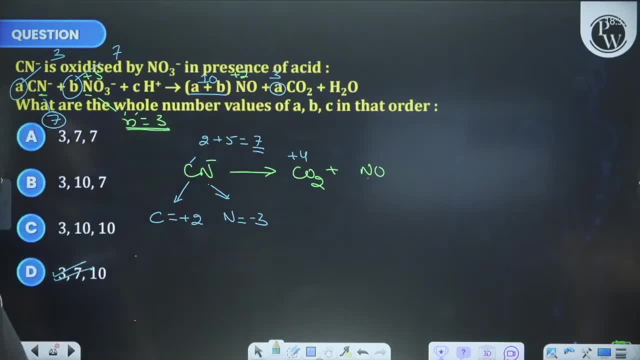 This is your 3.. Yes or no? Yes or no, Yes or no? Okay, And now check it out. What else will we check? Check it out, Check it out, Check it out. There is room 40, point 10.. 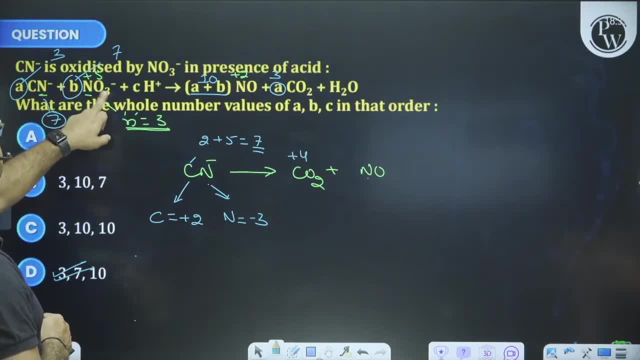 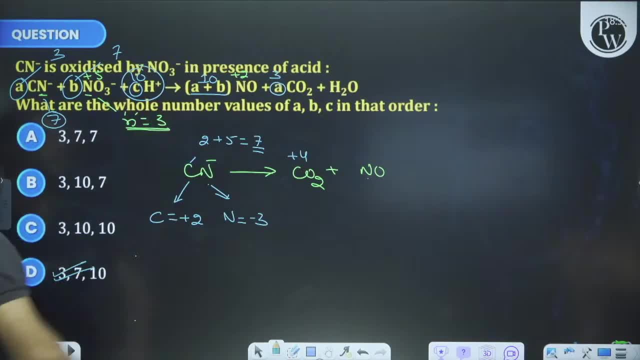 SPEAKER 2 is lying on the 2 point, then your cell is comparatively 1 point longer here than the unconscious B there. The third of these four numbers, Yes & No. Yes, and what do you have? 2,5,6,. here are. 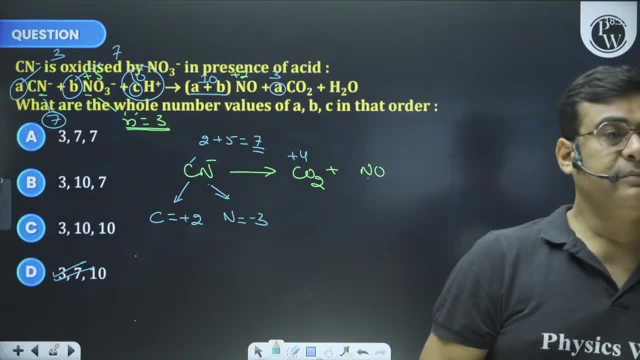 yes & no, Otherwise No. Also, you can book a quick morning nossos classes where he explains our English course. Yes, and cooling, I think, can get smooth. Thank you, and This is the question I would like to discuss in the next episode. 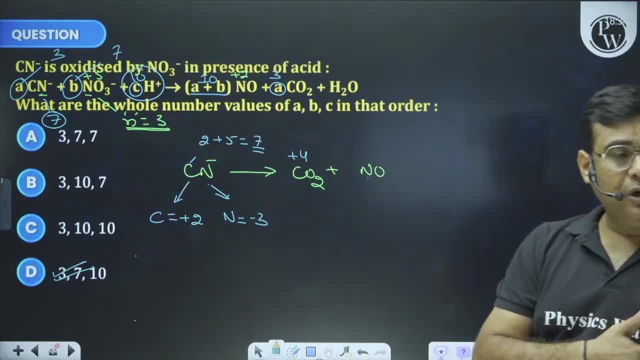 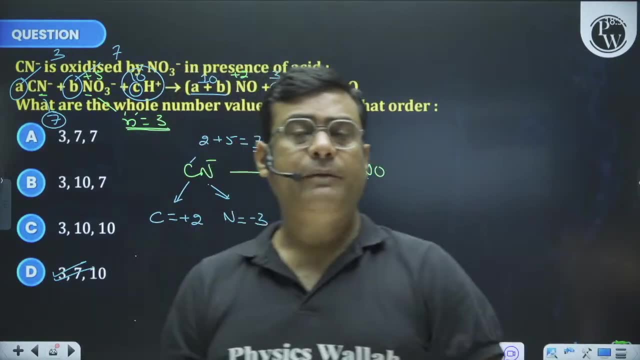 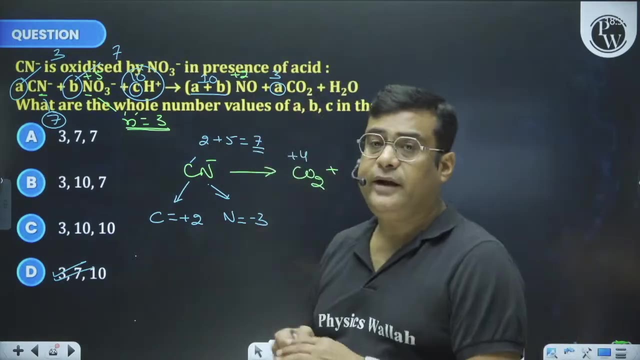 one day. No, thank you. thank you. It might be possible. it might be possible that your day is not good, you are not well, something happens. So one of the techniques of this type of question is that you can cross-check by keeping this. 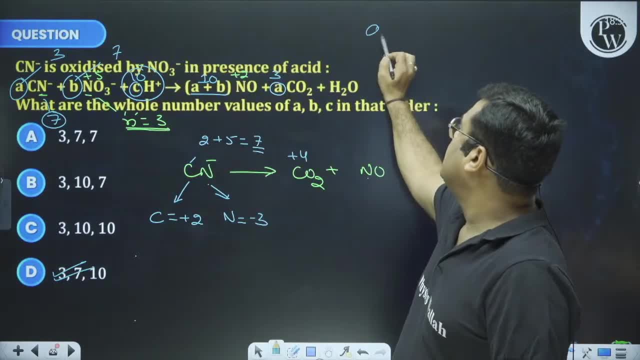 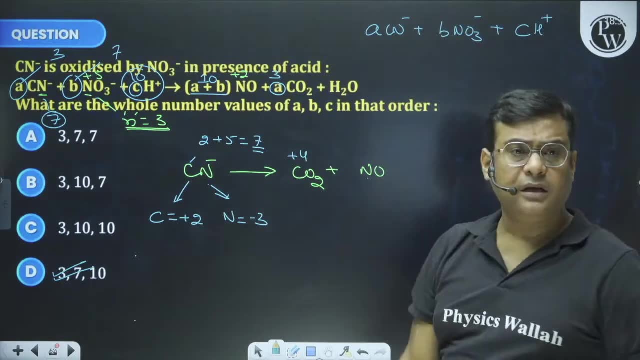 coefficient. See how, sir. what do you want to say? A is cyanide, B is nitrate and C is your H plus. God forbid. if you do not understand anything, then how to do the charge count, I will tell you on that. 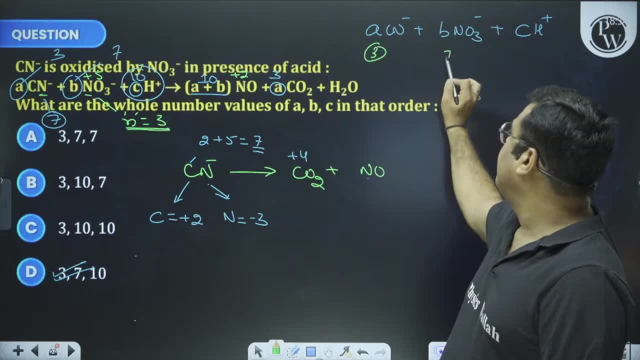 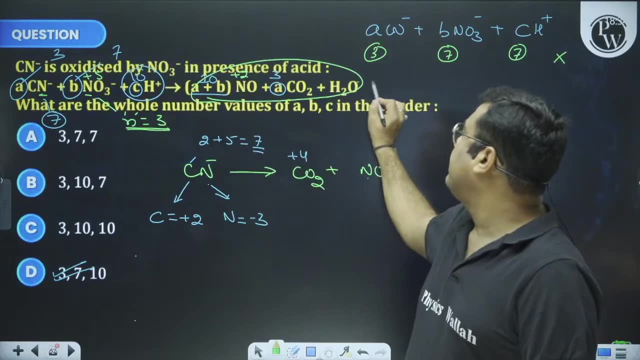 Now the first option is: A's value is 3, B's value is 7 and C's value is 7, then this cannot be done. Why There is no charge in the right hand side? then the right hand side is completely neutral. 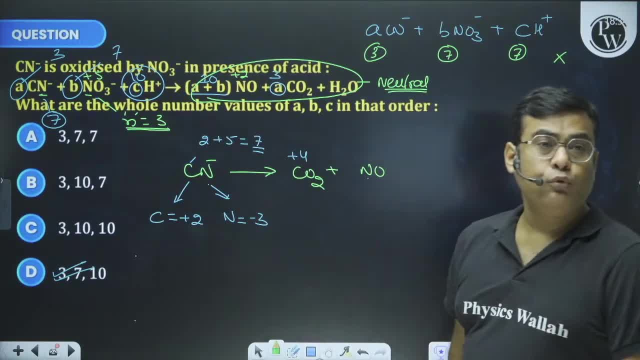 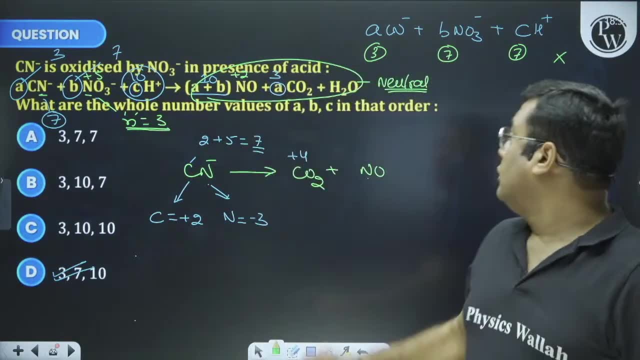 the right hand side is completely neutral. the right hand side is completely neutral, okay, So this means that the positive charge should also be negative in the left hand side. so this is a negative charge. so now, this is minus 3,. this is minus 7,. this is plus 7,. 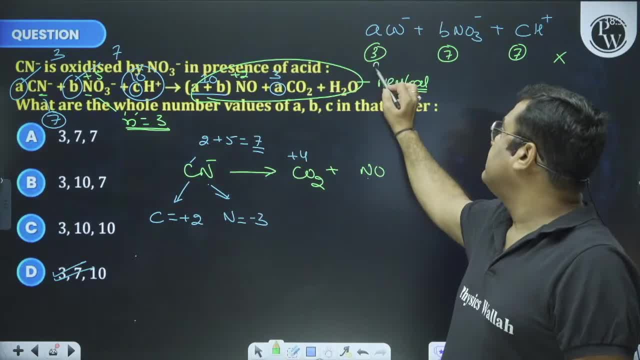 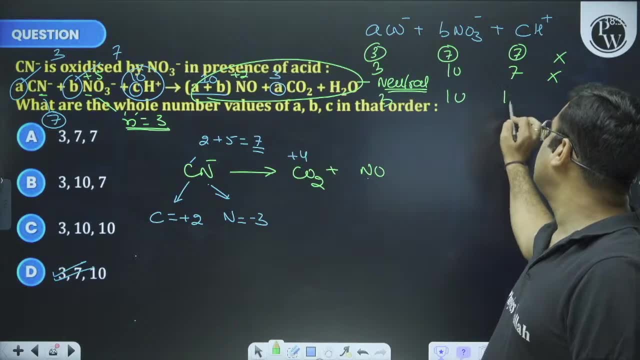 the charge balance is not happening. Next see 3, 10, 7,. there is no chance of this happening. the opposite negative is increased. 3, 10, 10,. there is no chance of this happening. the positive negative is removed. this is: 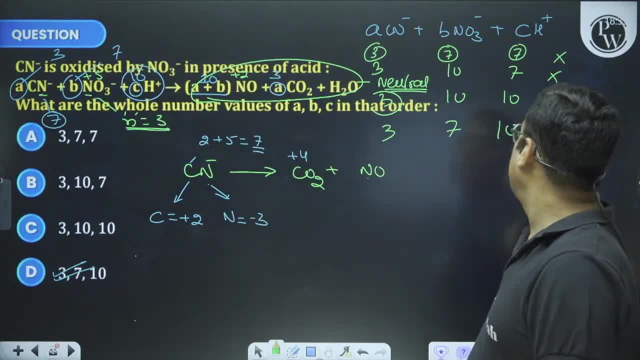 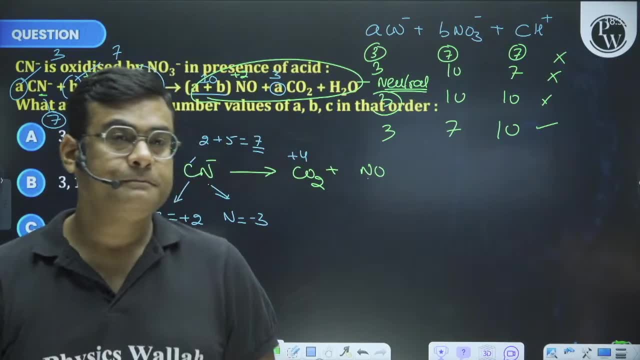 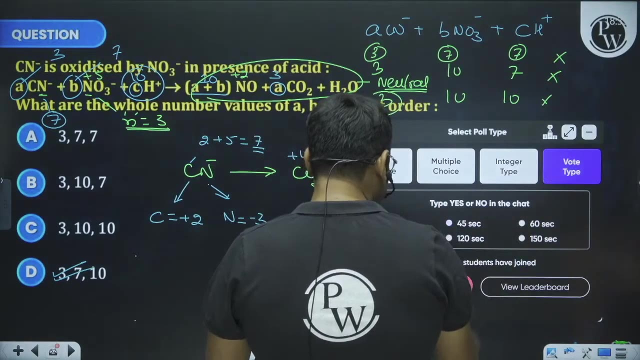 saved. So this means that only the last option will be correct, which is happening? Did everyone understand this trick? Did everyone understand my lovely trick? Tell me, tell me quickly that this question was good. the trick was also said in such: 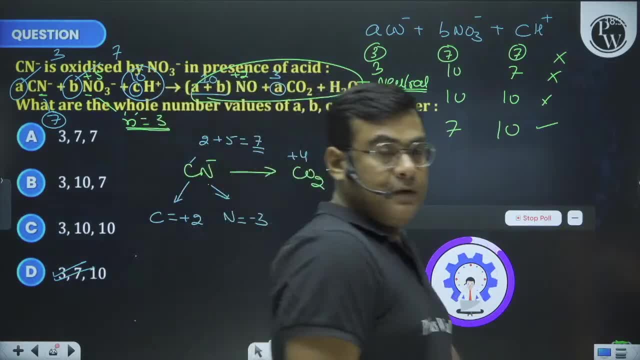 a new way. Tell me quickly my son. there is no sleep. see, you will have to stay energetic. There is an exam after 4 days. most of you have many children. some will have them after 5 days, some will have them after 6 days. your son will have to stay in the exam room, that's. 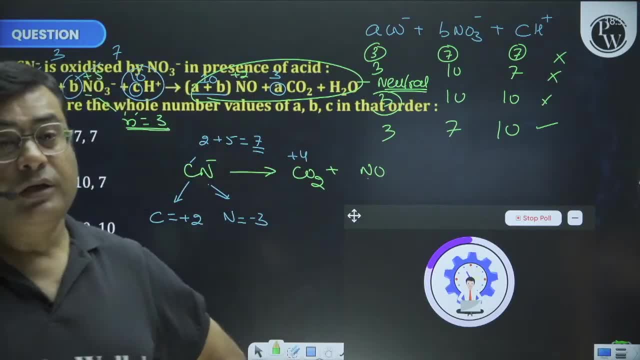 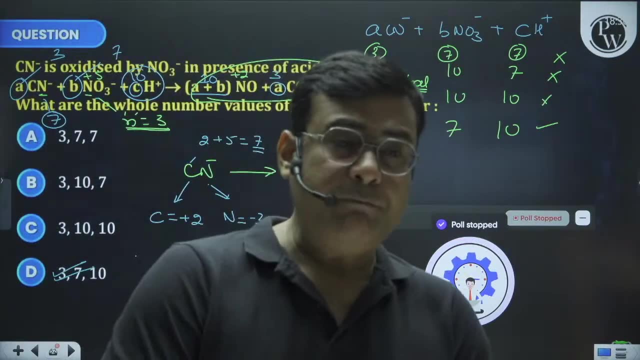 what you should do. So tell me. tell me quickly. So, brother and I am ready to give this written guarantee that you will get a question from them. You will definitely get a question from them. so did the children understand this trick and feel new? 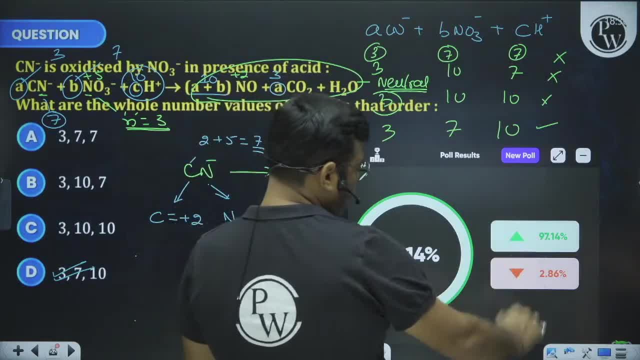 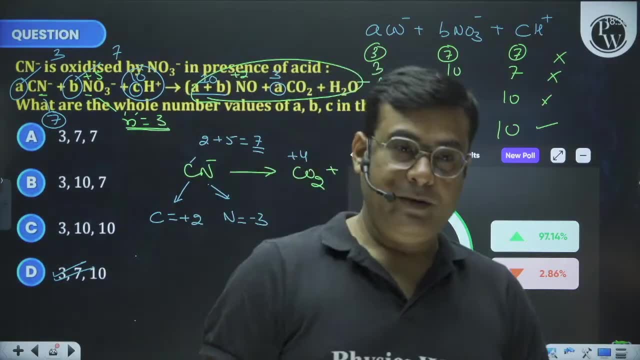 What does our poll result say? Oh, ho, ho ho. Thank you very much. Ninety-seven percent of the children are saying that the head is amazing, Thank you. Let me tell you once again the factor of CN son I just told you. 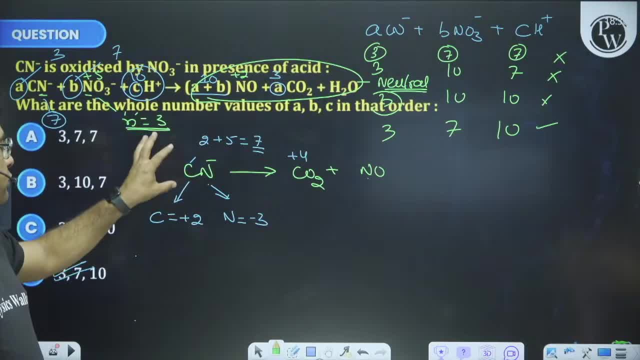 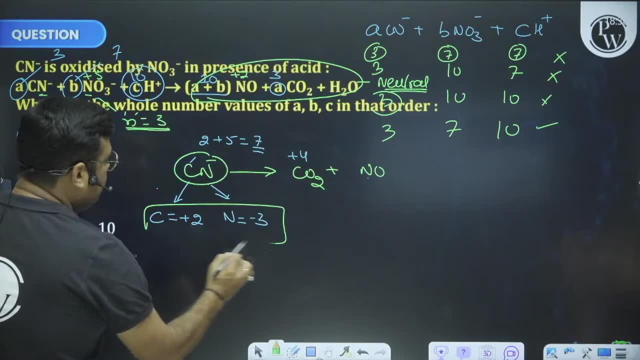 There are two elements in cyanide at once that are changing their oxidation number. and I have said cyanide in the beginning. Those who do not remember, they must remember. In cyanide the carbon is in plus two and the nitrogen is in minus three. 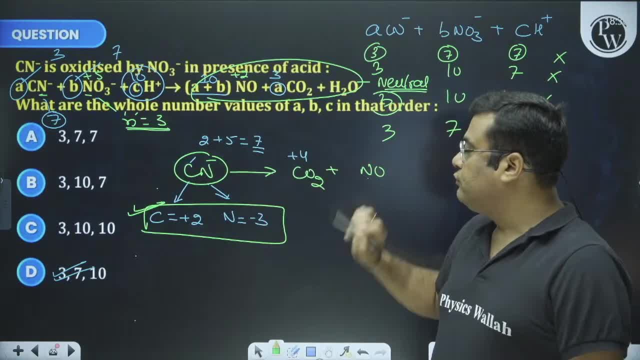 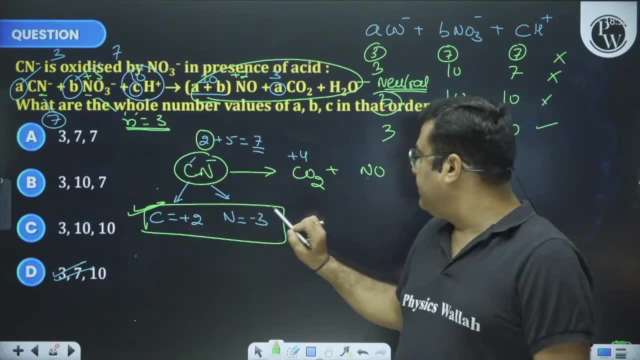 So carbon went from plus two to plus four. in CO2, plus two to plus four. Change of two, Change of two, For whom Nitrogen was in minus three, From minus three to plus two. So how much change is there from minus three to plus two? 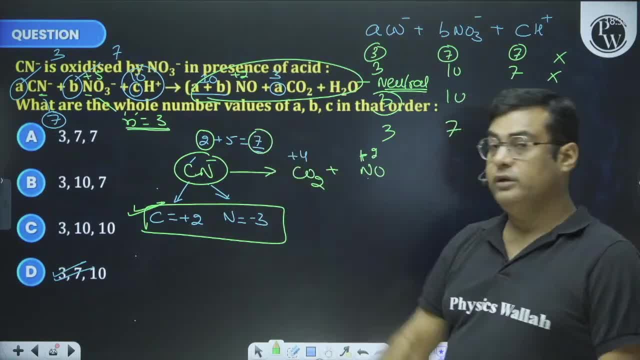 Children of five. So it is five. That's why it is seven. That's why it is seven. Okay, Come on, let's move ahead Now. look now I am telling you some questions of JEE. I am telling you of JEE. 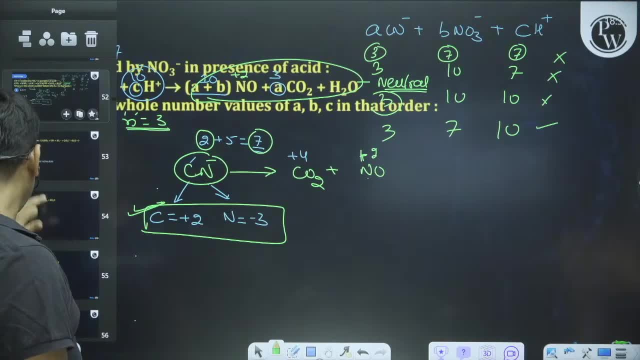 I am telling you of JEE Because there is also time. We have to move on to the next chapter. Now look such questions come: Value of N in the reaction. Children, I just said that the n factor of dichromate is six. from you right? 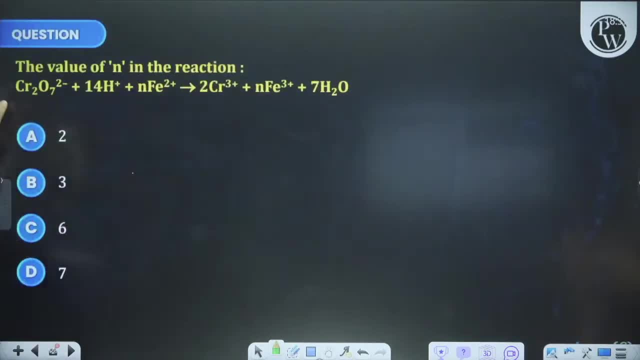 And how much is the n factor of Fe plus two One? What is the n factor of Fe plus two One? What is the n factor of Fe plus two One? What is the n factor of Fe plus two One One? 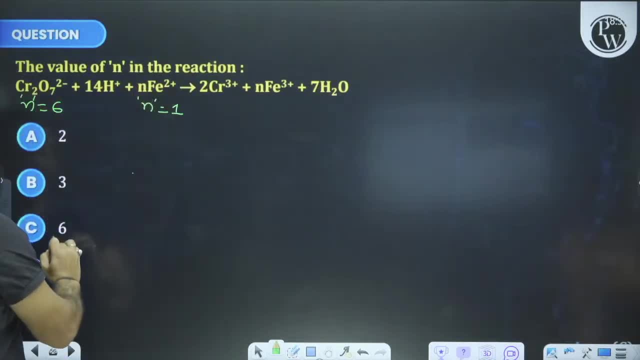 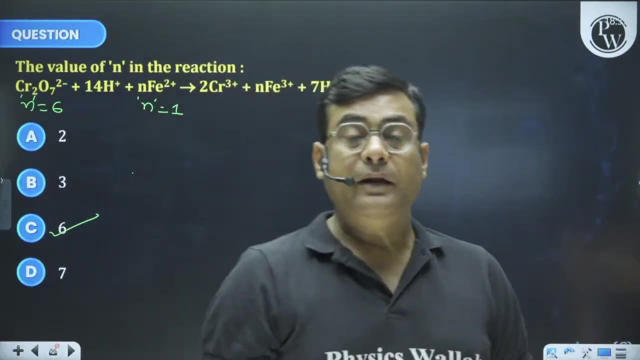 Are you there? You have answered straight in six. Now children are writing a question about redox. Sir redox, I have not understood this chapter from beginning to the end. And now, dear son, the time to understand is gone. Whatever has passed will be cut off. 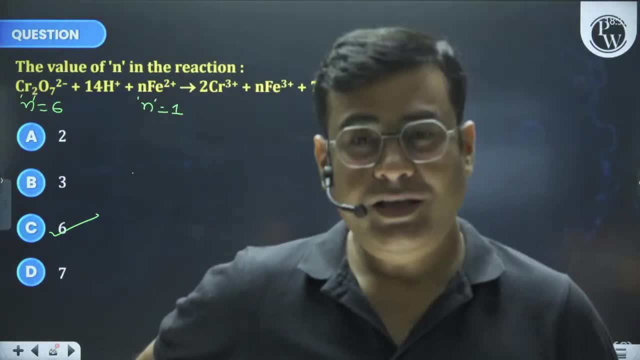 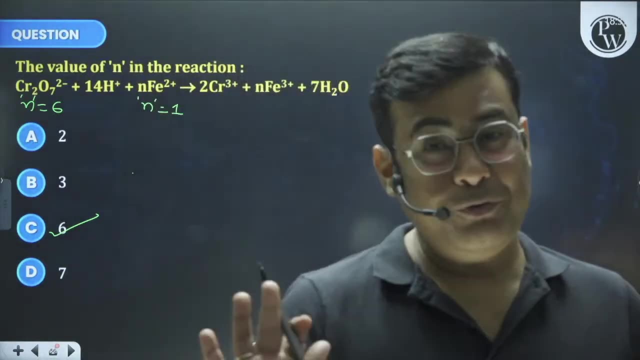 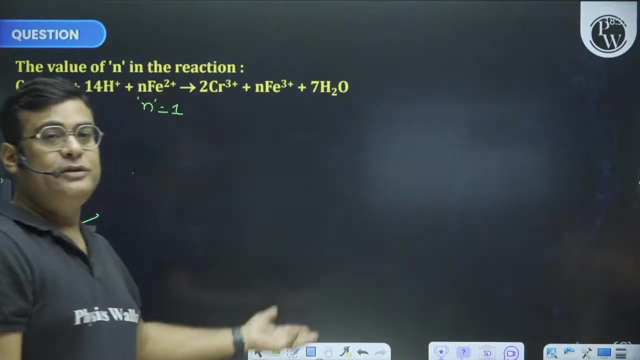 Except for you, no one else will come now. Now no one else can come. There is no one in four days who can't understand redox, so get the person. please climb, change, Wow. question is very easy to answer. 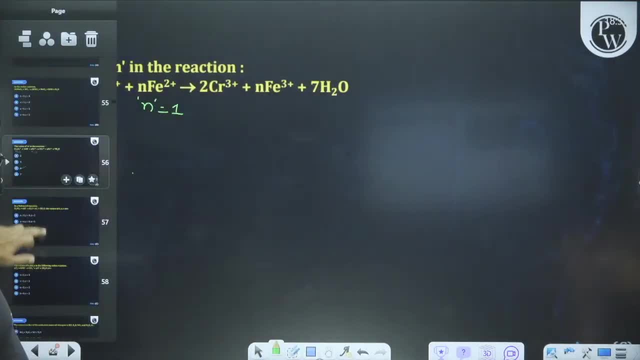 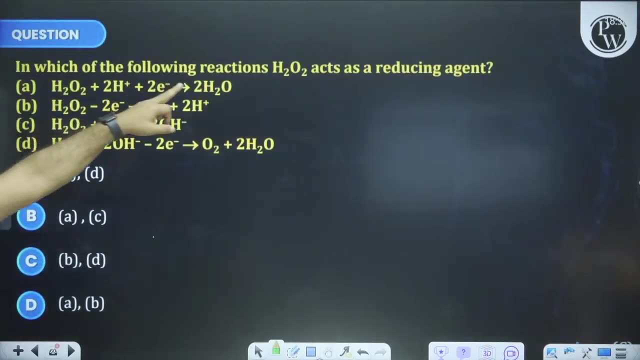 Let's see these questions. Let's see the time. Let's see the time. Now look at the questions of H2O2.. In which are the following reactions: H2O2 act as reducing agent. Now the child gets worried. 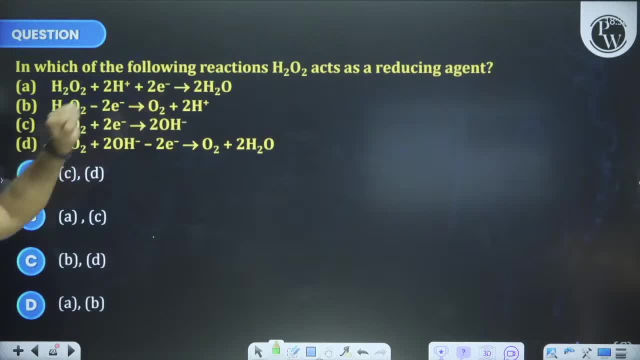 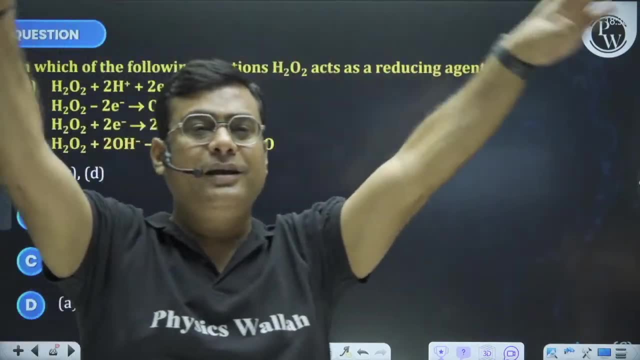 Some have electron plus written on it, some have electron minus written on it, some have electron left, some have electron right. Nothing to do. Nothing to do. If he has told you reducing agent, I have just told you the code of RO. 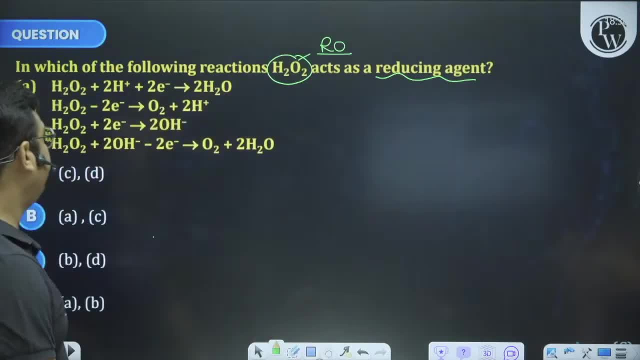 If oxygen is visible, then reducing agent. Is oxygen visible in A? No sir. Is it visible in B? Yes sir. Is it visible in C? No sir. Is it visible in D? Yes, sir. The answer is C. The story is over. 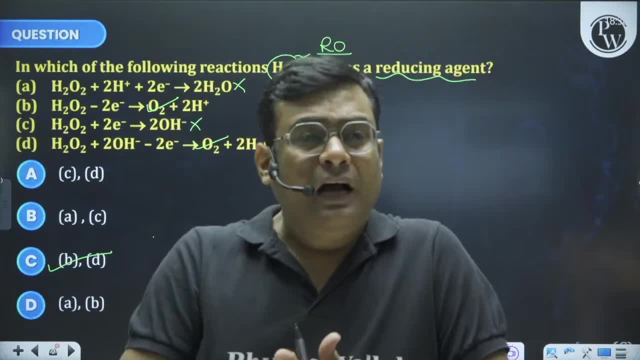 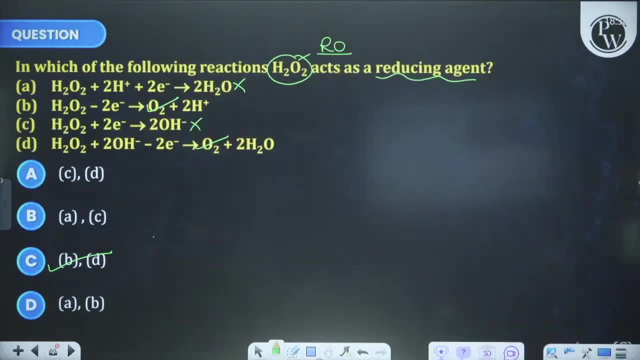 Now this question also. I know that even today you don't have to do it. I have told you such a lovely trick that after this trick you will never have any problem with the questions of H2O2.. You will never have any problem. 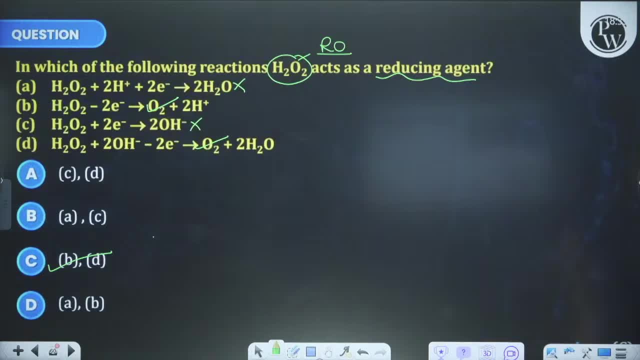 with the questions of H2O2.. No sir, No sir, I can only tell you this much: Remember this trick of H2O2.. No question in the world can be wrong. Okay, And if you like things, if you are enjoying it. 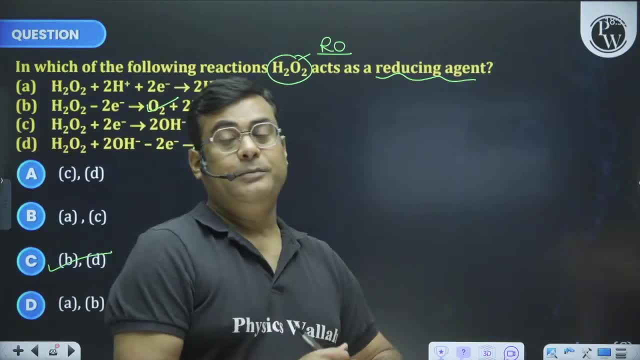 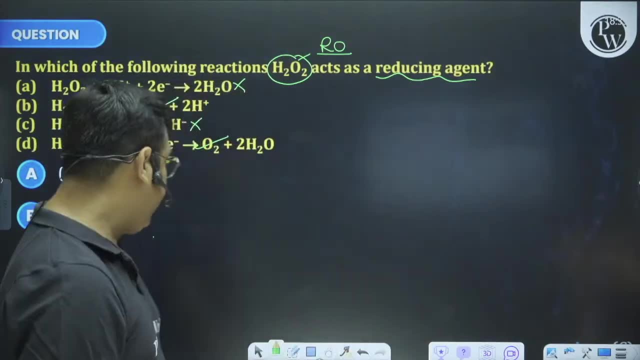 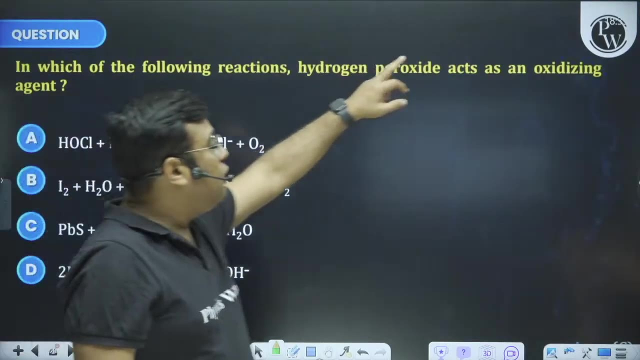 then do like it. I don't know how many children are watching me, listening to me and following me. I will see the likes at the end. Let me tell you more about H2O2.. In visual following reaction, hydrogen peroxide acts as an oxidizing agent. 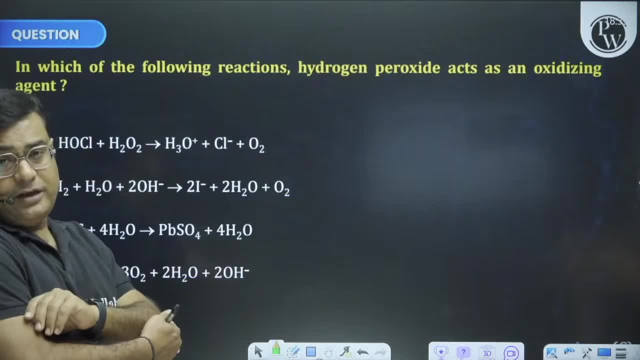 Now children. it is said to be an oxidizing agent. It means that O2 should not be visible. First O2 is visible. Second O2 is visible. Third O2 is visible. Third O2 is visible. Fourth O2 is visible. 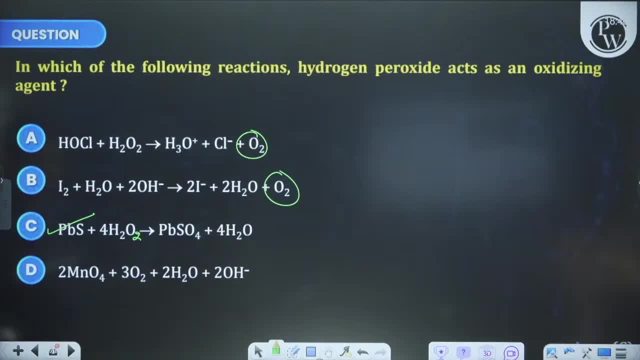 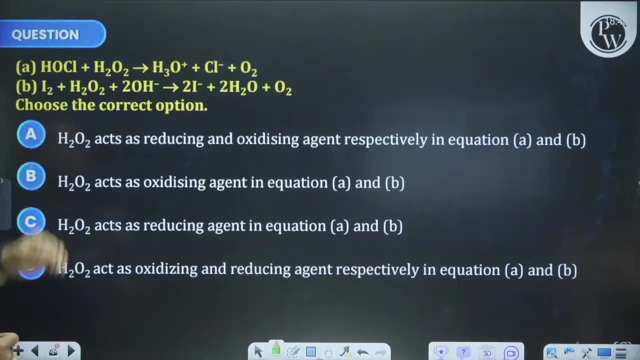 I can't do anything about the fourth one. The operator may have written the reaction wrong, But it is also wrong in this, Although it will be H2O2.. Fourth is completely wrong. So right now, what is your option? C option. 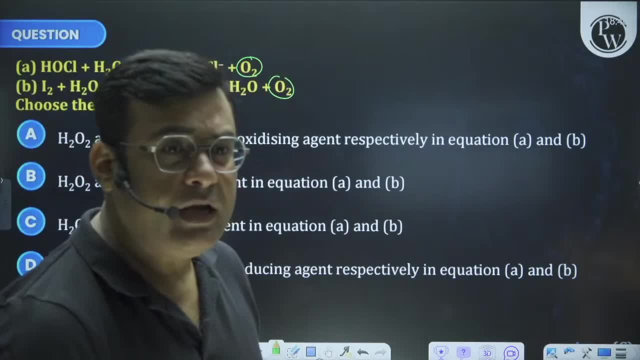 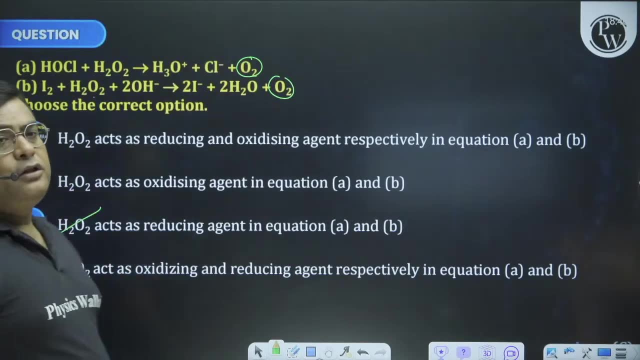 Let me tell you more. This is the reaction. Choose the correct option. H2O2 acts as an oxidizing agent in equation A and B. I have given you such a great trick And I fully hope that the 5 days paper will be. 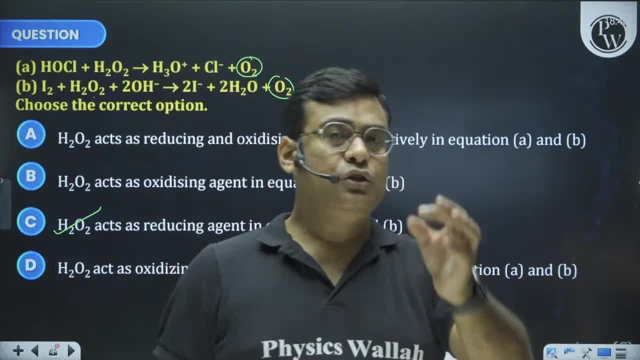 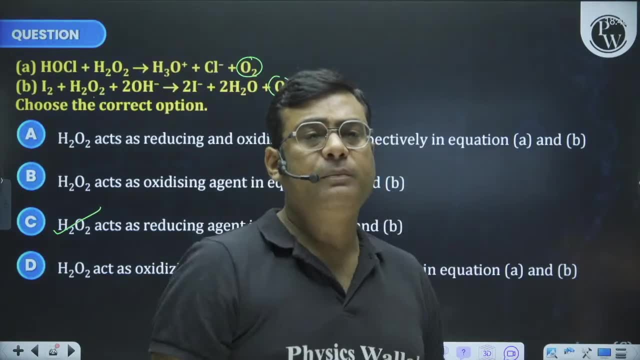 5 double 10.. Out of 10 days, someone will get the question of H2O2 again. You will get the question of balancing, Do cross-multiply. The story is correct. Is there a redox reaction or not? 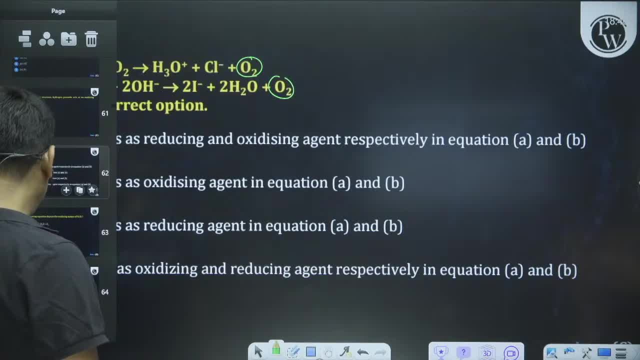 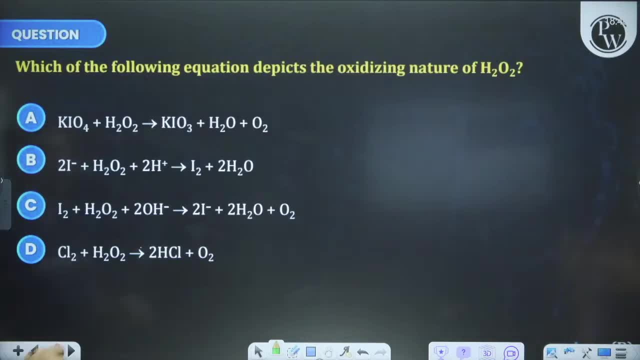 You will get the question on this. In some 1 or 2 questions you will get the answer. The following equation depicts the oxidizing nature of H2O2.. It is oxidizing nature. O2 is visible. O2 is visible. 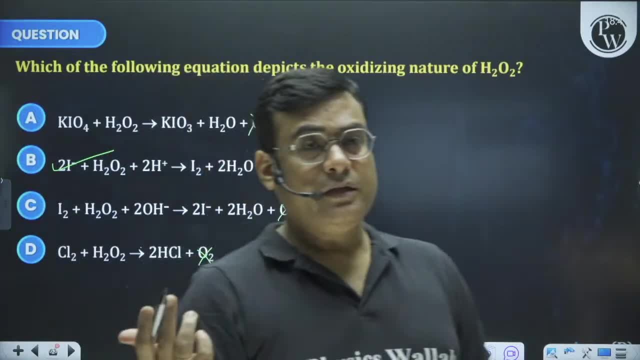 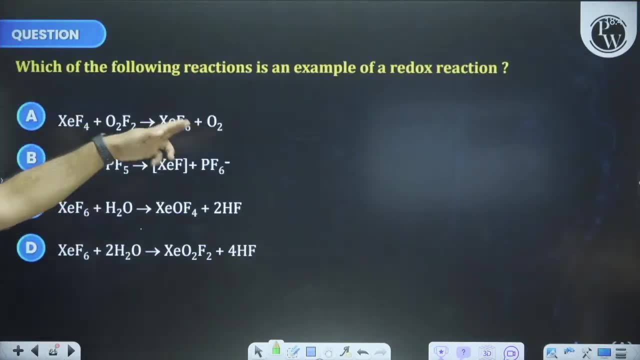 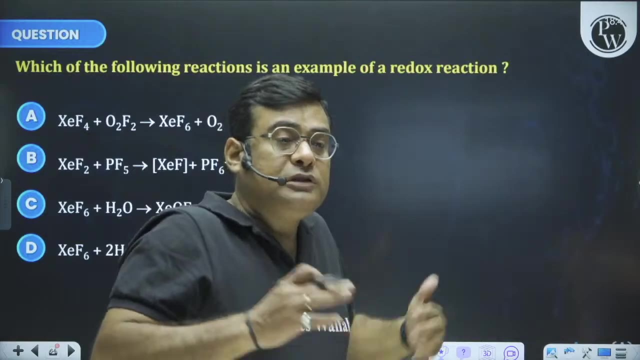 Option B is over. The story is over. It was fun. Everyone is saying with heart: Which of the following is the redox reaction? I have removed the ERVR In some questions. I have brought the redox reaction Because you got the questions. 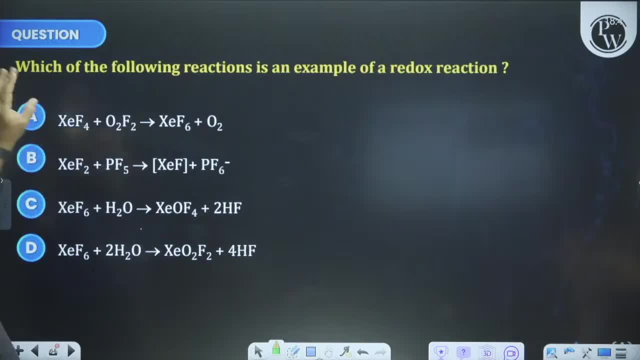 in a jumbled way. I have brought some of my own. Whenever the element goes to the compound, the compound goes to the element. That is the redox reaction. Earlier I saw the relation between the compound and the element Below. I don't need to see. 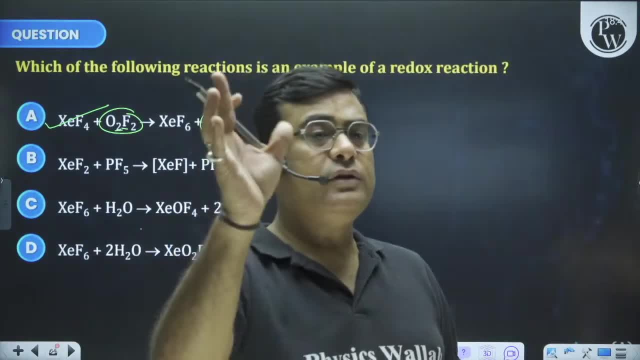 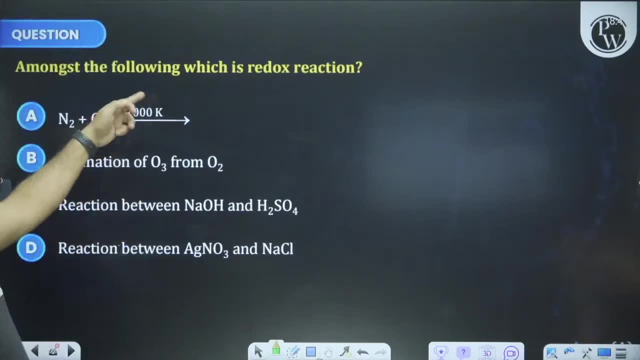 any reaction Below. I don't need to see any reaction In this way. if you put your mind conceptually, which of the following is the redox reaction? This is the question. I can't do anything. It is in the elemental form. 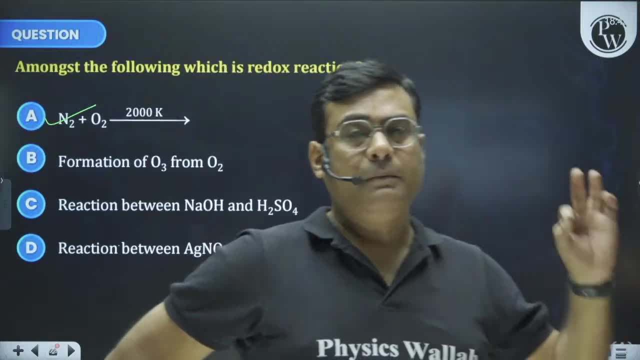 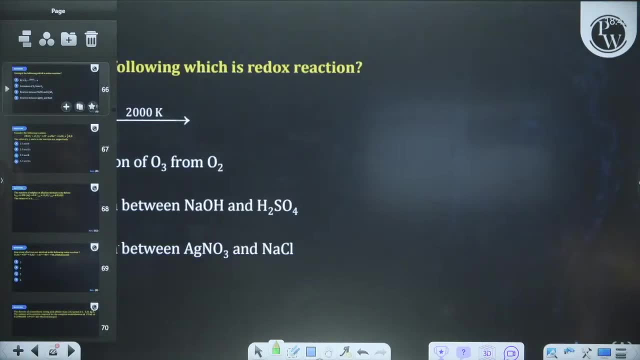 It will definitely become a compound. It is clearly written in the book of Nitrogen and Oxygen NCIT that they combine at 2000 Kelvin. So this is definitely your redox reaction. The story is over Now, you will say sir. 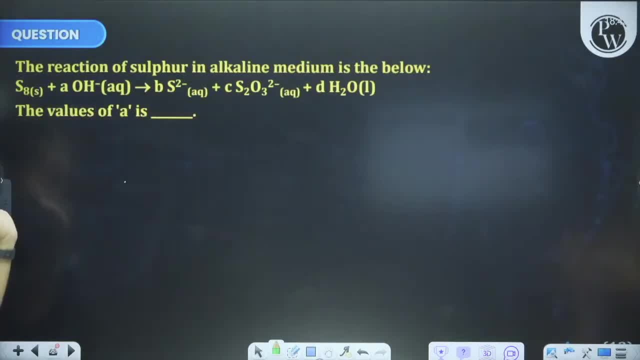 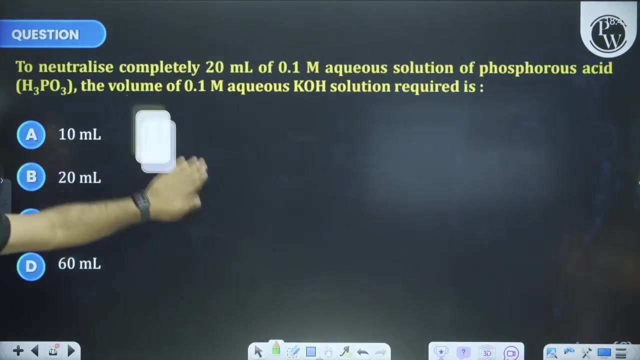 where do you get titration-based questions? Now, there are so many questions and you can easily balance all these questions with the technique I just told you You can balance it Right. Let me tell you about titration in one and a half questions. 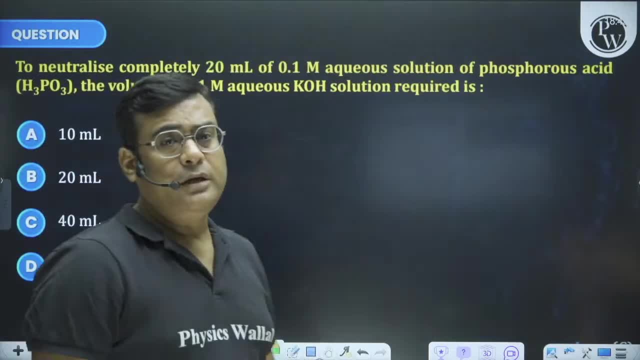 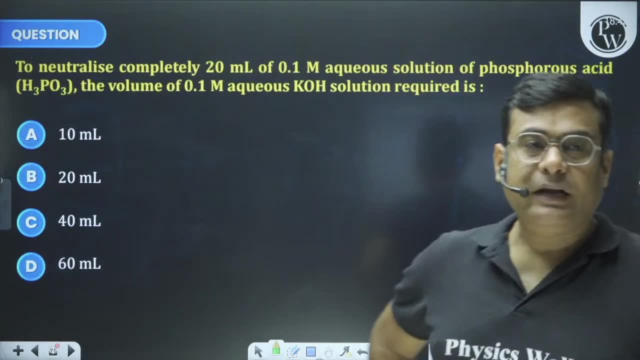 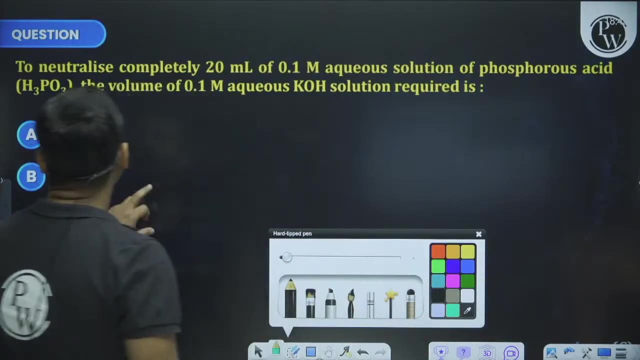 You can ask questions with the mole concept. Here you can ask questions with the titration concept. What is the difference between the mole concept and here? In the mole concept? there is no need to balance. See what is this question trying to say. To neutralize 20 ml of 0.1 molar aqueous solution of Phosphorus Acid H3PO3.. Yes, now you have H3PO3.. In the question of titration, the equivalents have to be equal And there are only two formulas. 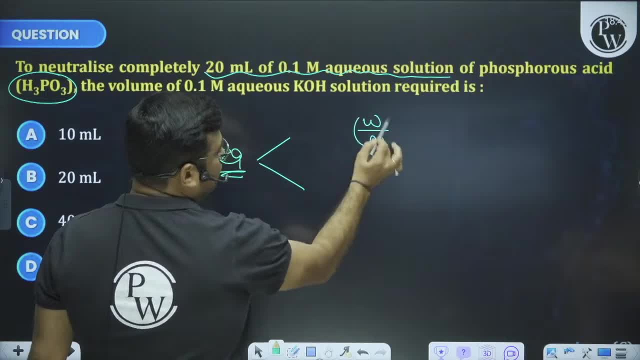 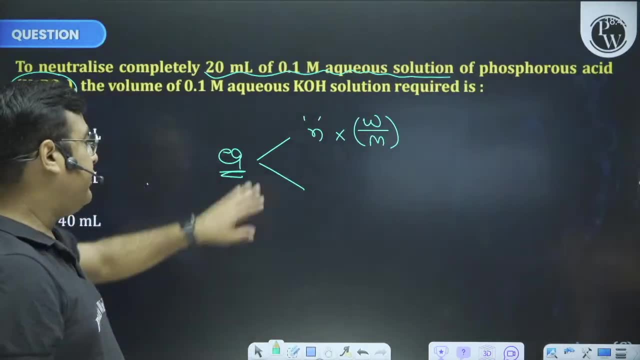 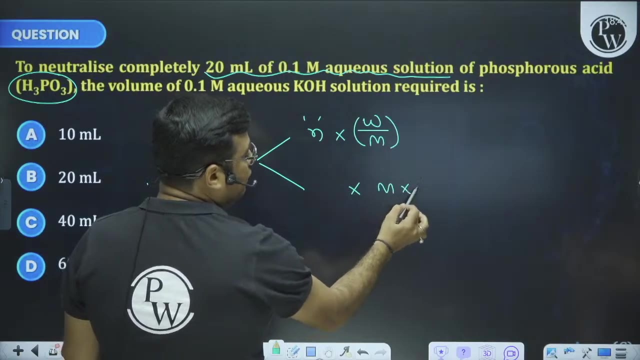 of equivalents. If the mass is given, then divide the mass by moles. What will this be, sir? Moles into N factor. N factor is equivalent. In the same way, if the molarity and volume are given, then if you multiply the molarity, 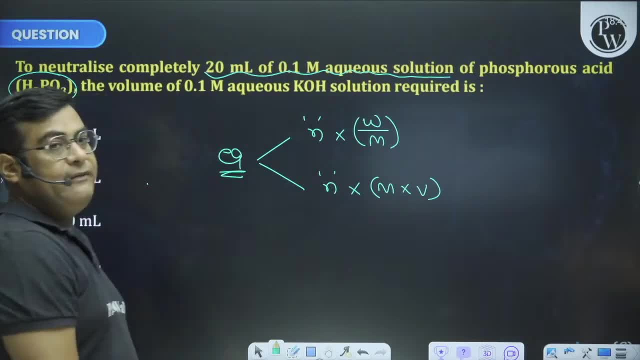 by the volume, then it will be moles. And if you multiply the moles by N factor, then it will be equivalents. Now you should know the N factor of H3PO3.. Sir, the N factor of H3PO3. 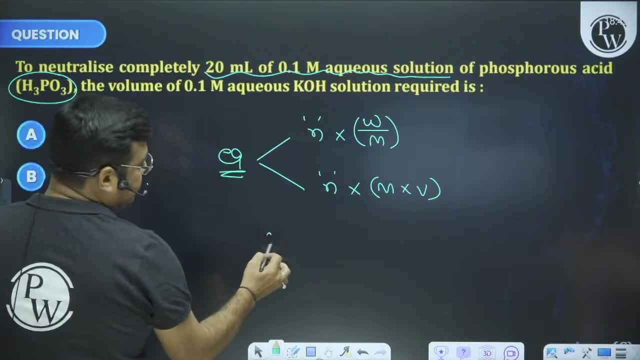 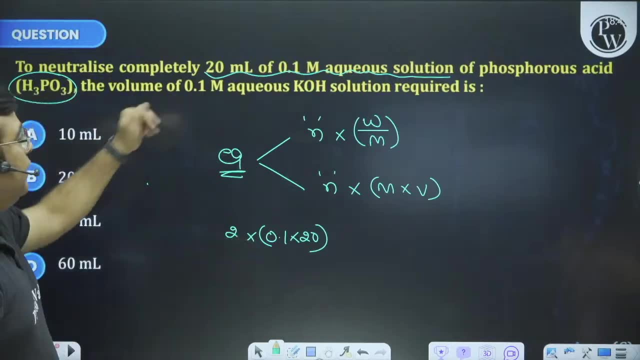 is equal to 2 of Phosphorus Acid, Sir the molarity is 0.1.. Sir the volume is 20.. And the N factor is 2.. This is the equivalents of H3PO3.. Now for KOH. 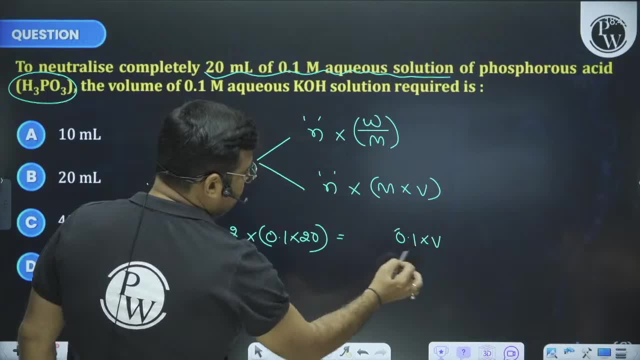 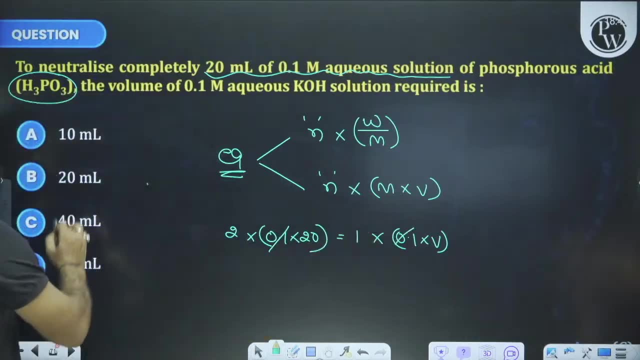 Sir, the molarity for KOH is 0.1.. The volume is V And the N factor of KOH is 1.. Because there is only one OH in it, This is cancelled. How much is the value of V? 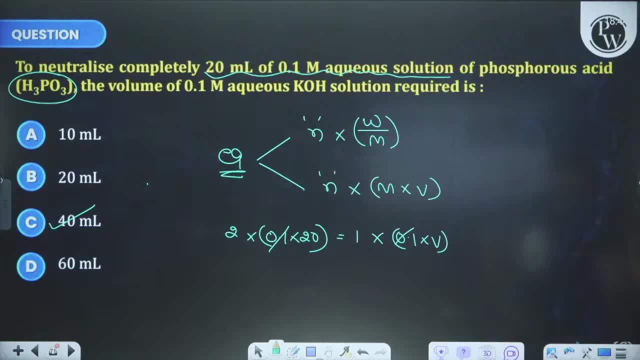 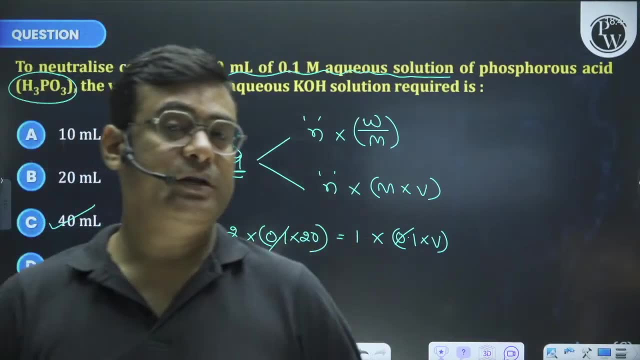 40 ml. So children are also afraid of the question of titration. See, it is natural to be afraid. But now we have studied so many times. We have given the first attempt of JEE Mains in January. We have been doing rigorous practice. 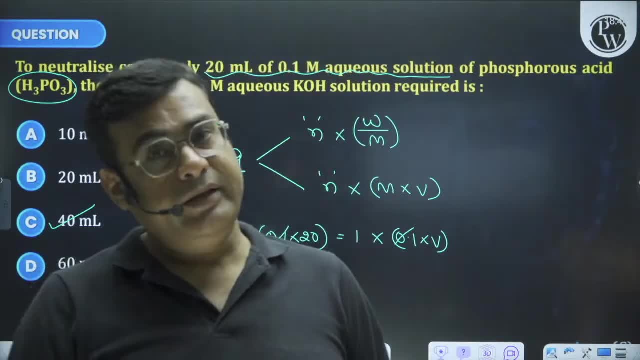 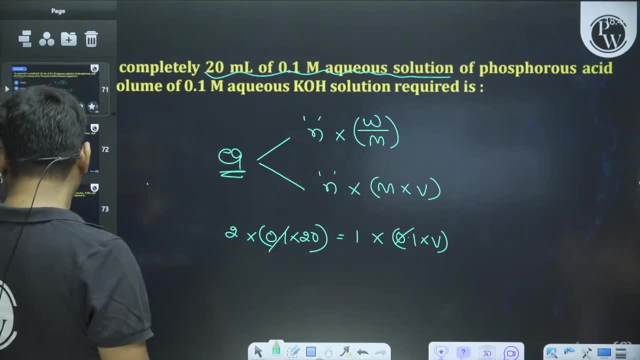 for the last two months. So now we should get rid of that fear. Now I will tell you the question of redox titration. See, this is a good question of JEE Mains. That is why I have brought it. This is a good question of JEE Mains. In order to oxidize a mixture containing one mole of it, of Paris Oxidate. I have told you that the most important of JEE Mains is Paris Oxidate. The N factor of Paris Oxidate is 3.. 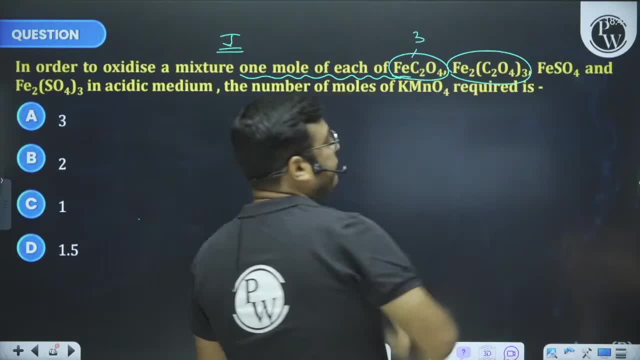 Paris Oxidate, Paris Oxidate, Paris Oxidate. You should know the name at least. You should know the name at least. Okay, I have brought tea once again. If you get a little tea in an hour, you will enjoy it. 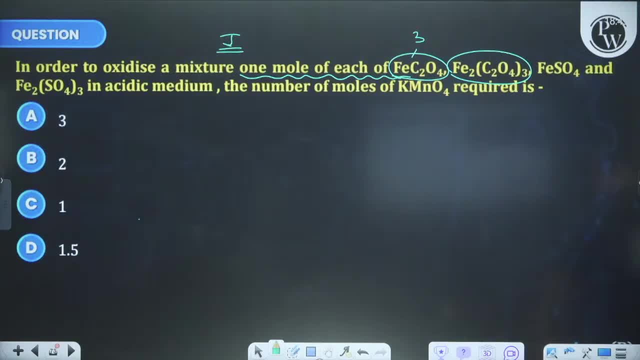 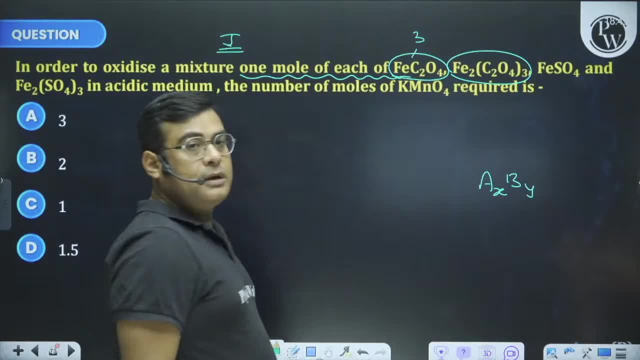 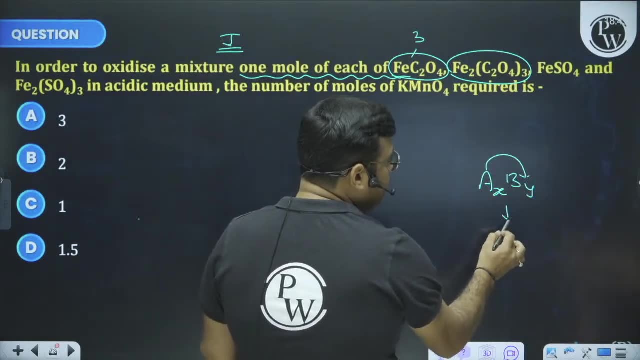 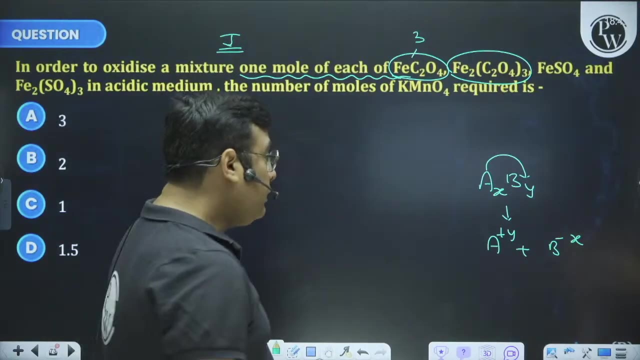 that the compound of AXBY type is. If the compound of AXBY type is written like this, then the charge on A is plus Y, The charge on B is minus X. It is opposite. So this will give you X, A plus Y ion. 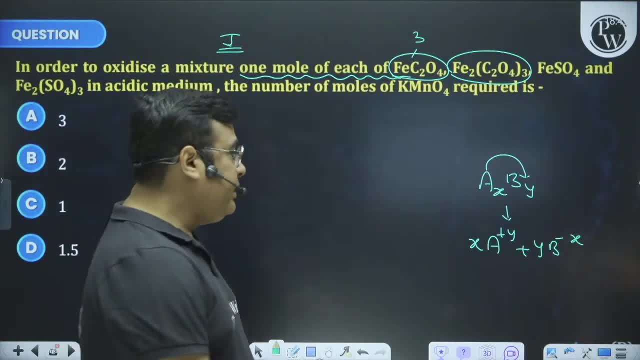 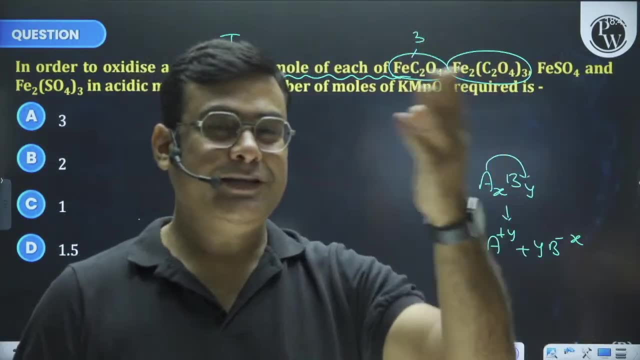 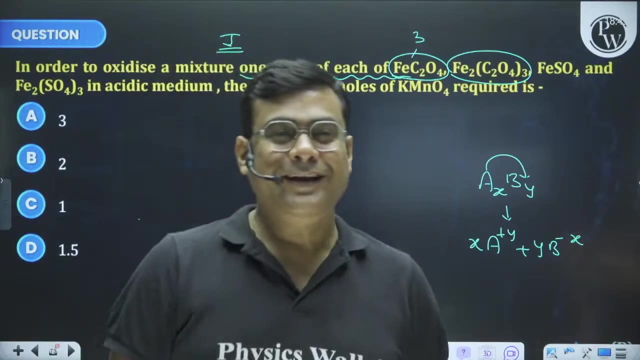 Y B minus Ion. This small thing is required. I also read in Redox. The child wrote that I am laughing. A cup of hot tea is also coming. Someone will give it to him Now. the one who will give it will not come here. 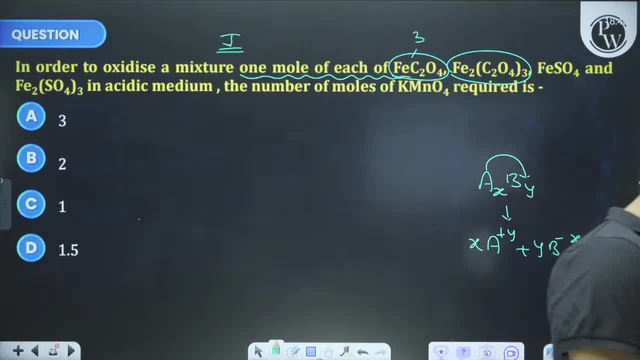 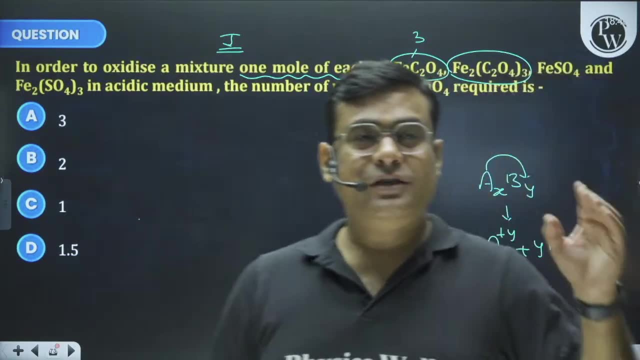 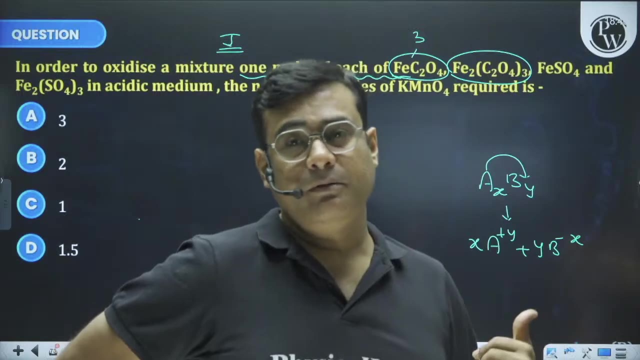 So I will have to drink it myself. So I am ashamed, You guys have embarrassed me. Hmm, I am telling you guys that this small thing is required. This small thing is required. You are reading in Redox. It will be read in the Liquid Solution chapter. 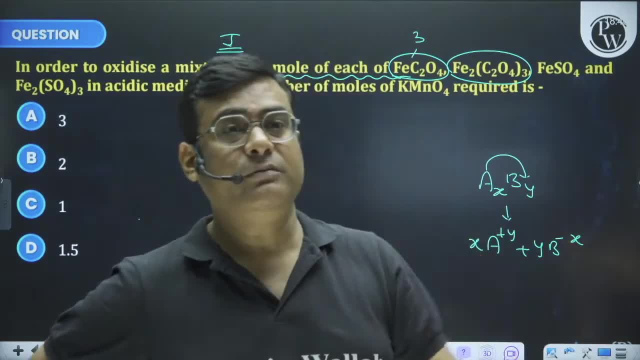 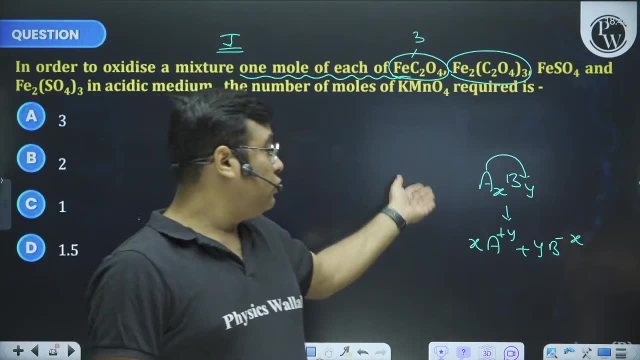 It will be read in the Mole Concept chapter. It can be read in Ionic. It can be read in Electrochemistry, In Electro. In Electrochemistry, when you study Colros law, you have to break the electrolyte in ions In Liquid Solution. 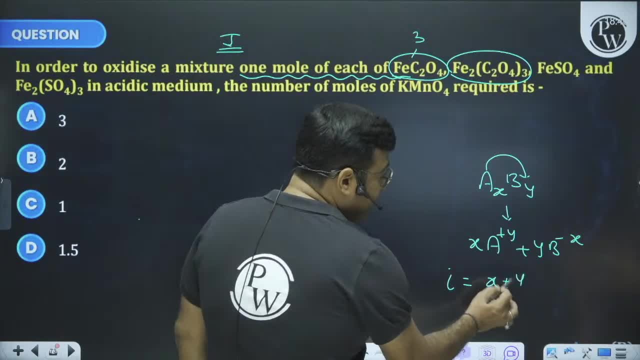 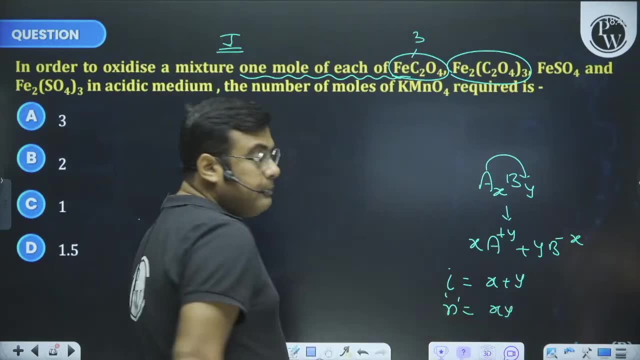 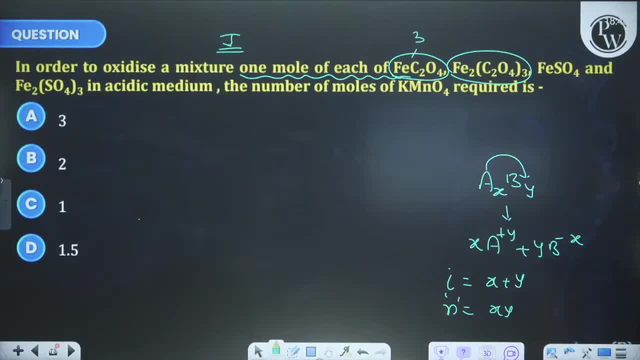 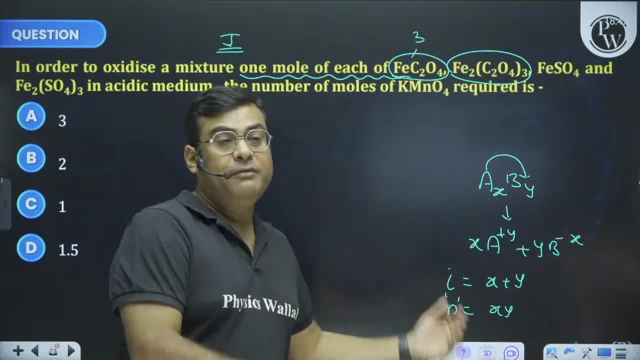 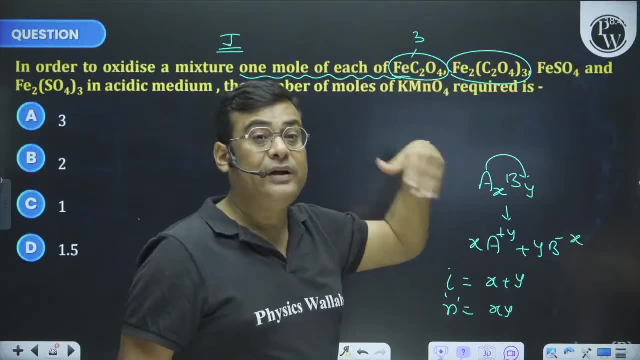 If its concentration is 0.2, it can be read in Ionic. So in this Fe is the oxidation number plus 3. And the charge of oxalate is minus 2. That's why it is ferric oxalate. That's why it is ferric oxalate. Now, in ferric oxalate, ferric can't be oxidized. In ferric oxalate, ferric can't be oxidized. ferric can't be oxidized. 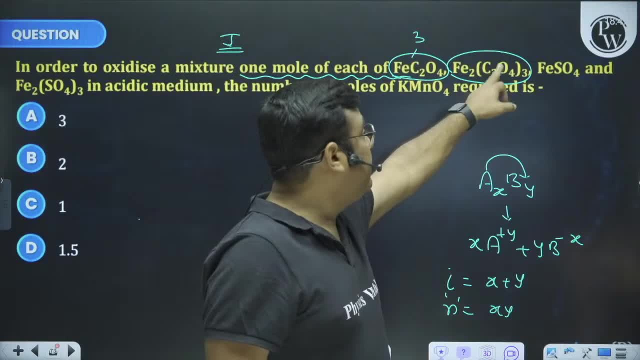 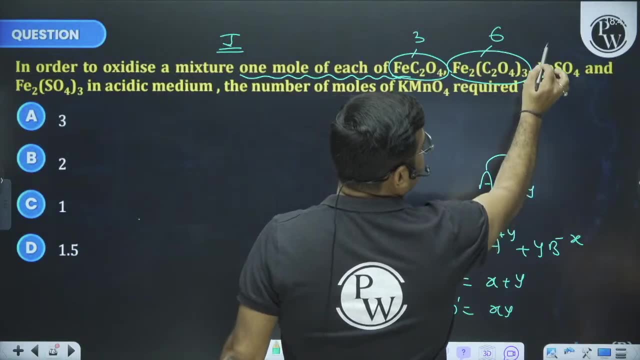 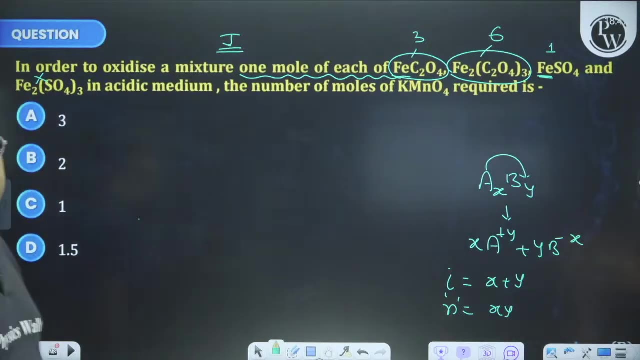 So who will be the only oxidized Oxalate? Oxalate is 3.. Carbon is 6.. In ferrous sulfate, ferrous will be oxidized. N factor is 1.. Next is ferric sulfate. No one is going to be oxidized. 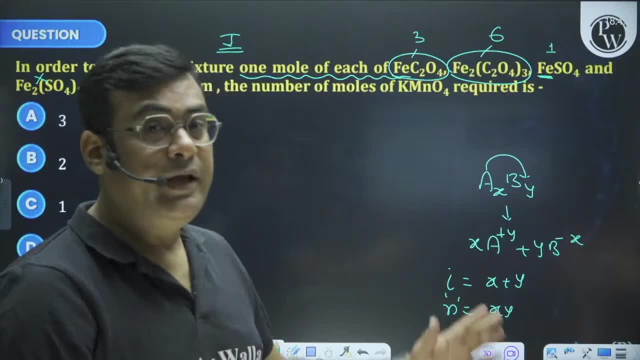 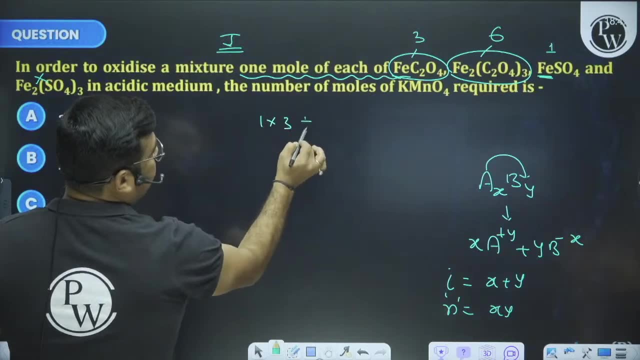 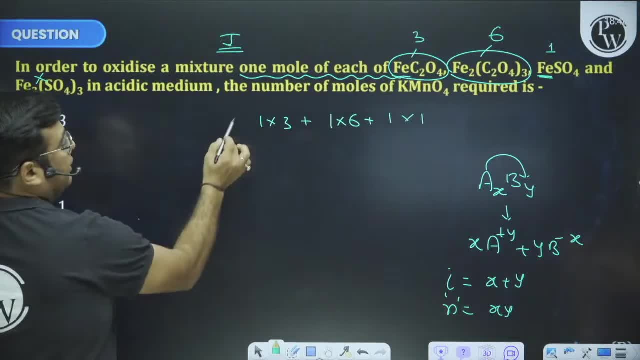 Its 1 mole into N factor is 1.. Equals to: In acidic medium KMnO4, N factor is 5 into its moles A. What a lovely and tough question. So 3 plus 6, 9 plus 1 is 10.. 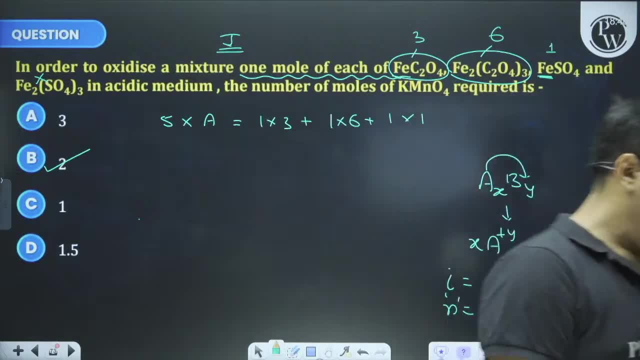 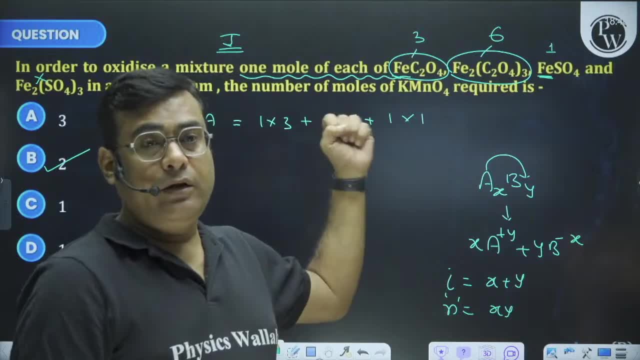 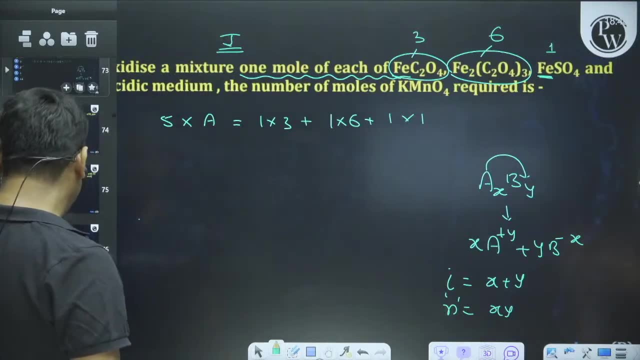 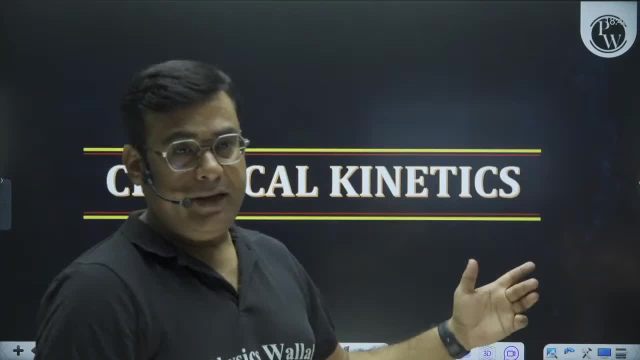 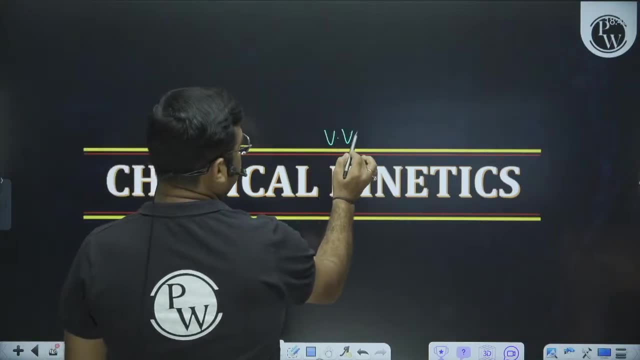 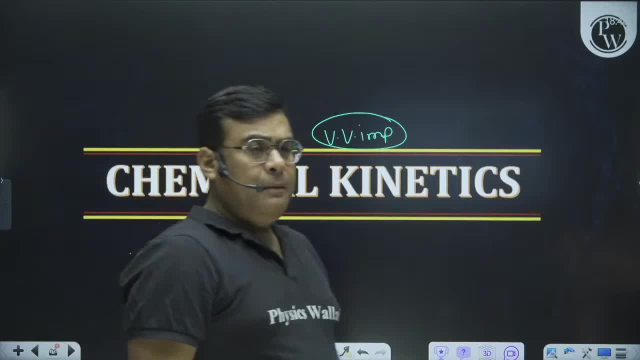 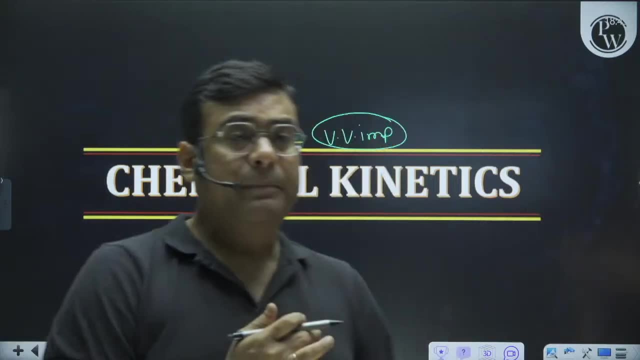 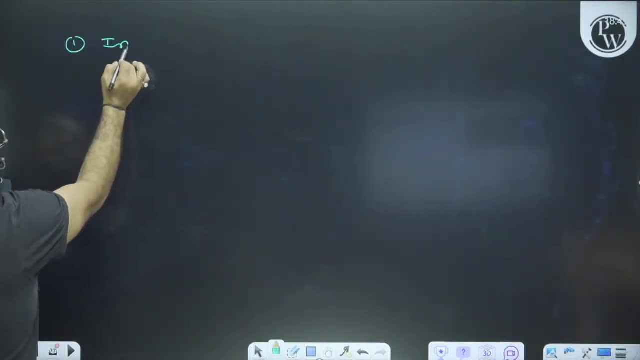 In chemical kinetics. I will give you an initial rate method of 2 minutes. Questions have come in full on this. You have questions on zero order and first order. Apart from that, children, you have questions on the effect of temperature. There are a lot of questions on the effect of temperature and there are also questions on the normal rate of reaction, etc. 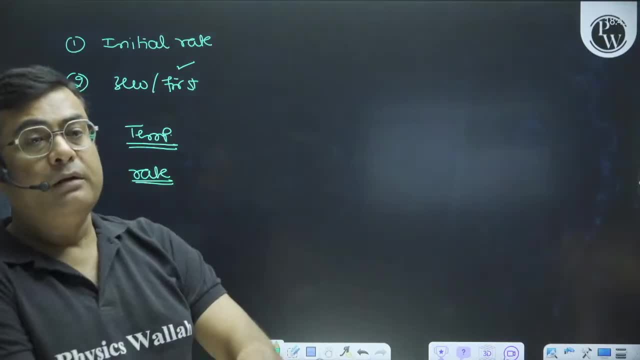 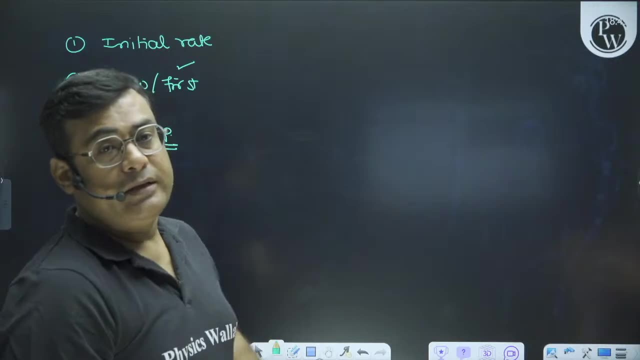 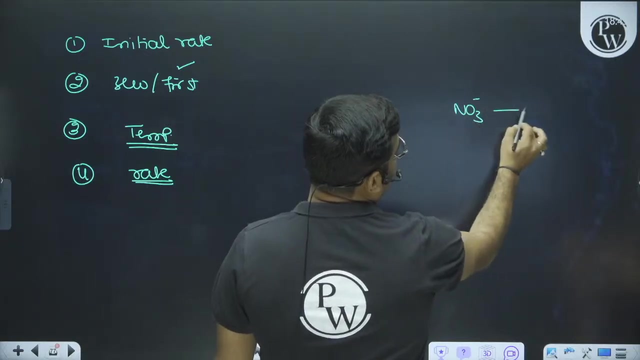 You have a lot of questions on these four things. Then, how to find the n factor. I told you to remember the well-known ones. For the rest, if I am telling you that NO3- is changing to NH3, then it will tell you. 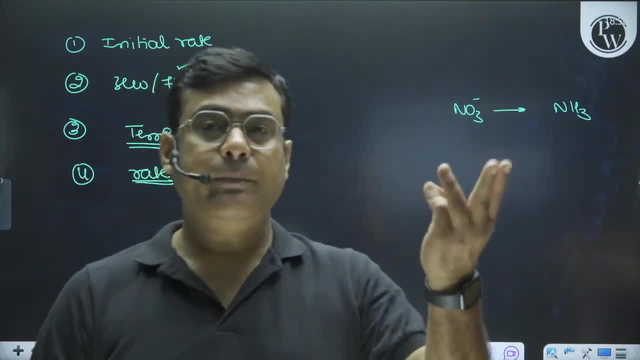 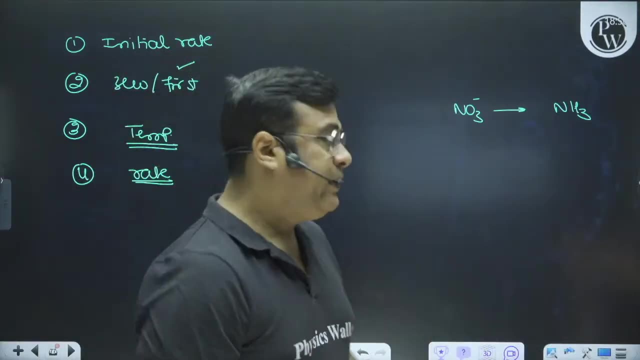 Yes, Which are the well-known ones: K-MnO4, K2Cr2,. I just wrote the list, I can't go back. Sir, how is 5 in the acidic medium? Child A was considered moles and n factor is 5.. 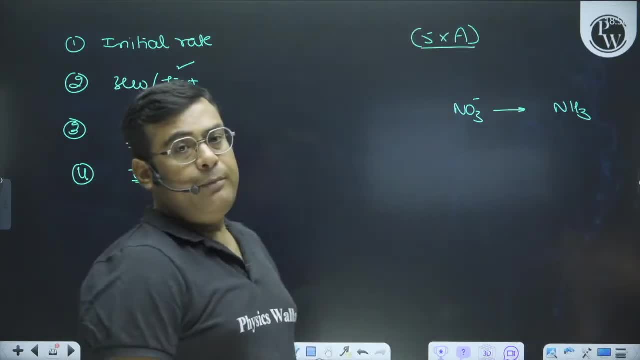 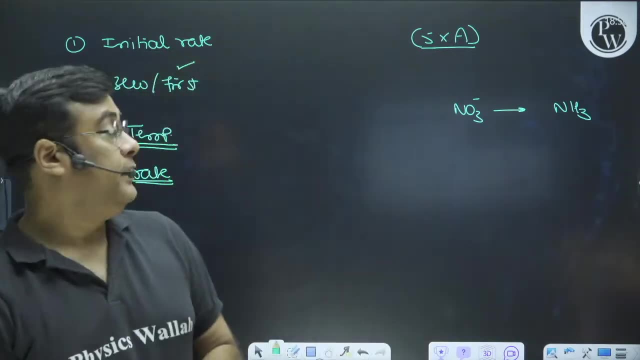 So moles into n factor is equivalent. The n factor of K-MnO4 is 5 in the acidic medium, Right? The n factor of K-MnO4 is 5 in the acidic medium. Okay, So now if the well-known ones. I just wrote it now. 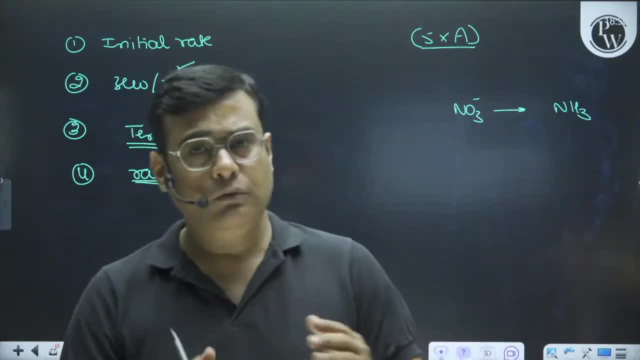 Now, when this video is closed, It will be closed. I am not going back. I am explaining it to you orally, If you had a request. So now you can see: K-MnO4, K2Cr2, ferrous is written. 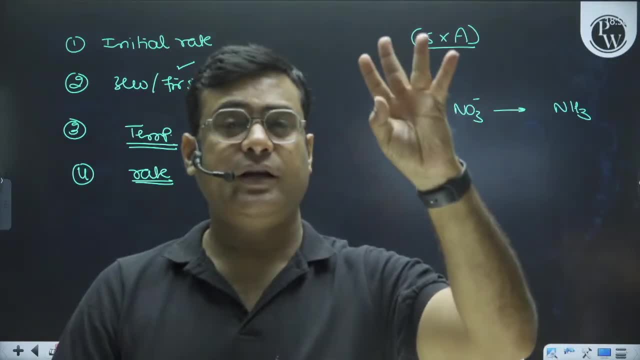 Oxalate is written, KI is written, H2O2 is written. For the rest, child, if there is nothing else, then in the rest. if you are only given change, then in NO3-, in the oxidation number of nitrogen plus 5.. 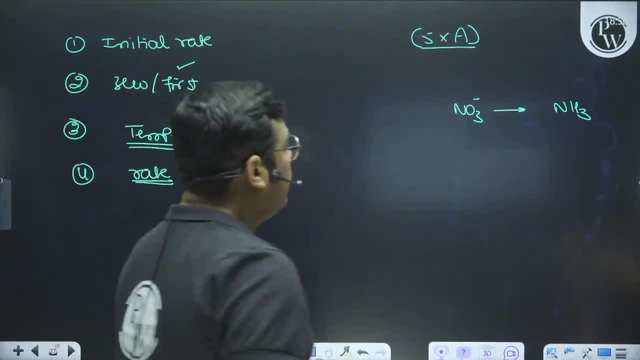 Sir, in ammonia, in the oxidation number of nitrogen minus 3. Right Plus 5 to minus 3.. How much has changed? children 8.. So you will say its n factor is 5. Yes, Yes. 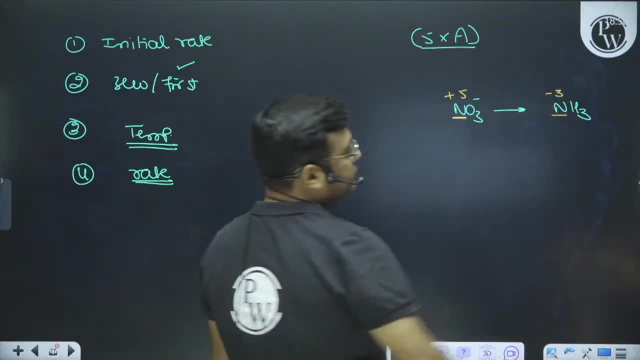 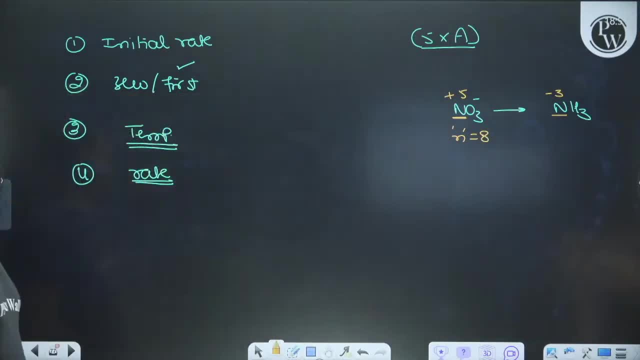 Obviously you have said ferric, Then Fe plus 3 is there. So iron cannot be oxidized. Iron cannot be oxidized. And in sulfate, child, look in sulfate, in sulfur, in which oxidation number Plus 3.. 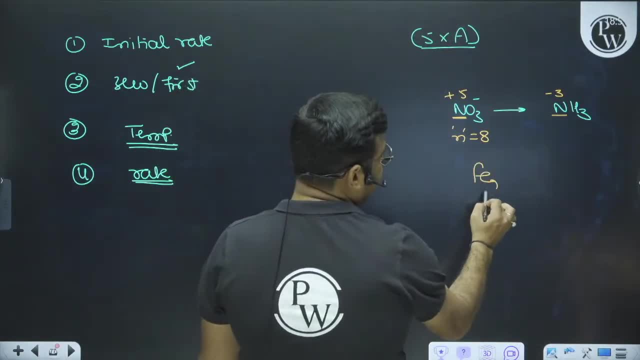 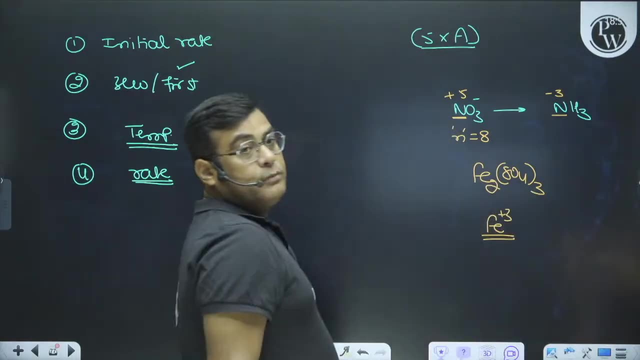 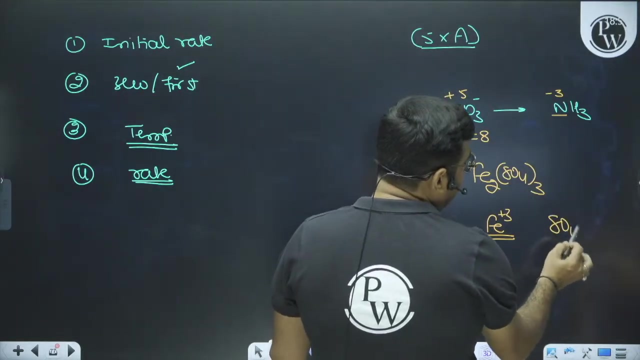 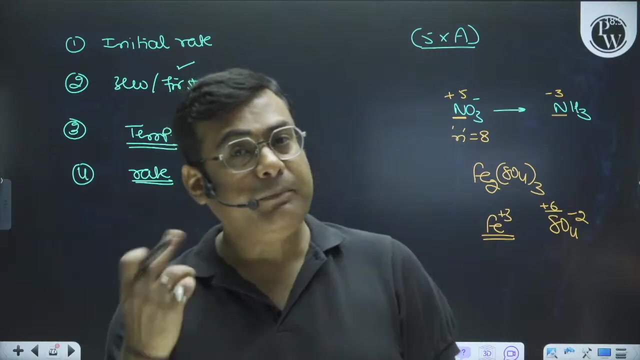 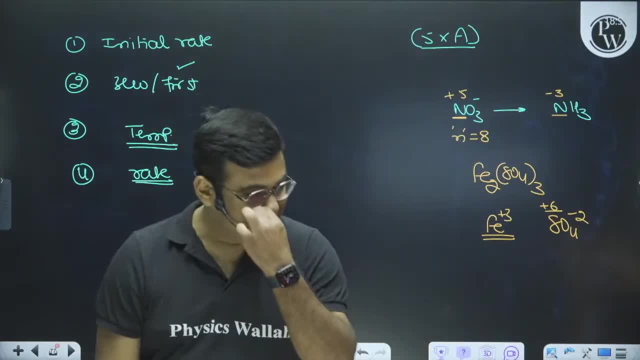 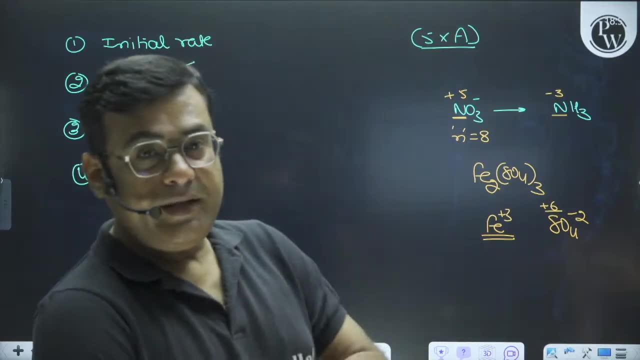 What does oxidizing agent do? The oxidizing agent functions to oxidize the opponent, But the oxidation will be done by him who is in the lower oxidation number. Okay, it's fine. So this is the kid. Now, 0 order. Ki is nothing but. 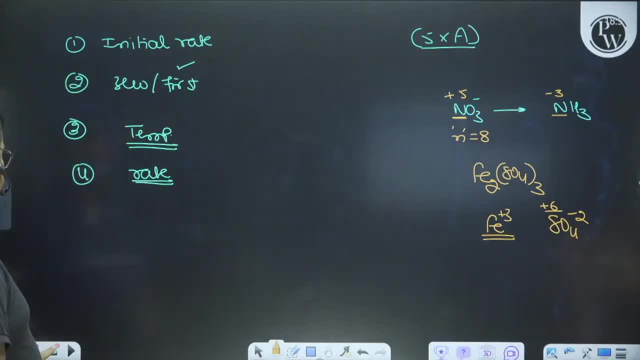 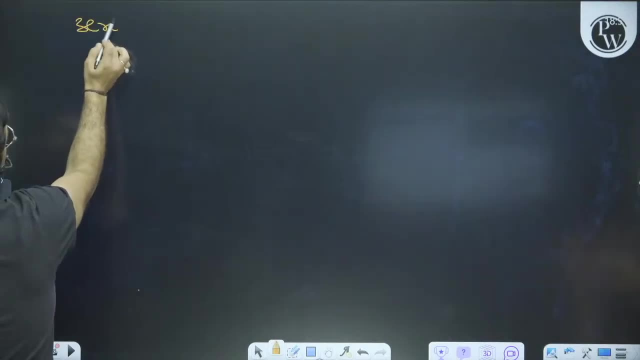 And if you add further, then 0 order Ki is nothing but wspól compte. 3 formulae: direct noses. okay, Is it such that it doesn't appear? First is that it manages the win part of squad 2.. Yes, agree. 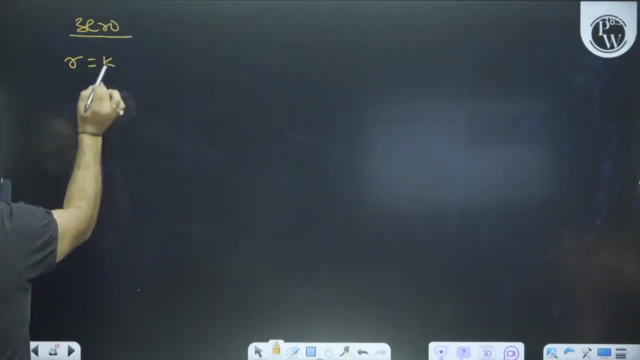 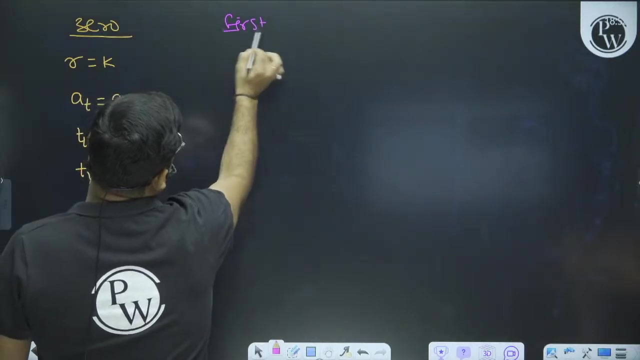 First rate is equal to K. if rate is asked, then second, 80 equal to A0 minus KT, or their lifetime will ask children, then A0 by K, and if their half-life time will ask, then A0 by 2K. If I talk about first order, first order kinetics, because almost the most questions come on first. 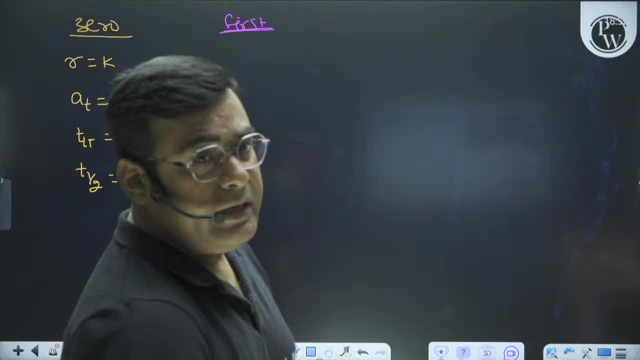 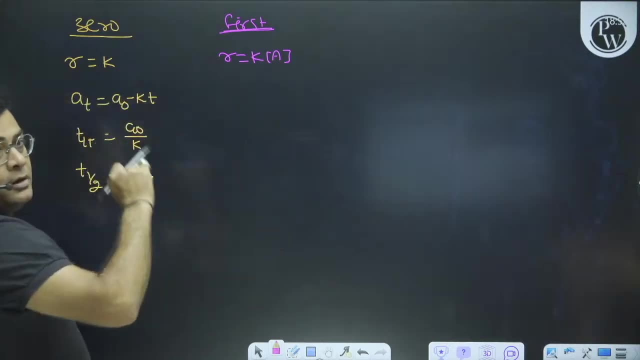 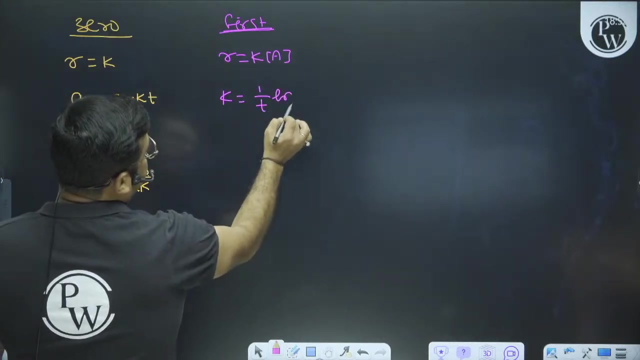 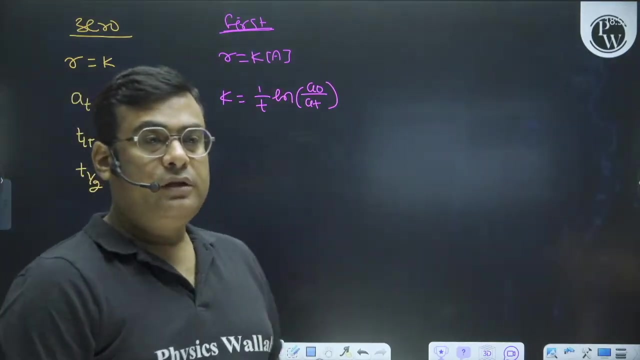 order kinetics. If I talk about first order kinetics, then its first formula is of rate. So R is equal to K into A. The formula of taking out K is 1 by TLN of A0 by 80, and if you write it in log, then 2.303. 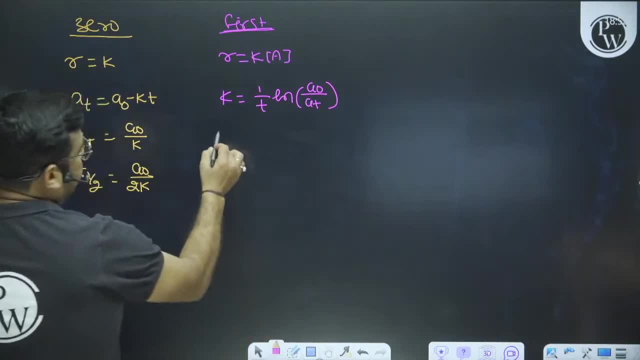 by TLN of A0 by 80. Its formula of T- half, T half- is equal to 1 by TLN of A0 by 80. Then the formula of taking out T is 1 by TLN of A0 by 80.. 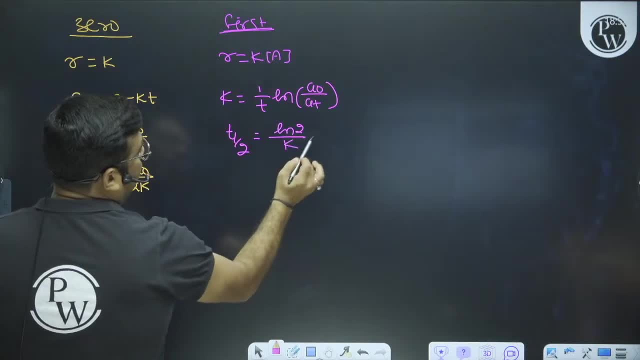 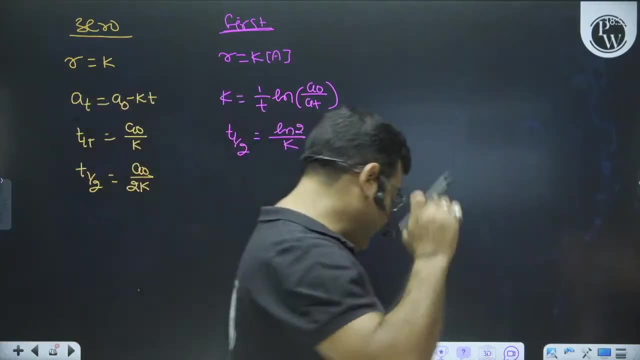 Then the formula of taking out T is 1 by TLN of A0 by 80.. And then the formula of taking out T is 1 by TLN of A0 by 80.. If this equation is written, then this third formula is Ln. 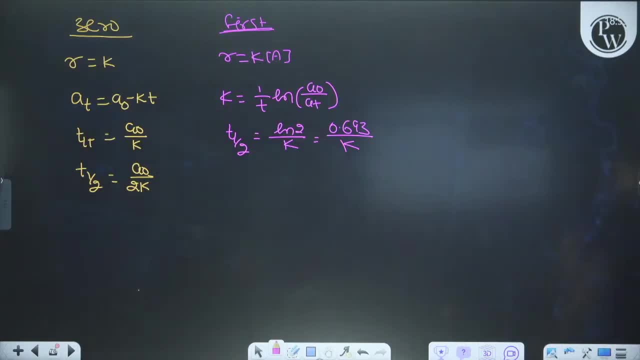 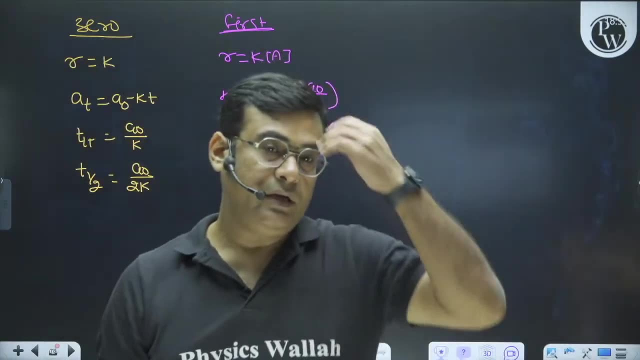 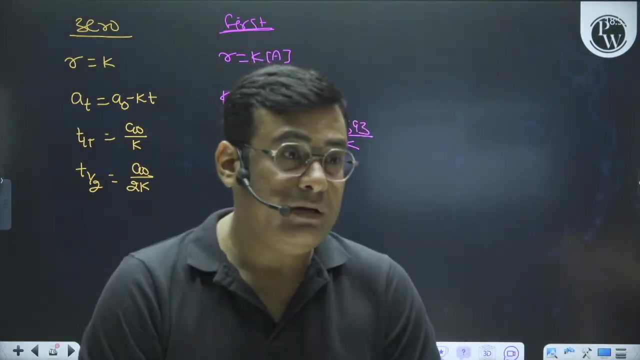 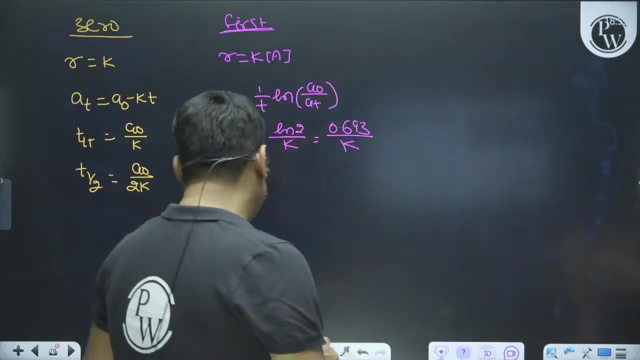 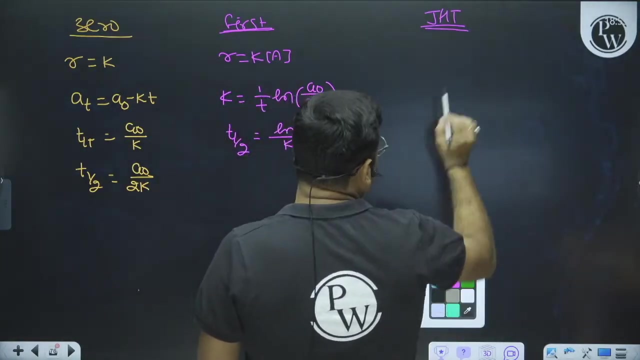 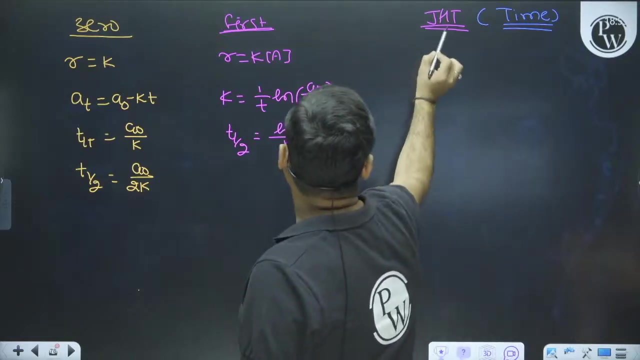 Then you will get Ln. Third formula is Ln In 2.102 equation. it is Federation of month. Why? Now? I am going to tell you some JHT. now, what is this? and this is some very, very important time, children, JHT means a little odd time. it is valid only for first order, this time. 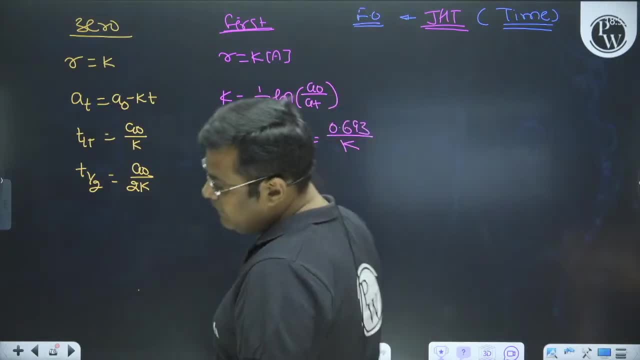 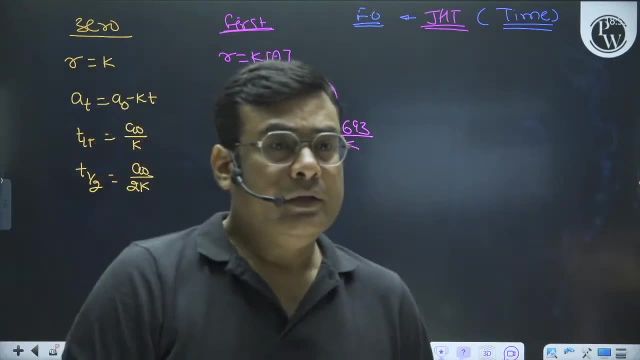 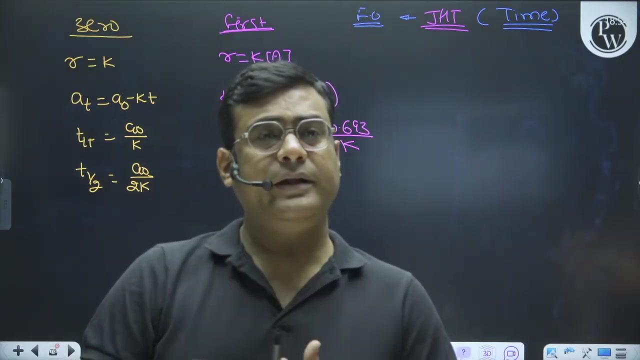 is valid for first order. now. this is the time, children, which is the first time I have read. last time JEE meant T90%, 10 by 3, T half was written, 400 was typed in the answer. NT gave 390 as the answer you are saying absolutely right. I am telling you the reason. 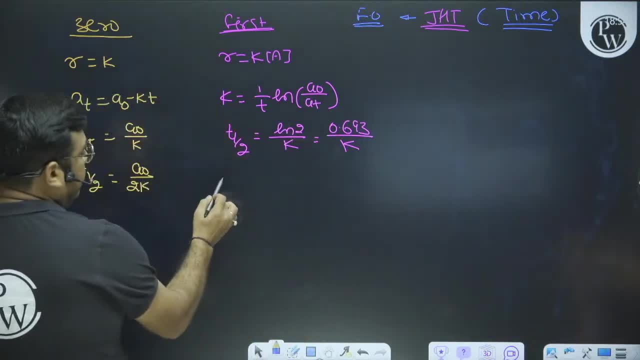 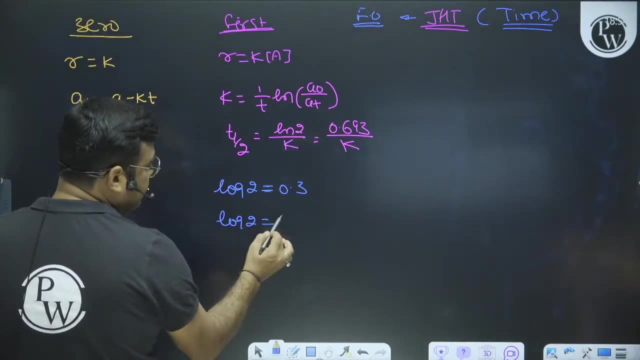 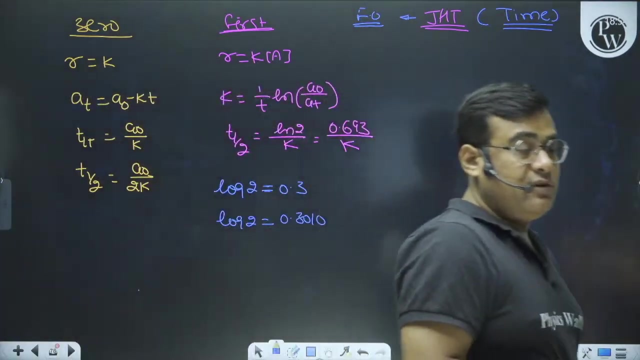 for that? the reason is that we are going to write this time, in that we are going to write the exact value of 0.3, whereas the exact value of log2 is 0.3010,. now this question which you said, son. maybe some child had put this message on WhatsApp from me, right I? 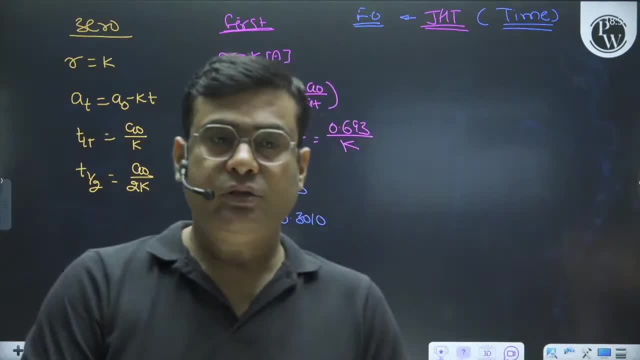 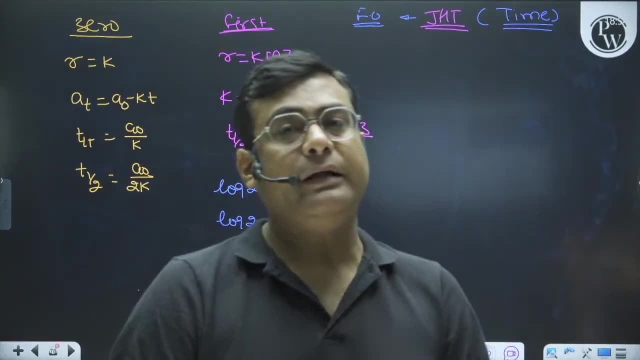 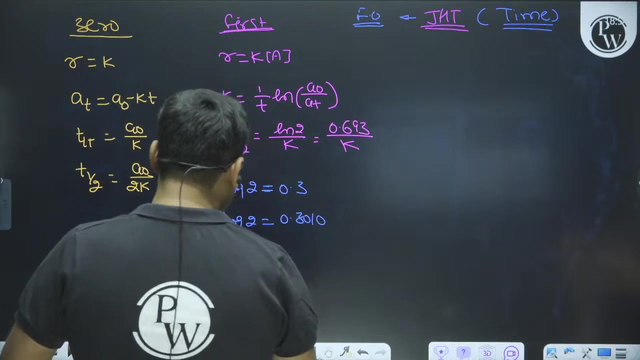 had also answered him right. I had also given some answer to him. that, brother, this JEE has written in that question: son, you have RTA right to information at. you have to fight this thing immediately there, because I have also seen that question. from now on, 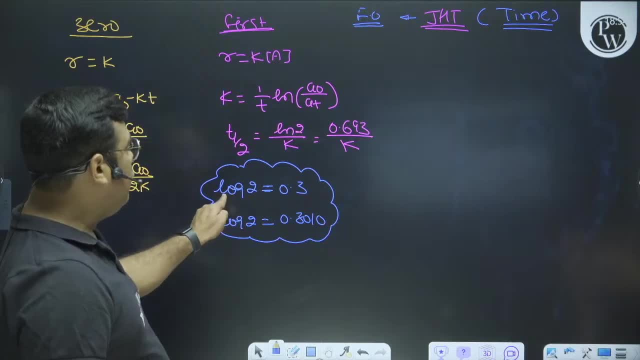 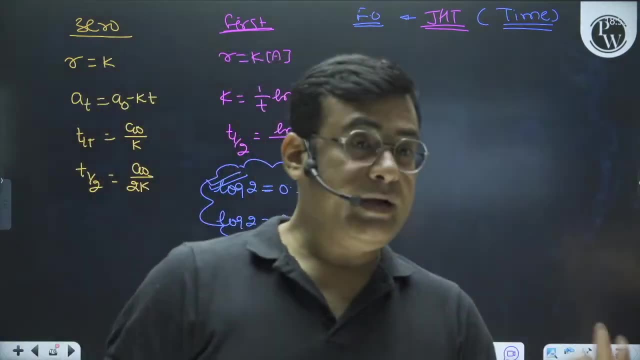 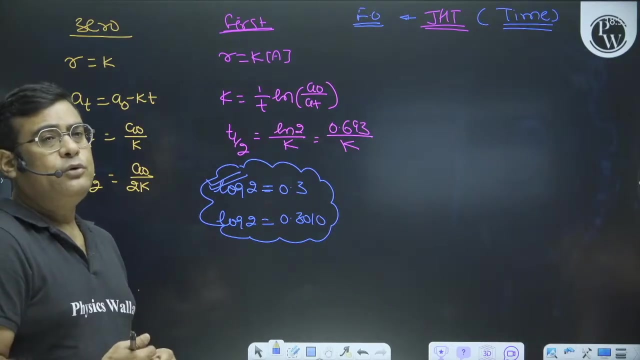 I am telling everyone again that the time I am writing, son, I have written the time as 0.3 in that log2, right, I have written as 0.3, the mistake you have made is because 10 by 3 into 10, by 3, into some 120, right then, your 120 by 3, 40 into 10, 400, you have. typed the answer, whereas that JEE has written the answer as 0.3 into 10 by 3,. right then, you have written the answer as 0.3 into 10 by 3, right then, you have written the answer. 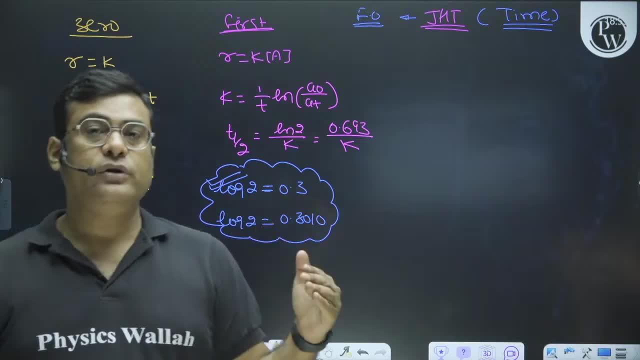 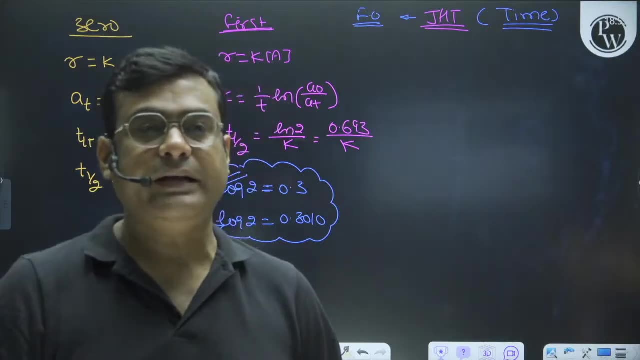 as 0.3 into 10 by 3 in this. only at that time I have thrown it as 0.3 inside. you have written it K Here. the answer is correct. this JEE então memorable to you. I said this answer then. 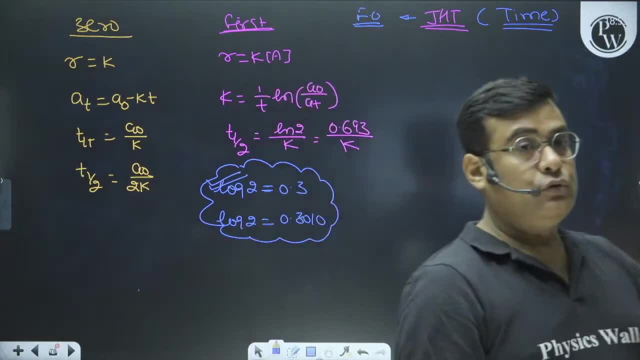 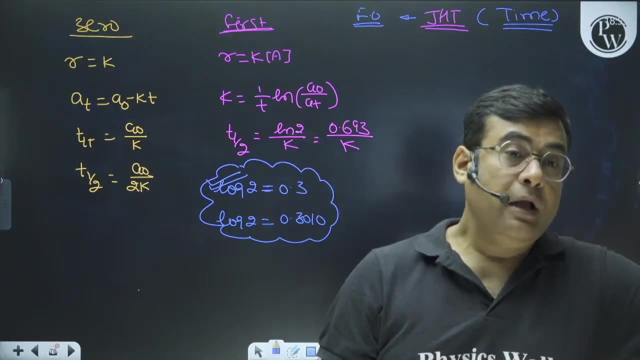 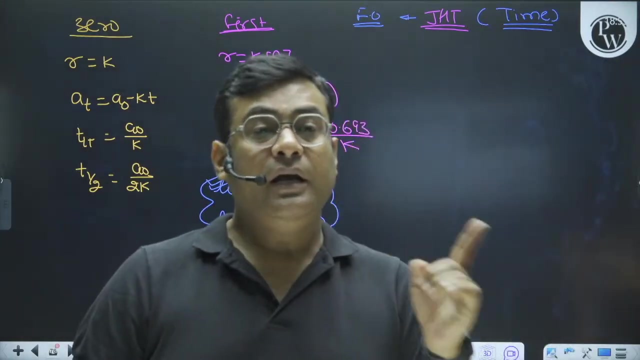 in return. please write Now every Jew combination into second part. that is Sh可能. how do I run through it that? I have seen the very second part of this question. he has told me, with respect, that We have not given the value of log2 as 0.3 nor as 0.3010, so it is his mistake, this mistake. 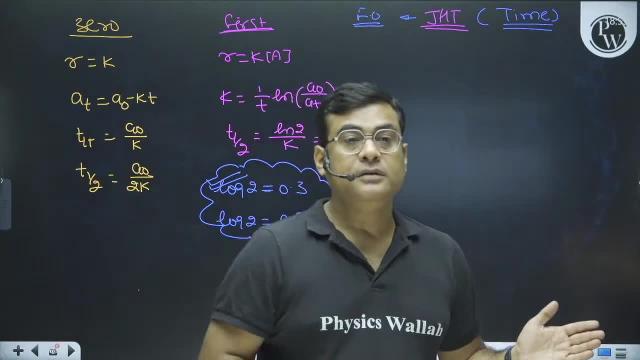 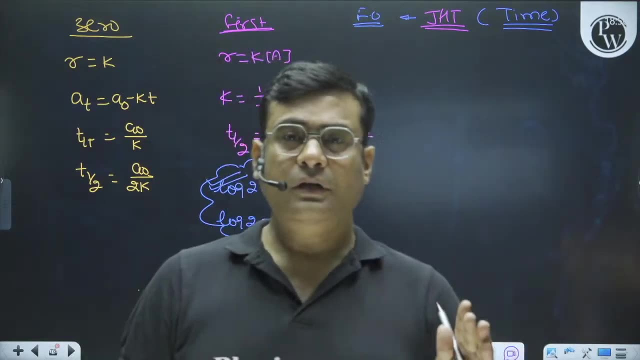 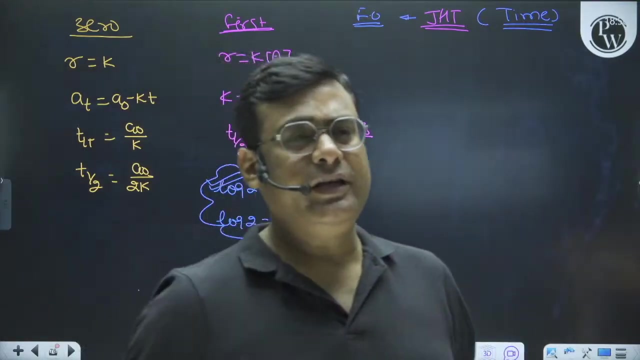 will be considered as his mistake, not ours. we will not give the break now. I will give the break around 8 o'clock. I have also brought a paratha for myself. I will eat it in that break. then we will pull it. now. read for 3 hours continuously, complete 4 chapters. 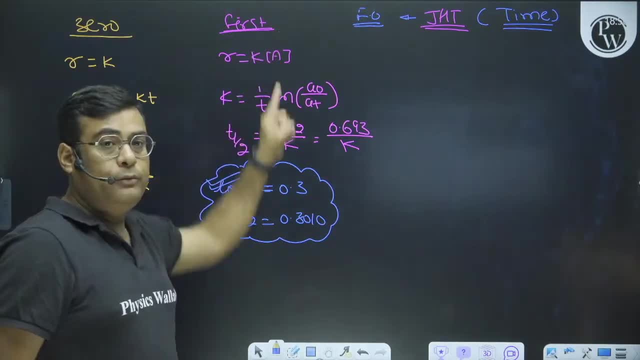 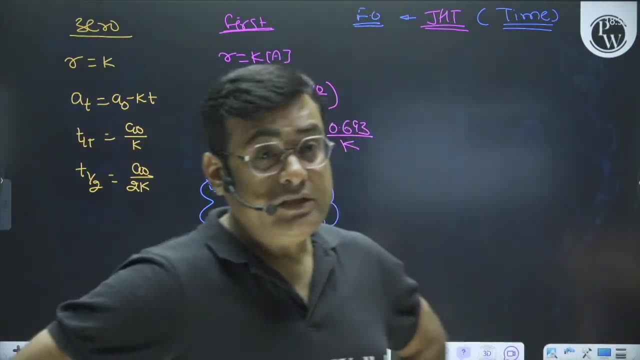 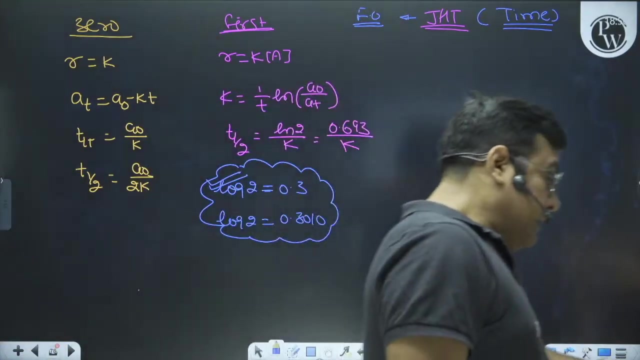 so please tell me this thing from now on, son: for these times I have considered log2 as 0.3,. actually, log2 is your 0.3010, so that's why, please, please, please, Rohan Singh, take my name too, son. I will take everyone's name, son, because here I have come to take. 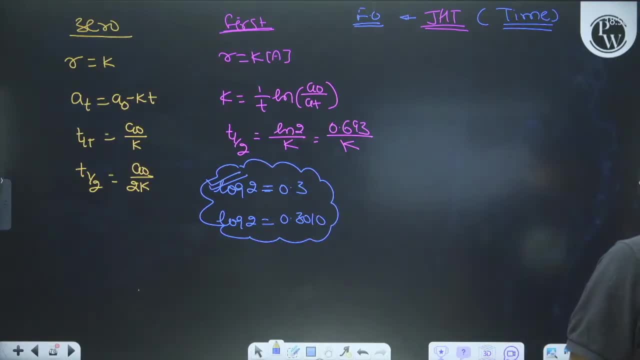 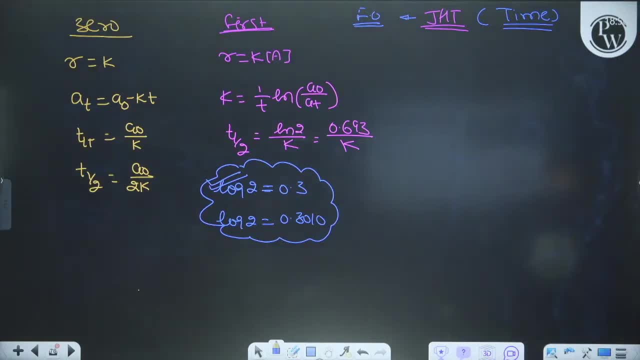 Brother, the likes should be 10k by the time the session is over. come on then. leave it now. what am I saying, son? even then, I have been studying for so many years and I will always keep studying. considering log2 as 0.3,. I have written the time. t will ask the time. 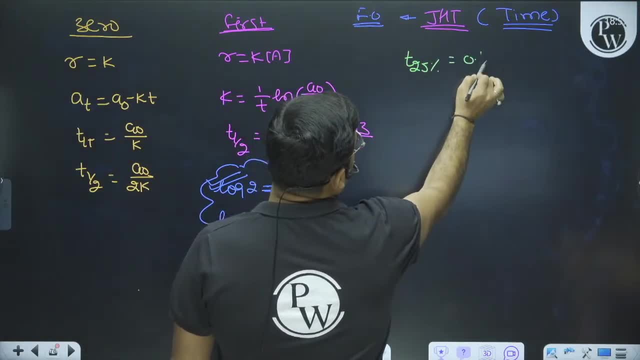 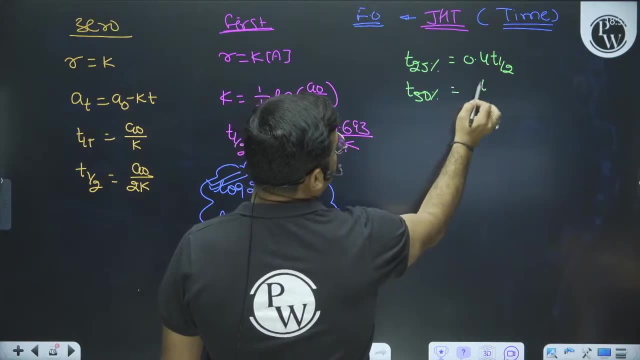 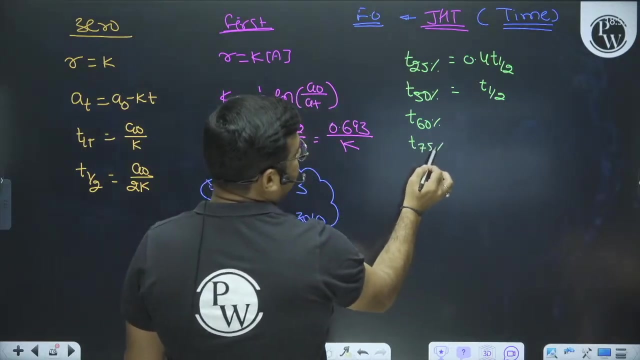 of 25%. it is 0.4 times of t half, isn't it? t is 50% of you. it is 0.4 times of t half, isn't it? t will ask you 60%. after 60, you will ask 75%, you will ask 80%, you will ask. 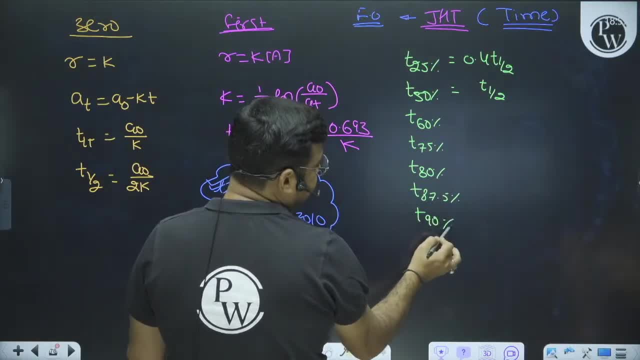 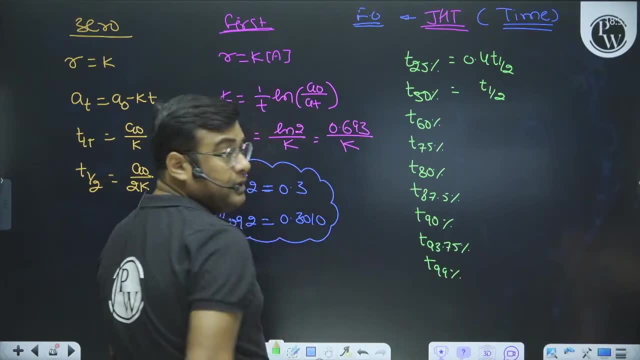 87.5%, you will ask 90%, you will ask 93.75%, you will ask 99, and I am going to show you a lot of questions, children, you can ask 99%, you can ask 99.5%, you can ask 99.5%, you can. 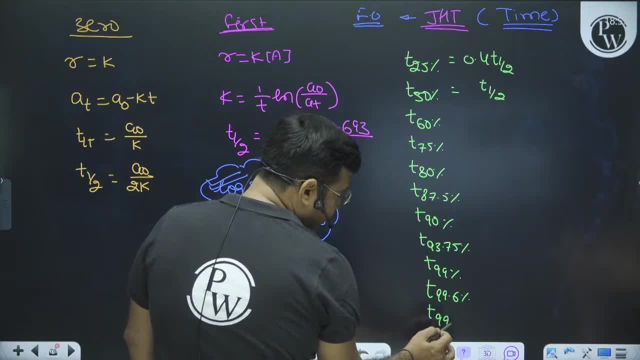 ask 99.6%, you can ask 99.9%, you can ask 99.99% and I have come. son, this has come in 2024, the question we were talking about now. if you remember them in terms of t half then 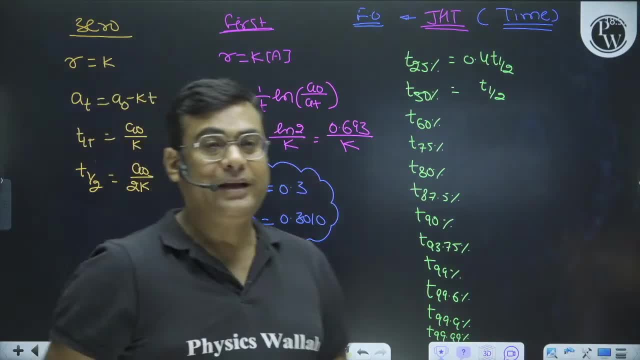 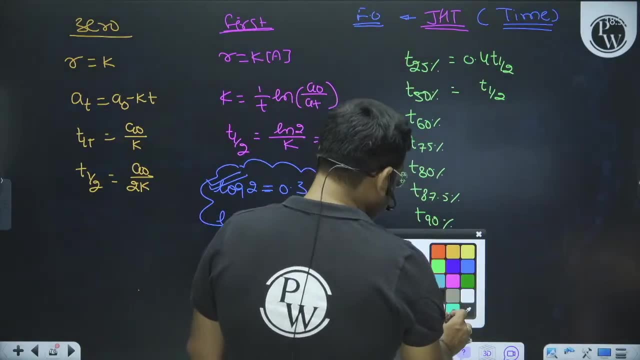 these are the times, children, which will change your time in the exam, because after this, you will have to take the question like this, isn't it? you will have to take it. then t 60% will be the time, then t 50% will be the time, then t 50% will be the time, then t. 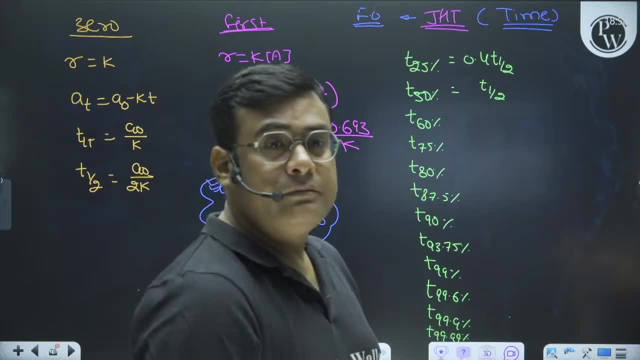 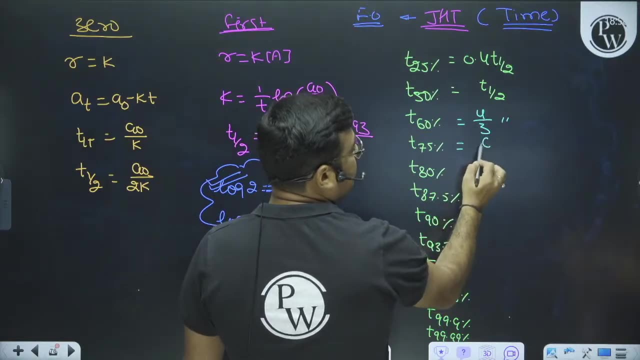 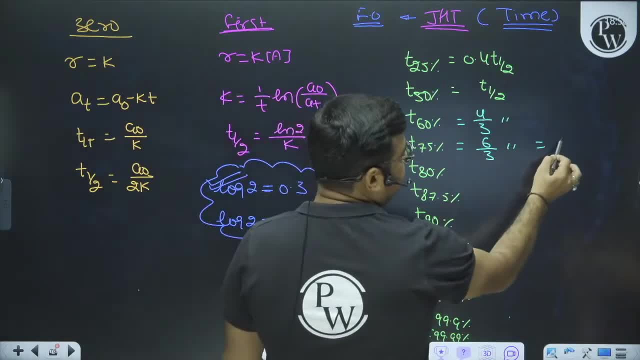 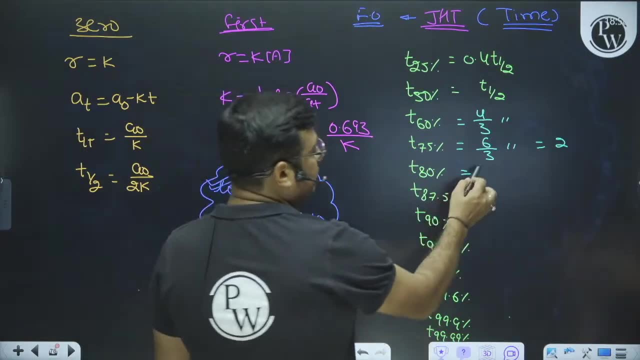 of by 3, actually this is 2t half, 6 by 3. this time right, I had written 2t half, I wrote 6 by 3, then 80% is why I am writing in the terms of 3, because in the increasing order. 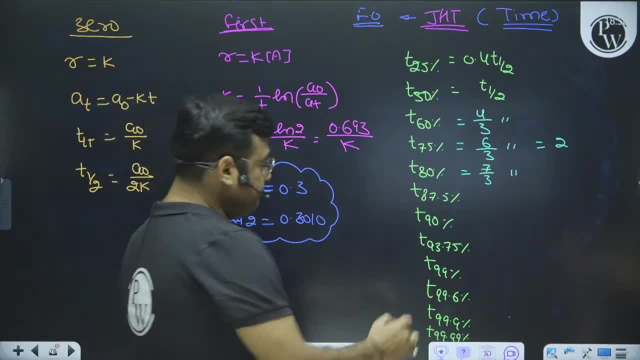 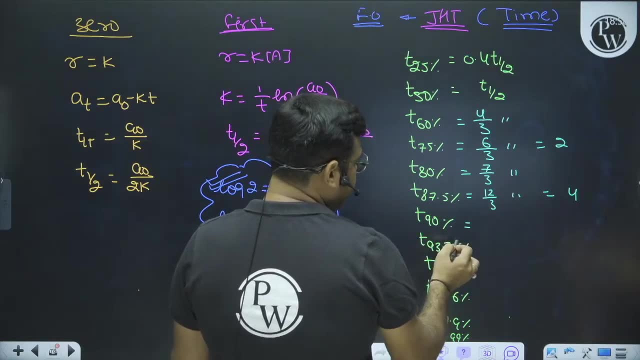 you will remember, 7 by 3 t half, 87.5% is 12 by 3 t half, which you call basically 4, 90%. no 12 by 3. why 9 by 3 t half? because it is 3 t half. 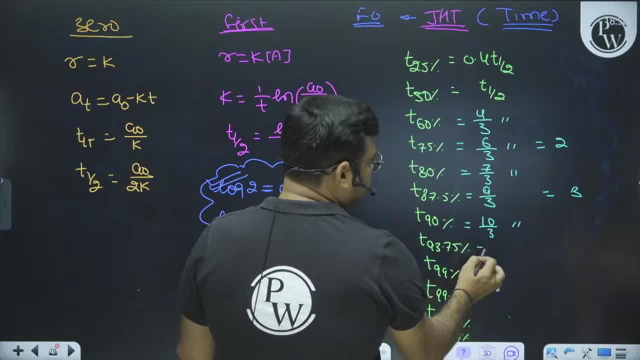 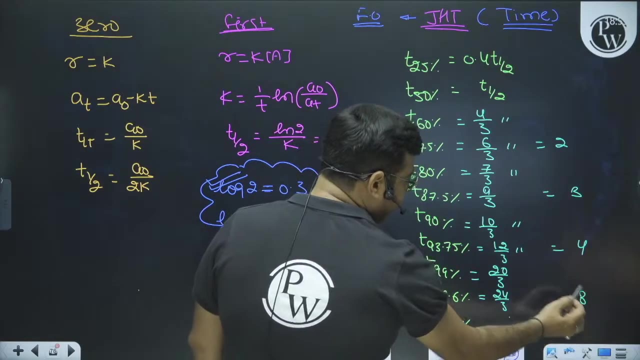 right by this: you 10 by 3 t half 93.75%, you 12 by 3 t half, which basically you say 4 99%, 20 by 3 t half. 99.6% is 24 by 3, means basically 8 t half. 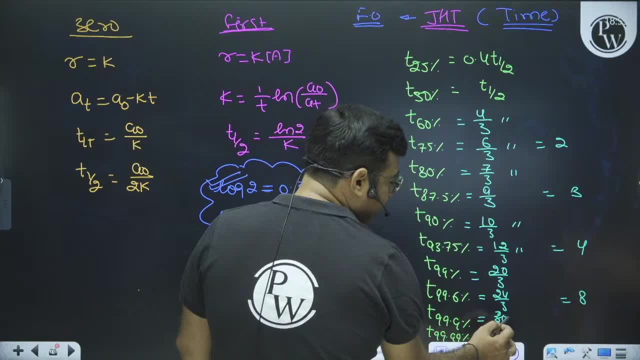 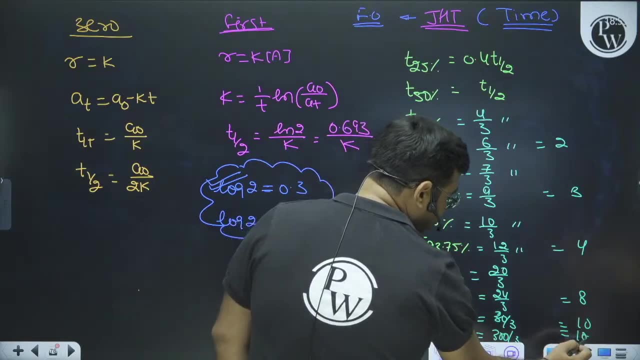 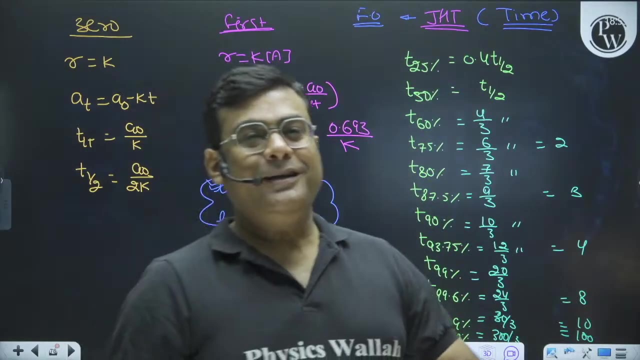 99.9% exchange rate is 30 by 3, that is 10 t half, and 99.99% is 3 by 3, that is hundred. you slowly do this, my dear, and do tell tricks for cheating, for exam. Cheating tricks I can tell for when you reach in IIT. 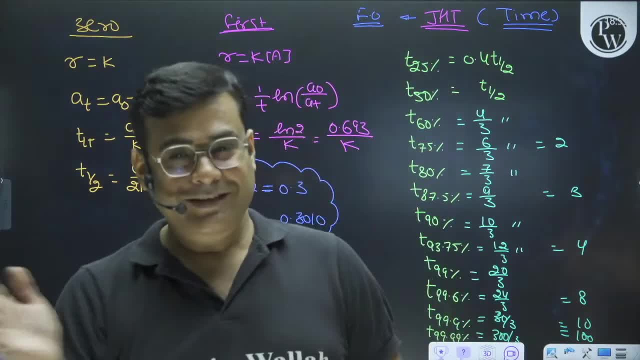 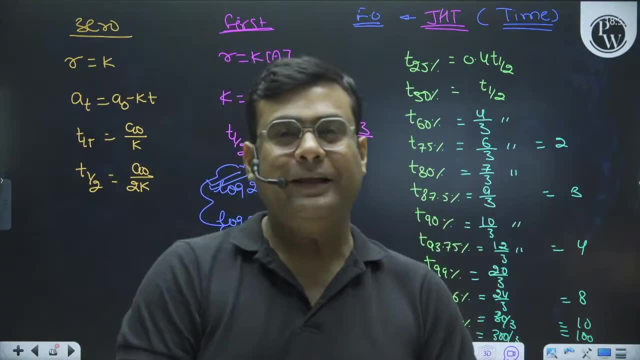 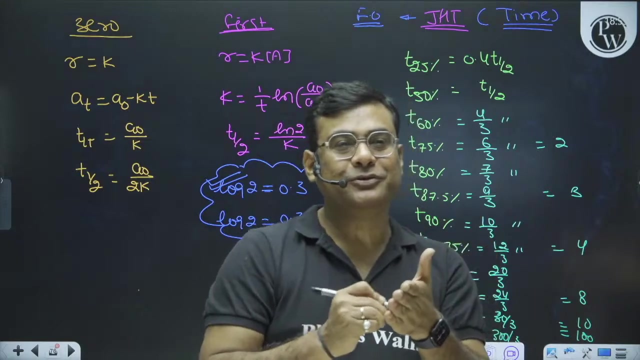 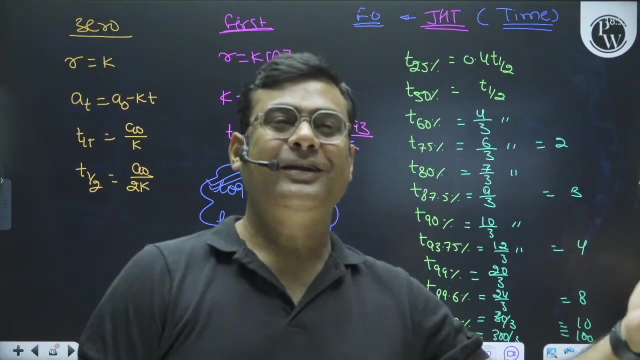 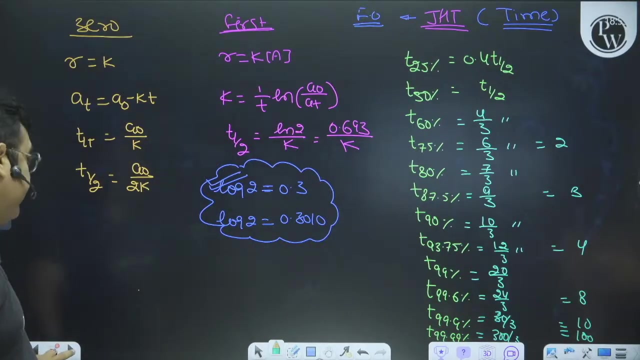 Because I used to do sometimes In IIT. there is not chance for this. there is any idea about this and I am going to show you the question on these times. remember this. apart from this, I think we have already discussed the effect of temperature in two formulas. let me tell you that is. 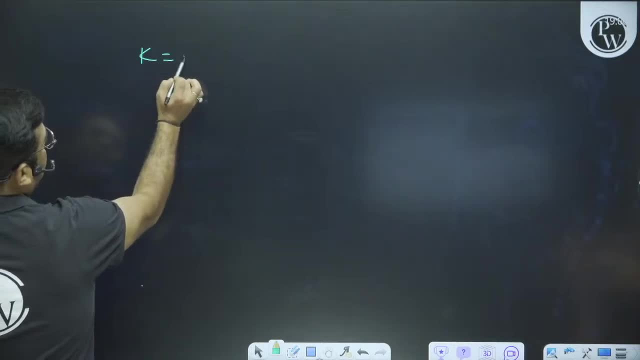 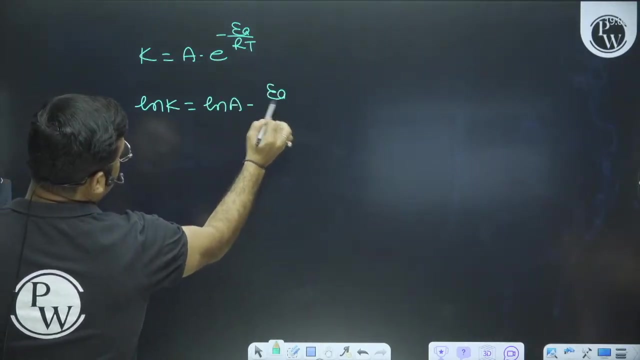 also very, very much important. in effect of temperature, you get K equal to Ae power minus of Ea by RT. in this equation you get a lot of questions apart from this. if you change this to ln, then ln K equals to ln A minus of Ea by RT. that is also a very good equation. 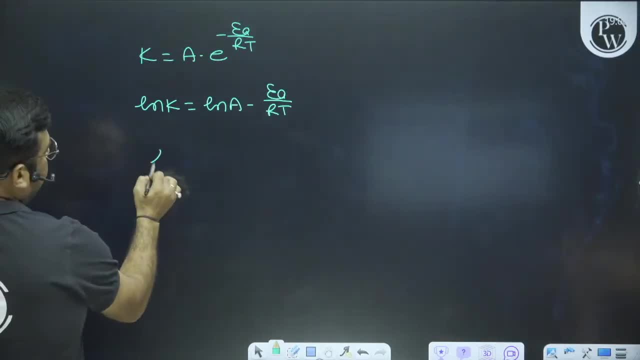 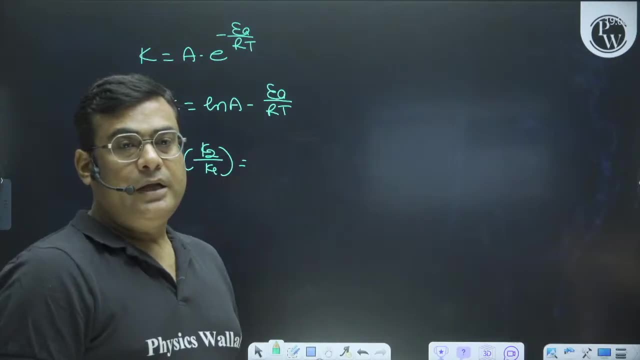 you get a lot of questions on this too. apart from this, if you change this to ln A, then if you take this in the form of two locks, As soon as two temperatures come in physical chemistry, you will get the comma for ln. 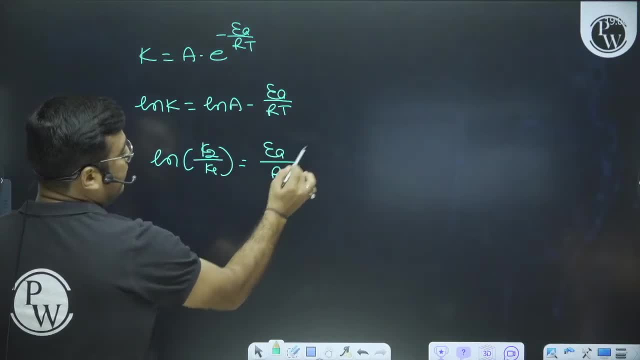 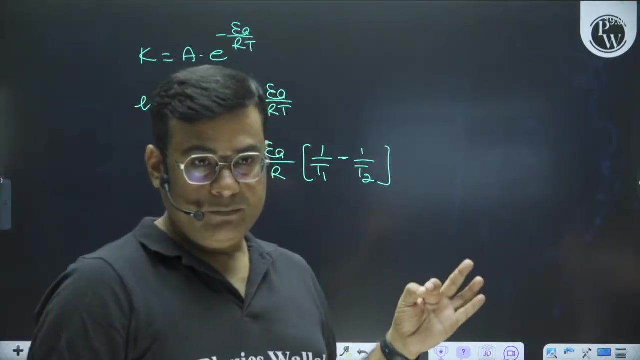 K2 by K1, ln K2 by K1 is Ea by RT1 by T1 minus 1 by T2, if you lock it in this, then here too 2.303 will come, and here too your 2.303 will come. so if the temperature goes, 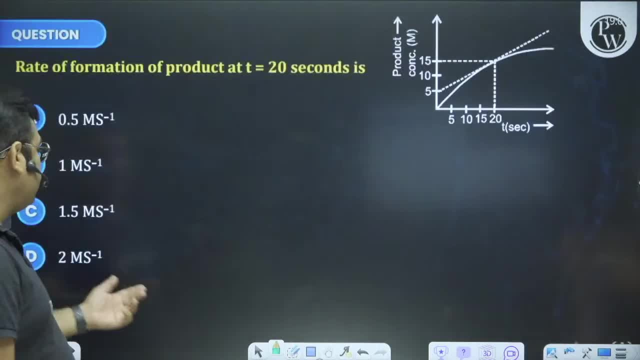 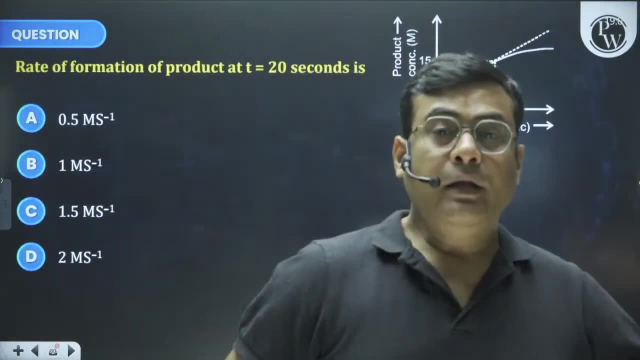 to 3, then it is known: Yes, Yes, Yes, Yes, Yes, Yes. Remember the formula of the temperature. now I will show you some questions. rate of formation of product at t is equal to 20 seconds. rate of formation at t is equal to 20, so the graph. 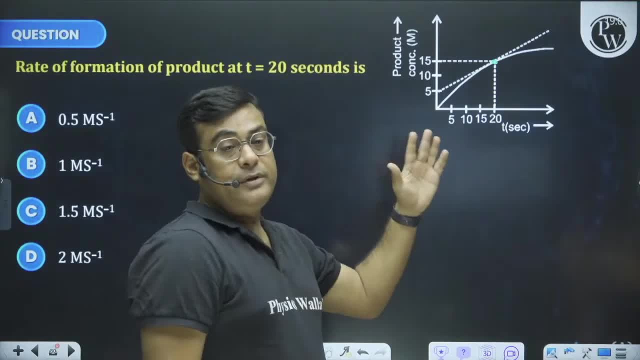 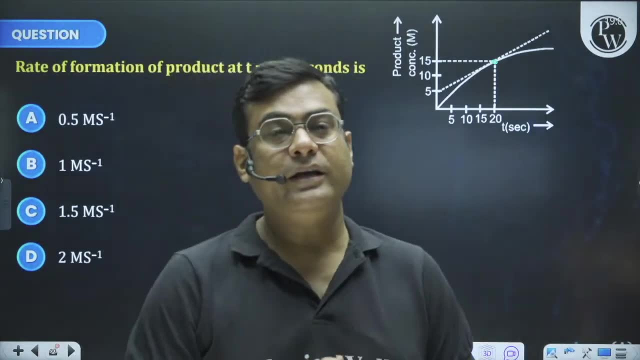 will be given to you. you should know that the graph will always be given in the question, because if the graph is not given, then some line will bend a little, some line will move up and down a little. this can cause a mistake, so now you just have to find the slope then. 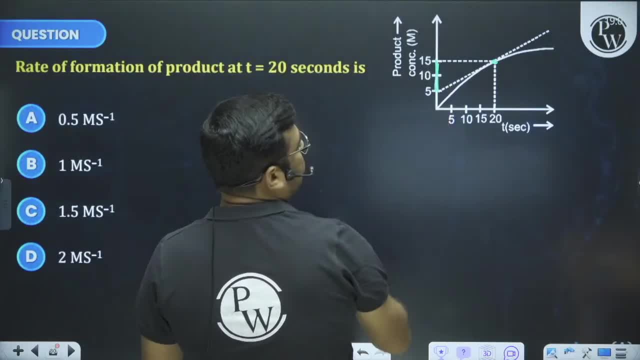 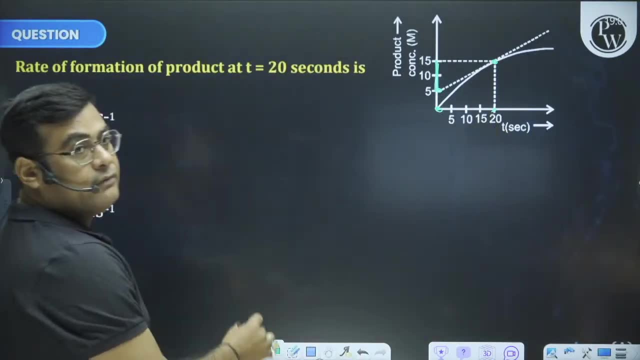 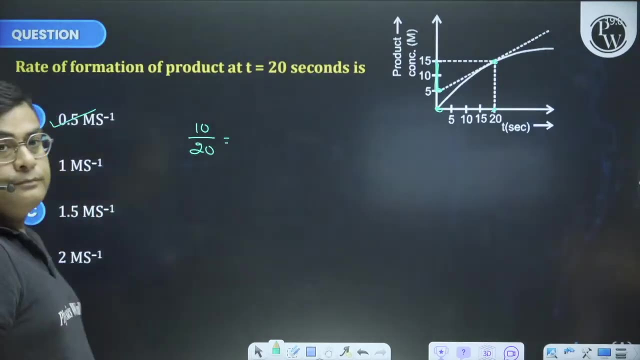 how do you find the slope? the intercept of y axis is 15 minus 5 is 10, x axis intercept of 5 is 0, value of 15 is 20, so only and only 10 by 20 means 1 by 2, that is 0.5, kinetics. 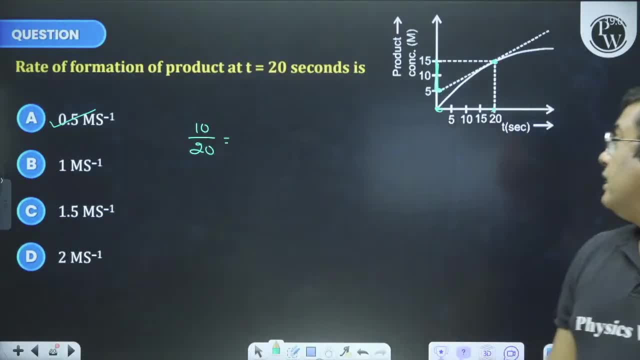 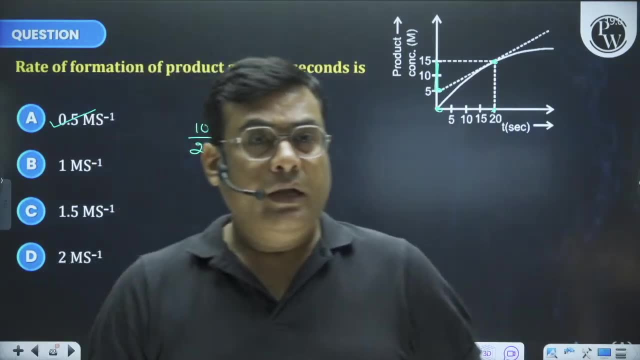 is also a little scary. kids understand this weird chapter, but it is not like that. it is a very, very easy topic, isn't it? What is there in the physical? The calculation is wrong. do it properly. do it properly. we are also trying, you also? 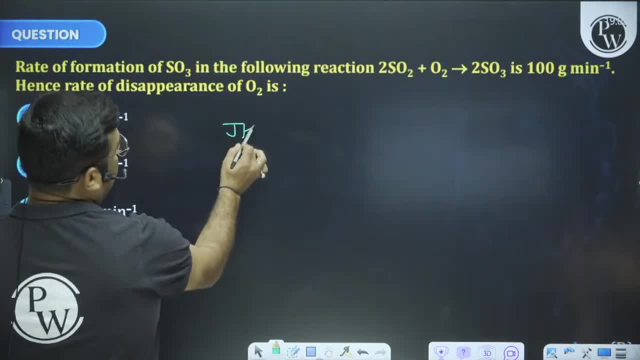 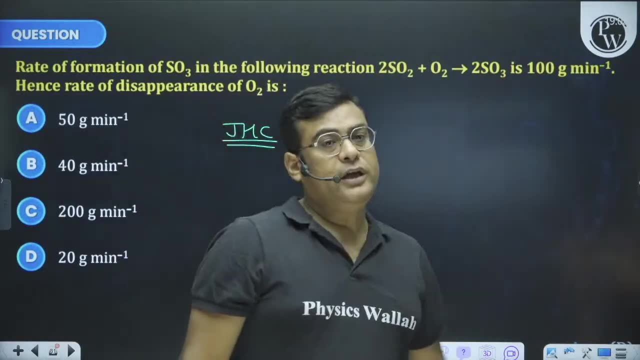 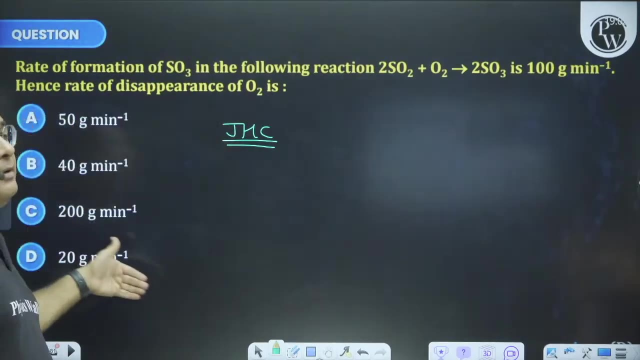 do it now. take another JSC in this too in JEE many times children. the rate of formation of SO3 in the following reaction to SO2 plus O2 gives to SO3 is how much 100 grams per minute. so rate of disappearance of O2 in grams per minute. pay attention. 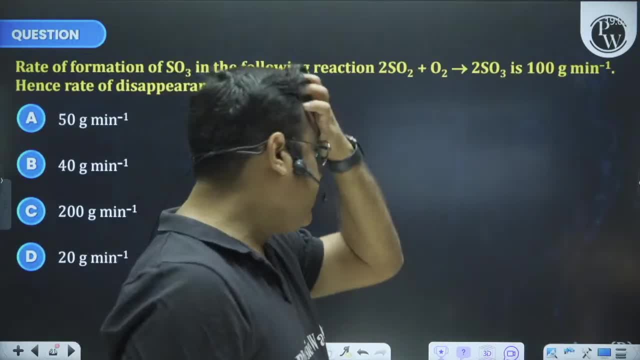 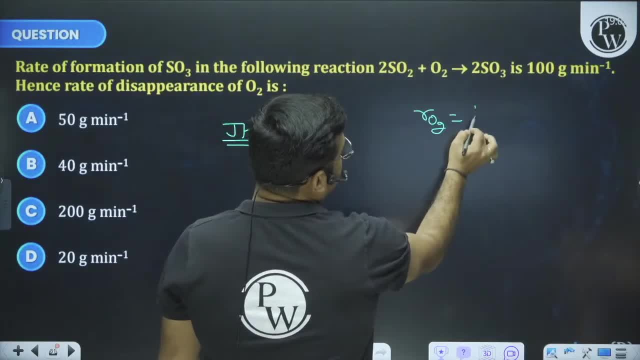 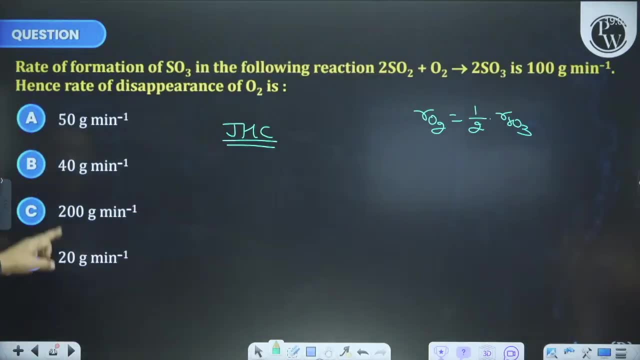 one who writes 1 by 2 should be given and written as 1 by 2, and the rate of depression of SO 3 should be equal to 1 by 2 of rate of SO3,. you know that he has given 100 of SO3,. 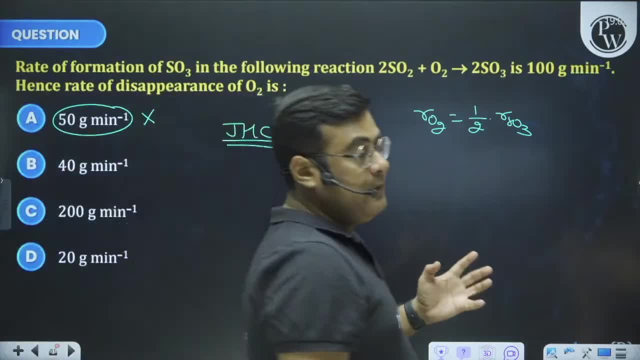 divide 100 by half, 50 have already been given and the tick gets wrong and it is called JEE son. he knows, see, many of you are giving option A to your child. he knows that this is nothing after telling this thing to the child so many times, and he also warns that. 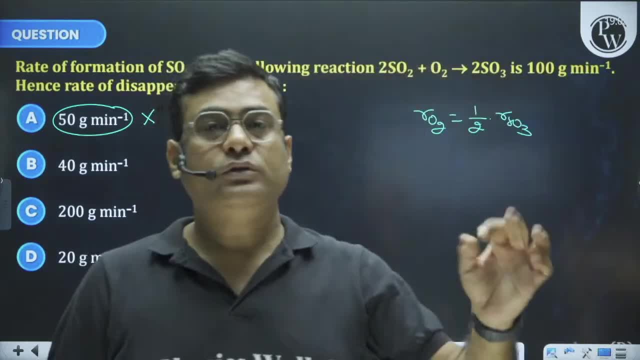 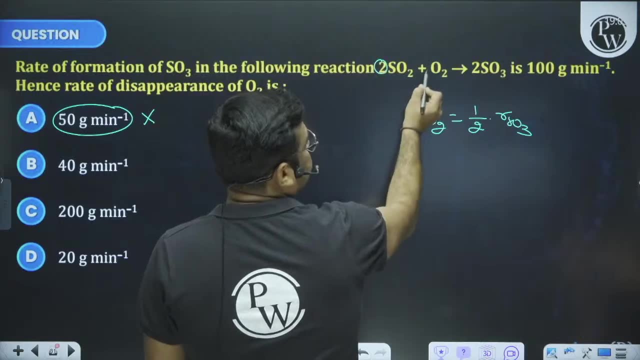 if you don't listen, then whoever teaches you this method, they will not help you. and and he makes it wrong. Now, what is the mistake in this? I had just told you that this is 2, there is nothing written in front of it. it is 1.. 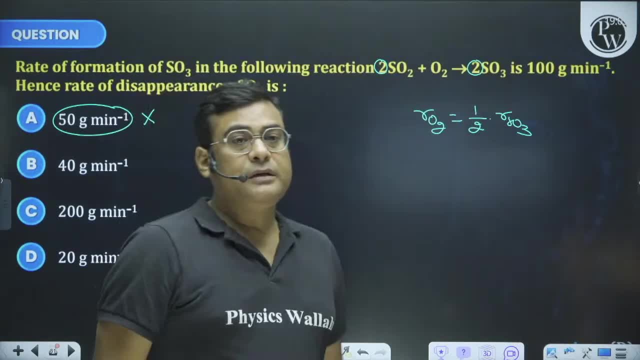 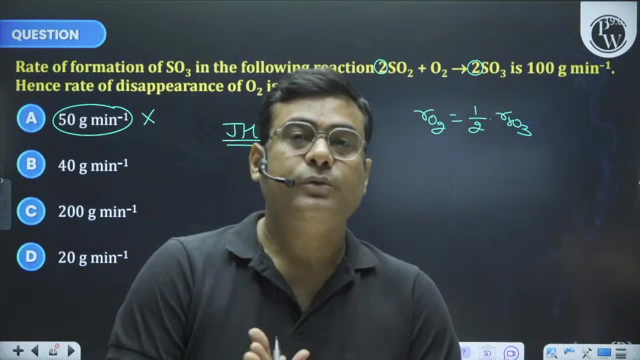 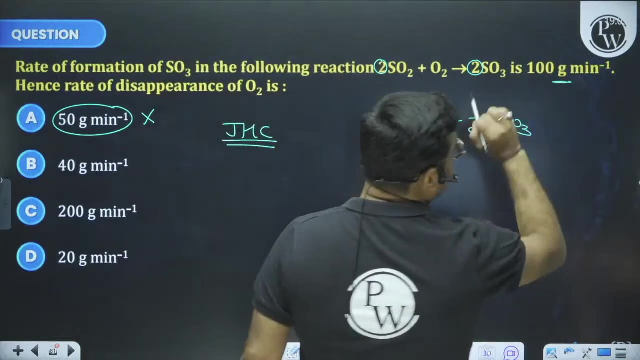 There is 2 written in front of it. All of these are statuometric coefficients, And the statuometric coefficients are in the terms of moles. The statuometric coefficients are in the terms of moles. Here the unit given to you is given in the term of mass. 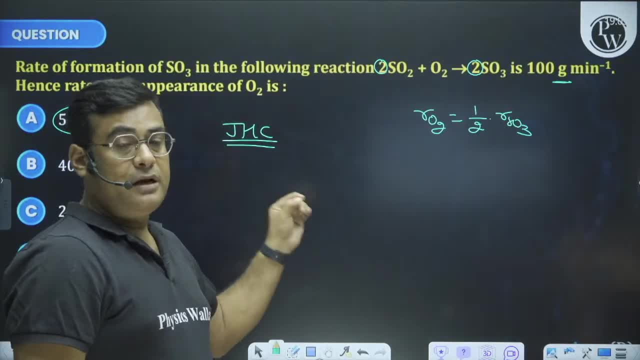 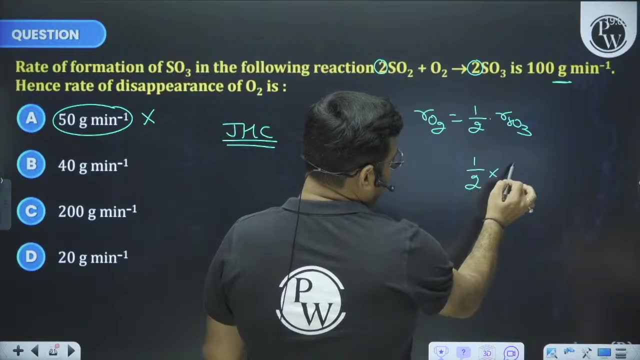 That is why I am telling you this kind of question: That, brother, you have to write the relation. After that, you have to do this much. Now you have done only 1 by 2 into 100.. That is why your answer is 50, which is wrong. 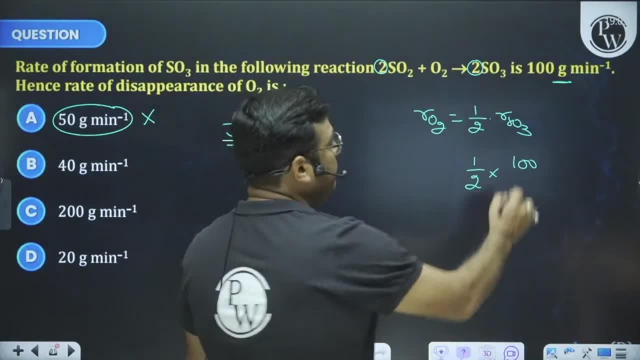 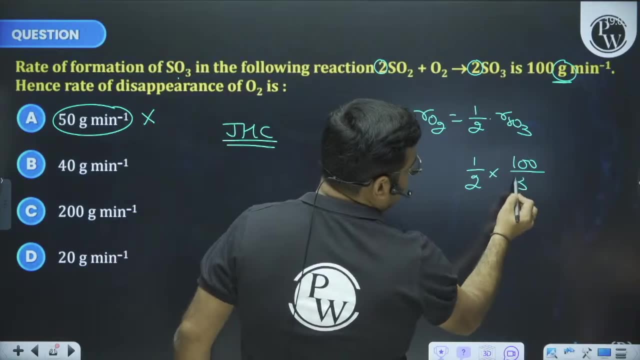 If the question is about mass, then, brother, whose mass is given? whose rate is given in the terms of mass? Sir, whose is this SO3.? Divide it by its molar mass. How much is the molar mass of SO3?? 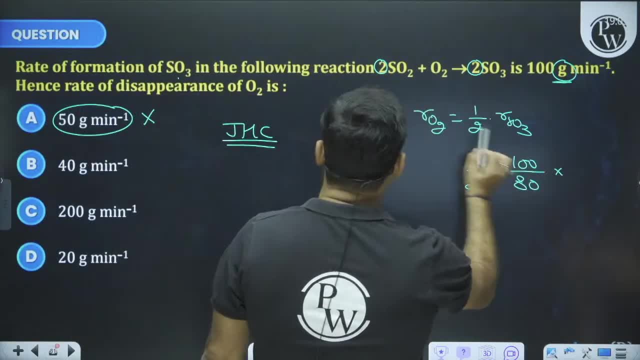 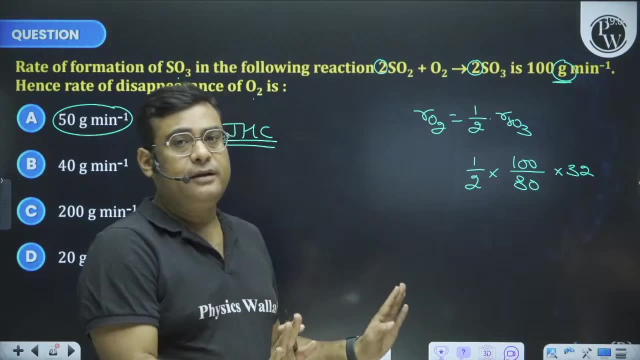 80. Divide it by that. And the one who is asked Sir, who is asked Oxygen, Multiply it by its molar mass. Now, this is the logic. These things are going on. Now I am telling you, just keep in mind. 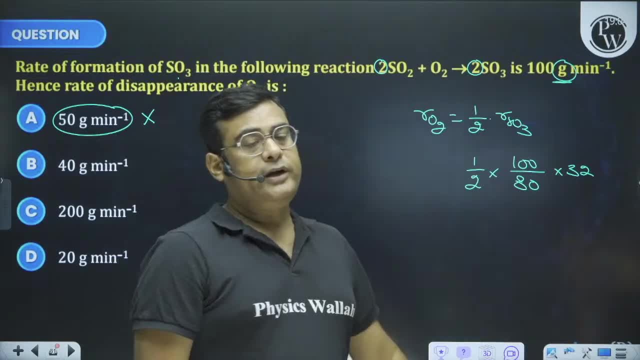 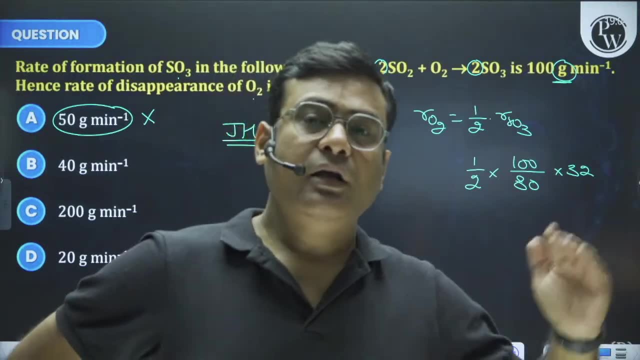 To do it quickly. I did nothing. If I am dividing 100 by 80,, then I got the moles. I got the moles for me And later I multiplied it by 32.. So by multiplying the moles of oxygen by 32,, 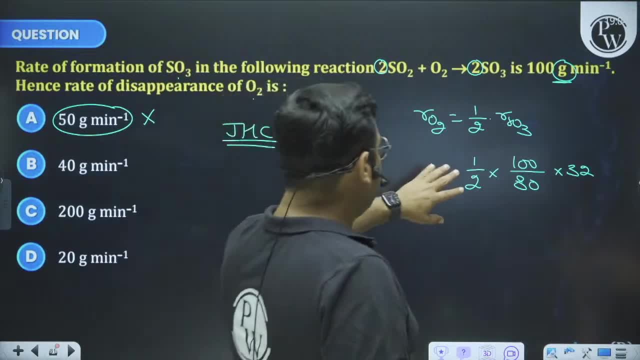 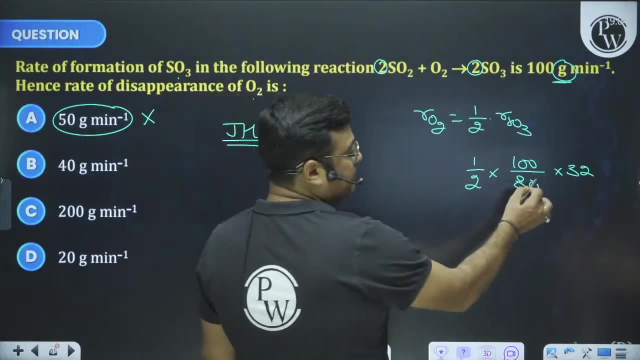 the mass came. So that's why I am talking about the exam. There is not much time in the exam We have to keep in mind. We just have to keep in mind one trick of mine: JSC. Now you see, your question has become easy. 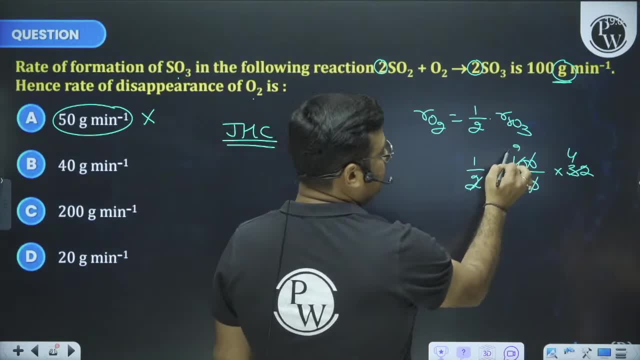 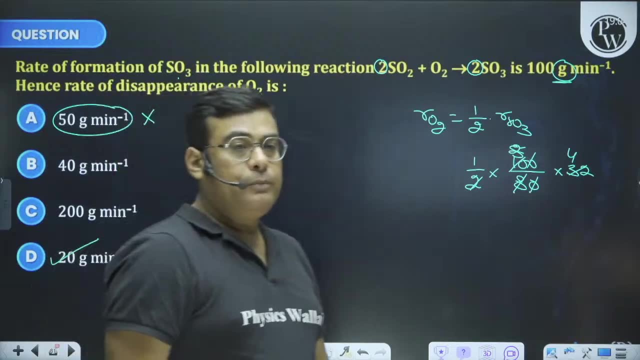 8, 4, 32.. How much is your 2?? Sorry, 5. And 5, 4.. How much is our answer? Son 20.. In Jaldivazi, the answer is normally: student ticks 50.. 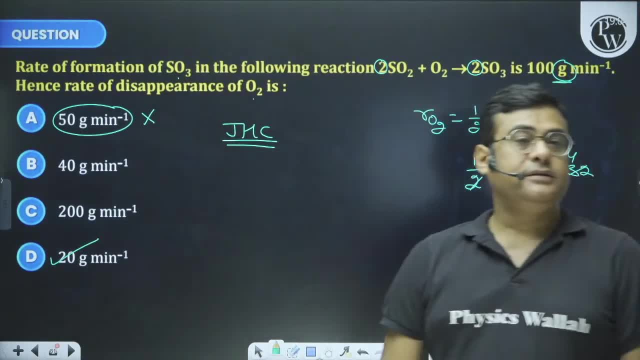 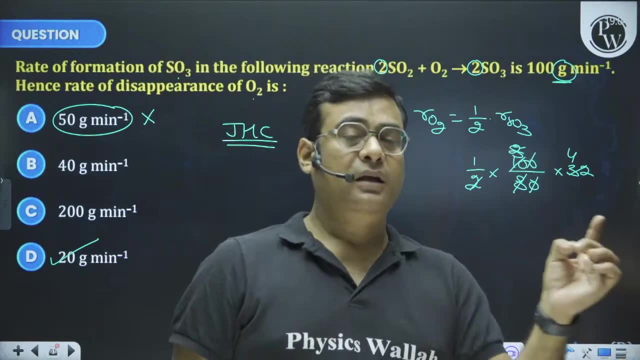 And even among you, maximum children gave the answer A. That's why my rating of this question is important: That it can come, Many children can get it. Only this small, small trick. Be sure to keep in mind. Okay, my dear children, 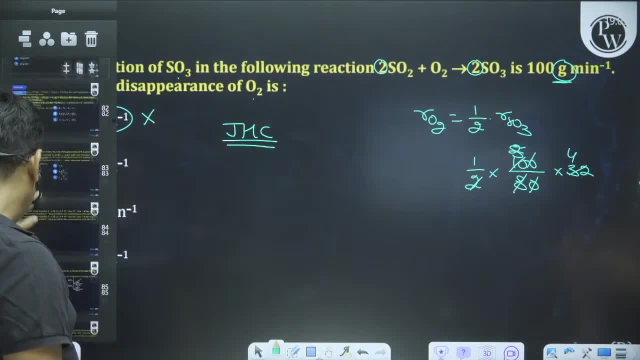 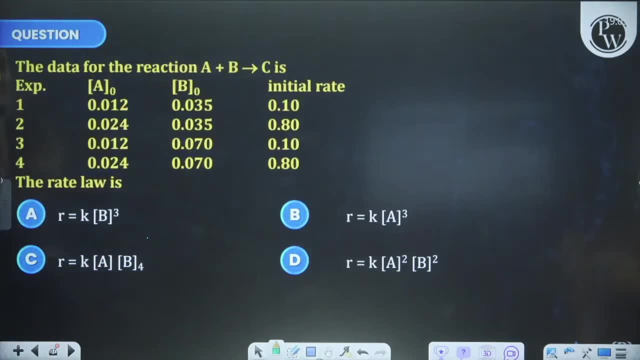 Now there is no end to the questions, But we will do more questions now We will do more. Come on, Like this question, I will tell you. Question on the Initial Rate Method. Now, how do you still do this? I don't know, son. 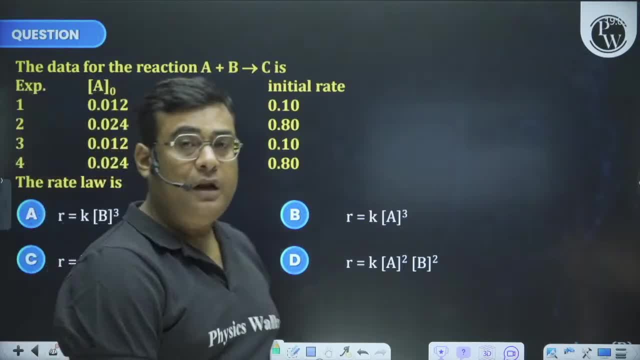 How will you do it now? I know that for sure. I am telling you how to do it now, So I can definitely tell you that to keep in mind. in this kind of question, you don't have to write anything, Just your eyes, your eyes. 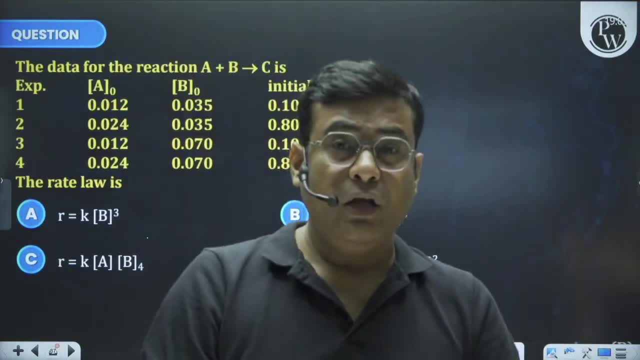 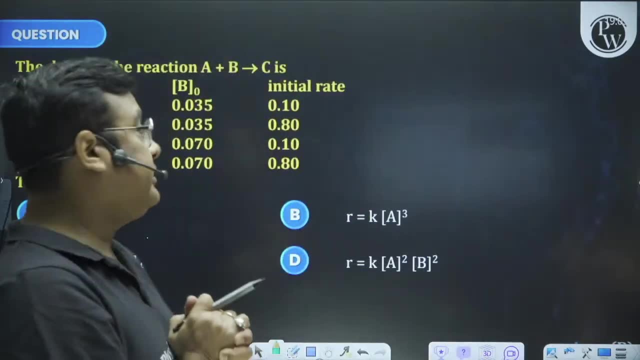 and the brain that runs with you. that's what you need, son. Only those two things are needed. What are you trying to say, son? I'm trying to say this, son: You see, in the first and second experiment, 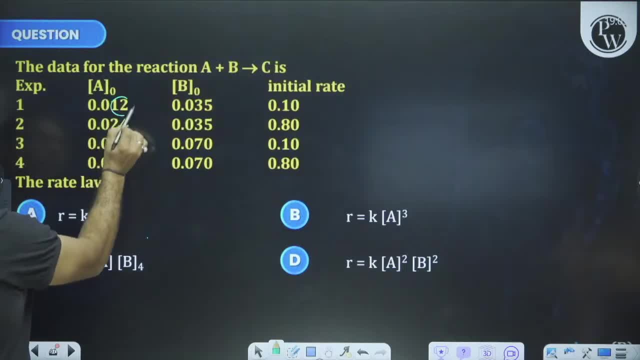 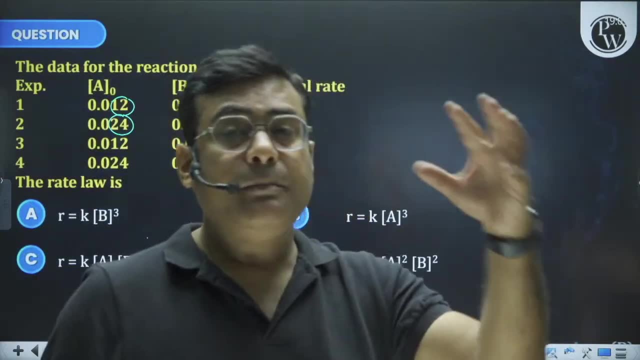 the first thing I said was that after the decimal, the places should always be the same, The power should be the same. Tie a knot in your mind That it will happen, That it will happen. Tie a knot in your mind That it should happen. 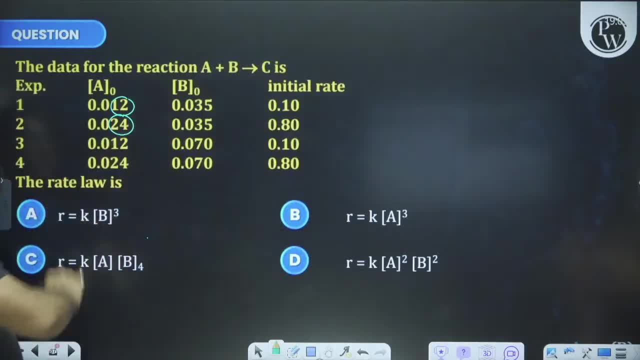 If it doesn't happen, then there can be a mistake. Now after the decimal, like 0.012 is there and 0.024 is there, So I will not increase it to 0.012,, son. After the decimal, when the places are the same. 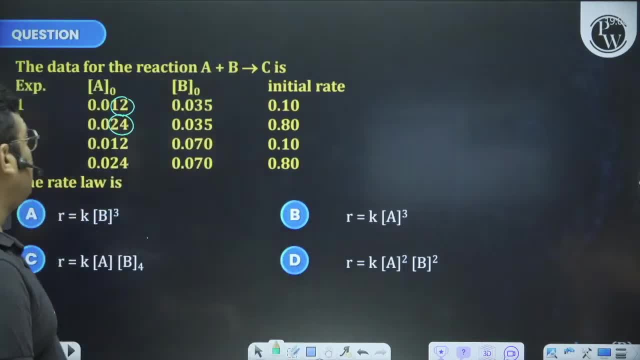 I will increase it to 12.. I want to say this: So from 12 to 24, the rate became double, That is, the concentration of A became double Here. 35 to 35 was also there. No change, Right. 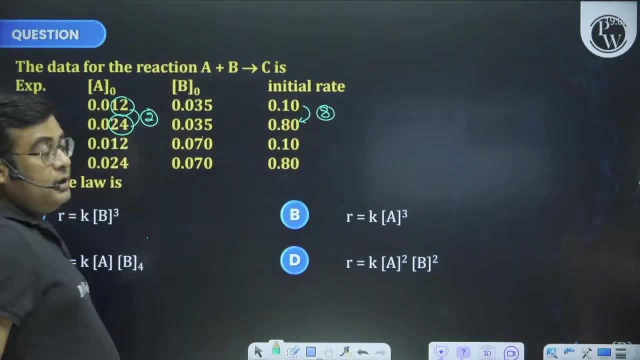 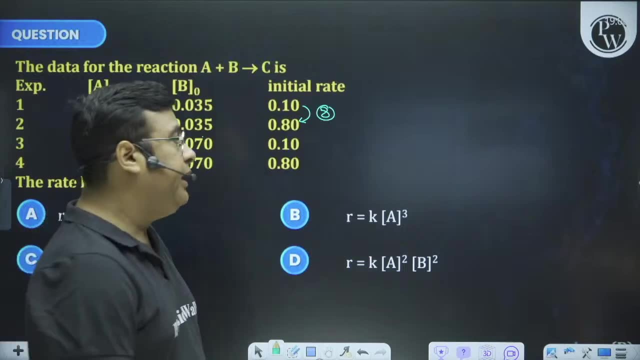 Now let's say 8.. How many times did it change? 8 times 2 times. 2 times the concentration changed, The rate changed 8 times. So, brother, 8 equals to 2, to the power of n. 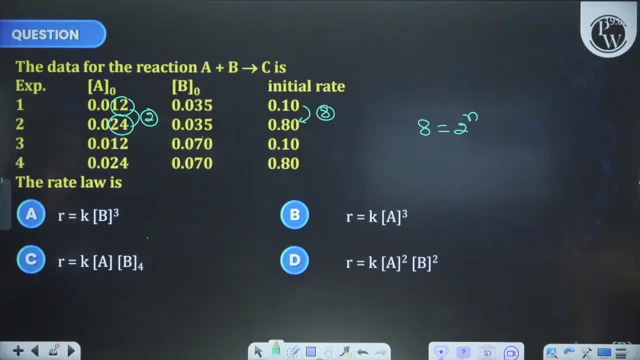 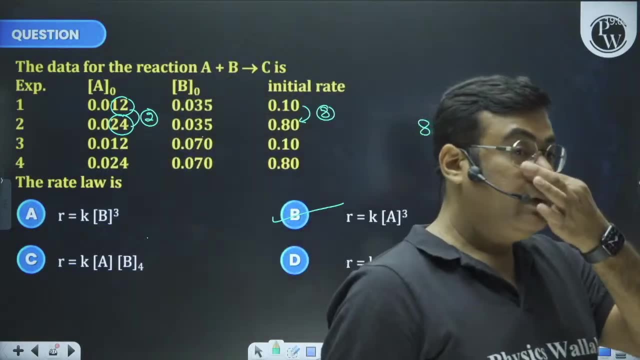 What is the value of n 3.. That is, there should be an order in respect of A. I only saw option number B. I don't need to do anything further. I don't need to do anything further Now. I don't need to see any experiment further. 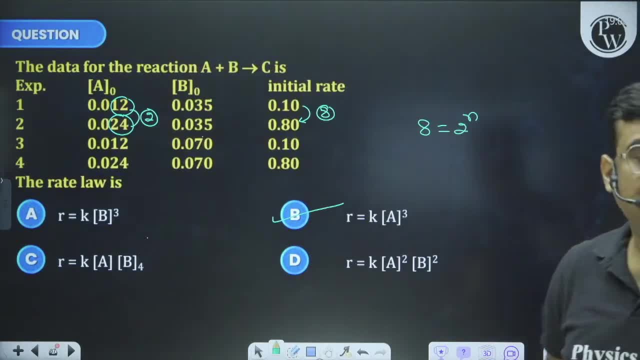 Now I don't need to see any experiment further. Sir, if the power of A was 3 in two options, then what do we do We see in respect of B? Right, Suppose I saw these two experiments. Which ones? Suppose I saw these two experiments. 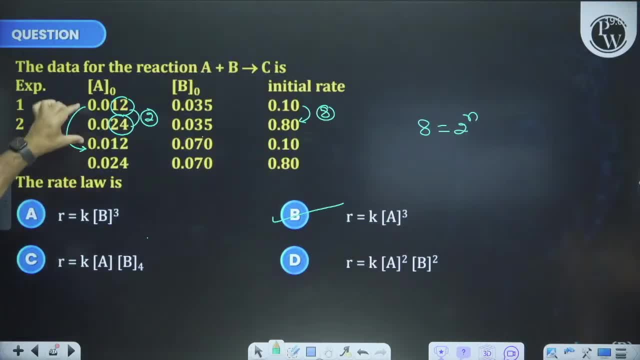 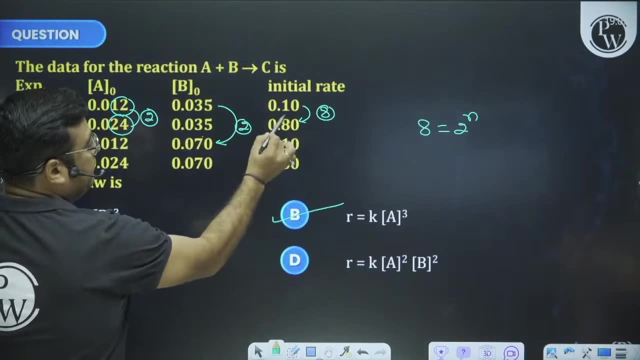 1 and 3.. 1 and 3. In this A is same. 12 to 12 remained the same. 35 to 70 of B became double. But if I see the rate then there is no change in the rate. 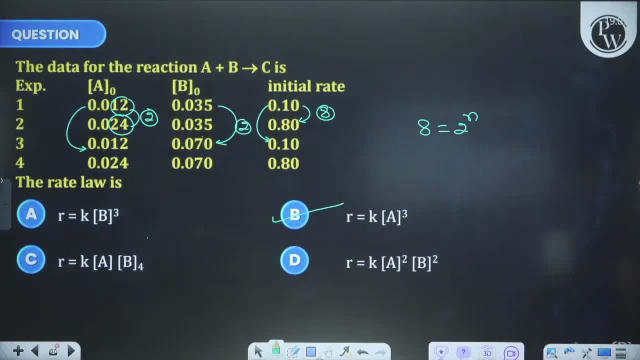 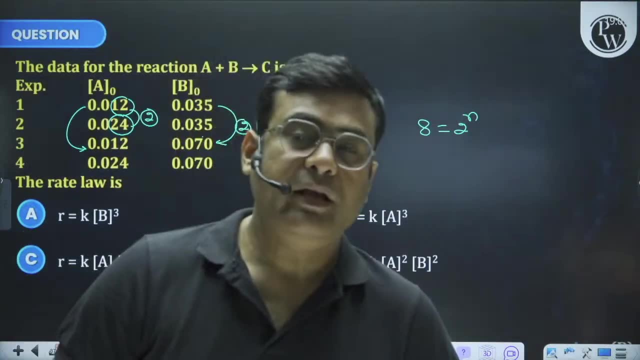 If the concentration changes, then there is no change in the rate. If the concentration changes, then there is no change in the rate. Then such a reaction is of zero order. In respect of B, the order is zero. So I just want to explain to you that. 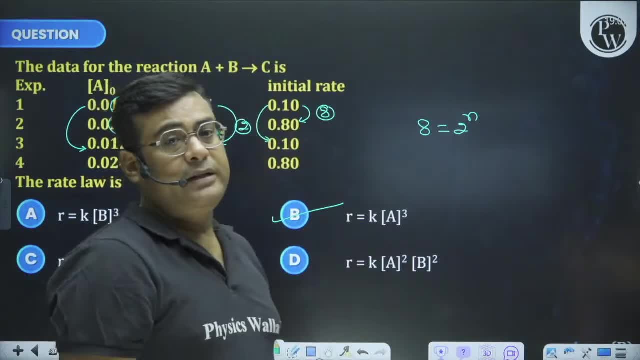 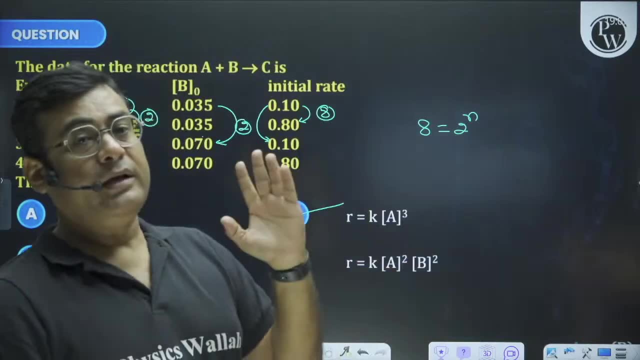 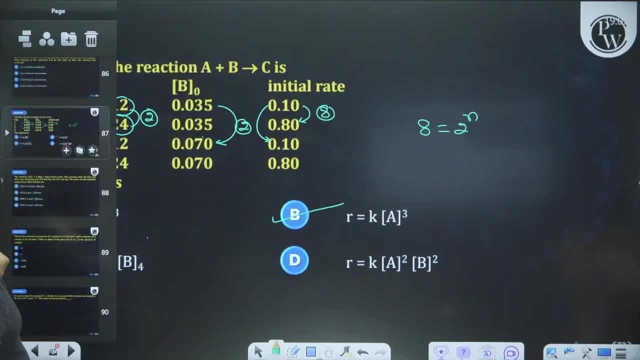 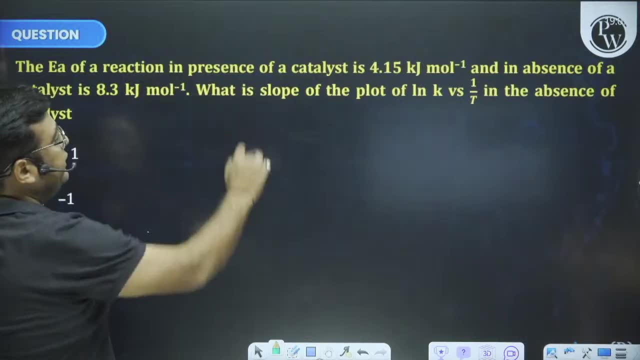 My dear children And I will give you good questions in my support. I have answered the questions of rate. Next question is the question of A? A of a temperature reaction in presence of catalysis. Next question is the question of A? A of a temperature reaction in presence of catalysis. 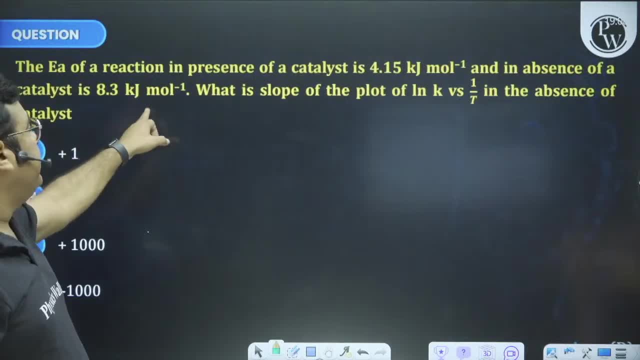 In absence of catalysis, 8.3 kJ per mole. What is the slope of plot of LnK versus 1 by T? in absence of what Catalysis? Now, I have mentioned that Lnk equals to Lna minus of Ea by R. 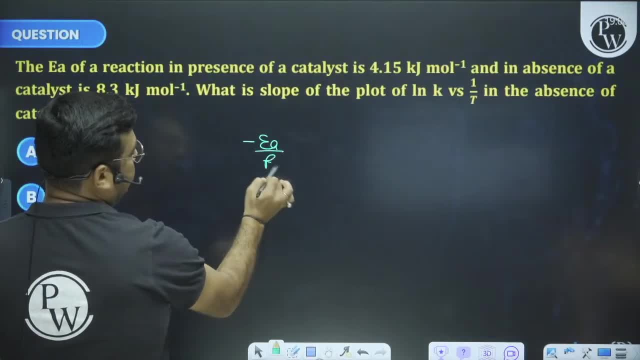 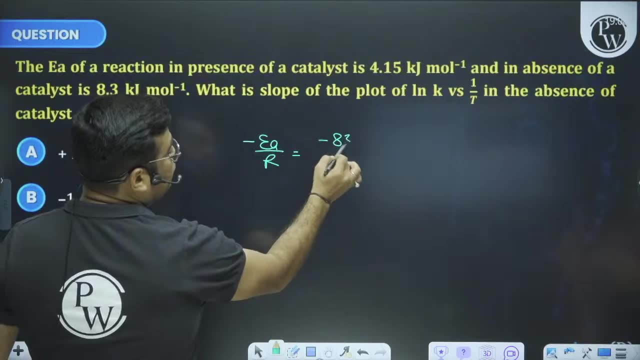 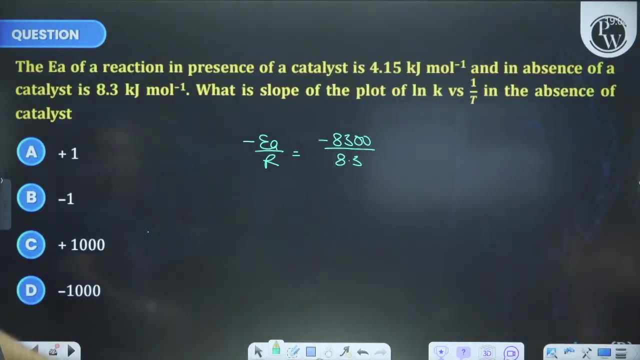 So slope is minus of Ea by R. So slope is minus of Ea by R. The slope is minus of Ea by R. he said how much is the value of Ea? 8.3 kilojoules, Changed kilojoules to joules, and if we take the value of joules of R 8.3, then 8300 by 8.3, straight answer is minus 1000. 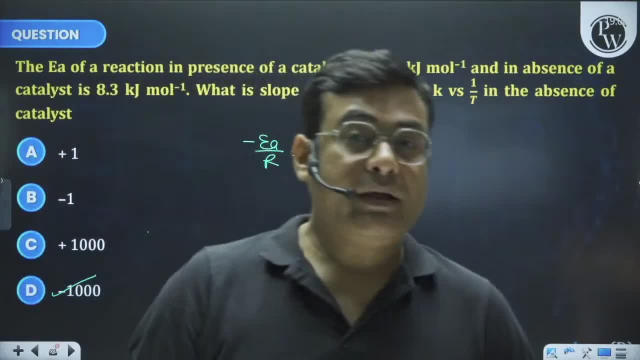 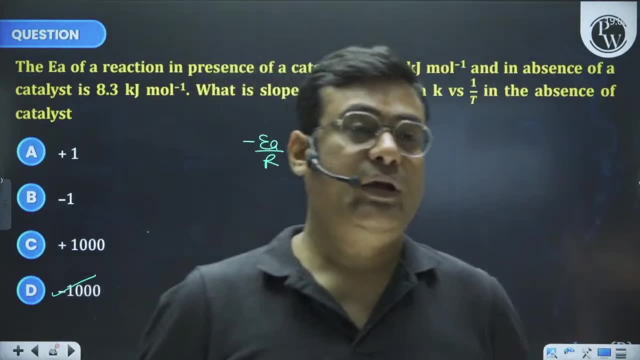 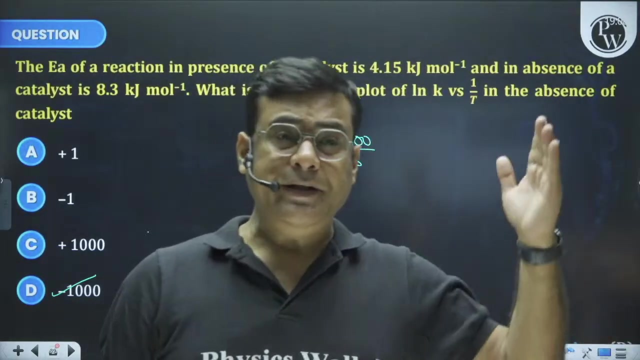 In JEE at least, son, the slope question has come 5 or 6 times. Why has it come Then? why are you asking that question so many times? The logic of asking is this much, son, because JEE has 10 papers of 19,, 20,, 21,, 22,, 23 and 24.. 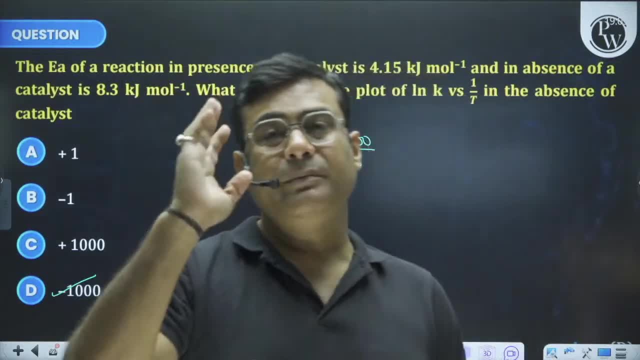 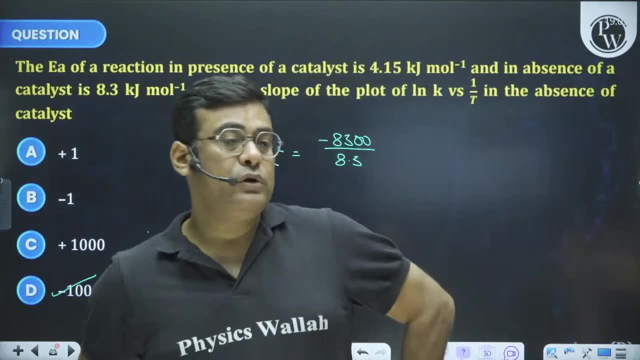 So if you mix the whole year so far, then 70-80 papers have been done, son, And in 70-80 papers if he has asked you 7-8 times, then only 10% has happened. If he wants to ask a question from chemical kinetics, son, then the weightage of these questions is there. 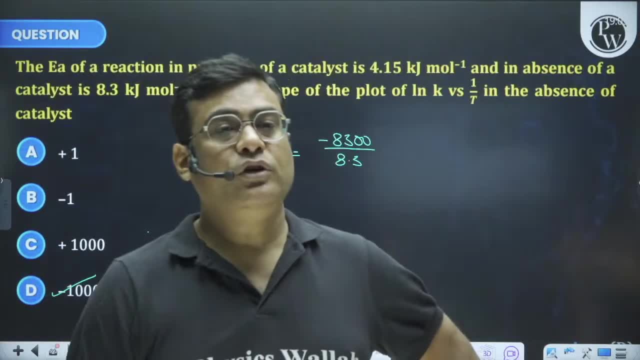 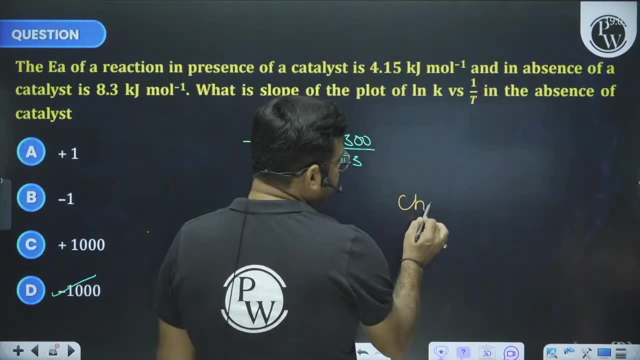 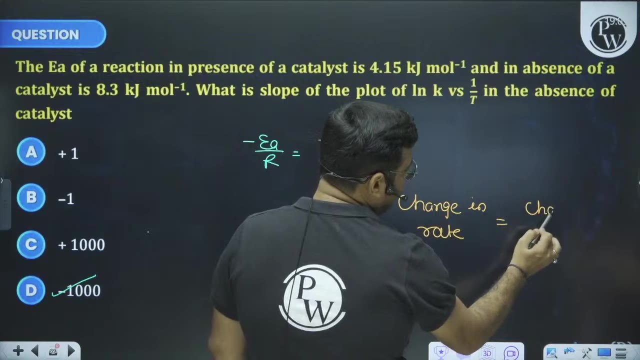 You will get them. You will have to ask him Where did the expression of rate equal to 2 to the power n come from, Son? that is the formula. If you do not know, I am telling you that Change in rate should be equal to change in concentration's power order. 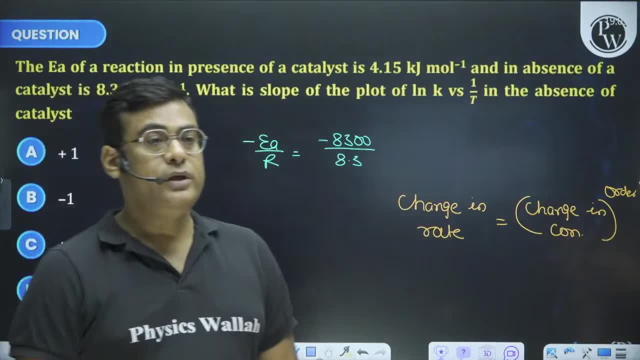 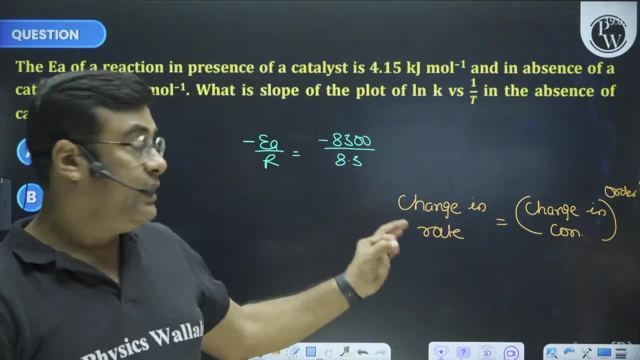 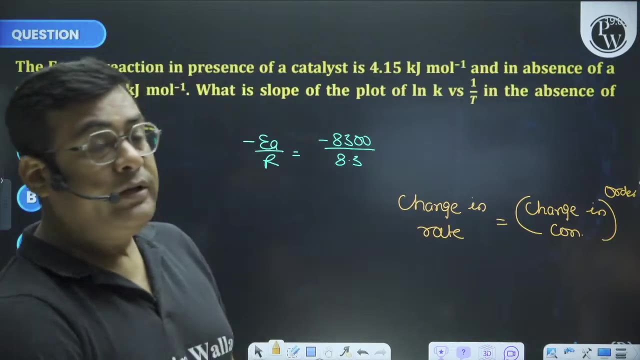 Son, those children who do not know this formula, son be sure to keep in mind What is change in rate? Change in rate equals to change in concentration's power order. Change in rate equals to change in concentration's power order, Son 2.303.. 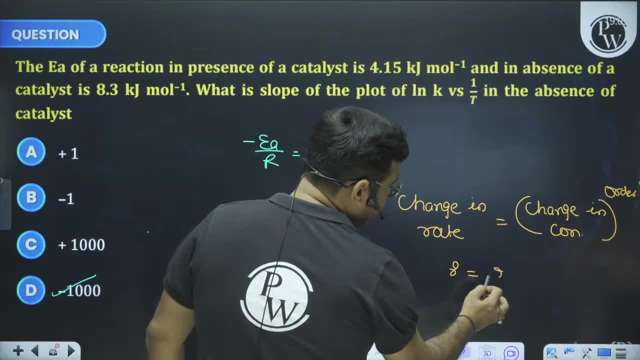 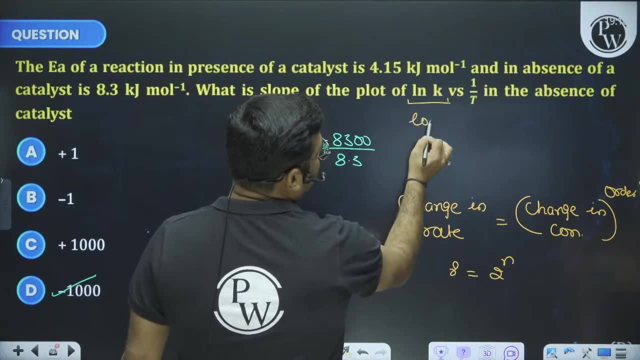 So change in rate was 8, son, Change in concentration was 2.. I took n as the order, Son. 2.303 is there? son, I told you that Maybe you did not hear. If it was log k here then minus of Ea upon 2.303 R would have been there. 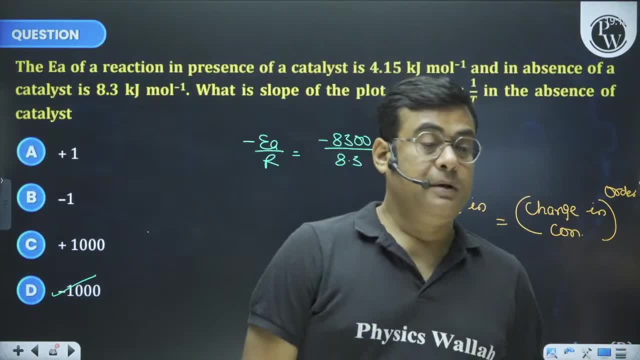 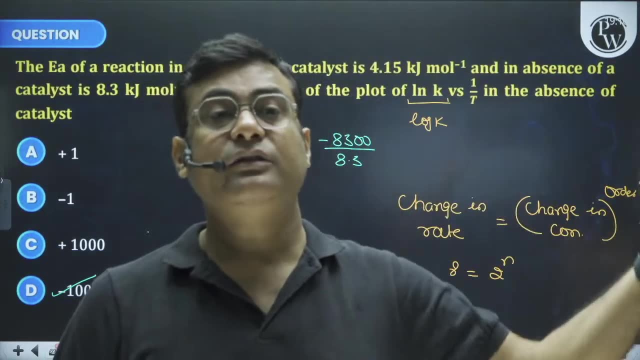 That is why, son, Now the exam is after 4 days, Isn't it Okay, Son, formula can be there. Son someone tells you, teacher does not tell, can also ask a question directly. I am at least making you recall formula, son. 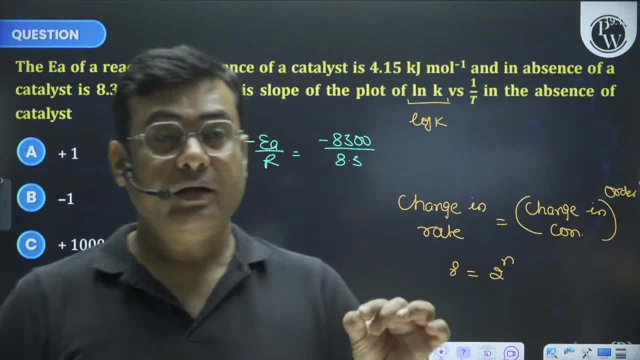 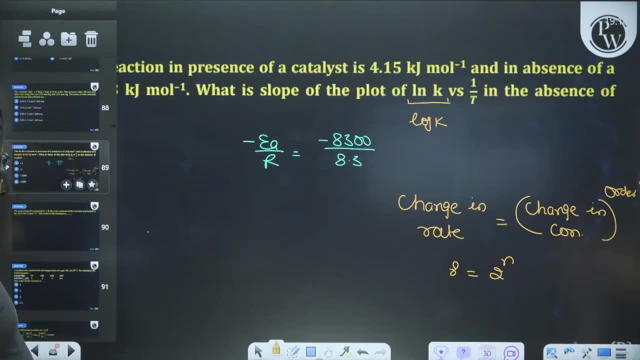 So I will also request, son, If I am making you, then be sure to keep it in mind. So, be sure to keep it in mind. Okay, Let me tell you another question, son. Look, we will have only this much time. 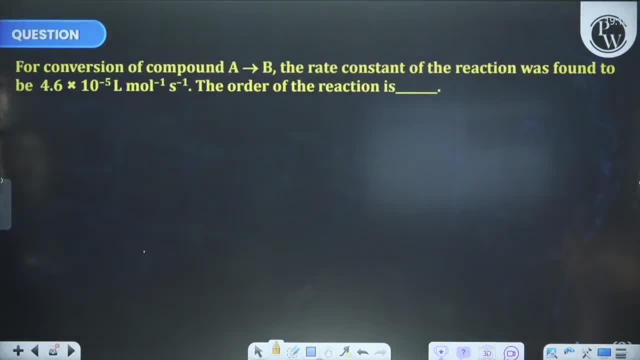 Look, the next question is JEE's question. This is also Son for conversion of compound A to B. Conversion of compound A to B, the rate constant of reaction was found to be this order of reaction. Now in JEE, this is also a question that has been asked for 3-4 years. 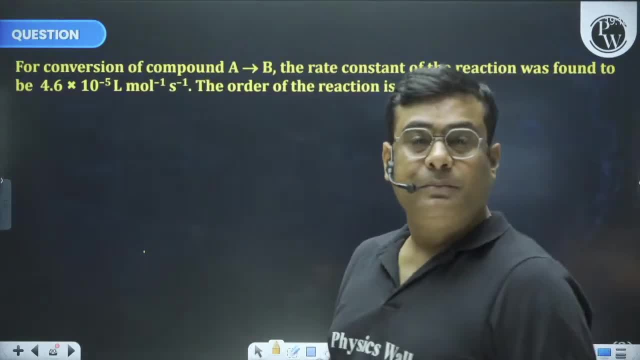 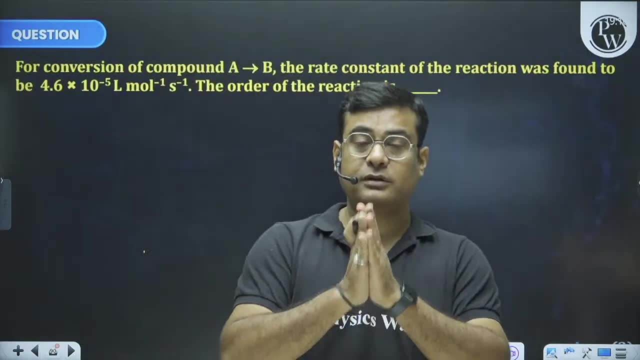 You will feel that, sir, what a joke you have made by raising so many simple questions- and you are talking about JEE questions. I have no status. I am the world's smallest creature. I am the world's smallest creature. I have no status in this world. 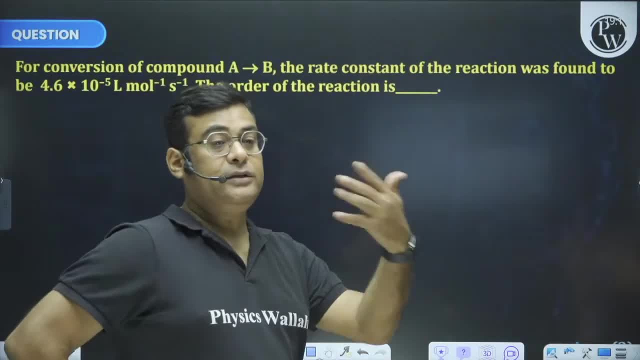 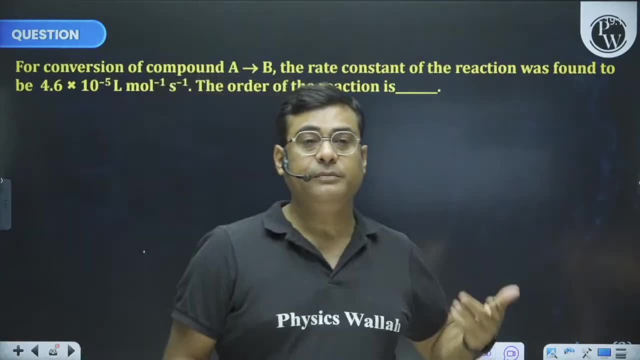 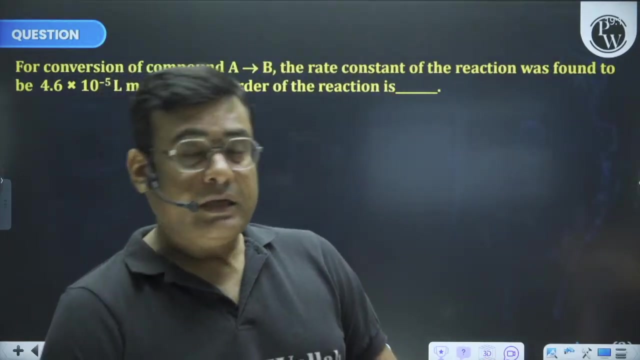 My status is that you are like children who study from me, who understand things, and many of my students have become doctors and engineers in thousands, so that's why I have a little status. Okay, but the brother of JEE who is asking? he is asking, we will have to answer him. 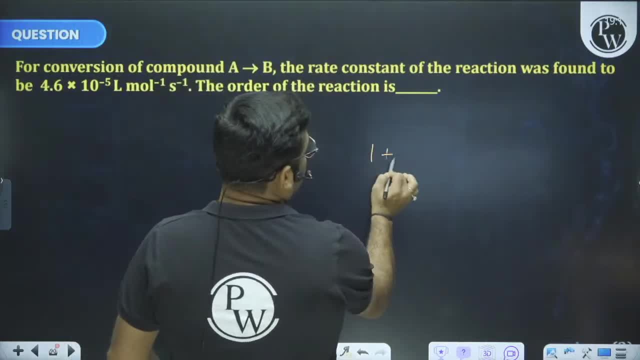 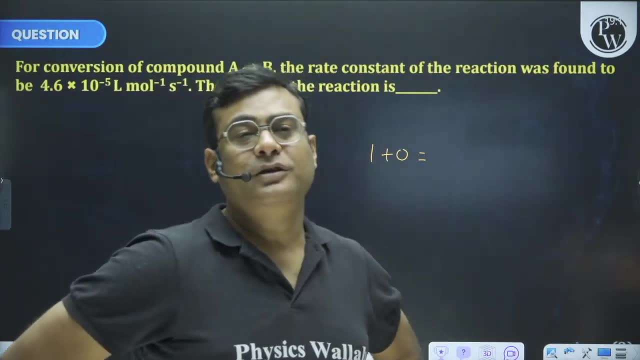 Tomorrow. he told you that 1 plus 0 is not how much. it is that the question should come, So you will not say that this question is not of my level. I cannot fall so much that I will answer this question, Brother. 1 plus 0.. 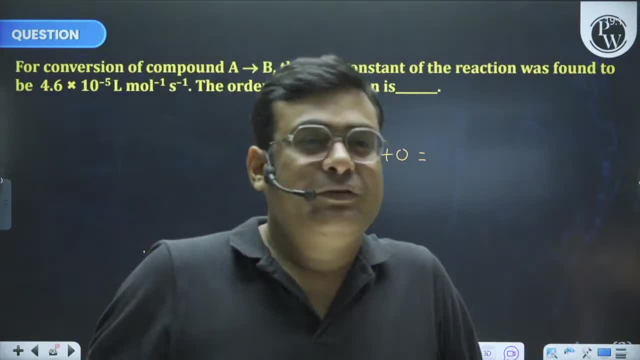 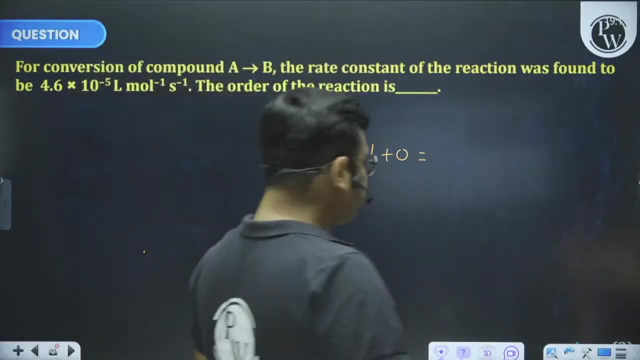 1 plus 0 is 1, you tick yourself, move ahead, right. So that's why we have to answer whatever the brother will ask. It is his wish, whatever he asks, Okay. so, brother, in support of this question, I am showing the next question again. 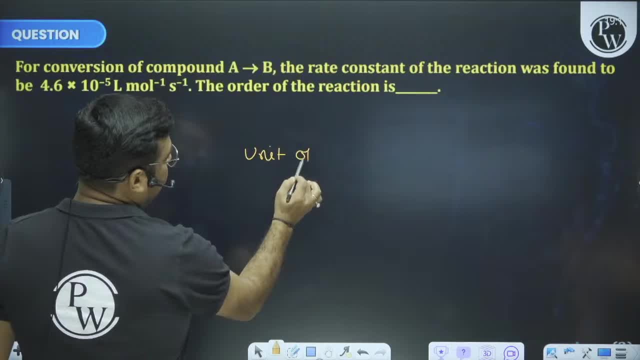 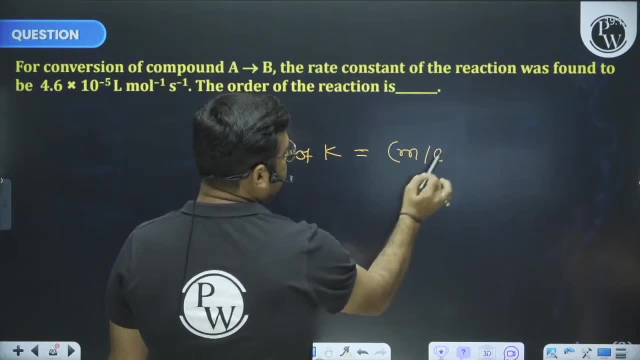 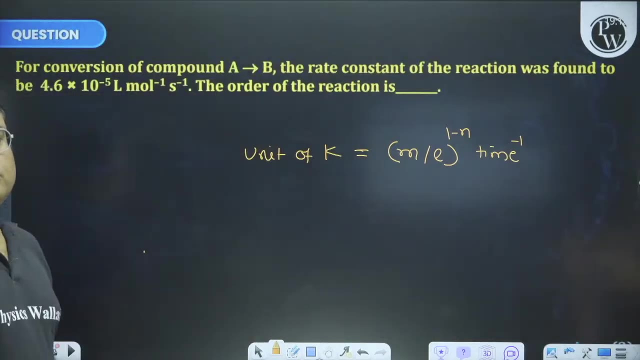 We should know the general unit of K which gives me full hope. Maybe every child of you will know. it is the power of mole per liter, 1 minus n and the time inverse, where n is the order of reaction right. 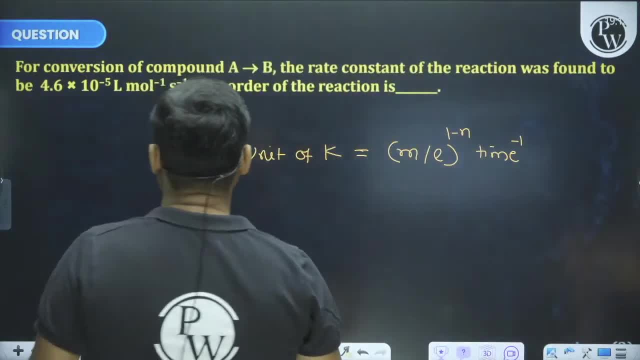 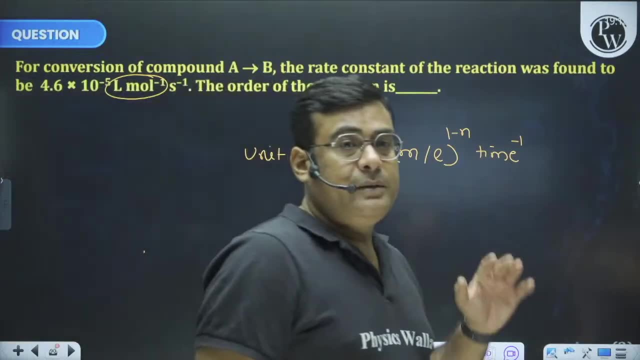 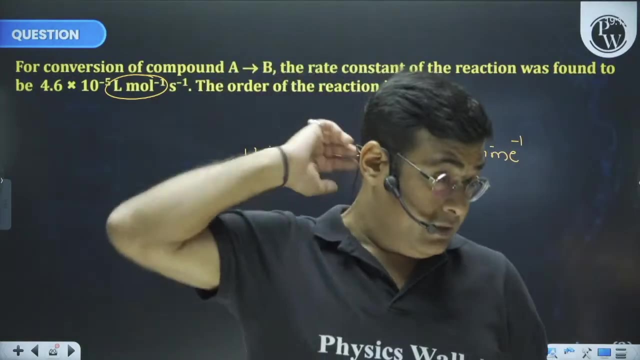 It is the order of reaction And if you see here many children are confused. what else is given? So when this chapter is taught, any chapter in the world any teacher has taught you, he must have said again and again that we know the order from the unit of rate constant. 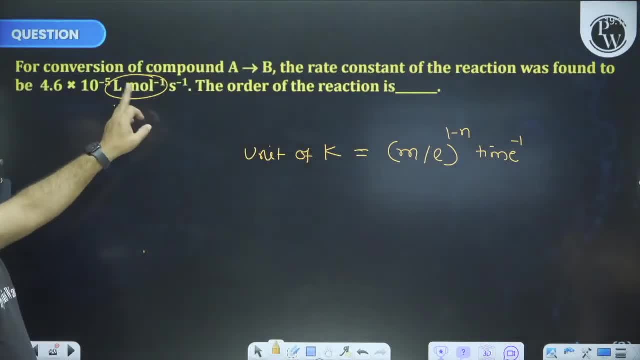 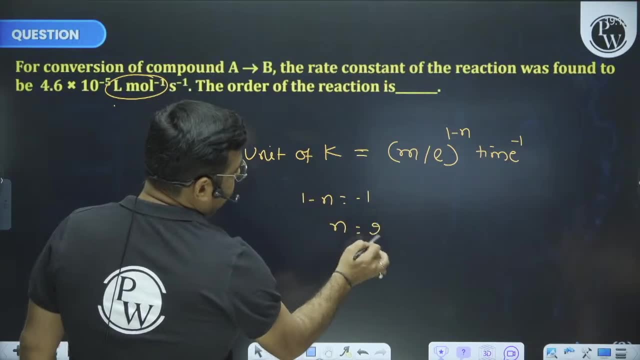 And JEE has asked this question many times- Children. I can write the mole per liter as the power of mole per liter minus 1, and 1 minus n equal to minus 1, that is, the value of n is 2, right. 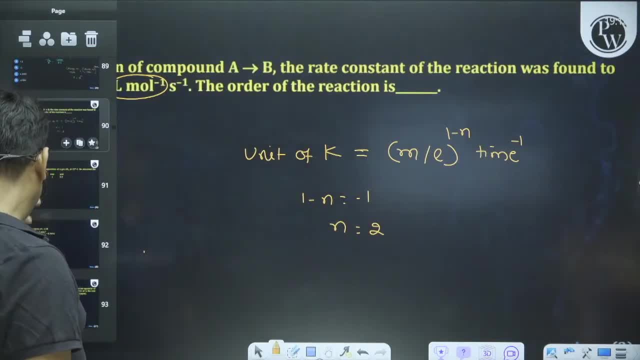 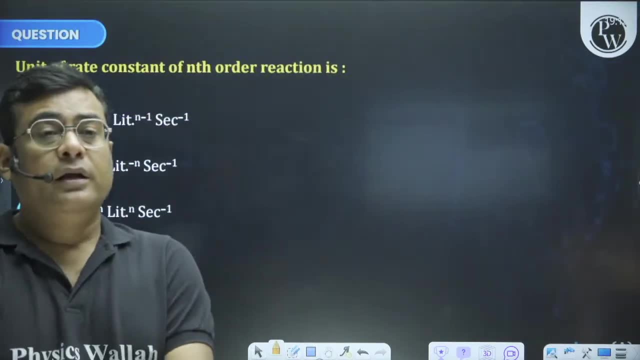 In my proof I am showing it again that. what did JEE do? JEE also asked this question once. Unit of rate constant of nth order reaction. Unit of rate constant of nth order reaction. I have asked directly, right, What did he do? children? 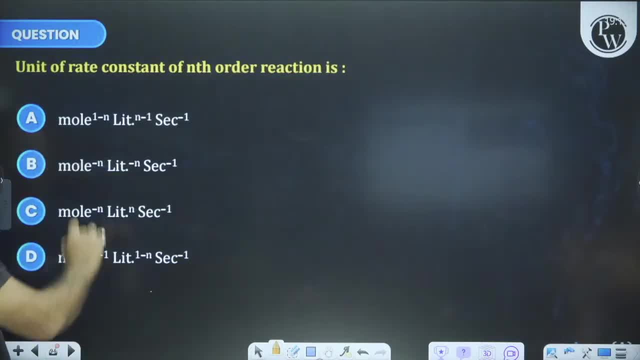 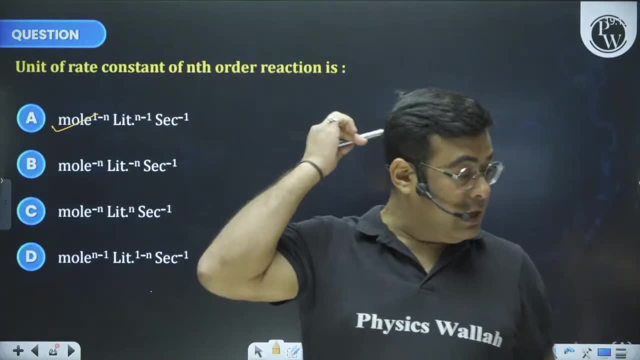 Opened, elaborated and written. So the power of mole is 1 minus n, The power of liter is n minus 1.. The second is inverse. Okay, We consider JEE as air. We make it, Although I am saying again and again that this is a repetitive exam. 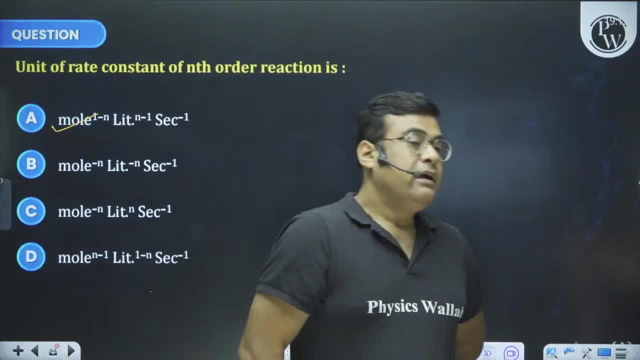 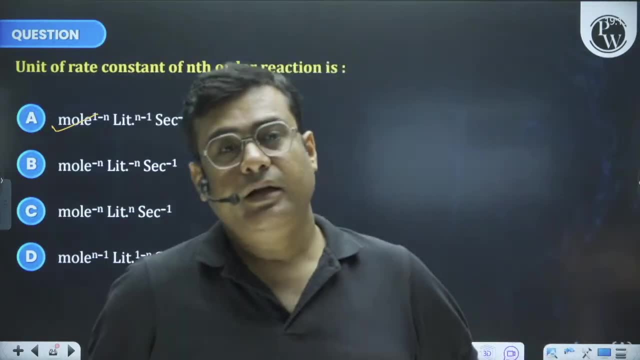 If you have taken the names of all the years that I have taken right, If you have attempted the questions of the previous year properly, child, then you will see again that you will get the same question in repetitive form again and again. In fact, I am ready to give you a guarantee. 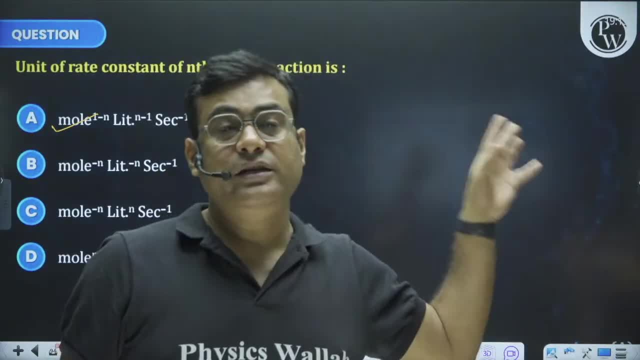 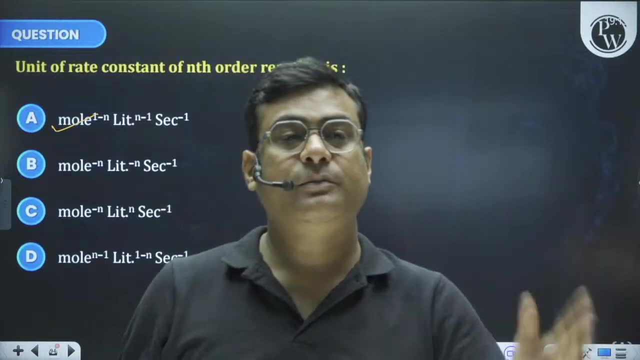 That JEE means the last question of the January attempt of 2024, which I have given you together. If you do that too, then you will see 20 to 25 percent of the questions will be repeated. Okay, Now let me tell you some questions of my time. 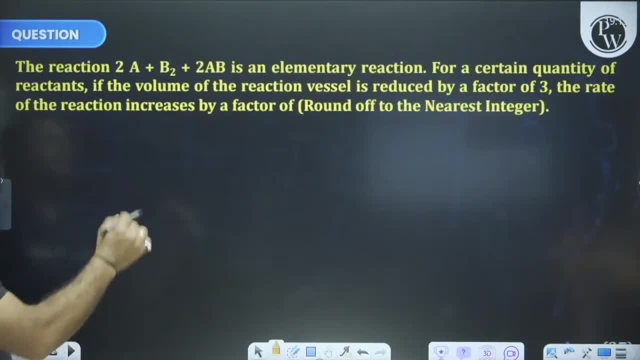 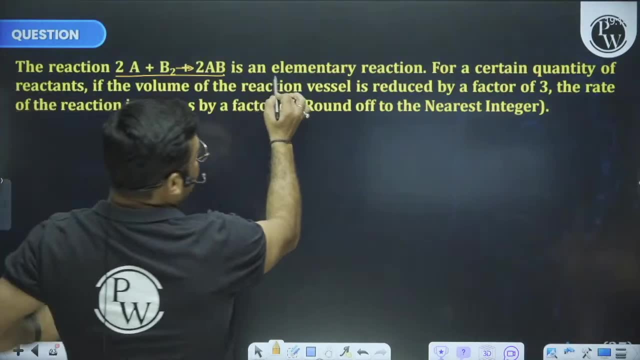 See, there are also such questions in this. The reaction 2a plus b2 gives 2ab. The error made by the operator is an elementary reaction. Now, as soon as I get the elementary reaction, I should understand What is an elementary reaction. 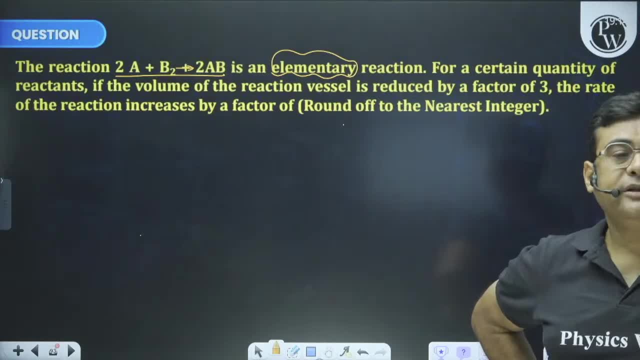 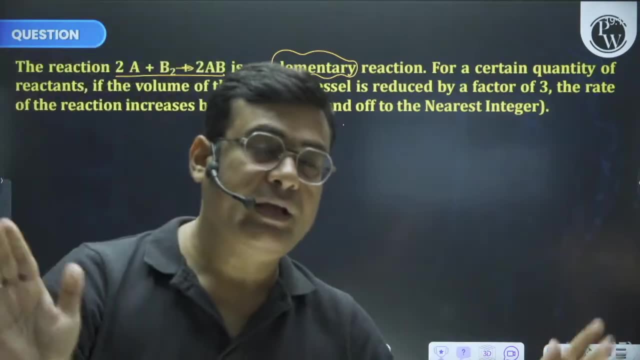 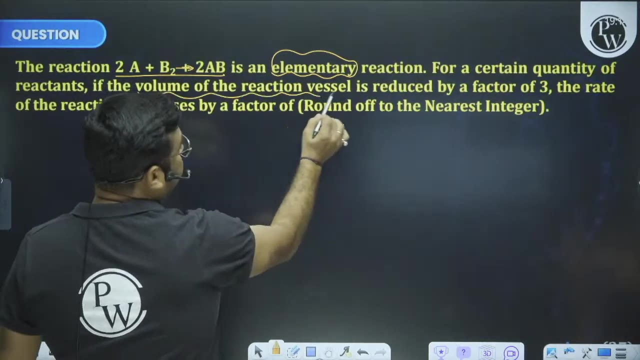 There is an elementary reaction child in which the reaction is completed in a single step, in which no reaction is intermediate, whose graph is of a single mountain For a certain quantity of reactant, if the volume of the reaction vessel is reduced by a factor of 3,. 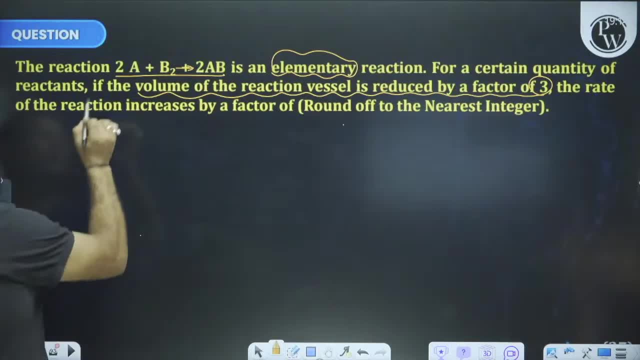 what is the next point of the elementary reaction child, Which is the coefficient? The order is the same, So the coefficient of a is 2 and b2 is 1.. If the rate law is written, because the elementary reaction has also used this word many times- 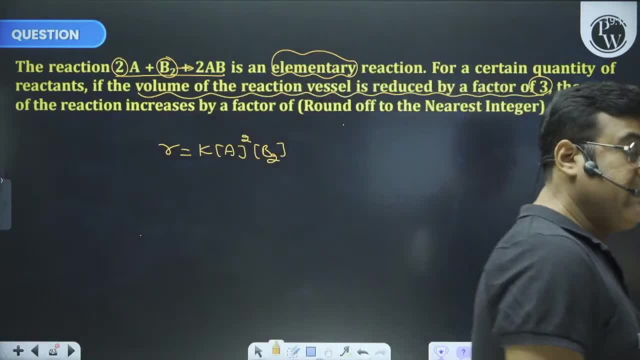 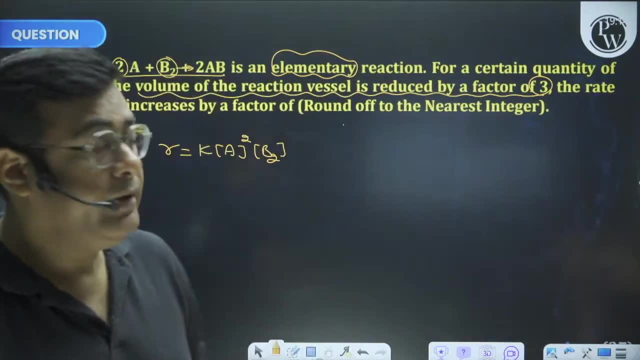 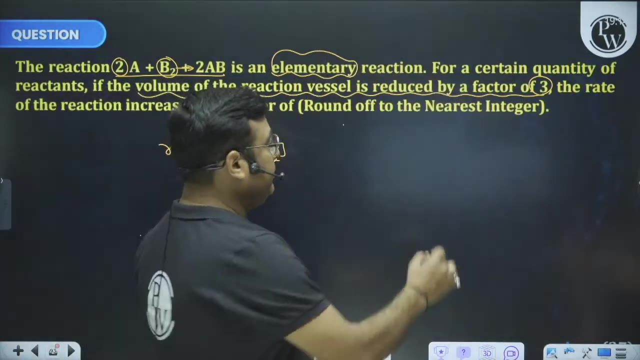 I hope everyone knows, but in the revision we want that everything is covered. Okay, So I should know all these points. with respect to the elementary reaction, So if we reduce the volume by a factor of 3. I know that the concentration is inversely proportional to the volume. 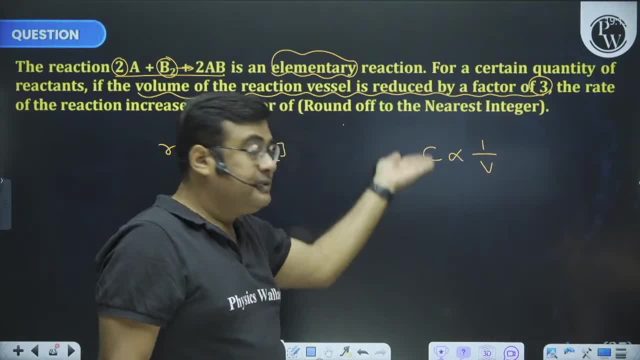 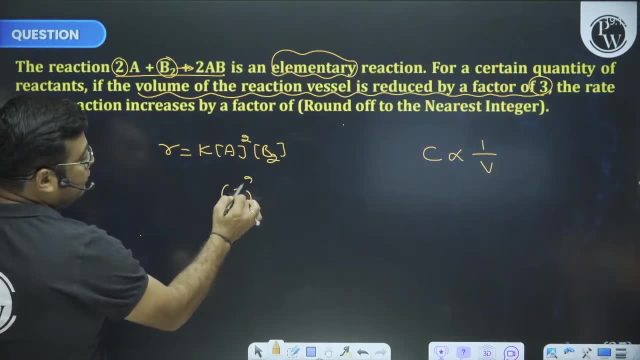 So if the volume is reduced by a factor of 3 and the concentration is increased by a factor of 3. Whose Sir a's and b's? So the concentration of a is 2.. The concentration of b is 1.. 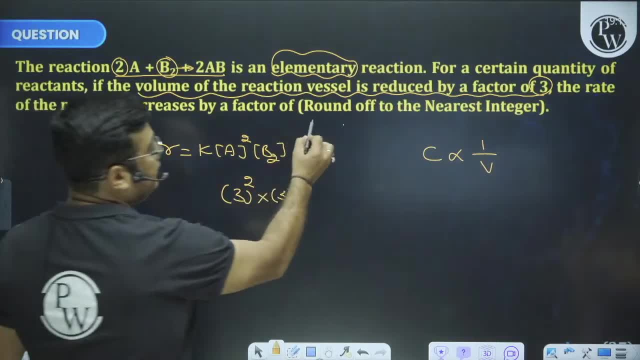 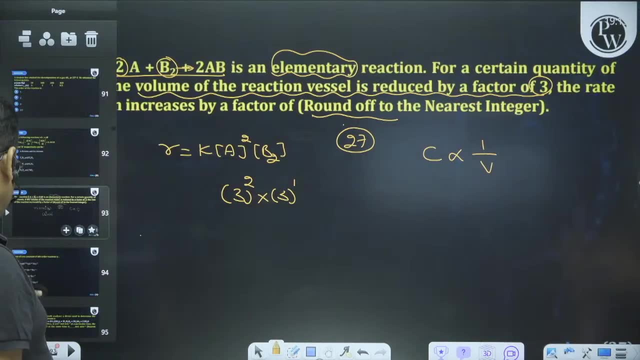 The square of 3 is 9. And 9 times 3 is 27.. Round off to the nearest integer. This is the answer. This is the answer, my dear children. Okay, What should I tell you? See, the next question is also written on the rate. 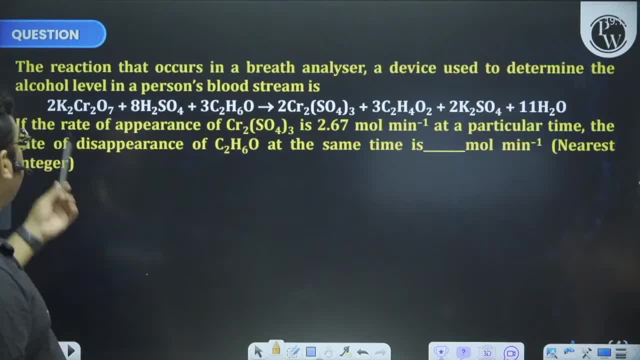 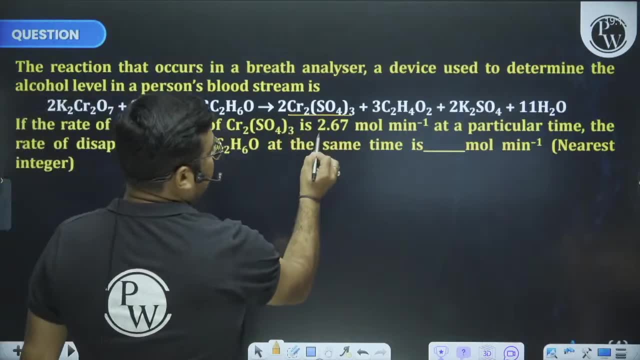 Reaction that occurs in a breath analyzer, a device used to determine alcohol level in a person's blood stream, is this: If the rate of appearance of chromic sulfate is 2.67 at a particular time, The rate of appearance of C2H6O? 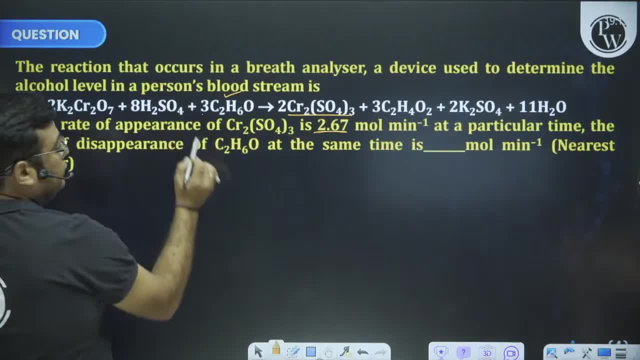 What is the method, my children? If its coefficient is 3, then 1 by 3 into R. If its coefficient is 2, then 1 by 2.. If its coefficient is 2, then 1 by 2 into R. 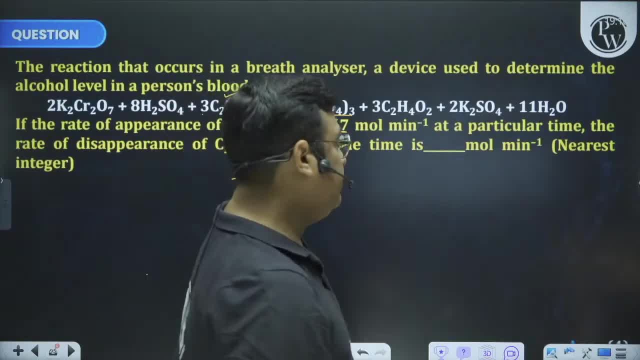 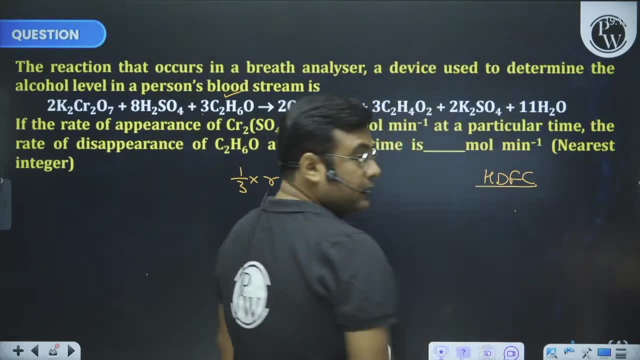 Now you do not have to write, You do not have to spend time. Now again, shall I tell you HDFC, Shall I tell you HDFC, Khirwani's developed fast calculation. What, Brother, if I write 2.67 here, you will enjoy it. 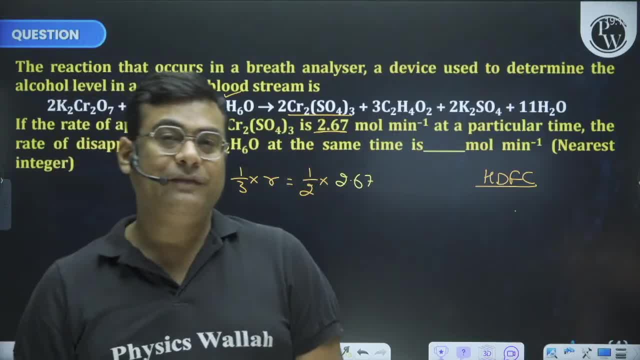 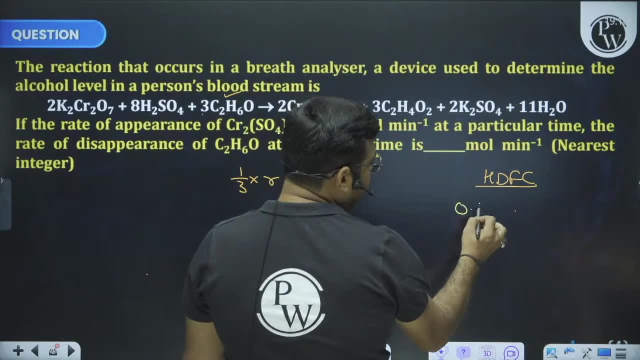 You will enjoy it. It will take so much time to solve. Then divide, multiply. But now I am going to explain HDFC to you. What? If it is 0.33 anywhere, write 1 by 3.. If it is 0.67 anywhere, write 2 by 3.. 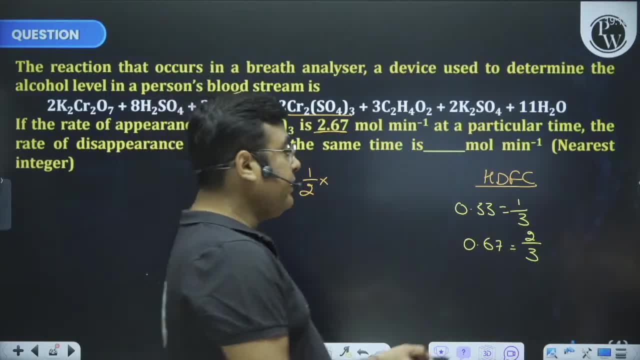 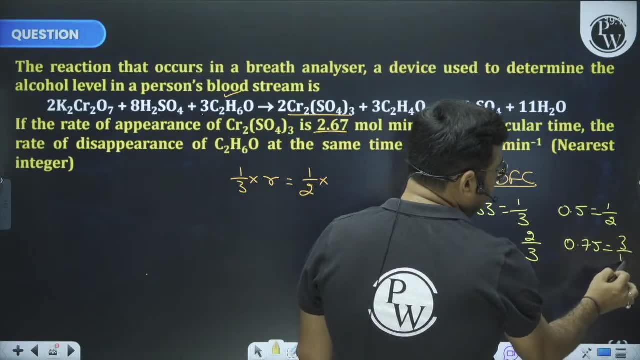 Will you keep this much in mind? If it is 0.5 somewhere, you will write 1 by 2 to 0.5.. If it is 0.75,, you will write 3 by 4.. These are small things. 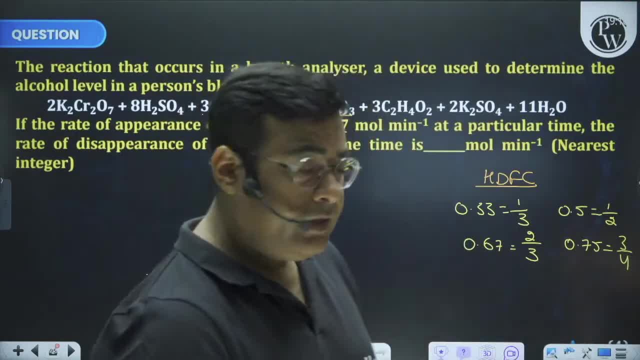 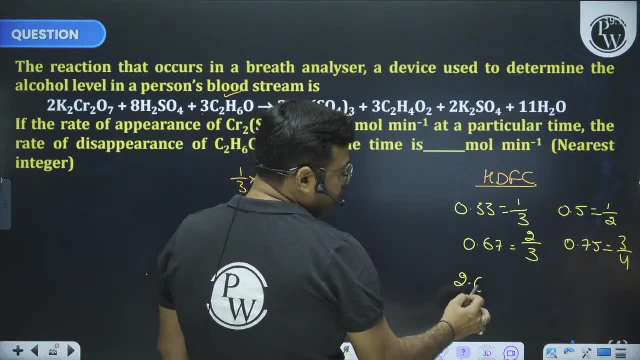 I am telling you again and again, It will fill your pot with drops. Okay, So now, sir, this is fine. I have done this much. This is 2.67.. My dear children, do I have 2.67 in my mind? 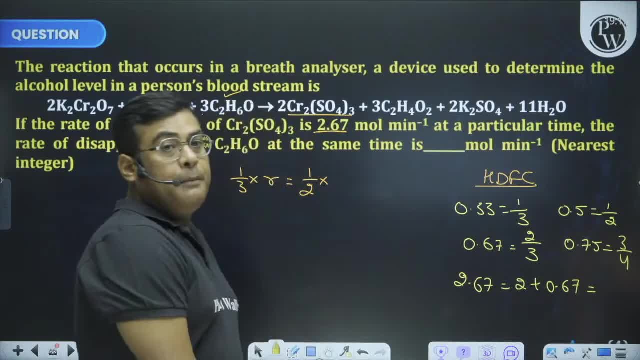 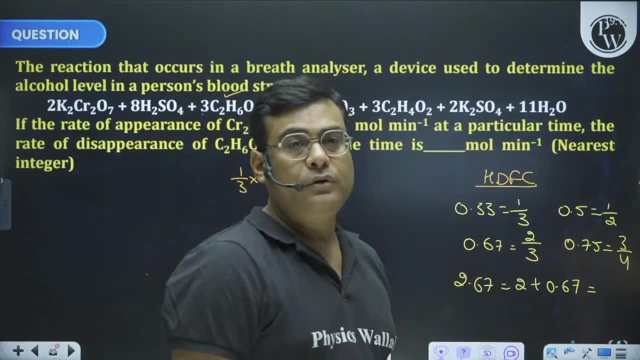 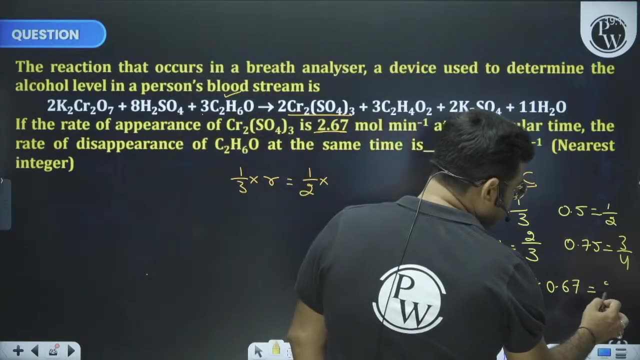 Now you have so much mind, dear Mathematics will be more speedy than you. But we do not think that. And to think that I am explaining you all this: If you write it 2 plus 0.67, then basically it is 2 plus 2 by 3.. 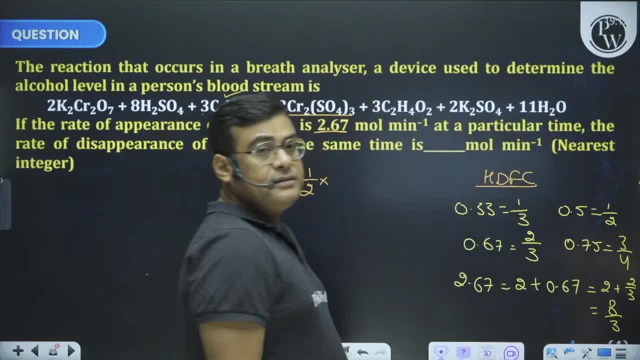 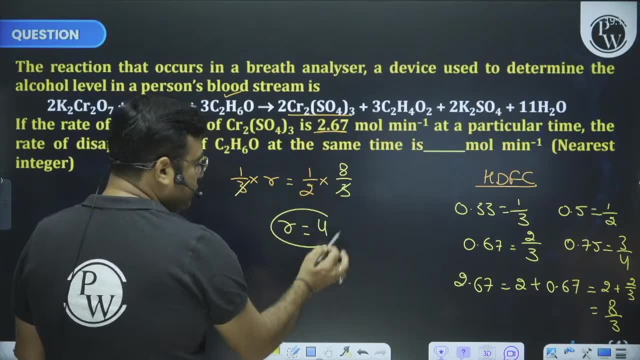 8 by 3 means it is 8 by 3, so even if your answer is in nearest integer, if I write it 8 by 3, see, if you clap on this thing, then the heart will be happy. how quickly, how easily. 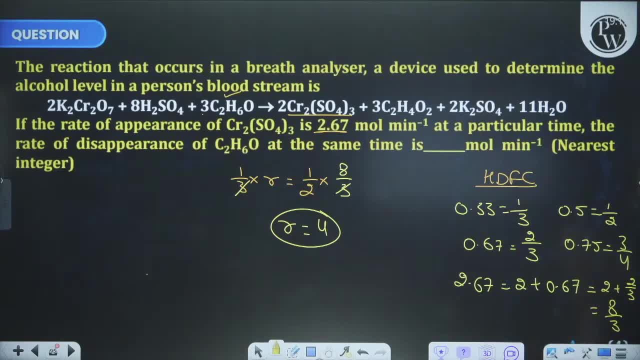 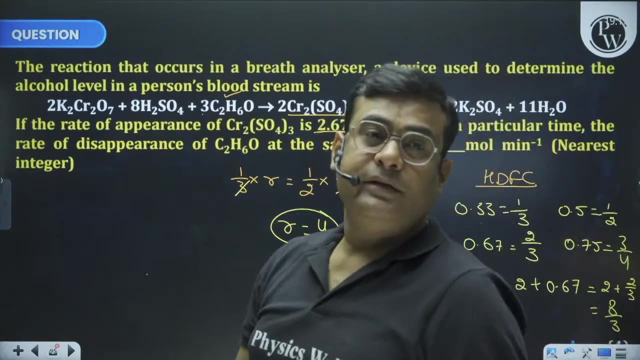 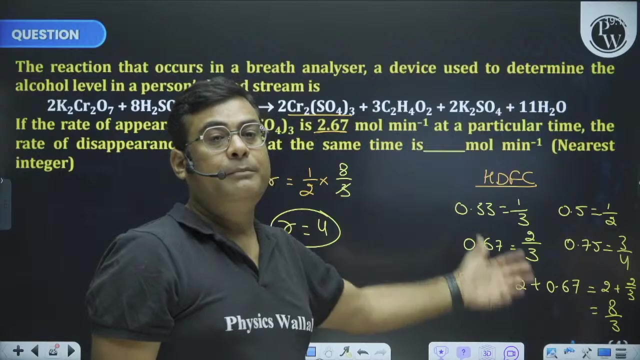 your answer came. tell me how quickly and how easily your answer came. if you had written 2.67, then do 2.67 into 2, then divide it by 4, the answer will only come in the nearest integer. the answer will only come in the nearest integer. so I had promised you a little while. 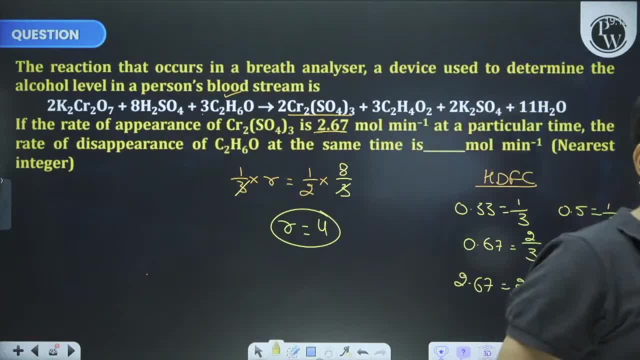 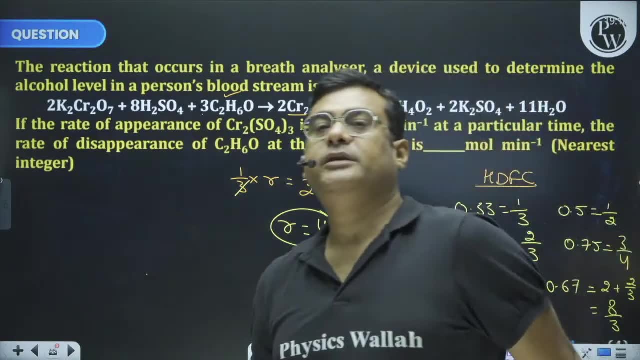 before starting the session: right now, our session is only 2 hours. we have talked for 10-15 minutes, son, and you have not seen at least 15-20 tricks till now. some calculation improvement tricks had also been seen. so if you have not seen any of these tricks, then 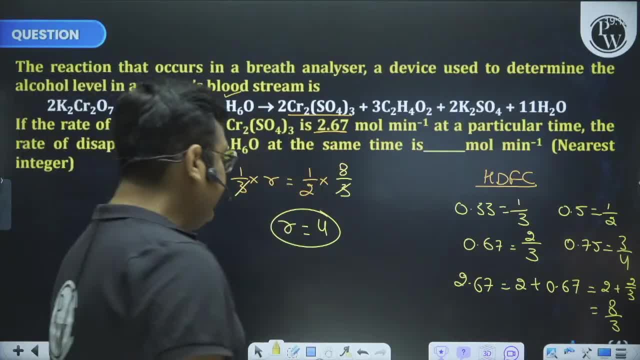 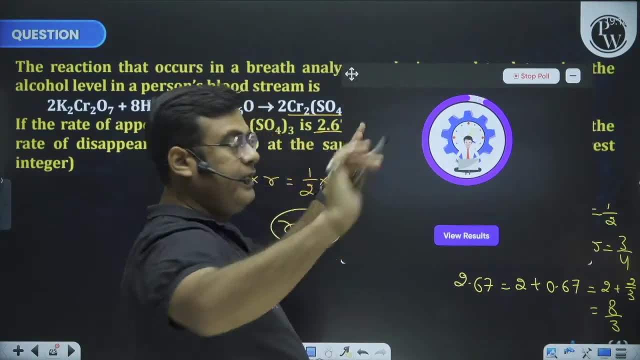 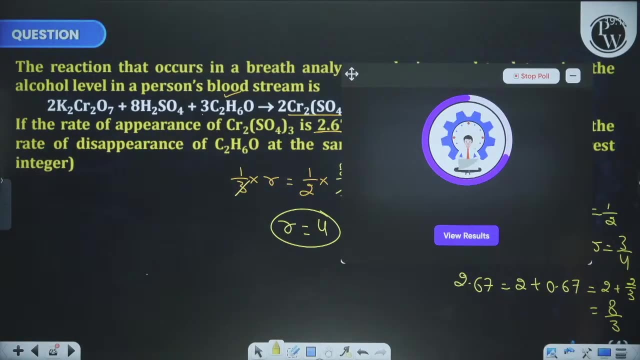 I hope one poll will be done one minute. I will also have a rest of 30 seconds. tell me if we still have things present in a different way, and our promise is that 40-50 things are absolutely new and you will learn unique things. if in 2 hours we have learned 15-20. 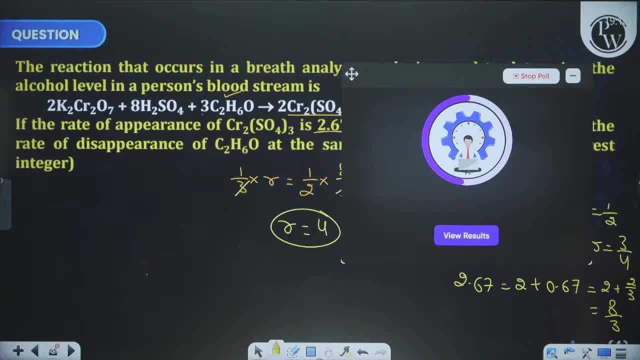 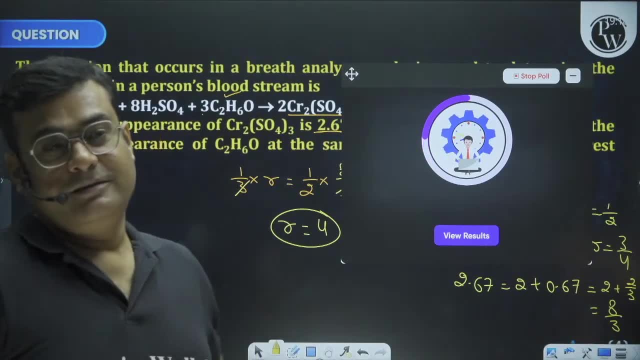 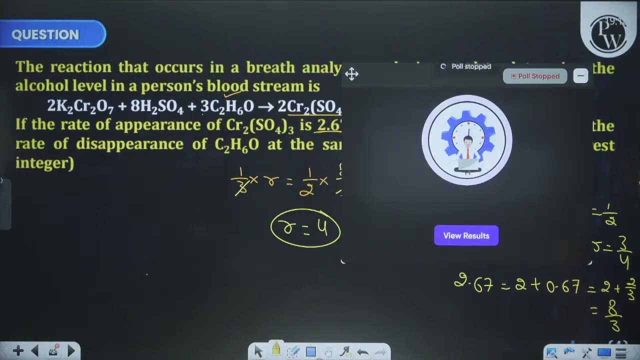 new, unique things. then if we take a session of 6 hours, then 40-50 things are absolutely new. we will learn and go He질, tell him, tell him, tell him talk. you can't bring yourself, but here I will. 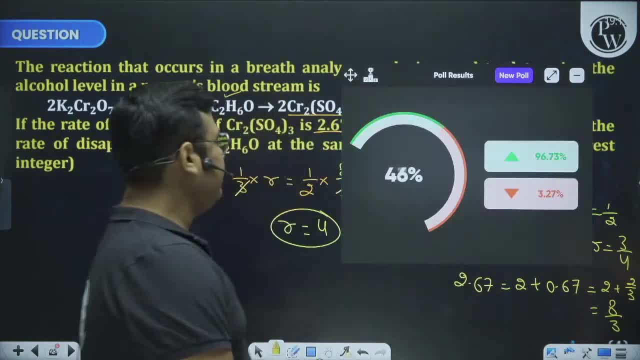 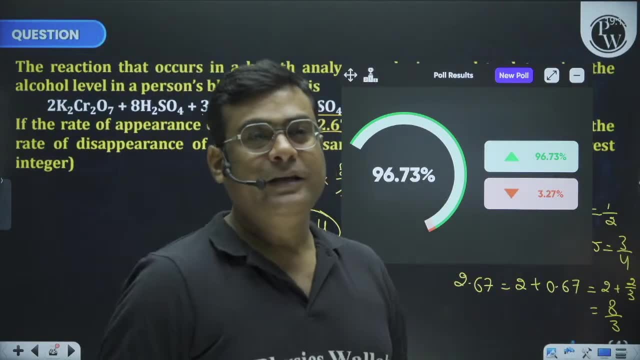 surely see the results by the way in the chat. yes, it has been completed. and well, here too it has been completed. 96.73 is considered to be 97. only means 3% of children are wrong. they said, no, we know more than 13,, so that's it. but at least 1-3% is possible then here. 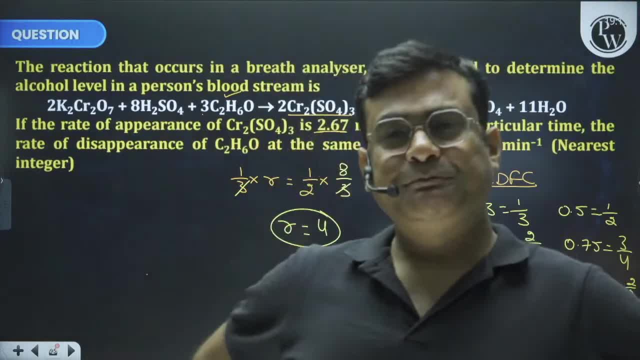 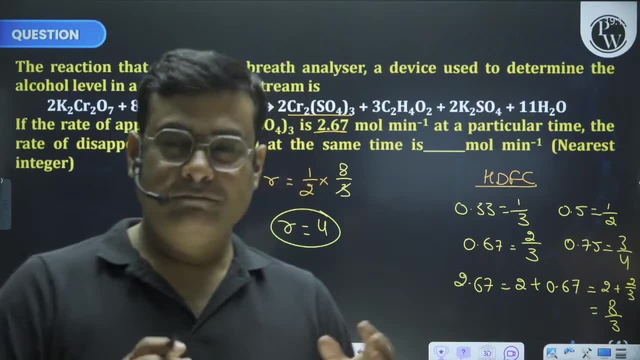 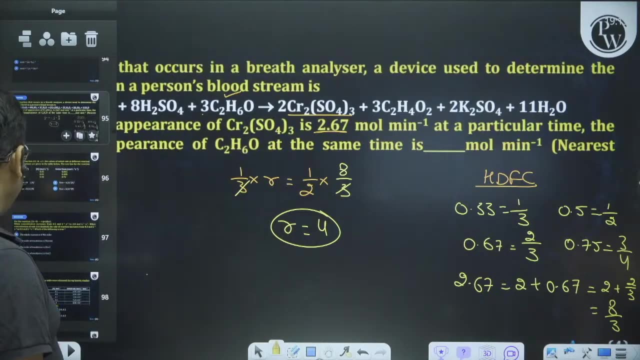 We have come to see you, then it is different. otherwise all the children are giving 97% together. that no, sir, we are learning a lot of things relatively, which you have promised. ok children now. I have told you so many formulas of the first order, son, let's go to the rate quickly. 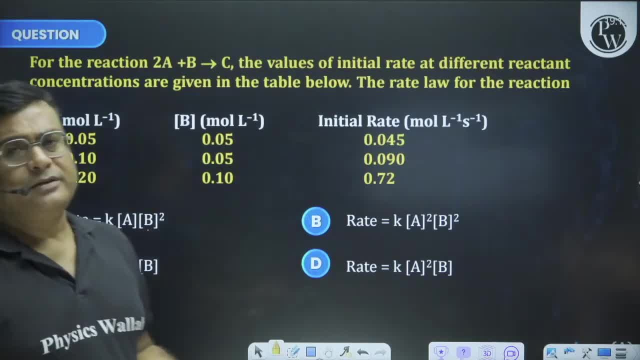 let me tell you one more question. our target is to get a question in the range of 20-25-15-25,. you will get an idea. see again after the decimal. it is the same place. 10 out of 5 means it has doubled. 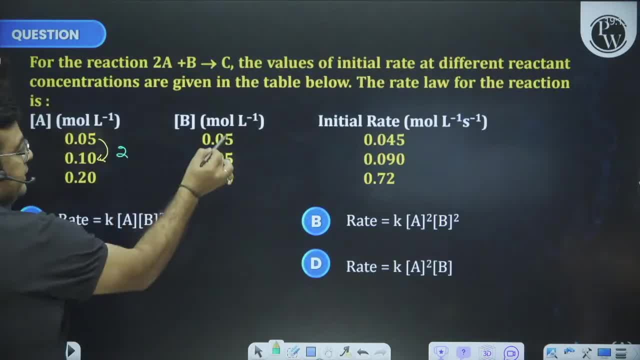 let me change the color of the marker. it has doubled. here no change: 45 to 90 has doubled. double means order 1, then the coefficient of A should be 1,. the coefficient of A is 1, there are two places. 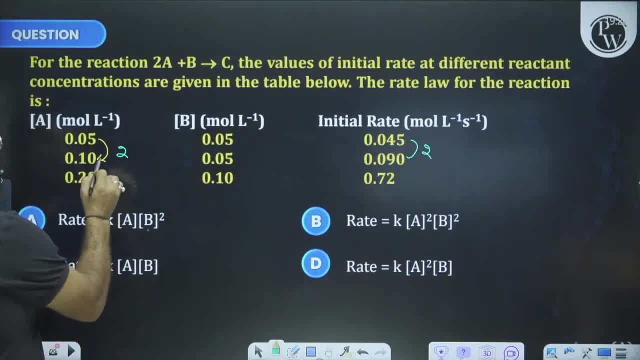 let's see the next one too. now what now see: 0.1 to 0.2 has doubled. 0.5 to 0.5 to 10 has doubled. now see here the decimal is twice. that is why I am teaching again and again after the decimal: keep the. 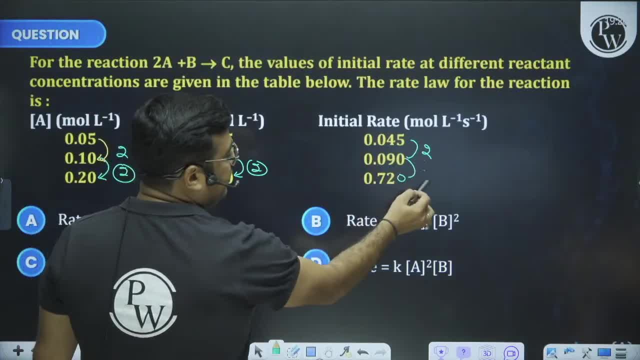 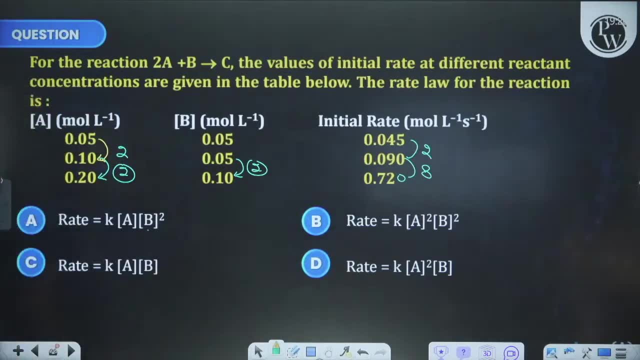 place same so that the decimal can be avoided. so how many times is it 9-720?? 8 times now, because of the 8 times, the 2 times have increased due to a. that means b has increased four times. so how much? the order in respect of B will be 2,. ok, the end. 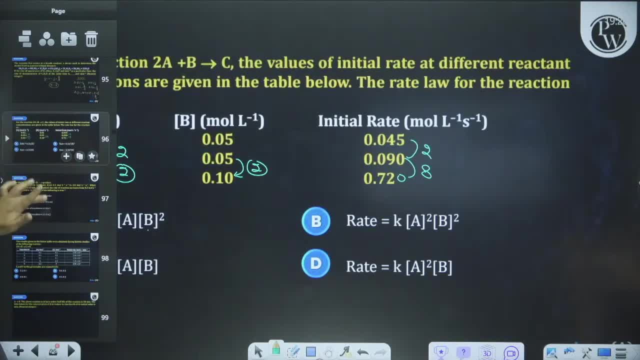 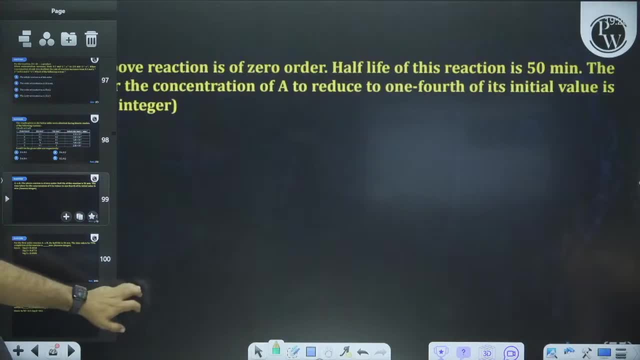 of the question has not yet been. son, if I still want, then I could have brought so many questions I brought. I am leaving something for you. like you have got the question of the initial rate back then shallow, he can a zero order copy question, but I do a to be our reaction. 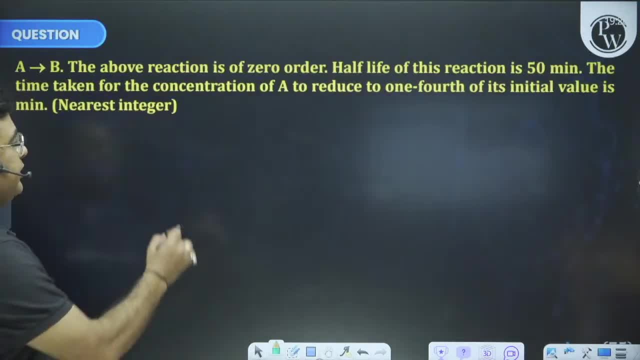 is of zero order. half-life of this reaction is 50 minute. matlab 50 should be equals to a naught by 2k. take a time taken for the concentration of a to reduce to one fourth of its initial value. agar, a patcha surprise to give one fourth of its initial value. matlab: pick a, kick a. 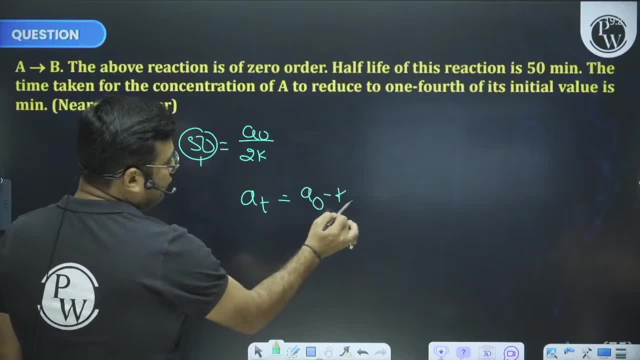 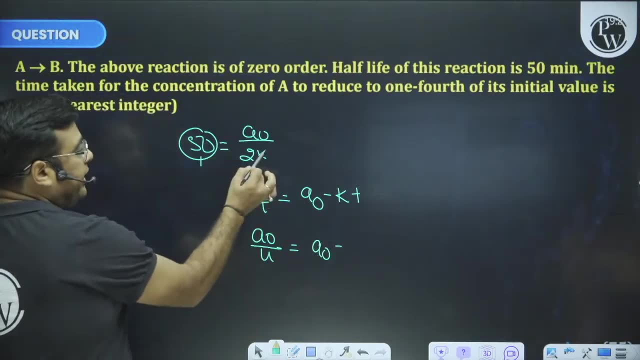 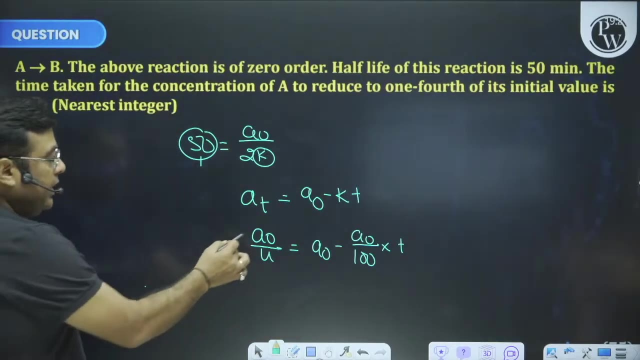 formula: lager 80. Bera huge a note minus Katie to one fourth on a Katika we gotta cohort adenward by for a Nort minus Kica character. gay sir, a naught by 100 in tutti bus international question la hier singing or Natalia one. 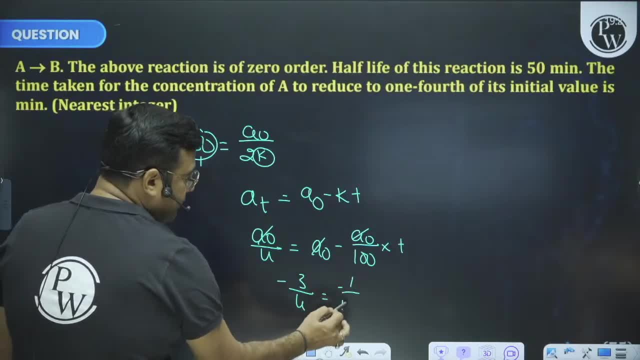 minus 1 by 4, minus C by 4 is minus. you will see, because that's a question only. the question is an article by the 4th is minus 3 times 2 by 4 and you will see a button: 10 times plus 1 minus 1. 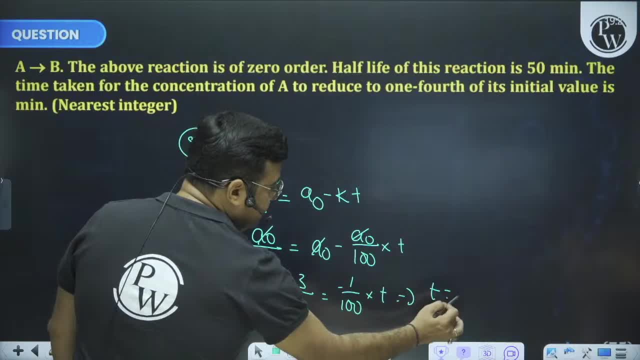 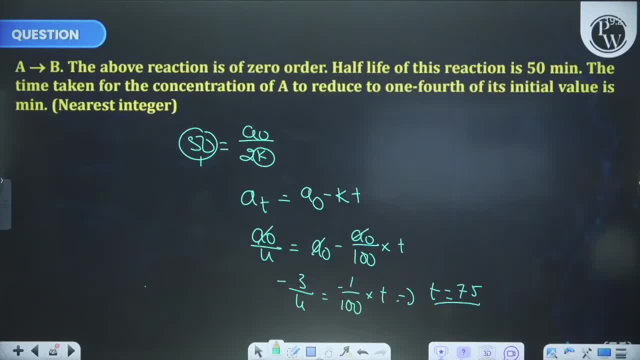 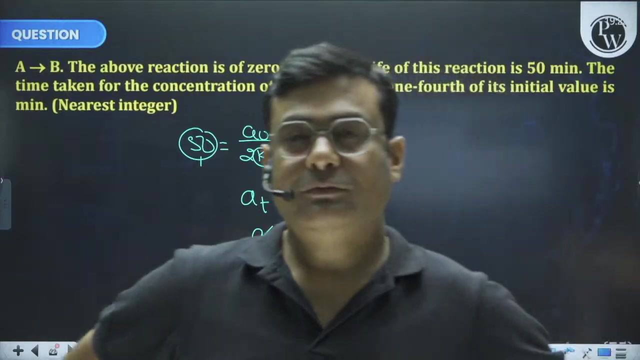 Now, some of these questions are these, some are mine, Son, some children are writing again and again. sir, why do you have to do PYQ? Okay, for your information, let me tell you that almost 70% PYQ is there. if I would have written here the year too. 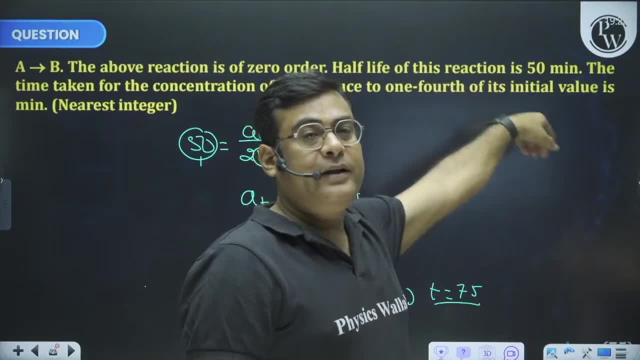 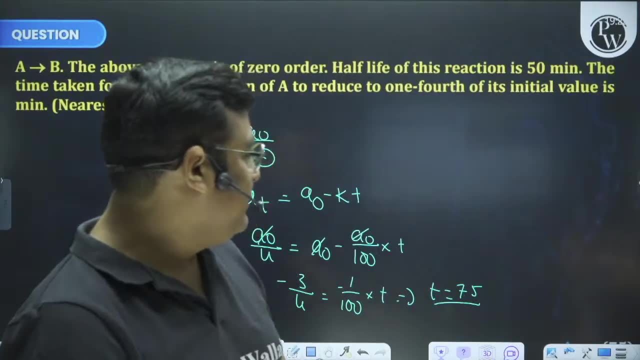 JEE Mains 20, 2019, February attempt and whatever this is. then you would have opened the book and started shouting the answers like this: In the beginning you could see the answers. no one was solving. you see, at least the answer is not visible. some children are solving. 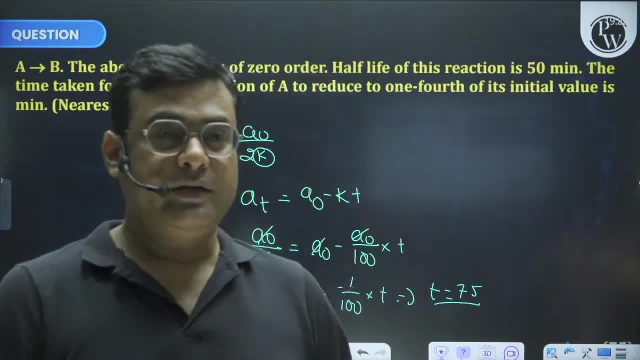 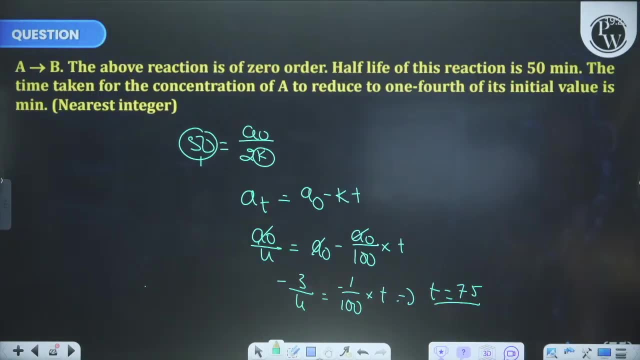 so this session is also for children, sincere children, right? The children who are not sincere, see, no one can do anything for them, son, no one can do anything for them. This is for sincere children who really want to learn something. who really want to learn something, right? 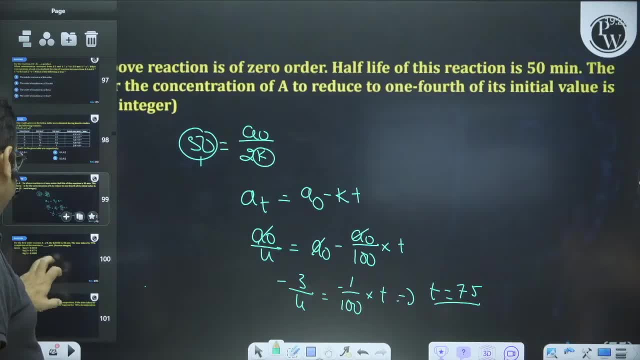 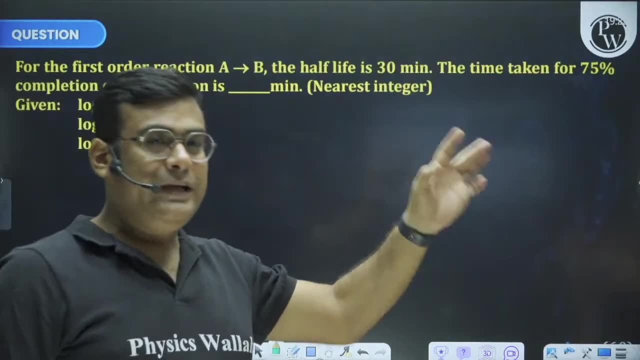 And they must be getting things in their understanding. now I come to the shortcuts of my first order. these are all questions of JEE. let me tell you clearly: I have removed the year game. maximum question is of JEE. I have removed the year see. 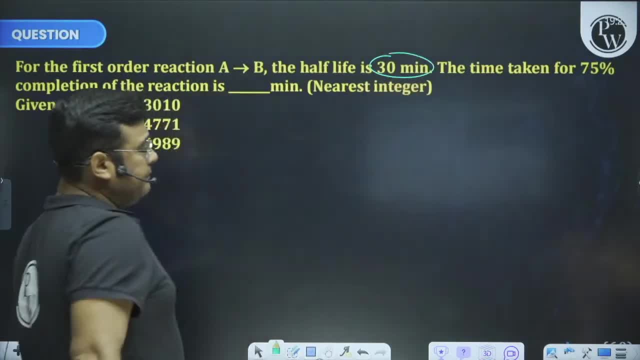 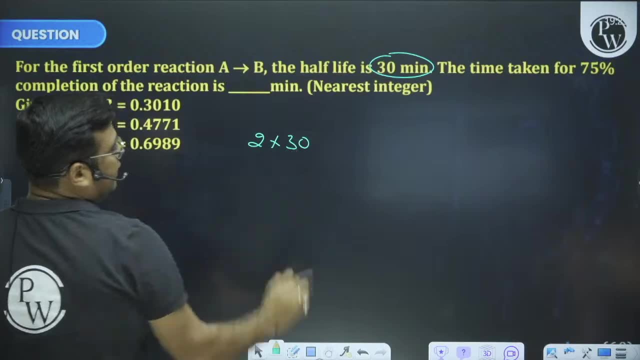 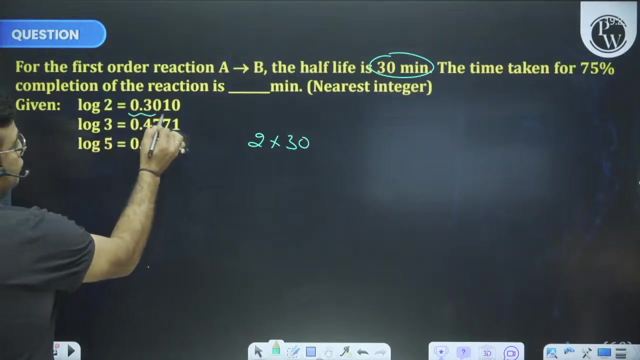 for a first order. reaction A to B: half life is 30 minutes. I am telling you time taken for 75% completion. now I said 75% time is 2 t half. the answer is directly 60,. now he has given log 2 too. and now I said some child was getting angry. 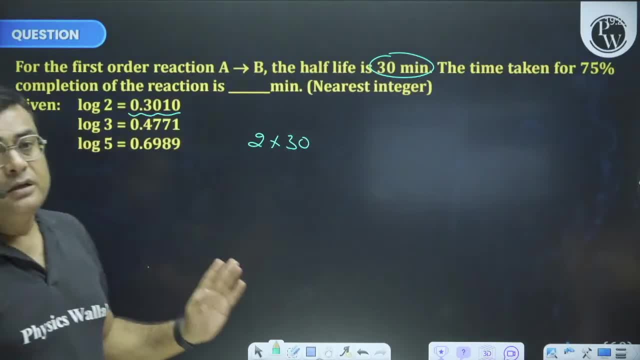 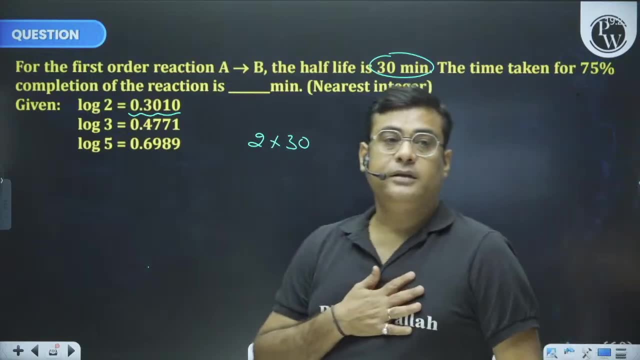 sir, you gave a very bad explanation. I did not give any bad explanation. son, from the law of log 2, JEE should also be given 0.3,. if he is not giving it by writing then it is not my fault, because the actual value of log 2 is 0.3010,. 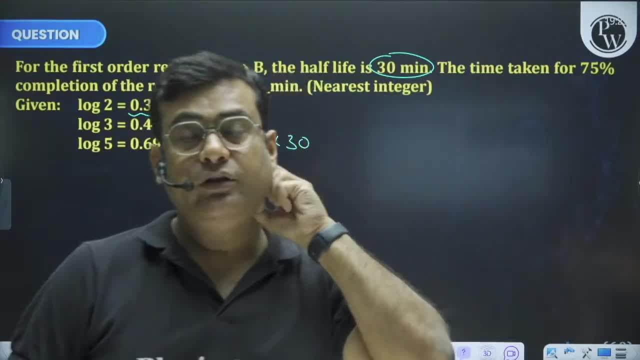 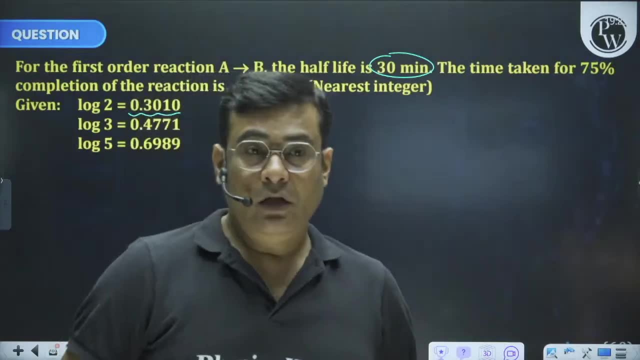 and in that entry question neither he wrote 0.3, nor wrote 0.3010,. so I cannot do anything. see the thing where it is wrong. son, I have no shame in saying it wrong. if I also make a mistake then I will hide it. 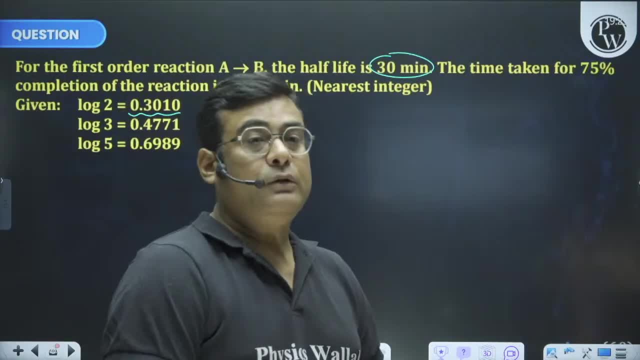 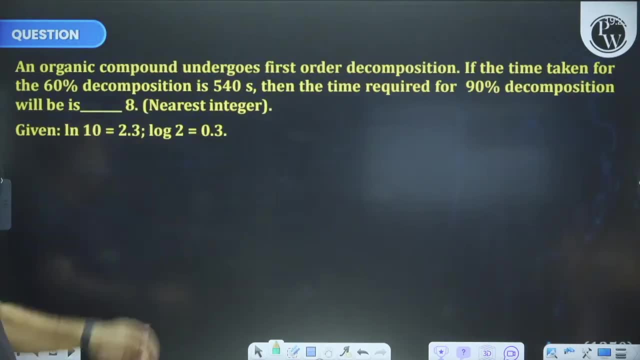 it is the biggest thing to admit the mistake, brother, but it was necessary to give its explanation, then the story is over. okay, see the next question. an organic compound undergoes first order economy if time taken for 60% decomposition is 540 seconds. now t 60%. I have just written how much. 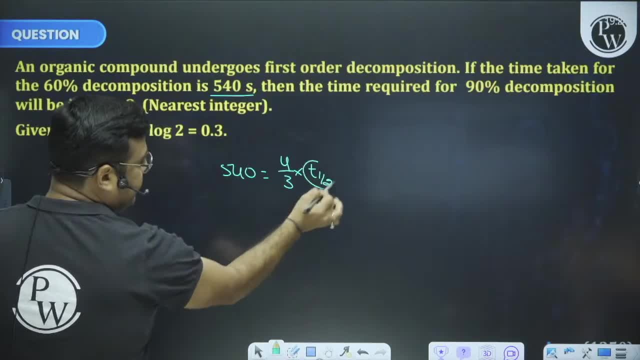 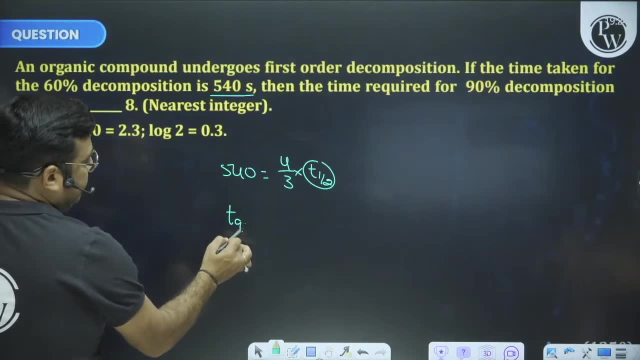 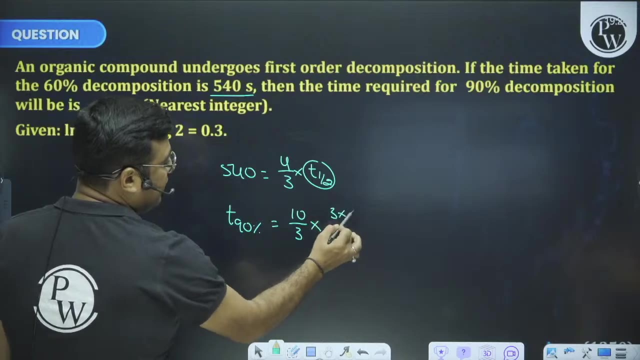 sir, 4 by 3 of t half from here. t half will come from here, t half will come then. time required for 90% completion. now what was written for 90%, sir? 10 by 3 of t half, so 10 by 3, and how much t half came from here? do not waste your time by solving now. 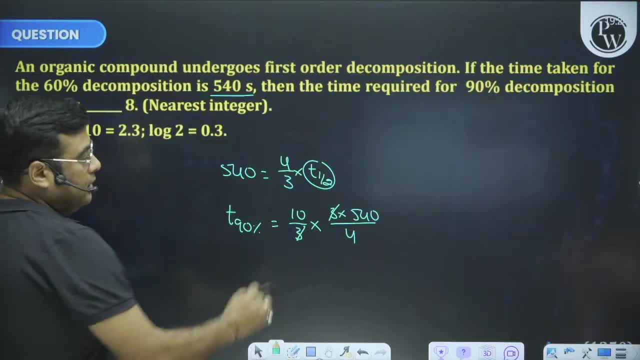 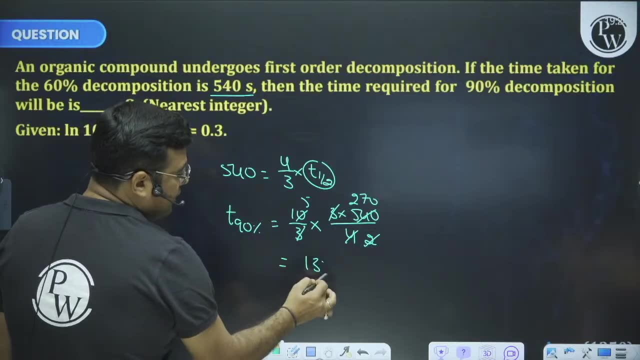 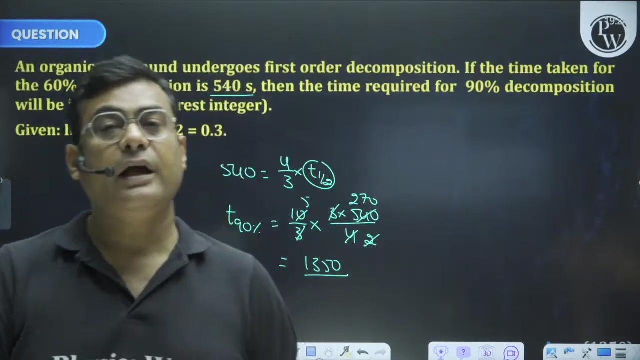 see it is cancelled. see it is 5,. it is 2,. see it is 270, and 270 is 5 times. you can also do it. see the answer is done if you want to do it with the method of normal first order. if you want to do it with the method of normal first order, then what will you have to do? 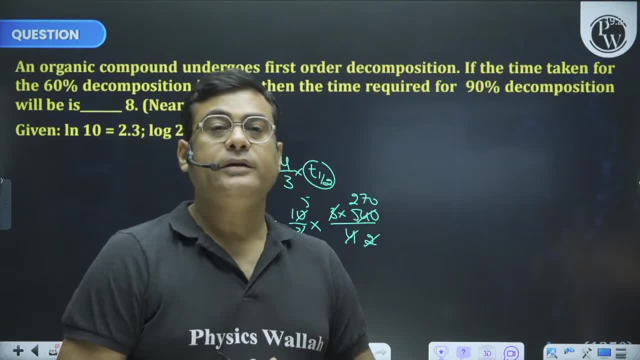 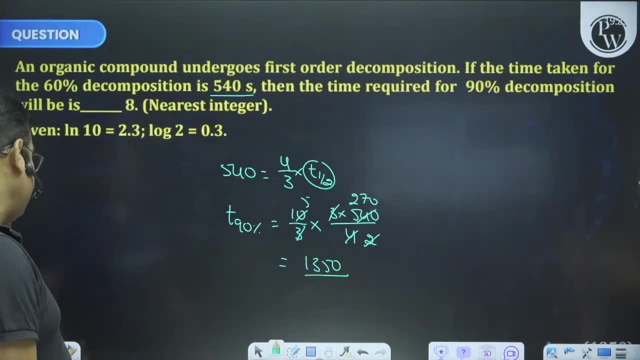 then first you have to do it with k equal to 1 by t, ie anode by 80, then you will have to use the formula twice. once you have to get the value of k first, then you will have to use it again. 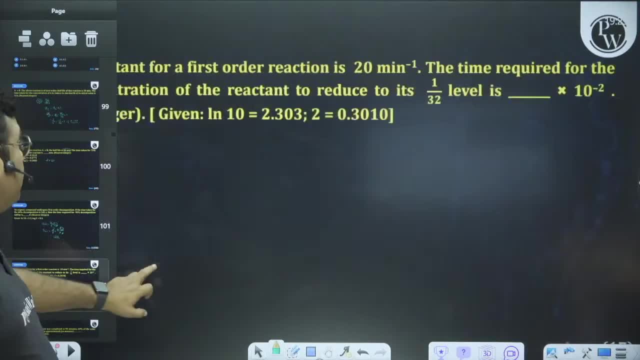 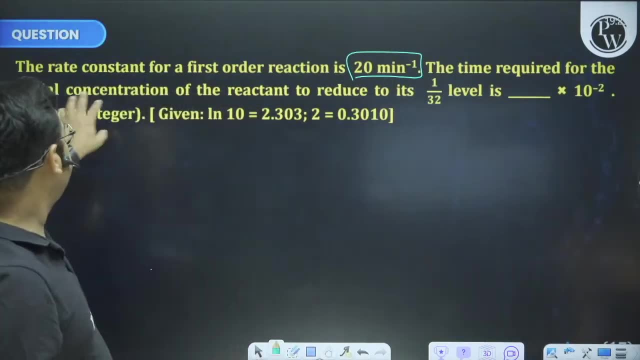 is there any other question like this? as far as I remember, there are more see rate constant for a first order reaction is 20 minutes. inverse ok time required for the initial concentration of the reactant to reduce 1 by 32 level. 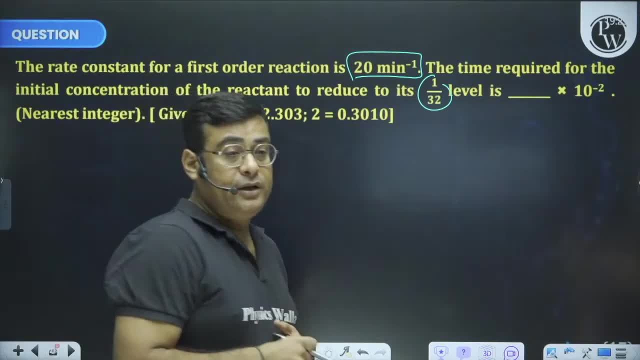 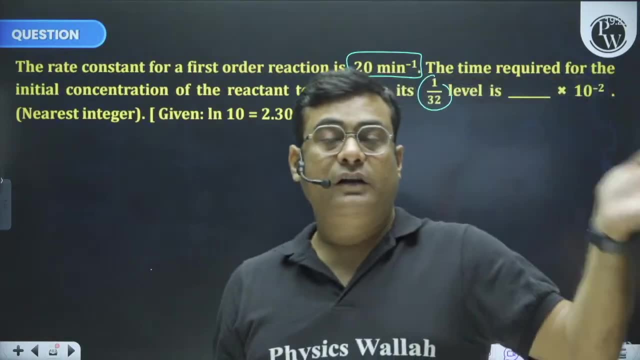 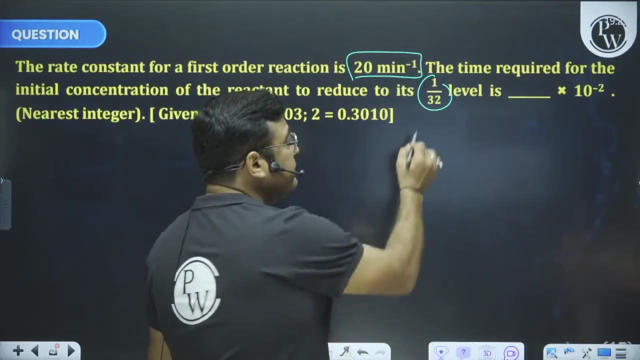 now, brother, you must be knowing what is the unique property of the first order reaction. their concentration is always half. it is the same, ie the first time 1 by 2 happened in the next t half: 1 by 4,, 1 by 8,, 1 by 16,, 1 by 32, and in this way, 32 means how much is the power of 2, 5,? 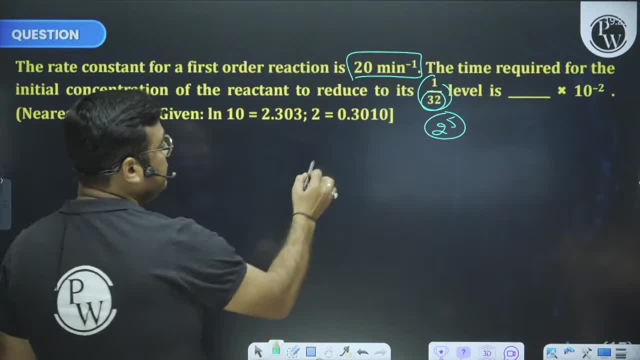 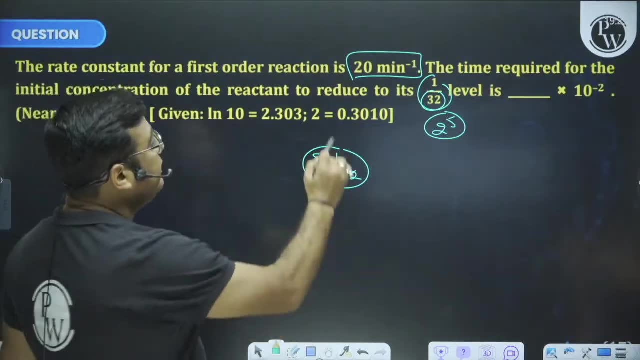 means this process is done in how many t half, sir? in 5 t half. isn't it in 5 t half, not 100,? son, it is wrong. he gave the value of k. this is the value of k: 20 minute inverse. 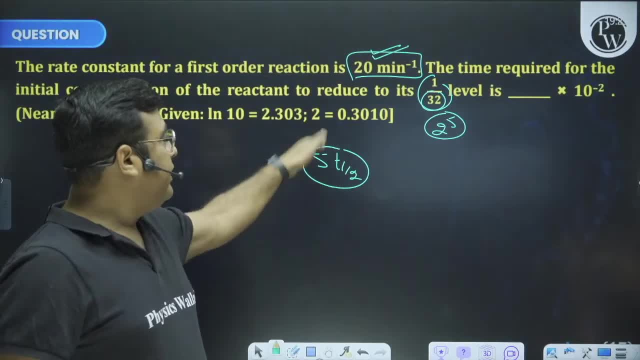 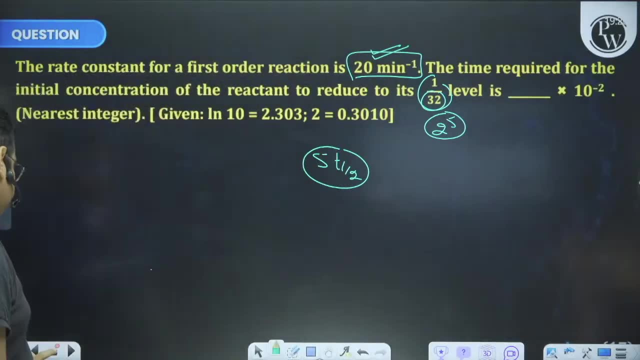 not the value of t half, isn't it not the value of t half? is it 5 minute inverse? if you do 5 into 20, you will do 100, you will have to take out t half. that's all I want to say, isn't it? you will have to take out t half here. 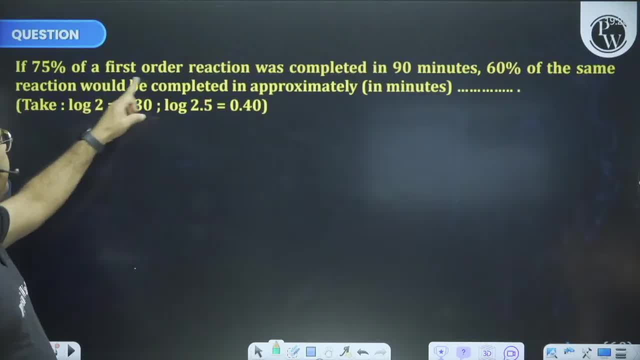 is there any other question? yes, according to me there is more. 75% of the first order reaction was completed in 90 minutes. now what was the time of 75% children? 2 t half means 2 t half's value is 90 minutes, so t half happened 45 minutes, isn't it? 60% of the same reaction would be completed in approximately 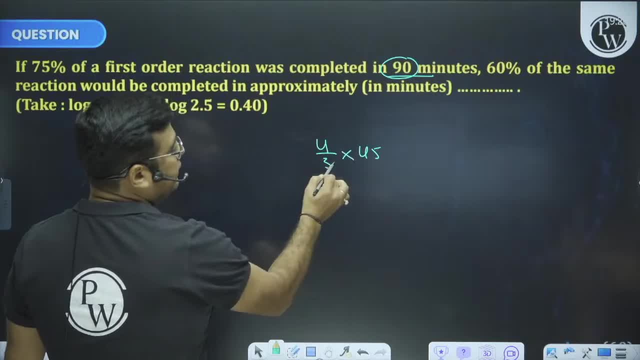 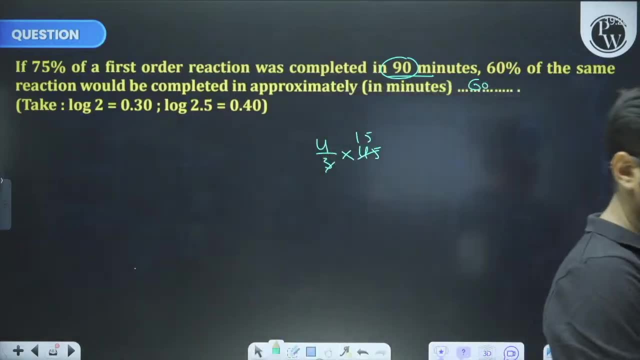 brother. what was the time of 60%, sir? 4 by 3 of t half, this became 15, 15 divided by 60, I had just said to you, son, isn't it what I had said? that if you remember these times properly, then your time is going to change, isn't it? a child is demanding. say op for j s sir in the chat. 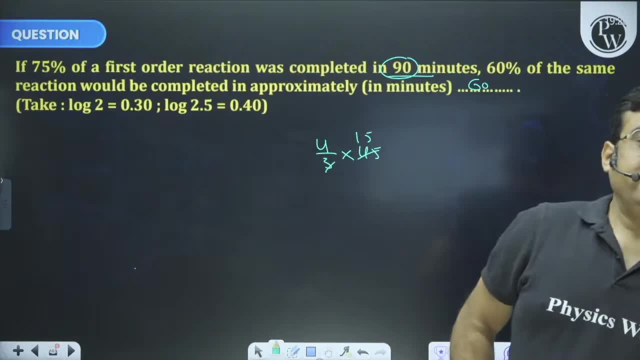 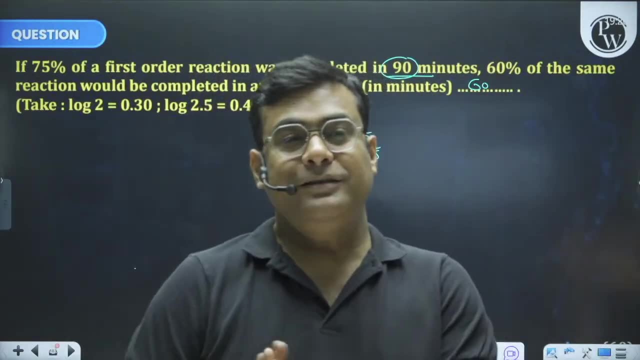 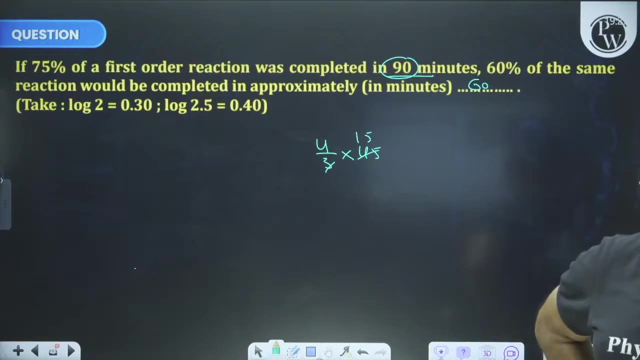 come on, say it once. we will also get excited a little if it seems that, yes, this is, isn't it so far? we are in everything in all these questions. I'm also saying in the YouTube on my phone. 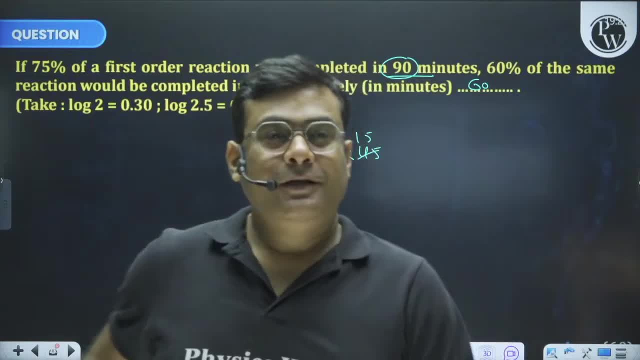 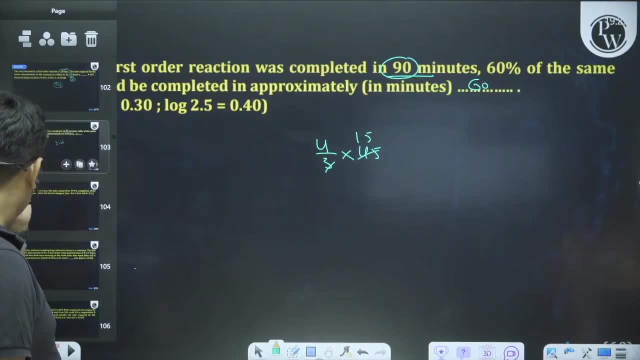 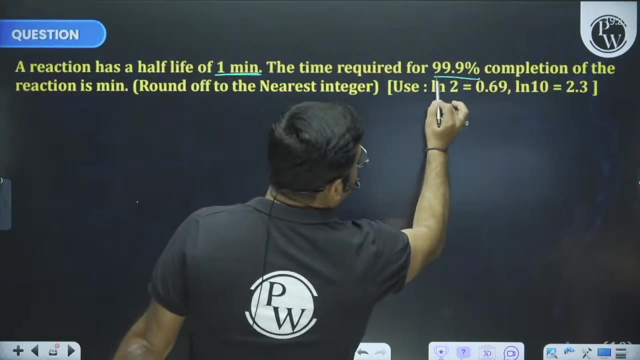 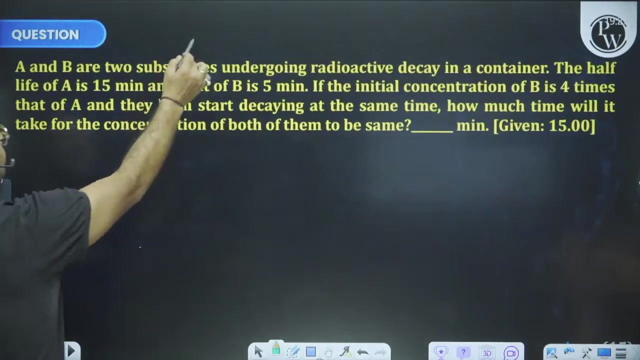 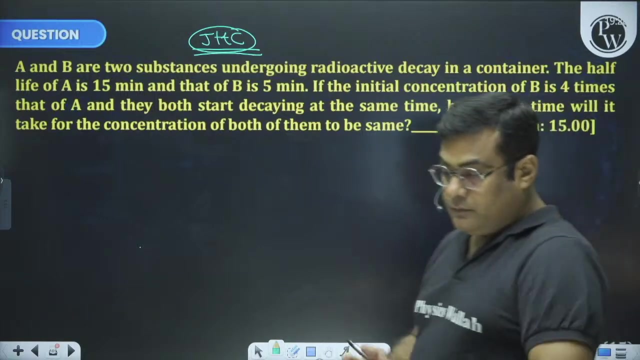 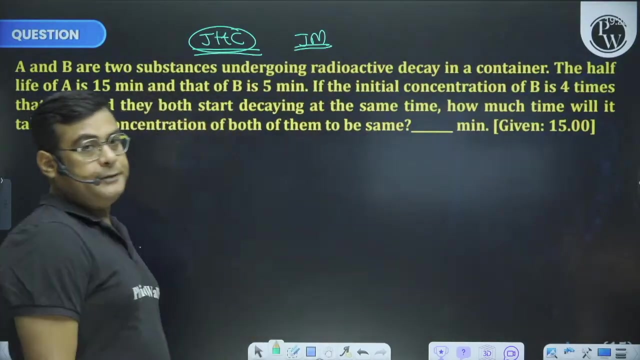 I'm also saying in the YouTube on my phone. I'm also saying in the YouTube on my phone: Answered the question again. will repeat again and again in JEMains. Answered the question again. will repeat again and again in JEMains. 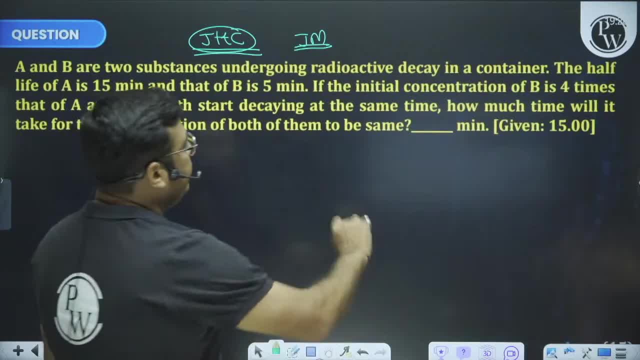 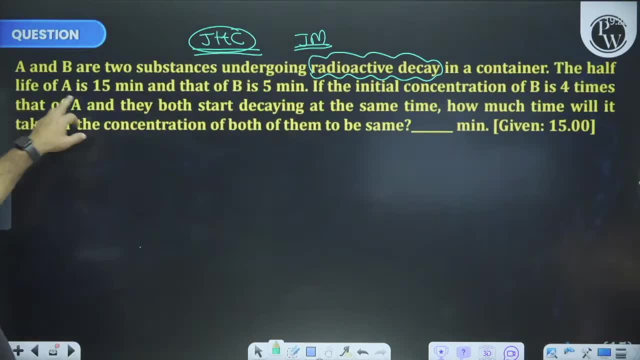 Answered the question again. will repeat again and again in JEMains. Everyone knows that Directclub punishment- also cuts- is 15 minutes. One is 15 minutes of a half-life of b is 15 minutes of b's. all of where b is 15 minutes, all of where b is equal to each other. 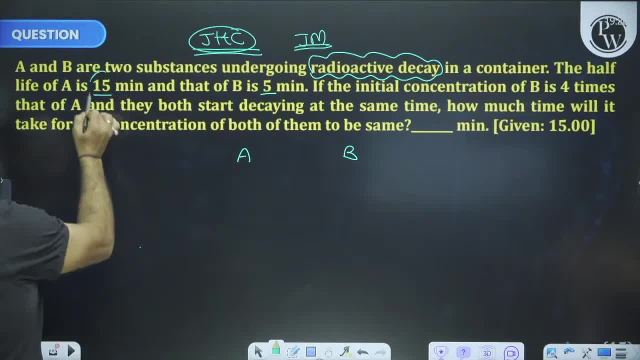 Ok, JSC, they are always normally present in multiples. now, if initial concentration of B is 4 times of A means if it has X, then it has 4X. it has given the condition and they both start decaying at the same time. both are starting to decay at the same time. how much time will? 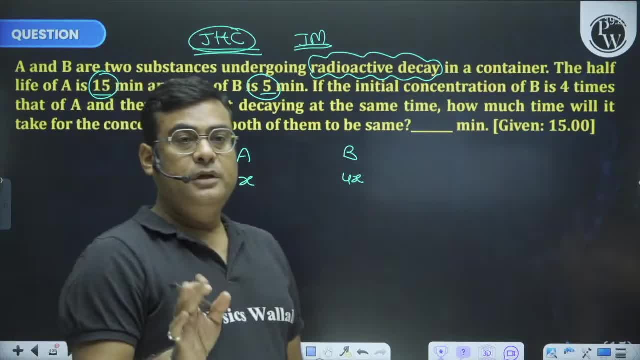 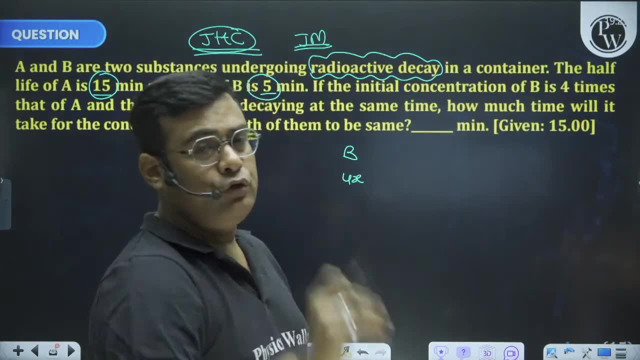 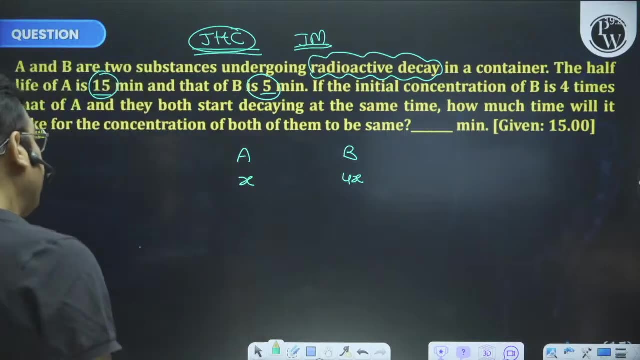 it take for concentration of both to be same. then first listen to my JSC because some children can get to see this question in these 10 papers. because he has not asked this in the January attempt, now ask in the April attempt that any question of this kind that 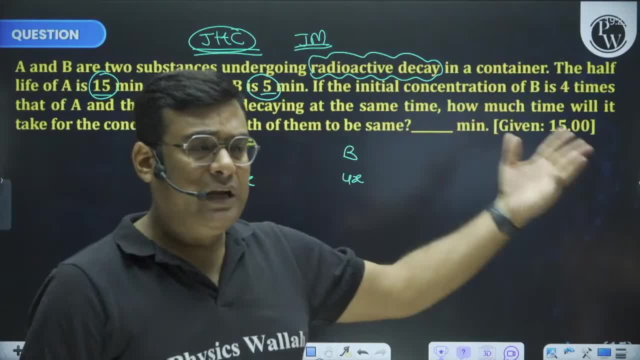 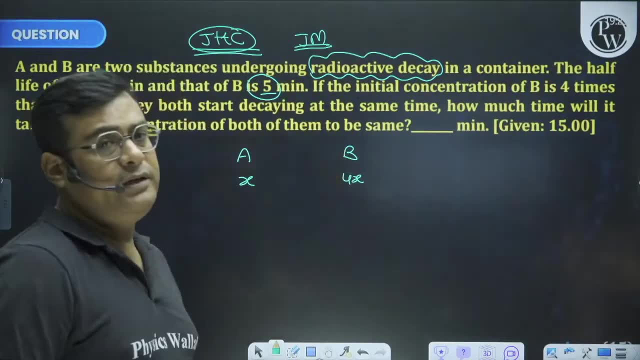 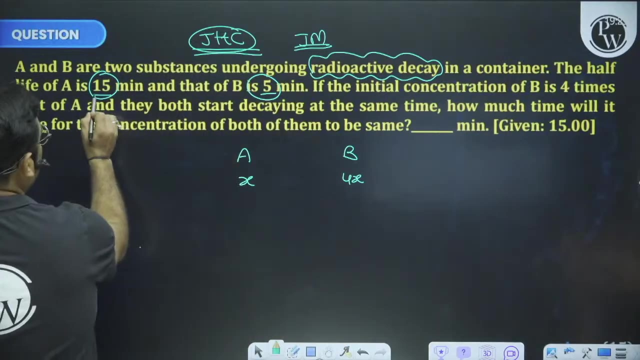 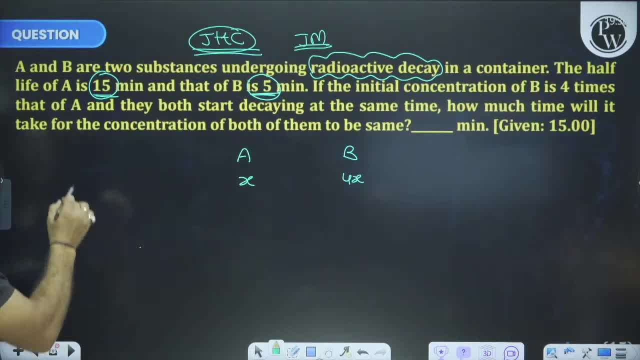 order, then if you can solve the problem, then the answer will be in your hand, that there will be a good answer. then it will be a good answer, then you will know that the answer will be good. and you will know the answer will be good because it depends upon: 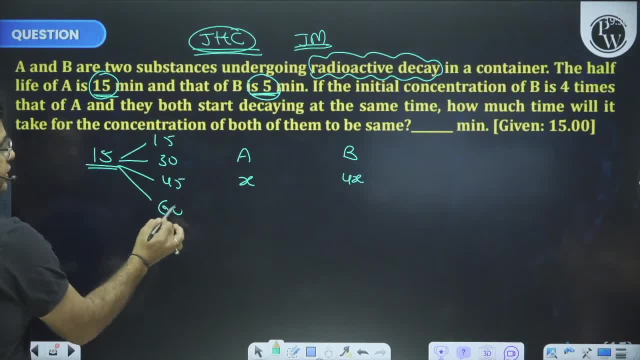 the LCM of X and Y. how much LCM of X and Y is 15?? then our answer: in the multiples of 15, either 15 will be, or 30 will be, or 45 will be, or 60 will be, and so on this first lesson keep my attention immediately. any question of. 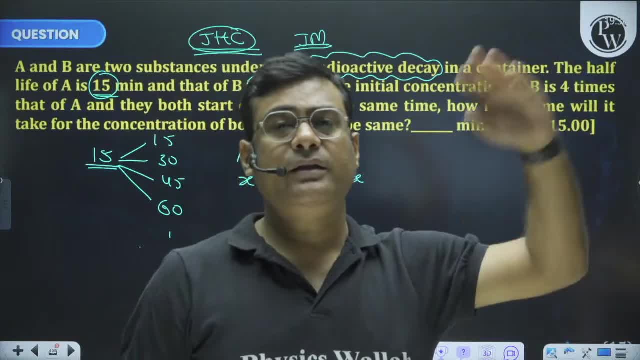 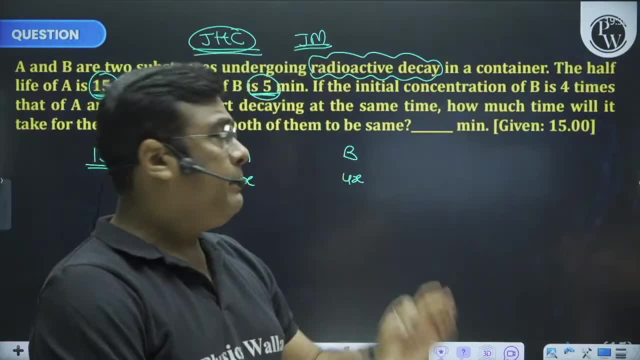 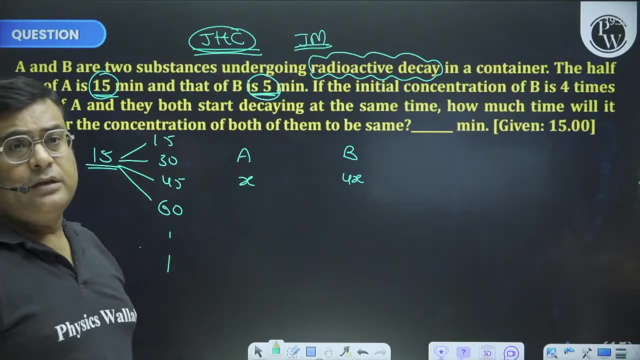 this kind comes. it has come, it will come even further in these give any condition. My first logic is that it will always come in the multiples of T1, T2, T3, T4, T5, T6, T7, T8, T9, T10, T11, T12, T13, T14,, T15,, T16, T17,, T18, T19,, T20,, T21, T22, T23,, T24, T25,. T26, T27,, T28,, T29,, T30,, T31,, T32,, T33,, T34,, T35,, T36,, T37,, T38,, T39,, T40,, T41,, T42,, T44,, T45,. 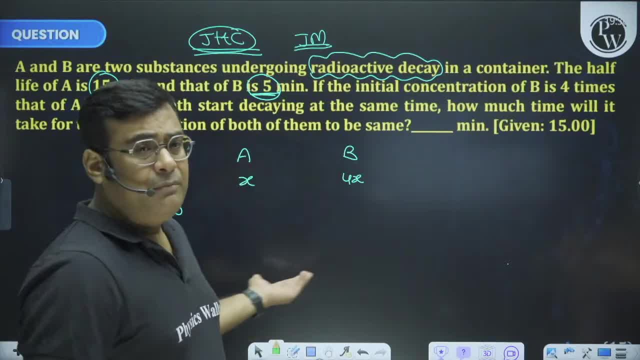 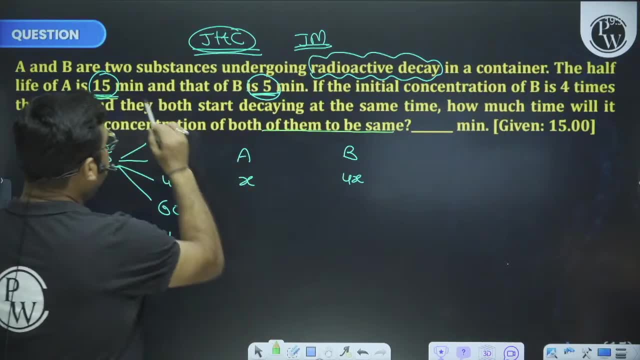 T45,, T16,, T28, T. It shows that it is a. it'll be a half way there. So, as both is looking at how long it is longer than the solution, but because solution is that is how longer it is. 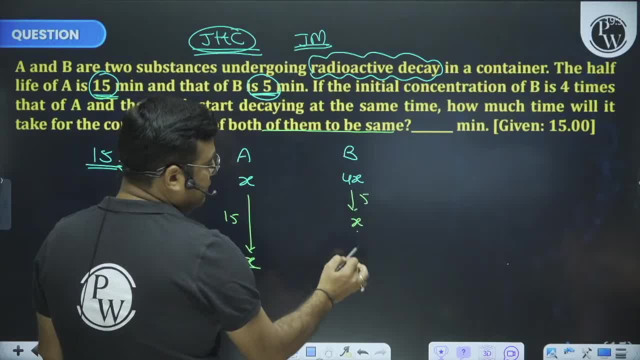 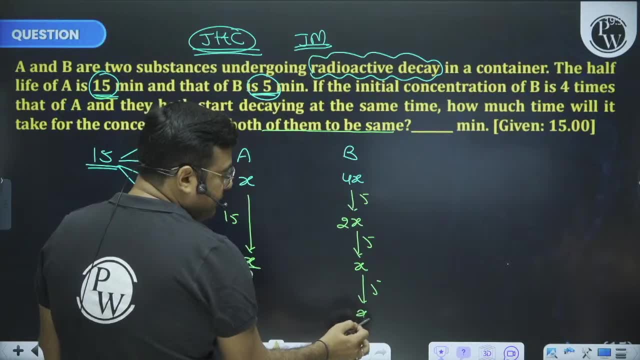 We'll do it morally, son. look what is the condition of one and half lifetime. how much time the concentration of both is to be same. One is 15, it goes directly after 15 minutes. cut xilty. see after وبعة xty. 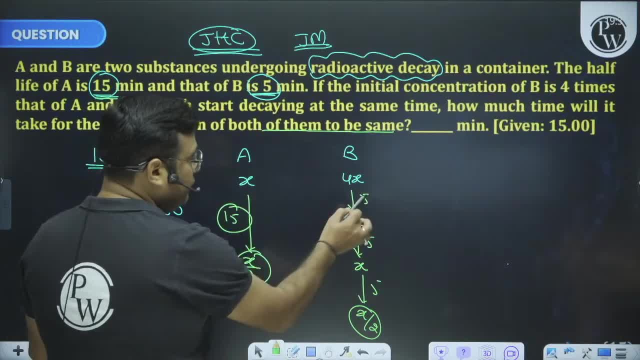 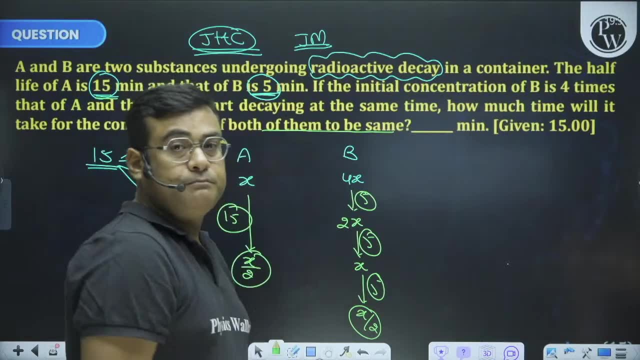 This happens after the first 5 minutes. The second half is x. the second half is x. after the next five minutes And the next half is x20. establish to be worse than you: ically, are balanced dog eyes in settlement of normal. take out, Sir, this was done in 2015,. this was also done in 5, 5, 10 and 5, 5, 15,. this was also done in 5, 5, 5, 15,. the story is over. 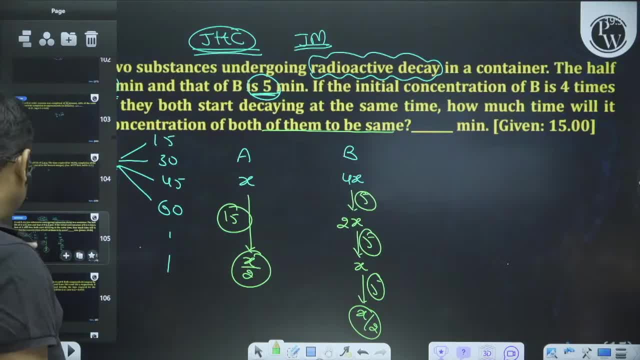 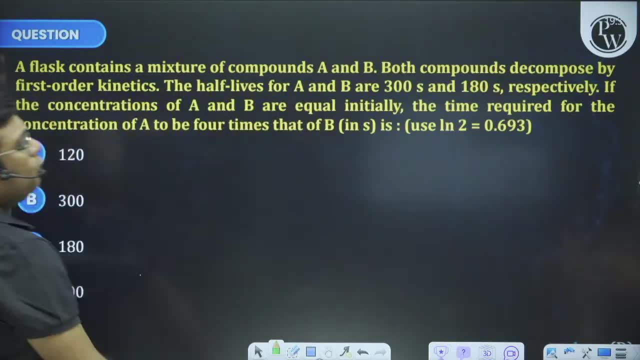 Tell me, did you understand the logic? And again, in my support, there is one more question. See, they have also given the answer in this. A flask contains a mixture of compounds A and B. Both compounds decompose by first order kinetics. 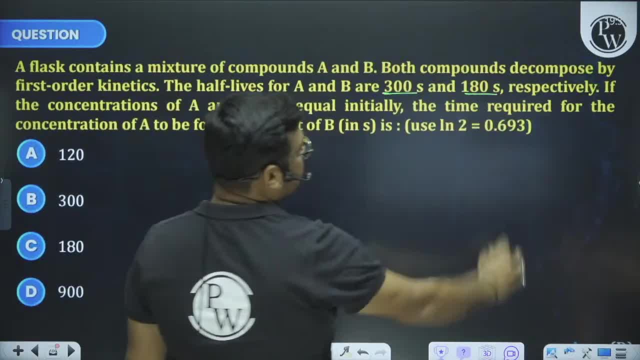 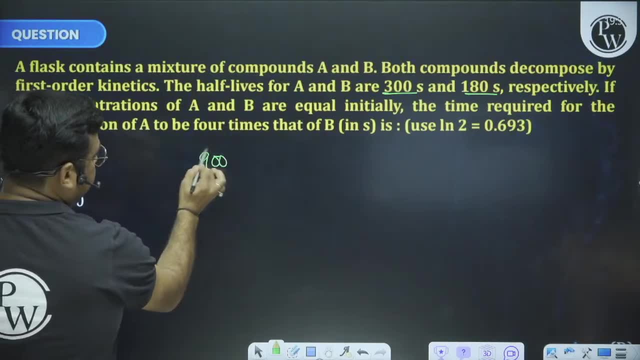 Half-life for A and B are 300 and 180.. If you know how much will be the LCM of 300 and 180? 900.. Right, How much will be the LCM of 300 and 180? 900.. 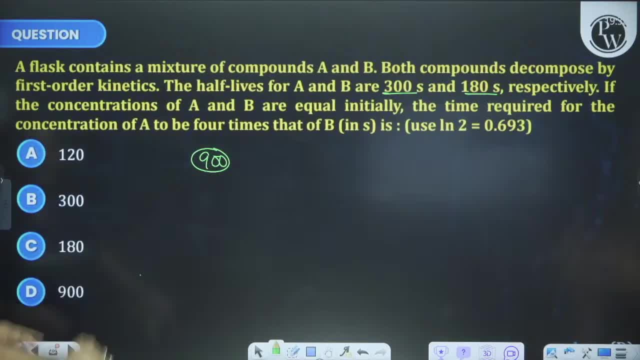 The answer should come in the multiples of 900.. If the concentration of A and B are equal, initially, time required for the concentration of A to be 4 times that of B. whatever the condition in the multiples of 900, the answer will be D. 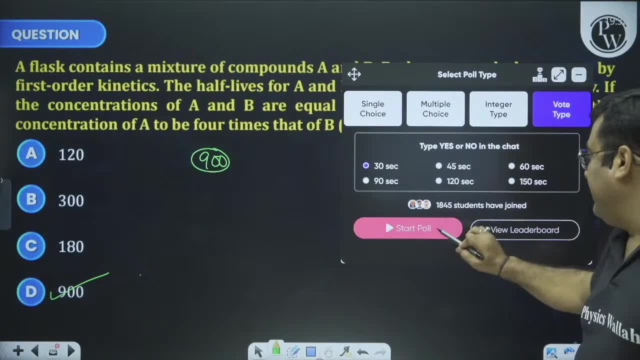 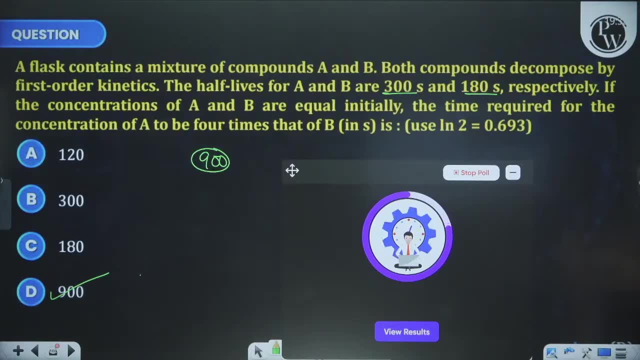 Right, I know that I am not going to get 100 percent, Tell me, But my wish will surely come to my heart that no one will know this trick. Do I have a 100 percent right on this? Tell me. Do we have a 100 percent right on this? 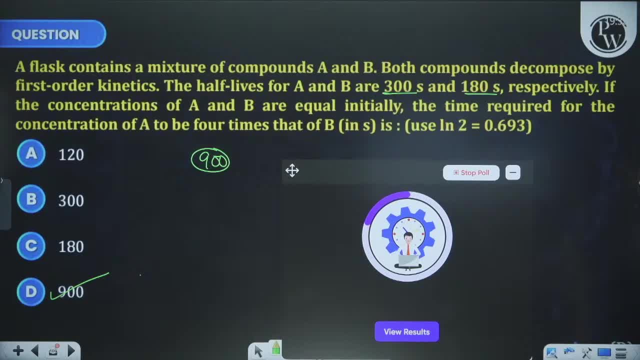 Sir, this is amazing. Does this also happen? And this is also a question of JEE? You can see that This is also a question of JEE. You can see that This is also a question of JEE. You can see that. 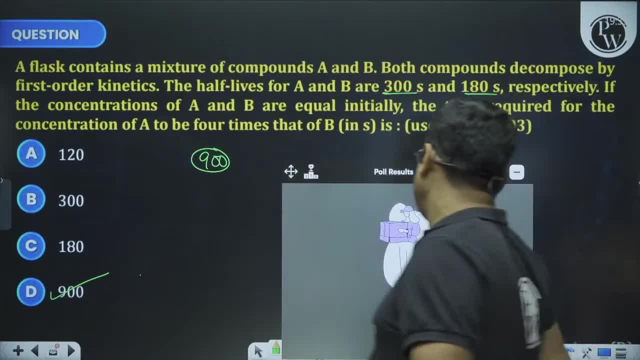 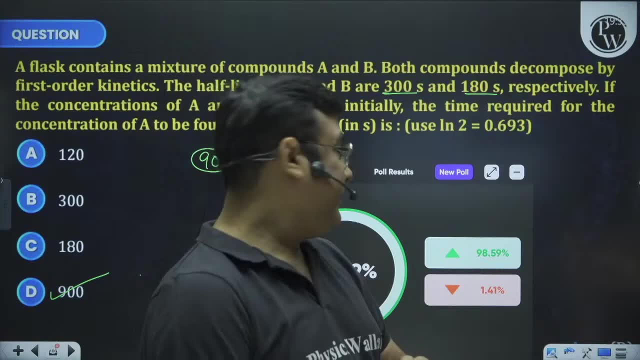 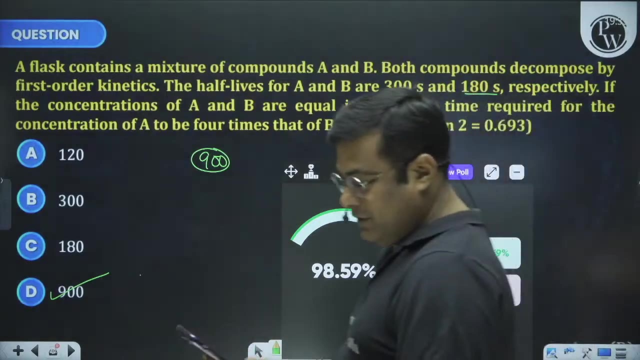 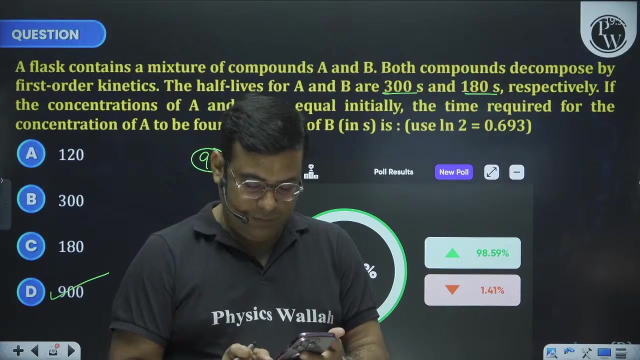 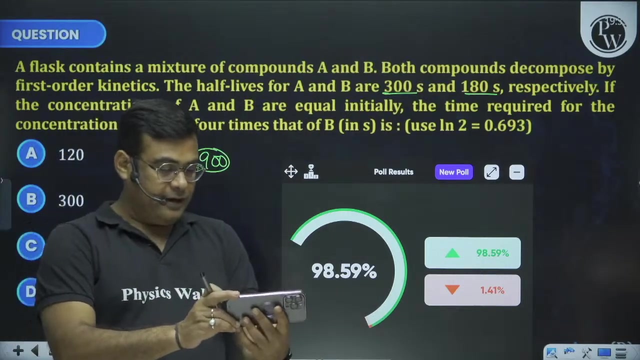 It's done. The poll is over. What does the world say? You slipped a little bit, sir. You slipped a little bit. It is 98.59%. I don't know how to take a selfie like this, but a 98.59 is made. why is it looking upside? 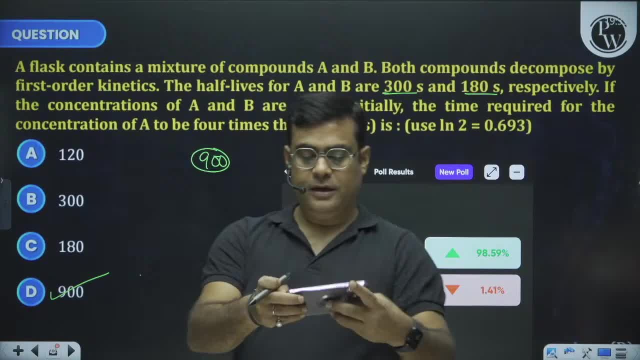 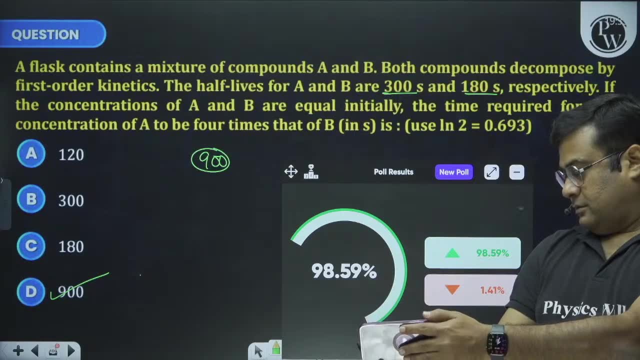 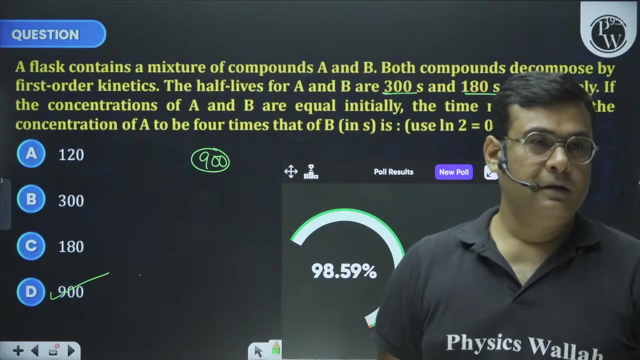 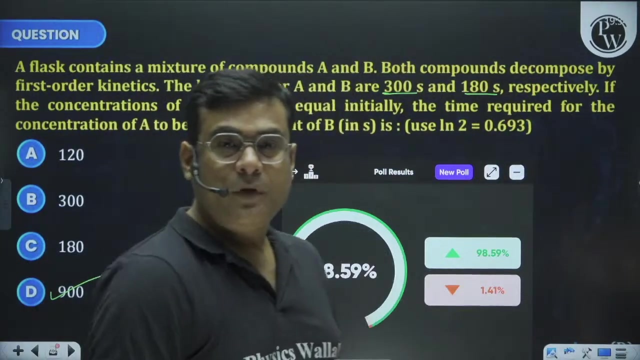 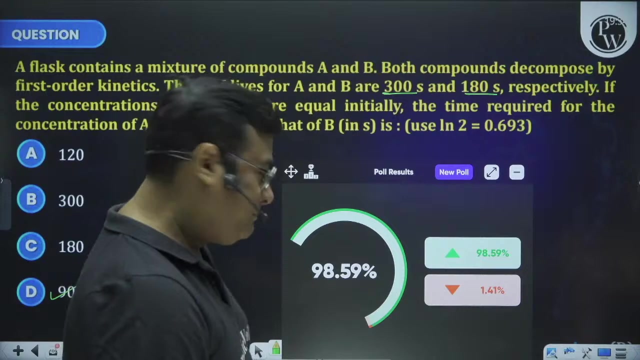 down. It will come upside down. this will make more trouble. Thank you very much. thank you very much. what has happened? what has happened? I mean the timer, Thank you. thank you very much, children, but try to put one or two hundred. 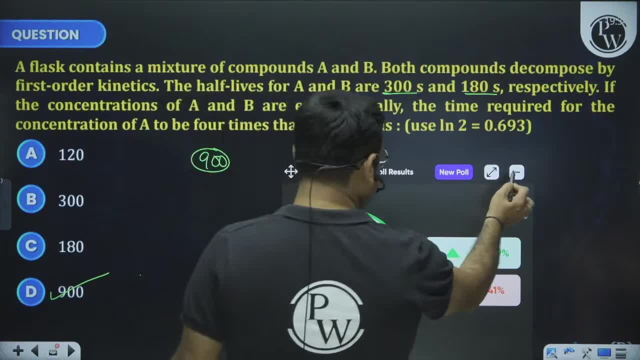 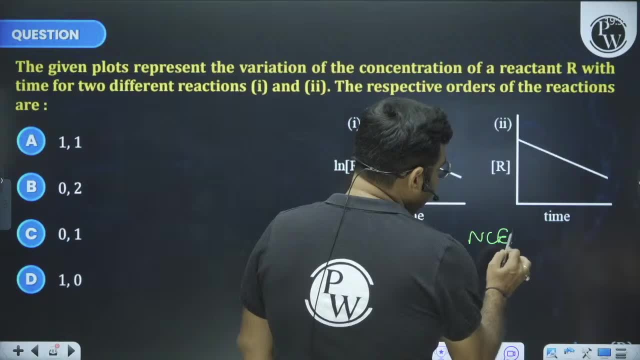 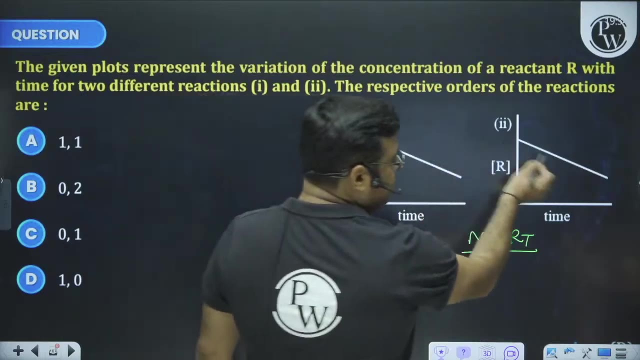 Now see, this is a question of children. the answer is directly a graphical question of NCERT. If the concentration of reactant versus time graph is of a straight line, then the reaction is of zero order. If the concentration of reactant versus time graph is of a straight line, then the reaction 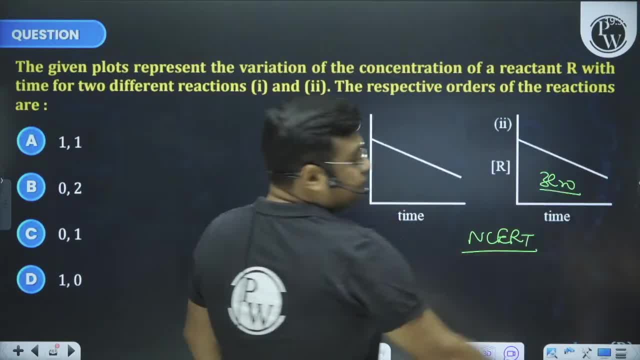 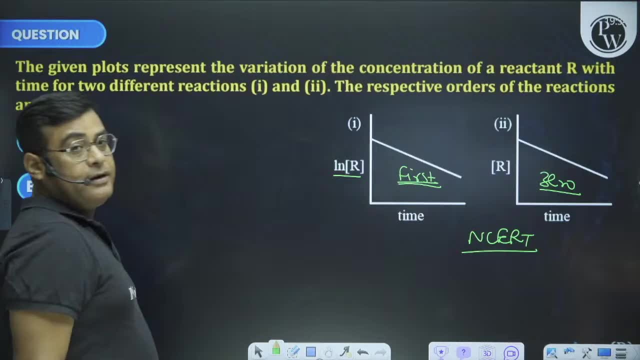 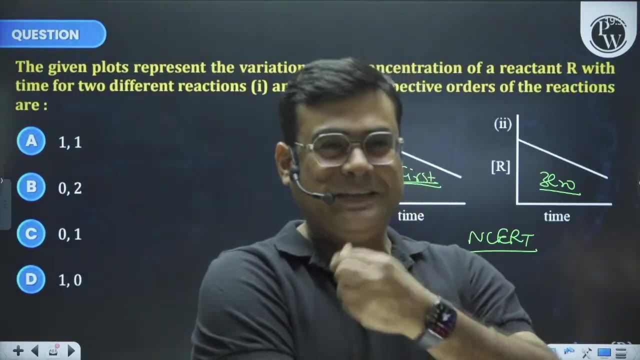 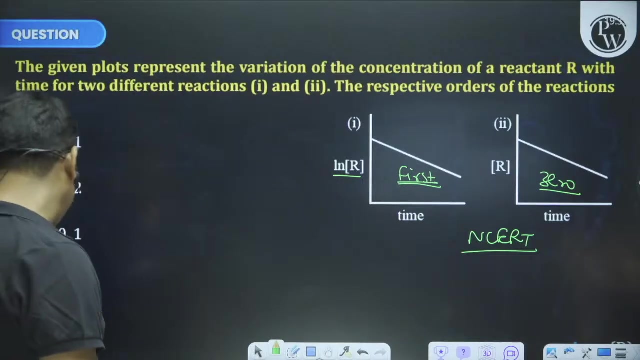 is of zero order. But if the concentration of reactant versus time graph is of a straight line, then the reaction is of first order. Remember my brothers, everyone. the way of showing an iPhone is a bit casual. what a thing. you have won my heart, son. if you were here I would have given you a party. 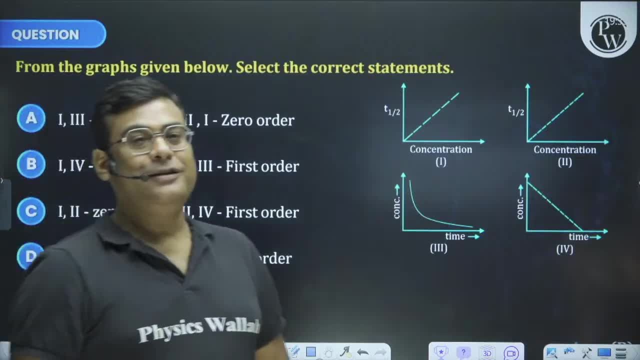 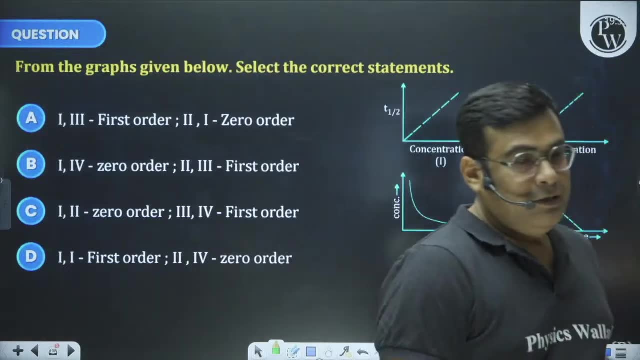 right. If you were here I would have given you a party. Our children have become so fast these days I don't know where we have been, in which world we have been. Thank you very much. If there was a way to show the iPhone, then people in PW as soon as they start the class. 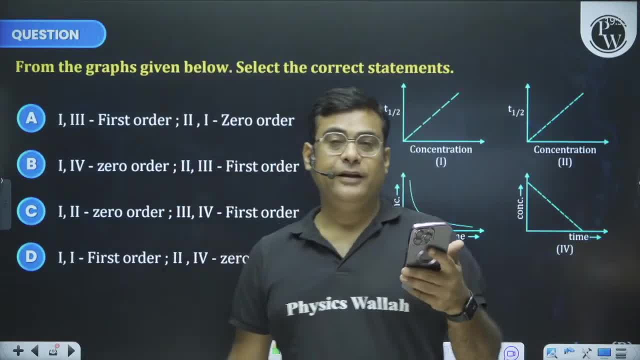 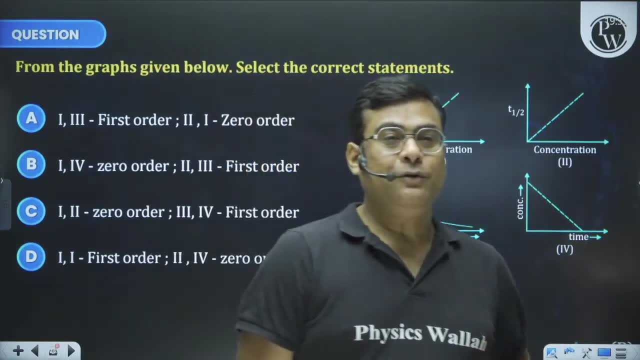 they take the mobile in their hand from the beginning and see it. Normally- I am talking about 99% teacher, I can say 90%- they start here in the beginning and hold it in their hand like this. I got a good thing, so I said: okay, this photo is made. 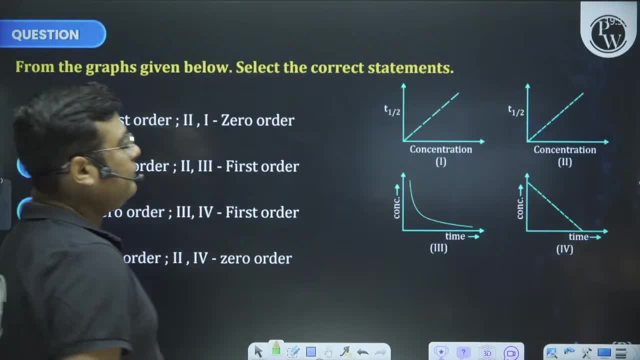 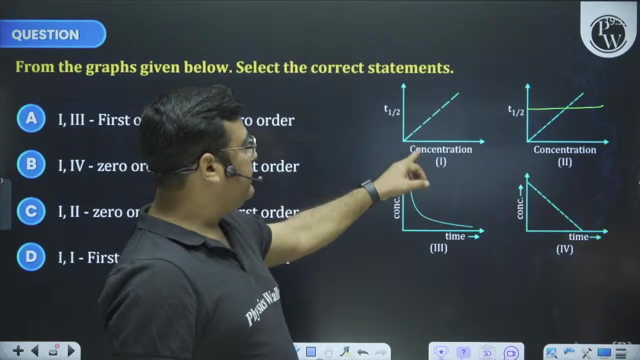 Come on, I am saying that this graph is wrong. these two graphs are the same. So these are all the questions of JEE. What do you call it in first order? kinetics: Graphical questions should also come in chemical kinetics. If the graph of T half versus concentration is of straight line passing through origin, then zero order. 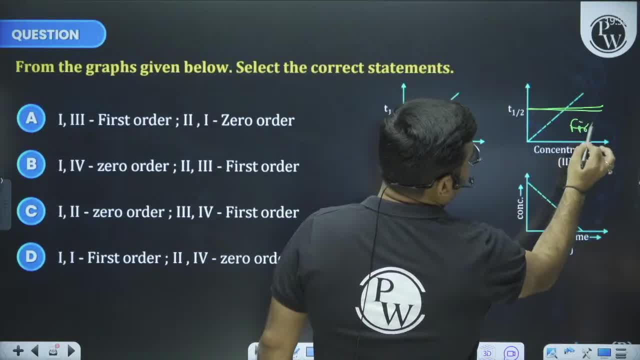 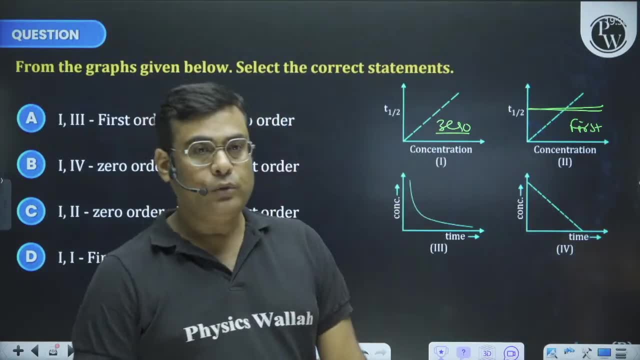 And if the straight line is parallel to the concentration axis, then first order. Why? Because the formula of first order is T, half ln, 2 by k and its formula is a0 by 2k. I am trying to revise the whole chapter in your way. 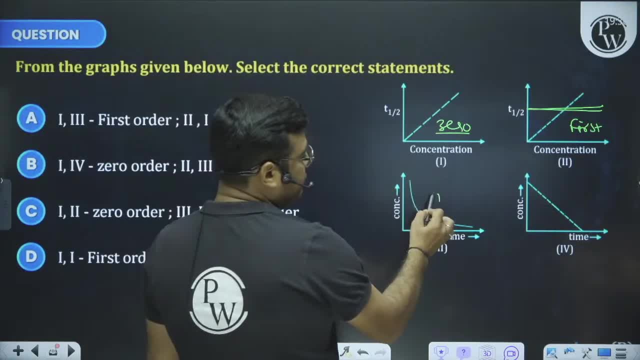 Concentration versus concentration. If the graph of T half versus concentration is of straight line passing through origin, then first order, And if the graph of T half versus concentration is of straight line passing through origin, then zero order. I just told you. 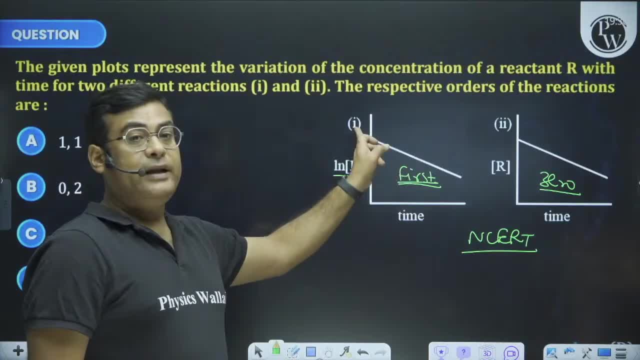 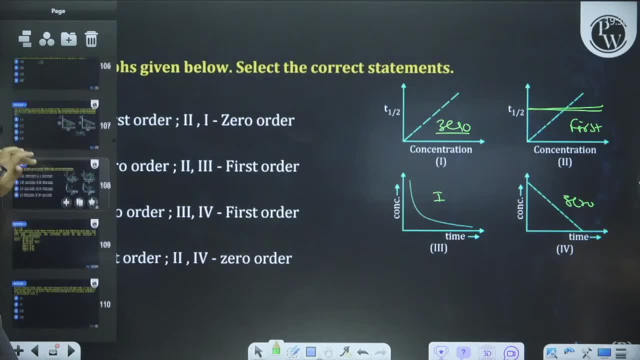 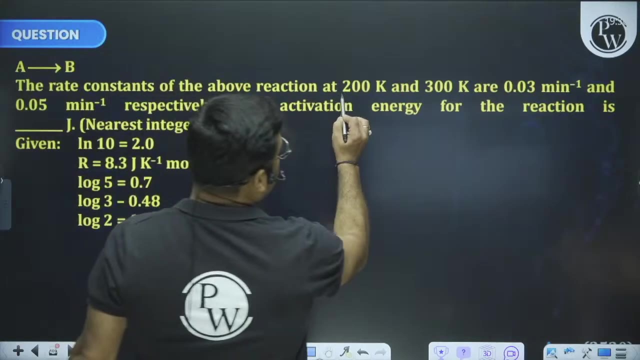 If the graph of T half versus concentration is of straight line passing through origin, then first order. So these graphs were asked. Now I will ask you some questions. On which graph? On the temperature graph, So that we can move ahead. The rate constant for the above reaction is 200 Kelvin and 300 Kelvin. 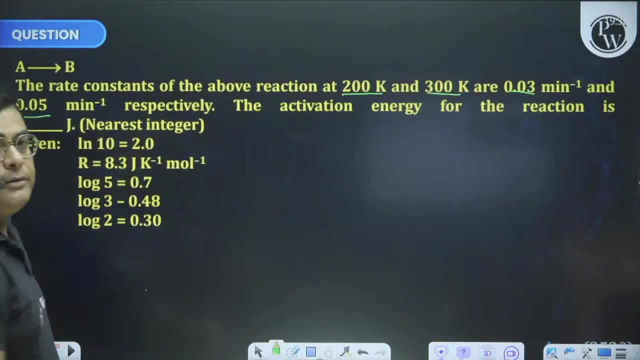 This is the activation energy for the reaction. Now children quickly understand JSC. There is a formula. Look at the value of ln 10.. Some of you were saying, sir, that what should we take? Those who will take should be mentioned here. 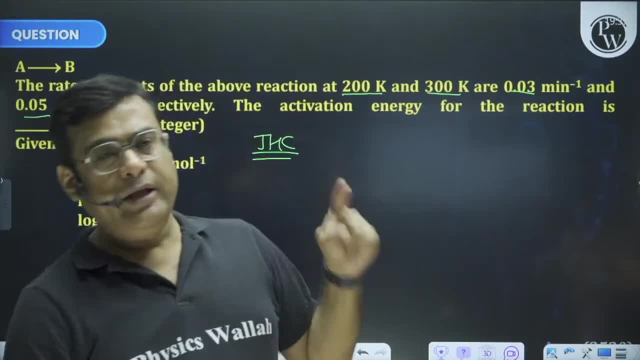 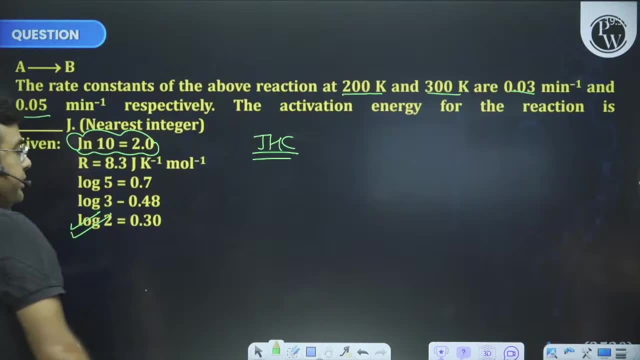 I am saying this much. If the NTA did not mention, then in my time I have told you clearly that I have written 0.3 to log 2. And he has mentioned it here. If he has not mentioned it, then his question was wrong. 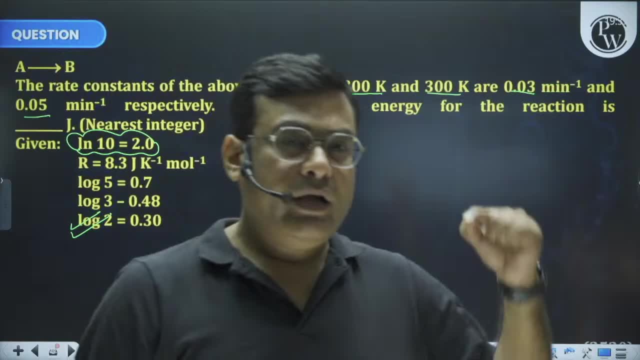 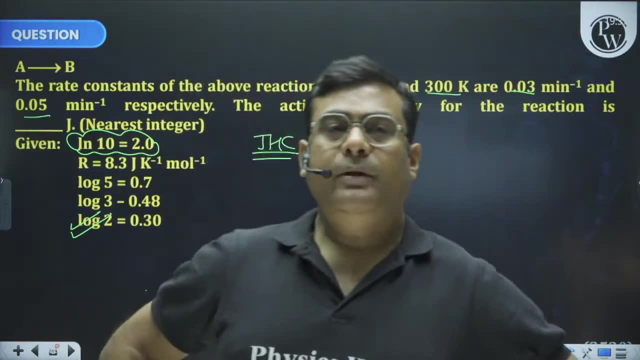 Because I was also saddened. Some children are getting 400.. Someone has 399. And he believed 399 to be correct. So we were also saddened. You must be thinking I don't know, some child wrote the best explanation ever. 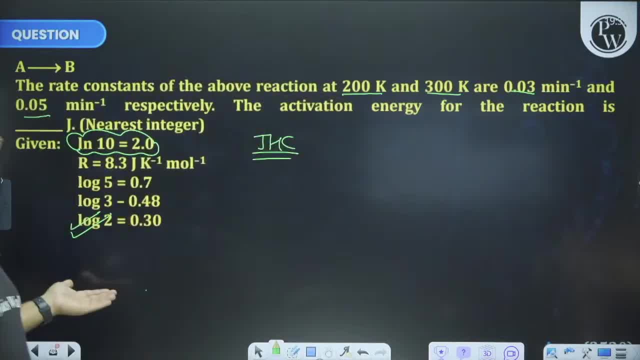 Now what is this best explanation? I can give the proof It should be written in these questions: How much value do I have to take in log ln? 10 is 2.3.. Tell me he gave 2.. He gave a margin of 15%. 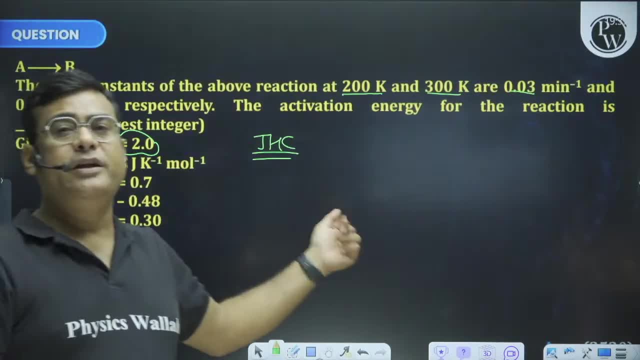 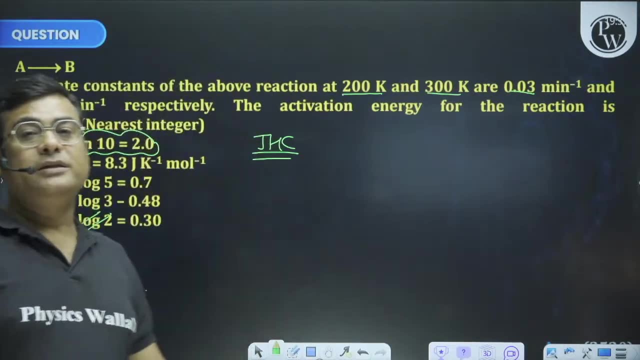 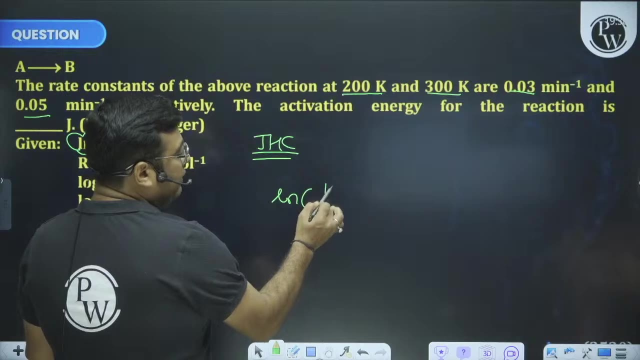 And here 0.3010.. There is no difference at all, But in a single integer there is a difference in the answer. It should be known. Okay, So now I will tell you this too- That you have the formula ln k2 by k1.. 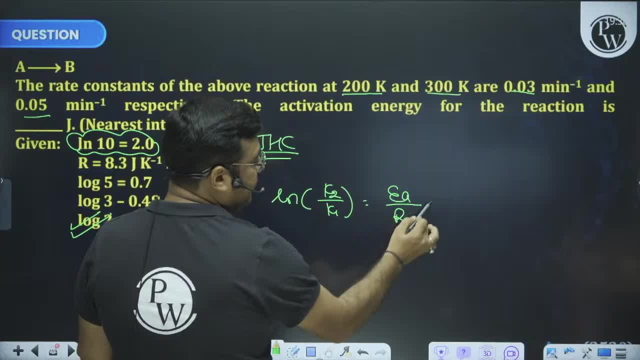 Now listen to it. from my point of view, It is Ea by R, Which is 1 by T1 minus 1 by T2.. Because there is only one question on the temperature. I will tell you only one question on the temperature. 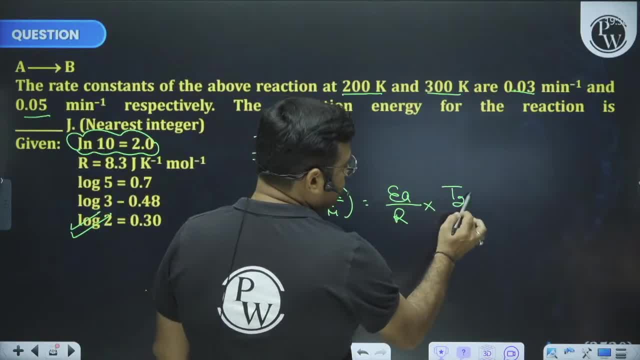 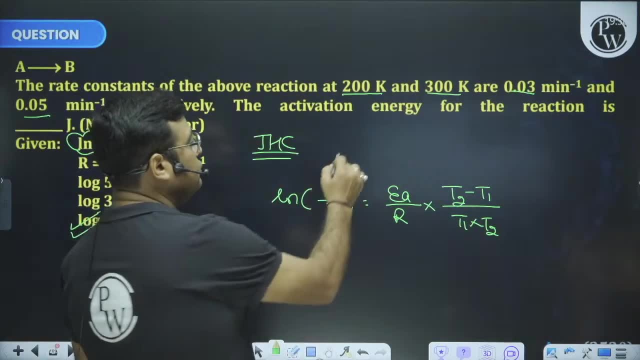 And I am moving towards the chemical equilibrium Children. write it directly: T2 minus T1 by T1, T2.. Write it, It should be in your mind Because I am telling the maximum children from you from now, Minimum 10% of the children. 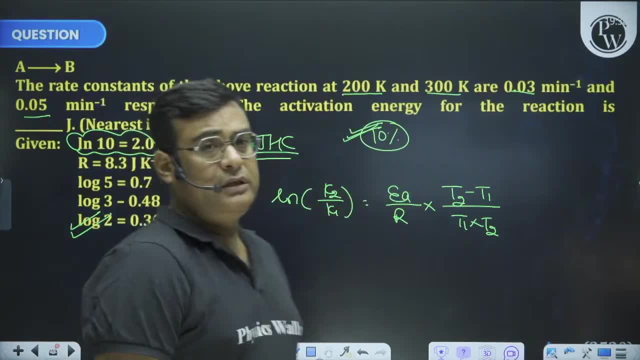 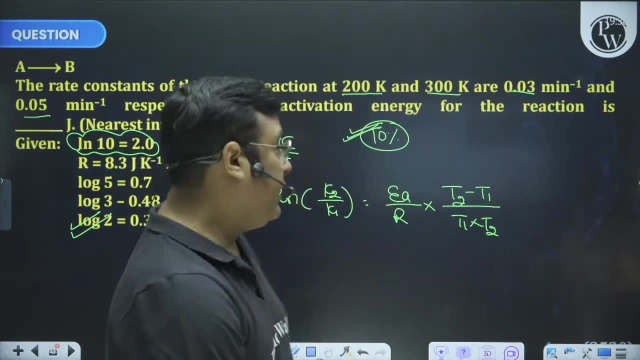 I am ready to say it with a chest. The question on the temperature is going to be seen in the April attempt this year, Isn't it? In this year's April attempt they are going to see the question on the temperature. I am telling you the guarantee. 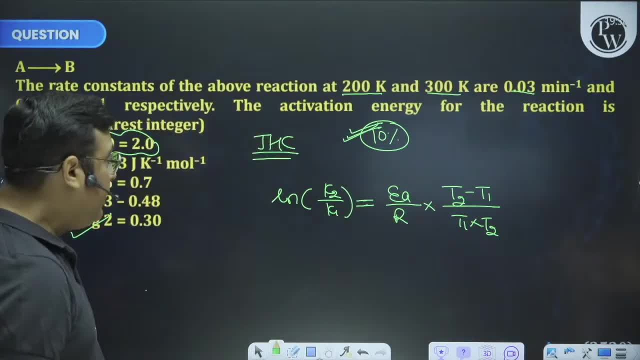 I am telling you the guarantee. I am telling you the guarantee from now. I am telling you the guarantee from now. Okay, Now, brother, Okay, 1.05 and 1.03.. That is 5 by 3 came inside the ln. 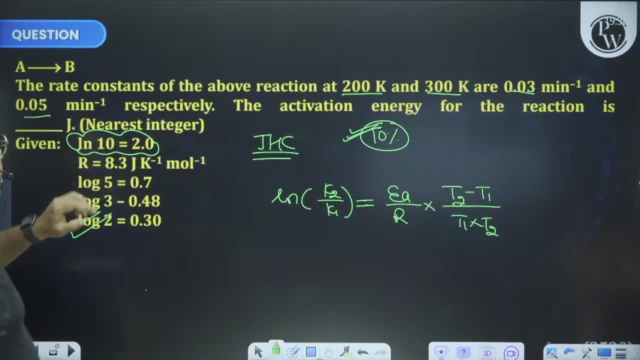 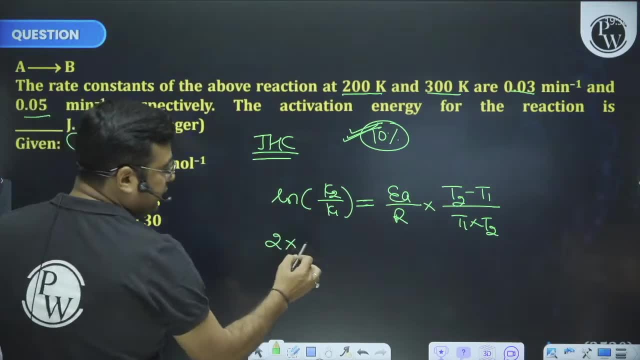 5 by 3 came inside the ln. If I change ln to log, Then, brother, It became 2.. Log 5 is 0.7.. Log 3 is 0.48.. I gave the difference of both: 0.22. 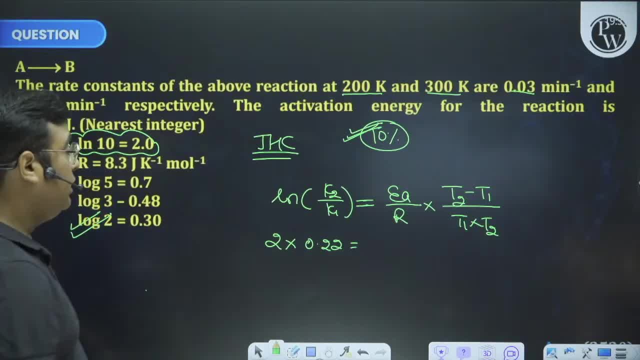 I am explaining the calculation trick. Everyone knows this formula: Ea by R. You see, children? He has also given you the value of R: T2 minus T1.. T2 minus T1.. Isn't it 200.. 300. 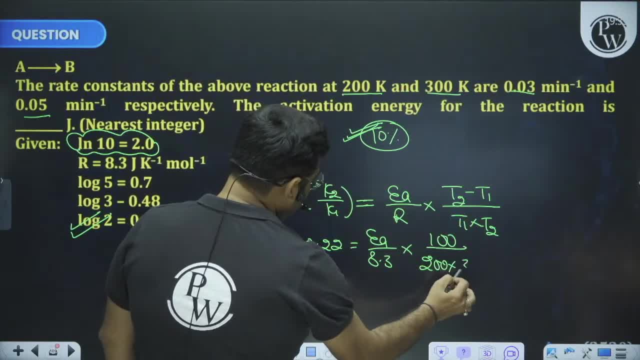 What is the difference? 100.. Below 200, into 300.. Now you tell me that we will not even do this much calculation. The question is over, Isn't it This much calculation From 2 to 0, this also went. 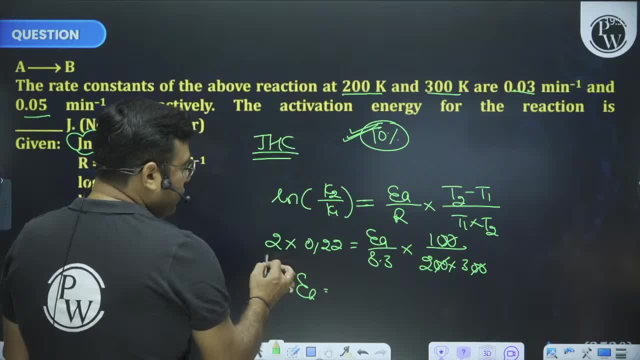 So for you, the value of Ea 2 into 22. 44., 44 into 2. 88. And here, 8.3 into 3. 24.9.. This is your answer. This is your answer. 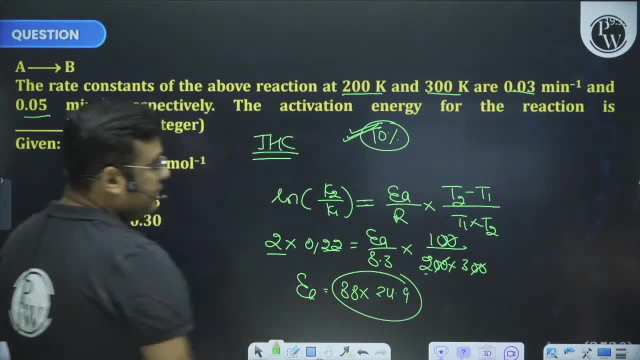 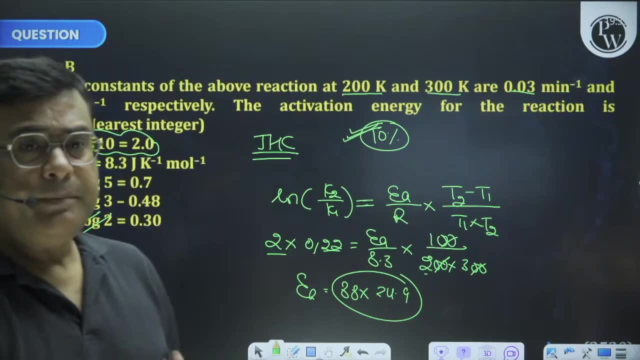 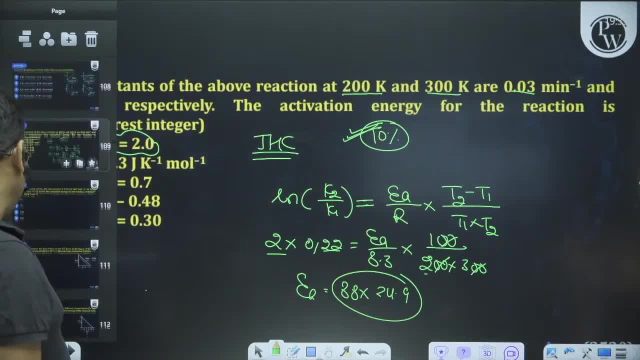 So, in this way, the lack of temperature issues, again, it is a question. See, this is the next question. The graph is given: LNK Versus 1 by T is given, The slope is given, Isn't it? And by giving value at 400 Kelvin, use 500 Kelvin. 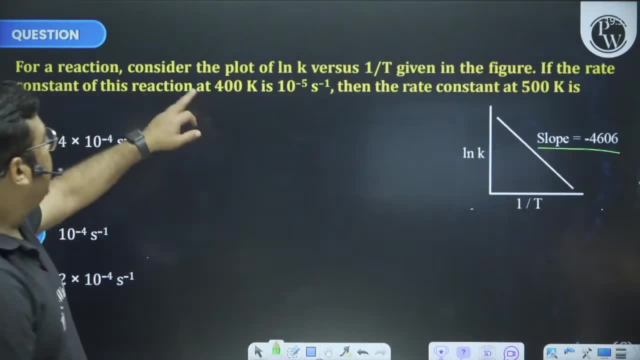 Again, the temperature issue is same. There is no time to do it again Now you will do. The graph is given: LNK Versus Tn by 3. The activation energy is asked. It would be the slope, only There is 10.. 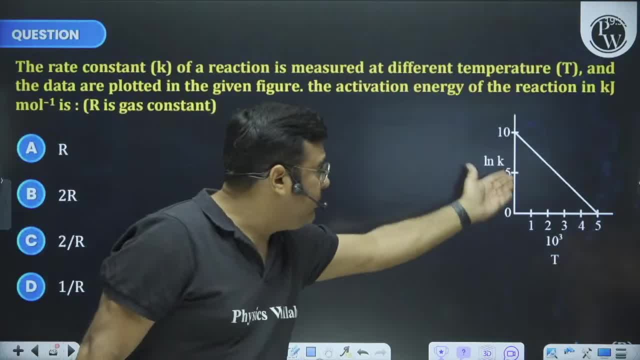 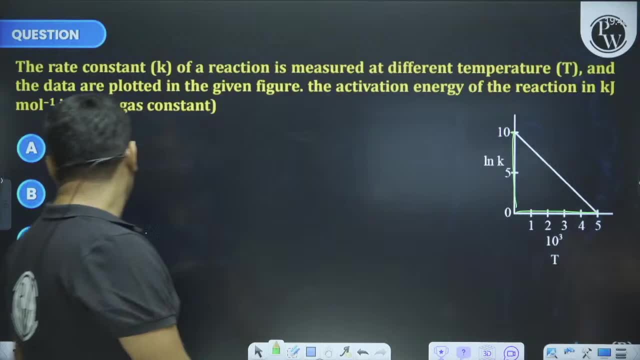 There is 5.. And 10 by 5 means 2.. And after that the less ÖI get from this equation. So what happens? The episode addition of Ea 1 by 6 to C, equal to 1.. I have asked you, it is slope. here is 10,, here is 5, and 10 by 5 means 2, and R will be multiplied by 2R. 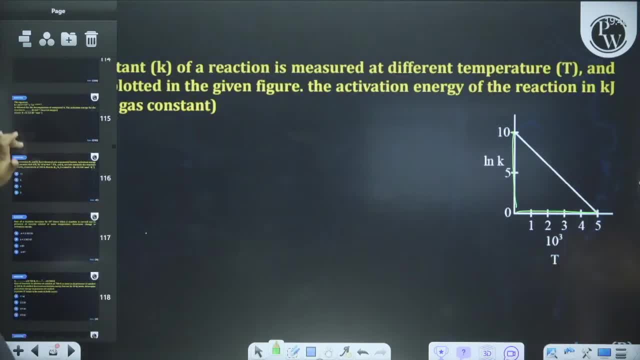 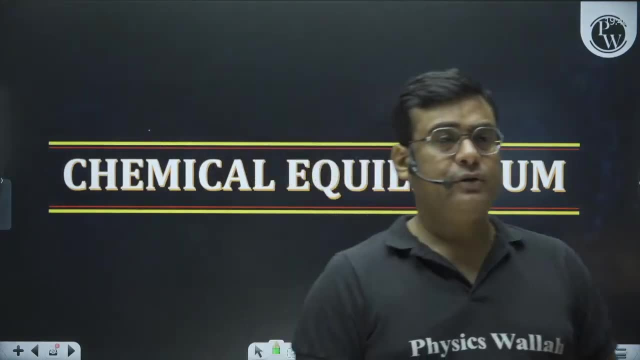 Okay, dear. so now there are more questions. I will leave that to you, dear, because you will do it now. we are increasing the chemical equilibrium. This is not that important chapter, children. after this we will take a break. okay, so this will be over soon. 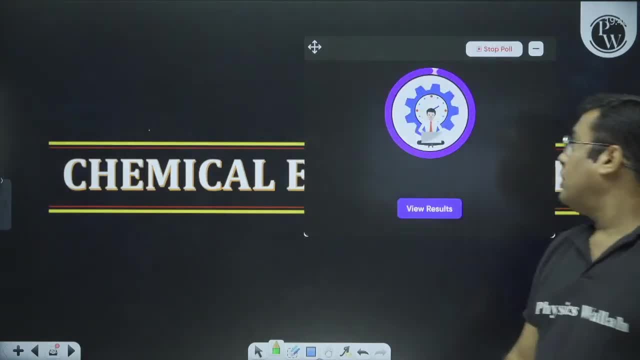 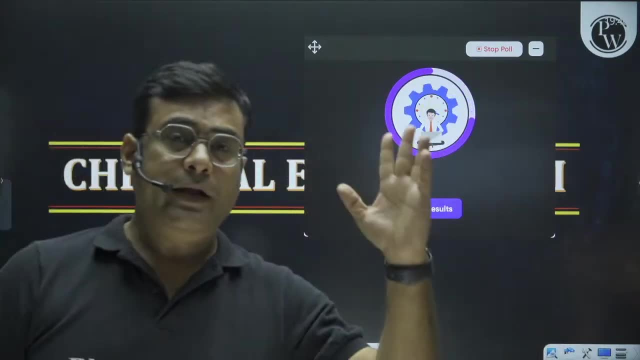 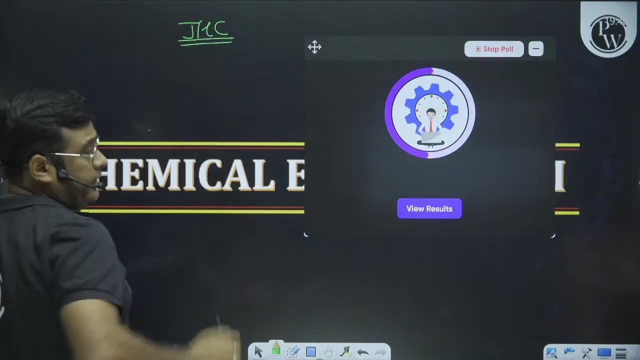 I will make a 30-second poll again. have we got to learn a lot of new, good, beautiful things in three chapters, and the chemical kinetic is still the third chapter. see, your JSC is a little bit of a concept now. what happens is that when it wakes up, it is morning, isn't it? 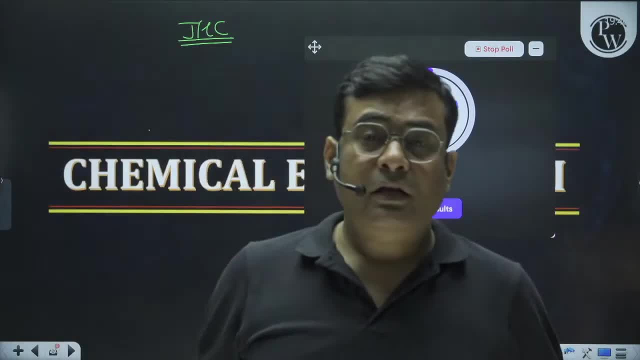 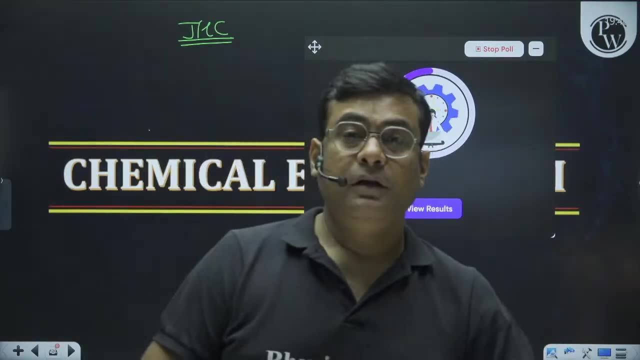 These days the TV. people have also made an ad: come, let's do something stormy. so many people have started the session at 5 o'clock. now they are coming at 7 o'clock. 40 minutes now. say now, what is JSC? 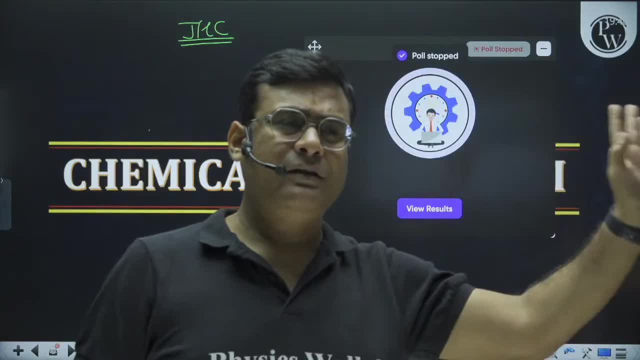 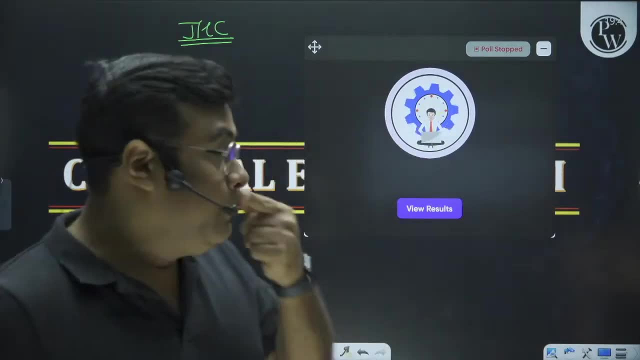 Now they are in the mood to do stormy, that for two and a half hours those who have gone go to hell. now let's see how much stormy it can be. so he has come to do stormy, okay. so tell me quickly, children, isn't it? 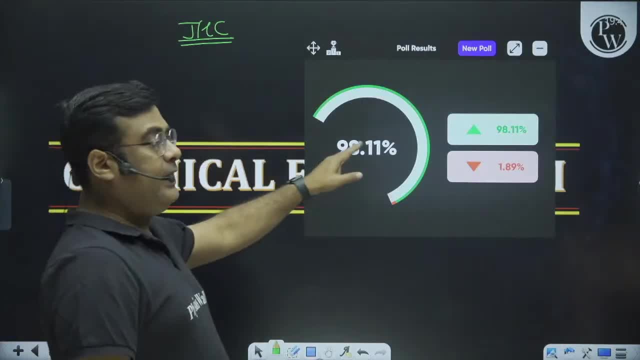 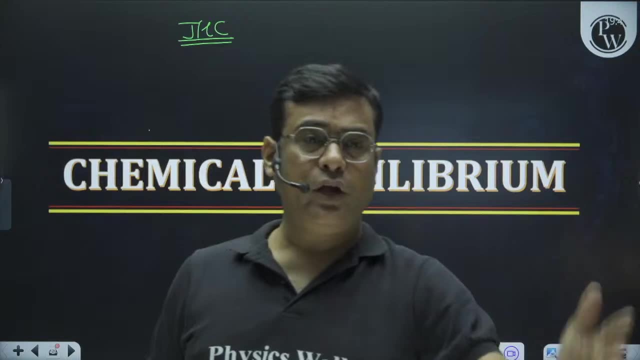 Our motivation is your understanding: power 98.11, good thing. so, in the MOL concept, the little bit of your fear that hype, hype must have gone away in Redox, then you have learned interesting things, brother, isn't it? 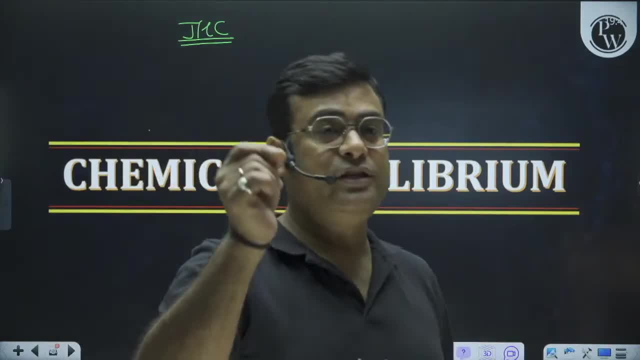 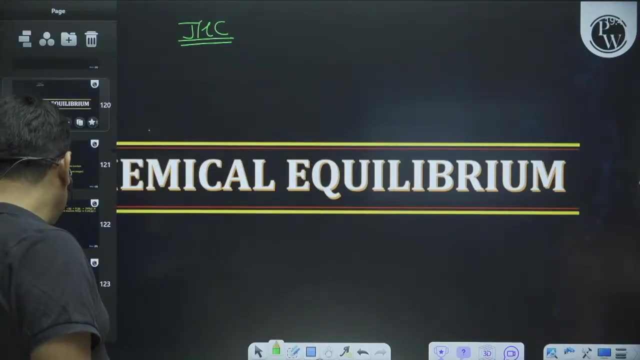 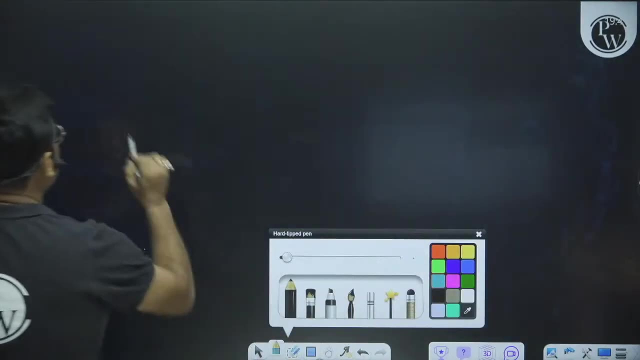 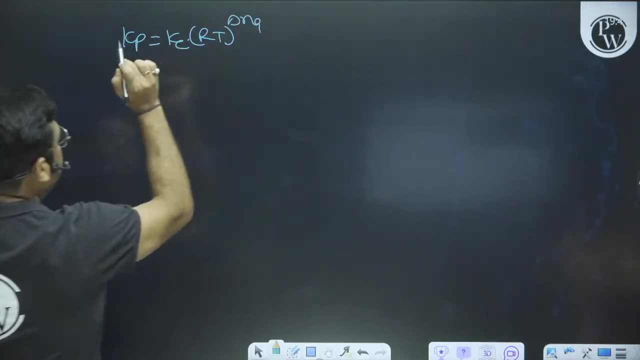 100% guarantee is there, and what is it In the chemical kinetics, the calculation you are involved in, you must have understood that now there are not many new things in the chemical equilibrium, son, I don't have, but still there are no new things. still, I will tell you in this too. first, I will tell you that in this, after all, more is asked. you all know, son, KP equal to KC, RT's power, delta is not there, brother, he is crazy. he is crazy. he is crazy. who is crazy? this one on this formula? children, isn't it? 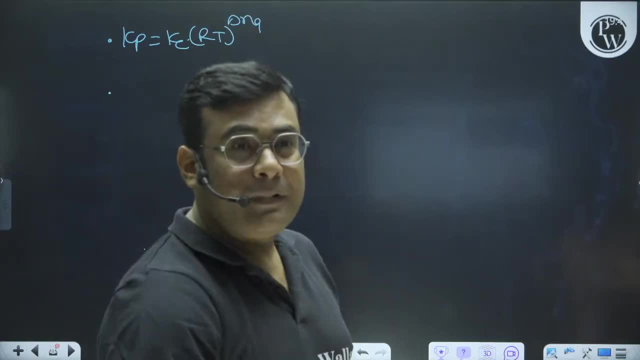 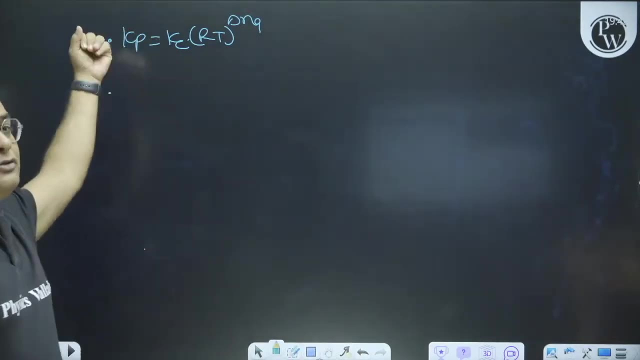 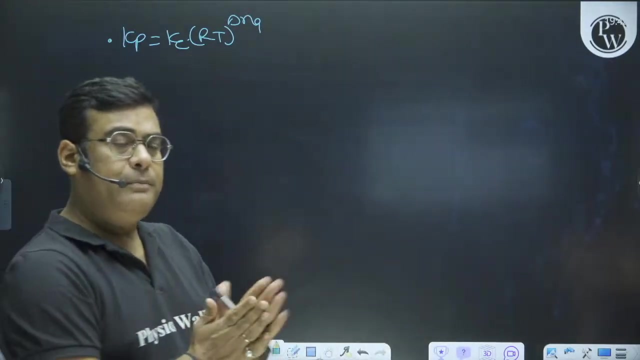 Isn't it Isn't. it Is this hundred. there is no other error. it is a good thing. okay, it will be a good thing. there will be an error? Yes, well, no problem. then this small equation: KP is equal to KC, RT. yes, there are no questions. so this topic of ours is only fifteen, twenty minutes. at eight o'clock we had talked about break, so we take a break for five to eight, ten. 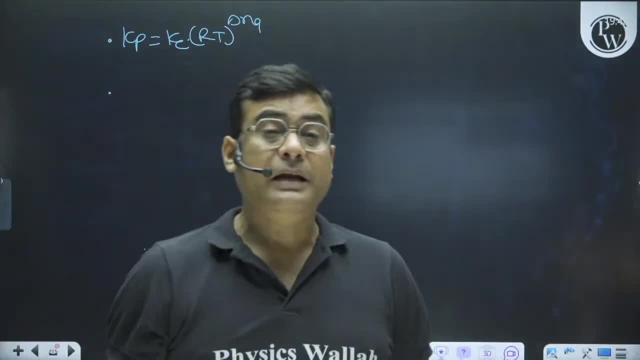 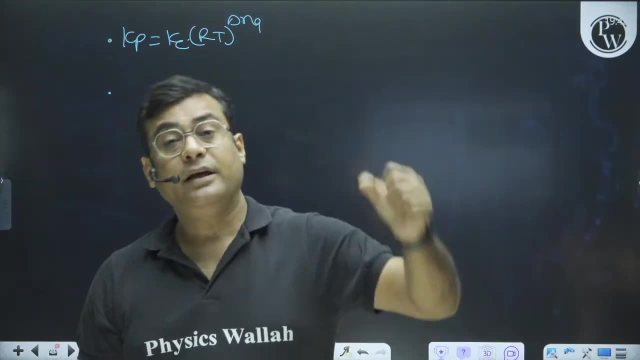 Is it right? I will definitely come after that. so after break we will come on the I-NIC, after that we will come on the electro. I have told you the sequence. so after the break With energy, Get back to the issue. 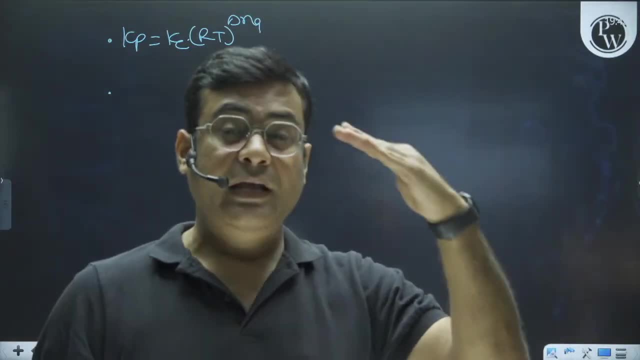 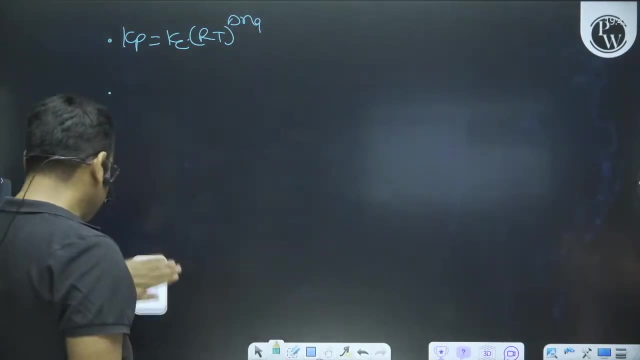 Bring tea or coffee with full energy, because ionic, electro and then your liquid solution, thermo, will come in this order. So this formula must be taken care of. next one is N2O4 gives 2NO2,. now write: A gives B, X gives 2Y. I will request the formula of Kp to all the children. remember the terms. 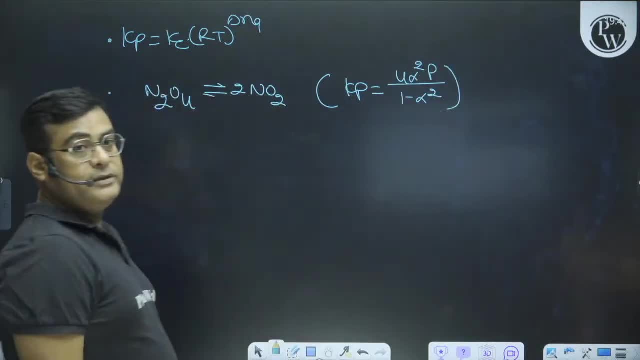 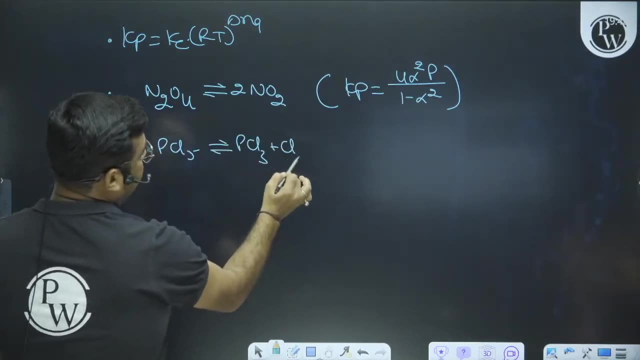 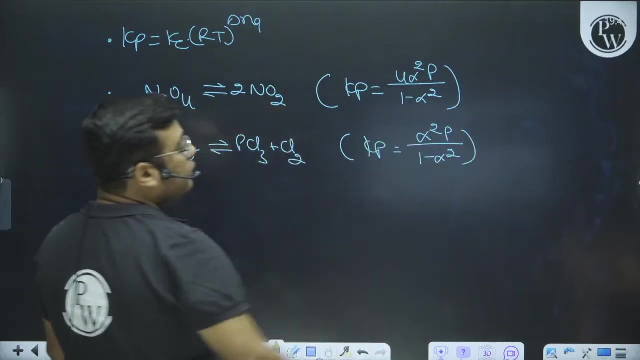 of alpha, 4, alpha square, P upon 1 minus alpha square. In the same way, PCl5 gives PCl3 plus Cl2, its formula of Kp, the formula of Kp of both, is same. the only difference is that because of 2 here the square of 2 becomes 4, it is 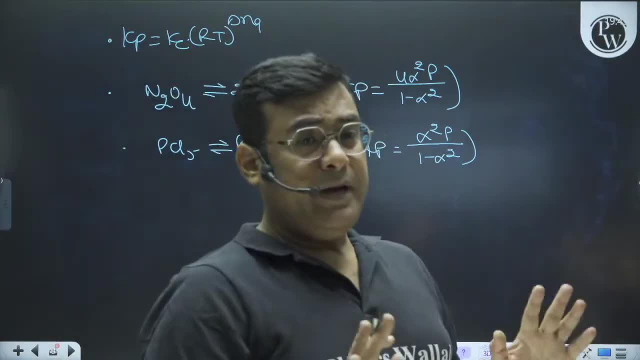 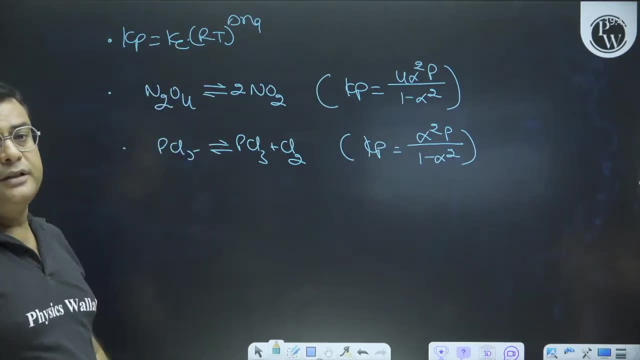 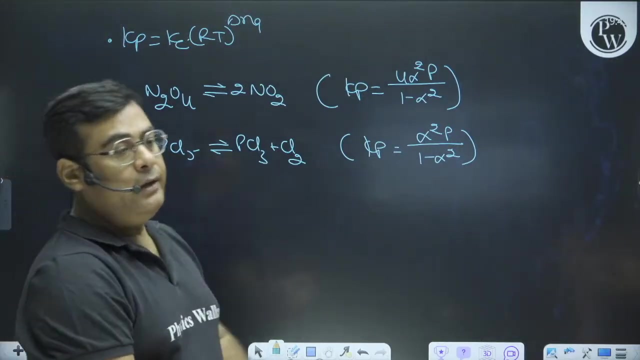 not here. it is not here. so these are some things which are absolutely important, son. the questions come on this formula, the questions come on them. that's it, Sir. if you do not understand anything, son, if you do not understand anything, then 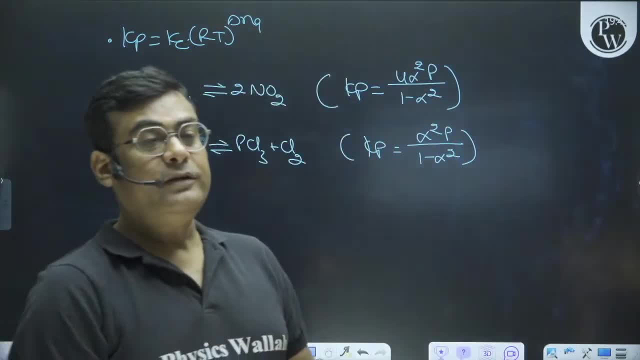 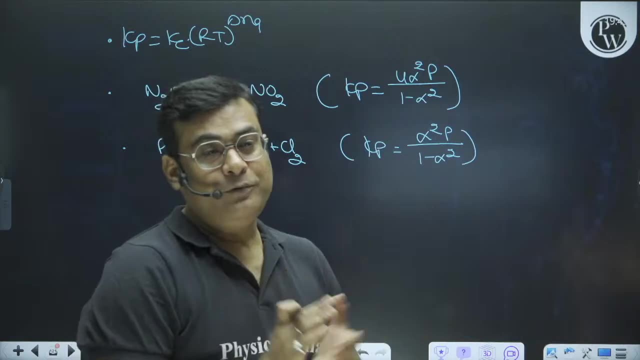 you should get out of here quickly. you should get out of here, son. there was no need to waste so much of time that you are writing your message and wasting your time right. hopeful girl Shanta bhaarti- the names are also very interesting. I do not understand. 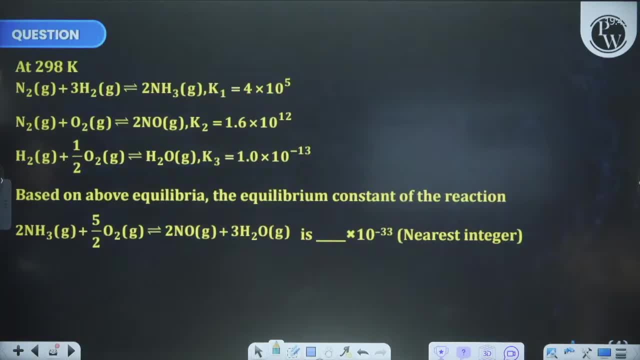 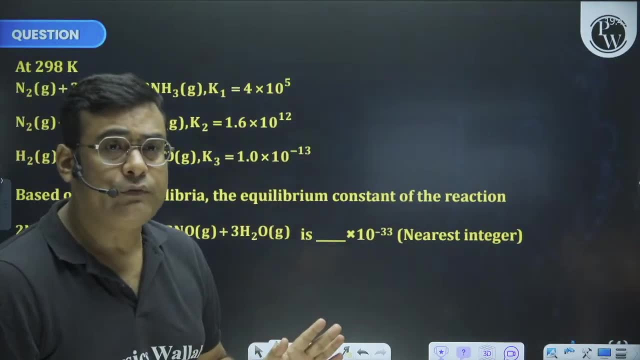 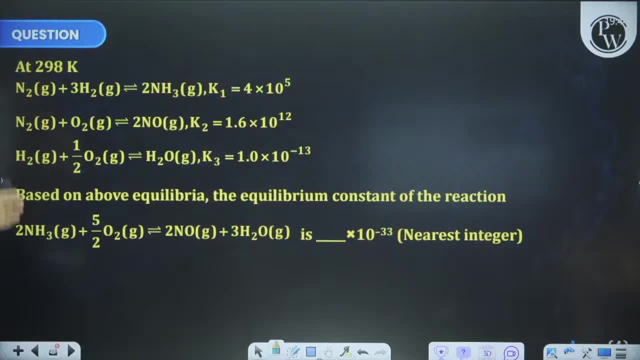 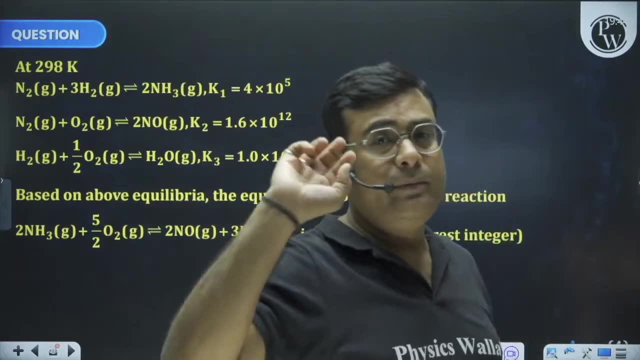 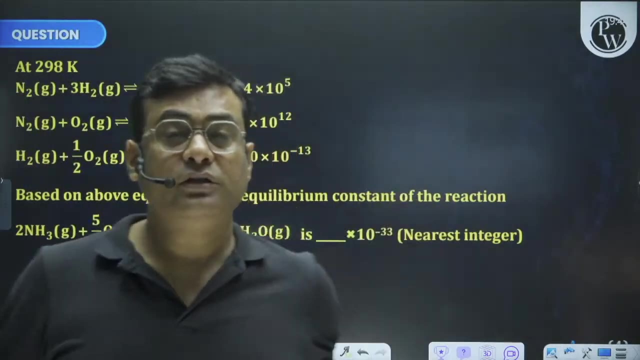 telling you the trick- this is also a question of JEE- by giving three reactions, by combining one now in this, you guys have told me 100%. till now you must have wasted a little time, son. but now listen to me. concepts hit the confusion and the concept of Holi Holi. 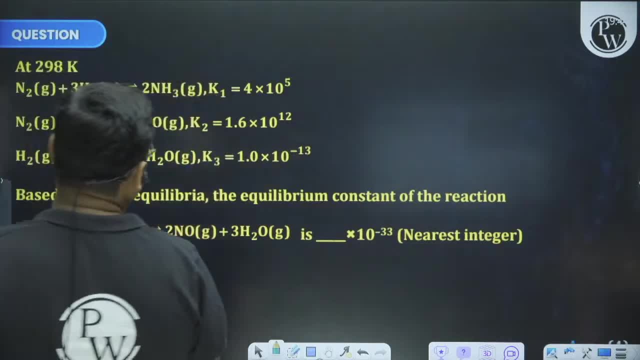 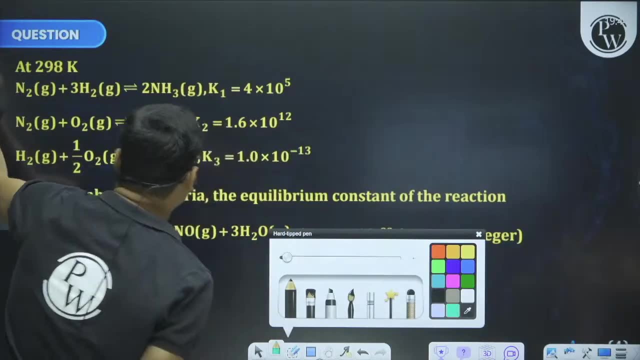 must have been celebrated a lot. you were on March 25, and now on March 30,, we are learning the Holi of physical chemistry. what has to be done in this son? learn to catch the uncommon species, ammonia. right, ammonia was the reactant side. the product side went. 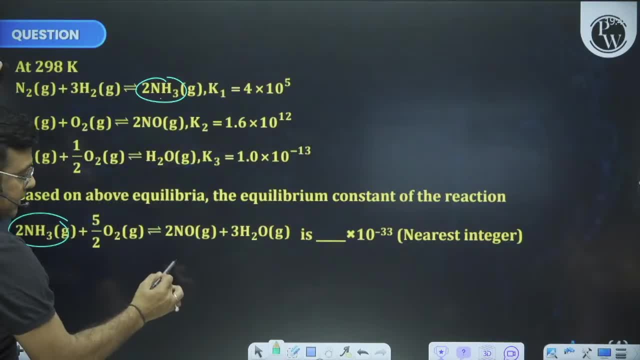 whenever the reactant goes into the product, then, you know, its rate constant becomes inverse. sorry, the rate constant comes in the chemical equilibrium. reverse it. then. look at the coefficient, sir. there was a coefficient 2,. there is no change in the coefficient 2,. 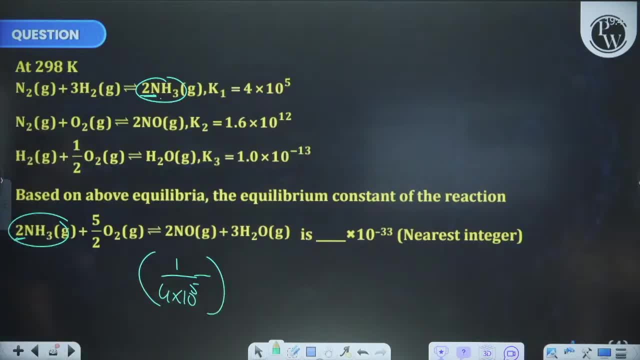 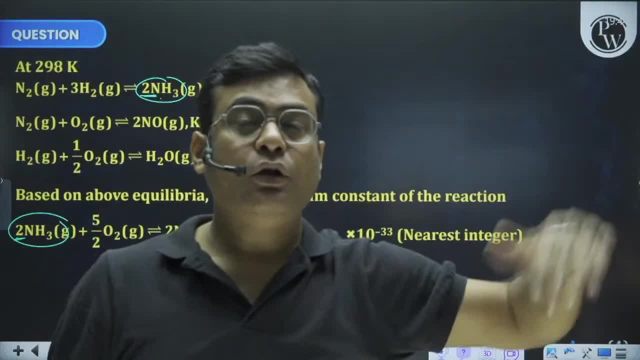 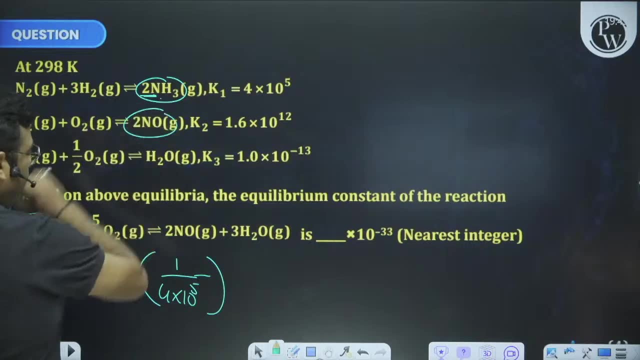 coefficient. if two changes to four, then they do the square, if two gets six, then they do advances. you will know, I am telling you all of this only, son, that how do you do it quickly, sir? two of them, sir. they are products. they are products, okay, right, meaning its Idle. 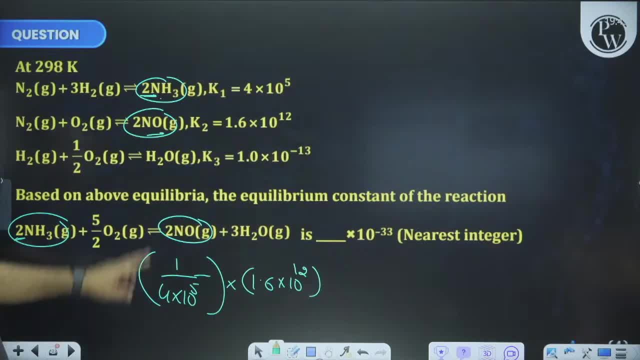 class is going to be now. it is not going to go inverse O richtige on his right and exercise the lowest mission is over at the product. the product side is there, then there is 10ωp. what will happen in this situation? what will happen in this situation, brother, which is: 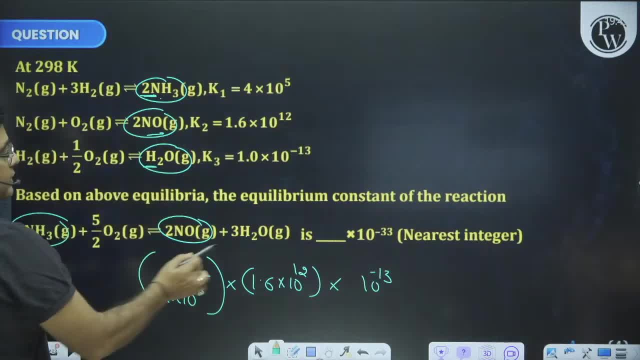 10 to the power of minus 13,. but sir F2's coefficient was 1, we have done 3, which means I will have to do it into 3,. the story is over. I am done with the story. just solve it whatever. 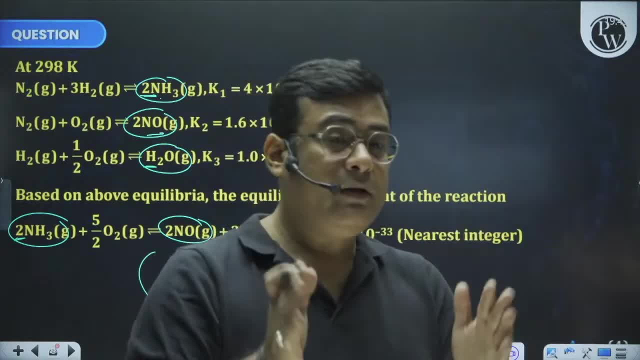 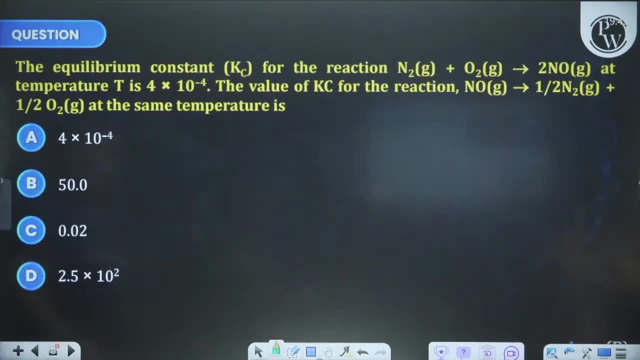 answer comes in your nearest integer. so these questions have also come in full. some reaction equilibrium constant will be given. with the help of them, the equilibrium constant of the new reaction is to be taken out. see this again. this is of J, N2 plus O2 gives 2. NO, the equilibrium constant is 4 into 10, to the power of minus 4,. 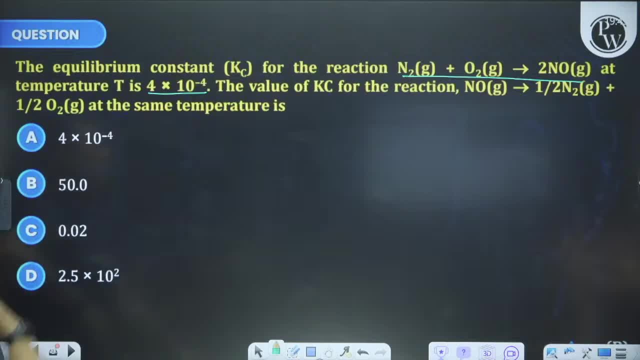 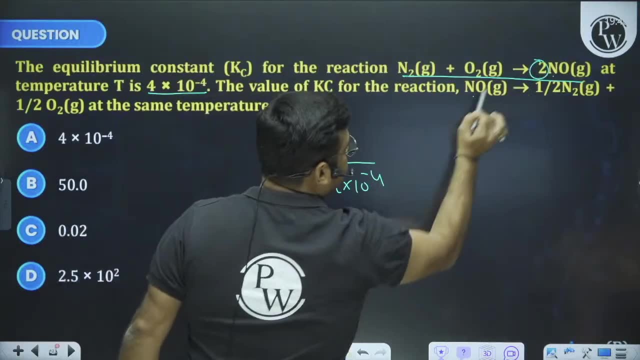 so it is saying NO gives half N2 plus half O2,. brother, the product was in the reactant first. do the opposite, sir. did the opposite, sir. the coefficient was 2, we have done 1, that is. from how much did you multiply from half? 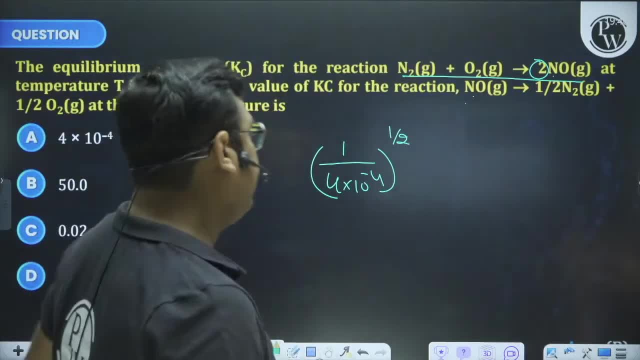 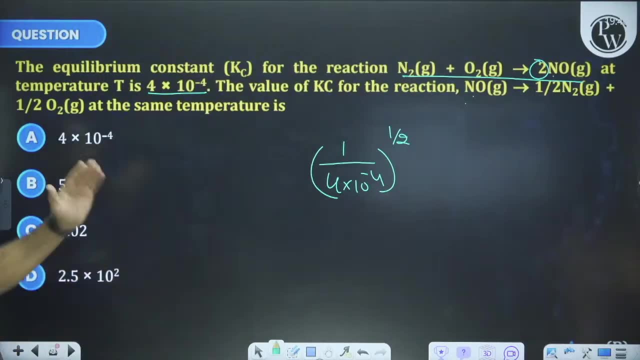 from which you will multiply, son, it will raise with the power that is under root of 4 into 10 to the power of minus 4, under root of 4, 2, under root of 10 to the power of minus 4, under root of 10 to the power of minus 2, went up from below 100,. 100 by 2 is 50, clap. 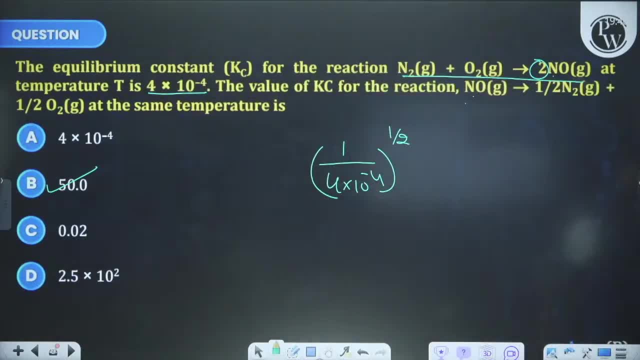 if you knew this trick, then it is a good thing, but if you do not know it and now come to know, it has become a little fast due to this, sir, your work. this is a question from the session on January 26,. absolutely, absolutely, yes, clap. if it is good, son, it is good. 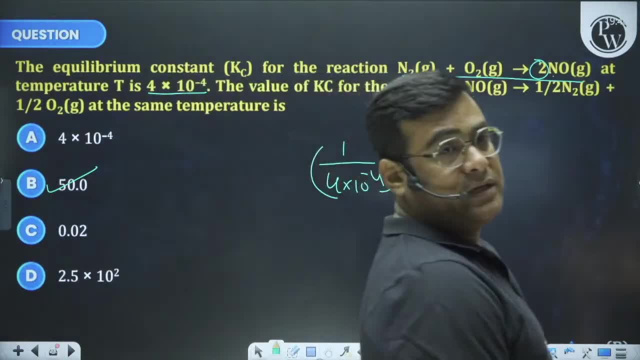 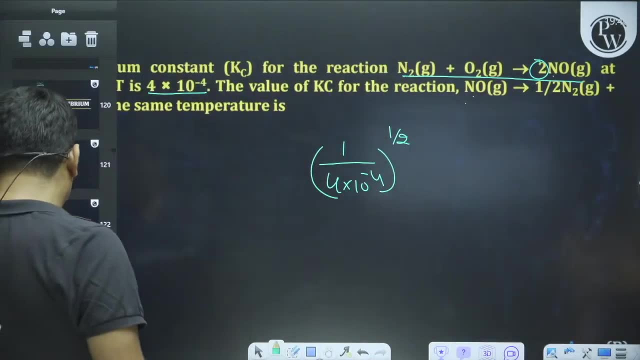 I did not know, and now I know. then any of you will get to see this question again, you will get it. you will get it. I am telling you from now, right now, there will be more questions like this. I am leaving it up to you. see it again now, if you do not know it. 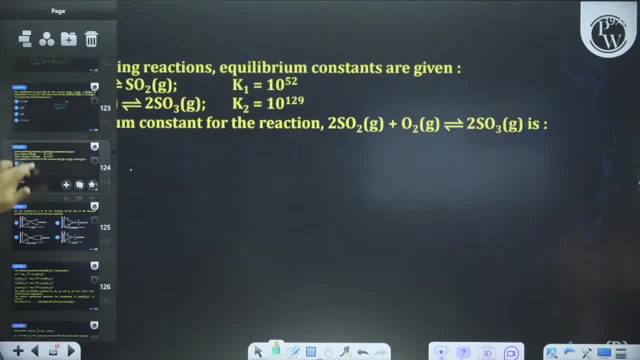 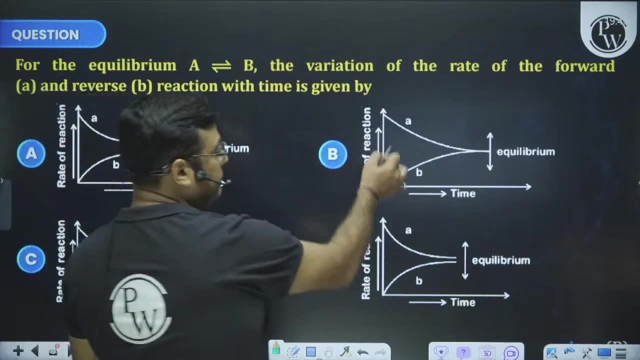 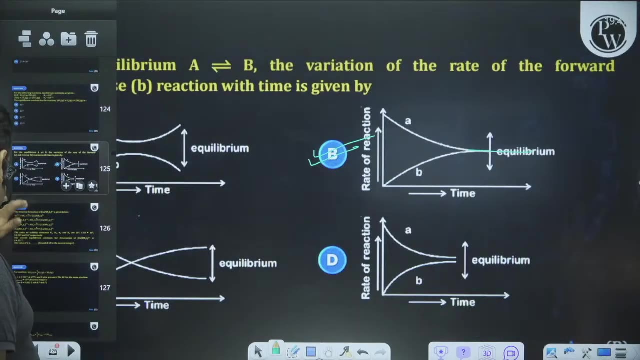 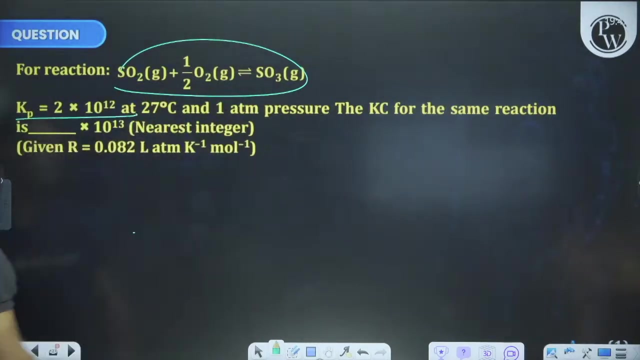 because k1 and k2 are given. we have to get them out. I just want to tell you we should know the graphical question. when the equilibrium is established, when the rate of forward reaction and backward reaction are equal to each other, and after that they are always the same, we call that equilibrium ok, kp and kc's question is said. it comes in full. this is the reaction given. if kp is this much, then kc for the same reaction. 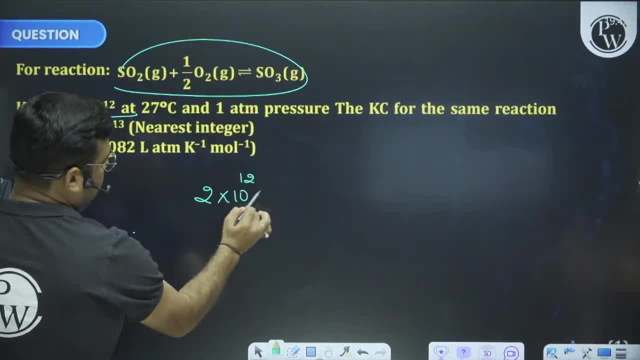 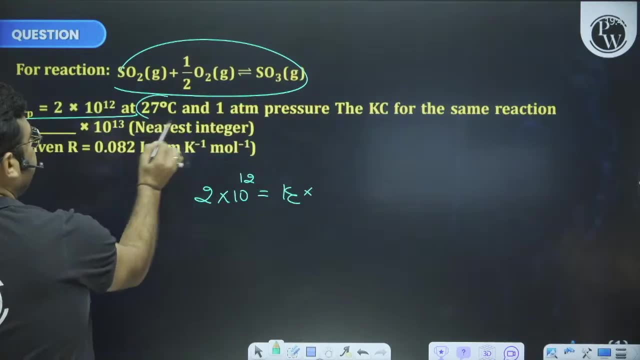 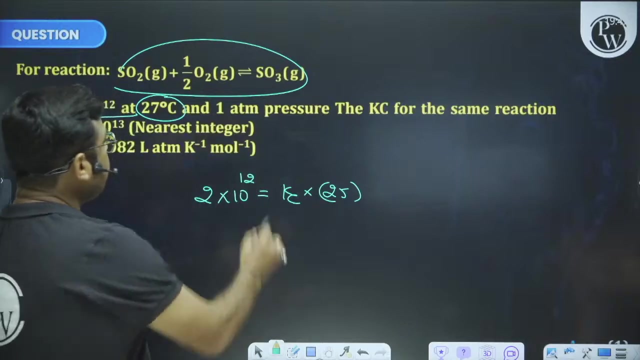 2 into 10 to the power of 12 equals to kc into RT. I just said, if the temperature is 27 degrees Celsius, then write the value of RT without shame, even if it is in nearest integer. write 25,. I told you 25, now delta ng. 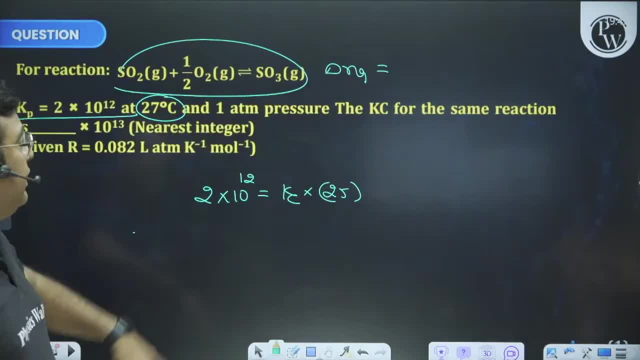 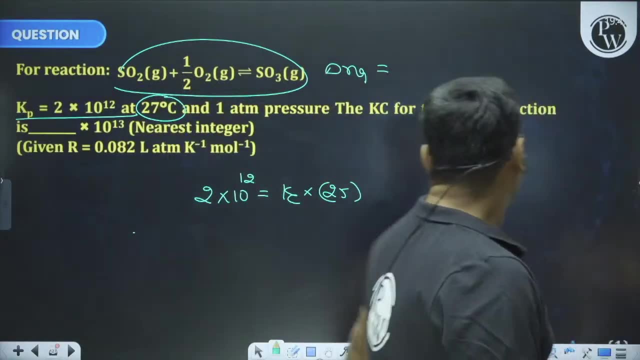 it is possible that some of you do not know how to calculate delta ng. so delta ng means delta means children, change, n means number of moles, so g means gas. so delta ng's value is 1 minus. 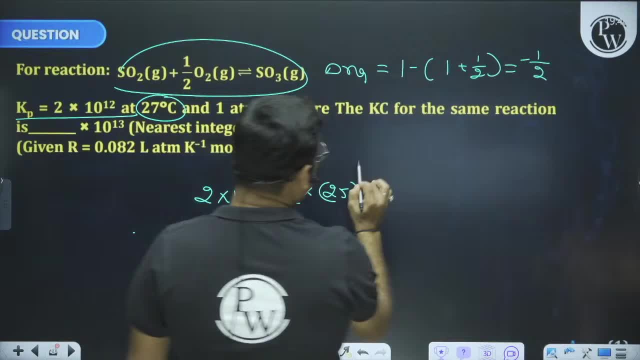 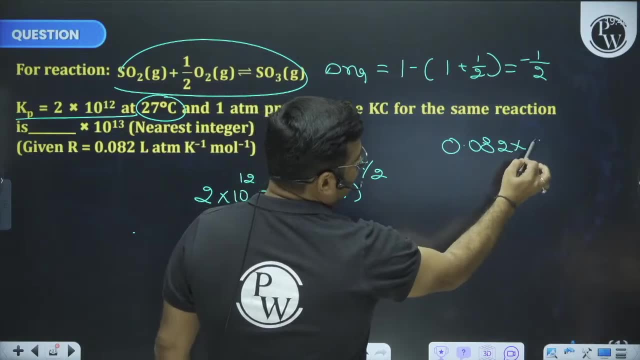 1 plus 1 by 2, means minus 1 by 2, this is minus 1 by 2, what you do, son? I am telling you your technique too. you multiply 0.082 with 273, temperature, sorry. 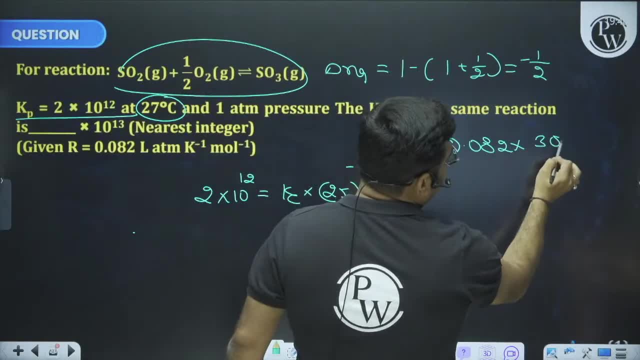 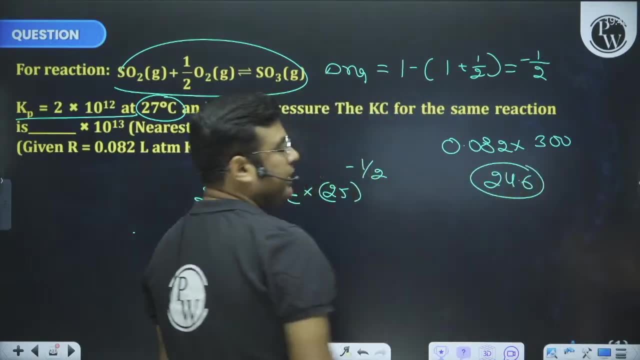 273,. I am writing from 300,. let's do it. let's put decimal decimal. let's do something. let's do something you do lambda. I know it is 24.6, because why I do, lambda? 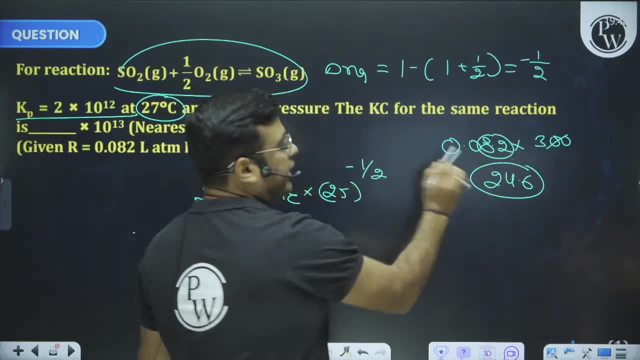 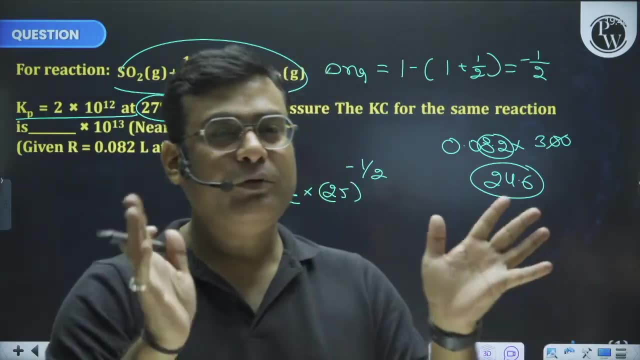 I do this decimal from 2 to 0, 8.2,, 8.3 into 3, now you tell me if you want to take 24.6's under root and 25's under root. there is no difference between them. 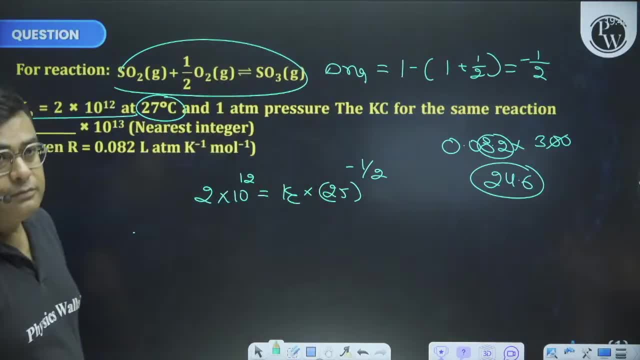 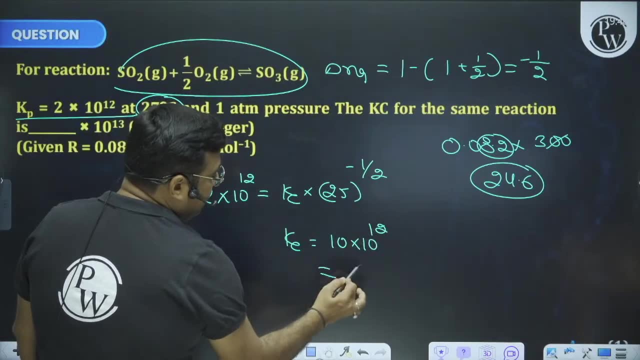 it will remain same in nearest integer. 25's power minus 5 by 2, means 1 by 5, means kc's value 52010, into 10's power 12, means 10's power 13,. he has given this. 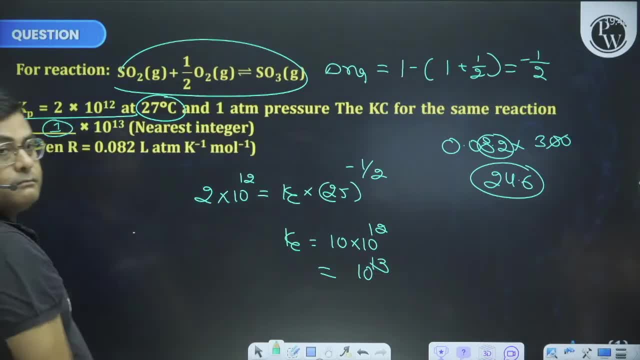 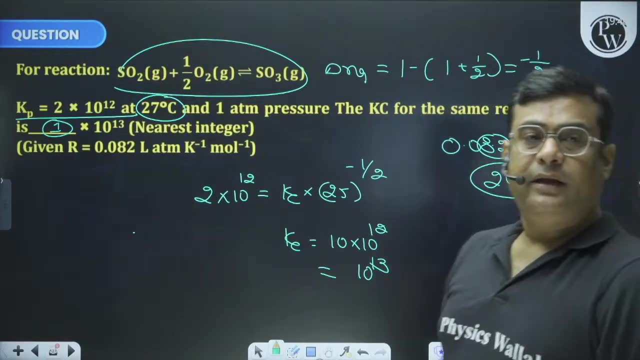 that kc for the reaction. this is the time, little bit, you people right, it must have been done for a year. but actually, what is it that it is believed that the calculation will be done by the child and my? 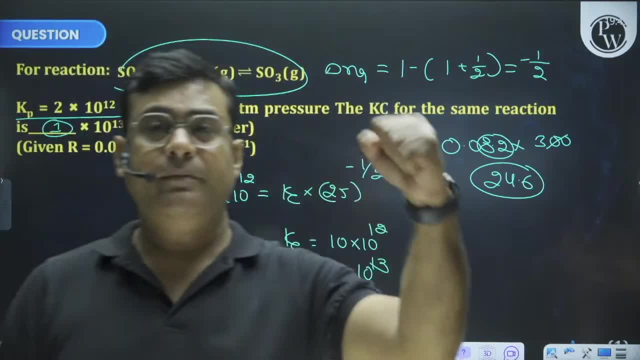 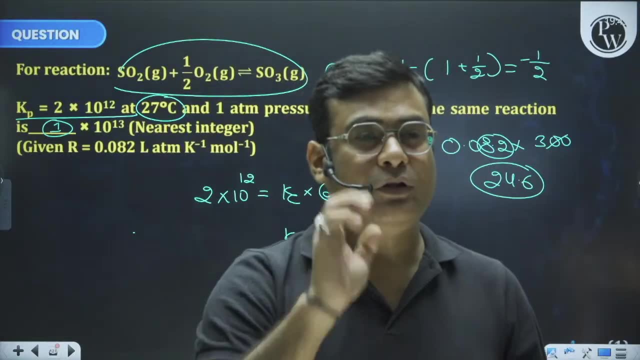 our army. right, sir? this is the question of the 26th January session. great, okay, I am not able to read it completely. son, I am your, but our army 3.2,, Prayas 3.2,. 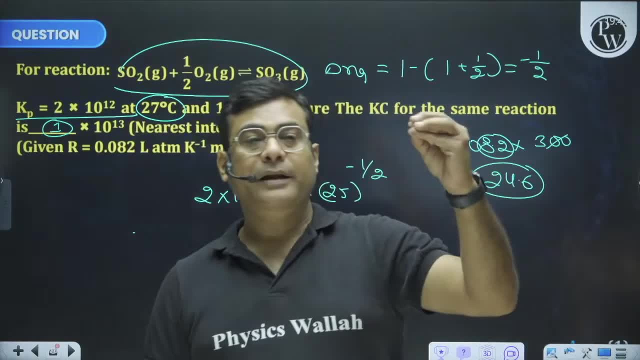 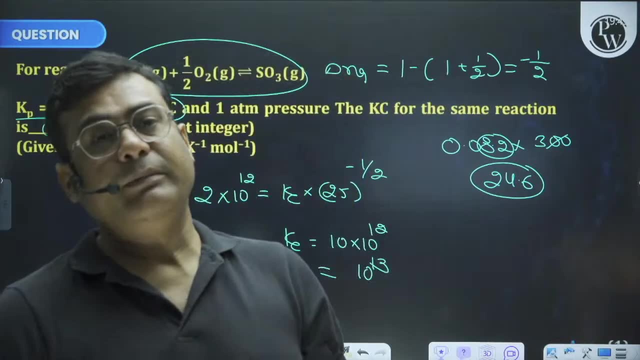 I have calculated their calculation too, because I have given them throughout the year. I have given them, I have given them, I have given them throughout the year. keep explaining right, because I believe children, that children will understand the calculation. 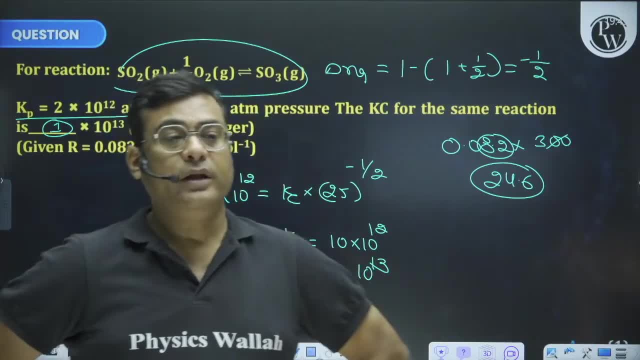 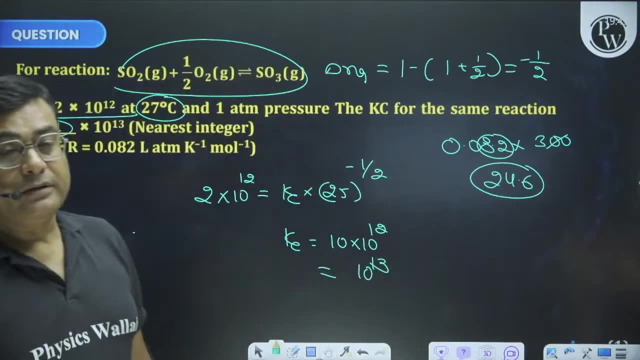 only then he will be able to do the calculation effectively. for this say: leave it, brother, you do this. right, you just have to do this calculation. no, if you teach, then the child will learn. son. 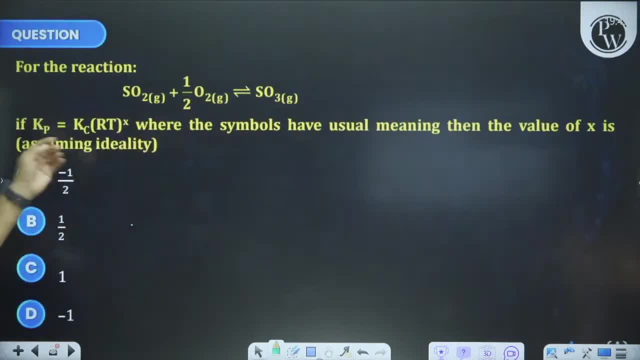 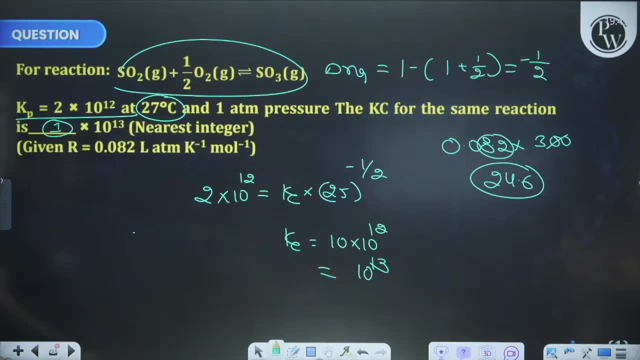 only then he will learn to apply. okay. so on this too, see again the same question right in this. KC has asked here. he has said that if Kp is equal to sorry, excuse me. 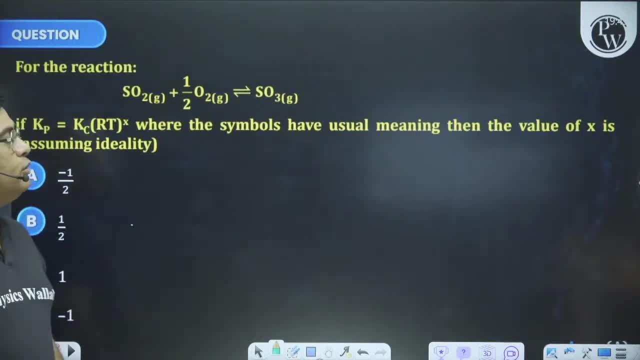 if Kp is equal to Kc, Rt, power, X, where the symbols have usual meaning, then tell me the value of X son minus 1 by 2, delta NG asked: sir, do you ever teach in Kota? 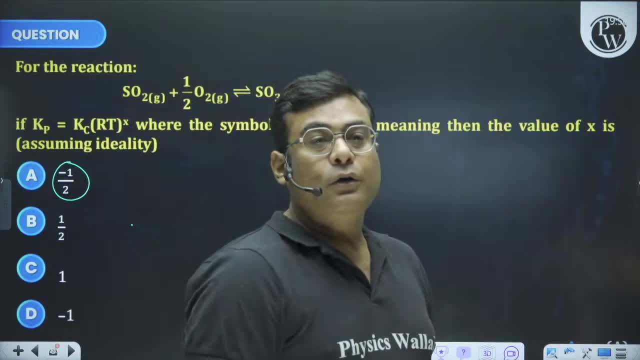 son, I have been teaching in Kota for the last 23 years. right, I have been teaching in Kota. right, I have been teaching in Kota for the last 23 years. just in the middle of one or two years. 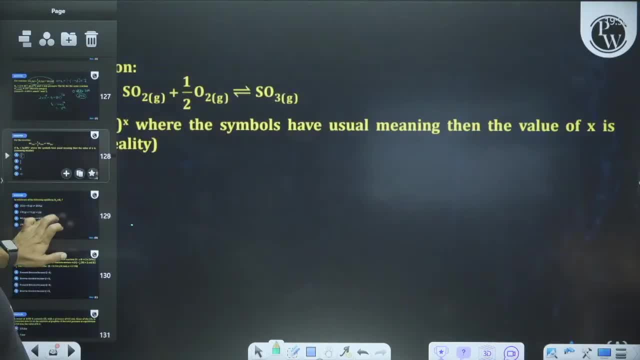 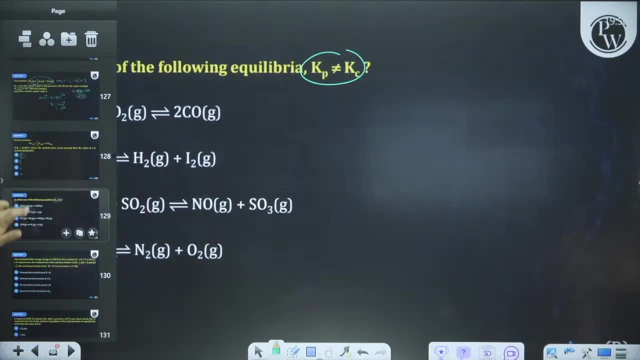 I must have gone here and there, otherwise I teach in Kota again. in which of the following: Kp is not equal to Kc. you have to do, son. I am just telling you that the questions of equilibrium. 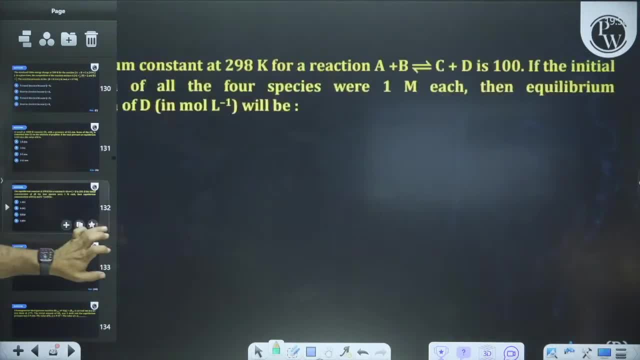 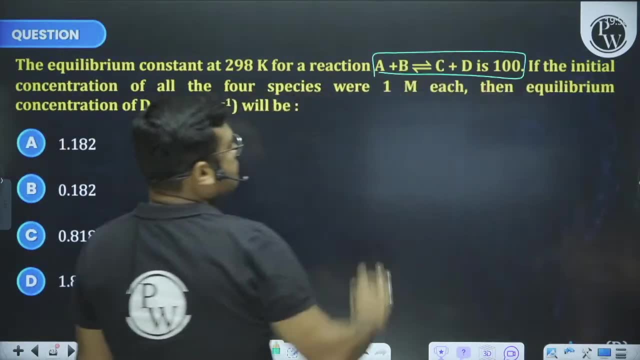 come relatively less those that come. I am explaining to you. now I will talk about a numerical question. I am telling you that too, equilibrium constant at 298 Kelvin for the reaction A plus B gives, C plus D, is 100,. 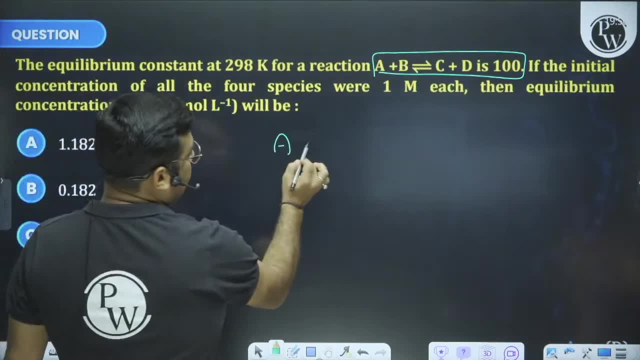 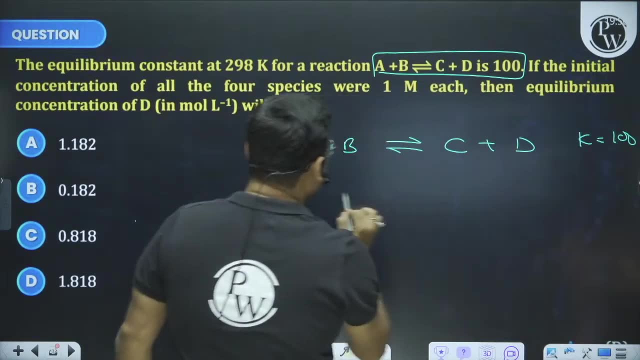 right, if, initial concentration of all four species. if the numerical question comes, then how will we do come? I will tell you that too. its equilibrium constant is 100, now see, son, everyone has one one, one given. 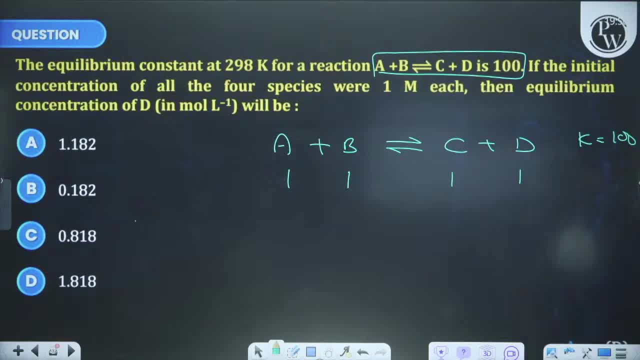 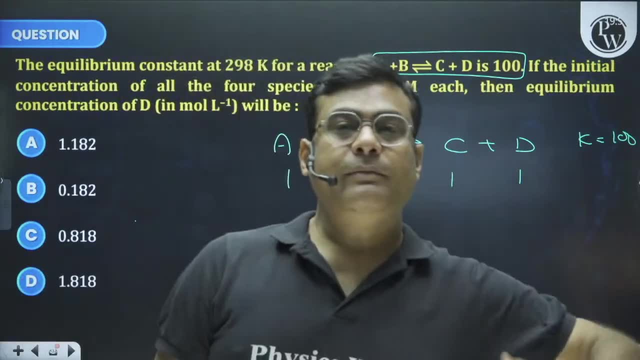 now how to find the direction. so, children of JEE, there is also a packed question on the direction right of JEE. son, how much is your net worth son? my net worth son right now? 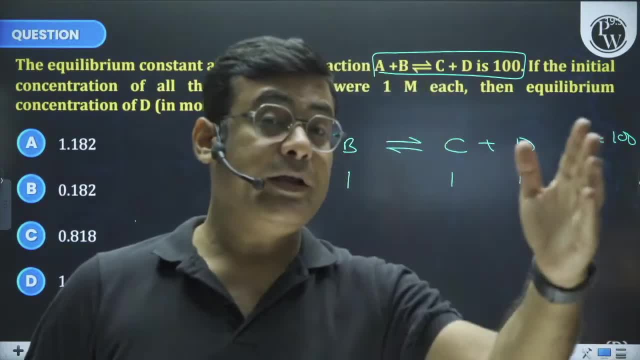 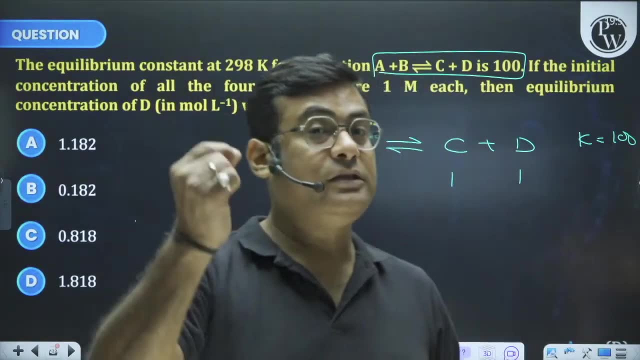 it will be less than what will happen in the next 10 years, because now India's economy is growing very fast and you are such sincere children. you are working so sincerely right? if you have such good doubts, then you will select from All India Rank 1,. 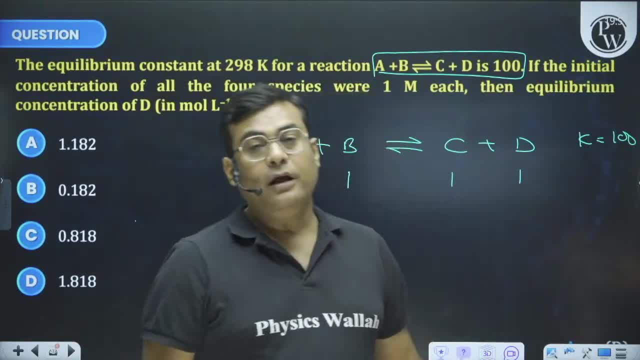 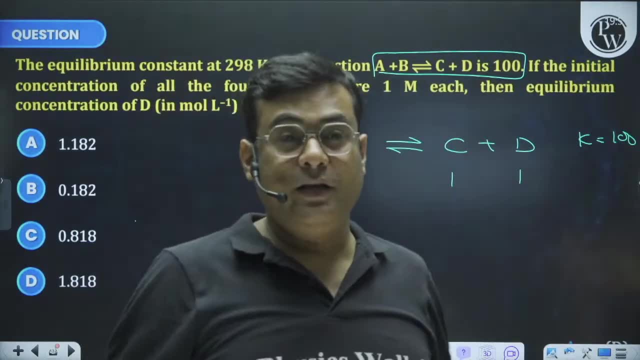 and if you select from All India Rank 1, right, then obviously every institute of the whole world will come to you, right, will try to buy in the beginning. we will give you so much money anyway that you give us your name. 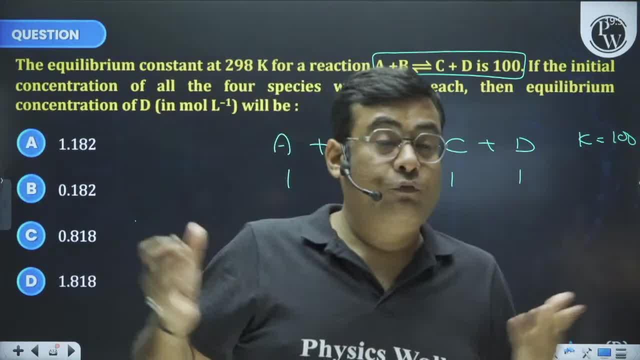 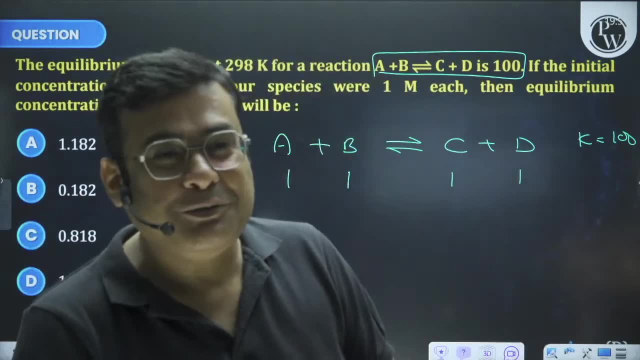 then your net worth will be so much more than the first day right, and then you will make a little bit in IIT. so see how good things, so many things, will be great together. so think how much your net worth will be. 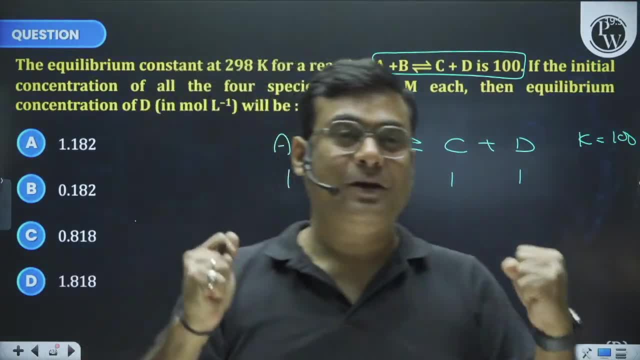 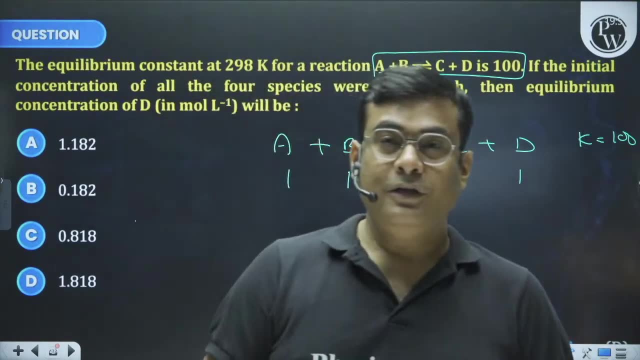 right because you are working so sincerely, you are working so hard. the world is your hard work, right. I had said one very good thing: if you remember that the more you spend on yourself, the more the world will search you on Google. 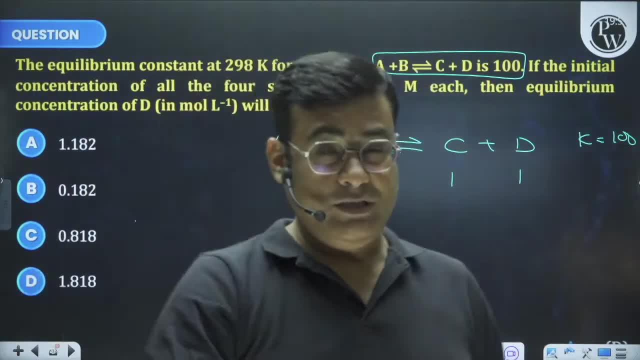 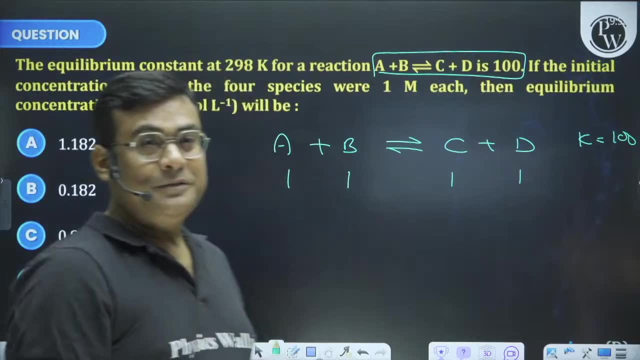 how much fun you are spending on yourself. then, brother, you will have to search the world on Google, whatever happens. how to calculate delta NG son? I had written so lovingly and told you, son, don't be such an enemy. 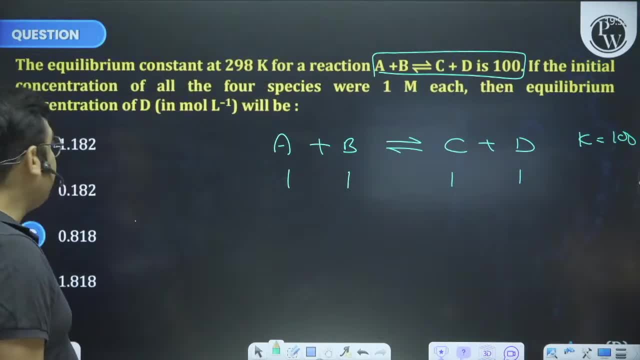 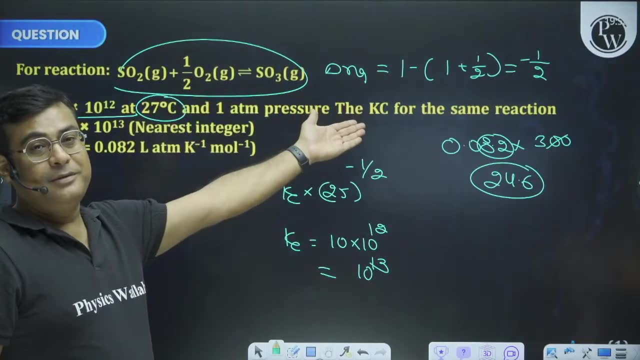 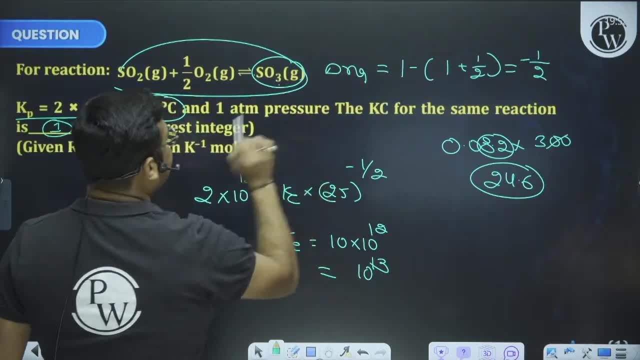 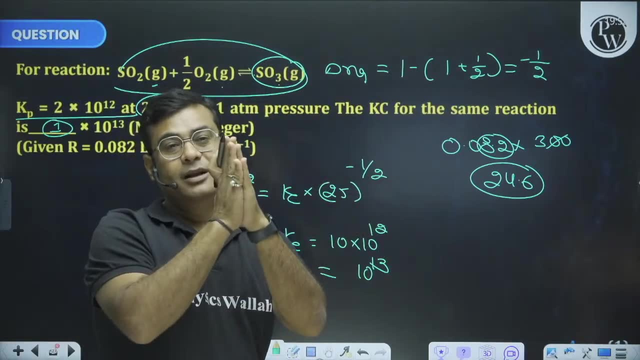 gas's moles. the coefficient of gaseous moles is only one, sir, minus reactant's gaseous moles. SO2's coefficient is one. O2 is half. I had told you so lovingly, my red. 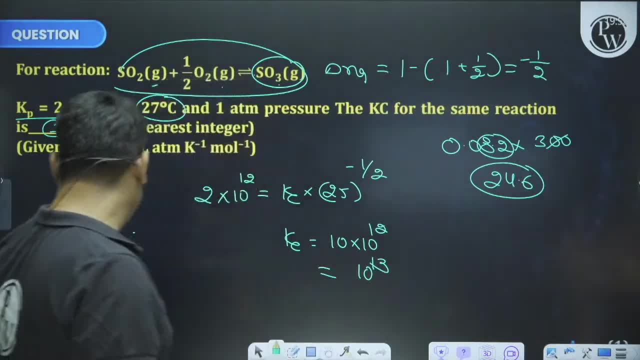 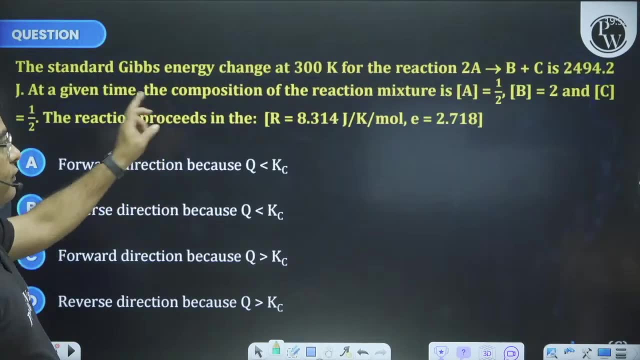 my yellow, my green, my black. yes, right. so I am saying, son, that the question of JEE, this question is also on it. reaction will go in the forward direction, backward, right the question related to it. 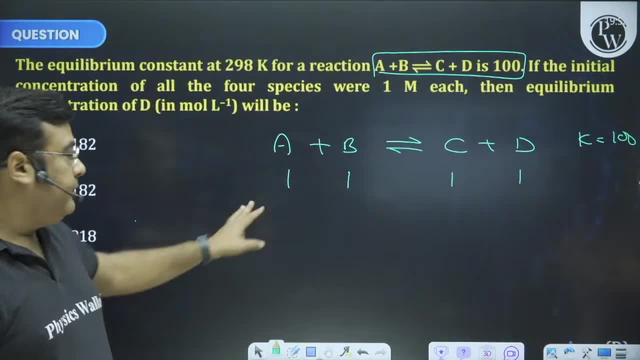 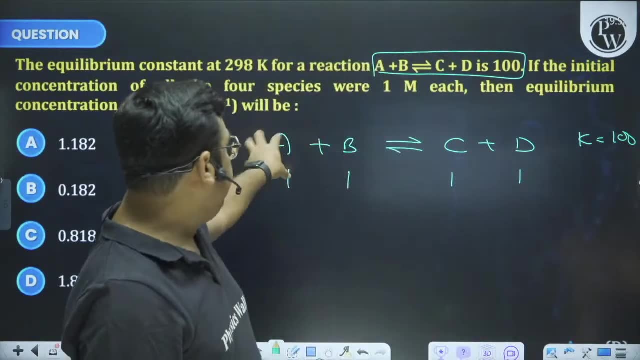 I was getting it done in front of you: A plus B gives C plus D. now how do we know, son, this reaction will go forward or backward, because to go forward, I need A and B. do I have? yes, sir. 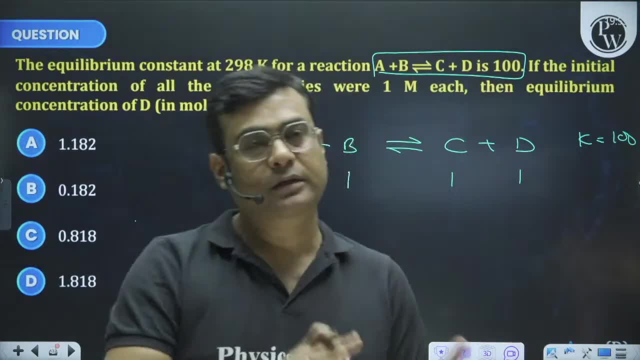 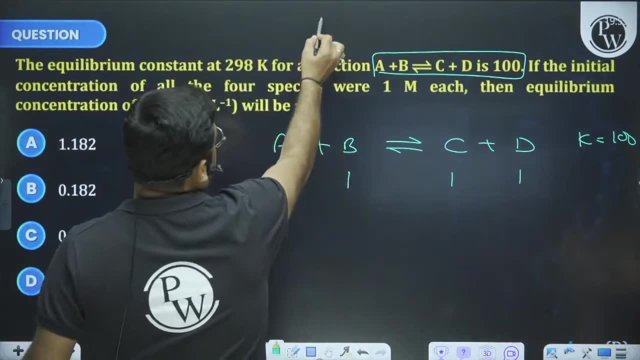 to go backward, I needed C and D. do they also exist? yes, sir, they also exist. so how will I know this reaction will go forward or backward? son, there is a way for this reaction question, and this is the favorite of JEE. 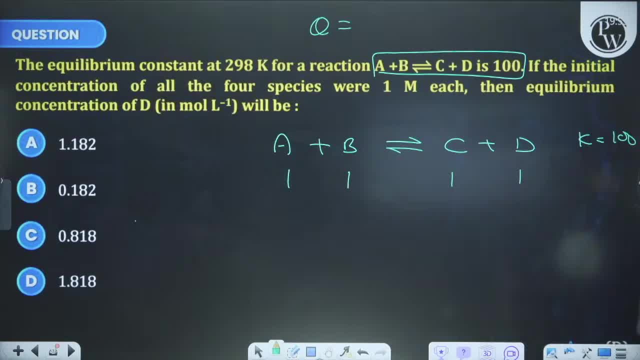 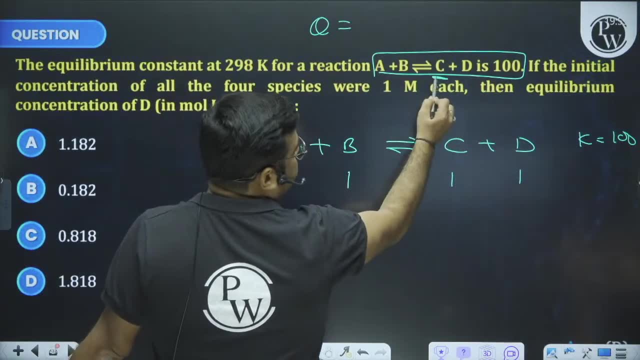 nowadays, all the topics have been closed. ask about reaction question and I hope that you will know how to find the reaction question. the expression of equilibrium constant: write C above, write D above coefficient is 1: 1,. 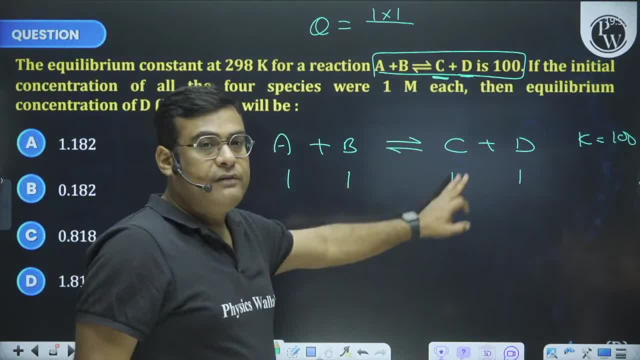 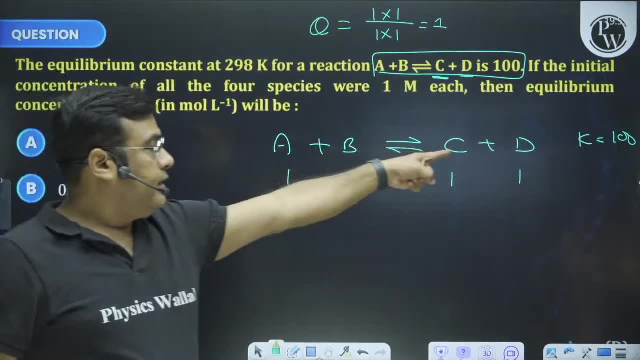 so power will also remain 1, 1,. so brother C is 1, D is also 1, below A is also 1, B is also 1, so reaction question is 1, and if the reaction question right. 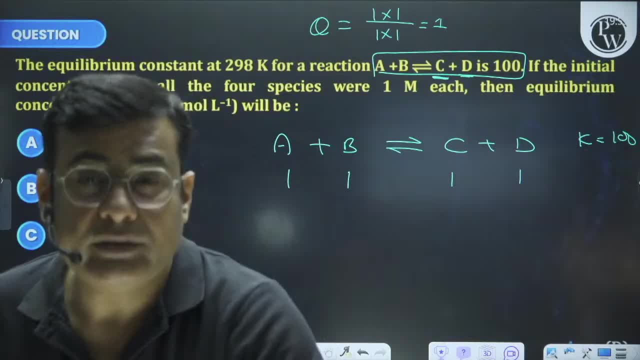 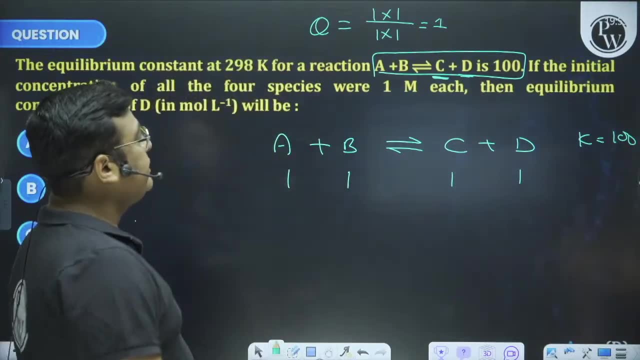 is smaller than equilibrium constant, then we will say: reaction is moving in. in which direction forward? if it comes equal, then we say equilibrium. if it comes big, then in backward, right. so now this reaction because it is smaller than 100,. 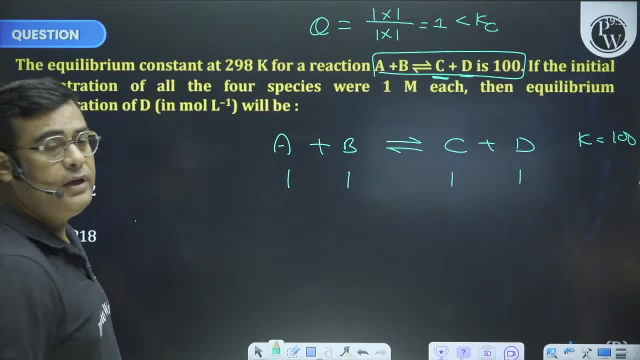 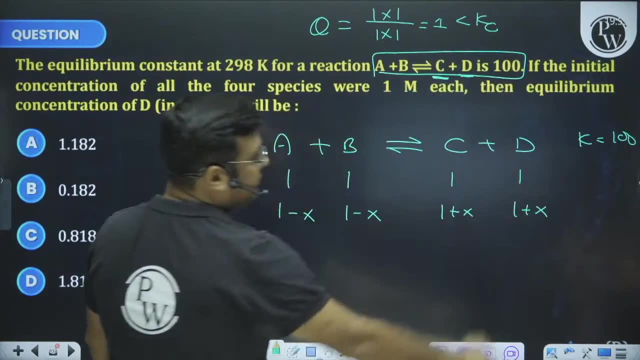 smaller than KC. means this reaction is moving in forward direction. means this will be 1 minus x. this will be 1 minus x. this will be 1 plus x children, and this will also be 1 plus x. 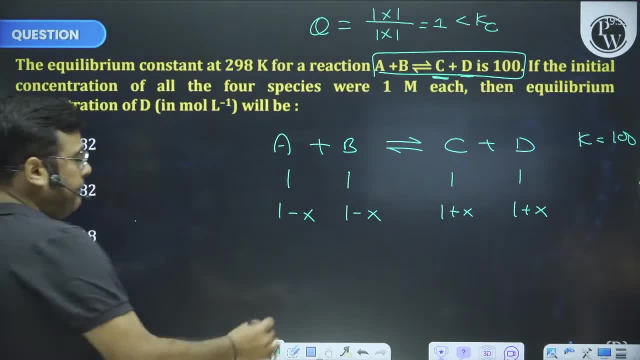 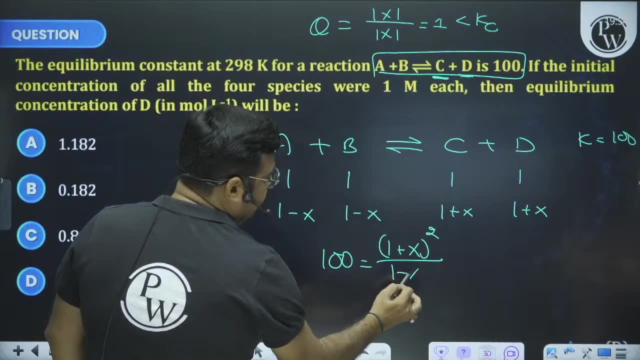 right now, children. 100 equals to 1 plus x. into 1 plus x means whole square of 1 plus x. below: 1 minus x into 1 minus x means whole square of 1 minus x is the square. 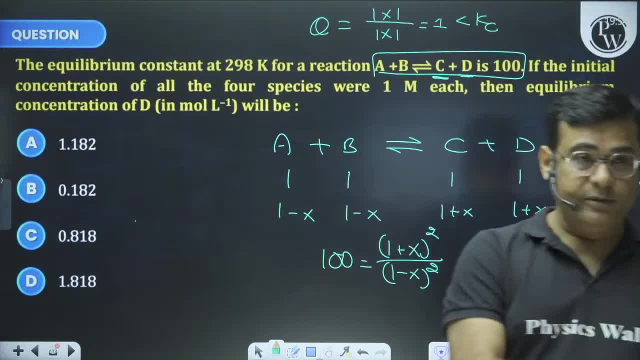 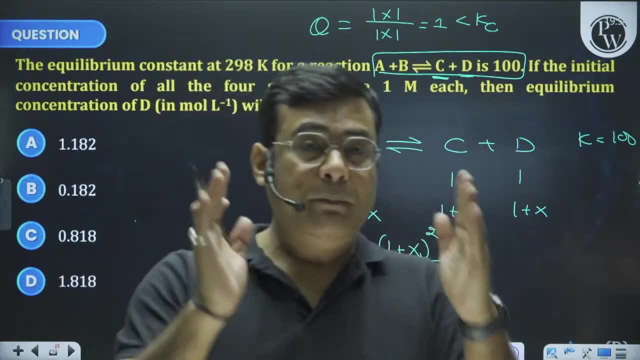 children, be careful, keep it under your attention. children, I am telling this right. children, keep it under your attention. I am telling this: that you feel that the equation is quadratic. many of you children will also give the quadratic. 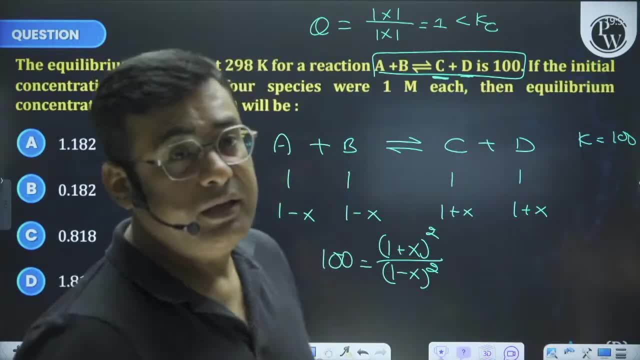 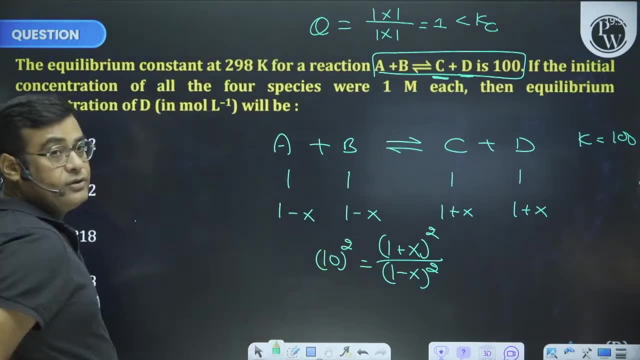 son, but take care for the exam. that 99.99% chance is that he will not give you the quadratic because otherwise it will be lengthy calculation. it will take more time. so the purpose of providing 100,. 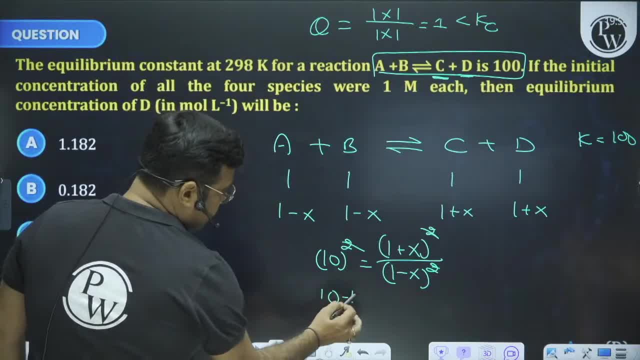 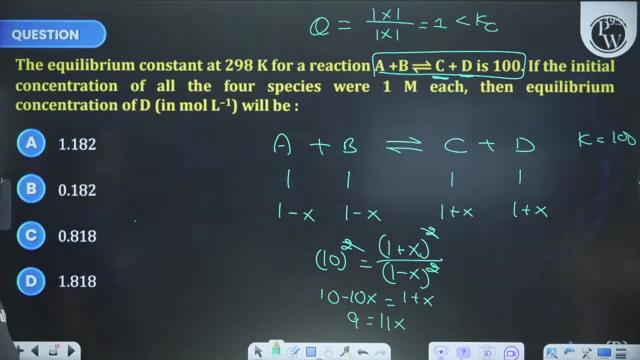 its 10 square right. this you took under root. then 10 minus 10x, 10x equal to 1. plus x means 9 equal to 11x. so x value 9 by 11 means approximately 0.8. 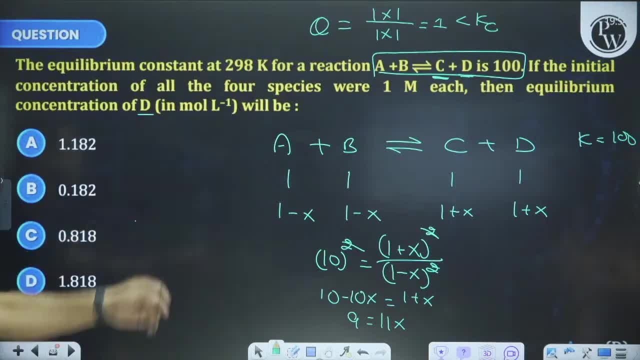 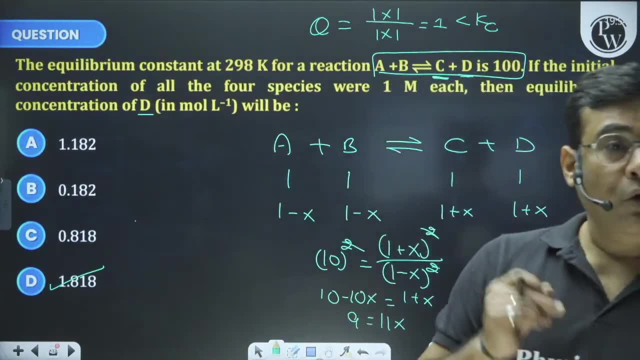 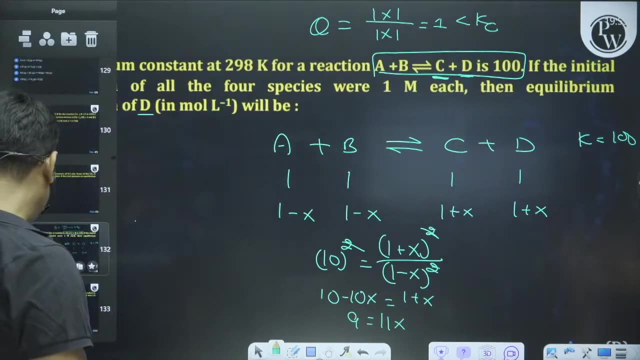 we have been told to tell concentration of D. so 1 plus x means 1.8 something. option is D. so numerical questions can also come. my red and yellow are and you will have to solve them. ok, you will have to solve them. ok. let me tell you one more question. 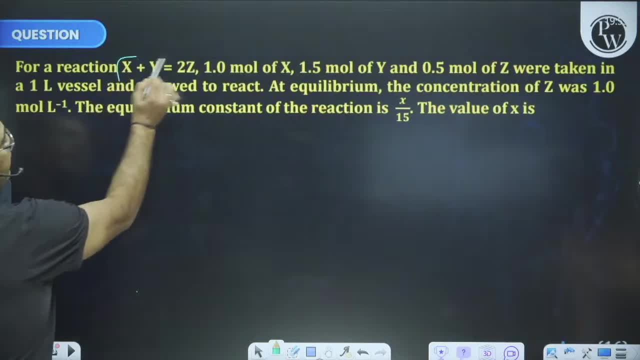 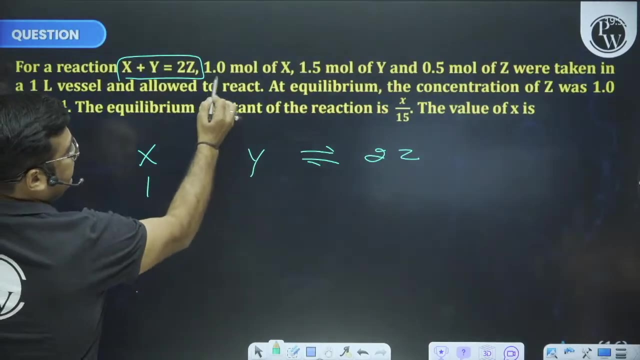 let me tell you one more for a reaction: x plus y gives 2z x. when you also solve it, write it a little far away. you will get a rough copy in the exam. ok, and in that you write it carefully: 1 mole of x, 1.5 mole of y. 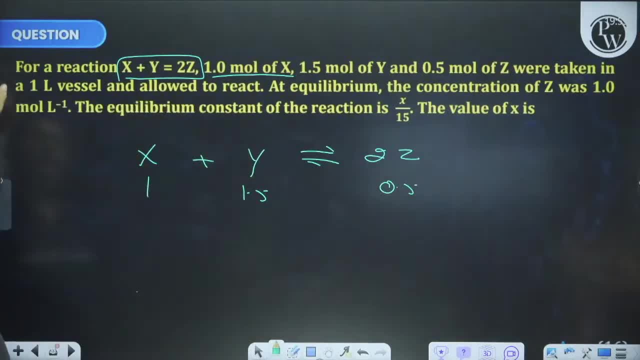 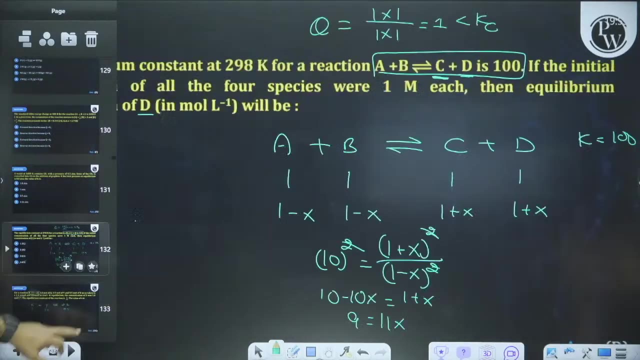 and 0.5 mole of z were taken in 1 liter vessel. volume is 1 liter. no need to worry, because concentration is moles by volume. concentration is moles by volume. concentration is moles by volume. this is the only option. why will you get c? 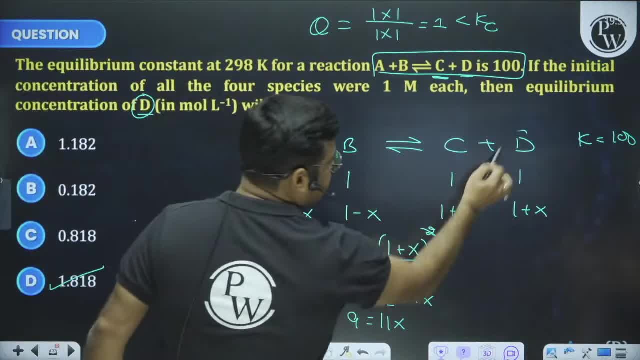 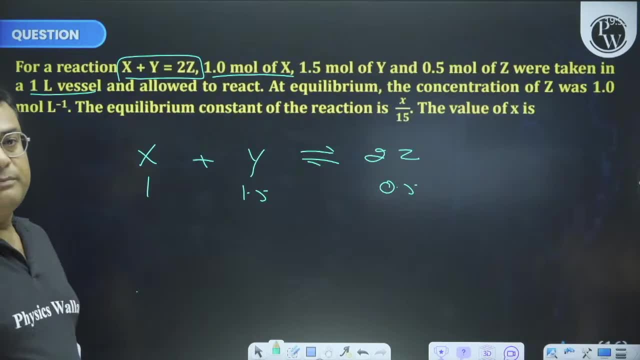 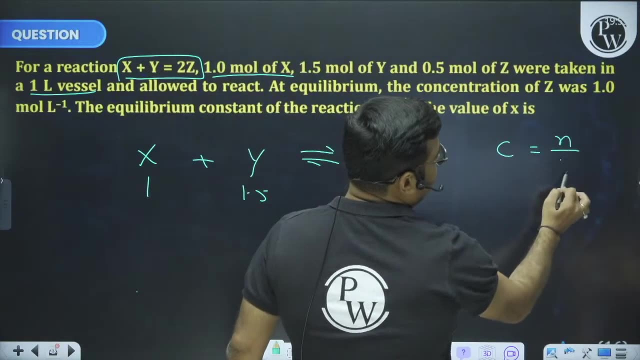 my brother has asked concentration of D. this is 1 plus x at the beginning of everyone's 1, 1 mole. so 1 plus x has 1.0. you have many of you so see. concentration is moles by volume and KC means concentration. 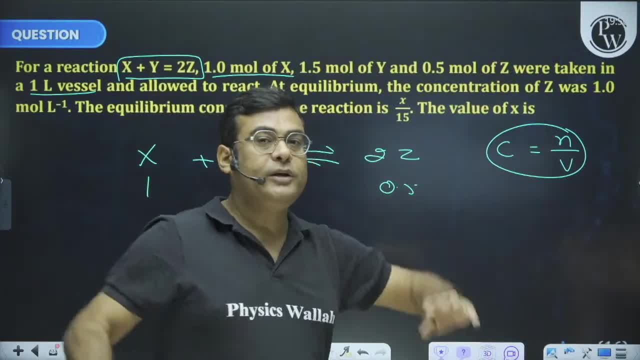 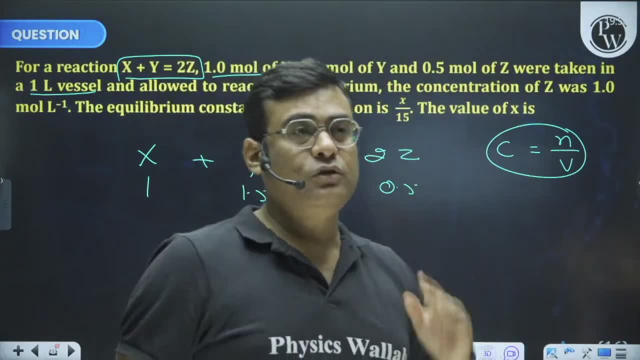 C means concentration, but by having 1 liter volume celebrate happily. Volume 1 liter makes you happy because as soon as volume 1 liter is there, concentration of moles become equal. Now he is saying that at equilibrium, concentration of Z was 1 mole per liter. 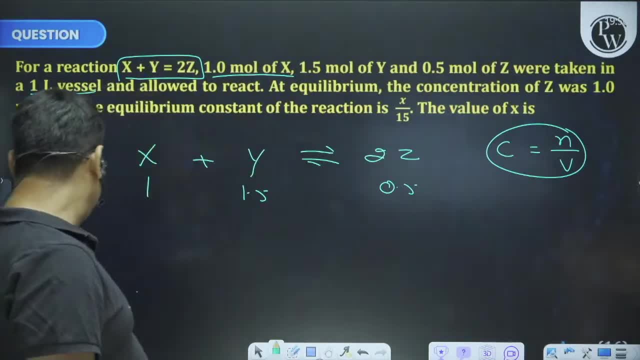 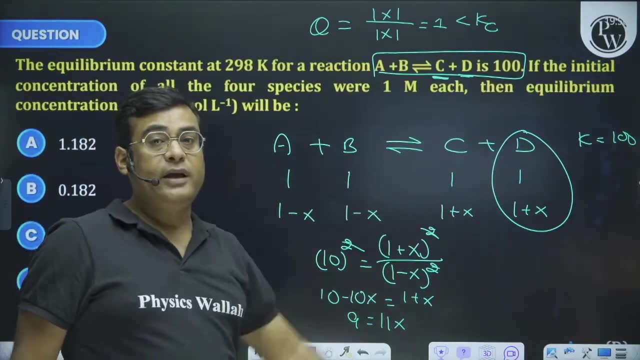 So tell me the equilibrium constant of the reaction. Now, in the previous question, brother, brother, brother, brother, everyone's concentration was given, K was given. Okay, but in this question, initially everyone's concentration is given, K is not given, it is asked in reverse. 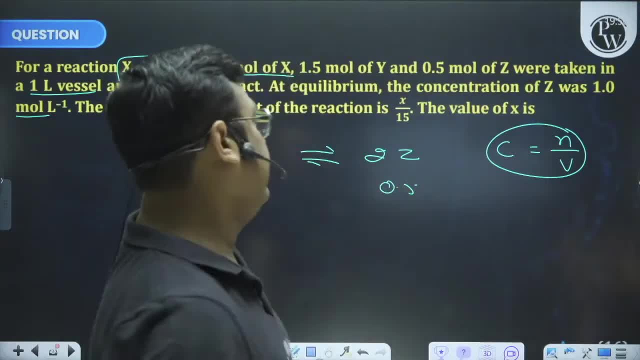 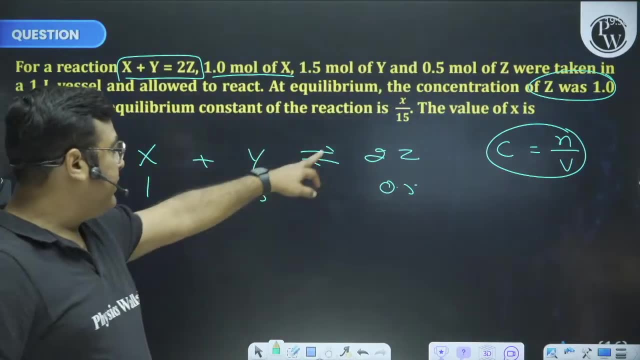 So how to find the direction? how to find the direction, brother? the direction itself is given in the question, my dear children. He said that the concentration of Z has become 1.. In the beginning the concentration of Z is 0.5, so you have to take the mole concept first. 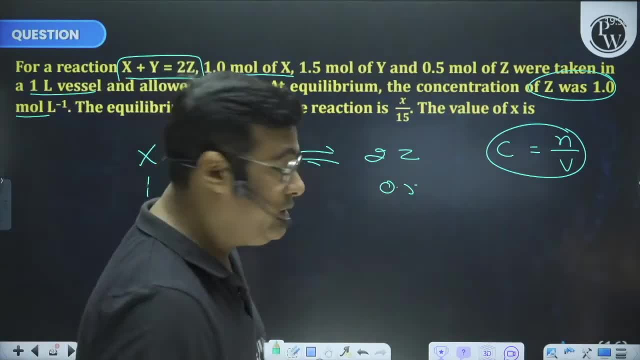 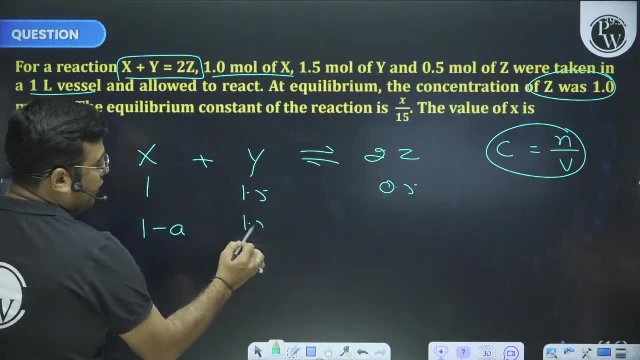 And he said that the need for the mole can be found in chemical equilibrium and kinetics. You have to write 1 minus X instead of X. write A, because X is written 1.5 minus A and 2 Z, So you have to write it. 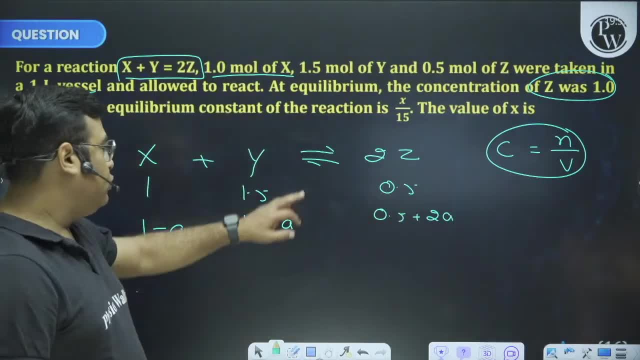 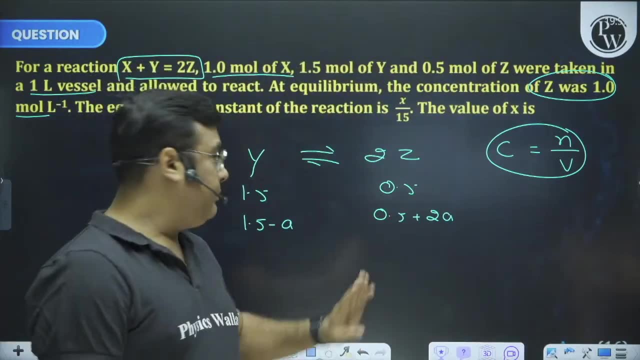 1.5 plus 2A In the mole, because in the beginning we were considering Z to be 0, right, But I am giving a break. I will take 2-4 minutes more 5 minutes. I am giving a break. 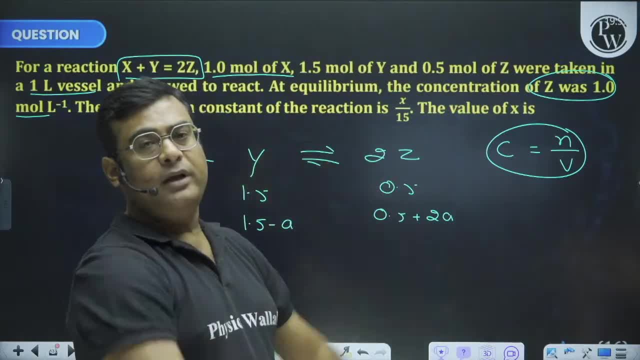 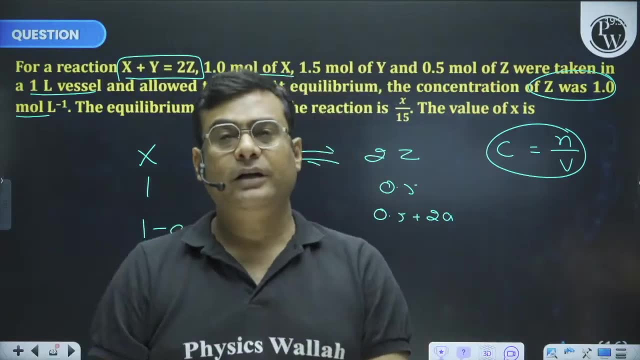 I also need some energy, Although I am getting energy from your heart, from the pole, from the like, But at least there is a dinner time. a little energy goes away. So then it will be fun to take 2-3 hours more session. 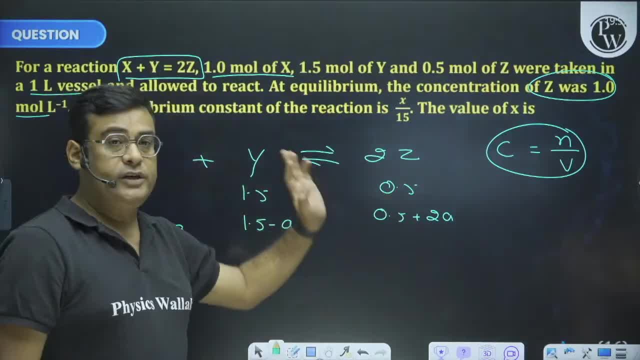 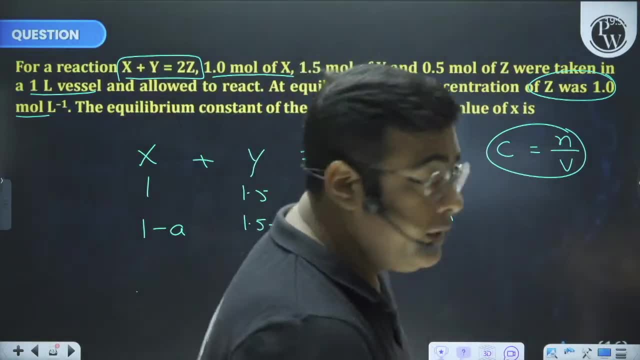 Okay, so this 0.5 plus 2A, whatever is the coefficient In the mole, normally the product is 0. But in chemical equilibrium it is not necessary that it gives you 0. Here 0.5 is given. 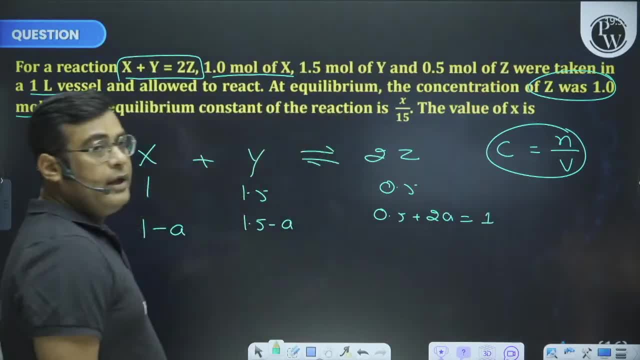 Now the value of this 0.5 plus 2A is 1.. So it means that the value of A has become: Now listen to my calculation trick. here Means the value of A has become Children. how much, Sir? 0.25.. 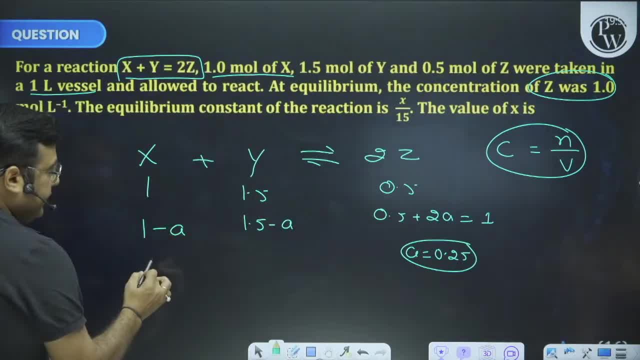 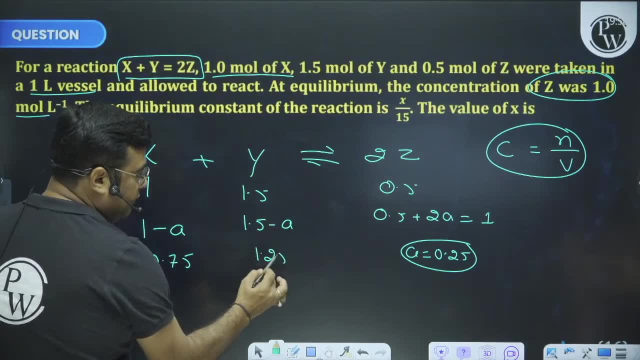 Hasn't it come? Yes, sir. Now see 1 minus A. So 1 minus 0.25 means 0.75.. 1.5 minus A, So 1.5 minus 0.25 means 1.25.. 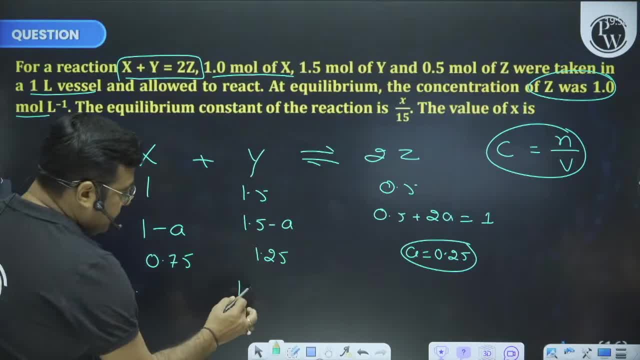 And this is 1.. Now take out the equilibrium constant Kc, Because the volume is 1 litre. so it is a good thing. So the square of Z, sir, the square of 1.. Upon Upon, Sir, the concentration of X is 0.75.. 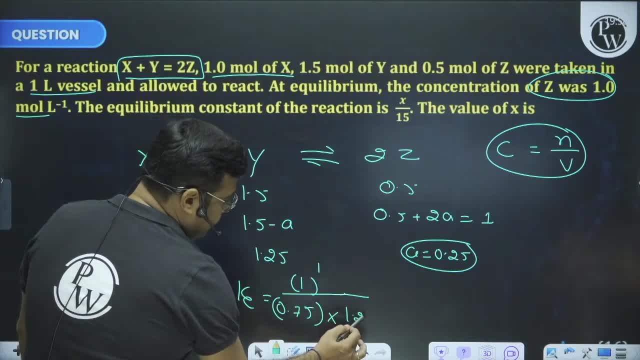 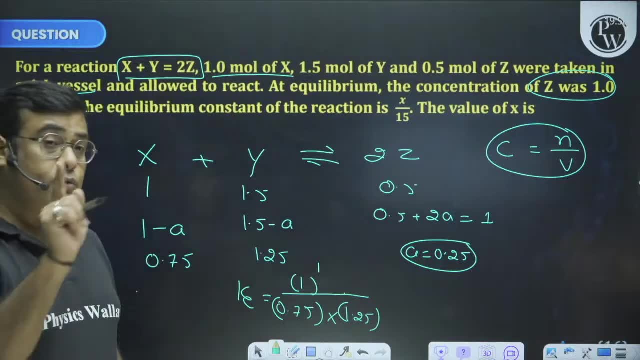 Into the concentration of Y is 1.25.. Now listen to me, son. If you are listening with your heart, then there should be 500 likes on this. If you are listening with your heart, listen, See. he said the equilibrium constant of the reaction is x by 15.. 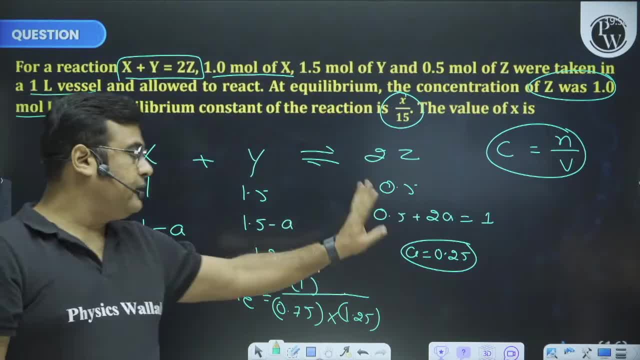 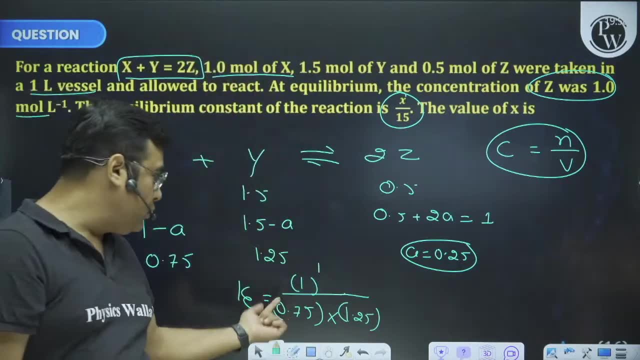 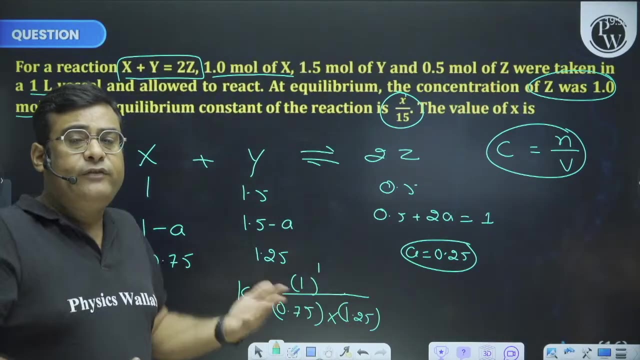 So tell me the value of X Now. I hope everyone has understood by now. Now you have as much strength as you have, son. Put the strength of your grandparents First. multiply these two numbers Right. First multiply these two numbers. Then put it in the terms of x by 15.. 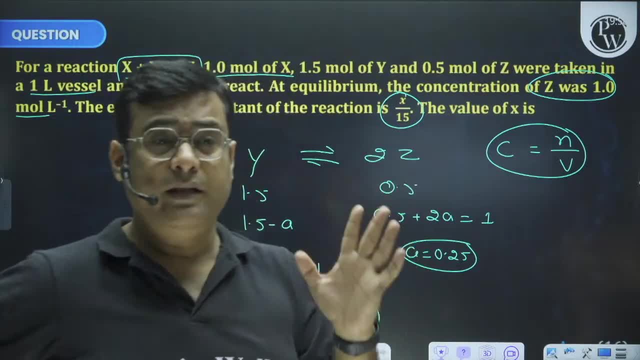 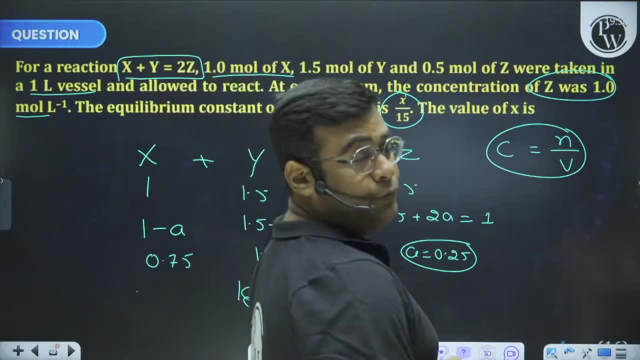 Do it and show it Right. Do it and show it. You will come under my shelter. Write the slogan once After understanding Hirwani Baba Sharanam Gacchami. This was my slogan of UCC 2.0.. 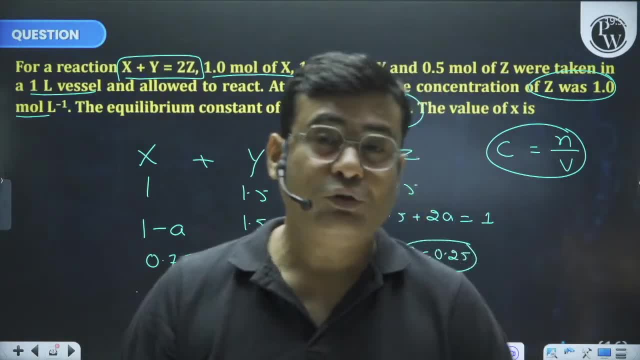 This was the slogan of Ultimate Crash Course 2.0. Right. This was the slogan of UCC 2.0. Right. The children had given it Hirwani Baba, Sharanam Gacchami, Right. So listen. 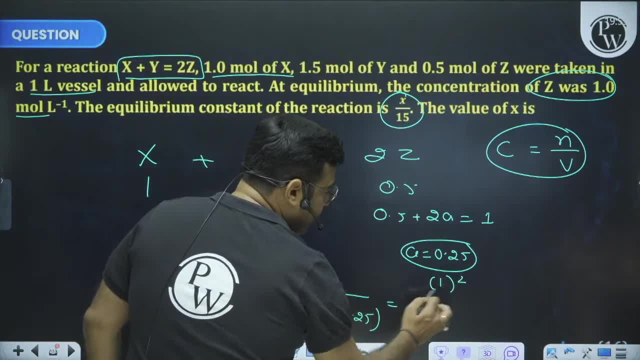 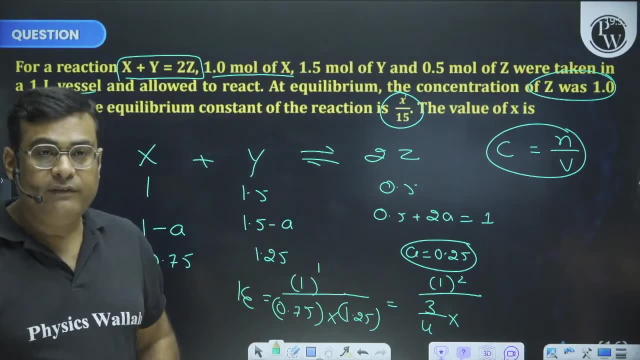 I had just said, son, if 0.75 comes anywhere, then write 3 by 4.. Right, If 1.25 comes anywhere, write 1 plus 0.25.. And what is 0.25?, Sir? 1 by 4.. 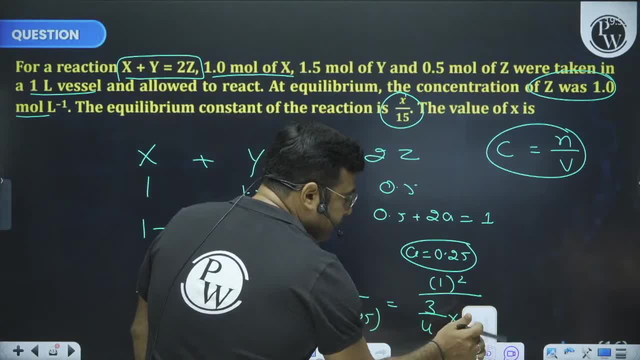 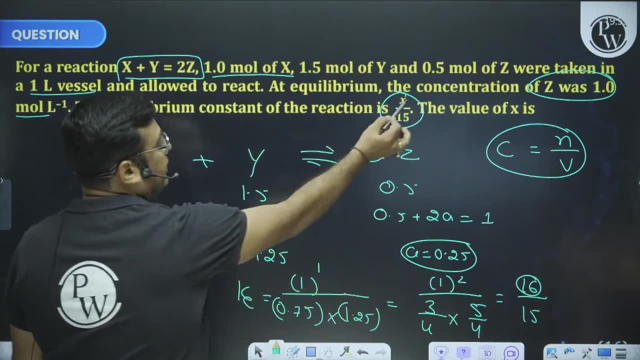 So 1 plus 1 by 4 means 5 by 4.. Right, 4 by 4 or 16 goes up, 3 by 5 or 15 goes down. He has made this x, And the value of x is 16.. 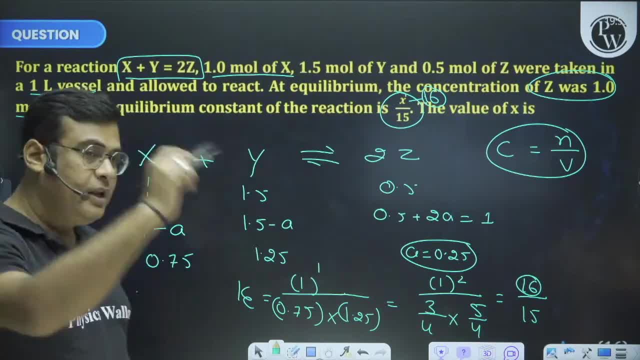 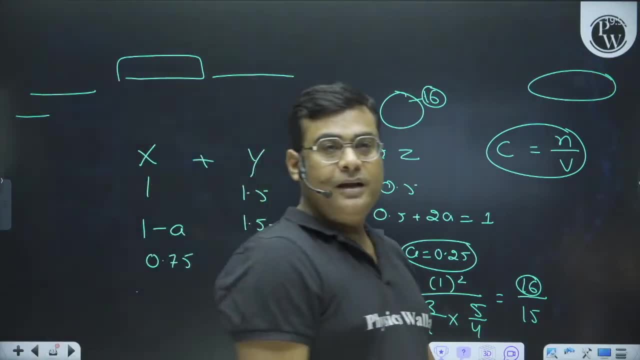 You can clap on this son, Or whatever I said. write in Hirwani Baba Sharanam Gacchami, Because if you did not follow my technique, Right, If you did not follow, then think how you solve this question. 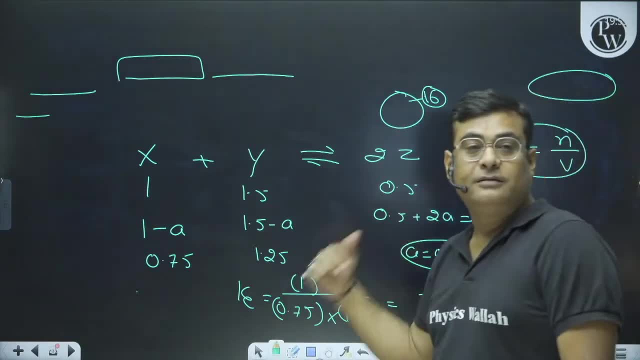 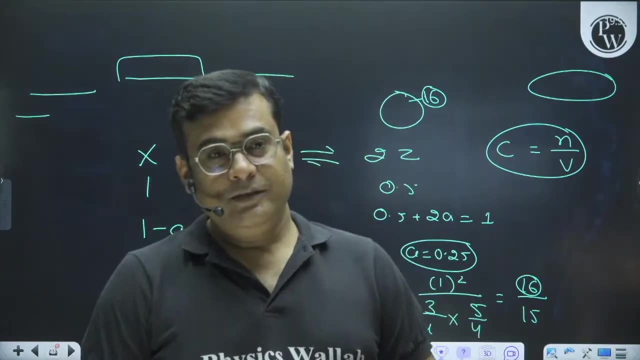 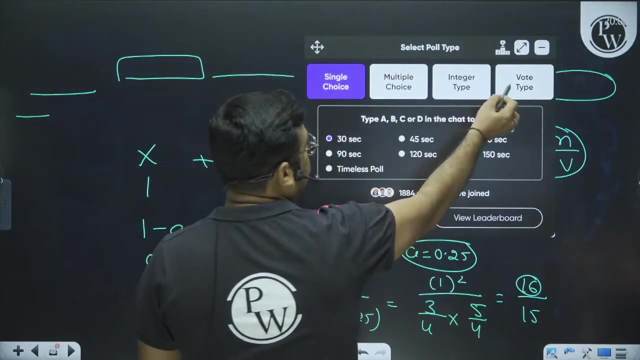 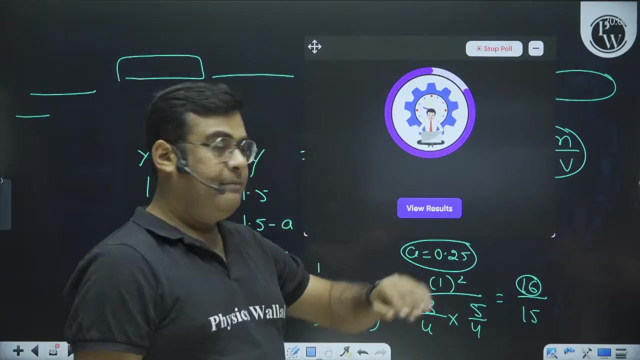 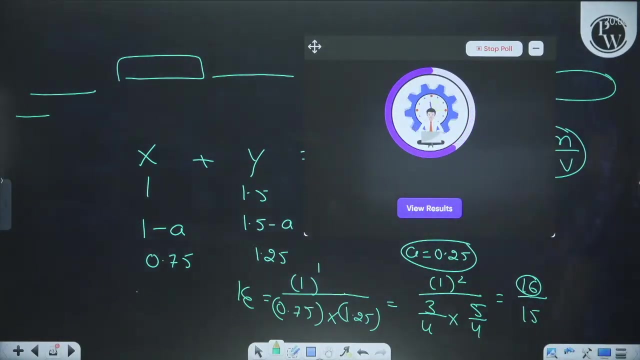 And if you understood my technique, then from what speed have we knocked out the answer? From what speed have we knocked out the answer? Right, I know you won't give me 100% pole, but there is one last pole break. let's take a break of about 20 minutes. I also bring a little energy, but it's 8 o'clock. I had promised a break. there is nothing more to understand in this chemical equilibrium than this. I have explained as much as there was. give me 100% pole, then my heart will be happy. 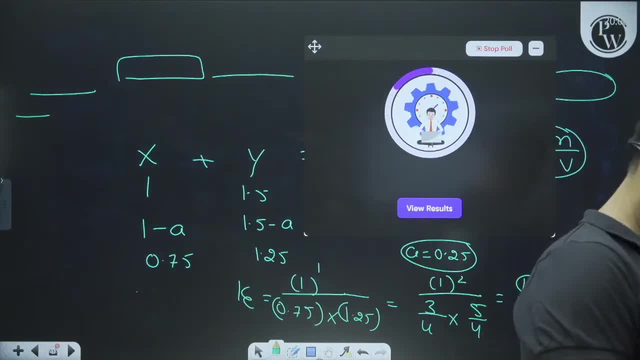 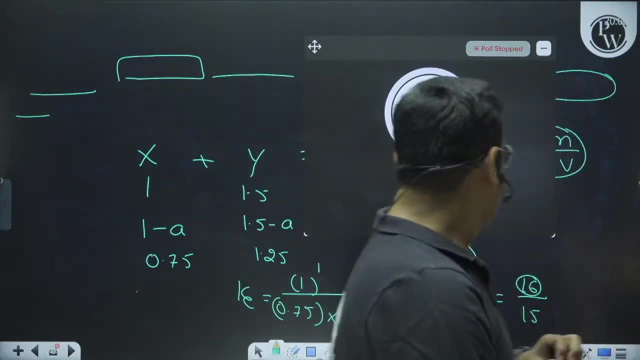 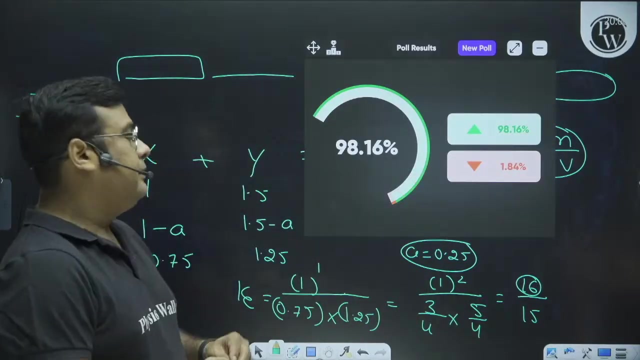 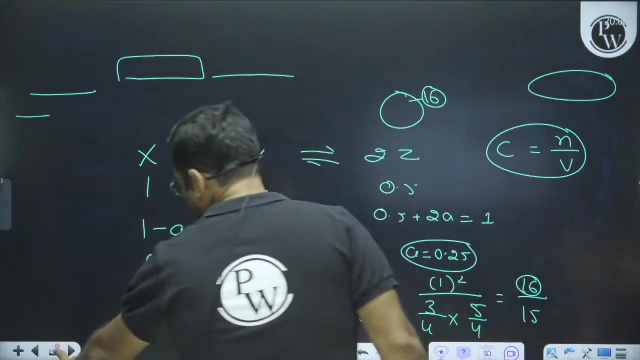 So in this exam, you think that the calculation comes dirty. it doesn't come. I haven't seen it. it won't come. it won't come. it's again a good figure. thank you very much. okay, so the calculation doesn't come dirty. I am just telling you this much. remove the fear of it, because now you know everything. son, I told you a quick review. 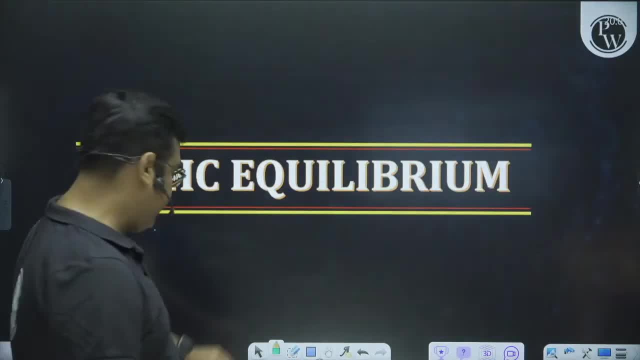 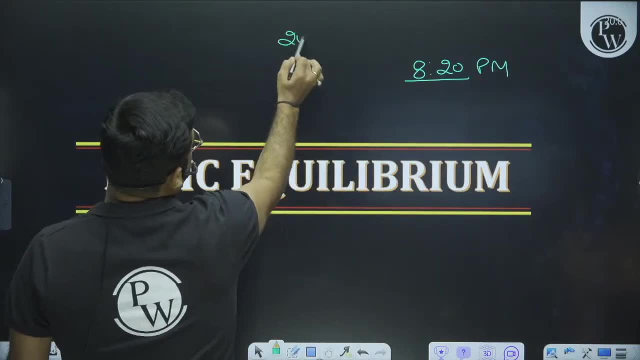 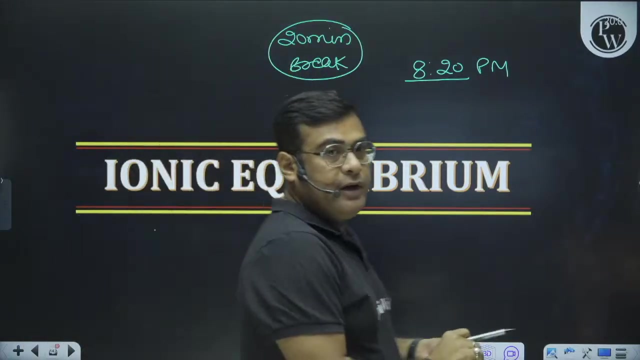 I am coming to do a quick revision, so we are now in the ionic equilibrium. after the break, it's 8 o'clock, it's 8.20 pm, which means I am giving you a break of 20 minutes. 20 minute break. it's a 20 minute break. we will meet at 8.20,. you will also have a little fun, right, you will also be sitting and eating popcorn. you will be having fun, but I am not eating anything, so I need a little break now, right? okay, 20 minutes. 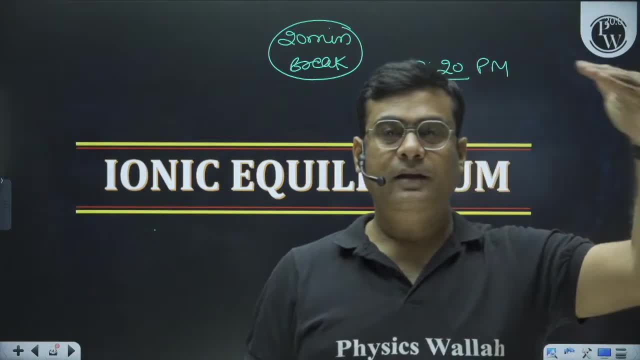 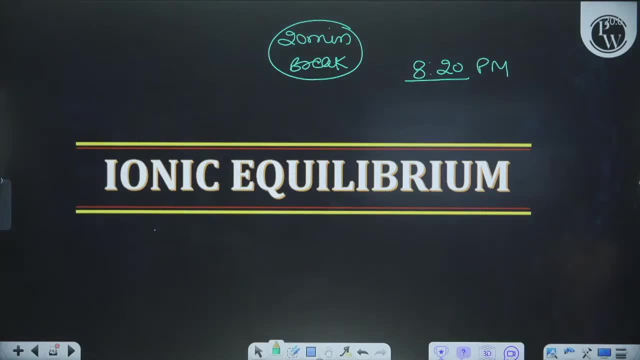 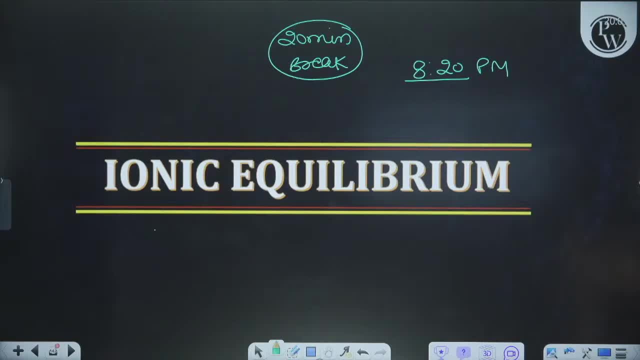 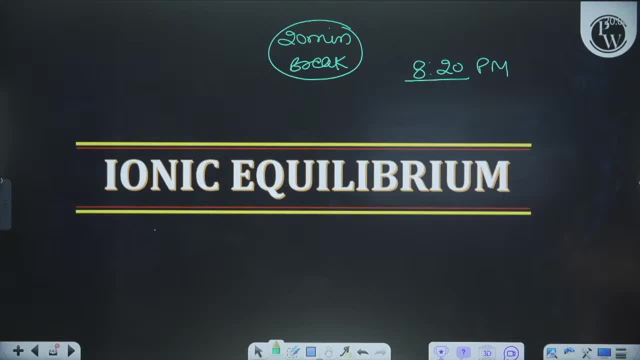 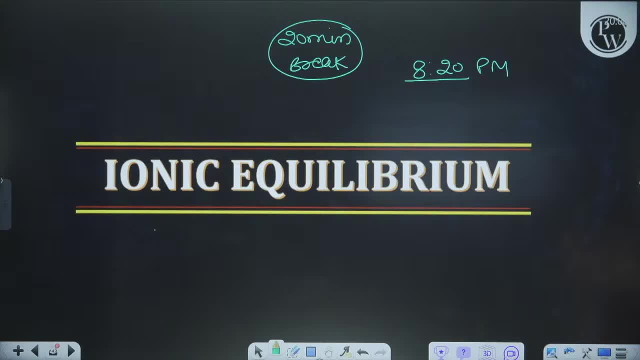 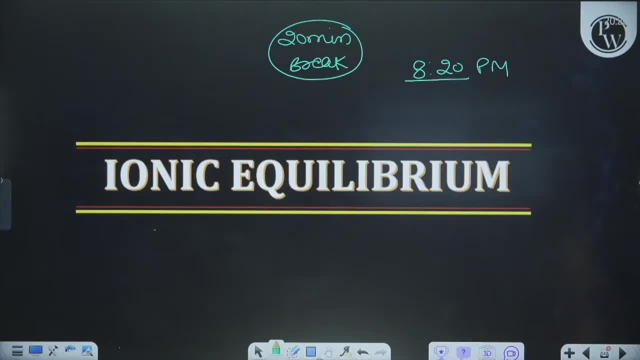 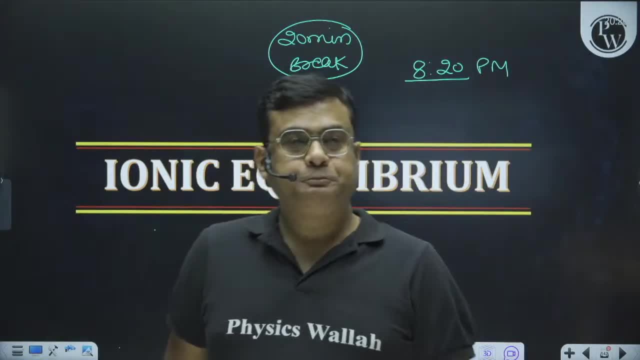 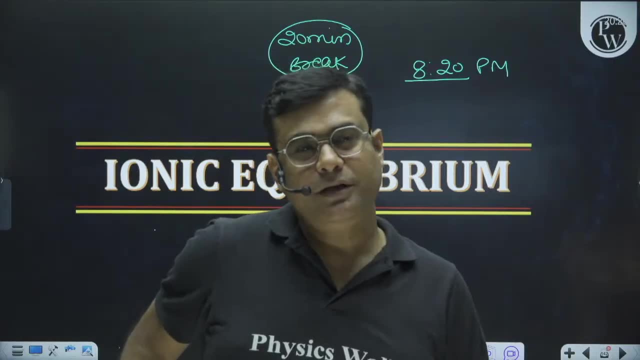 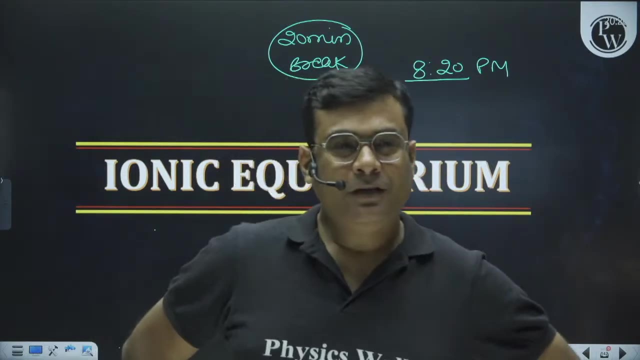 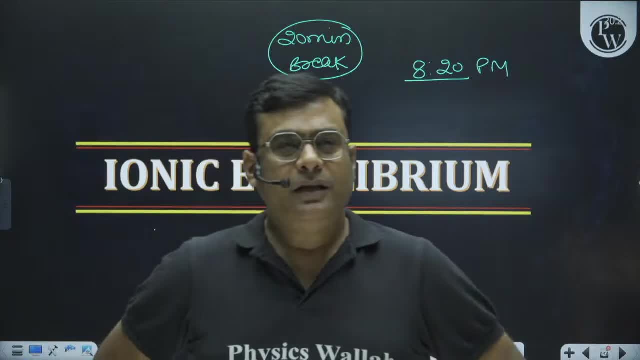 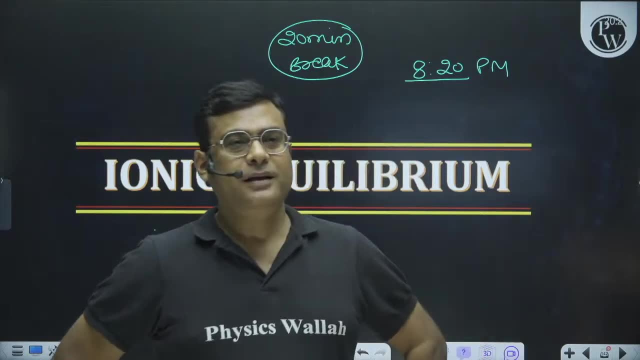 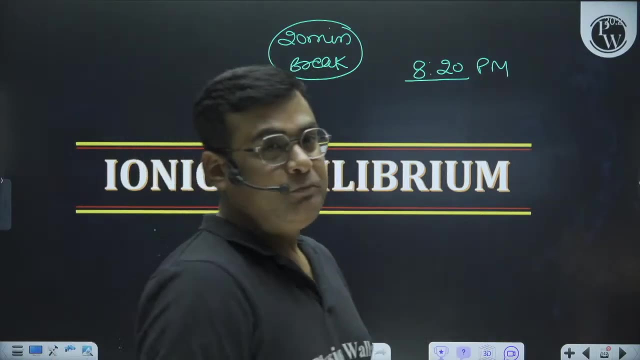 Jaate, jaate. ye toh bata ja hum jiyenge iske liye Chai piyoge beta aayi toh jaroor piyonga chai Chalo ji jaldi se aajayi ab hum aayinik or electro ke concepts ko. 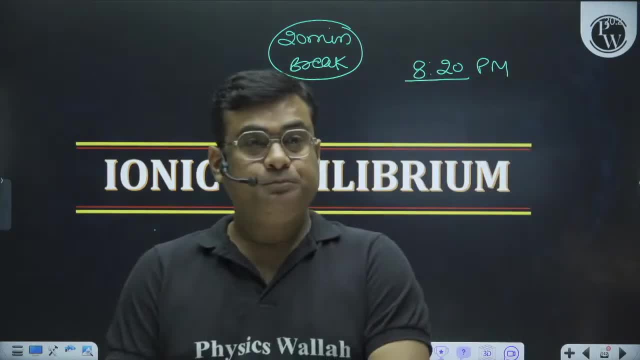 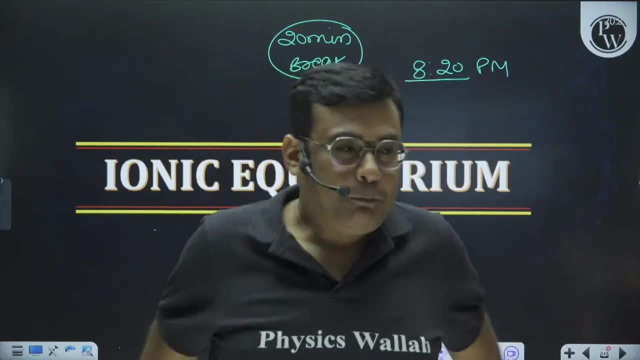 Usme kya, kya hamare paas khazane hai, Sir, aapka naam batao. sir, please, bitta naam hai, hi nahi mera. kuch bhi Be naam huye, toh kya hua naam nahi hua kya. 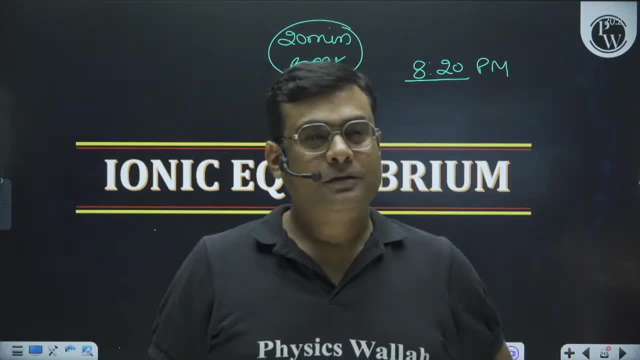 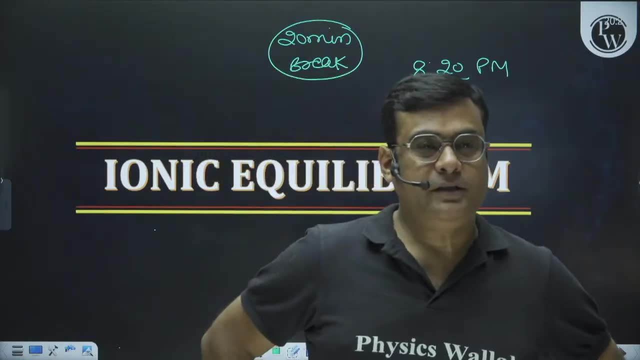 Jalgaon ko kiska center, koon ta Chalo ji aajayi bitta, jaldi se aajayi, jaldi se aajayi. I hope aapne bhi hai na energy le li hogi ab. 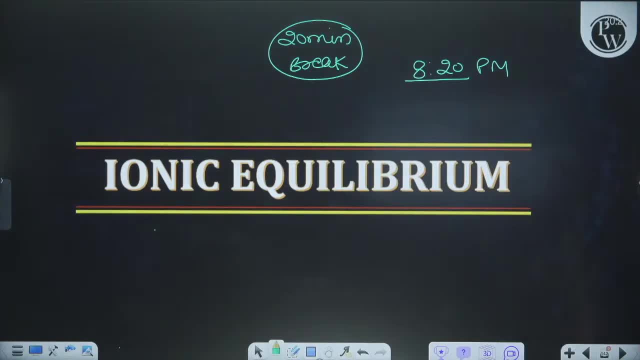 Aur ab hum hamare Chalak Agare Padao ki taraf Sounds like Chalek Angle padao ki taraf. chalek Jhc ka full form boli: ye jara hut ke concept. bitta jo kuch unique concepts maa abko de raha hu. 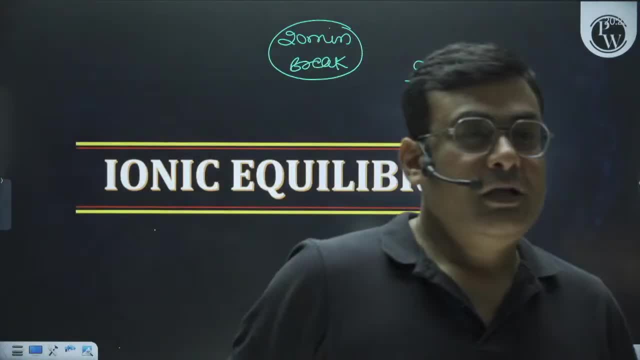 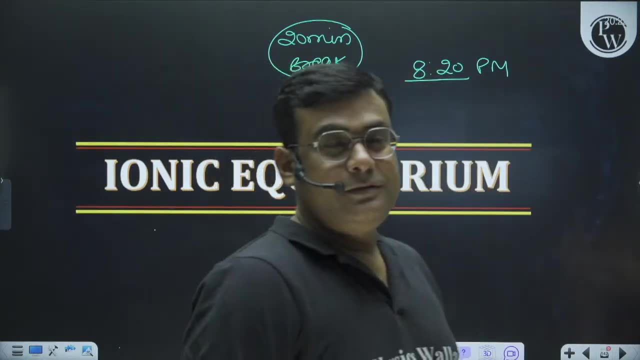 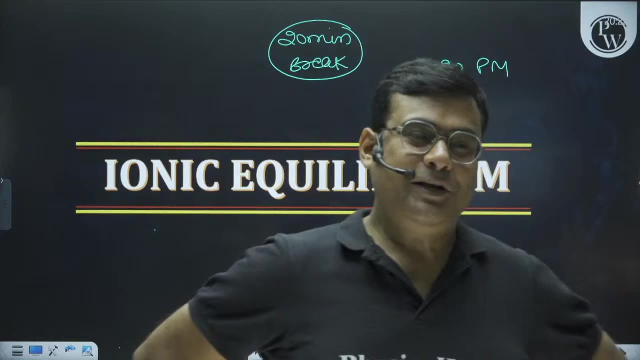 Na UCC 2.2 se humare kaapi batchaa aagay hain RCB. kya hai nanja Jitendra Shraganam Gacchami to listen better? please leak the paper. the whole paper is getting leaked. 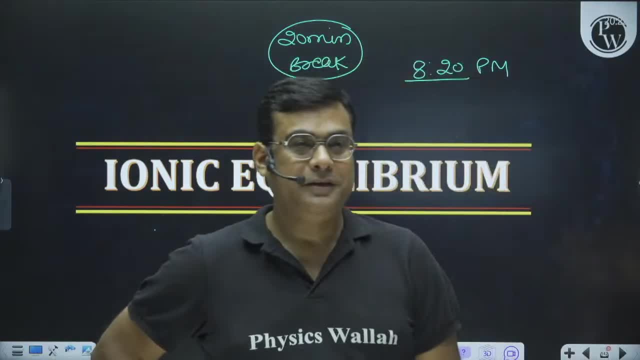 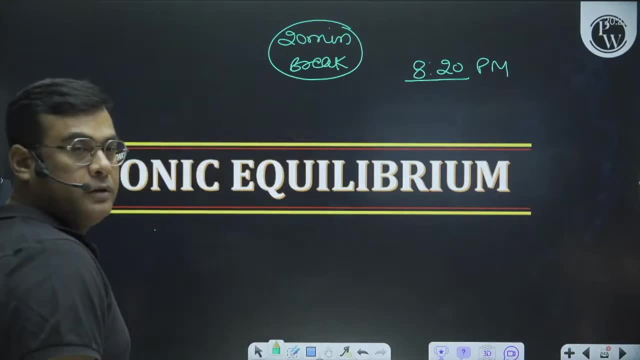 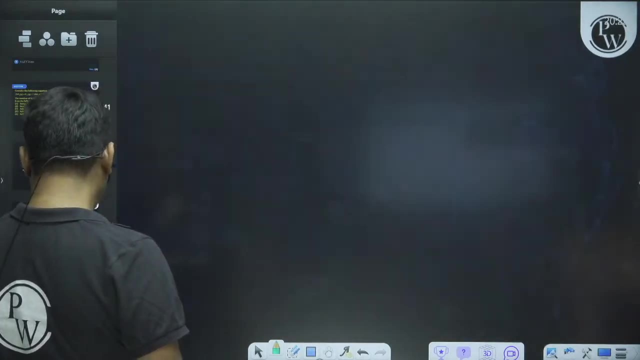 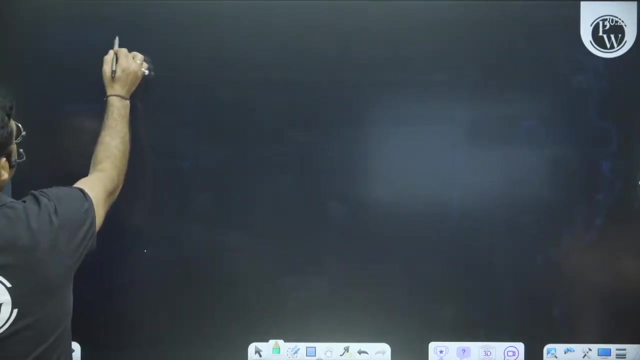 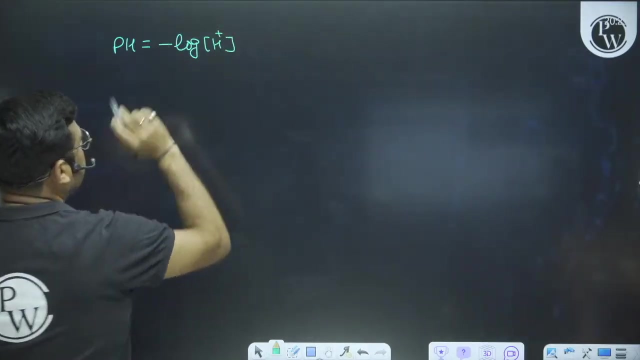 this whole paper is getting leaked, ok, ok, so now we will move on to Ionic equilibrium. first I will tell you some key concepts in Ionic equilibrium. first question you will get on pH. and pH is minus of log concentration of H plus. ok, H plus and pH are inversely proportional. 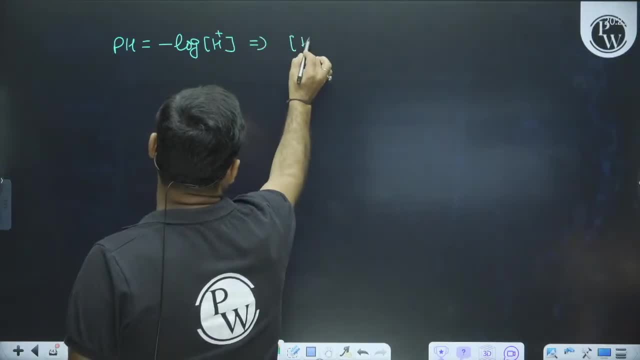 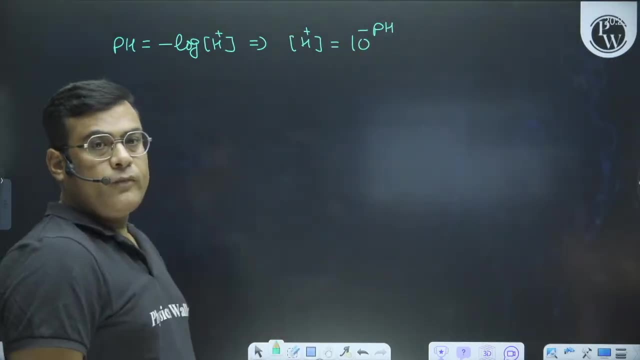 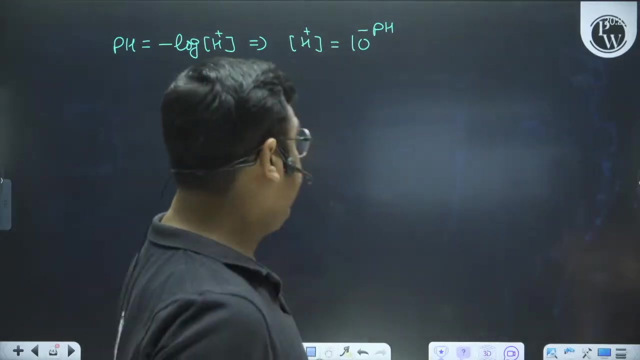 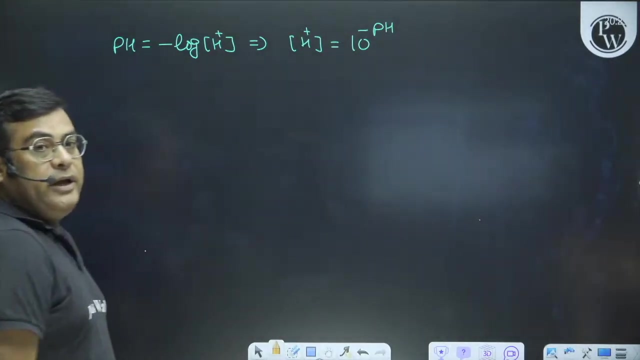 to each other. let me tell you: I can write concentration of H plus as 10 to the power minus pH concentration of H plus. so I can write 10 to the power minus pH. ok, so from here we will learn many times that pH and H plus. 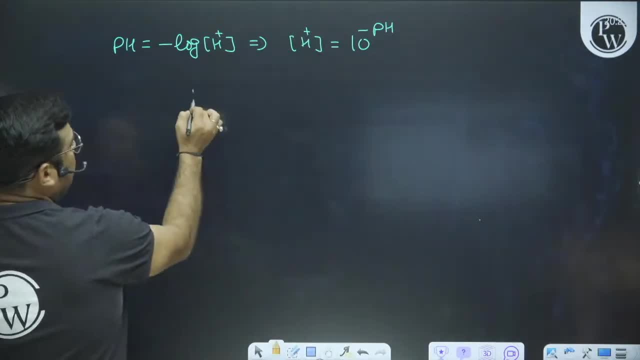 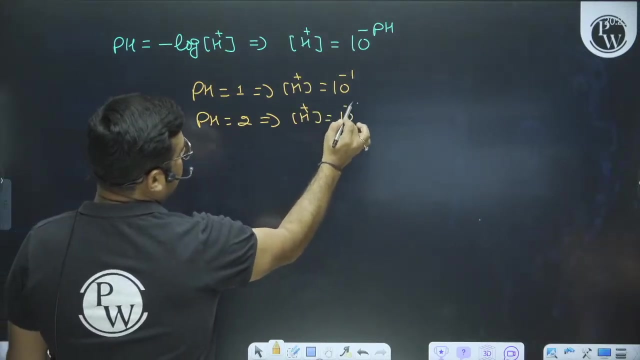 are inversely proportional. if I am telling you that pH is 1, then you will say: concentration of H plus is 10 to the power minus 2. if I am telling you that pH is 1, then you will say: concentration of H plus is 10 to the power. 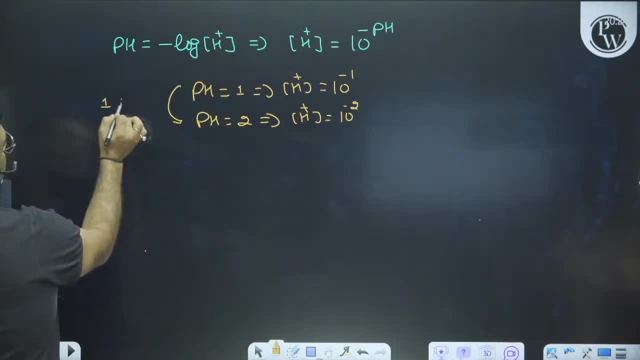 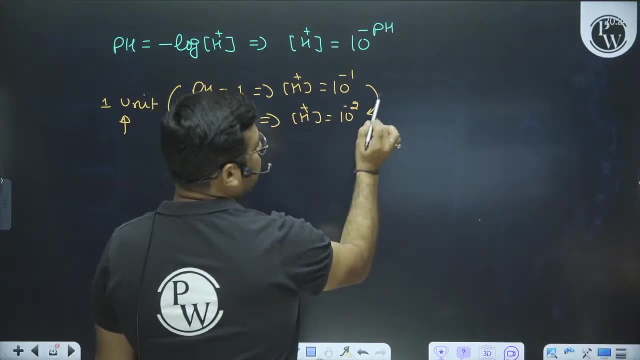 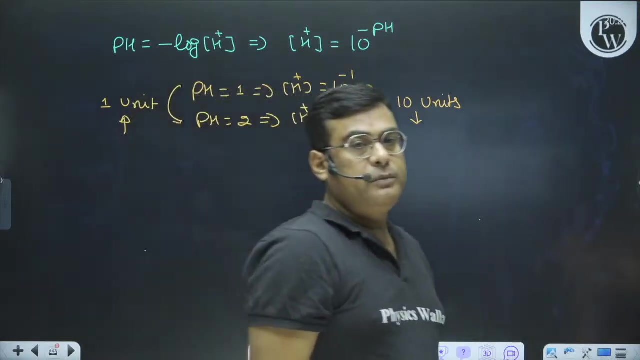 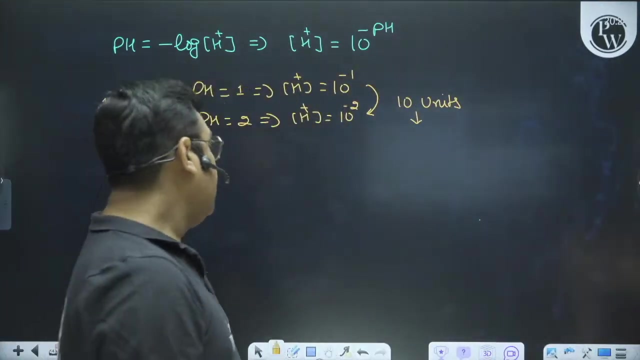 minus 2. ok, if I am telling you that pH is 1, then you will say: concentration of H plus is 10 to the power minus 2. if I am telling you that pH is 1, then you will say: concentration of H plus is 10 to the power. 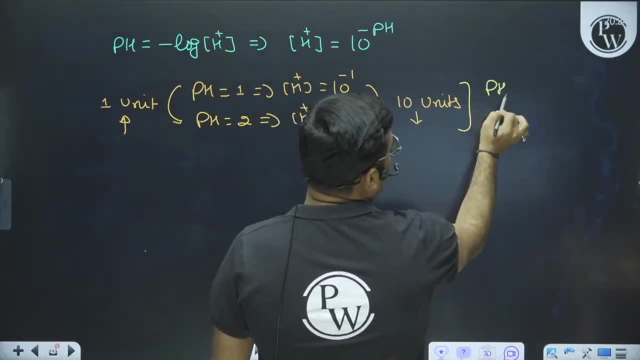 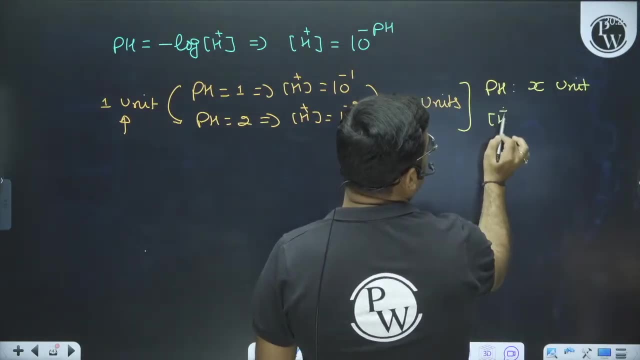 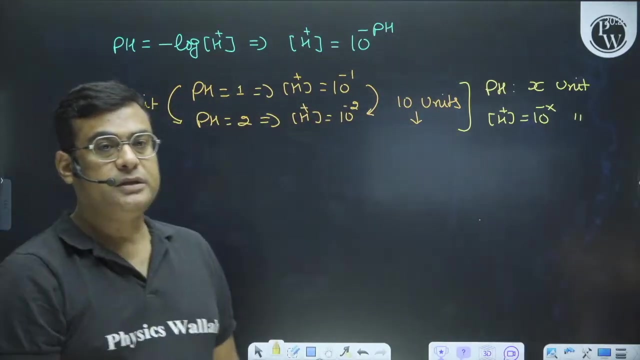 minus 2. if I am telling you that pH is 1, then you will say: concentration of H plus is 10 to the power, minus 2. ok, so this is the first lesson you have to keep in mind. so this is the first lesson you have to keep in mind. 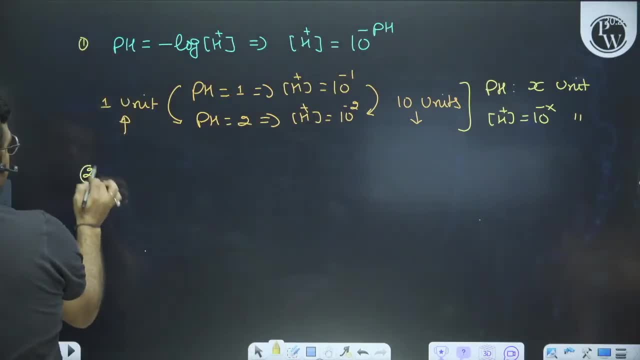 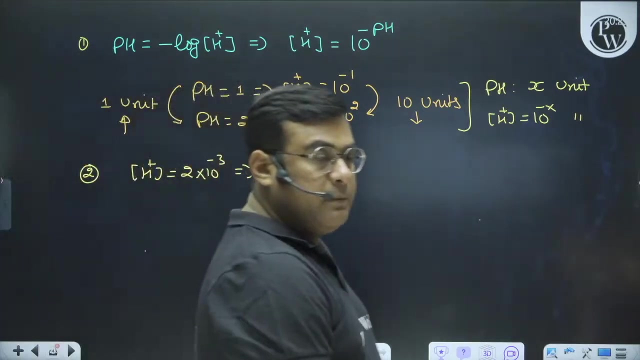 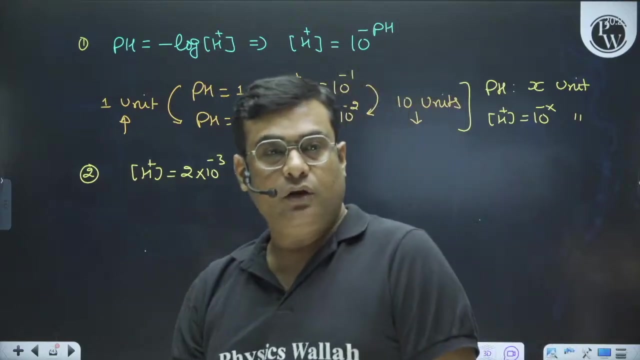 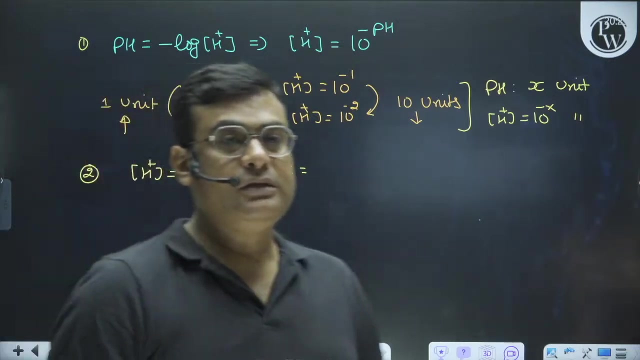 so this is the first lesson. second lesson: many students, if they are given concentration of H plus that 2 to the power, minus 3, and they are told to tell pH. but but you have to get out yourself and if they ask you to tell pH, then you. 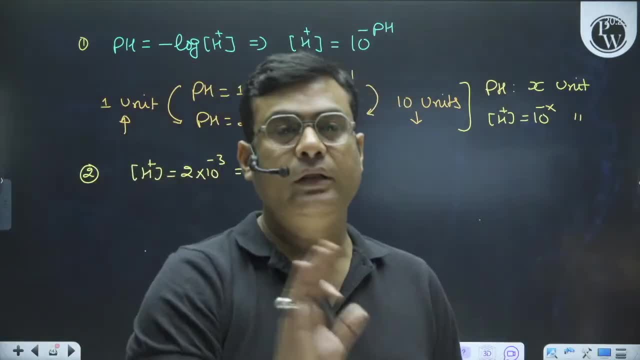 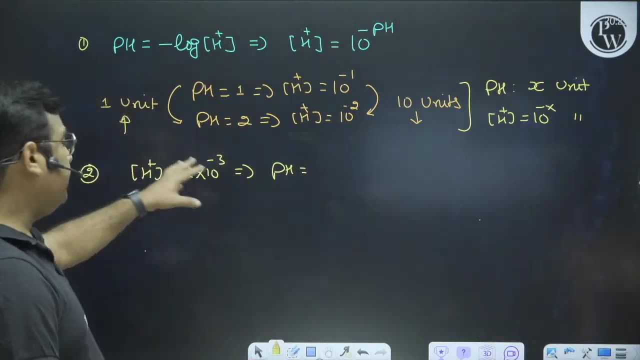 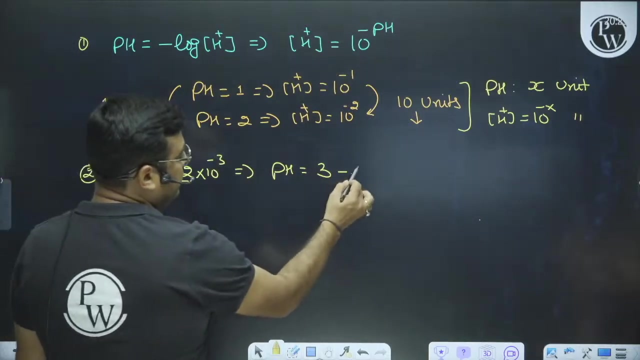 I have seen many students that they immediately from H plus to pH and from pH to H plus. they can not start converting. they make a mistake. I am telling you: the short trick of 10 to the power will be 3 minus. the number 2 will go in the log. So from now on, I hope that you do not. 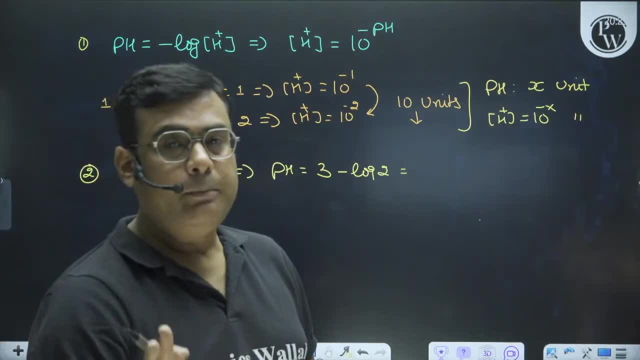 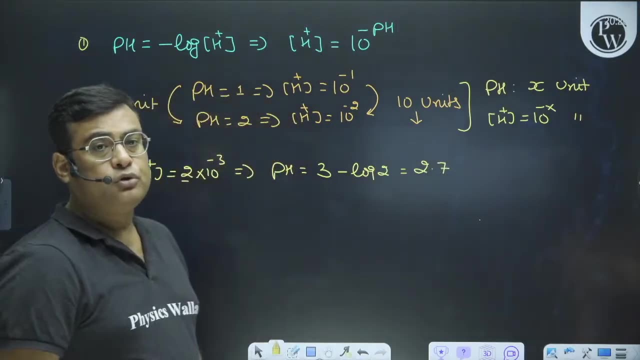 need to write this Now. I have said log 2, that I am assuming 0.3 only. So 3 minus log 2, 0.3, that is 2.7.. This will make your work quick. You will not even need to write this. 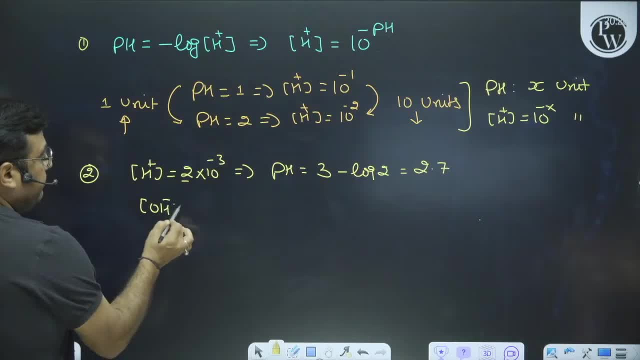 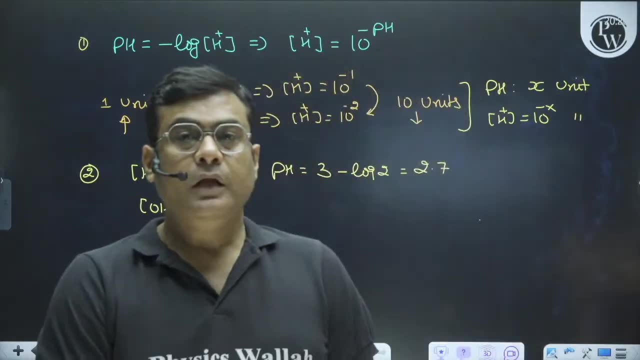 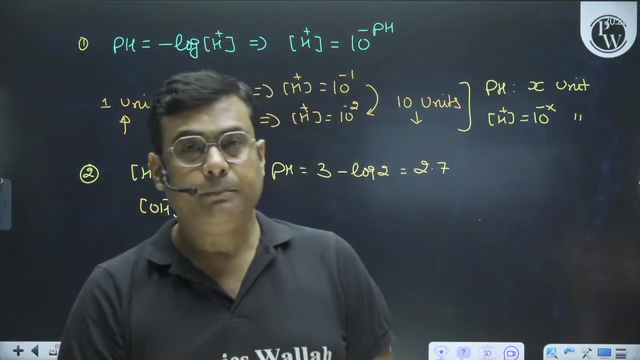 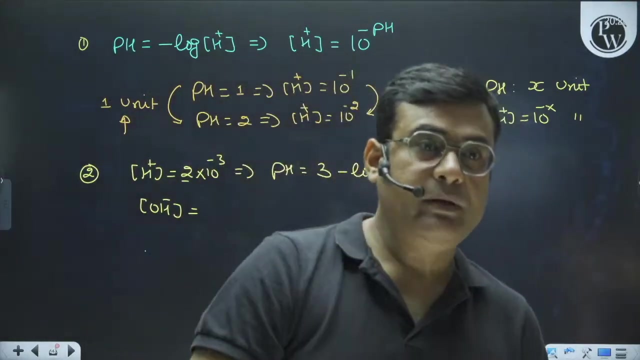 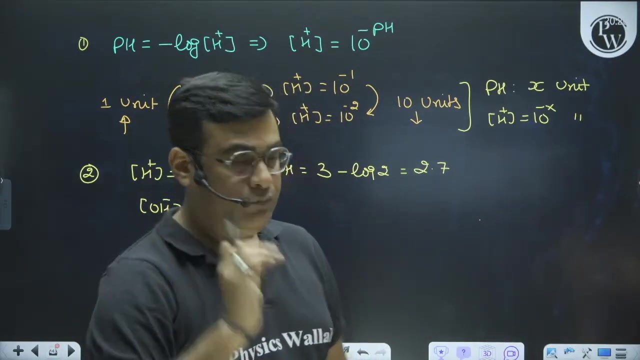 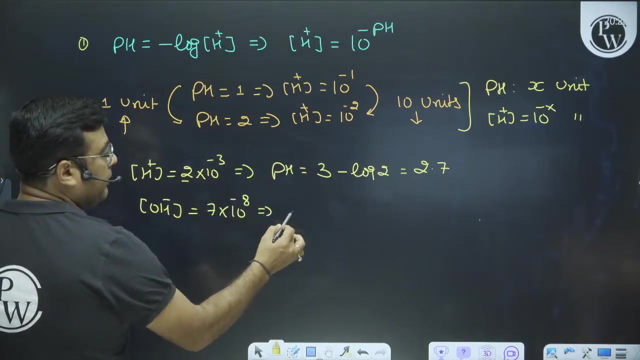 So we have already gone through all these people. I will tell you exactly what you need to do. For example, here: these two have reached their application. also, If I am saying that the concentration of OH- is 7x10-8 and I am asking you to tell me the pH of this, 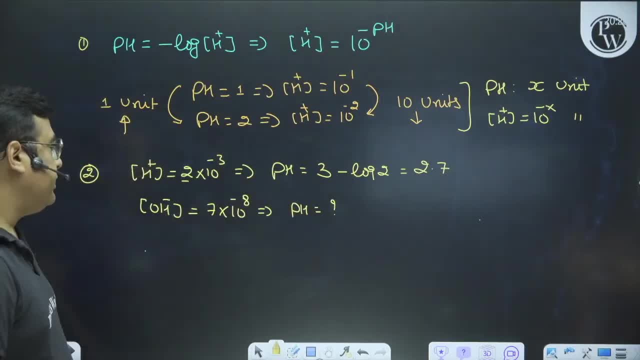 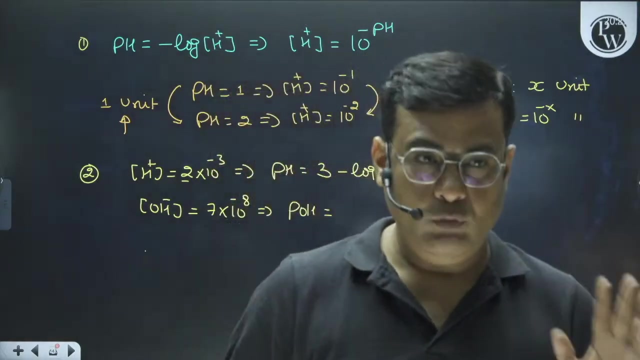 So you should know that if you have given the concentration of OH-, then obviously your pOH will come out first. And how will pOH come out? I just told you a trick: that you have to do: 8-log7.. Now log7 will be given in the question, which is 0.85.. 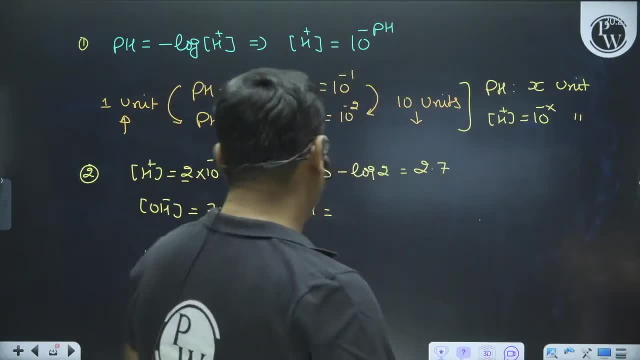 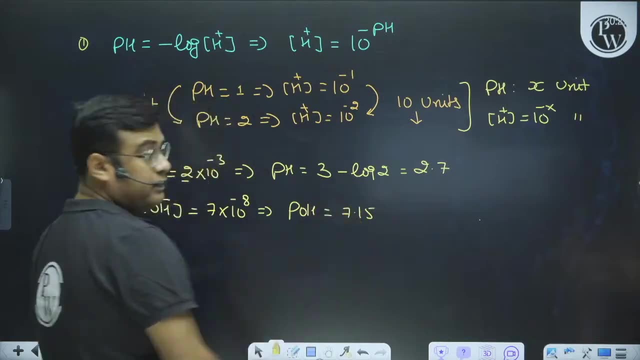 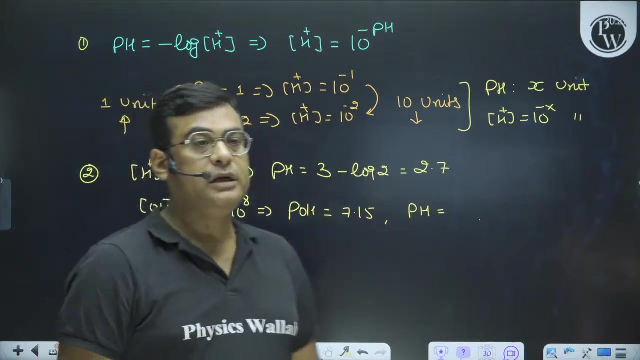 It is important to have log values, given. I am telling you this again and again. So 8-0.75 means pOH is 7.15.. And since you asked me about pH, we know that by default, we always take the temperature as 25 degrees Celsius. 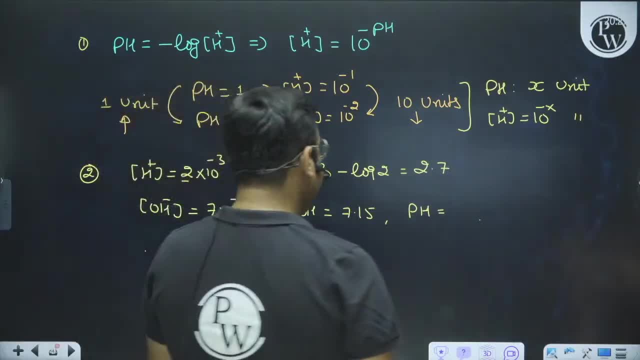 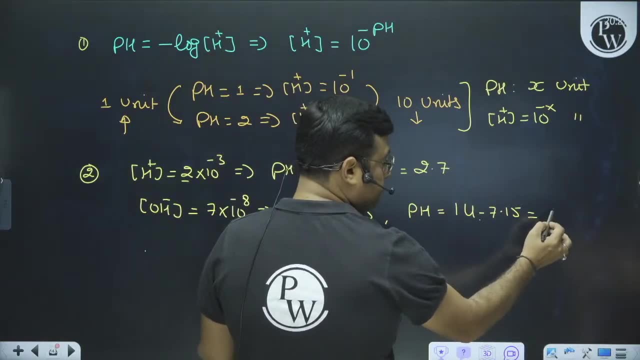 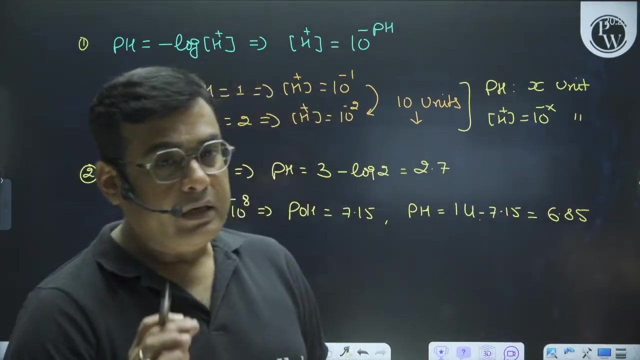 The sum of pH and pOH is 14.. So pH will be 14-7.15.. That is how much. That is 6.85.. So please- this is a small request to you, children- that you should be able to interconvert these things. 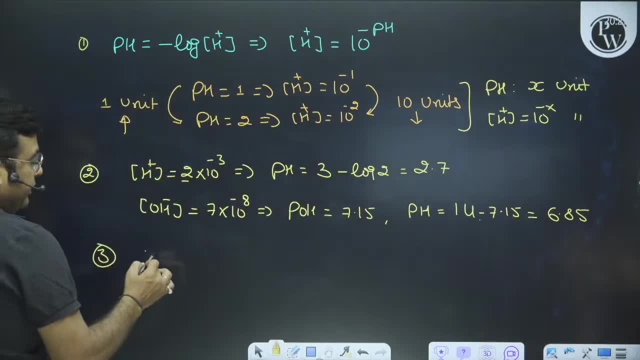 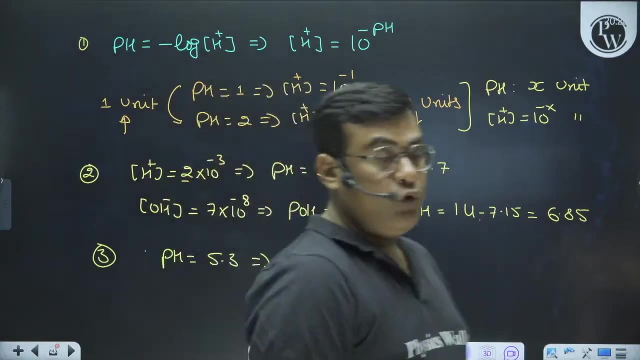 Third is my JSC That if you give us pH in any question, that the pH of any solution is 5.3. Now tell me H+, Now tell me H+. So now you have to take anti-log in this. And in taking anti-log I have seen that the child makes more mistakes. 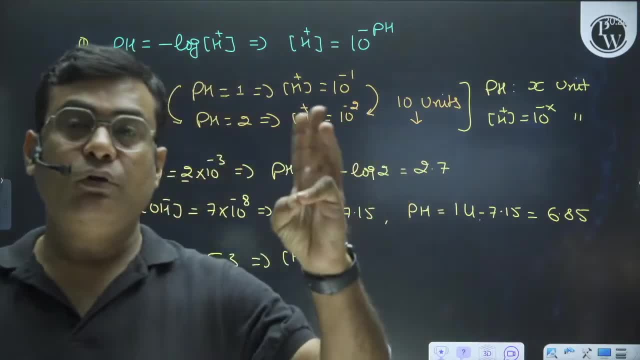 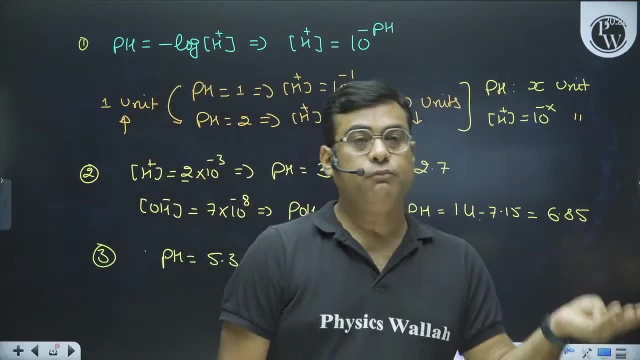 In your chemical kinetics chapter you need log-anti-log. In ionic equilibrium chapter you need log-anti-log. In electrochemistry chapter you will need log-anti-log. In thermodynamic chapter you will need log-anti-log. 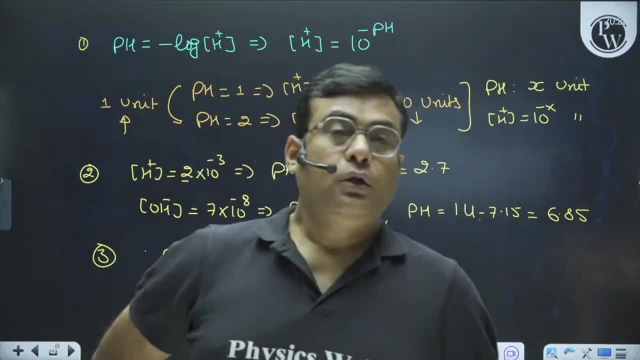 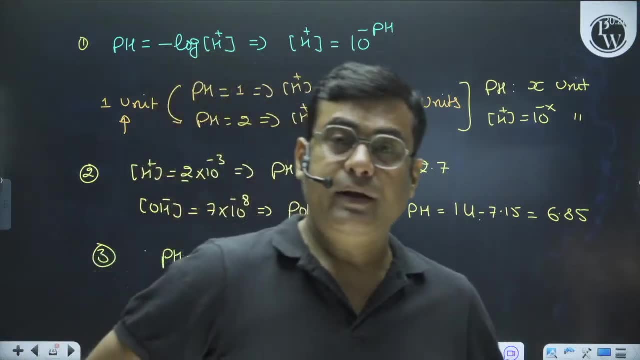 Because there you know the formula of work done: isothermal process. So minus of nRT ln of V2 by V1 is there. Everyone will remember, Yes or no? Are you remembering or not? So delta G0 equal to minus of RT ln of K, equilibrium is there. 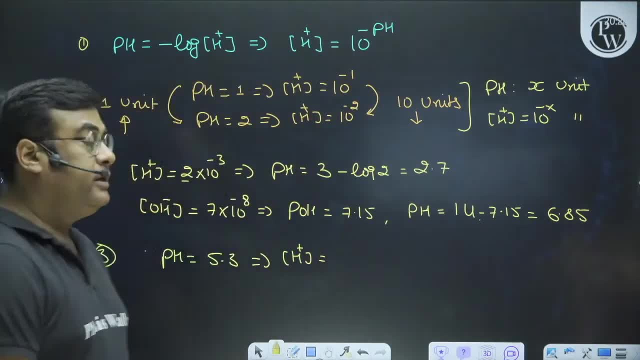 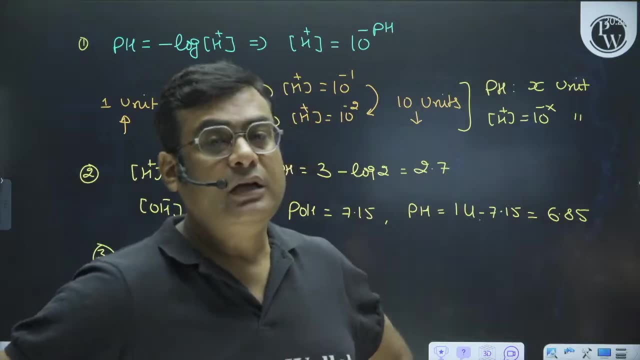 That will also be required Now. if a child writes that, we will directly say 10 to the power of minus 5.3. That will not be considered correct Because we always have to write in scientific notation. So I am telling you the trick of that. 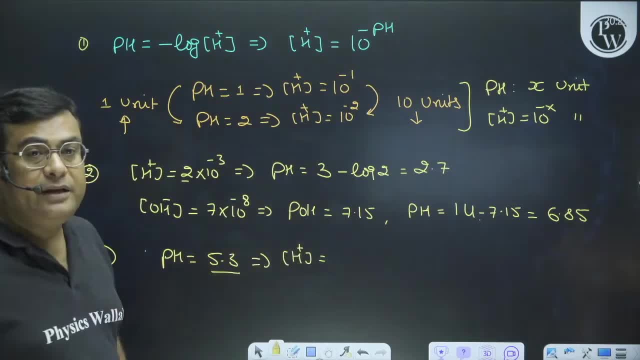 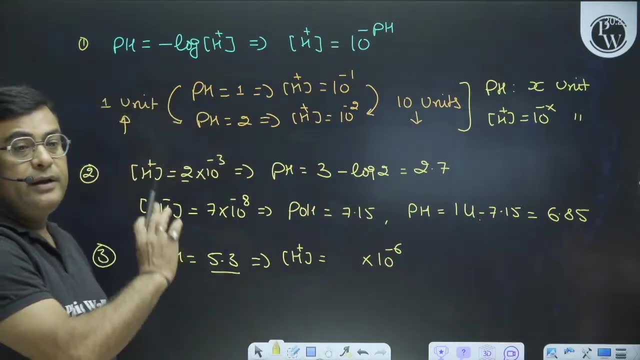 It is 5.3.. What is the next integer of 5.3? Sir 6. Sir 6.. So you have to write 10 to the power of minus 6.. I am telling you the direct question. 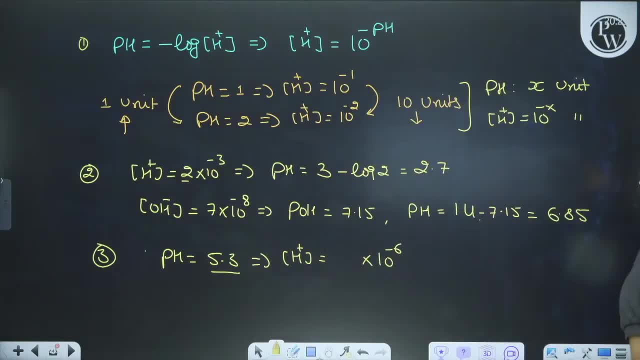 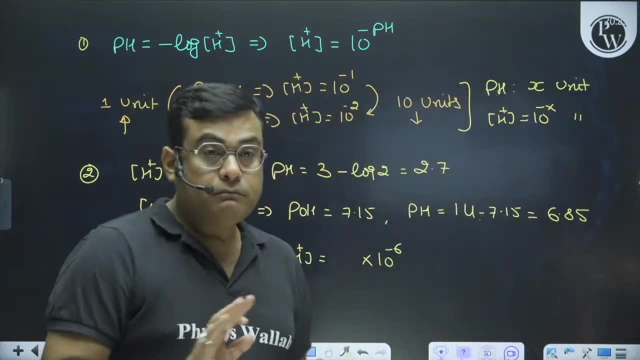 The technique of direct. Excuse me, I am telling you the technique of direct, Sorry, In which we do not have any time loss. Okay, Now, how much extra did you add To make 5.3,, sir, to make 6.. 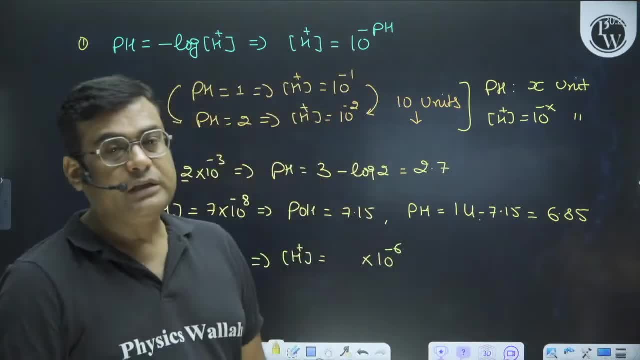 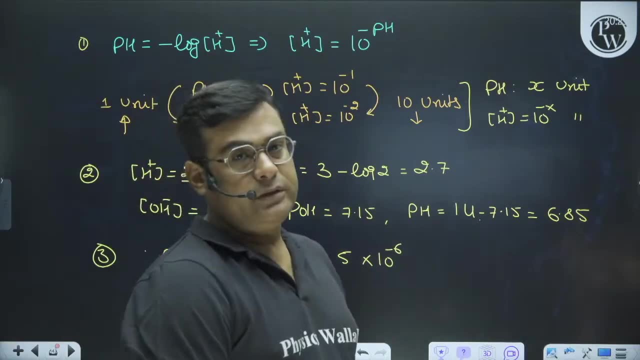 The extra I have added, sir, is 0.7.. And what is the log of 0.7, children, 5.. That is why your answer is 5 into 10 to the power of minus 6.. This log will be given. 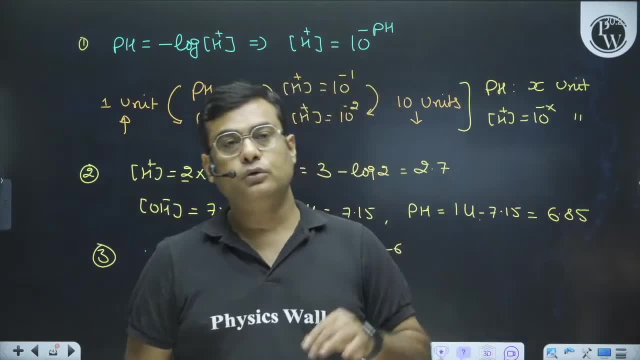 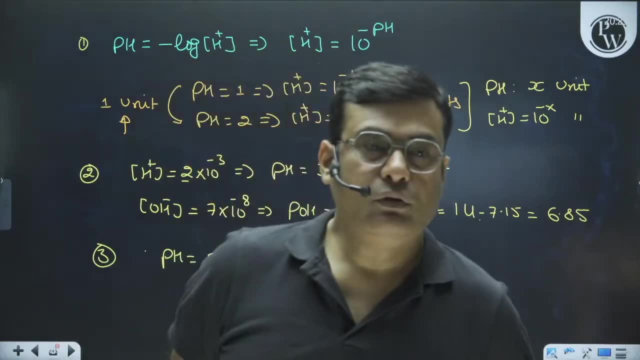 Even then, I request you that you have a log. 2 is 0.3.. Log 3 is 0.48.. Log 5 is 0.7.. And the log 7 is 0.85.. Remember these four logs. 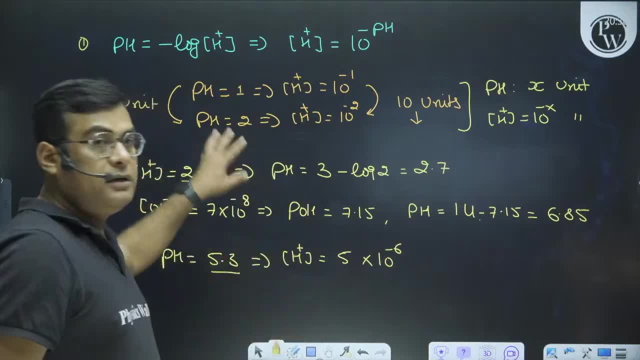 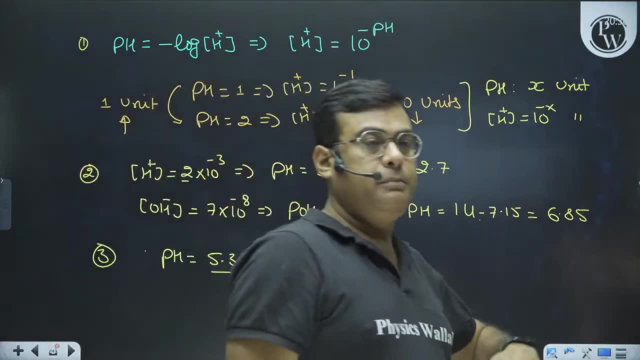 By the way, it will be given Okay. So that's why our first short trick is: understood, Everyone understood. Okay. In this way, you can solve all the questions like ph poh, pk, k, pkb, pkb. 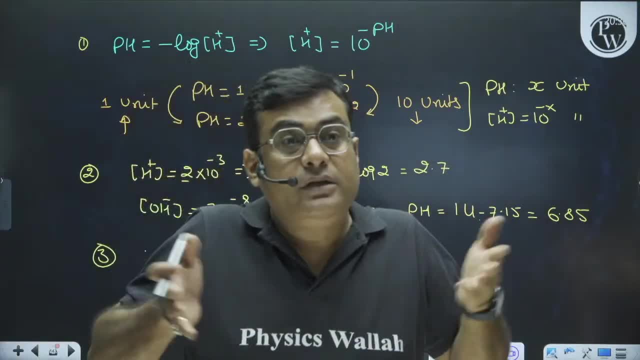 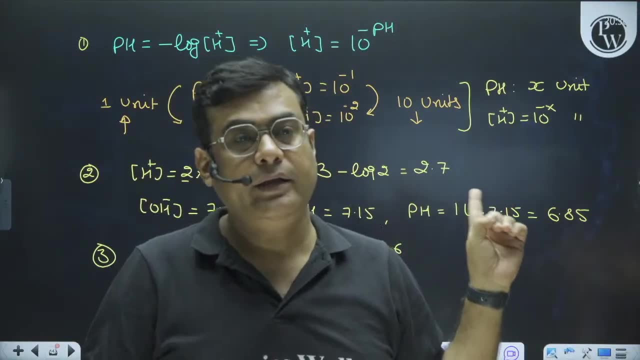 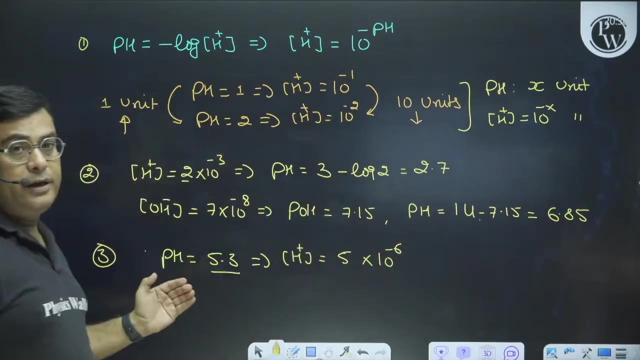 In which the child has taken out h plus, now he is not able to convert to ph, Or he has taken out ph, now he is not able to convert it to h plus. You will definitely keep this thing in mind. You will definitely keep this thing in mind. 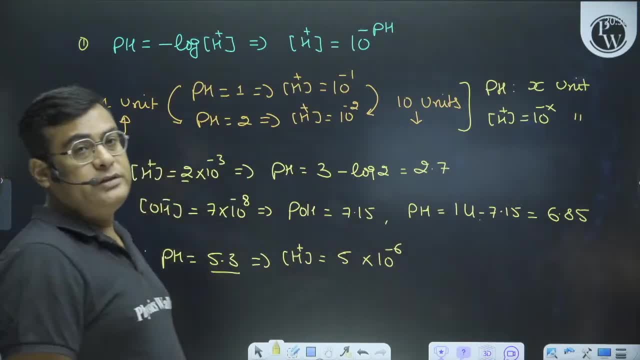 And you will definitely get a question on top of this. Yes, it is 0.69.. We just said that. I have considered the log 2 as 0.3.. Log 3 as 0.48.. Log 5 as 0.7.. 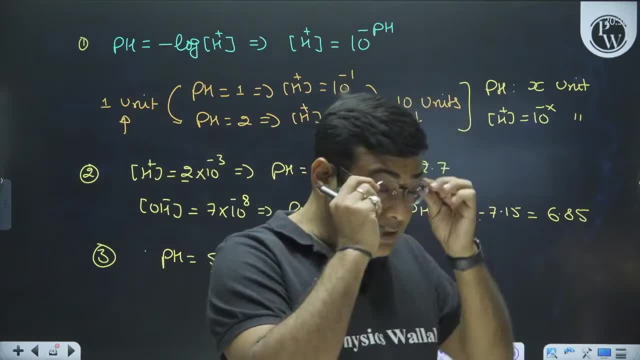 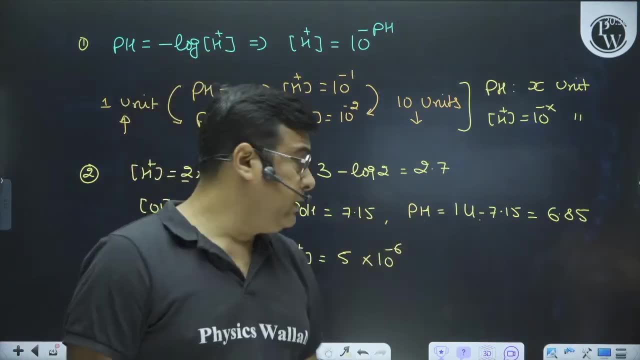 And I am taking the log 7 as 0.85.. And I have shown you a question from chemical kinetics in my proof. I have also shown you the data. Okay, Apart from this, children, my next unique technique is that, if there is a question on the buffer, 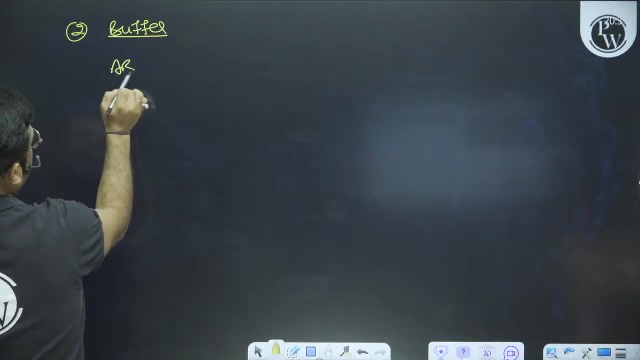 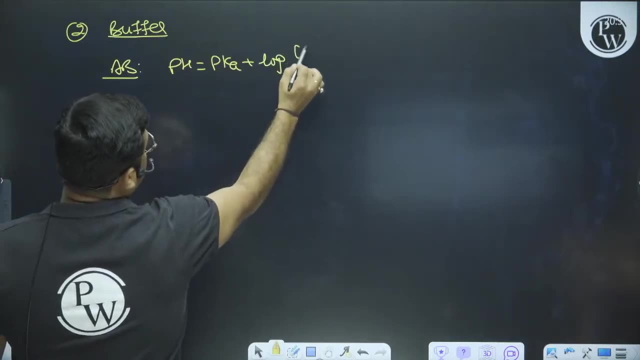 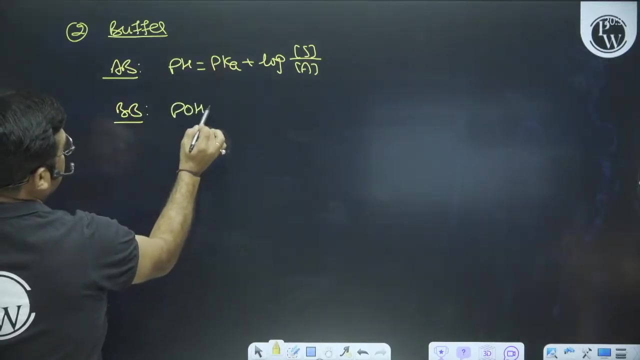 So buffer children. So you should know the formula of acidic buffer. what is pH equal to pKa plus log of concentration of salt upon acid? If there is a basic buffer, then the formula of pOH is applied in the basic buffer, which. 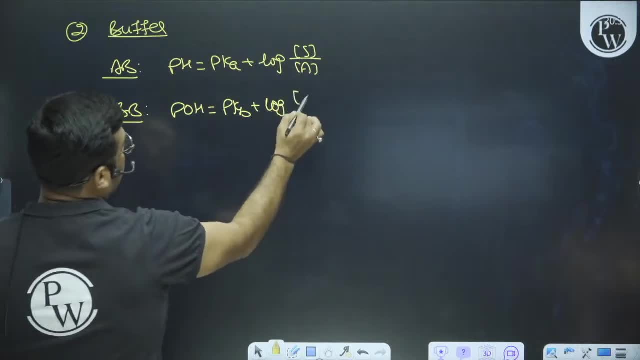 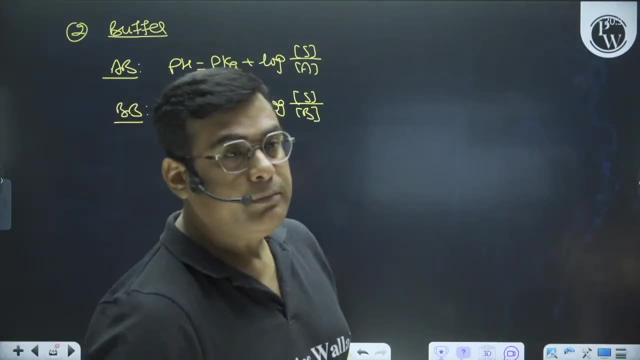 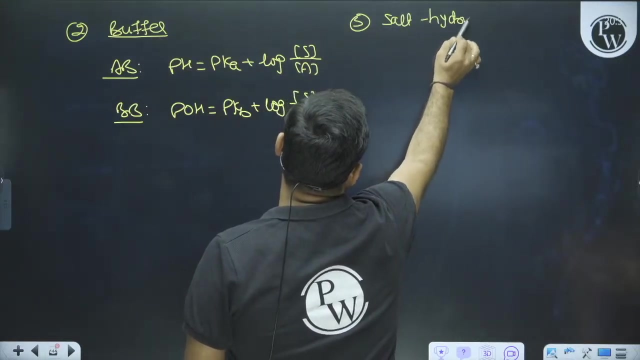 is pKb plus log of concentration of salt upon base. So be sure to keep this in mind in the question of buffer. The 3rd thing is that you should also remember all the formulas of salt hydrolysis, because the level of J mains will be of direct formula based question. 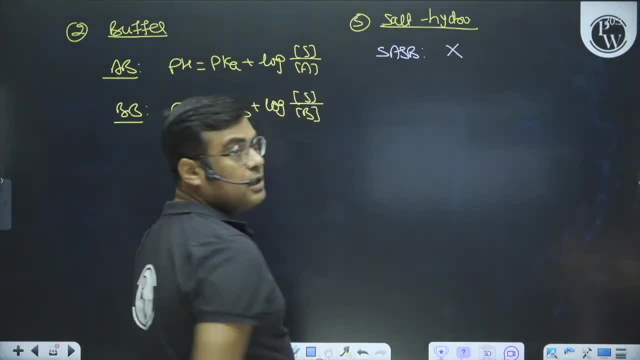 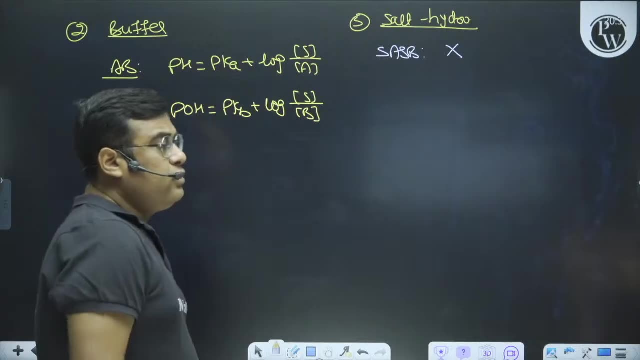 The first condition in this is that there is no hydrolysis of salt made from strong acid and strong base. and if there is no hydrolysis, then there is no formula of pH. Strong acid and strong base neither make the buffer nor there is hydrolysis of salt made. 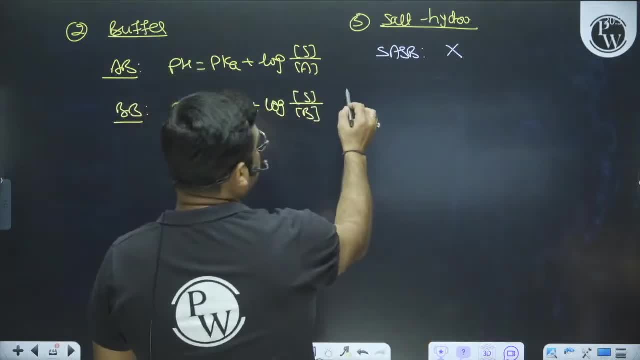 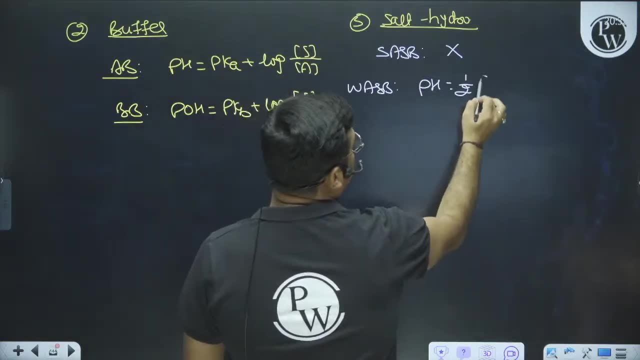 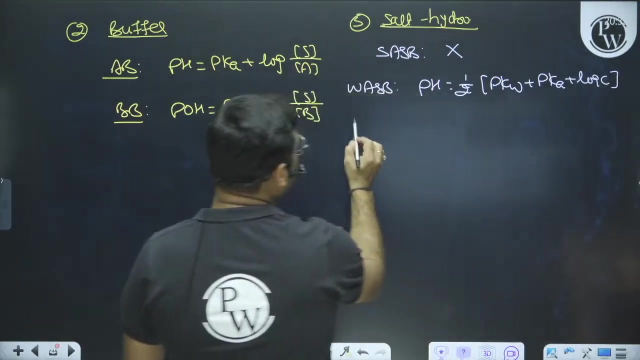 from them. Rest, brother, if weak acid is made from a strong base buffer, then there is no hydrolysis of the salt. of salt, then its pH formula is 1 by 2, half of pKw plus pKa plus log C. If strong acid 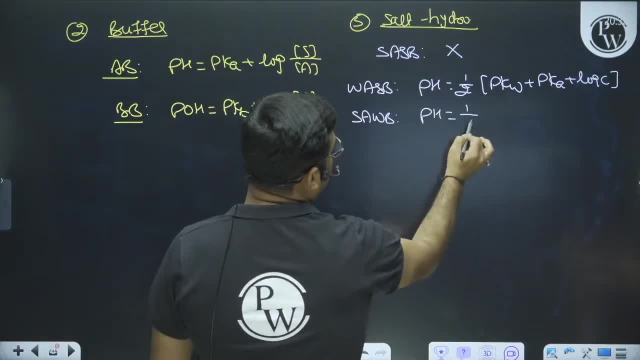 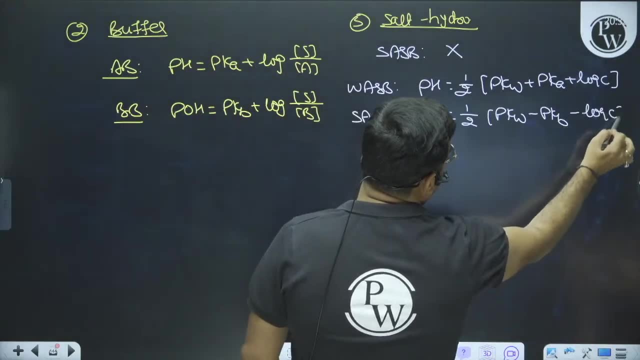 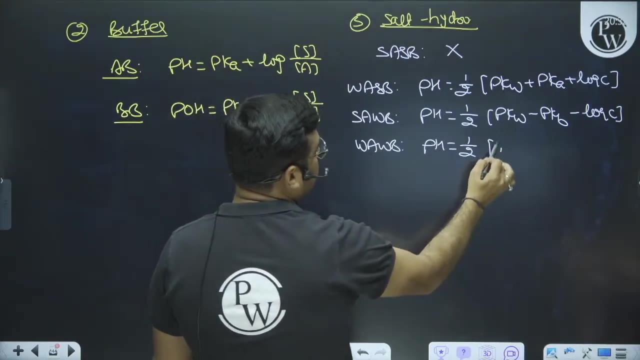 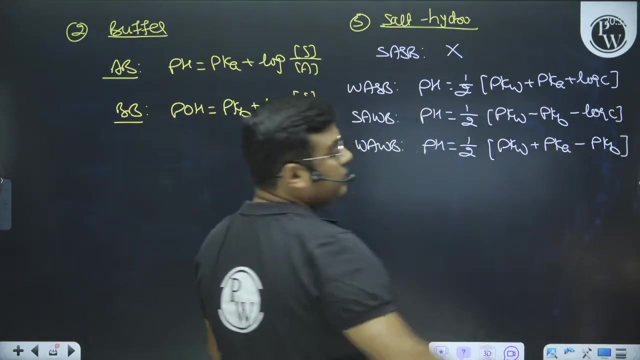 has weak base, then its pH formula is half of pKw minus pKb, minus log C. And if weak acid has weak base salt, then its pH formula is half of pKw plus pKa, minus pKb. These three 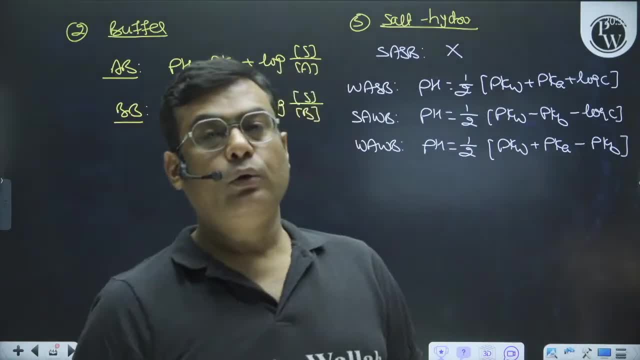 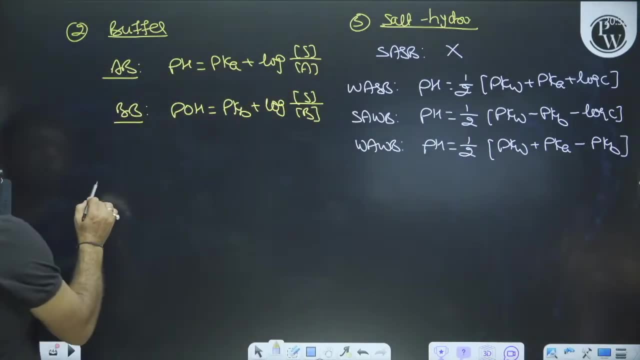 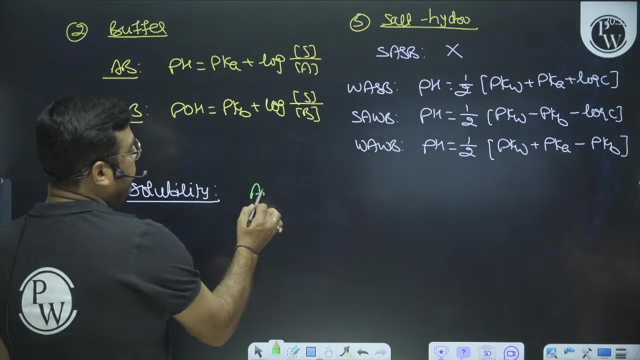 formulas are compulsory for salt to be remembered immediately. Apart from this, if we talk about the fourth formula related to solubility, then we will see 10-15 questions. What are the fields related to solubility If the salt is AB? 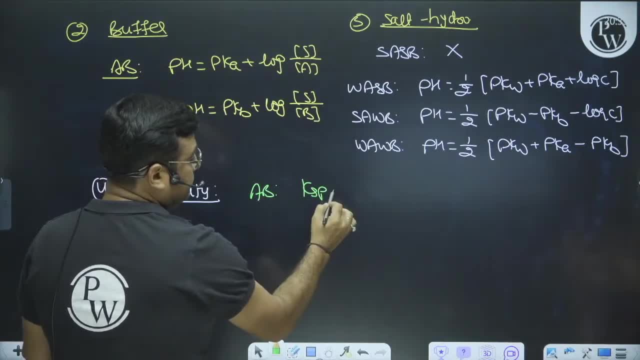 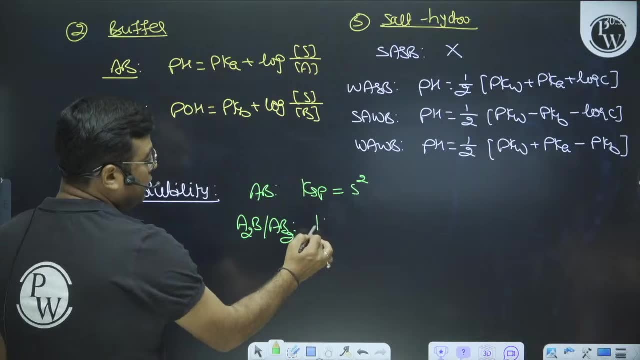 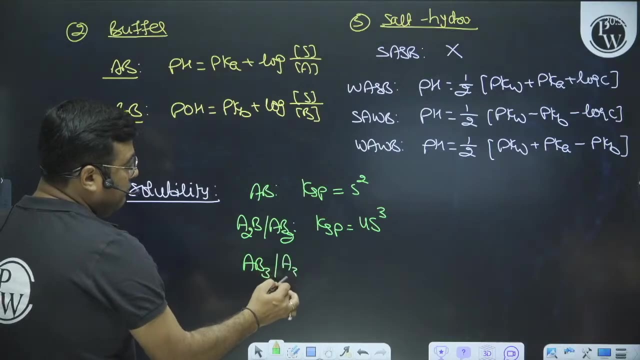 then its KSP formula is SQ, and if your salt is AB2,, then its KSP formula is SQ, and if your salt is AB3 or AB3B, then its KSP formula is CQ. If you use this difference, as always, y are responsible for ABS2 and AB3, and if you have 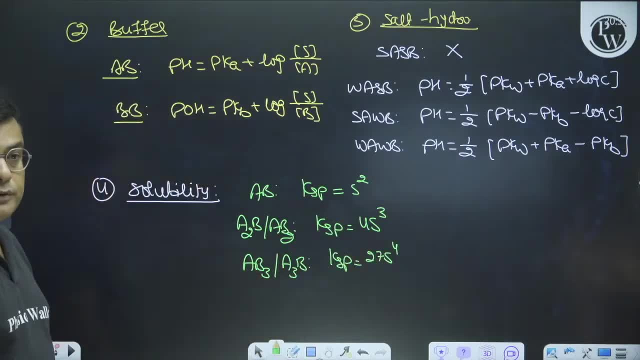 a solo type. Aye, you are responsible to solve this problem. The first B type is idea B2 is an problem of solubility. now, Now, if we say that we go to material based onิ 27s power 4, ok, and if your. 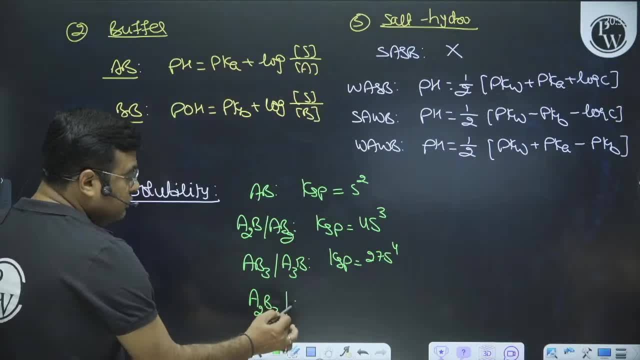 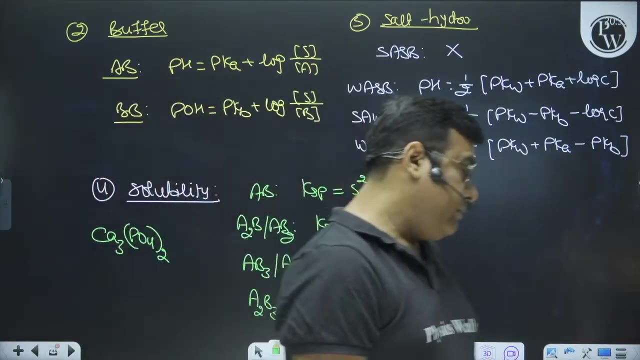 A2, B3. most common salts are these type. you have to recognize what is the meaning of type. if you are given by writing calcium phosphate- I hope your is inorganic- then you will get some knowledge of salt analysis solubilities. you have to remember all. 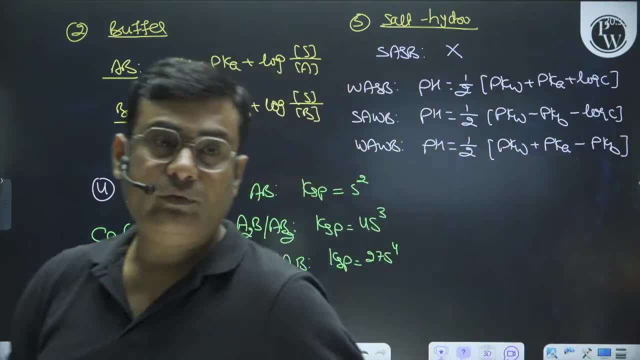 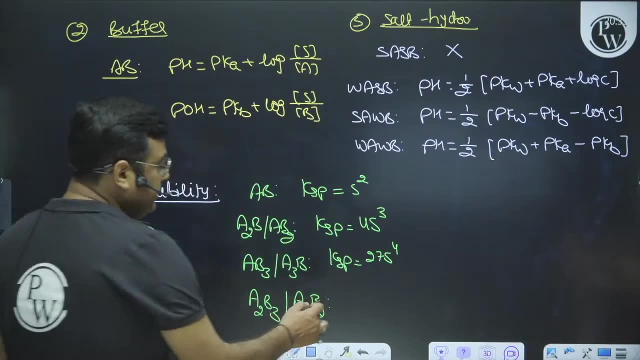 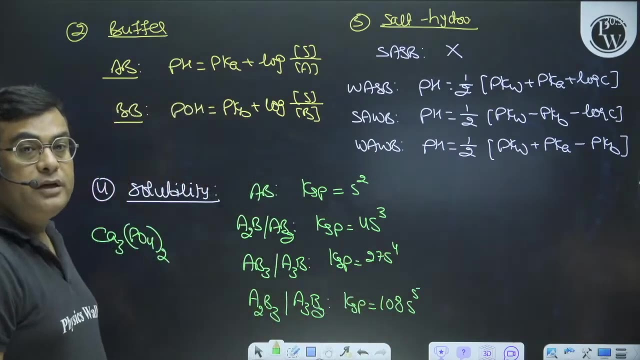 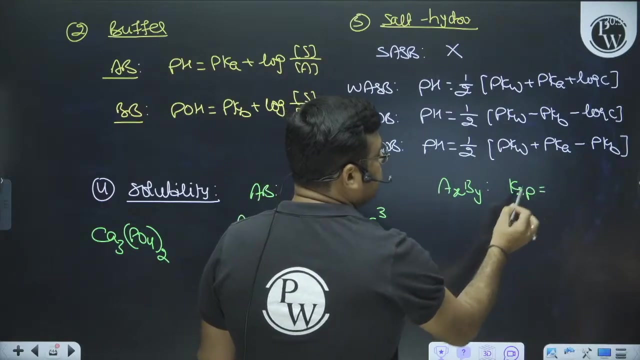 like calcium phosphate. calcium phosphate is insoluble. so which category of salt is it? A3, B2 type? so what is the formula of calcium phosphate, 108s, power 5 and in general? in general, if your AX BY type salt is there, then its formula. 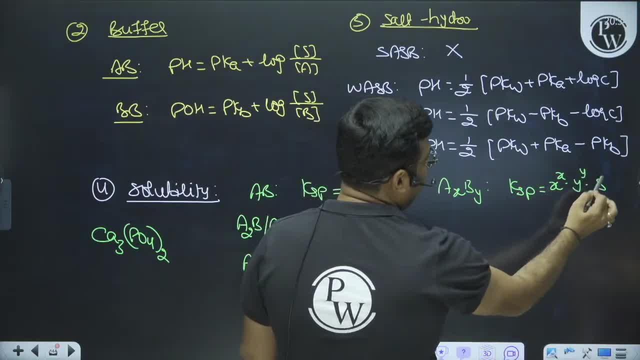 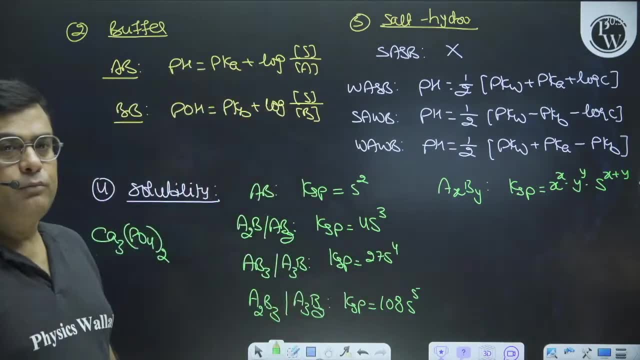 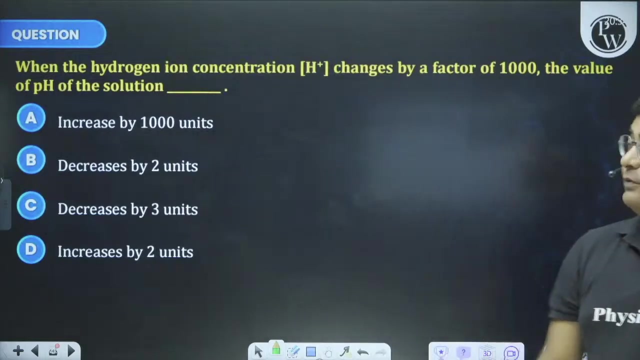 X power, X, Y power, Y, S power, X plus Y. something like this: increase the speed, increase the speed. so welcome your birthday. this is a basic formula you know, and now we see all of them, let me see some more questions on it. ok, some on the question. 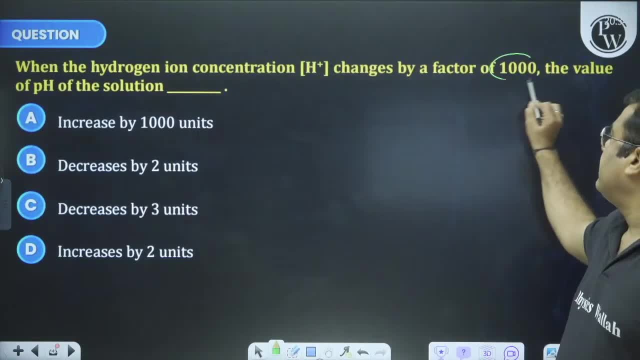 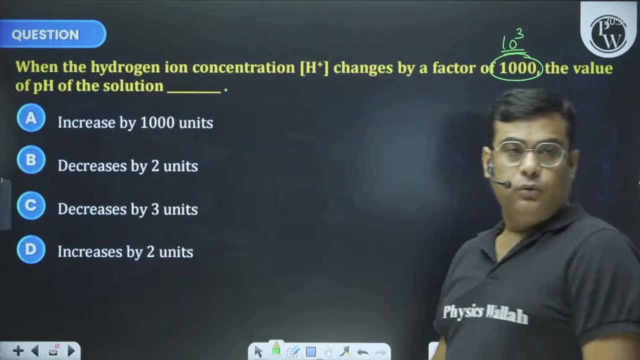 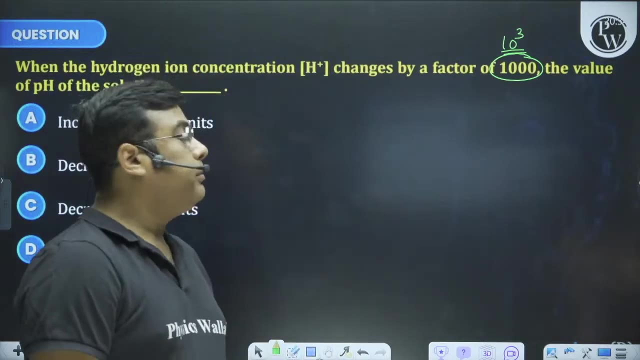 What is reported when the hydrogen ion concentration changes? thousand, what is the meaning of thousand? it means 10, power 3. so I wrote you the first rule: what you have written, you write. what you have written, you write How many times. if 10 to the power of X time is changing, then how many times will the pH change? 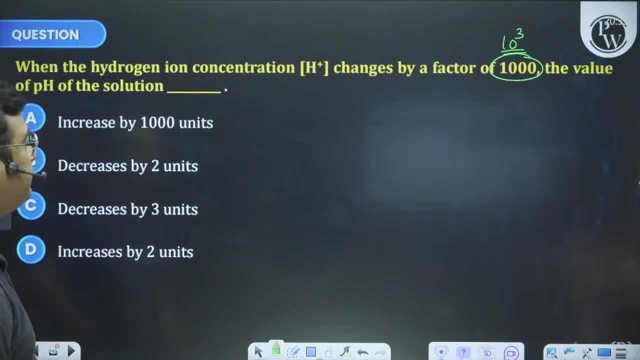 X, time is 10 to the power of 3, then the value of pH of the solution will change three times. Now, what will be three times your change? and three times? there is only one option for that. then I have to think of increase and decrease. 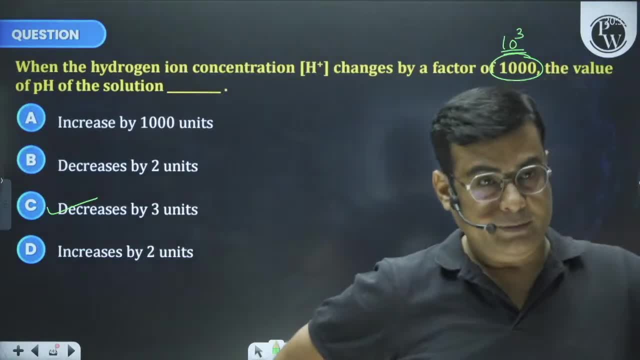 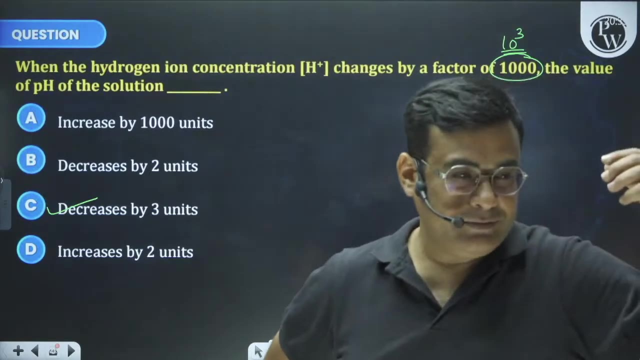 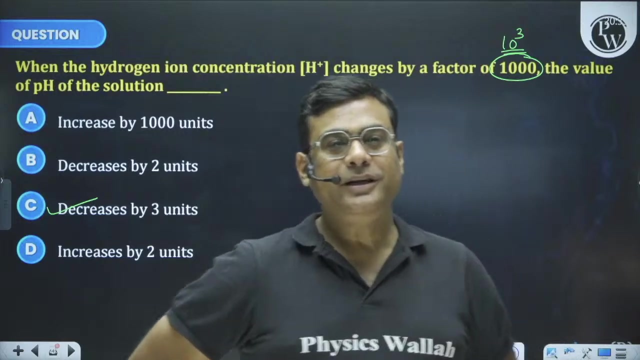 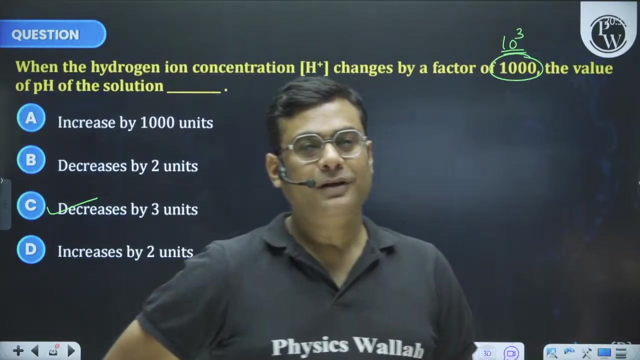 There is no need to think here When you put the answer pot on the spammers. If you put the answer pot on the spammers, then the one or two people who are here are involved in these things. You listened to me. I will tell you my love story. who is he? how is he the queen of your dreams? 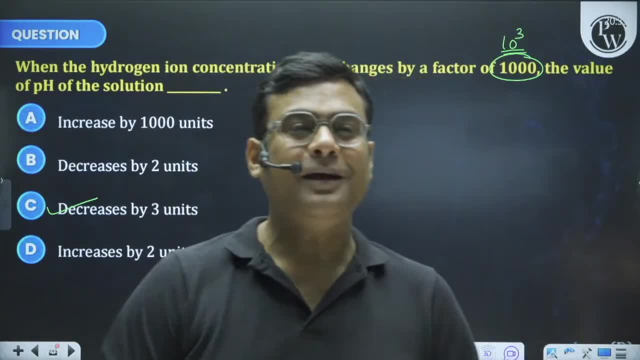 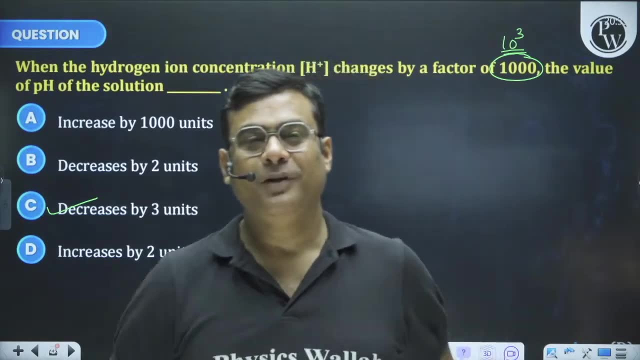 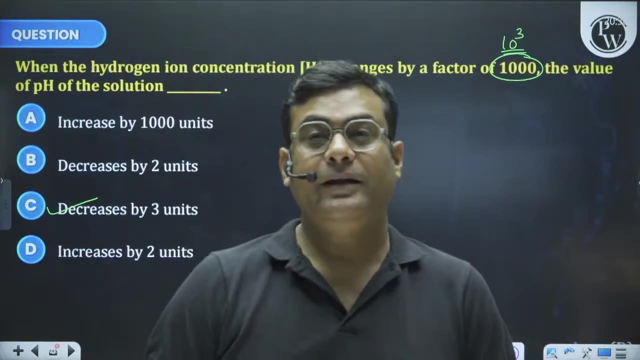 So where is all this? The stories that two or three people will be doing? they will disappear on their own because no one will be looking at them. so you have to keep these things sensible, And I think you should motivate such people more. son, that is the inspiration for the coming generation, that how our future is made short. 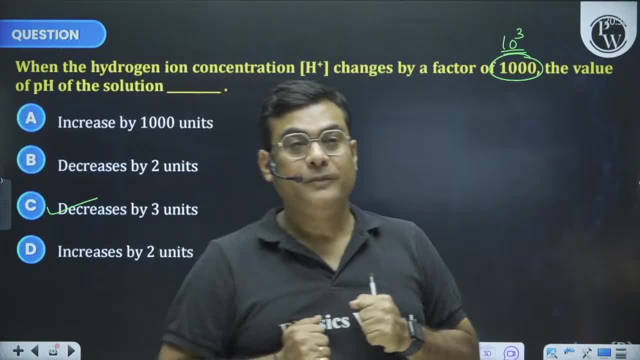 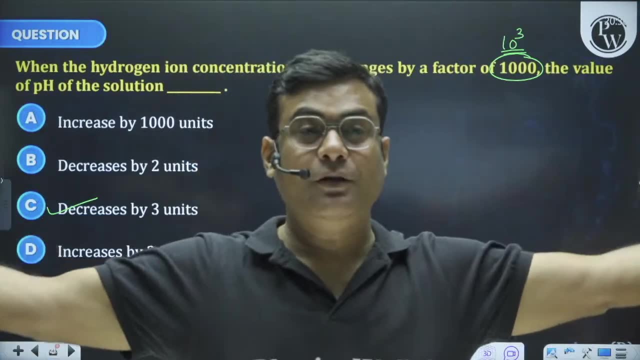 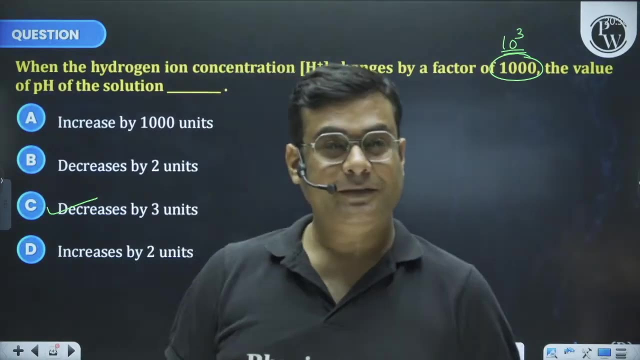 There should also be two or three examples to give people that they had a good opportunity to study and make a future, but they said: no, I will waste time, We will waste their time after that. So we also have some examples, son. 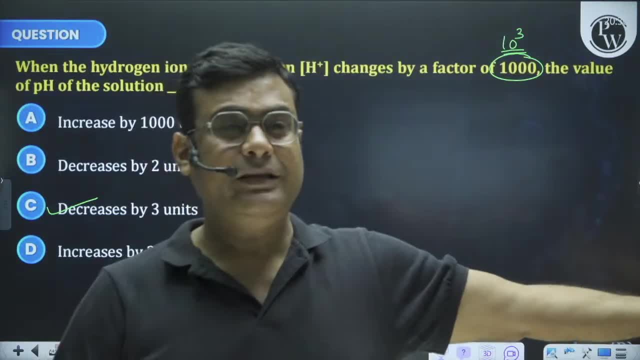 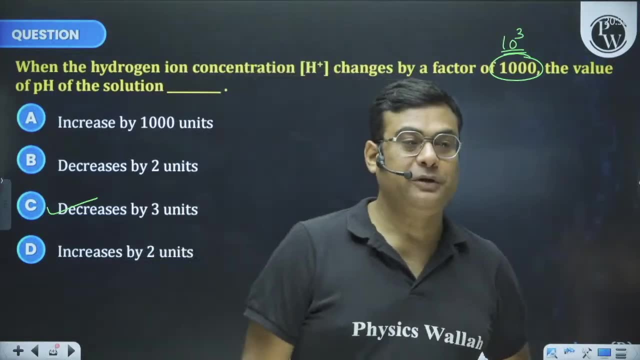 Why, brother, I am not sure how his father's future is also managed. and then the job of the broom and dungeon is involved. And see, for example, we should have two or four Come every time. theай become an engineer, then who will epoxy theployments? 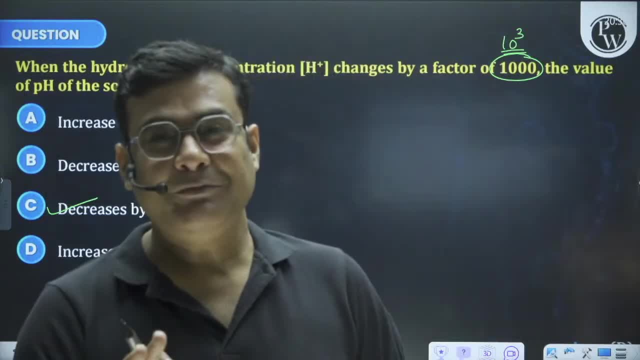 One would also need to do something to help someone earn so many royal crores or billions. God will give them a month's work and NOBODY will trust you. Who will sacrifice you or I commit you to someone? You are right here. you should take this responsibility. 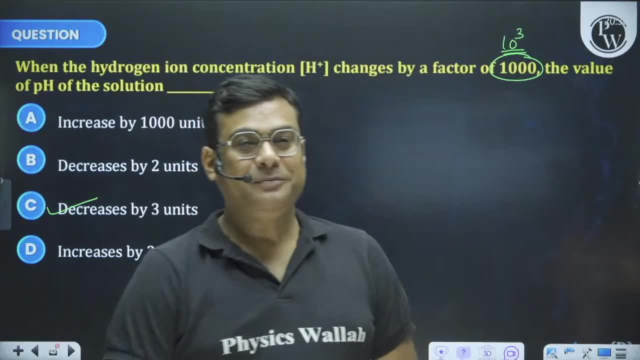 You are right here. you should take this responsibility. If you earn in lakhs and crores of rupees per month, then you will also need it, right? Okay, so such people should have 2-4, right, Sure, let's go. 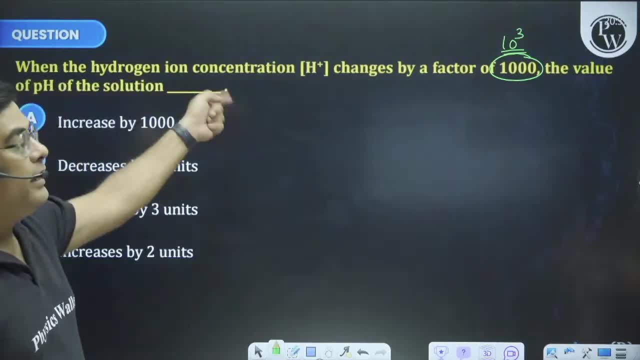 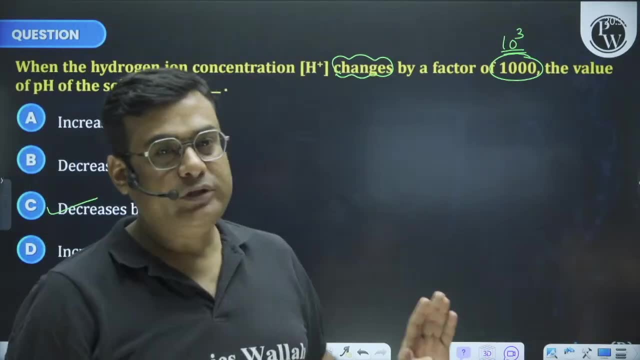 Sir, now how to find out about increase and decrease in this son He did not give. son he did not give, he put the word changes. When he put the word changes himself, then I don't know if he is increasing or decreasing. 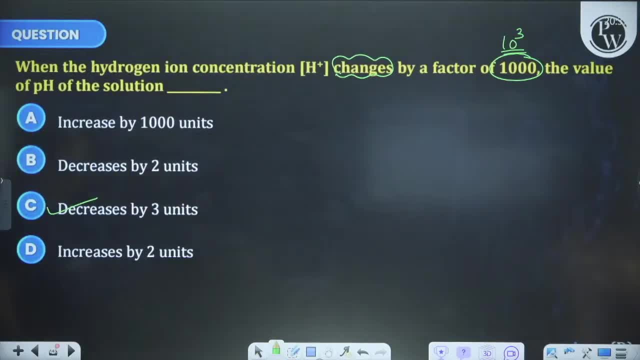 What logic did I give? You may not have heard right, You did not hear. you did not hear. I gave the logic that if the power of 10 is 3, then there will be a change of 3 in pH, and the change of 3 is only in one option and not in any other. 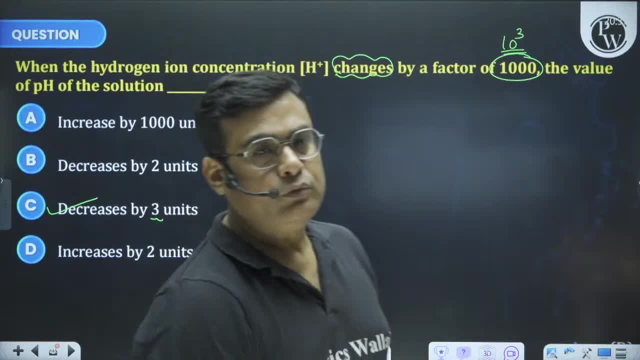 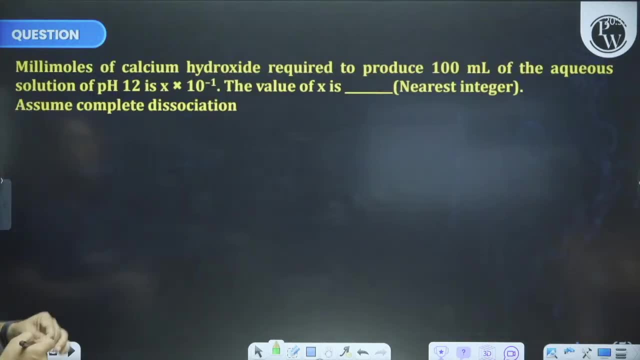 I gave this logic. If he would have written increase and decrease, then I would have talked about it as well. If he would have written increase and decrease, then I would have talked about it as well. Okay, let's go. Millimoles of calcium hydroxide required to produce 100 ml of aqueous solution of pH 12: is this much? 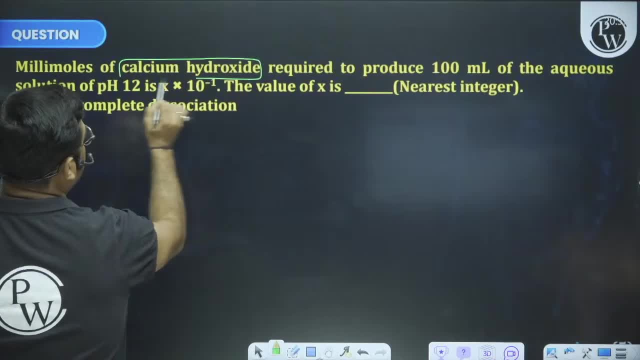 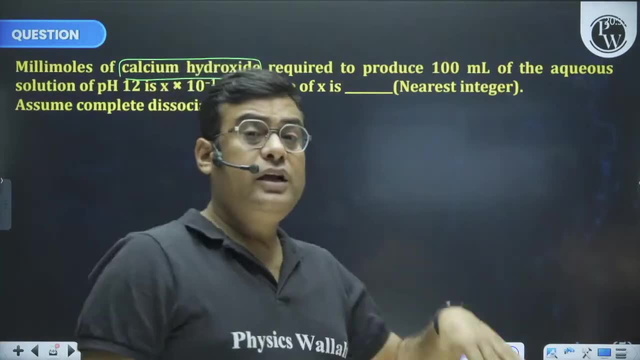 Value of x? tell me Now. I should know, son, if he told me calcium hydroxide's assumed complete dissociation. That means he has assumed strong what he has assumed children. he has assumed strong base. Now pH is 12.. 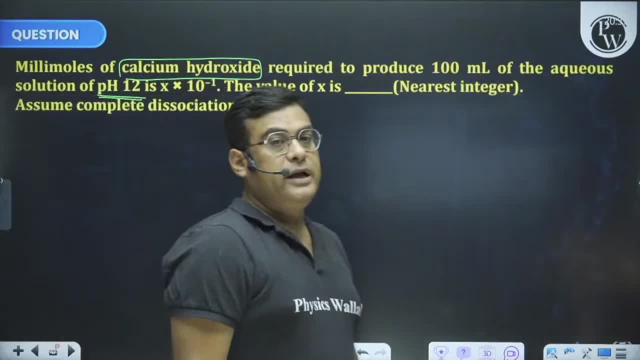 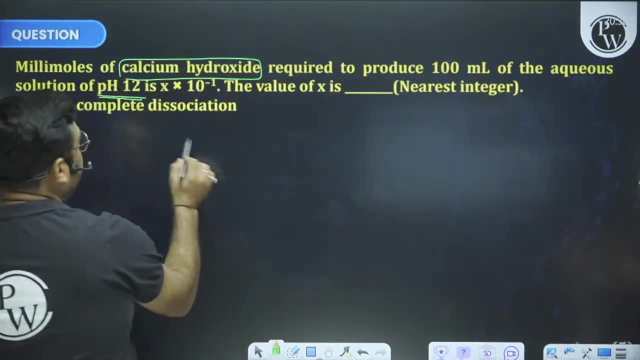 Now one more teacher. keep in mind that for base pH is not necessary, son. for base pOH is necessary, isn't it, Isn't it? Okay? so if pH is 12, then it means pOH is 2,, isn't it? 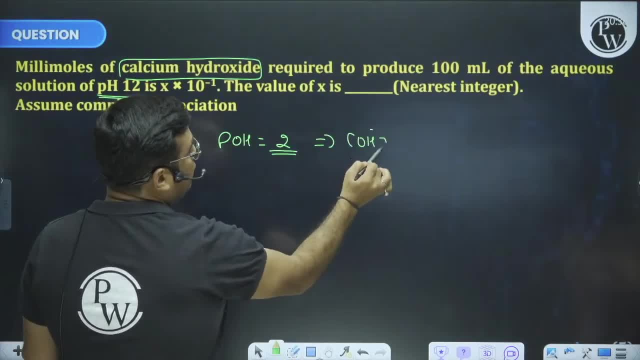 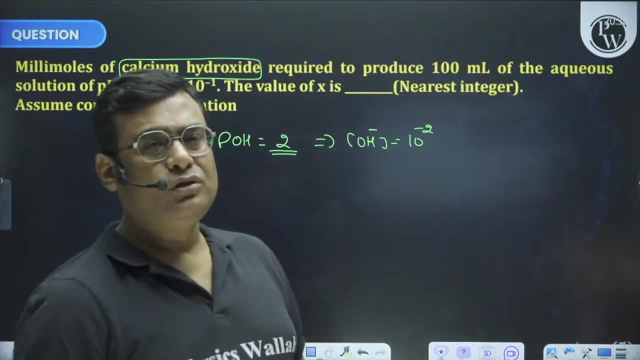 And pOH is 2, means concentration of OH minus. Look, so many children are afraid of ionics. I also know children, I have experience of so many years. So many tiny questions are there of ionics also. These are all questions of JEE. 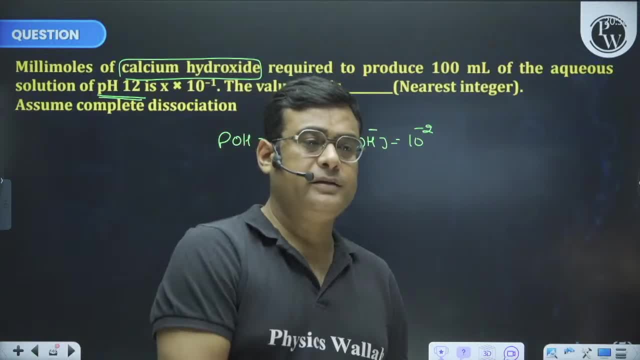 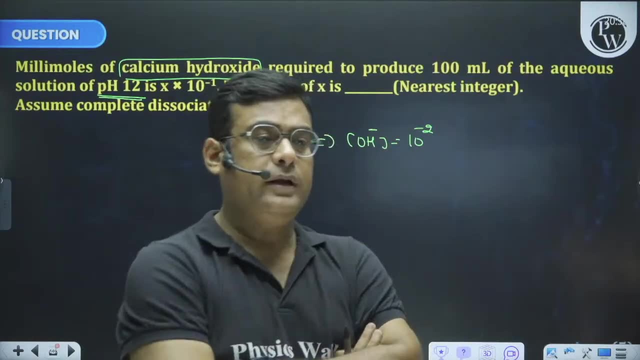 Isn't it? I have purposely disappeared ear, Because as soon as you write ear. some children have such brain. they have booklet and straight answer And they think that we remember one question. they don't remember anything. They are sitting with book. 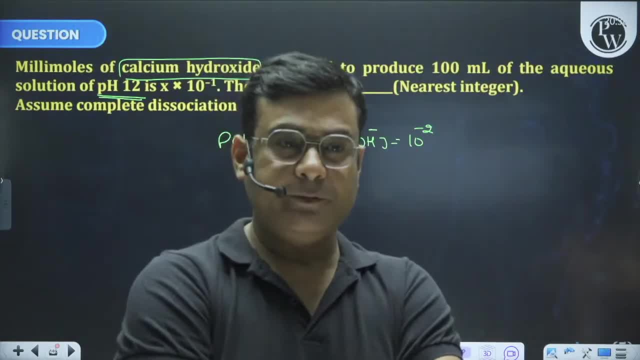 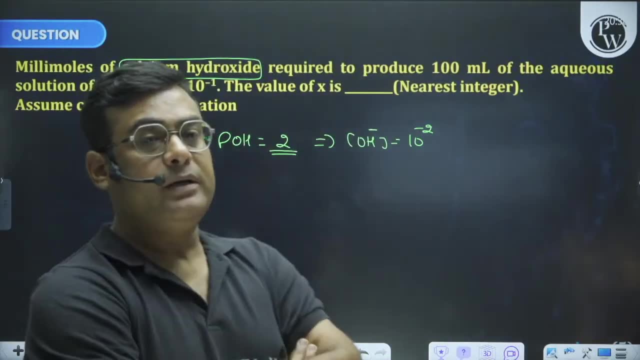 I have jumbled question and disappeared, ear, Okay, and there are some new things in between. I have mixed both things. Okay, sir, Because I have to tell you, I have to tell you the concept, how to approach the question, how to learn the calculation, isn't it? 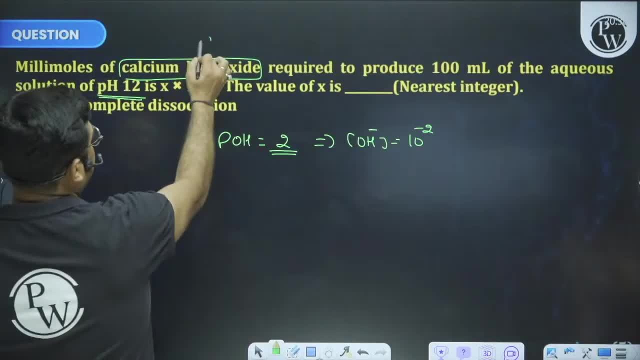 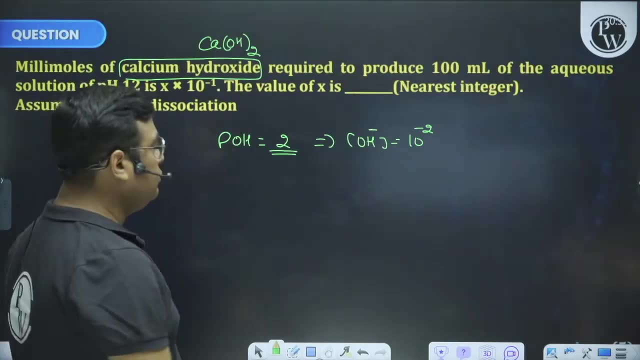 So OH minus is 10 power minus 2.. Now, because calcium hydroxide is there, then obviously CaOH will be whole twice. Okay, so if the concentration of OH minus is 10 power minus 2, then the concentration of calcium hydroxide will be 10 power minus 2 by 2.. 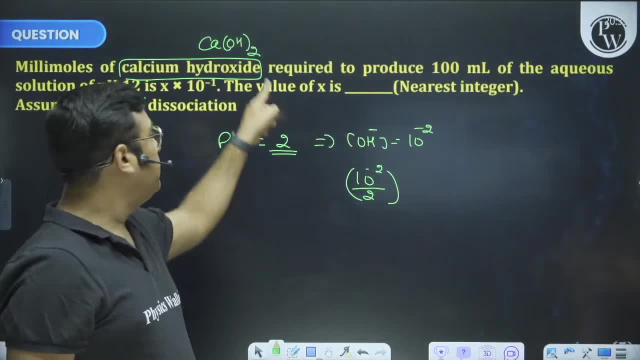 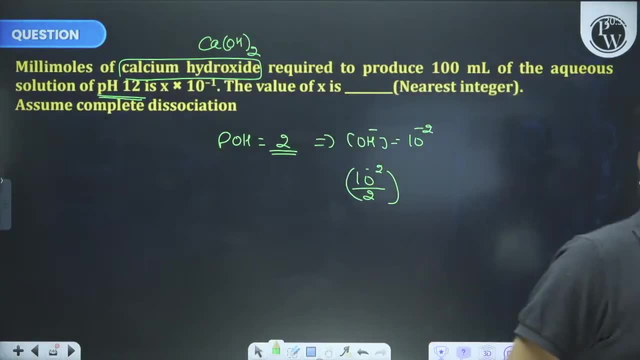 Agreed, Isn't it? 10 power minus 2 by 2 will be half, Because 1 is 2, 2 is the ratio. So I have just told you a little while ago, before going to the break, to break the compound into ions, to make a compound from ions, that how many chapters do we need? okay? 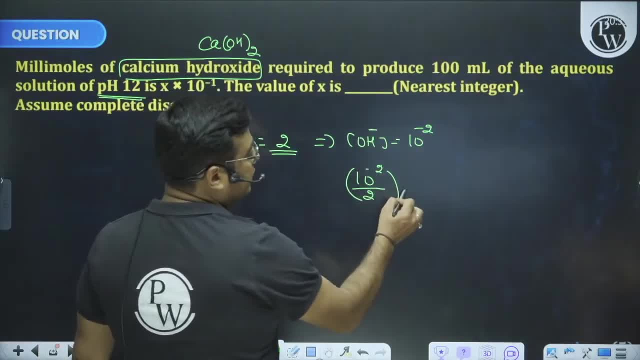 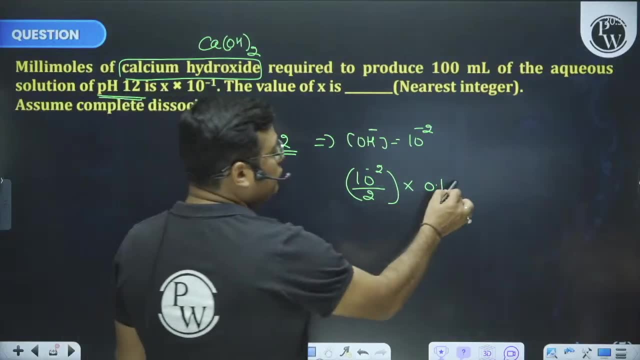 And apart from that, children. he talked about millimoles. This is molarity. Molarity into volume in liter, Isn't it? Molarity into volume in liter? These are the moles, But since millimoles are said, then you will do 3 more times 10.. 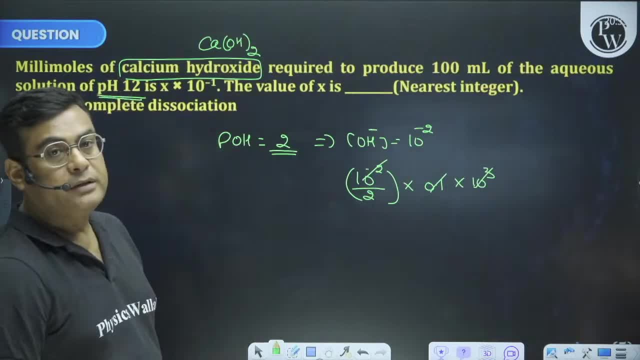 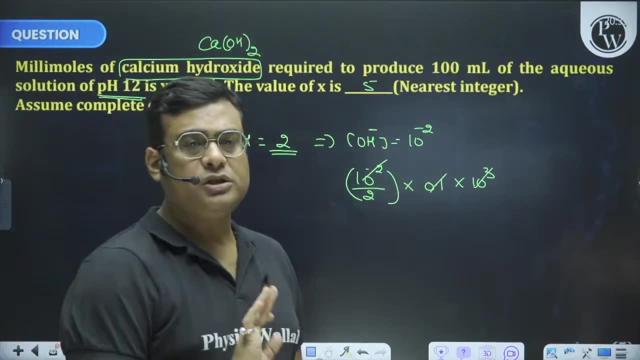 See this is cancelled. What can I write? 1 by 2,, sir, 0.5.. That means 5 into 10, to the power of minus 1.. Answer 5, children. Answer is 5.. Nothing to do. 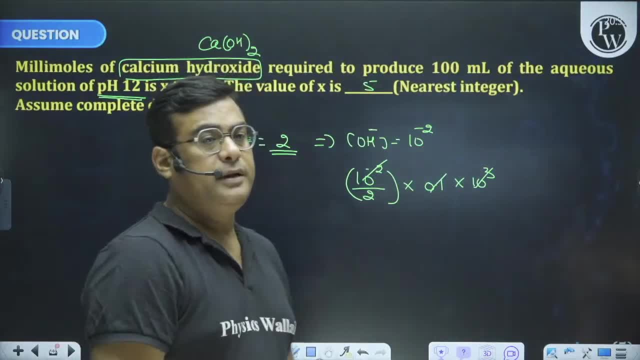 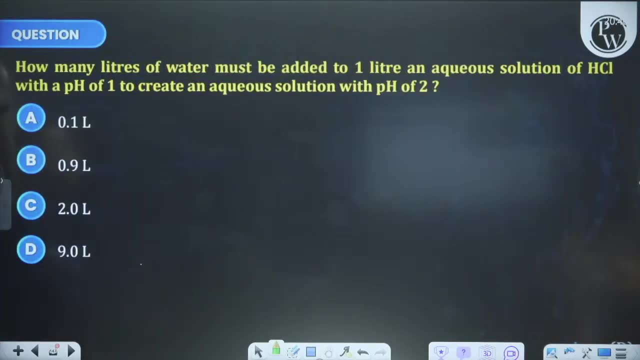 Isn't it Nothing to do? Okay, Keep in mind, You will have to remove fear. You will have to remove fear. Okay, See more questions. Come next question. Let's take a strong acid. How many liters of water must be added to 1 liter of an echo solution of HCL with a pH of 1?? 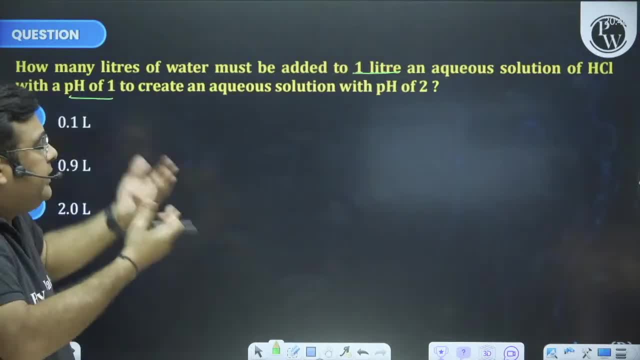 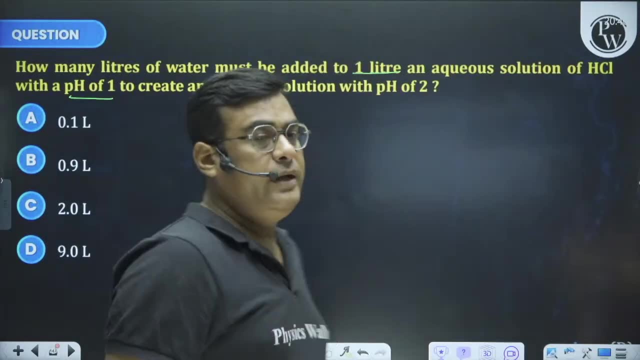 In the beginning it has a pH of 1.. Obviously, I will add water, So I will dilute the solution. I will add water. That means the concentration of H plus will be less, and if the H plus is less, the pH will increase. 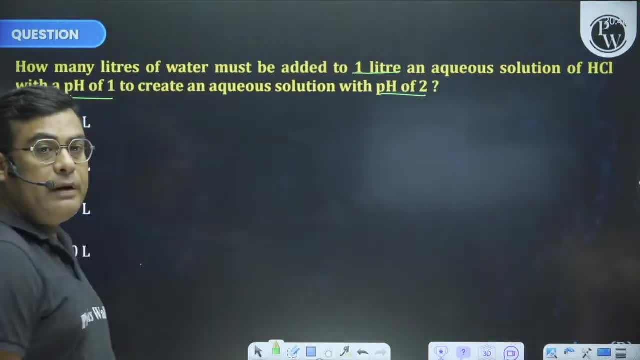 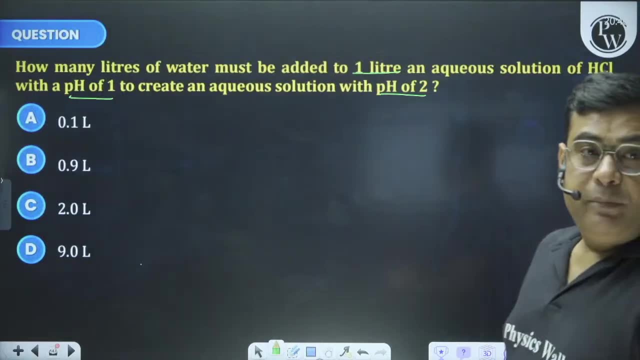 So he has said that, do a new pH 2.. Now again a new JSC will be running in your mind. There is no big deal in your mind, son, that whenever it is talked about removing or adding water, right. 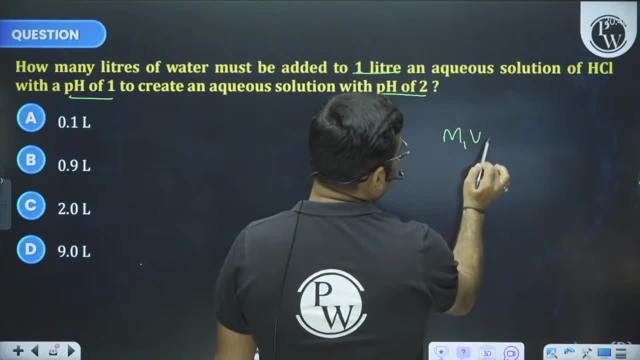 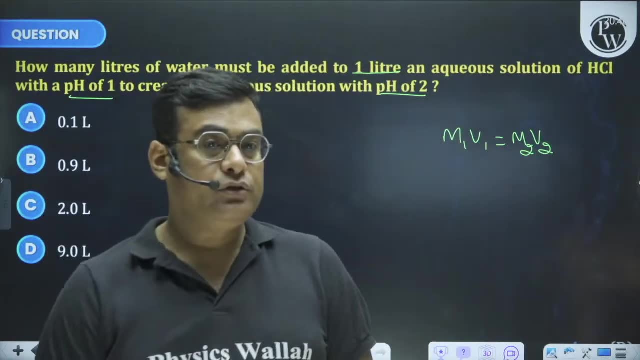 Whenever it is talked about removing or adding water, then the dilution formula will always apply, And the favorite of JEE in ionic is that it is often used by children on the surface of the water. If the question is wrong, then here your M1. V1 equals to M2. V2 is going to be applied. 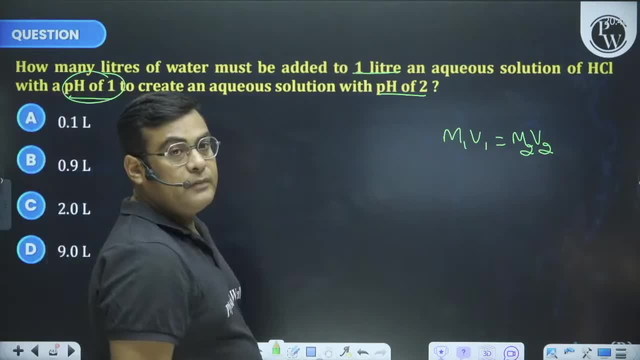 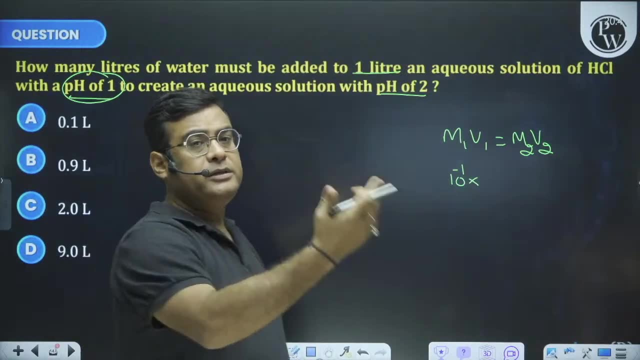 What is M1?? If it is pH 1, it means H plus is 10 to the power of minus 1.. That is why I told you those tricks as soon as I came that all this should be running in my mind. 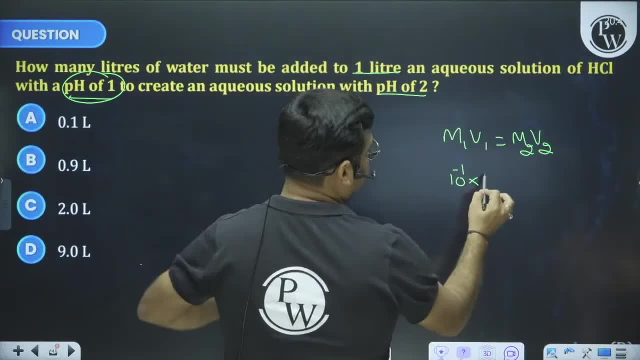 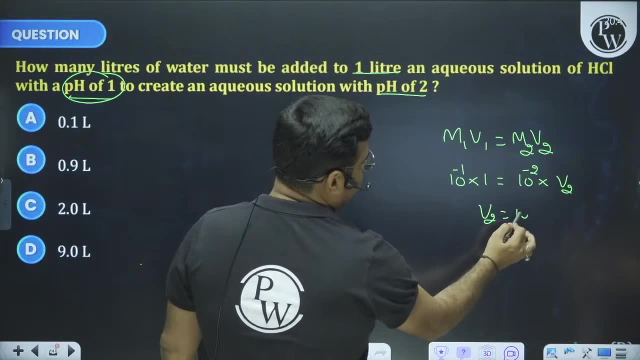 How much is V1?? How many liters of water? V1 is 1.. M2 is 10 to the power of minus 2 into V2.. So here V2 is 10.. Right Now, you are lucky that he has not given the option of 10.. 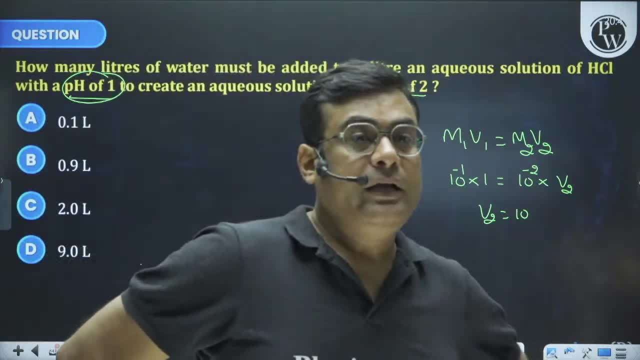 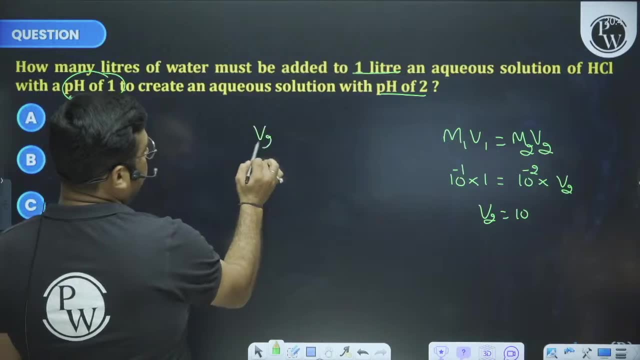 So some people do not give 10.. So be careful, son. In this formula the V2 is the total volume. Right Total volume means the V2 here is V1 plus volume of water. V1 is the original volume. 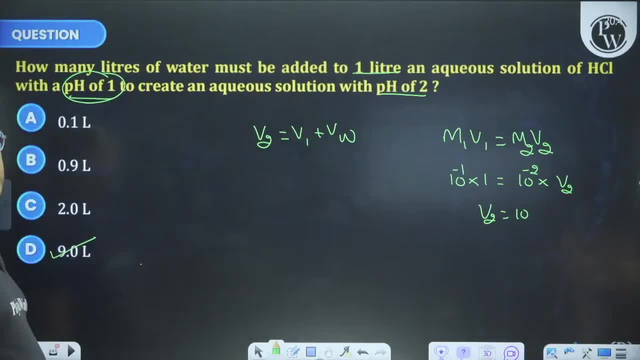 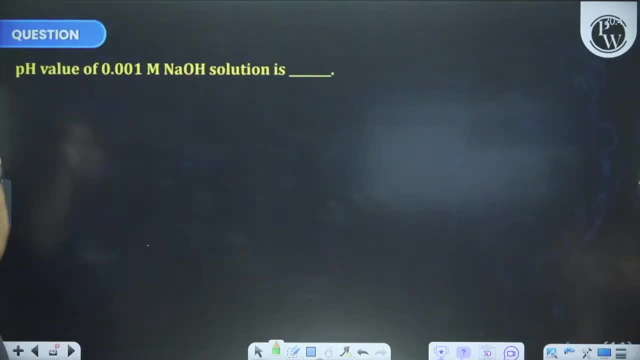 So this means that I will have to add extra volume. How many liters will I have to add? 9 liters, Right? So this means that I will have to add 9 liters. Look again Now, JEE people. 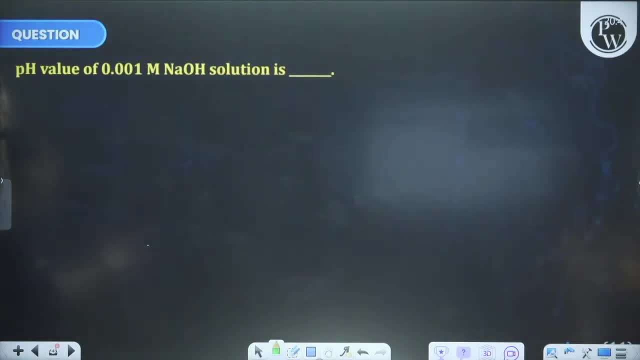 If you will ask an easy question, then what should we do, Right? Okay, We are so busy in the chat that we do not worry about our future. It is a different matter. Otherwise the question comes like this: pH of 0.001 molar NaOH. 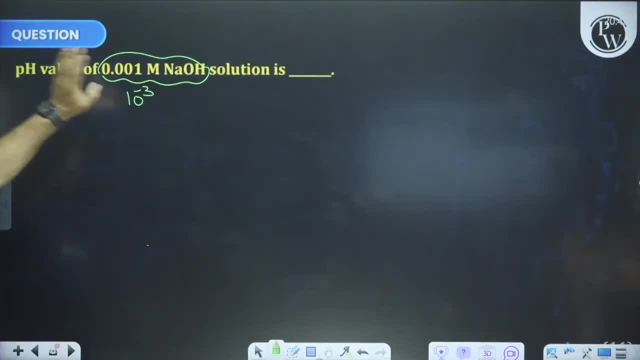 0.001 means 10 to the power of minus 3.. NaOH is a strong base And if NaOH is a strong base then the concentration of OH minus is 10 to the power of minus 3. Means POH is 3.. 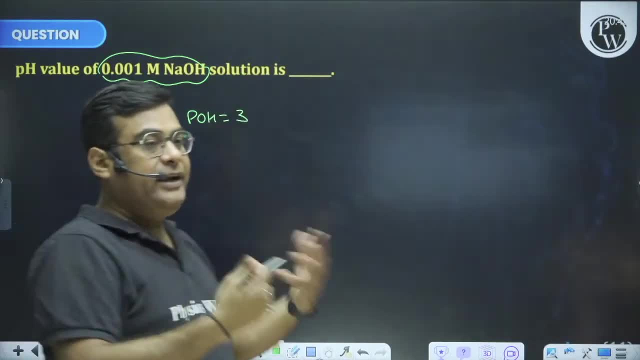 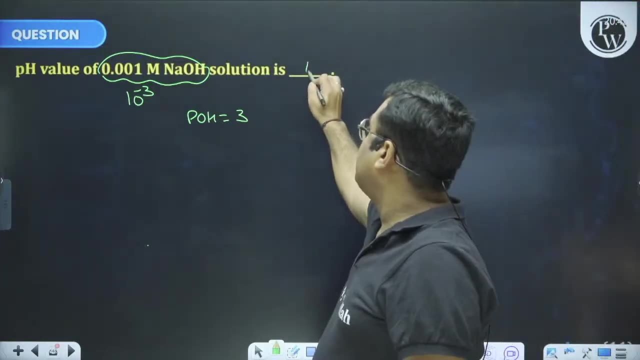 And there are many great souls who do not sit attentively in class or in exams, They will directly tick 3.. But he has not asked POH, He has asked pH, So my answer should be 11.. See, the chat should run like this. 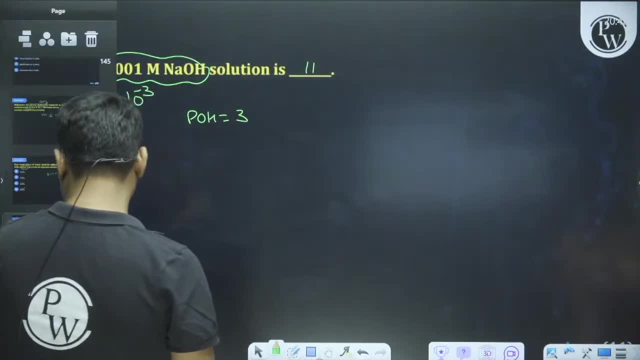 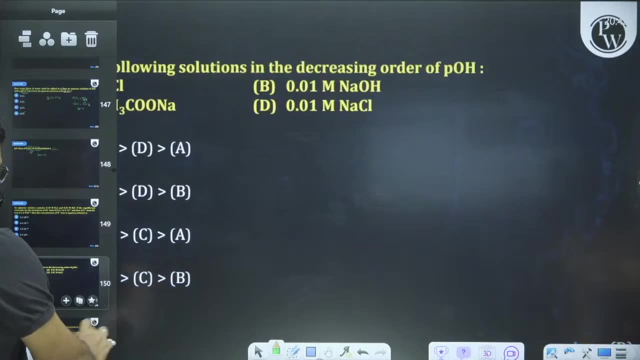 The answer should come like this: Right, So then the fun will start. Okay, Everyone is coming to understand. So in this way you see the next question. Let me show you more. He has asked the order of pH. 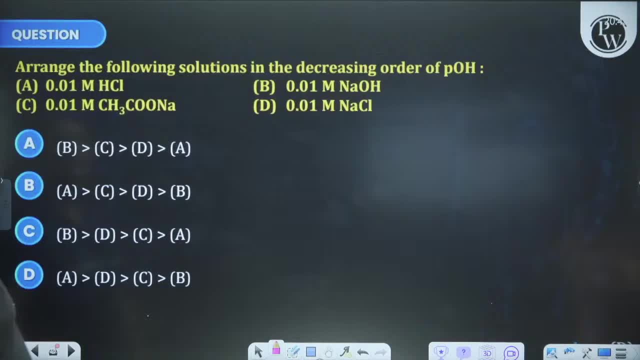 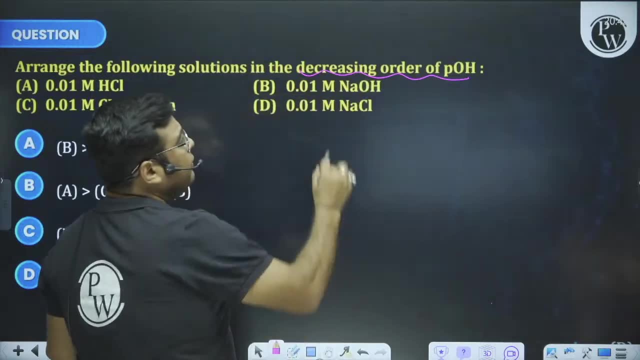 The next question is that he has asked the order of pH from you. Arrange the following solution in decreasing order of POH. Now, here, too many times, The children get confused. Decreasing order of POH means increasing order of whose. 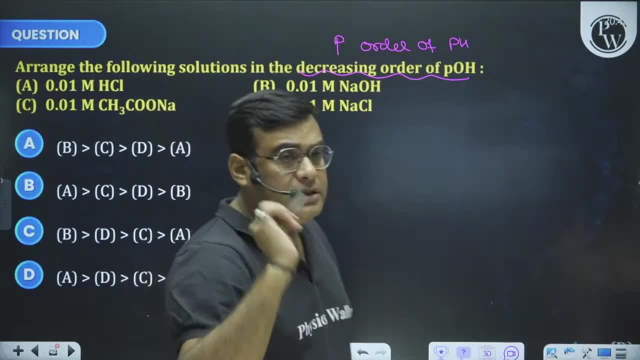 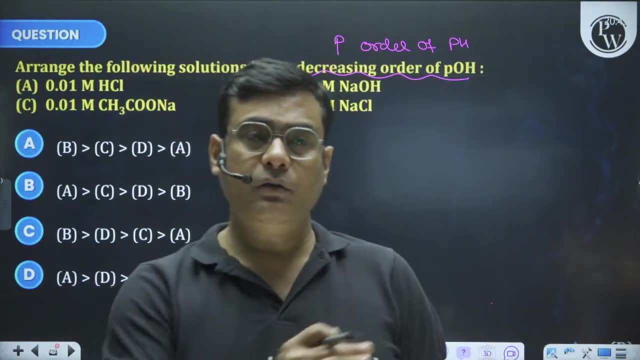 pH. First, even if it takes 15,, 20, 25 seconds, children, it will take you about 2.5 to 3 minutes to solve one question. If we take one question in 2.5 to 3 minutes, we will be able to reduce the number of questions from so many chapters. 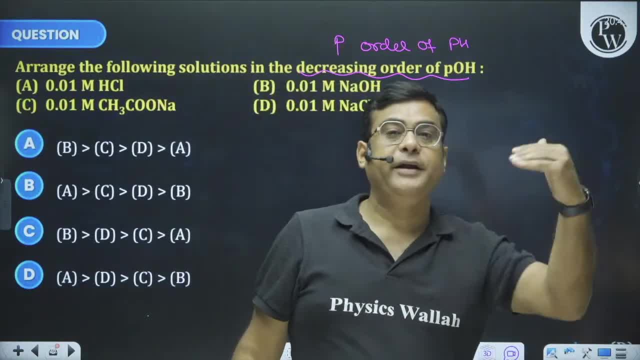 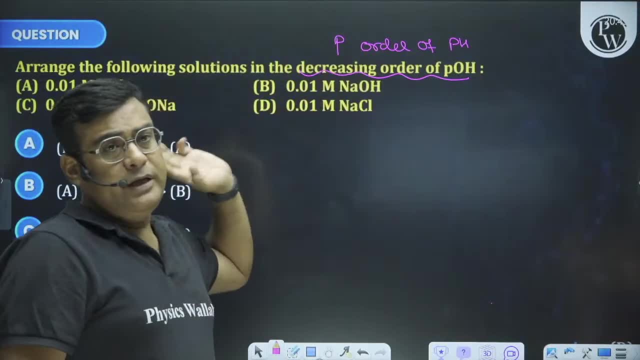 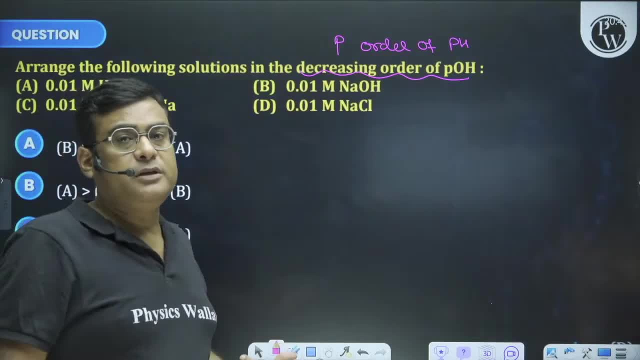 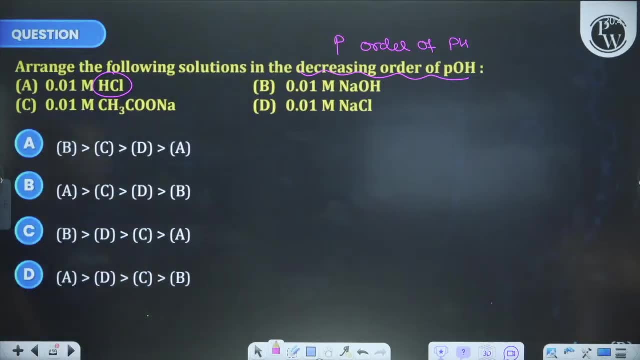 Base, Who would be the lowest Acid? Who will be the lowest in acid, Strong acid, Right. So who is strong acid in all HCL, Sir? strong acid, That's HCL, strong acid. What should happen in the increasing order of pH? 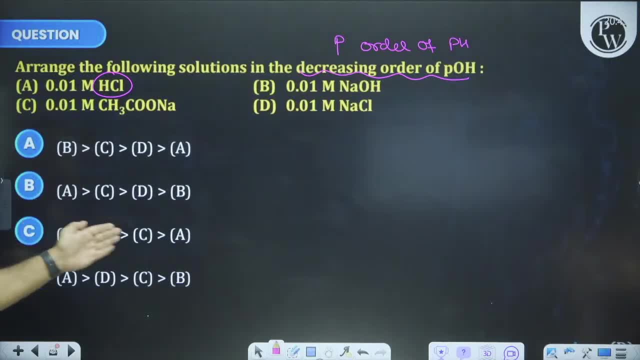 In the increasing order, less than less than should happen, but he gave the answer like this: So let's see the lowest pH of the child Right And the highest pH he has. Yes, Yes, Yes, Yes, Yes. 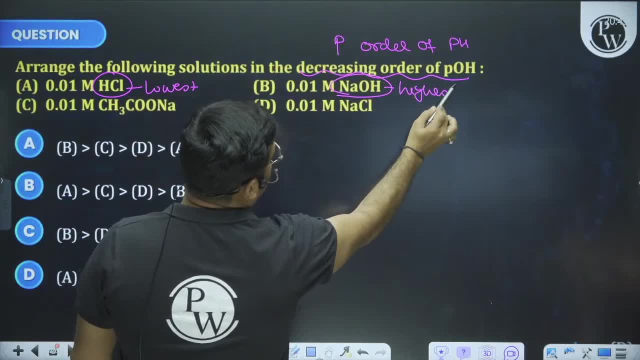 Yes, NACL is the salt of strong acid, strong base. its POH will be more and pH will be less, so the most POH should be of B and the least of A. how to select NACL in COD? NACL is the salt of strong acid, strong base. just now, I had written in the formula that SASB never has hydrolysis, okay, and if it does not have hydrolysis, my dear children, then it always remains neutral. meaning, meaning, meaning, meaning. and when sodium acetate is a salt of 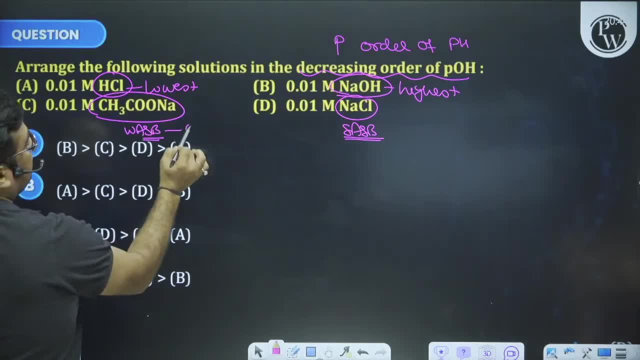 Bic acid strong base. because it is a strong base, then it means that it will be of basic nature. and if it will be of basic nature, then its POH will be more and its pH will be less. then, on this basis, your answer will be B, D, C, A. the story is over, okay, so in this, 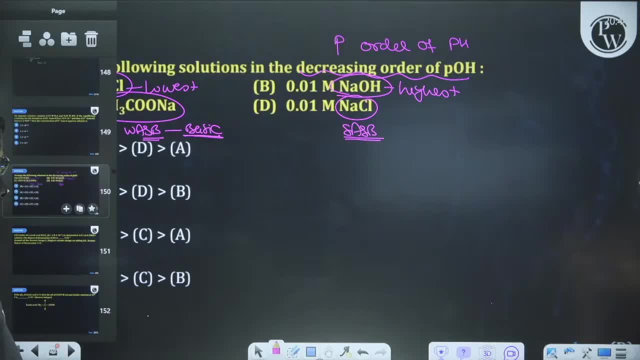 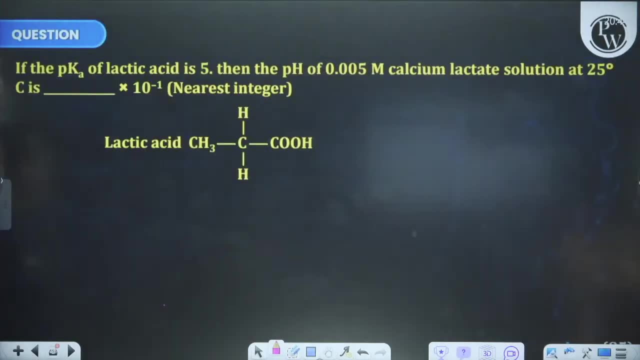 way children look at the emotions of time. we will do the questions, but we will do the same as we did earlier, Like now the question of salt hydrolysis, where the child makes a mistake in this. if PK of lactic acid is 5, now the formula of lactic acid is also given. if it is not given, 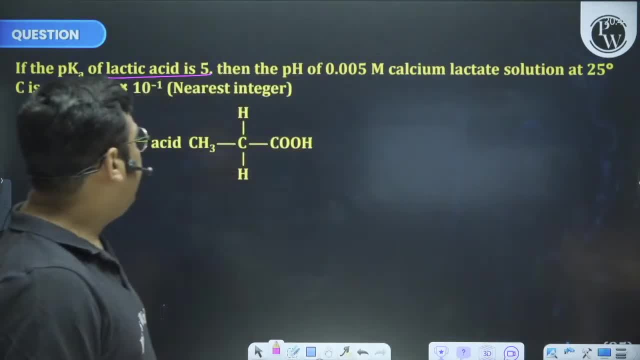 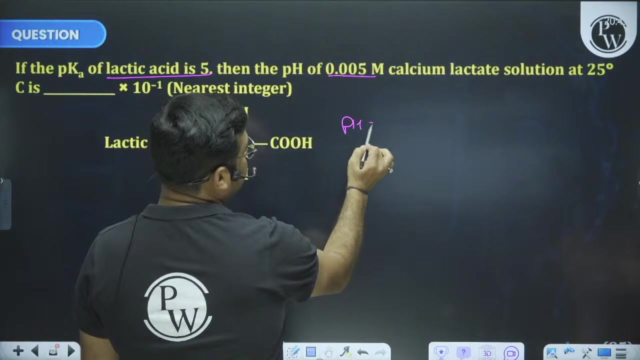 by law, then the question would be better. okay, now he is saying that the pH of 0.005 molar calcium lactate solution is now the child will eat it. that, sir, we have not given the log. we need the log of 0.005 because, sir, you had written the formula of pH half. 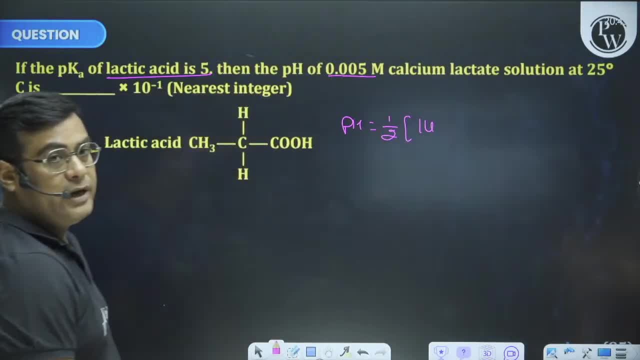 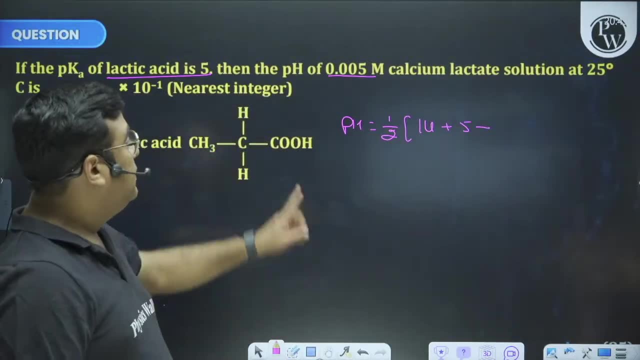 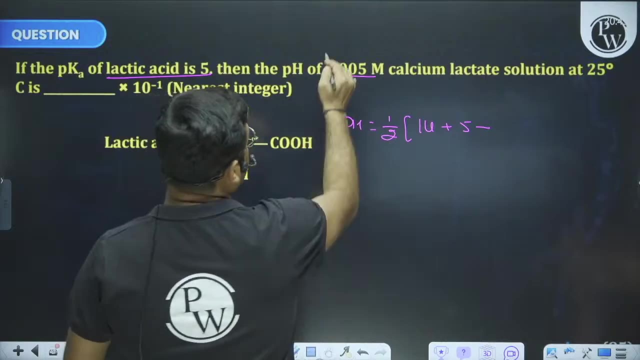 of PKW. That is 14, PKW is 14, plus PK is 5 and plus you had written log C. now C is 0.005, then your question will be wrong there. What is the meaning of calcium lactate, child Ca L, C whole, twice right: Ca L, C whole. 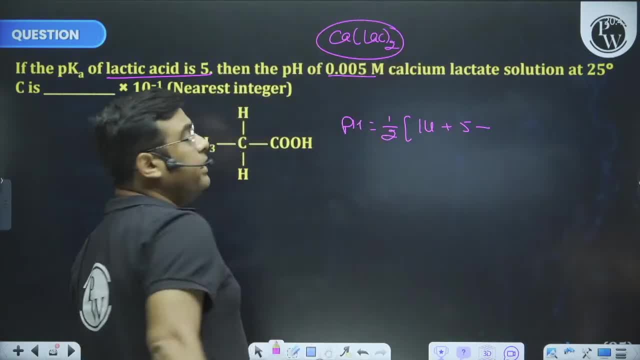 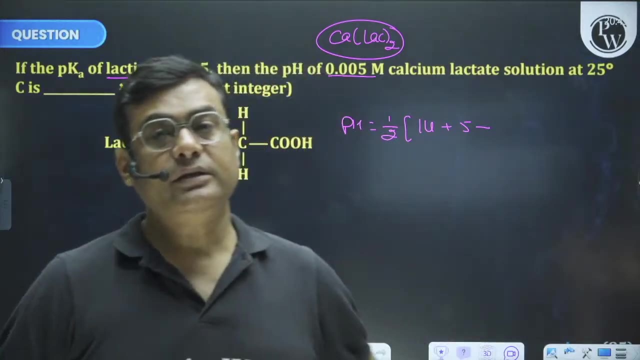 twice means. and the formula we are writing in C, children, right? the formula we are writing in C is Ca, L, C, whole, twice right? Okay, is the concentration of which hydrolysis is happening then here: lactate ion hydrolysis. 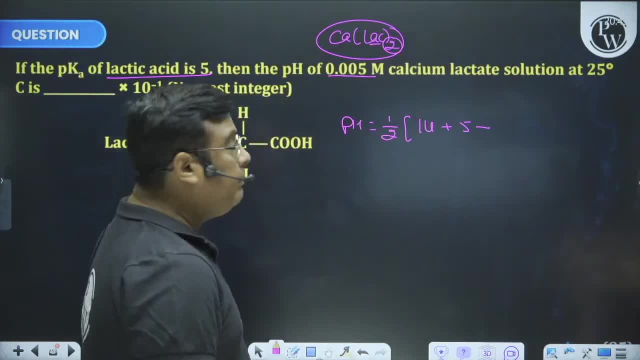 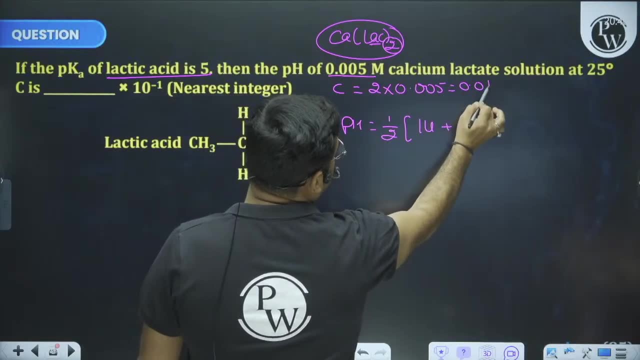 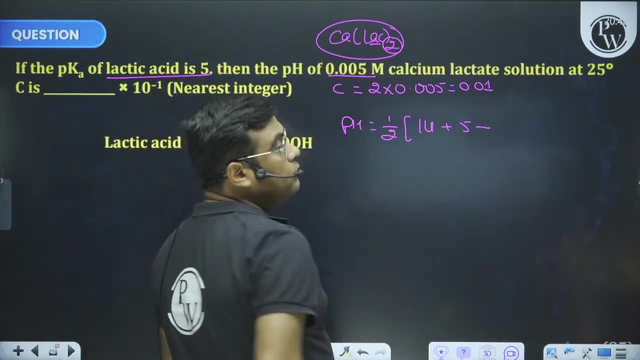 will happen. but since the concentration of lactate is 2, then for me the value of C is not 0.005,, it is 2 into 0.005, that is 0.01, that is how much 0.01? and if it is 0.01, then 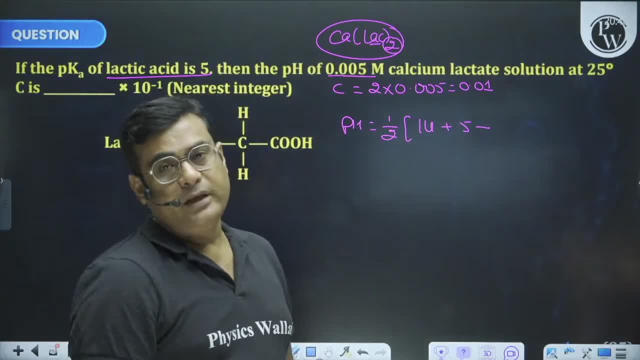 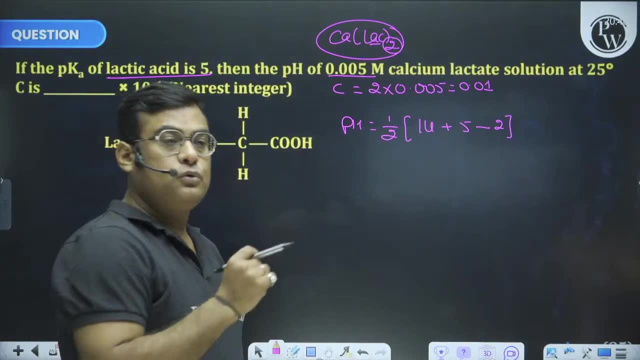 I can write 10 to the power of minus 2 and I know its log. that log of 10 to the power of minus 2 will be minus 2, that is why it has not given the log. then you have to listen to things carefully and understand them. then you will enjoy the question. the rest of the 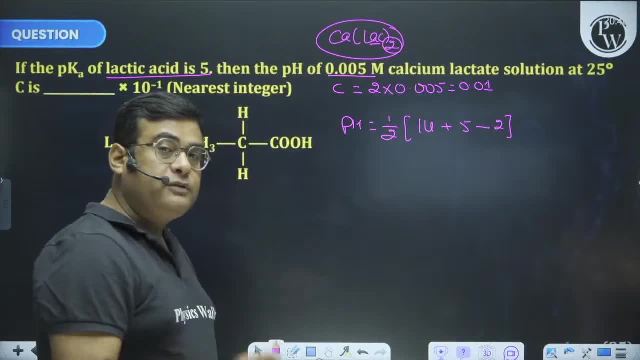 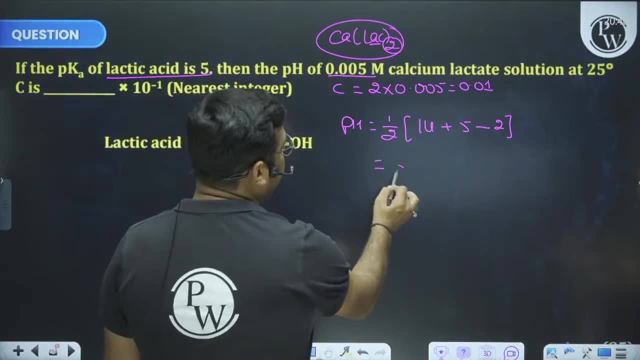 questions were very easy: 14 plus 5 is 19,. the formula will come as the base question. I am giving you the guaranteed written ok: 2 out of 19 is 17, by 2 is 8.5, because it. 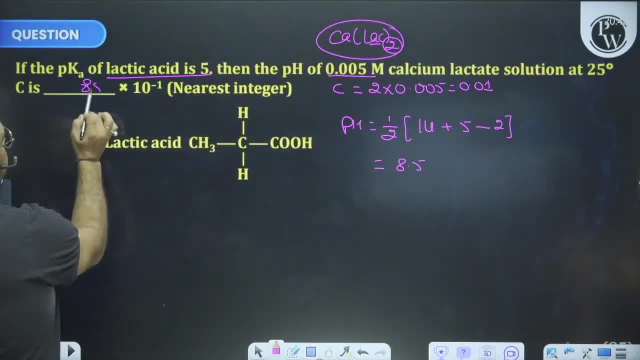 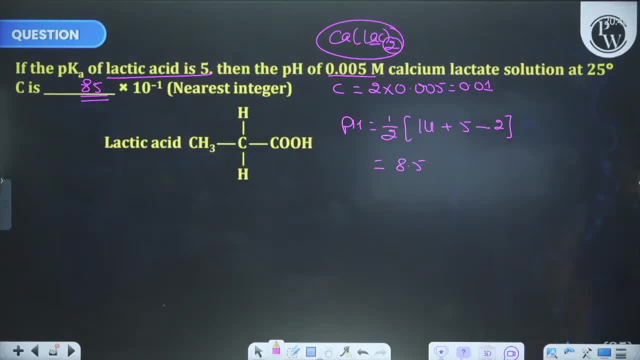 And the answer here is: even if the answer is, and if the answer is correct, this means that 48 ohm is less than green. but if we do not come up with a solution, so we will have to do the same. I didn't give you the answer to the last question. I gave you the order. 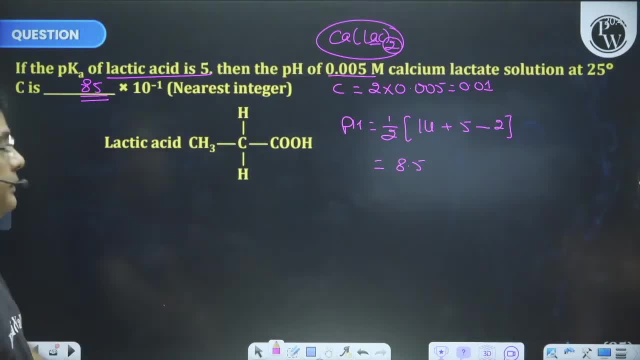 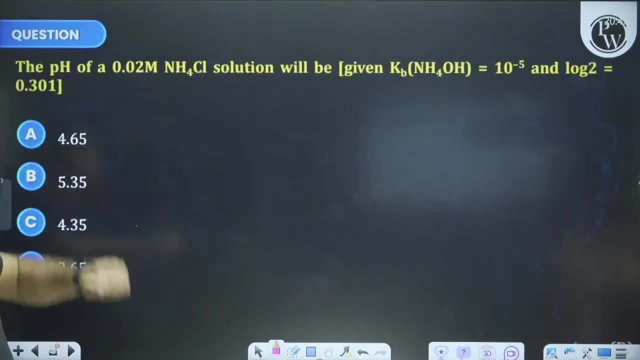 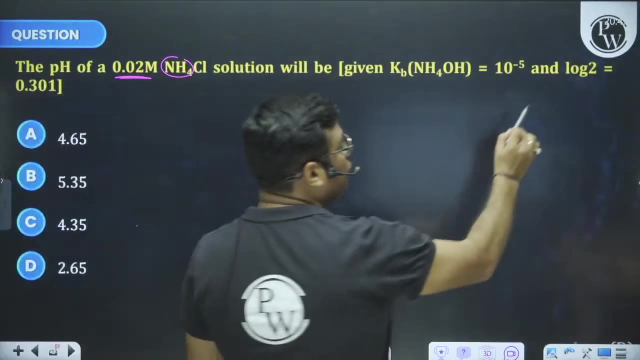 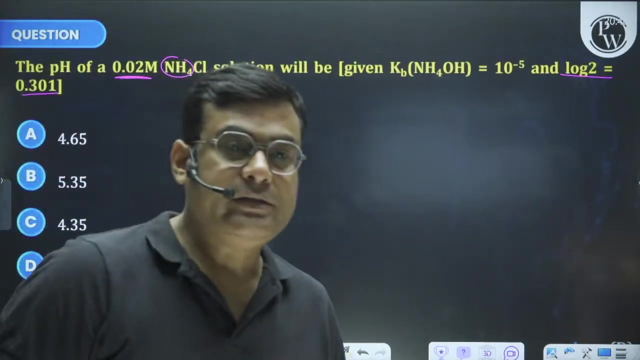 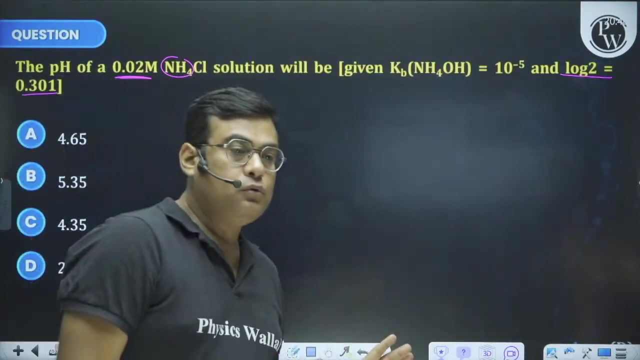 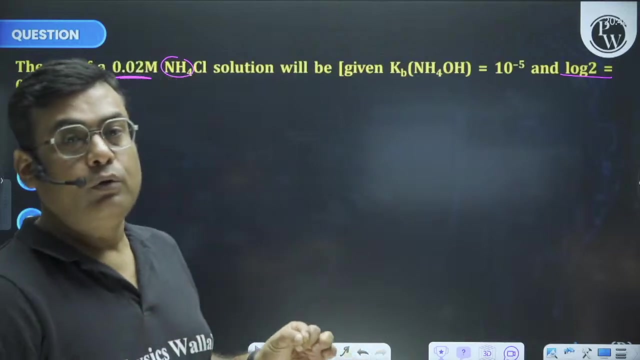 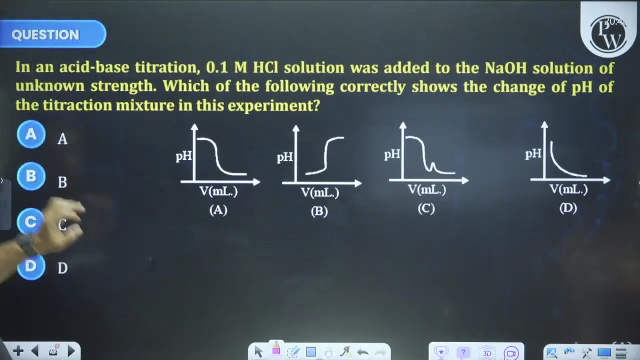 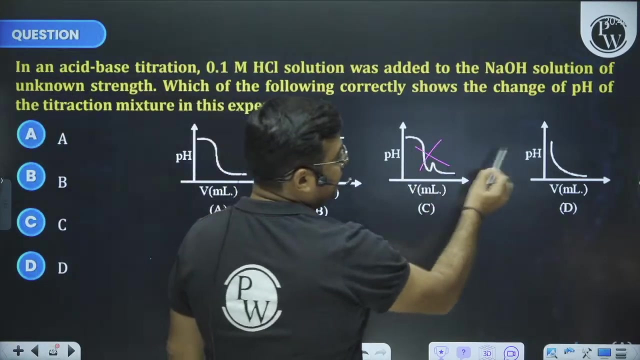 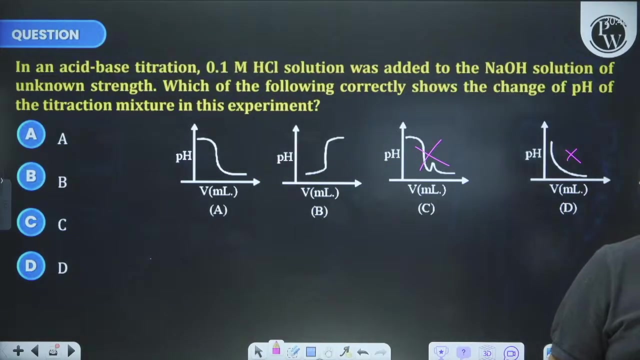 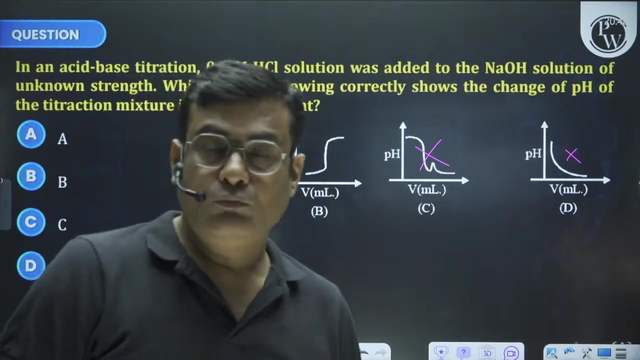 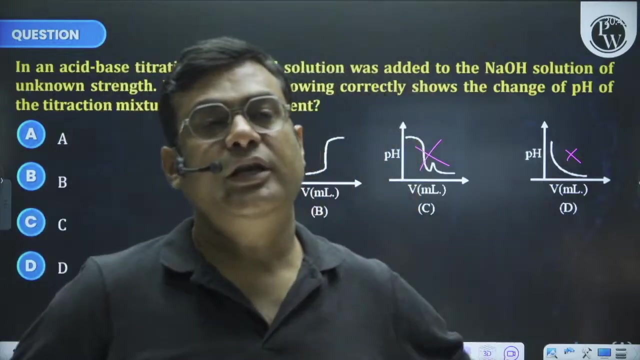 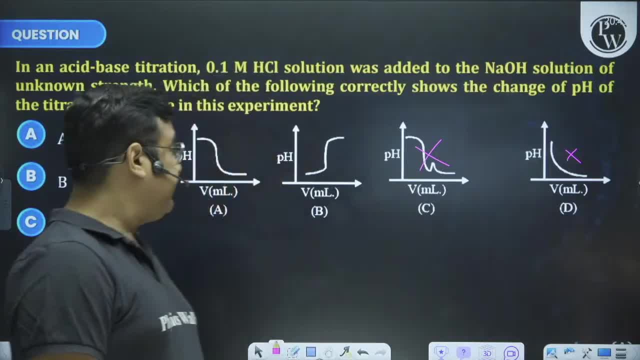 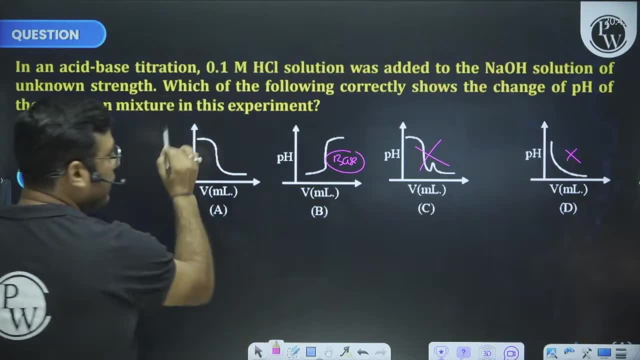 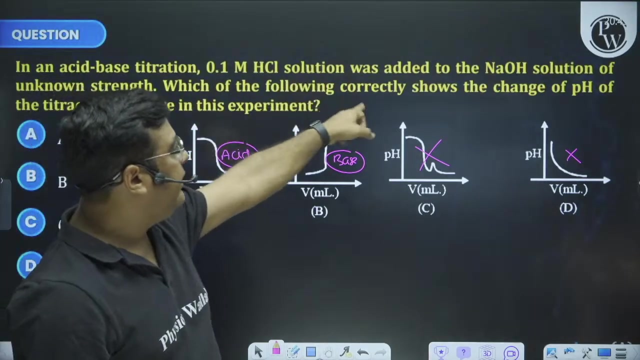 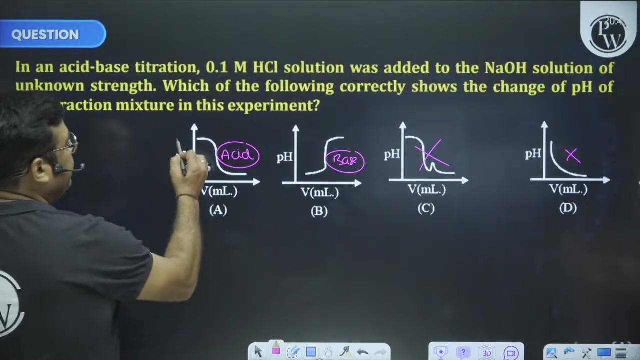 I didn't give you the answer to the last question. I gave you the order: 精 Doo do do Enęp run. 精 doo do do enęp run. Which of the following correctly shows the change of pH of the titration mixture in this? 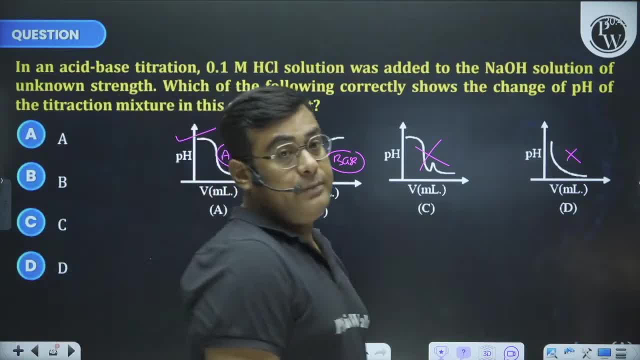 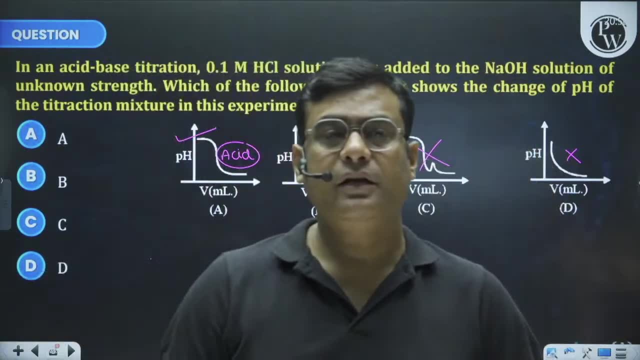 experiment. The answer is A. So sometimes the child is afraid of these graphs too. There is no need to be afraid children. you have studied so much theory, you have been working hard for so long and full of hope. children whose first attempt was not so good. 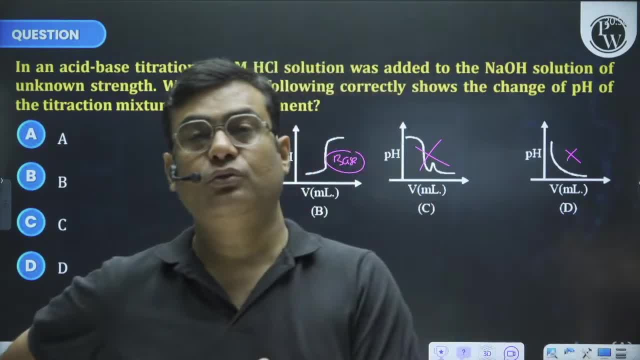 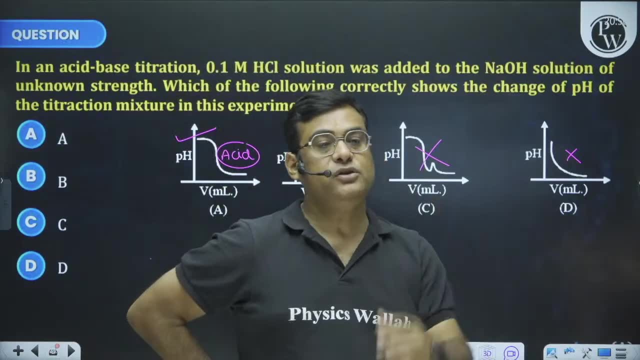 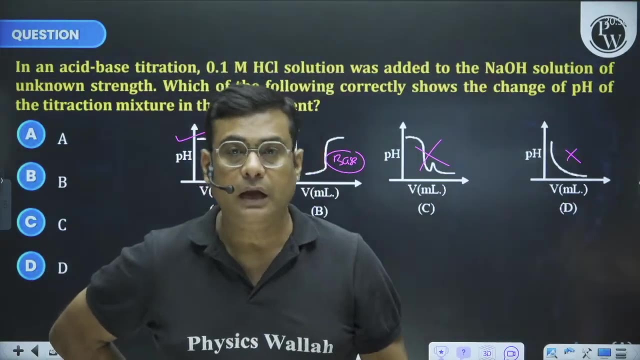 but in these two months he sincerely returned things Sincerely. the whole of February, the whole of March will be over almost tomorrow, so in two months you will have sincerely read things again. child, I have come to work as a little catalyst in your selection, because now I have to give. 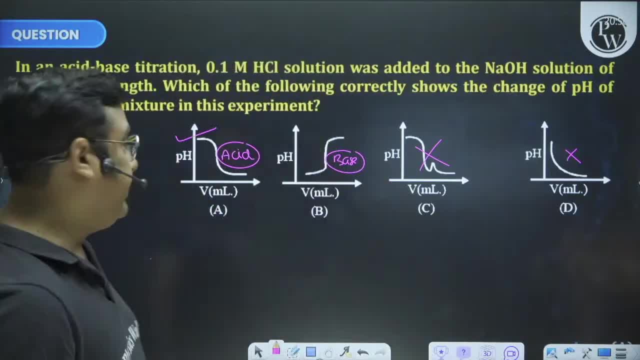 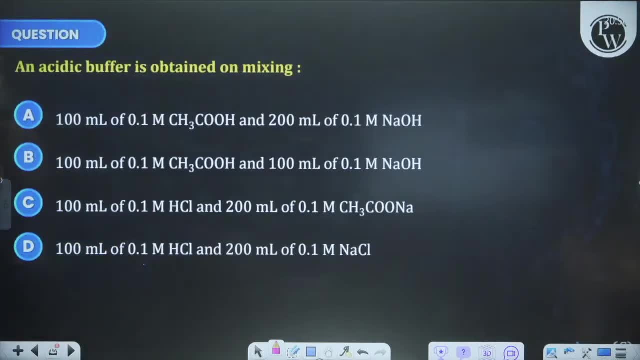 you the idea by revising the theory again through questions. Okay, let's see some questions of the buffer too. Look, the buffer has come. An acidic buffer is obtained on mixing. Now what is the meaning of an acidic buffer In which there is a weak acid plus its salt? 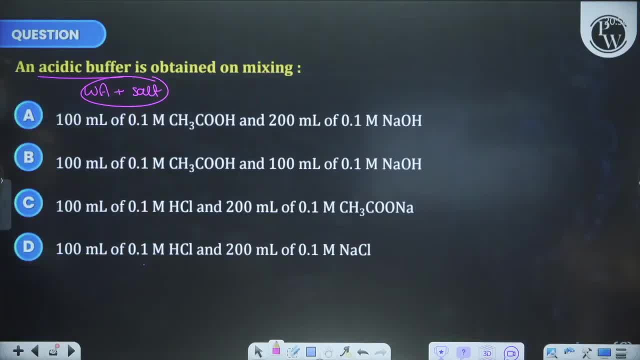 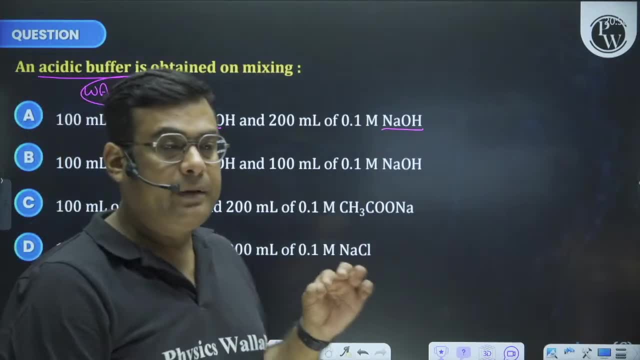 Only then that buffer will be called an acidic buffer. Sir, there is a weak acid here, but it is a strong base. If this is given children, it means that there will be an acid-base reaction here. If this is given, then there will be an acid-base reaction here. 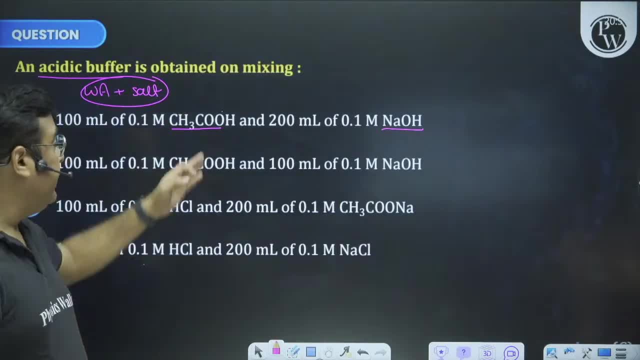 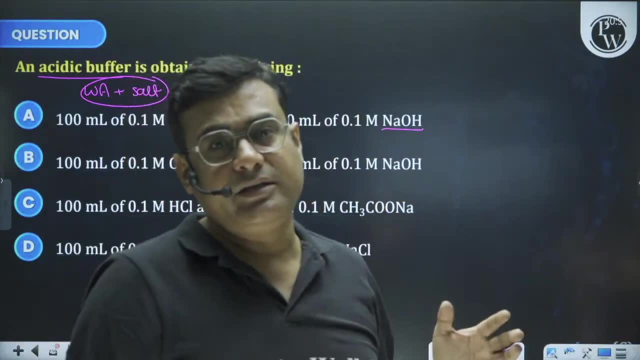 Okay, and if there is an acid-base reaction after this, there is one H. after this there is O, There is one OH. So the reaction does not mean that I have to write the reaction. I have put so much time to check all four options. then my Lanka will sink. 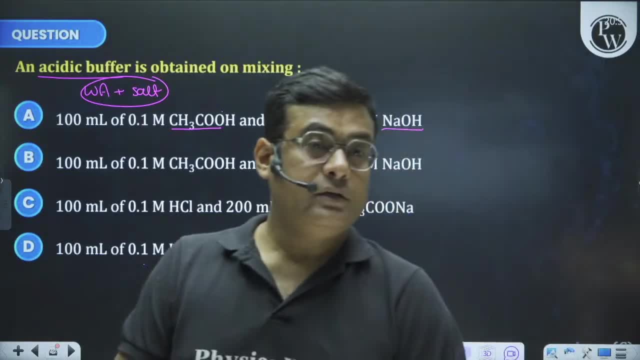 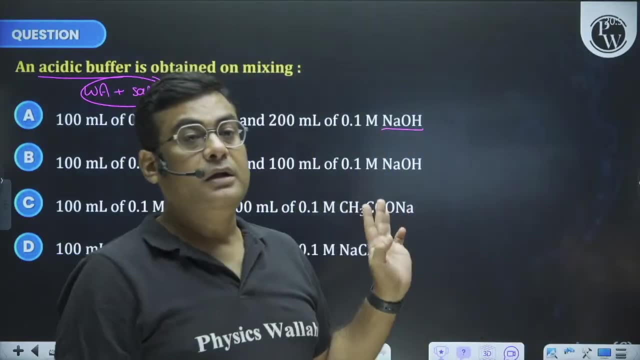 Two questions from the front will go ahead. Whoever has read the chemistry properly understood it will know some JSC in reverse, That time will go ahead of you. two questions in this time. So, sir, what is the technique, brother? 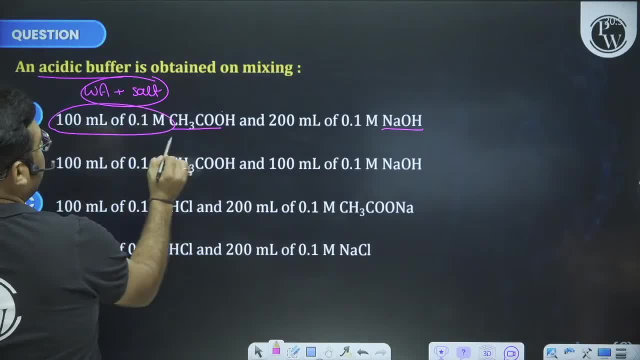 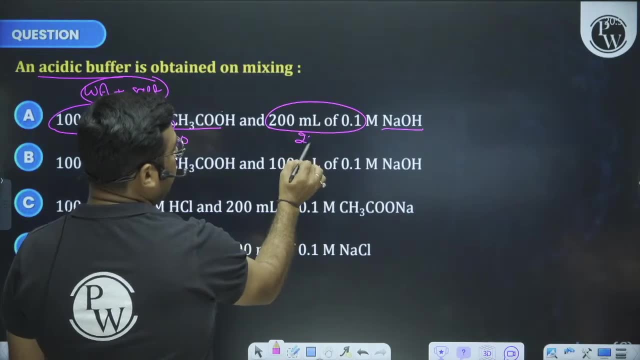 Brother, how much is its hundred into point one? Molarity into volume? we have made 10.. Its 200 into point one. how many have become 20?? To become the buffer it is necessary to have weak acid Here. the weak acid has been finished. it will not be made. 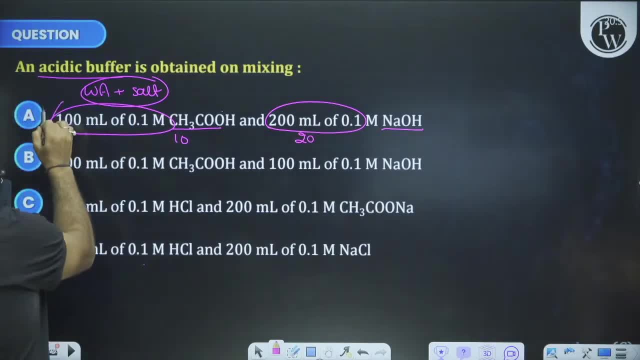 Look again in the next. both 10 are also finished and the buffer cannot be made. It is not. It is strong acid, this is weak acid. strong acid, this is strong base. salt. Strong acid or strong base never makes a buffer. 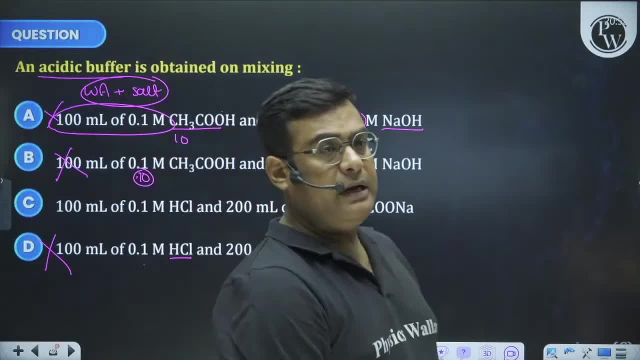 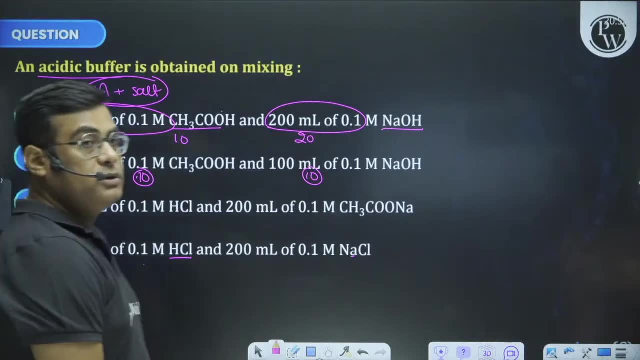 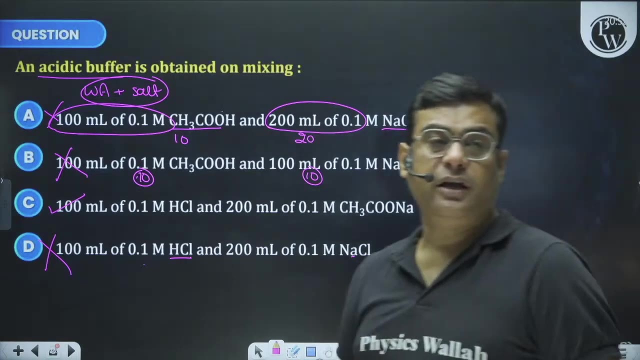 So now we are going to see what happens to these two. So if you consider the JEE paper to be tough, then these are all your JEE questions and you don't even know that so many easy questions come in JEE. I told you the logic in the question without doing anything. 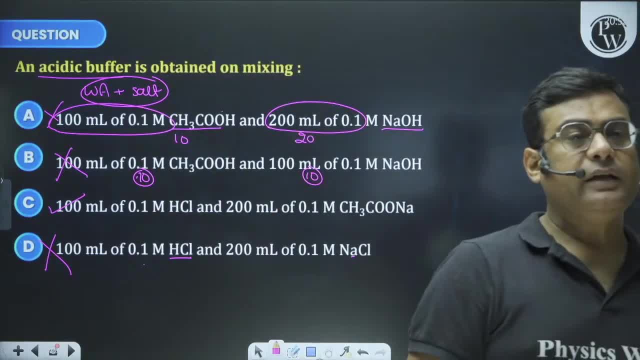 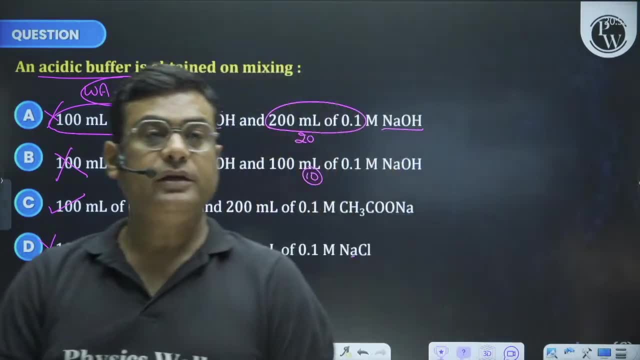 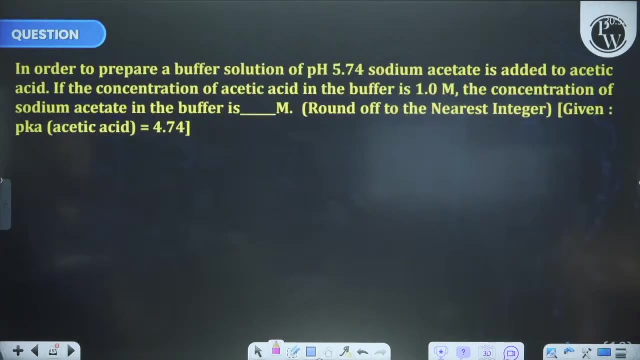 If you want an acidic buffer, then it is compulsory to have more weak acid, Strong acid and strong base. never make a buffer, Or you can get such questions about buffers. In order to prepare a buffer solution of pH 5.74,, make a buffer whose pH is given. 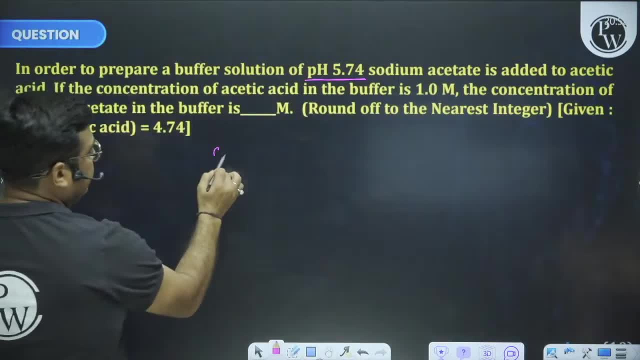 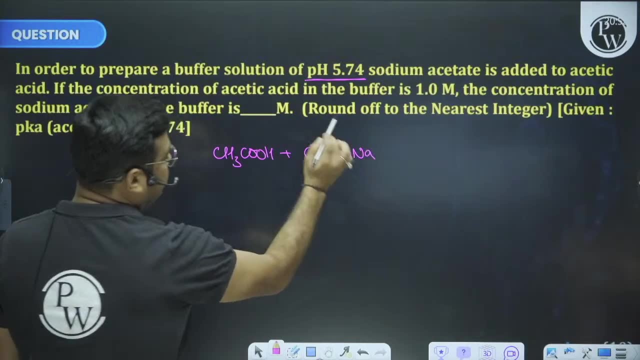 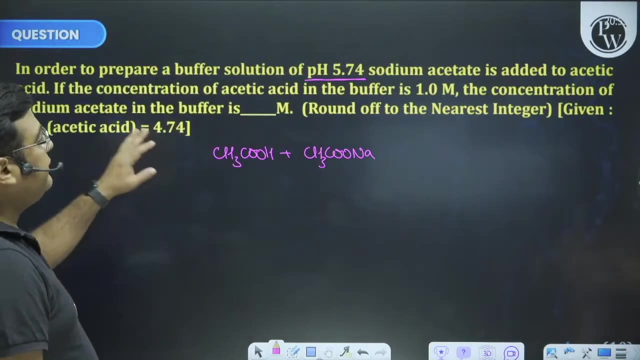 Sodium Acetate is added to Acetic Acid, so we also have Acetic Acid. obviously weak acid and also Sodium Acetate, Weak Acid plus salt with strong base comes. so this will definitely be your buffer. Now he is saying that if the concentration of Acetic Acid in the buffer is 1, then tell. 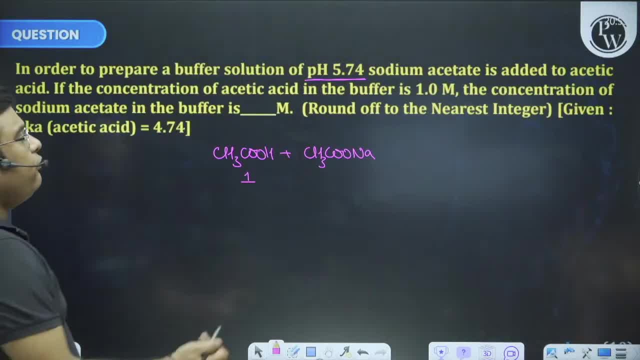 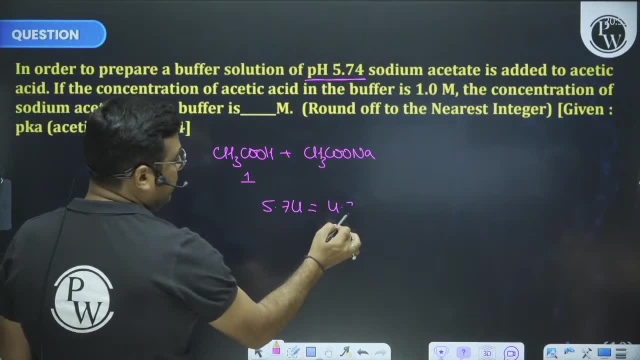 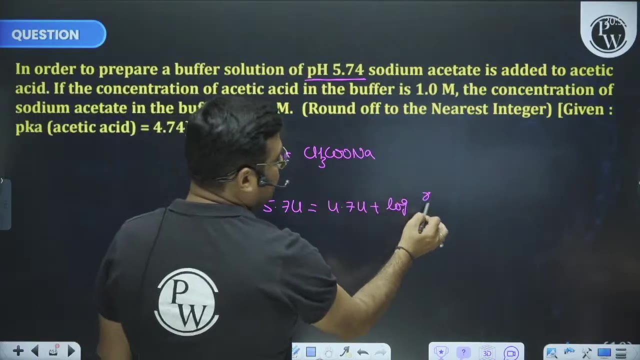 me the concentration of Sodium Acetate. in the buffer Brother you have to apply the formula pH is given as 5.74 equals to pH, equal to pKa, 4.74 plus log concentration of salt, which you need. Suppose X: below is the concentration of Acid, which is 1.. 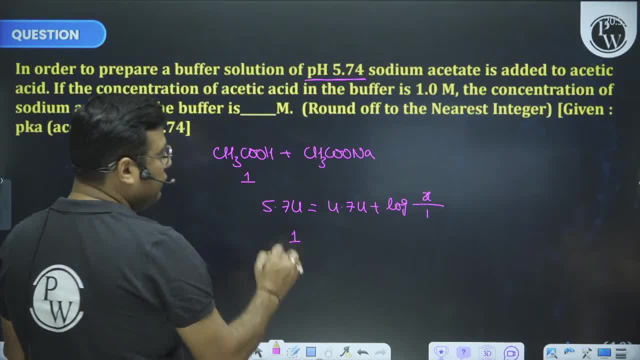 And this goes here Son 5.74 plus log concentration of Sodium Acetate, which you need, And this goes here For 4.74 plus log concentration of Sodium Acetate, 4.74 plus log concentration of dadide. yet I have taken which is 5.74 formed. 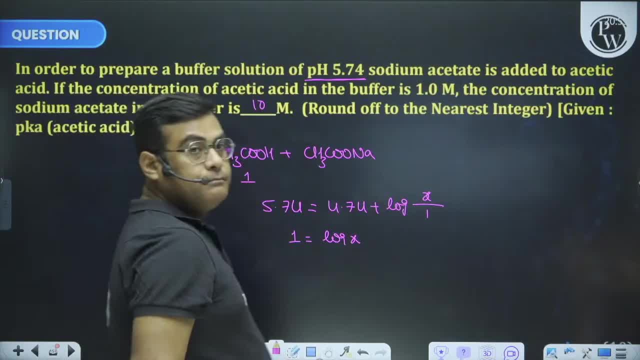 Name 4.74, 1.. If I am going 1 equal to log X, that means the value of X is 2.. 3 Is the value of code 10?. From what you will talk to us, sir, we have a clicker here. I will make hisatives to. 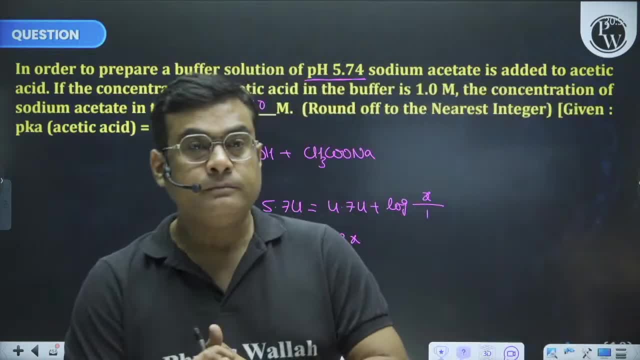 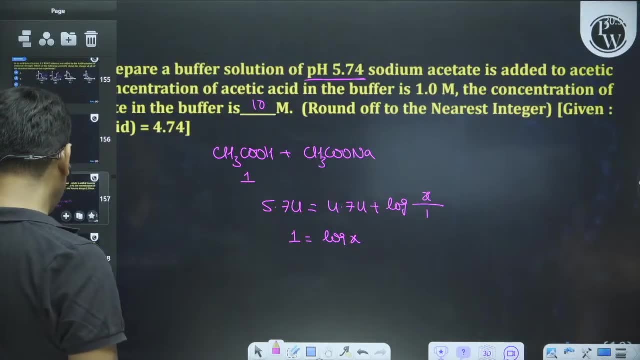 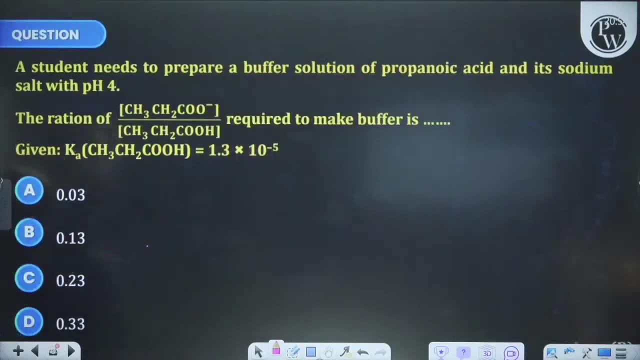 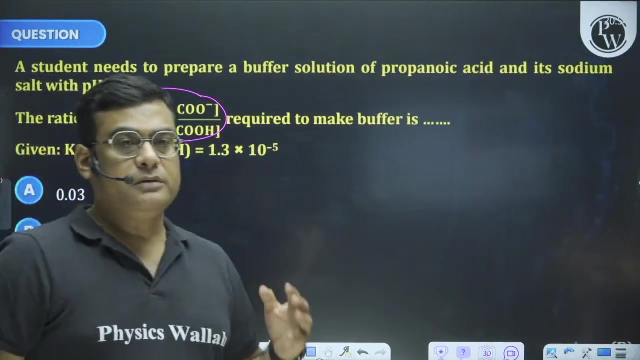 the noise and show you, Brother, Sir Max, school is up to 9.. It will be up to 9, son. You understood the story. you understood the story. okay, keep doing this way, keep understanding the questions, you will never feel any trouble in anything. now look at the same buffer. again, he asked the ratio in one question, that is, he asked the concentration of one. now, again, he gave you PH4, right, he asked the ratio by giving K. again, you just have to apply the formula: PH equal to PK plus log of sir. tell me anti-log. please come in this. 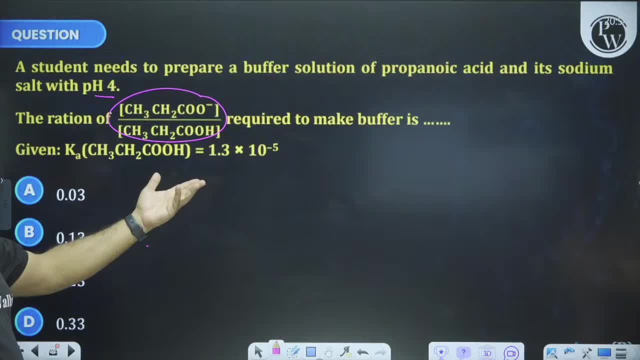 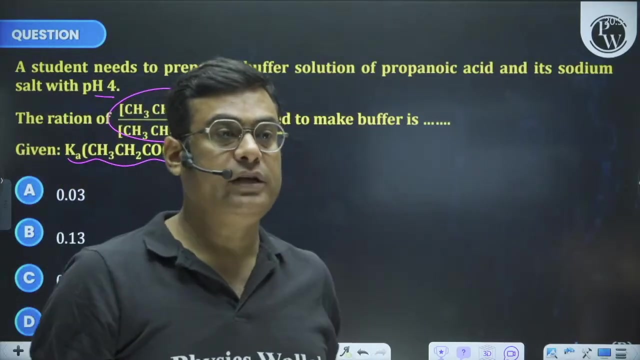 tell me anti-log. you called and we came. now what did you say in? this student needs to prepare buffer solution of propionic acid and its sodium salt with PH4, so PH4 equals to PK. now look what he did. he gave K and along with that you did not give the value of log 1.3,. you had to listen to the sincere children who are in the exam, right in the exam. you have to go sincerely. 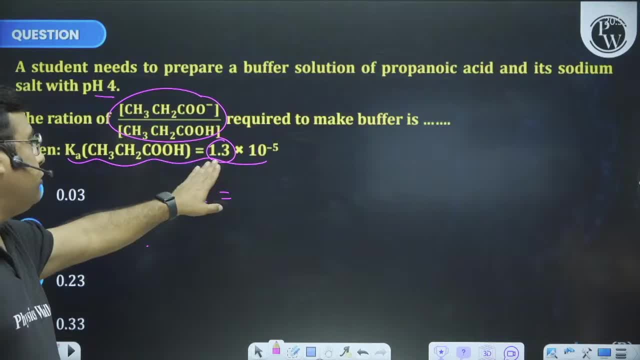 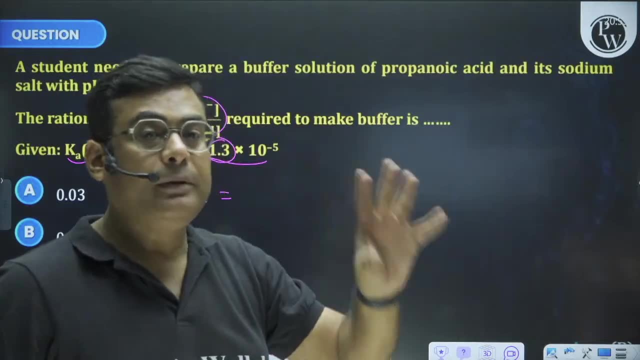 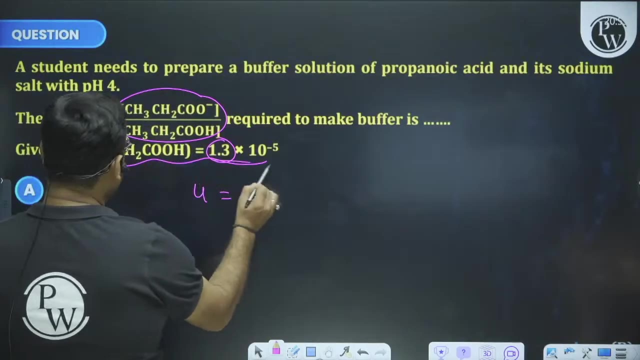 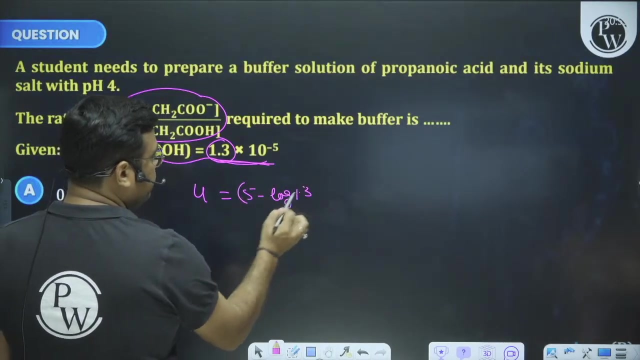 understand things. so if you are seeing the value of the log in any question, that I needed it and did not give the log- I am talking about the buffer- then it will not be given when the log will automatically cancel out. right, like 4, equal to now its K. is this much then what can I write? PK? now I told the method that the power of 10 is PH and H plus right. take the power of 10 separately minus the number right. 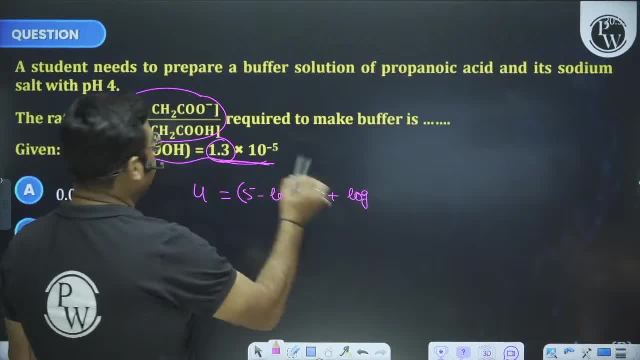 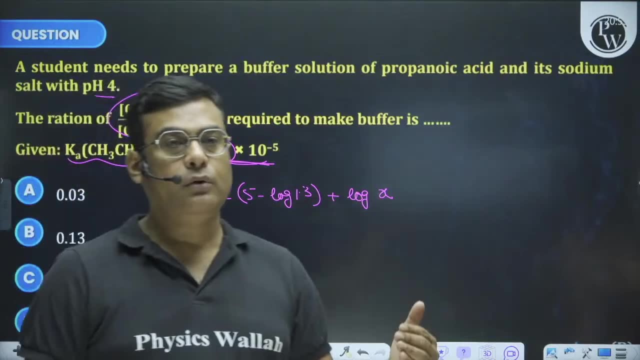 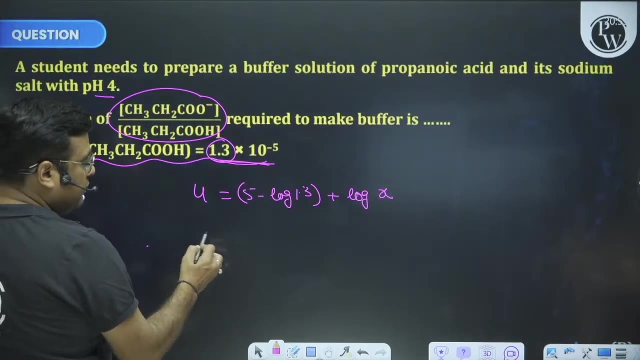 plus log of what plus log of this? above the concentration of salt, below the concentration of acid? by writing it again in this way, there is no need to quote your time. we have written X right now by going here. this 5 is minus, then minus 1, and this log has become minus children. it has become plus agreed equal to log X. now children think that I did not give the log. how do I solve, brother, minus 1, do I give log of? 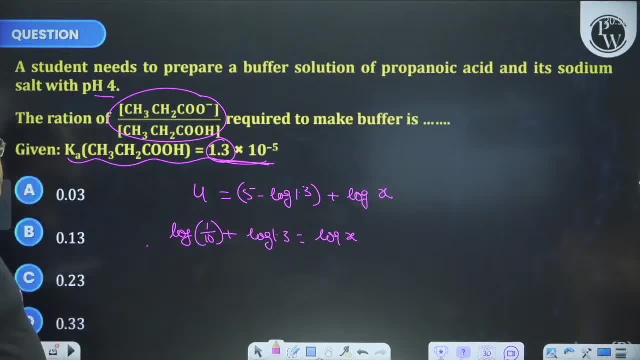 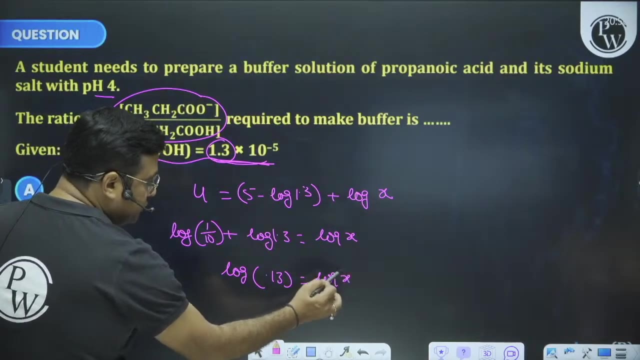 I can't write 1 by 10,. I can write, brother, mathematics is yours, right, mathematics is yourgest, is it now? what does log A plus log B mean? log of AB 1.3 by 10 means 0.13, equal to log X, and if I take entry log, then the value of X is 0.13,. okay, so please, I am telling you that, brother, in the question of buffer, if by mistake, right, if there is some error. so if you do this OKstep, then you will get this value mom uploaded. ok, let's see the solution. OK, I will not send buffer in the test. so the question of buffer: if, by mistake, if I do some error, but I have done- then isn't this recurring tex which shows here, then what will be the tex? ok, raise up. I want to write this afteringe on the question of buffer. 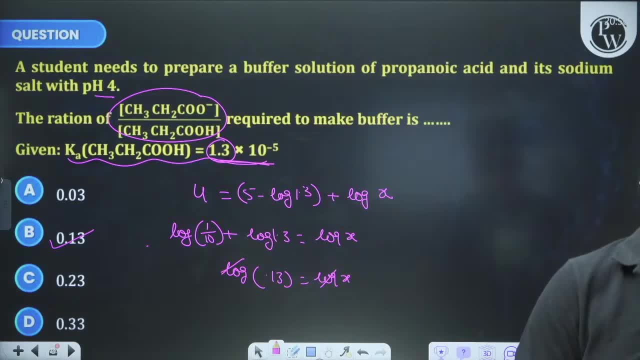 So if By The unified constitution- please- you are random- have done so, you have to keep in mind that there is nothing like this. ok, so this thing, you will keep a little attention that you know every situation, children, you know every situation, know that brother in what way if? 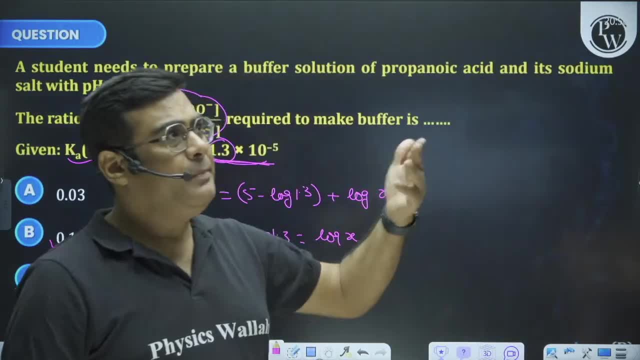 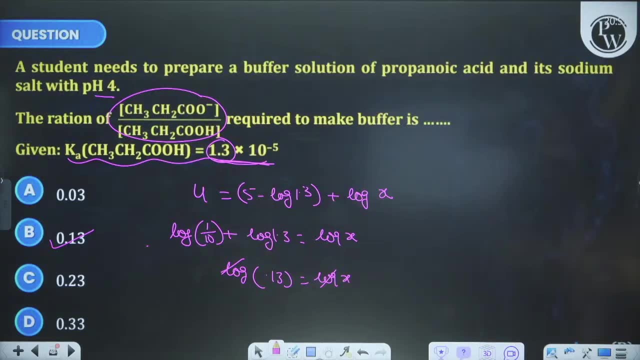 If you have not given a log walk, then there is no need to be afraid. my son is not ill. it is going on like this, so maybe it is cold. the rest is like this: I am all good with all of you. God, everything is fine. then it will be a little cold because of the AC running. 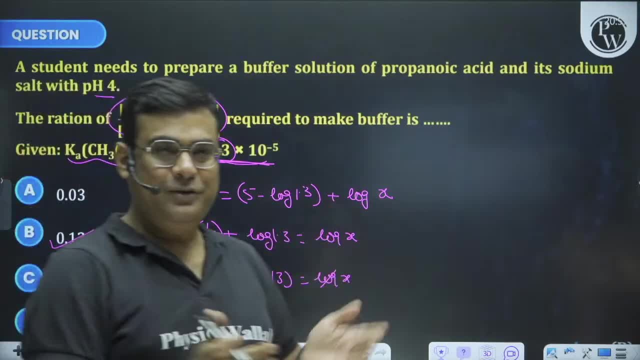 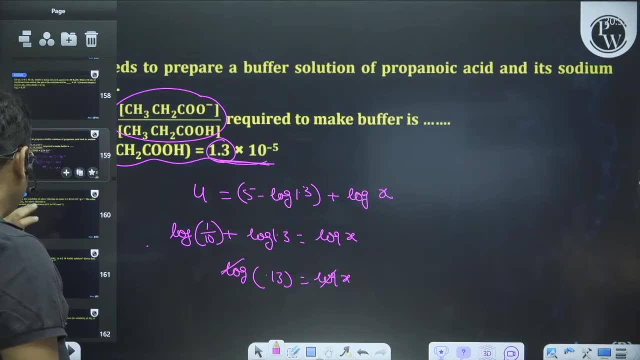 nothing else. everything is ok and you guys pray that everything will be fine. right, some medicines say some prayers. ok, and come on, we also look at this premise now. see the question of solubility. if we talk about the solubility, then the question of solubility. 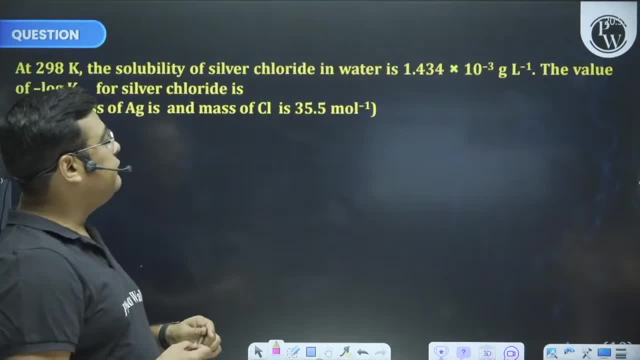 is also simple. at 298 Kelvin the solubility of silver chloride in water. if it is so much, then the value of minus log KSP. you see, now see the button. you must know that AG has not given the molar mass of AG. 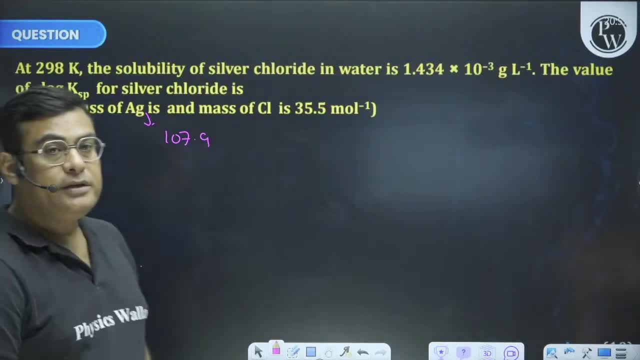 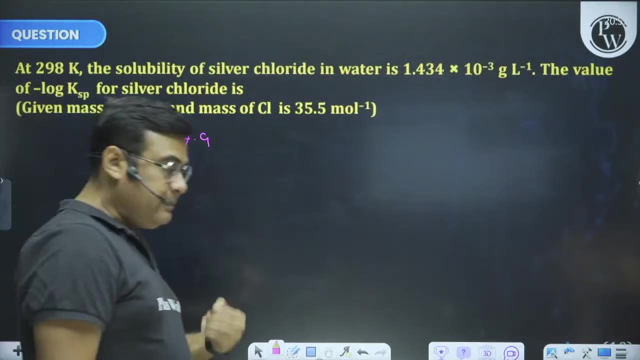 107.9 is normally the molar mass of AG, which happens, which is 108, but in this question, right in this question, they had given 107.9, which by mistake was missed by my operator. then how to make an acidic buffer, son, for an acidic buffer you have salt with weak acid. 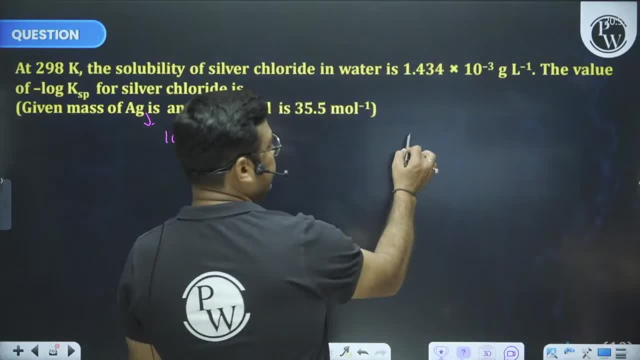 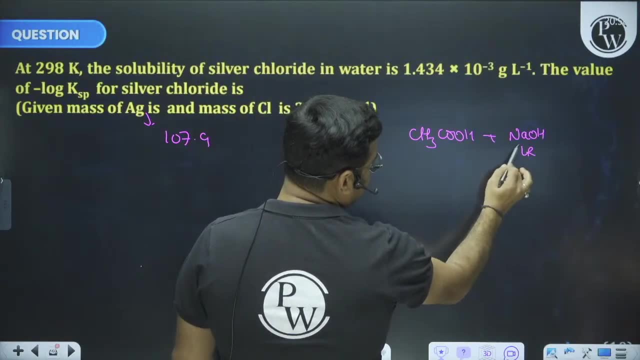 right. like weak acid, you have acidic acid. it is not when you put the NAOH in it, and the NAOH should be the limiting reagent. if there is a limiting reagent, then what will happen? it will end then when the acidic acid 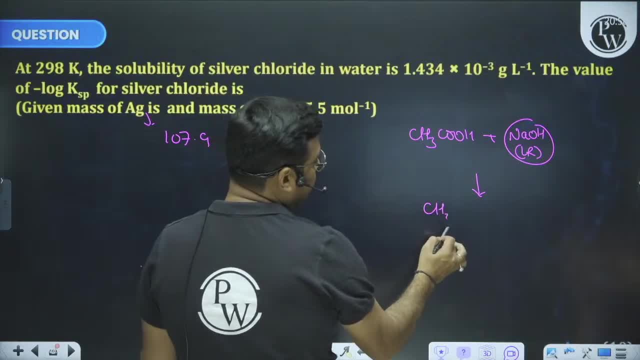 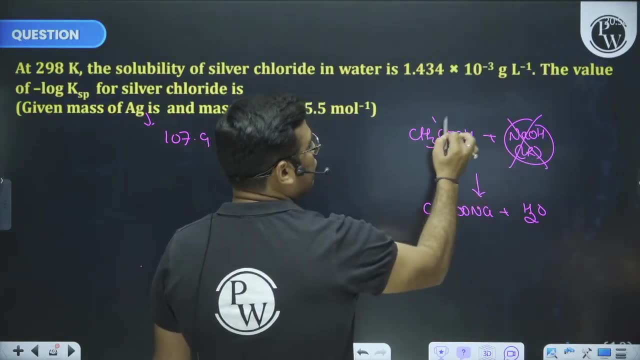 reacts with the NaOH. so it makes what TS3, COO, Na plus water, right. if it is the limiting reagent, then it will end. then you see, with the help of weak acid, what has come, kids salt has come- and with the help of weak acid salt has come, which means it became your acidic buffer. now see, if we go to the solution layer, then we have salt Right now. when we go to the solution layer, it is the AWL. we go to the solution layer. 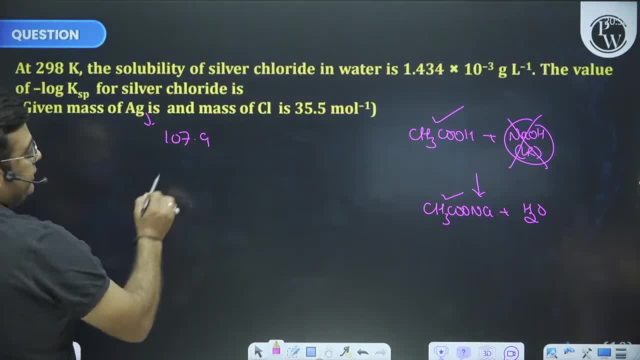 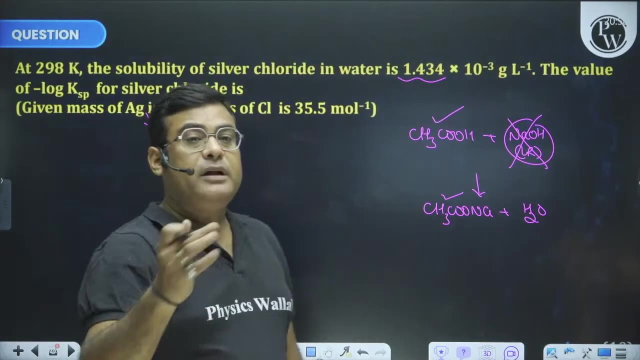 I am saying this because if I take out the molar mass of AGCL and add it, then 9 plus 5, you find the calculation difficult in the questions of JEE. it seems that there is such a bad calculation. Looking at this data- 1.434,. if I were you I would also get upset sitting in the exam. 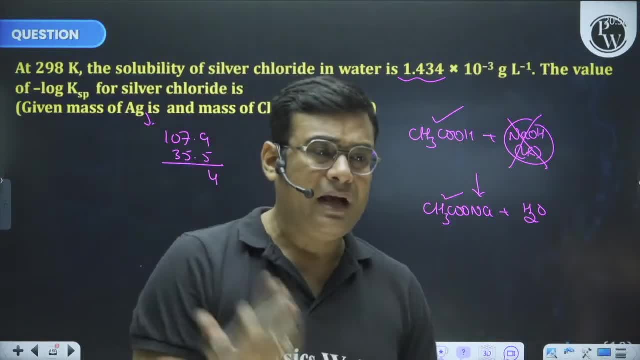 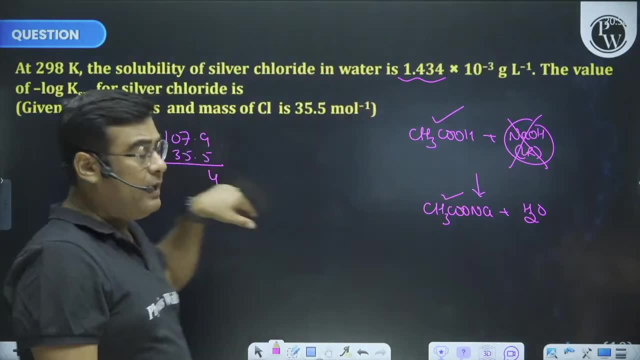 I mean I feel like getting upset that R has such a bad value of 0.0821.. So it has been given purposely because, if I look here, 9 plus 5 is 14,, 7 plus 5 is 12,. 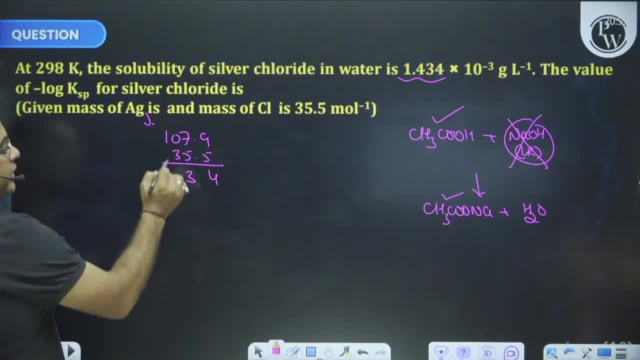 12 plus 1- carry forward- is 13,. 3 plus 1 is 4 and this is 1.. You see, its molar mass has come to 143.4.. Its molar mass has come to 143.4.. 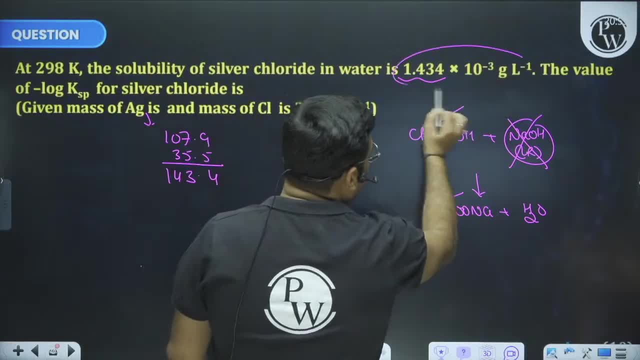 So why has it come? Because the unit of solubility given here is in grams per liter. When it is given in grams per liter, it is given in grams per liter, But the solubility should always be in moles per liter. 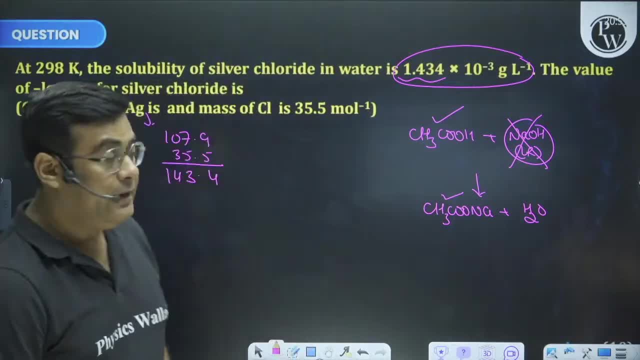 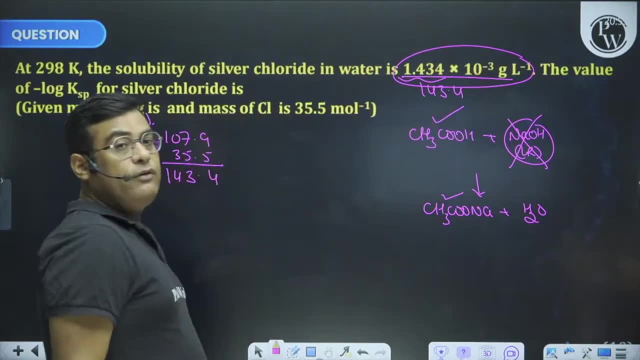 And what should the solubility be in In moles per liter? So if I have to take it out in moles per liter, then I will have to divide this value from its molar mass. That was the purpose that they have given 1.434.. 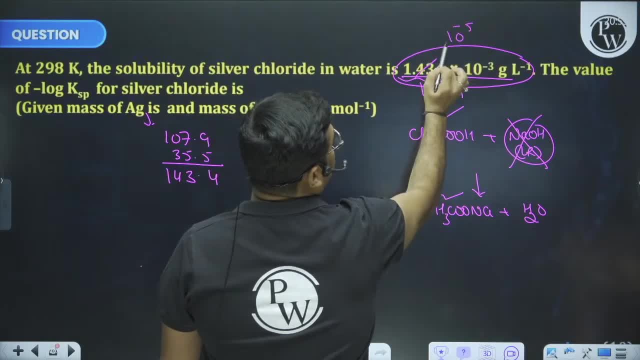 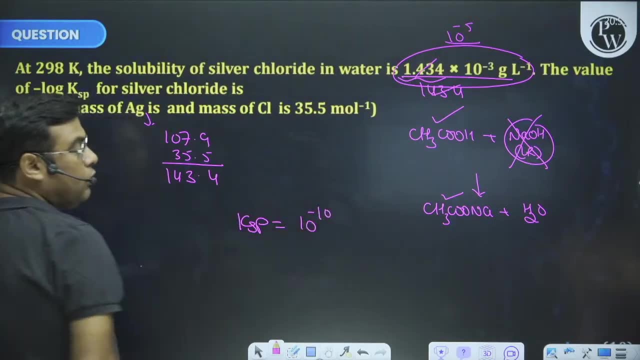 So now this is 1 by 100, which means you have its solubility 10 to the power minus 5.. So if you take out its case from this, then it will be 10 to the power minus 10.. And who did it ask for the value children? 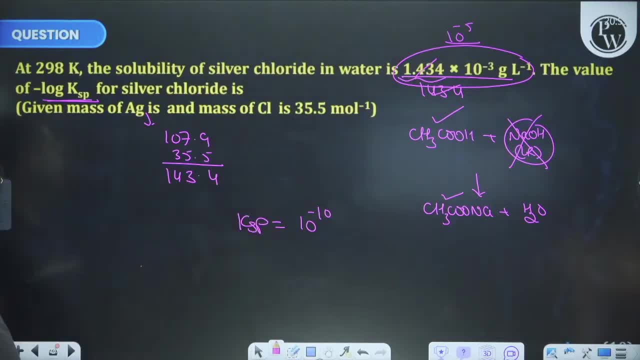 First take the log, Log KSP. Take the log and then minus 10. Then you have removed the minus as well. So the answer is 10.. Now, if you have learnt how to make an acidic buffer, then make a basic buffer also. 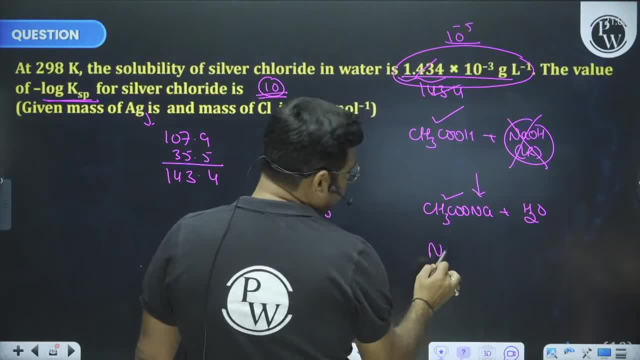 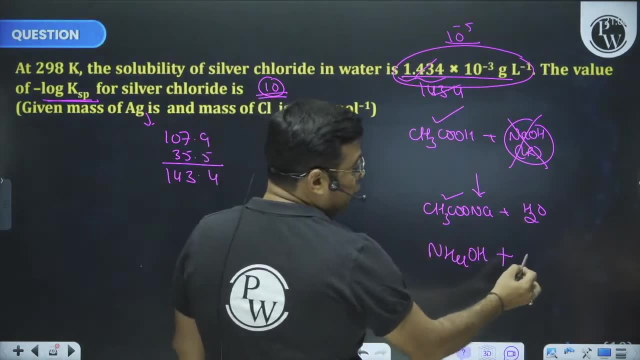 For basic buffer. take the base, weak NH4OH. Why are you getting so confused? You can learn only one thing: The other thing will have to be implied. And put strong acid in it, HCL, And limit it. Do this. 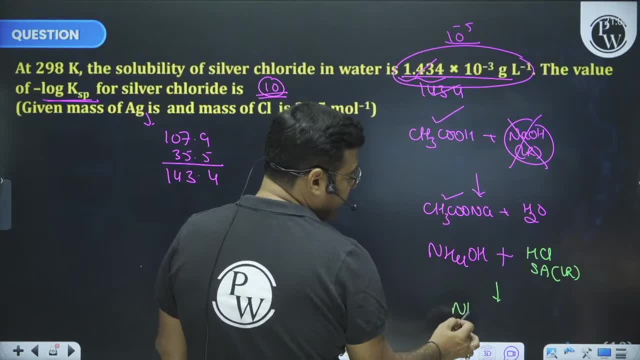 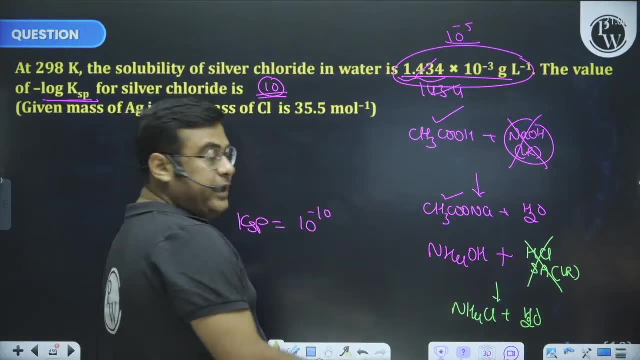 So if this is the limiting reagent, then what will we make by making NH4OH and HCL react, NH4CL plus water. If this is the limiting reagent, then it is over. Okay For basic buffer weak base and its salt should be there along with it. 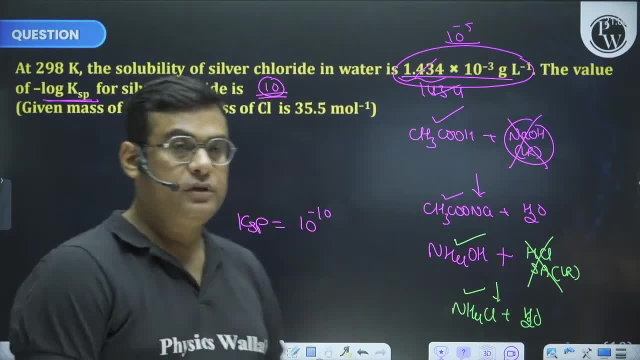 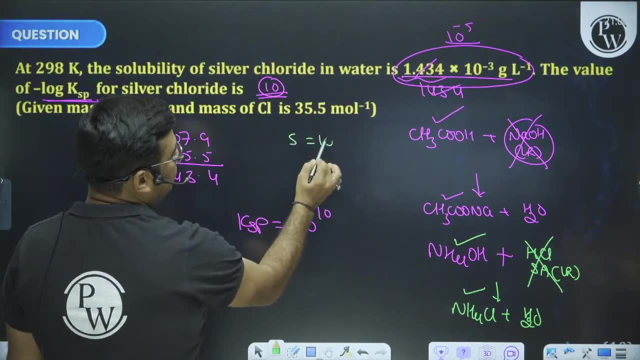 This came For basic buffer weak base and its salt along with it. Okay, Okay, Okay, Sir. how? 10 to the power minus 10?? Now I have told you the solubility S children: 10 to the power minus 5.. 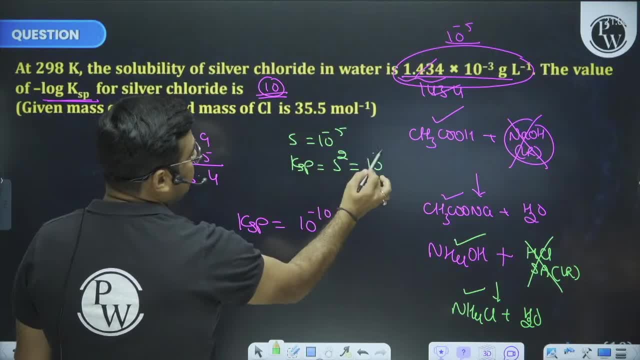 And KSP is equal to S square. That means S square is equal to 10, to the power minus 10.. And have a little shame, children, Because after four days you may have to give the paper I don't have to give. 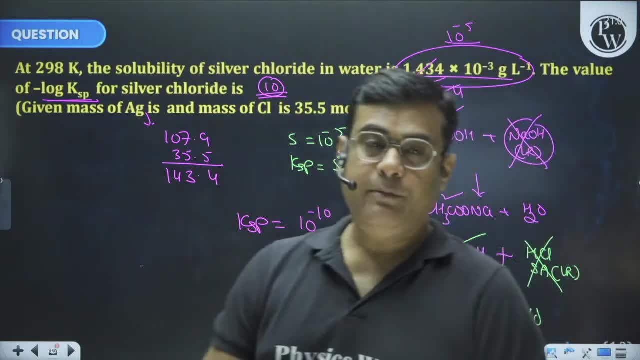 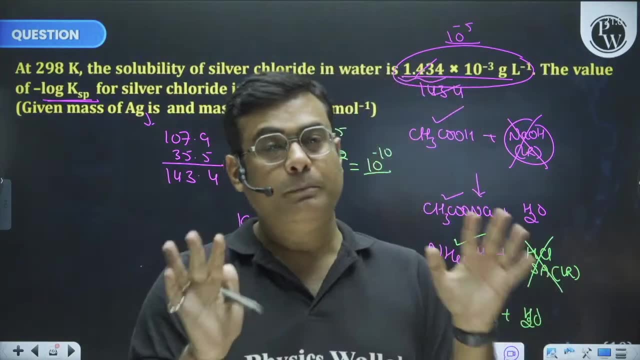 Those who are asking for this kind of dog acidic buffer. There is nothing to tell me. I will tell you as long as you want. When you don't feel like talking nonsense, it's a different matter. Okay So, but you should also have a little shame. 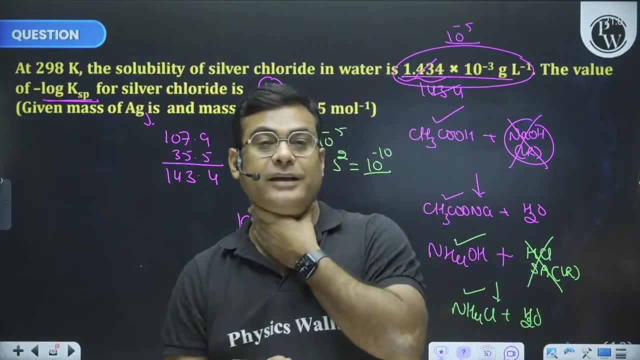 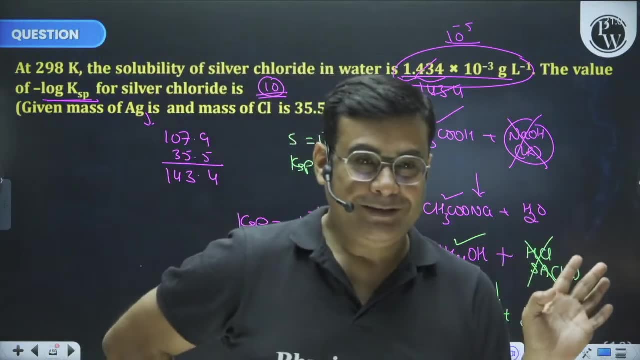 That after four days. assume that you have a paper on the 4th. Yes, if you have a plan for next year. if you have a plan for next year, then I can't do anything, Okay, Okay, But if you have to give the paper after four days, then at least what is the acidic buffer? 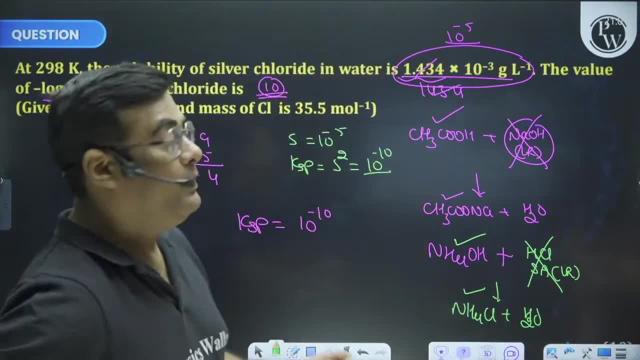 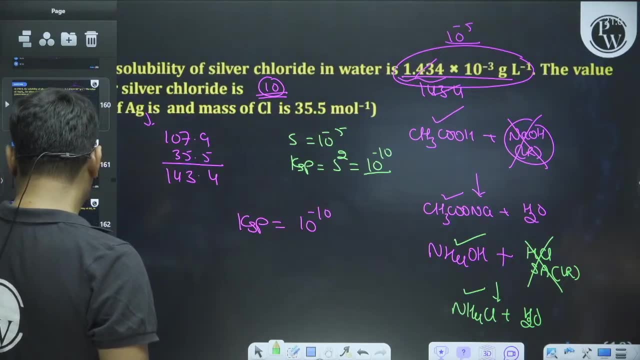 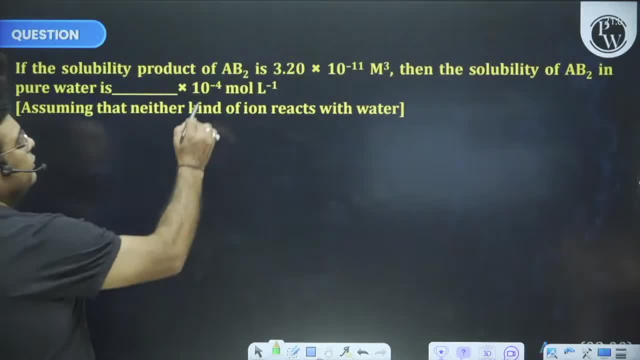 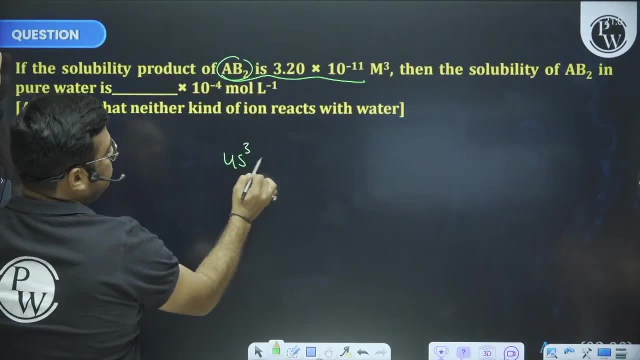 It is so simple If the solubility product of AB2 is this much. Now, I had just said that AB2 type of salt is there. So how much is KSP for AB2 type of salt? 4 S cube, Isn't it? 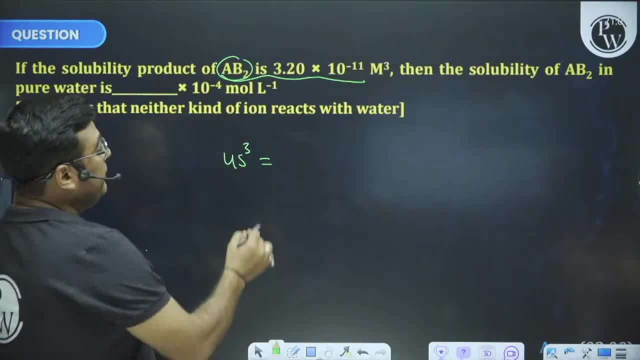 4 S cube. Now it is 3.2.. Now I write it 32.. I did minus 12 to 10, power minus 11.. So it is 8.. The value of S cube is 8 into 10 power minus 12.. 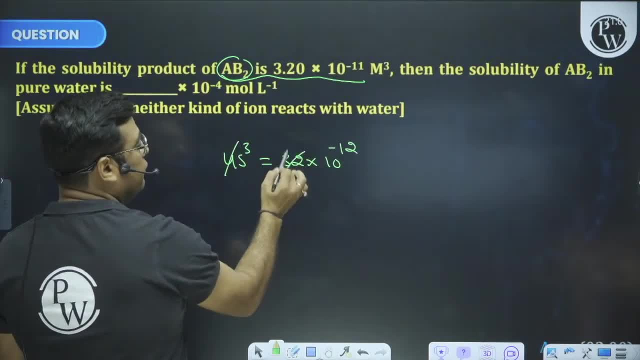 Now what do I do? I take its cube root. What is the cube root of 8?, Sir 2.. What is the cube root of 10 power minus 12? 10 power minus 4.. This answer is done, Okay. 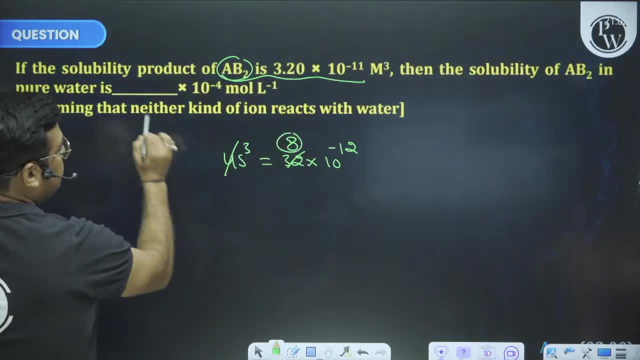 Okay, So there is no end to the questions. children, I can give you an idea here. Look, there are such questions in this. So this is the answer. Okay, So this is the answer. Okay, So this is the answer. 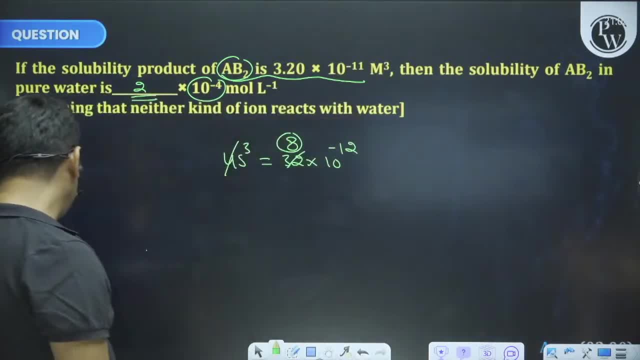 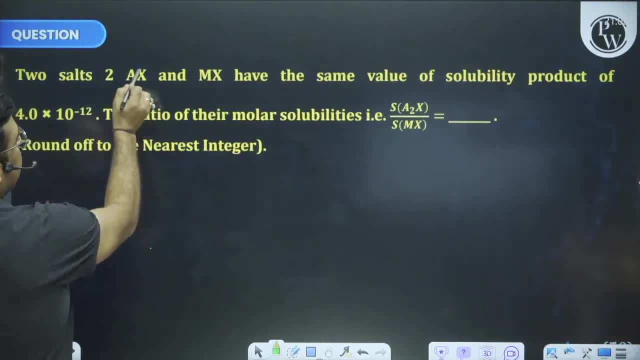 It will be 8 to A to X. 8 to A to X and MX have the same value of solubility products. The solubility products of both of them are same. Now tell if there is a 2X. What will happen is 4 S cube. 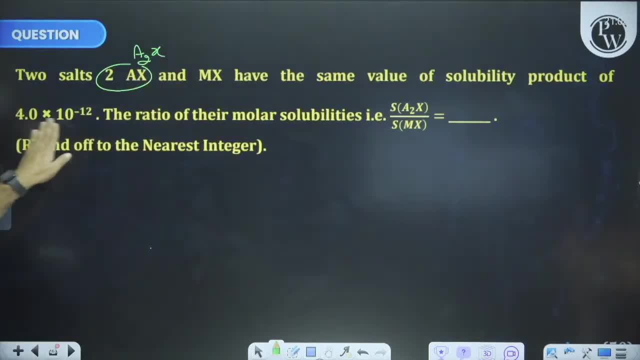 4 is cut. Why is it 10 to 10 power minus 12?? Sir, 10 power minus 4.. Okay, The second one is of MX, Meaning of AB type. AB type, This is A t, but it is now stolen for. 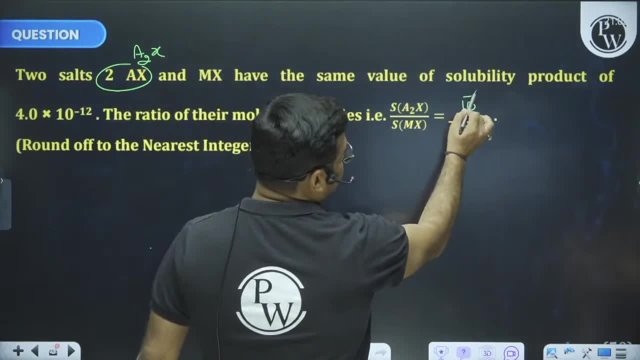 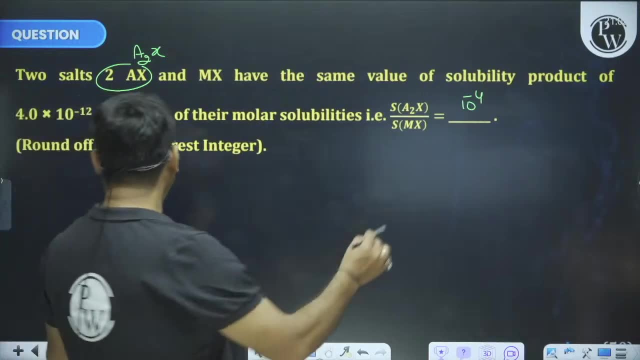 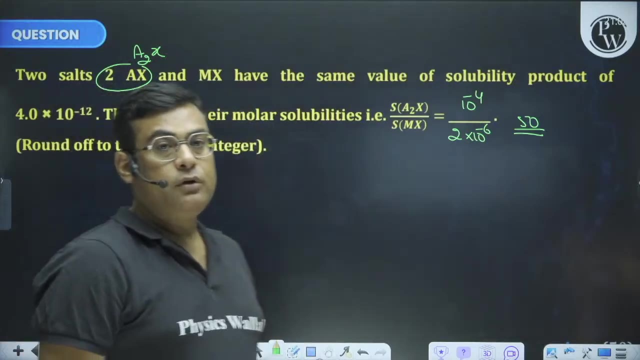 the same value, or how shall its name be? Prime one, gonium 9 here. Yes, Okay, Let us see. Yes will be s square under root of this. so 2 into 10 to the power minus 6, how much is the ratio children 50? how much is the ratio children 50? 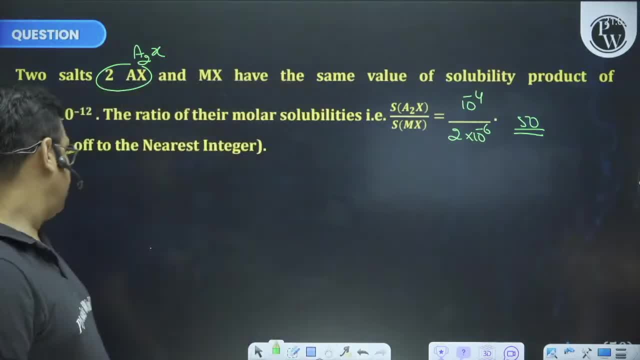 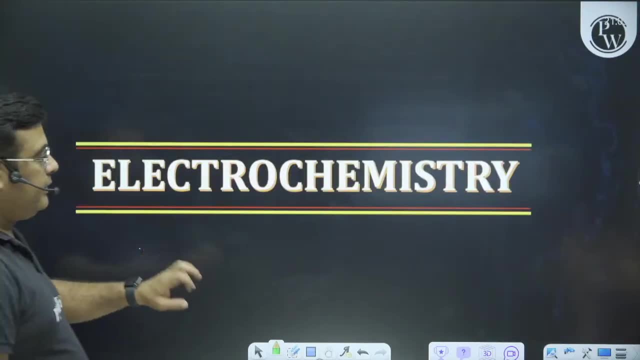 ok, how much is the ratio? it is 50, ok, come on, let's understand the matter in this way. children, you have to keep this in mind and in the same question I had brought it quickly, we will definitely do a poll. that brother. a little bit of fear from iNIC. 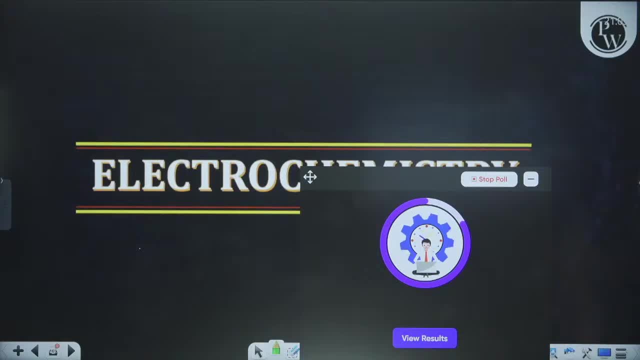 came out or did not come out too much. I can't say, son, if you haven't done at all so far, then different things, but if a little bit of work will have to do, then from these 10, 15, 20 questions you will definitely get a relatively confidence level of iNIC. 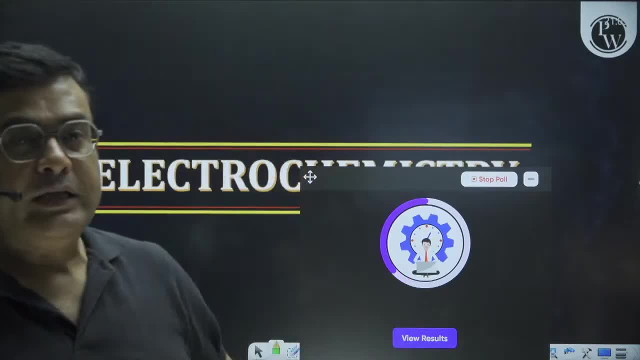 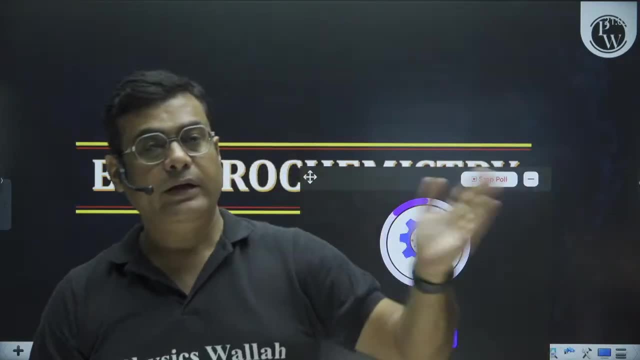 but calculation tricks would have also be understood ok in which the log is not given. that was found out, that if the log is not given then in anti log will be cancelled automatically. to recognize the buffer, to recognize graphical questions, to recognize the salt. yes, i did not do that. 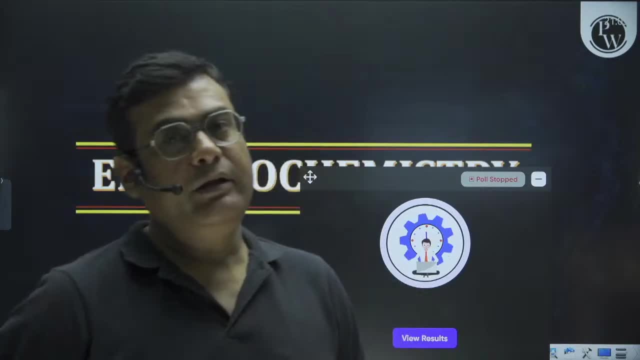 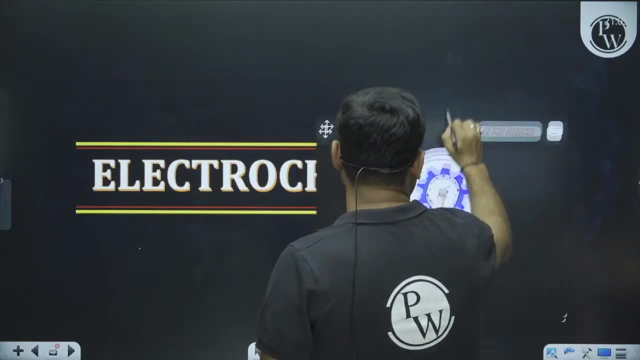 If I know all these things properly, then it will help in solving the questions of: what is your ionic equilibrium? Hey, what happened? I was doing it from above. What does the people of our country say? 95.8 means 96% of the people are saying yes, right. 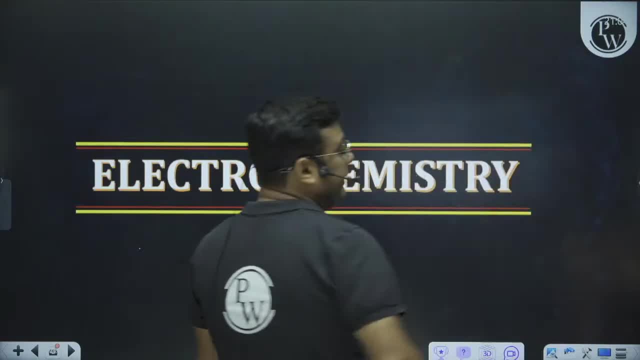 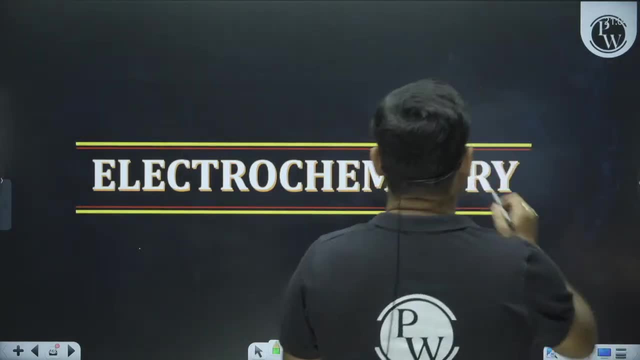 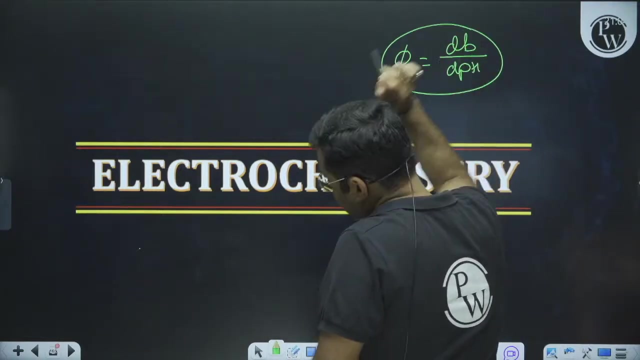 Sir, get the buffer capacity done, son. there is nothing like buffer capacity. the buffer capacity is 5, it is DB upon DPH. now, the question has not come in the JEE yet, son. this session is of MIQ, the most important question on which there are chances of coming. 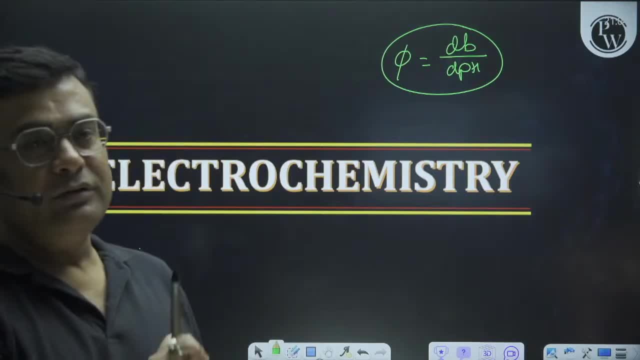 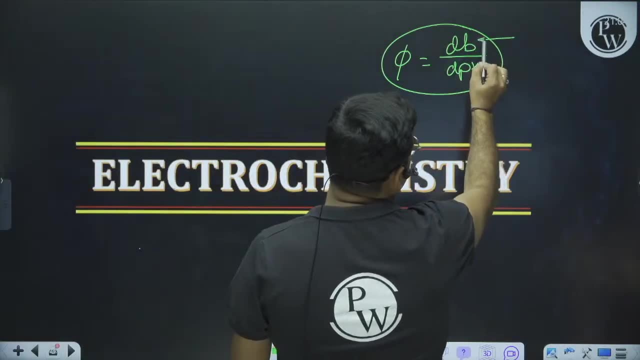 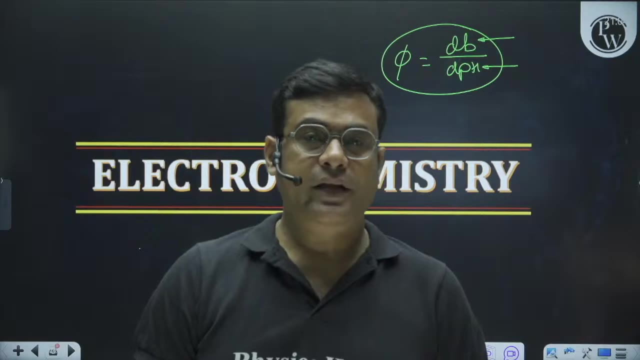 now it has not come on it, so its chance is also very less. so 5 is equal to DB by DPH. what is DB? Number of moles of acid or base added per liter of solution and what is DPH? Due to that, how much change has come in the pH of the solution? so if you ever have a 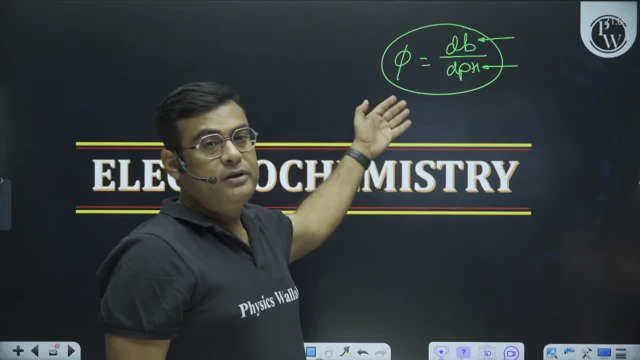 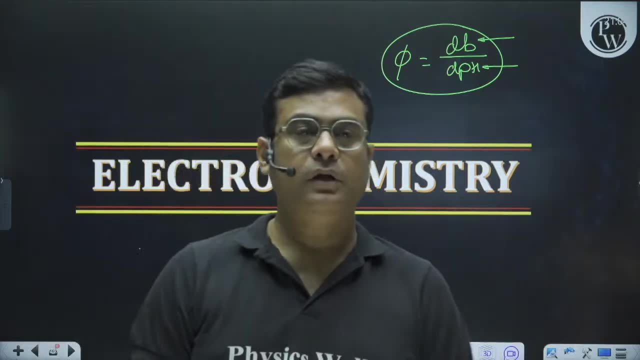 question of buffer capacity, then you will get the value of both DB and DPH. so if you have the value of your solution, then the value of the solution you got for the solution is 10.. For the solution that is given, the value of your solution will be given. just take its. 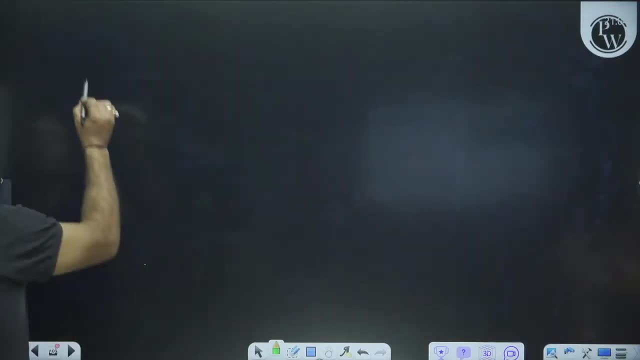 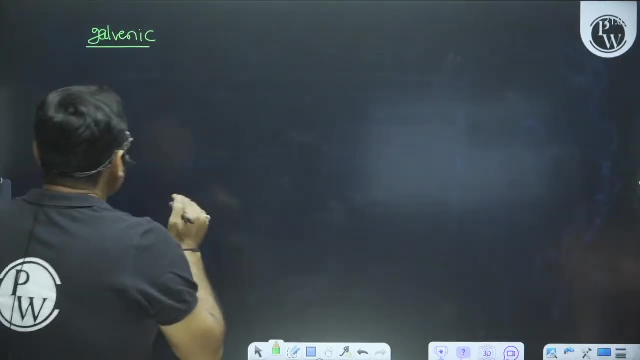 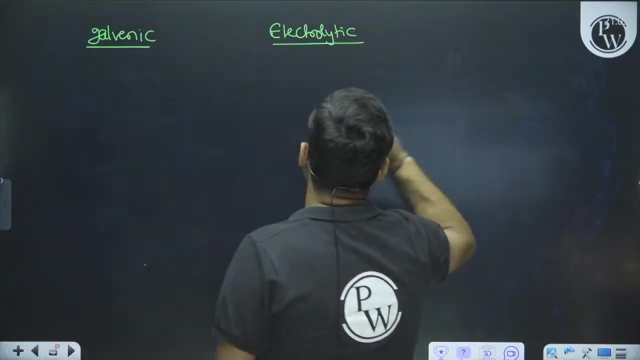 ratio. take its ratio and your work will be done instantly. ok, Now what do we know in Electrochemistry, children? in Electrochemistry, you have one galvanic cells. this is the second electrolytic cell and the third is your conductor. 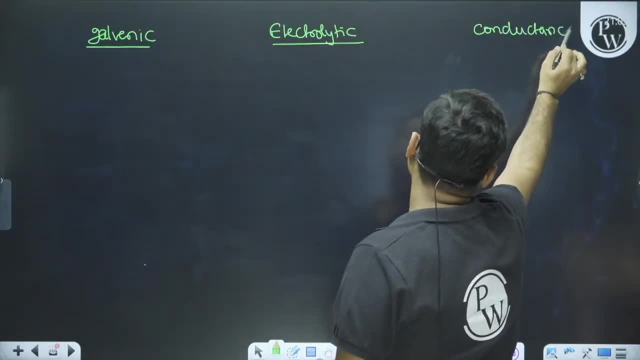 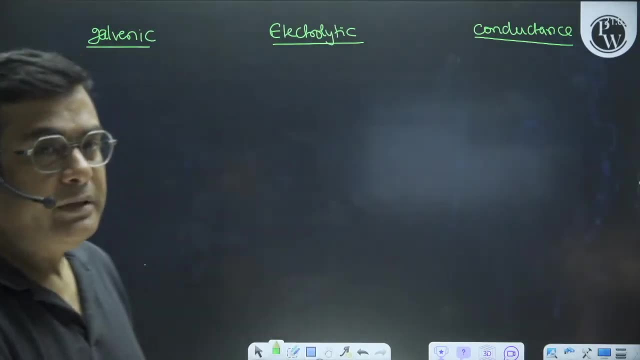 This chapter is 3 parts, So this is a very simple chapter which is not clear yet, but otherwise it is very simple. chapter In galvanic cell. you all know that majorly you have to use NERST equation E0 minus 0.059. 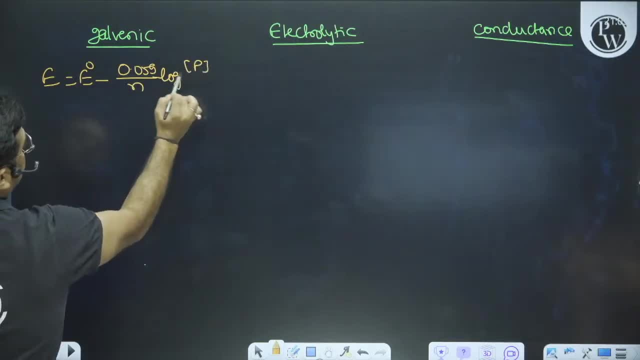 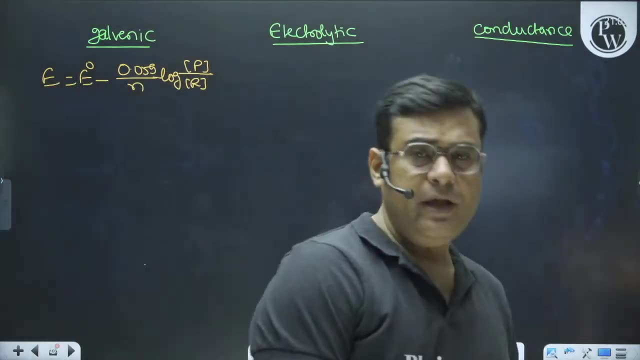 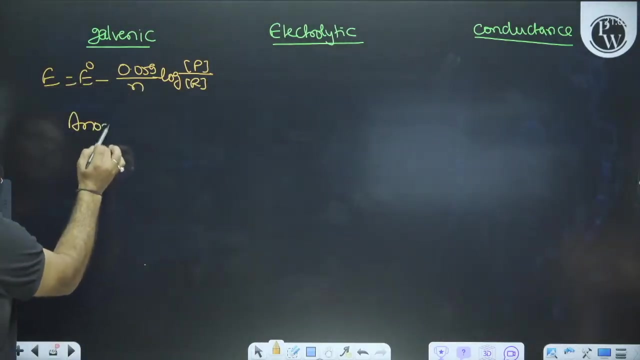 by N log of concentration of product upon reactant. This you should know. by use you in which way, any cell given to you On anode we know oxidation. oxidation means loss of electrons. On cathode reduction, reduction means the gain of electrons. 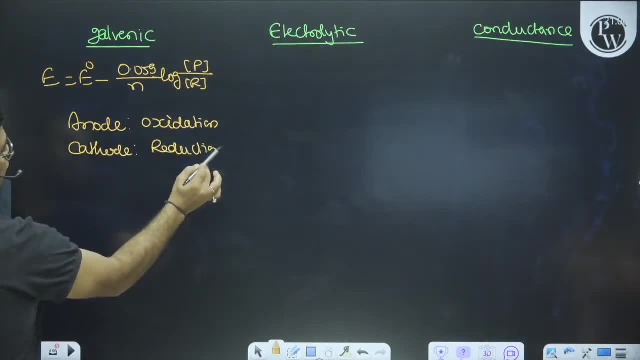 So whatever cell you give to you, you just have to write reaction in it's form, and after that you have to write the operation of the cell, that the product is on the side. bless everyone, son, everyone's ninety-nine plus percentile. 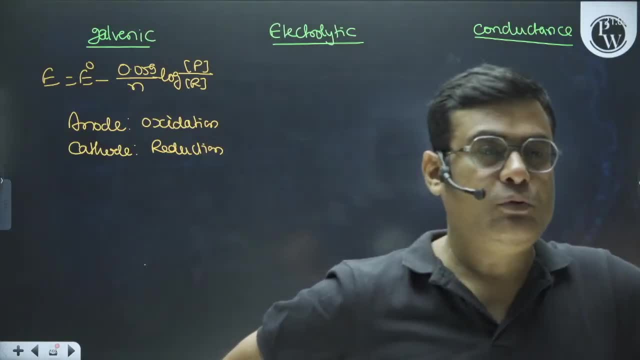 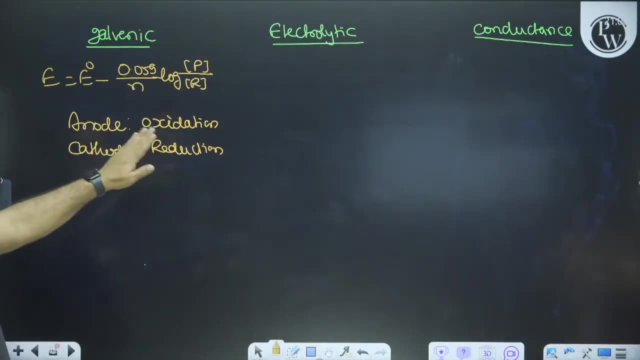 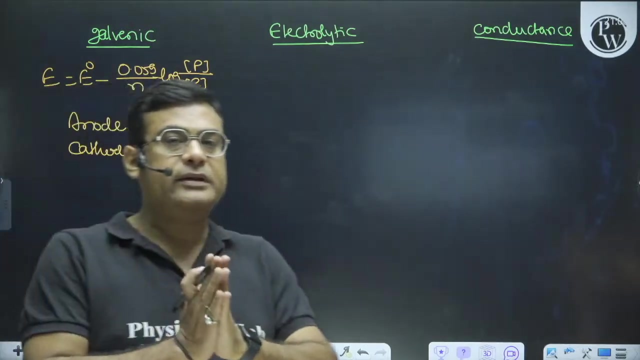 is made. this is our prayer son. this is our prayer son. ok, so I am saying this to you. that, what am I saying? ok, write the reaction in the right hand side, the product will come. in the left hand side you will apply the reactant, NERST equation, hopefully the galvanic cell. 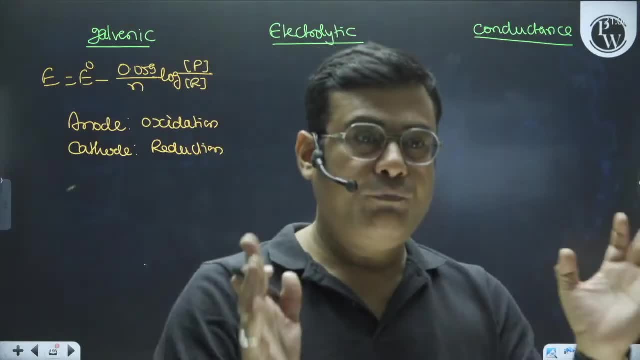 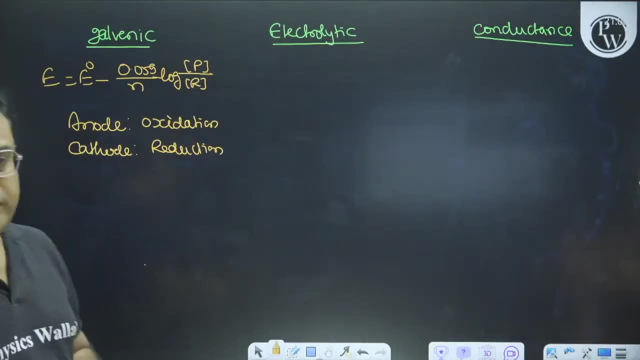 is not going to stop you. hopefully the galvanic cell is not going to stop you. ok, I will ask you a little bit: which of these is good oxidizing agent, which is good reducing agent? then you should know, children, in the electrochemical series, lithium comes at the top, which is the best of the lithium world. 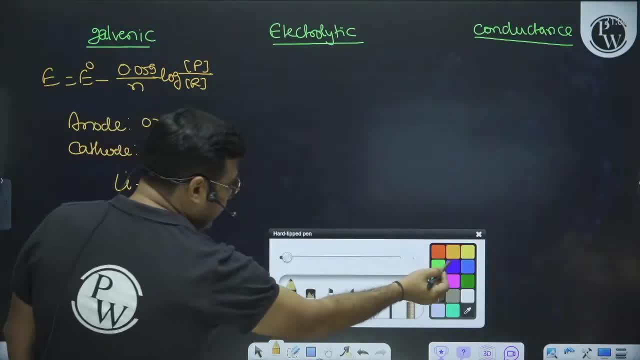 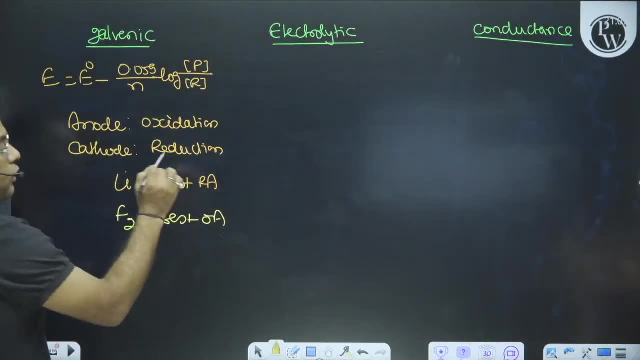 which is the reducing agent. lithium itself is always oxidized, reduces others and fluorine comes at the bottom. son, fluorine is the best of the world, then it is good in this way. there are only so many small things through which I am explaining. 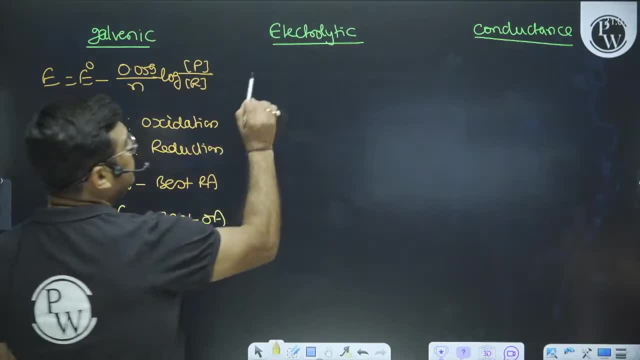 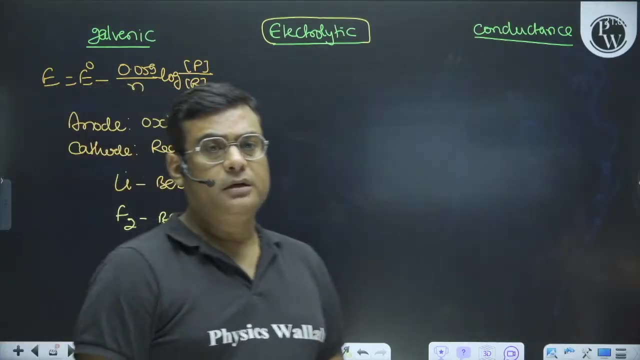 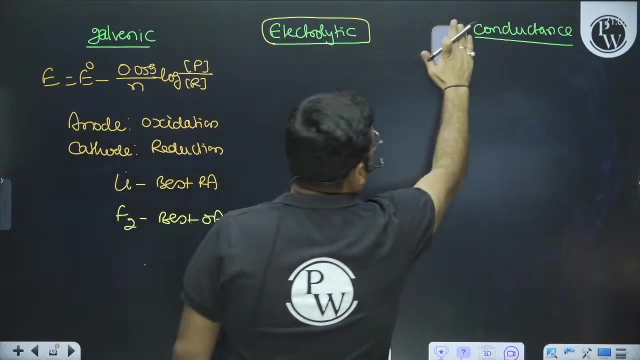 yes, it is right. so, after the electrolitic cell brother, only one of which is Farraday's law of electrolysis, of which I am going to tell you jsc, which will ask all of you questions now, I am telling her, that question is that now I will remove the conductor, I will take the next page. 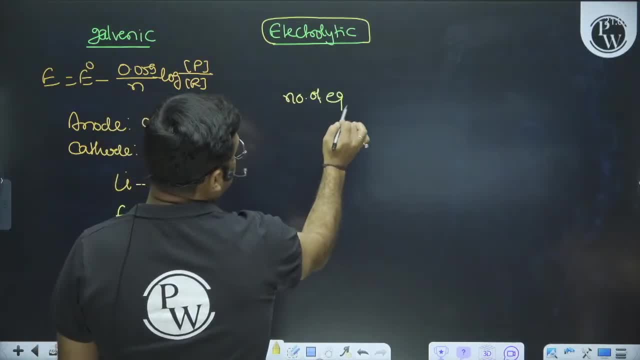 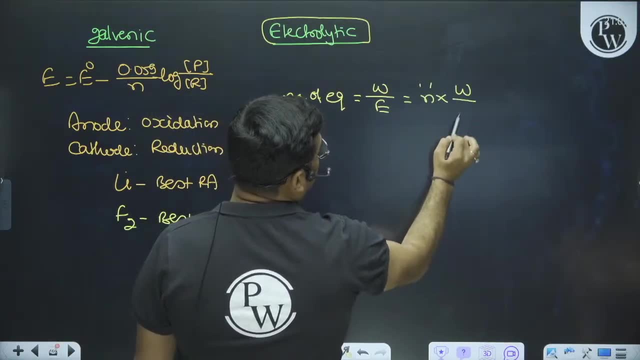 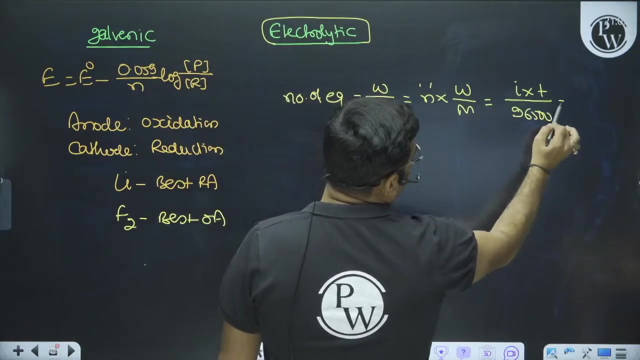 the number of equivalence, That is, W by E, equals to N. factor into number of moles equals to IT by 96500, and IT is also called Q by 96500.. The story is over. Apart from this, there is no other formula in the world. 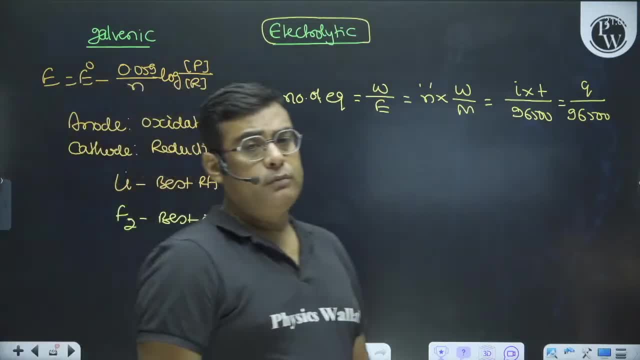 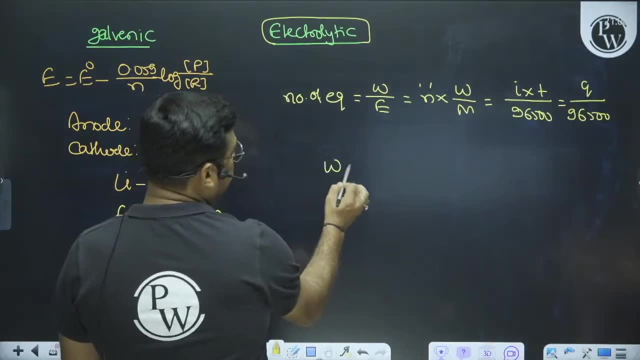 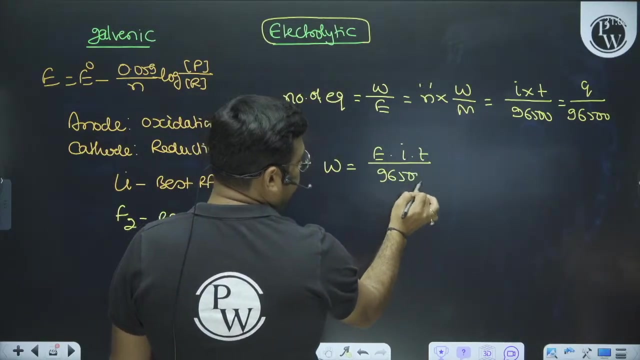 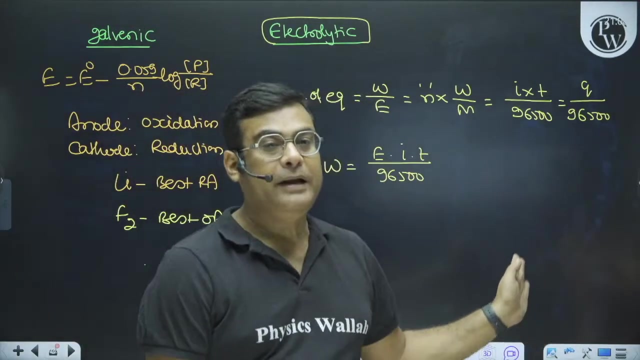 You remember the formula, Even I know it. You will say that, Sir, I remember this formula: W equals to EIT by 96500.. Even I remember this formula, but my writing method is different. I have just done this much that I have brought E down, W by E has become and IT by 96500. 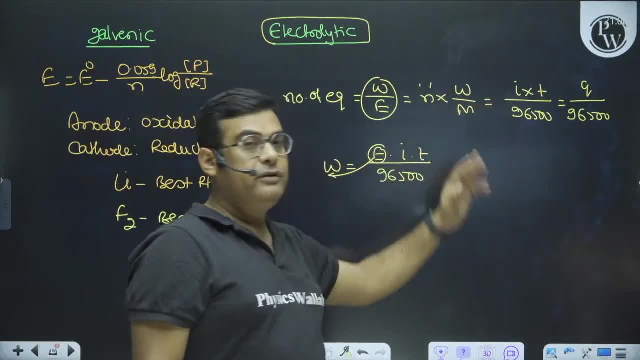 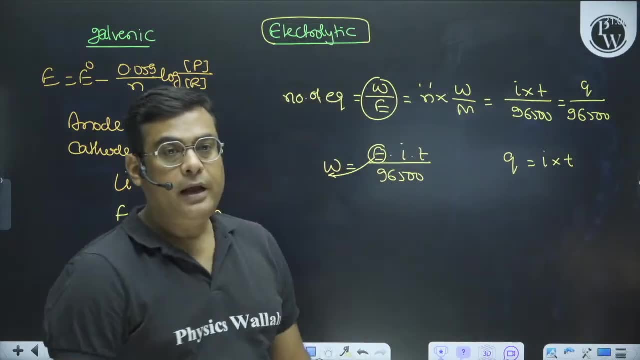 has become. You will know from physics that Q is equal to IT by 96500.. So I have written Q by IT by 96500.. But, but, but keep in mind that to be a column in your SI unit, the I has to be in Ampere. 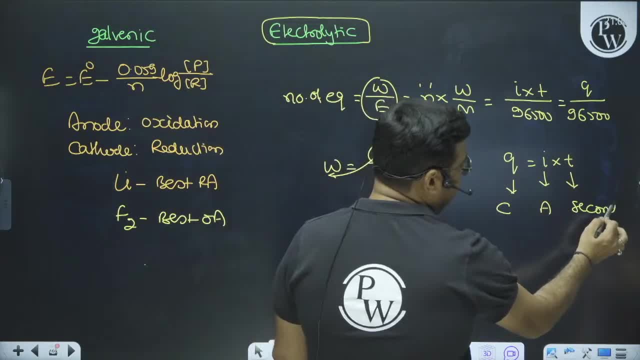 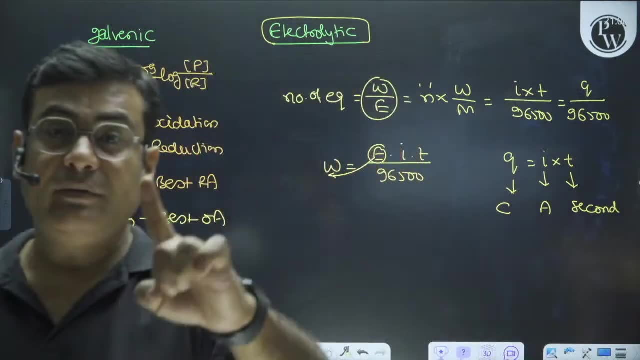 and the time has to be in seconds. So if in any question time is given to you in minutes or hours, then it is not the responsibility of the examiner to change that Right. The responsibility of reading that is yours, not the examiner's. 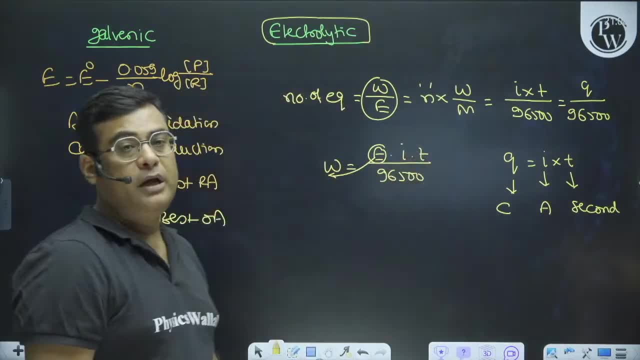 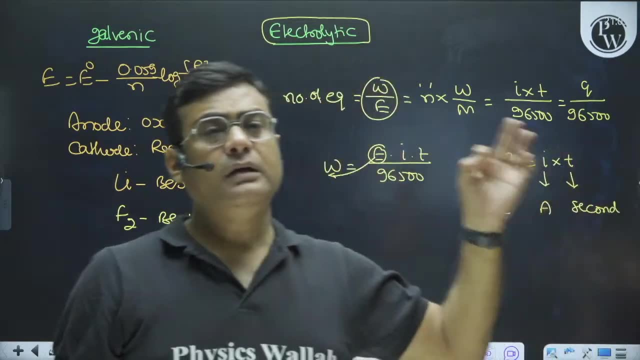 Okay, So apart from this formula, there is no other formula. Okay, I swear I don't know this formula. If I knew, I would have told you. Till today my question has not gone out, except for this formula. All my questions end with this formula. 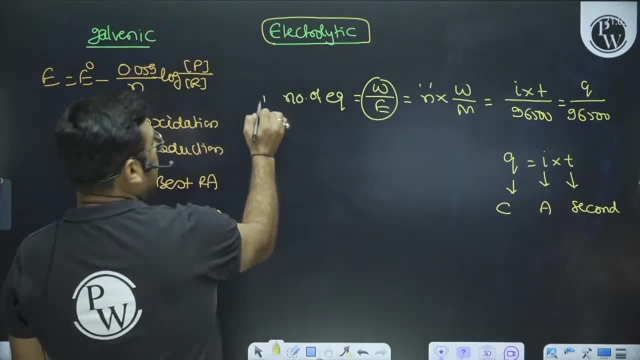 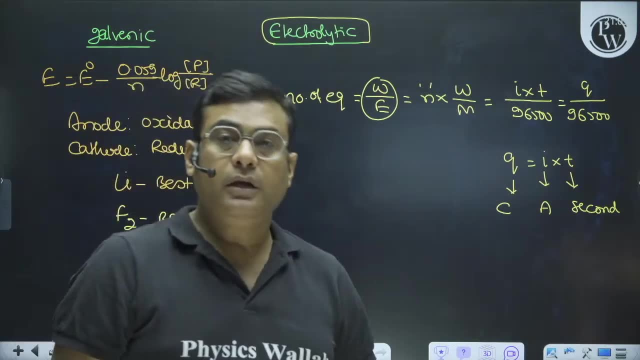 Right, Okay, I have explained you this first thing, The second shortcut of Electrolytic Cell. I will tell you this formula then it will be used. children, when the time of the charge current or the time is being talked to you in the question. 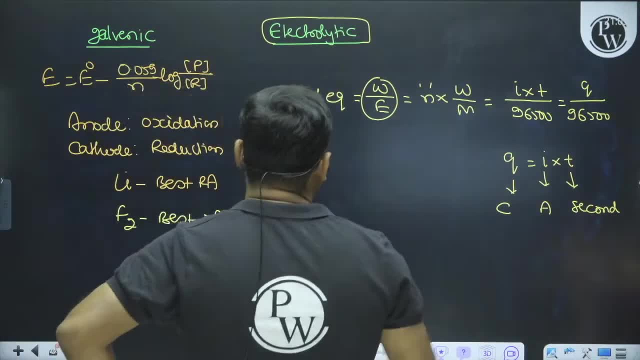 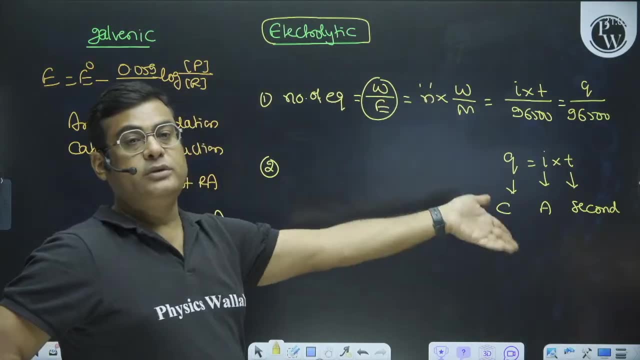 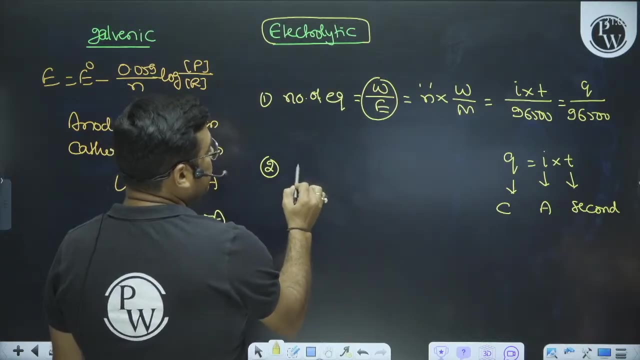 Right, It is being talked. It is not being talked. I am telling you that if the number of grams of any substance is made, then how many grams of the other will be made from the same charge? Then, brother, then you have to write the equivalence of A, that is, we will write it directly in. 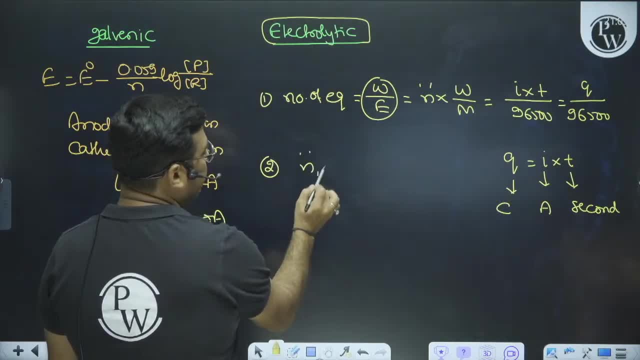 the formula Right What W A upon. Yes, Write it down in the terms of n factor. The first n factor n1, into its mass W1 upon molar mass m1.. The second n factor n2, its mass W2 upon molar mass m1. 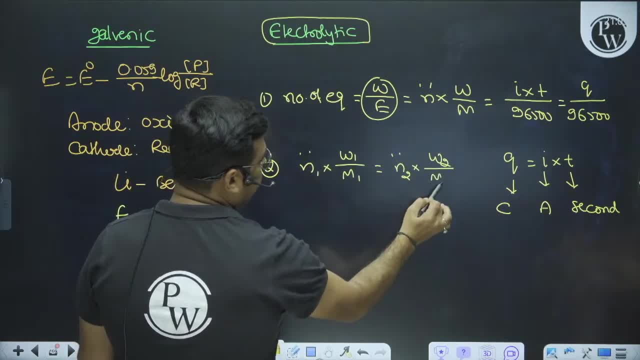 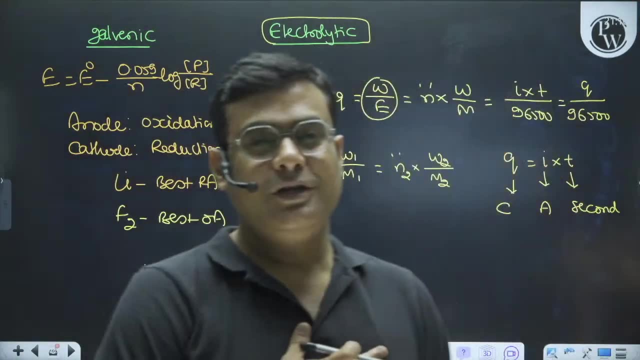 Right, W2, its mass W2, divided by your m2.. This formula is yours, Oh, son, I have read it. Thank you very much, Sir. you read very well, Thank you. Thank you very much, son. You have also written so many times, but pay attention to some studies. 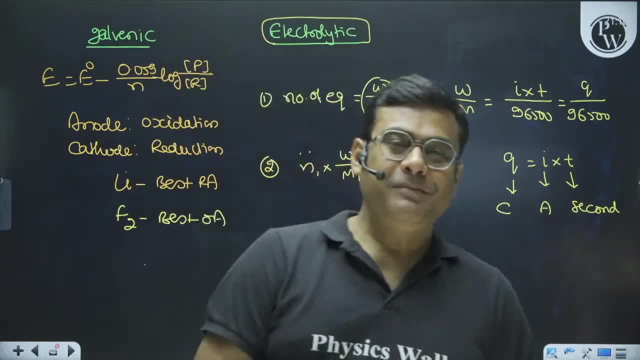 My dear, I had read your answers and I was so happy from the heart that you were in front of me. I would have kissed your hand, But now we will focus on some studies. For a little time we will be together Only ten to fifteen questions. 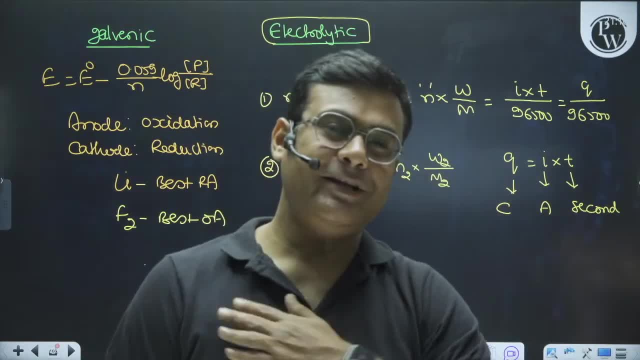 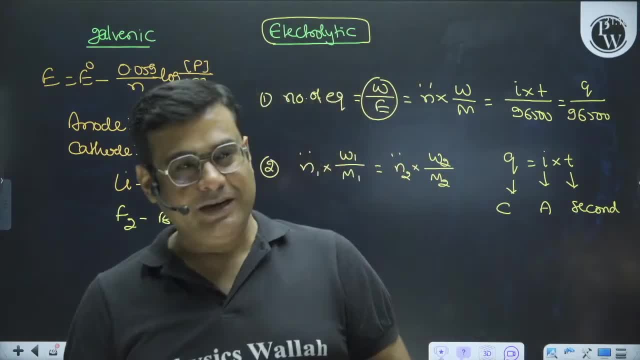 But now we will focus on studies for a little while, We will stay along for a little while. Only ten to fifteen questions. We will do the same for every topic. I will do the same for every topic. I will do the same for every topic. 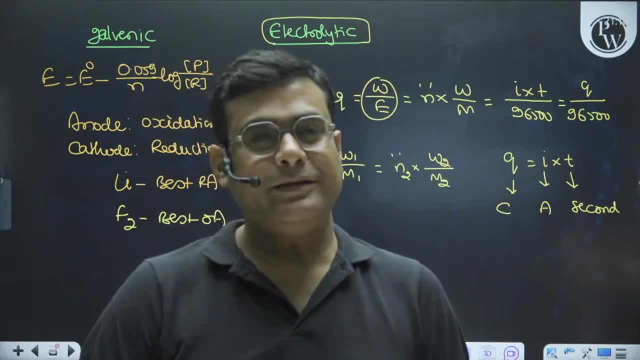 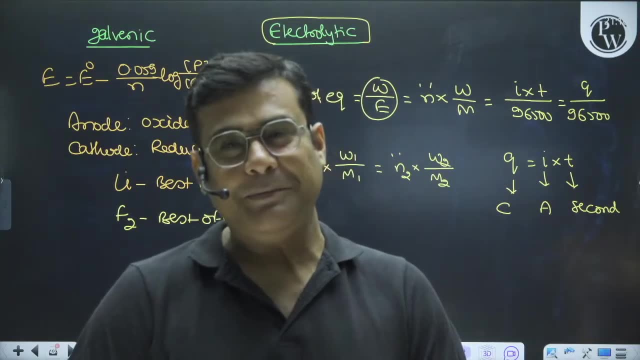 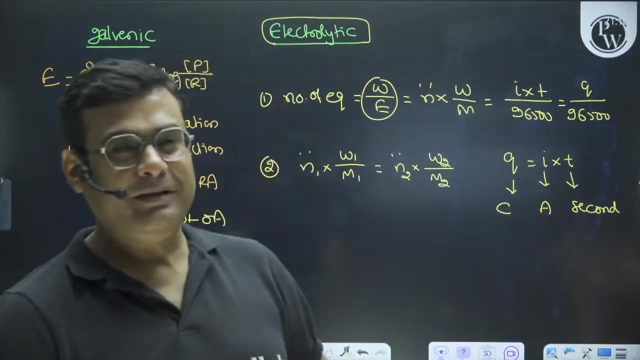 You are very cute. I have also read this and my wife also says that you are very cute. and what am I giving you the answer for it? I have no shame. Shame is coming. Tell me about the Electrochemical series. Let me tell you the order of your child on the shop. 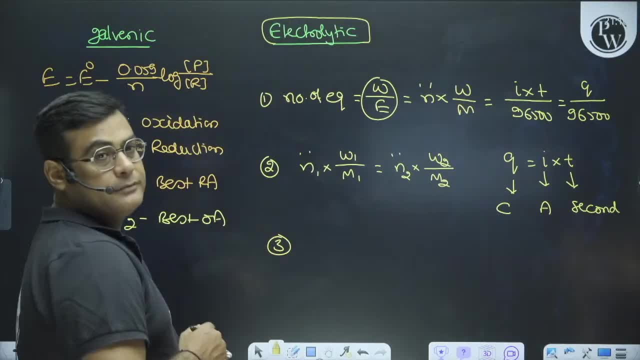 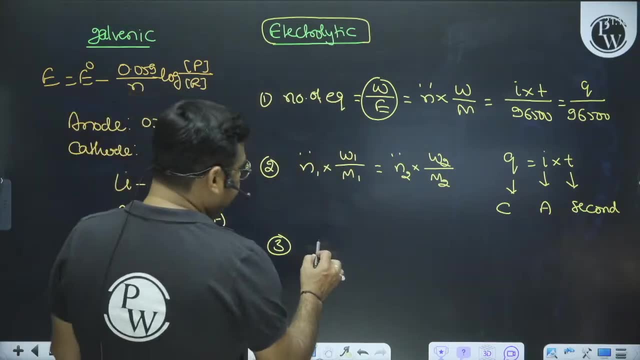 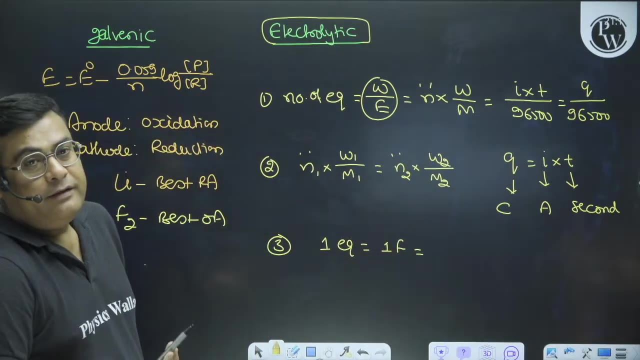 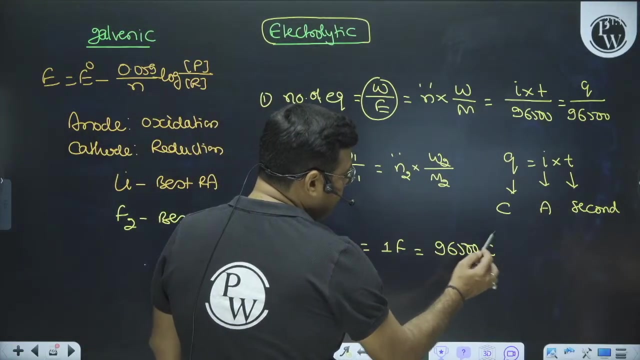 What was the third thing going to say? Faraday uncle did not live in this world, but Faraday uncle told us that one equivalent of any substance will be made from one Faraday of charge. and one Faraday of charge means how much coulomb of charge? 96500 coulomb means it is charge on one mole of electron charge. 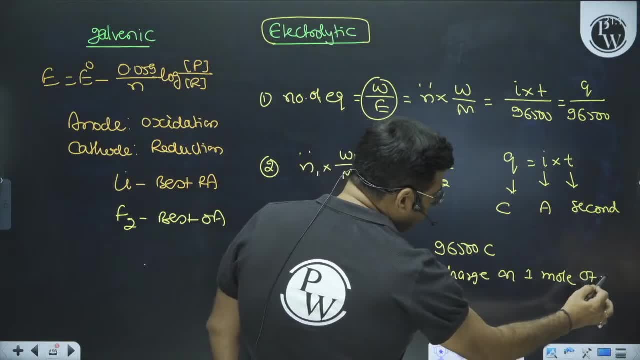 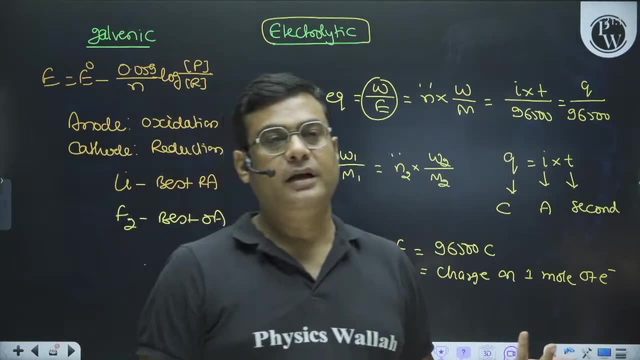 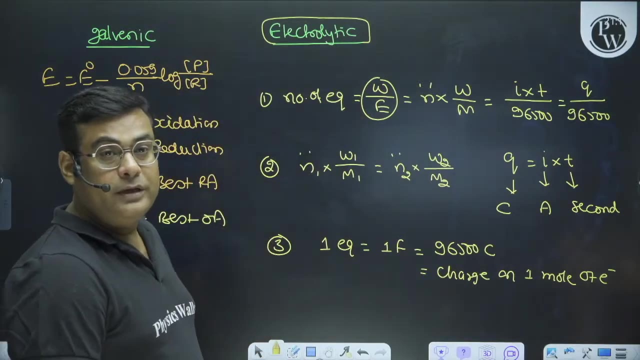 on one mole of electron. ok, so if you want to make half equivalent, then half Faraday, two Faraday will be there, then two equivalent will work quickly like this. so you have to keep these things in your mind, because if it is winter then the tempo will be down then. 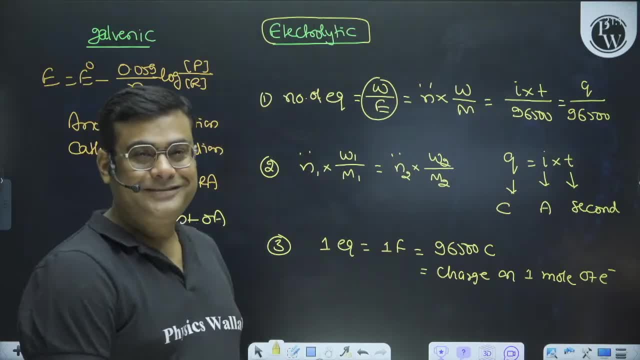 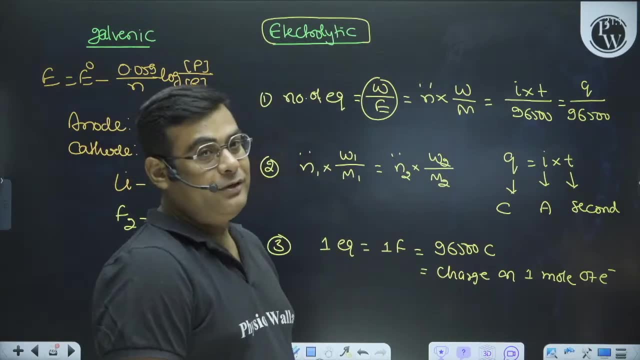 you are not cute, you are cutie pie. cutie pie, cutie pie. theoretical questions are coming more now. will not come son ask once now he will ask numerical question- that how much charge will be made from one Faraday of charge? 96500 coulomb of charge. 96500 coulomb of charge. 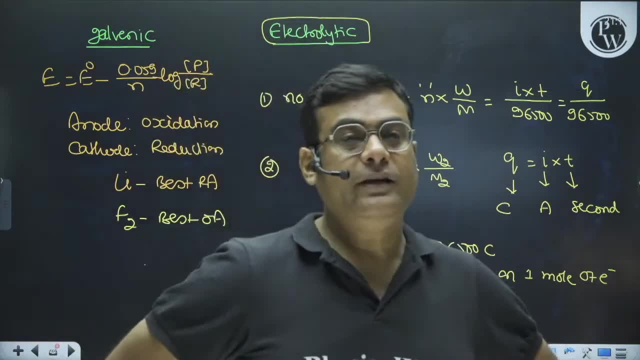 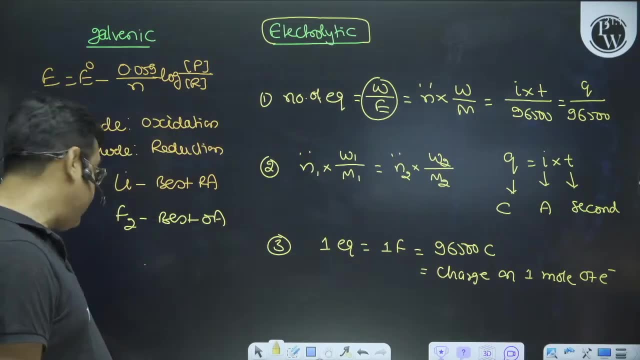 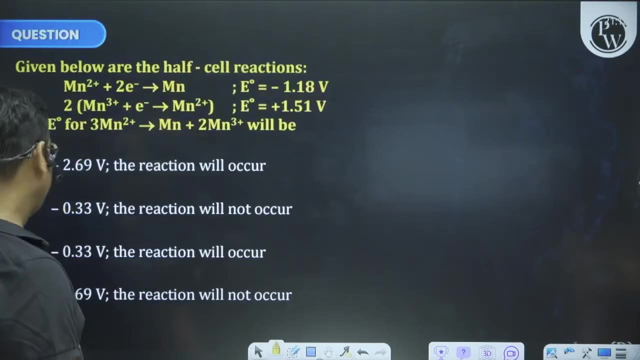 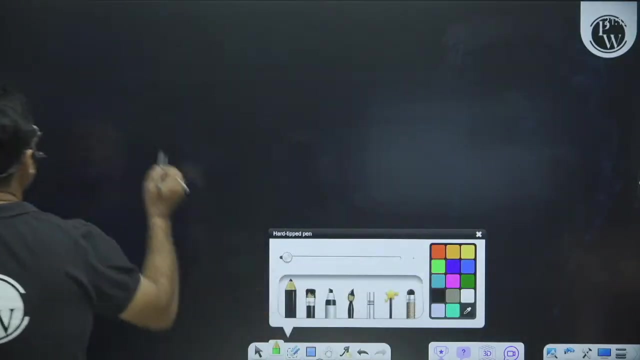 is it from one Faraday of charge 96500 coulomb of charge 106500 ela". all this we have here now, all these 975, 00 plays for 96500 coulomb and if the number of charge is short, like an 8, then it will all be zero. may be whenever you have a 3 übers. 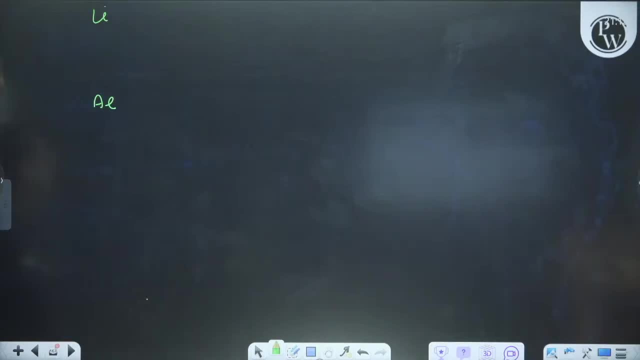 start with L and end with L, start with L and end with L and in between C K N M, C K N M. that is, Calcium, Potassium, Sodium, Magnesium, Aluminium. so these are the six elements. that is why I said that the electrochemical series starts with Lithium at the top. 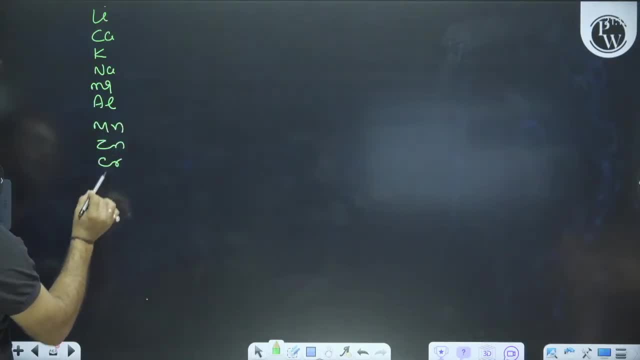 Man Jan Kar, Phir Sunenge Prabhu. after that comes Hydrogen, then comes Chapa, Copper, Mercury, Silver, Platinum, Gold. this is called Chapa C, H, A, P, A. and finally, at the end, comes Fluorine. 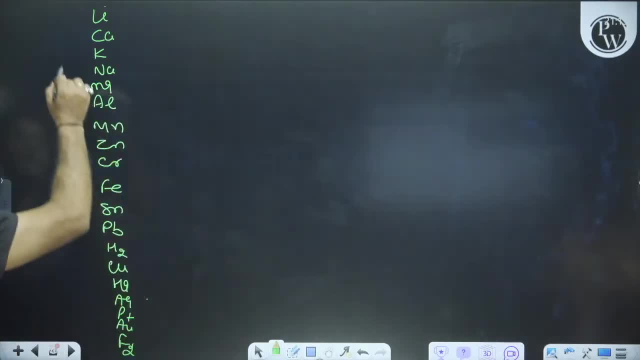 this is the electrochemical series. after going down, reducing power is reduced, oxidizing power increases. that is why this is the best reducing agent. this is the best oxidizing agent. from this series, you get the idea about reactivity. this is what you are saying. L, K, K, N, M. 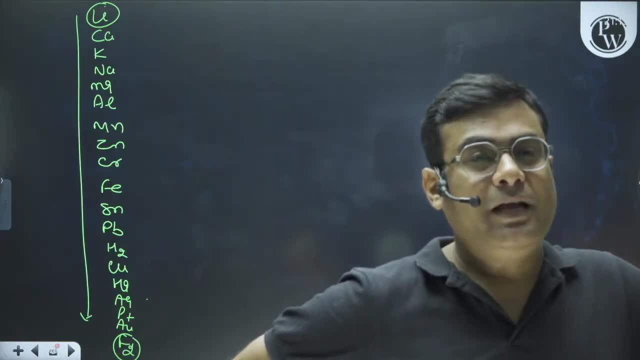 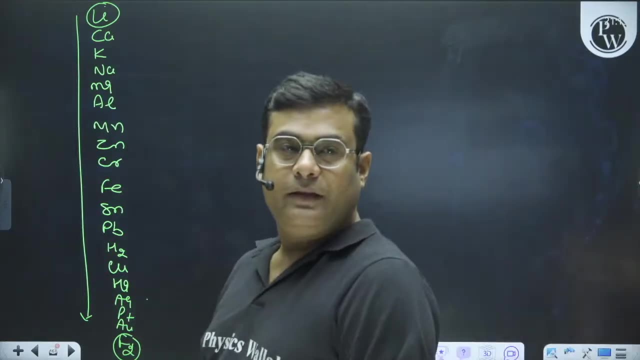 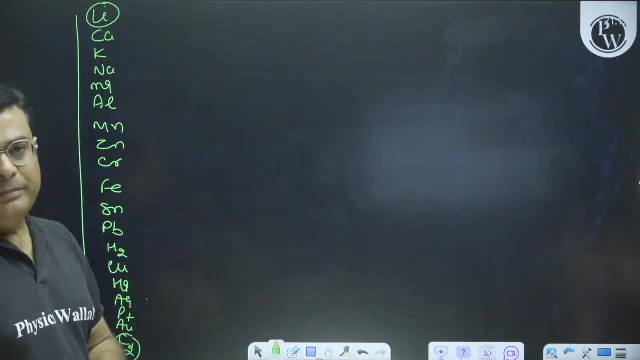 Man Jan Kar, Phir Sunenge Prabhu. Man Jan Kar, Phir Sunenge Prabhu by me. B BAT, P, A, U, W, V, F, I N makla I MADP C Ay A, G, L, A merge. 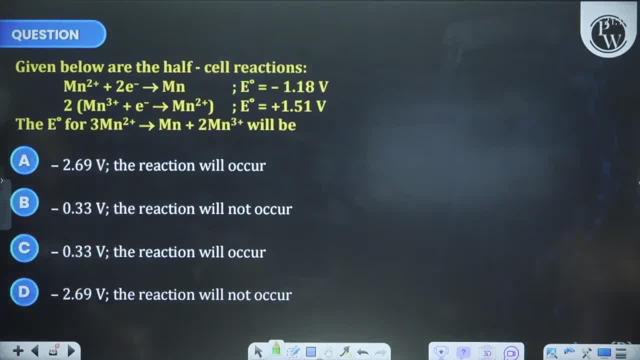 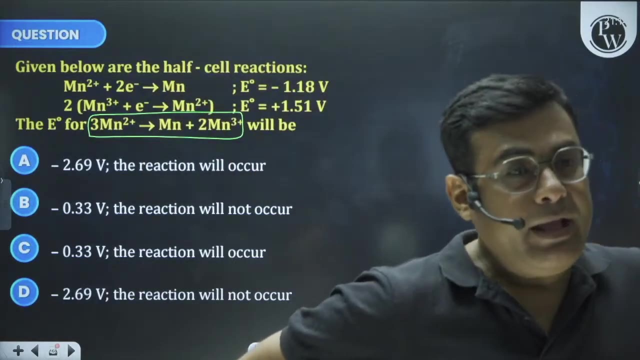 then comes Clan 거 Man Jan Kar Phir Sunenge Prabhu, Man Jan Kar Phir Sunenge Prabhu at a number by their own, one R lagi hai. I will get it. this is the question. what have you seen? they can't even remove E0. 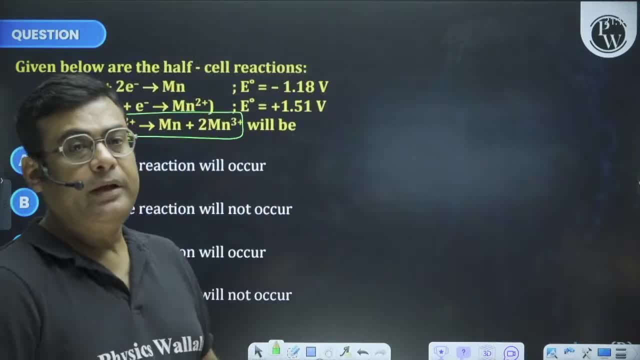 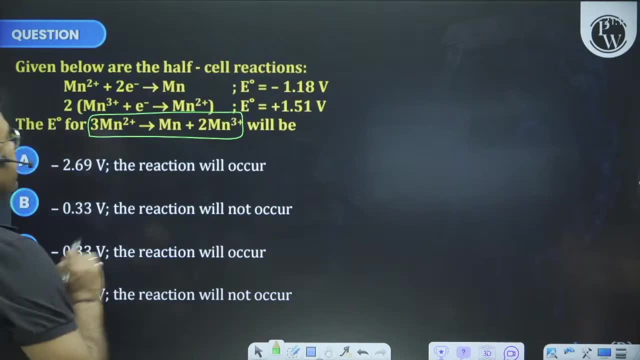 E0, whereas to remove E0 you don't have to do anything. to remove E0 you have to see whose oxidation is happening, whose reduction is happening, coefficient to coefficient. you don't have to see Mn plus 2 Mn, Mn plus 2 Mn, so minus 1.18. 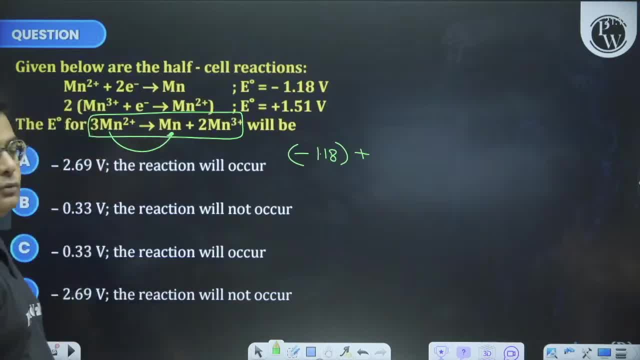 if reaction is leaked, then the problem is over. plus what is happening: Mn plus 2. Mn plus 3. Mn plus 3. Mn plus 2. Mn plus 3. Mn plus 2 means if I have to take plus 2 to plus 3, then reaction will have to be reversed. 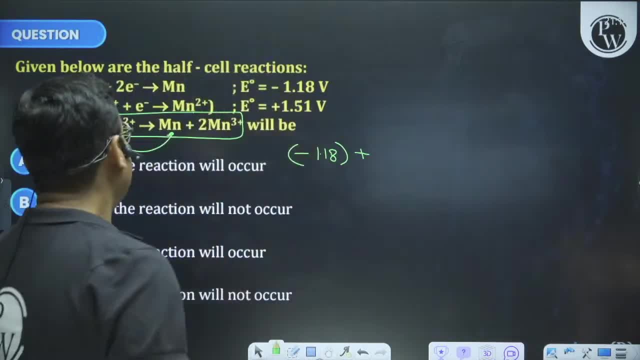 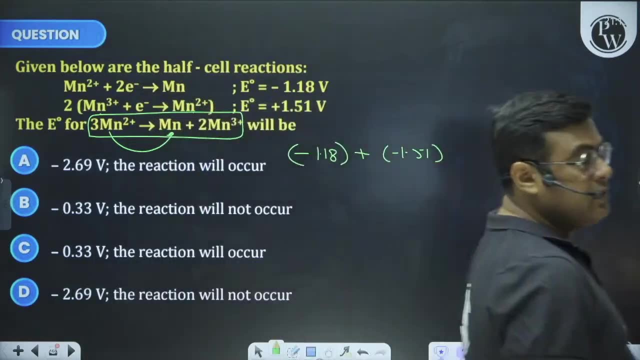 and reaction will have to be reversed. so this means I have to minus it, because I need to know these things about E0: that E0 after reversing reaction. what does it mean to reverse reaction? the OP became RP and E0 became Mn. the RP became OP. 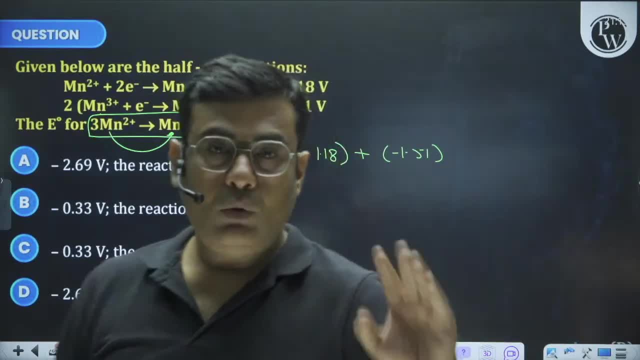 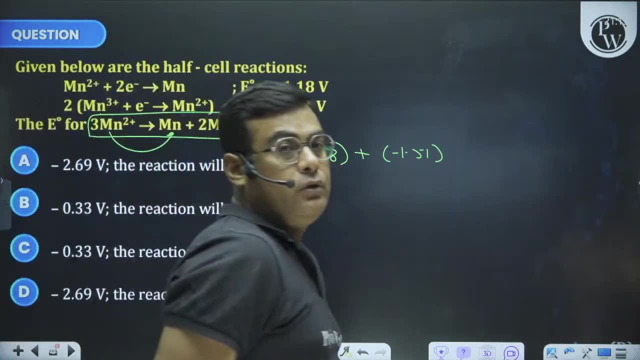 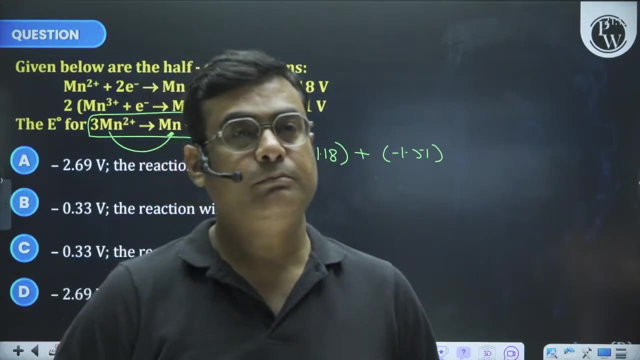 so after reversing, it has to be reversed. after reversing, it has to be reversed first thing. second, E0 is an intensive property. because it is an intensive property, because of being an intensive property, if you, if you multiply this reaction with any number, then in your E0 value, 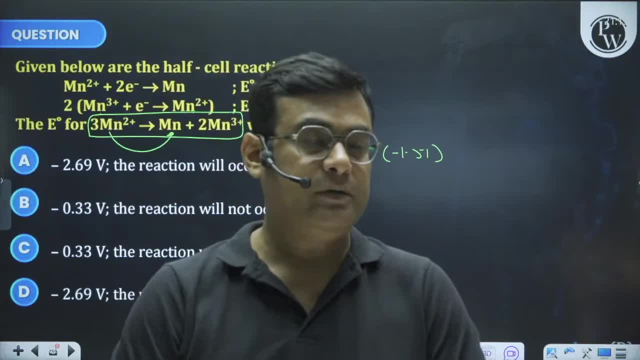 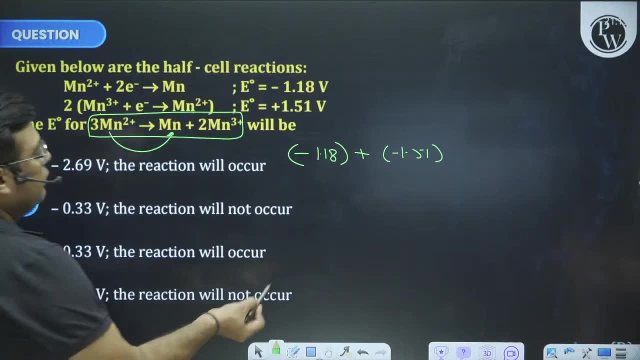 there will be no change. if you multiply it with any number, then any number will be changed. so now you have to add E0. if you add both, then my value will be minus 2.69, and if E0 becomes negative, then it means that this reaction is not feasible. 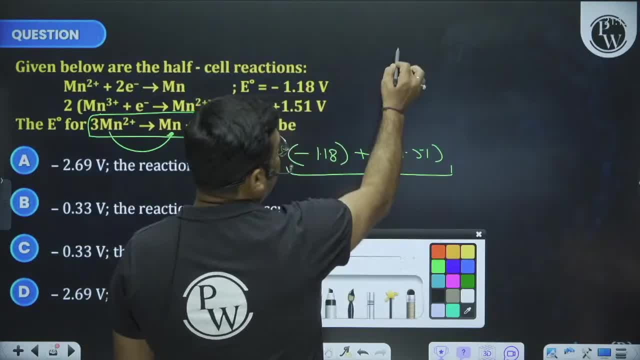 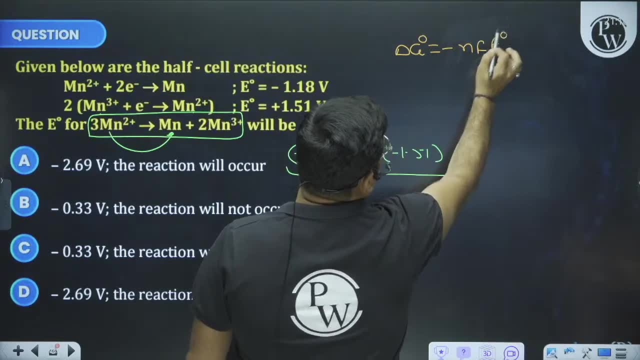 because now we are going to come to thermo. you all know that delta G0 is equal to minus NF E0. delta G0 is equal to minus NF E0, so if E0 becomes negative, then it means delta G0 is positive, and if delta G0 becomes positive, 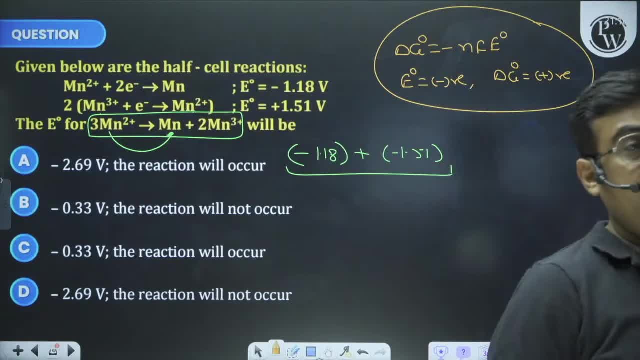 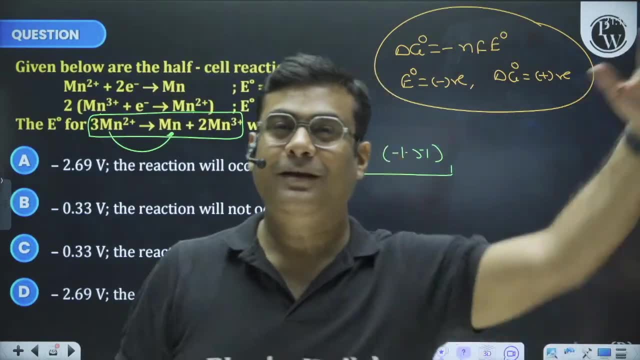 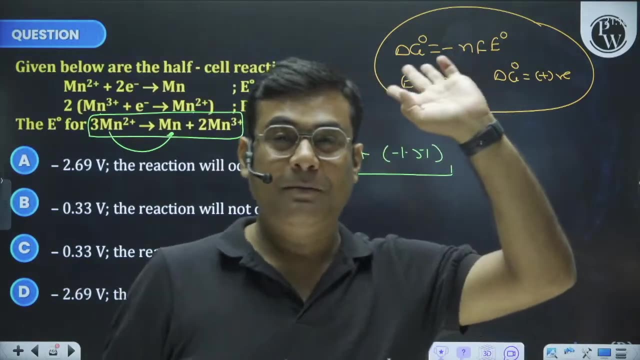 then GIFS Baba will be angry. GIFS Baba had said: till I remain negative, till I remain in RIN, till then I will keep doing all the processes. people always think about their benefit. they say: give me, give me, give me in plus. but GIFS Baba of thermodynamics? 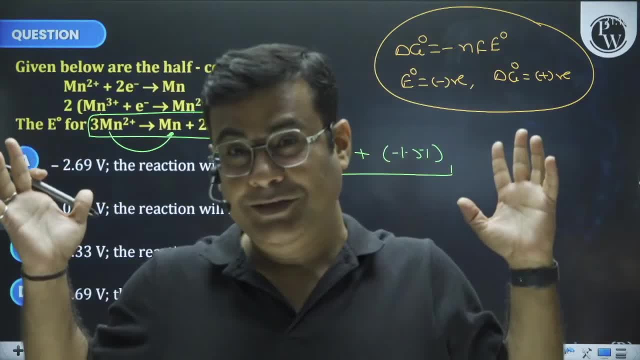 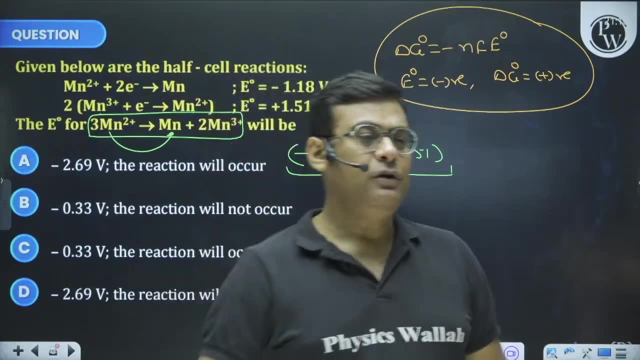 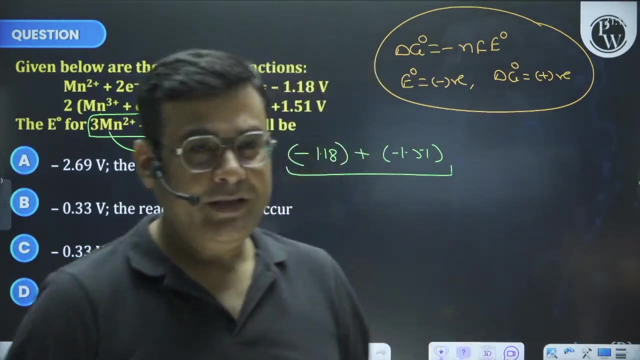 he was great. he said: till I remain in RIN, till I remain negative, I will keep doing all the processes, keep doing, keep doing more negative and keep doing your work, keep doing more negative and keep doing more negative. ok, this way your work is done. so this story ends here. 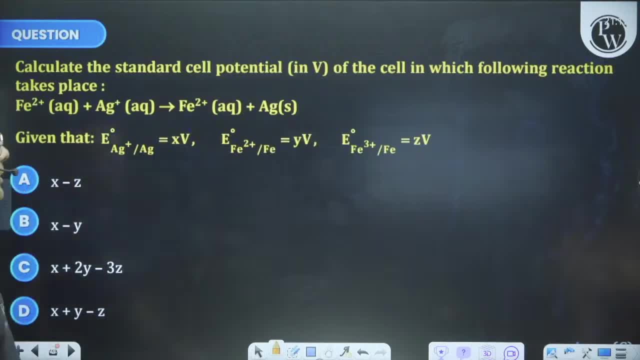 now see. many questions like this came now I will calculate the standard cell potential of the cell in which the following reaction takes place. now the same story for this reaction. so in this case, the first reaction is A G plus A G, Sir the X of A G plus A G. 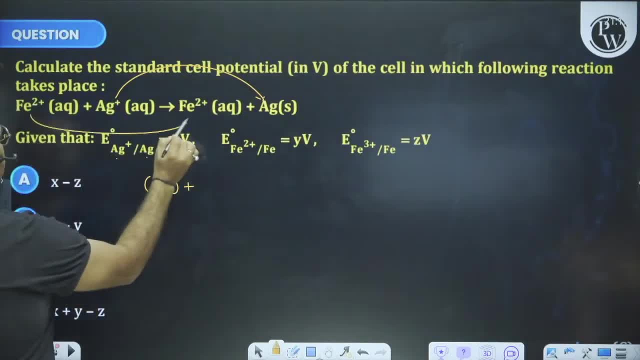 ok, x is done. plus F, E plus 2. you know, obviously its reduction is happening, so the F? E will be the oxidation means. here the operator made a mistake. it should be F? E plus 3. I will change the marker so that you can see. so I want F E plus 2. 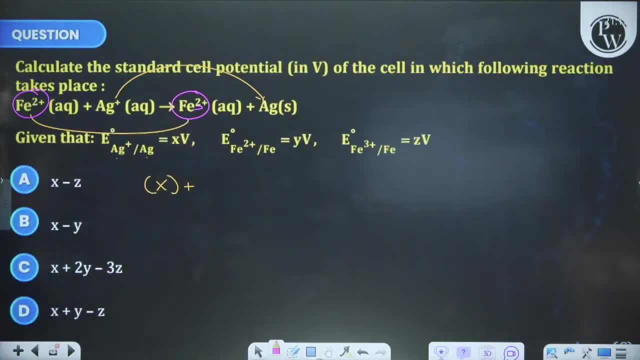 from F E plus 3. this is also the JEE's favorite question and my children who are studying My educated students have also given their formal exam. You see, you want FE plus 2 to FE plus 3.. But here FE plus 2 to FE is given. 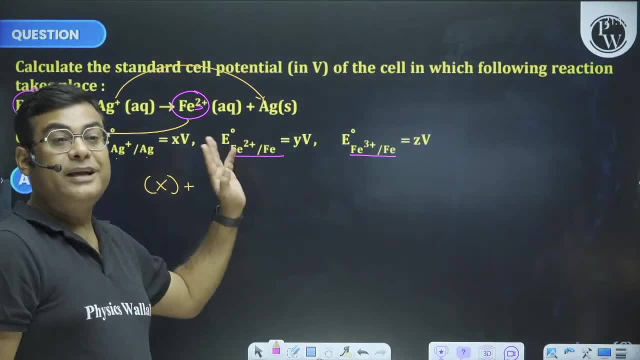 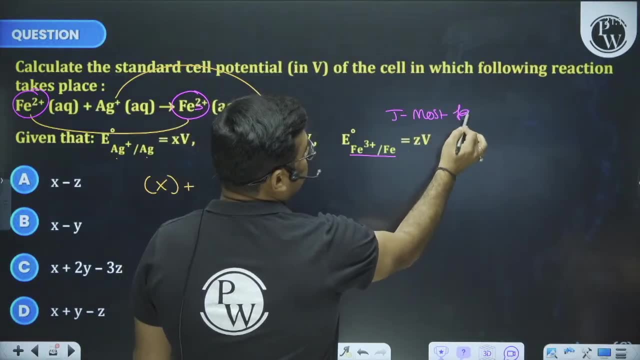 FE. plus 3 to FE is given, Plus 2 to plus 3 is not given. So in this case you have students, And this is JEE's most favorite topic. I am telling you from now that some of you children 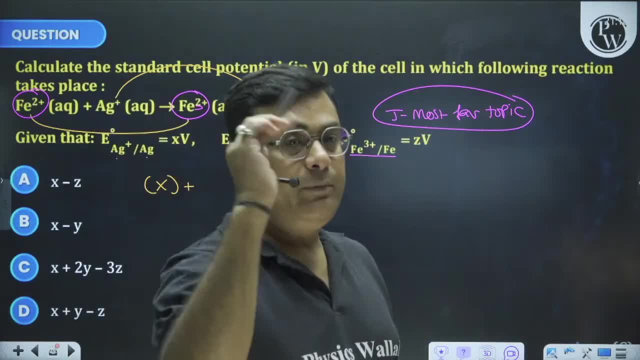 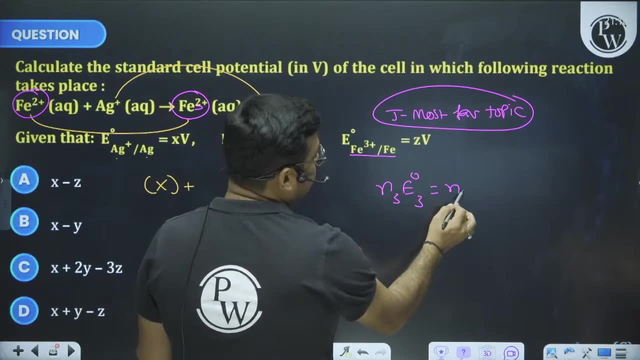 I can't say every child, but some children are definitely going to get it, Definitely going to get it. Okay, its method is N3E03 equals to N1E01 plus N2E02.. Now I will tell you both the methods: children: 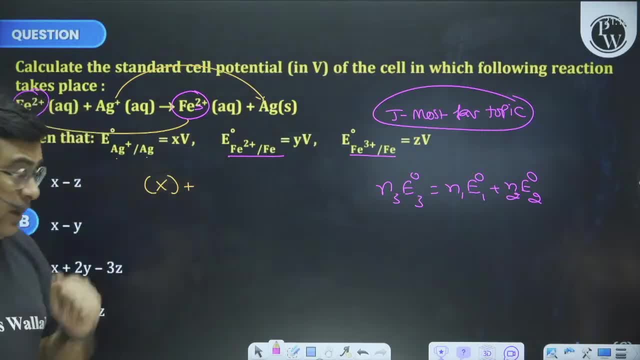 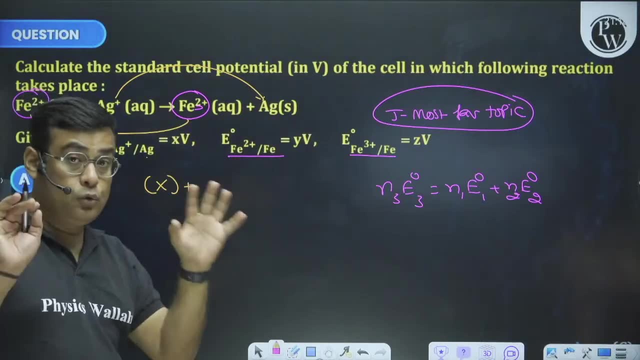 If you are sitting in the exam, then how to do it. Okay, if you are sitting in the exam, then how to do it. Those who only know that this will be the formal Whenever one metal, write the rule: children. 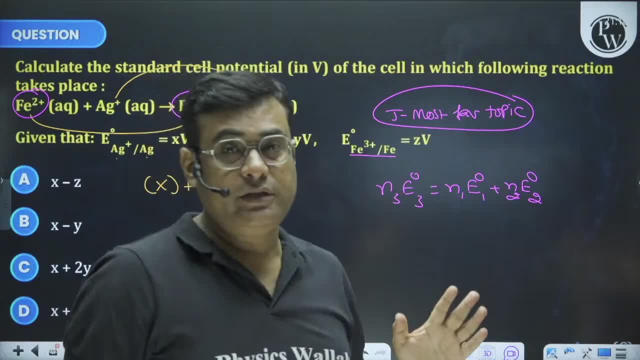 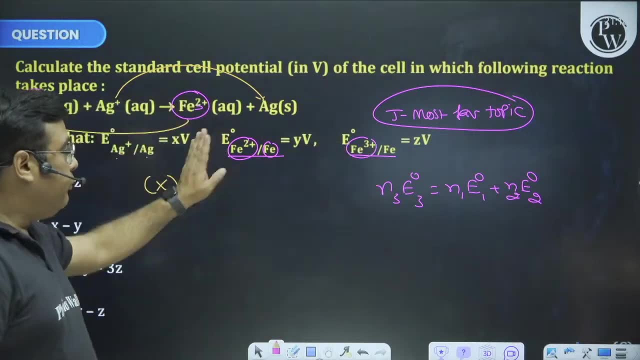 Whenever one metal is in its three different oxidation states, Like FE, FE is in 0,, FE is in plus 2.. FE is in plus 2,, FE is in plus 3. And if you have to take out the potential of 2, FE is in 3.. 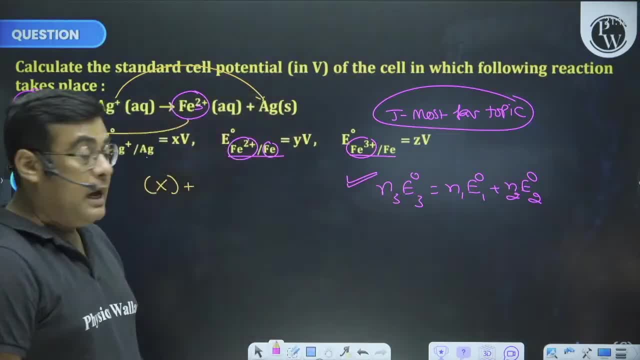 It will always run from this formula, children, From this formula. Now I don't even need to apply this formula here, Why not? I can see son, this is X. In the next ones I see two electrons in one. 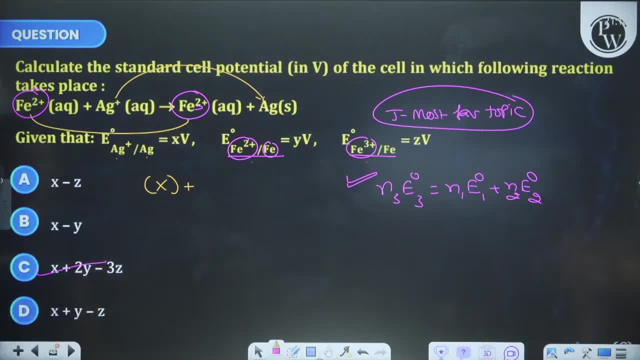 Three electrons in one. That means there should be a coefficient 2 in one. There should be a coefficient 3 in one. It is confirmed. Now, if I had sat in the exam, this would have been the question of JEE. I don't solve it at all. 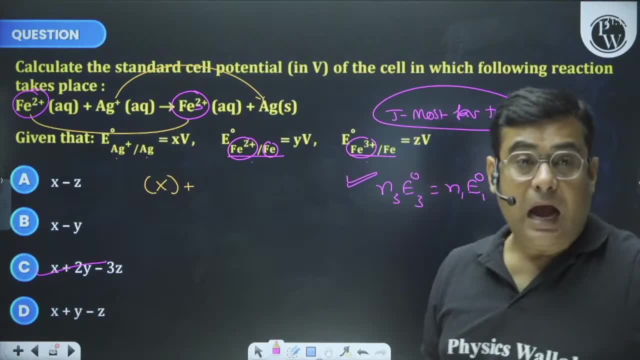 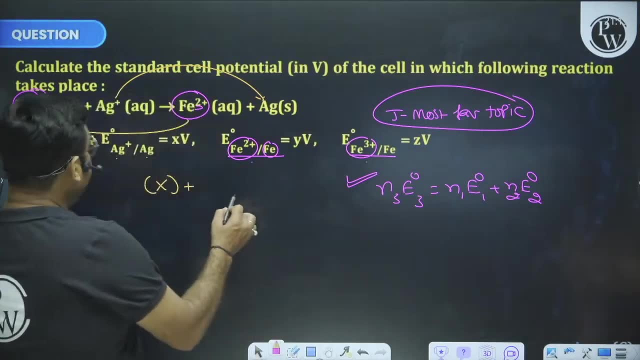 I don't solve it at all. I just look at it and tick it and move on. For you children to teach the use of this formula, I am definitely solving it. What is the meaning of N3, sir? What reaction do I want? 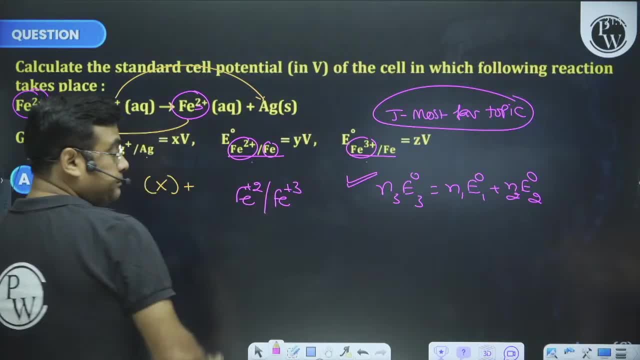 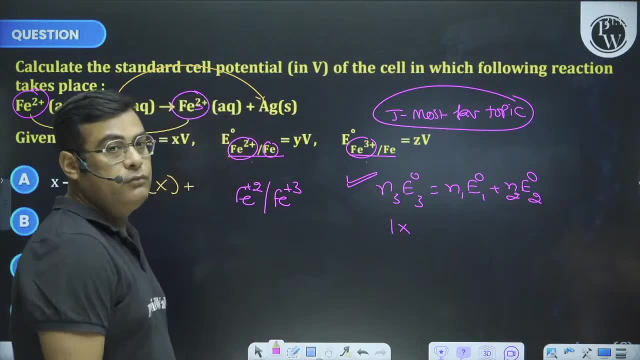 I want, sir, FE plus 2 to FE plus 3.. Okay, so how much is its N, Sir? its N is 1.. Into E naught 3, that's what I have to take out. That's what I have to take out. 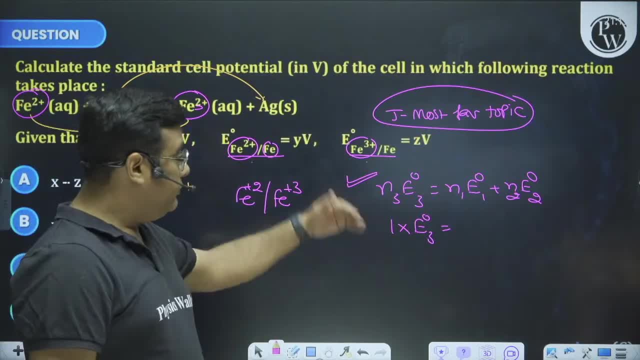 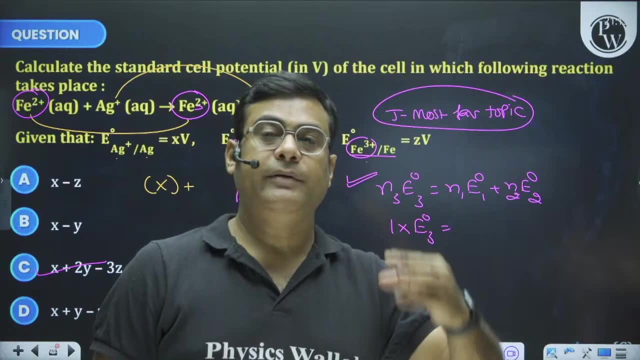 Son, you don't even need to say it. sir, Can you play? How to use? I will tell you myself, son. This is my moral responsibility. son, I am standing here because if, after my teaching, two questions are more correct than that of any of my children, 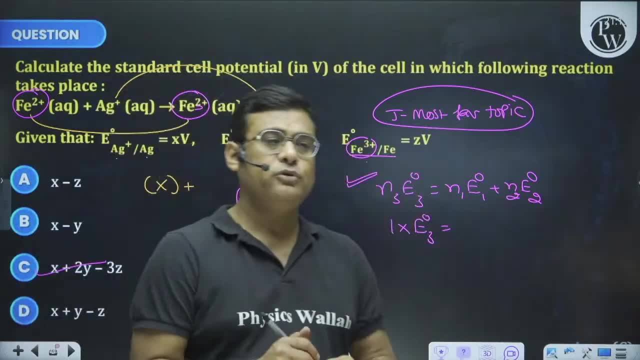 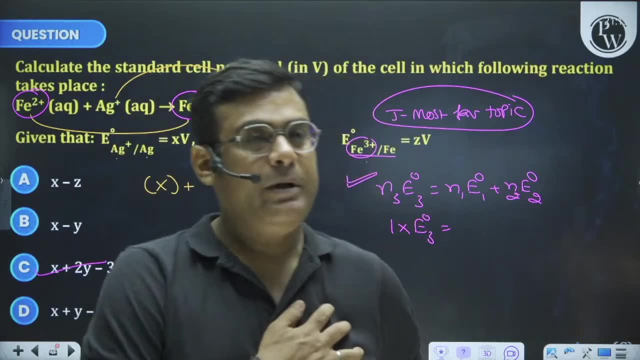 which were happening, they are happening. If one question leave two, if one question is more correct, then it will become its future And that will be the most happy thing for me. I have been coming from 5 o'clock to 9.30 all the time, son. 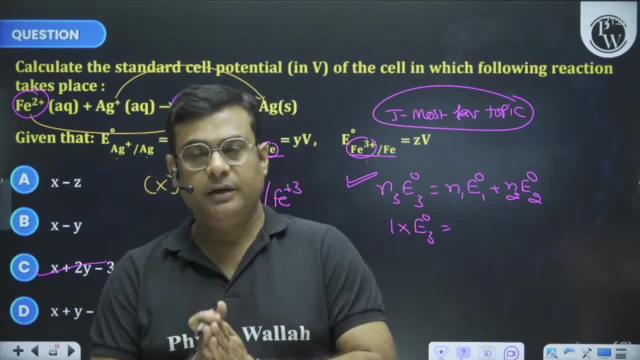 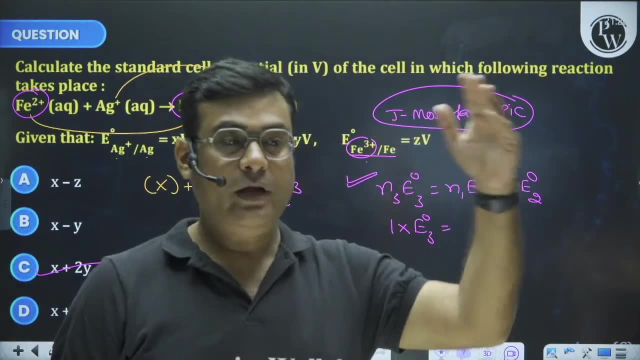 I am standing for you Only with the belief that, after this session, if one question is more correct than that of any of my children, then he will praise me. Maniman will remember me right And, because of that, his selection of one question. 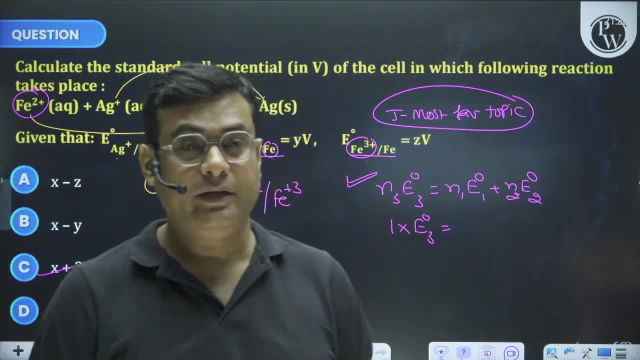 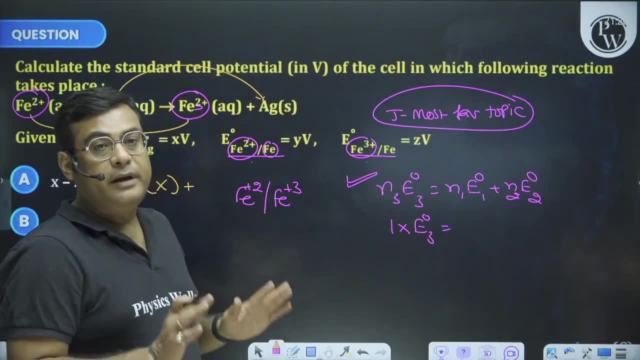 children. you know how much difference it makes. Now the game of in and out comes. Okay, now N1, sir. now these two have been given, Sir, who to believe in N1 and who to believe in N2, it's up to you. 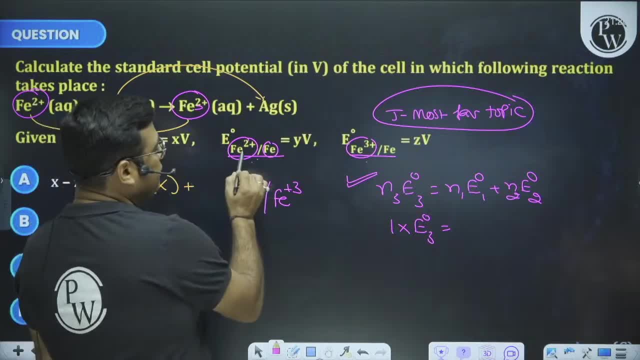 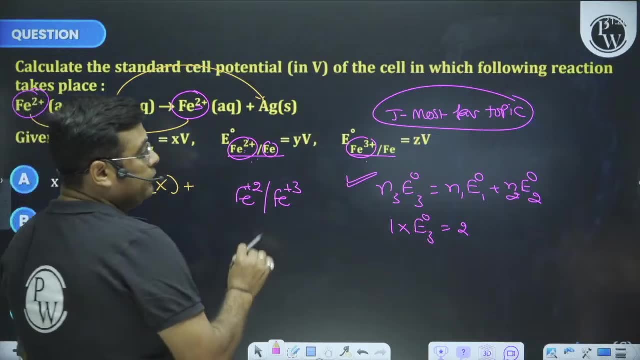 You have to believe whoever you want. I believe the first one to be N1,. so plus 2 to 0. The value is 2 into E01.. What is E01?? Now see where do I want FE plus 2, children. 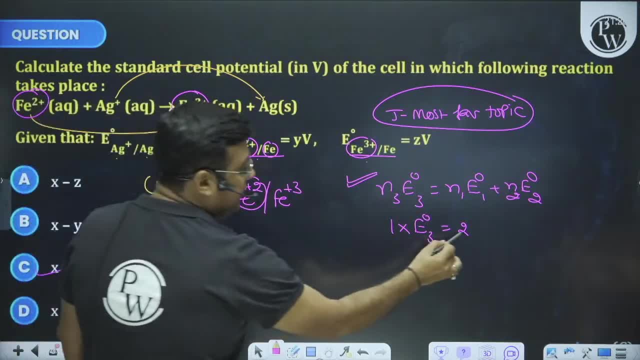 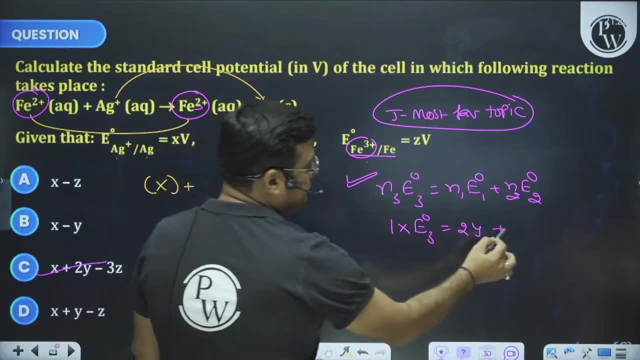 Left side. given is also on the left side, so I have to keep it as Y. I don't need to change its sign. This is over Plus N2. plus 3 to 0 means the value of N2 will be 3.. 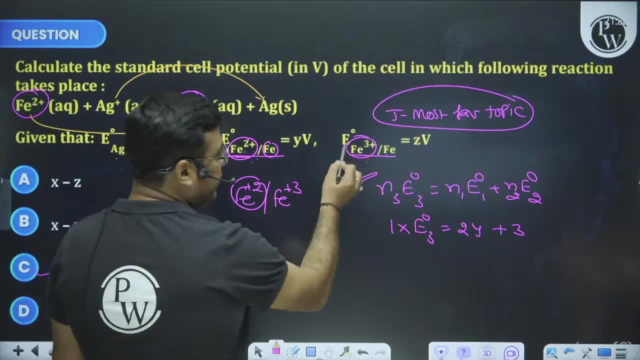 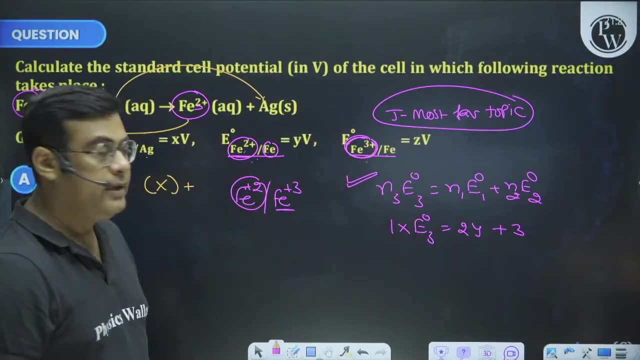 E02, where do I want FE plus 3?, Sir, the product side? Which side is given The reactant side? That means I will have to reverse this reaction. If I have to reverse it, then its E0 minus Z will have to be done. 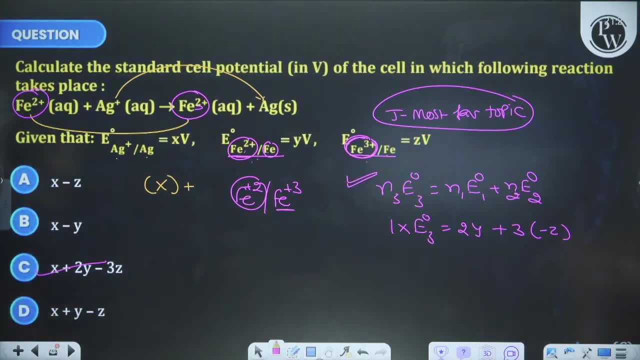 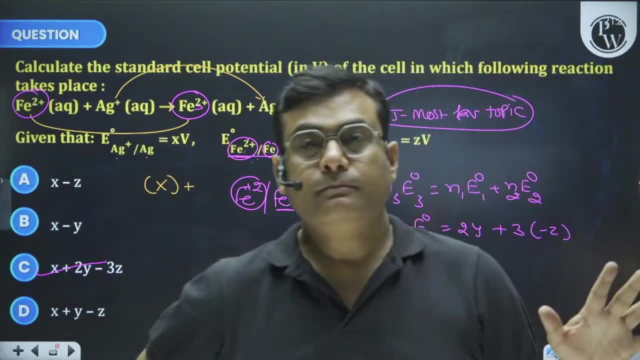 That's why the answer is 2Y plus, 3Z minus. That's why the answer is 2Y children is plus and 3Z is minus. Who is 3Z? It is minus. That is the reason. 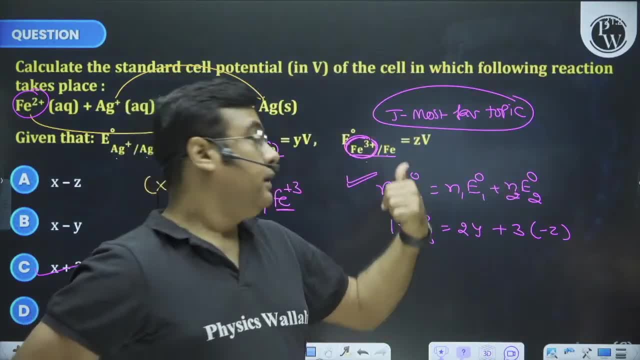 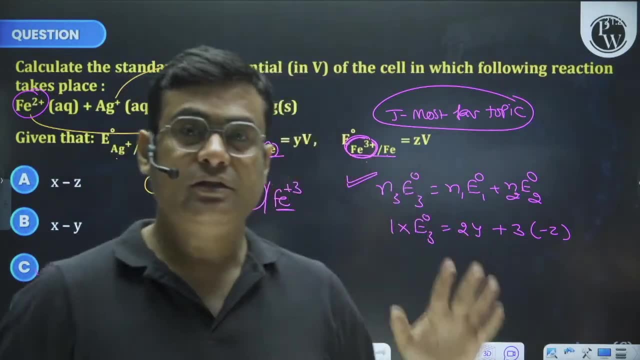 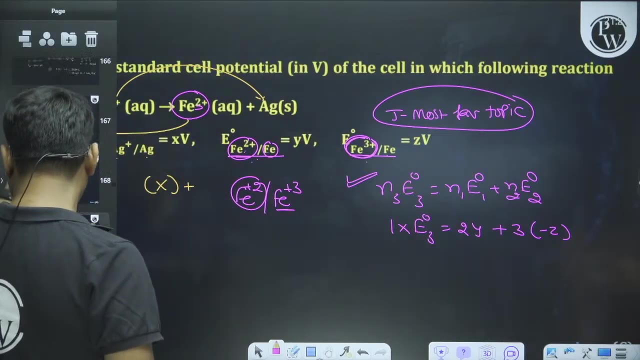 So, on this children, definitely some of you children will definitely get this question Because till now JEE has 8,, 10, 15 times on it. He has asked many things, whether it is main or advance. Okay, come on, let me tell you some more questions about the nurse equation so that you can get an idea of the nurse equation. 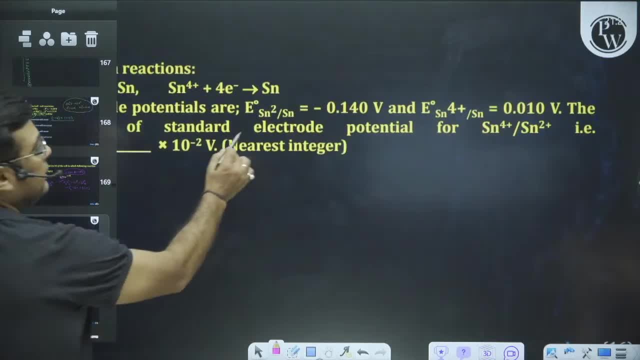 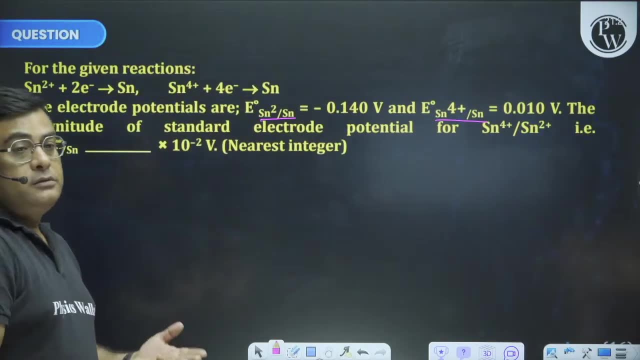 See the next question. I will not solve it now, but I am telling you: SN plus 2 to SN, SN plus 4 to SN. I know that there are two oxidation states of TIN, ie plus 2 and plus 4, apart from zero. 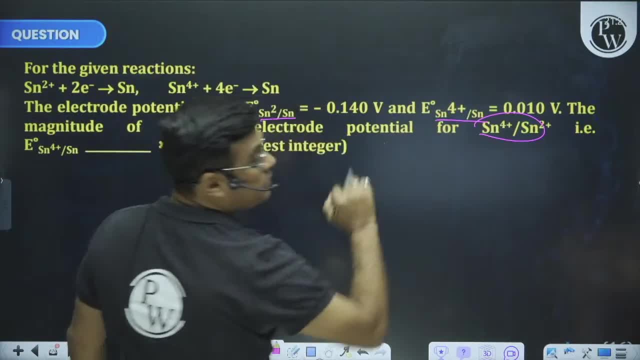 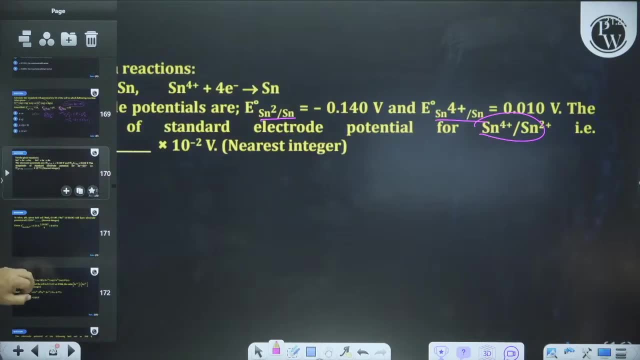 You have those two given and I have asked you whose is plus 4 to plus 2.. You will apply this formula, you will get it. You will get the answer as soon as you apply this formula. Okay, okay, okay, okay. come on, let me tell you some more questions. 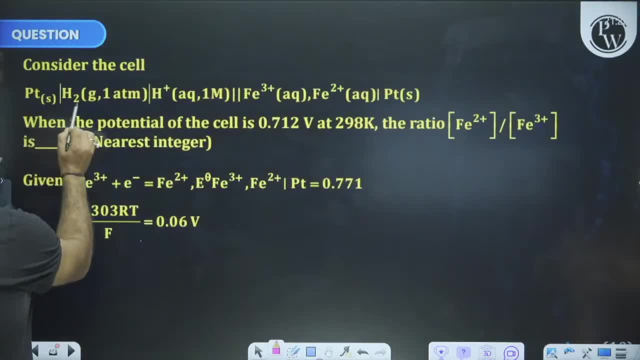 Come on, I am telling you about the nurse equation: PT: H2 gas: 1ATM. H plus aqueous, 1 molar. Fe plus 3, Fe plus 2 PT. When the potential of the cell is 0.712 volt, the ratio of Fe plus 2 to Fe plus 3.. 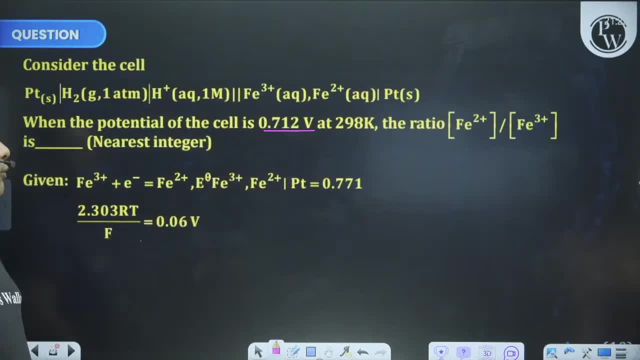 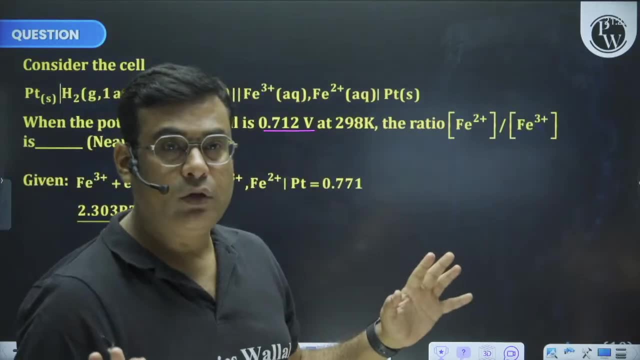 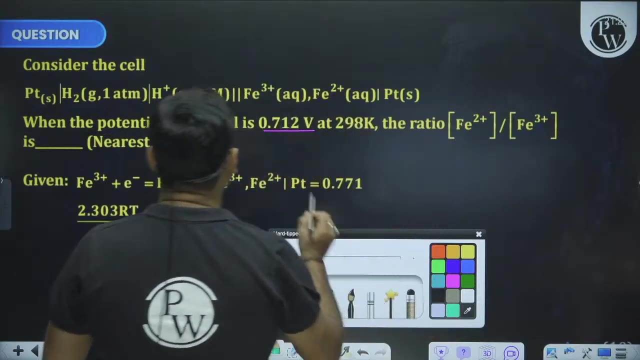 It is given, below the potential of Fe plus 2 to Fe plus 3 is 0.771.. And along with that, the condition is given that you can take 2.303 RT by F as 0.06 volts. Okay, now I am going to tell you about its JSC, then you can tie your waist belt. 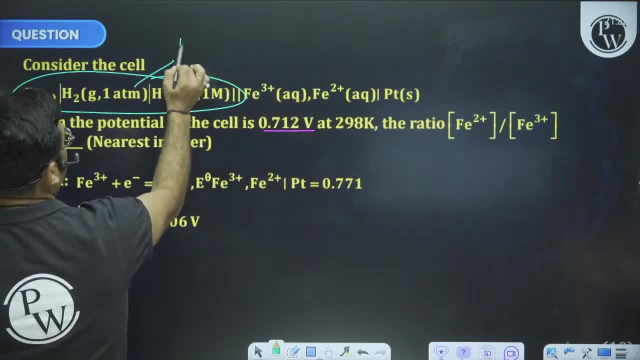 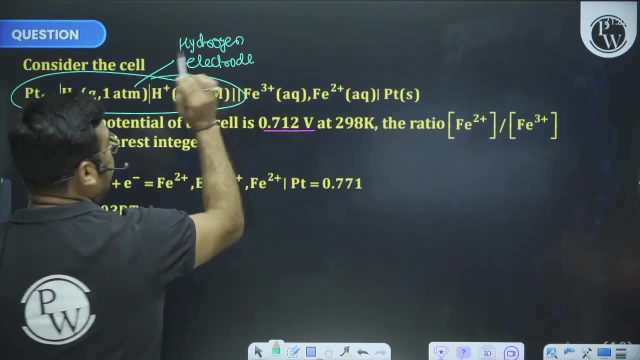 This is the hydrogen electrode. you will have to hear the name: This is hydrogen electrode. this is hydrogen electrode. You will hear the name: SHC- standard hydrogen electrode. IUPSC has considered it as a reference electrode And its potential. 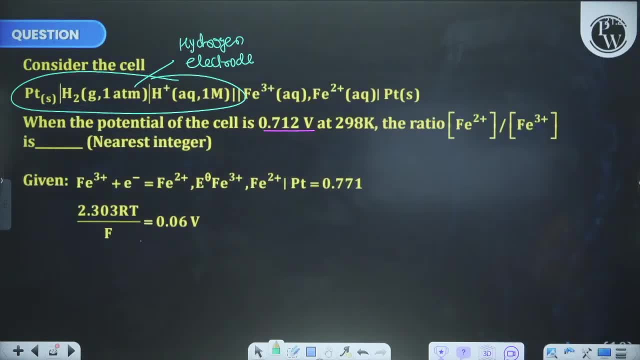 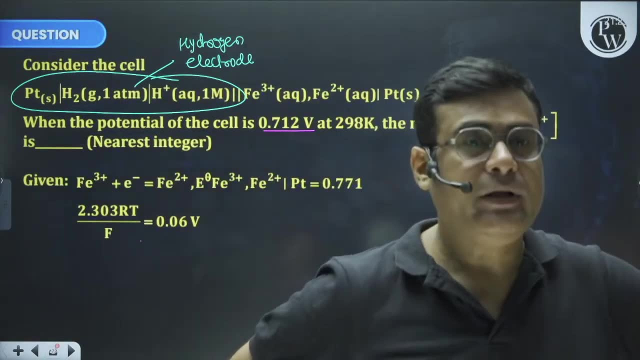 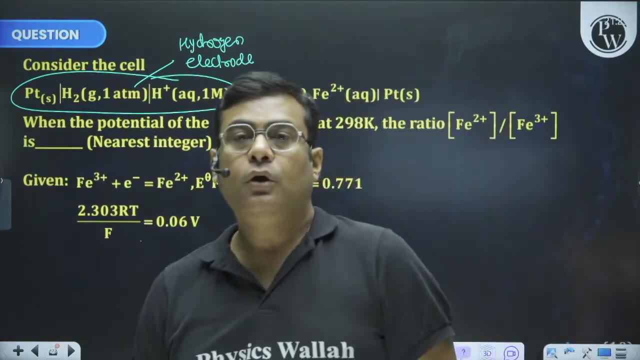 IUPSC has considered it as a reference electrode. Its potential is 0,, but it is a standard electrode potential. And when it is 0?? When the concentration of H plus is 1 molar and H2 gas pressure is 1.. 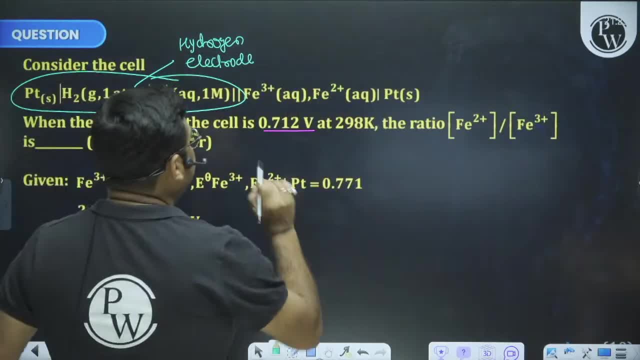 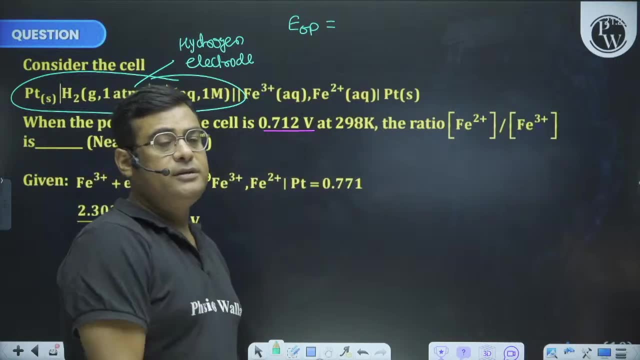 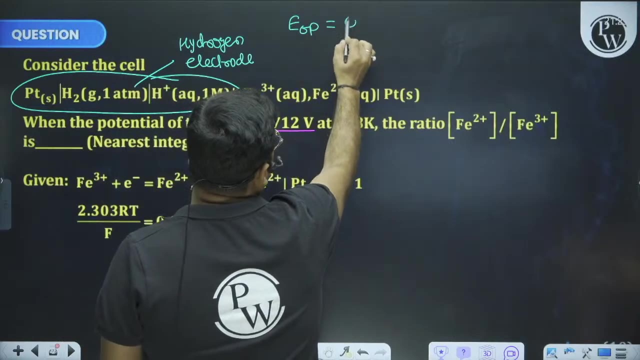 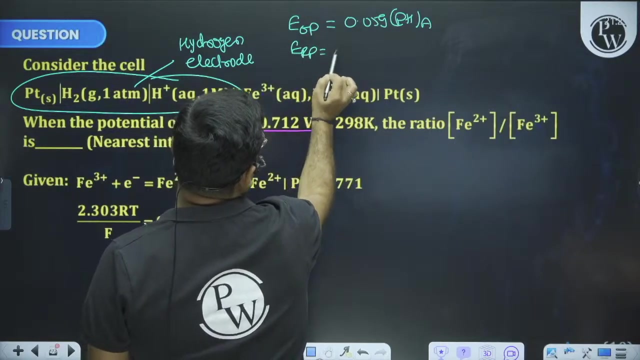 And if otherwise it is not there, then I will tell you its special formula Whose use this year. It has been in the January attempt in 2024.. Its oxidation potential is 0.059 into pH of anode. Its reduction potential formula is minus 0.059 into pH of cathode. 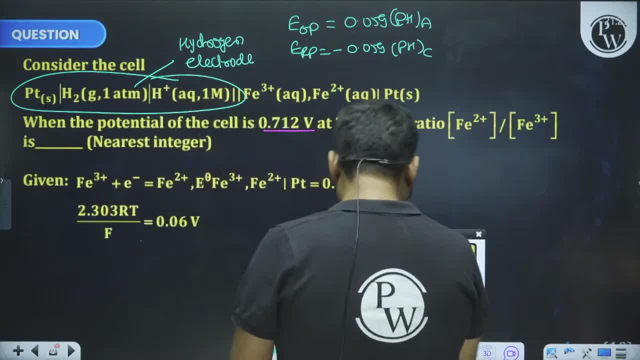 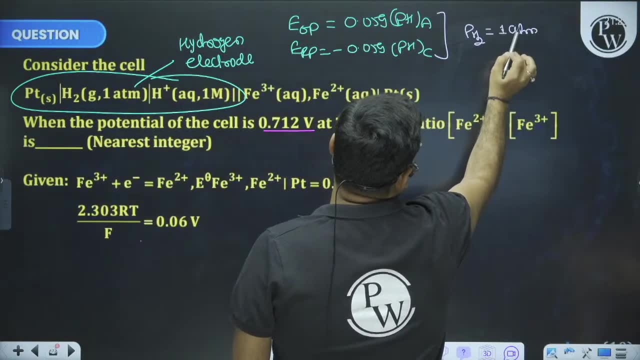 And if ever. and these two formulas are applicable when the partial pressure of hydrogen gas is 180.. If given 1 ATM is good in the question, Then what to do if it is not given? If it is not given, then always take 1 ATM. 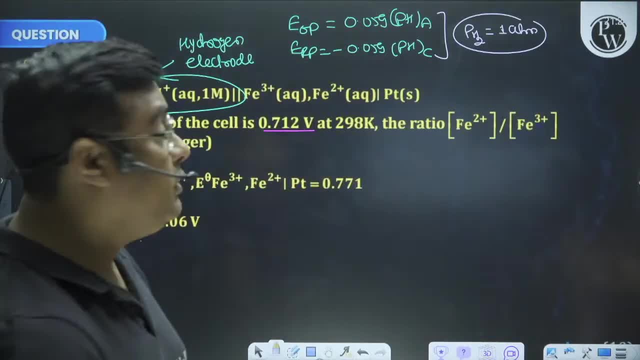 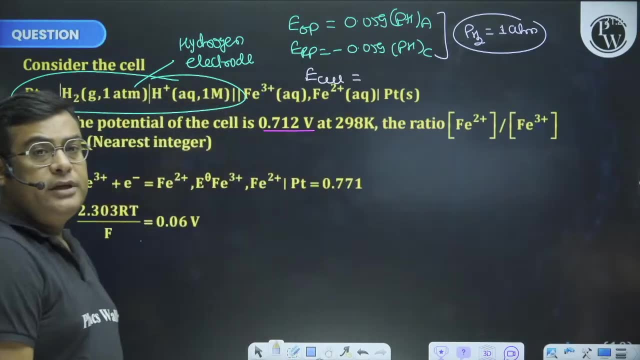 If it is not given, then always take 1 ATM. And if you have made a concentration cell from hydrogen, What happens in the concentration cell? The material of the anode is the same material of the cathode. Then you will add the formula of your cell. 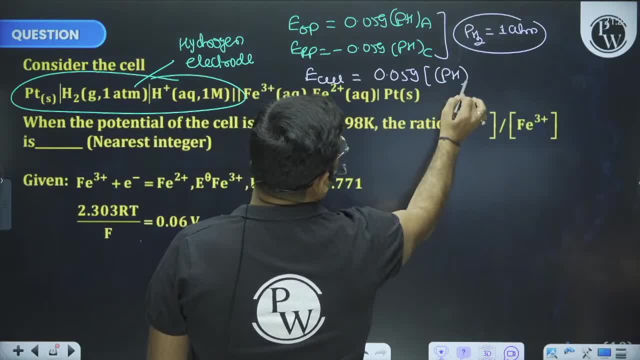 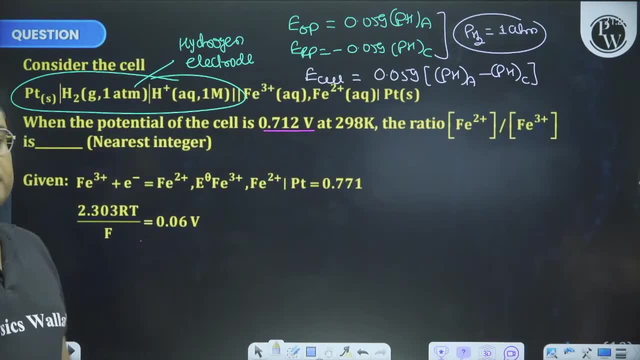 0.059 will come out to be common. What is left pH anode Minus pH cathode? What is left Your pH anode minus pH of your cathode? Rs 100 pay C, JSR 1 by cost C. 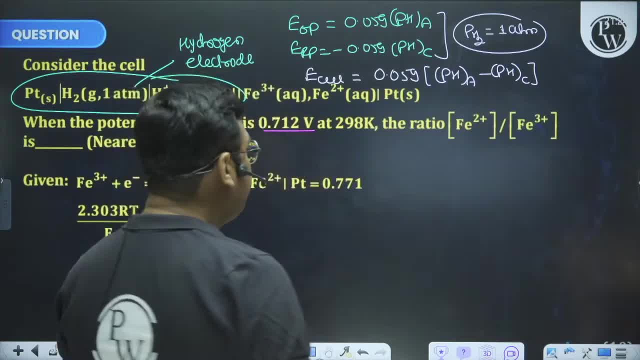 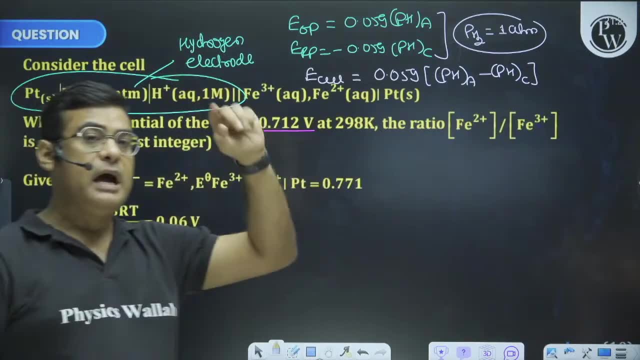 Good thing your message has disappeared And don't even do this kind of thing. Okay, now see what I want to tell you. These are the shortcuts of hydrogen electrode. This year, some of you might also get to see the question on it. 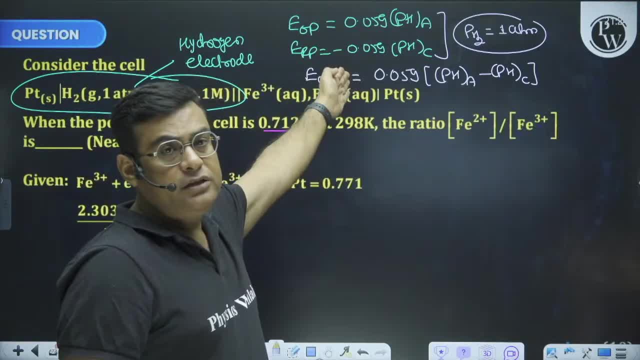 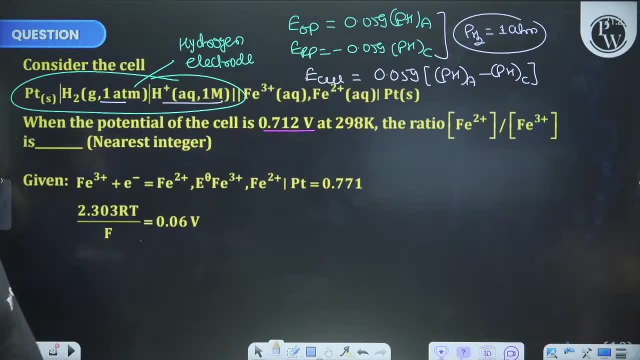 If the question comes on hydrogen electrode, Maybe these three shortcuts- You will click on it Now look here: The pressure of hydrogen gas is also 1.. The concentration of H plus is 1.. If the concentration of H plus is 1, then the pH has become 0. 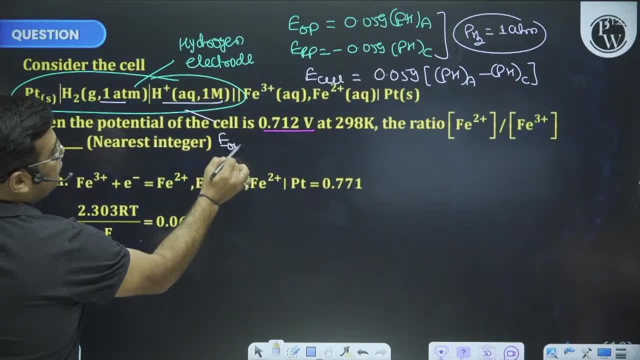 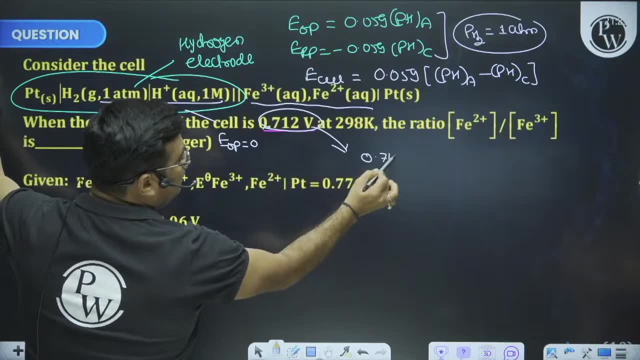 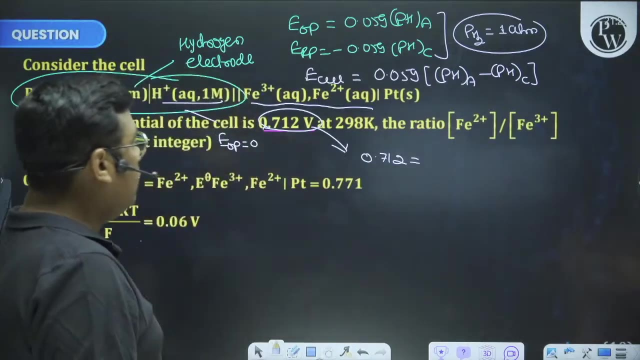 That means the oxidation potential of this cell has become 0.. That means whatever this potential is, children, it is only its reduction potential. So if I try to understand things properly by looking at them without any reaction, Then 0.712.. 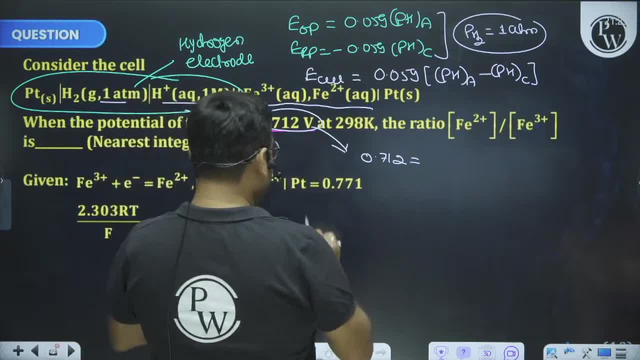 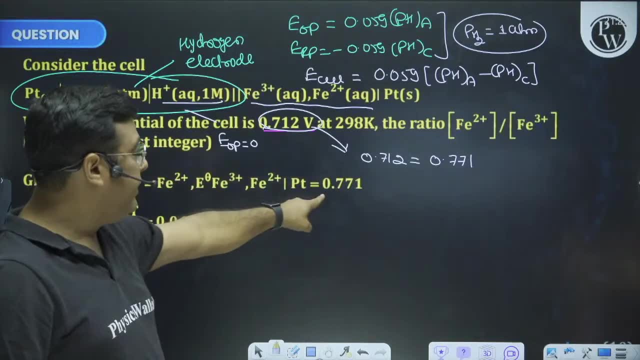 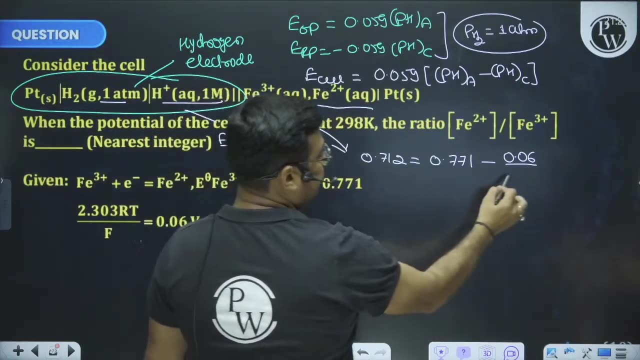 Reduction potential is equal to 0.771.. Agreed, Agreed. The given value is minus. They gave the value of RT as 2.3. The value of RT is 0.06.. By N it is going to Fe plus 3 and Fe plus 2.. 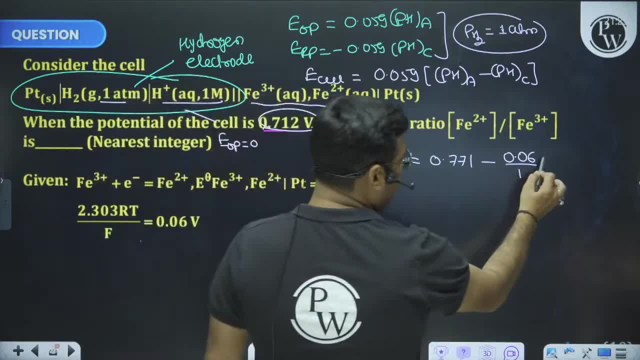 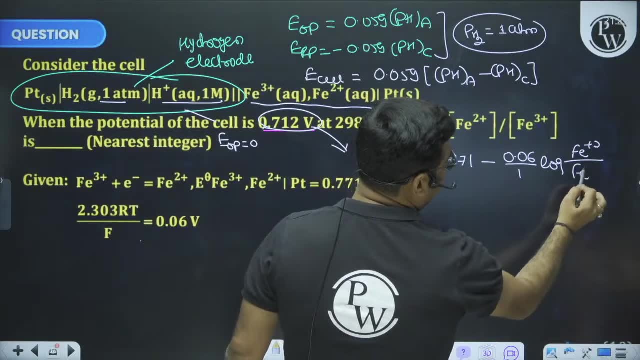 So the value of N is 1.. What is the log? of Reduction is happening. It will go to Fe plus 3 and Fe plus 2.. Up will come Fe plus 2.. Down will come Fe plus 2.. Down will come Fe plus 3.. 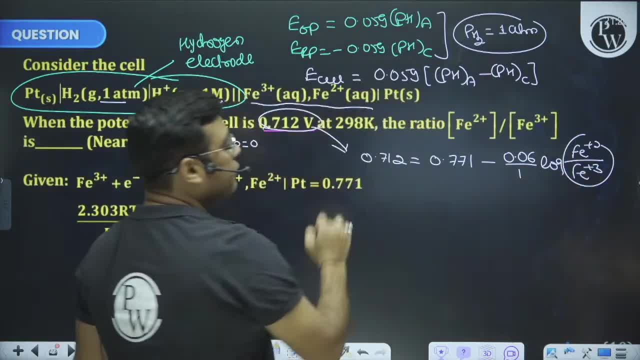 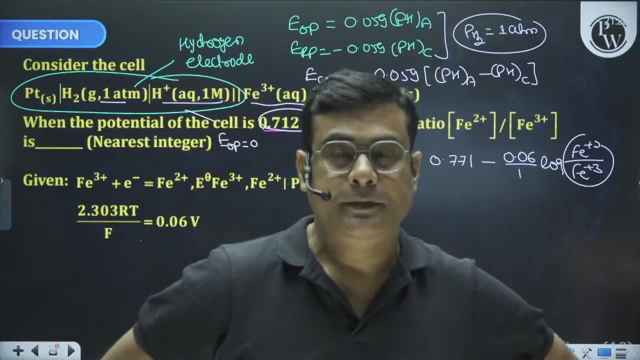 This is the only value asked from you. Take it here. After doing minus, your answer will come. Now you can see the solution in the book. You will have to clap fast. What will be the solution in the book? The reaction of anode will be written separately from H2 to H plus. 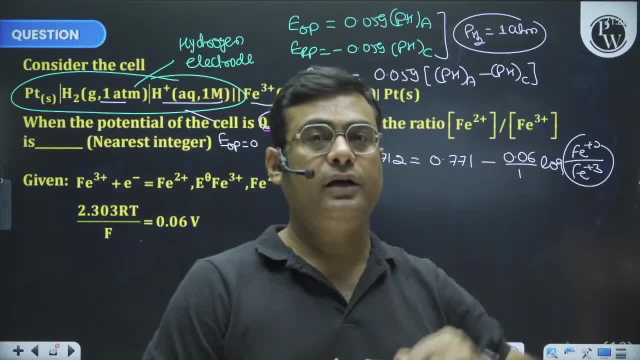 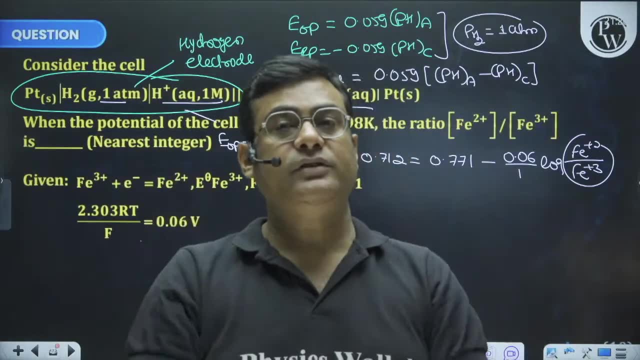 Its anode is 0.. The reaction of the cathode will be written separately, Then the net full reaction will be written by adding both. Then they will have put the NERST equation to add on both. So the answer will be 5-6 steps. 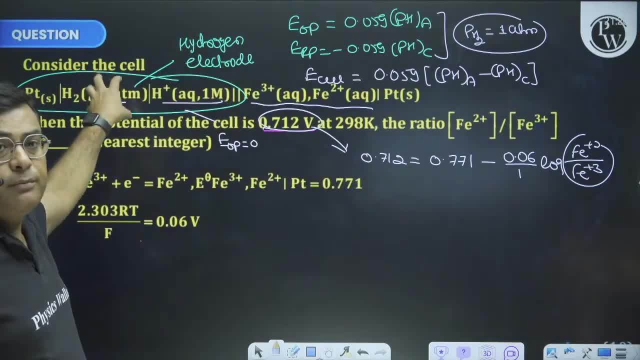 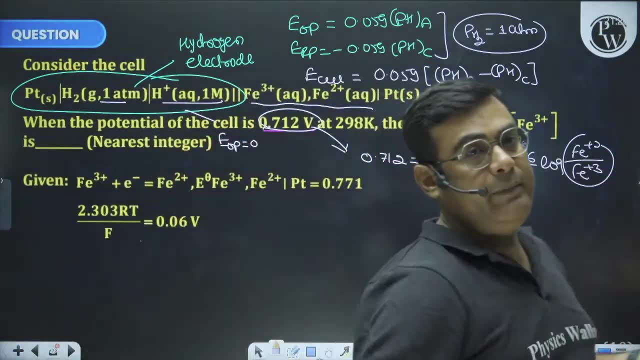 But if I knew this method, I saw clearly that its potential is 0.. Whatever the potential is of this cell, that reaction, if I have clarity in my mind, if we have read everything properly, then this is a revision session going on kids. 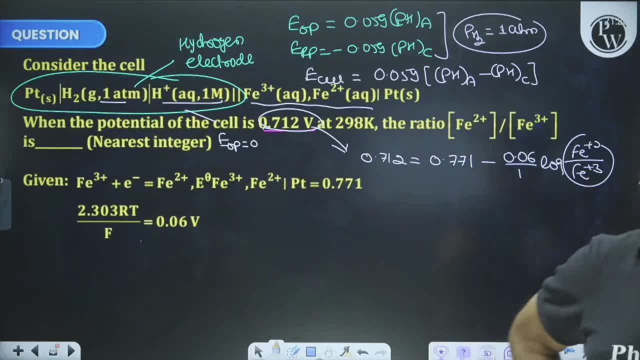 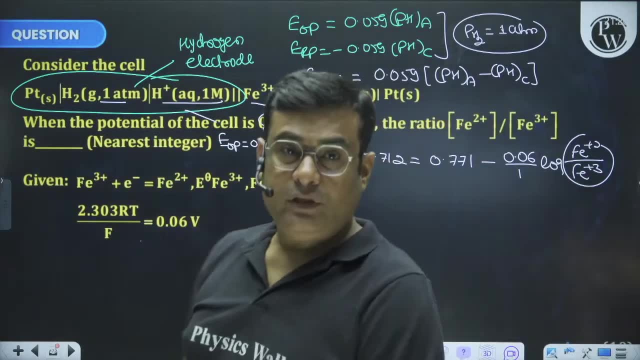 This is a revision session, kids, So if you have read it, then you would be aware that it is a cathode half cell reduction: 3 Fe plus 2 will go. Tell me, is this thing worth clapping? Did you understand this story? 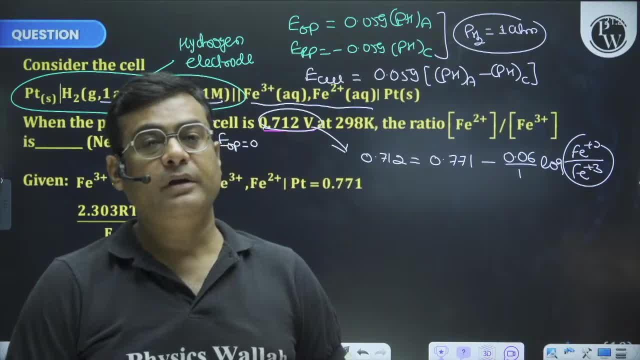 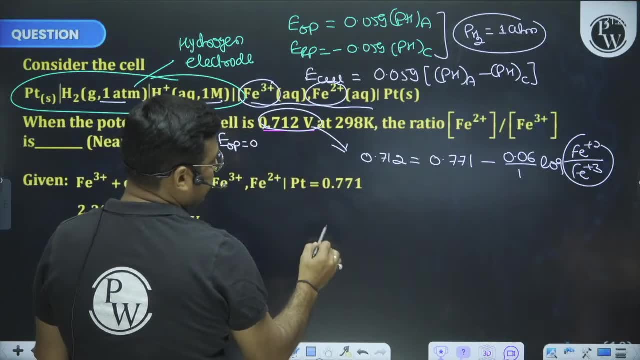 What did we say? In this way, you children also have your time here. Sir, please explain the one above and below. Reduction is happening right In reduction it will go to Fe plus 3 and Fe plus 2.. I mean, if you do not understand, then I am also writing the reaction for you. 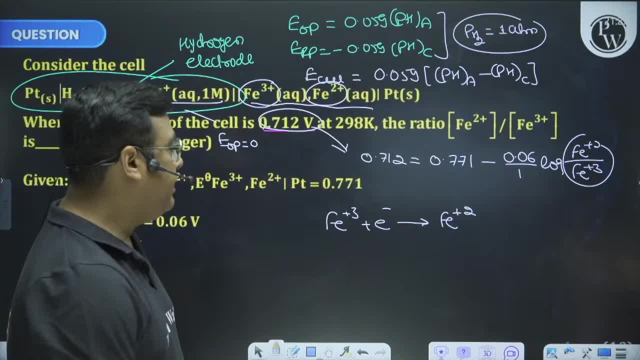 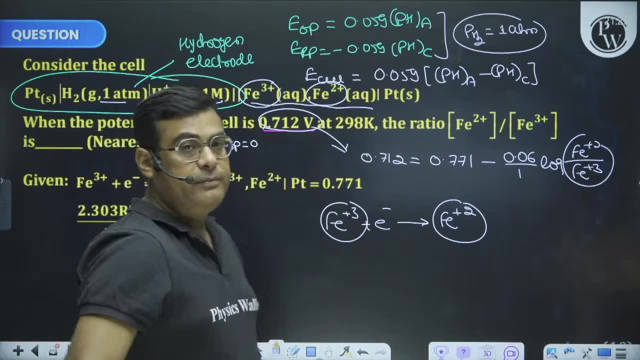 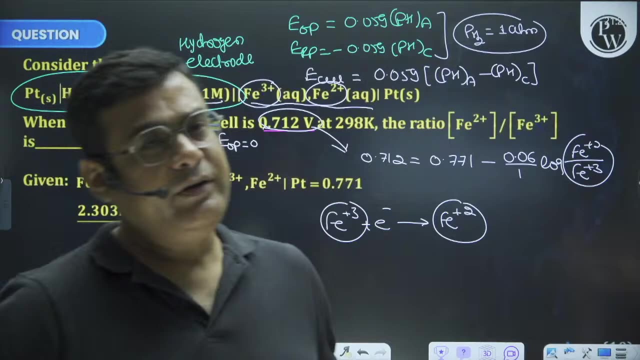 Fe plus 3 will go to Fe plus 2 with the electron. So obviously this is the product side. so this will come up. the product comes up. this is the reactant side. then it will come down. my dear children, See how many chapters are left: Liquid thermo and your little atomic. 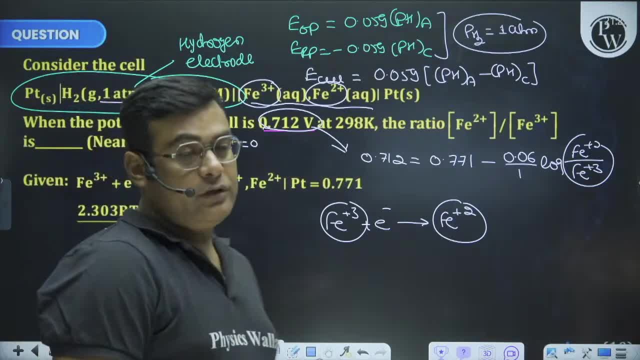 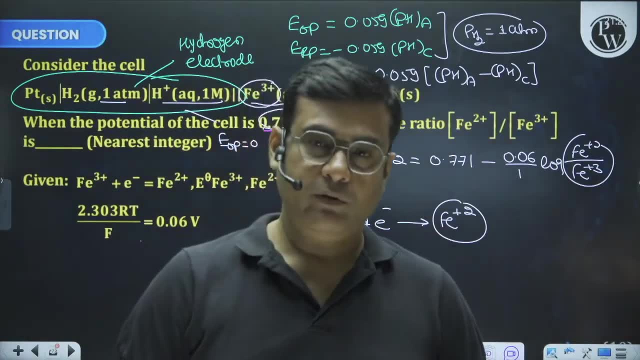 Why do I keep thermo and atomic last? I will tell you the reason for that: Because they both are common with physics. Tomorrow, when you will study physics of eleventh, you will study thermo very well, As well as the physics of twelfth you will study in that modern 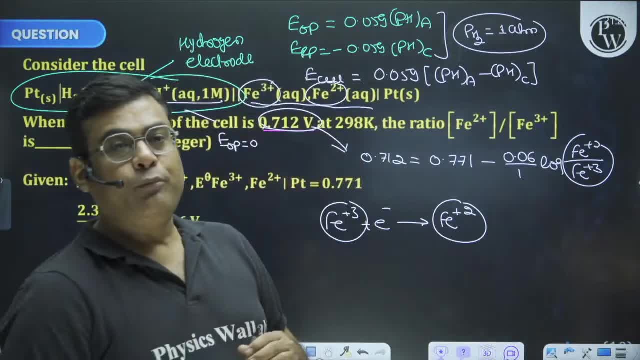 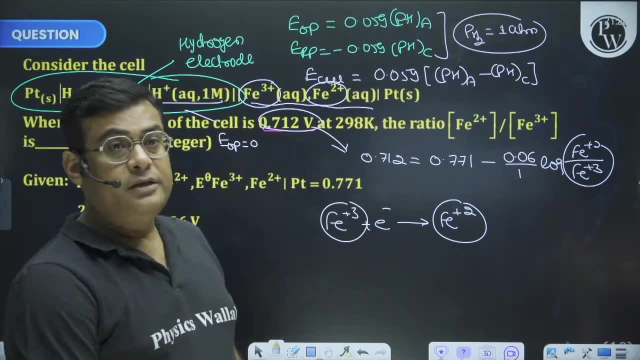 In physics, the whole atom is called Because of this. if 0.059 was given, then the calculation would have been good. That's what I am saying, son. This is the cleverness. The girl who wrote it- Priyanka is her name. 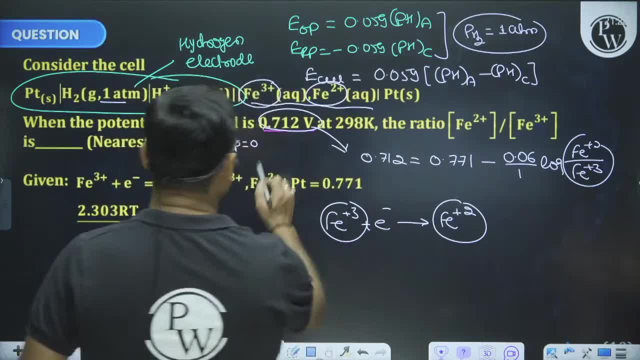 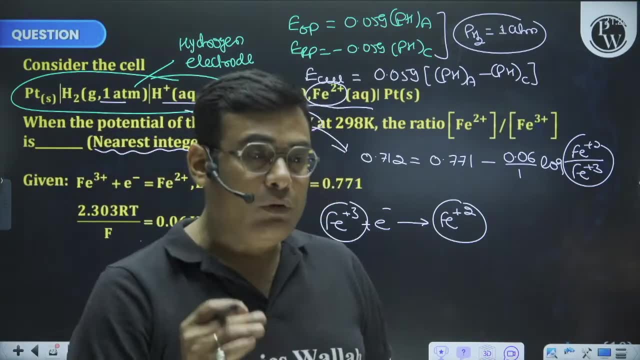 This is the cleverness, son, That he is also giving you nearest integer. So this is what I want to explain. I asked for today's session of Ladha Jagad that I should explain the calculation to the children That here you have not been given. you have to take it. 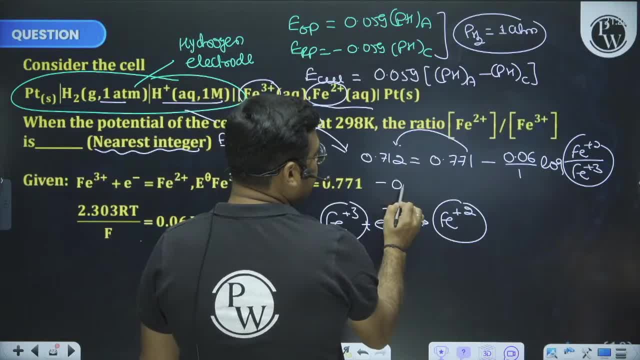 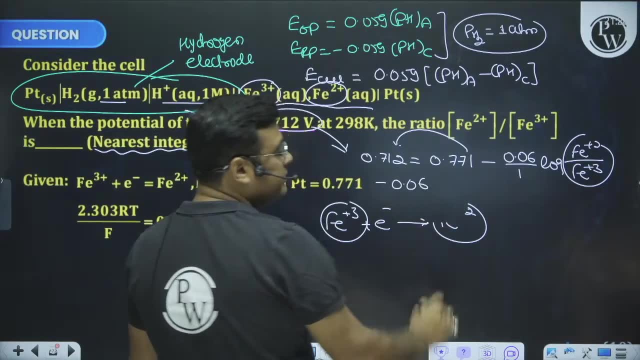 Because when you go here and minus it, then 0.059 of minus will come. So, brother, you do not take it minus 0.059, you take it 6 only Why? Because there will be no difference in nearest integer. 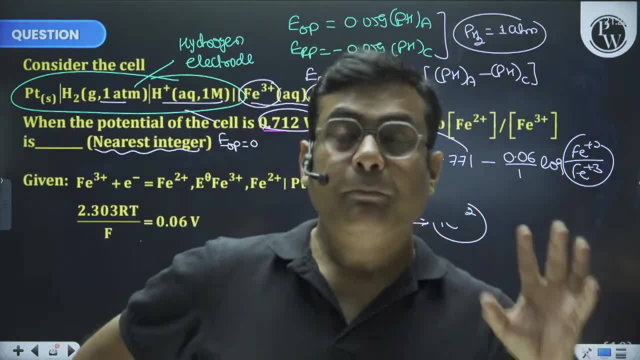 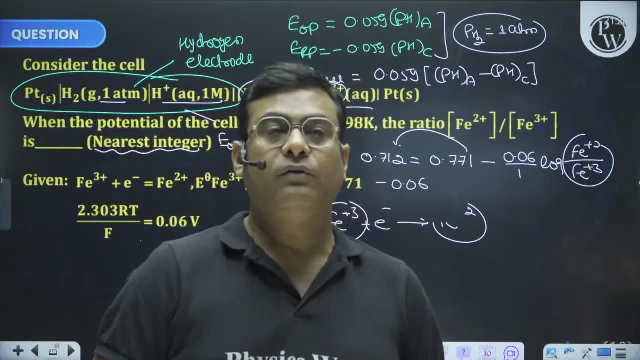 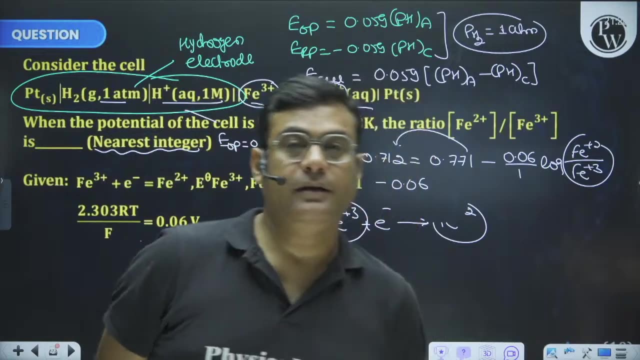 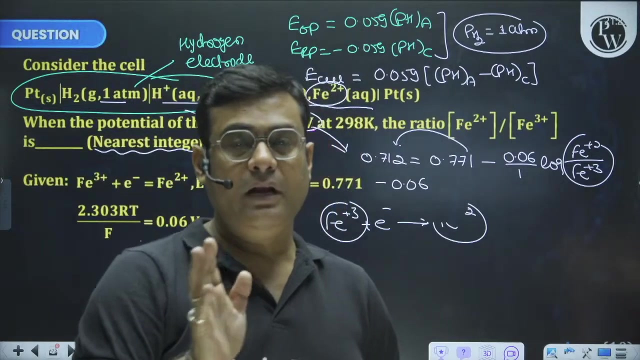 There will be no difference in nearest integer. I am trying to explain to you that brother in the questions of JEE you think that calculation comes very badly. He sometimes tries to do it, children. I also know that it is bad to give calculation, but if we are mentally prepared, so many questions, children, if I have taught you 150 questions in the class, explained it and with the calculation till the end, then you understand something. 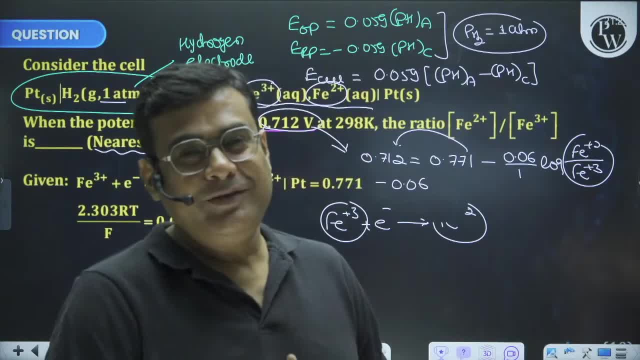 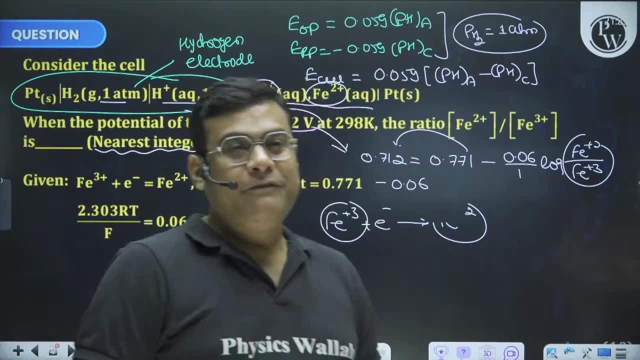 You said this right, that the chemists say in physics and the physics people say in chem. Now, son, whatever is coming, it will keep going, Isn't it? In physics, priority is given. Tell me, chapter wise, priority, chapter wise, son. the most important ionic electrode is there. 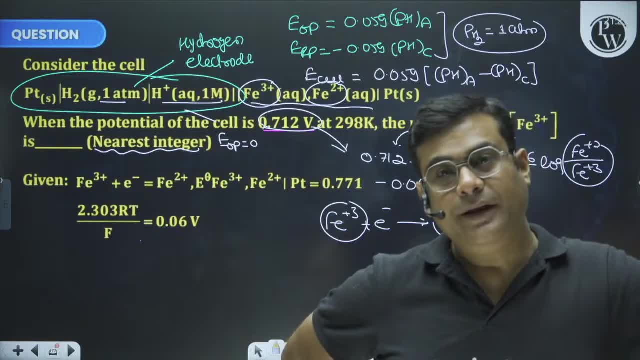 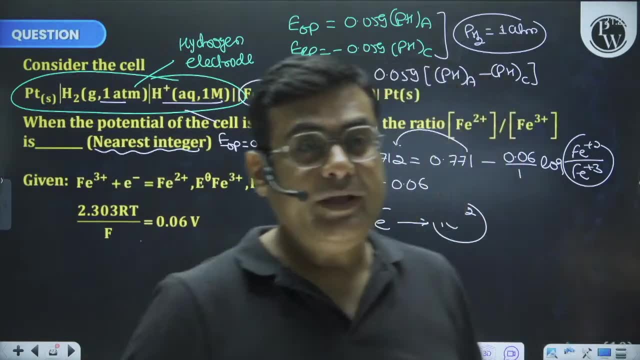 There are guaranteed questions on them. You will definitely come to the question of delta g naught in thermodynamics. Question is correct. There are questions on the question of delta g naught in thermodynamics. There will be a question on the first order in kinetics. 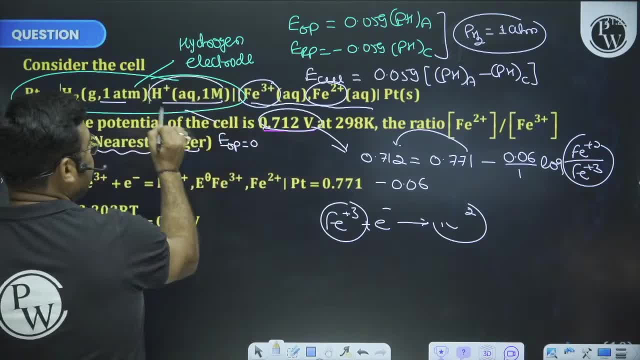 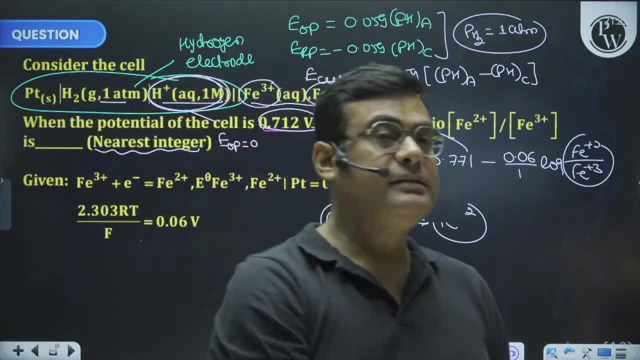 Sir, why is EOP 0?? Son, if the concentration of H plus is 1 molar, you guys get lost. I don't know That you are in the exam. How will you stay concentrated for three hours when you forget here? 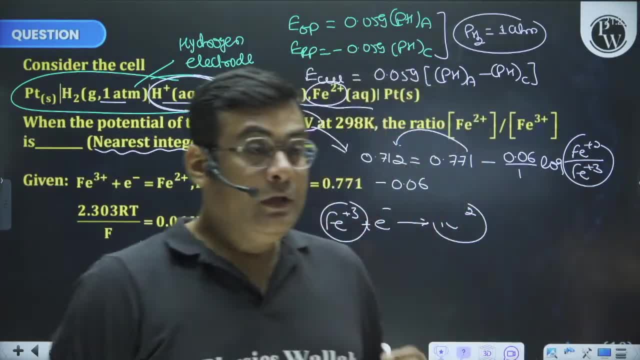 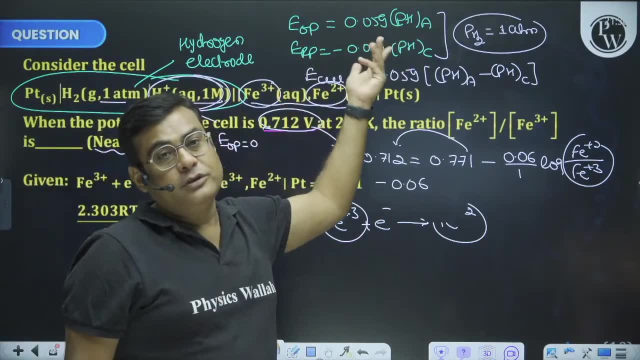 You are not. Concentration is your loose. Okay. So if the concentration of H plus is 1 molar, then pH is 0 and 0.059 into 0. Multiply 0 with any number, it makes it 0.. 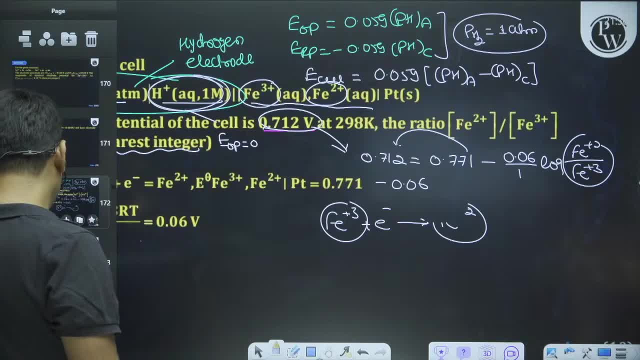 That's why it became 0.. Okay, let's go. Let me tell you some more, Son. I'll tell you more in a few questions, Son, I'm telling you more in a few questions Now, as this is the question of the equation. 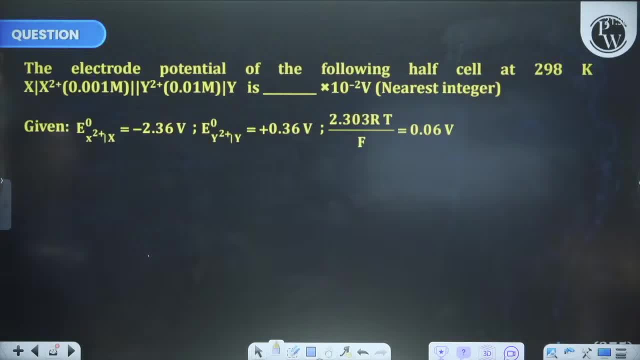 Son, I'm telling you more, Son, I'm telling you more in a few questions. Now there is a question of the equation. But if we show a little time- see Oxidation of X- they have given reduction. 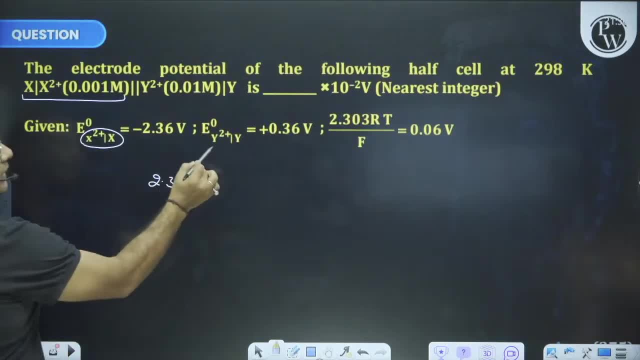 So do minus plus 2.36.. Reduction of Y2 is plus 0.36.. This is your E0.. E equal to E0.. E equal to E0.. Yes, the solution is the chapter after this, Son. the next chapter is the solution. 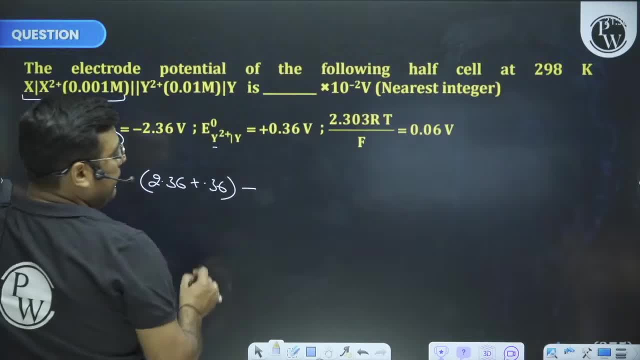 2.36 plus what is your 0.36?? Minus- Now they have seen 0.06.. Minus- Now, they have provided 0.13.. That's why the cái n is like 0.16.. 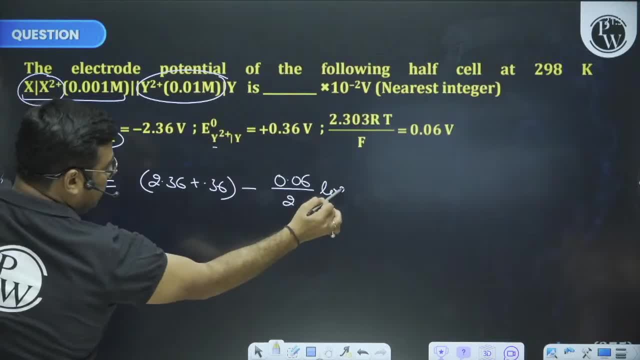 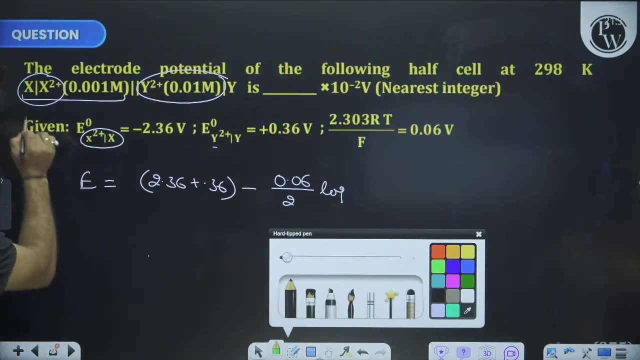 and here n is constant. But as we go this much way, It is getting further. Now the reaction is not: what is patented is done or reduced. щее is not. Now you tell me that. what will be the value of this n? 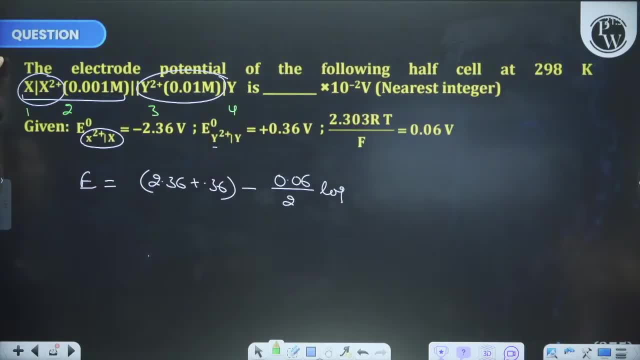 If there are two electrons here, then here too there are two electrons, So n becomes two. only Now let me tell you one more trick: to swim reactant side. comes product side with E1 number, comes reactant side with odd number. 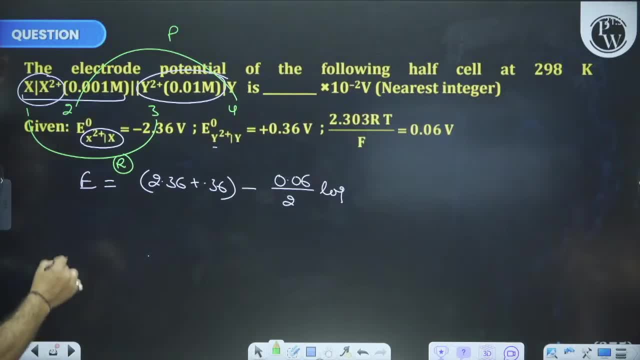 comes, because if you write its reaction, I am explaining by writing the reaction. what reaction will you write on anode X gives X plus 2 plus 2 electron. what reaction will you write on cathode reduction of Y plus 2 plus 2 electron gives Y. now you will add: 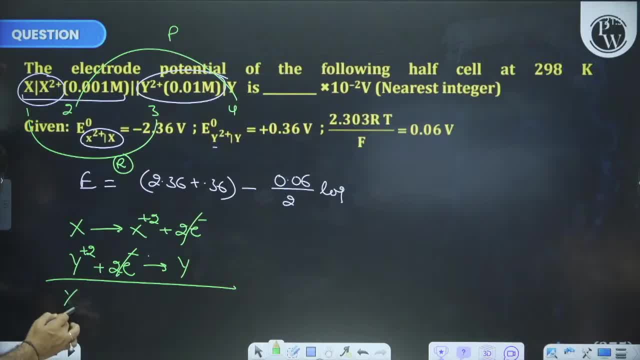 electron. electron cancels X plus Y plus 2, gives X plus 2 plus Y. now you see, this is written on 1, this is written on 3, both are reactant side and these two are product side. so 0.02 log: X plus 2 comes up 10 to the power minus 3, Y plus 2 comes down 10. 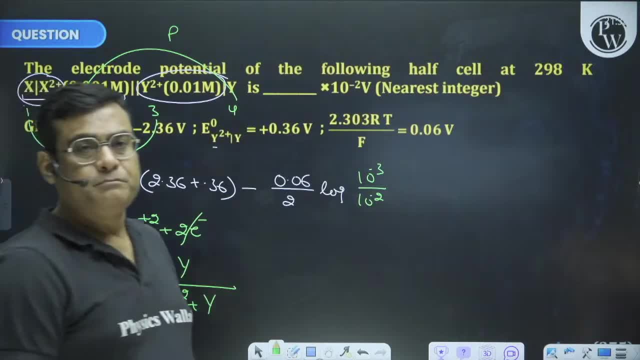 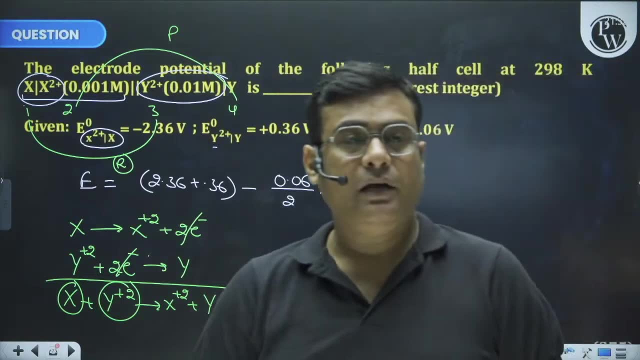 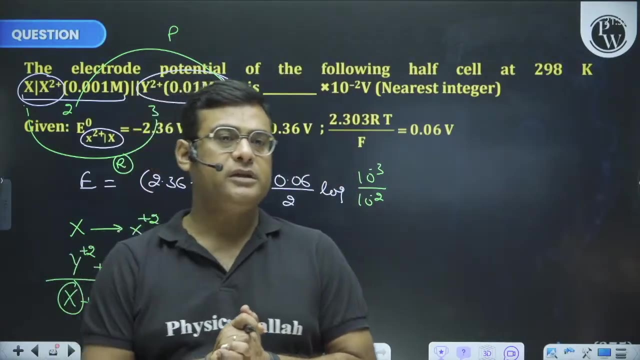 to the power minus 2, this is not over. ok, we all, every child. we make the same mistake chapter when we read it for the first time. make a backlog and make it long, otherwise simple, simple loving things by understanding them. questions can be easily. 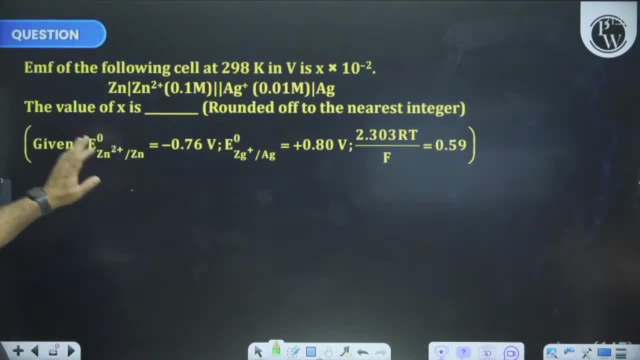 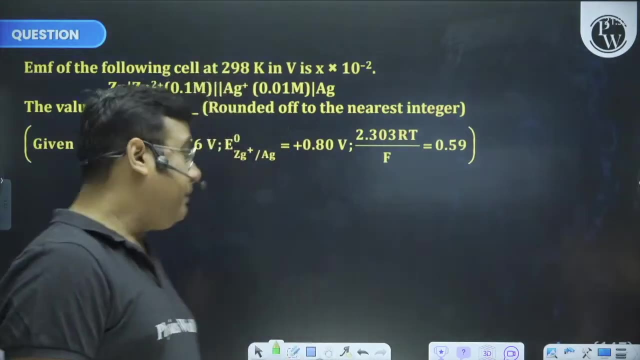 increased. can you understand what I am saying now? see, there are many questions. now there is no meaning of asking every question, but these are old questions of JEE. by this, how do you know about odd number? I have given proof of that. I am not lying. we have been studying for 23 years. 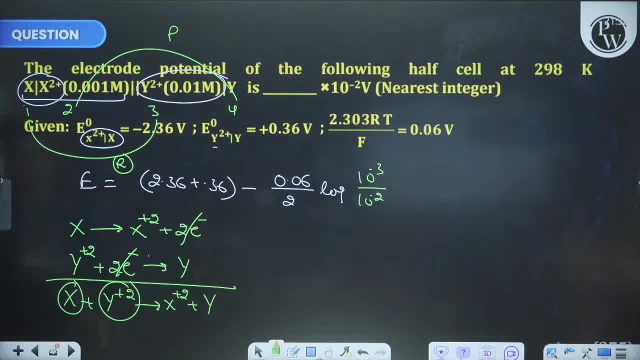 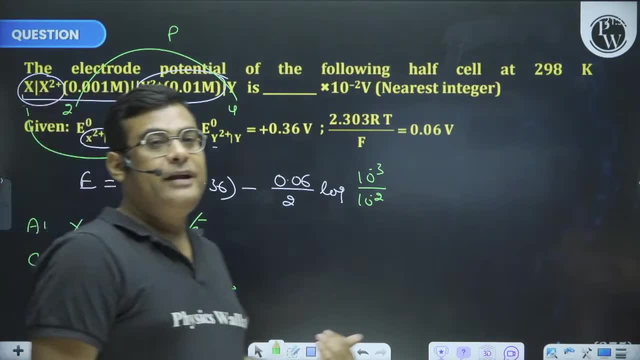 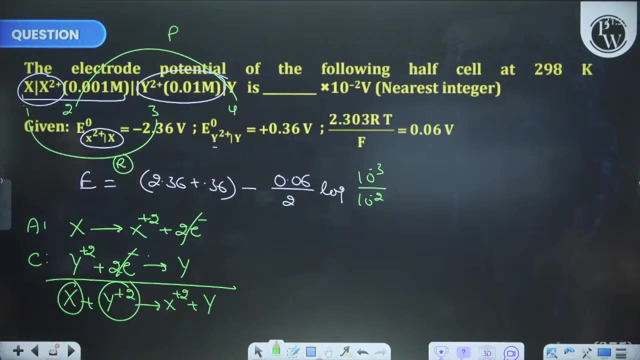 when we write reactions, every time we write the same reaction- anode per oxidation, cathode per reduction- and when you write like this, odd number, reactants will come and even number, products will come. there is no exception. now see in this ZN to ZN plus 2. 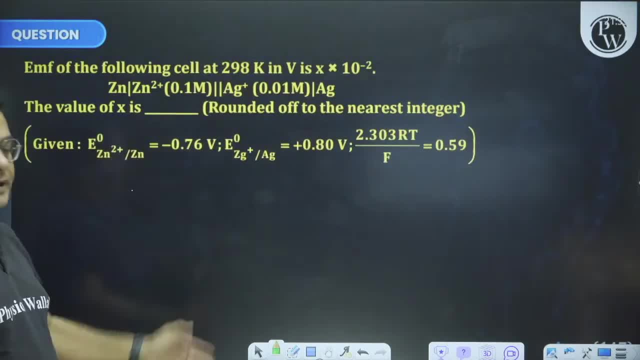 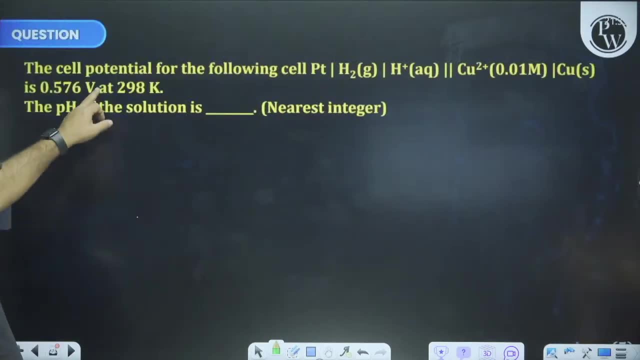 AG plus to AG. it will be done easily. see more. I will show you on electrolytic. now see gas ion with PT H2 H plus Cu plus 2 Cu, cell potential pH of the solution. no problem, just put NERST equation, answer will come see. 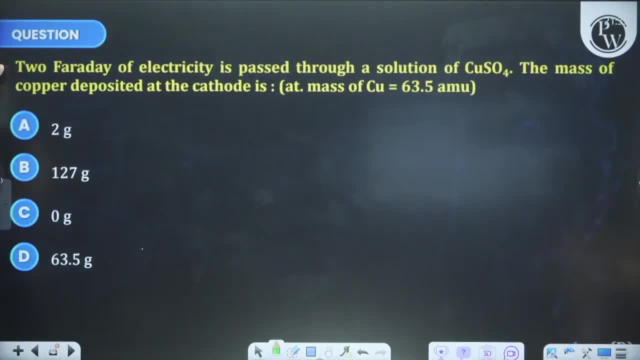 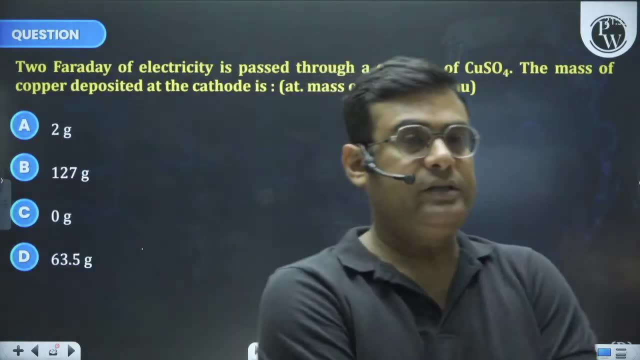 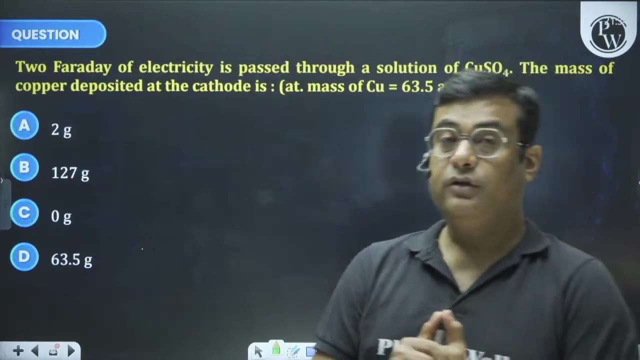 you will talk about electrolytic cell. tell me about some conductance, sir. tell me the answer of HW. answer is for all. there is no problem. in the next 4 days time you must solve the remaining questions. I am telling you in conductance. I can't leave conductance. 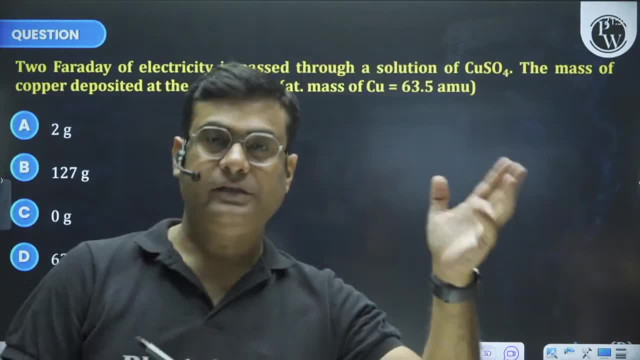 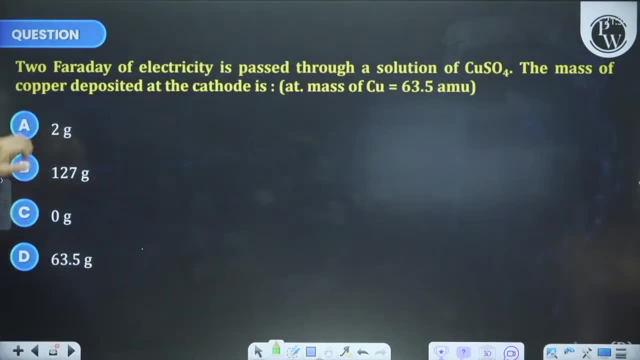 conductance is important in that I have more good techniques to explain. see what I am doing on electrolytic cell: 2 faraday of electricity. as soon as 2 faraday comes in your mind, 2 equivalent should also run immediately. now what is further in the question? 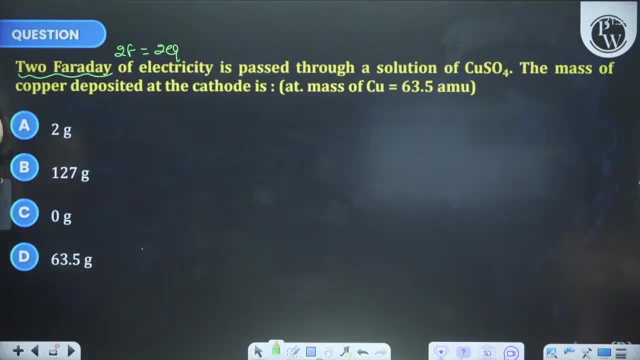 I don't mean. I am saying 2 faraday is written, 2 equivalent should run in your mind- is passed through a solution of CuSO4, the mass of copper deposited at cathode. 2 faraday means 2 equivalent. now I have written the formula. I know one formula equivalent, equal to N factor. CuSO4 has copper valency plus 2, means its N factor is 2 into W. the mass asked divided by atomic mass 63.5. the answer of W is 63.5 gram. the answer of W is: 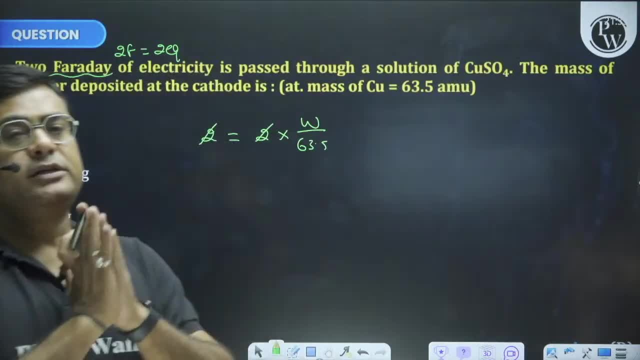 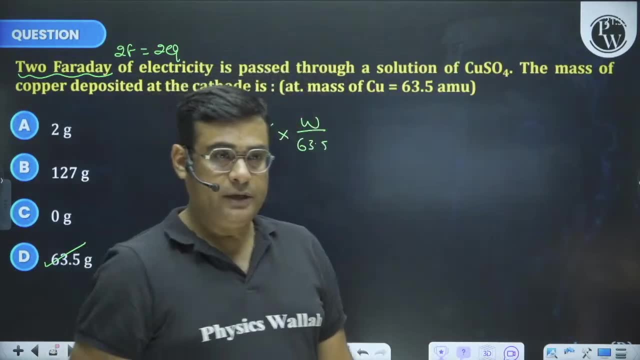 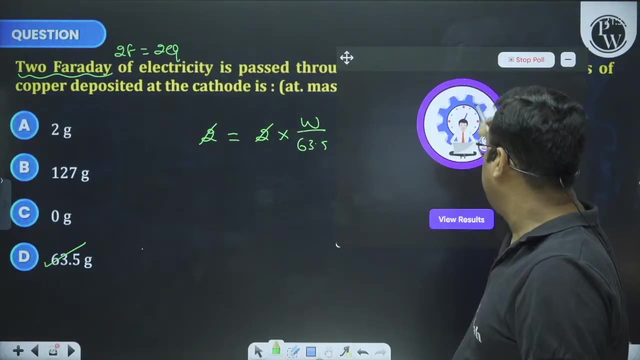 63.5 gram. we didn't do anything, we just logically, what you know, what you have forgotten, what you know. ok, we will do a poll of 1 minute and 2-4 minutes. sorry, 2-4 minutes. you will get tired. I will sing a song. 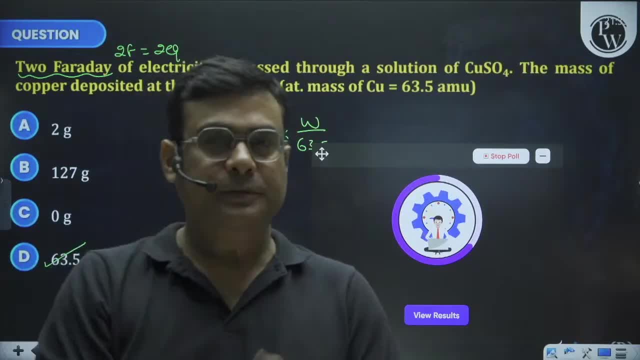 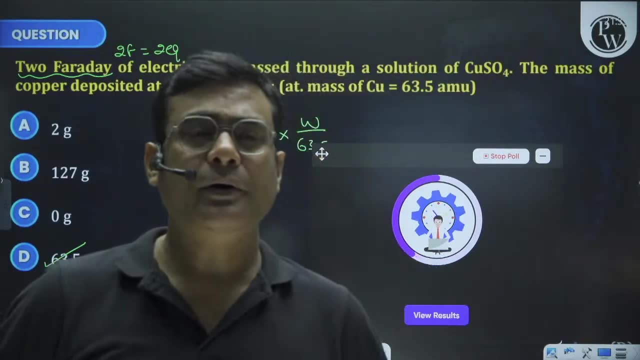 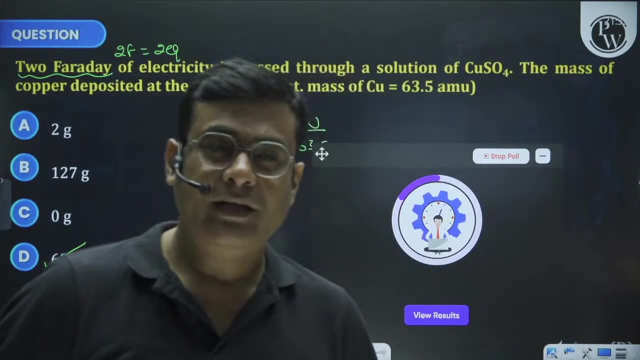 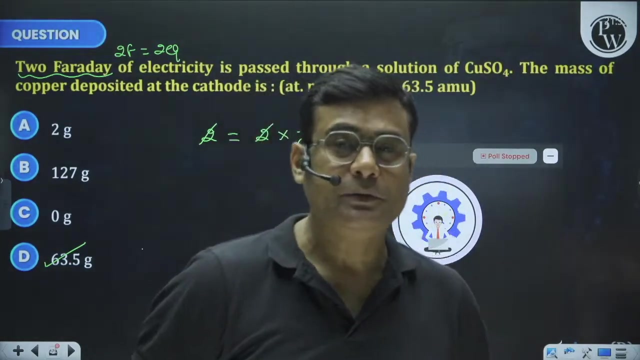 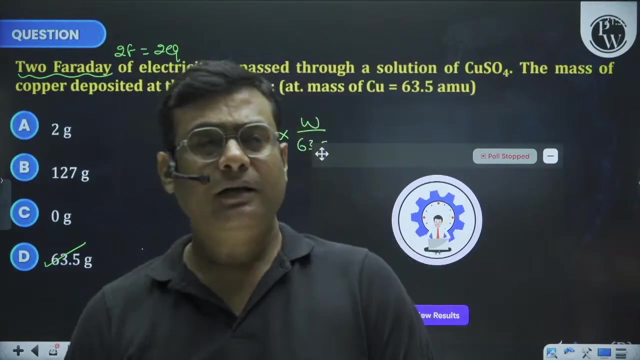 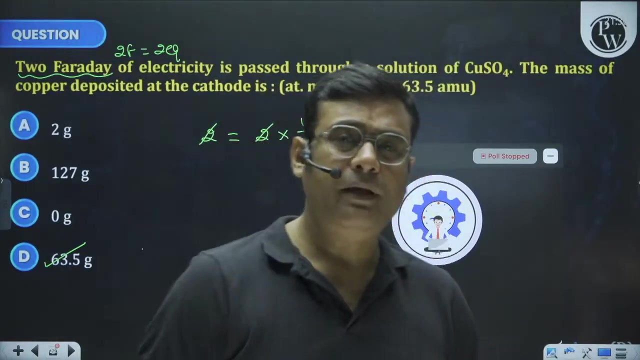 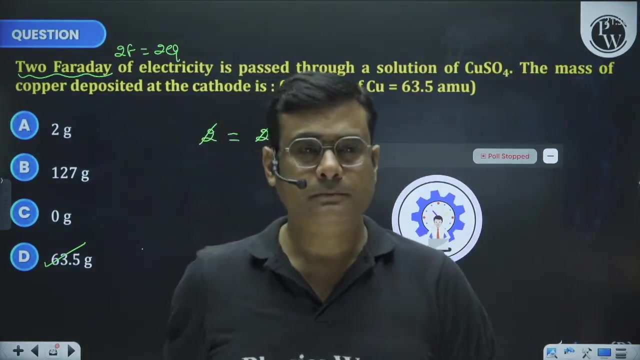 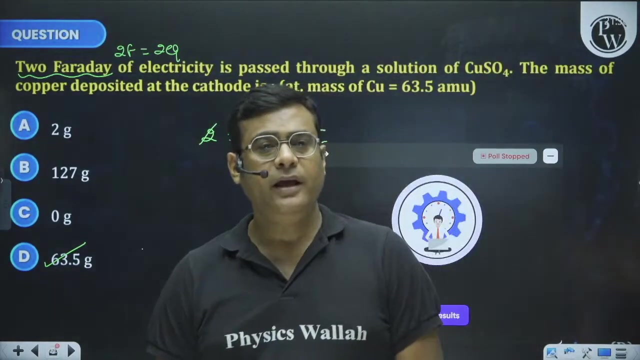 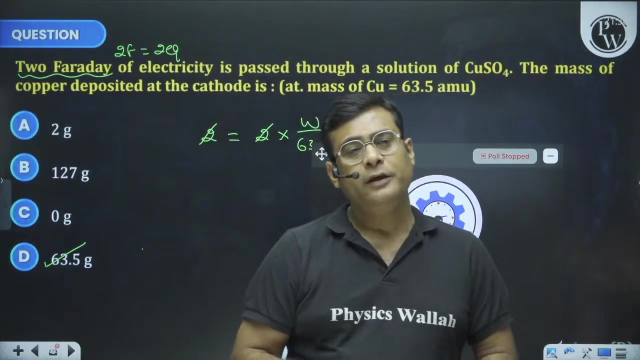 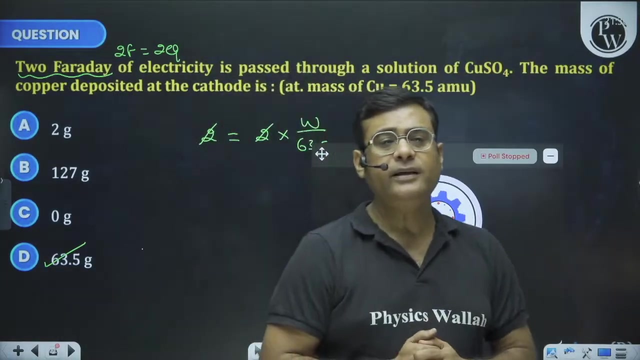 my favorite song. many children will sing. you will like it. our mind will change my moonly beloved. when I thought I, yes, you are exactly like. I thought, yes, you are exactly like. I thought: no promises, no surprises, no tip make. when I now BHA DI I. 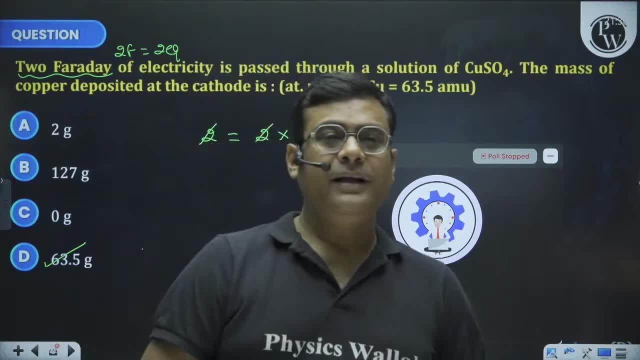 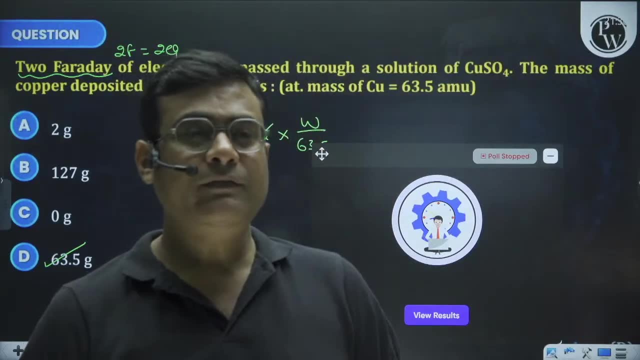 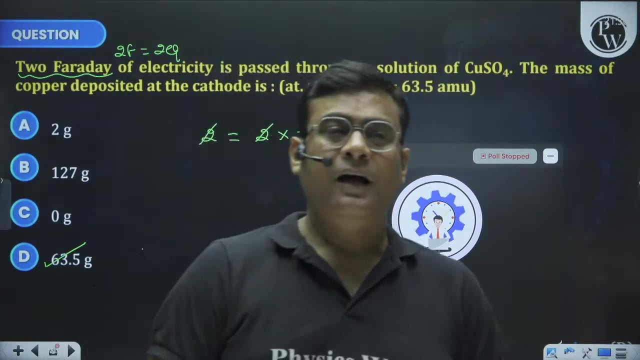 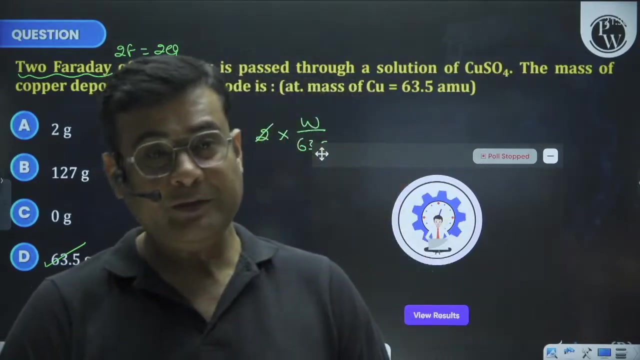 said: K춰 Jaisa maine socha tha haa tum bilkul waisee ho Jaisa maine socha tha haa tum bilkul waisee ho Jaisa maine socha tha. 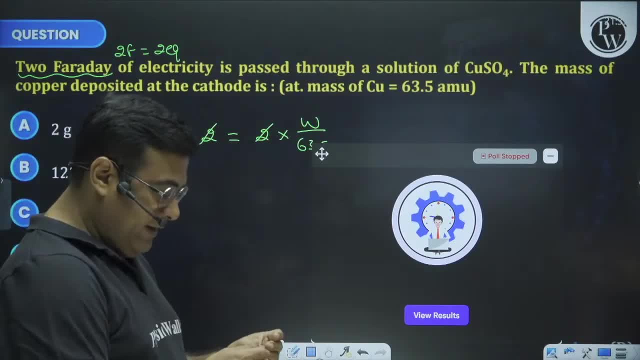 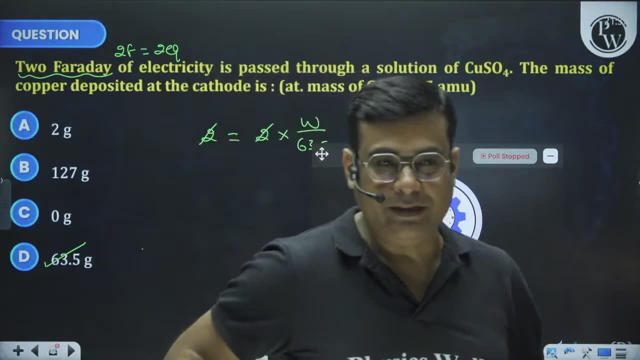 Theek hai, yeh bachcho toh yeh gaana mein apne IIT time se, jab se mein IIT Kharagpur mein hoon, tha, tab se mujhe suna. jab mein hai, toh mujhe khub pasand aata hai, aur mai. 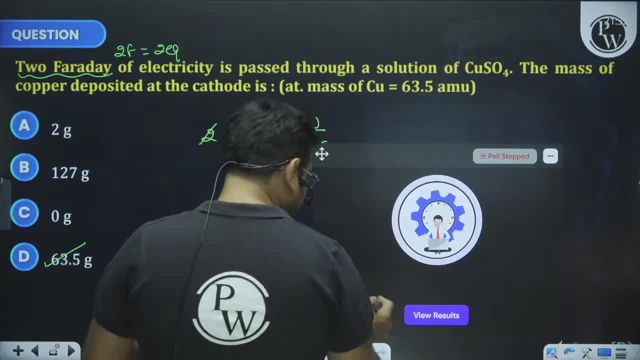 khub baar gunun aata bhi hoon theek hai na Mumbai aane ki toh okaat nahi itte toh paise hi nahi mere paas theek alo are. yeh toh record toh, yeh toh record tohde bhai. 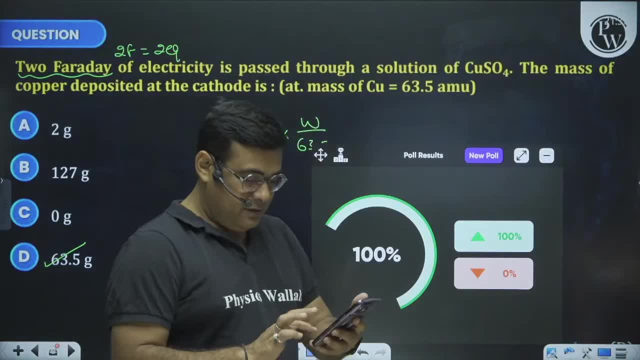 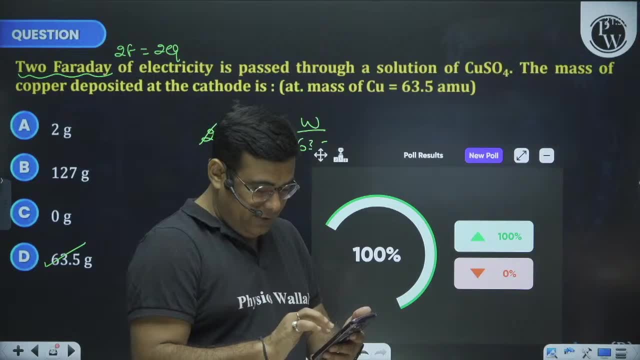 hai, na phale mai iPhone, apna dubhara dikha doon aapko jisko chidna hai wo chide. but it is a achievement. maine eh bol diya, sorry, galti se angreji thodi poor. it is an achievement. 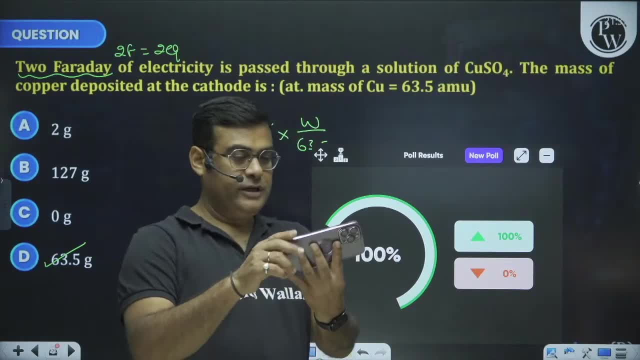 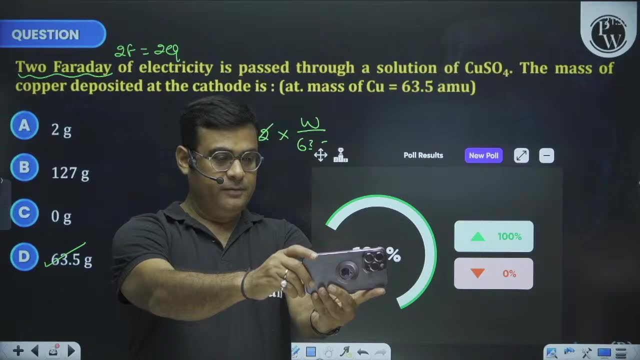 yaar, hundred percent par humne count humara pohucha hi diya. theek hai yeh hundred percent humara count, a chuka hai very, very nice yaar. thank you, thank you very much, thank you very much. theek hai urgency toh. 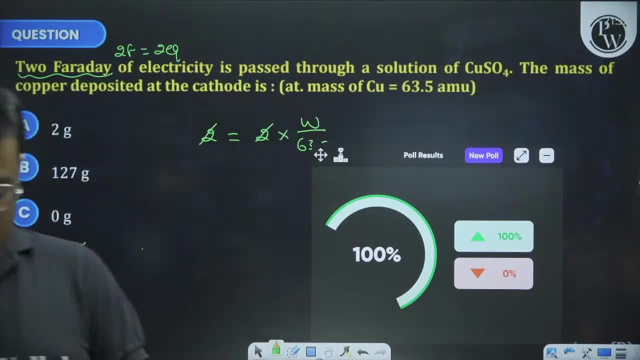 nahi hu, beta, itna maja mat lo, tum bhi merko lagra. tumhe main hi mila hu, aaj maja lene ke liye. haan, but haan theek hai, acha lagta hai, aur waise bhi, beta, dil se kari hui. 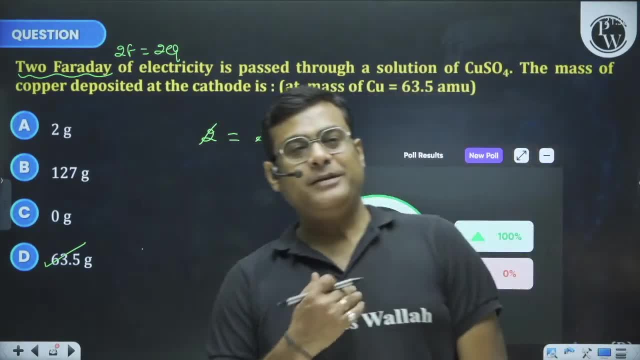 har cheez ne waise bhi achchi hi hoti hai hai na So kamsaham iss gaane ko toh ma kubh zyada dil se gaata hu. toh kisi ko acha laghe bura. 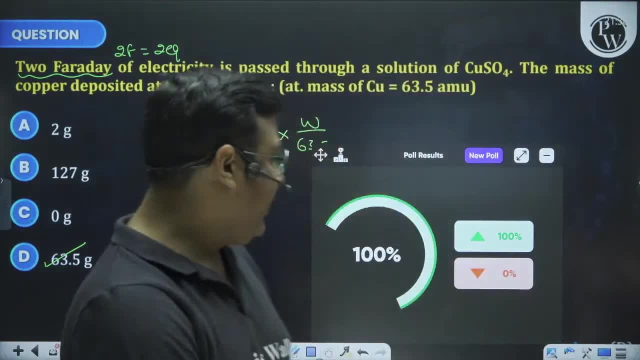 laghe ma utana sochta nahi hu theek hai ji chalo very good. thank you very much, bachchon. thank you very much ki hume itni chiji hai samajh mein aar rahi hai, bas meri. 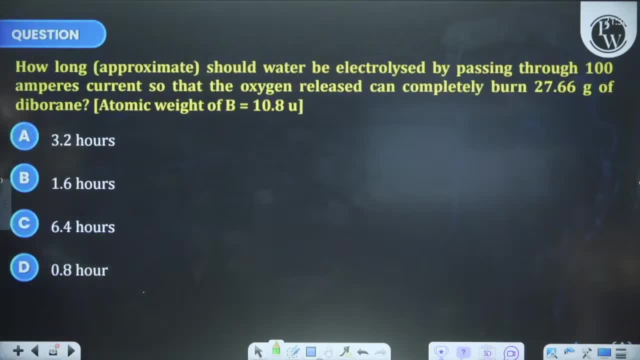 liye khushi ki baat yeh hai. chalo, dekho na ab agla question bata hu aapko. issme bhi ek maha, maha, maha bhayanak, mai aapko JSC bataane jaa raha hu na pehle toh question. 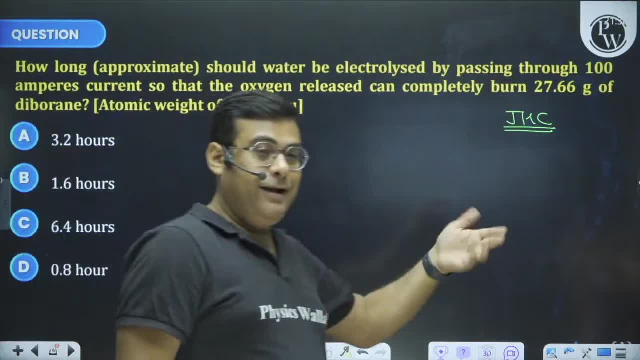 padh le beta, aapka toh mood fresh ho raha, meri aapka toh question. padh le beta, aapka toh mood fresh ho raha. meri aap gala betha jaa raha hai na gala matlab sardhi ki wajah. 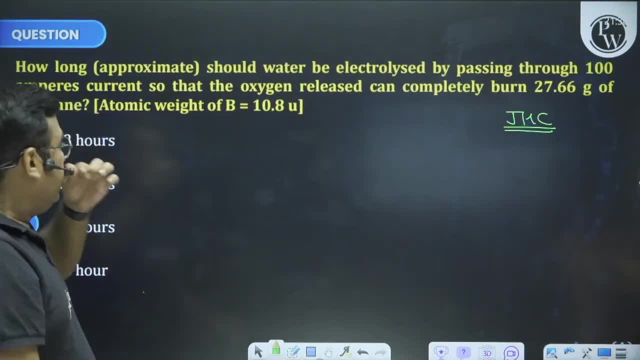 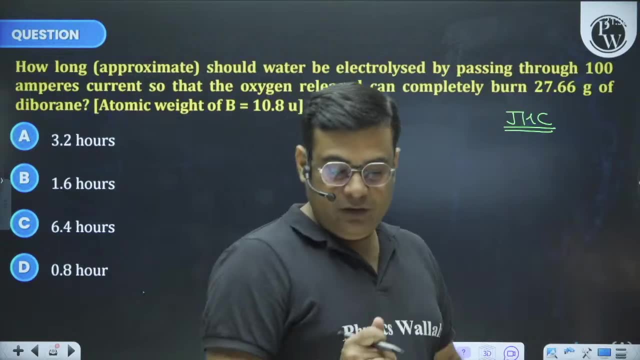 se jo naak mein dikkat ho jate na, woh parishan kar deta hai hai na aur garmi mein sardhi lag jaye toh, phir toh aur matlab ajeeb, saa matlab sharid, hi hi hai na duration beta. 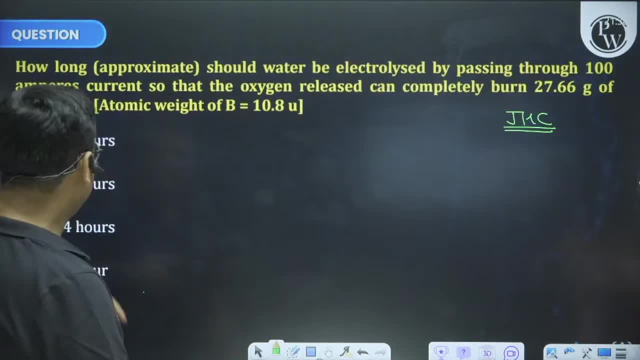 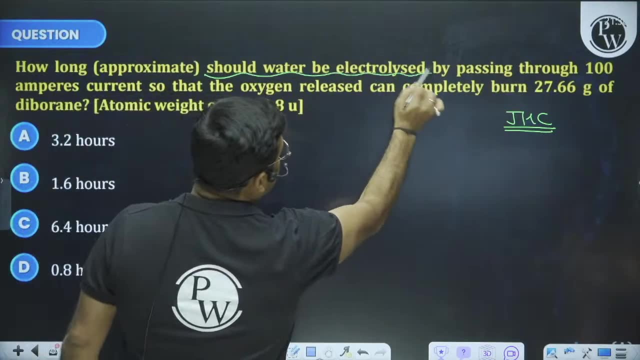 abhi ek ghanta sawa ghanta, toh laghi jayega cholo, cholo question. sabke dekh le: how long approximate should water be electrolyzed? bhaiya, water ka electrolysis pata nahi, kyo mujhe. 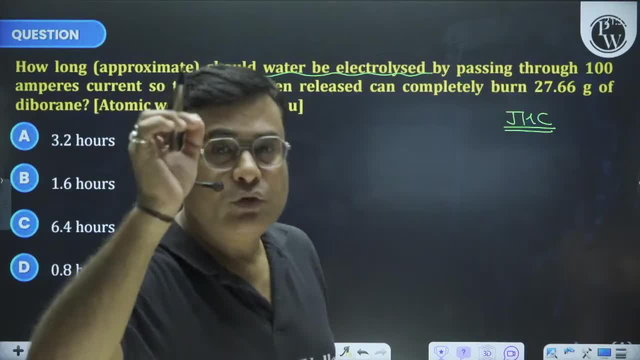 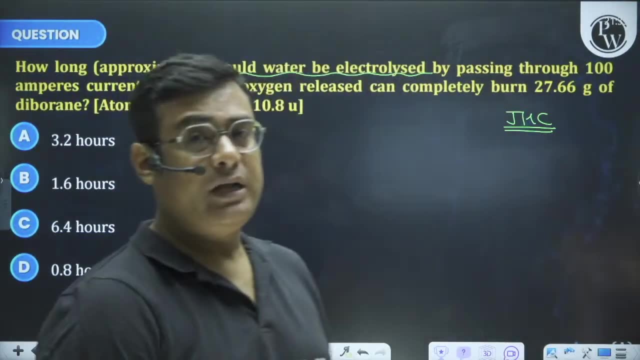 lagta hai, kubh important thing is: how long should water be electrolyzed? bhaiya, how long should water be electrolyzed? kubh important hai question aayega, hi aayega. aur uske jo shortcut mere paas hai. aaj tak aapne dekhe nahi hongi kubh shandar wale hai hai na by. 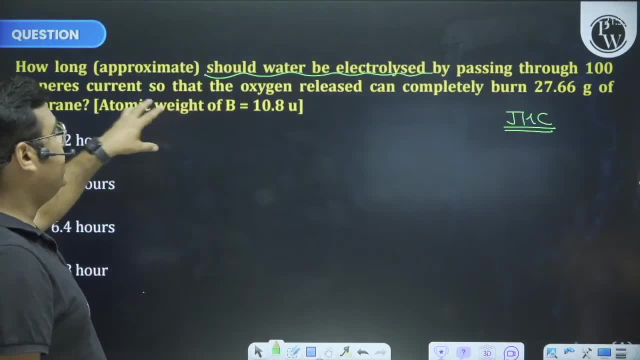 passing through 100 ampere current, so that oxygen release can completely burn. 27.66 gram of diborane aaj kal jai wale ki chalaki chal rahi bata hai, na do reactions ko mix bhi. 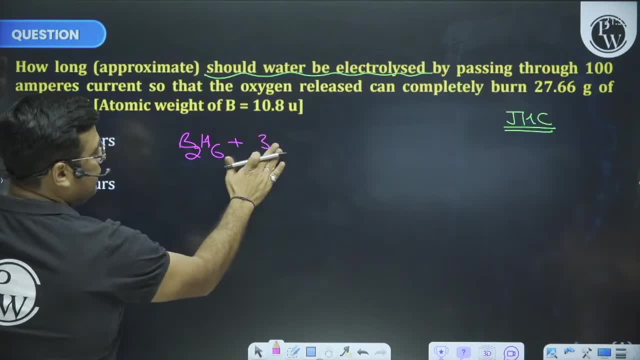 kar dena. kabhi, kabhi toh B2S6 ka combustion hum agar karate hai hai na inorganic mein combustion reaction hai na kubh important hai question aayega, hi aayega, aur uske jo shortcut. 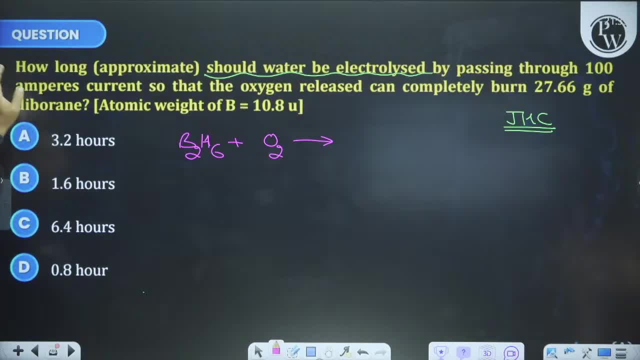 mere paas hai. kabhi kabhi toh B2S6 ka combustion hum agar karate hai hai na bhi kabhi. kabhi sya reaction hai, kabhi favorite reaction hai, jab bhi aap combustion karate. 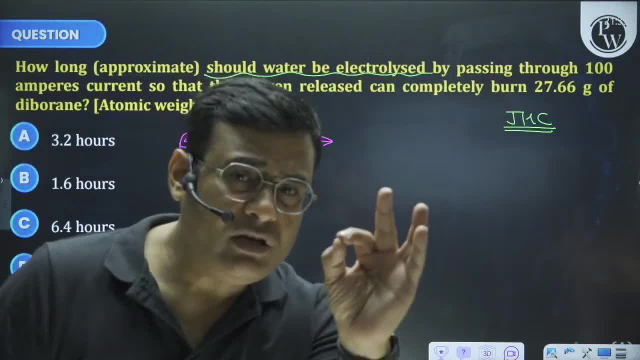 hai bhyta, toh jise combustion of hydrocarbon kena aayega hain combustion ka general rule, mujhe samajh lena hai. kya hai general rule combustion ka hai? na ha, maine wada kiya. 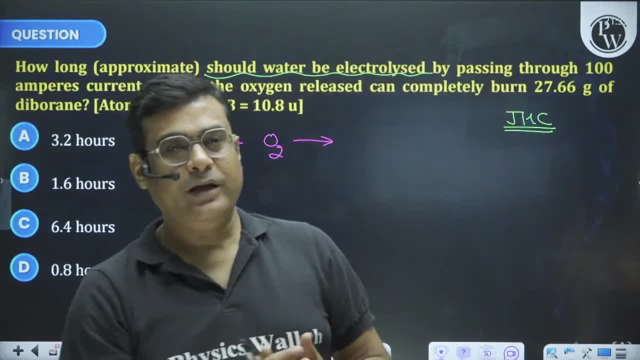 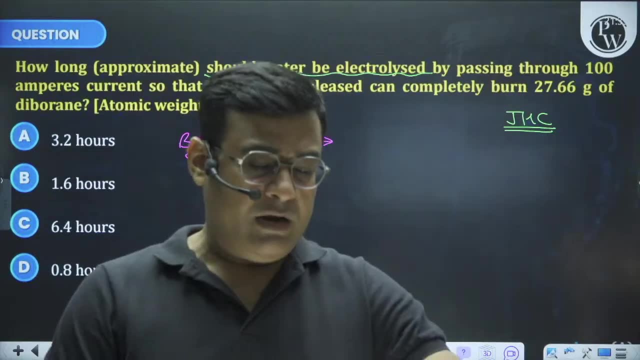 tha iphone ka bhyta theeka na toh aap abh dukul wada poora karenge. aap select hohi aachi rank se theeka na toh hydrocarbon mein carbon aur hydrogen they bhyta carbon ne bhi. 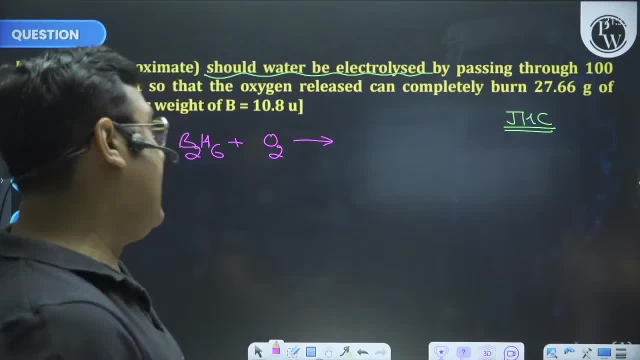 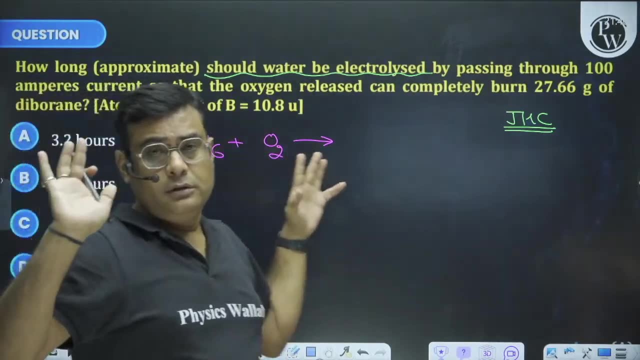 apna oxide bhanaya hydrogen, ne bhi apna oxide bhanaya yaha. par bhi wahi kahaan ni bhyta When you will do combustion of anyone except Nitrogen, Gold and Platinum. Nitrogen is inert. Nitrogen reacts with Oxygen. 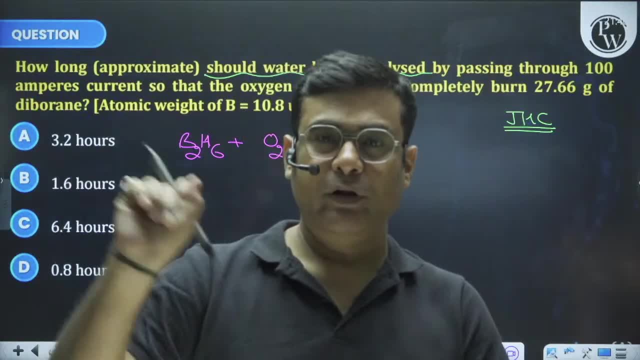 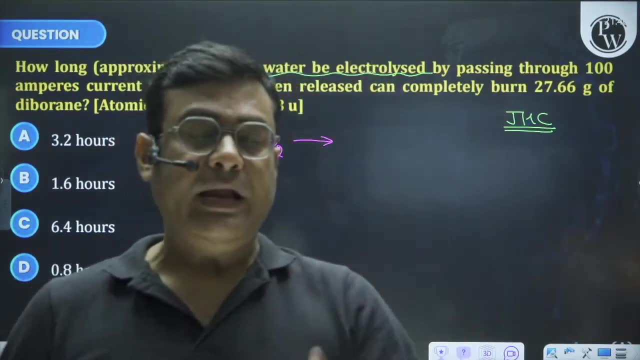 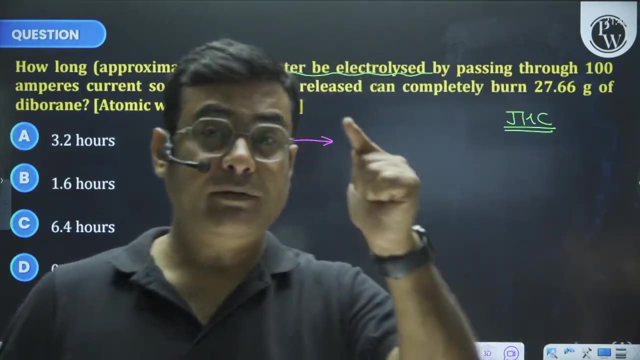 What happened. There is a cut in the thumb. there is a slight bleeding. you will not be able to see it. that is why my attention is going on it. So what I am saying to you is that Nitrogen reacts with Oxygen, but only at very, very high temperature, and in today's session we have done 2000 Kelvin. 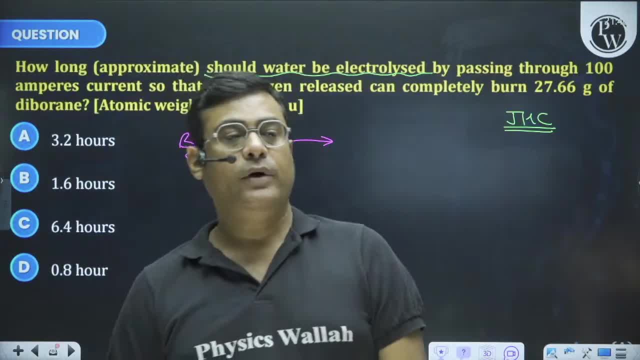 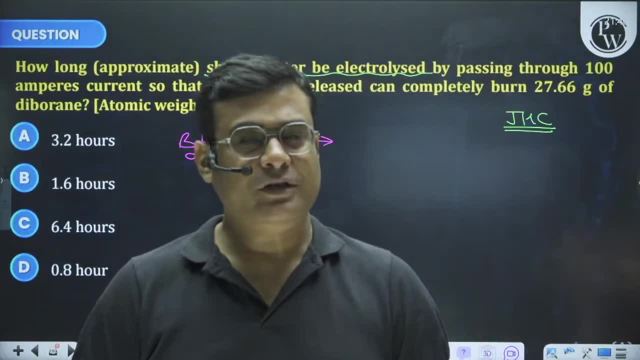 This thing is clearly written in the NCERT book. this thing is clearly written in the NCERT book. Are you understanding everything? I am from Kharagpur. Jamshedpur was not far from Kharagpur. Right Right, Jamshedpur was not far from Kharagpur. 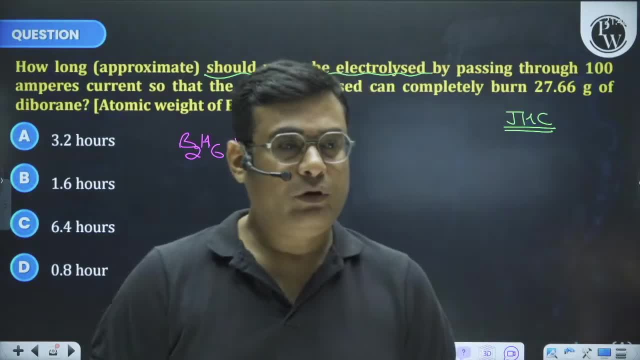 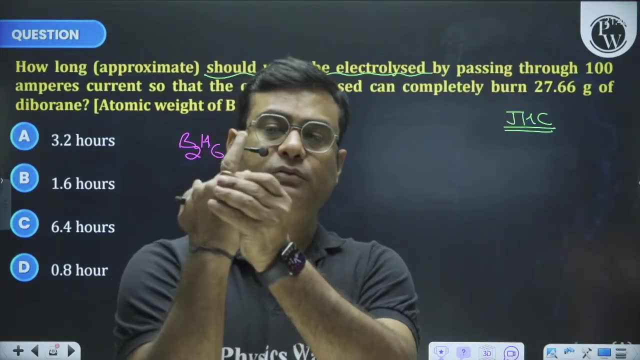 And what I am saying to you is the second thing. What I was saying. I forgot Right And Gold and Platinum. children, Gold and Platinum, like a small ring. I don't even have pure gold. I don't know how many years I have worn it. 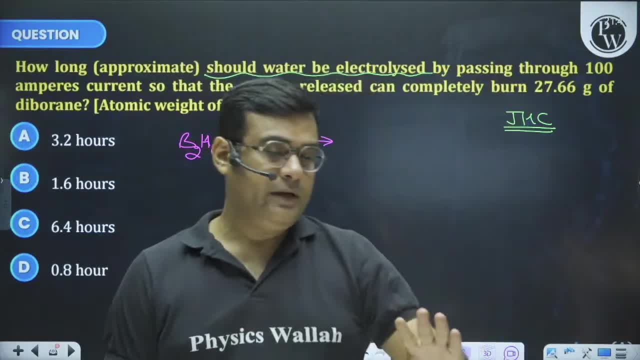 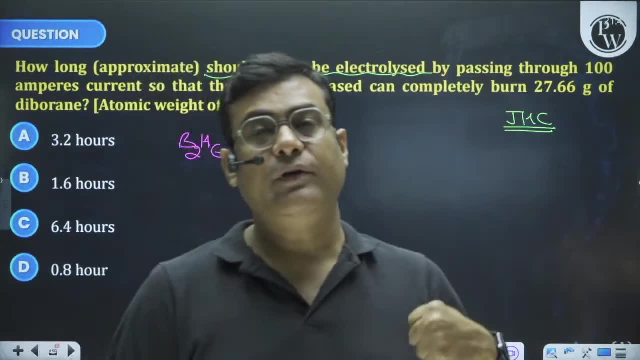 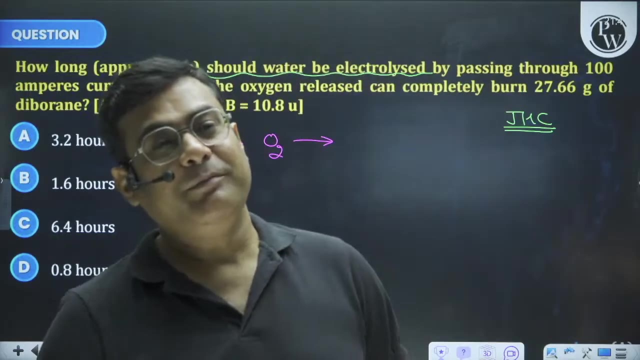 Gold and Platinum are two such metals whose length is not possible to apply Oxygen. You must be knowing. they can dissolve only and only in Aquaresia. They dissolve only in Aquaresia. You must be knowing. you will definitely know Right. That is why the jewellery is made of Gold and Platinum. 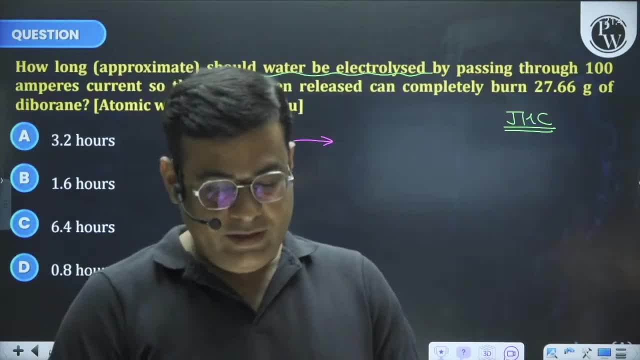 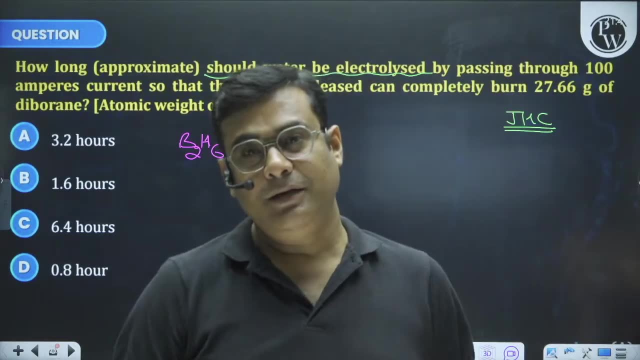 Otherwise, brother, If jewellery is made of Gold and Platinum but it spoils quickly, And if you make it of any other element, then there is no point. Every month the family will trouble you. It is wrong to say family. 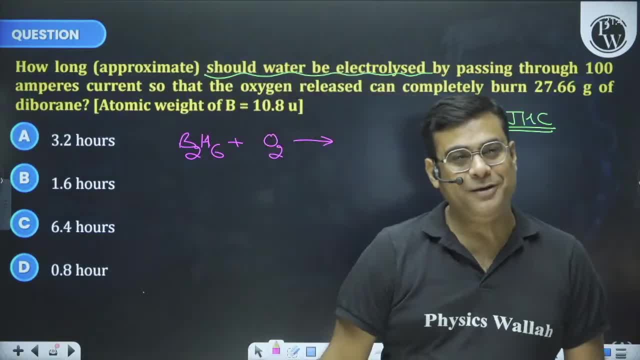 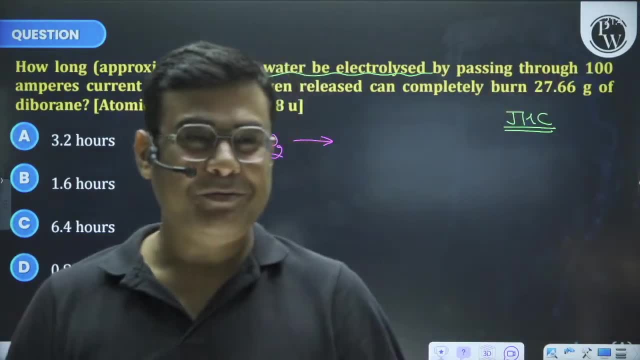 Actually the family should say: it will trouble you. My jewellery is spoilt, change it. And you are also going to come to this pari soon. You also know children, Right, You also know. So because of this the story gets a little messed up. 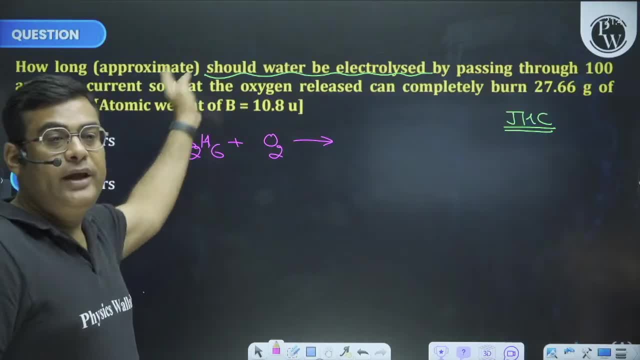 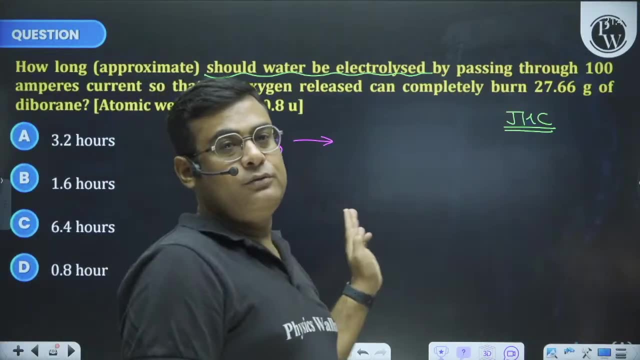 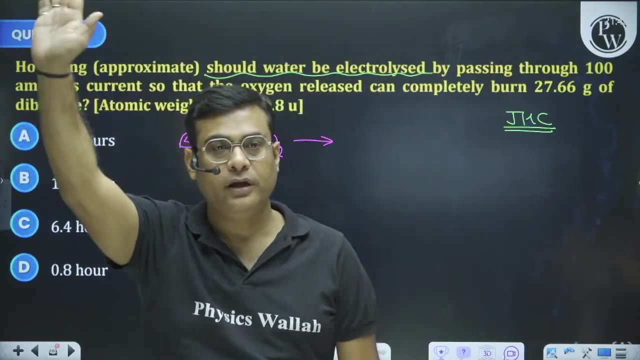 Otherwise children, Oxygen, which will be the element, changes them directly into their Oxides In ITKGB. sir, were you also a Hindi medium student? The first Hindi medium student son is standing in front of you. I am a pure Hindi medium student till 12th. 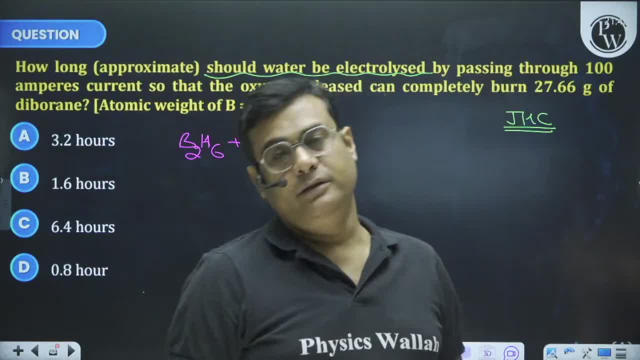 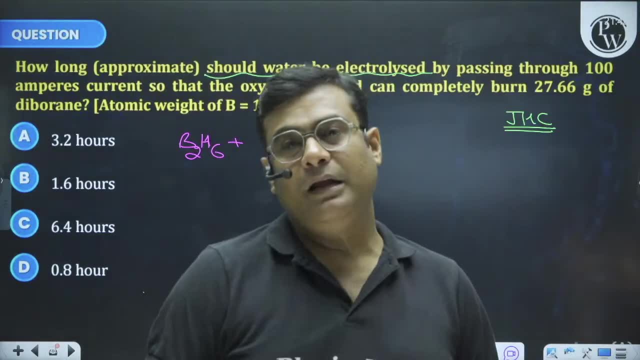 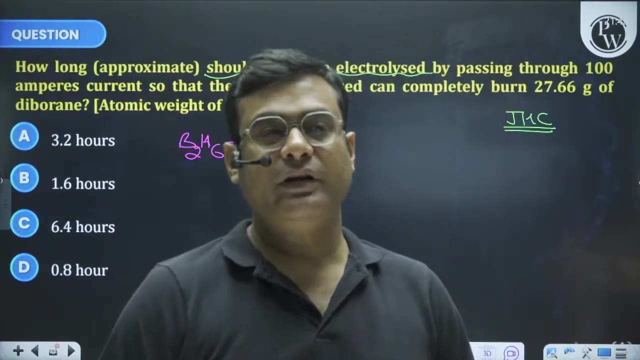 Right, But I was not crying and washing like you, Right? Because the world is not going to listen to your crying and washing son, Right, The world is not going to listen to your crying and washing, Right. She will see what you have achieved by seeing your hard work. 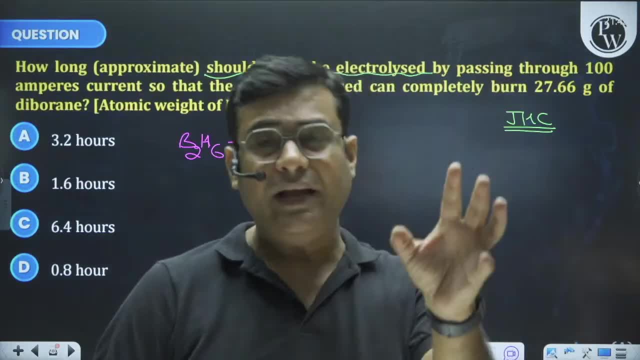 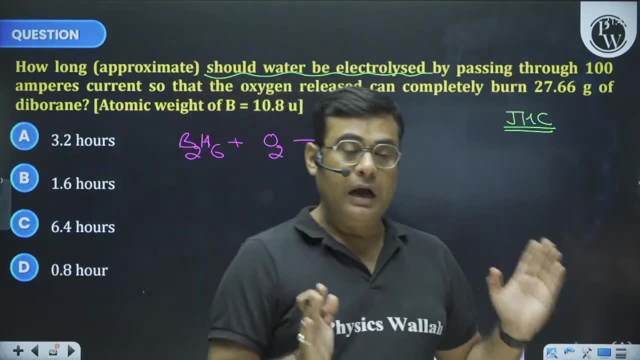 Right. You may have also seen the 12th film, One of the most inspiring movie, Right, Which I have seen. What a lovely movie it is, So you must have seen it too, son. That too was a Hindi medium. 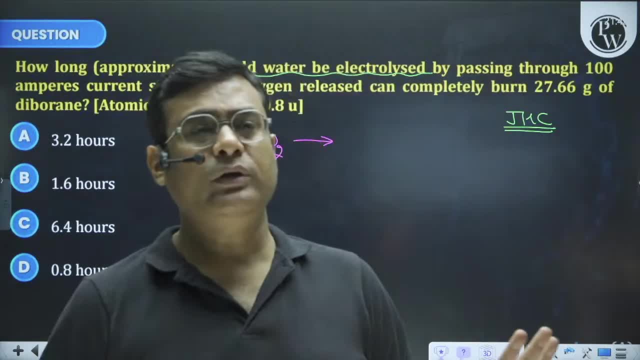 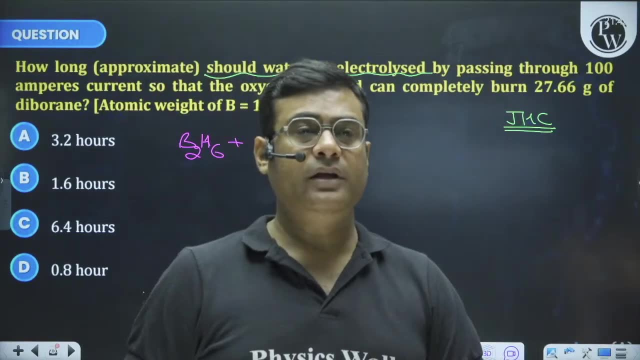 From where did it grow? It is not going to work by just speaking, crying and washing, son, The selection is of those who have courage. son, They are now of Hindi medium. They are rich, They are poor, They have nothing to do with it. 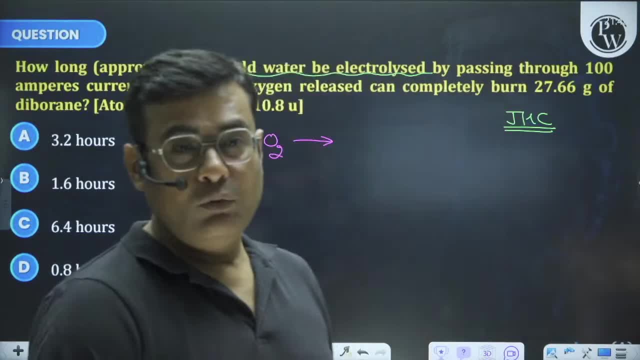 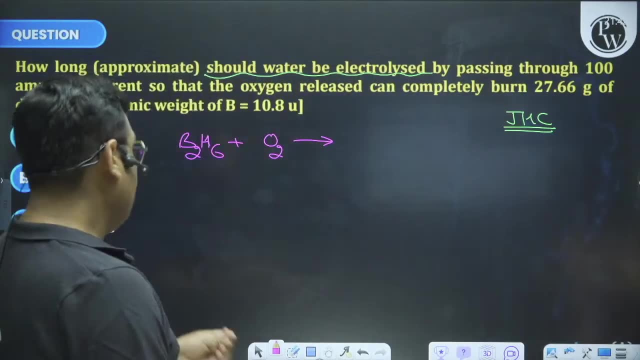 Courage From here, son. Courage should be there. Courage, Their selection is there. The spirit of hard work should be there. Courage should be there. The selection is theirs Right, Come on. So I am saying, son, There is boron. 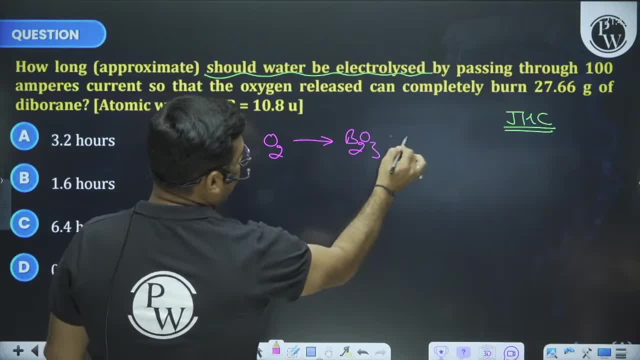 So boron oxygen By burning it in its oxide. Now we all know the boron oxide. children, There is B2O3.. Right, Right, Son, the 12th film is a real story. You do not know. 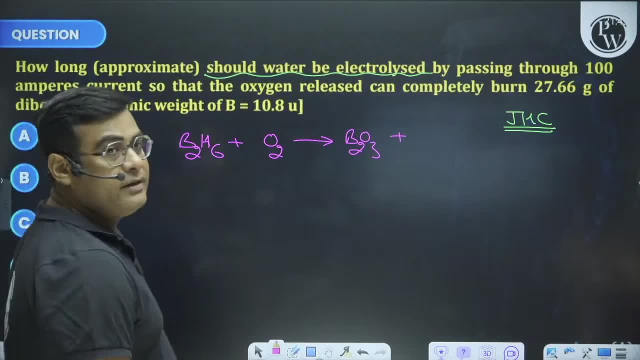 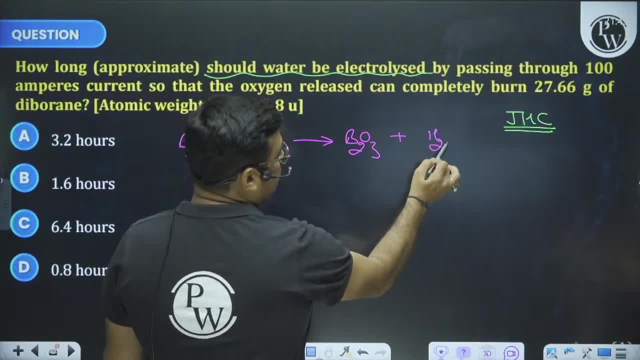 It is a real story. There is hydrogen. Hydrogen will make its oxide H2O Right. There is 6 hydrogen, So make it 3.. Boron was 2, only Made it 2. Now balance the oxygen. 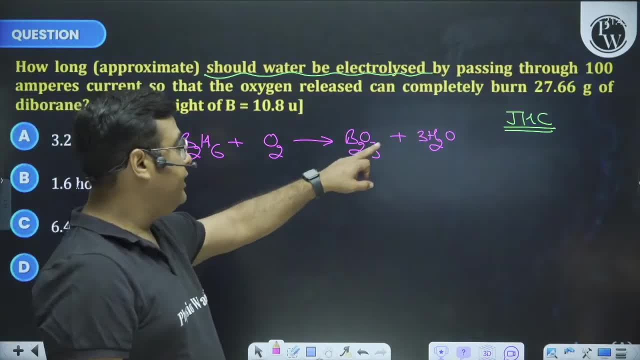 3 here, 3 here, 6.. That means: how much O2 will it take? children 3 O2.. Right, How much O2 will it take? children 3 O2.. Right Now, this is balanced. 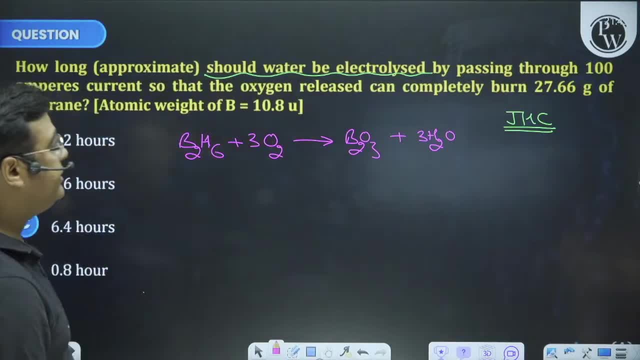 So what condition have we been given? That we have to do electrolysis of water till then with 100 ampere current. So that we have to do electrolysis of water till then with 100 ampere current. So that we have to do electrolysis of water till then with 100 ampere current. 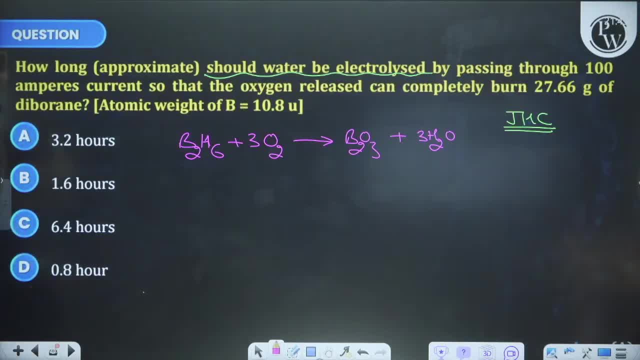 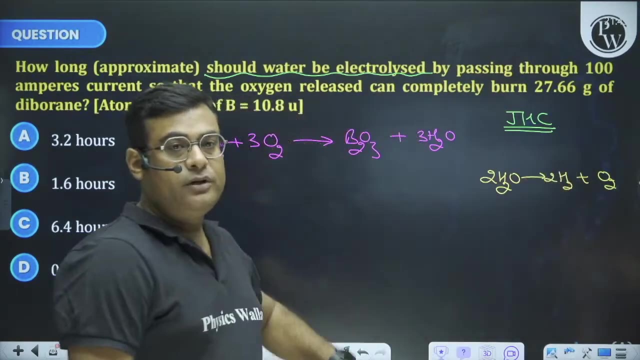 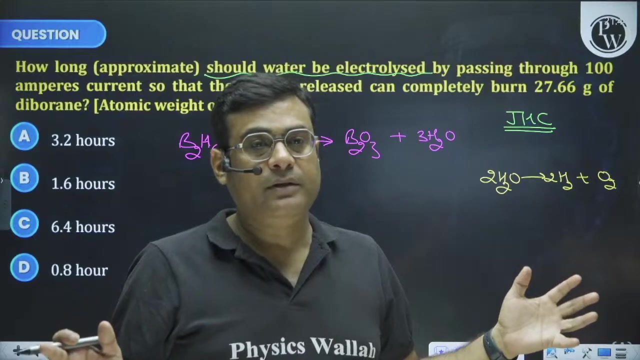 Now I should know this, children: Whenever water is electrolyzed, I was going to tell the short-cut of the water and I have adjusted the question according to all my short-cuts and put a lot of effort so that I can tell you everything. 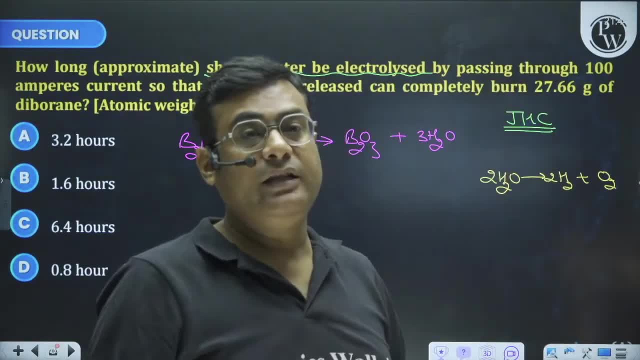 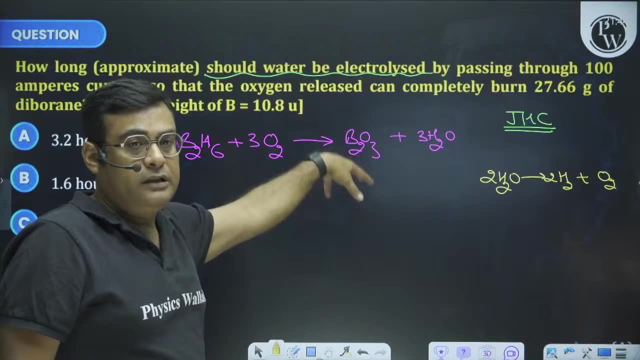 I have told so much about jsh time. Right, how many questions have come at this time? now the electrolysis of water is there. I would have written it in the beginning. till then you would have forgotten. so I will tell you this along with the question. 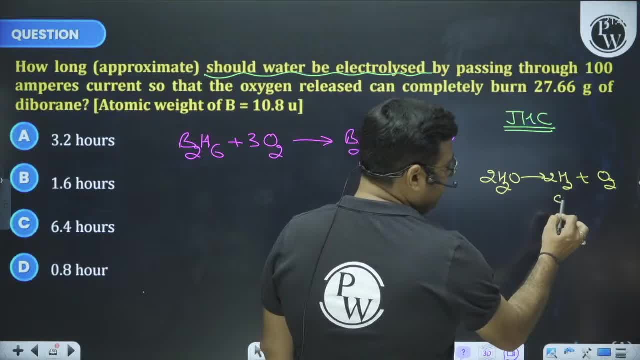 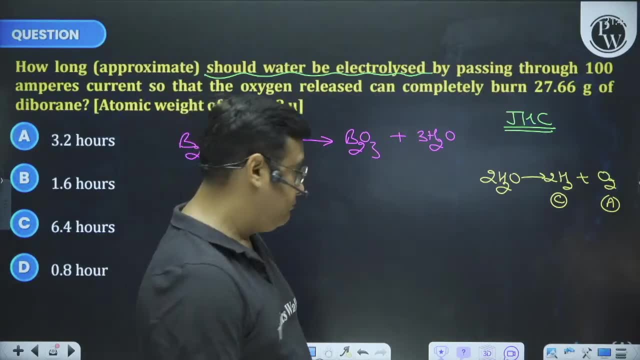 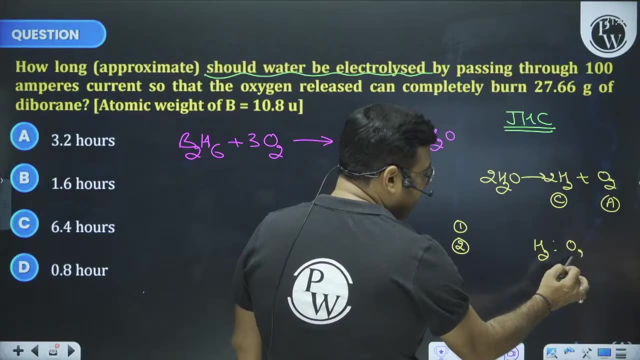 so the first thing I should remember from the electrolysis of water is that hydrogen gas is made on the cathode, oxygen gas is made on the anode. this is the first information you have to have remember. second information is that if you ask the equivalence ratio of hydrogen and oxygen, then the equivalence ratio is always 1 is to 1,. 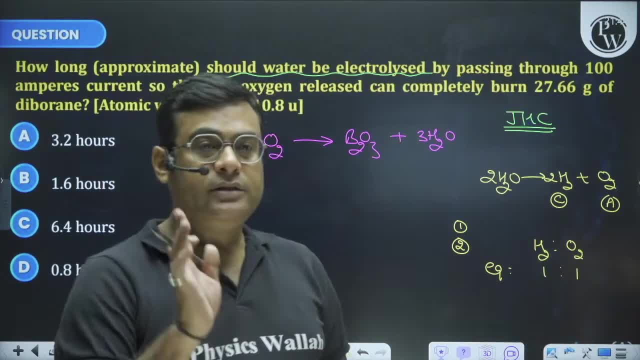 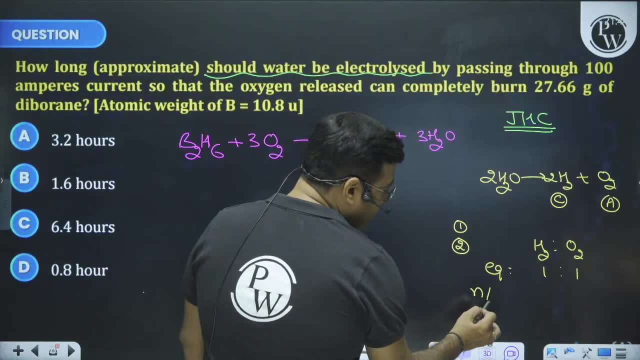 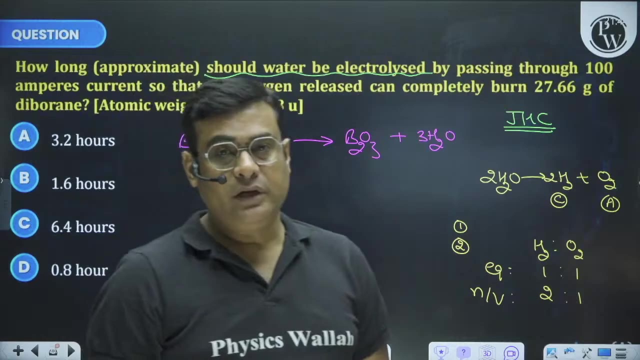 so the same charge is going on the cathode and anode. if the charge is same, then the equivalence will also be the same. now I have told you again and again. but if he tells you the ratio of moles or volume, then the coefficient is visible. hydrogen has 2 moles, oxygen has 1 mole. so the ratio is 2 is to 1,. 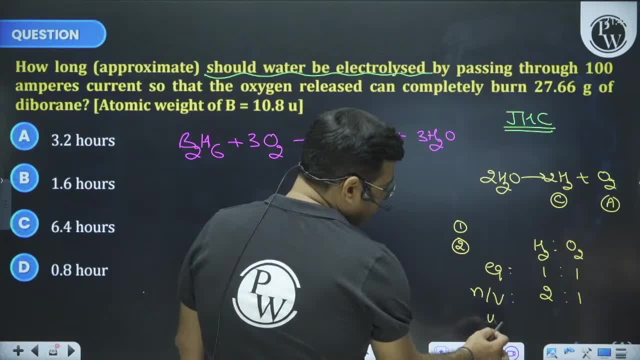 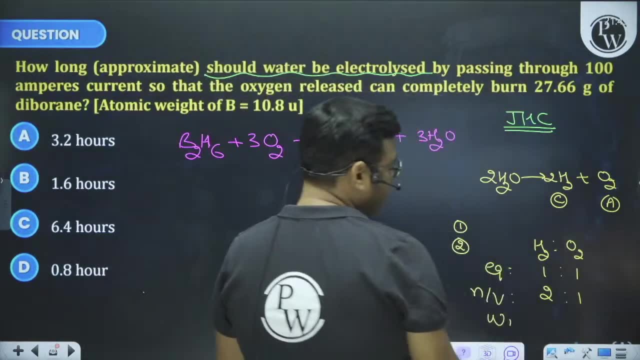 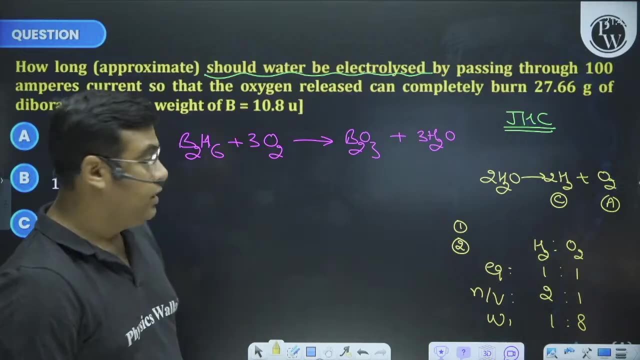 but if he tells you the ratio of mass, 2 moles of hydrogen means 4 grams and 1 mole of oxygen means 32 grams. so 4 is to 32, means 1 is to 8 grams. this is the second JSC for electrolysis of water and the third and most famous JSC which will be used in numerical questions. 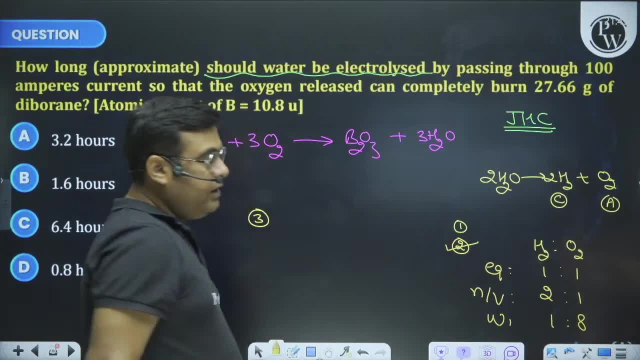 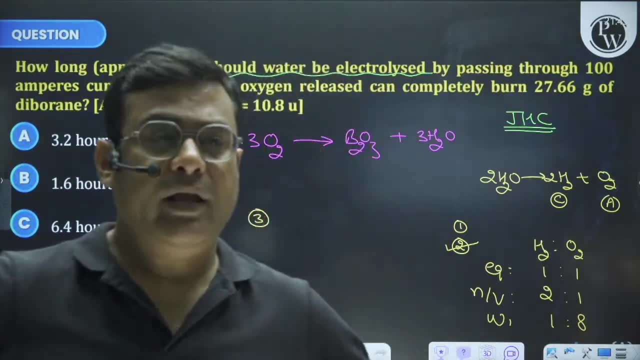 second is also used in any question. I will give you that if the electrolysis of hydrogen is given to you from the electrolysis of water, then tell me. if 2.5 grams of hydrogen are made, then tell me how many grams of oxygen will be made. 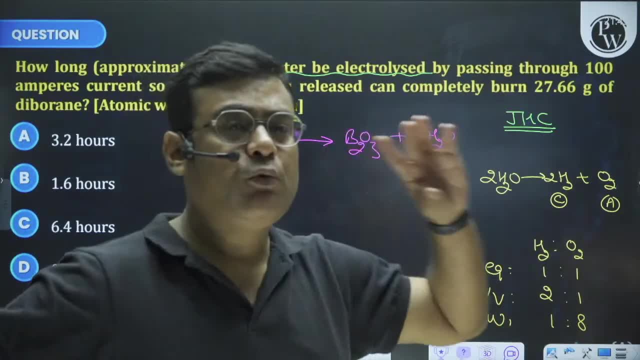 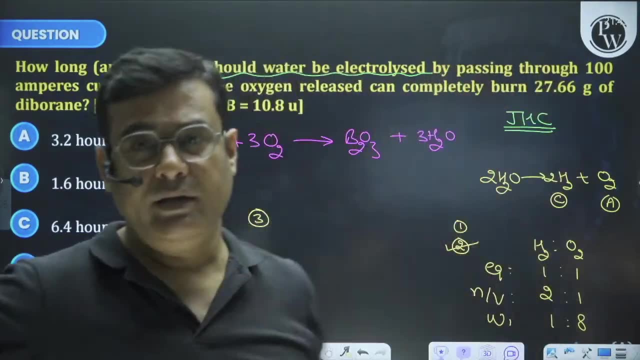 so if you remember this thing, my information, you don't have to do anything in that question. just increase it by 8 times. 8 times of 2.5, 20 grams. the story is over. you are understanding my things definitely clap because here is the third shortcut. 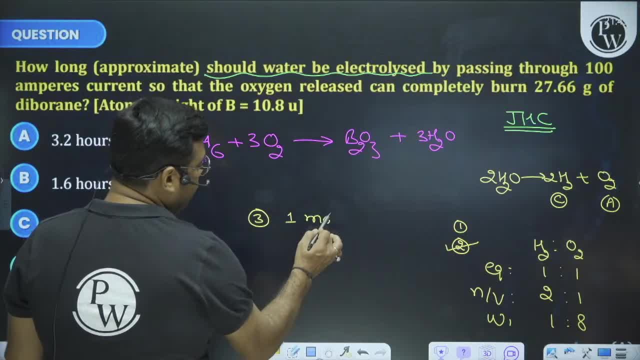 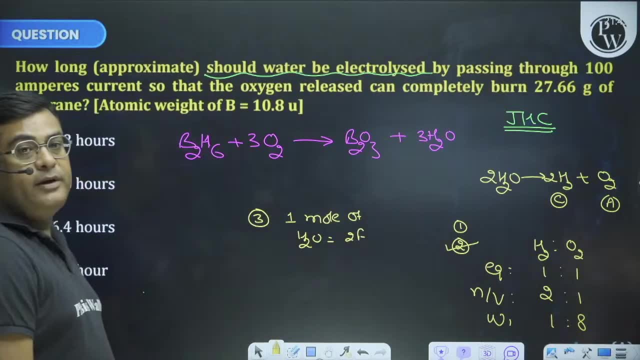 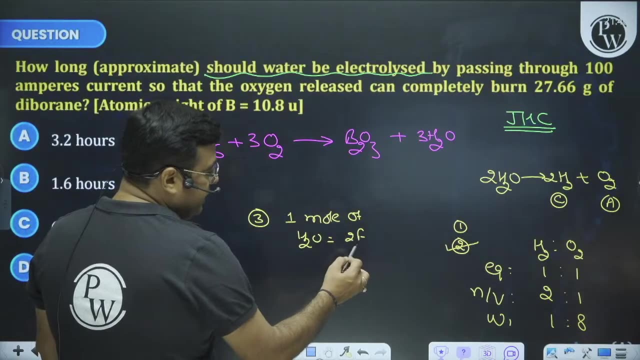 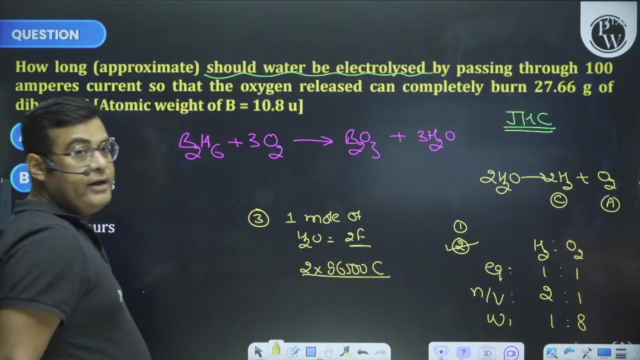 the third shortcut is to electrolyze 1 mole of water. 1 mole of water to be electrolyzed, 2 Faraday charge is required. 2 Faraday charge is required for 1 mole of water to be electrolyzed. and what does 2 Faraday charge mean, children? 2 into 965: 00 open, which you can write anything in the form of IT later. 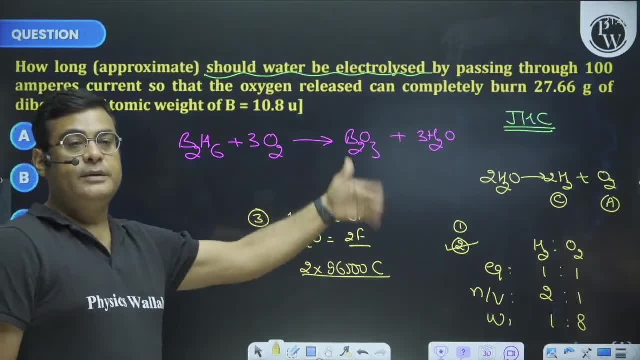 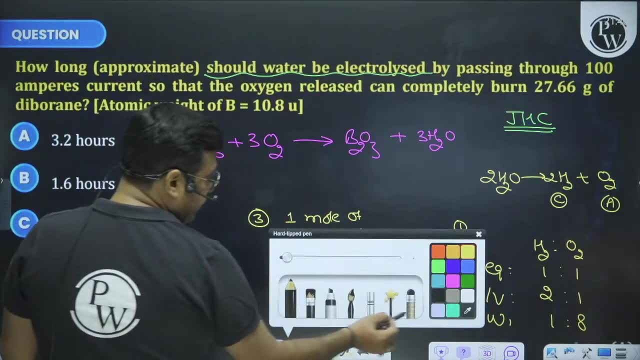 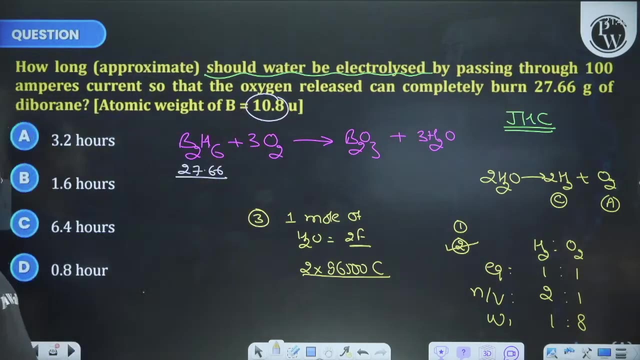 for 1 mole. according to how many moles there will be, I have to keep changing it proportionally. so now see what is happening in this question: 27.66, B2 S6 is divided by 2, boron double of 10.8 is 21.6,. 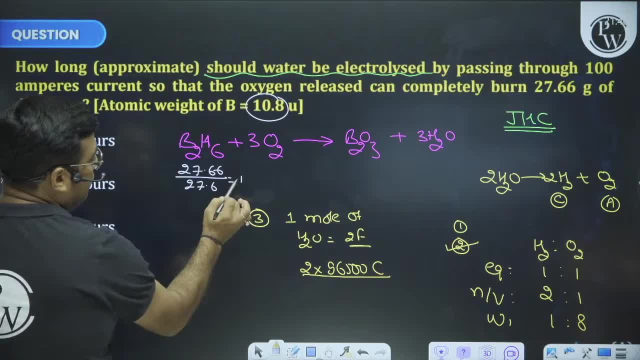 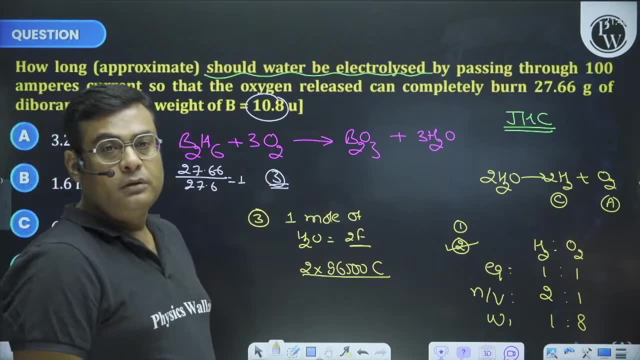 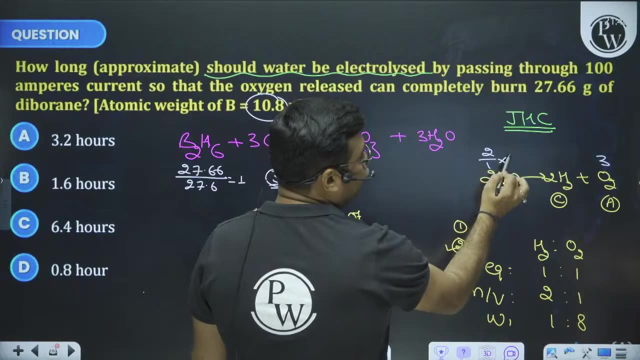 6. hydrogen is 27.6, means 1 mole. 1 mole of this is 3 moles of oxygen. 1 mole of this is 3 moles of oxygen. okay, and 3 moles of oxygen. then I have already told you the concept of mole. how many moles of water? 2 by 1 into 3 is 6 moles. 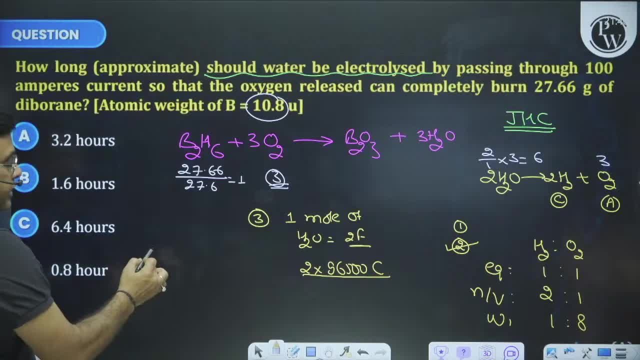 and if 6 moles of water then 4 moles of hydrogen, then how much is the charge, sir? 12 Faraday, because 2 Faraday for 1 mole, now there are 2 Faraday. if there are 12 Faraday, then 12 into 965, 00,. 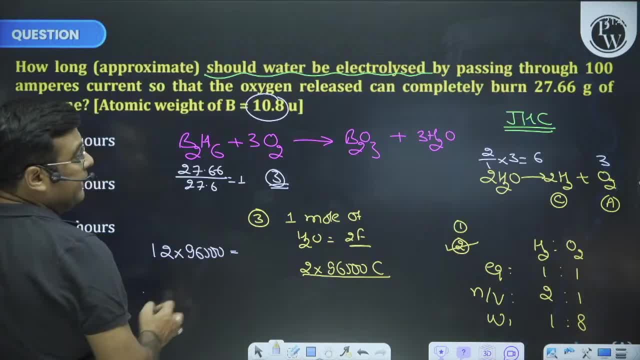 for Kulam and whose Q is equal to children ITK. how much is I, sir? 100 into T. this is from 2 zeros to 2 zeros. this is the answer, but it is in seconds in which he asked in hours. so, brother, 1 hour. 1 hour equal to 3600 seconds. 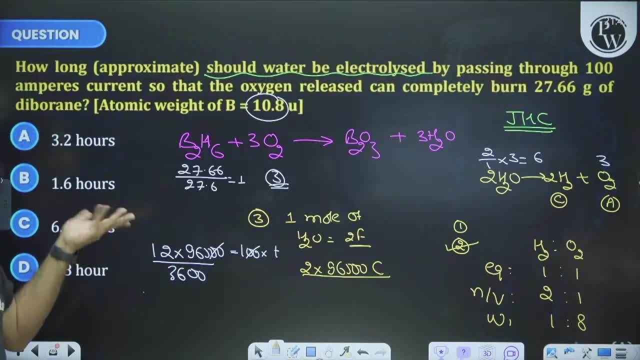 divide it by that. according to me, your answer has come now. if you think in this children that normally our bad habit that we always write the reaction in the question of electrolytic cell, then try to remove the infector, etc. in that your story will be a mess. 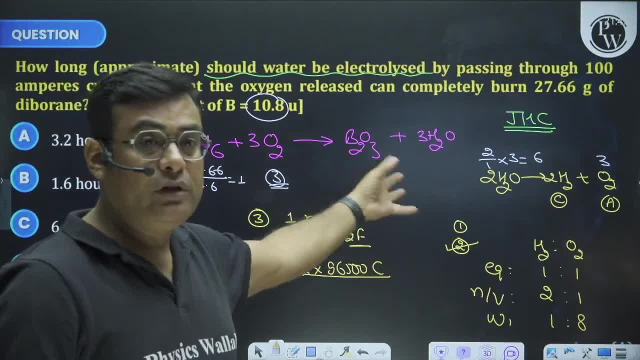 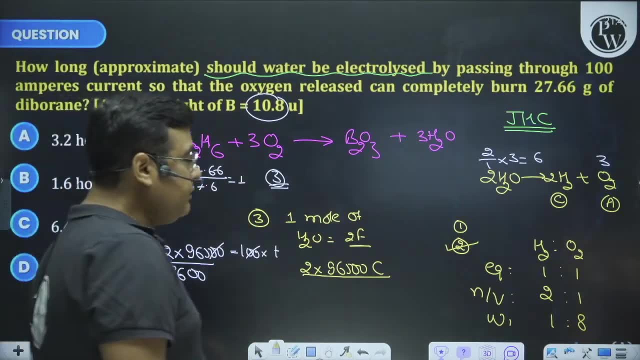 right, because in the electrolysis of water if you know these 3 shortcuts then your question will be oral, quietly, right. first of all I am telling JSC again, the electrolysis of water. I hope everyone will know this reaction of water children. 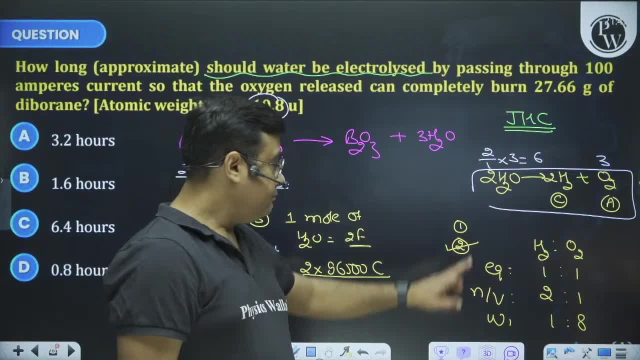 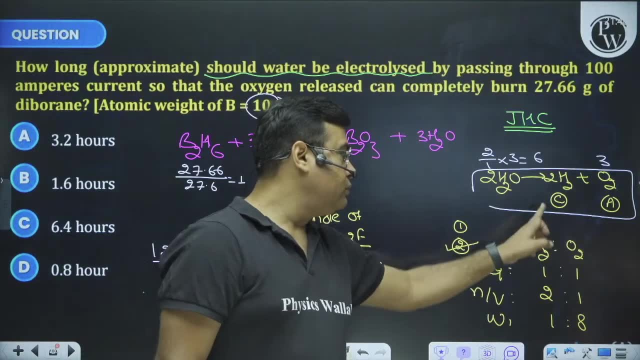 from that, only all JSC is being made. 2H2O gives 2H2 plus your O2, right, hydrogen and oxygen is always 2 is 2, that is, hydrogen in the cathode and oxygen in the anode is made. 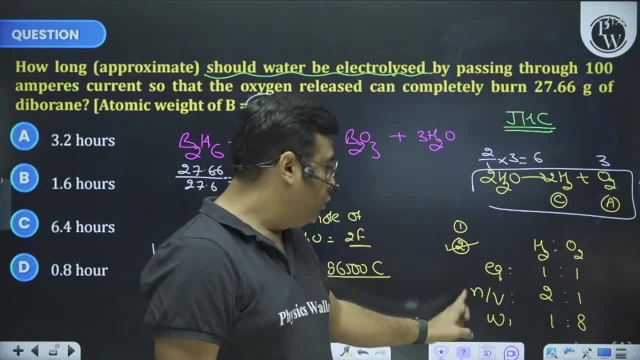 if you talk about the ratio, the ratio of the equivalents is 1 is to 1,. the ratio of the volume from the mole is 2 is to 1, right. the ratio of the mass is 2 moles, which means 4 grams. 1 mole means 32 grams. 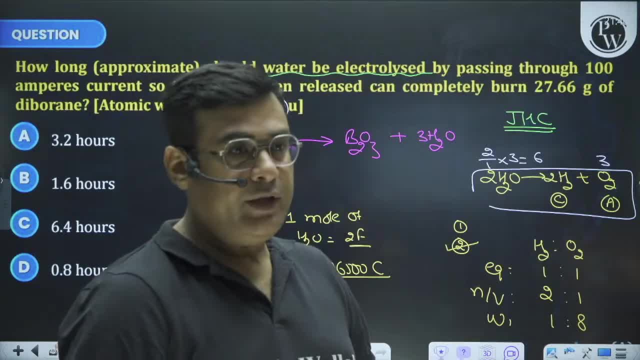 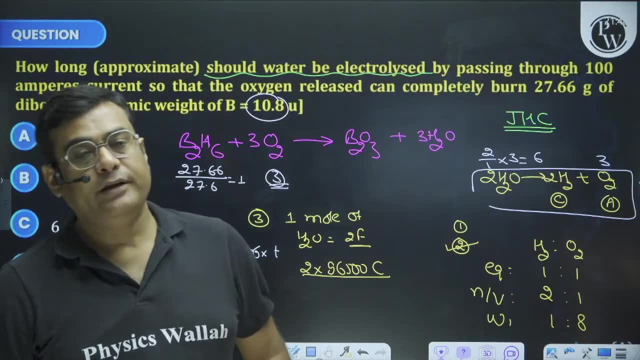 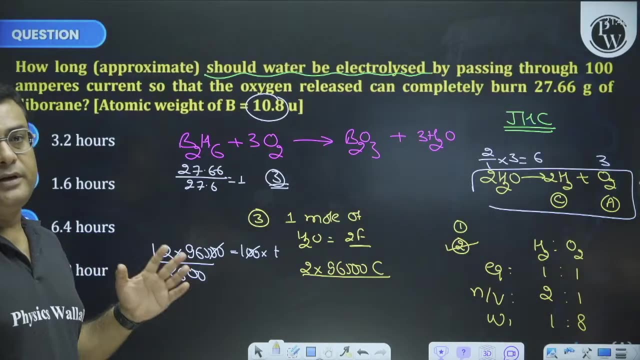 4 is to 32 means 1 is to 8, right apart from this, children last to electrolyze 1 mole of water, you always have a requirement of 2 Faraday charge. but remember this. much from that, I have immediately solved your question immediately. 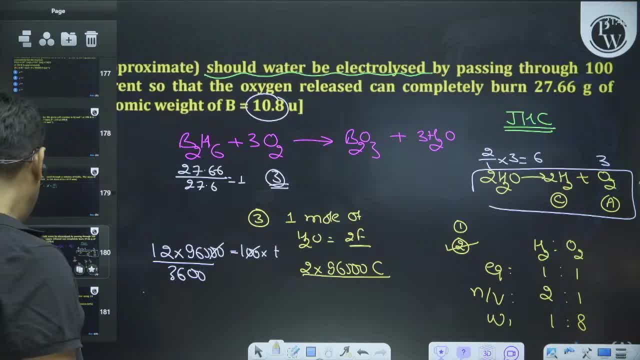 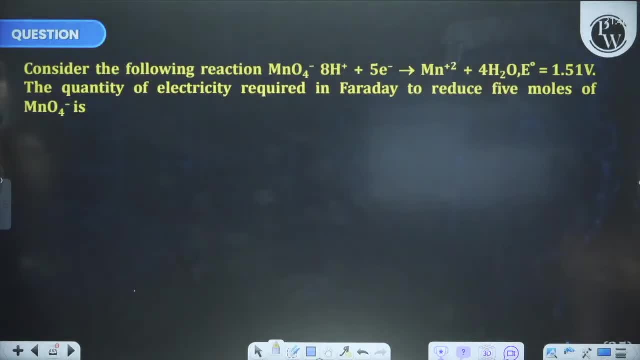 right, my dear children. now let's see if there is any other question, so let's see that too. now this question is: consider the following reaction: MnO4 minus 8H plus 5 electrons. this reaction is so important, children, right? 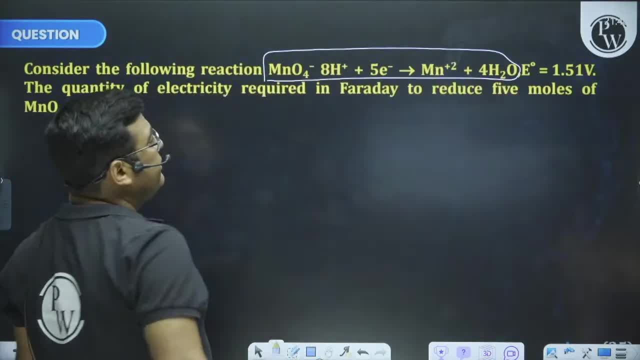 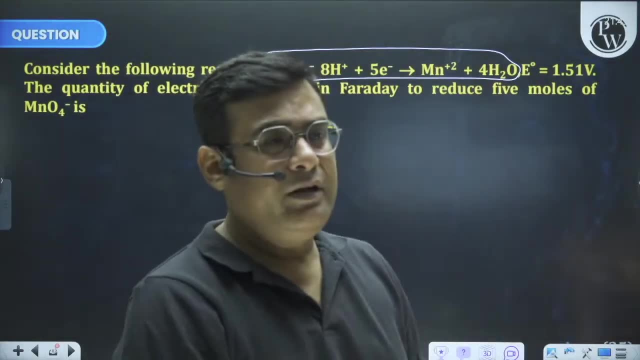 you study in D block, you study in redox, you study in electrochemistry, you study in salt brother. the reaction should go to the rut. the acidity of KMnO4 is n factor 5 in the medium E naught. is this much now? is E naught needed or not? look ahead. 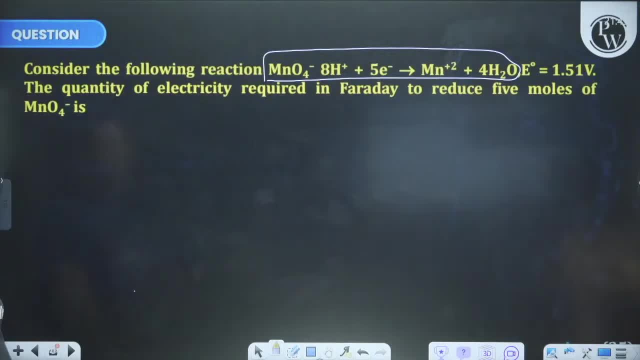 quantity of electricity required in Faraday to reduce 5 moles of NO4 minus right now, talking about the quantity of electricity, children, this means there is no E naught here, right, you don't have to give E naught here. 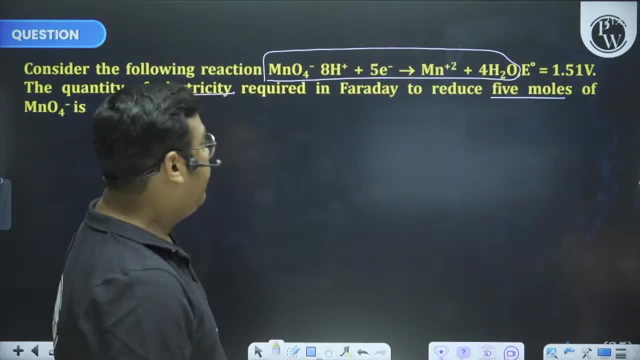 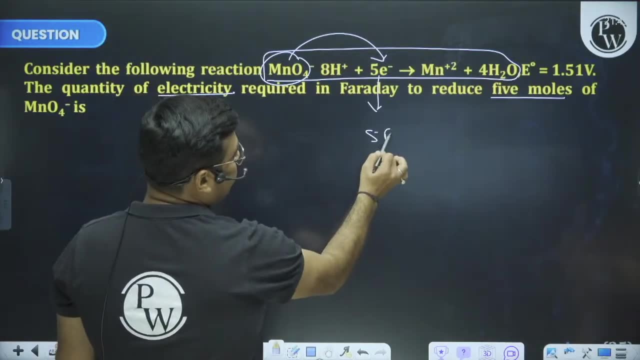 to reduce 5 moles of whose MnO4 minus how many electrons for 1 mole child: 5 moles of electrons. 5 moles of electrons means 5 Faraday. 5 moles of electrons means 5 Faraday. 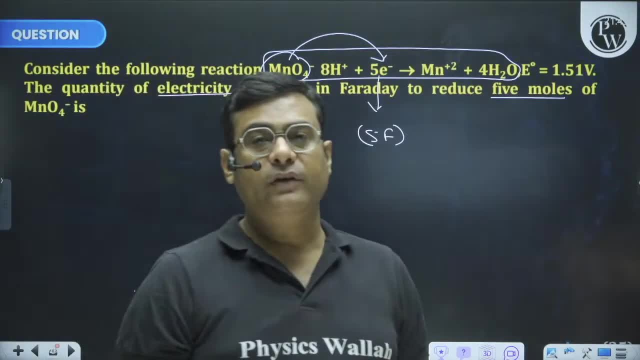 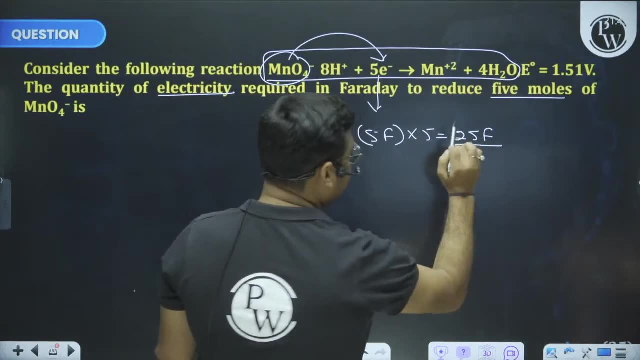 because charge on 1 mole of electrons is called 1 Faraday. so there are 5 moles. so 5 Faraday into 5 means your answer is 25 Faraday. 5 Faraday for 1 mole, 25 Faraday for 5 moles. 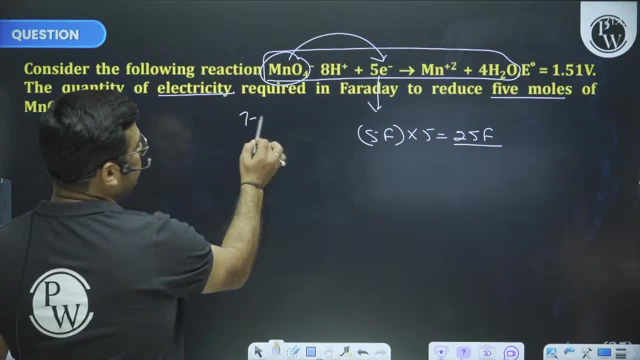 now this question, at least in this way. similar questions have come in 7 to 8 times in JEE. similar questions like this- children- have come in 7 to 8 times in JEE. you can do nothing about them. 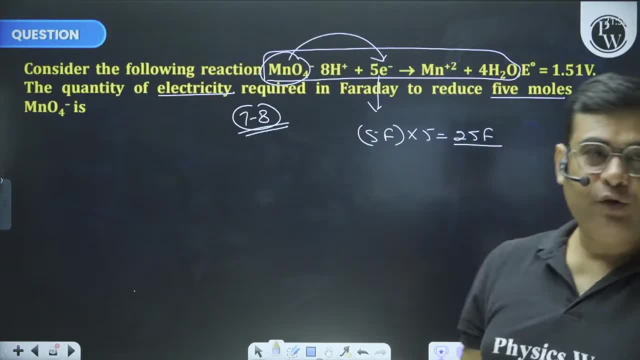 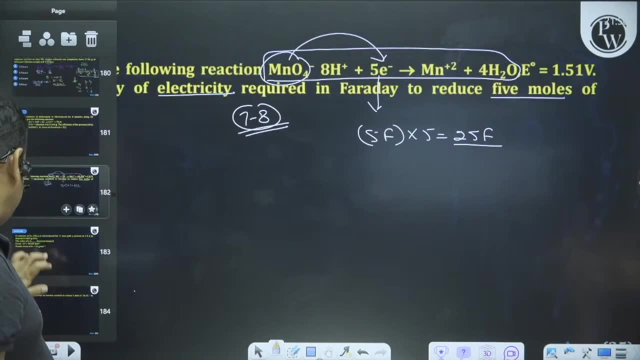 you just have to do this much. you have to solve the question and give the answer right. so now we have talked about it sufficiently, children, now I will tell you. now see this too. let me tell you that you are saying 7 to 8 times. 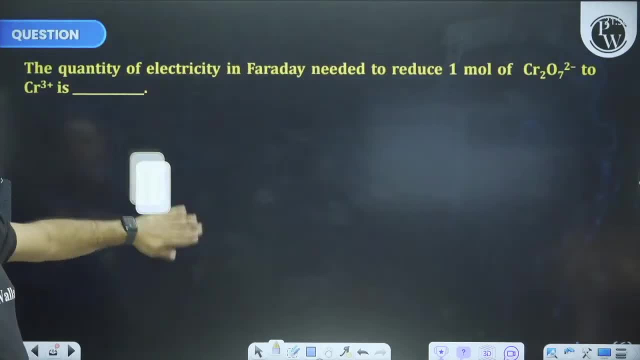 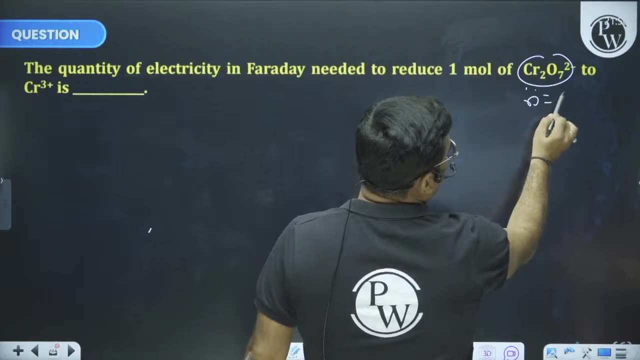 I am not cheating. take this quantity of electricity in Faraday needed to reduce 1 mole of dichromate to this. now I had told you child dichromate's n factor is 6, because in dichromate chromium is in plus 6,. 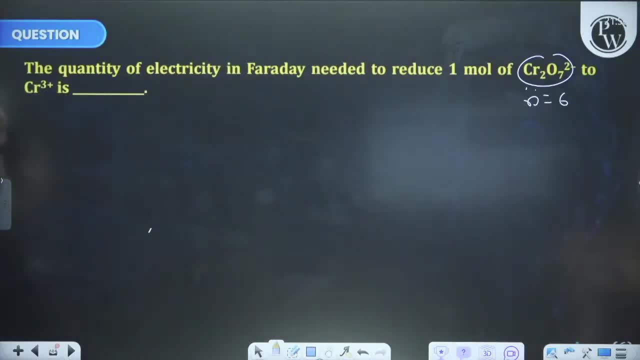 it always goes from plus 6 to plus 3, how much is the change? 3, and there are 2 chromium atoms, so 3 double 6 happened. okay, so if n vector is 6, that means 6 moles of electron happened. 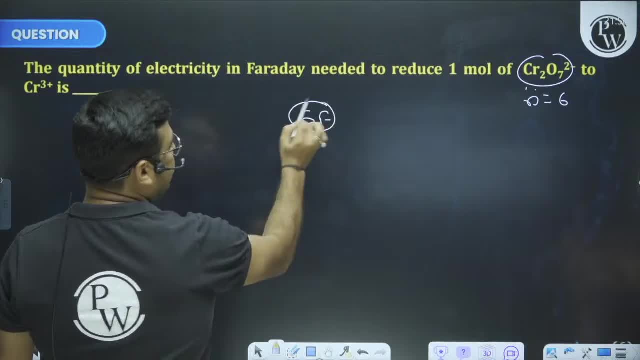 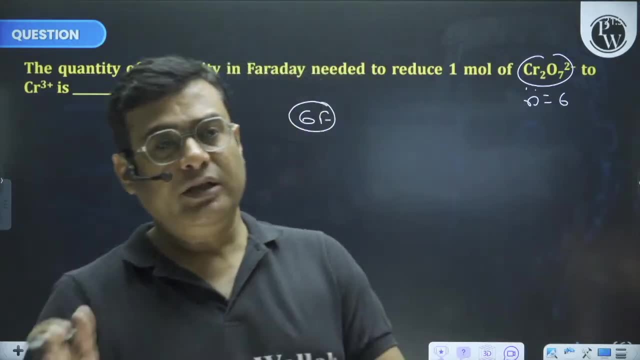 and 6 moles of electron means 1 mole will take 6 Faraday. in the question also, 1 mole is 6 Faraday. I have not brought every question child. I am telling something similar to that. I have kept 1,, 2 questions with me. 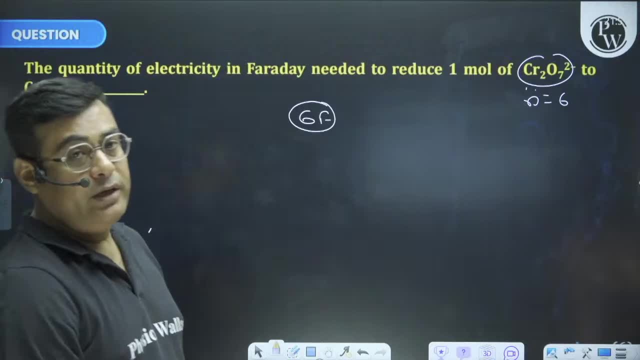 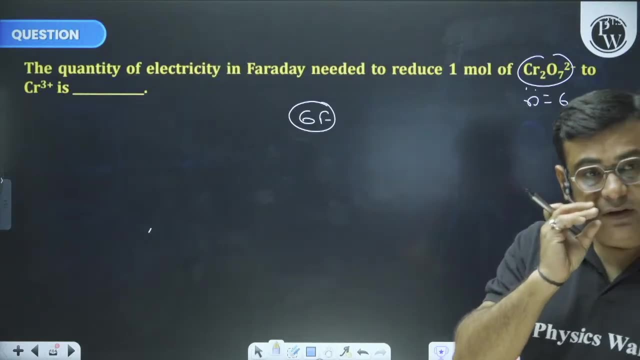 now these 3 children. they have not changed yet. they have not changed yet. see, you make this mistake again and again. you make this mistake again and again in n factor children. it is also important to take care of the number of atoms. 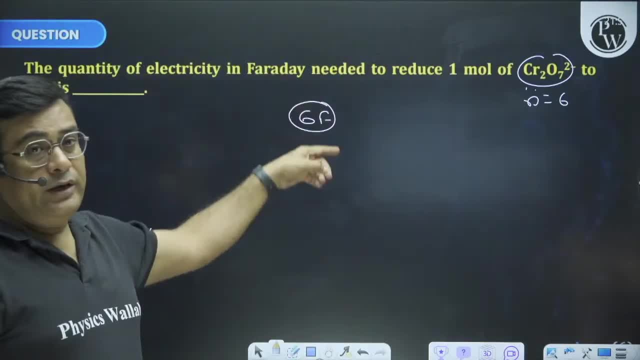 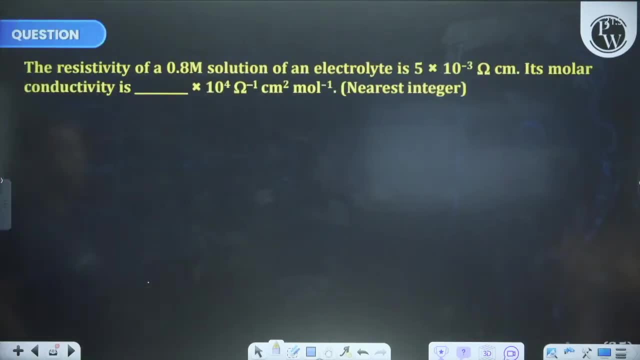 number of atoms. chromium has 2 atoms, so you have to do 2 into 3, 6, chromium has 2 atoms, so you have to do 6,. now you are talking about conductance. come in, conductance, children. 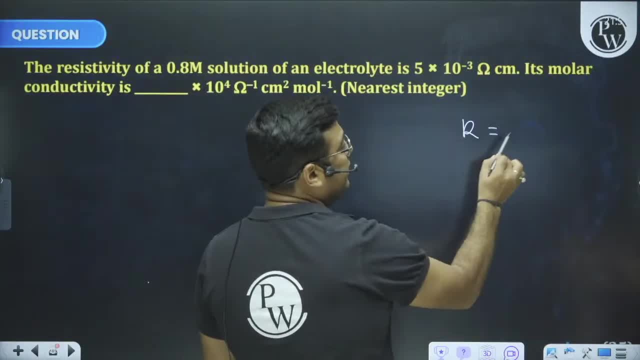 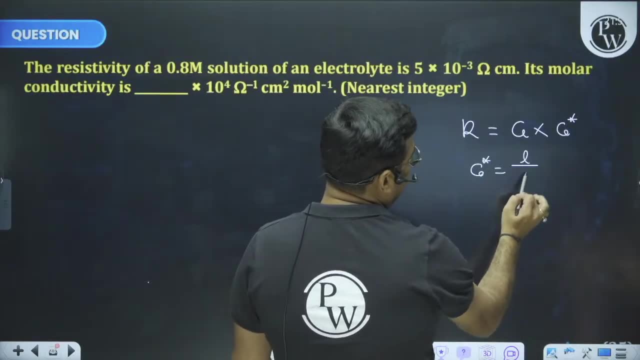 one is the formula of conductivity. the formula of conductivity is conductance into cell constant. I hope the formula of cell constant, everyone must know it is the ratio of distance between the electrode to the area of electrode. okay, apart from this, children, 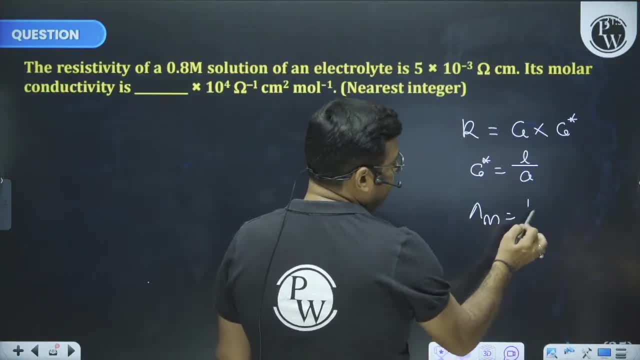 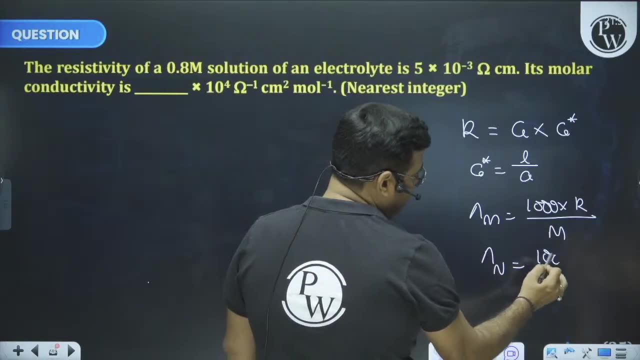 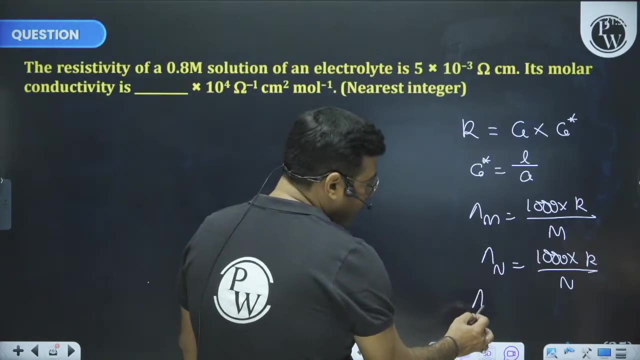 say the formula of molar conductivity 1000 into kappa by m, the formula of normal conductivity 1000 into kappa by m, hopefully, and Debye-Heckel-Onsecker equation. everyone will know, lambda m. 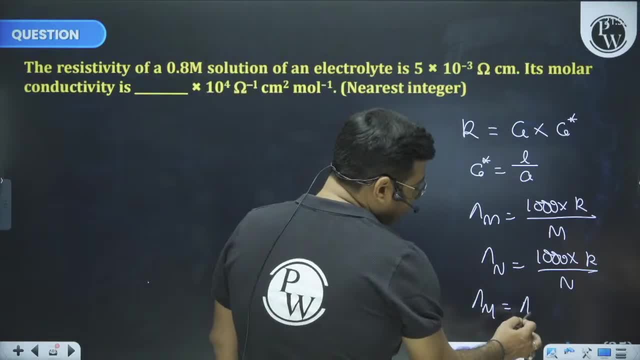 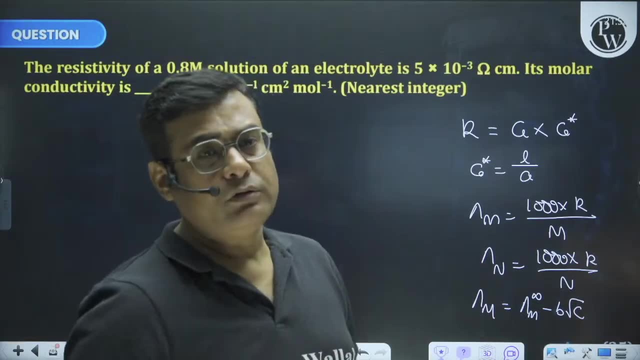 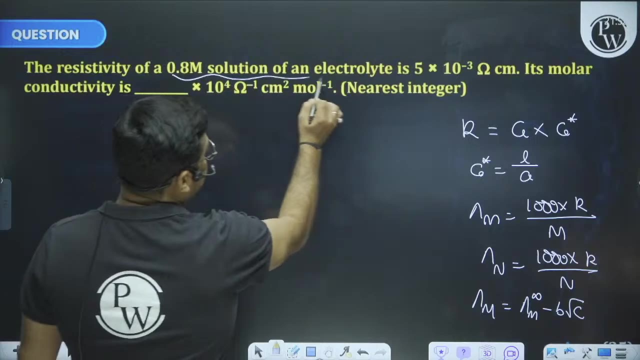 lambda m equals to lambda m, infinity minus b root c. okay, and Kolroth's law? Kolroth's law. we will talk through the question. okay, now see what he is saying. resistivity of 0.8 molar solution of an electrolyte: is this much? 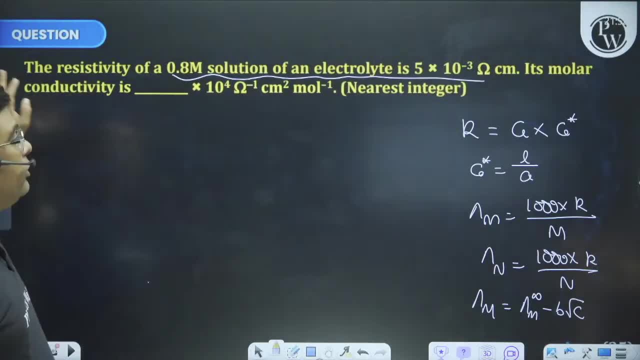 resistivity means the reciprocal of kappa, its molar conductivity. the question is over children. I am writing the values but you do it. so lambda m equals to 1000 into kappa, its reciprocal, that is 5 into 10, to the power of minus 3,. 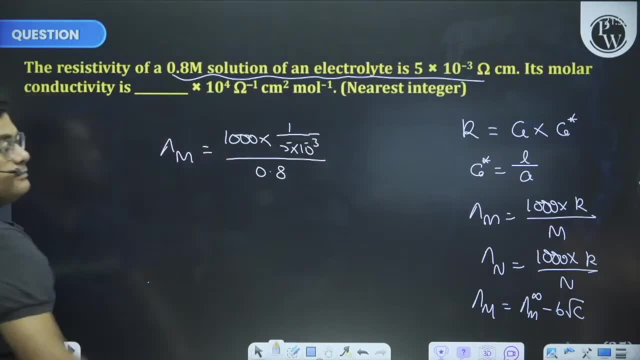 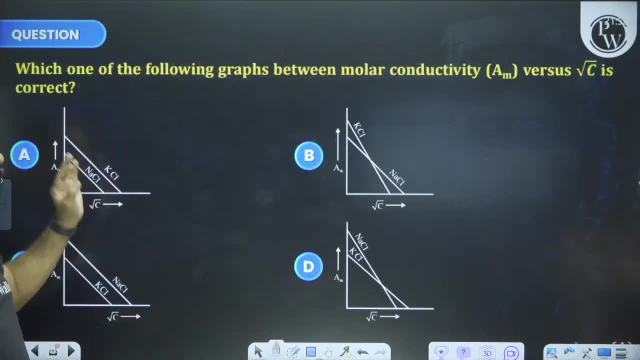 and below the molar conductivity is 0.8,. okay, this is how it will be now. see, this question is also important. you all will know Debye-Heckel-Onsecker equation lambda m. I just said. 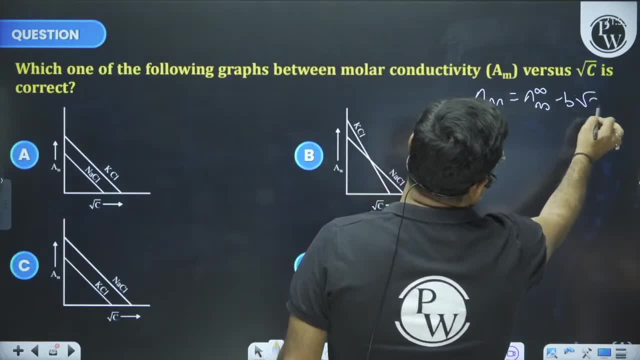 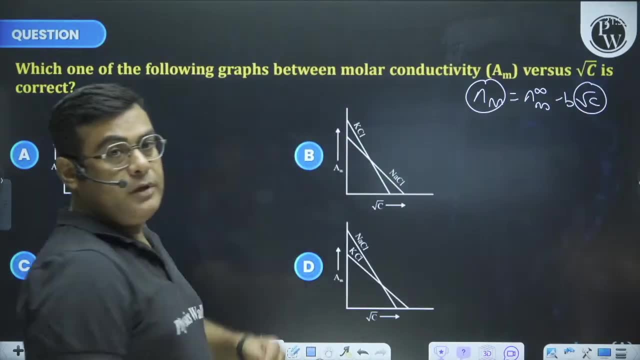 equals to lambda m, infinity minus b root c. okay, so if if you are asked the graph of lambda m versus root c, if you are asked the graph of lambda m versus root c, then what is the graph of lambda m versus root c? 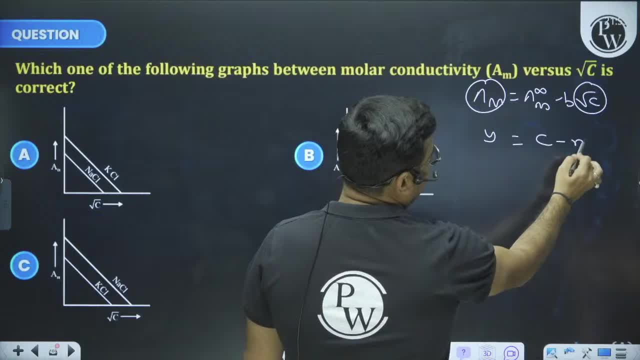 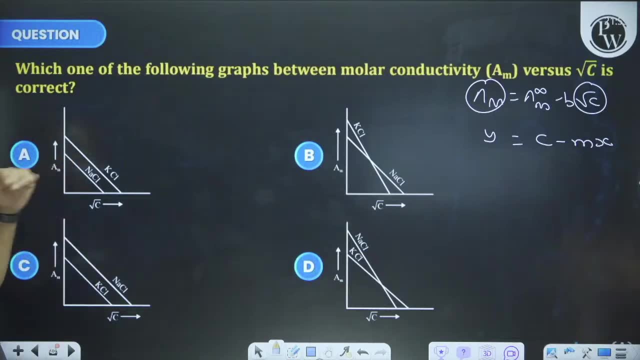 children. y equals to c minus mx, straight line with negative slope. now he has made a comparison of two. right that one is NaCl, one is KCl. what kind of graph will it be? pay attention, children, the graph is never going to cut. 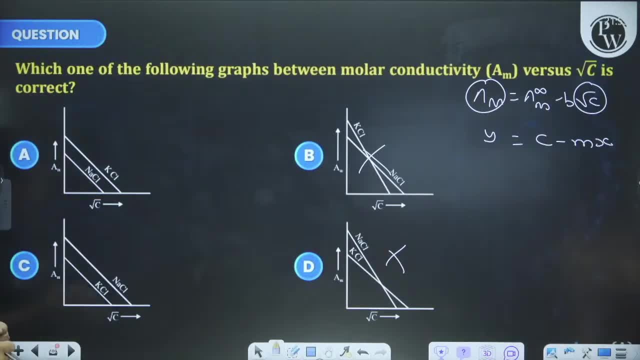 it runs parallel. NaCl is also a strong electrolyte, KCl is also a strong electrolyte. the graph is not going to cut. it will run parallel, children, okay. first thing, if we run parallel, then we have to decide who is above and who is below. 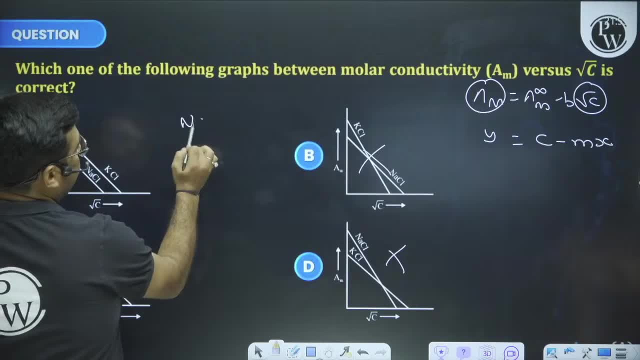 right. so all of you must have read in bonding children: Na plus aqueous and K plus aqueous. who is heavy? the ion is as small as the ion is as thick. you must be knowing so Na plus is a small ion. 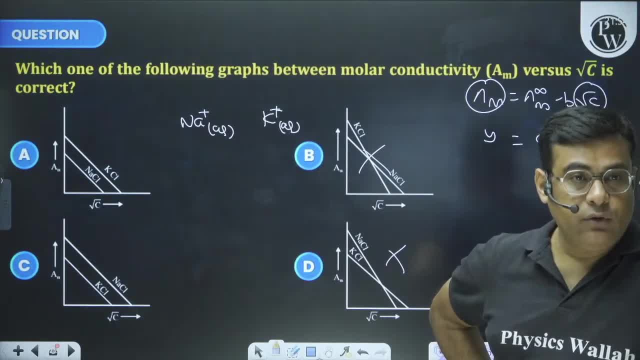 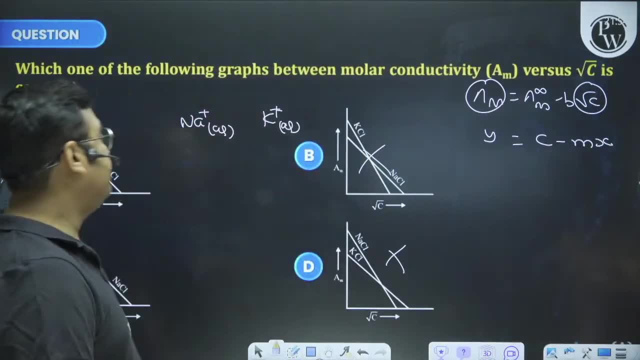 means its hydration will be more. it has become so heavy. and if it becomes heavy, son, then it means its conductance has become less. so in Na plus and K plus, the conductance is more than K plus, so the graph of K will be above. 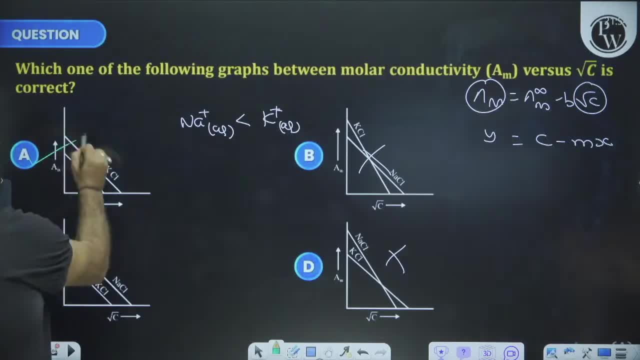 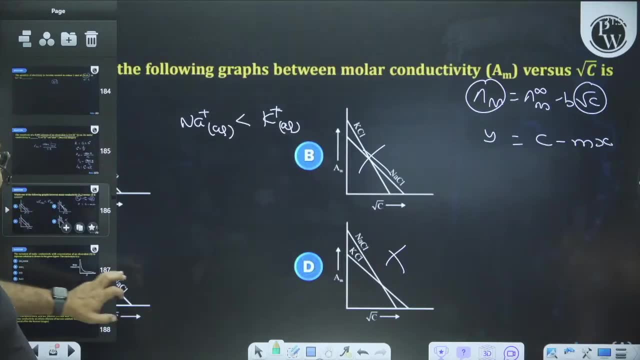 so the graph of K will be above means KCl above NaCl below, KCl above NaCl below. everyone understood the next thing. now look at this. the graph of lambda M versus root P is given. I have asked which of these will be an electrolyte. 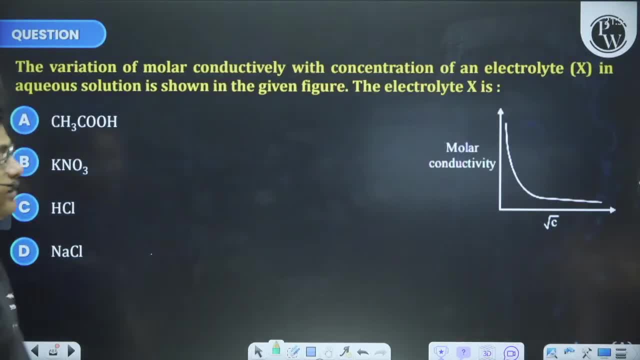 so, brother, the graph of lambda M versus root C, if it is not a straight line, it is a curvature, then it means it will definitely be a weak electrolyte. it means which electrolyte will definitely be a weak electrolyte. 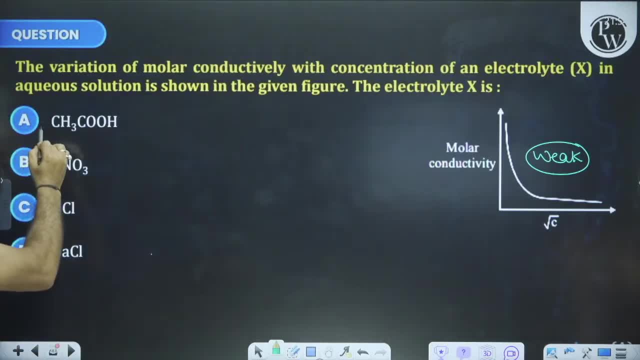 now in all of them. weak electrolyte is only acetic acid. salt is a strong electrolyte. salt is a strong electrolyte. SCL is a strong acid. the story is over when simple, simple questions come. children. the only difference is that 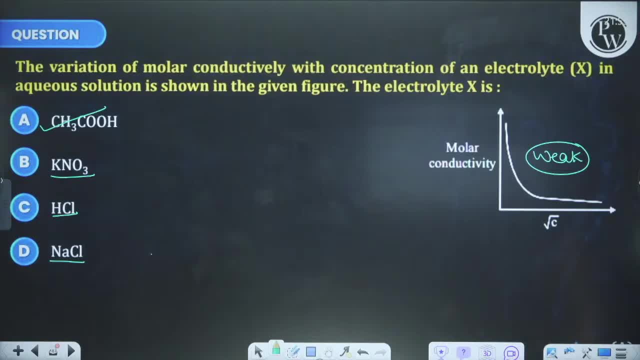 we may not have understood those questions that much. with that maturity, my purpose was that at the last moment, I will give you a little idea through all the questions that brother. our questions are very simple. we are a little afraid of them. 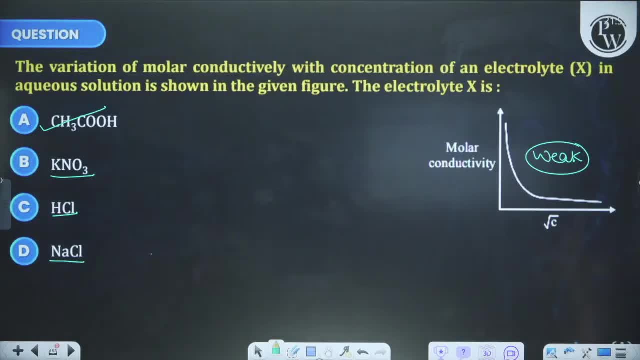 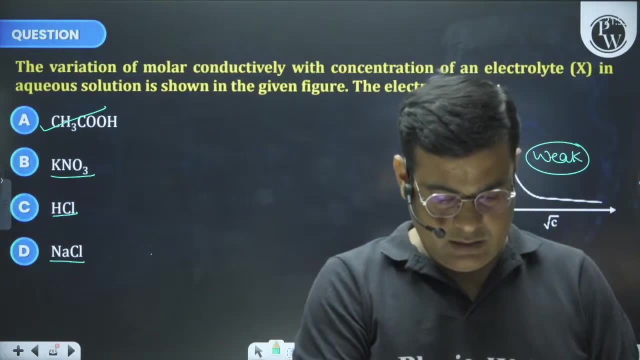 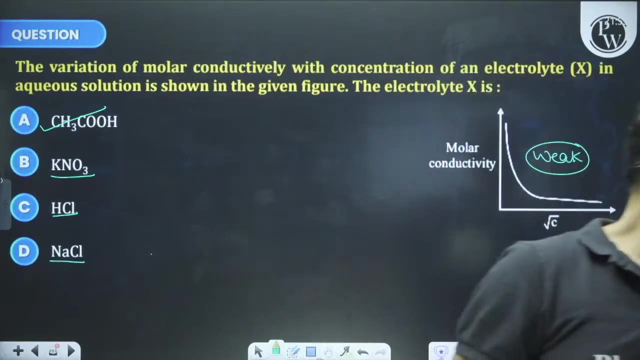 by confusing them. we are making a little mistake, and if we are saved from it, then our work will be relatively easy. the voice is not coming. is the cell over? is the voice issue coming? let me ask: is the battery okay? 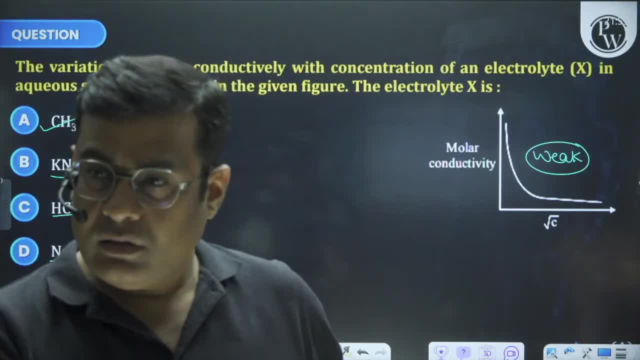 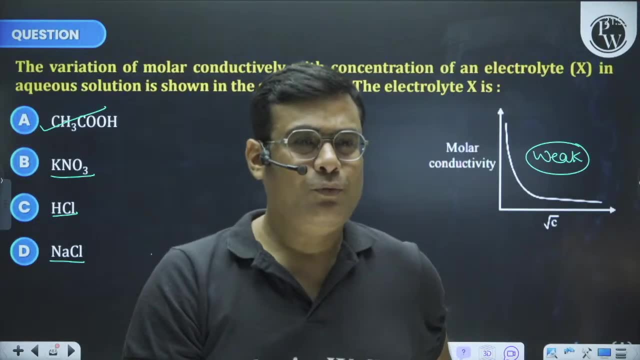 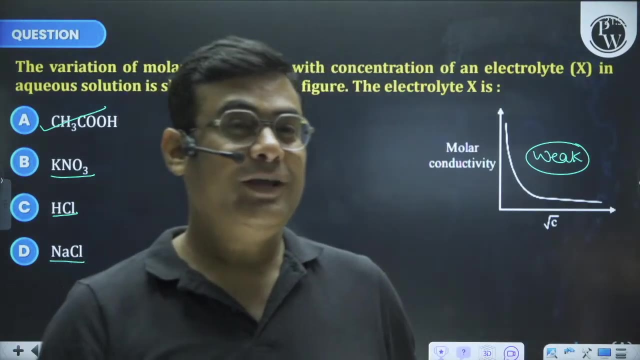 will it work? now, some children, son, it's coming, no issue. ok, don't do this. don't lie, lie, the crow will bite. be afraid of the black crow. I will leave the class and go. you keep watching. 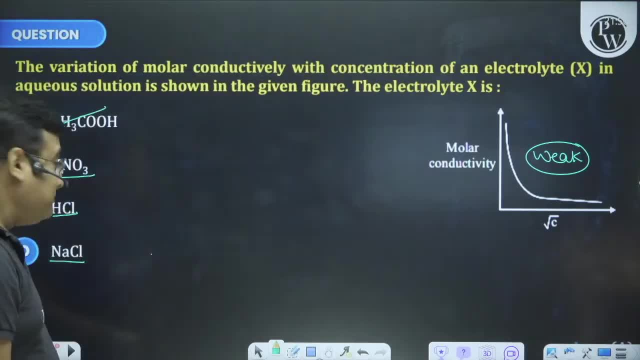 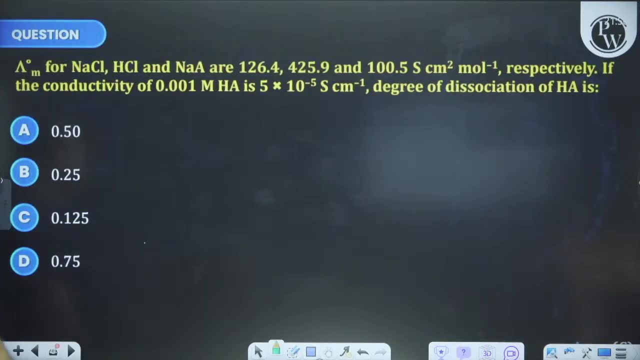 it's not like that. don't try to run away. ok, son, come on. so I hope children, I have given a lot of ideas. now I will give you the last one. I will give you my idea on Kolrosh law. 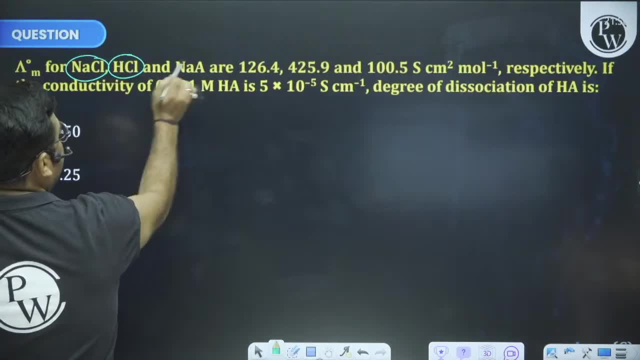 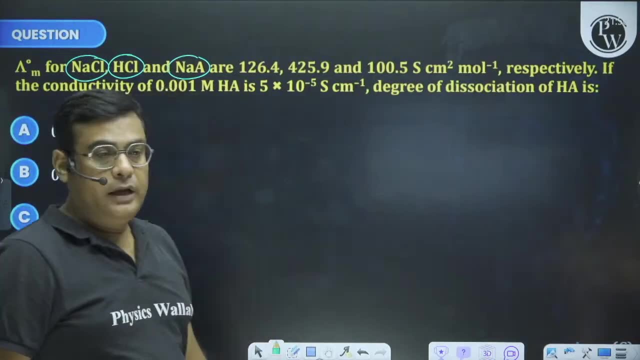 Kolrosh law see NaCl, HCl, Na. the conductivity of these three is given the conductivity of 0.001 molar HA. is this much? tell me the degree of distortion of this right. what are the formulas of Kolrosh law? 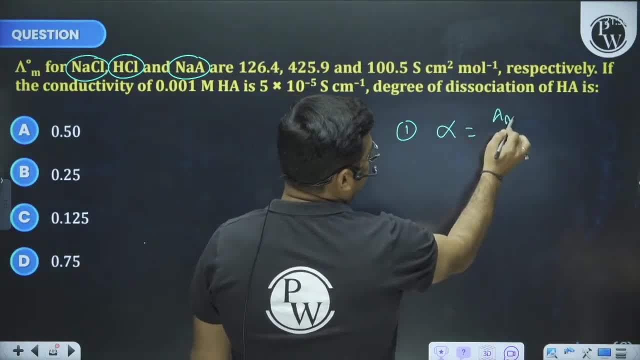 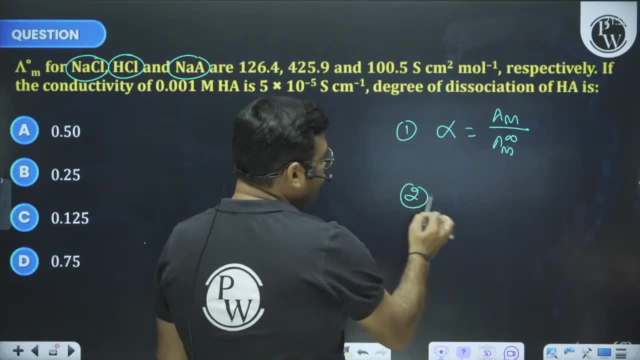 first, if alpha is asked, then lambda M upon lambda M, infinity, ok, right. second, the solubility will ask son, and once alpha comes, then the distortion constant will ask T alpha square upon 1 minus alpha. 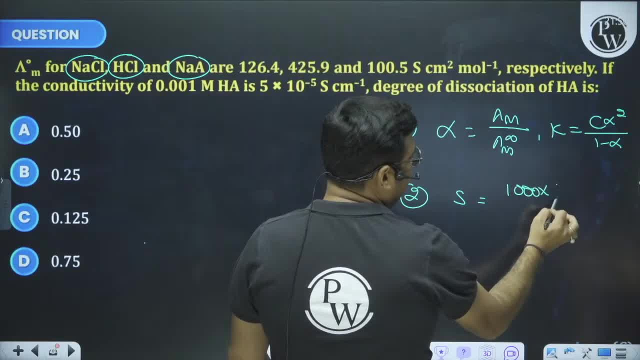 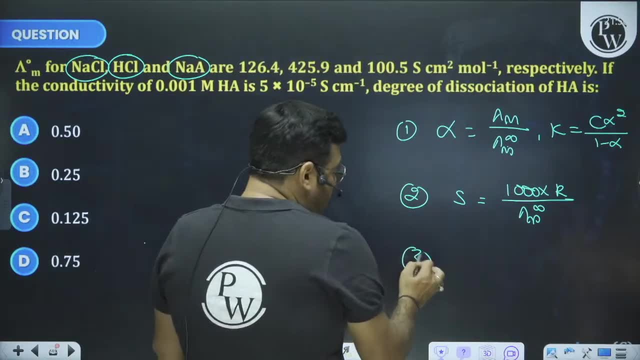 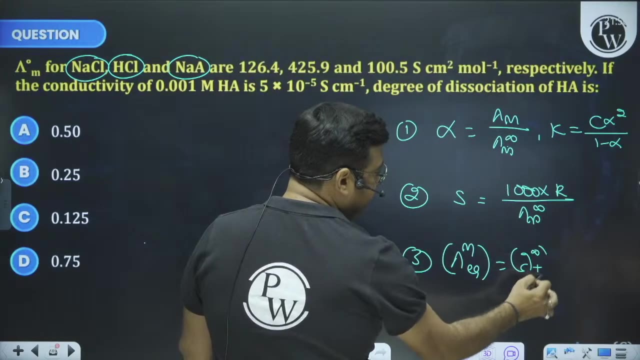 the formula of solubility is 1000 into kappa by lambda, M, infinity right, third children, that the equivalent conductivity of any electrolyte will be equal to the sum of the equivalent conductivity of cation and anion. the most important thing in Kolrosh law. 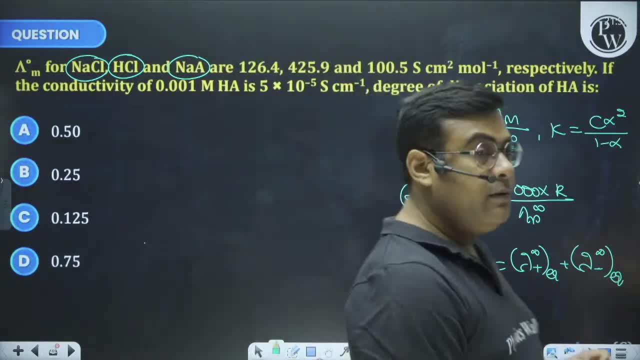 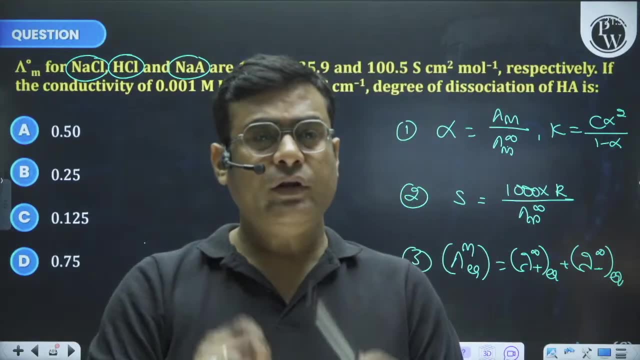 you have to keep this in mind, children, that Kolrosh law is applicable only for infinitely diluted solution. right, right. it is applicable only for infinitely diluted solution and you cannot apply it on anyone. keep this in mind, and this is the fourth type of question. 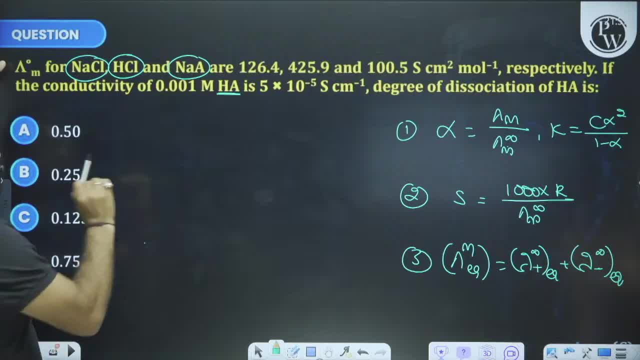 now see here which is weak electrolyte: HA. so if I want HA children, then many times children are unable to remove it. so you have to listen to my rule. HA is three are NaCl. 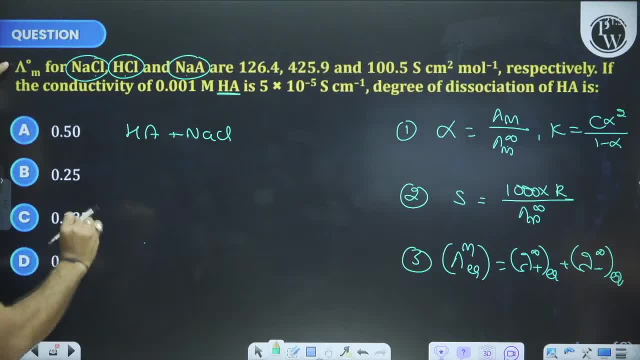 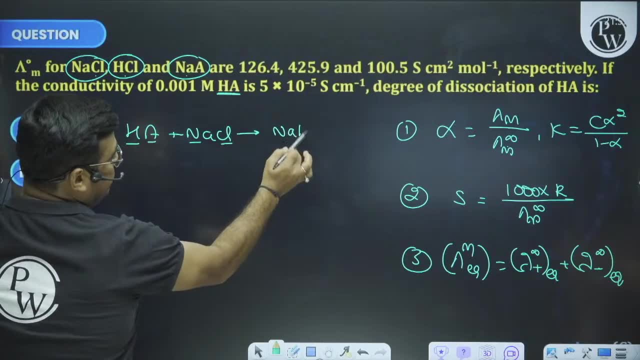 NaCl. so take NaCl. take two electrolytes whose four ions are different. okay, if these two react together, then what would happen? NaCl would be formed and HCl would be formed. so if I want to remove HA, 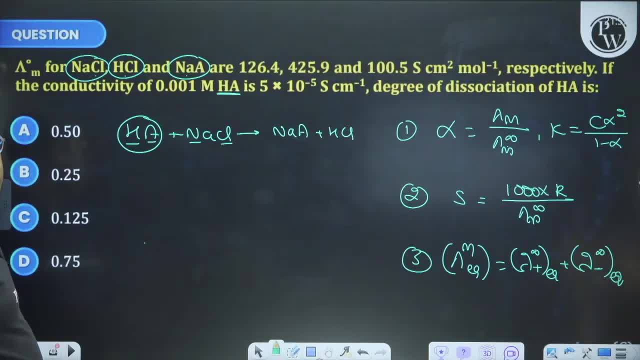 limiting molar conductivity. listening is also the most important thing many of you children will get. so you have to add NaCl to HCl and you have to minus NaCl. you have to add NaCl and HCl. sorry, 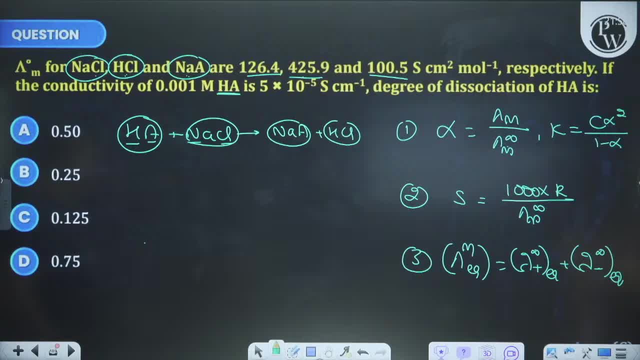 you have to add these two children and you have to minus this. now you also get used to some rough calculation. consider this as 426, in 426, 100 plus 526, and reduce 126,, then 400 is left. 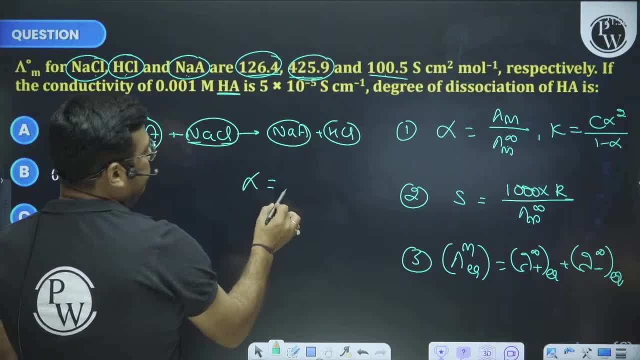 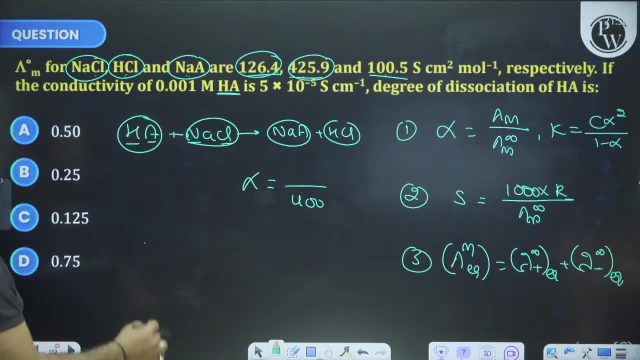 so the value of Alpha is: see. the value of lambda m infinity. how much? 400, see now. it has given conductivity 0.001 molar HA. so conductivity, okay, take out the molar conductivity from it. 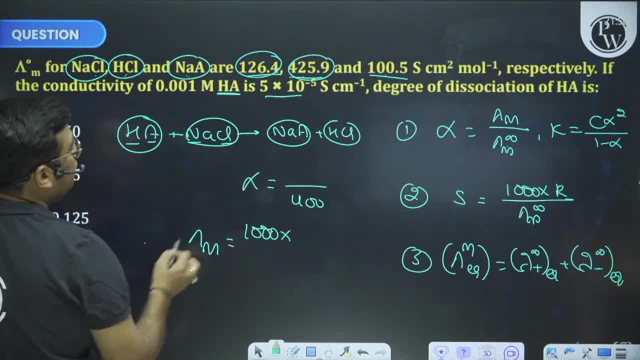 lambda m. how much 1000 into kappa? kappa is 5 into 10 to the power of minus 5. divided by 10 to the power of minus 3, this becomes 50. so 50 divided by 400 means 1 by 8, and 1 by 8 means 0.125. 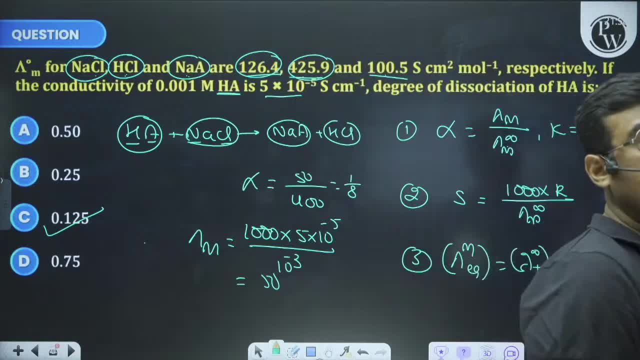 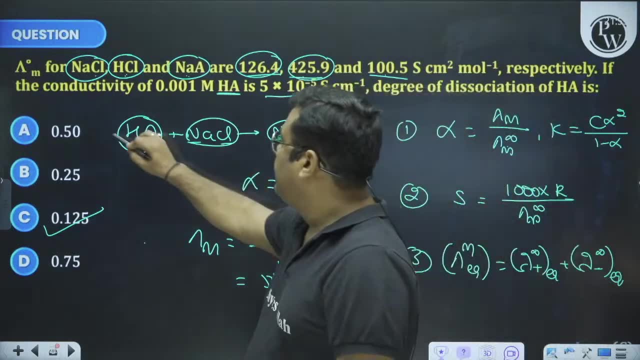 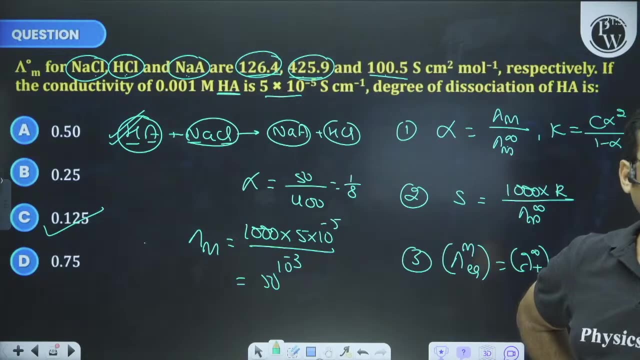 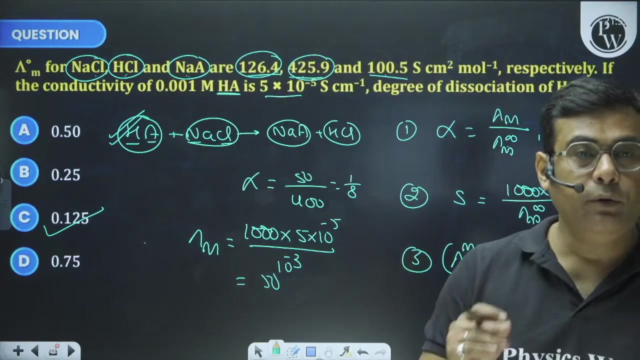 in kohlrausch law. if you remember these 3-4 things, then your work will be done. and the most important point of this is that whenever in 3 electrolytes in kohlrausch law the conductivity of 3 electrolytes is given and after that you have to take out the 4th, 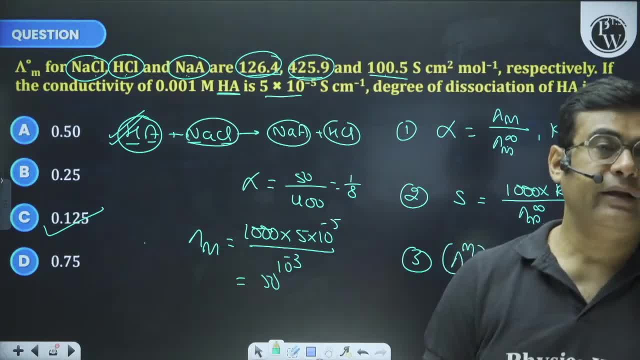 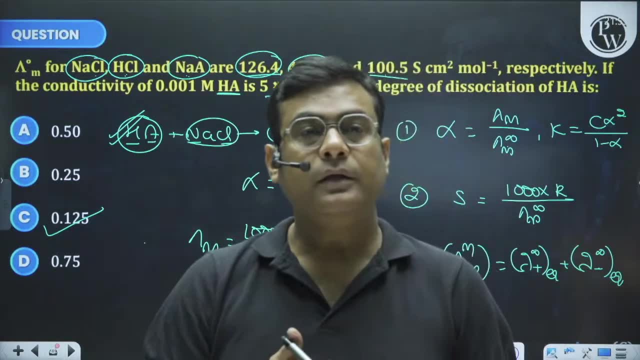 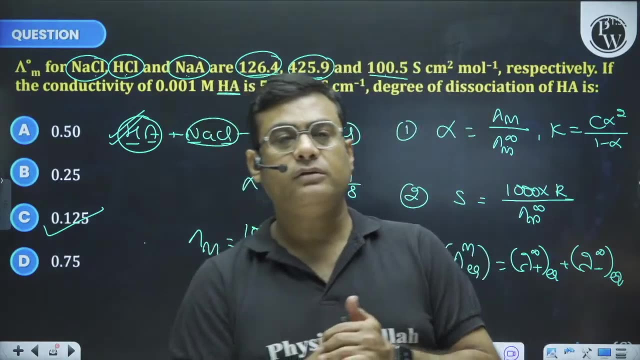 then you will have to apply this technique always, because in books the normal option of this is that even if there is a CH3CAA option, then only this answer would have been there in the previous question. because in salt all the electrolytes are strong. salt, all the electrolytes are strong. 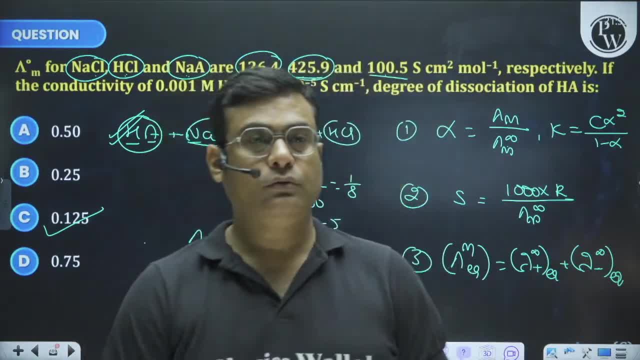 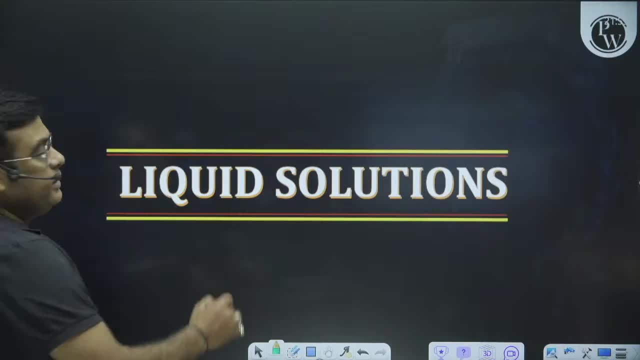 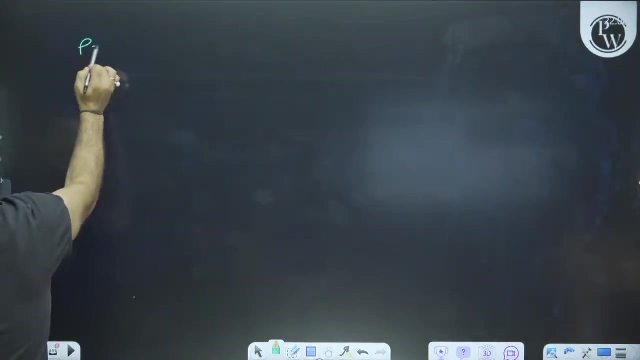 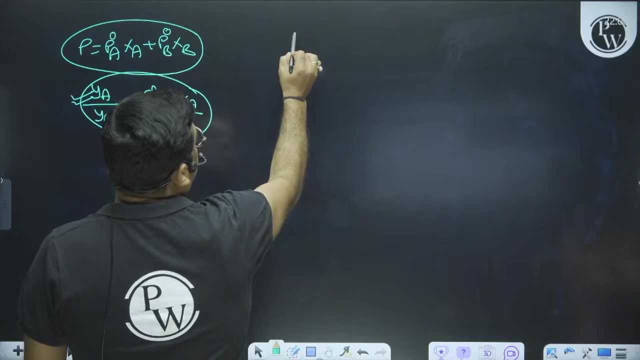 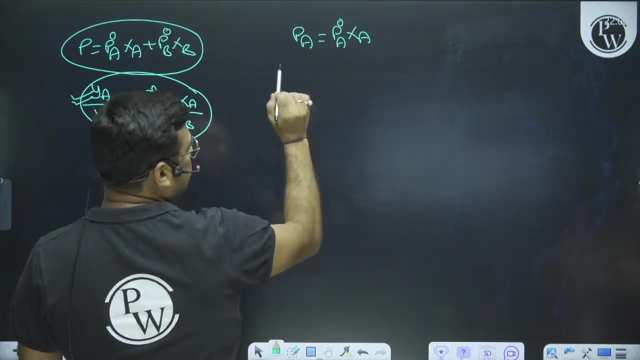 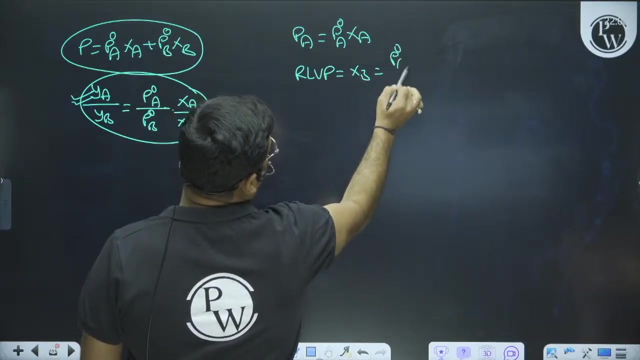 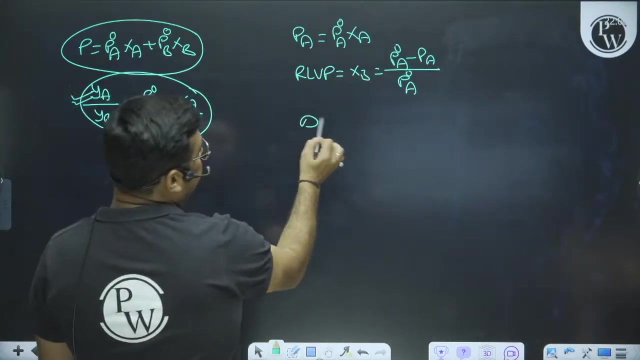 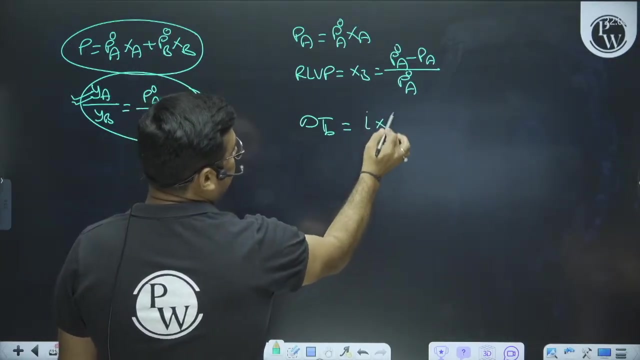 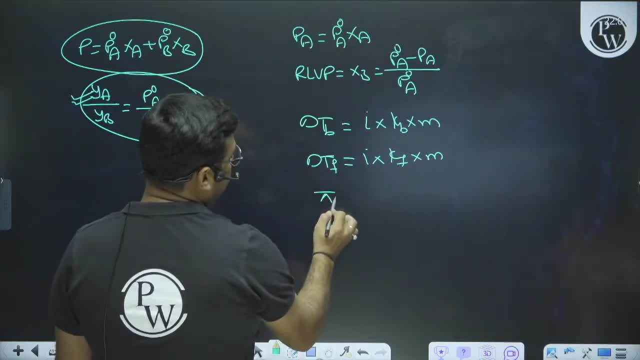 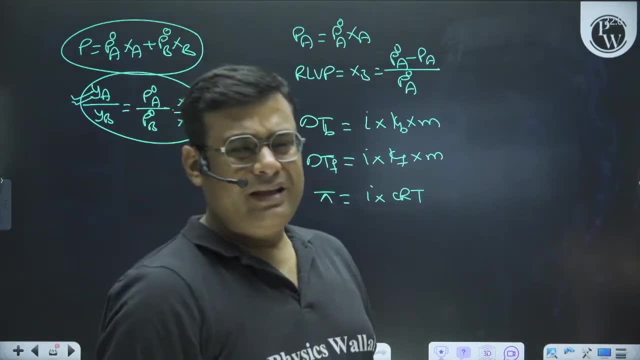 F into M. Osmotic pressure is pi, which is I into CRT. In the shortcut through the questions, what will you ask for a break, son? Now let it run in the break. Let's finish it in an hour and a half. 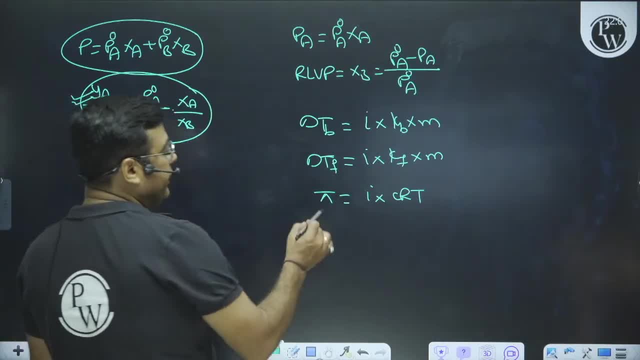 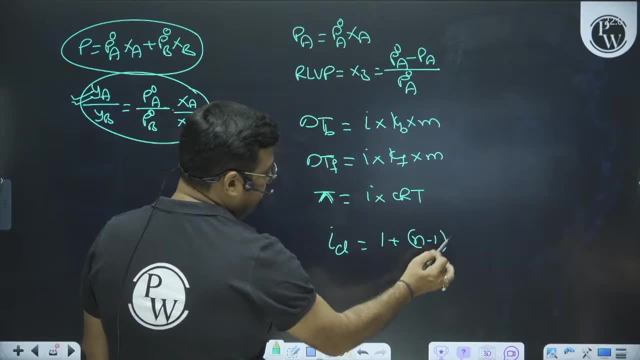 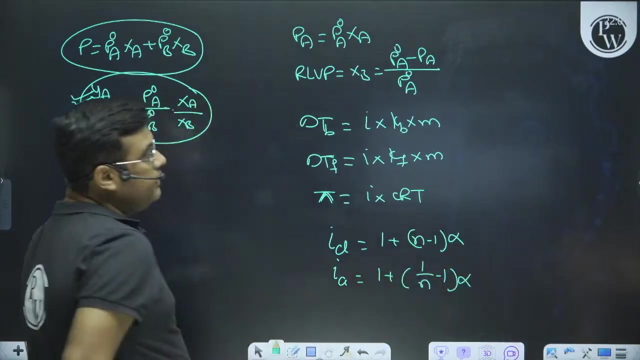 So pi equals to I into CRT And apart from this, children, apart from this children, the formula of I is of dissociation is 1 plus n minus 1 into alpha and the formula of association of I is 1 plus 1 by n minus 1 into alpha. So if you just have these small formulas, 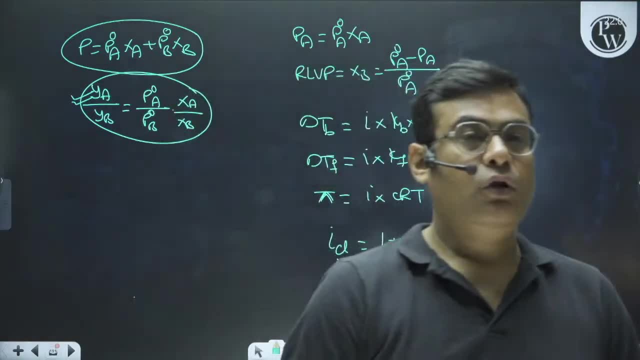 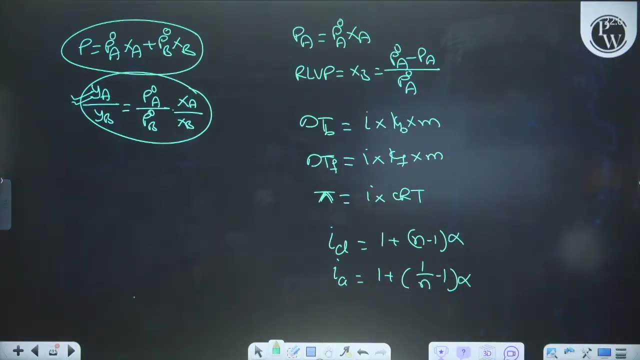 now. their calculation is very good and I will explain it to you right now. I will tell you right now, in this topic, I am going to tell you short tricks, so everyone should tie their waistband. everyone should tie their waistband because you are going to get good, good, good. 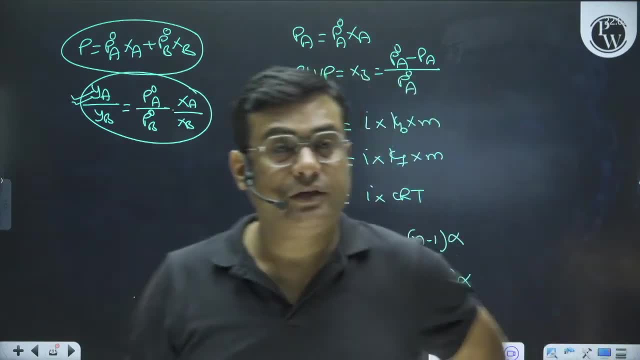 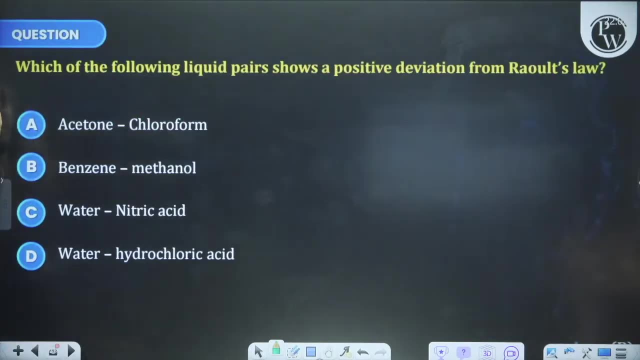 results in this Shortcut. you are going to get good, good shortcuts in this. okay, let's see what is it? which are the following: liquid pairs show a positive deviation from Raoult's law. This is a question of ratification. all the pairs you have given in the NCRT book, right? 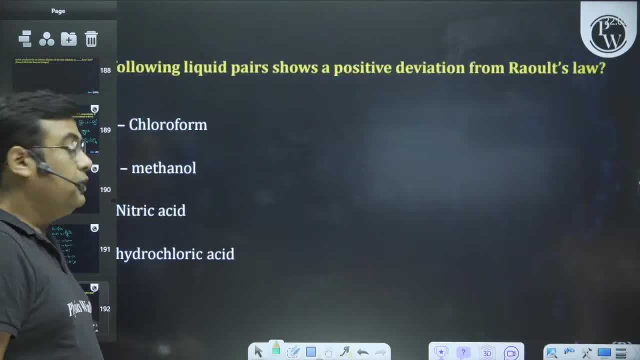 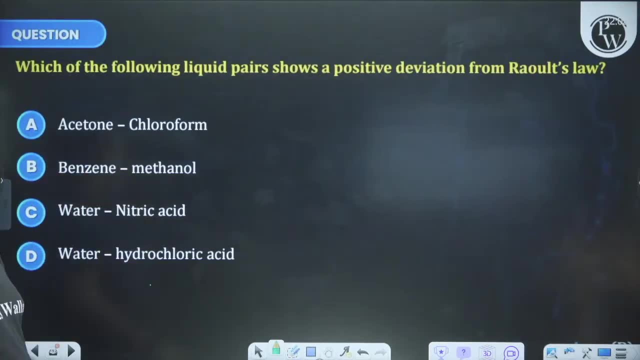 all the pairs you have given in the NCRT book children. okay, it is important for you to remember that right. it is important for you to remember that right. so acetone and chloroform: negative deviation, all of you should know right. water, nitric acid: negative deviation. 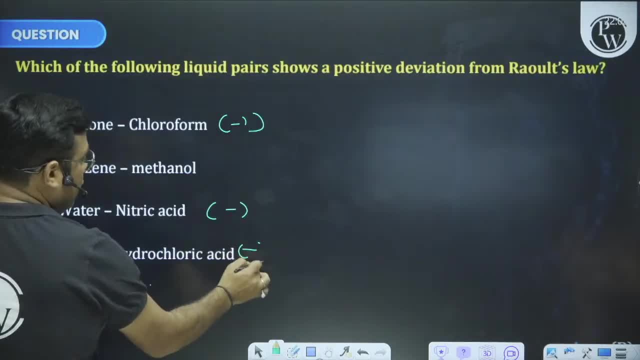 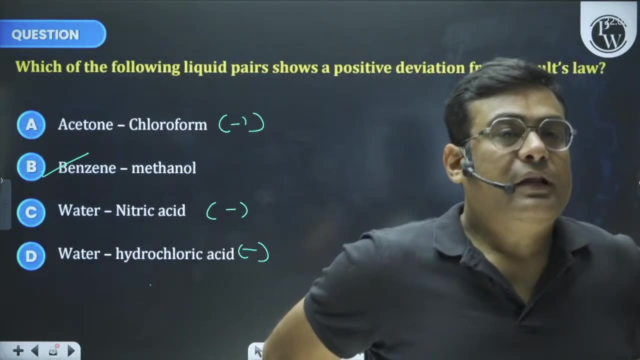 take any strong acid along with water. I am showing them who have come. but apart from this, if you remember that there is a pair in the NCIT, only benzene and methanol. why is this, sir? kids were hydrogen bonding in methanol when you put benzene in methanol. 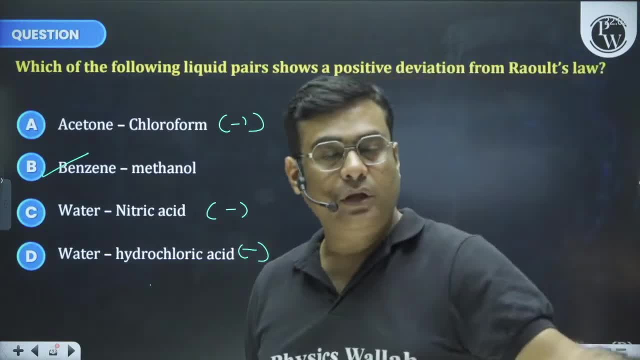 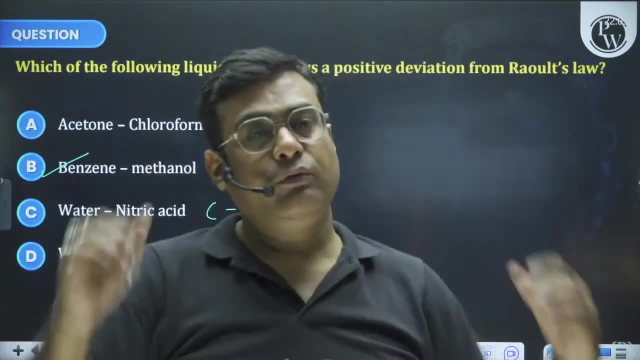 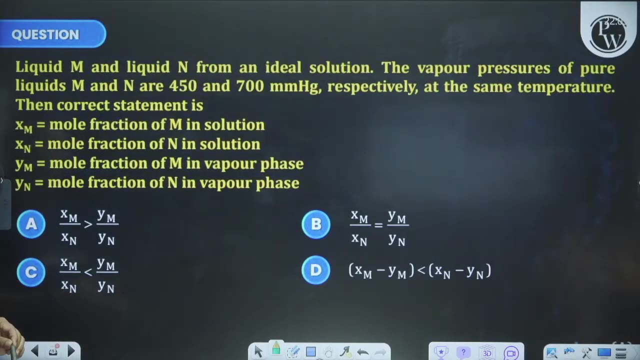 then methanol broke the H2O bonding of benzene and broke it. then the force of attraction increased and the force of attraction reduced. the force of attraction decreased and the force of attraction has decreased, then the tendency to vaporize has increased. then what else is there, sir? come on. this formula has been directly asked of you. 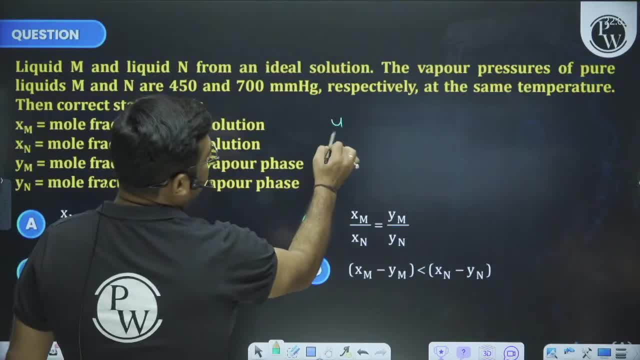 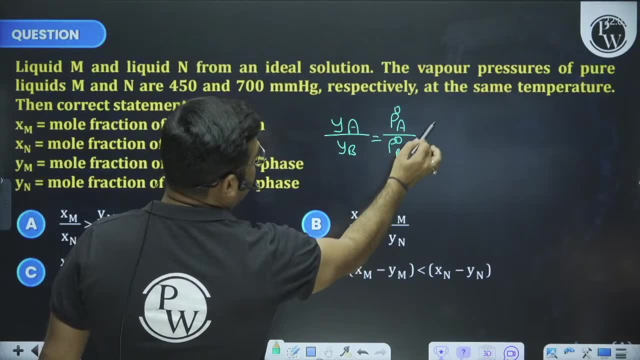 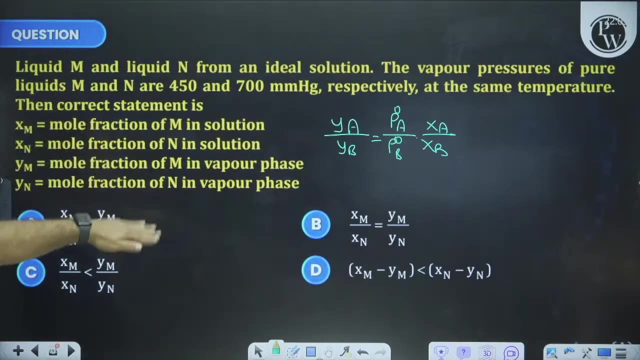 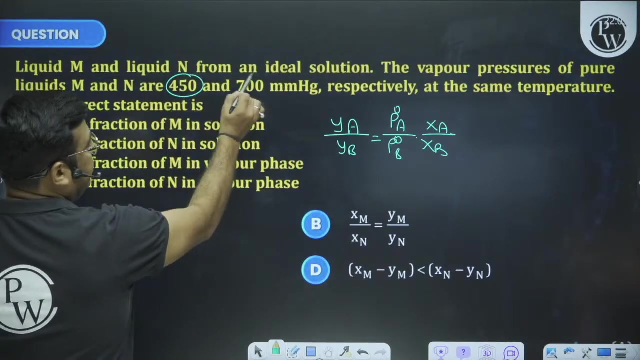 right now. I have written the formula from you: y a upon y b equals to p0a upon p0b, into xa upon xb. this direct question has come on it. I have considered a and b as liquid. they have considered m and n, isn't it? vapor pressure of pure m is four and a half hundred, one is seven hundred. 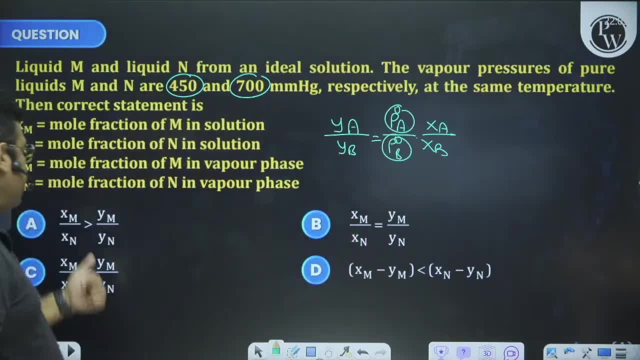 one will be four and a half hundred, one will be seven hundred, and after that you have to judge the relation. what will happen after this? you have to check the relation. okay, you will do that. I hope so much. now I am telling you a shortcut for this type of question. 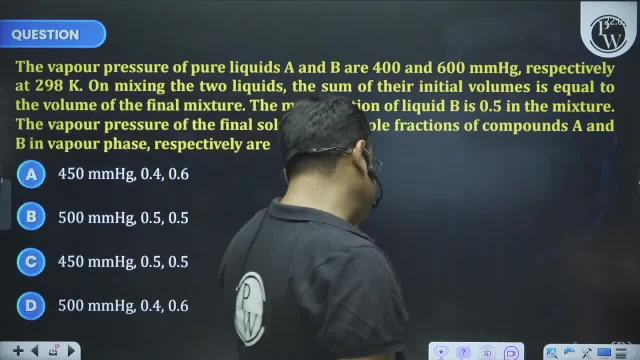 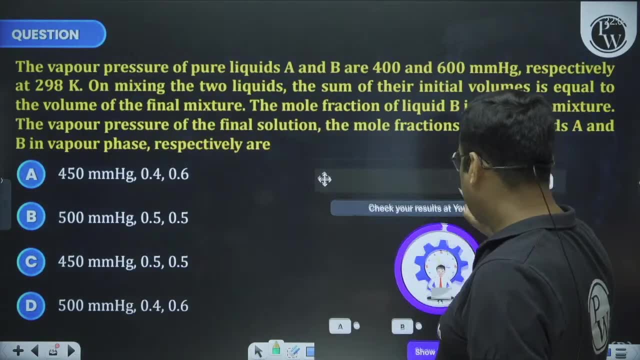 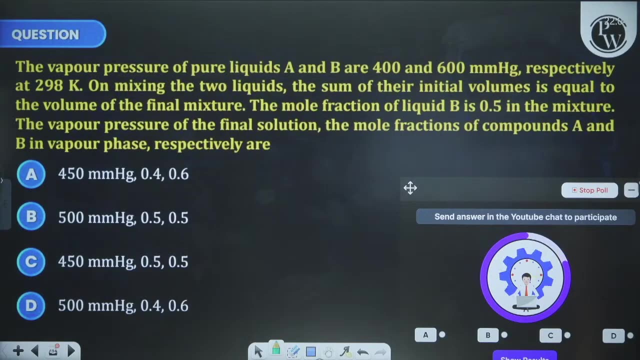 everyone read this question. there is no answer in this. come on, I am giving time of forty-five seconds. let me see how many questions can be done. how many children are now attentive that everything has been diverted a little here and there? 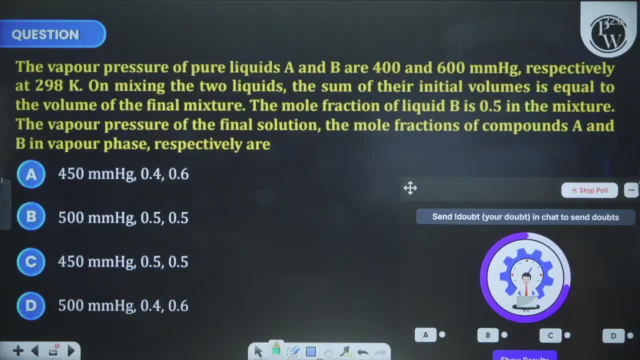 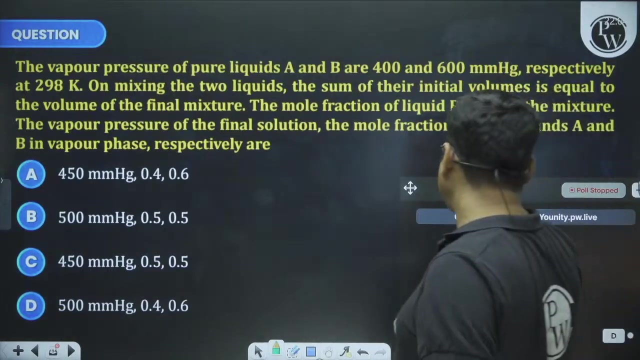 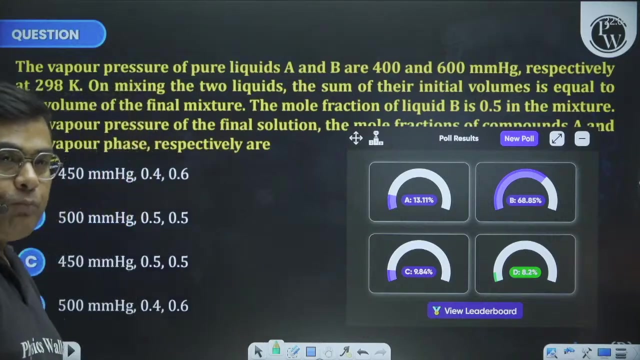 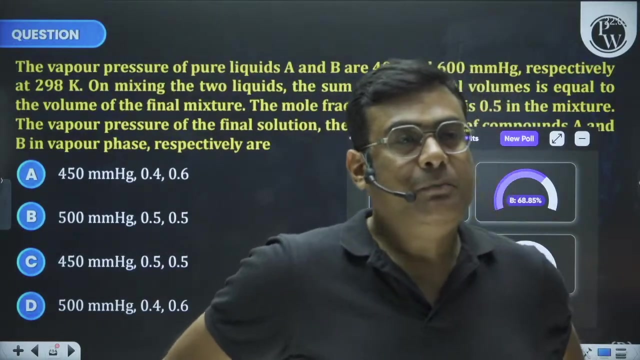 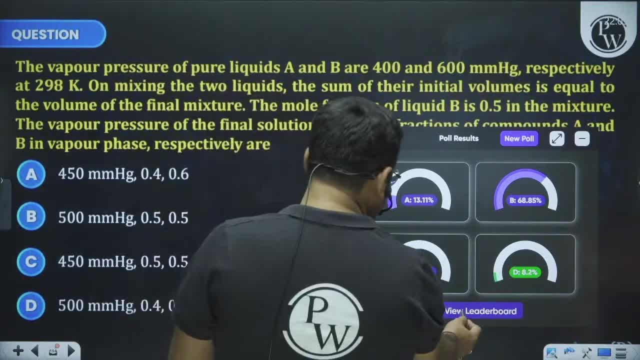 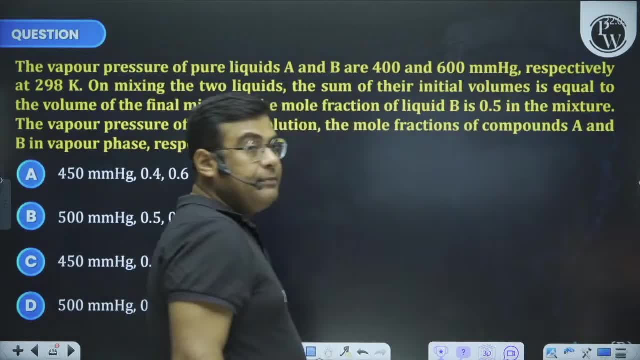 ok, Let's see the leaderboard too. Tamar Tawale, Yuvirao, Sandeep Bhajara, Sumit Om Parmar. ok, Now look at this question. I know that maximum of you did not solve it, son. they saw a bomb. 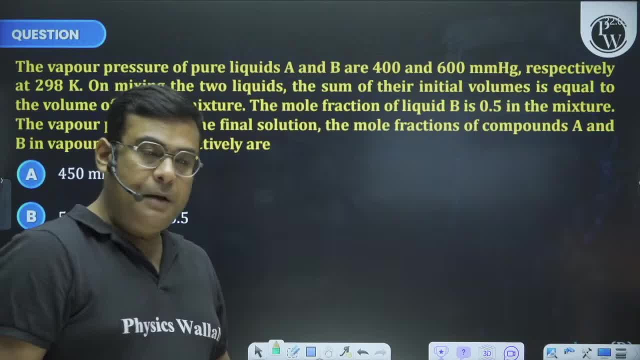 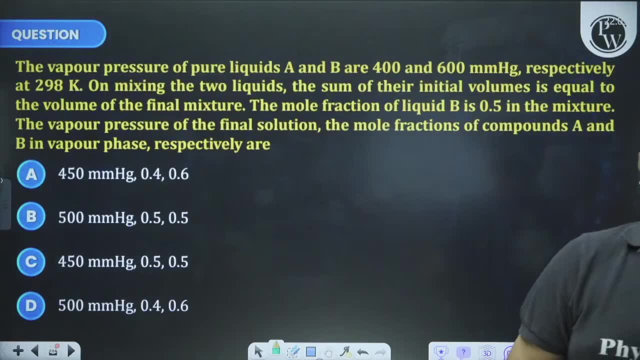 there and they killed it. Now, those who have solved it honestly, those who have solved it, they may have solved it hopefully. If they have also cheated, then it is a different matter. but actually there was no need to solve this question. 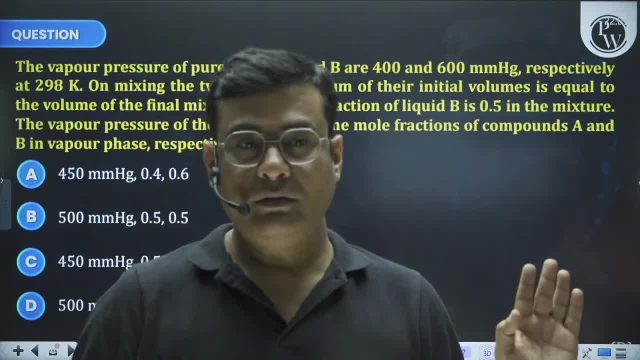 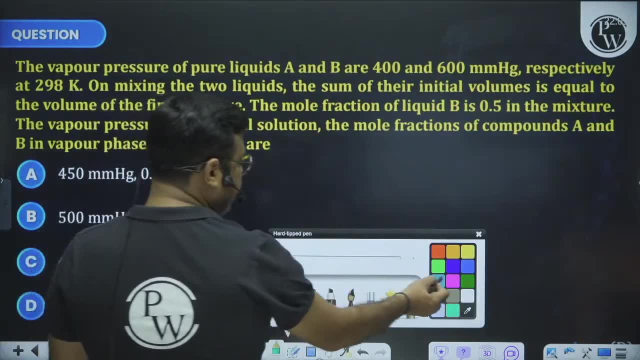 There was no need to solve this question. should I tell you the reason how only JSC has to be applied? it is the same shortcut that I wanted to tell you. the vapor pressure of pure liquid A and B is 400-600,. on mixing two liquids, some of their initial volume. 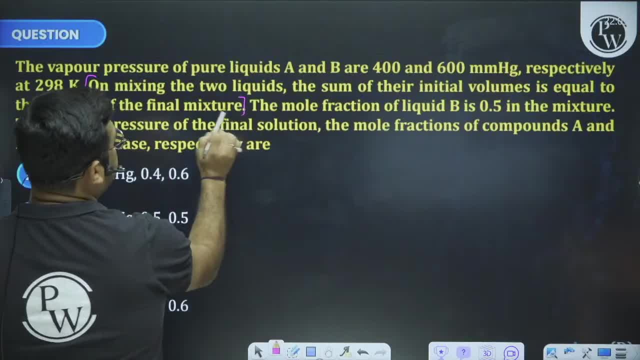 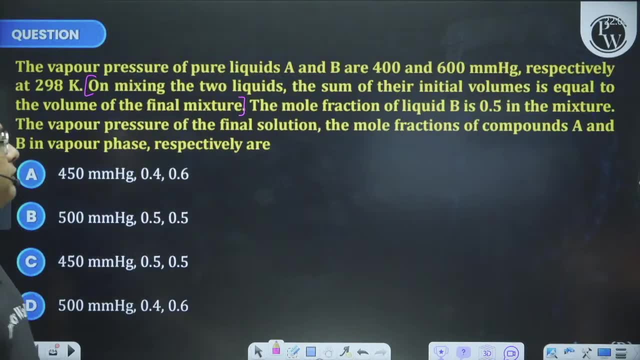 is equal to the volume of 500.. In the first line the vapor pressure is 100-600, now there is an additional volume of 200-300.. Now this is the last line. this is the final mixture with this. I got to know that this. 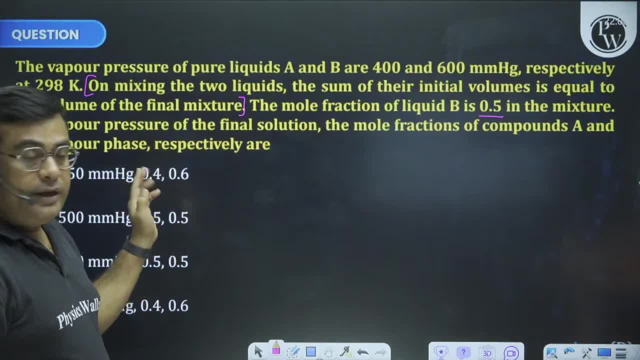 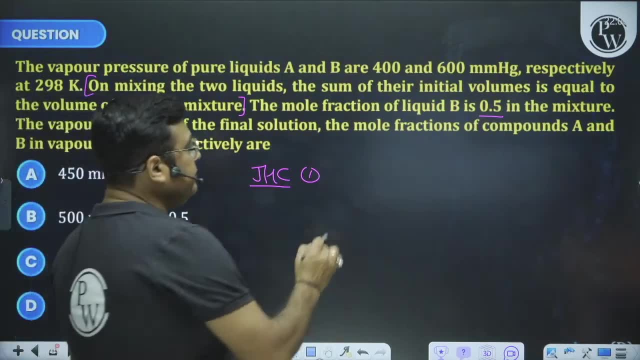 is making an ideal solution. The mole fraction of liquid B is 0.5 in the mixture. so if B is 0.5, then A is also 0.5.. Now, first is my JSC, First JSC. if first JSC, the vapor pressure of one is 400 and one is 600.. 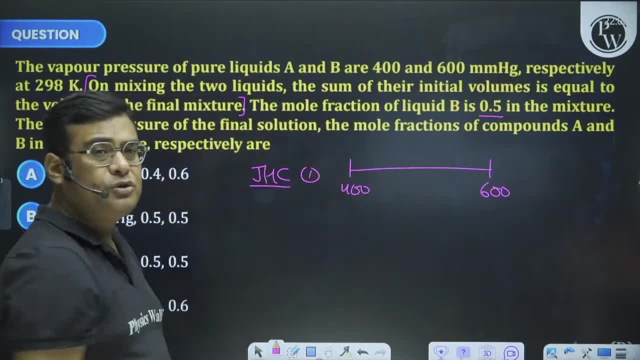 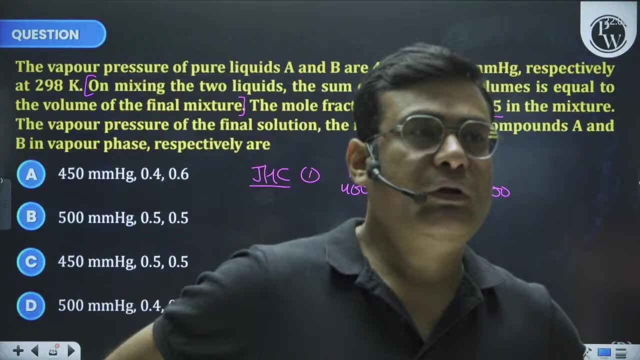 Now, this can be 200-300. also it can be 200-800.. Now, this is the first JSC. this is the vapor pressure of one and this is the vapor pressure of one. So, guys, the first rule is that the final vapor pressure of two volatile liquid mixtures will always come in the middle of the lower and higher value. 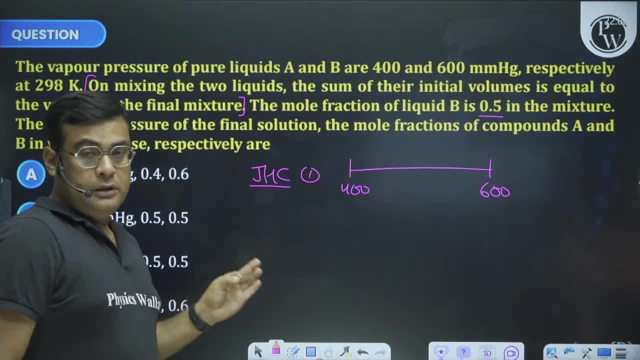 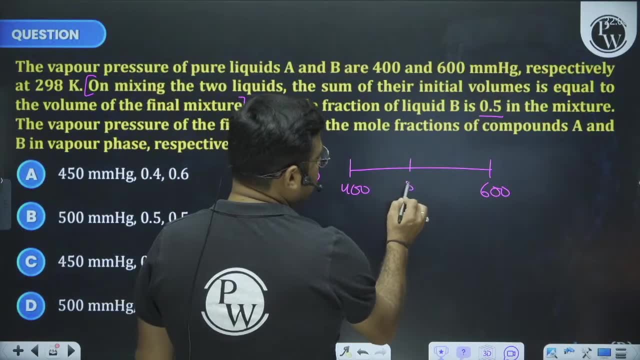 It cannot go beyond this. This is the rule. This is the question of JEE, so I am telling you that it cannot go beyond this. The second rule is that the exact average of 400 and 600 is 500.. The average of 400 and 600 is 500. 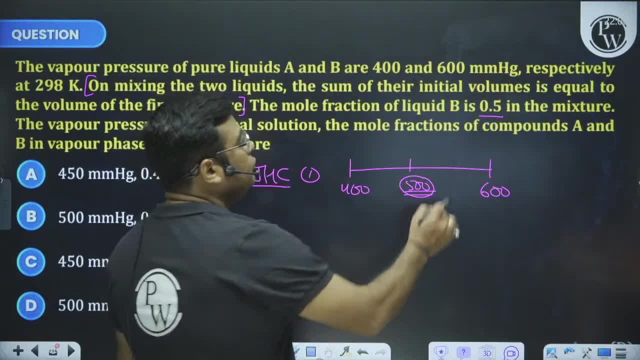 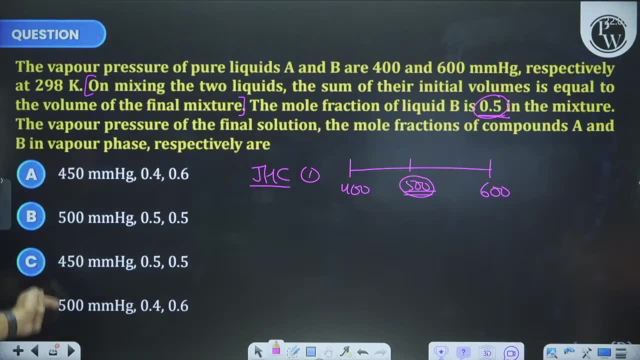 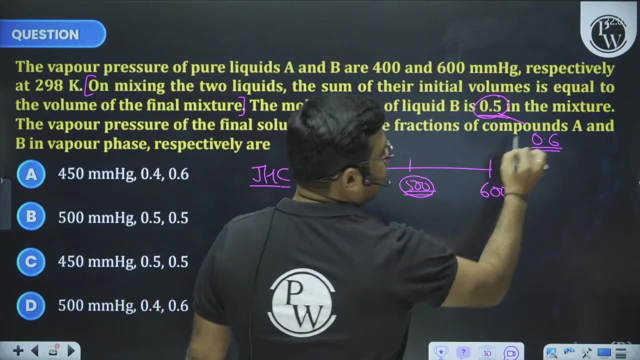 When will the average come? The average will come when the mole fraction of both is equal. Here, B is 0.5 and A is also 0.5, so the answer will be from B or D. Sir, what would have happened if B was 0.6?? 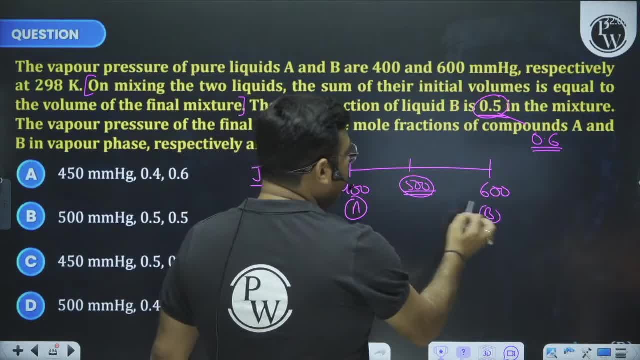 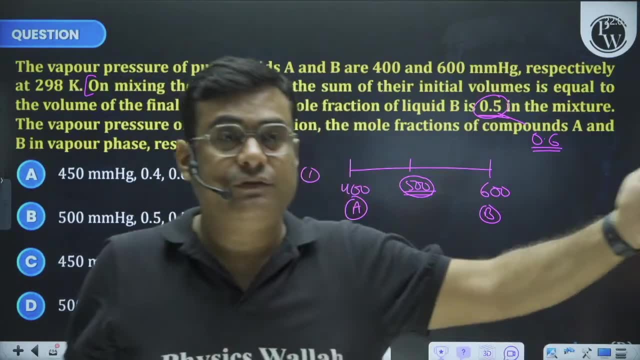 This is the vapor pressure of A and this is the vapor pressure of B. If you increase the mole fraction of B, then your answer will come between 500 and 600.. That means it will shift towards B. And if you increase the mole fraction of A, then your answer will come between 400 and 500.. 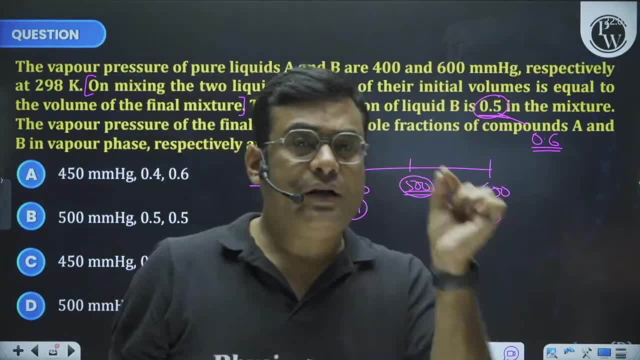 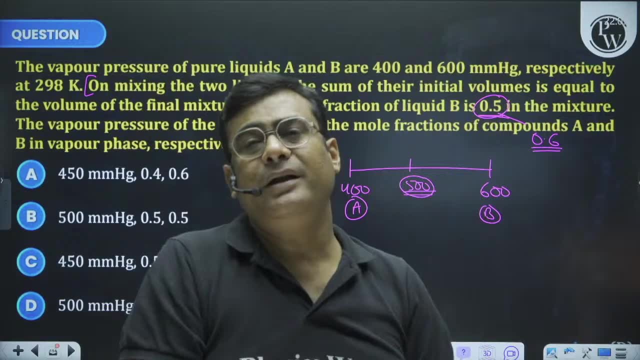 So if you keep such small shortcuts in mind, then you will definitely benefit in the exam. And this is not a shortcut, son. This is basically an application of mathematics, Because when you are a child, you say a trick. Sir, you taught me a trick. 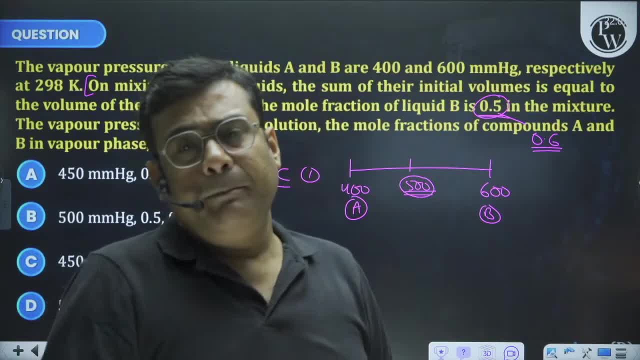 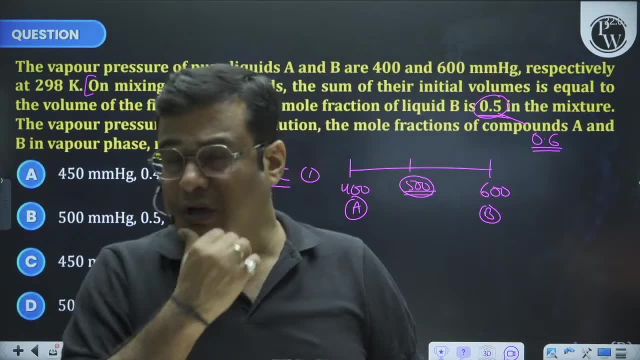 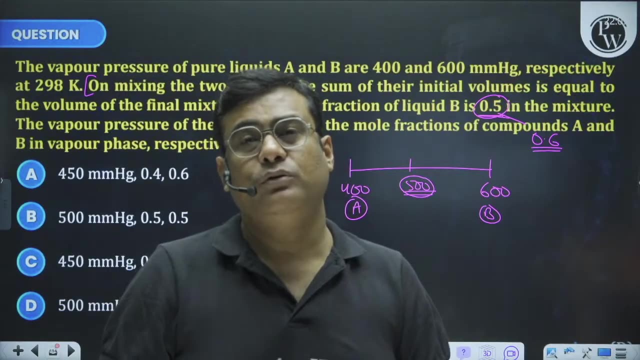 This is not a trick, son, It is the application of mathematics. I have 20 notes of 20 rupees and 10 notes of 10 rupees, So I have a total weighted average of 30 notes. Their weighted average. obviously, if both had equal notes, then the exact average of every note would be 15 rupees. 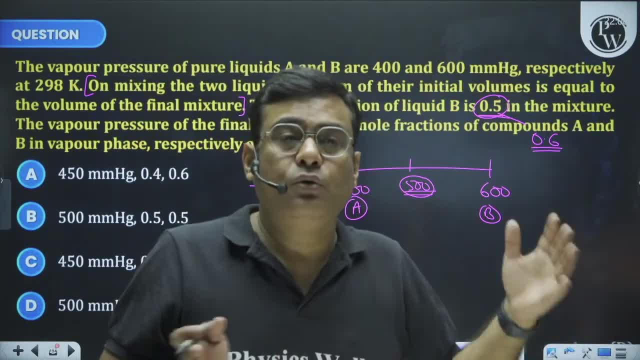 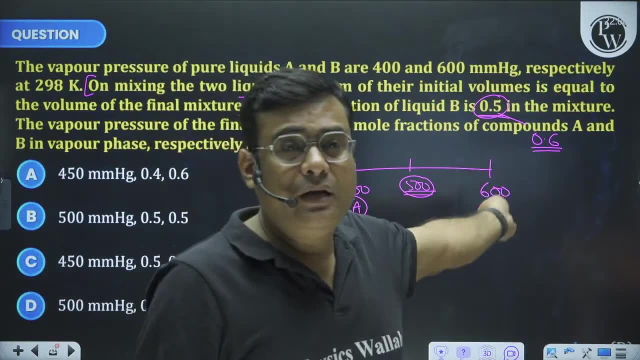 But if the notes are more than 20 rupees, then my total average will be more than 15 rupees, And if it is more than 10 rupees, then it will be more than 10 rupees. I am telling the same story here. 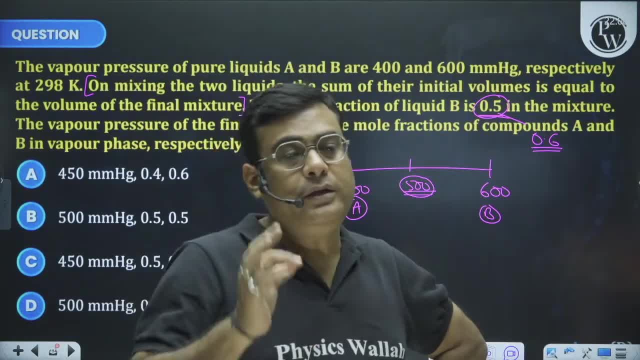 I am telling the same story, son, Isn't it? The thing is that those who don't feel that much mathematics, they think: oh, my God sir, then tell me the tricks of Kaltuki. This is not a trick, son. 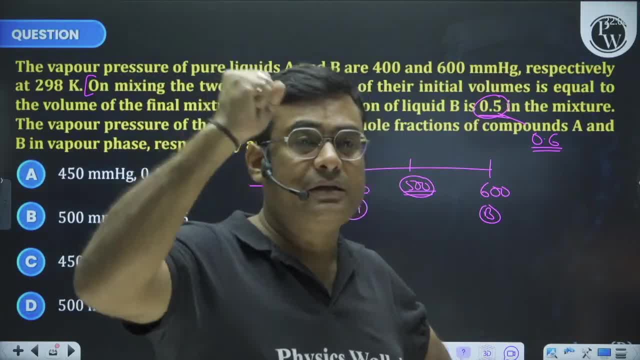 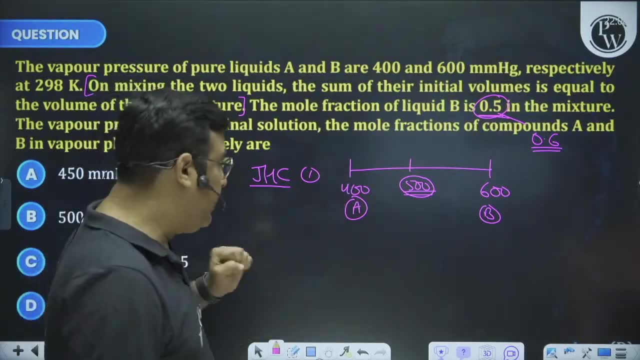 This is the power of your simple thinking and understanding of your mind, that can you think like this, Isn't it? This is the power of your thinking and understanding of your mind, Isn't it? Now the second thing, children. What is the second rule? The mole fraction of that component will always be more in the vapor phase, which will be more volatile, Isn't it From the liquid phase? In the liquid phase, the mole fraction of that component will be more than the liquid phase, which is more volatile. 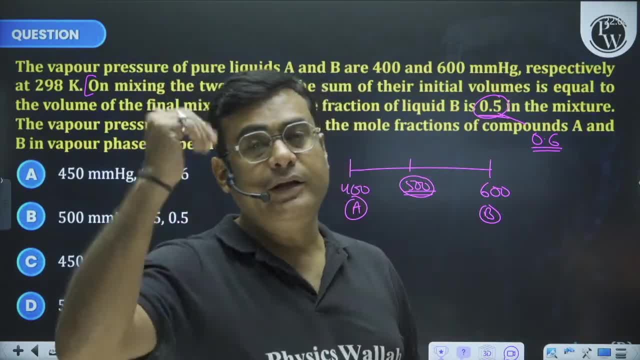 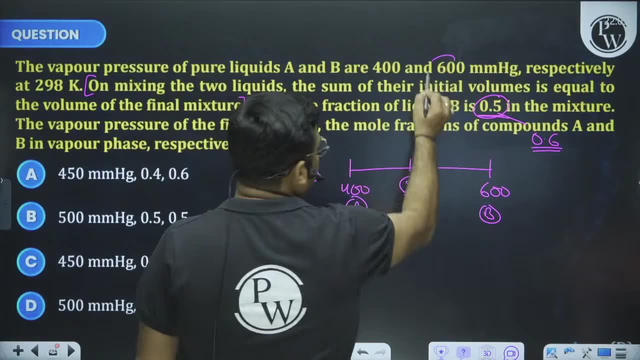 What does more volatile mean, son? The tendency to vaporize is more. The meaning of more volatile is that the tendency to vaporize is more. Okay, sir, Here B is more volatile. So if the mole fraction of B was 0.5 in the beginning, 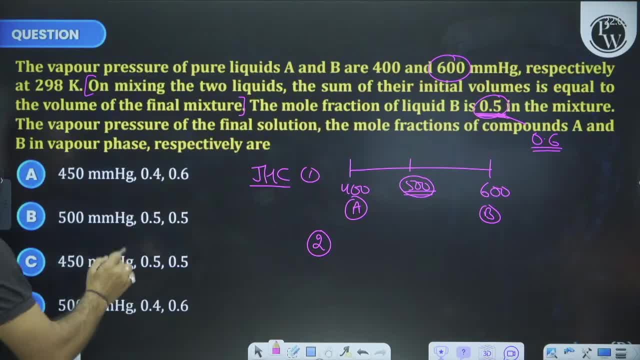 Isn't it? The first thing I am saying is that if there is 0.5 in the liquid phase, then there cannot be 0.5 in the vapor phase. Okay, If the answer had to be 500, then there was no chance of this happening. 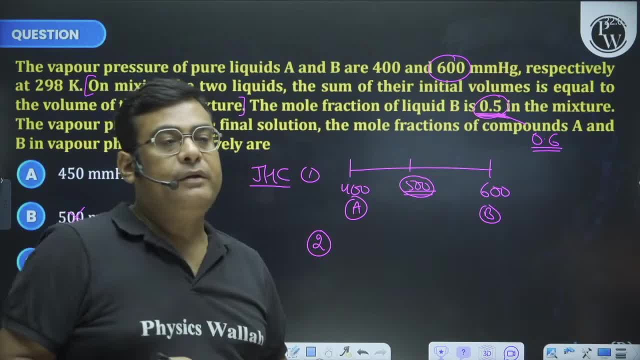 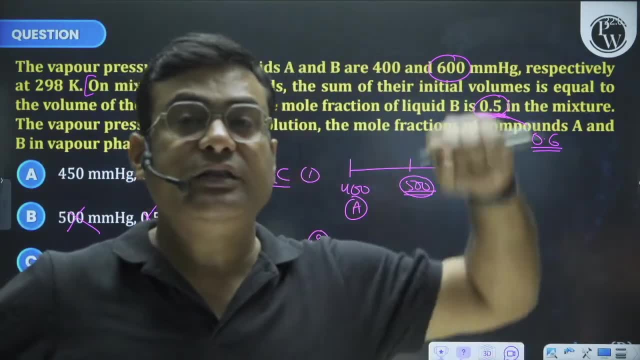 This was left, But I am also giving its logic: brother In the vapor phase, Isn't it? Isn't it In the vapor phase, brother? its mole fraction will be more than its liquid phase, which will be more volatile. 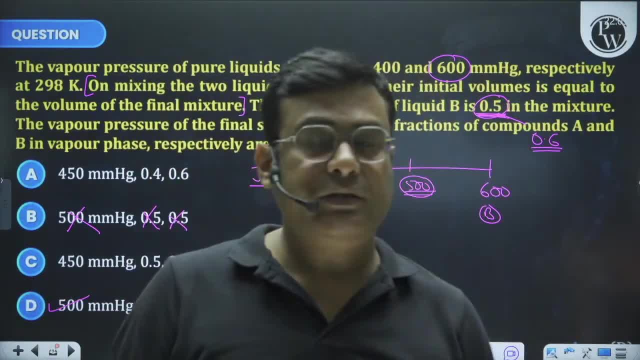 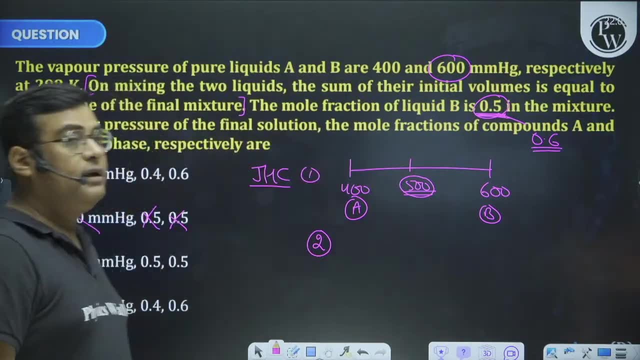 Because if it is more volatile, then its tendency to vaporize is more, Isn't it? If it is more volatile, then its tendency to vaporize is more. That's why, if the B was 0.5, then it will be more than 0.5. 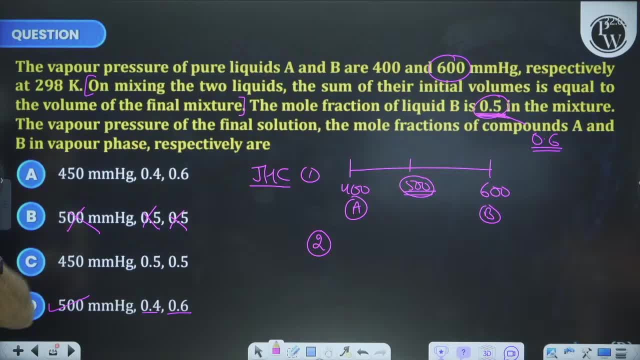 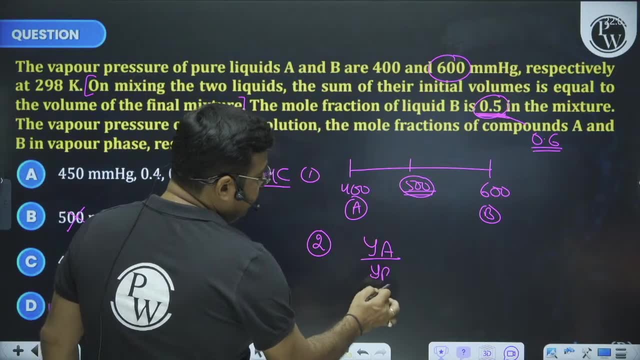 0.5 is more than 0.6 and this is less than 0.5. now may be, you have to calculate numerical value. so now I have said Y A upon Y B equals to P0 A upon P0 B, into X A upon X B. 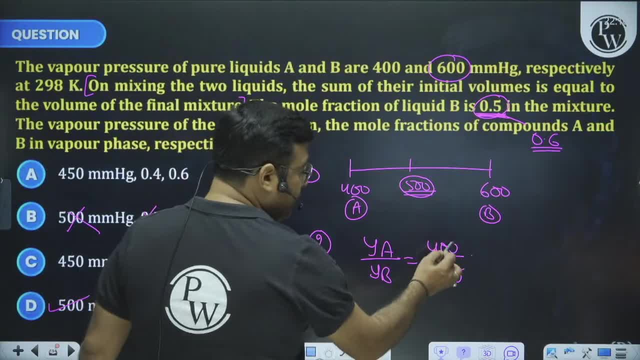 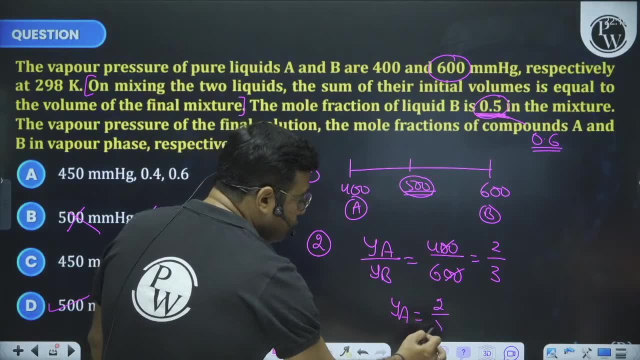 X A and X B are equal, there is no need to write them. this is cancelled. this is 2 by 3. if Y A upon Y B ratio is 2 by 3, then Y A value is 2 by 5. Y B value is 3 by 5. 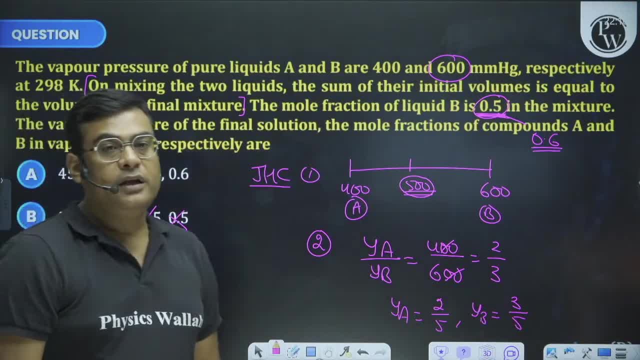 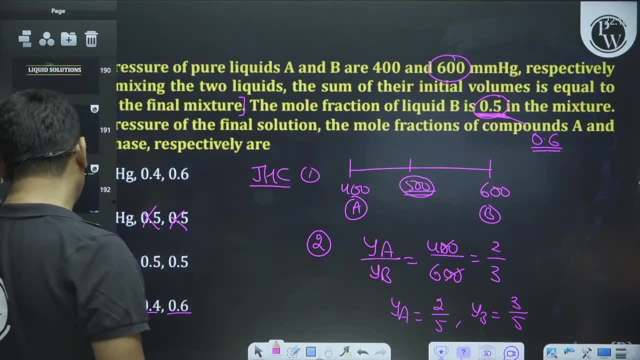 and 2 by 5 is your 0.4 and 3 by 5 is your 0.6. so please keep in mind my small short cuts means the work you will do will be easy. you will not face any loss. see in the next question I will not solve. 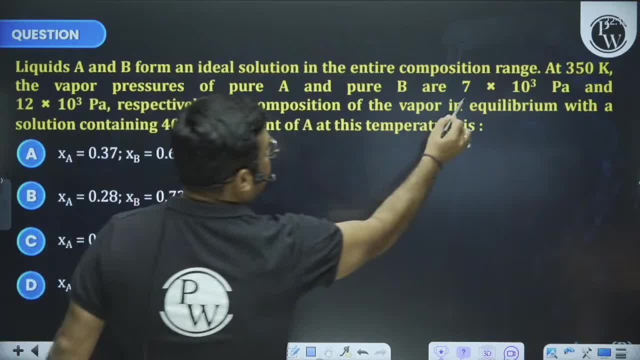 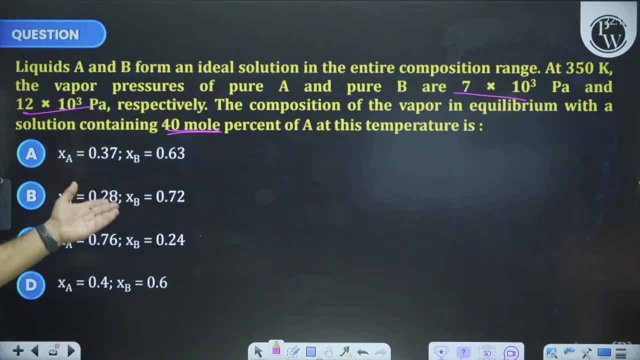 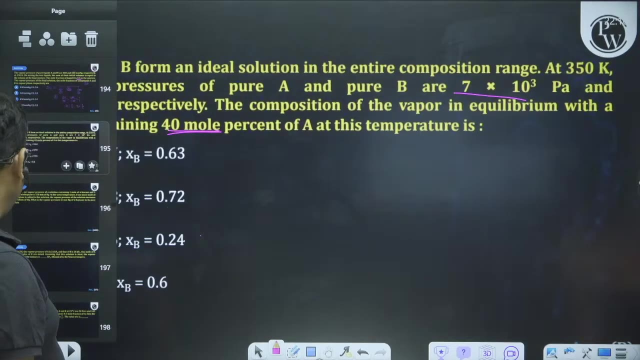 I am just telling you again: A is 7 into 10 to the power. this is the question. B: is this much composition of vapor in equilibrium in which A is 40%? again put my formula and it will be fun. thank you, it will be fun, it will be fast, otherwise in this kids keep on doing unnecessary calculation. 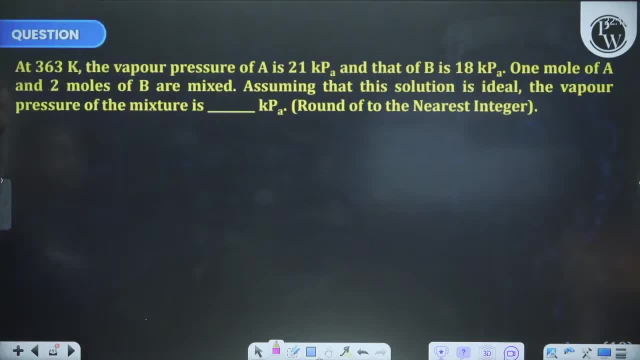 unnecessarily calculation. keep on doing. one more question: see vapor pressure of A: 21 kilopascal. B, 18 kilopascal. now it is saying 1 mole of A and 2 mole of B are mixed. assuming that this solution is ideal vapor pressure solution. now again such questions. 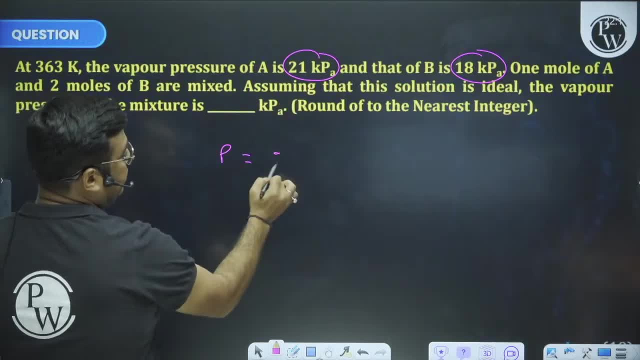 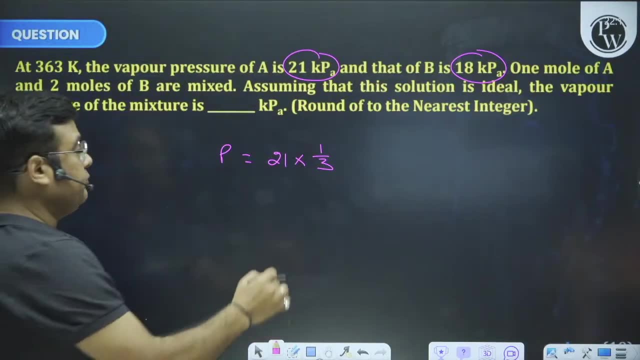 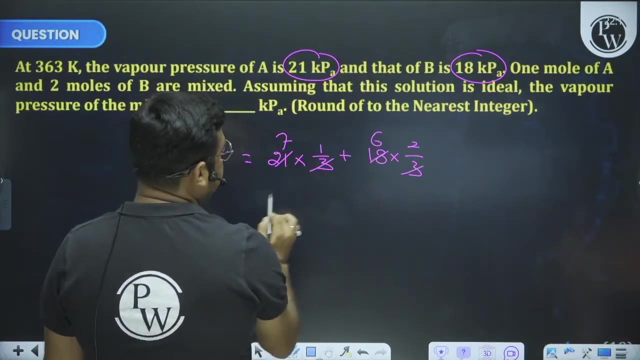 come: kids: P equal to P0 A, 21 into X A, so 1 by 3, because one of the 1 mole is 2 of B, so their are 2 moles plus P0 B18 into XB. this has become 7, this has become 6.6ст. Commonwealth: 12 plus 7, 19. same kinds of questions are coming opportunuges. 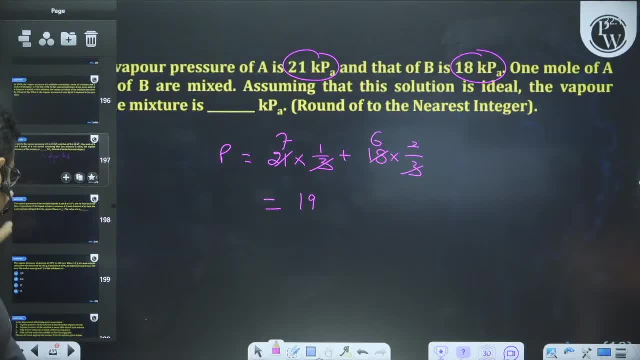 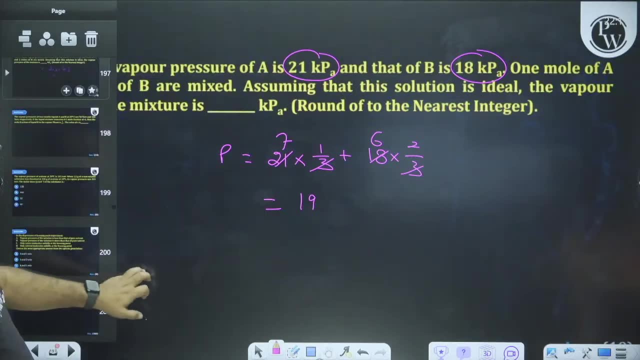 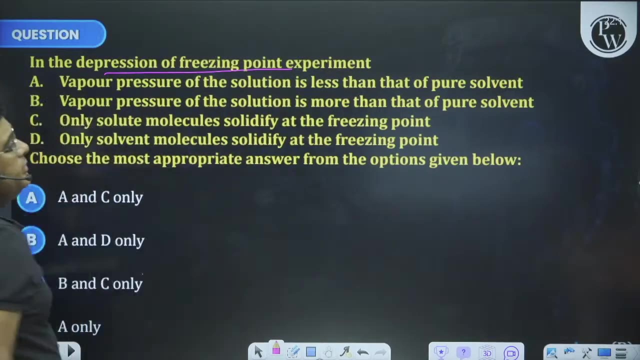 in JEE that we sometimes feel shy to get done sometimes comes out to us but do want to do, have to do. theoretical question. are you saying it is a theoretical question? vapor pressure has not yet The depression of freezing point experiment. vapor pressure of solution is less than that. 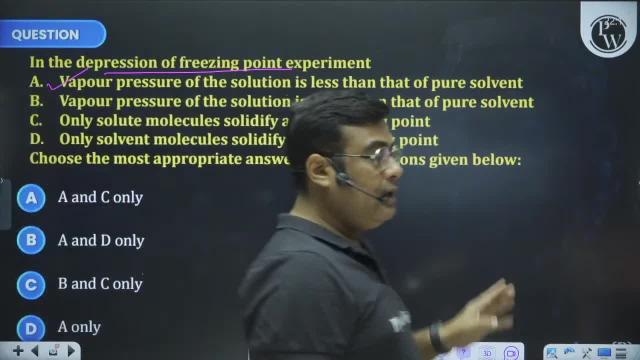 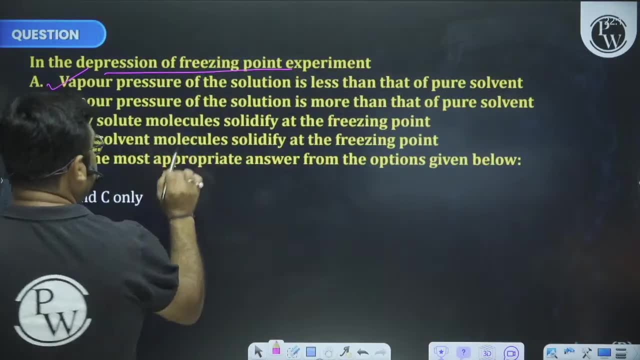 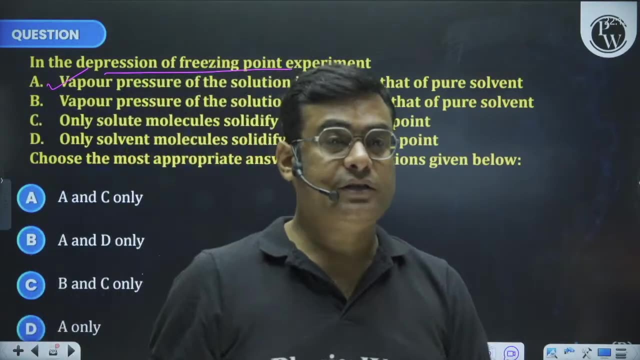 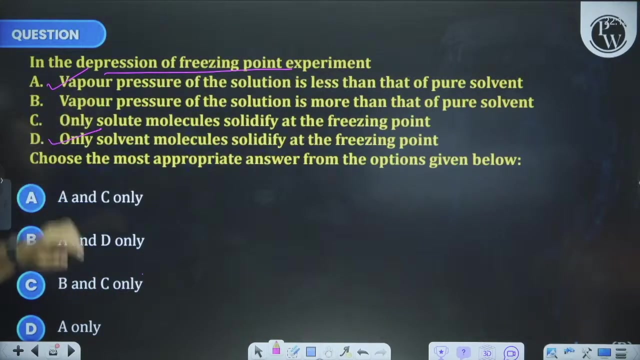 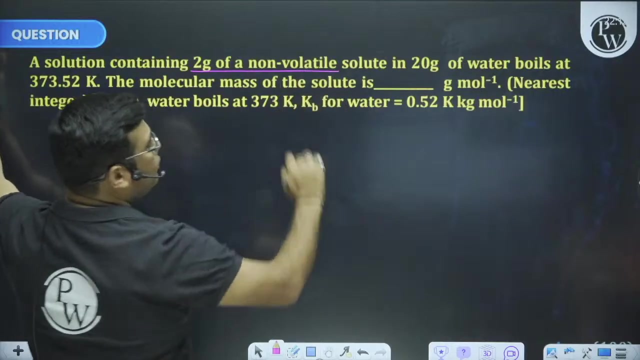 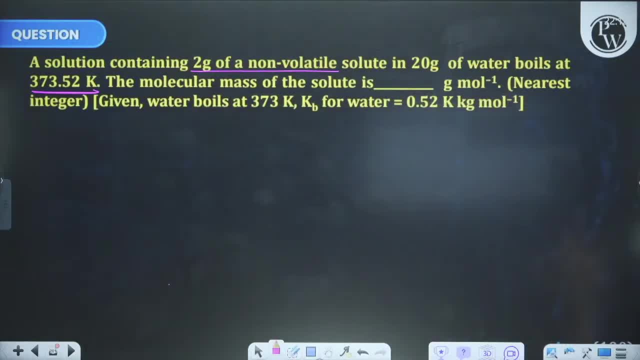 non-volatile solid will be added. its freezing point is what happens to the children? it increases. its freezing point increases from the previous one. it increases how much pure water is boiled at 373,. now he is saying: tell me the molecular mass of solid. so delta TB is 373, this is 373.52,. 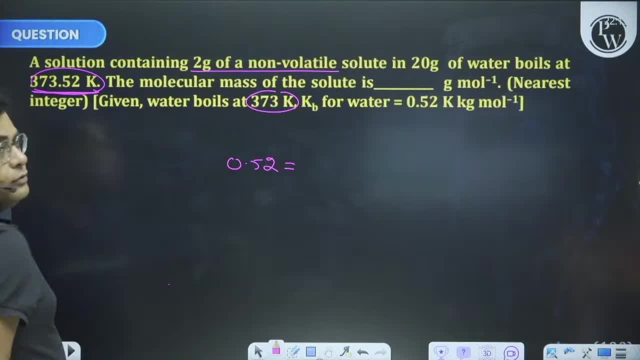 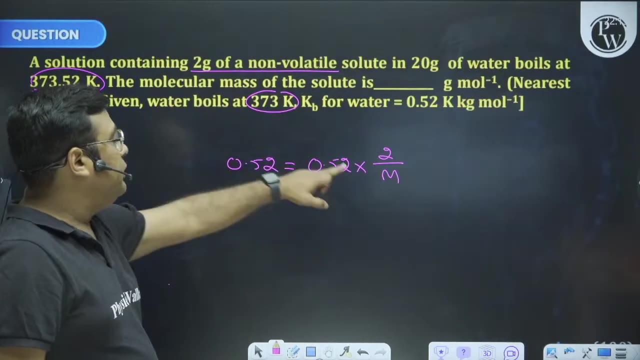 how much is delta? TB 0.52, equal to kb 0.52, see the data into molality. so the way to write molality. try to understand from me how to write. write immediately. take the two upon its molar mass down. 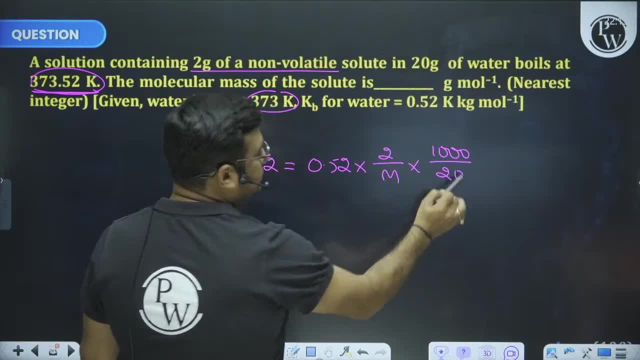 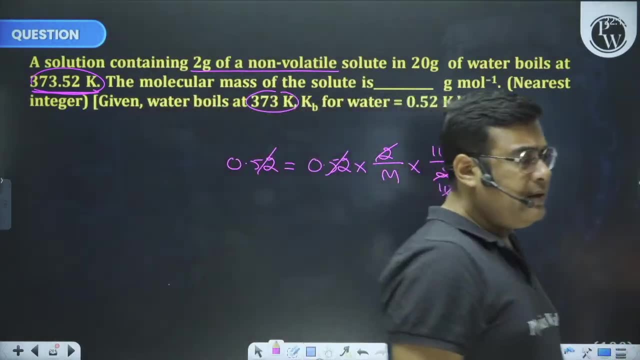 keep the thousand above and keep the water mass below. the story is over. this is the answer to this. 10 has been done. the answer is 100,. you see, If it takes more than 10-15 seconds, it means that something is going wrong. 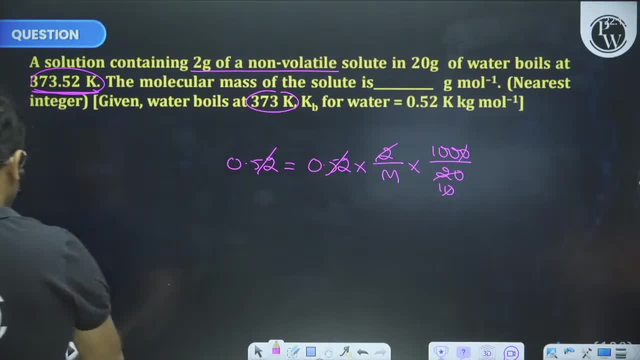 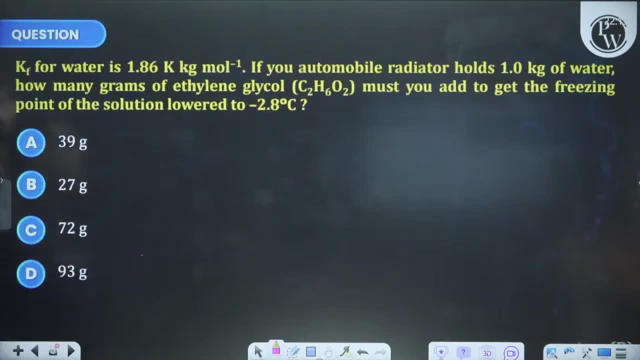 I said before starting the liquid solution, it is the most, most, most simple topic. Okay, let's reverse this. let's do a reading question and see KF of water: 1.86 Kelvin kg per mole. if your automobile radiator holds 1 kg of water, 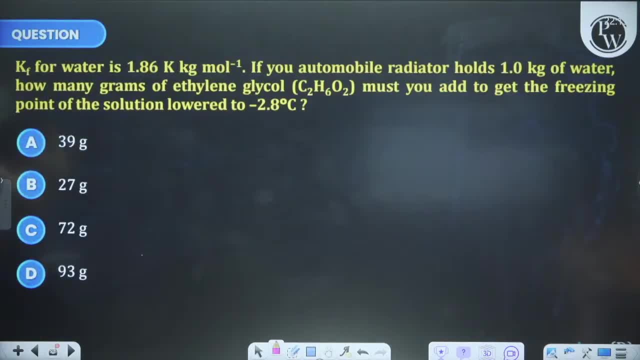 Now, if the water is 1 kg, then there is no need to write water. 1000 by 1000 is over. This thing should run in your mind. I just want to understand this: How many grams of ethylene glycol must you add to get the freezing point of solution lowered to minus 2.8 degrees Celsius? 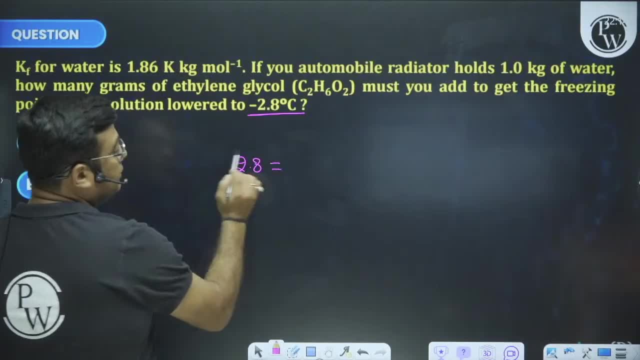 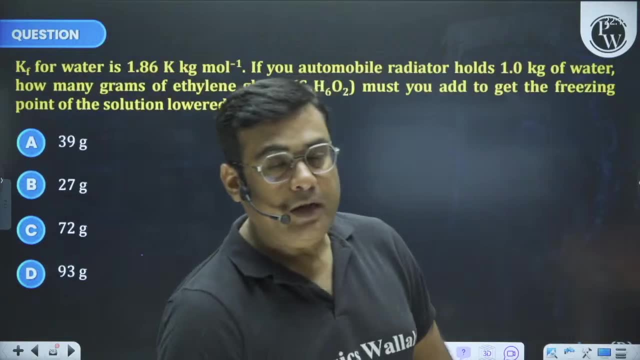 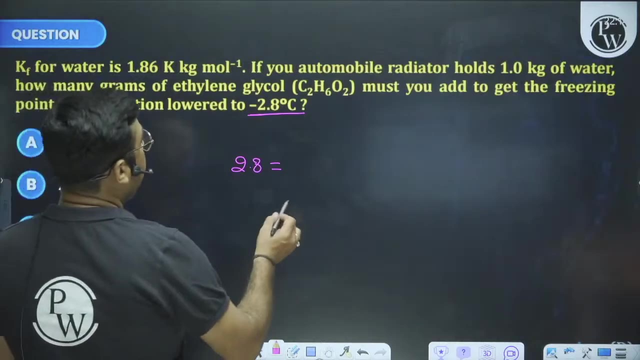 Brother, I wrote delta TF as 2.8, because pure water freezes at 0. Now I have added so much that the water is freezing at minus 2.8.. Equals to KF. KF is given as 1.86 into molality. 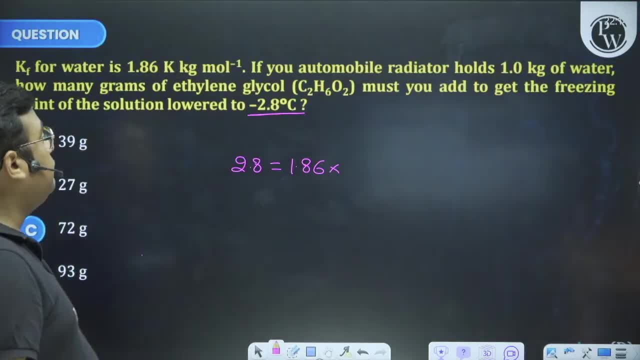 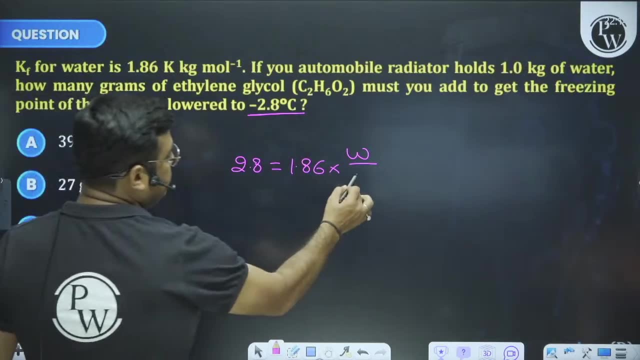 In molality. I have said that 1 kg of water is over KL moles. Now the mass of ethylene glycol is W and its molar mass is 62. If I am saying again and again, first remove the decimal by doing the same. 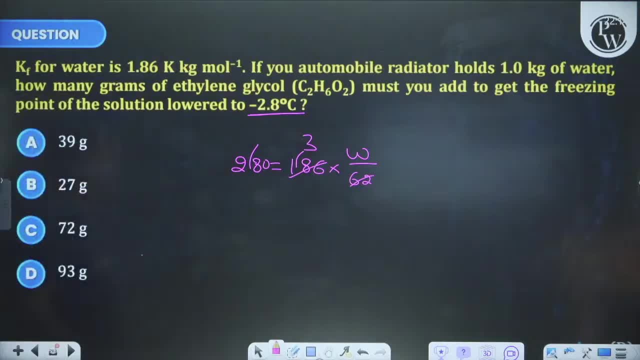 The triple of 62 is 186, so the value of W is 280. by 3 means 93.. Tell me quickly: are you sleeping or awake? Are you sleeping or awake? Are you attentive that everything is over? Tell me quickly, then only I will move forward. 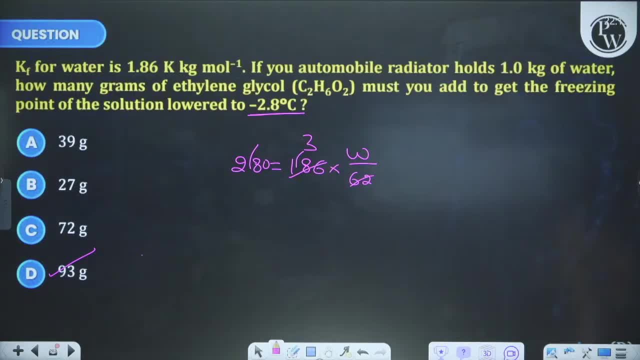 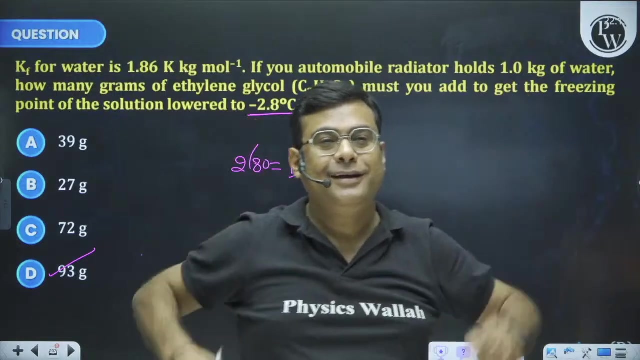 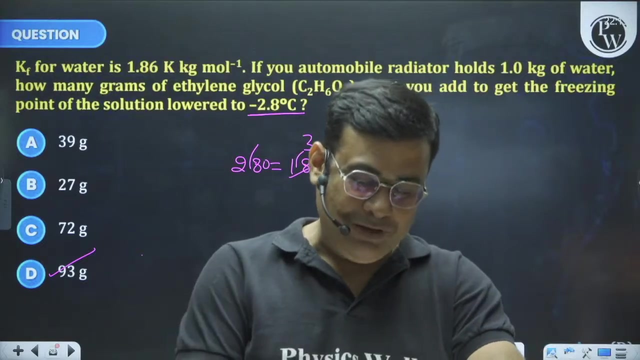 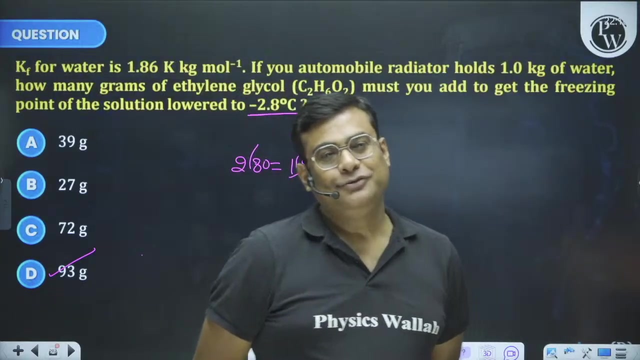 I am sleepy, I am very sleepy By getting sleepy, by cooking you. it is increasing more and more. Is there a song like this in your mind? Why, Son, it is not the time to sleep? If you have to sleep, then the one who sleeps is the one who is lost, and the one who is awake is the one who is found. 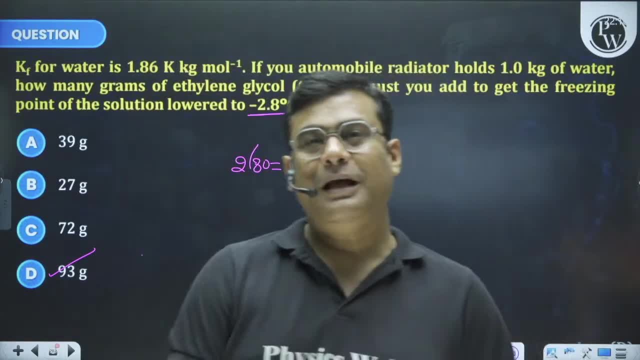 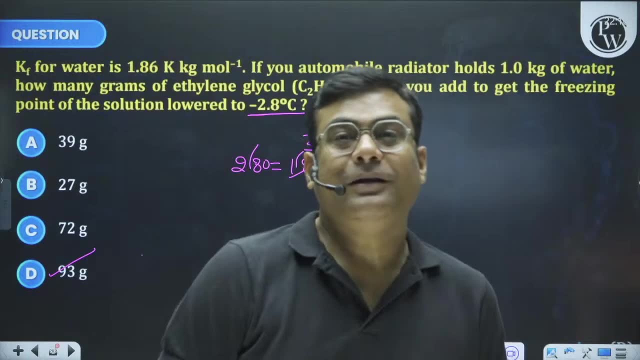 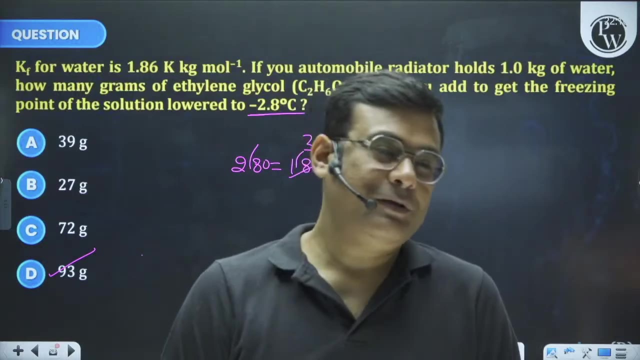 You see your hard work, see the hard work of the masters, Son. you must be sitting and studying somewhere comfortably. These masters, who are getting old, son, they too are attentive and are attached to you with the same energy. We do not want to work hard and we see the dreams of all. India, rank one. 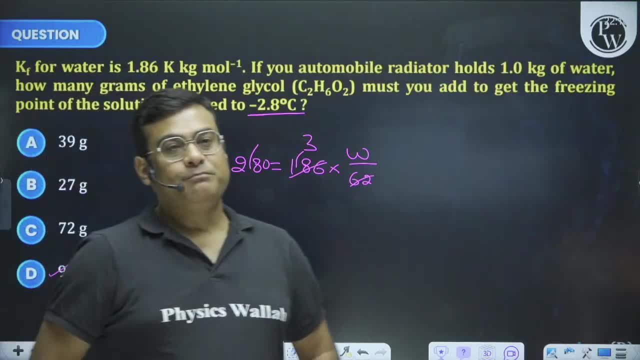 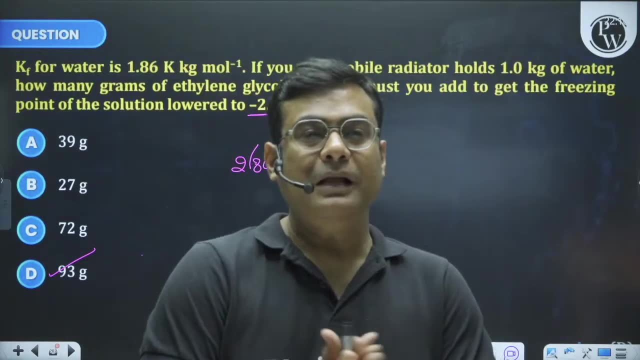 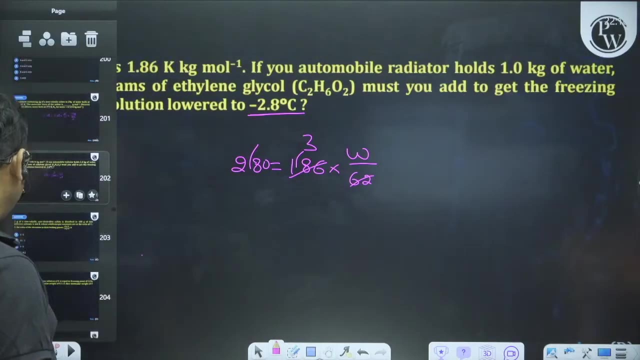 So that's where the story gets messed up. That's where the story gets a little messed up. That's why we go back a little bit. So you have to keep it safe. So in liquid solution I think children see more questions. 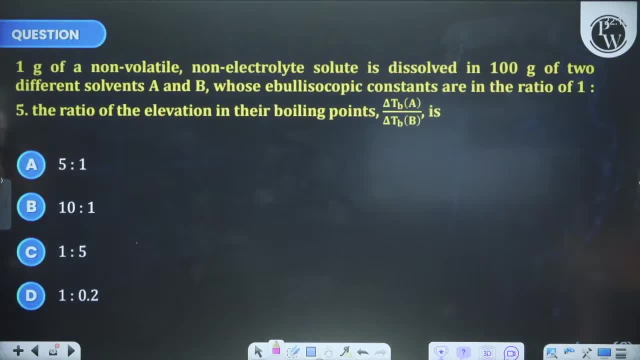 This is a simple question. See: One gram of non-volatile, non-electrolyte solute is dissolved in so gram of two different solvents, A and B, whose biblioscopic constant are in the ratio of 1 is to 5.. 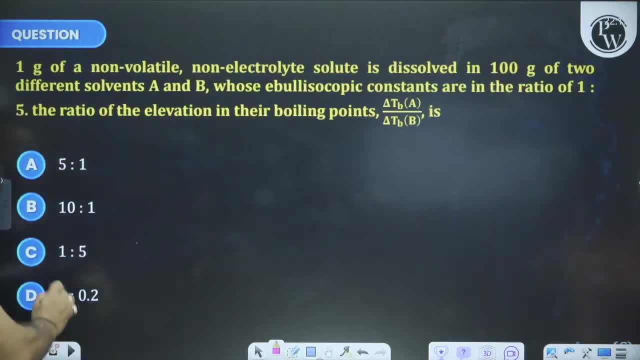 The ratio of elevation in their boiling point 1 is to 5.. Why? Delta T is also equal to KB into M. Wow, nice ginger tea has come. It was cold anyway. So delta TB is equal to KB into M. Now M is the same. 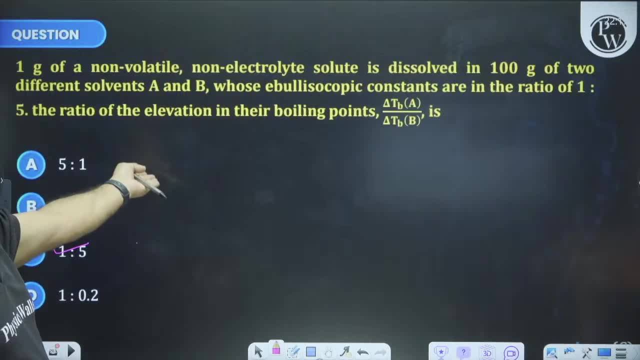 The mass of the water is fixed, the mass of the solute is fixed, So MM has been cancelled. That is, the ratio of delta TB has become KB directly. The ratio of delta TB has become KB Son. I am drinking tea. 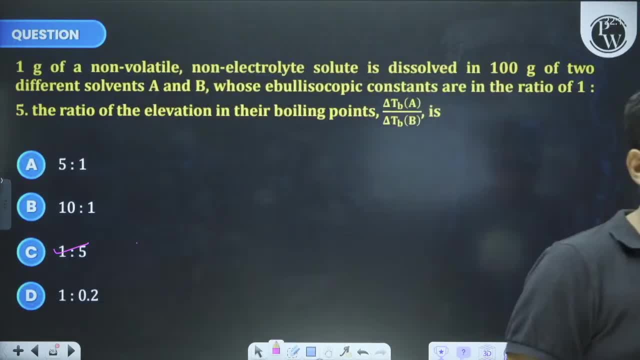 I am not eating anything. Where will I eat? I am drinking tea. My mouth is running like this, Your mouth is running like this. Okay, So in this way, students understand these things, Understand, understand. Now see, I will also tell you the next question orally. 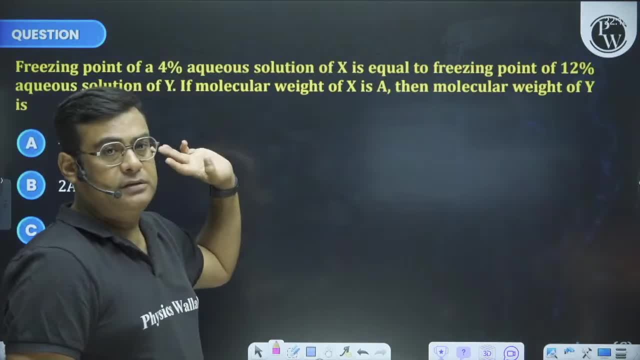 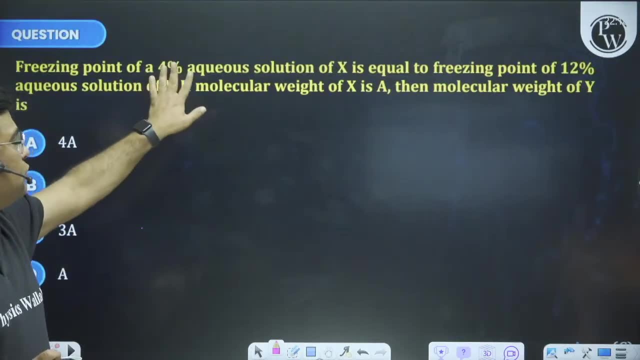 Frithing point of 4% aqueous solution of X is equal to frithing point of 12% aqueous solution of Y. Now, which is in percent, is not given. It does not even mean: If molecular weight of X is A, then molecular weight of Y 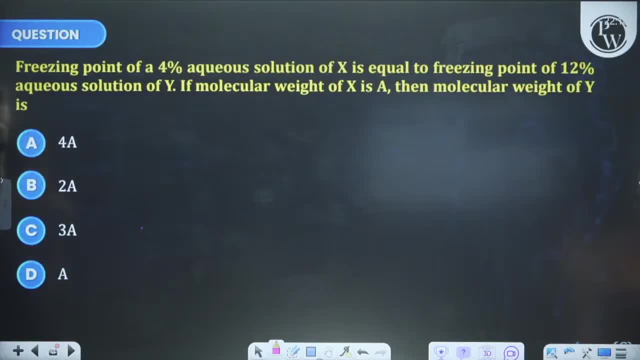 If both the freezing points are equal, that means both the molarity should be equal. That means if this is 4% and this is 12% and it is 3 times, then if its molar mass is A, then the next one's molar mass should also be 3 times. 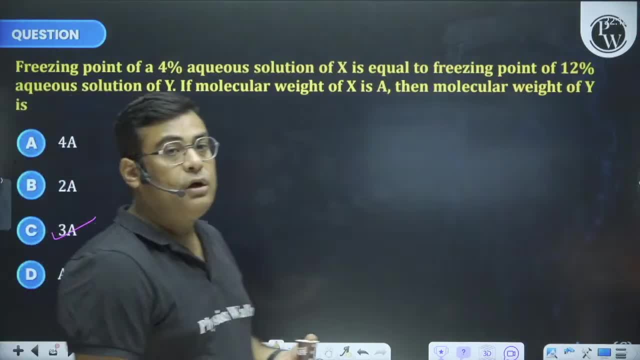 That means it should be 3A. There is no need to write anything and solve it. There is no need to write anything and solve it. And all of these are the questions of your JEE. All of these are the questions of your JEE children. 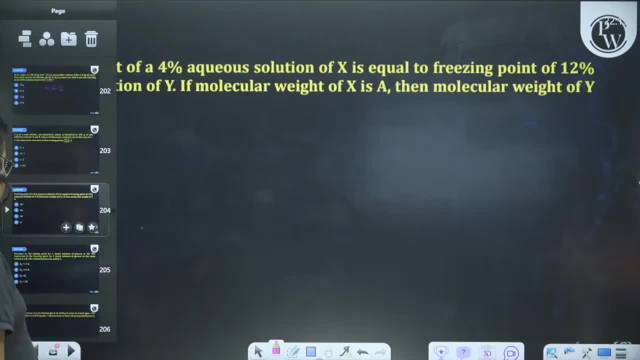 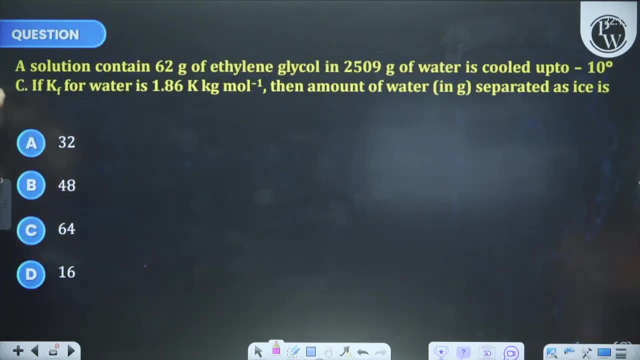 So this is what I am telling you: that questions are made very easily and with confidence. There is no problem. If you have any questions, then definitely tell me about the ice question. I like the ice question very much. In this, one thing is wrong. 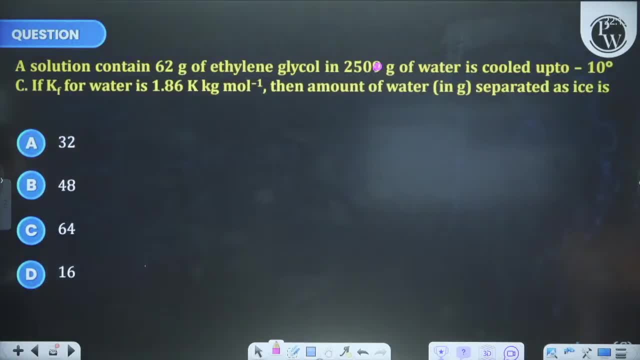 It is not 2509, it was 250 grams. Okay, sir, I did not understand the previous one. I will explain it again. son, There was a 4% solution and there is a 12% solution. Both the freezing points are the same. 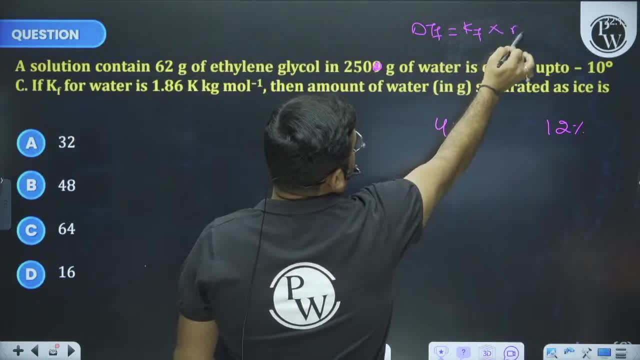 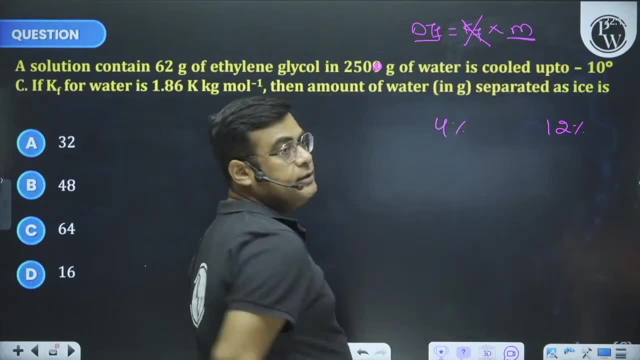 Brother, delta TF is equal to KF into M, Right? If the solvent is same, then KF is same. If both the delta TF is same, then both the molarity should be the same. Now for the molarity to be the same. 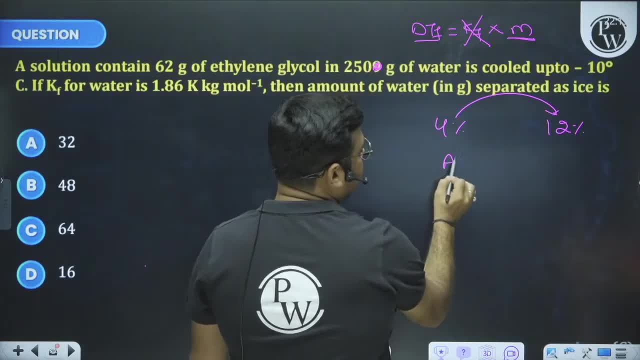 now for the molarity to be the same. now for the molarity to be the same. if it is three times, then the molar mass of one was A, So it will be 3A. Only then the molarity of both will be the same. 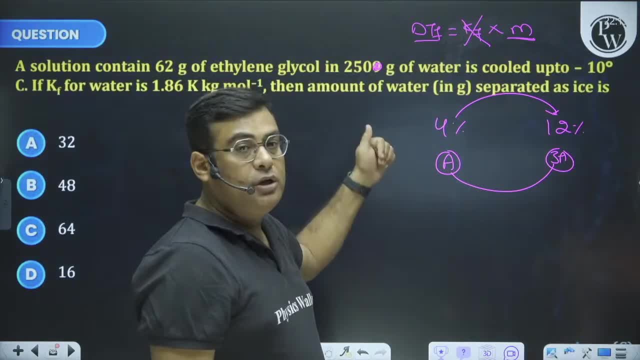 What will you do in the molarity? You will keep the mass above and the molar mass below. So 4 by A is equal to 12 by 3A. So this will also be 4 by A and that will also be 4 by A. 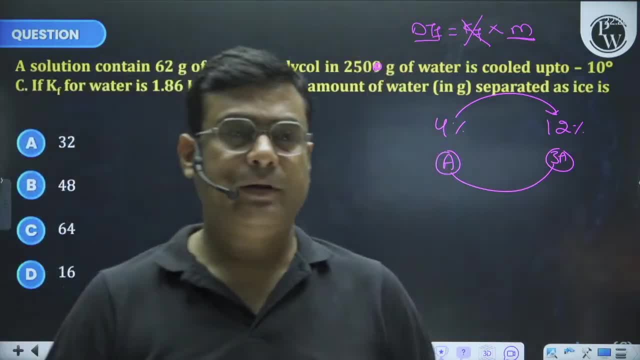 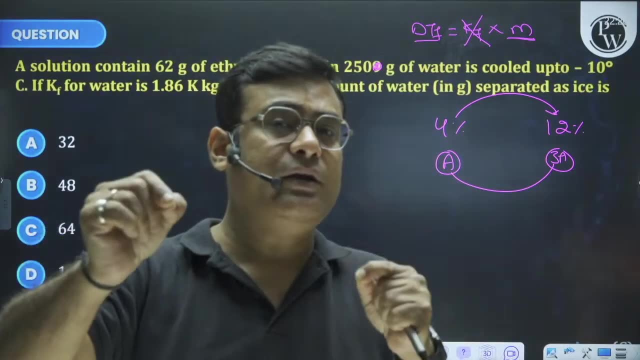 The story is over. You will have to think a little. from the brain, son. I am not saying that. do this in the exam, Do it by writing in the exam. But while writing, as soon as you write, your brain will break automatically. 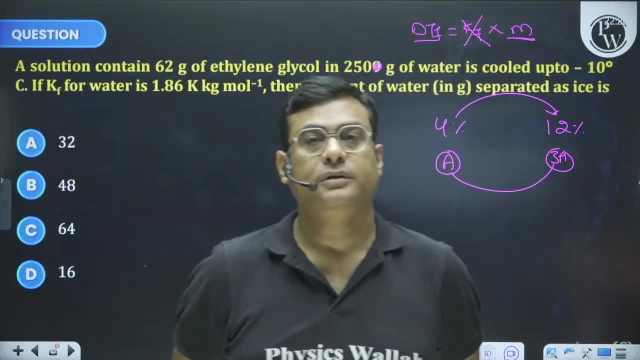 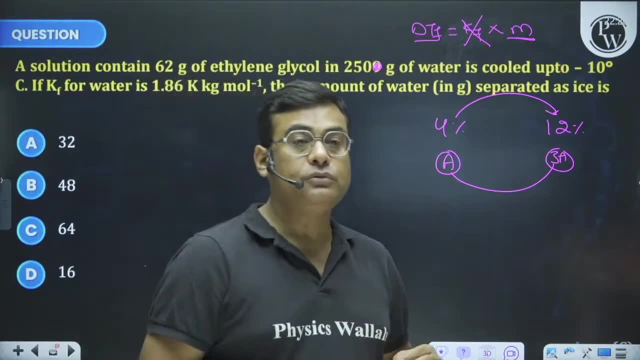 It will start thinking that I have done this kind of thing. That's why I have come to teach you that approach. I have come to teach you that approach from which we can think things. Okay, Now look at this question. I consider the question of ice to be very important. children. 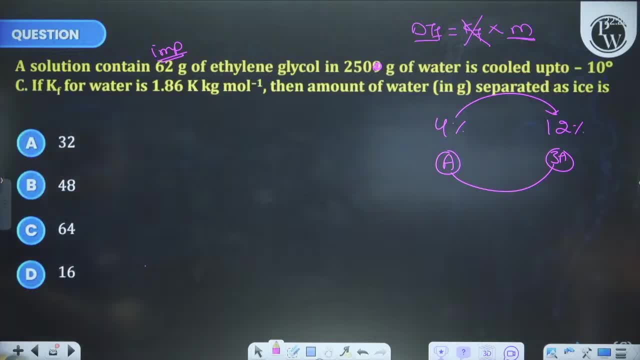 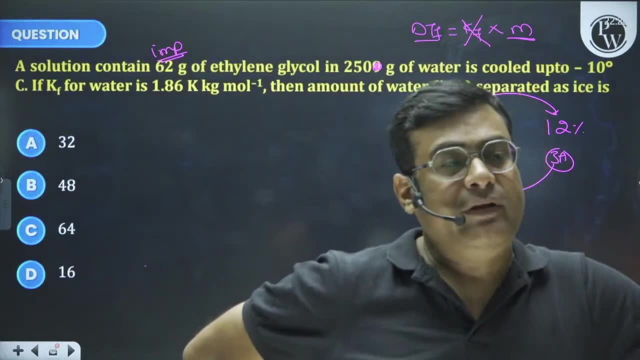 Let me tell you from now, Understand the concept of this. Tell us all, son. In cold days, there are many countries like this, where the temperature goes down to negative. So how does the aquatic life survive there, Isn't it? 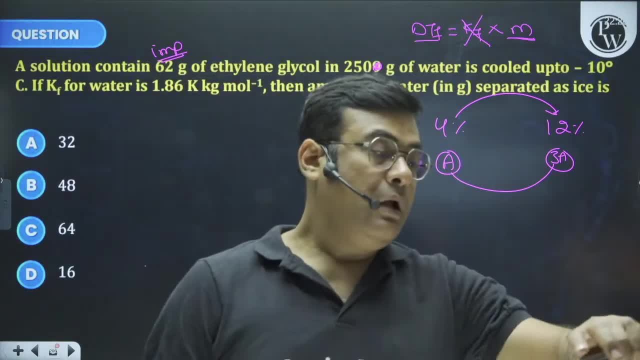 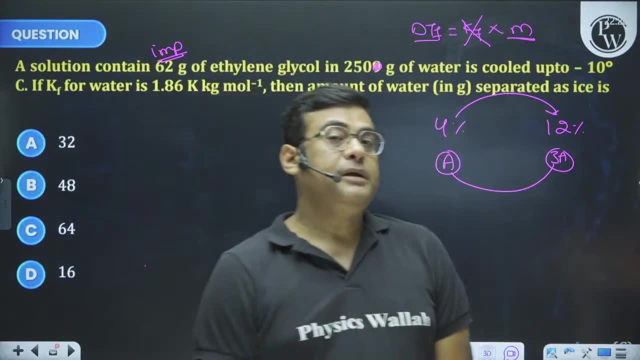 Because if the temperature goes down to negative, then the water freezes at zero And the water freezes at zero. So it means, brother, whatever the whole river and lake should be sub-freezed, Then the aquatic life will end. How is it possible? 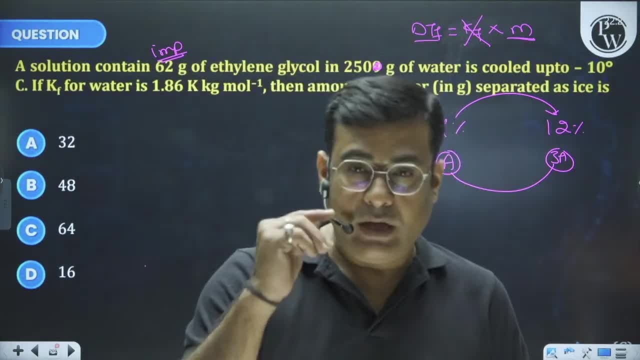 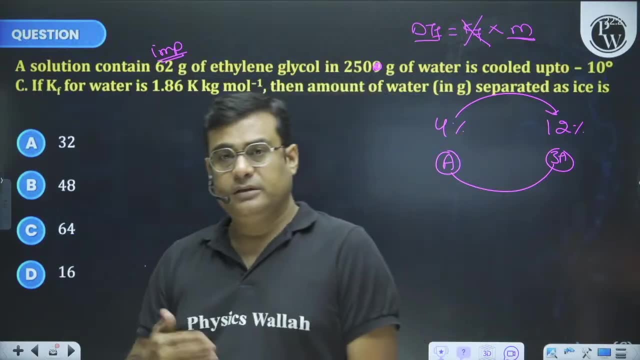 Tell me, Isn't it? There are two reasons for this, son. The first reason is that, whatever water is in the rivers and lakes right now, like I went to Goa for 5-6 days on vacation in March, Many of you have also gone to Goa. 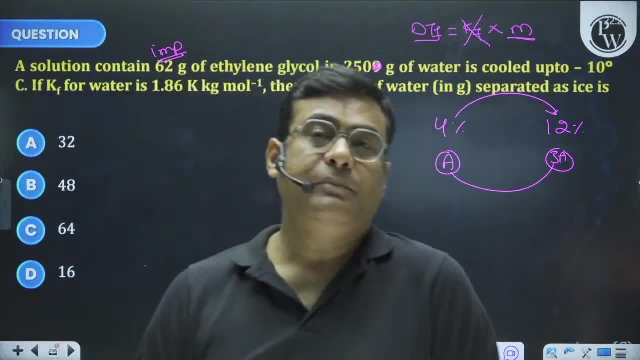 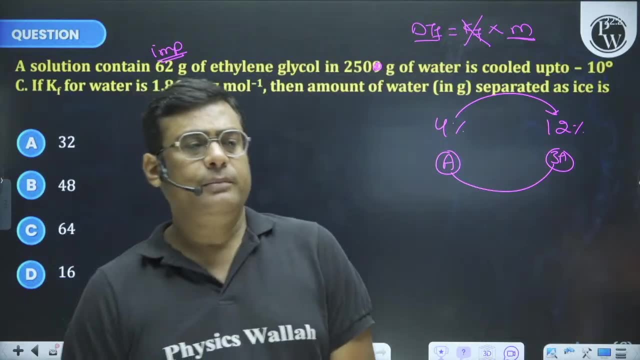 I have gone to Goa for vacation. I have gone to Goa for vacation. You must have also gone to the beach somewhere. So why am I talking about Goa? To tell you that I went to Goa? No, When we go to Goa, son. 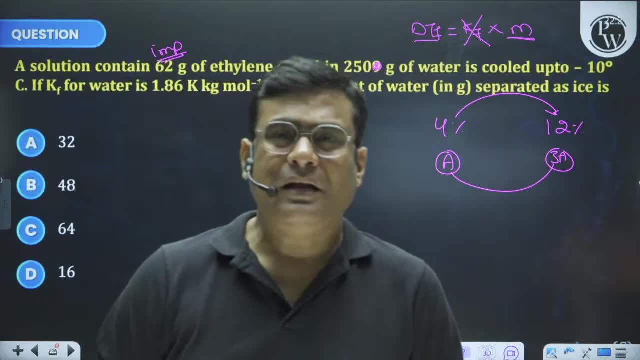 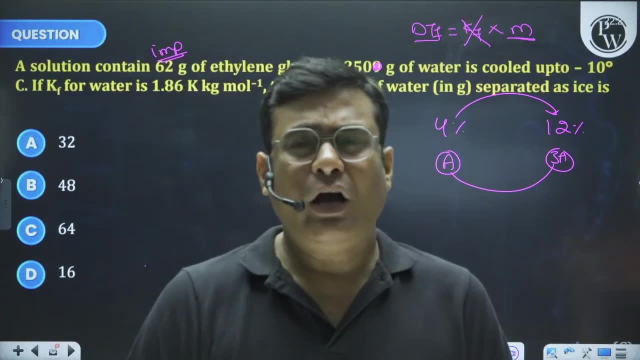 when we go to the beach to bathe, then the water that goes to the beach in our mind, isn't it? It makes our face dirty with salt and weird And we get angry That I wish this water was pure, Isn't it? 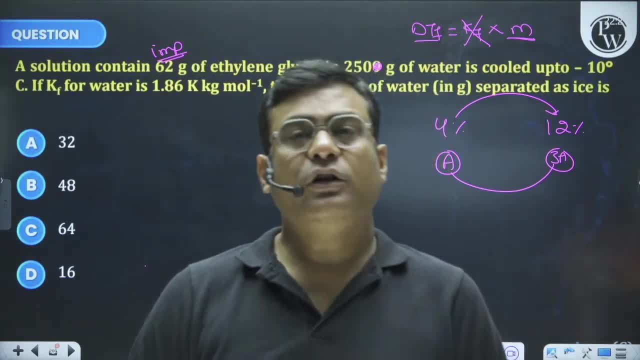 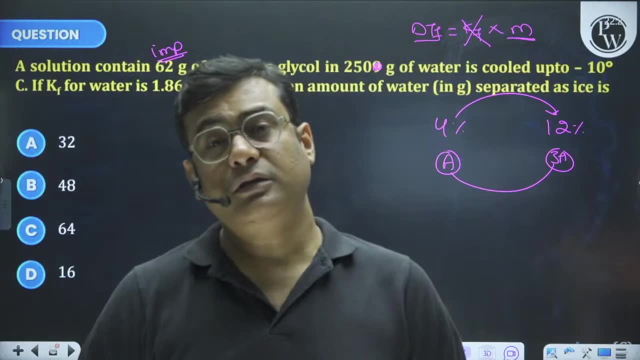 Like swimming pool, the good swimming pool of the hotel. the water in them is pure. It is crystal clear. There is no salt in it. There is no salt in it. So we think I wish this water was also pure like this. 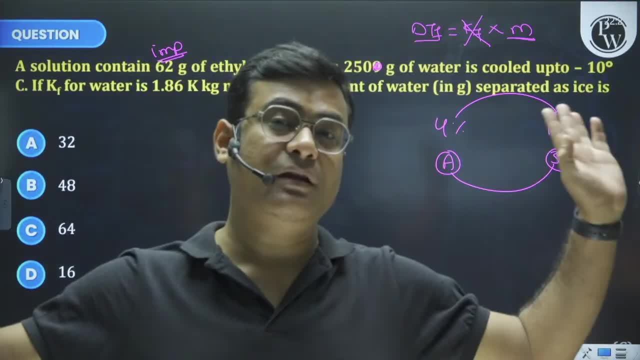 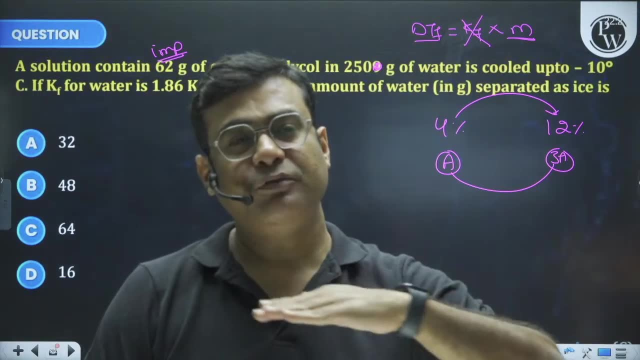 It would have been fun. We stay in the beach all day, right By the sea. But, son, if that water had been freezed, then it would have frozen completely as soon as it reaches a negative temperature from zero degrees Celsius, And on the contrary. 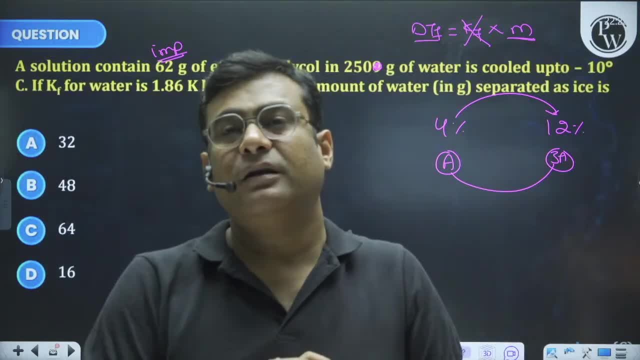 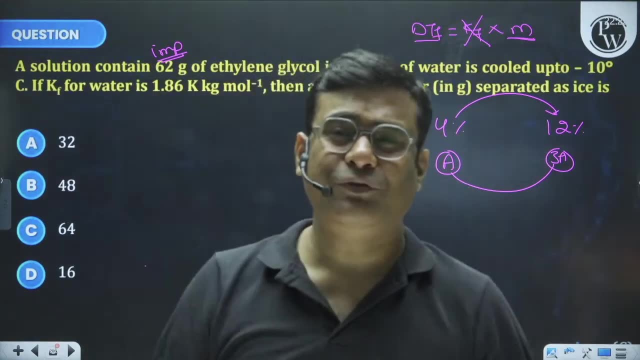 all the aquatic life in it, whatever it is, whatever is inside- there is fish, there is trout, there is turtle. whatever it is, it is not a turtle but in general, all the seafood in it. all of them will die. 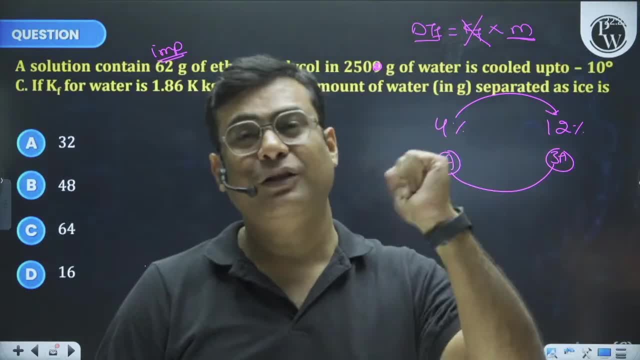 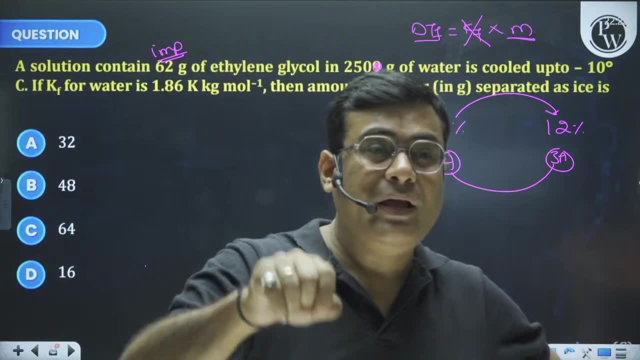 And if they die, then the water will get dirty with the smell. So that salty water is there, son. Because of that salty water, salt is added in it. That is the reason that its freezing point is less than zero. It means now: 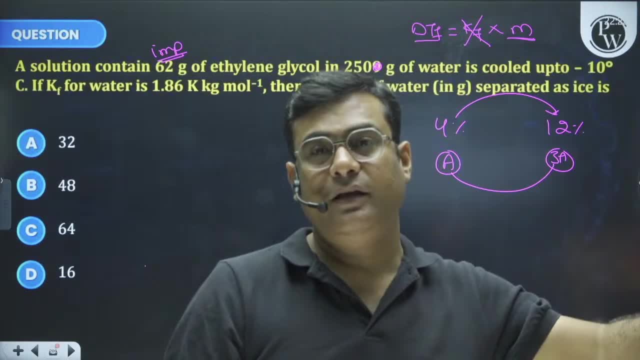 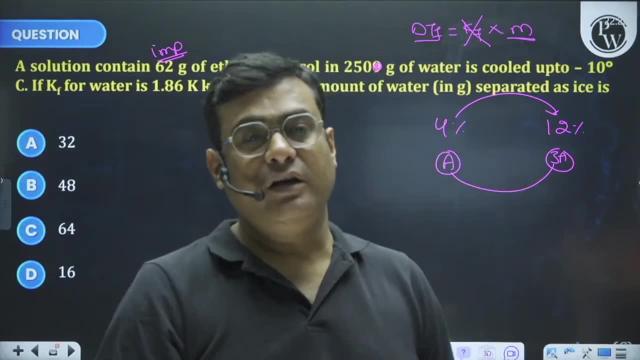 it is not being able to freeze in the negative, Okay. And it is not being able to freeze in the negative, Okay. Because of this, aquatic life can survive. First thing: Right When you see the water in the freezer, right? 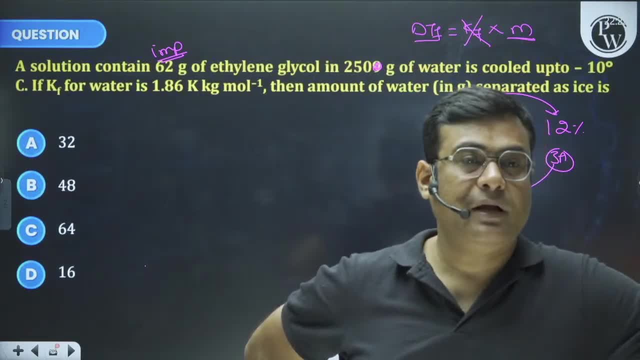 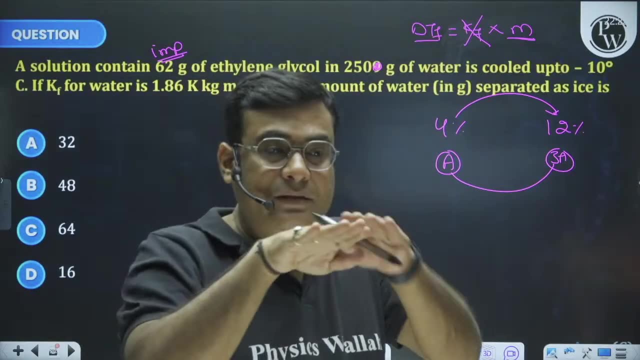 If you have kept the water in the freezer, then the water does not always freeze straight. You must have seen the papdi being made on the top. First the water freezes on the surface which is freezing, Then it freezes on the sides. 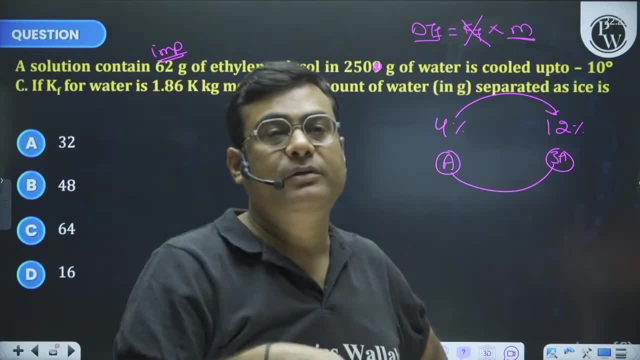 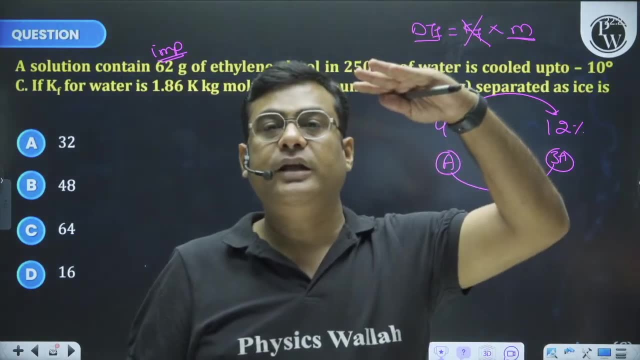 In depth, it freezes later. In depth, it freezes later. And you must have seen many such movies in which, brother, on the top there is a thick layer of ice, but somewhere there is a weak point: The hero and heroine. 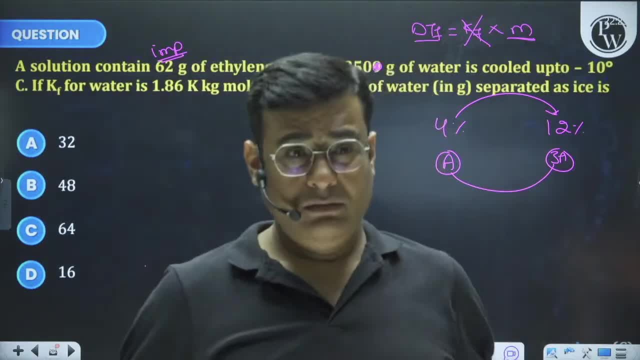 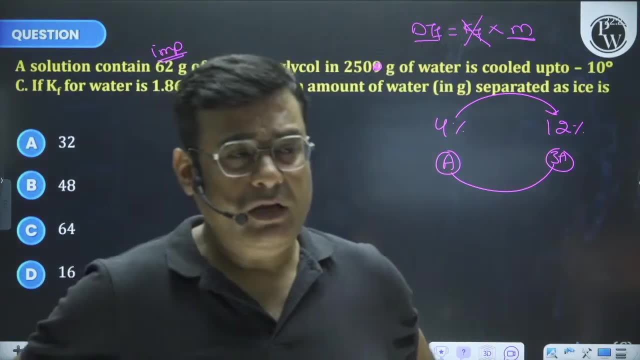 get stuck in someone's feet and can't get out. You must have learned many such things, children. You must have seen. So make them feel that only brother right, Only while watching movies. brother right While watching movies. 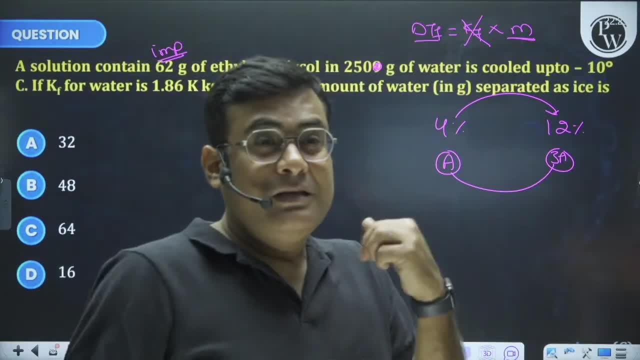 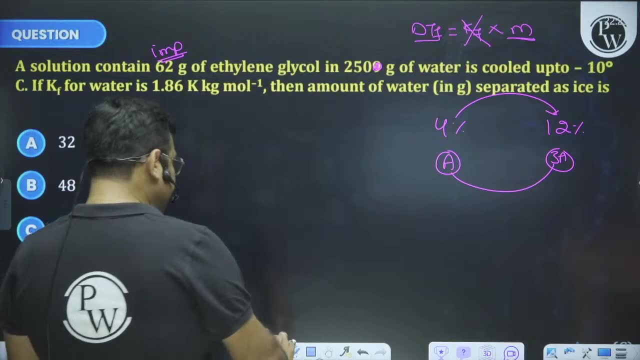 your mind entertainment. I knew that you will get the name immediately, right, Sir? you live in Omkothari. this also came. Someone found something from somewhere In the middle. these things can be learned. We should pay attention. 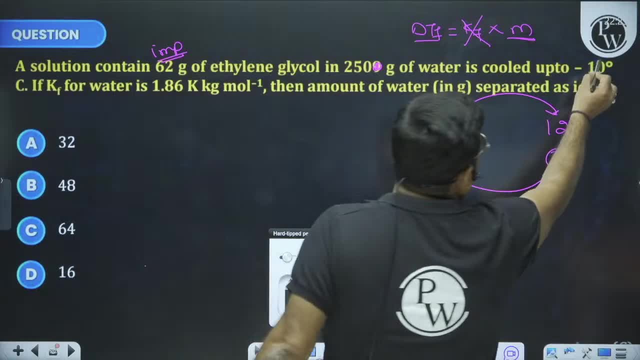 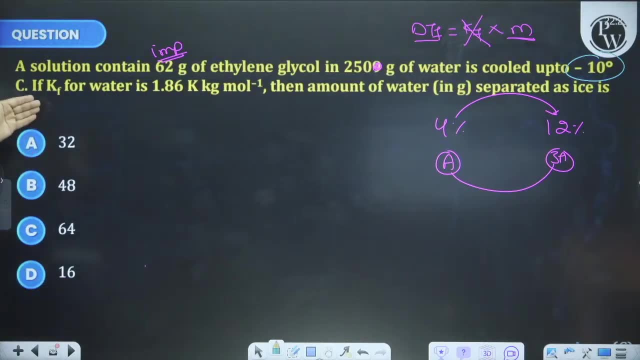 I am saying the same. Now see, he has said that the water has cooled down to minus 10.. If the KF of the water is this much, then tell me the amount of water separated ice. Now you can see that there is no. 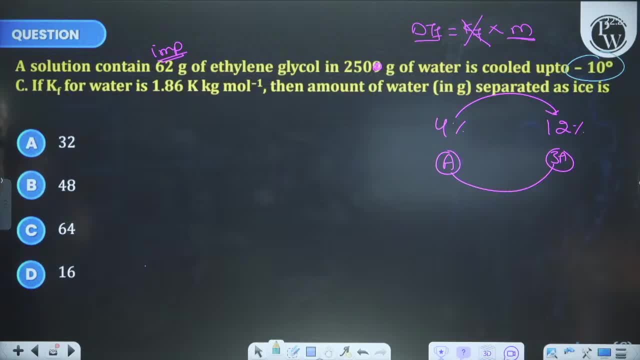 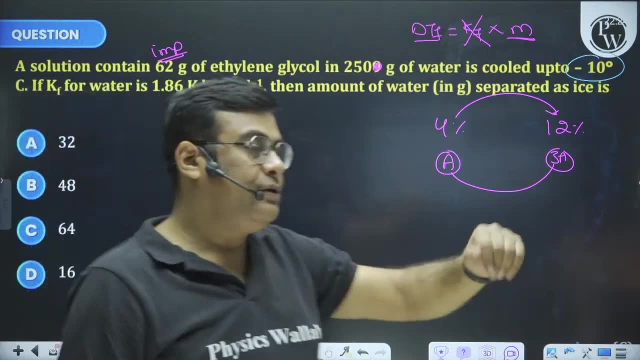 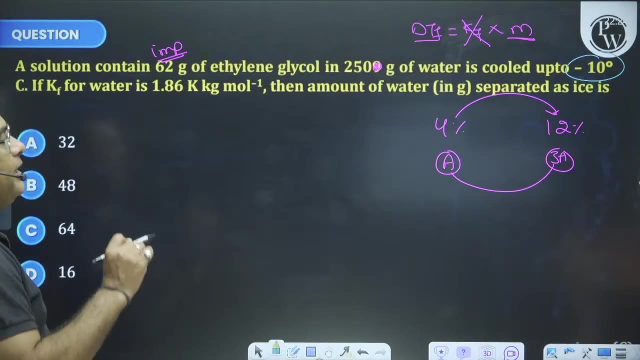 answer below 250,. son, That is the entire water has not been frozen. Entertainment dog. I knew everyone will remember because your memory is fast everywhere Except studies. your memory is very fast in other places. So, brother, I hope the question. 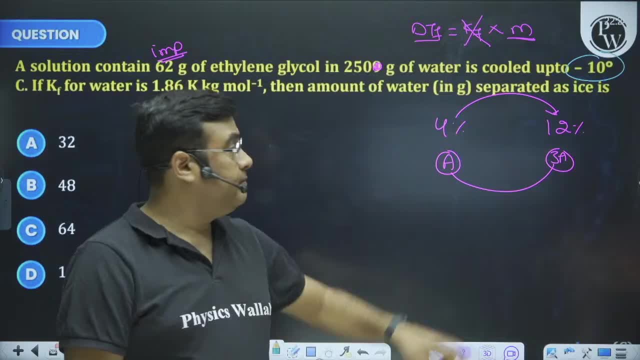 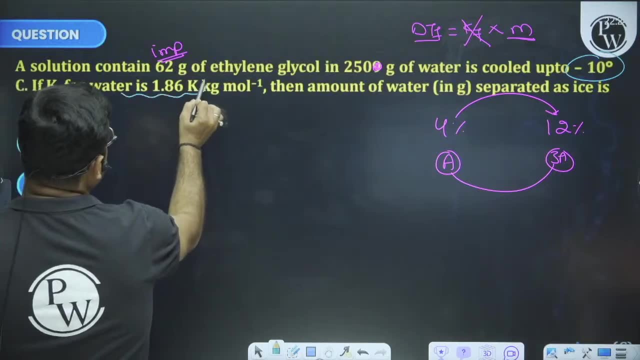 of freezing of water. I have explained the concept to you. Now how do they do it, Brother? if KF is seen, son, if KF is seen somewhere in the paper of JEE of physical chemistry, then there is no formula. 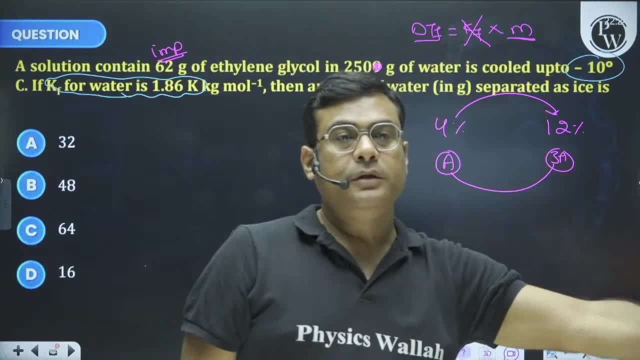 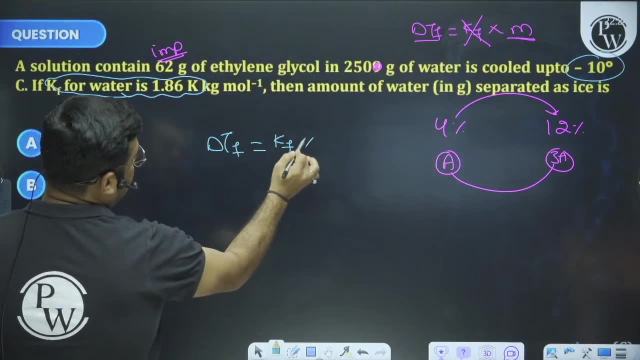 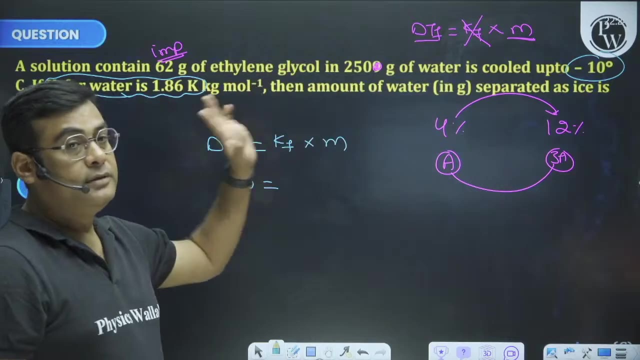 of the world other than delta TF equal to KF into M. Right, There is no formula, So you still have to use KF into M. Now, how much to keep delta TF? Keep 10.. How much to keep delta TF? 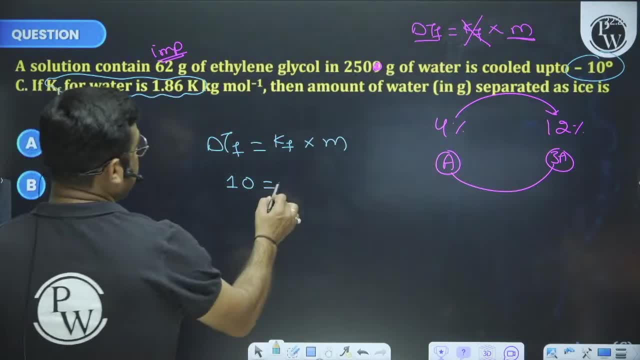 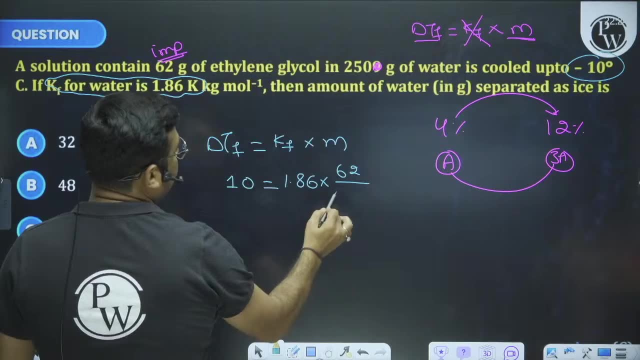 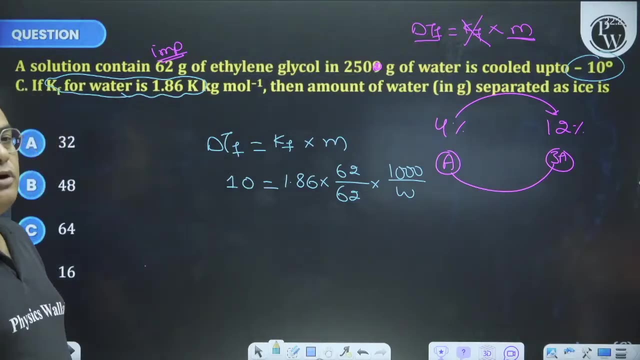 10.. You are assuming that we have taken it up to 10.. Equals to KF 1.86 into molality. For molality, I just said 62, mass of solute upon its molar mass is also 62.. 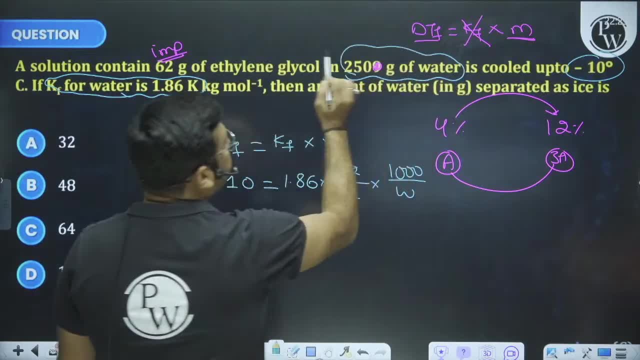 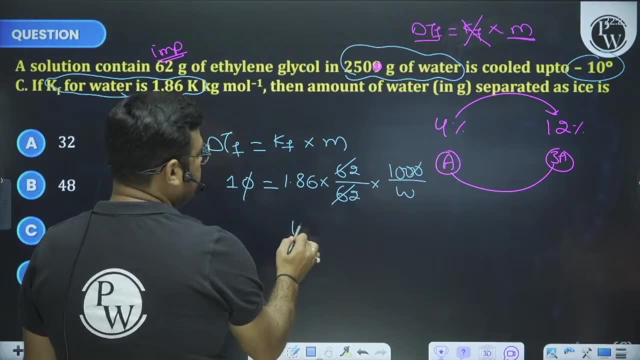 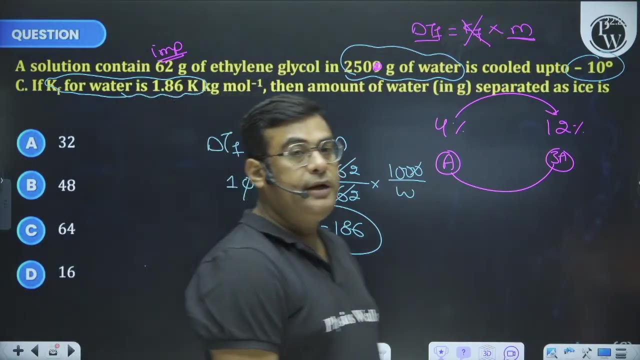 Now you don't know how much water is in this disogram. That's why I don't know that. Right, So this is cancelled. From 10 to 10, W became 186.. This is the W which is still. 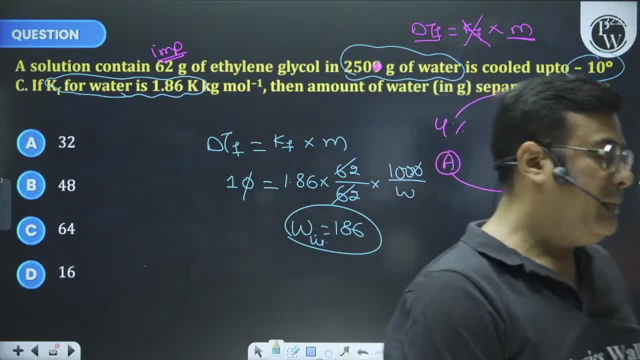 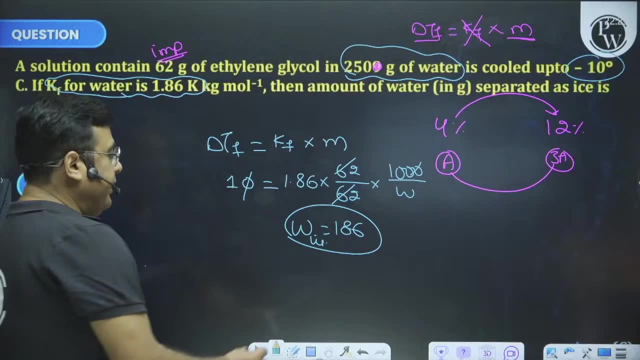 in the form of liquid, Because in molality the mass of water is 186 grams. So if this is 186 grams, then how much ice is there Out of 250, minus 186 means 64 grams. How much? 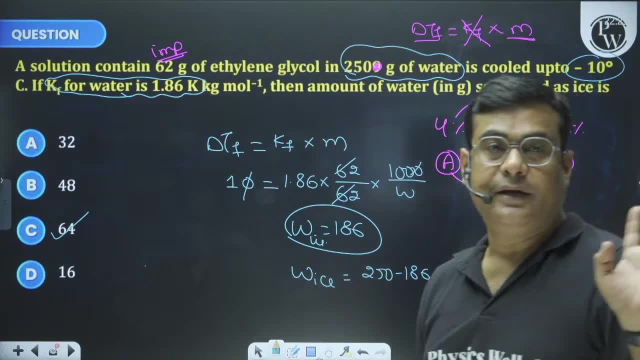 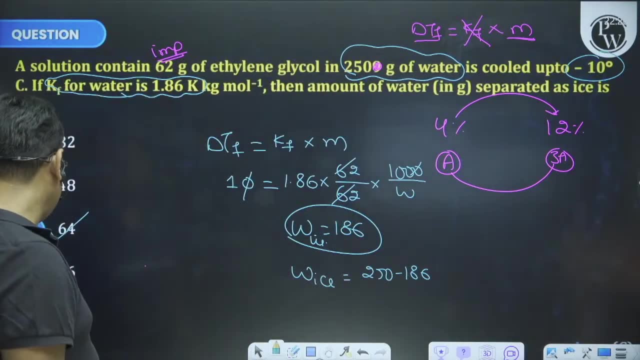 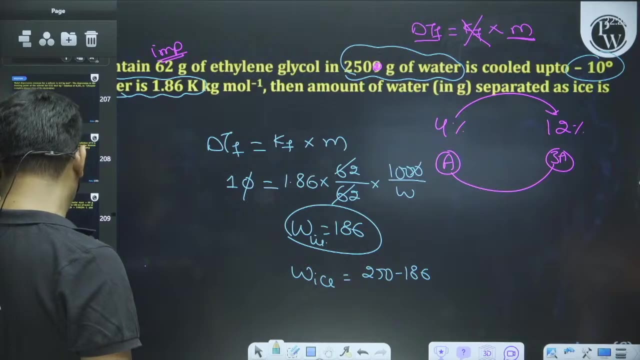 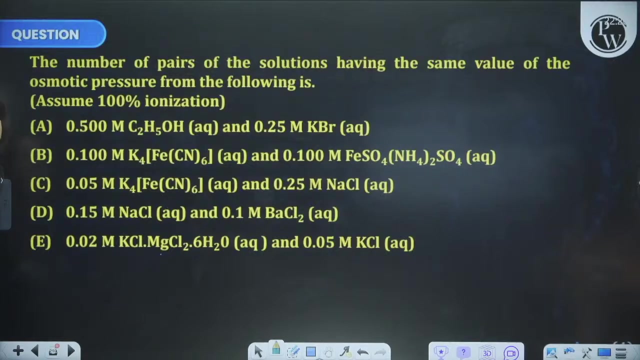 ice is there 64 grams? How much ice is there 64 grams? Does everyone understand what I am saying? This is the story. I am leaving you with some more questions. You must attempt Now. this question seems very important to me. 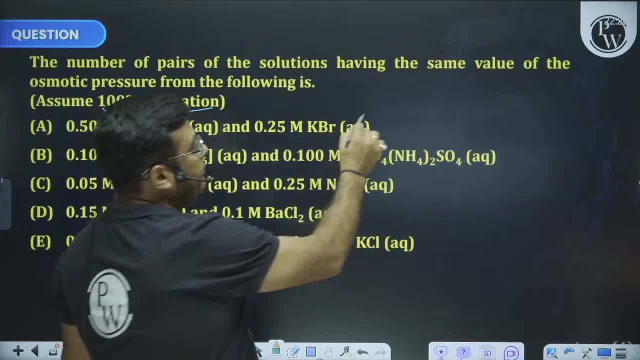 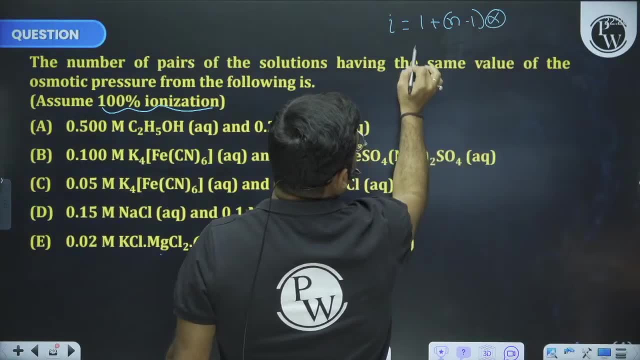 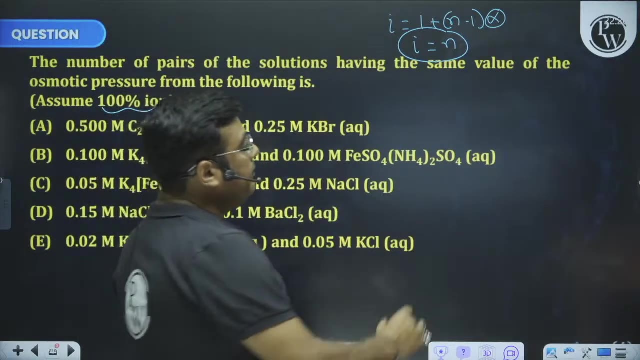 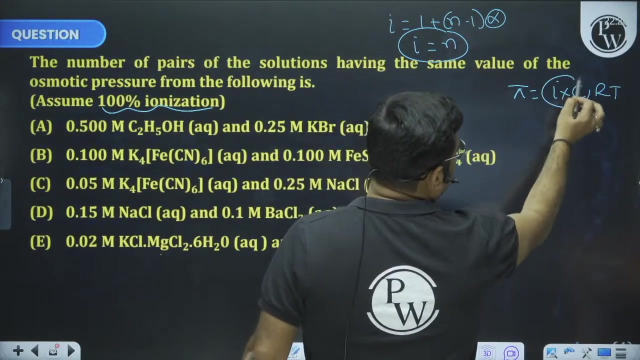 Let me tell you The number of pairs of solutions having the same value of osmotic pressure. Assume 100% ionization. If the ionization is 100%, then the value of the osmotic pressure is the same for those whose. 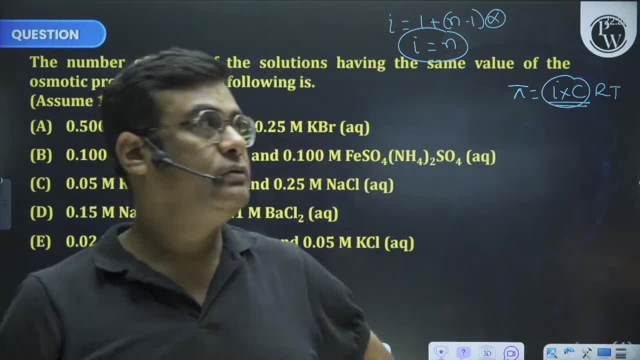 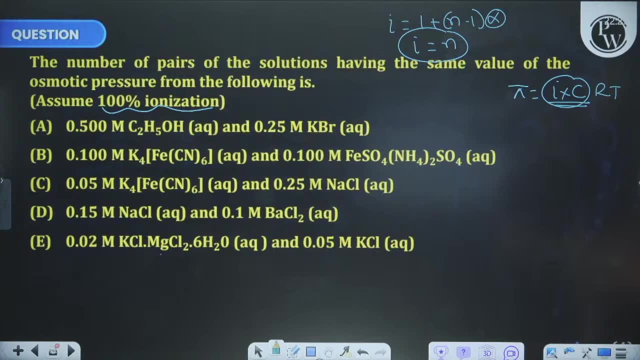 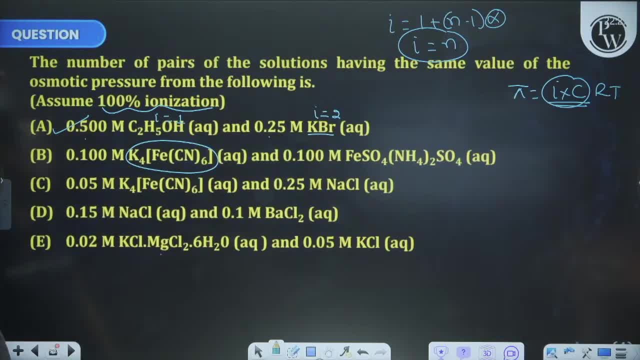 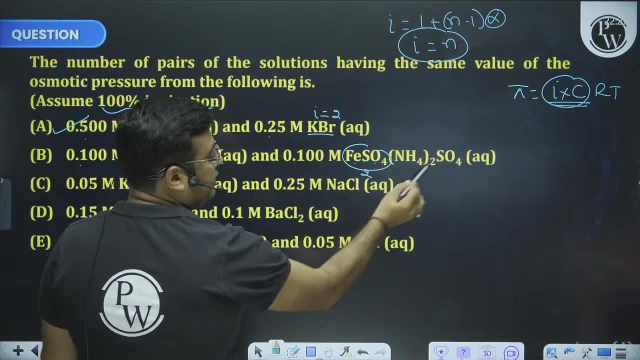 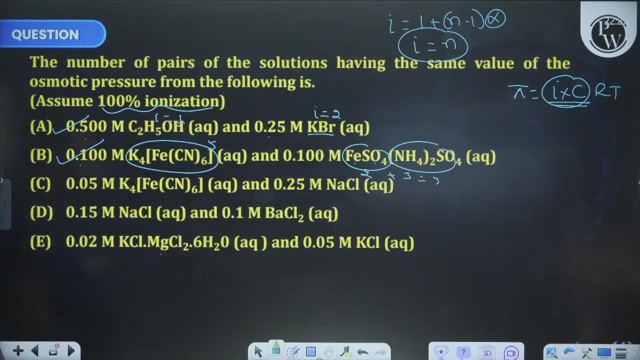 or 0.3 or 0.4 or 0.4 or 0.5 or 0.3 or 0.3 or 0.4 or 0.4. 0.5 sulfate is 3.. So 2 plus 3 is 5.. This is also equal. Just keep checking like this. 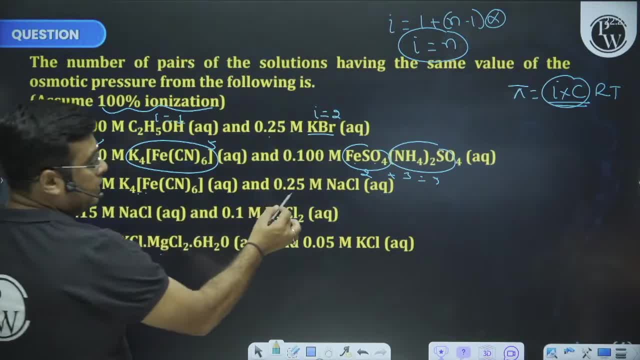 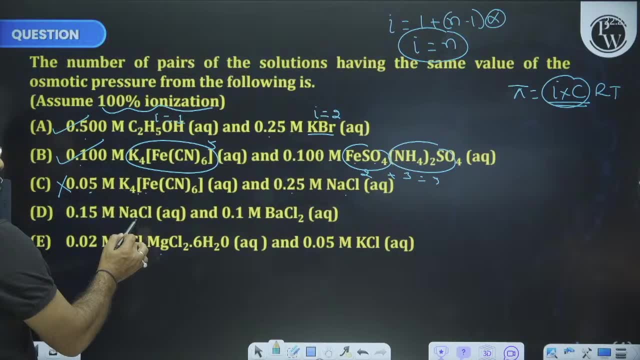 Again 0.05 x 5, 0.25.. Now, 0.25 is the I2 of NaCl. it is not equal 0.15 x. its I2 is 0.3.. 0.1 is its I3, 0.3 is equal Its I, its 2 and its 3 is again 5.. 0.02 x 5,. 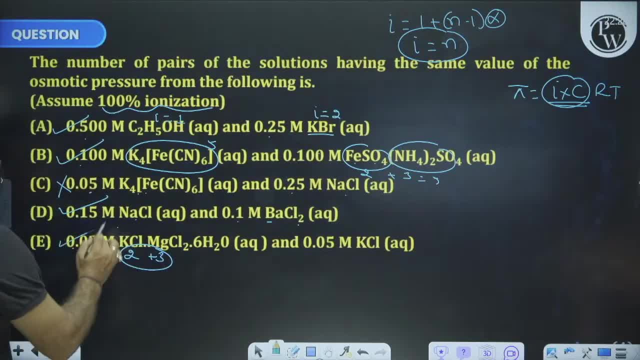 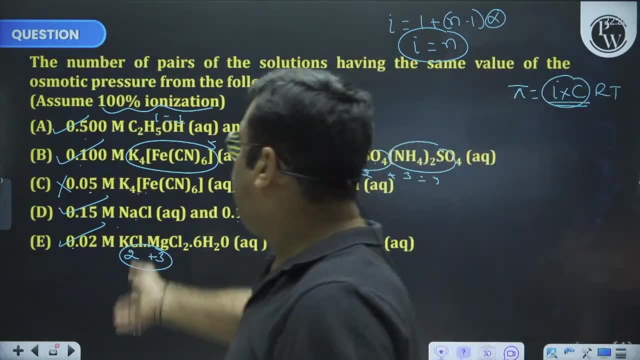 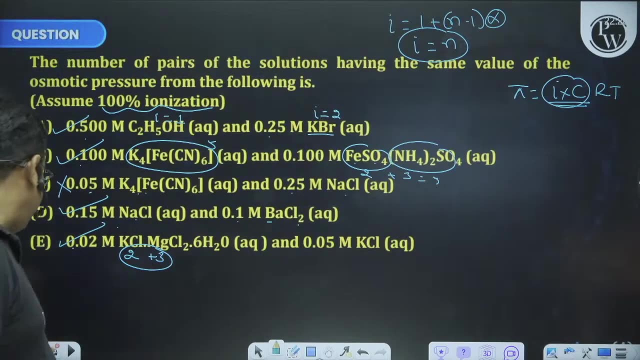 0.1, 0.05 x 2, 0.2,. excuse me, So it is equal to 4.. Nowadays in JEE, in integer type, questions are also coming like this: to know how much is equal. So I have done all the. 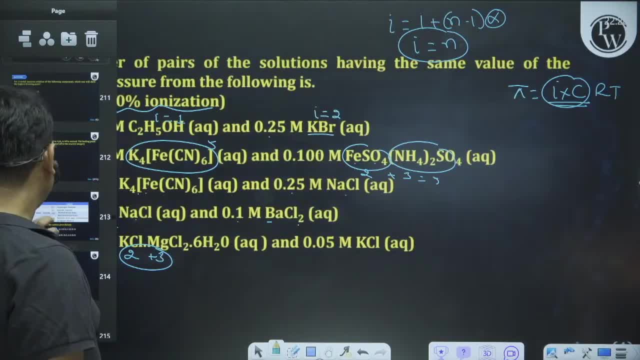 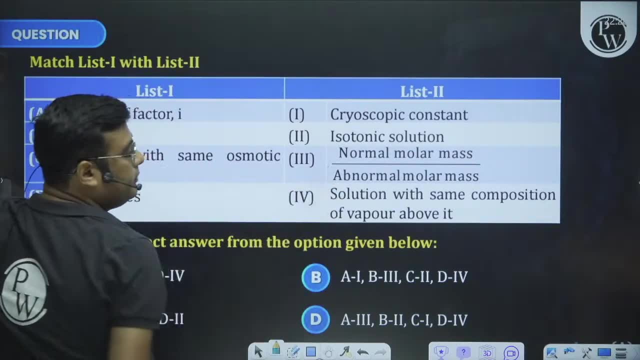 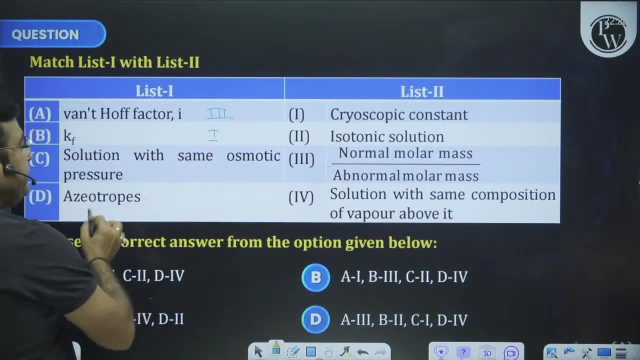 questions that I thought were important. These kinds of questions also come. I am taking the last question. I have asked the formula directly: Quantum factor I: normal molar mass upon abnormal molar mass, KF, Sir. KF is cryoscopic constant Solution with same osmotic pressure, Sir. 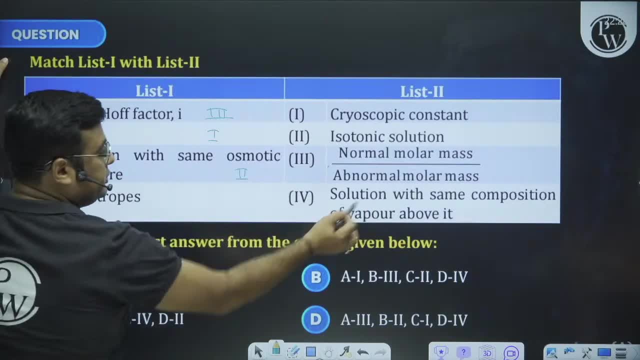 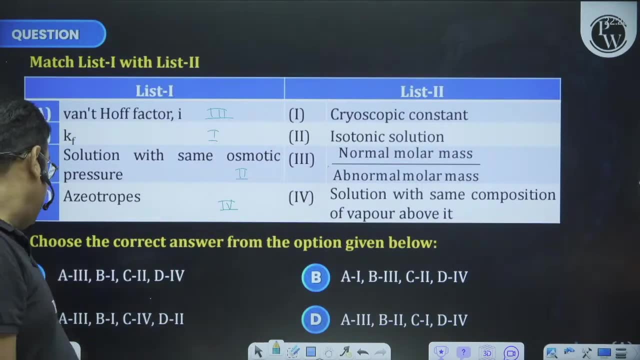 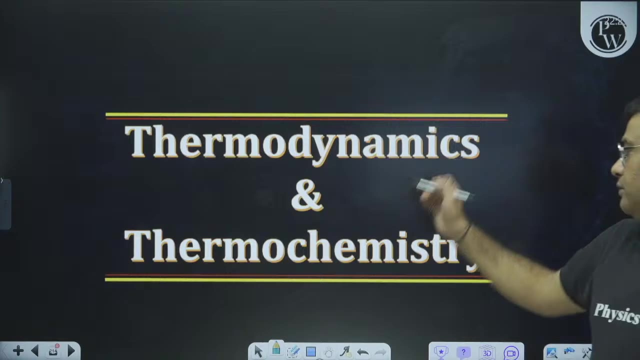 they call it isotonic solution, So azeotrop solution with same composition, vapor above it. Check from below, Check from below. Ok, So that's it. In this question. I have brought some 8-10 questions for you. You will do that. Now we are moving towards thermodynamics and thermochemistry. 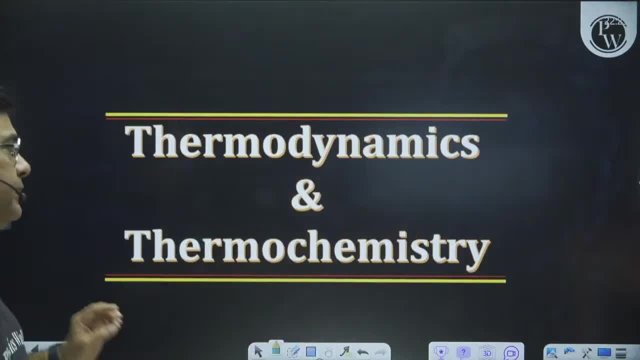 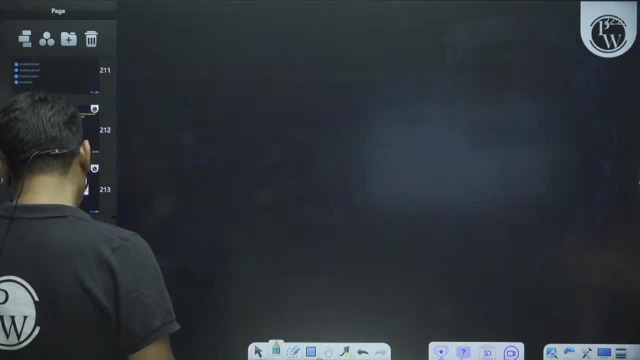 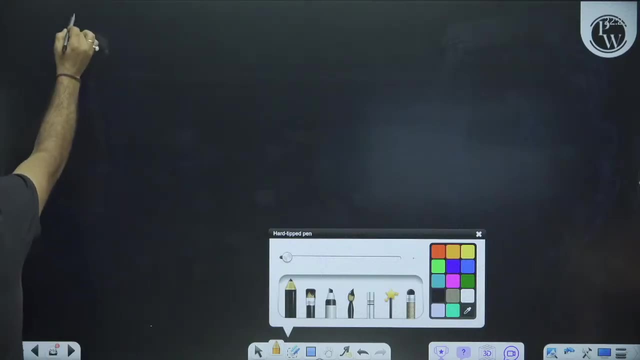 Now, even from this chapter, you should also have a good understanding of thermodynamics. But this chapter is also very, very easy. I will tell you the crispy formula. see what formula will be used in this chapter. see, the question comes the most on the ideal gas. 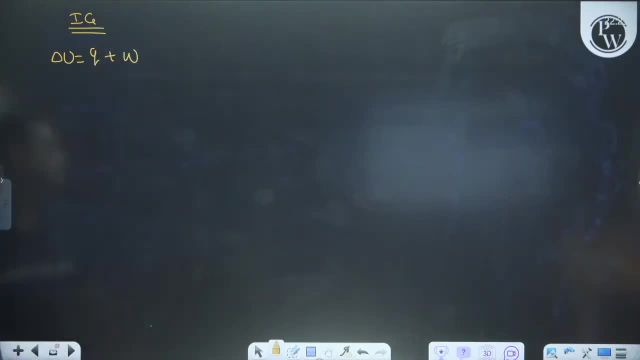 first law of thermodynamics: delta U equal to Q plus W. apart from that, the ideal gas delta U will always come out of NCB delta T. delta H will always come out of NCB delta T. work will always come out of minus integration of PDB. that child is different from different. 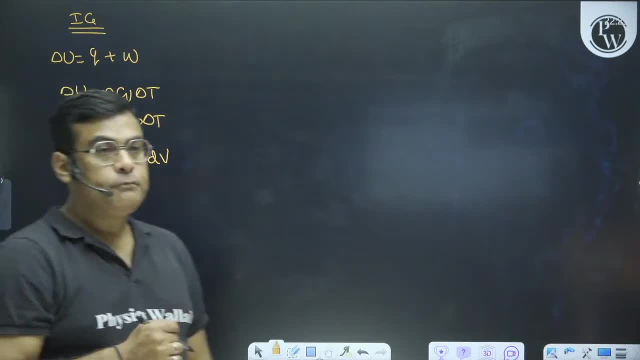 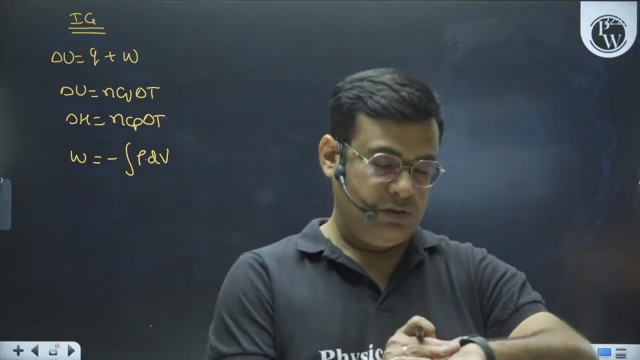 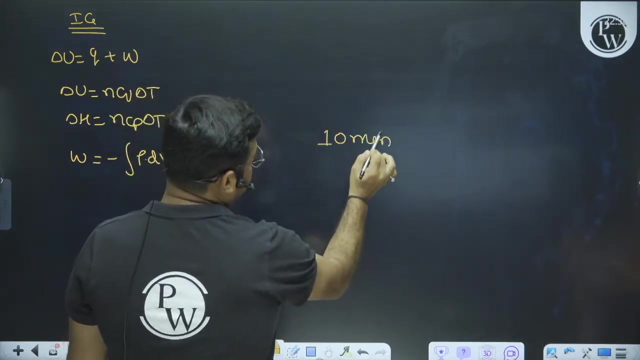 processes. right, that is different from different processes. okay, so much insistence on the break. let's give it. let's take a small break. let's take a break of 10 minutes. you are also getting worried. we allow you a break of 10 minutes. okay, after that, these 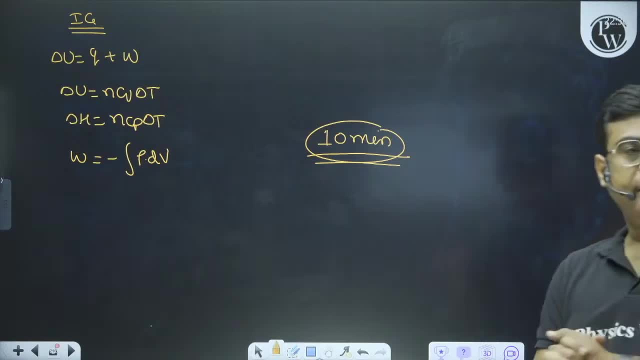 are only two chapters. we will finish it in about an hour. take a break of 10 minutes. you are also getting worried. two and a half hours have passed. okay, let's meet after a break of 10 minutes, Thank you. 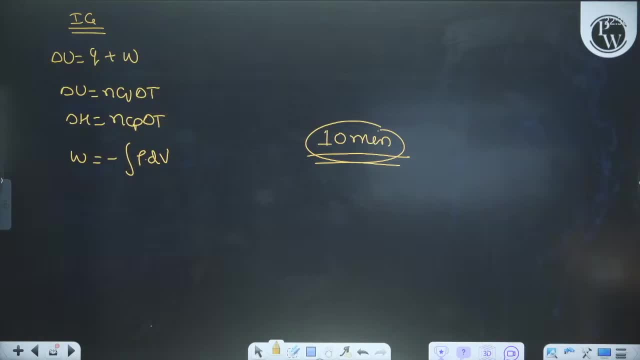 It will be done in half an hour or so. Oh, it has opened. Hmm, It has opened, right. Well then, let's put it back to the awesome. Yes, It's done, All right. Well, I'm glad you guys are here and you have a good morning. 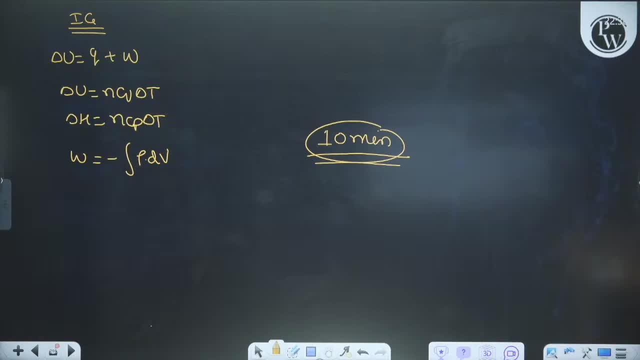 Yes, sir. Thank you all for coming. Oh, you're welcome. I'm glad you are Okay. So what does this mean? So the map here says we're going to a different part of the world. Let's go there. 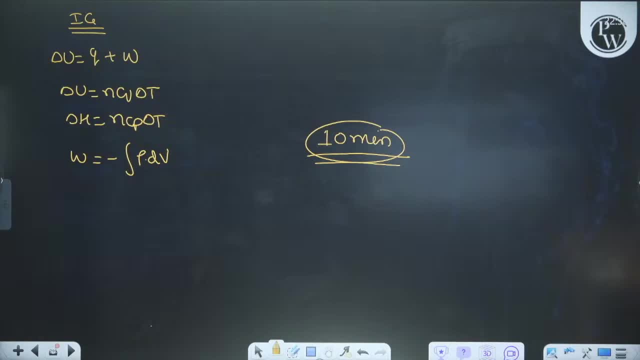 Okay, great, So we're going there. I see, Excellent, thank you. So you're going to go there. So you're going to go there. Sure, yes, All right. well then, let's go there. 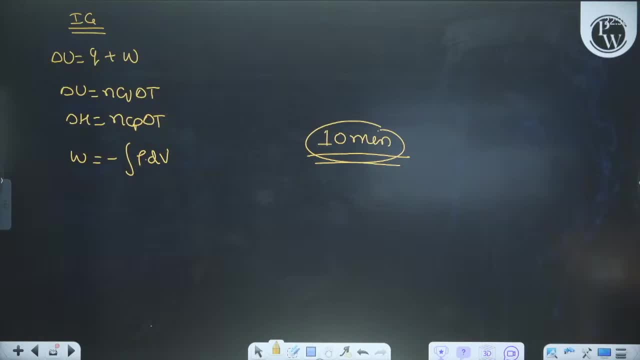 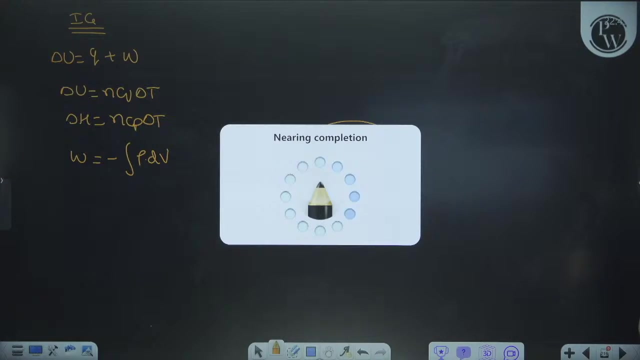 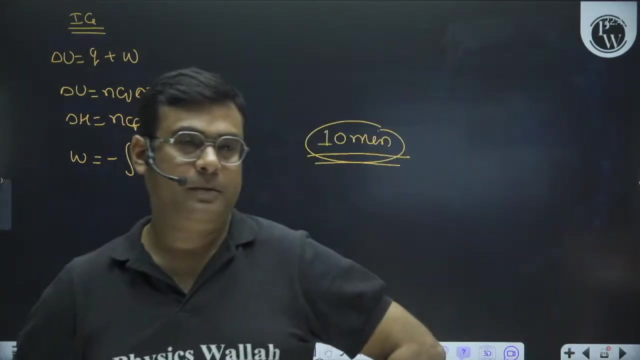 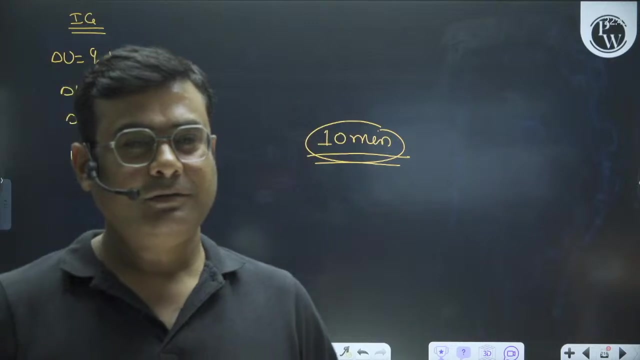 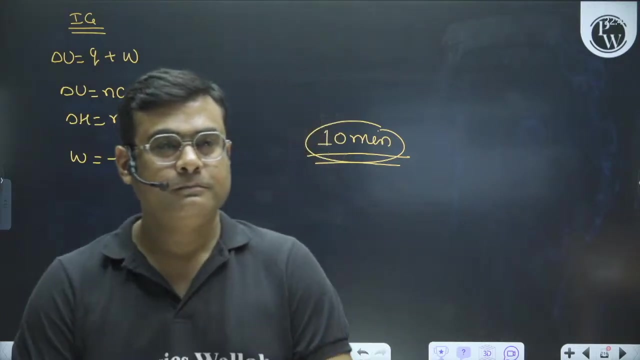 Okay, well, let's go there. Thank you, All right, good, I see, So I'm going to go there. Good night. 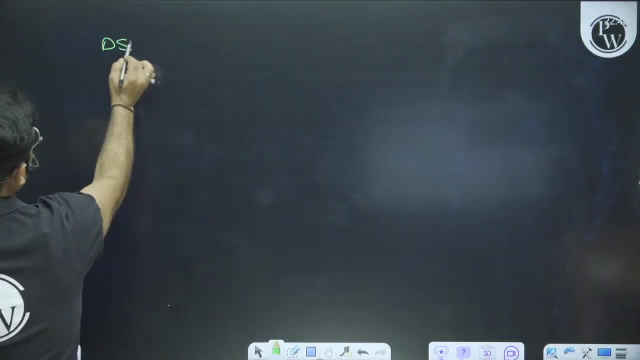 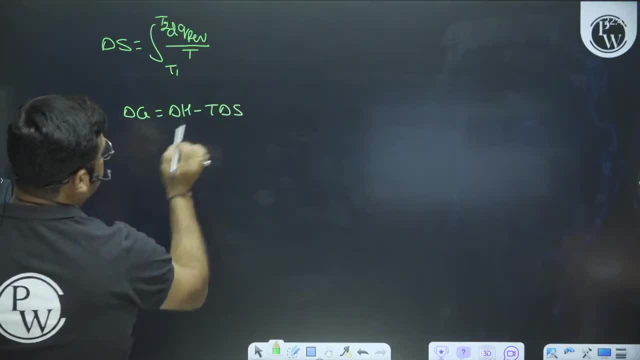 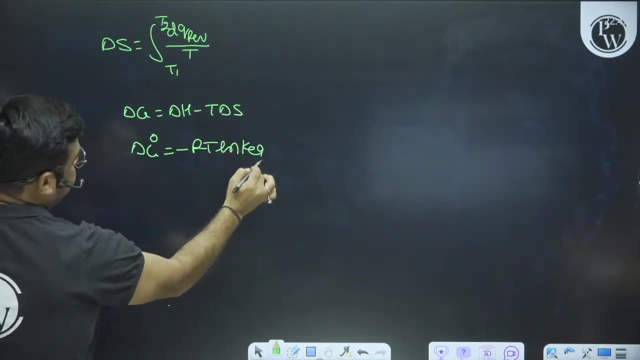 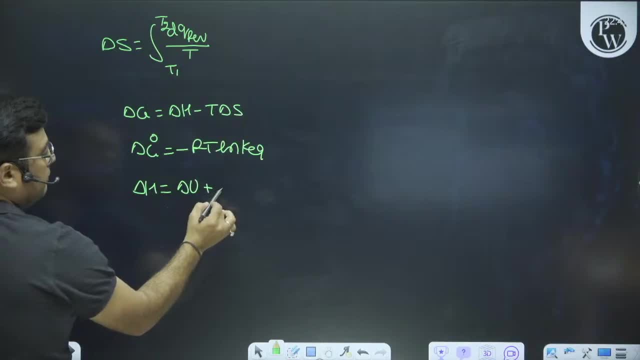 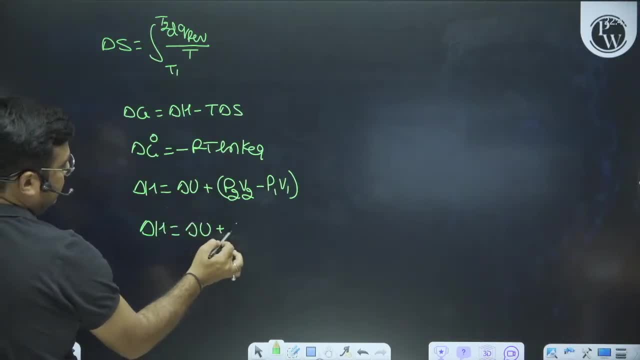 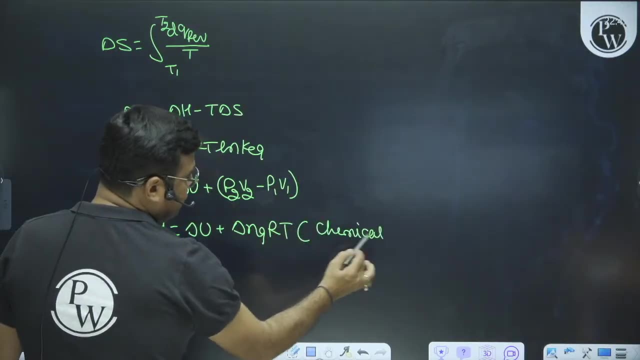 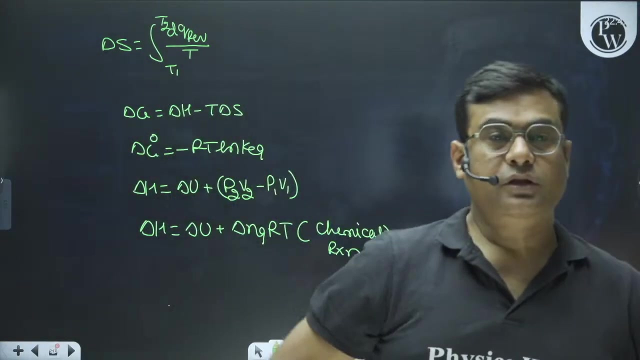 And if we counter this, then delta H is equal to delta U plus delta NG RT. This is what it looks like for chemical reactions. So if you remember some of these formulas, then the questions you have. Sir, this concept has been asked in 2024 questions. 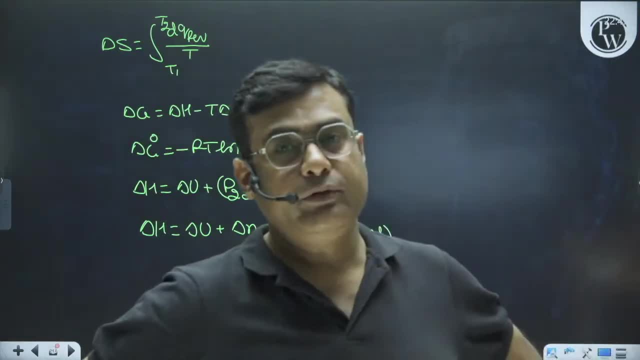 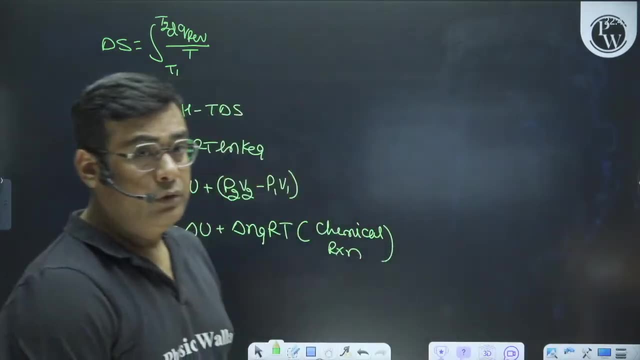 So 2024 has also come in your January attempt, children. So along with that you will also get questions on these only in the April attempt. I will also tell you this from now on. So these are the things, just obviously. children. thermodynamics is such a big chapter. 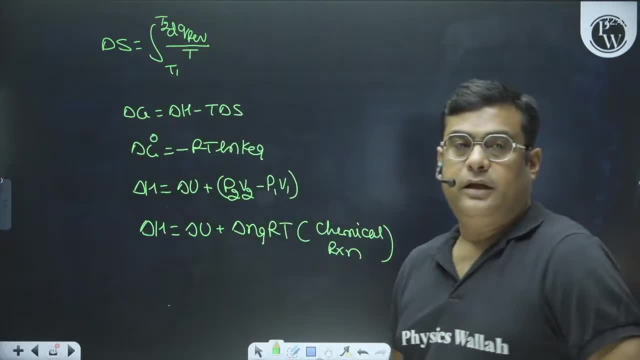 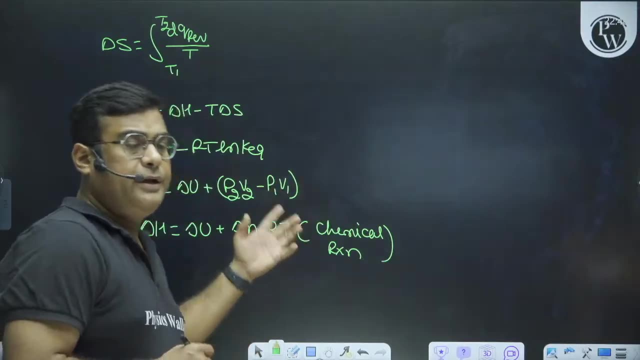 that normally you will know in the year long that 15-20 turns- 25 turns- are also taken to study this. This is the minimum. But now what to do? for a quick reason: that if we remember these formulas then we can easily ask questions on them. 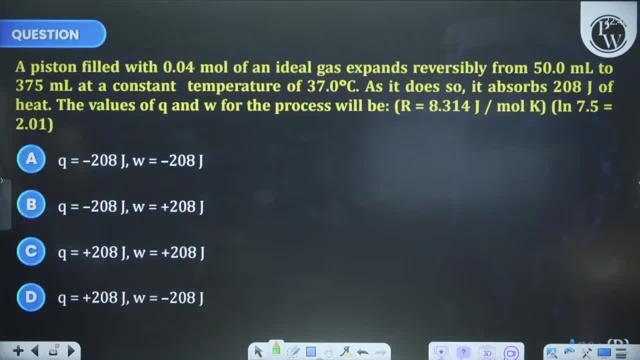 Okay, if I show you some questions. see what he is saying. A piston filled with 0.04 mole of an ideal gas expand reversibly from 50 ml to 365 ml at a constant temperature. It is clearly written that it is a constant temperature. 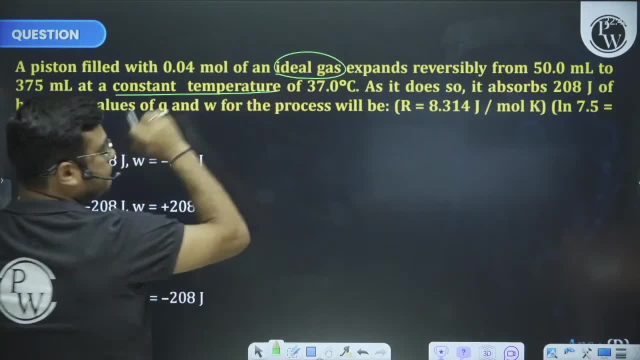 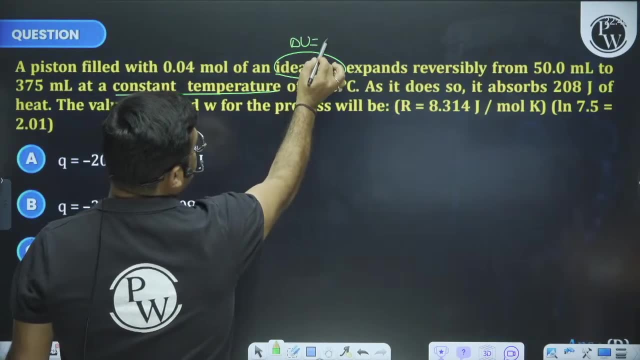 Okay, right, What is it filled with With? an ideal gas? He said ideal gas, he said constant temperature. As soon as delta T is 0,, delta U becomes 0. And if you put a float, then Q and W will be numerically the same. 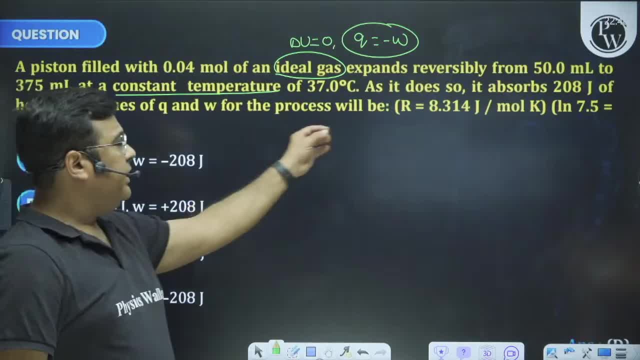 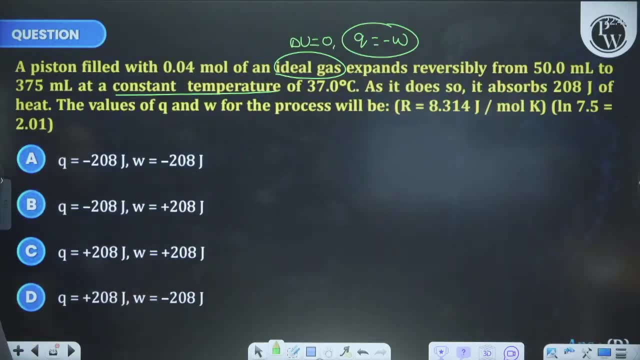 The sign becomes opposite. Okay, As it does. so it absorbs 208.. 8 joules of heat It is absorbing. that means Q plus will be 208.. W becomes minus 208.. He has asked this: Q W. tell me. 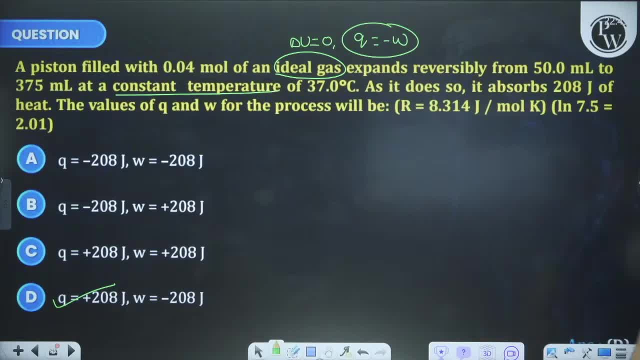 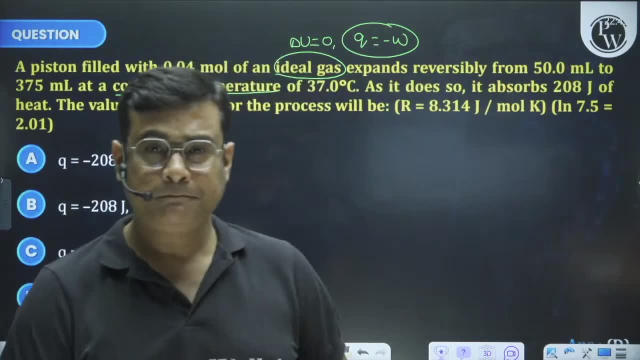 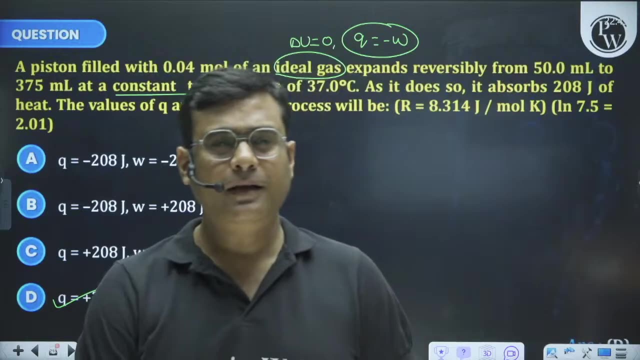 Now there are many of us children who sit down to sing songs. Which one? Let's see how much strength is in this. Keep your feet firm, My friends. He starts putting his strength in every question. He starts putting his strength in every question. 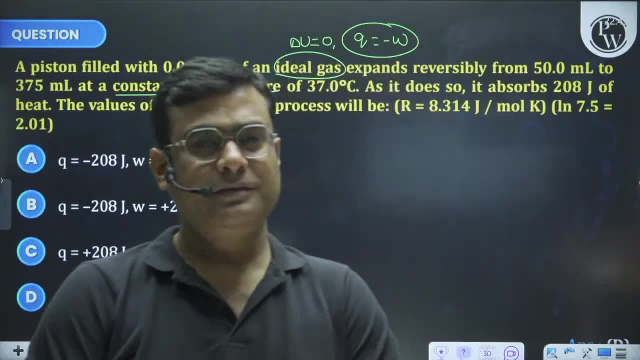 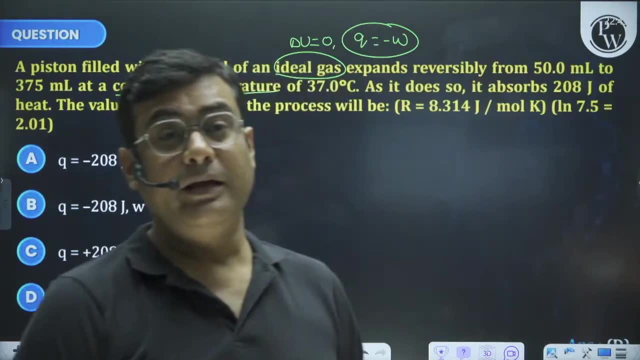 He starts putting his strength in every question. He eventually stays out of the game, and So he says this to wittsamed people like me: I'm very brow. Let's put a, put a, put a. Let's call it a taken best bet goose. 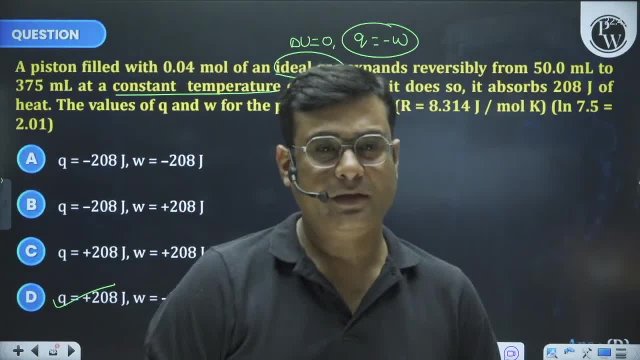 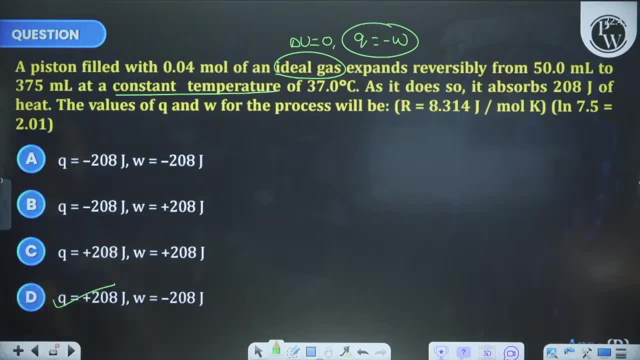 He pulls a coconut for a objections. So give it a putt. So let's go for the question. OK, So I'm going to put a put a putt on it And I'm going to select. Okay, there's no SECOND cure. 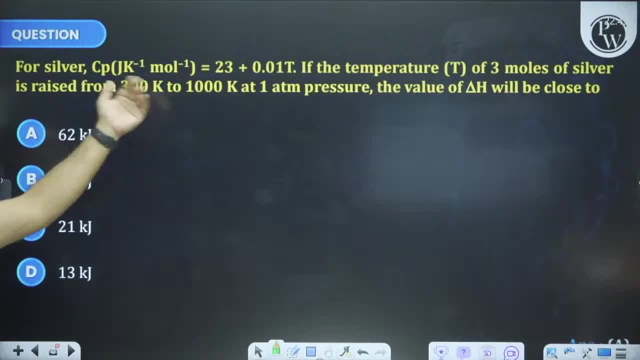 No, go ahead. Yes, sir. Okay, All right. If the temperature of 3 moles of silver is raised from 300 to 1000, then delta H is applicable for ideal gas. The second condition is that we consider Cp to be independent of temperature. 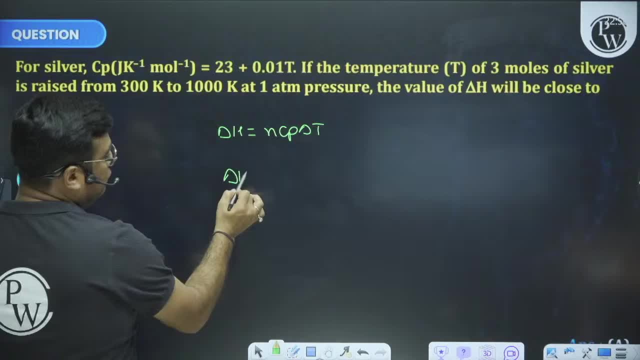 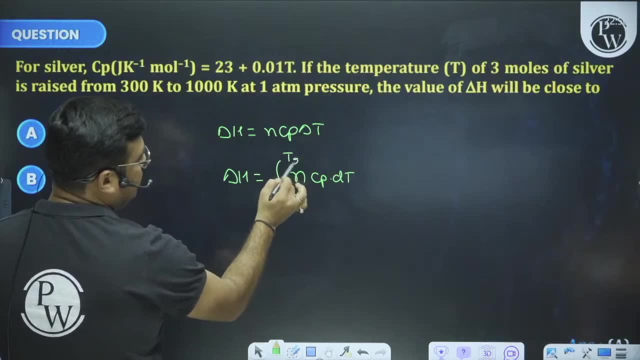 Sir, if Cp is not independent of temperature, then you will integrate it by writing n Cp dt. The story is over. You know more mathematics than me. If I were a student, I would have been talking about 96-97, because I had cleared JEE in 97.. 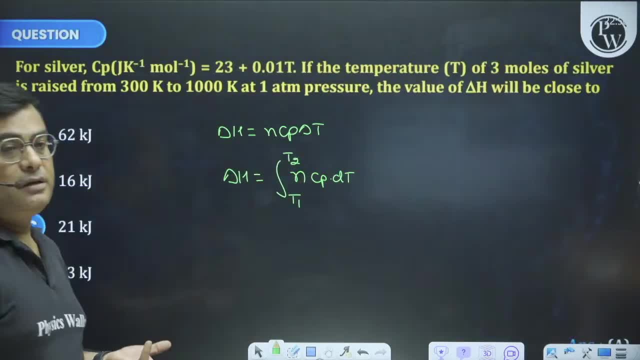 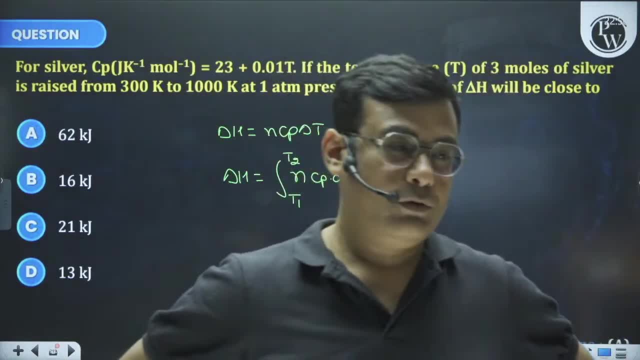 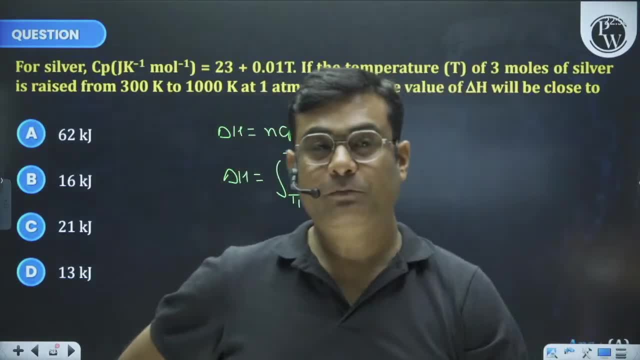 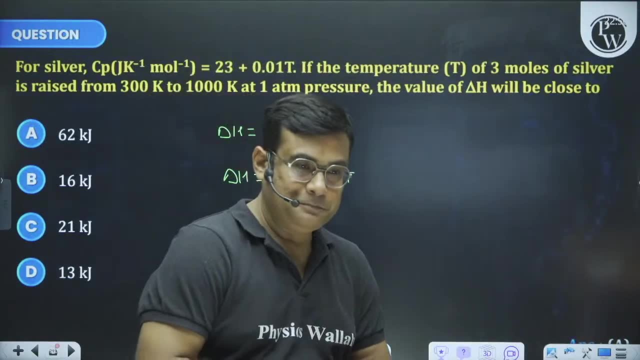 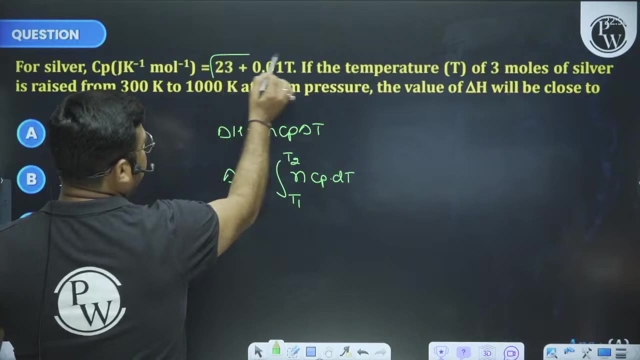 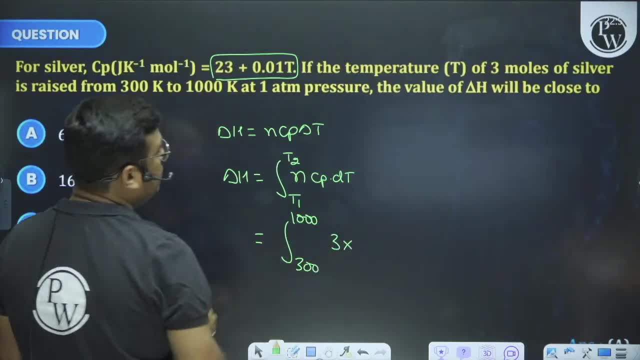 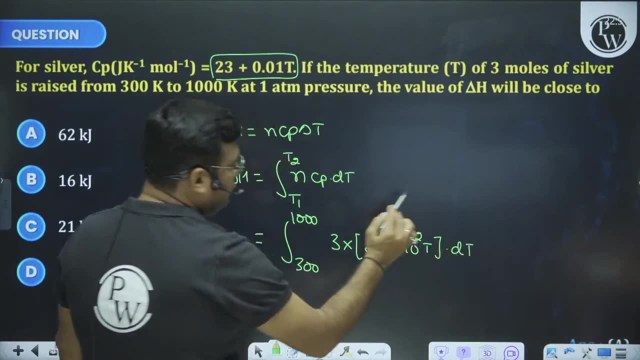 If I stay on the form of p, then I will write n- Pb as well as ng here. Then you have to also write element of power of 2, as well as element of g. You have to write element of power of 2 and you have to write element of power g here. 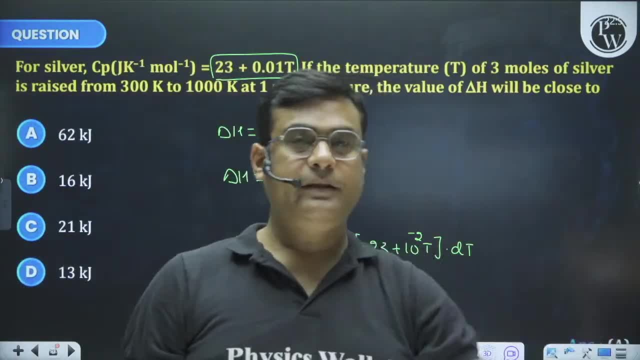 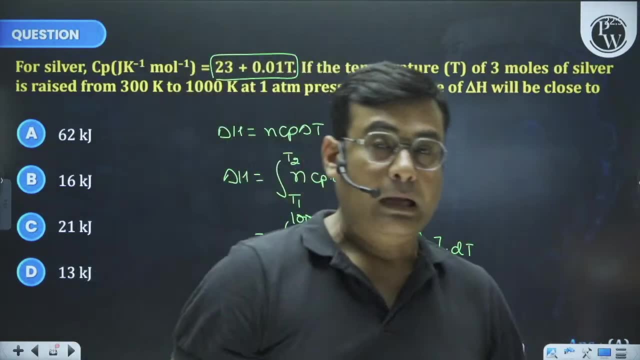 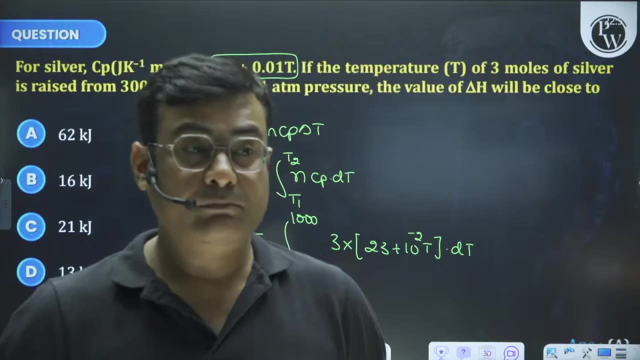 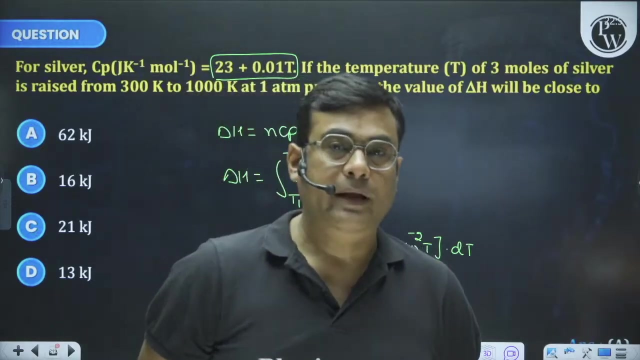 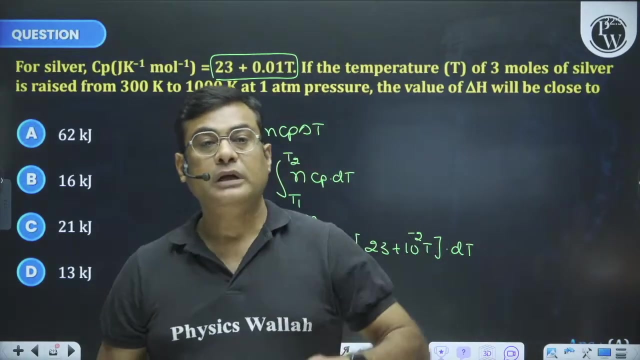 Don't take me wrong, It is all fine. Okay, Okay, All right, This is all fine. My role in your selection is only of a catalyst. I say this to my children again and again: a catalyst can never initiate any reaction. a catalyst can increase the rate of the reaction. 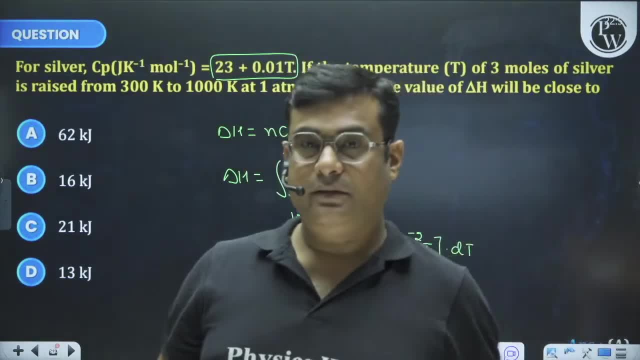 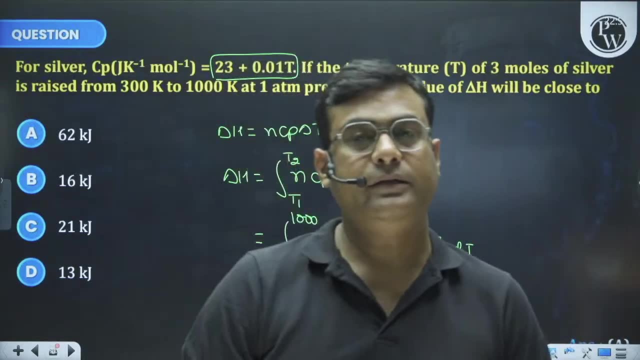 that is already going on. that is, if a child is not studying, then he is not going to be selected by attending any teacher's class in the world. But if a child is not studying, then he is not going to be selected by attending any. 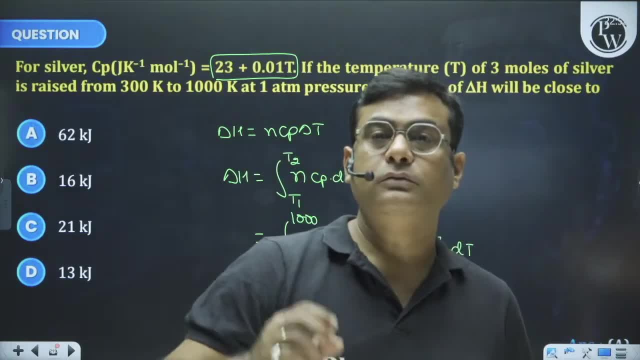 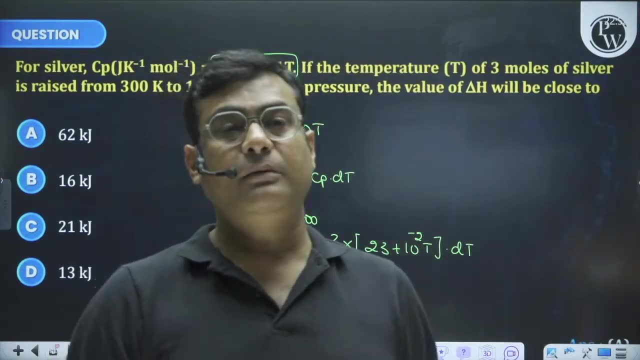 teacher's class in the world. If a child is studying the question to be answered, the time it takes to understand the concept- it may take him 5 minutes in some questions. then if I work like a catalyst, then maybe the question starts to be asked in two minutes. 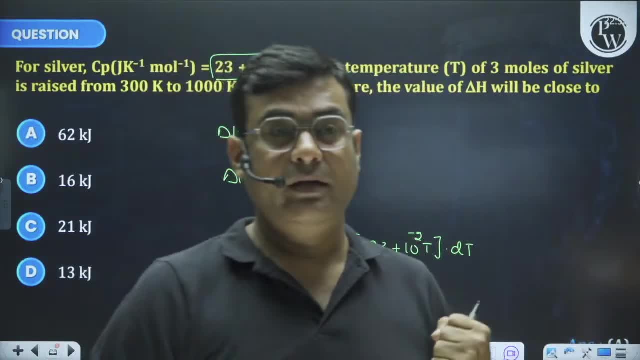 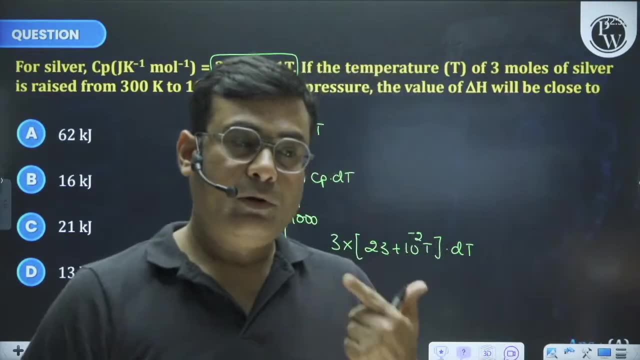 The concept, which took an hour, he will understand in 15-20 minutes. So this is the story of children. alright, So I am the catalyst, because if you don't study, if you don't study, I am giving you homework- you will not solve it, you will not apply the concept, then nothing will. 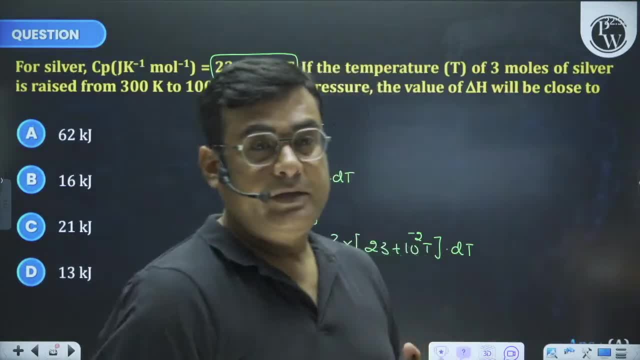 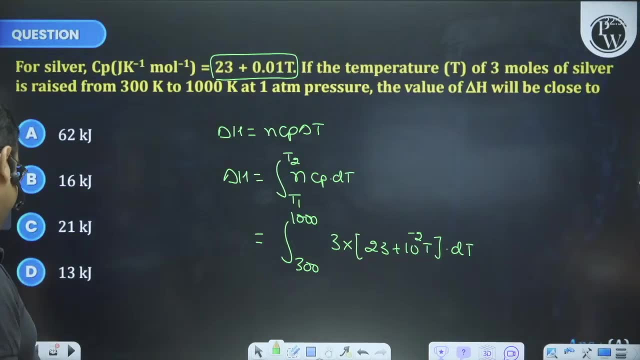 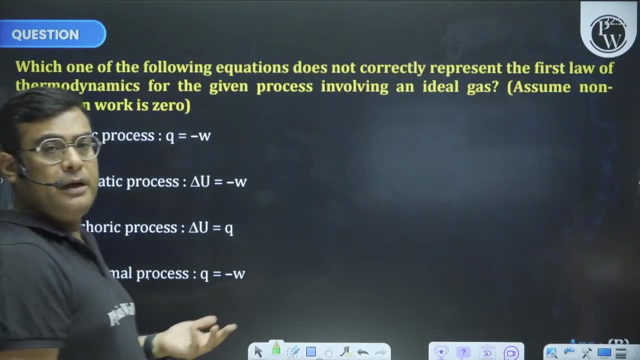 So I hope you will do the integration and the answer will come in front of you. So in this way, I will tell you some questions Now. the questions are simple. We have to scare them, So it is a different thing. 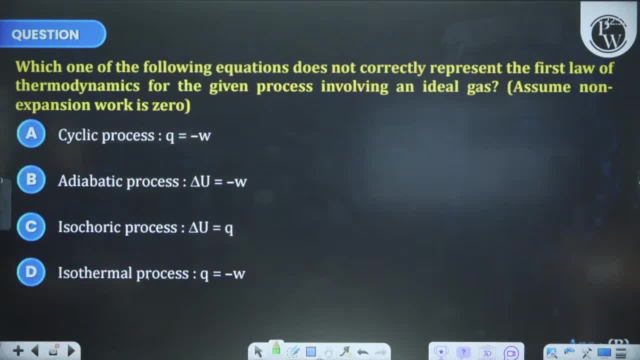 The next question is in front of you. Which one of the following equation does not correctly represent the first law of thermodynamics for the given process? In the cyclic process, Q minus W is absolutely correct, Because in the cyclic process delta U becomes zero. 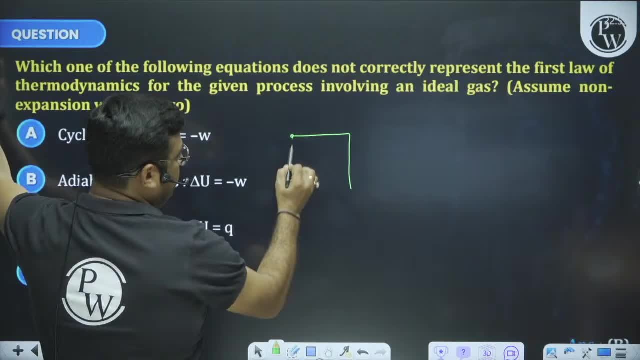 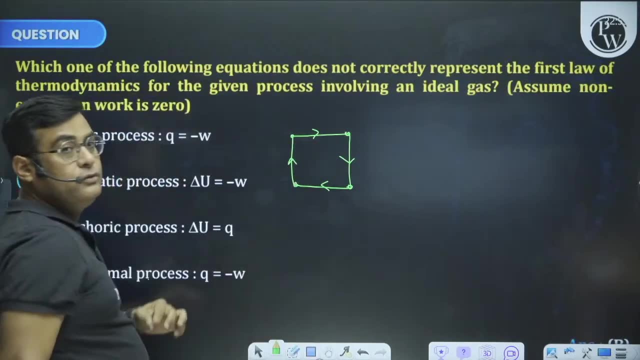 From where the system runs. the system comes back. So obviously U is a state function. so delta U becomes zero. Delta U minus W of the adiabatic process is wrong, Because the delta U of the adiabatic process is equal to W. 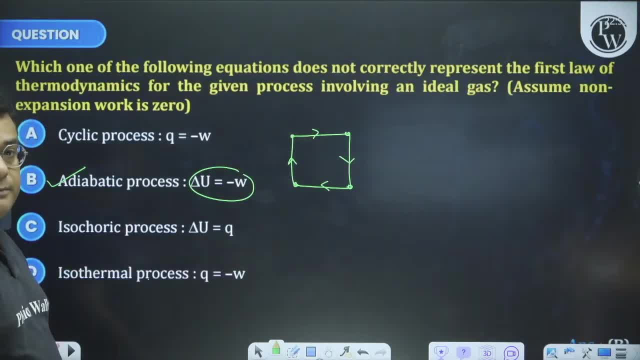 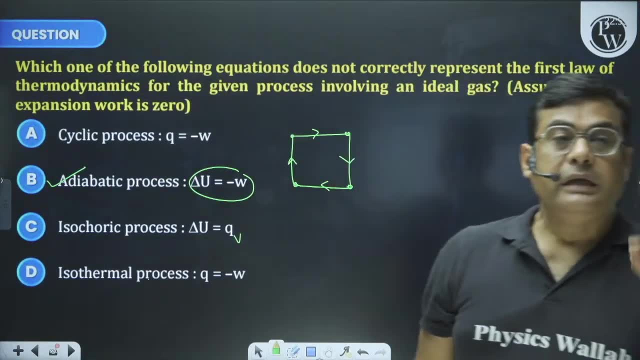 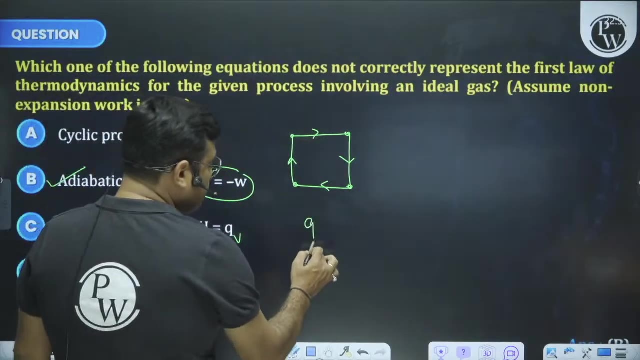 Delta U of the isochoric process is equal to Q, Absolutely correct. That is why you must have heard That sometimes we call the heat at constant volume as delta U. Okay, And the heat at constant pressure is also called delta H. 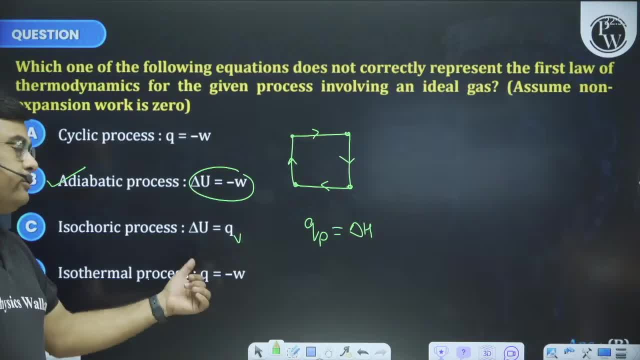 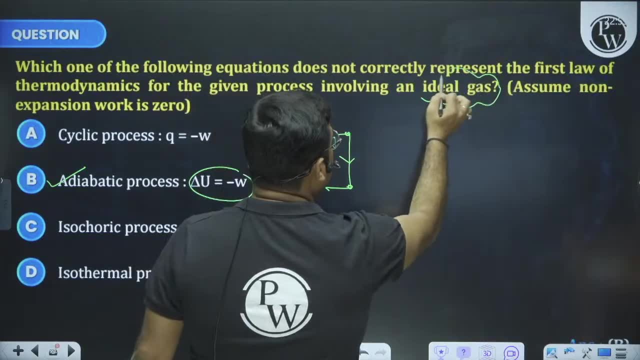 The heat at constant pressure is also called delta H, And the delta U of the isothermal process is equal to W. Okay, Look again. It is important to be written children ideal gas, Because if there is an ideal gas, then I will call delta U as zero. 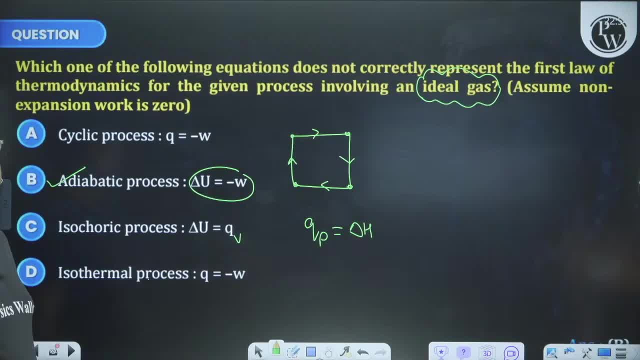 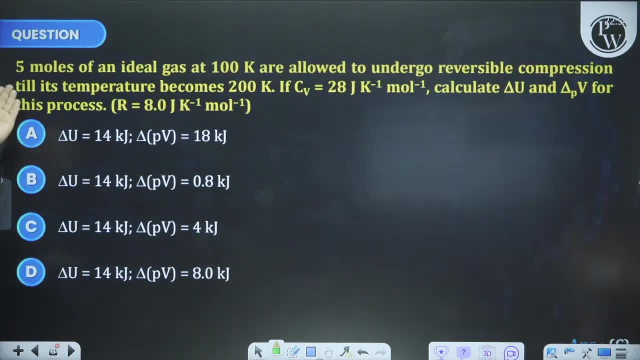 And if I call delta U as zero, then only I will take Q equal to minus of W. Okay, So do such simple, simple, lovely, lovely questions. Enjoy the world. Five moles: Give the number of moles, It is an ideal gas. 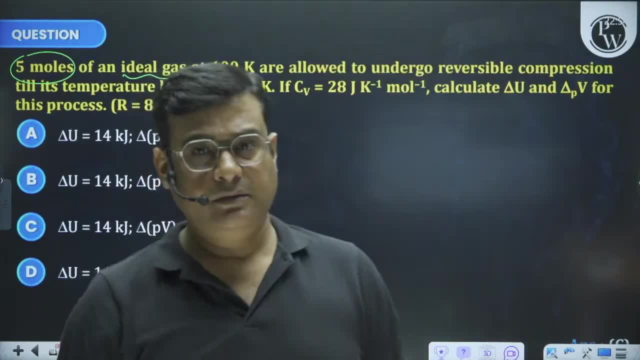 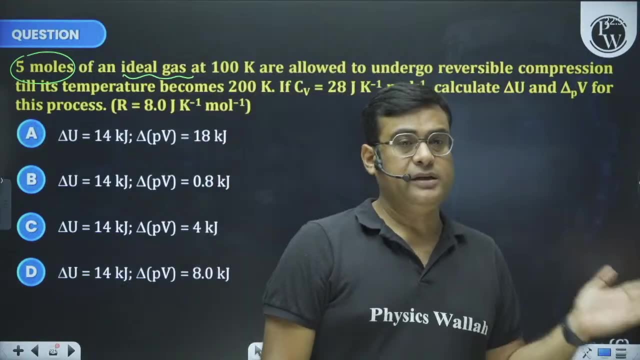 As soon as the ideal gas comes, raise your confidence in your heart That you have to break that question And it will definitely come. children, Whether it is in chemistry or in physics, I am telling you this too. In chemistry, the chances are less. 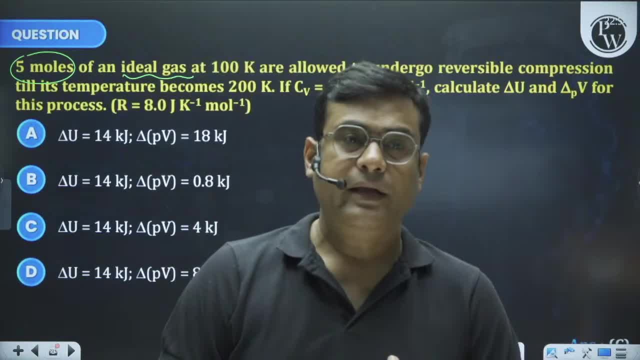 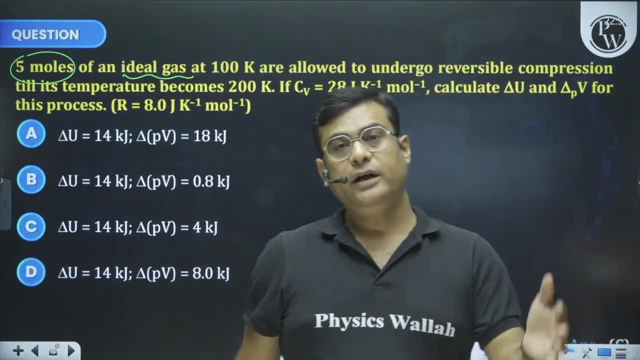 Because in chemistry it will mostly ask you questions on delta H or on delta S or on delta G, But in physics these three do not happen. In physics we only talk about delta U, delta Q and delta W, So it is compulsory to get the question. 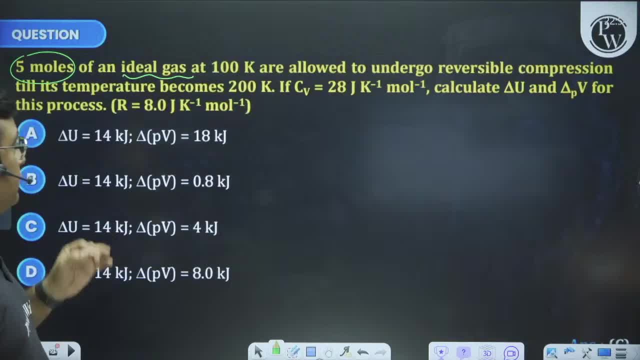 It is compulsory to get the question. Consider this: It is compulsory to get the question, Okay, So it is telling you that you are allowed to undergo reversible compression. Right, Reversible compression, Okay, Till its temperature becomes 200 Kelvin. 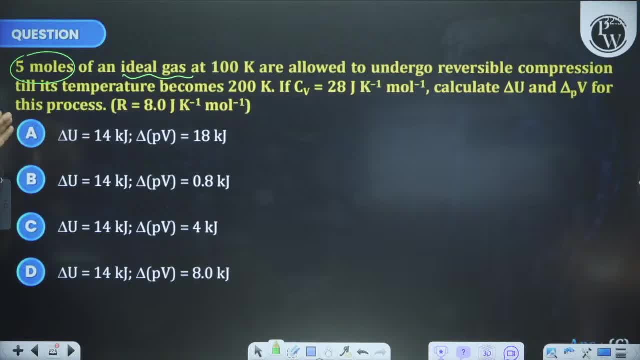 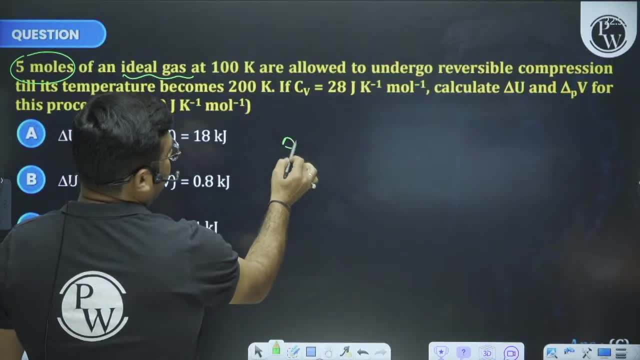 At least 200 Kelvin. If Cv is this much, then tell me the value of delta U and delta of PV. I don't think any child should have any problem. But the ideal gas has been said, Who will be equal to delta U? 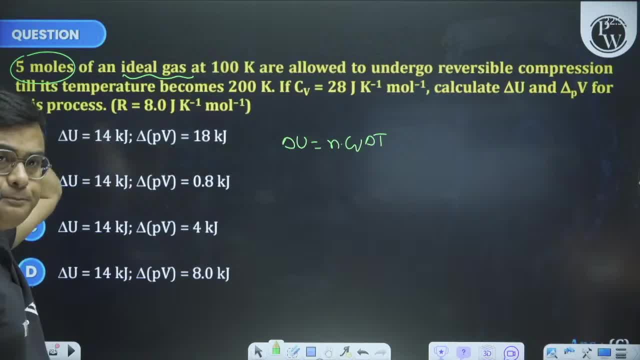 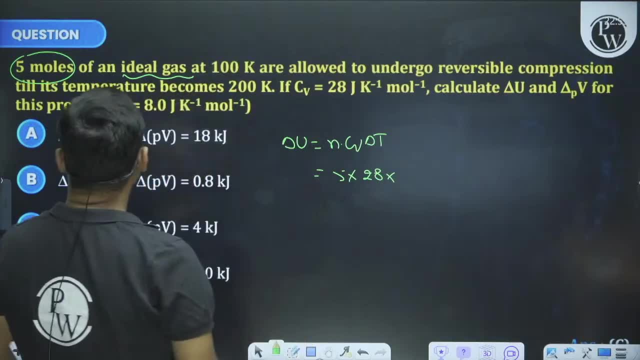 Sir N Cv. delta T. Yes, Right, Right, It will happen. sir N has been given to you. I am also doing the calculation And delta T Right, It has gone from 100 to 200.. 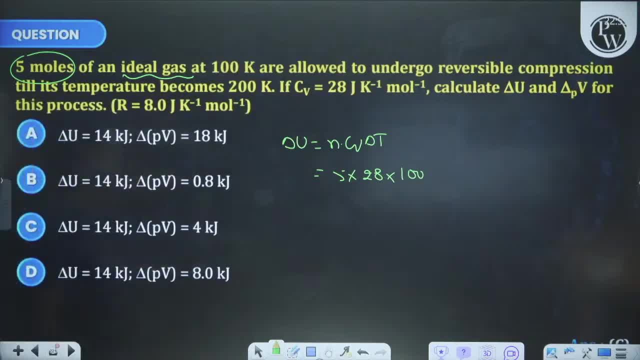 It has gone from 100 to 200.. The value of delta T: 25,, 8,, 140.. Right And 140 into 100.. 14,000 kilojoules, So 14.. Rabija's answer is: 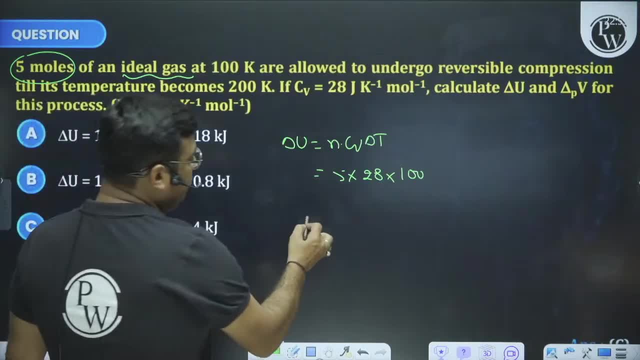 Delta of PV has also been said. So, brother, if it is the ideal gas, then delta of PV can also be written as delta of NRT. That means it is simply NR, delta T. And he said, brother, take R also as 8.. 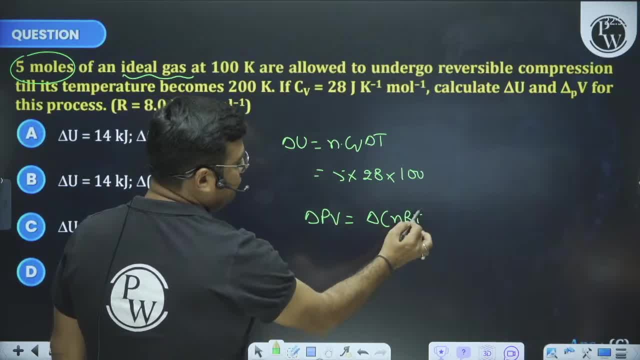 And what to do? more than this. The number of moles is 5.. R is 8. And delta T is now 100.. 5 edge of 40.. 4000 kilojoules For 4. 4.. 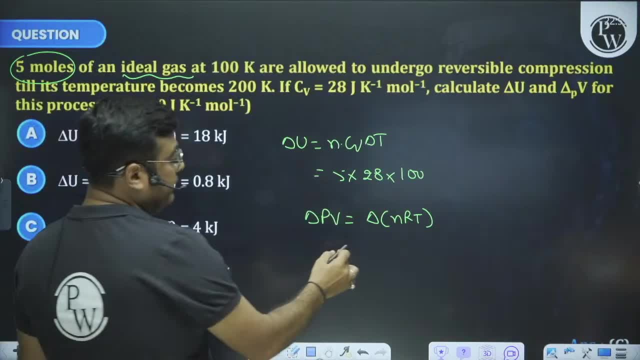 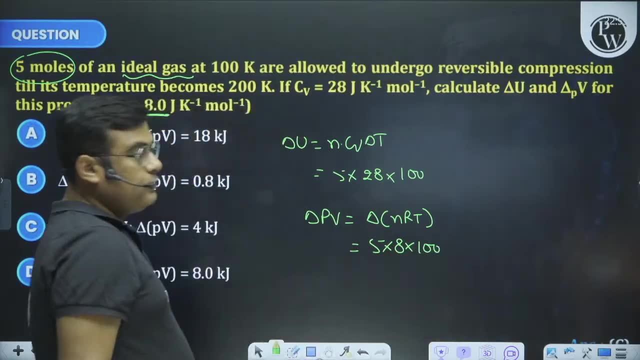 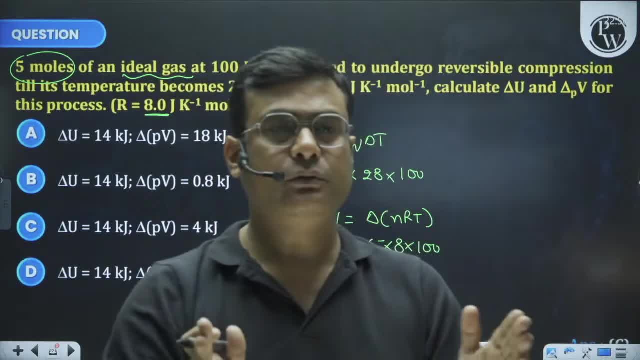 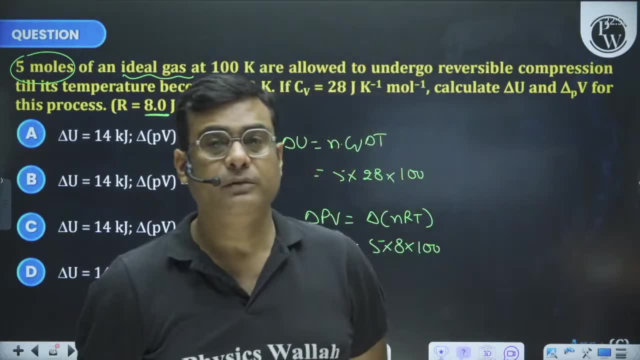 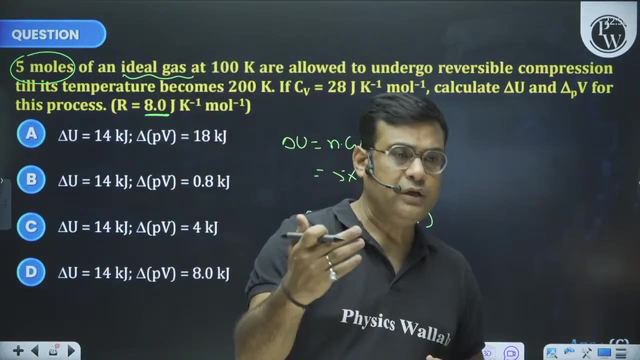 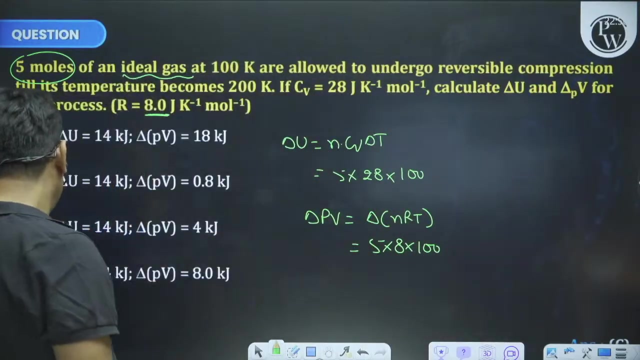 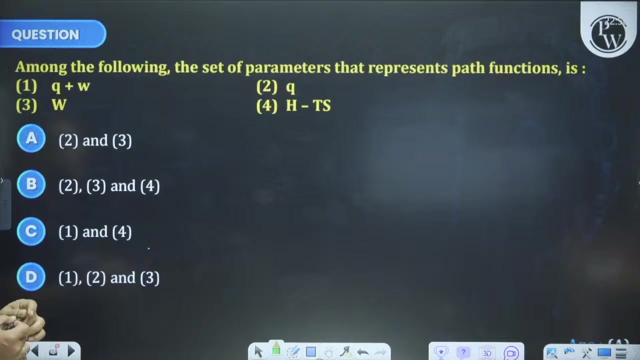 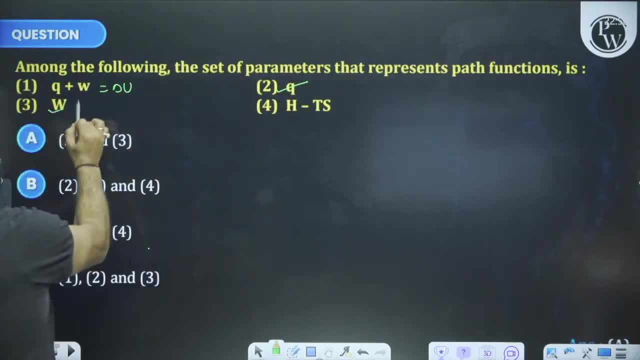 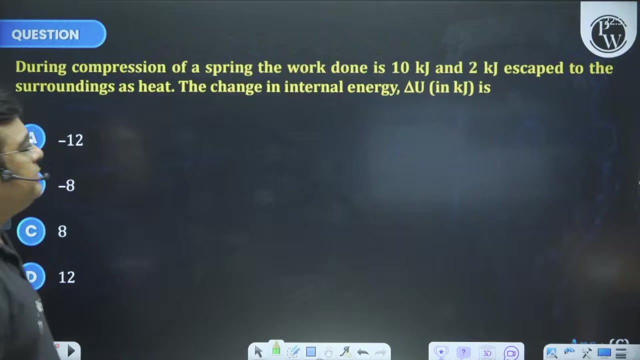 it is a straight function, Q is definitely a path function, W is definitely a path function and H minus TS. what is this, sir? this is G. so G means Gibbs energy, Gibbs energy means state function. so what does this mean, my dear children? KL2 and 3 means ok, the story is over. lovefully question during compression of a spring work done is 10 kilo joule. right means spring work is doing. so, brother, minus 10 with chemistry. 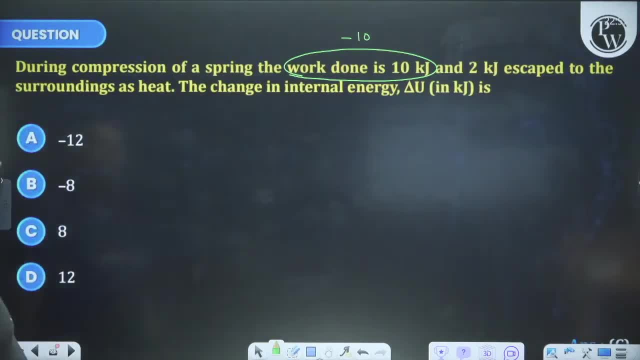 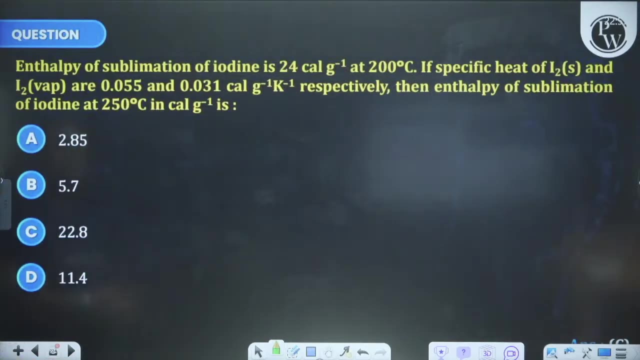 and 2 kilojoules escape to the surrounding as heat. so how much will we keep Q as minus 2, so delta U is equal to Q plus W minus 12 will be the answer. such questions, I can't do anything. simple questions you have to do. 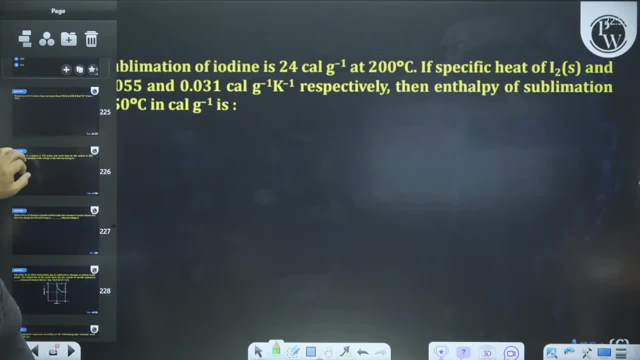 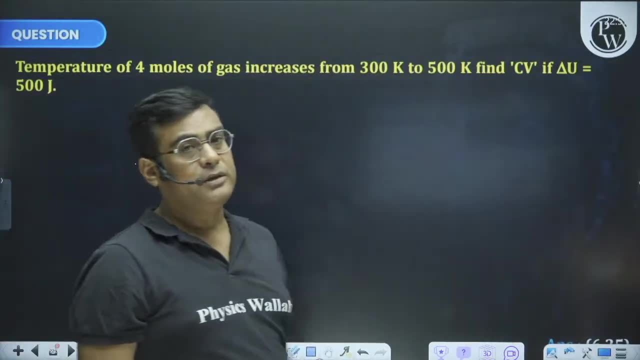 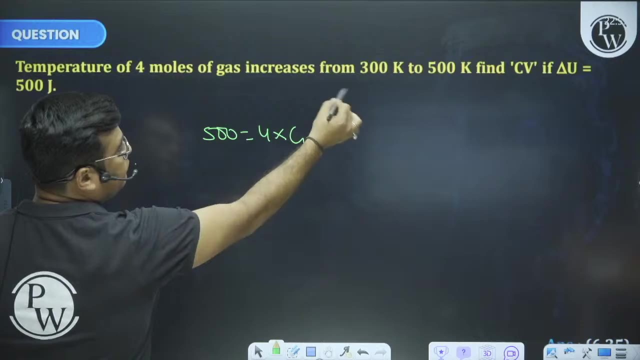 now you do this question, we will see some more. see this question has also come. temperature of 4 moles of gas increases from 300 to 500 cv. if delta U is 500 cv, so delta U is equal to N cv and I can see delta T is 300 to 500 cv. 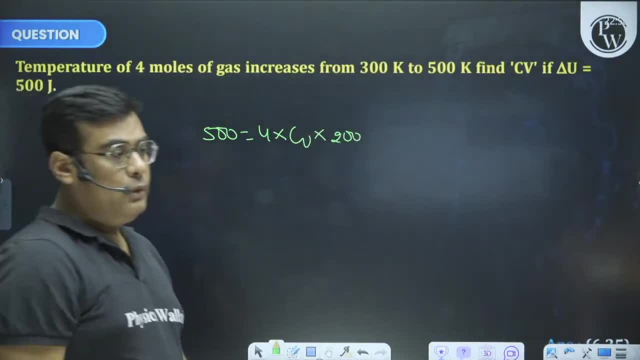 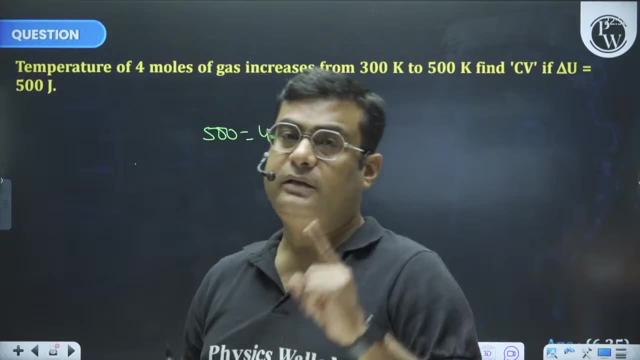 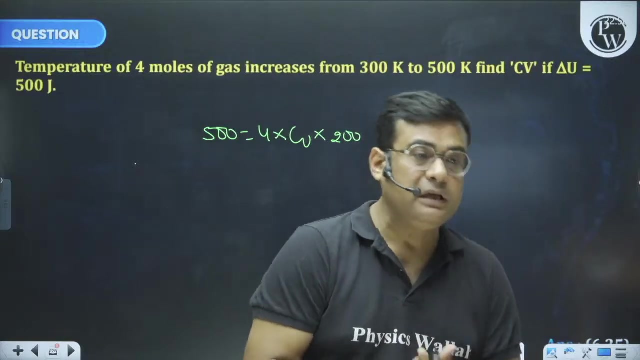 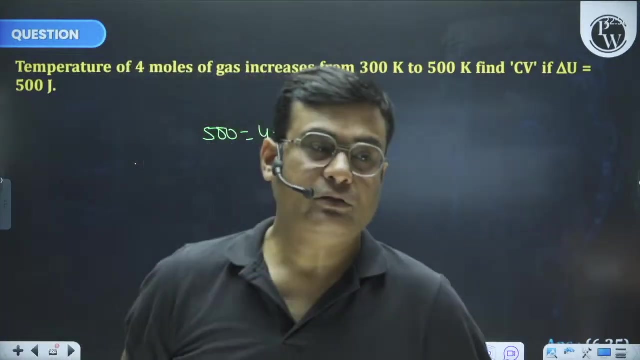 means 200 cv. you people think that JEE mains is a tough exam, but we start preparation from the beginning. just say this sincerely: stay together till the end. statement based questions will be from your theory knowledge. now I can teach theory. I can tell you formula based questions. 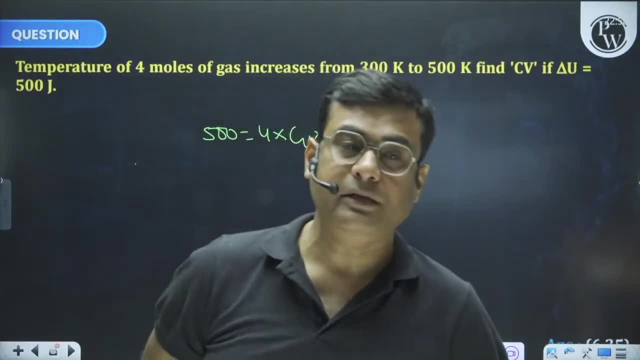 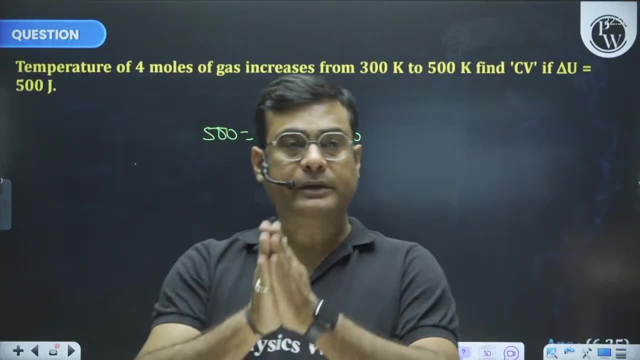 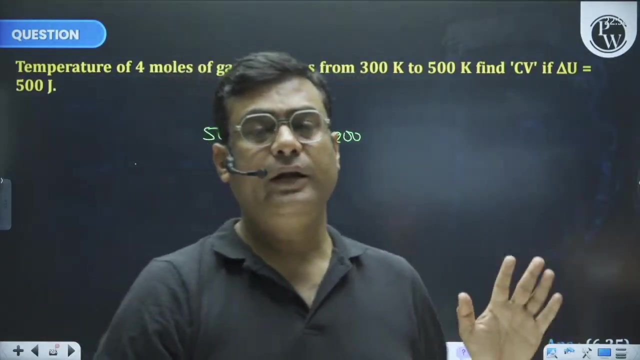 statement based questions. those questions will be clear in theory. if anyone has any doubt, first listen to these possibilities. you all know this 100%. if you want to get 99%, then you will correct 70% paper, you will get 99% and 70% paper will be easy, like this: 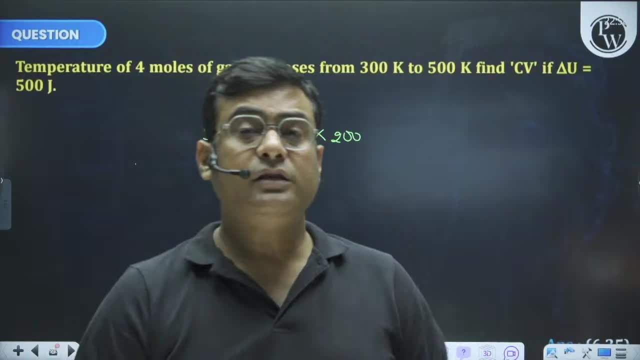 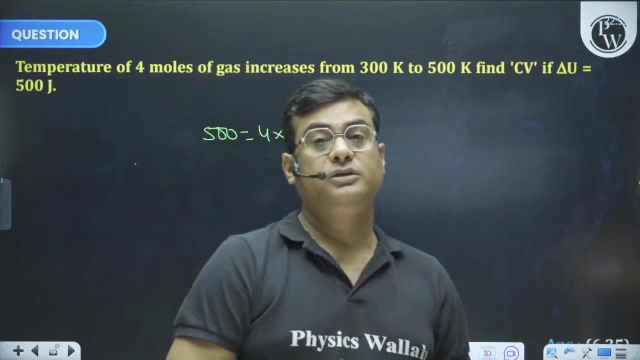 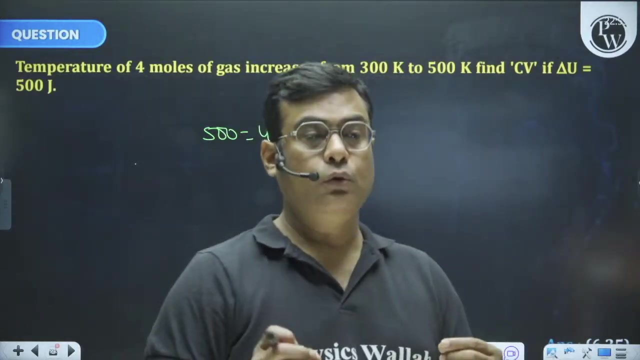 statement based questions will come 2-3 times. if you have to leave 30% of 30%, then you have the scope to leave 9 questions, 9 questions. think about things with your mind: how much scope I have. if mistakes happen, silly mistakes also happen. 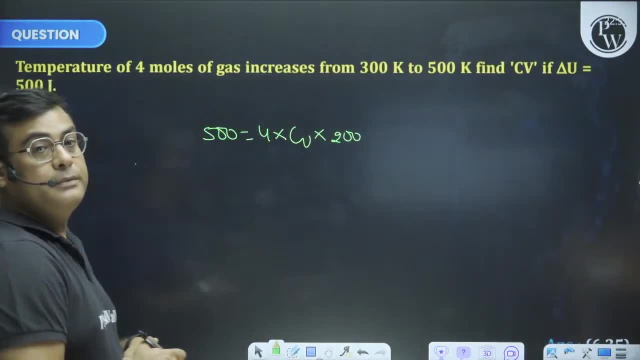 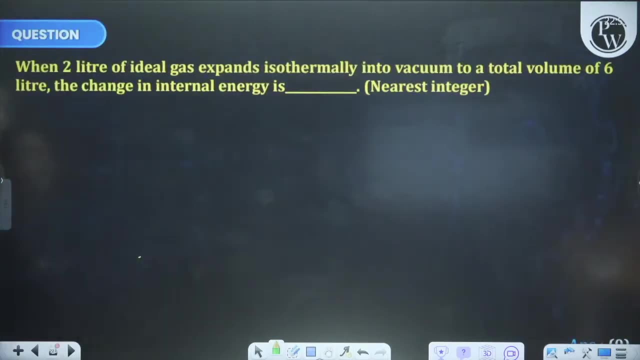 you are having the scope of 9 questions. you can easily ok my dear children. now this question has come: when 2 liter of ideal gas expires iso thermally into vacuum to a total volumetric liter change in internal energy? when he has said iso thermally? 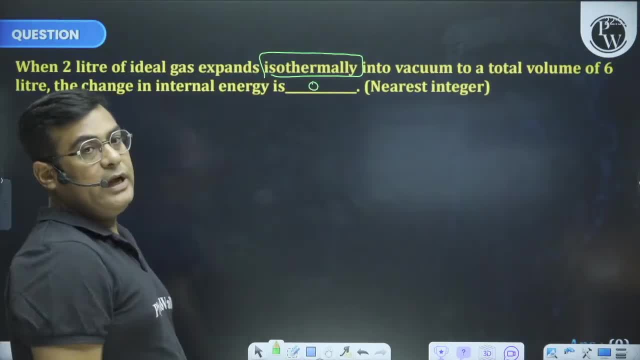 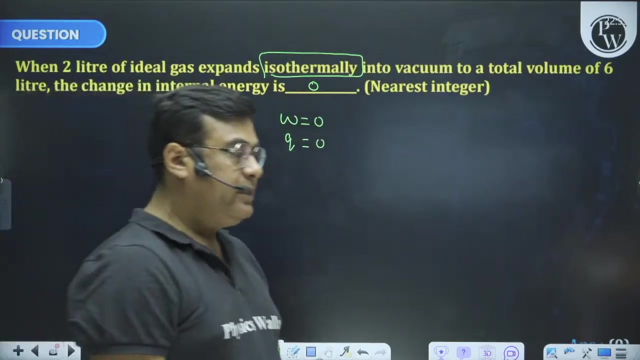 then internal energy change is 0, because for ideal gas delta u formula is ncv delta t. in fact, here everything will be 0, why in vacuum W is also 0 and plot Q is also 0, and you should know this is called free expansion. 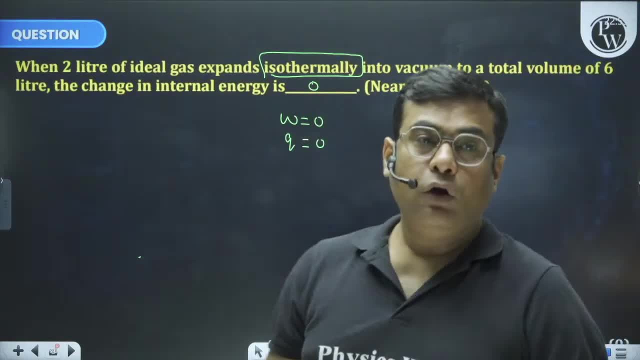 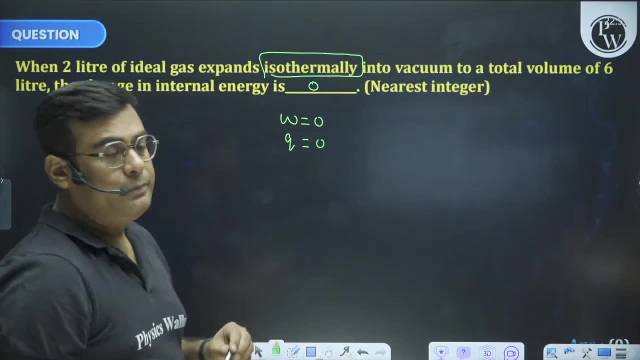 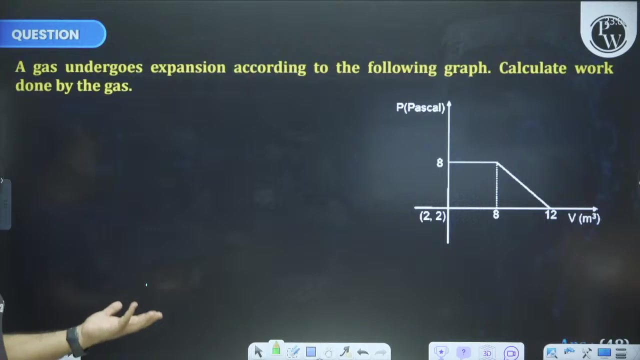 free expansion is an irreversible process. free expansion is simultaneously isothermal as well as adiabatic. free expansion is simultaneously isothermal and adiabatic. free expansion is simultaneously isothermal and adiabatic. now tell me what is the work done? formula can't you do? 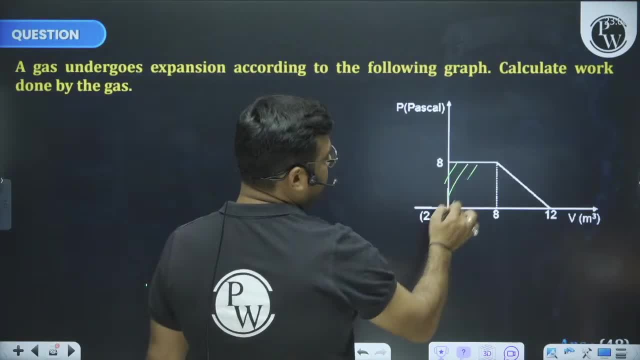 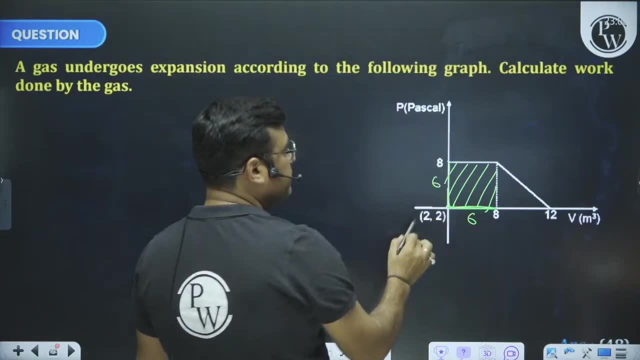 area under the curve in pv graph. you all know this is work done. this is a rectangle. 2 to 8 means 6. 2 to 8 means 6, so this is 36. this is a triangle. children triangle area is half base into height. 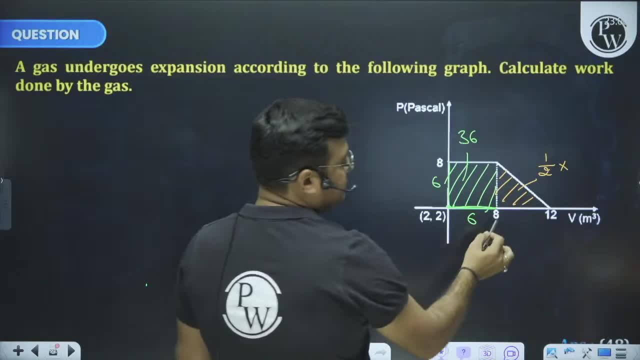 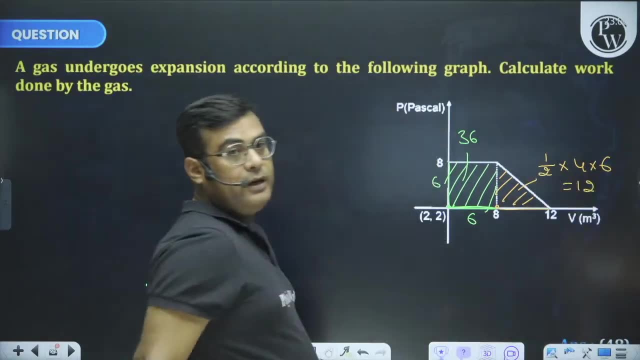 triangle area is half base into height. so half base 8 to 12 means 4. so half base 8 to 12 means 4. height is 6 only. so this is 12 and 36 plus 12 total is 48, and 36 plus 12 total is 48. 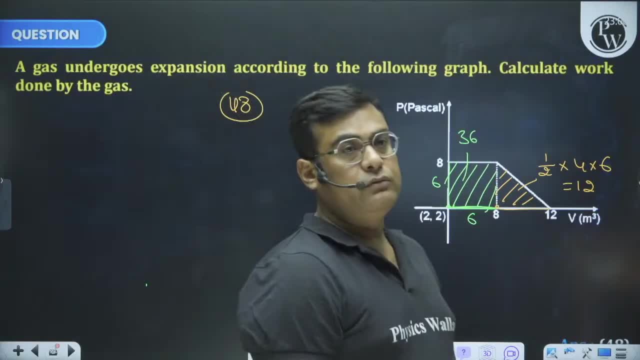 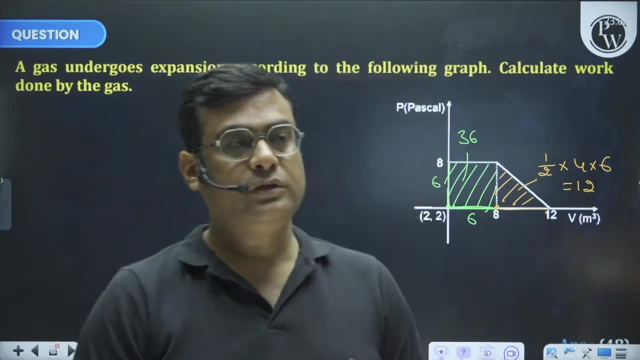 he has said work done by the gas. he has said work done by the gas, although he has not given any sign line: expansion or compression. so these things have not been discussed with us, so we don't need to worry about it. so we don't need to worry about it. 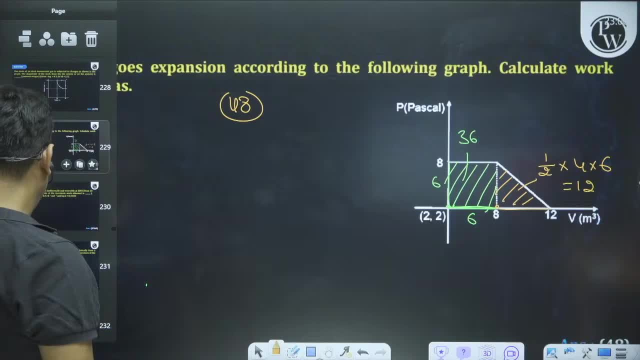 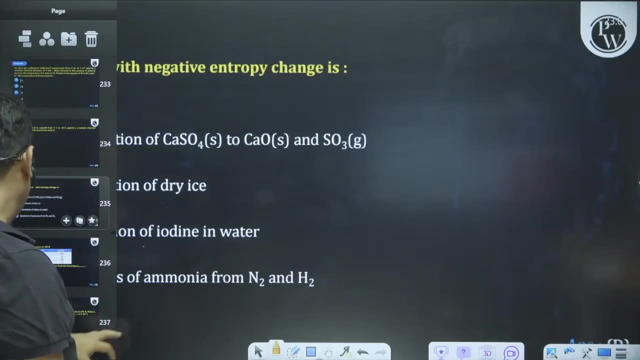 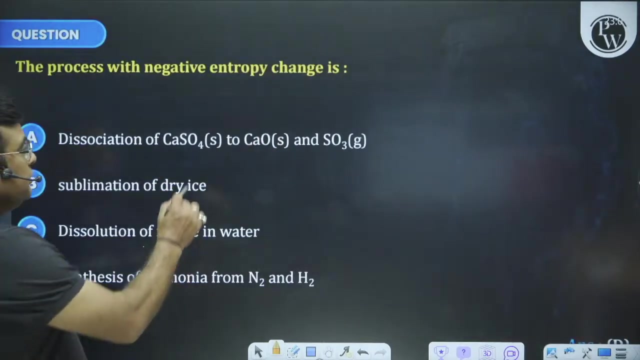 gave. what are those things? do you see any question so you can have an idea? now there are too many questions. same question, same question: see entropy change process with negative entropy process with negative entropy change distance� didn't have the based on it made a gas. 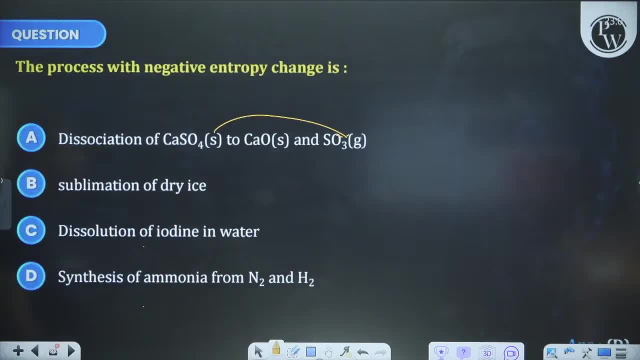 it is positive, get sublimation of dry ice. dry ice must all sublimation because I got a solid to get. this is also positive. dissolution of iodine in water via iodine 30 CB. ever dissolve with the hair taken at those solids. a cross form may. 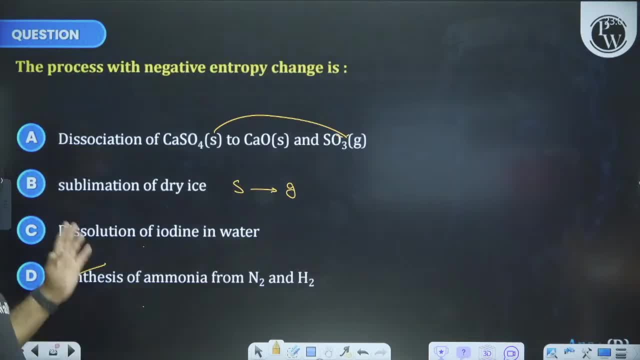 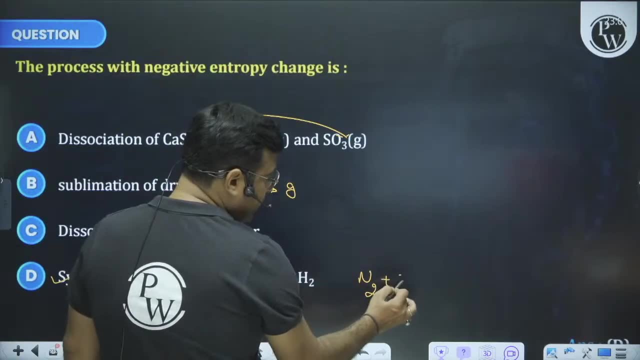 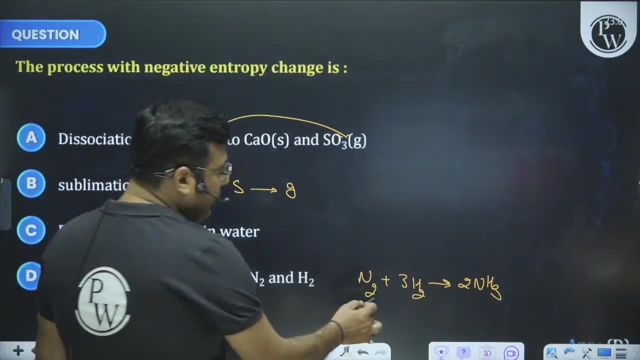 die, but Jana to come here, but Jitra be so. but she got a synthesis of ammonia from n to n is to kill. key is key. reaction. Bharat verse: K harik kone kaba chajanta Hoga shed 910 so say. but I'll be enough to end to gas, plus 3s to gas. 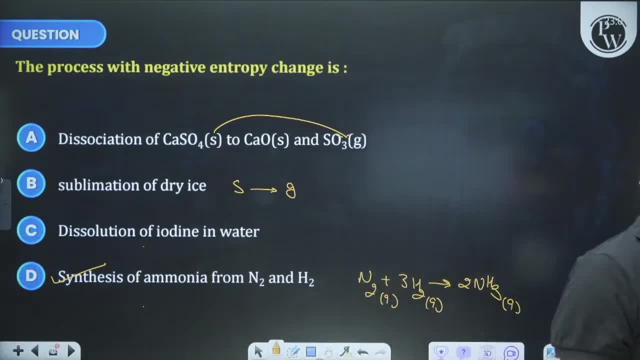 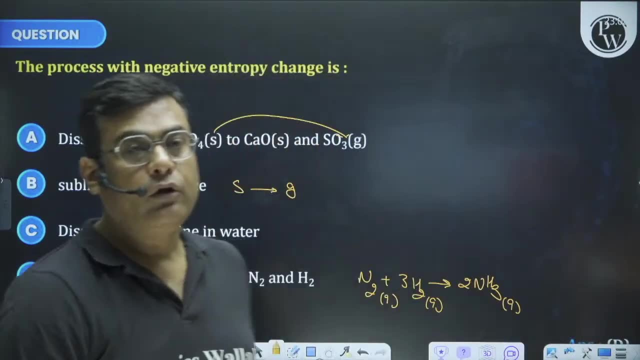 gives to an ecstasy gas up, they expect to escape. in time GK I saw this car in time G. negative a or other delta NG negative a watch on the paca isca. paca isca entropy change- we go over negative now gives energy. the question we see: 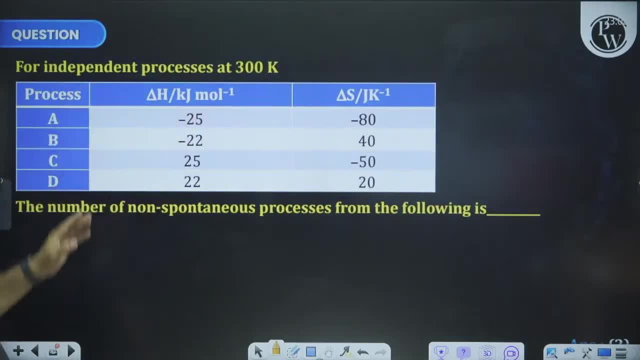 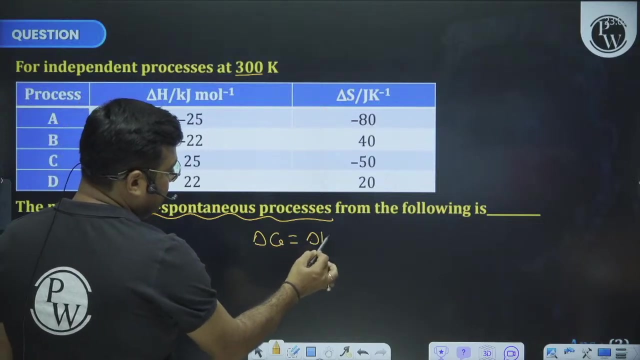 related hotel up coach our processes: de Gaia, delta G, delta H or delta s push ahead temperature in so number of non-spontaneous forces in teaser, type me non-spontaneous forces via delta G, kappa or mula duniya me kiss but check on a but I but oh yes. 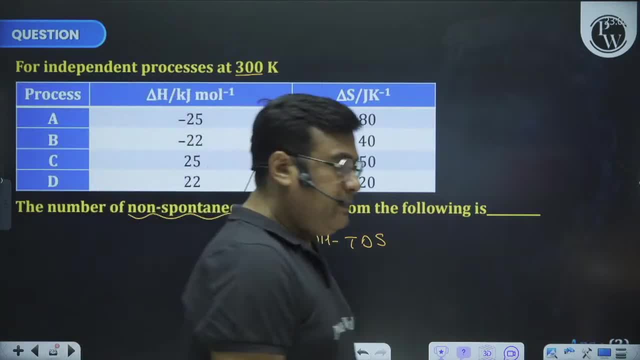 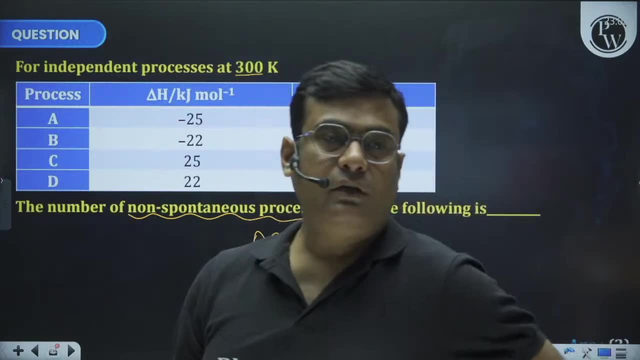 impulsive or mula much heavy. but I bet a gift energy say: kitana de la cata, I'm a much a be. looked at a cookie. this is a big of a booty. we say he teacher big of a student. ah, this is a big of a booty with a teacher big of a student of it, ah. so how many be hallowed? 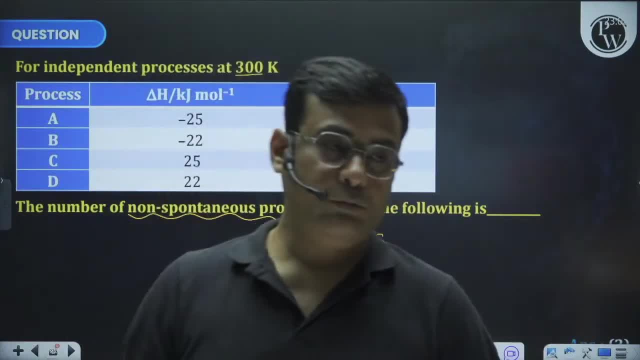 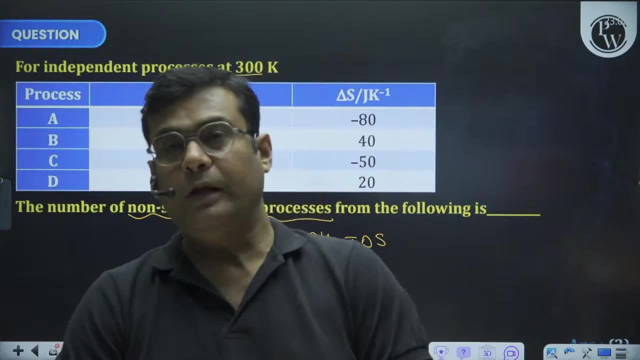 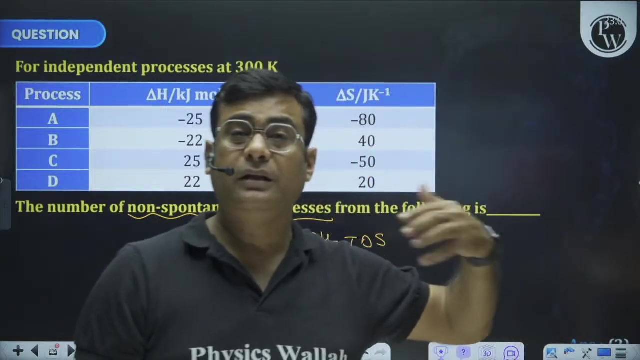 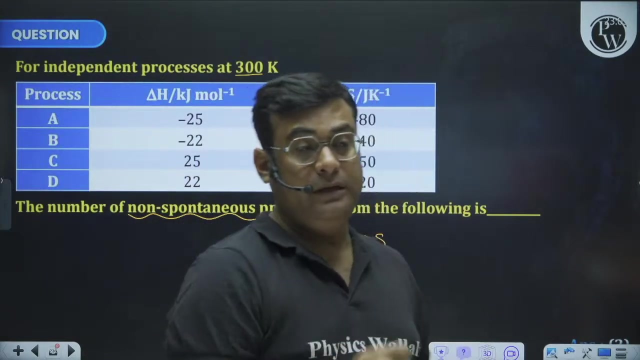 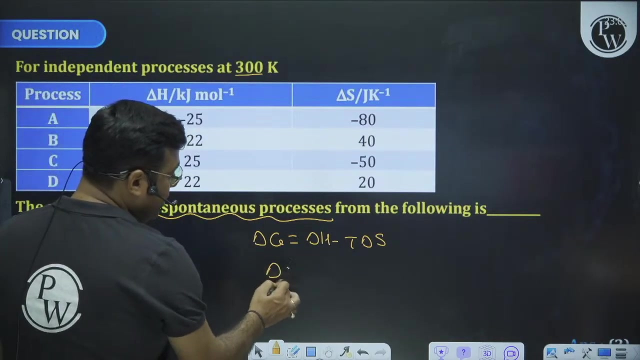 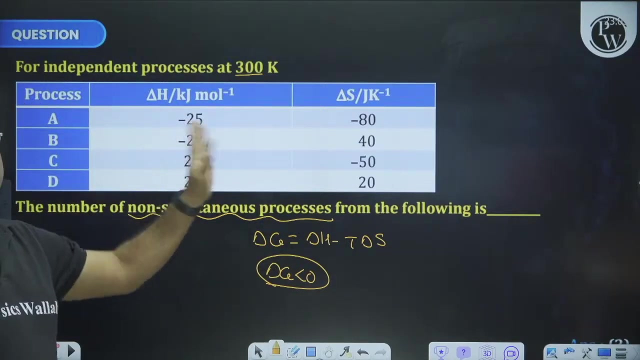 Khabib fis провola Durya Monterrey. you come, okay, you, Khabib Khas, in Amha, and the one whose delta is negative will be spontaneous and the one whose is positive will be non-spontaneous. you will get such simple questions. 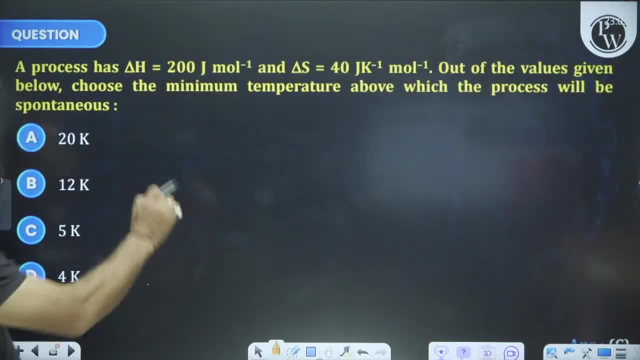 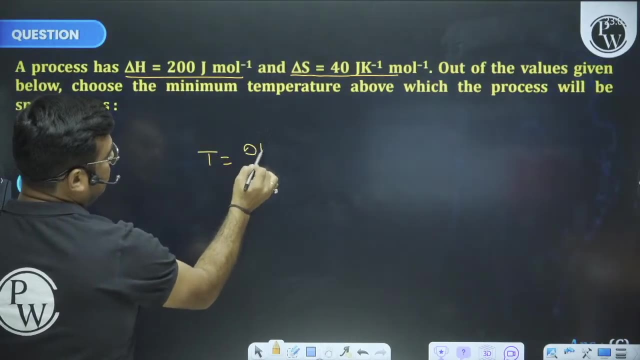 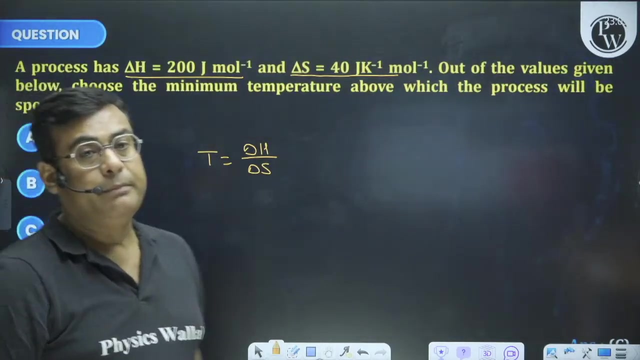 now process says: delta is 200, delta is 40. out of the values given below, choose the minimum temperature above which the process will be spontaneous. take out the temperature delta H upon delta S ratio: 200 by 40 means 5. go above the minimum temperature. 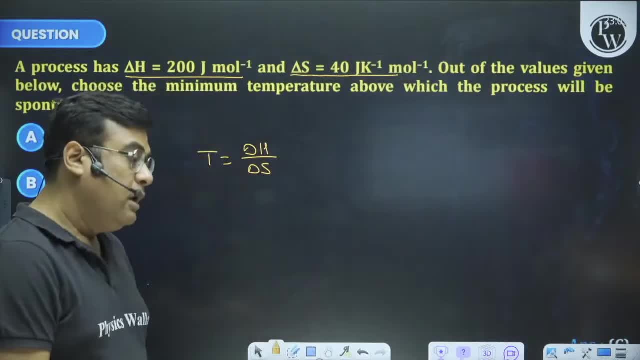 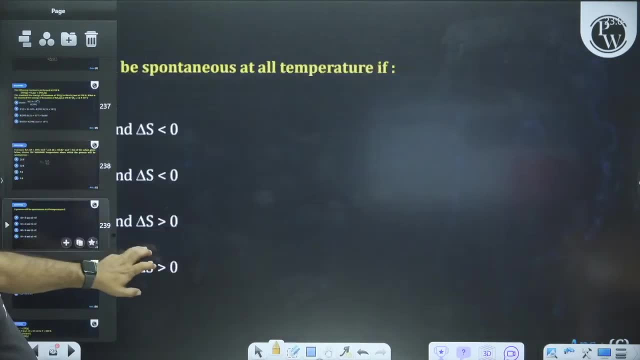 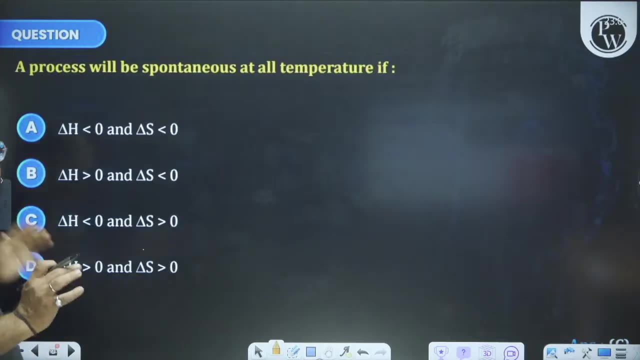 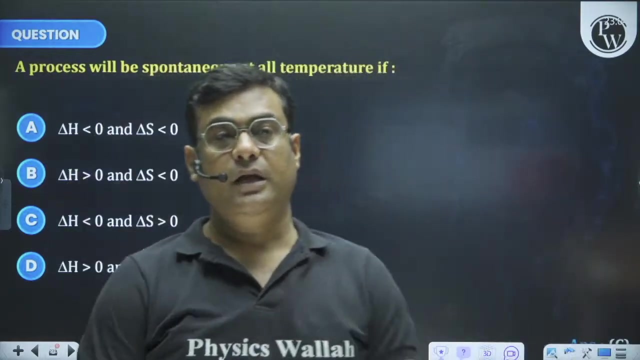 your process will be spontaneous. after going above 5, your process will be spontaneous. now everyone understood. see again: process will be spontaneous at all temperature. when will be spontaneous at all temperature? spontaneous means energy content wants to reduce every system and entropy content wants to increase. delta H is negative. 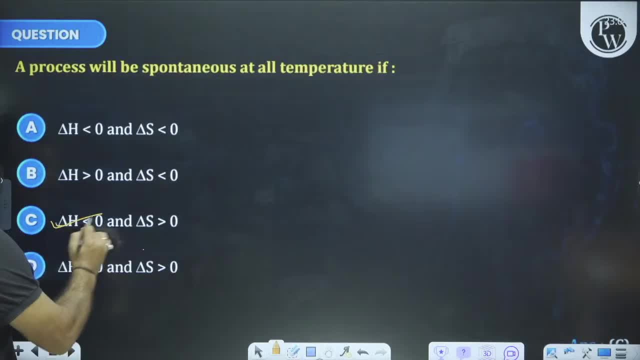 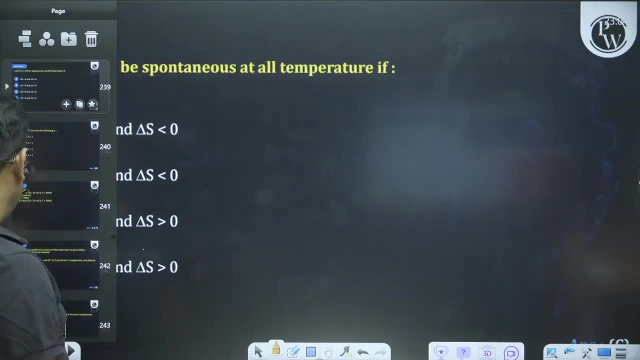 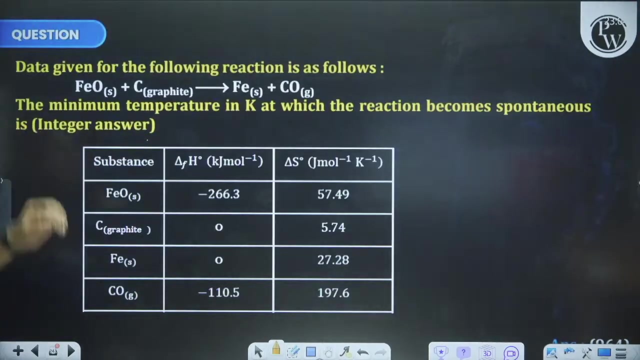 and delta S is positive, such a condition of process will always be spontaneous. I am also asking questions of thermochemistry. it is part of this. questions of thermochemistry are also very easy. this is not thermo. this is the question of delta G. now the question is directly from 245 to 200. 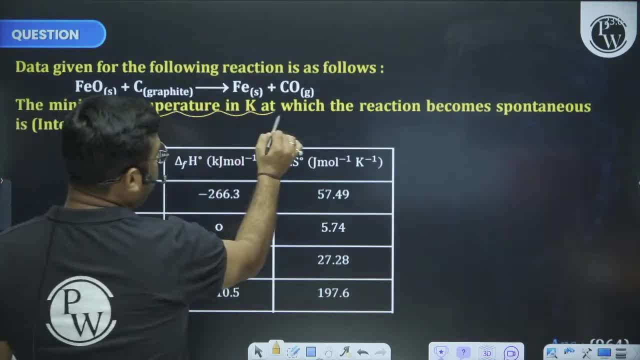 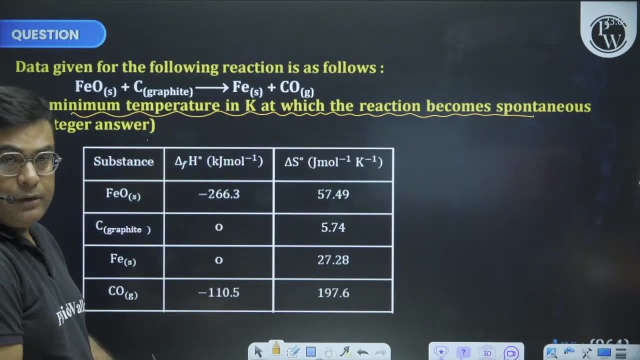 now, this is also the same minimum temperature in Kelvin at which the reaction becomes spontaneous, is it? ok, the question is the same. but now what to do in this? in this, you have to take out delta H directly, and you were saying thermochemistry, in thermochemistry, if you have to take out delta H of any reaction, 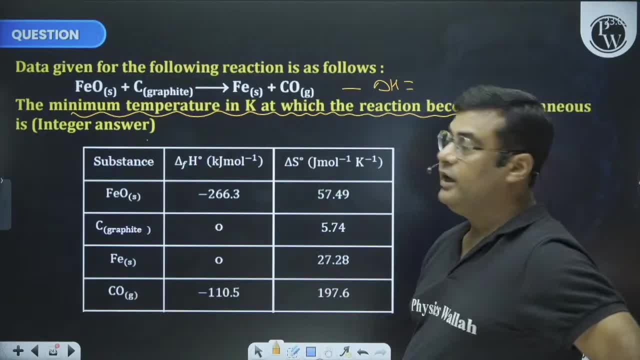 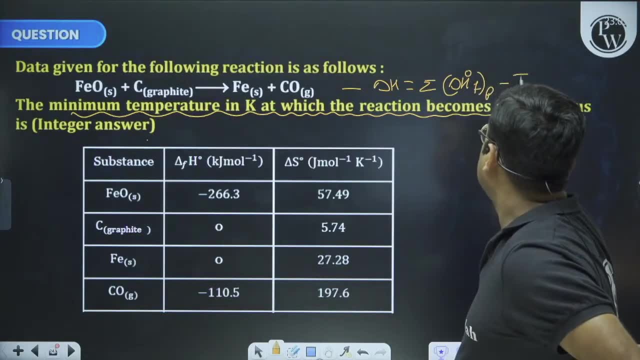 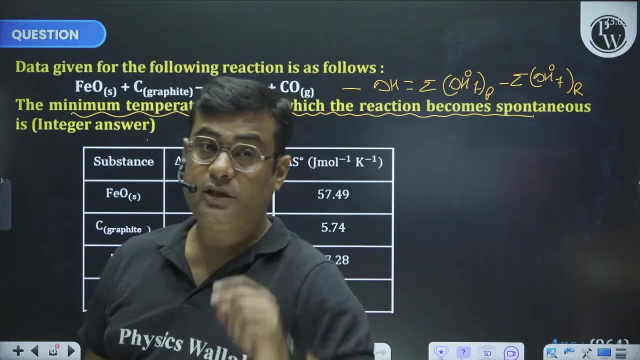 with the help of formation, with the help of formation. so what is the formula? summation of enthalpy, enthalpy of formation of products and minus summation of enthalpy of formation of reactants. and in that also you will know the condition that IUPAC has said one thing. 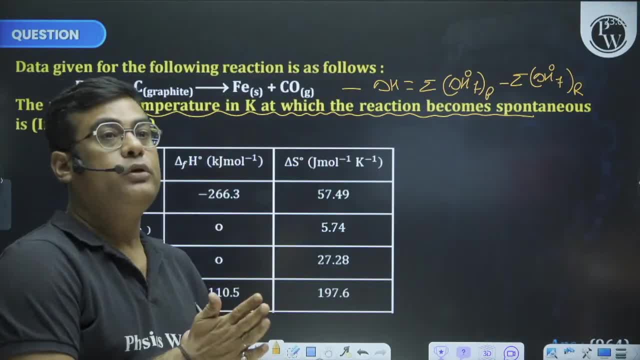 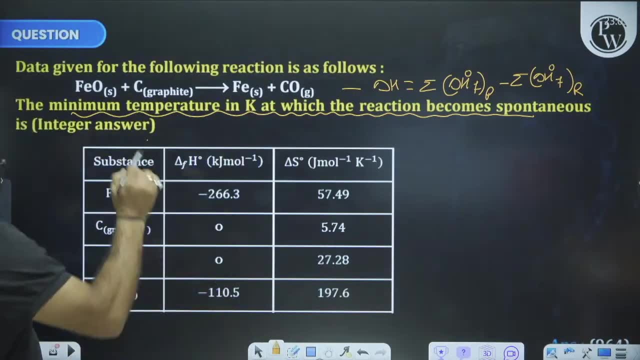 that if the elements are in their substance is in its pure and stable form, then its enthalpy of formation is zero. so here, C graphite will also be zero, FE will also be zero. see, they have given. so you have to take out delta H, whose product means CO. 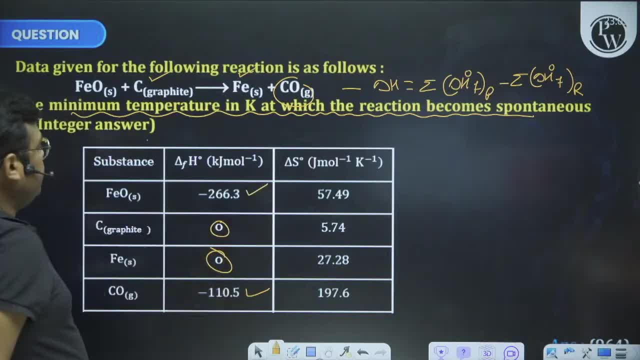 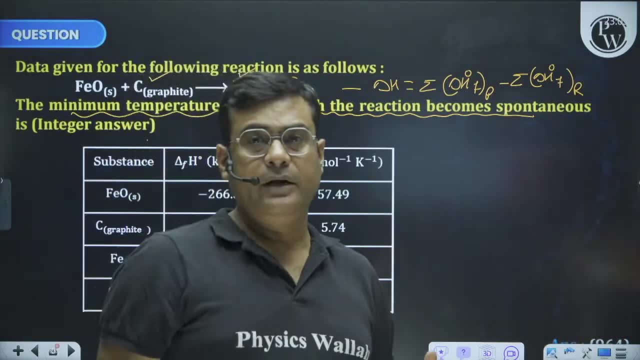 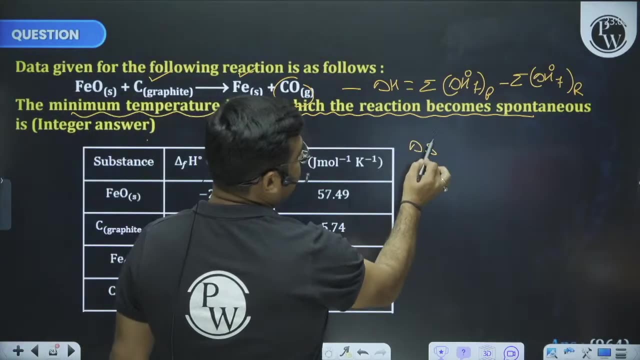 this is the value: reactant means whose FEO. this is the value. now, this small calculation, this small calculation you will have to do, this small calculation you will have to do, and here, how to take out delta S. this is also the formula to take out delta S of any reaction. 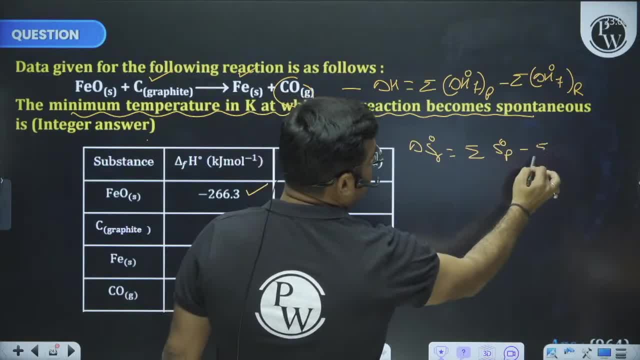 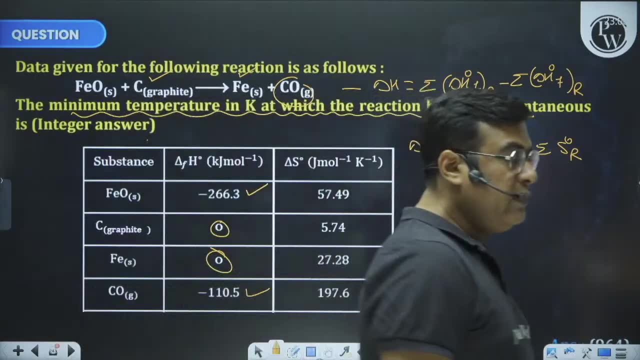 summation of entropy of products minus summation of entropy of reactions. entropy is of others: 0. absolute zero temperature has not been said. so it has not been said. that is what is your process now. that is what will be the entropy of all the children. there will be values. ​​and if there will be values, then 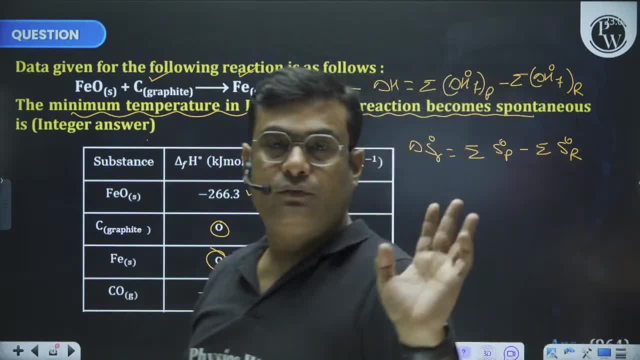 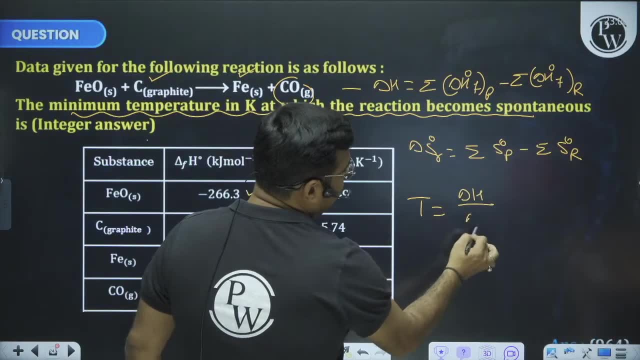 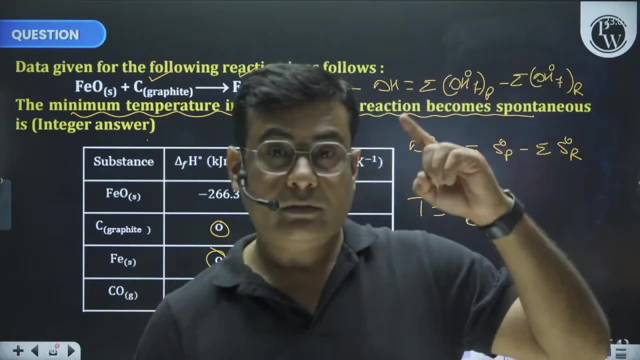 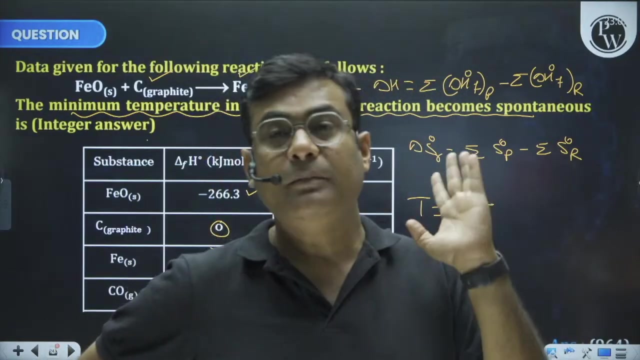 you will just apply this formula. apply this formula, take out their values ​​and again apply the formula for the temperature: delta H upon delta. now, this is a little game of fate: day and night. Fate is the day of hard work. What is it? that's all. and we say, son, that man's courage is the help of God. 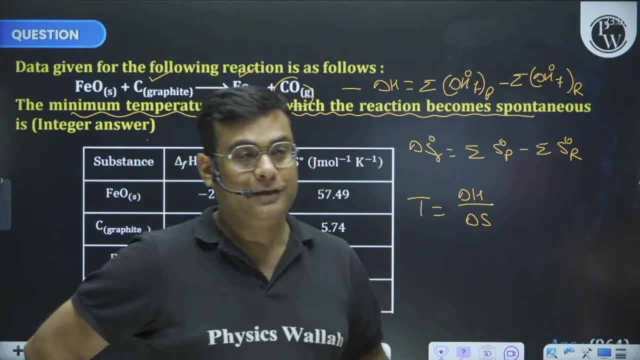 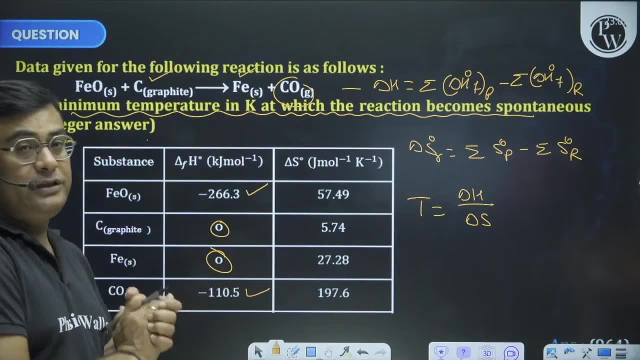 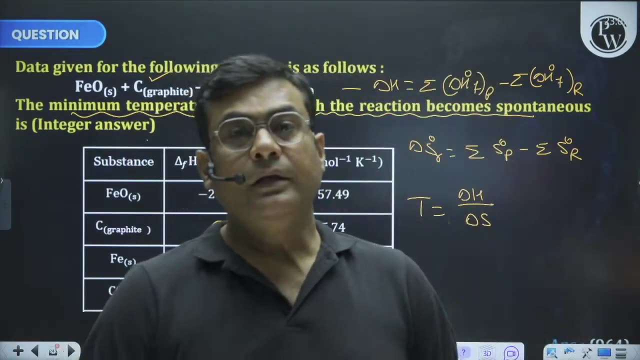 What are you trying to say, then? I don't know what the time is happening. is it time for you to sleep? No, it is nothing like that son whose fate will be good. what meaning is good? son, obviously throughout the year, works hard, sincerely right? okay, the sincerely working. 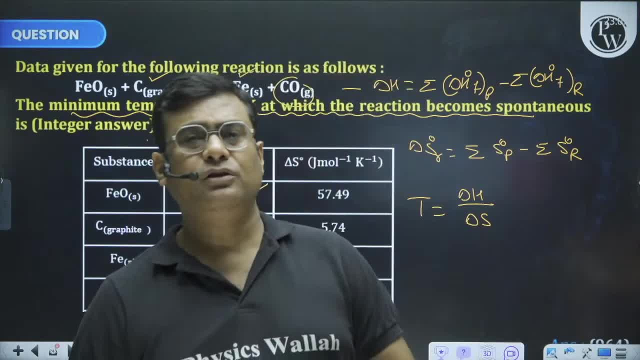 hard, the sincerely working hard. to work hard, it is good, right. the sincerely working hard. sincerely working hard: it is good right. the sincerely working hard, honestly working hard. He works hard and gets the blessings of the teachers and the parents. 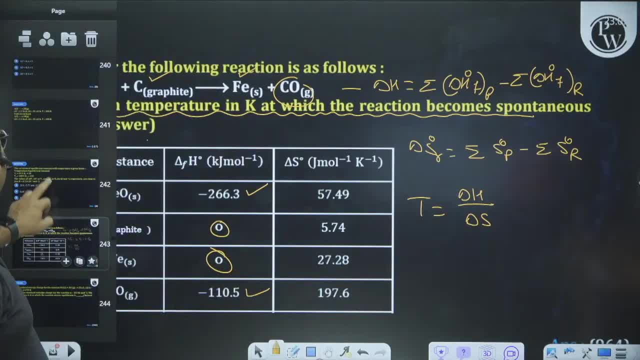 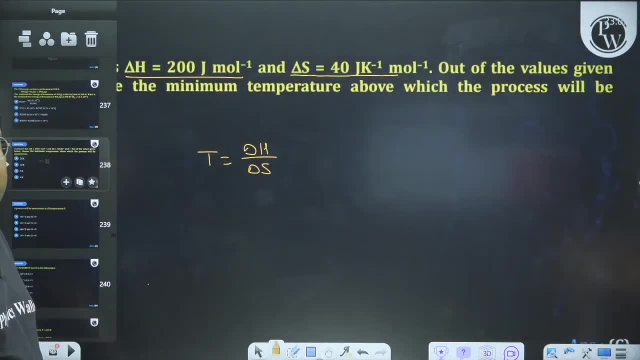 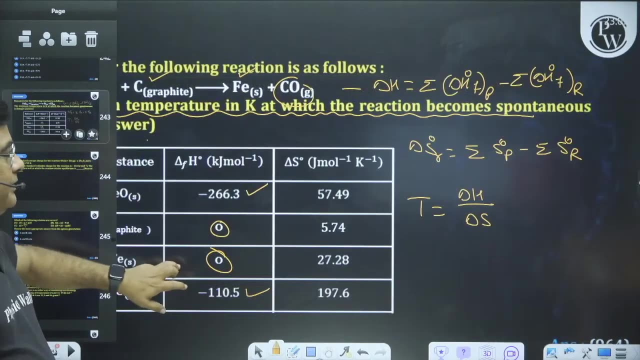 So now they will get this kind of question. He was given a direct value of delta H and also a direct value of delta H, But those who have not worked hard, who are already afraid, will get such questions. So this is the rule of fate. this is the rule of fate. that's why we have to work hard. 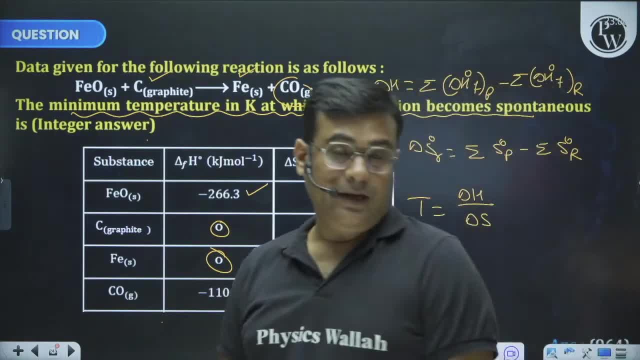 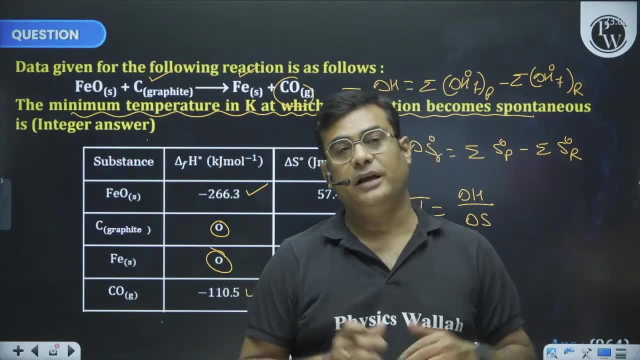 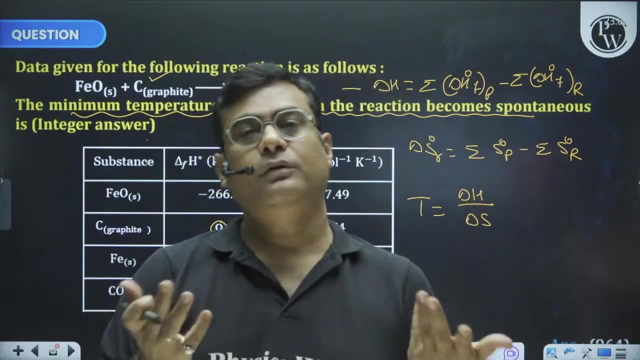 brother, whatever work we do, we have to do it with determination. it is not like we have paid the fees, we have taken the course, there is nothing left to study, so then they will be somewhere in the end. in this way, that universe, even if someone is watching you- 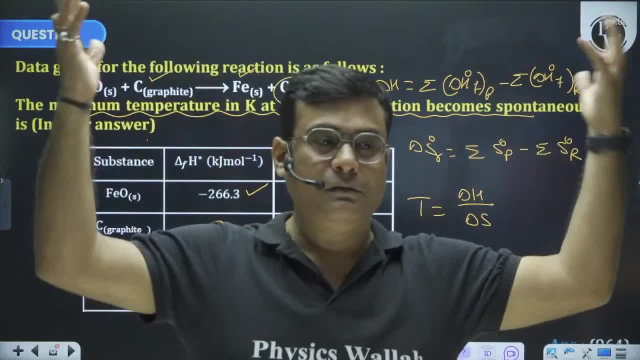 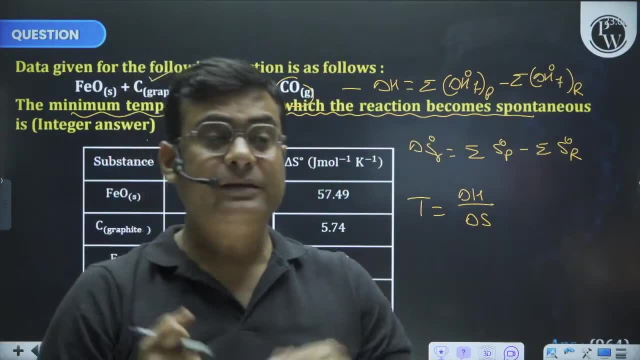 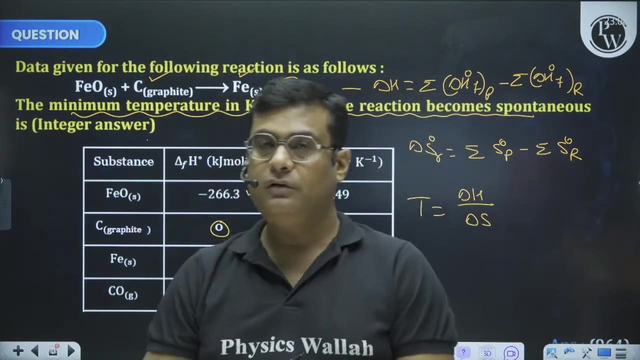 the universe. Many powers are present in the universe, so they are watching. why don't the hidden powers that we don't know? so someone is watching you and whoever is doing their work with honesty, that brother right, That universe's powers also do some kind of support. 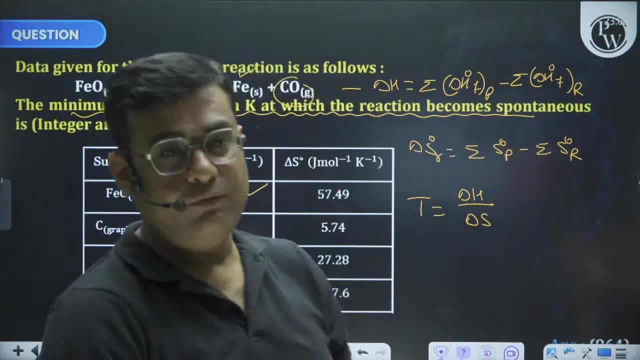 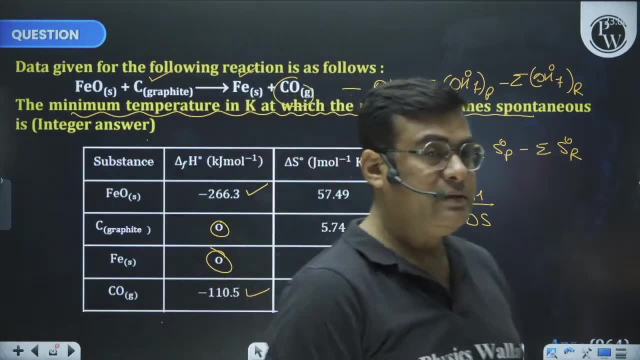 It's light. right, it's light. try it. sir, tell me a little strategy to attempt the paper based on me. the paper is always according to me. then we have to do it. I have to do it According to me you have asked. then I will talk that you should start with chemistry. 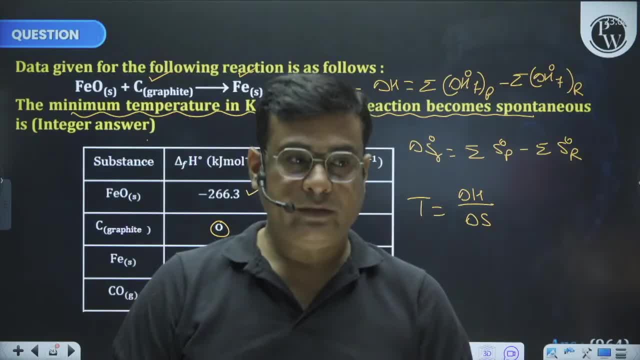 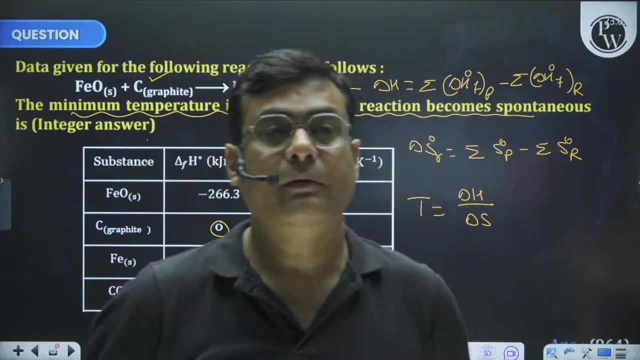 Chemistry remains easy. You have to assume that if there are 30 questions in a paper, then 30% of it means up to 9 questions. You can get tough or unmanageable people. You do not understand anything by looking at them, by reading them. 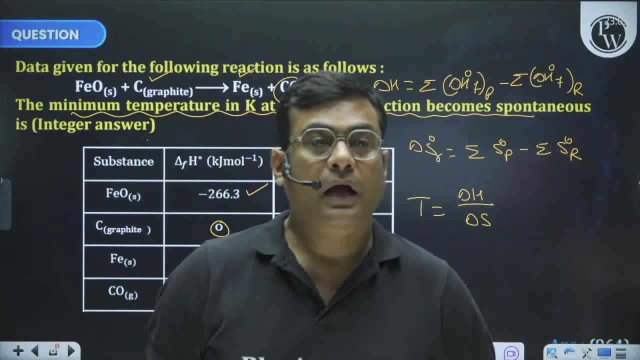 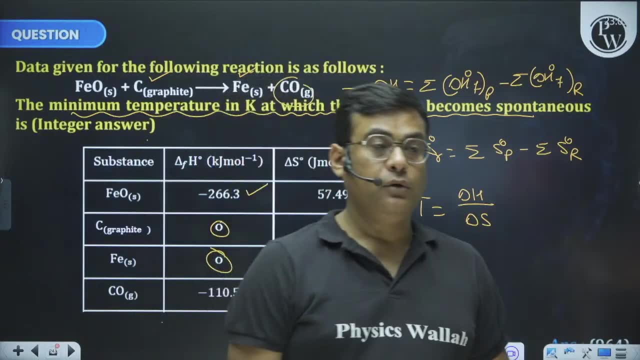 So do not be afraid. It may also be possible that you may get stuck with 3-4 questions from the beginning. Your luck may not be good on that day. the day may not be good, which is not being made by you. 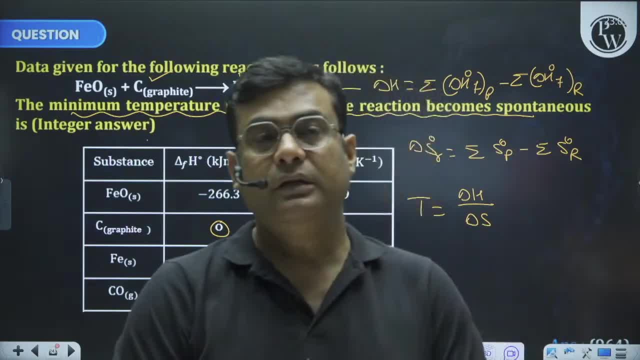 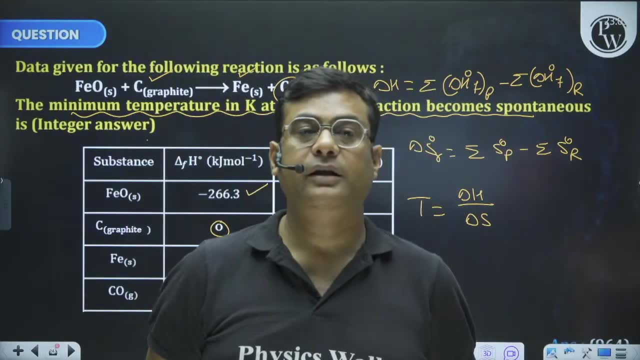 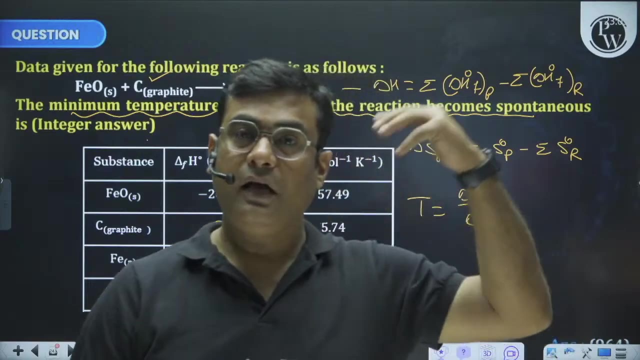 But if you are mentally prepared- that I have the respect to leave up to 8-9 questions- I have space- then you will not be afraid of those 4-5 questions. You will not be afraid. But if you do not have any planning in your mind then you will be confused after not having 2-3 questions. 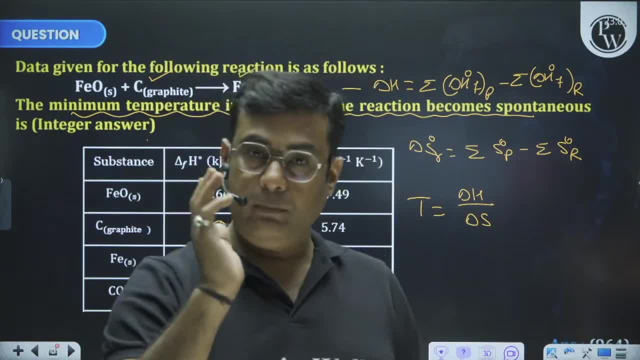 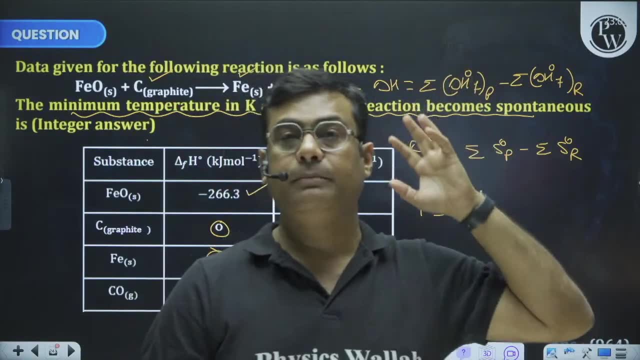 And after that the questions will come. You will also do something wrong. So keep this first in mind. You have to start with chemistry. You have to keep a scope of 5-6 questions up to 7-8-9 questions. 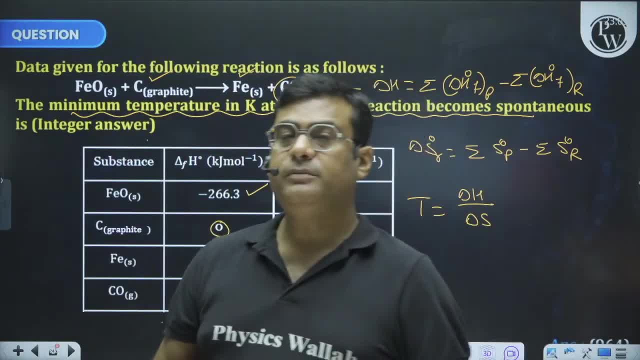 So that your paper will be on its own. Second subject is your choice. If your physics is good, then physics. If math is good, then math, And if it can be done in chemistry, then try to save a little time, Because the paper of chemistry is never going to eat your whole 1 hour. 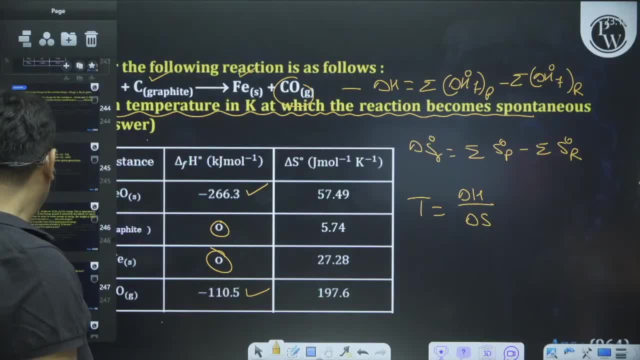 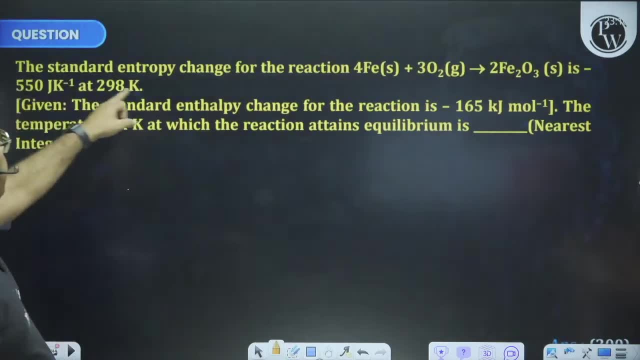 Okay, It is not Okay. And if you ask questions about thermochemistry, I am telling you guys, See, this is a formula-based question. It has come once more. This is it: Standard entropy change for the reaction is this much. 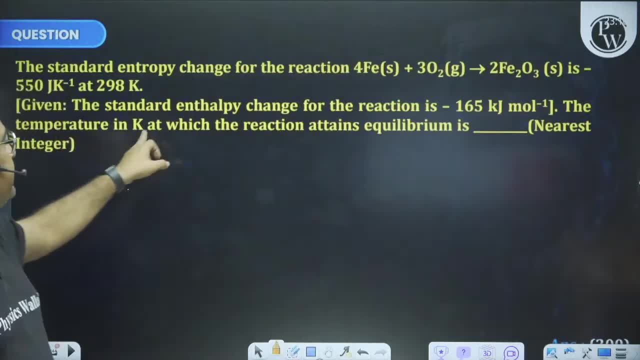 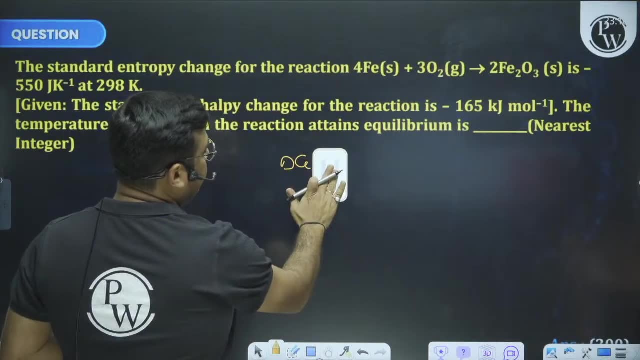 Given standard enthalpy change for the reaction, the temperature in Kelvin at which the reaction attains equilibrium. Now, what does equilibrium mean, son, Where delta G is zero? Equilibrium means that where delta G is zero, then indirectly it is asking you again the. 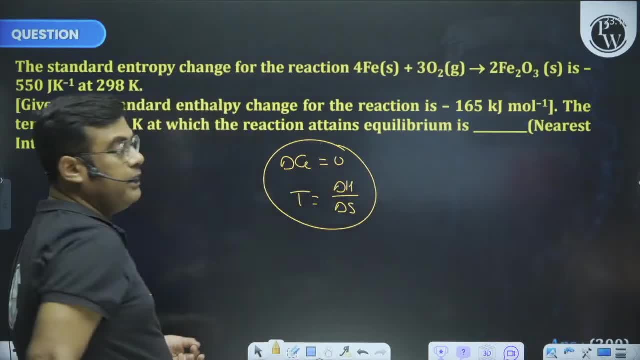 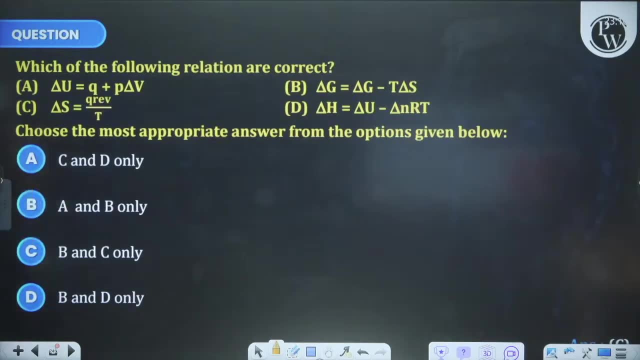 ratio of delta H upon delta S. Indirectly, it is asking you the ratio of delta H upon delta S. Okay, Now you look at the formula-based question also, Which of the following relations are correct? Delta U equal to Q plus P. delta V. 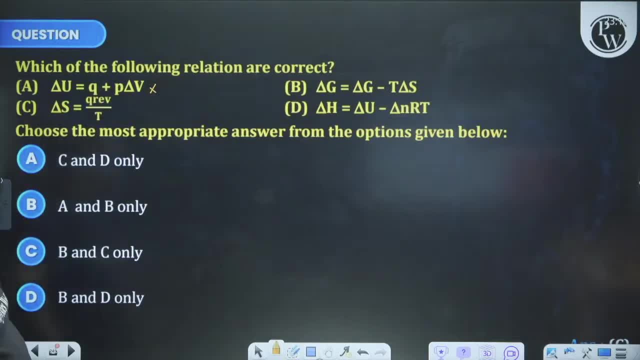 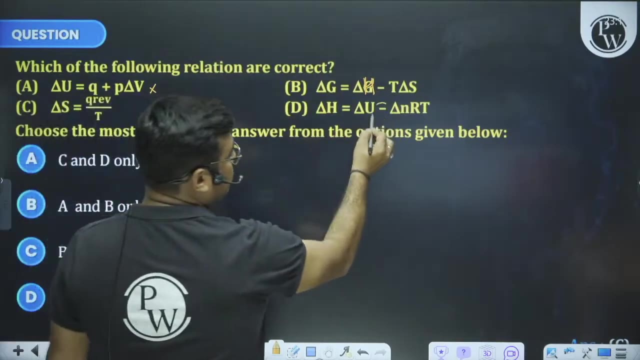 We will consider this wrong. Why Minus P, delta V should be for us Del G equal to. this is operator's mistake. Delta H minus T, delta S is correct. Delta H equal to Q, reversible by T, And del H equal to del U plus delta NGRT plus should have been given minus. 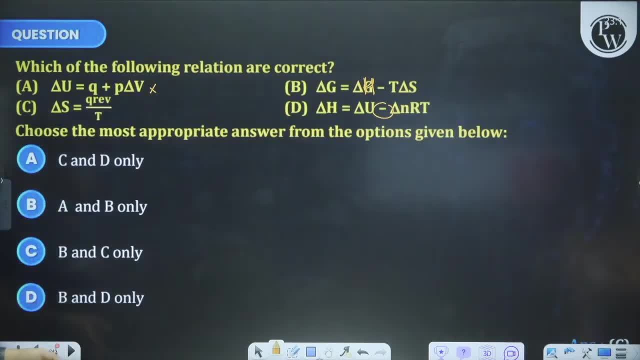 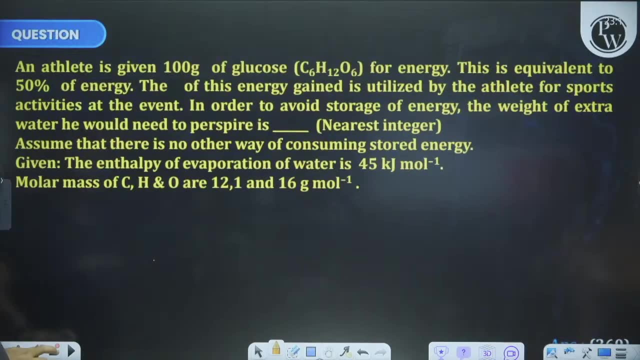 So B and C are correct In this way, formula-based. See, we have done so many questions. Now you think, come on, it is thermo-chemistry, This is thermodynamics. Shall I show you some questions of thermo-chemistry too? 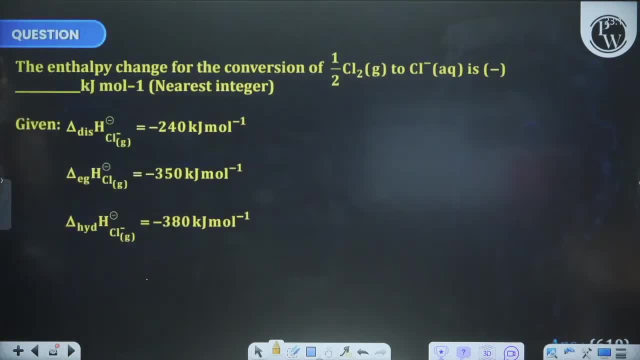 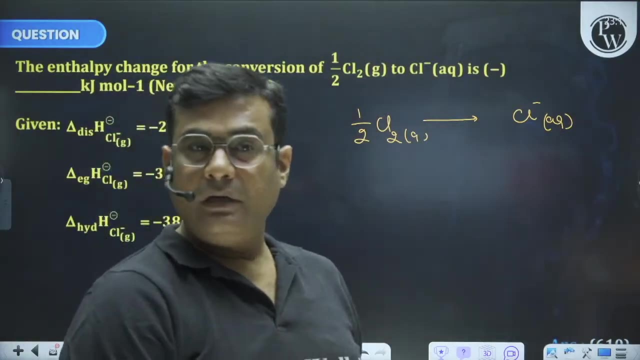 Here it is. We also have some questions of thermo-chemistry: Enthalpy change for the conversion of half Cl2 to Cl minus. Do we know how to convert it? This process, will it be done in one go? No, It will not be done. 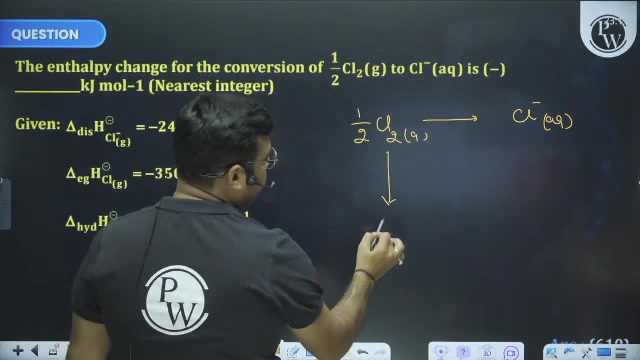 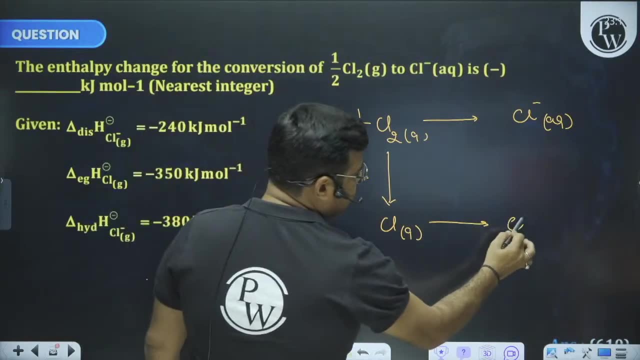 How will it be done? Right, Half Cl2,. first you will have broken its bond Cl gas. So here you will need half of the bond energy. Then you will need Cl minus gas plus electron Means. it will be applied here electron gain enthalpy. 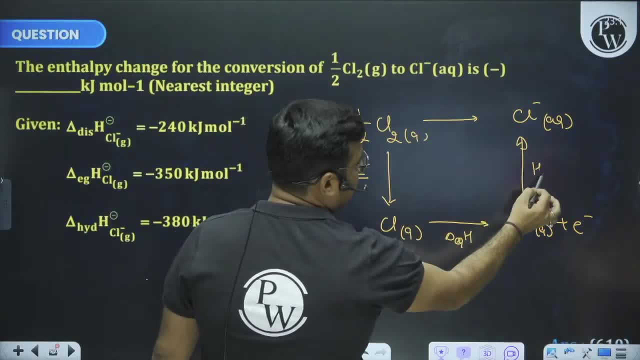 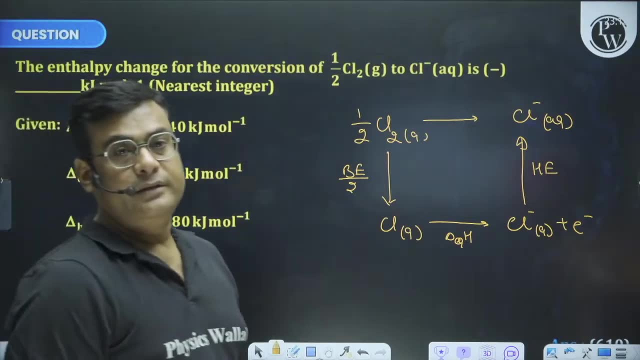 And then Cl minus gas to Cl minus aqueous Means. it will be applied here: hydration enthalpy: Right. The values of all three will be in front of you. Just add Right. All three will be added in this way. 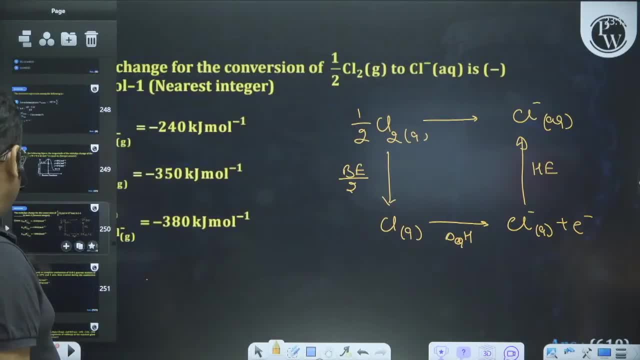 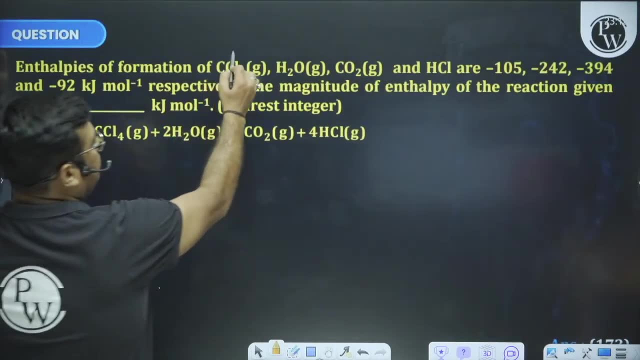 So thermo-chemistry, thermo-chemistry- many children are afraid of thermo-chemistry. Sir, what is thermo-chemistry? Hey, thermo-chemistry is also very easy Enthalpies of formation of this, this, this and this are: this, this, this, respectively. 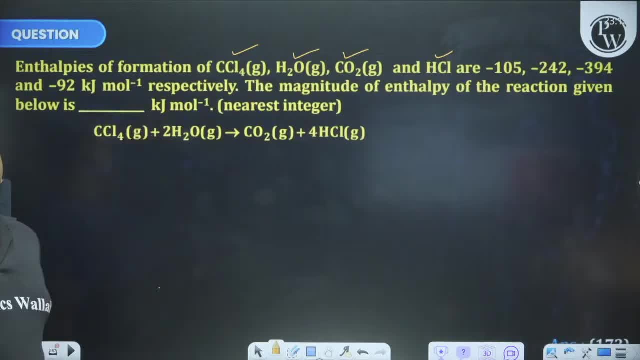 Magnitude of enthalpy: change of the reaction given below I just told you, children, Enthalpies of formation of product CO2 is given. This is always in per mole. It is important to keep this in mind. Now you have four. it has four moles. 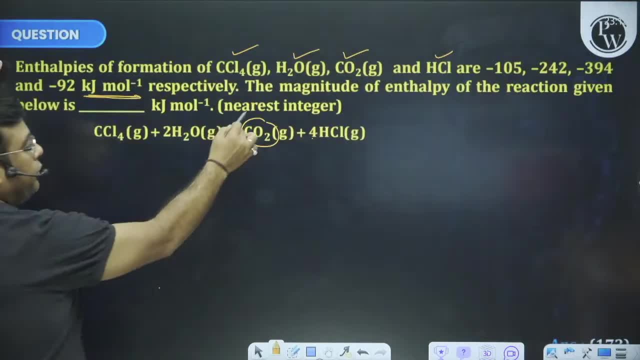 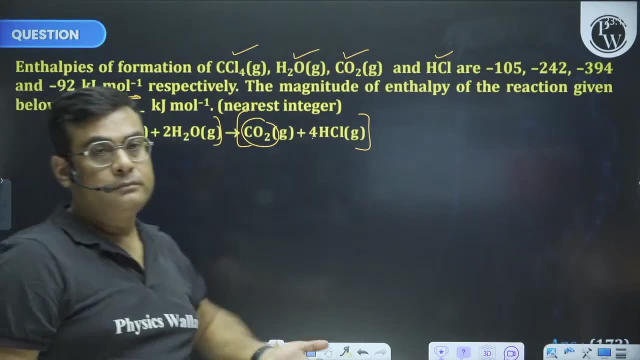 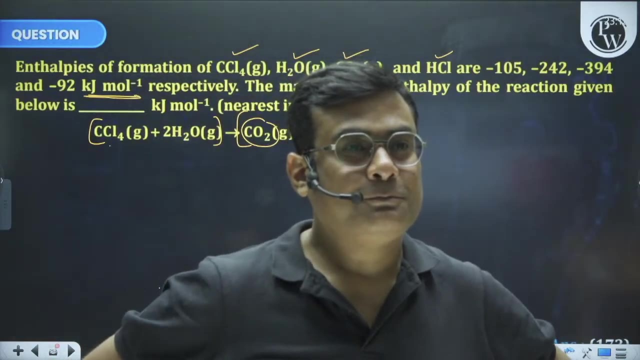 So you have to multiply its value by four. This is the product, Minus reactant. It has only one mole. It has two moles. Take them out separately, Minus both. Someone got angry with me. I had such an anger. 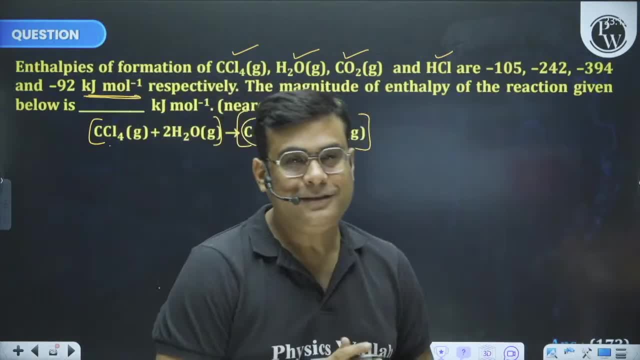 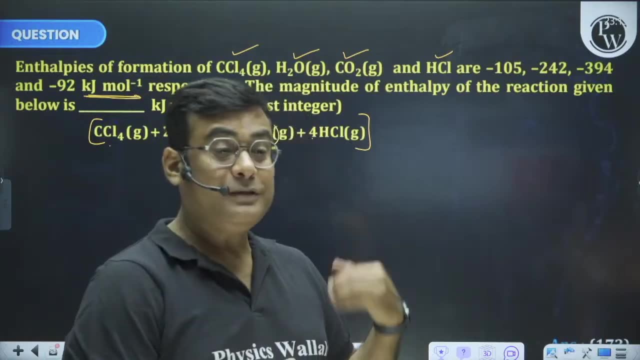 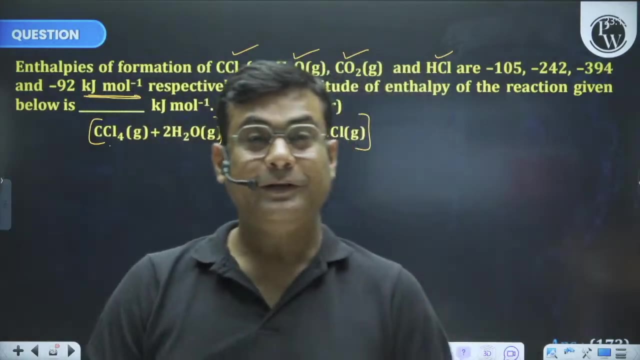 Right, Such an anger Did not see anywhere. Don't do this, my son. I'm just asking the questions, explaining. See that there is a question, Otherwise it will take five, five, ten, seven, seven minutes If you go to solve everything completely. I am explaining to you what to apply in which question. 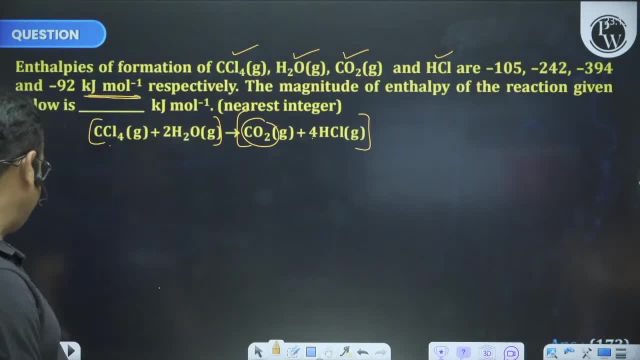 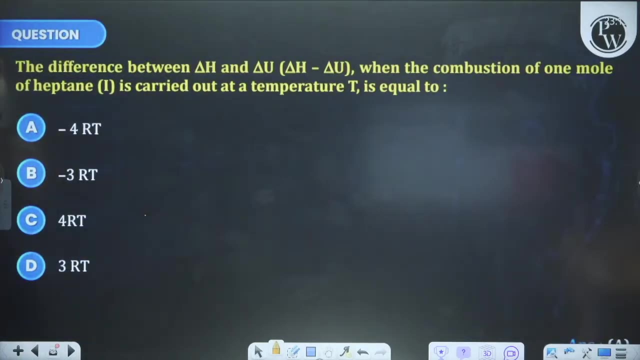 So that you can read it easily and understand. Okay, I am trying to explain that. Okay, Okay, Come on. So This is also a question that comes to the children. Difference between delta H and delta U when the combustion of one mole of heptane is liquid. 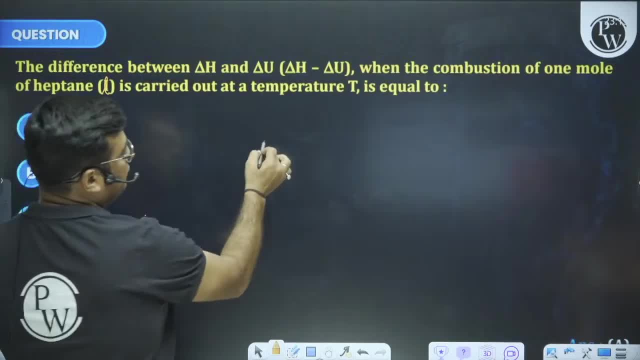 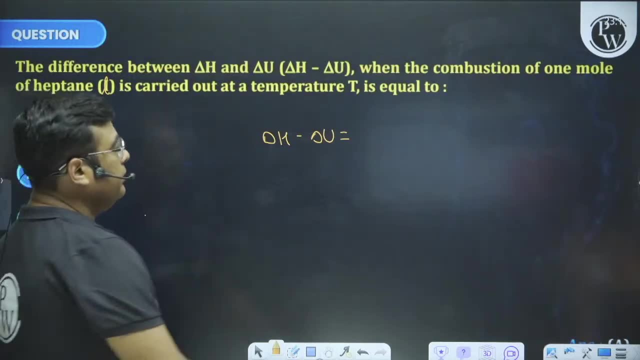 is carried out at a temperature T is equal to. Now I said delta H is equal to delta U plus delta NGRT. So here you have been asked: delta H minus delta U, So this will be equal to delta NGRT. Now, if you do it, then I am also telling you that you just think that what we are doing is right, or not? 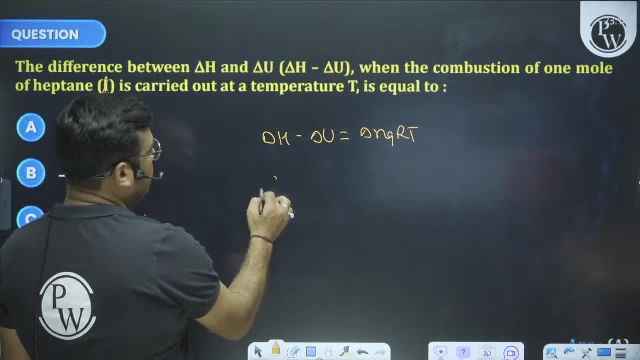 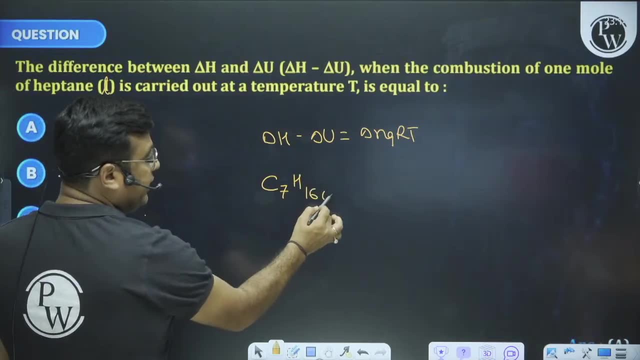 And how do we remove delta NGRT? What is heptane T7.. And how much is H 2N plus 2, 16.. It is liquid. Did I explain you? combustion of hydrocarbon? Yes, sir, I explained. 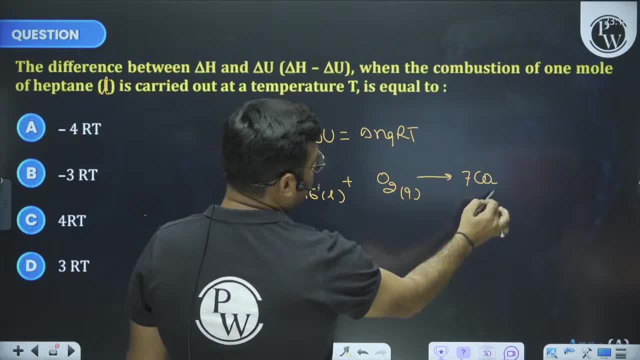 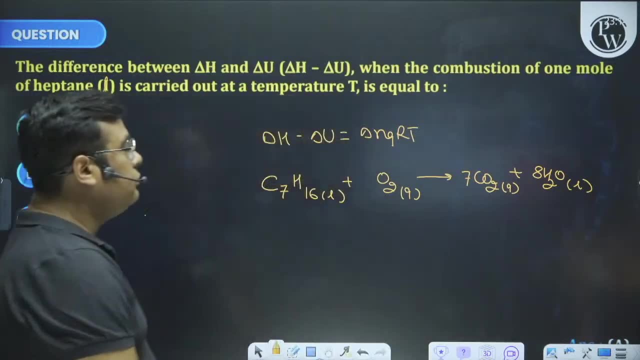 Combine it with O2 gas: Make 7 CO2.. Make gas And plus 8 H2O- Make liquid. Make 7 CO2 gas. What is 8 H2O? Make liquid. Is it coming to my words? 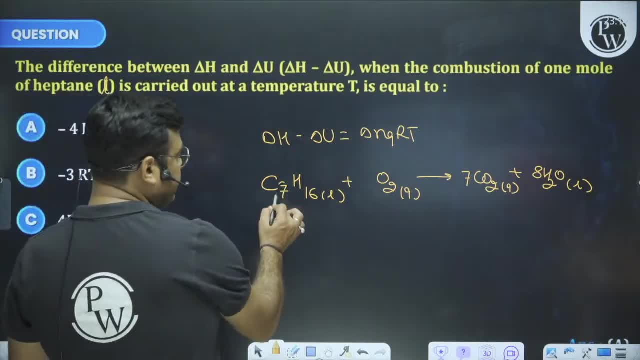 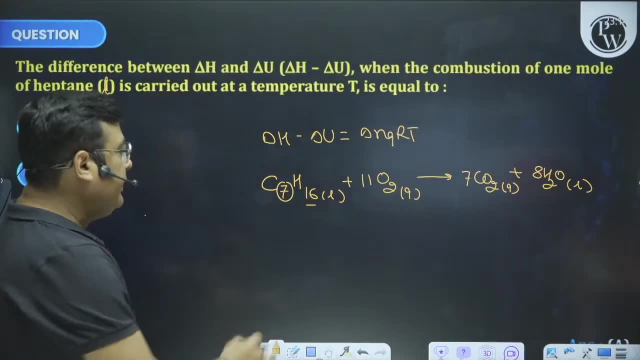 Everyone understands. Balance it: X plus Y by 4.. X is 7.. Your Y is 16.. 16 by 4 is 4.. So 7 plus 4 is 11.. There is no liquid count in delta NG. 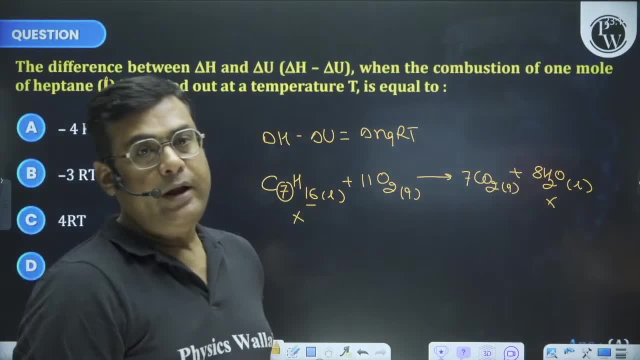 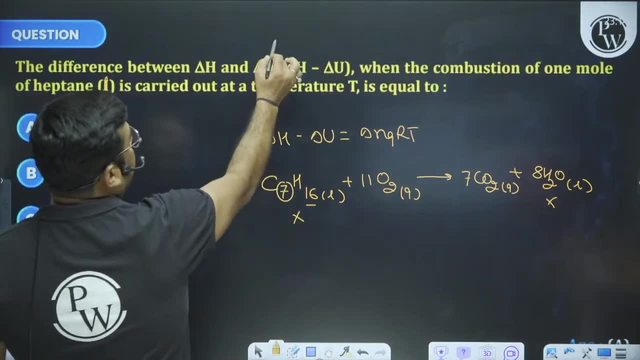 Sir, do we have to take liquid water? Right, But if the temperature is not given, then we have to take liquid water. Yes, But if the temperature is written more than 100 degrees Celsius in this question, greater than or equal to 100,. 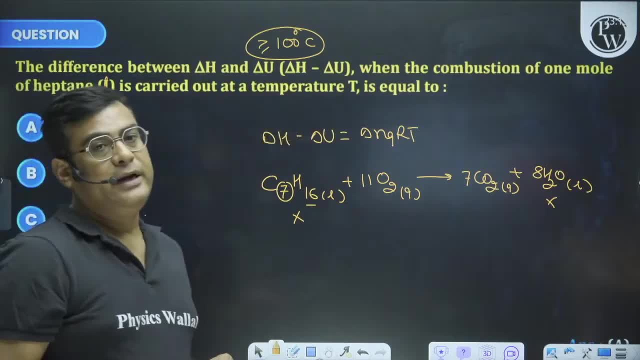 which is not written. right, Because if it is not written, then by default we take room temperature. But if it was written, then what would have happened? Then you would have to give H2O gas. So now 7 minus 11 will not be counted in delta NG. 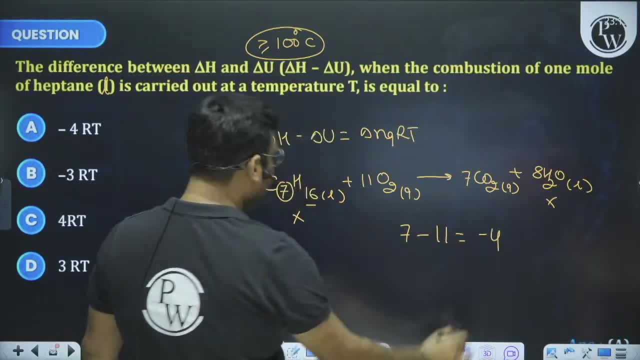 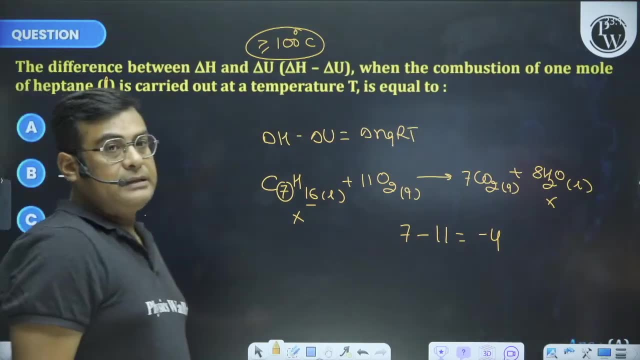 The product's gaseous moles minus the reactant's minus 4.. So your minus 4 RT will be answered. Sir, please tell me the sign convention once. Whose sign convention should I tell? I had just told you about work done. 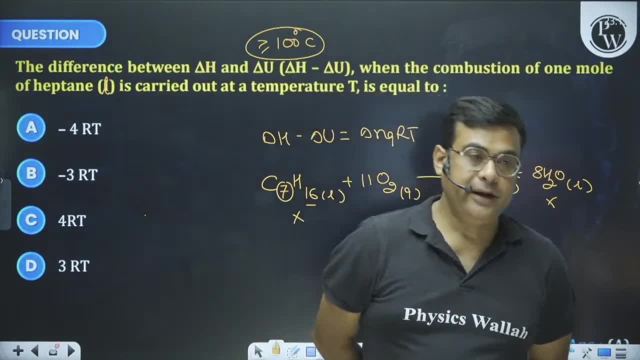 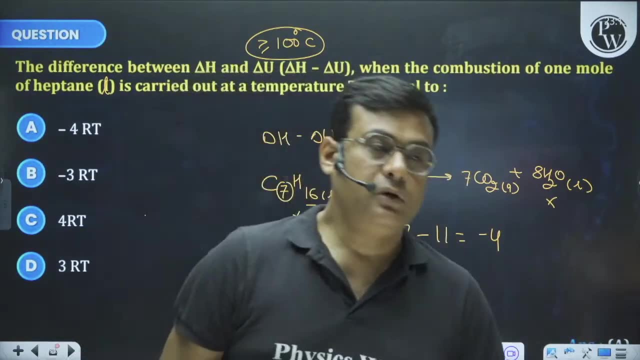 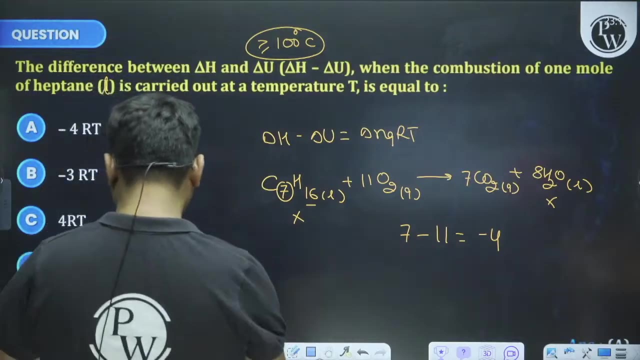 That the area of chemistry under the curve is negative. What does it mean? Work done by the system is negative and on the system is positive. For heat, heat absorbed by the system is positive and heat released by the system is negative. Okay, 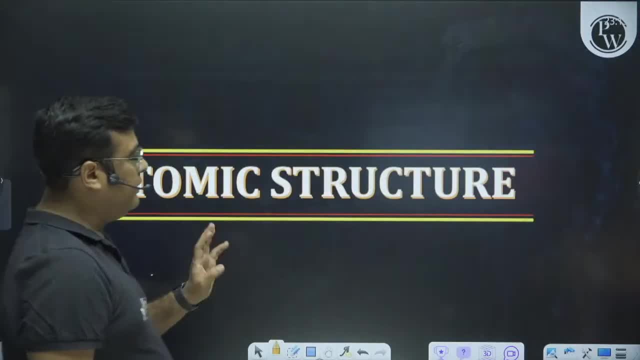 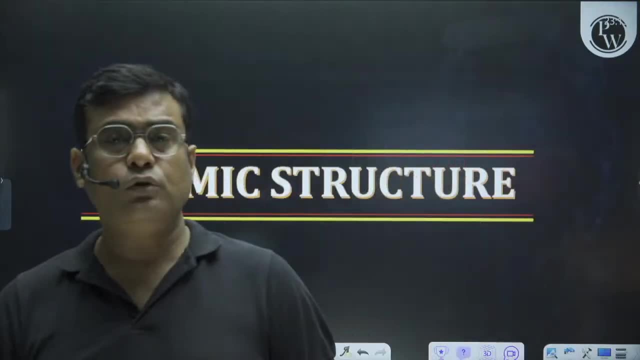 So now let's move towards the last and final chapter, Atomic structure. Okay, In which, again, children, I don't have much to tell you The new things. I will definitely tell them Right, Because the rest are related to your modern physics. 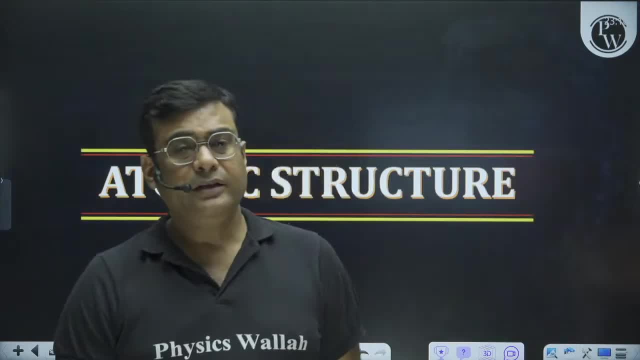 There is Bohr model, there is hydrogen spectrum, there is photoelectric effect. Okay, The time is also happening for you. So, apart from that, apart from that, what is your Planck's quantum theory? You must know a lot about them. 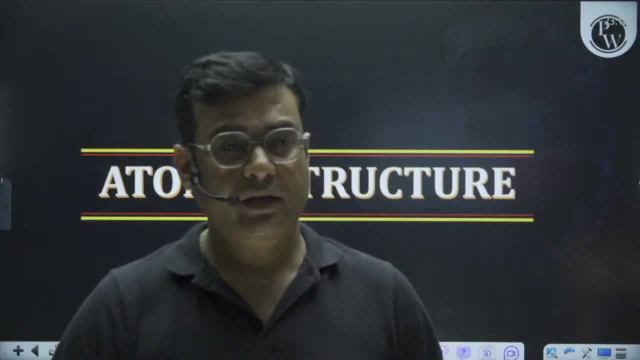 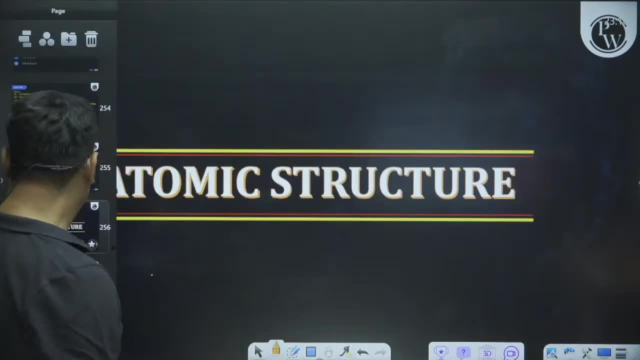 Children are very afraid of the Schrodinger wave equation. Okay, I am clearing that thing for you So that you get rid of that fear completely. You get rid of that fear completely. Okay, Okay, Okay, To get rid of that fear. 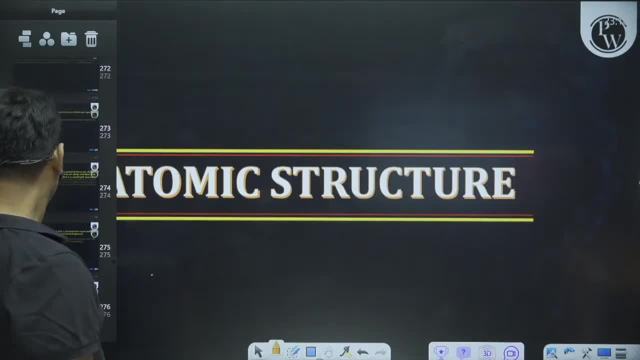 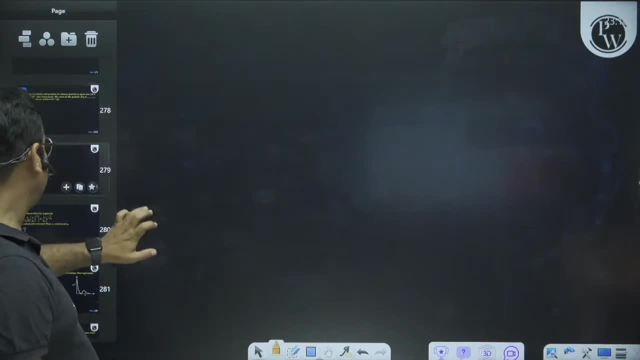 we definitely take some questions on Schrodinger in this chapter. See this: First of all, I will give you a little knowledge of Schrodinger. After that I have some questions. What is the knowledge of Schrodinger? First of all, children. 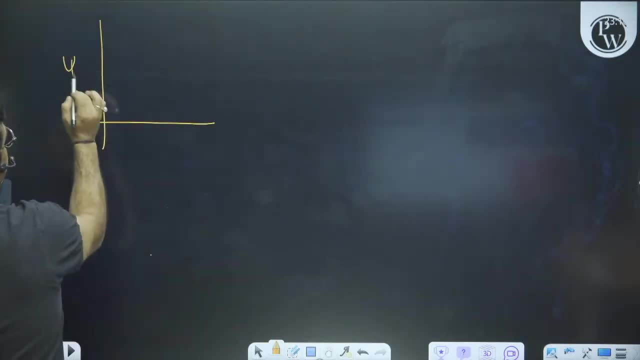 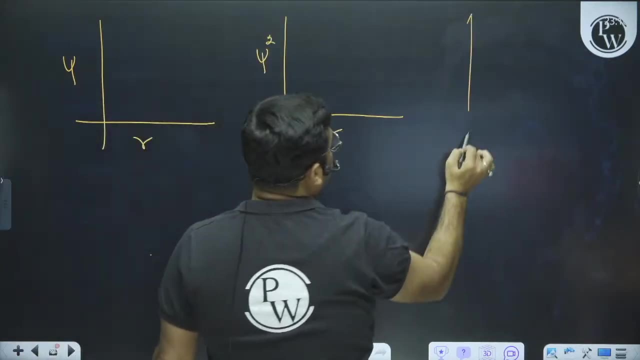 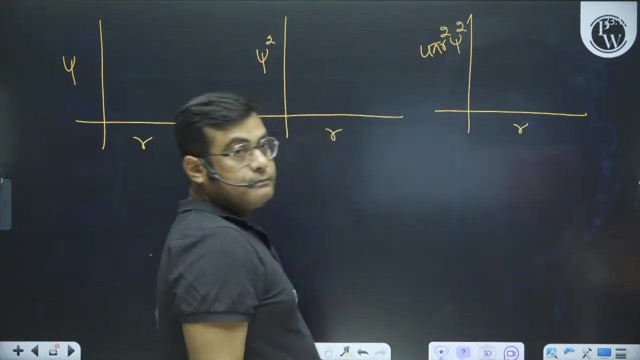 in Schrodinger from you, psi versus R Right, Psi square versus R And, which is the third graph 4, pi R square, Psi square versus R Right. These three graphs are most asked. Apart from this, you are asked about the radial node. 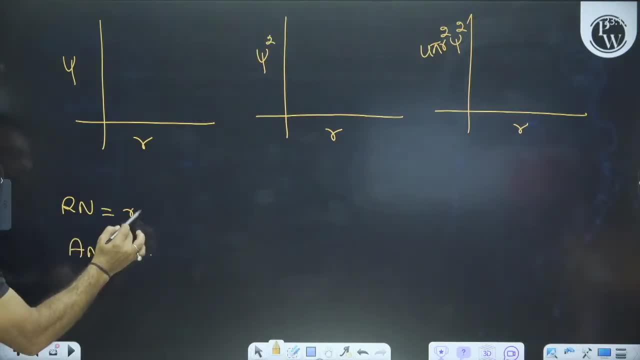 You are asked about the angular node. The radial node is n minus l minus 1.. The angular node is equal to l Right. What is n? We are talking about the total node. The total node is the sum of both children. 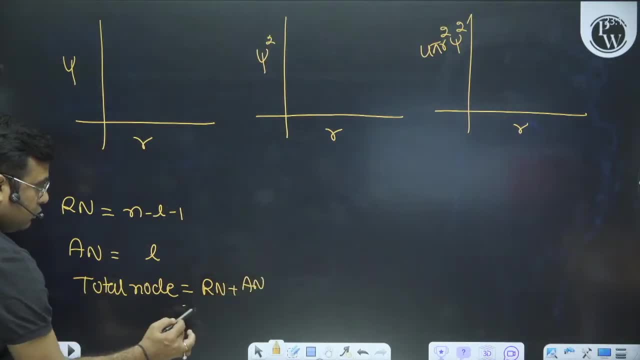 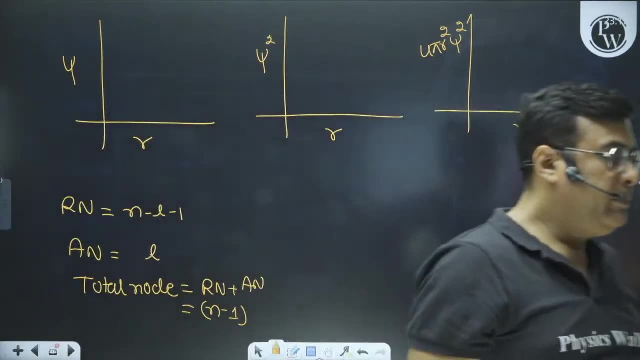 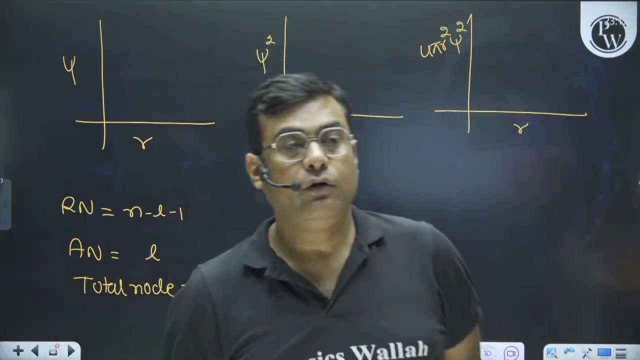 Rn plus An, And if you sum both, then n minus 1.. What is the node? The node is the region in space where the probability of finding an electron is zero. And what is the orbital? The region in space where the probability of finding an electron is maximum. 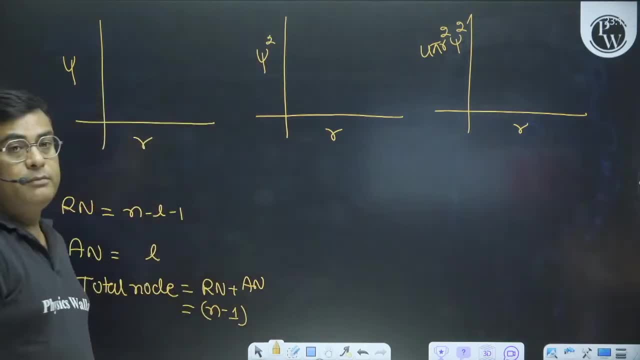 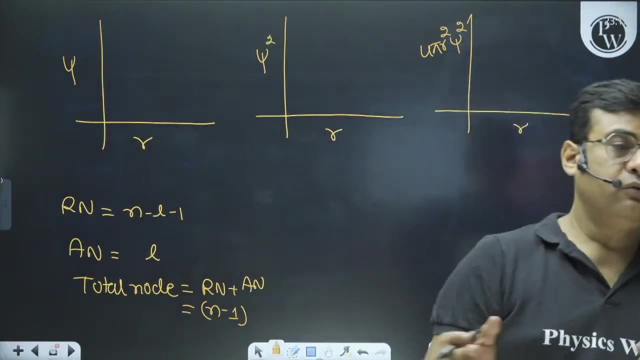 What is n? Here is the principal quantum number. What is l? Here is the assumed quantum number, which you must be knowing about. The value of n is from 1 to 2,, 3,, 4, up to infinity. 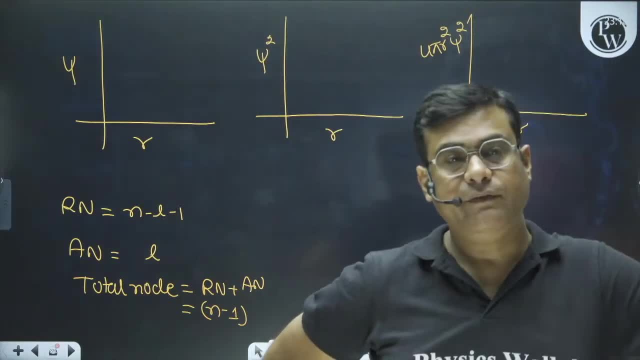 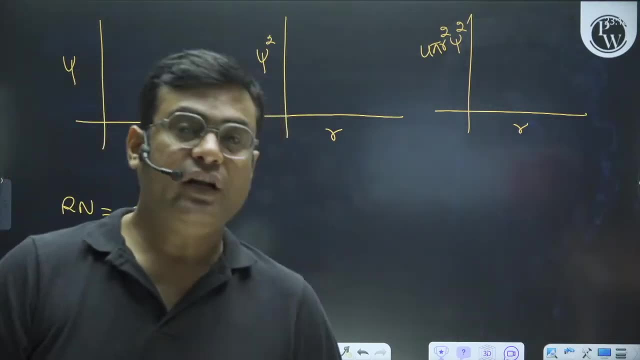 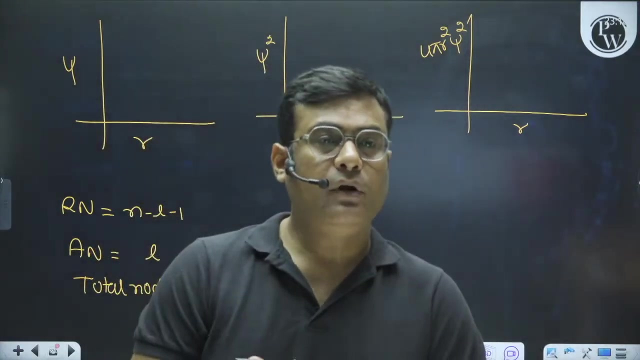 It takes only the integer values. The value of l goes from 0 to n minus 1.. The value of m, the magnetic quantum number, goes from minus l to plus l, including zero, And there are only two values of the spin quantum number. 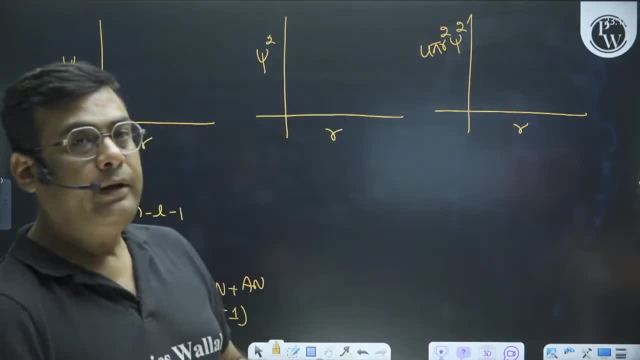 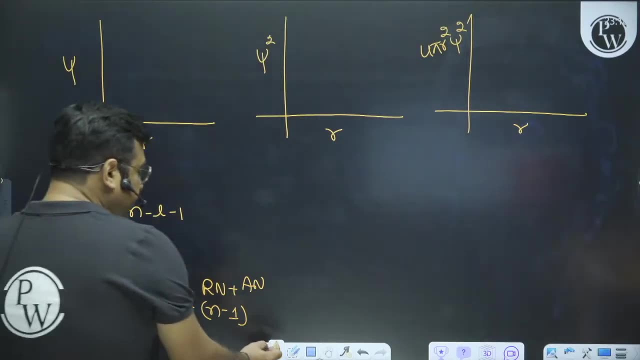 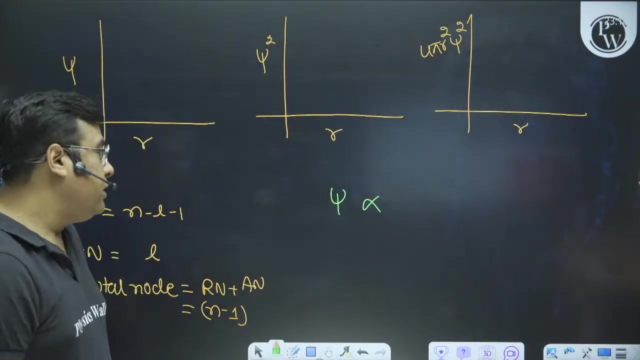 plus half and minus half. The nodal plane is also equal to l. These are the four things. Now the function of the psi of any atomic orbital children, listen carefully, I am telling you the most important thing. The function of psi is the product of three things. 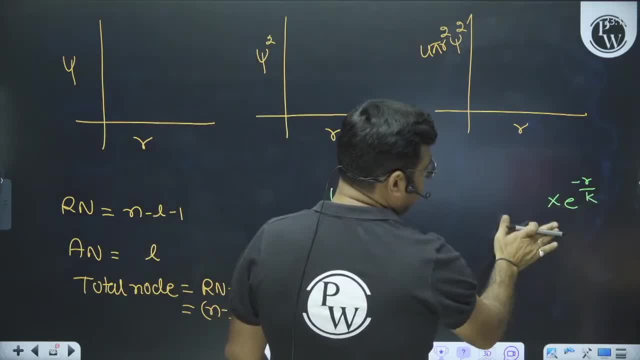 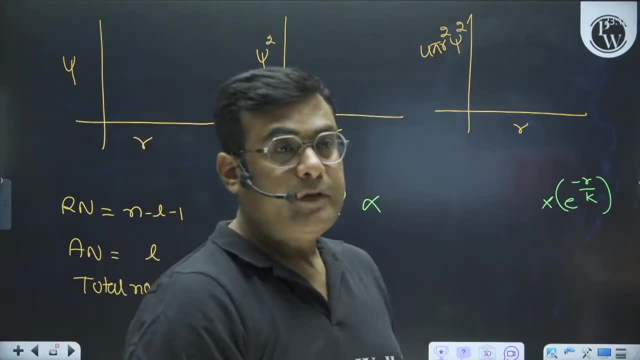 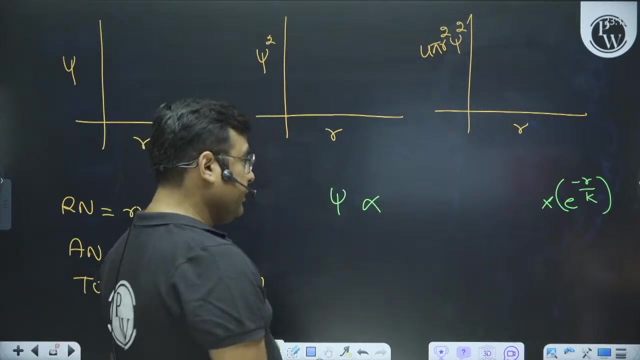 First, e to the power minus r by k. It is exponential. It is the same for every orbital, Isn't it? It is the same for every orbital, For every orbital, e to the power minus of r by k is the same. 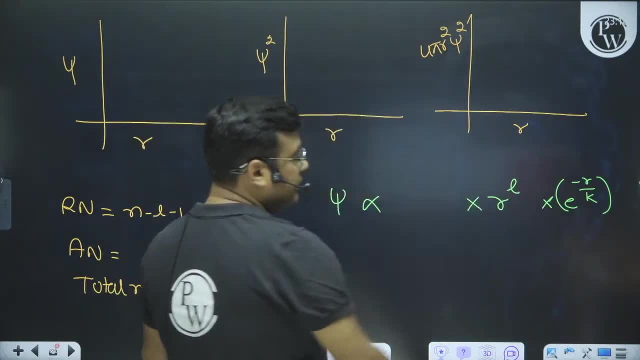 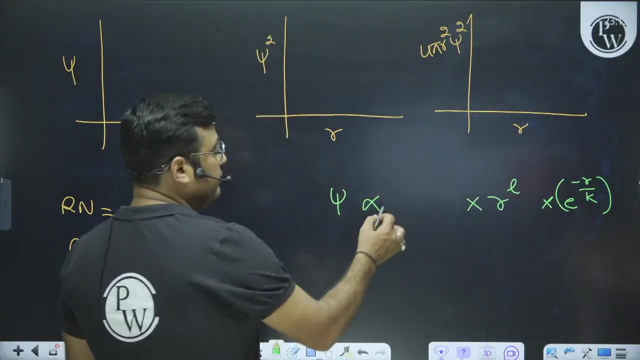 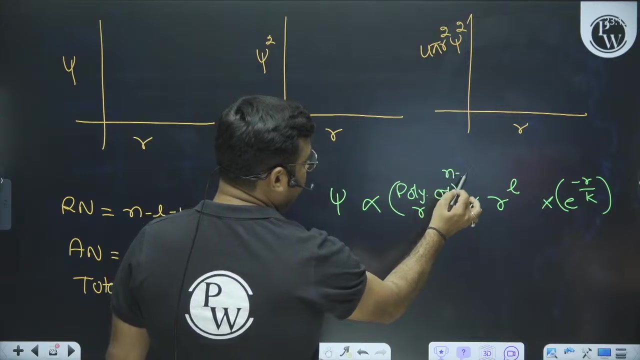 Second, r to the power of l, Isn't it? This will be different for each orbital because l will be different for all. And the third is children, a polynomial of r whose power is n minus l minus 1.. 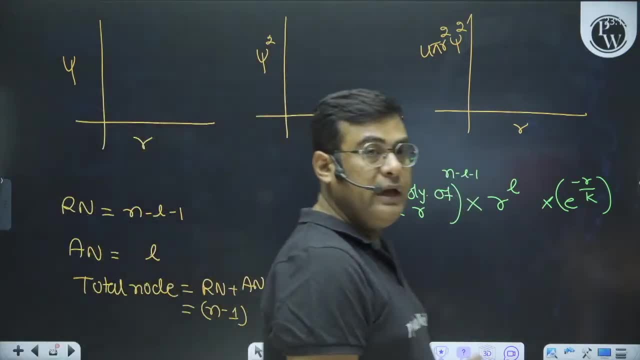 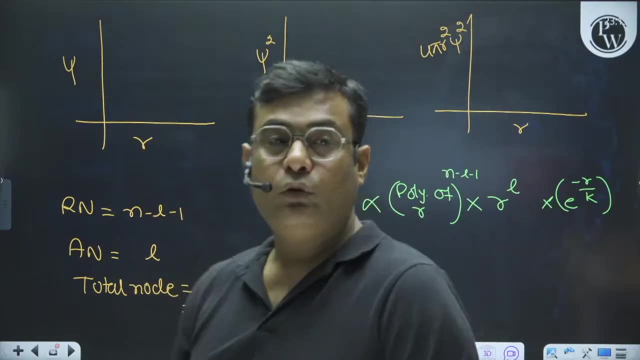 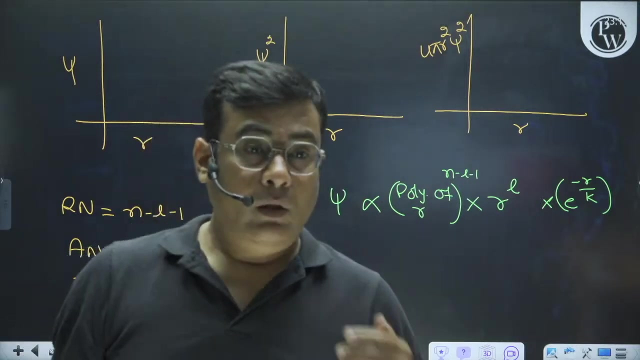 Basically, whatever the radial node is, children, the angular nodes. we are reading the last thing for simplicity, but Schrodinger has spent years on them, isn't it? Schrodinger first made the curves of all of them. After that he told the formulas of radial nodes and angular nodes. 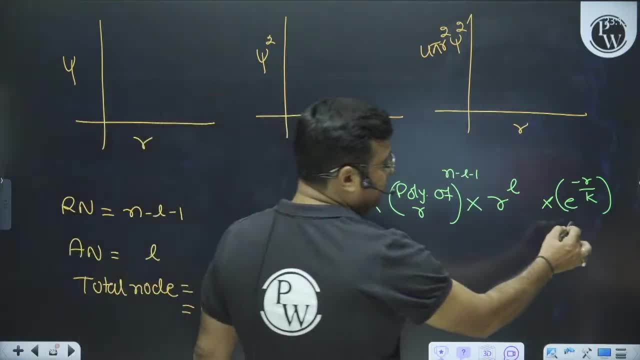 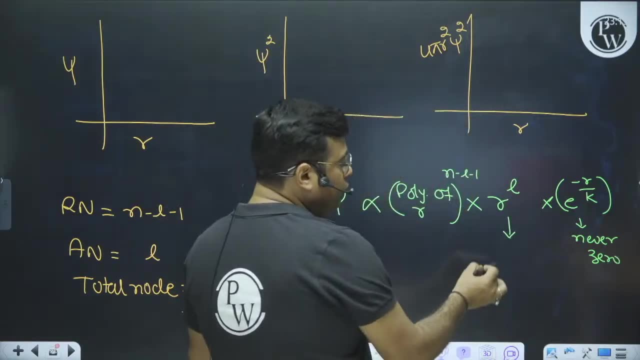 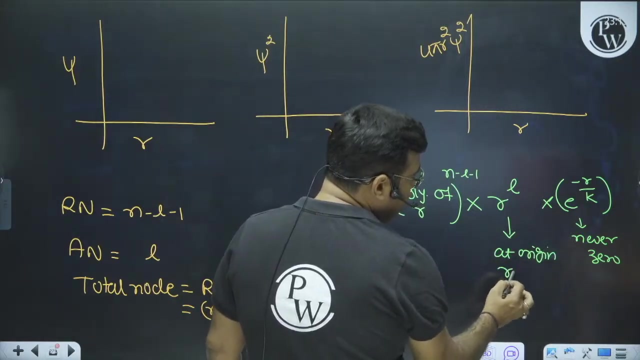 Okay, So this function, the exponential part, can never be zero, Never zero. It can never be zero. This will be zero For what? This will be zero at origin, Because we consider the nucleus at origin, And origin means r equal to zero. 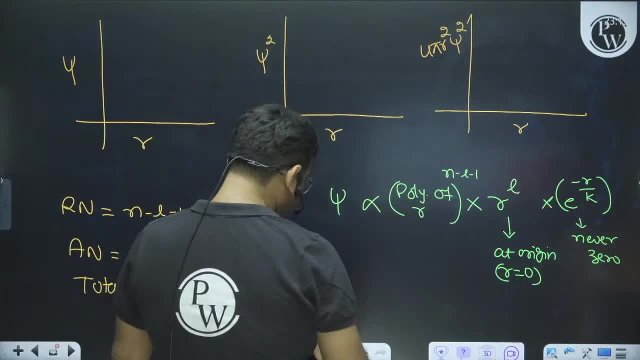 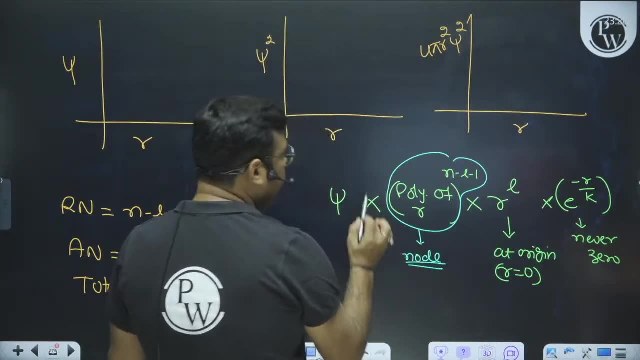 Isn't it Okay? So if the node is ever asked, then you get the node from this part. If the node is ever asked, how many radial nodes are there, Isn't it? We are talking about the radial part, So the radial node is always known from the power of the polynomial of r. 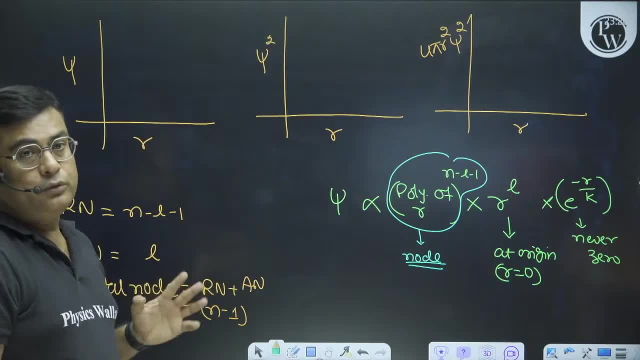 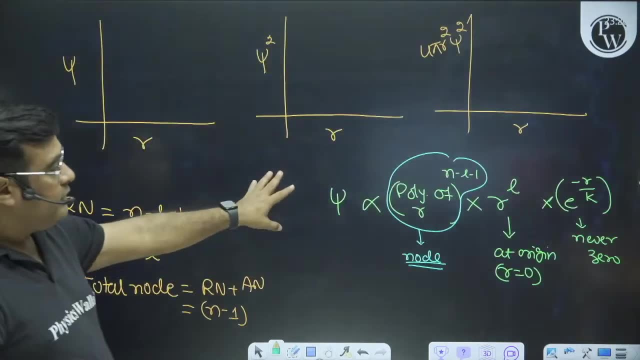 Okay, It is important for you to keep these three things in mind. Okay, Now, how does the question come on this sir? Now, sir, do I have to remember the function for any orbital, or not? I have not said this even once, that I have to remember this function. 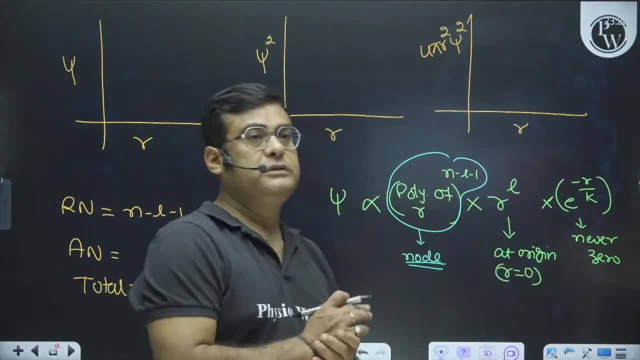 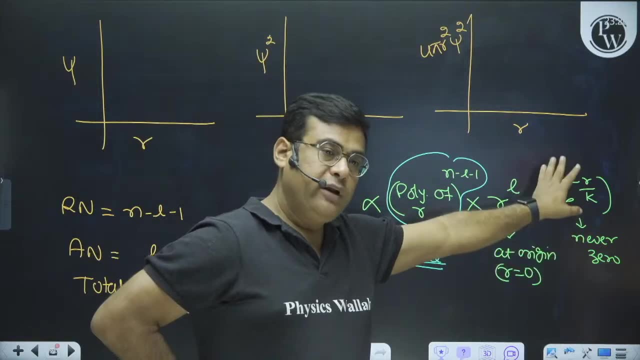 Yes, you have to remember this pattern, that the wave function of any atomic orbital is the product of three functions: e to the power minus r by k. for every orbital, k will be different for all. it will be constant, but it will be for all. 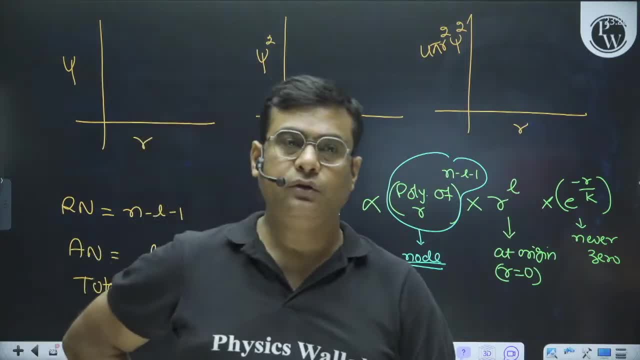 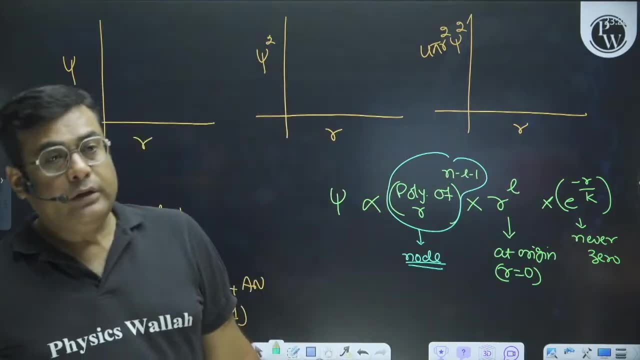 r to the power of l. Obviously, for such an orbital l is zero, So it will not be seen in that. For p: l is one, so you will see the type of r to the power of one. For d l is two, so you will see the type of r to the power of two. 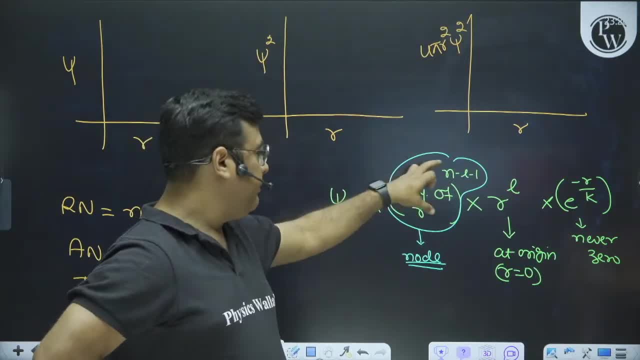 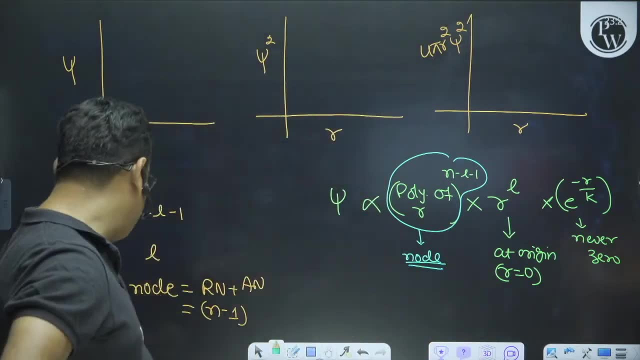 Okay, And the rest of the children will see a polynomial of r n minus l minus one. It will be different for different orbitals. Okay, It will be different for different orbitals. Okay. Now look, the one who asked this question once on this. 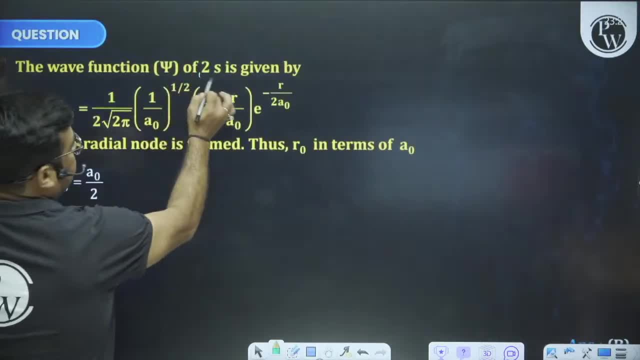 The wave function psi, of 2s, Isn't it? The wave function of 2s is given At r equal to r0.. Radial node is formed. Tell me r0 in terms of a0.. Now it is of 2s. 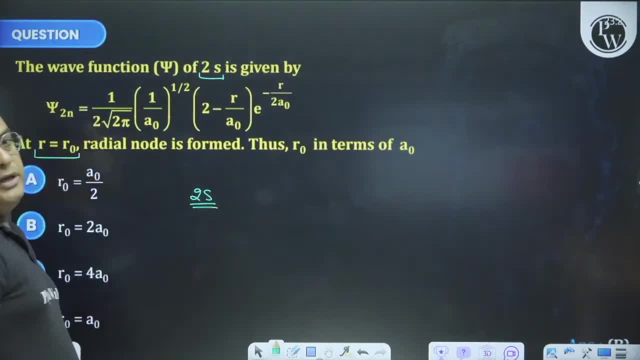 So the one I told you. check it. It will be of e to the power minus r by k type. Yes, sir, it is Here. it is e to the power minus r by k r to the power of l, Because for such orbital l is zero. 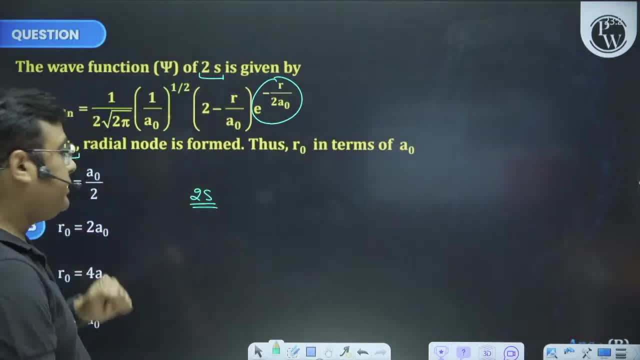 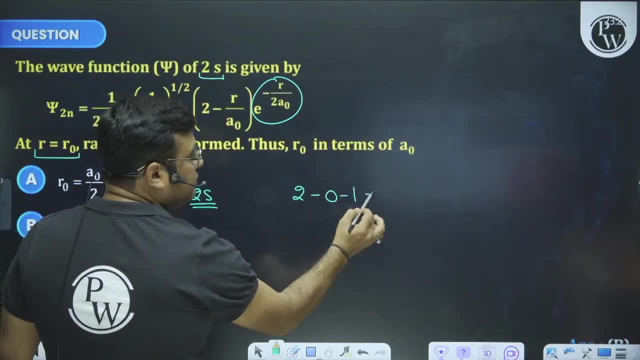 So the power of r is not seen separately. It is not there. The third one will be a polynomial Whose order will be n. It is two Minus l. Minus one Means one. So you see, this is a polynomial of two. 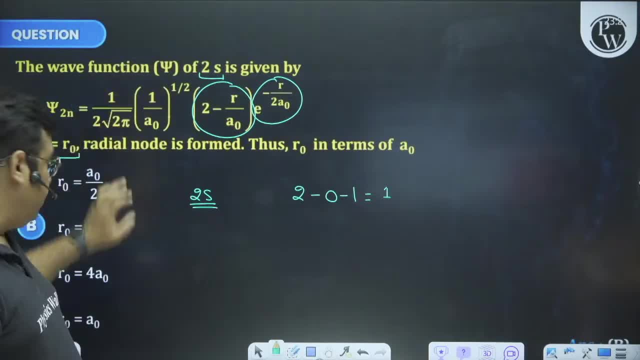 Of two minus r by a0 type And some constant, Because what I have written to you, son, is written in proportional, Isn't it In proportional? you can get any constant. Here it is, And I just told you. 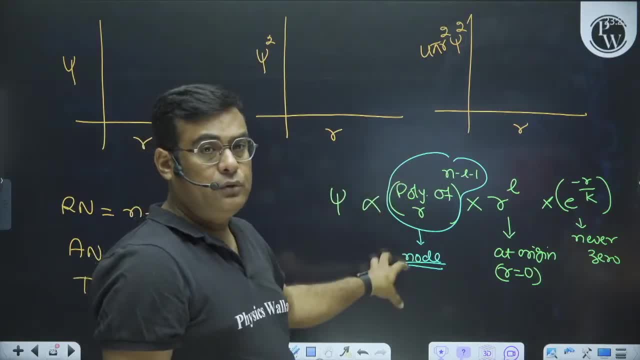 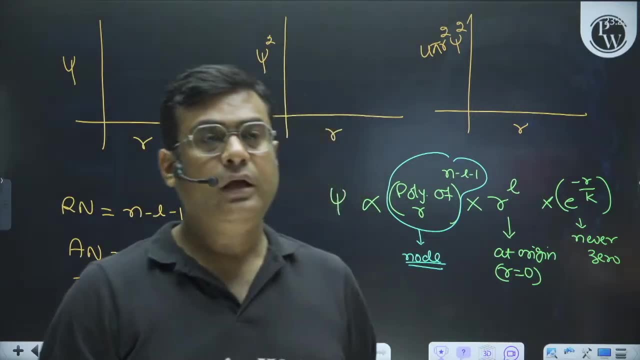 Whenever the radial node will ask, only this part has to be zero, Because this can never be zero. This will be zero on the origin And, by default, there is only a nucleus on the origin. And if there is a nucleus on the origin, 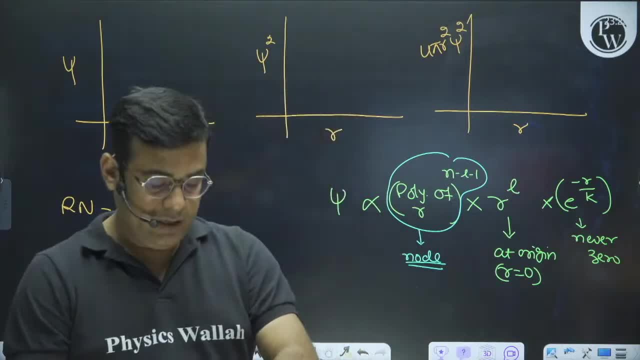 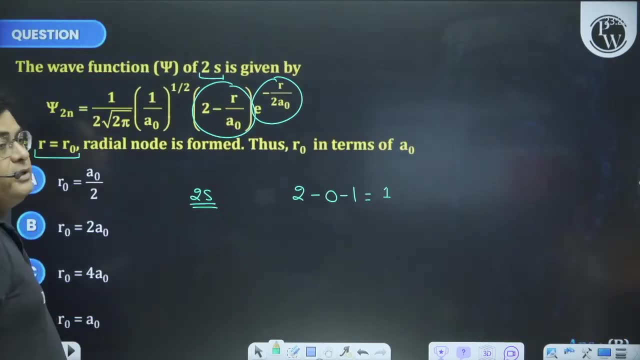 Then on the nucleus, Then there is no finding probability of the electron. There is no such thing. It will always be zero. It will always be how much children Zero? So here you are just Now. the children are scared to see the question. 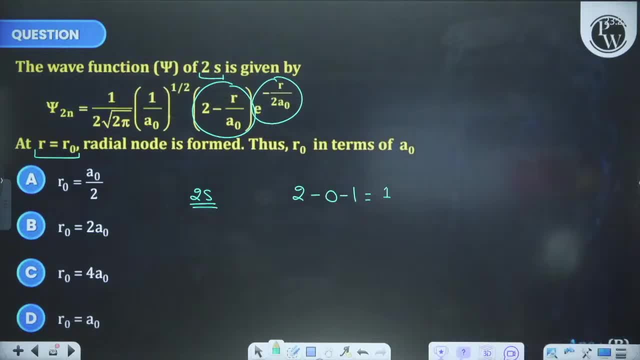 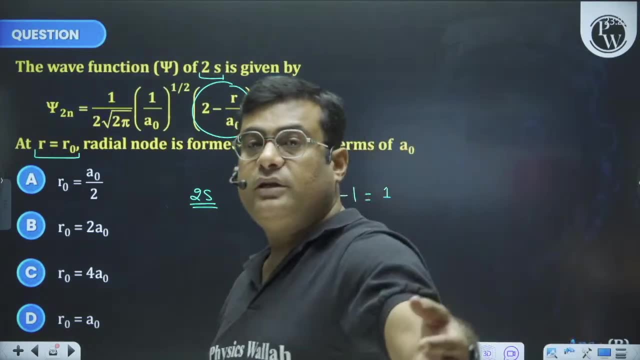 Those who do not understand the shape and line of Schrodinger. What is Schrodinger? They are afraid that Sir Schrodinger has not taught us properly. Schrodinger is not clear to me. Okay, I do not remember the function of Schrodinger. 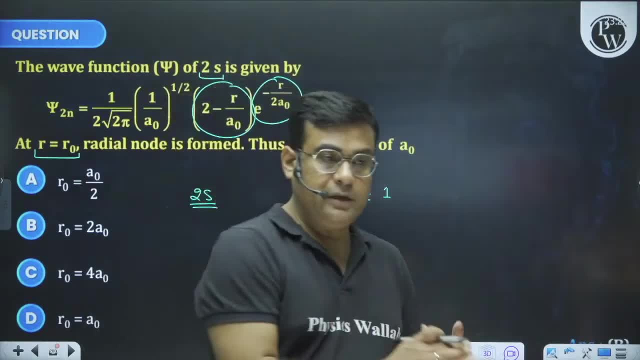 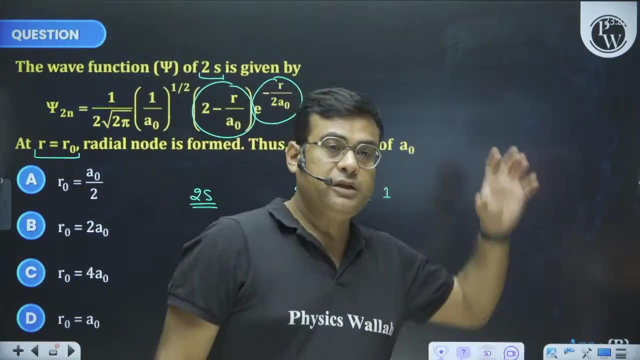 Brother, I do not remember even one, In spite of teaching for so many years. I do not remember the function of one. Because I will remember what is not needed, I will force you to write the function of ten orbitals- unnecessarily, No meaning. 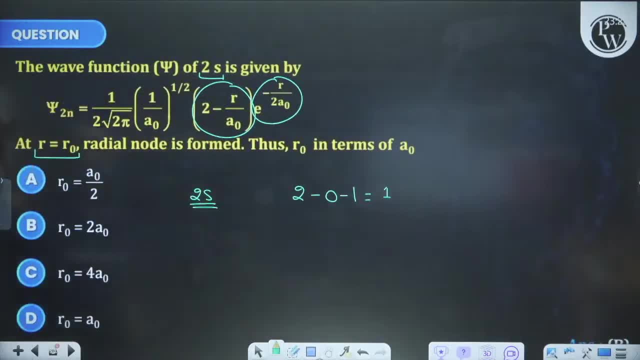 Whenever you get a question, the function of the node will be given And you have to make the polynomial part zero. If you make it zero, If you make two minus R by A naught zero, It is clearly visible in front of you that R equals to what. 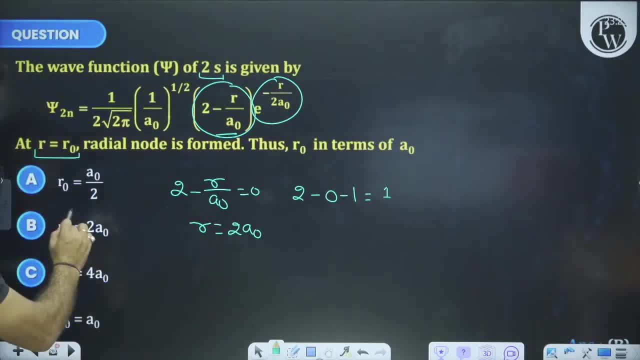 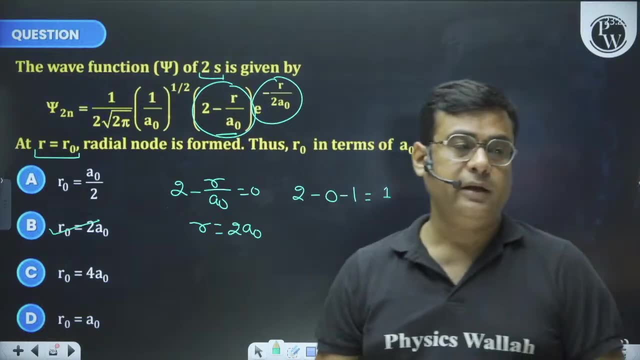 Two A naught, Isn't it? R equals to what Two A naught. Where is it? Here it is. The story is over. Now see this fear. It is necessary, Because if we do not have anything clear, Then there is no fear. 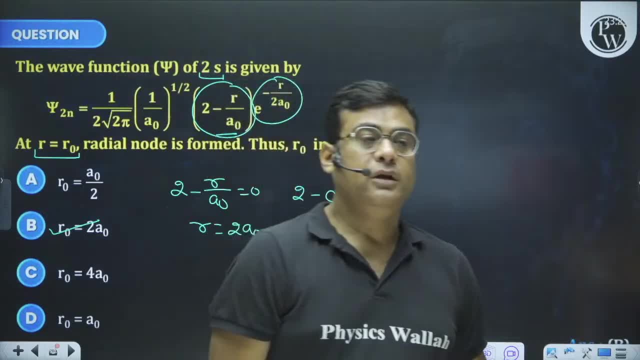 Now I do not know how to drive a car And I have to sit in the car and turn the key And then I have to spit. But if we learn to drive the car timely first, After that Drive the car after practicing, 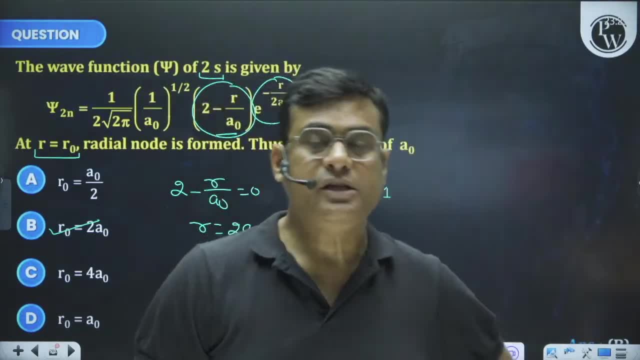 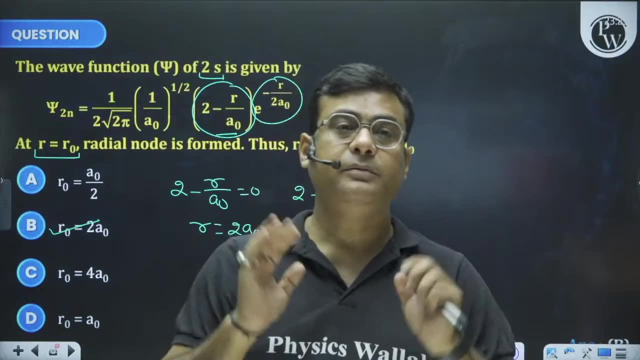 Then, brother, Even though we will drive very slow in the beginning, We will drive carefully, Isn't it? The car will be seen 10 meters ahead Before that we will put the brake, But at least we will not make an accident. 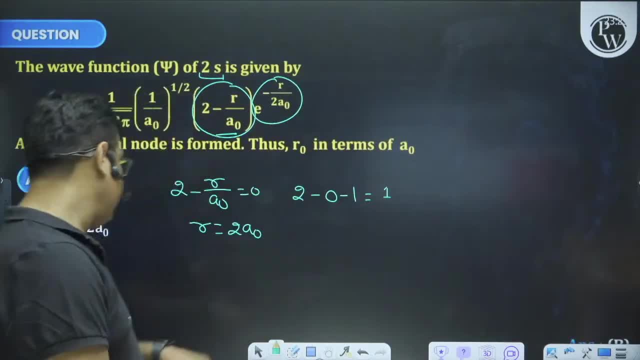 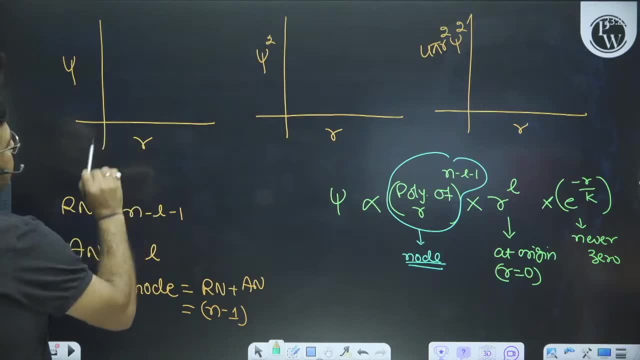 We will drive slowly, Slowly. Okay, I am explaining the same story Now, the story of the graph, Isn't it? You will say graph, So listen to the graph. The graph of psi versus r starts with a non-zero value for s orbital. 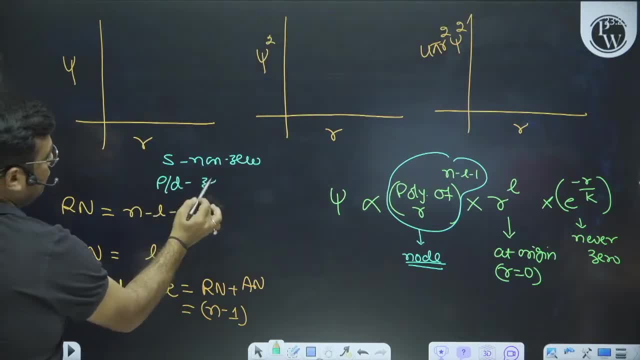 Isn't it? Starts with zero for p and d, Isn't it? The graph of psi versus r starts with a non-zero value for s And starts with zero for p and d. Why? Because in p and d, Power of r is one. 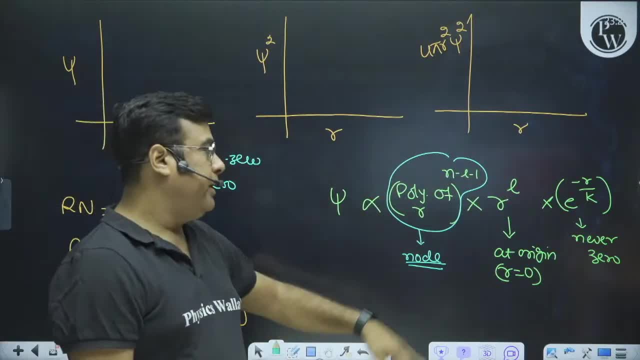 Power of r is two. Power of r is two And the power of r is zero for p and d. If the power of r is zero, then at some point this is zero. The power of r is zero at the beginning, Isn't it? 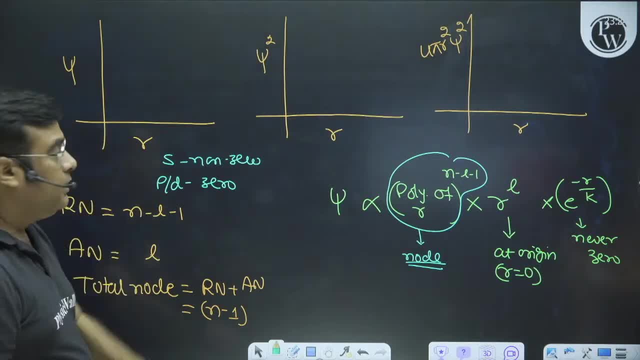 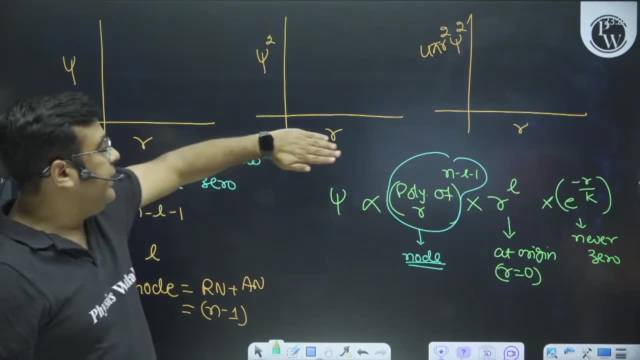 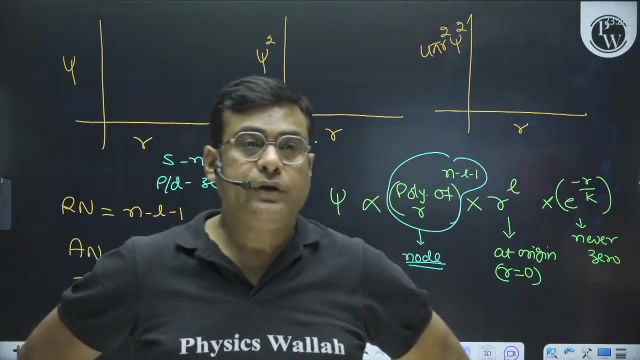 I found the graph of psi, so there is no problem in s, whether r or only r, Because the portion which is inside the negative points will move forward. That portion which is inside the negative points will move forward on the positive one, Because psi is there. 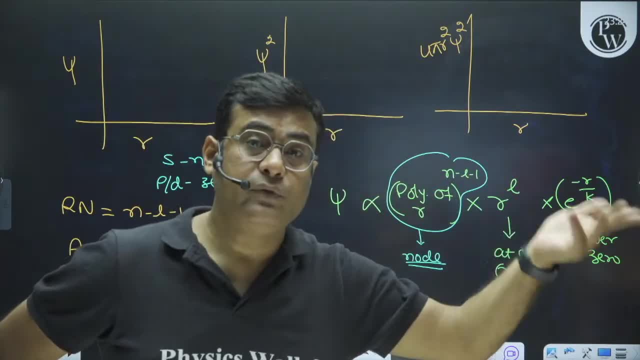 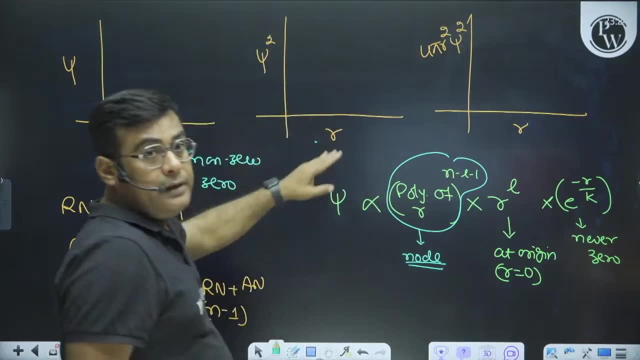 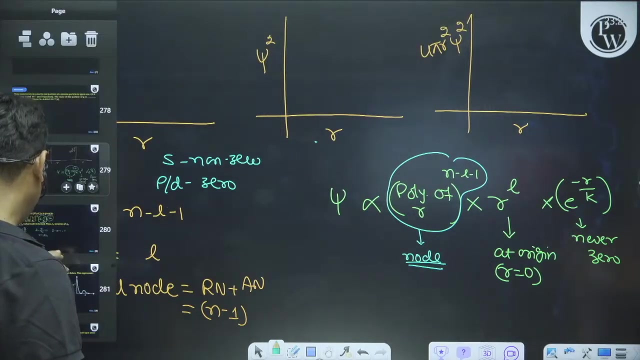 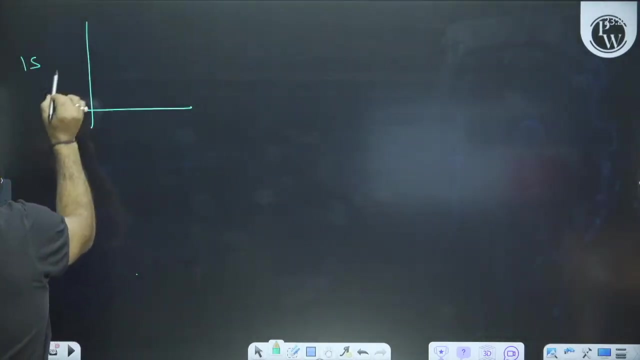 positive, negative, zero, everything can happen. but the square of psi in mathematics, if y is negative, then y square will be positive. it will always be positive, right? and how many times will it cut? it will cut as many times as the node will come right, like in my support. first I will add one or two pages empty, right? if I am telling you to make a 1s graph for 1s psi versus r, then you will say that it will start from above, something like this: why? 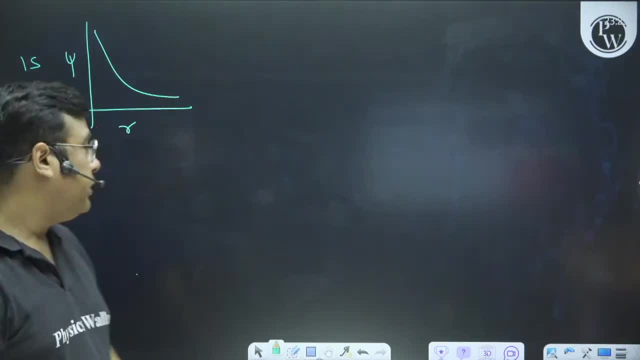 There is no radial node in 1s, right, what is the formula of radial node? the formula of radial node is n minus l minus 1, zero. so it will start from above. it will not cut anywhere. but if I am telling you to make a 2s psi versus r graph, then there is a radial node in 2s. 2 minus 0 minus 1, means 1, it will start from above. if a radial node comes, then it will cut. once here it will cut, then only psi will be zero. 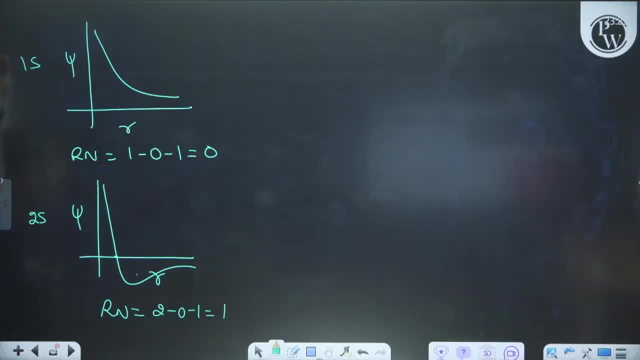 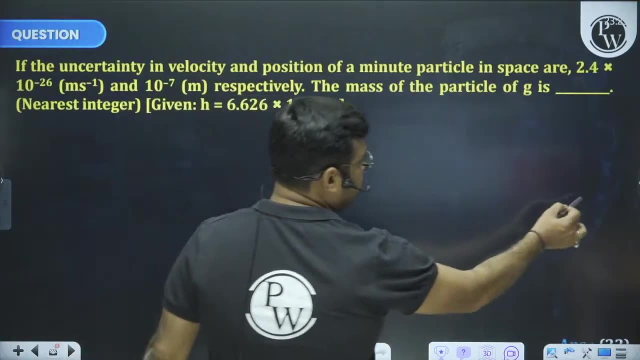 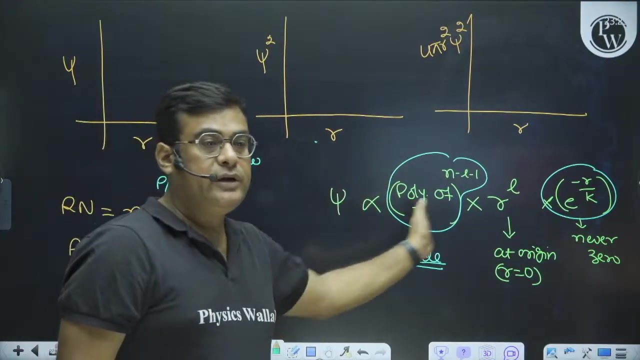 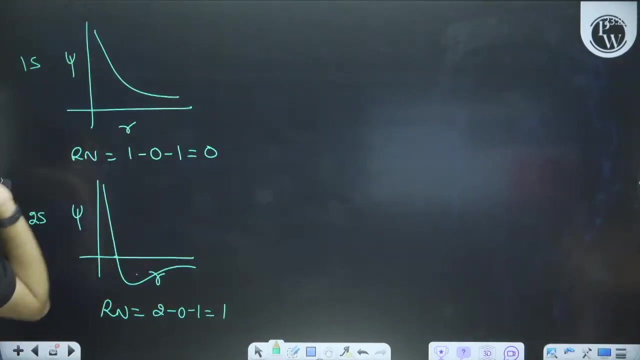 and psi will be zero, then only the square of psi will be zero. right, go every time because of the exponential function, because of the exponential function, because of the exponential function, right, as the r tends to infinity, the psi tends to zero. right, the psi tends to zero, right. so each graph will go to infinity of psi. it will just cut. right now, if I tell you to make a 1s graph of psi square versus r, then it will start from above, something like this: why? 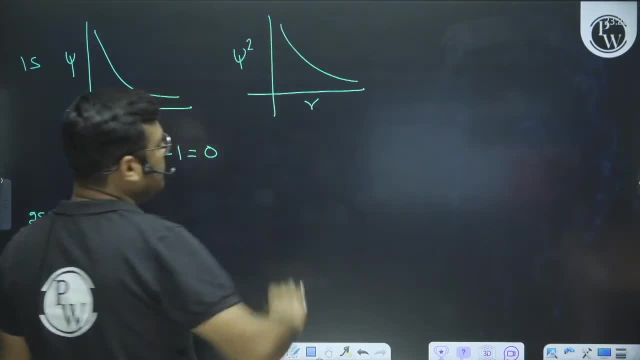 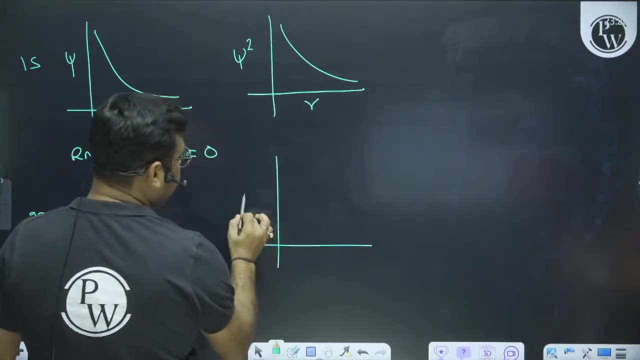 So you will say that it will be like this only. you will say that it will be like this only because you don't have to do anything. but if I said that, tell me the graph of psi square versus r. then you will say that this portion will remain like this only, and the lower one. 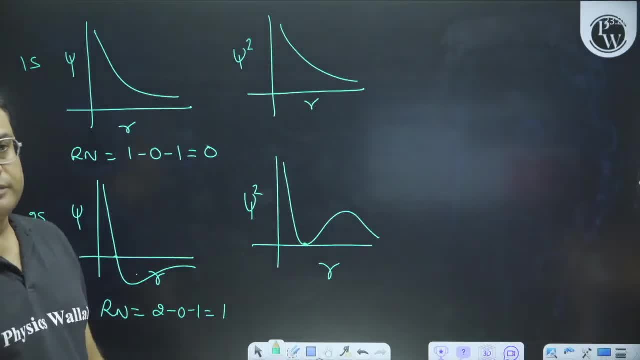 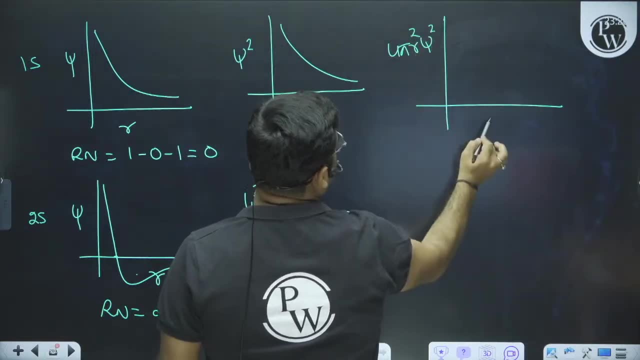 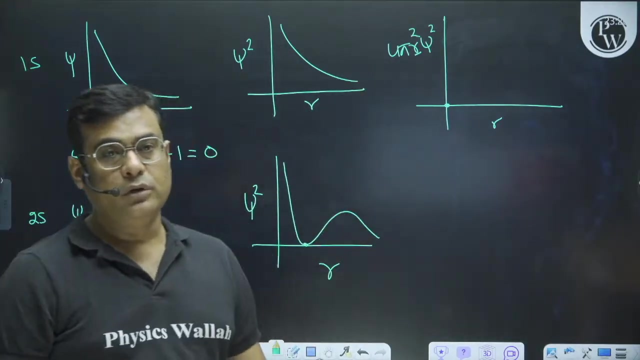 which was negative will be positive and go up what is not finished. and the third thing, which is 4 pi, r square, psi square versus r, because r has come. this graph is for everyone, whether it is S, P or D. it will start from zero for everyone as soon as r is zero. the 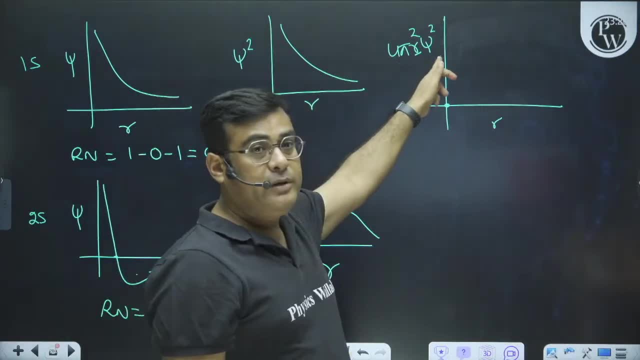 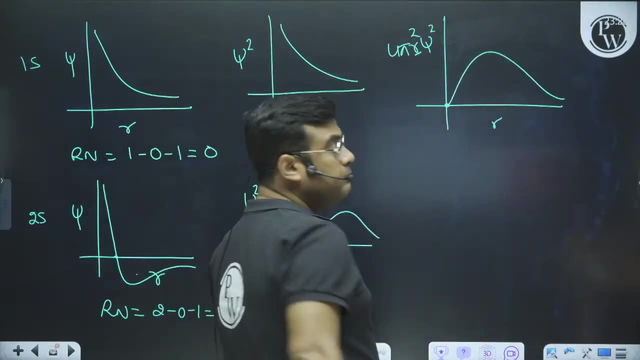 whole function is zero and because the square of psi is also coming r is increasing, psi is decreasing, then this graph of yours increases in the beginning children, then it decreases. there are mountain graphs. now, see in the mountain graph it has not touched even once. 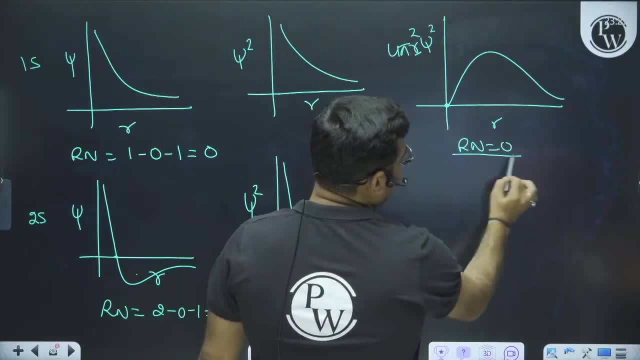 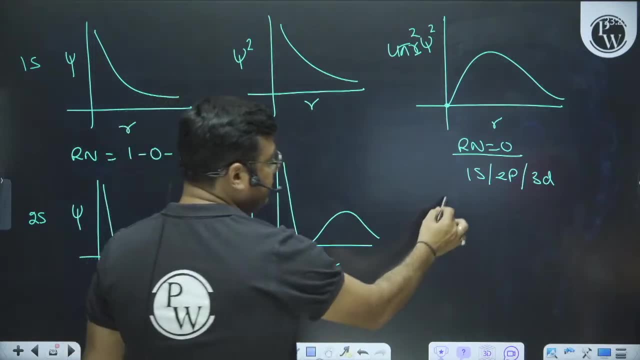 there is a radial node. it has become zero. now it can be of 1s, it can also be 2p, it can also be 3d, but if it would have touched it, the height of the mountains would increase. 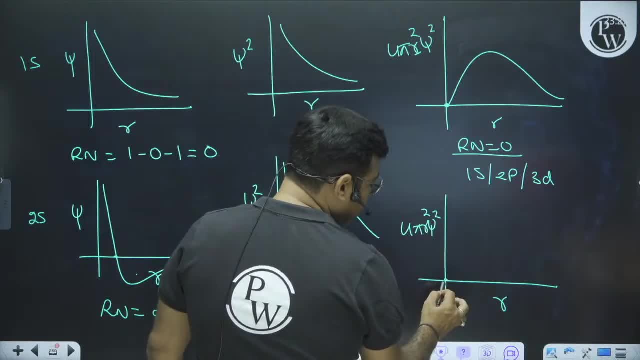 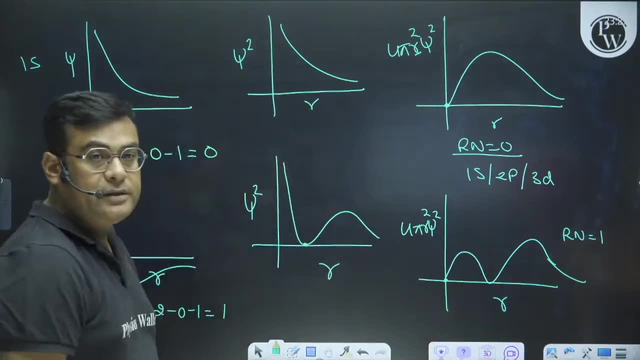 children. even if it had touched it like this, then we say that it has a radial node 1, if it touches it once, then it is a radial node. now it is a radial node 1, then it may also be of 2s. 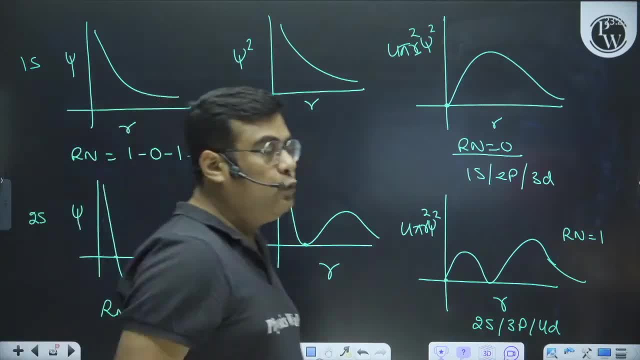 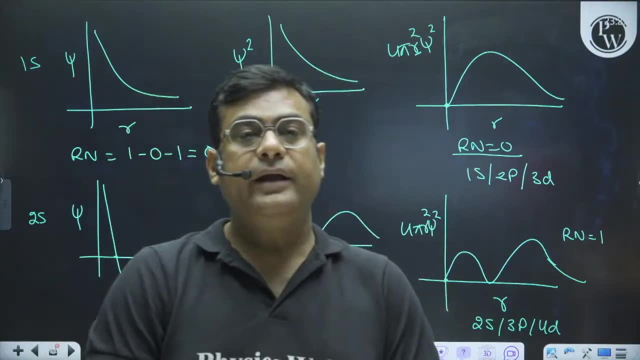 like this. So this question is on the graph. question on the radial node. question on the angular node. question on the angular node. question on the angular node. Now, maybe your J mains 2024 has a question on the radial node and the angular node. It is direct formula. 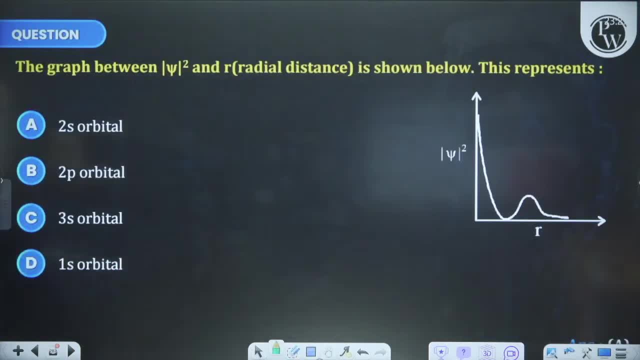 based. Maybe I am showing it too. This is done. Now, as this question came, This graph is given. tell me whose is it. It is starting from above, that is. it is of S, Sir. how many times is it touching? Once that is, there is a radial node. that means it will. 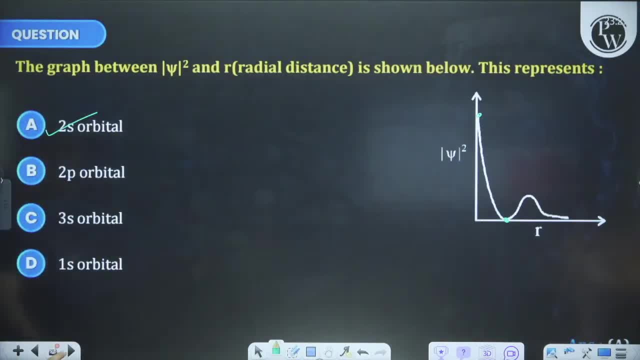 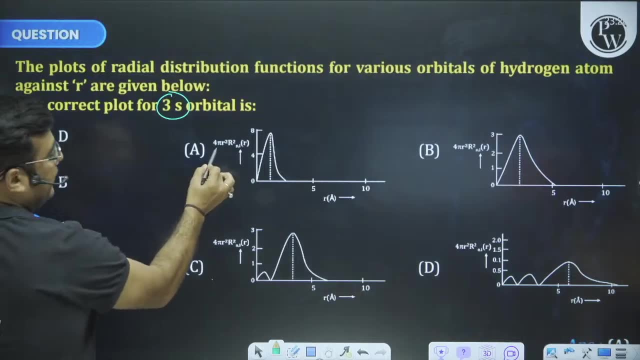 only be of S. The story was over. Maybe another question came. This is a graph, The graph of three S. has been asked Whose? four pi r square, sin square. How many radial nodes will there be on three S, Sir? there will be two radial nodes, Is it not correct? It will. 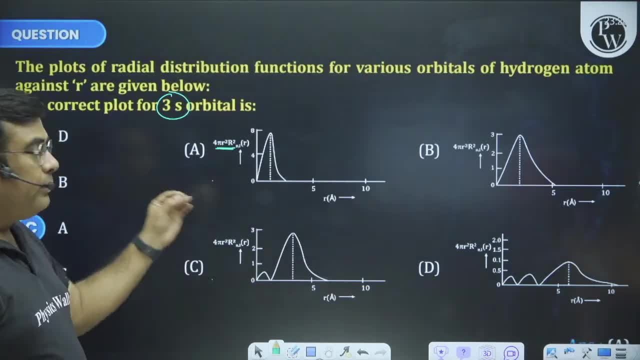 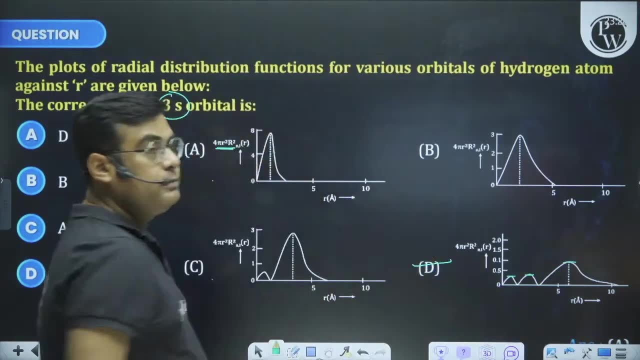 start from zero. There are two radial nodes. That means it will touch twice and the height of the mountains is increasing. See, You know that the height of the mountains is increasing little by little every time. so your option is that of D. In which D is? in which Option? 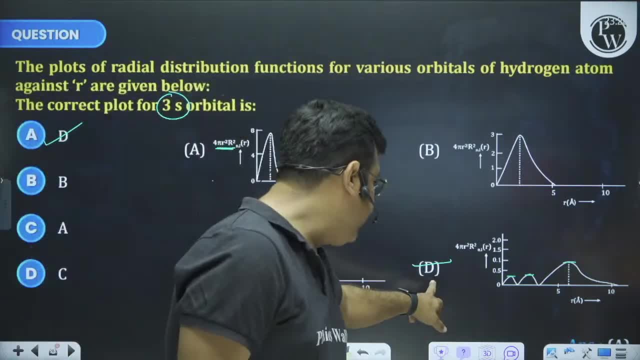 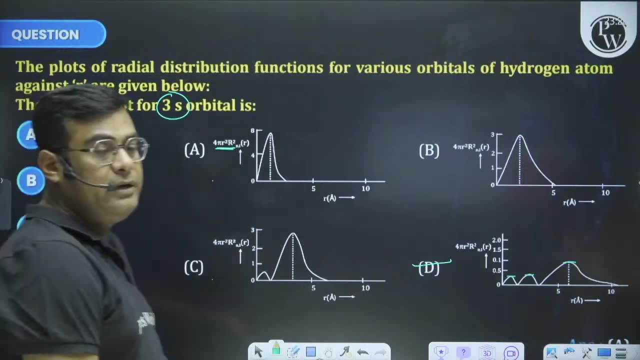 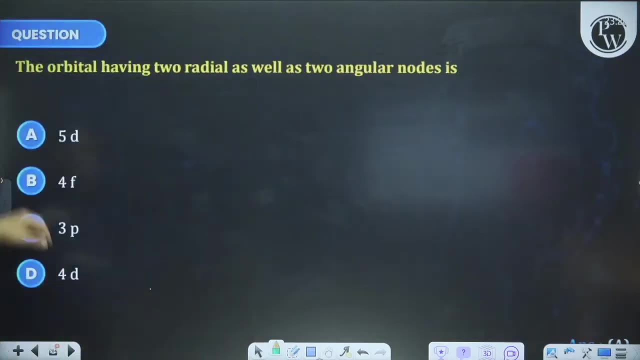 is here. This is the only answer, That is, if the height of a mountain is equal to 0. So This is also a smart thing to do. the option is D. it is not like we have to tick D in a hurry, but which option is correct in D, which is C? this is also a smart thing to do. okay, maybe the radial node and angular node. there is a question on this too, that orbital having two radial nodes, two angular nodes. two angular nodes means L is 2, now radial node N minus L is 2, minus 1, radial node is also 2,. 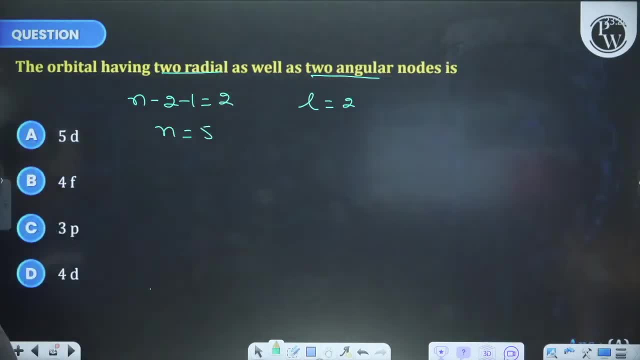 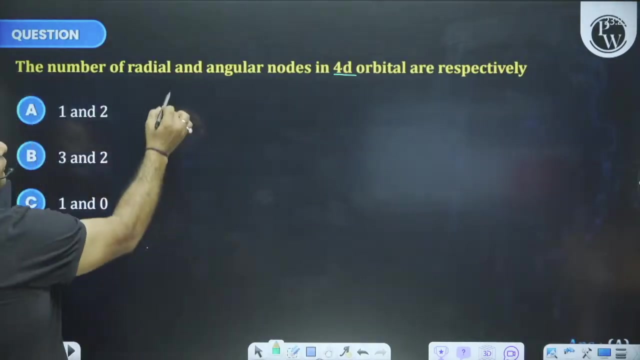 so it means: how much is the value of N? 5,, okay. L2 is children, L2 is for whom, it is for D. so your answer is 5D, okay, your answer is 5D, okay, my dear children. so in this way children see as much as there is. there is another question. here is the number of radial and angular node in 4D orbital, now radial node 4 minus 2, minus 1,, sir 1, and L value is 2,, so 1 and 2,. 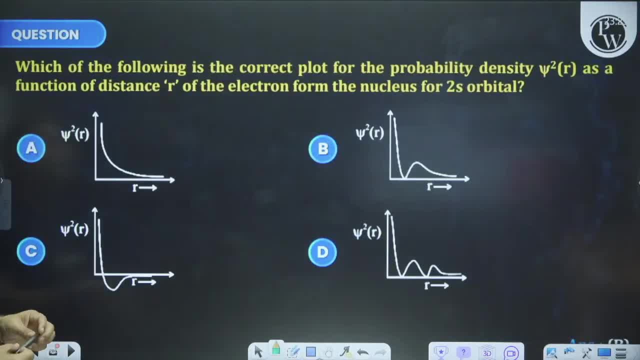 okay, let me tell you more visual of following is the correct plot for probability: density, size, square R for distance R of the electron for 2S orbital. now, how many radial nodes are there in 2S orbital, sir? there will be only one. if there is one, then it will touch once. it will remain positive. the story is not over, okay, is everyone getting the point? children, okay, okay. so now after this, children, I have all the questions of J, E, M, 20,, 24,, K B. I am not solving it now because I have put it on your table. 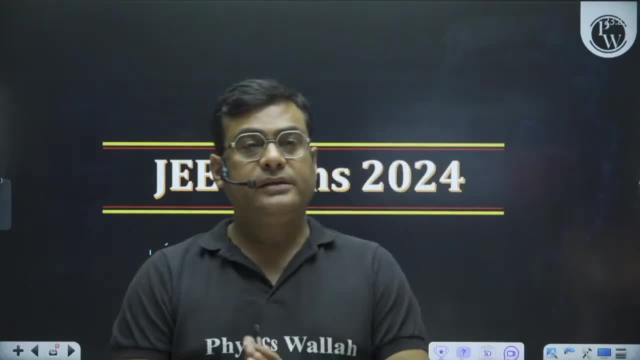 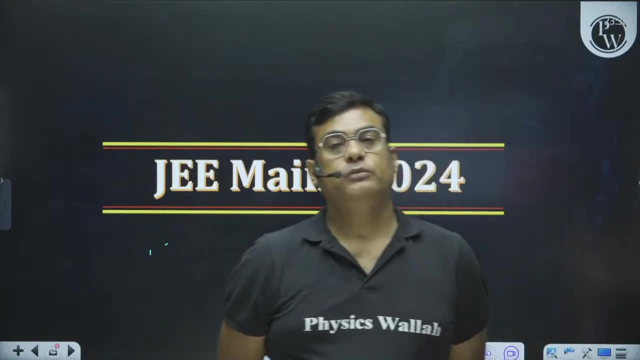 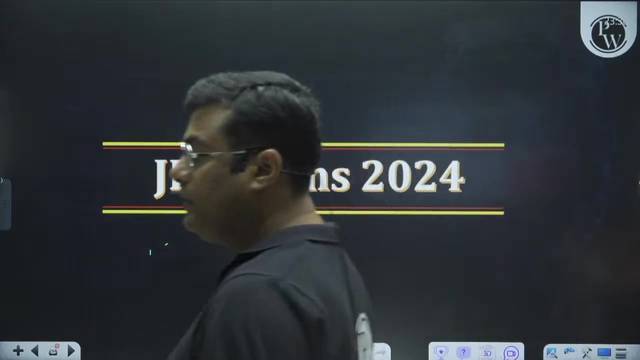 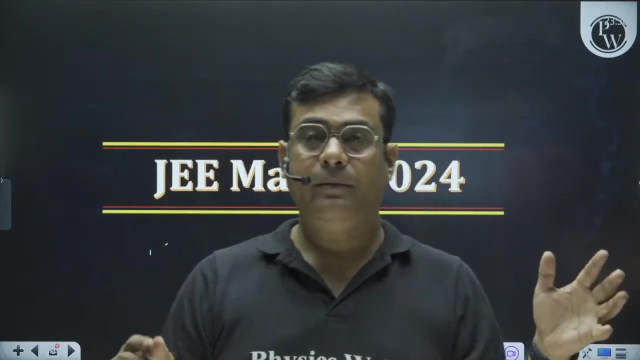 the session is almost sufficient, sir. extensive and intensive examples. extensive, that depends on the mass, intensive, that does not depend on the mass. extensive properties are those which depend on the mass of the system. almost It is a big piece of ice, so how much is its mass? how much is its mass? how much is its? 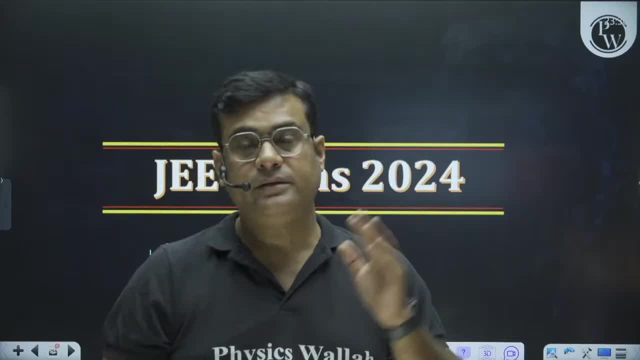 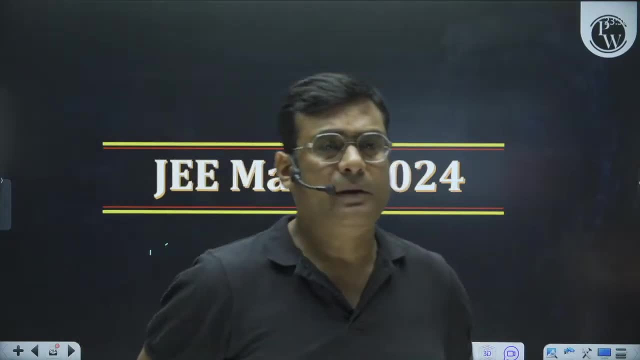 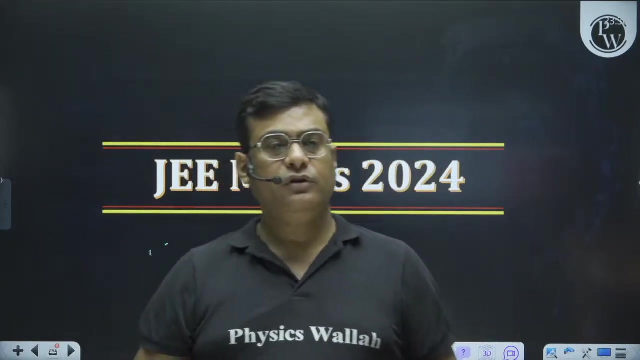 volume. This will depend on it, this extensive property. but if I talk about the melting point, the boiling point of the water, no matter how many constants I talk about, it will never depend on your mass. So sometimes if you get confused by this, then you can understand a small shortcut more. 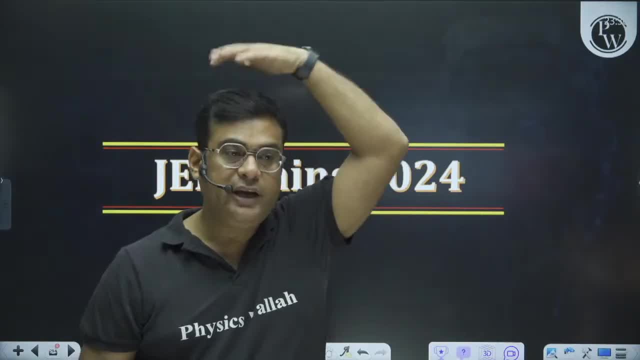 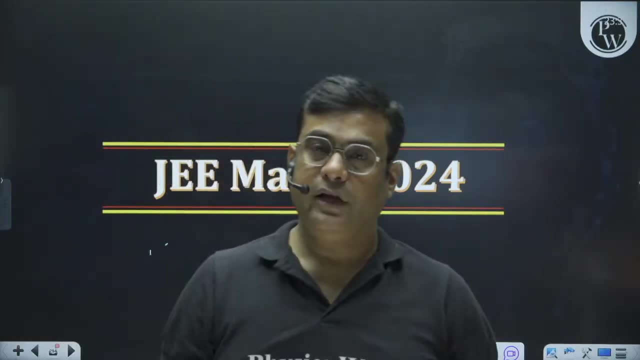 easily. Such properties change when the system is divided. There was a piece of ice that I broke, so if you break it, then the mass, volume and moles of different pieces will be different. so that is why it is extensive, but the temperature. 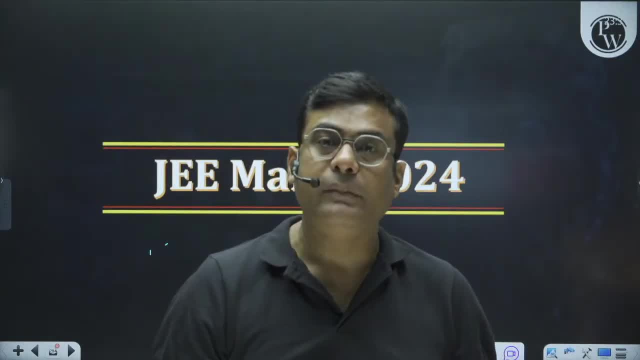 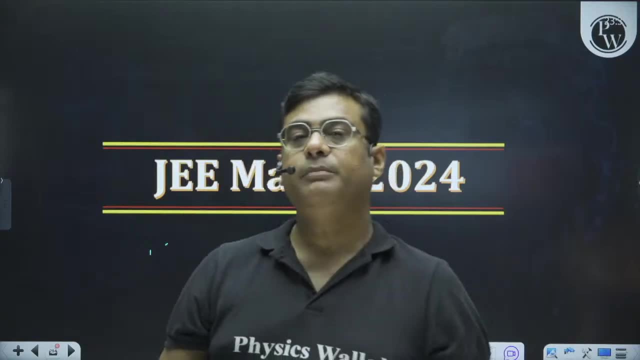 of different pieces will be the same, the melting point of different pieces will be the same, the density of different pieces will be the same, the properties that remain the same, then all of them will become intensive. Sir, how many number of spectra lines will there be? 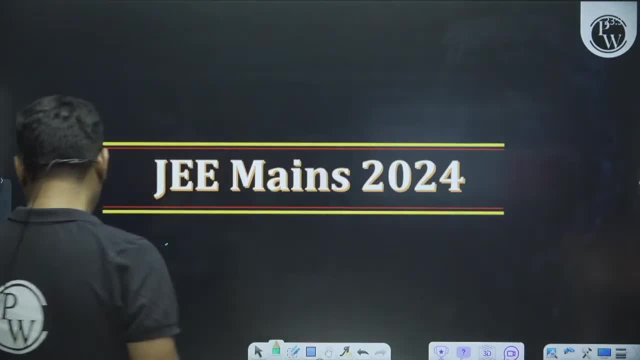 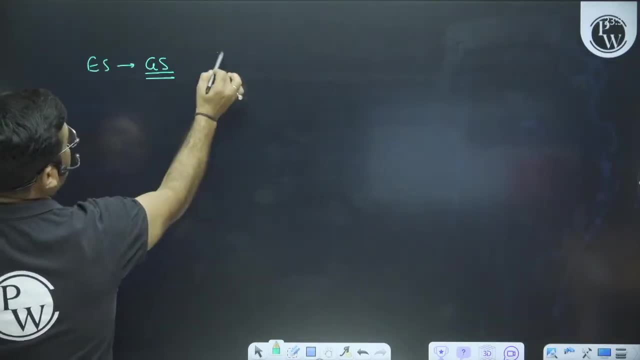 Tell me that type of question too. Sir, there is a formula for the number of spectra lines. If you are coming in the ground state from any excited state, then N into N minus 1 by 2, and from any one excited state N2,. some other excited state is coming on N1, then the 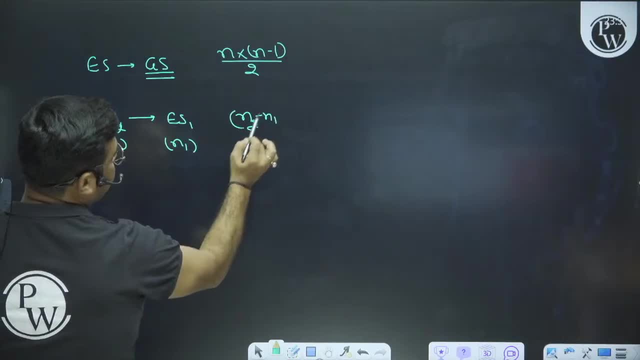 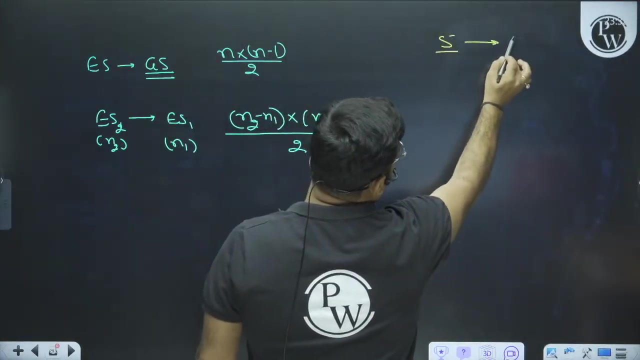 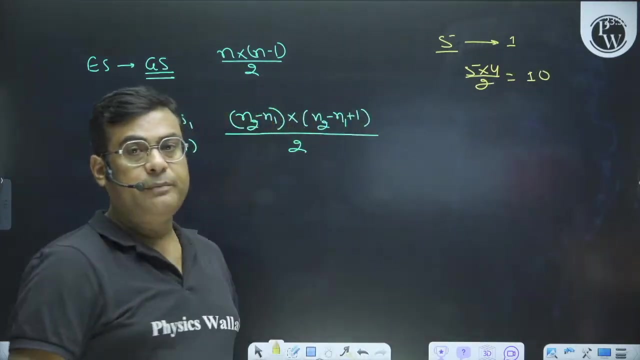 formula is N2 minus N1 into N2 minus N1 minus N2.. Okay, what is the meaning I am telling you? see, if you are coming in the ground state from the fifth state, then 5 into 4 by 2 means you will get ten lines: 5 4 0, 20 by 2, there are ten lines. 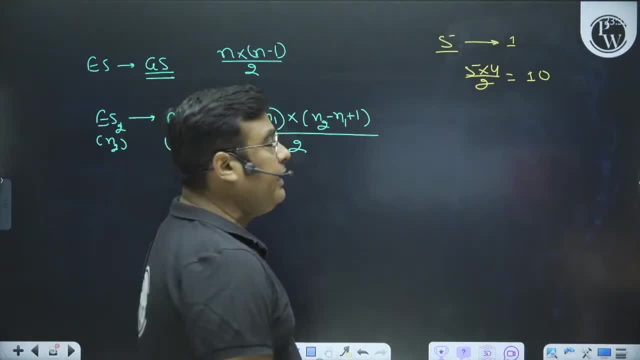 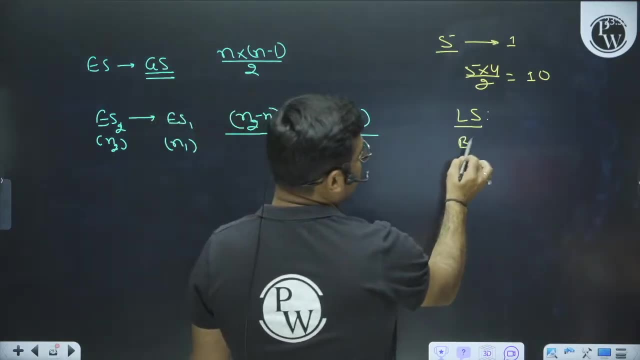 Now, let's do the trick in this that: how many of these are there in the Lyman series? how many are there in the Balmer series? how many are there in the Paschan series? how many are there in the Paschan series? 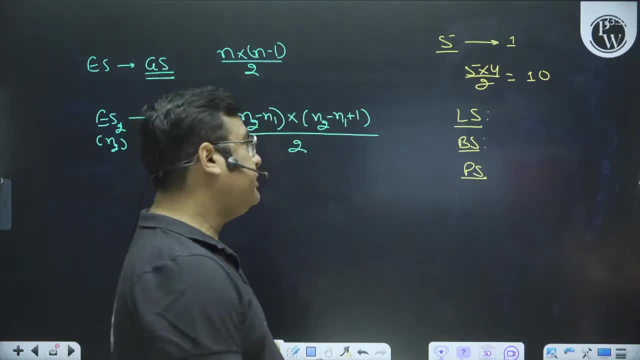 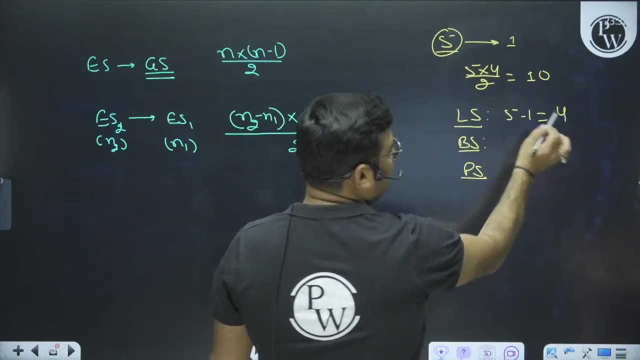 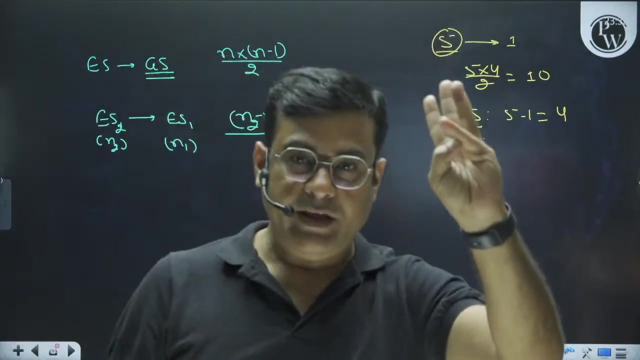 So the Lyman series will say children. then where does the Lyman series come on 1.. So, whatever is the value of N, N minus 1, by the way, you can also count on your fingers, son- there is a Lyman coming from 5 to 1,. there is a Lyman coming from 4 to 1, there is a Lyman. 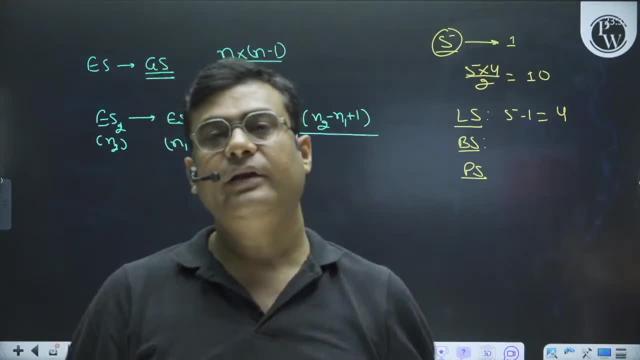 coming from 3 to 1,. there is a Lyman coming from 2 to 1, so there will be only 4.. But if there is confusion, then just do 2 minus for Balmer. why? Because there is a Lyman coming from 2 to Balmer. But if there is a Lyman coming from 2 to 2, then just do 2 minus for Balmer. But if there is a Lyman coming from 2 to 2, then just do 2 minus for Balmer. But if there is a Lyman coming from 2 to 2, then just do 2 minus for Balmer. But there is a Lyman coming from. 2 to 2, then just do 2 minus for Balmer, If you ask for the position, then do 3 out of 5, there will be 2.. The formula is the same- children, but sometimes different groups are asked for it, but once everyone sends red chili, green chili, absolutely right, absolutely because of a little cold. there was a little difference of 5-7 percent efficiency, son, but the energy was as much as I have explained to you, with all the energy, and I have full hope that you will. 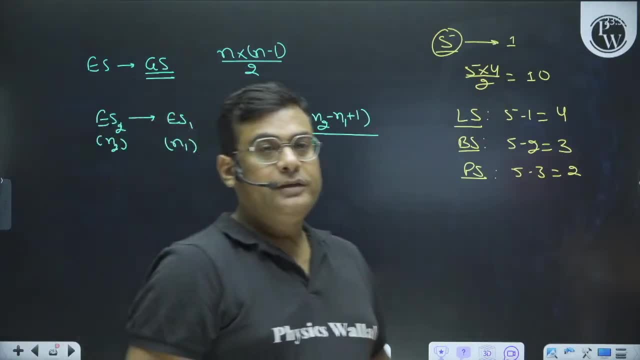 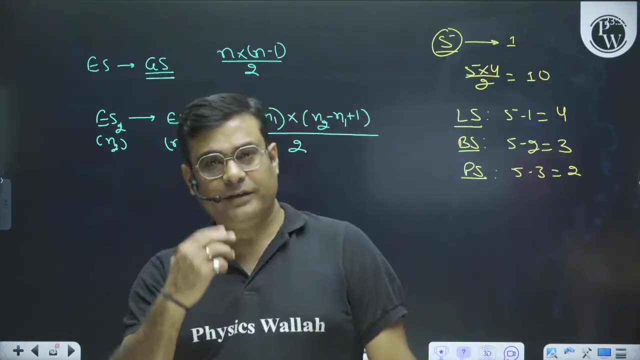 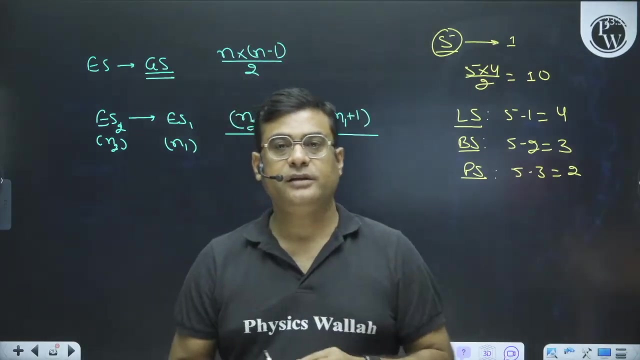 understand this, I hope, what I had promised you then. yes, still, I have said to you that I have made all questions for you in the JEEMains 2024, I have made all the slides with great hard work and all this is fine and it is fine so that you can understand. I also have given 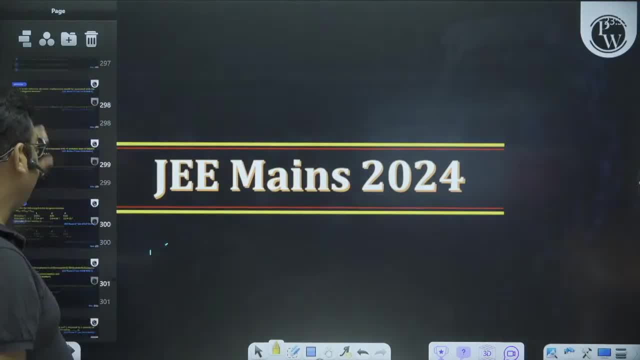 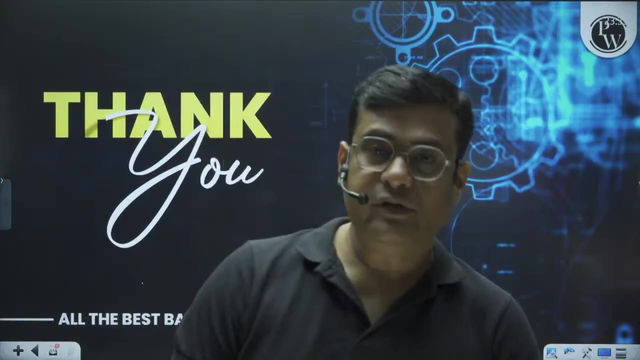 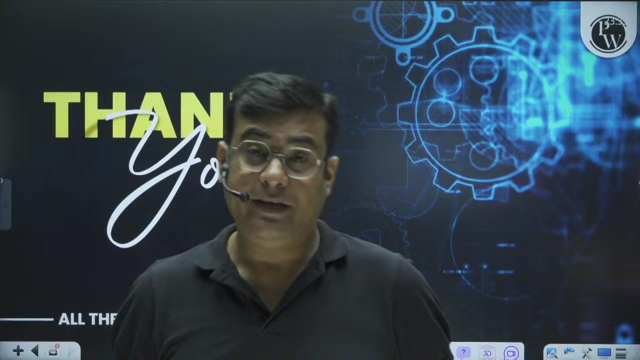 you the slides from the JEEMains 2024, and this is also fine. this is the best I can say. Thank you all. Now. I will attach it to you in the format of PDF then, once you have all the questions of J-Mains 2024, now you have time, my child. I counted it from the time I came. now it is not 12 o'clock, so it is right for us to say 4 days still. 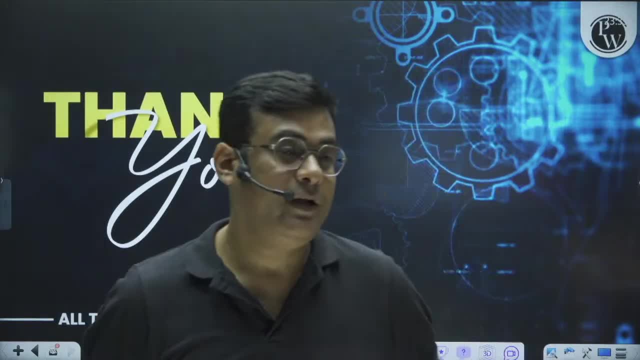 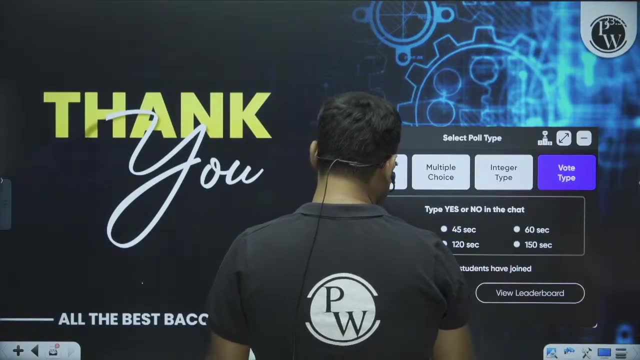 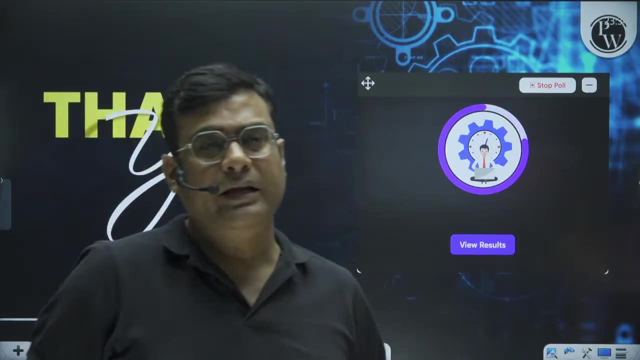 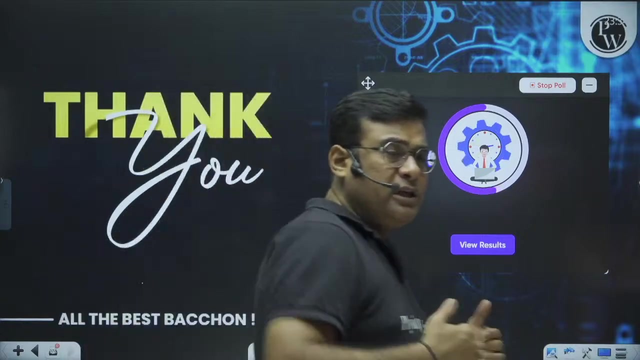 Okay, quickly give all the red, green, green, blue and yellow hearts. okay, and the session has ended. one last vote type: say 30 seconds, then do it. that brother, the 40-50 things I said something or the other, brother, you will definitely get something new right. that you will definitely get 40-50 things, something or the other, even if it is a new calculation. children, the vision to think about the question. okay, I gave you a little time to solve the question. 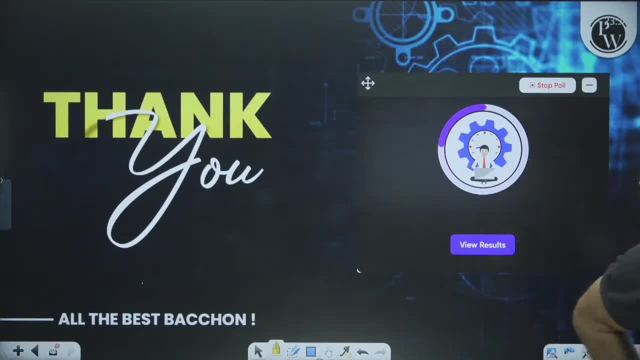 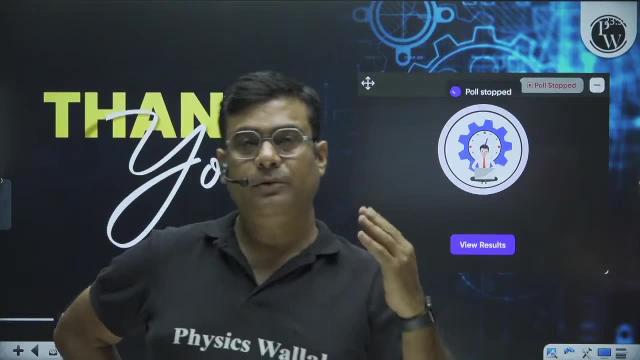 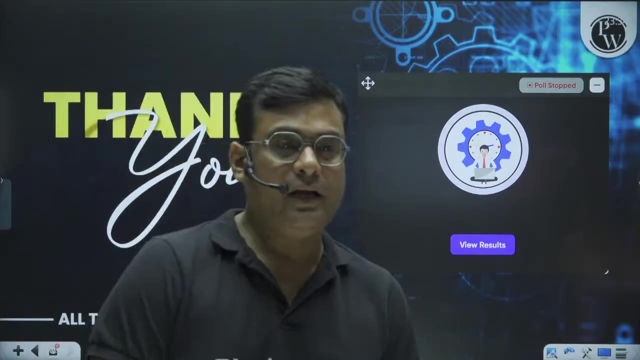 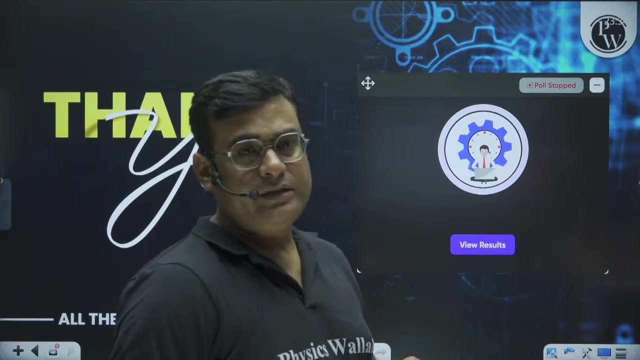 because then I can make the question less. my wish was that I could explain you as many questions as possible. that, brother, how will you attack to read? right for that I am a little sorry if it is left less. but still, brother, the purpose of my teaching was that I tried my best to complete it from my side. where will you get the PDF? the PDF will be attached. the session will be attached. the PDF will be attached to you in the session right. 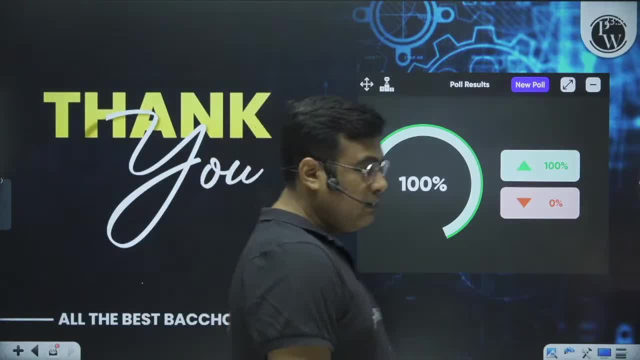 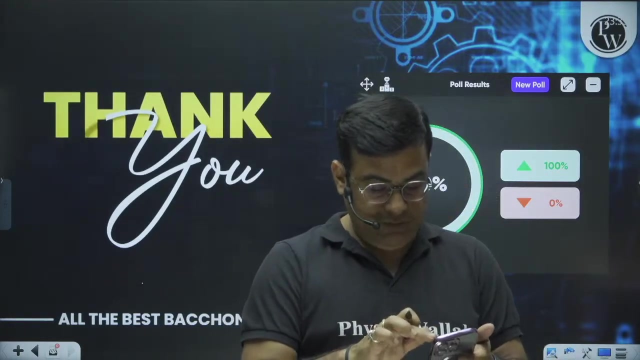 okay, oh, this is my brother. I did it right now. I don't know how many children are alive or what is it now I am definitely looking at it, because we don't see anything on the screen. now I am looking at it. so, still, one of the students are alive. like you have given 4.3, have you been angry? but okay, one of the students are alive and despite that, you are 100%. so, one photo in the last, you will give it to everyone, right? 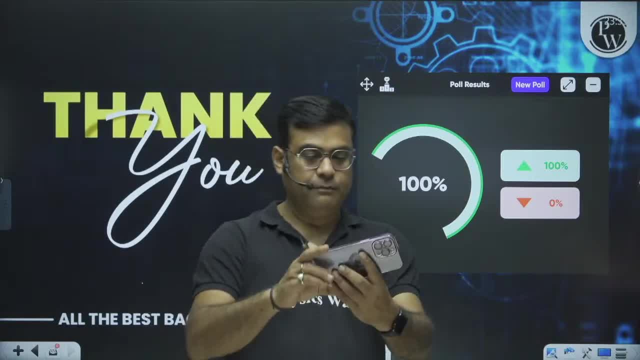 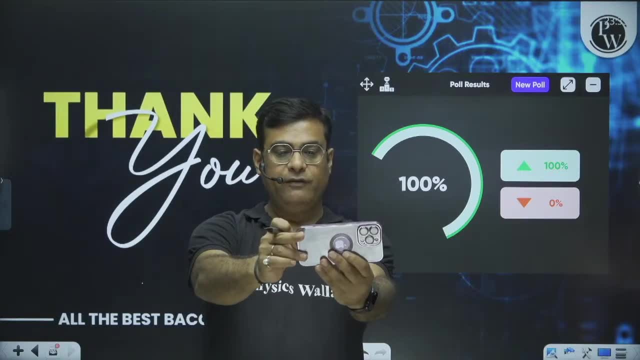 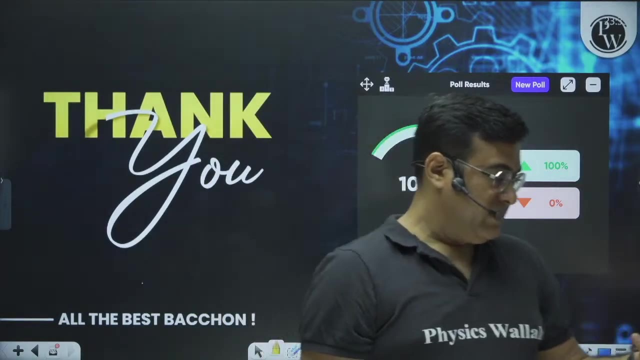 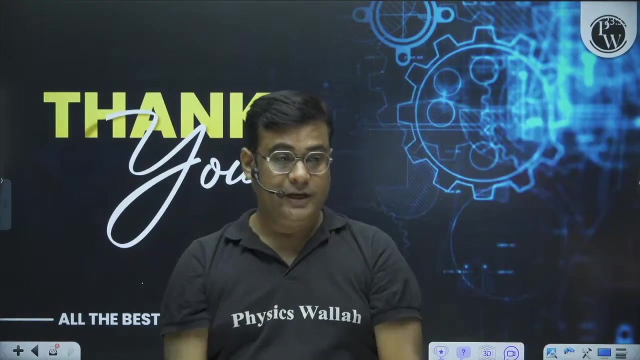 then when will you meet? that I don't know. understand. done, Nathan, brother, he is mine. I will get into the story of feeling from the audience. then look: 100% of the feedback. okay, 100% means what is the quality praise for the entry: 10-12-13,. thank you, thank you. thank you very. 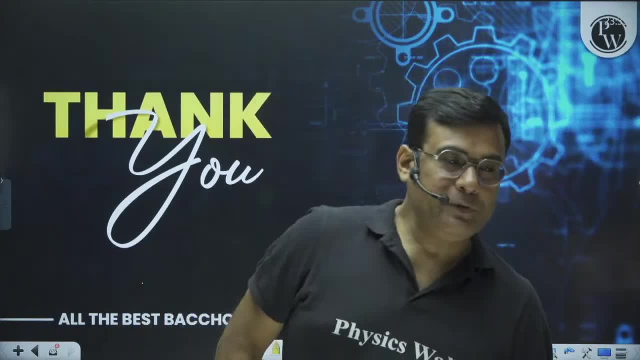 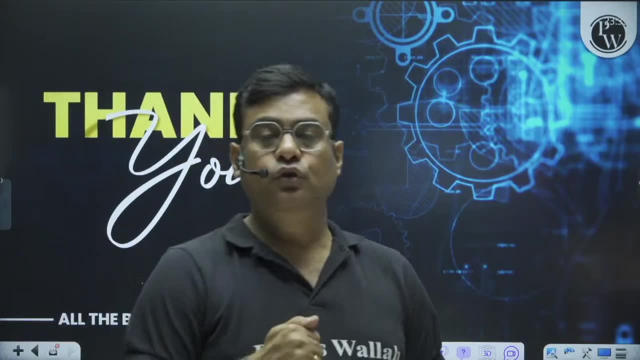 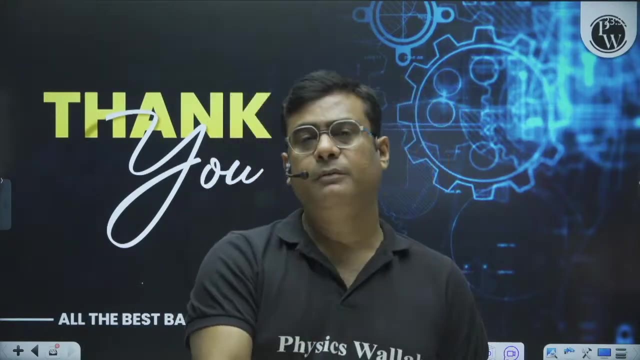 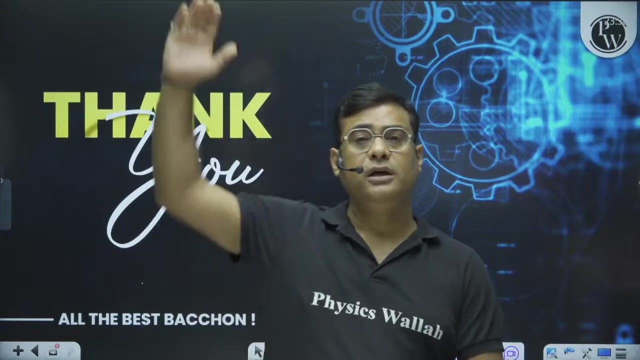 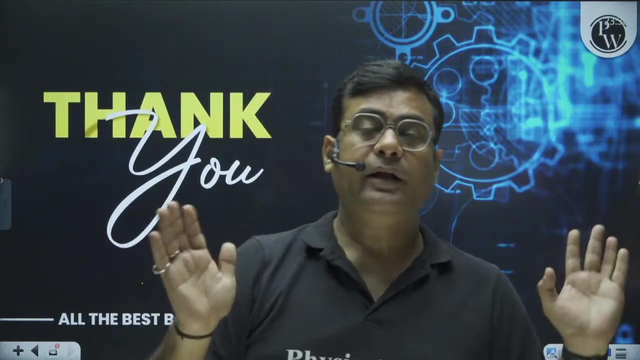 much looking at me, she burst. but you, like, you, really have some potential. why did not the children be alive In the beginning? there was some noise, there was some lots of noise. water was in her mind. the 게. with this hope you will take advantage of this session of children. there are still 4 days left. whatever you have left, there will still be 125-150 questions. do them and I am ready to take the guarantee that about 75-80% of your questions will come from these pdf questions. every child whose exam will be on 9th- he still has 10 days. he has 10 days. he has 10 days. then he can easily solve every question once again. 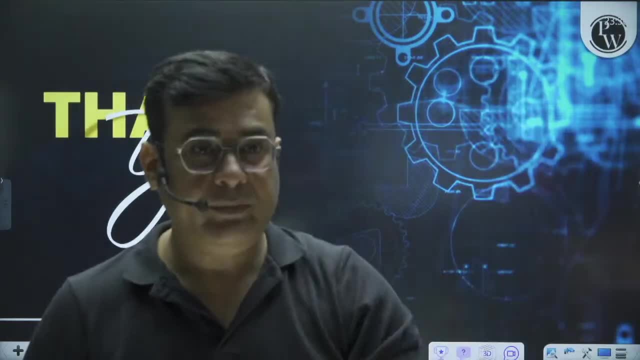 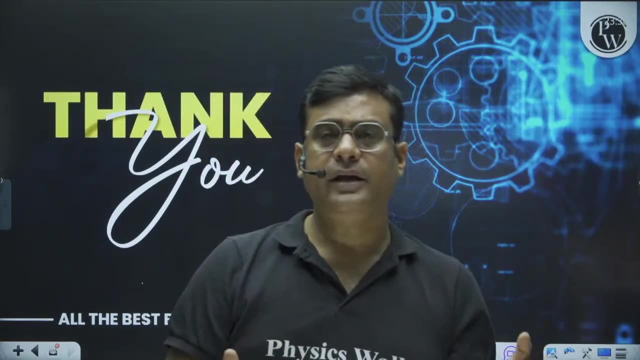 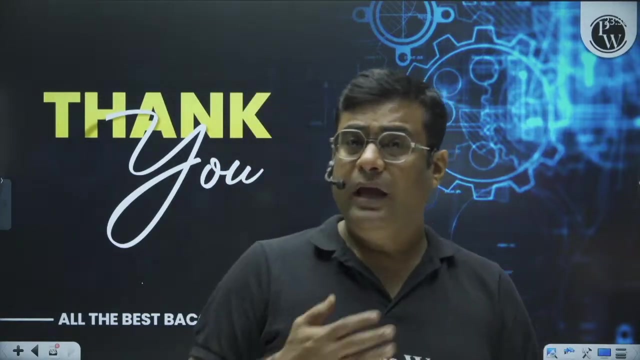 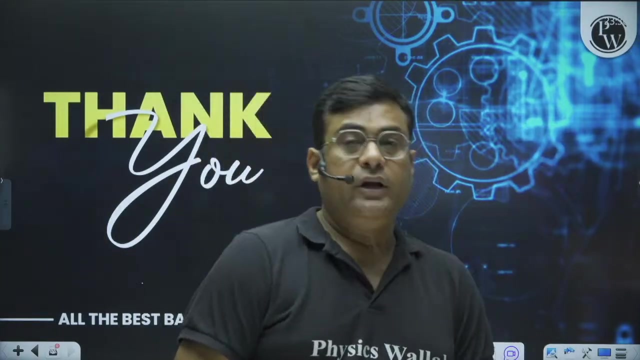 you can see this session again at 2x speed, children, you can see this video again at 2x speed. and do well, children, because your progress will be the progress of your family, society, country. one person studies, he motivates the 10 people around him. now, it is okay that the motivation of 10 out of 10 is not permanent throughout, but if one person has made 2 engineers, 2 good, educated persons, then it is okay. 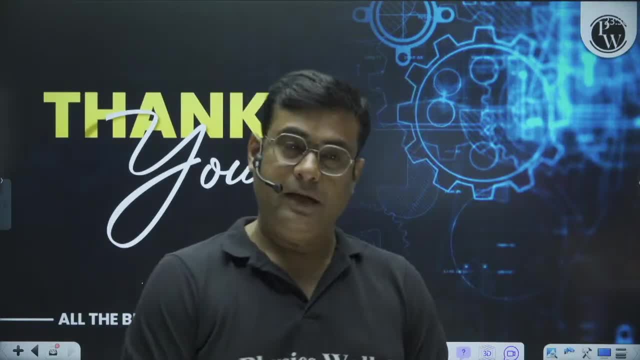 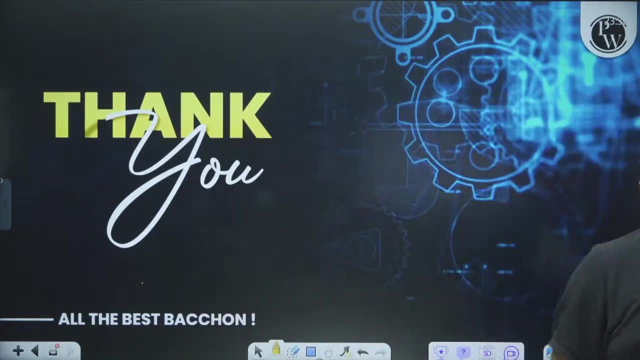 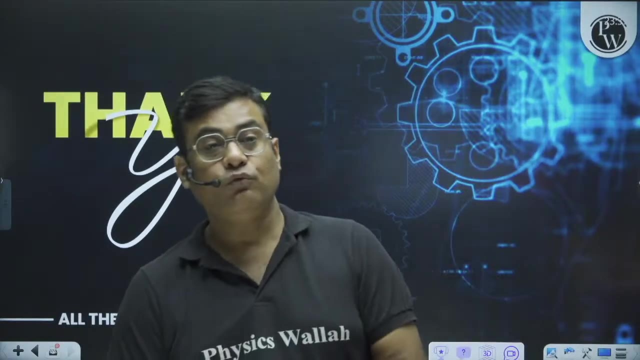 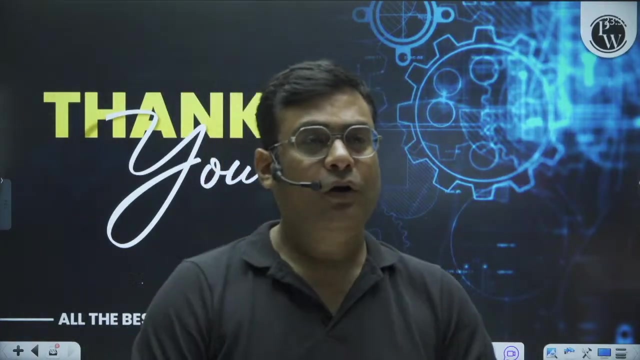 and this is the way our country is over. it is a responsibility to our country and it is a responsibility, children, that we can not do anything else for the country. in this way, if we can study and become a good, educated person, then we are doing a lot of work for our country, because many people are watching us. thank you, sir, for this amazing session on this amazing platform. you are very, very good teacher. thank you, thank you, thank you, children. 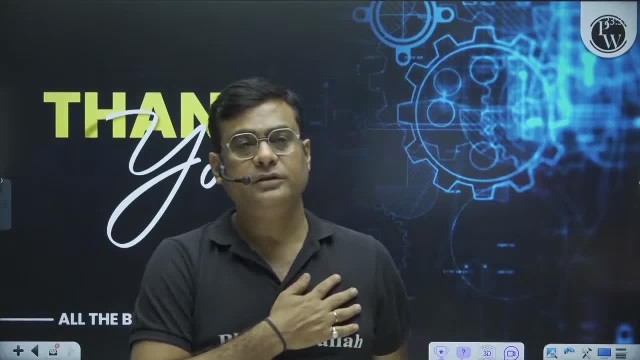 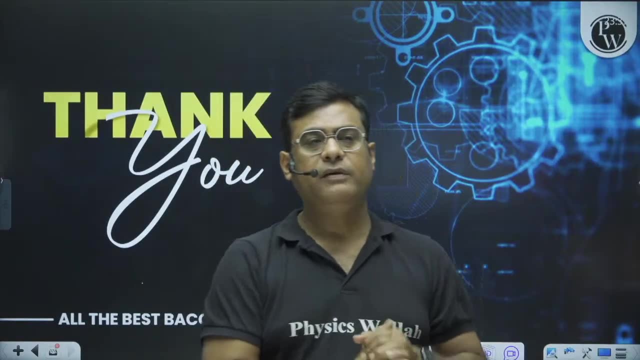 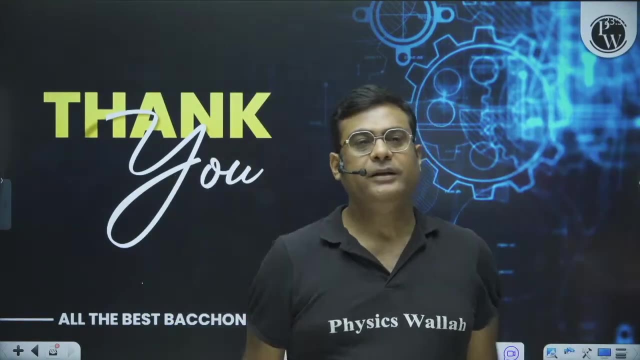 Thank you, thank you, thank you very much. I hope and pray from the bottom of my heart that all of you will make it to the quarterfinals and qualify for the advance, so that we can meet you again in the advance. We will meet you in the victory celebration and we will also be able to say that all these children are our students and we have taught them well. 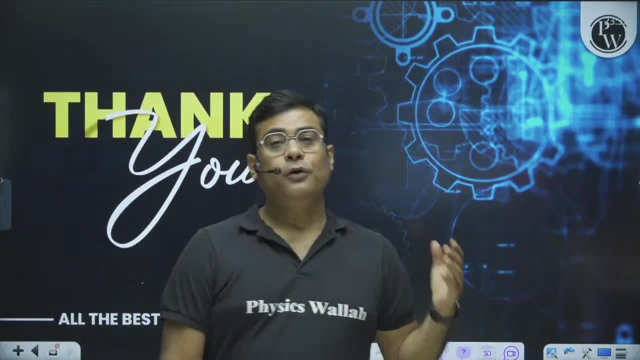 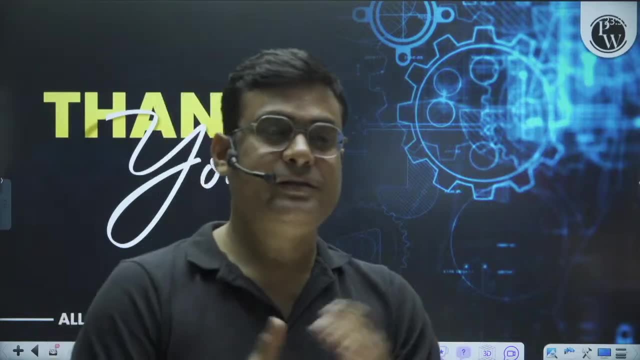 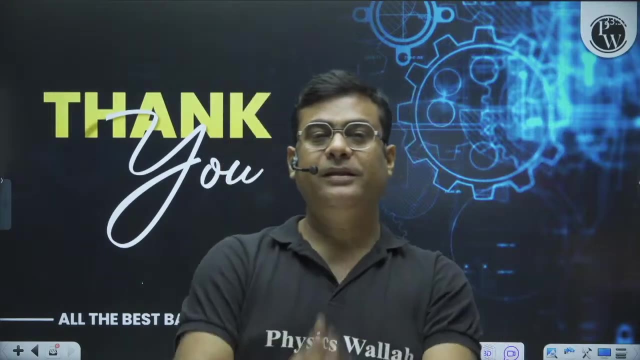 In their selection. we have played the role of catalyst Like a catalyst. we have been together with them, and these people have also followed the meaning of their teacher. Okay, so I will not waste your time. You have been with me continuously for six and a half hours. 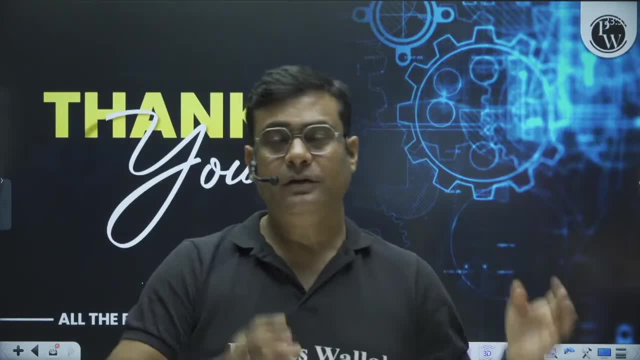 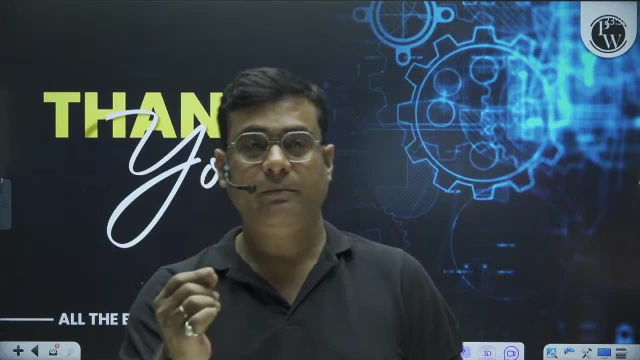 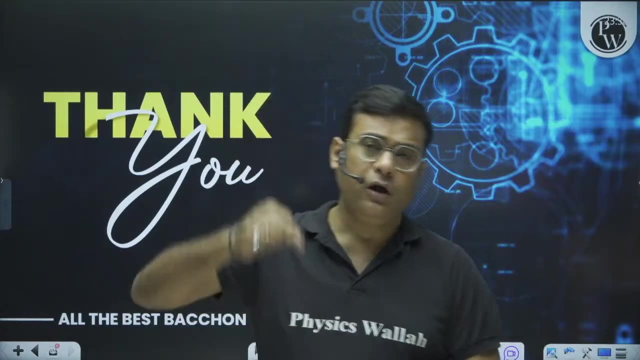 Now rest comfortably, sleep, wake up timely in the morning and go back to your remaining days, Son. there should be no mistake in any of them. Your time table will be fixed. Follow it, Study well. All the best to everyone. 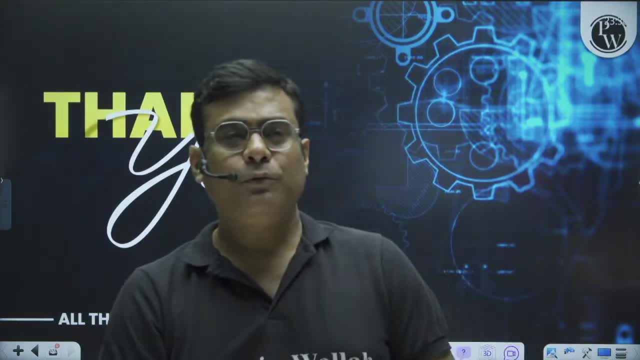 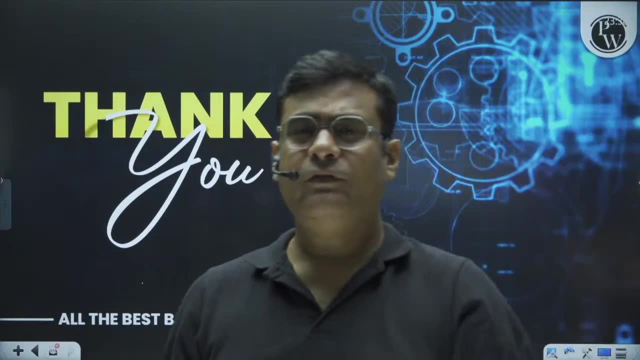 Son, there is no need to say all the best. It is coming out of my heart. I told you that I will not give up my chest, but I am giving up my chest for you all. All the best to everyone Right. Swear and go with full confidence and full energy that we will make it to the quarterfinals.